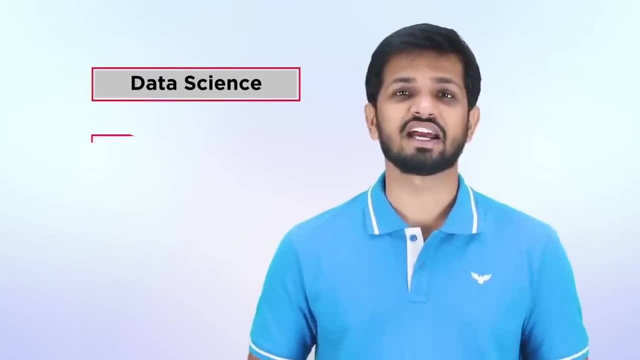 Mohan, each with over 10 years of experience in data science and machine learning, will teach you the various concepts of machine learning, including algorithms, and how you can practically implement them. First we will understand what is machine learning, and then we will go through various 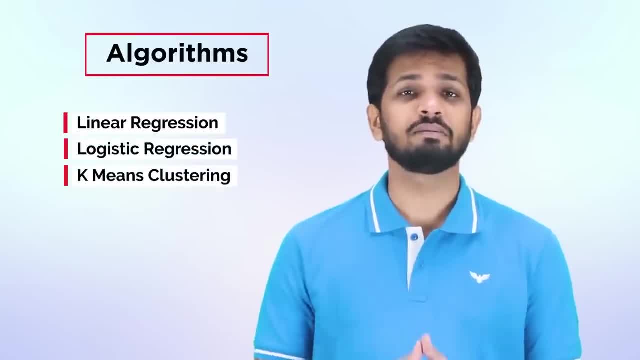 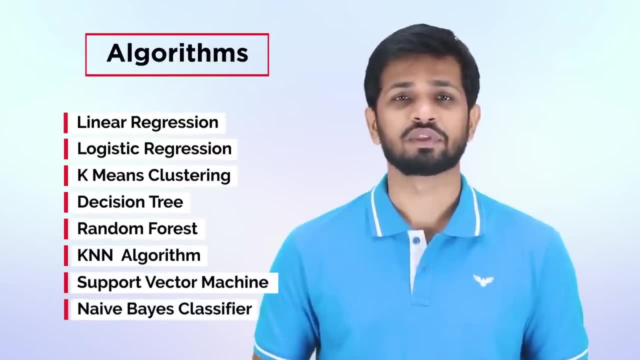 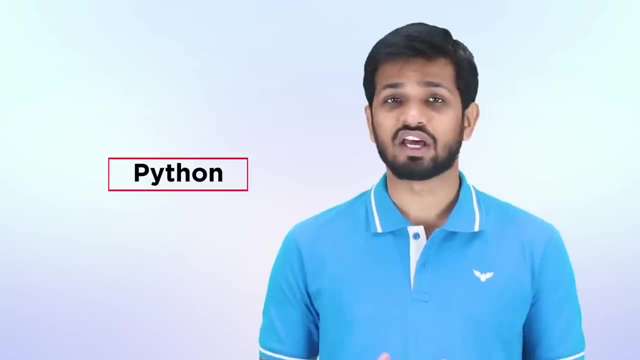 algorithms like linear regression, logistic regression, k-means clustering, decision tree, random forest, KNN algorithm, SVM and naive Bayes classifier. You will not only learn how each of these algorithms work, but also implement them using Python. Once you're done with this, you 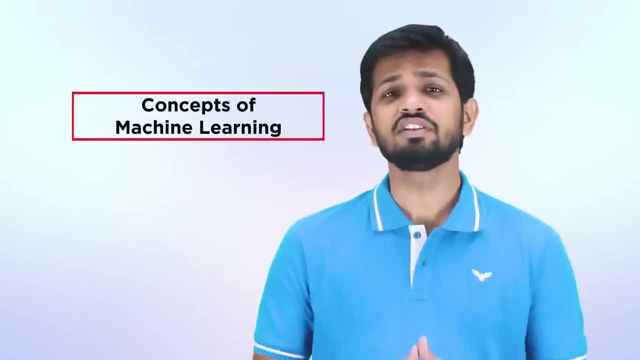 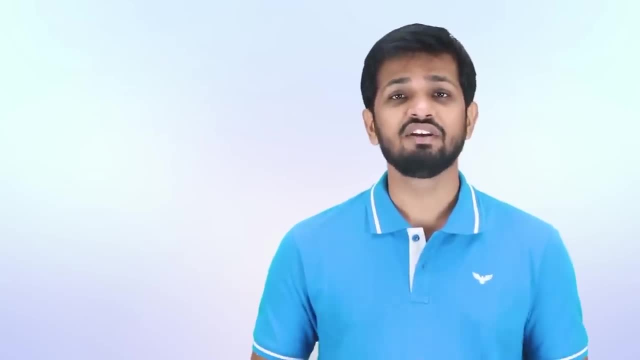 will have a firm grasp on the concepts of machine learning. After this comprehensive machine learning training, we will also go through some popular applications of machine learning, And then we will guide you on how you can be a machine learning engineer. And finally, we have collected 30 of the. 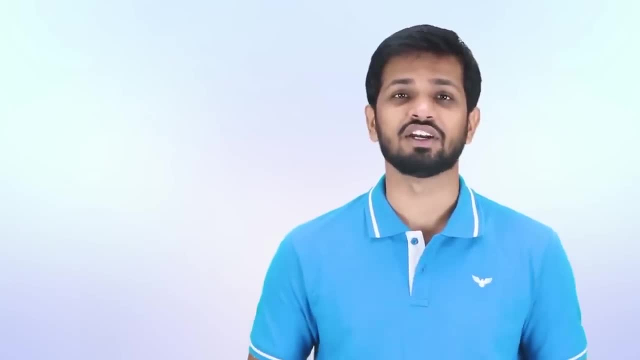 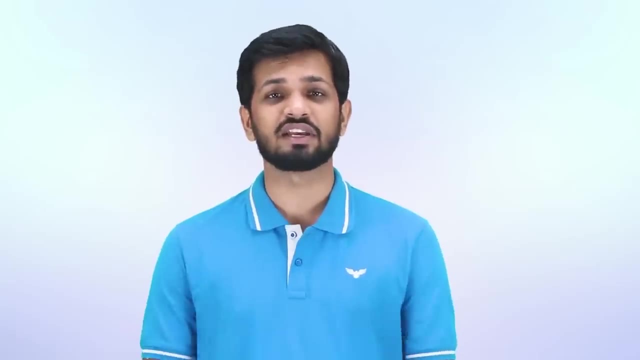 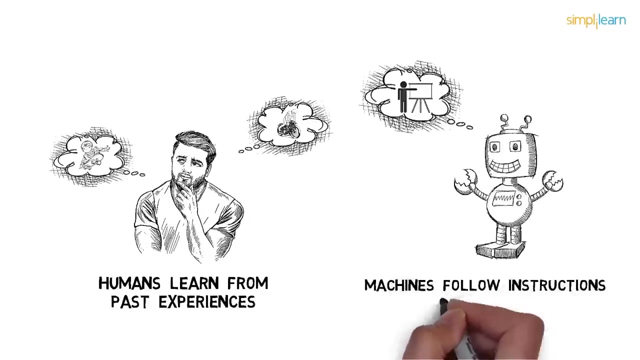 most important questions that you might face in a machine learning interview. Before we move ahead with the full course, let us look at a short animated video we have made so that you can learn from their past experiences. And machines follow instructions given by humans, But what? 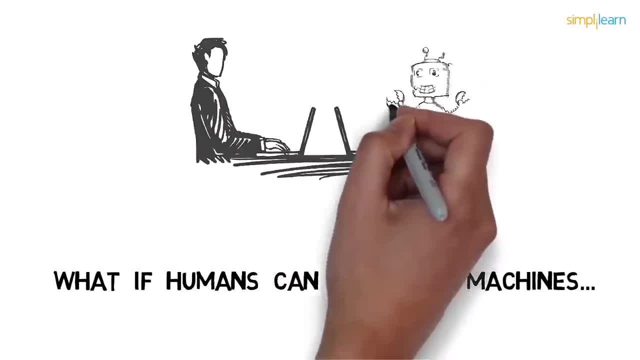 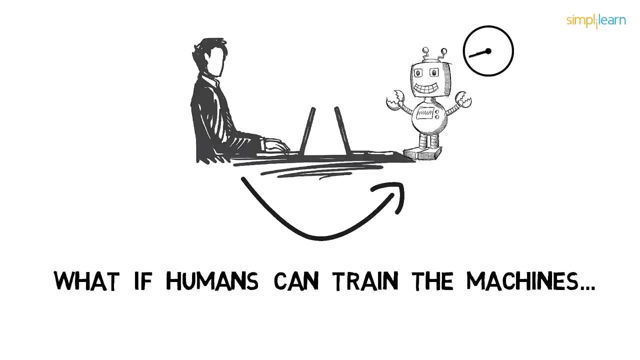 if humans can train the machines to learn from their past data and do what humans can do, and much faster. Well, that's called machine learning. But it's a lot more than just learning. It's also about understanding and reasoning. So today we will learn about the basics of 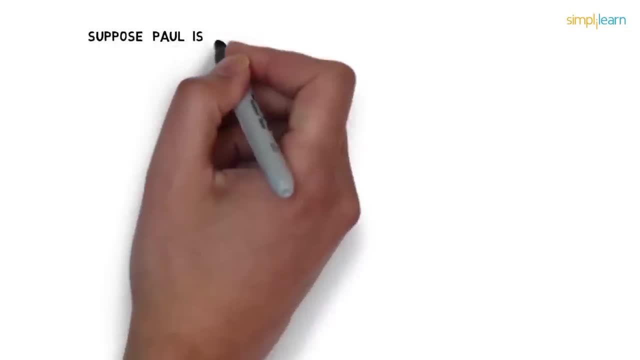 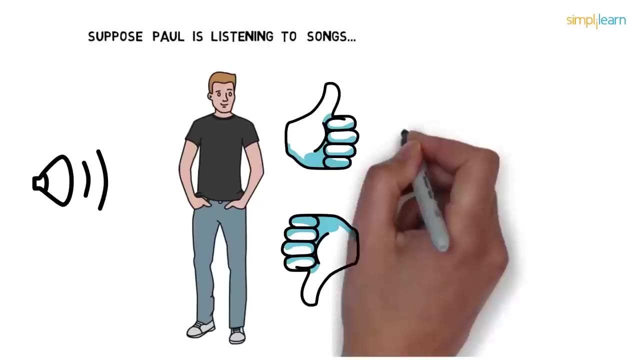 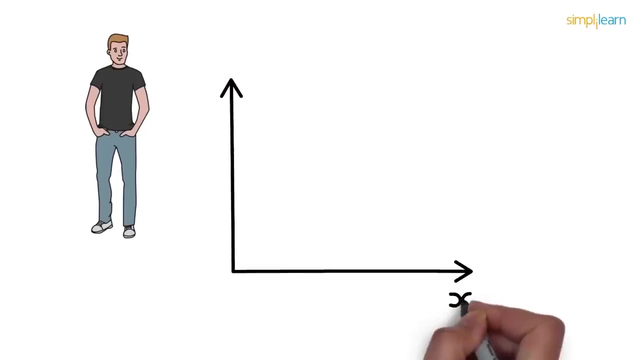 machine learning. So that's Paul. He loves listening to new songs. He either likes them or dislikes them. Paul decides this on the basis of the song's tempo, genre, intensity and the gender of voice. For simplicity, let's just use tempo and intensity for now. So here tempo is on. 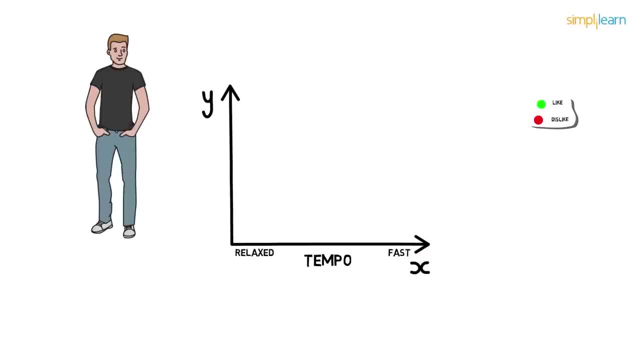 the x-axis, ranging from relaxed to fast, whereas intensity is on the y-axis, ranging from light to soaring. We see that Paul likes the song with fast tempo and soaring intensity, while he dislikes the song with relaxed intensity. So now we know Paul's choices. Let's say Paul listens to a new song. Let's name it as: 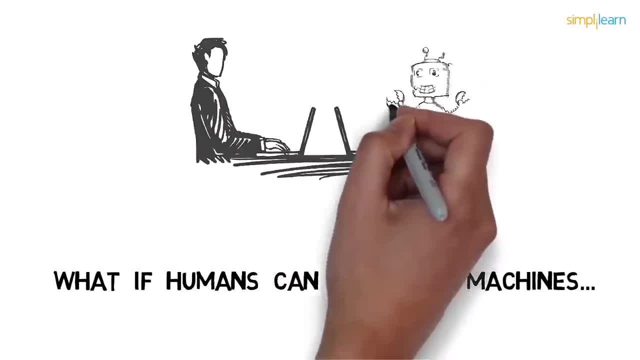 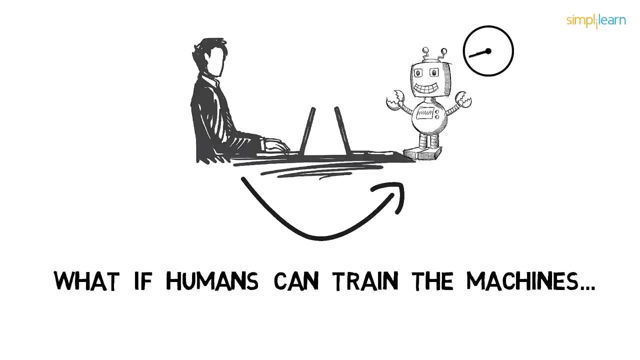 if humans can train the machines to learn from their past data and do what humans can do, and much faster. Well, that's called machine learning. But it's a lot more than just learning. It's also about understanding and reasoning. So today we will learn about the basics of 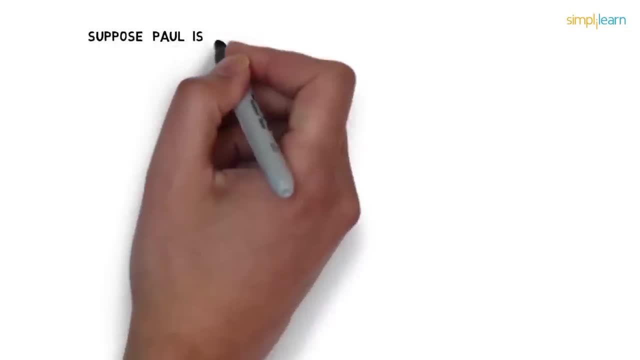 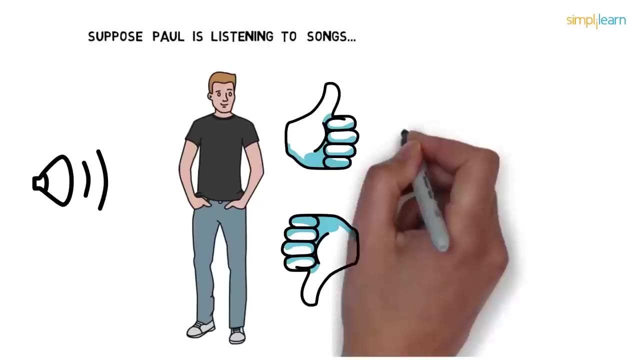 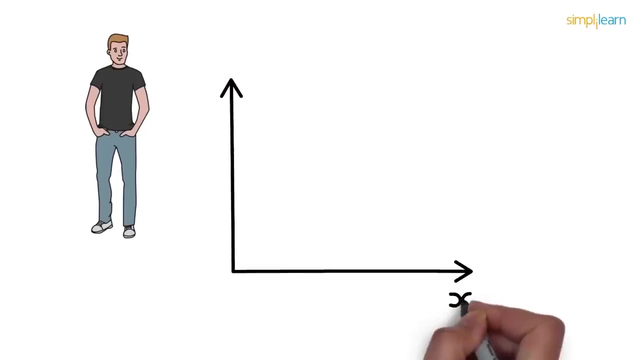 machine learning. So that's Paul. He loves listening to new songs. He either likes them or dislikes them. Paul decides this on the basis of the song's tempo, genre, intensity and the gender of voice. For simplicity, let's just use tempo and intensity for now. So here tempo is on. 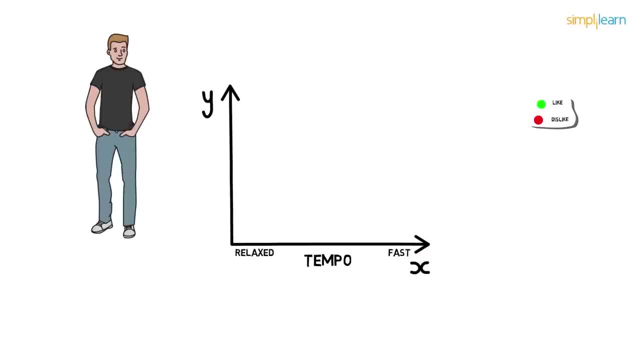 the x-axis, ranging from relaxed to fast, whereas intensity is on the y-axis, ranging from light to soaring. We see that Paul likes the song with fast tempo and soaring intensity, while he dislikes the song with relaxed intensity. So now we know Paul's choices. Let's say Paul listens to a new song. Let's name it as: 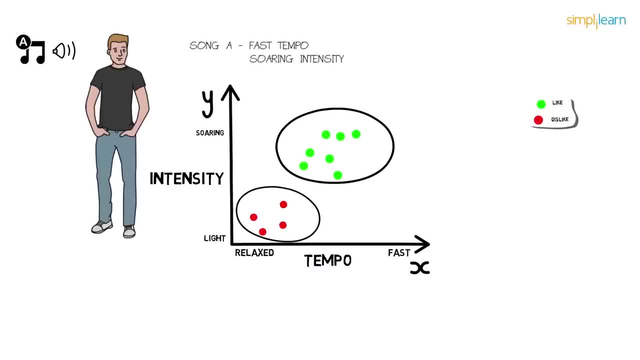 song A. Song A has fast tempo and a soaring intensity, So it lies somewhere here. Looking at the data, can you guess whether Paul will like the song or not? Correct, So Paul likes this song. By looking at Paul's past choices, we were able to classify the unknown song. 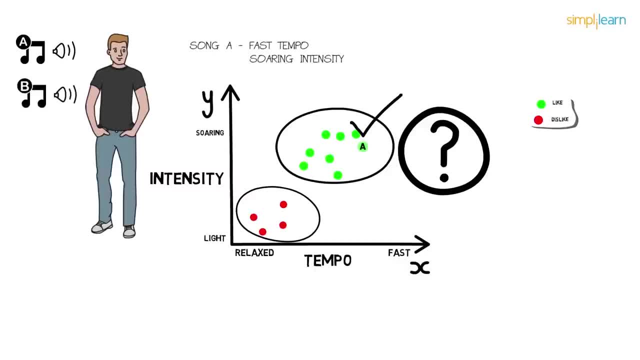 very easily, Right? Let's say now Paul listens to a new song. Let's see: Paul's choices are the same. The song A tends to be the same as song B. It's the same as the song B. So song B lies somewhere here with medium tempo and medium intensity. neither 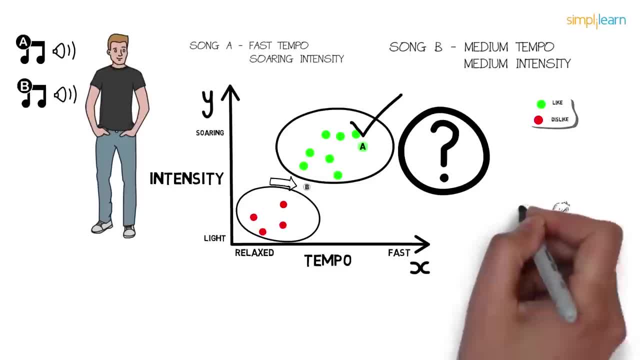 relaxed nor fast. neither light nor soaring. Now can you guess whether Paul likes it or not? Not able to guess whether Paul will like it or dislike it, Are the choices unclear? Correct, We could easily classify song A, But when the choice 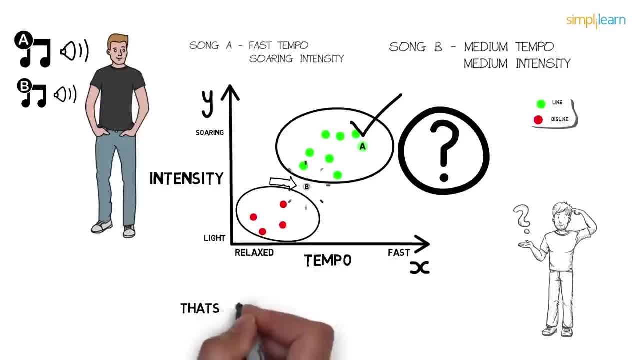 became complicated, as in the case of song B. yes, and that's where machine learning comes in. Let's see how. for song b. if we draw a circle around the song b, we see that there are four votes for like, whereas one vote for dislike. if we go for the majority votes, we can say that paul will definitely like. 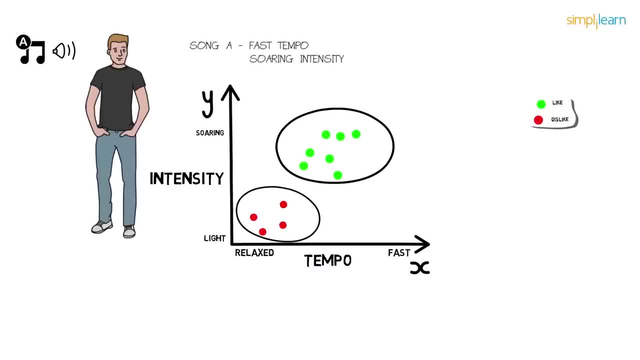 song A. Song A has fast tempo and a soaring intensity, So it lies somewhere here. Looking at the data, can you guess whether Paul will like the song or not? Correct, So Paul likes this song. By looking at Paul's past choices, we were able to classify the unknown song. 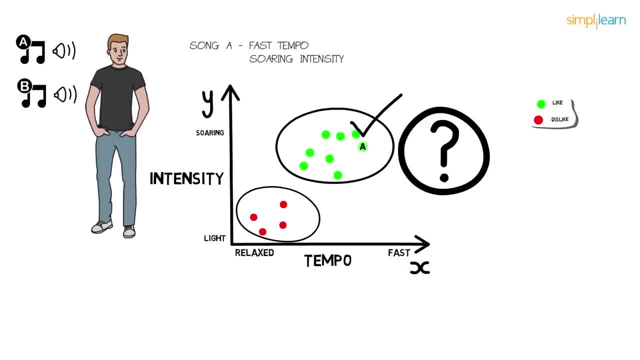 very easily, Right. Let's say now Paul listens to a new song. Let's see how —. In the same example, Paul listens to a song that is soaring. Right, The music is soaring, But the melody is soaring, That's it, So it can be easily classified as a song. 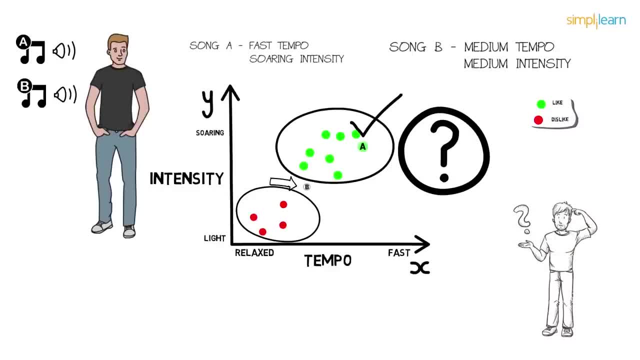 A, So we can easily classify that song A as a song B. But no, it is not as simple as Paul's choice. Paul didn't like the song B, So he didn't like the song B. But again, let's just say that Paul's choice was light. Now Paul likes. 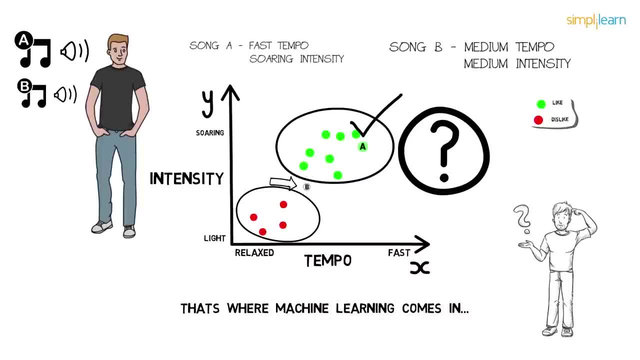 this song B, which is why Paul doesn't like it. example for song B: if we draw a circle around the song B, we see that there are four votes for like whereas one vote for dislike. if we go for the majority votes, we can say that Paul will definitely like the song. that's all. this was a. 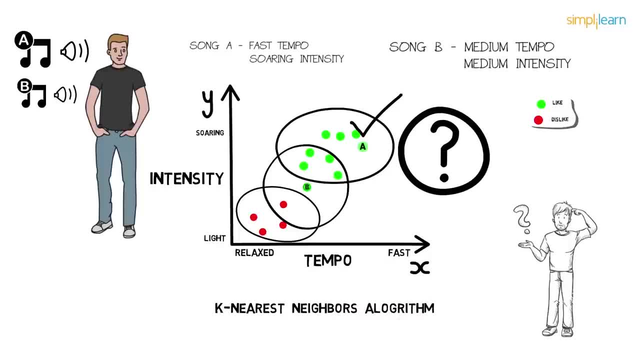 basic machine learning algorithm. also, it's called k-nearest neighbors. so this is just a small example in one of the many machine learning algorithms. quite easy right, believe me it is. but what happens when the choices become complicated, as in the case of song B? that's when machine learning comes in it. 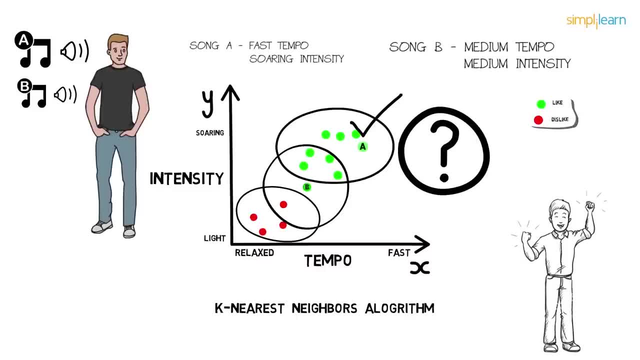 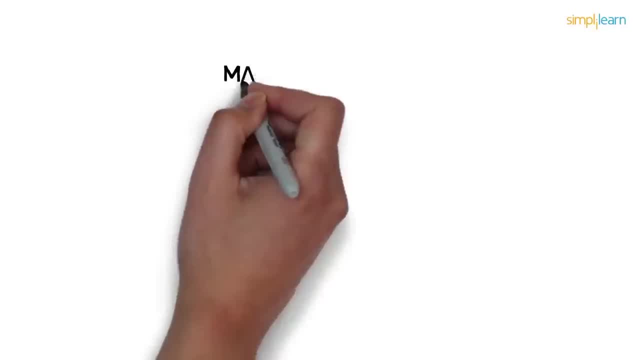 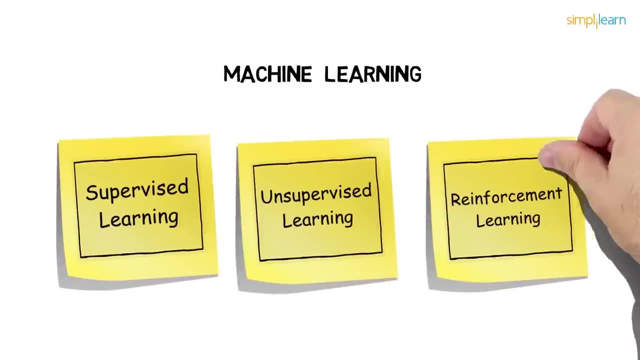 learns the data, builds the prediction model and when the new data point comes in, it can easily predict for it. more the data, better the model, higher will be the accuracy. there are many ways in which the machine learns. it could be either supervised learning, unsupervised learning or reinforcement learning. let's 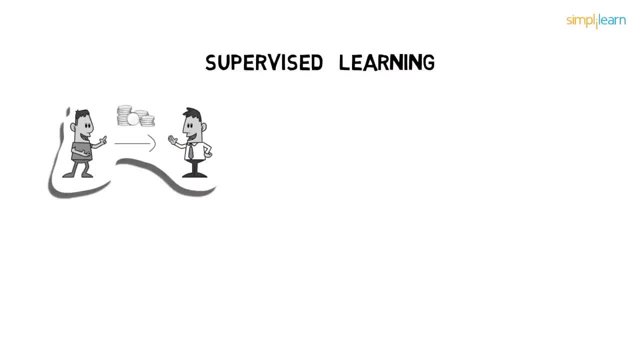 first quickly understand supervised learning. suppose your friend gives you 1 million coins of three different currencies. say once in a million coins. what happens when the machines learn to predict rupee, one euro and one dirham? each coin has different weights, for example a coin of one. 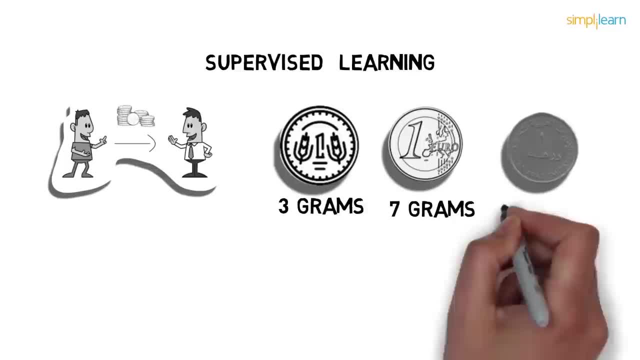 rupee weighs three grams, one euro weighs seven grams and one dirham weighs four grams. your model will predict the currency of the coin. here your weight becomes the feature of coins, while currency becomes their label. when you feed this data to the machine learning model, it learns which feature is. 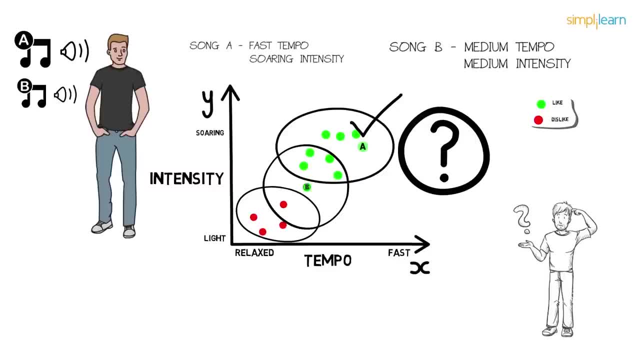 the song. that's all. this was a basic machine learning algorithm. also, it's called k- nearest neighbors. so this is just a small example in one of the many machine learning algorithms. quite easy, right? believe me it is. but what happens when the choices become complicated, as in the case of song? 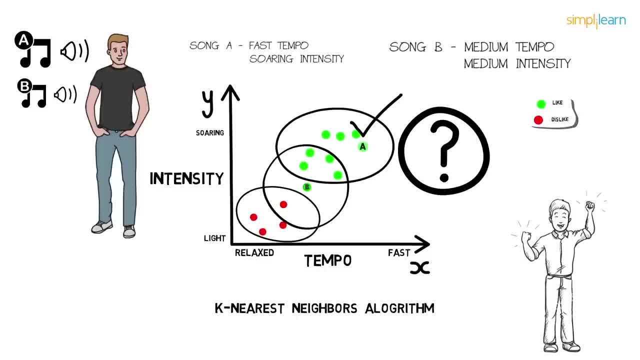 b. that's when machine learning comes in. it learns the data, builds the prediction model and when the new data point comes in, it can easily predict for it. more the data, better the model, higher will be the accuracy. there are many ways in which the machine learns. it could be either supervised, 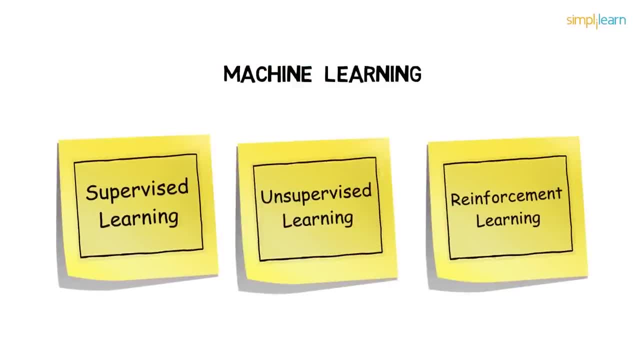 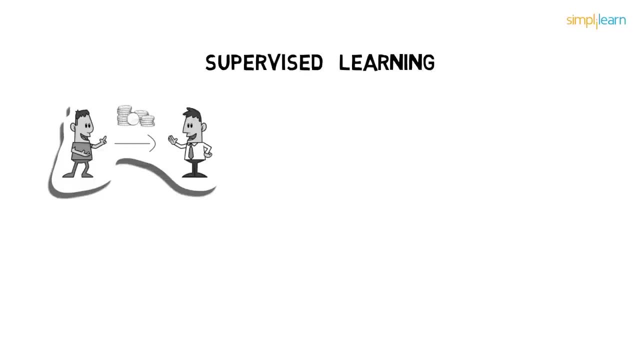 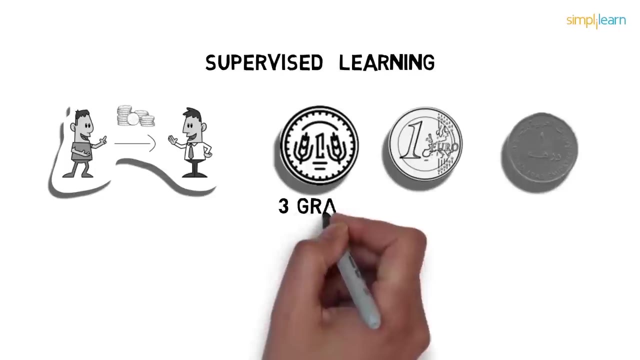 learning, unsupervised learning or reinforcement learning. let's first quickly understand supervised learning. suppose your friend gives you one million coins of three different currencies, say one rupee, one euro and one third gram. each coin has different weights. for example, a coin of one rupee weighs three grams one euro. 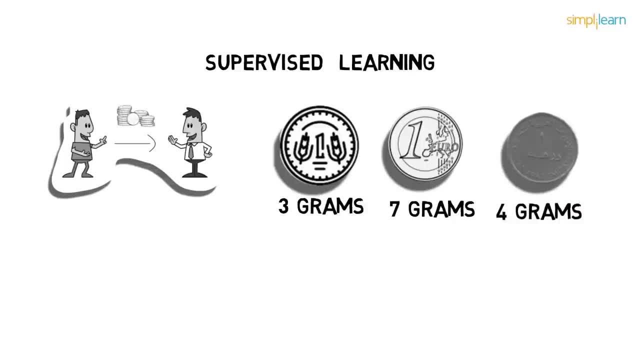 weighs seven grams and one theorem weighs four grams, your model will predict the currency of the coin. here your weight becomes the feature of coins, while currency becomes their label. when you feed this data to the machine learning model, it learns which feature is associated with which label. for 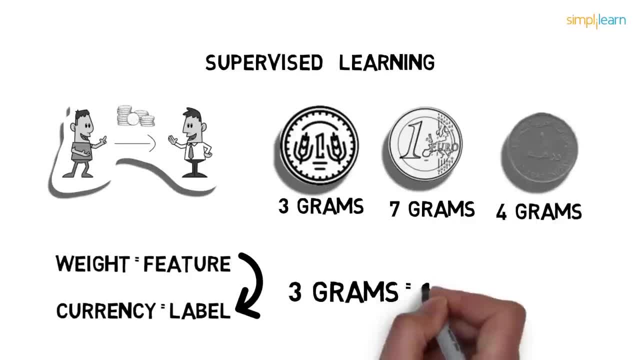 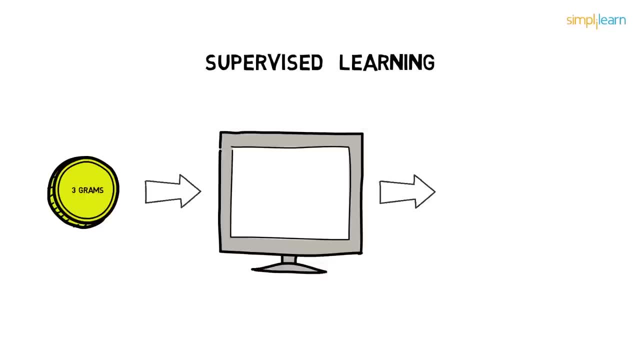 example, it will learn that if a coin is of three grams it will be a one rupee coin. let's give a new. the basis of the weight of the new coin, your model will predict the currency. hence supervised learning uses labeled data to train the model. here the machine knew the features of the object. 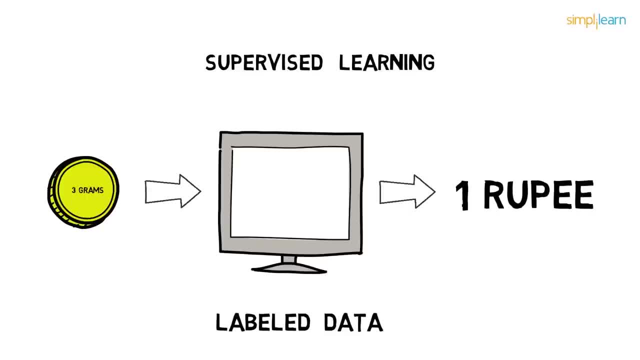 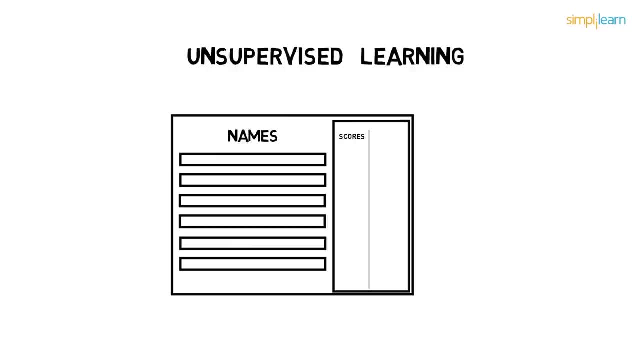 and also the labels associated with those features. on this note, let's move to unsupervised learning and see the difference. suppose you have cricket data set of various players with their respective scores and wickets taken. when we feed this data set to the machine, the machine identifies the 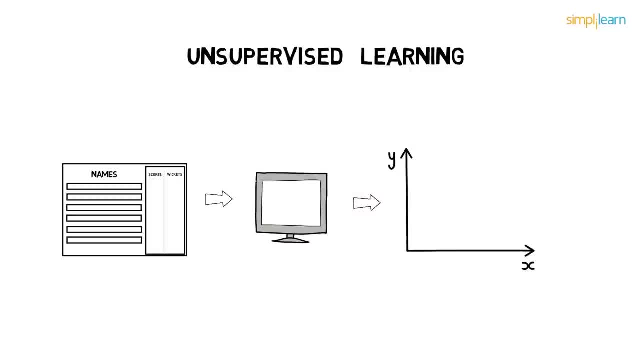 pattern of player performance. so it plots the sequence of the order of the dashed coin to the data, with their respective wickets on the x-axis while runs on the y-axis. by looking at the data, you will clearly see that there are two clusters. the one cluster are the players who scored high. 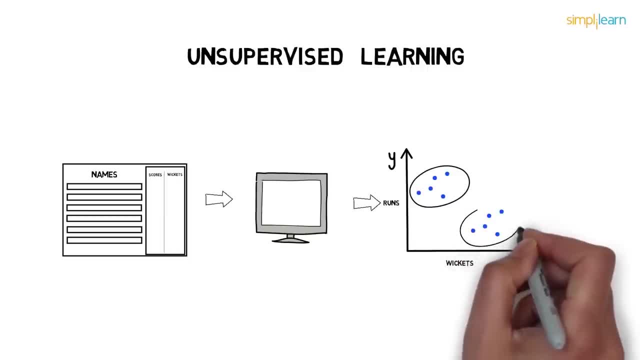 runs and took less wickets, while the other cluster is of the players who scored less runs but took many wickets. so here we interpret these two clusters as batsmen and bowlers. an important point to note here is that there were no labels of batsmen and bowlers, hence the learning with 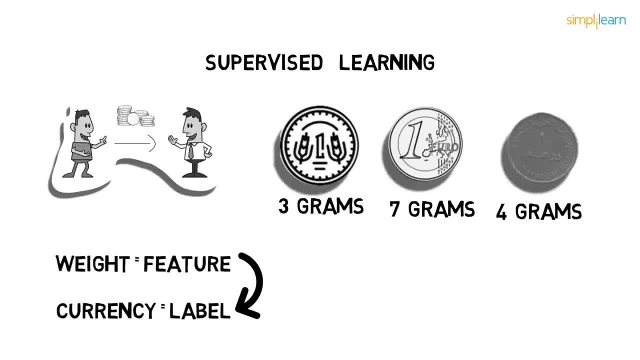 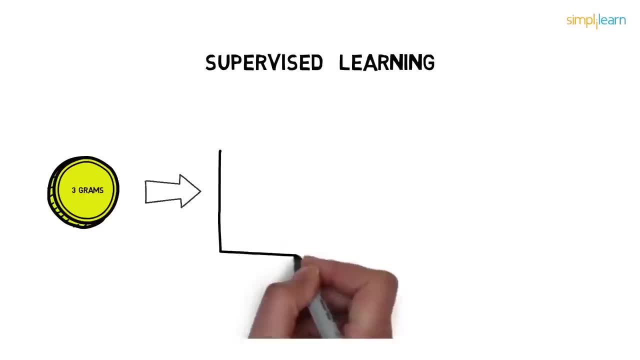 associated with which label. for example, it will learn that if a coin is of three grams, it will be a one rupee coin. let's give a new coin to the machine. on the basis of the weight of the new coin, your model will predict the currency. hence supervised learning uses labeled data to train. 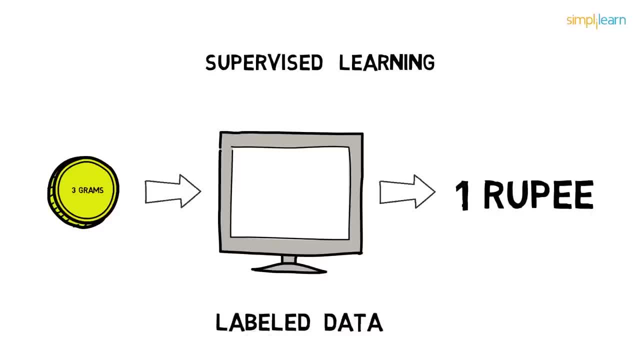 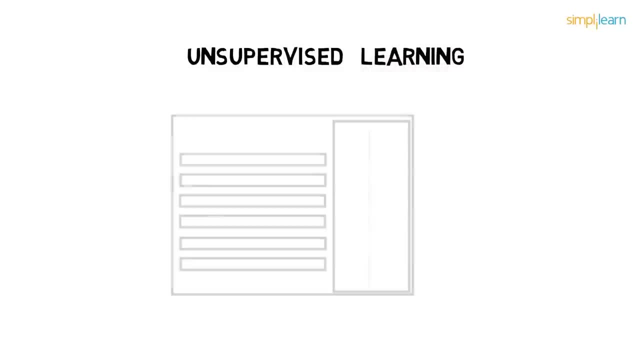 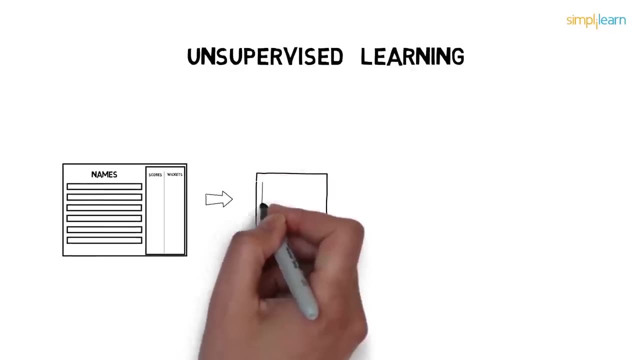 the model. here, the machine knew the features of the object and also the labels associated with those features. on this note, let's move to unsupervised learning and see the difference. suppose you have cricket data set of various players with their respective scores and wickets taken. when we feed this data set to the machine, the machine identifies the. 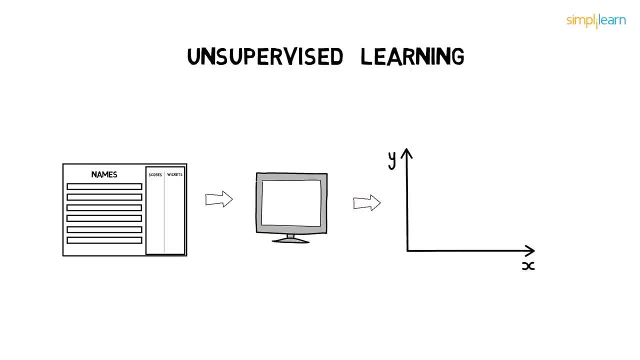 pattern of player performance. so it plots this data with the respective wickets on the x-axis while runs on the y-axis. by looking at the data, you will clearly see that there are two clusters. the one cluster are the players who scored high runs and took less wickets, while the other cluster 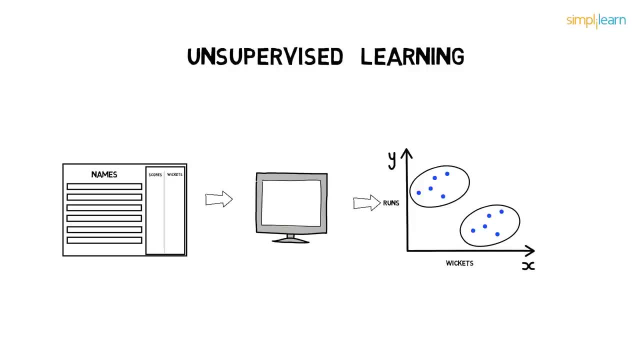 is of the players who scored less runs but took many wickets. so here we interpret these two clusters as batsmen and bowlers. an important point to note here is that there were no labels of the data, so we can say that unsupervised learning with unlabeled data is unsupervised learning. so we 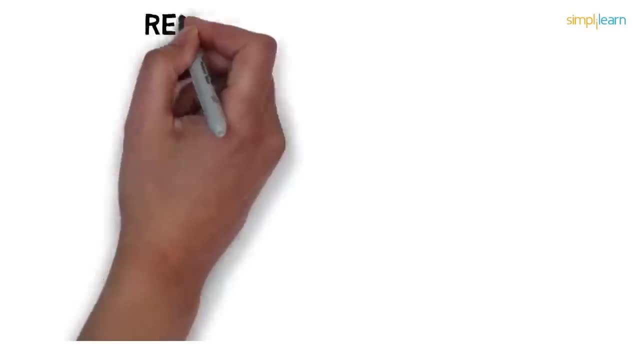 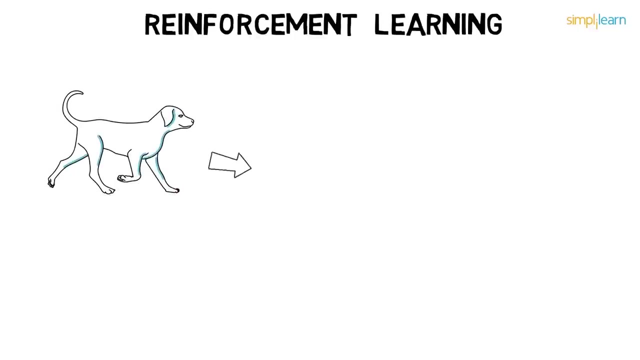 saw supervised learning, where the data was labeled, and the unsupervised learning, where the data was unlabeled. and then there is reinforcement learning, which is reward based learning, or we can say that it works on the principle of feedback. here, let's say, you provide the system with an image of a dog. 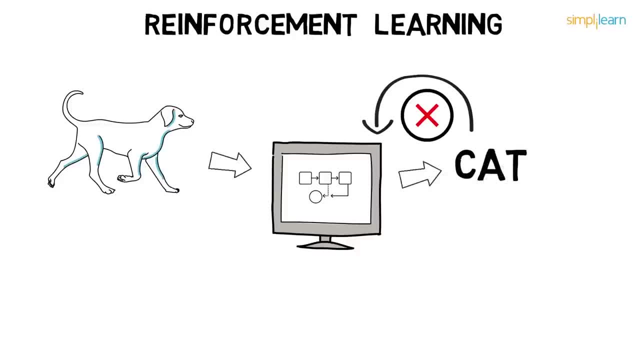 and ask it to identify it. the system identifies it as a cat. so you give a negative feedback to the machine, saying that it's a dog's image. the machine will learn from the feedback and finally, any other image of a dog it will be able to classify it correctly. that is reinforcement. 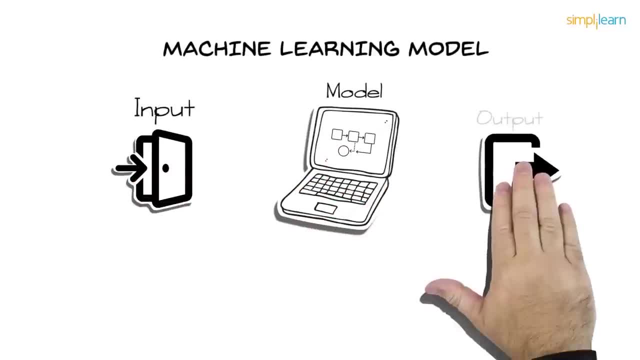 learning. to generalize machine learning model. let's see a flowchart. input is given to a machine learning model which then gives the output according to the algorithm applied. if it's right, we take the output as a final result. else we provide feedback to the training model and ask it. 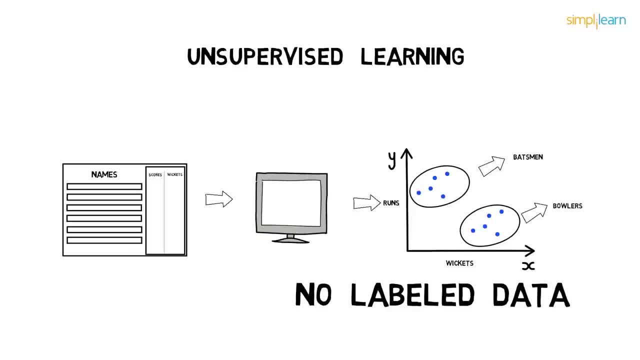 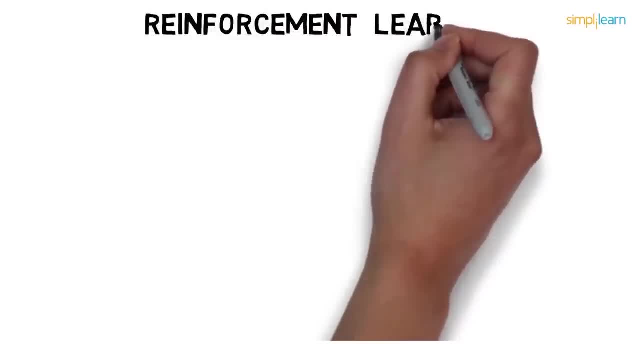 unlabeled data is unsupervised learning. so we saw supervised learning where the data was labeled and the unsupervised learning where the data was unlabeled. and then there is reinforcement learning, which is a reward based learning, or we can say that it works on the principle of feedback. 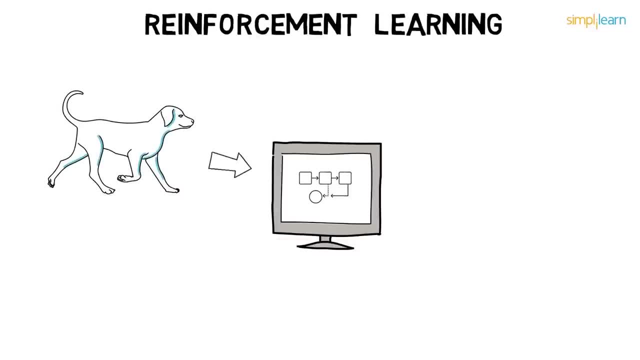 here. let's say you provide the system with an image of a dog and ask it to identify it. the system identifies it as a cat, so you give a negative feedback to the machine, saying that it's a dog's image. the machine will learn from the feedback and finally, if it comes across any 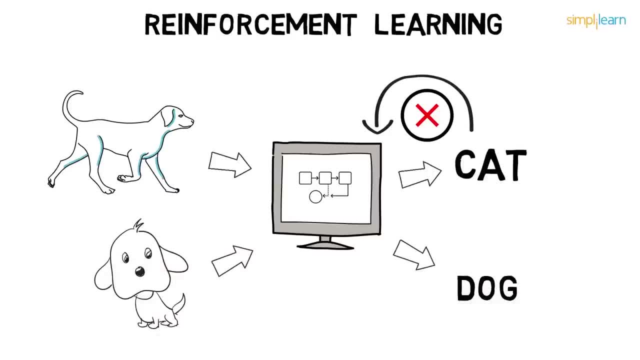 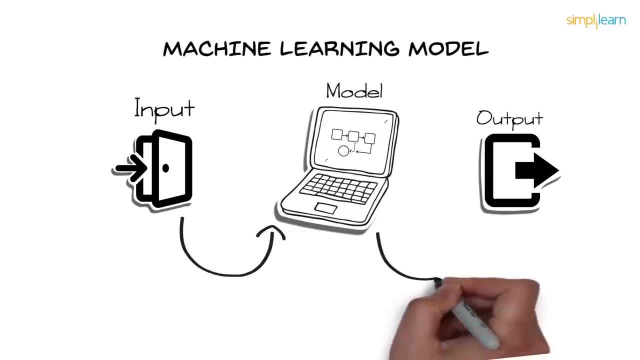 other conditional catch minute in cinnabar or university. whether it is snow, scan志 or other online learning image of a dog, it will be able to classify it correctly. that is reinforcement learning. to generalize machine learning model, let's see a flow chart. input is given to a machine learning model which then gives the 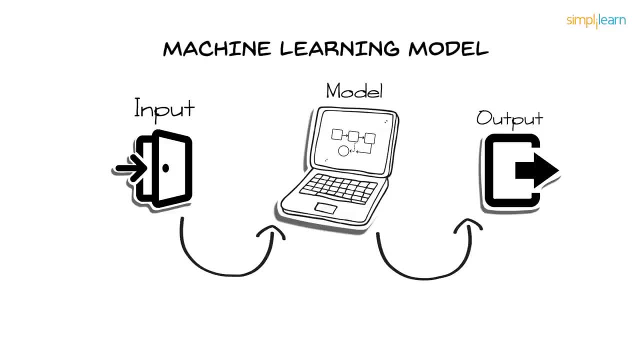 output according to the algorithm applied. if it's right, we take the output as a final result. else we provide feedback to the training model and ask it to predict until it learns. I hope you've understood supervised and unsupervised learning, so let's have a quick quiz. you have to determine whether 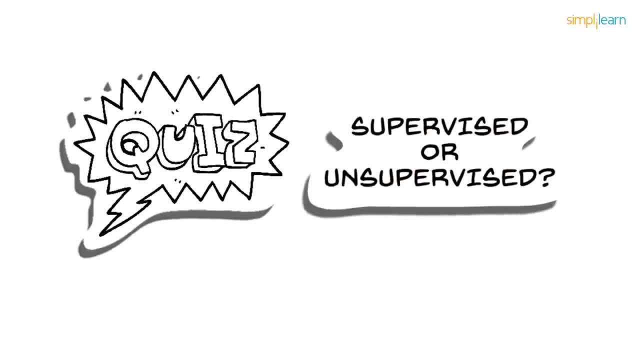 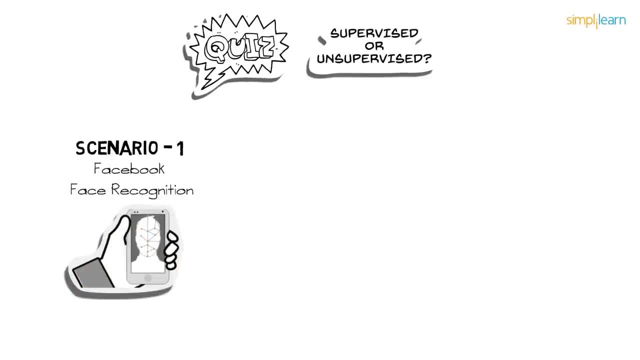 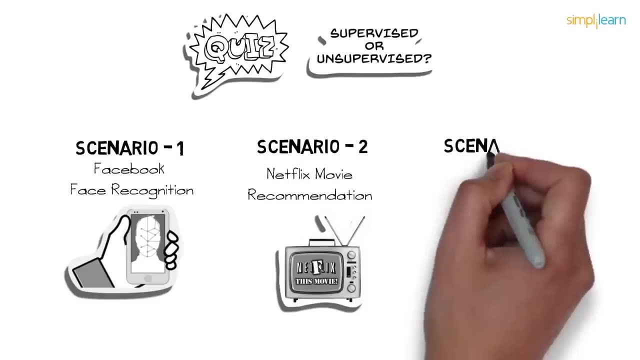 the given scenarios: uses supervised or unsupervised learning. simple right. scenario 1: Facebook recognizes your friend in a picture from an album of tagged photographs. scenario 2: Netflix recommends new movies based on someone's past movie choices. scenario 3: analyzing bank data for suspicious transactions. 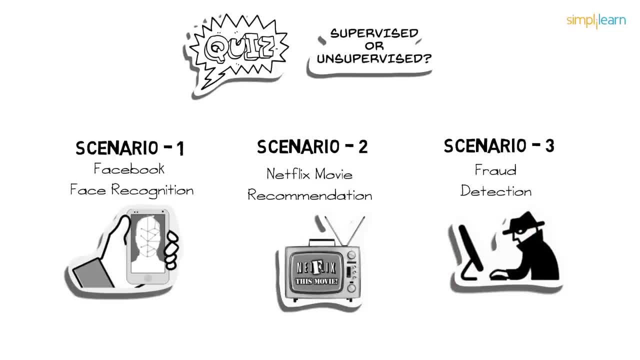 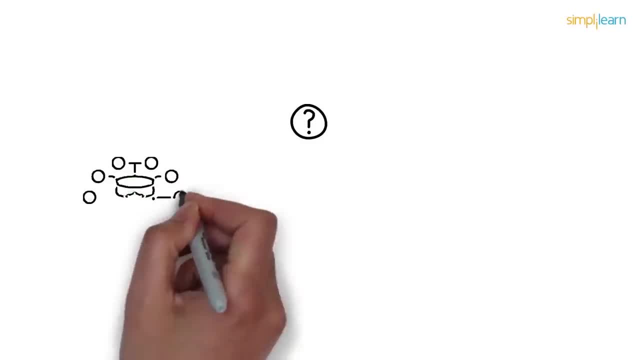 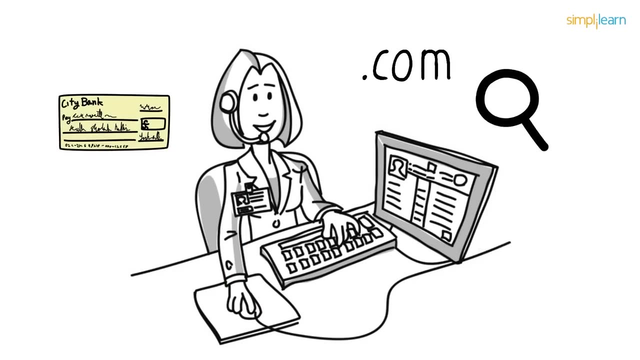 and flagging fraud transactions. think wisely and comment below your answers. moving on, don't you sometimes wonder how is machine learning possible in today's era? well, that's because today we have humongous data available. everybody's online, either making a transaction or just surfing the. 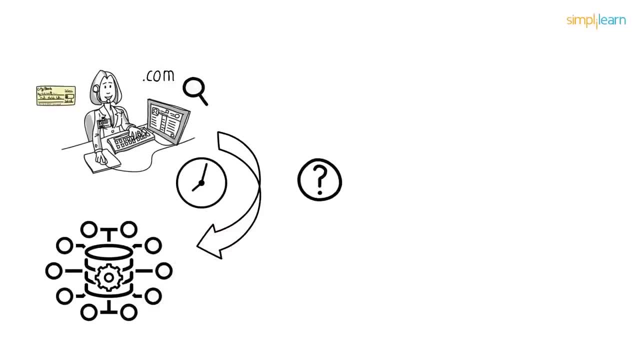 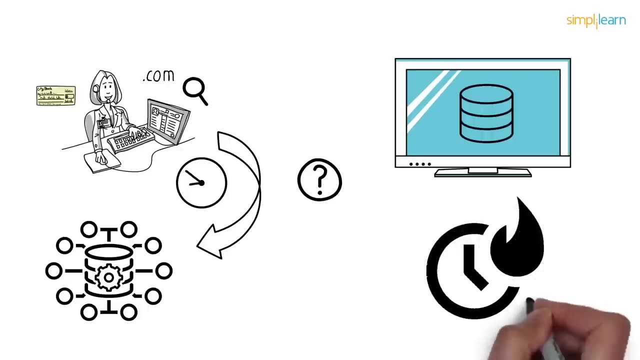 internet and that's generating a huge amount of data every minute. and that data, my friend, is the key to analysis. also, the memory handling capabilities of computers have largely increased, which helps them to process such a huge amount of data at hand without any delay. and yes, computers now have great 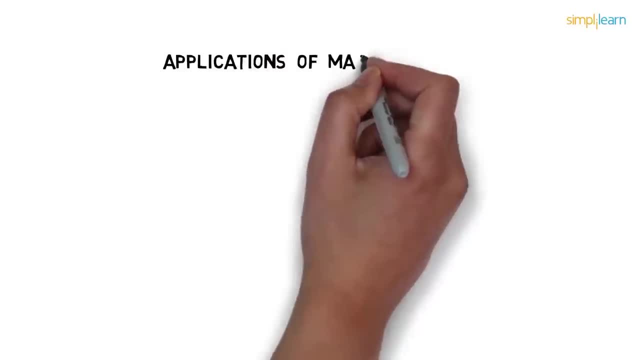 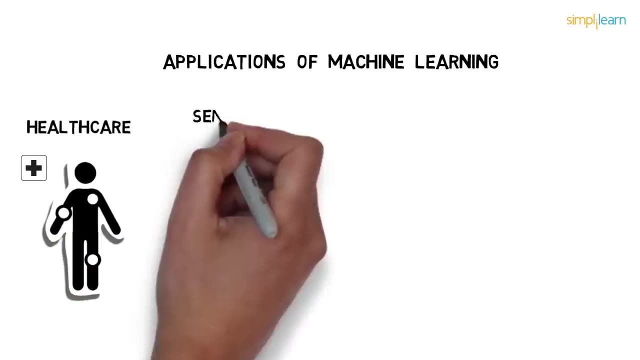 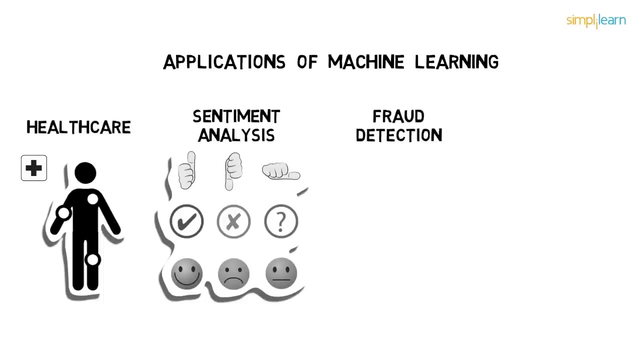 computational powers. so there are a lot of applications of machine learning out there. to name a few, machine learning is used in healthcare, where diagnostics are predicted for doctors review. the sentiment analysis that the tech giants are doing on social media is another interesting application of machine learning: fraud detection in the finance. 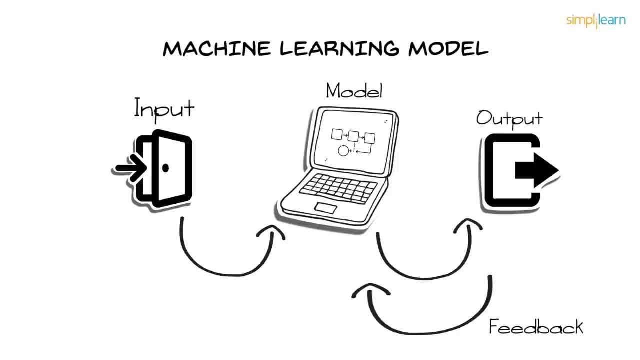 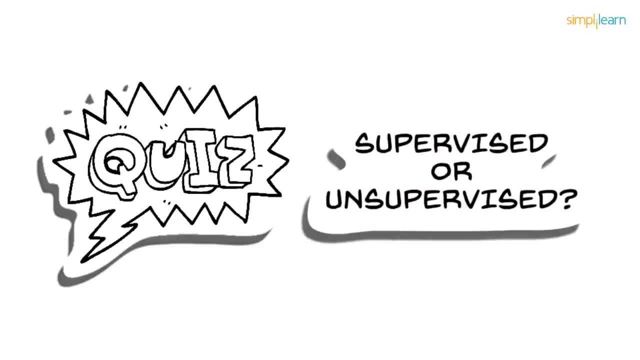 to predict until it learns. i hope you've understood supervised and unsupervised learning. so let's have a quick quiz. you have to determine whether the given scenarios, you have to determine whether the given scenarios. you have to determine whether the given scenarios is supervised or unsupervised learning. simple, right scenario one: facebook recognizes your. 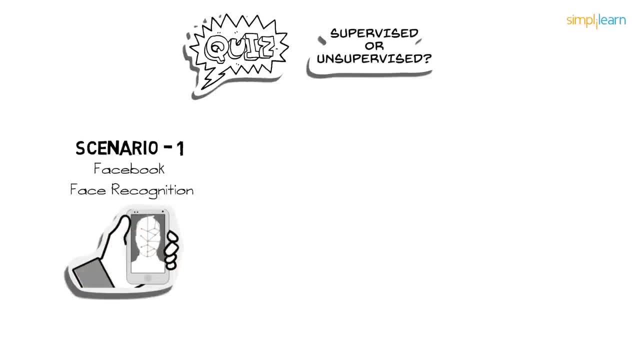 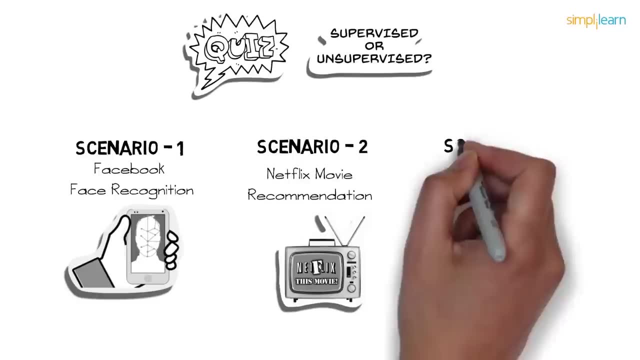 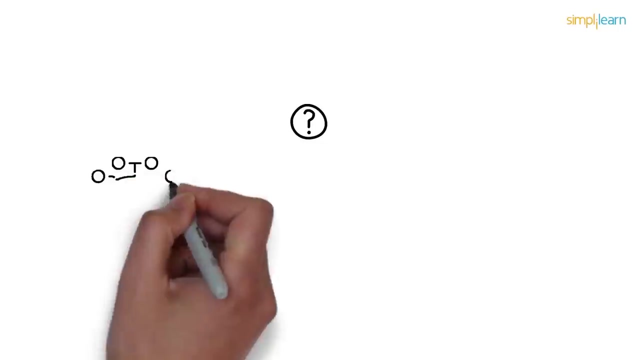 friend in a picture from an album of tagged photographs. scenario 2: netflix recommends new movies based on someone's past movie choices. scenario 3: analyzing bank data for suspicious transactions and flagging the fraud transactions. think wisely and comment below your answers. moving on, don't you sometimes wonder how is machine learning possible in today's era? 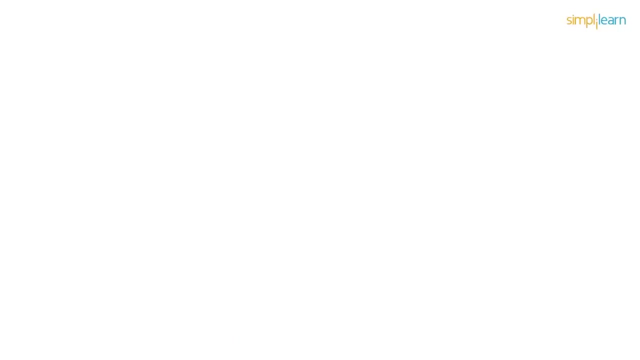 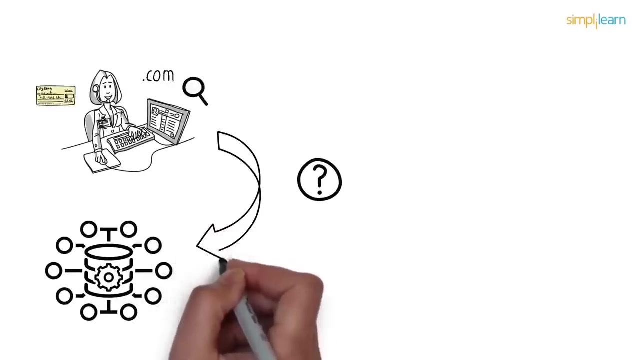 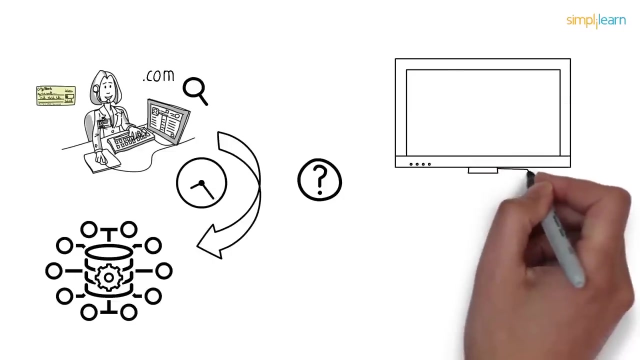 well, that's because today we have humongous data available. everybody's online, either making a transaction or just surfing the internet, and that's generating a huge amount of data every minute. and that data, my friend, is the key to analysis. also, the memory handling capabilities of computers have largely increased, which helps them to process such a huge amount of data at hand. 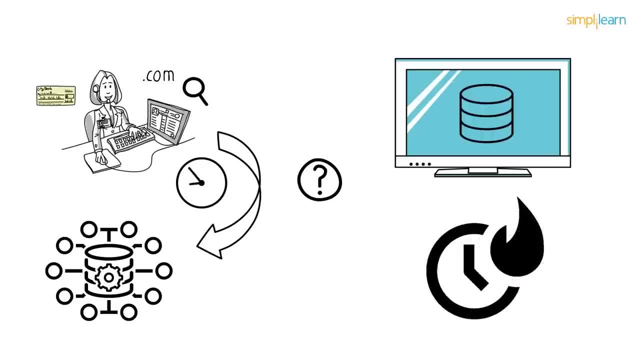 without any delay. and yes, computers now have great computational powers, so there are a lot of applications of machine learning to help them process such huge amount of data at hand without any delay. and yes, computers now have great computational powers, so there are a lot of applications of machine. 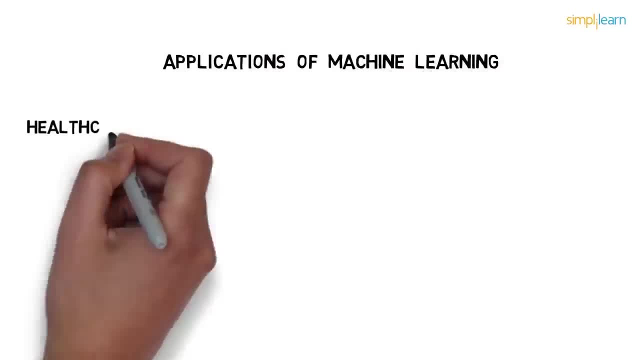 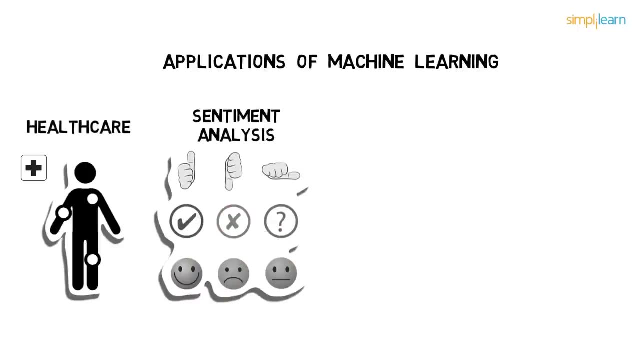 learning out there. to name a few, machine learning is used in healthcare where diagnostics are predicted for doctor's review. the sentiment analysis that the tech giants are doing on social media is another interesting application of machine learning: fraud detection in the finance sector and also to predict customer churn in the e-commerce sector. while booking a gap you must. 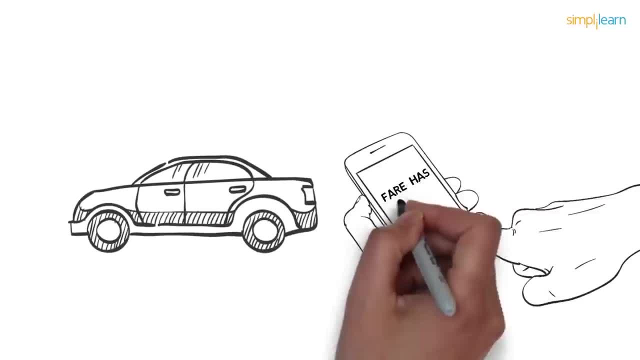 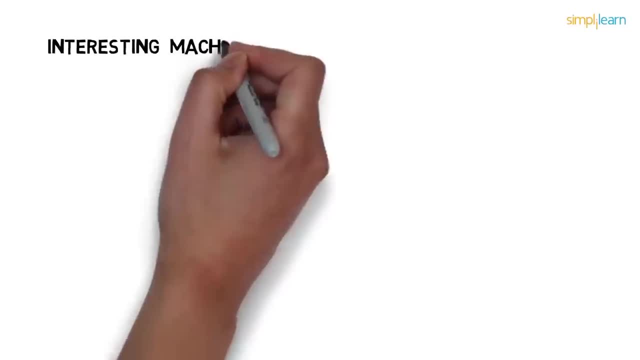 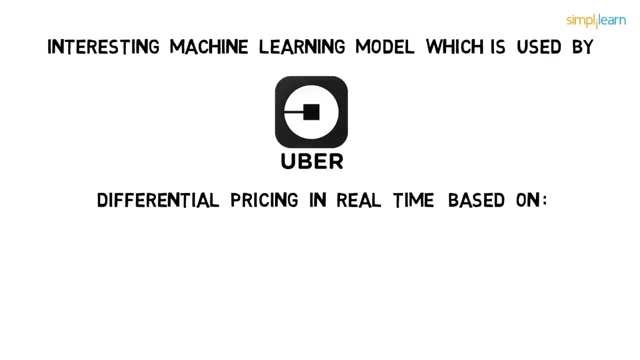 have encountered surge pricing, often where it says the fare of your trip has been updated. continue booking. yes, please, i'm getting late for office. well, that's an interesting machine learning model which is used by global taxi giant, uber and others, where they have differential pricing in real time based on demand, the number of cars available, bad weather. 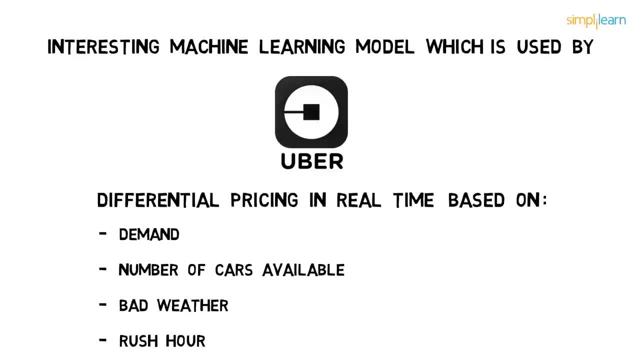 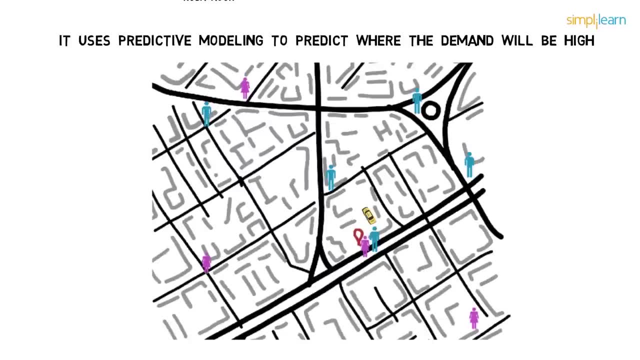 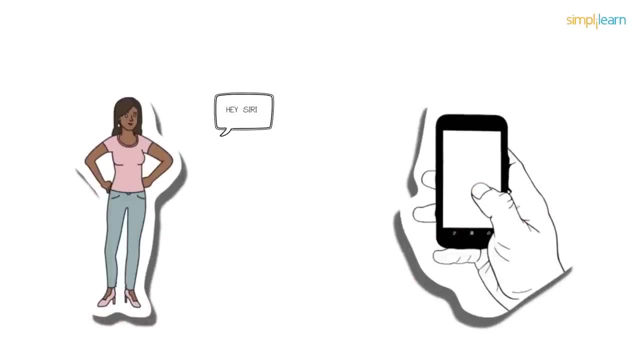 rush hour, etc. so they use the search pricing model to ensure that those who need a cab can get one. also, it uses predictive modeling to predict where the demand will be high, with the goal that drivers can take care of the demand and search pricing can be minimized. great, hey, siri, can you remind me to? 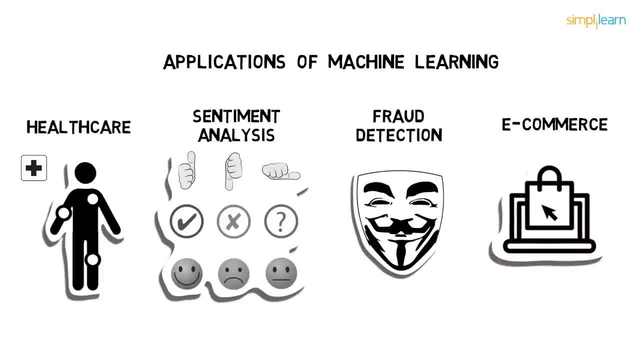 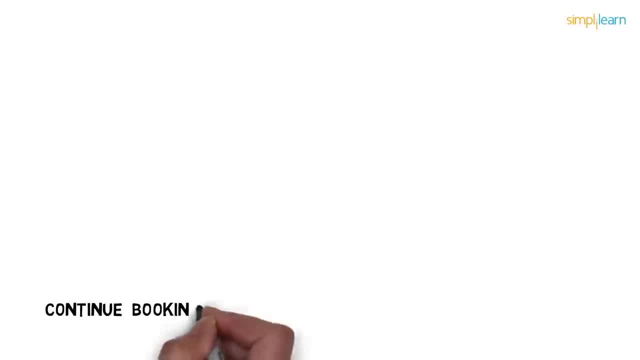 sector and also to predict customer churn in the e-commerce sector. while booking a gap, you must have encountered surge pricing, often where it says the fare of your trip has been updated. continue booking. yes, please, I'm getting late for office. well, that's an interesting machine learning model which is used by Global. 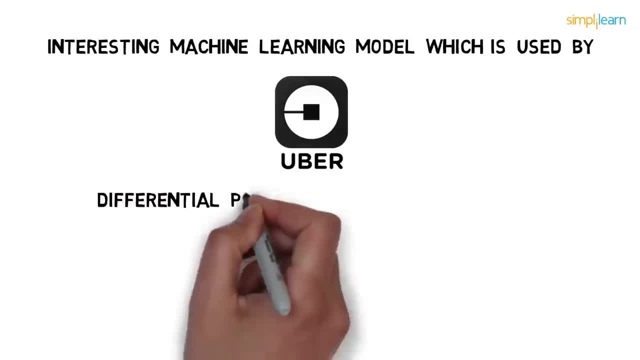 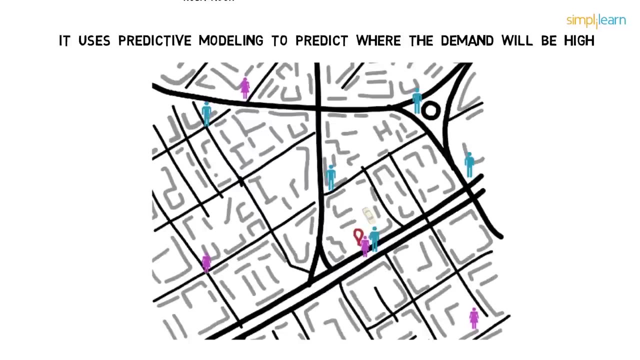 taxi giant, uber and others where they have differential pricing in real time based on demand, the number of cars available, bad weather, rush hour, etc. so they use the surge pricing model to ensure that those who need a cab can get one. also, it uses predictive modeling to predict where the demand will be high. 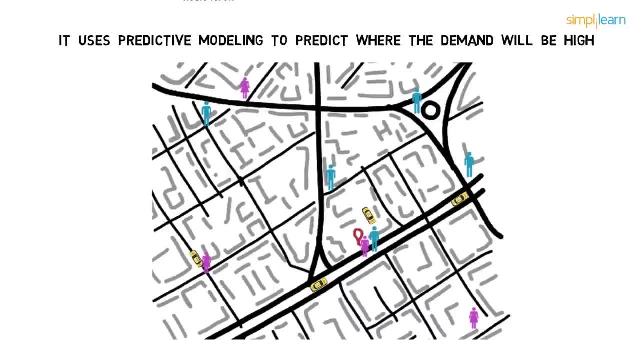 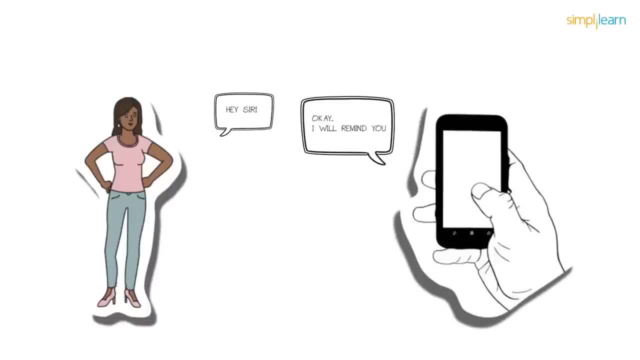 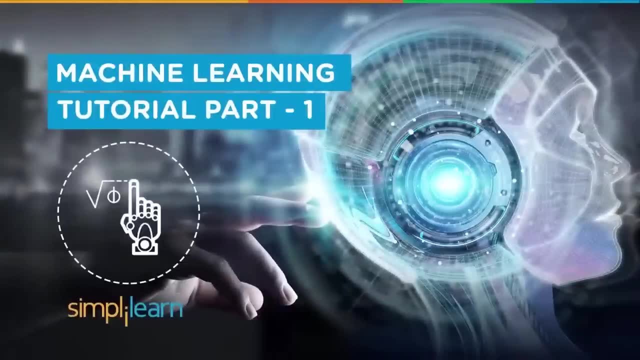 with the goal that drivers can take care of the demand and search pricing can be minimized. great. can you remind me to book a cab at 6 pm today? okay, I'll remind you. thanks, no problem, I hope that has got you all interested to learn machine learning. over to you, Richard. hello and welcome to. 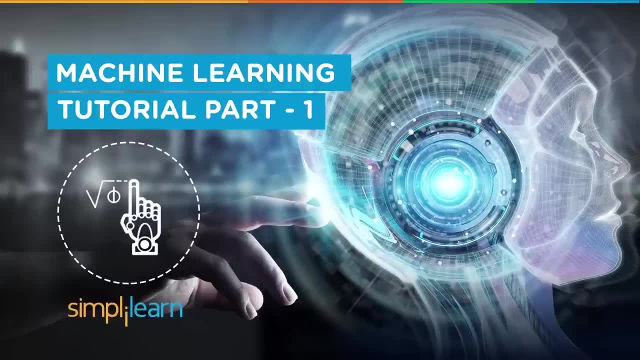 machine learning tutorial, part 1. this is part 1 of a machine learning series put on by simply learn. my name is Richard kirschner. I'm with the simply learn Team, wwwsimplylearncom. get certified, get ahead. so why machine learning? why do we even care about? 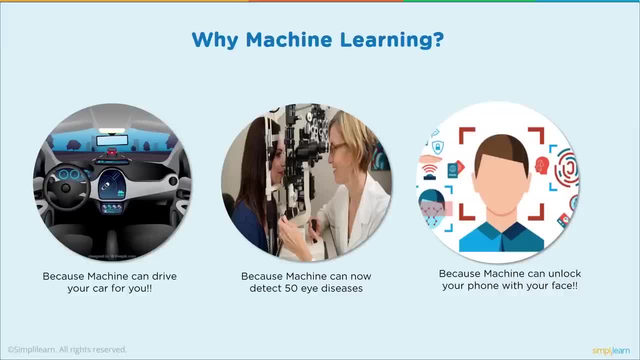 having these computers come up and be able to do all these new things for us? Well, because machines can now drive your car for you. It's still very in the infant stage, but it's just exploding, as we see with Google's Waymo. and then Uber had their program which unfortunately crashed, They know. 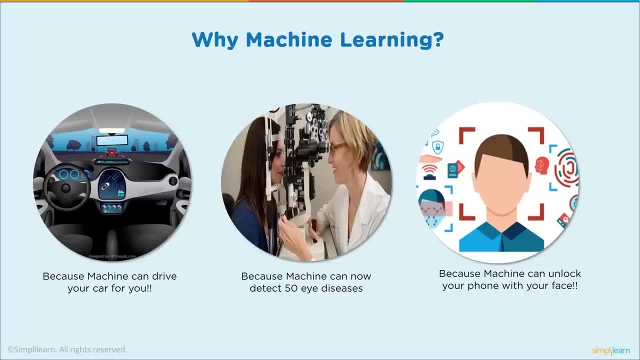 that this is huge. This is going to be the huge industry to change our whole transportation infrastructure. Machine learning has now used to detect over 50 eye diseases. Do you know how amazing that is to have a computer that double checks for the doctor for things they might miss? 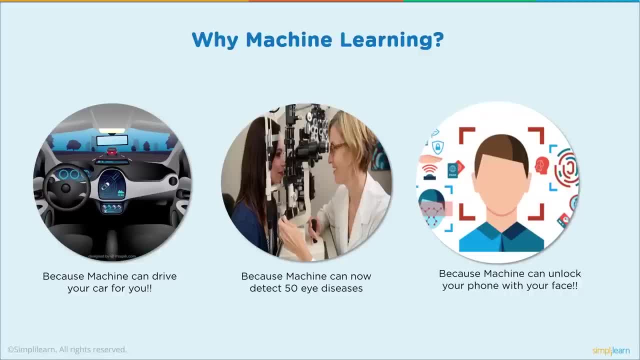 That's just huge in the health industry. Pretty soon they actually do already have that in some areas where- maybe not for eyes but for other diseases- where they're using the camera on your phone to help pre-diagnose before you go in and see the doctor, And because the machine can now 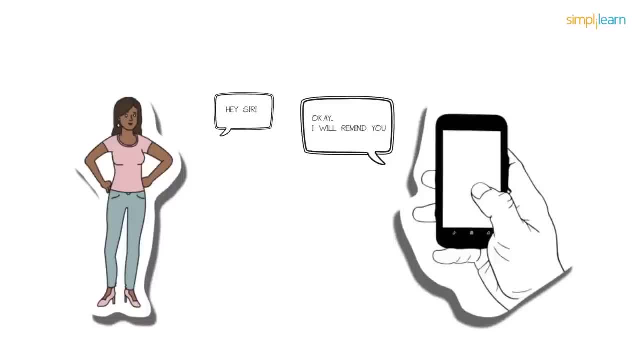 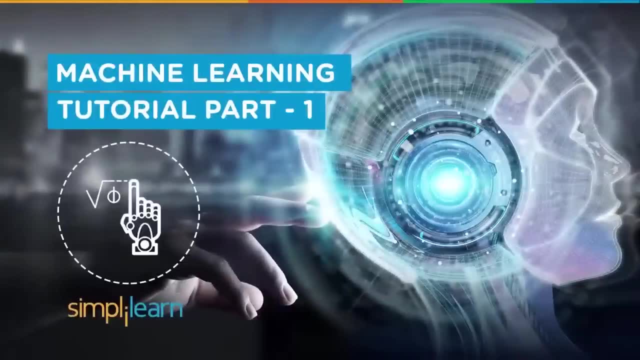 book a cab at 6 pm today. okay, i'll remind you. thanks, no problem, i hope that has got you all interested to learn machine learning. over to you, richard. hello and welcome to machine learning tutorial part one. this is part one of a machine learning series put on by simply learn my name. 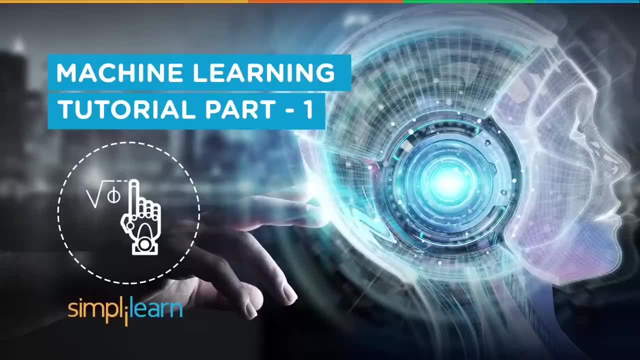 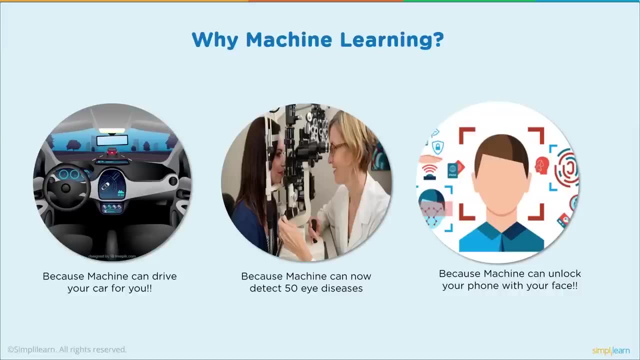 is richard kirchner. i'm with the simply learn team that's wwwsimplylearncom. get certified, get ahead. so why machine learning? why do we even care about having these computers come up and be able to do all these new things for us? well, because machines can now drive your car for you. 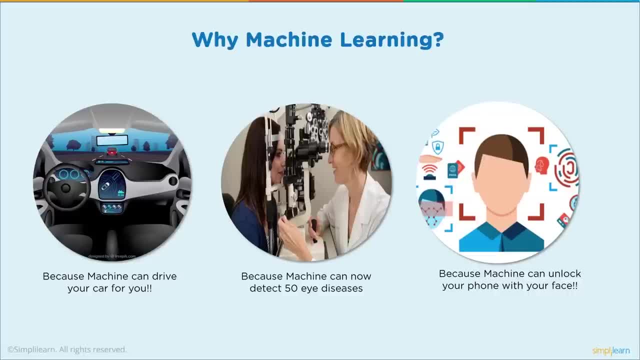 still very in the infant stage, but it's just exploding, as we see with uh, google's waymo, and then uber had their program which unfortunately crashed. they know that this is huge. this is going to be the huge industry to change our whole transportation infrastructure. machine learning. 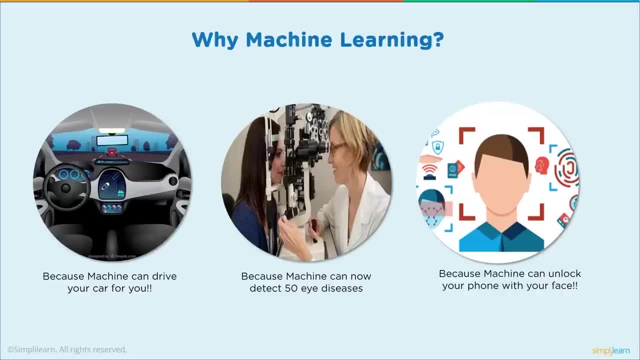 is now used to detect over 50 eye diseases. do you know how amazing that is to have a computer that double checks for the doctor for things they might miss? that's just the way it works. machine learning is huge in the health industry. pretty soon they actually do already have that in some areas where. 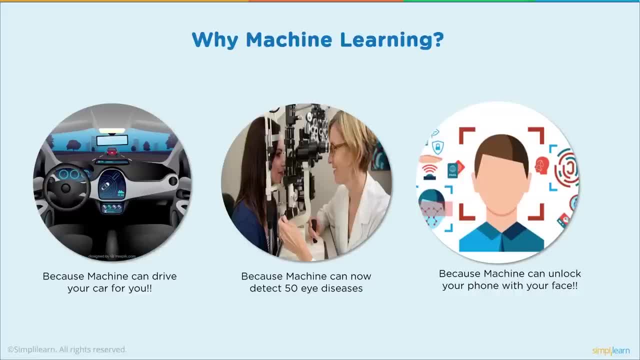 maybe not for eyes but for other diseases where they're using the camera on your phone to help pre-diagnose before you go in and see the doctor. and because the machine can now unlock your phone with your face, i mean that's just cool having it being able to identify your face or your voice. 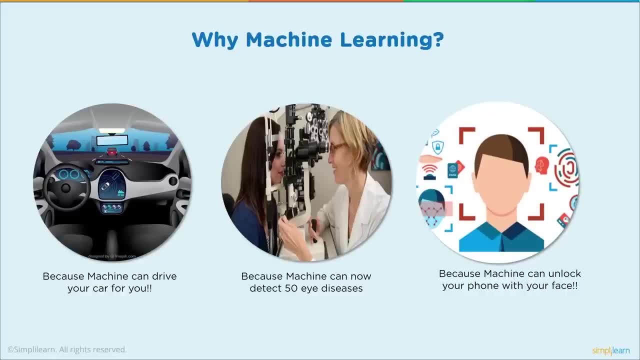 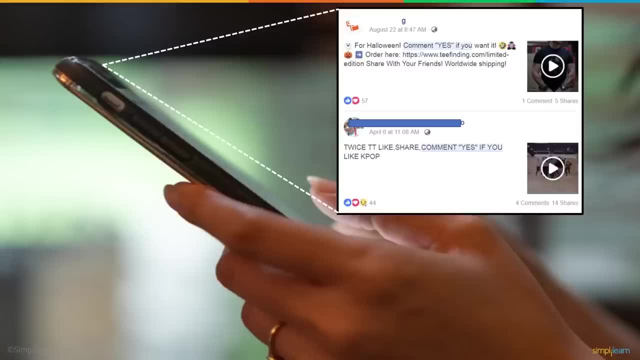 and be able to turn stuff on and off for you depending on where you're at and what you need. talking about an ultimate automation, our world we live in and, as we dig in deeper, we have a nice example of facebook, as you can see here. they have the facebook post with halloween comment. yes, if you. 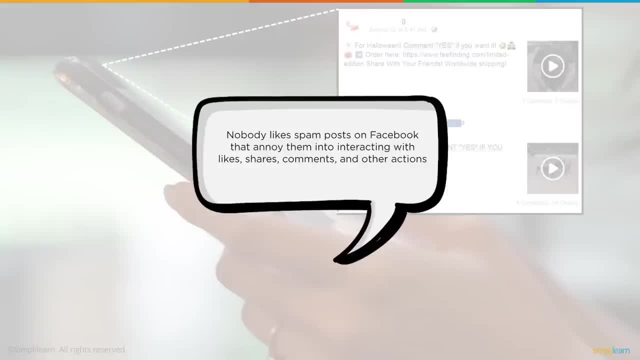 want it order here. nobody likes spam posts on facebook that annoy them into interacting with likes, shares, comments and other actions. i remember the original ones were all: if you don't click on here, you will have bad luck or some kind of fear factor. well, this is a huge thing in social media. 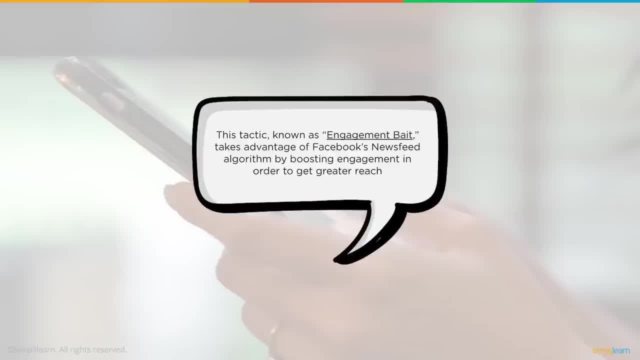 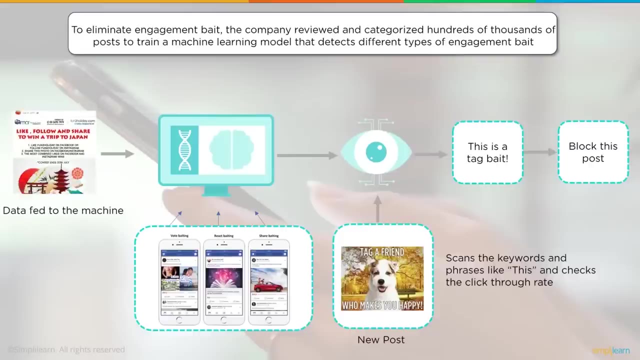 when people are getting spammed, and so this tactic known as engagement bait takes advantage of facebook's news feed algorithm by choosing engagement in order to get the greater reach. to eliminate engagement bait, the company reviewed and categorized hundreds of thousands of posts to train a machine learning model that detects different types of engagement bait. so in this, 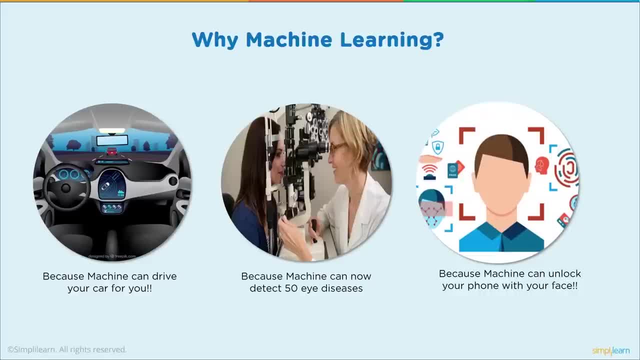 unlock your phone with your face. I mean, that's just cool having it be able to identify your face or your voice and be able to turn stuff on and off for you, depending on where you're at and what you need. Talk about an ultimate automation. our world we live in And, as we dig in deeper, we have a nice. 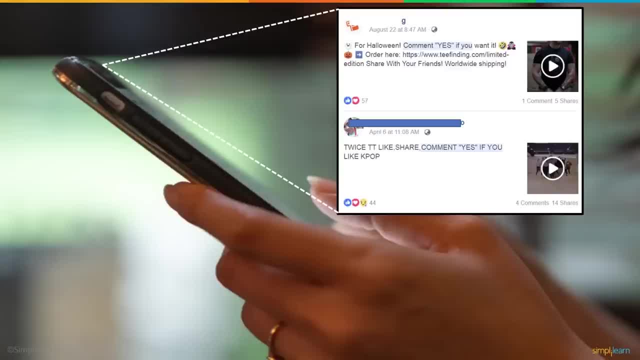 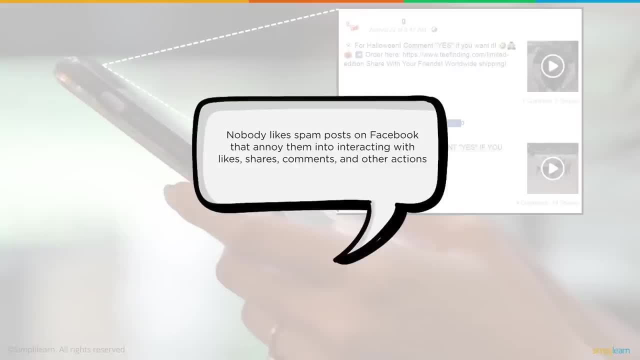 example of Facebook. As you can see here, they have the Facebook post with Halloween Comment. yes, if you want it, Order here. Nobody likes spam posts on Facebook that annoy them into interacting with likes, shares, comments and other actions. I remember the original ones were all. if you don't, 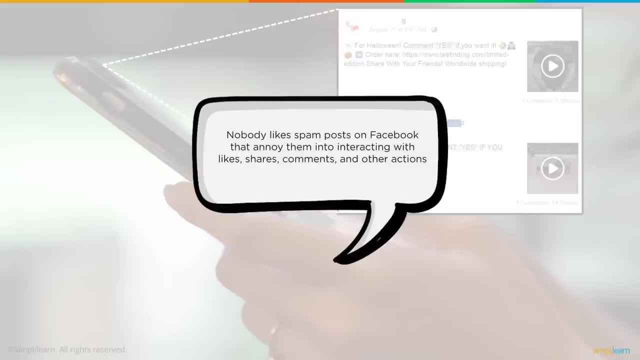 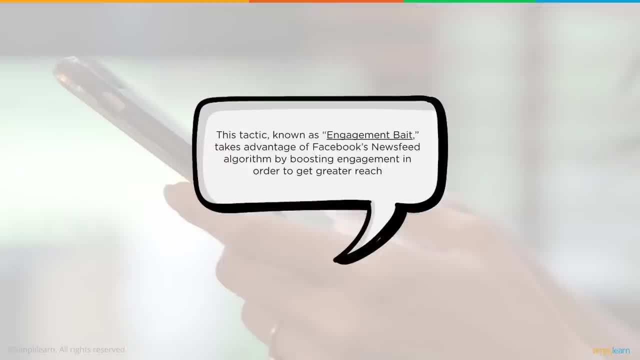 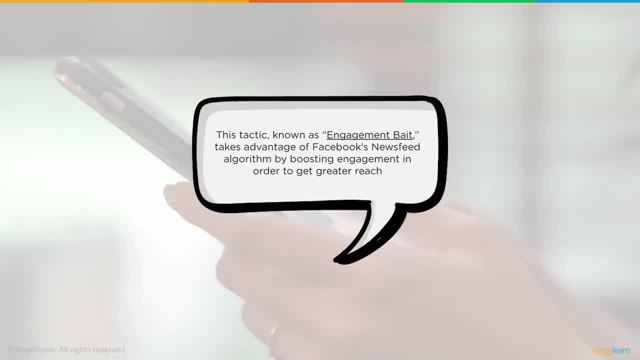 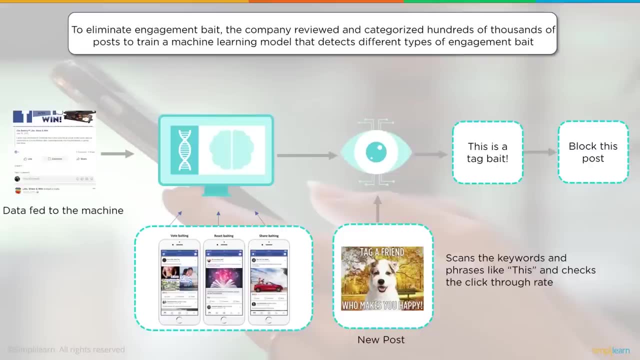 Facebook's news feed algorithm by choosing engagement in order to get the greater reach. To eliminate engagement bait, the company reviewed and categorized hundreds of thousands of posts to train a machine learning model that detects different types of engagement bait. So in this case, we have we're. 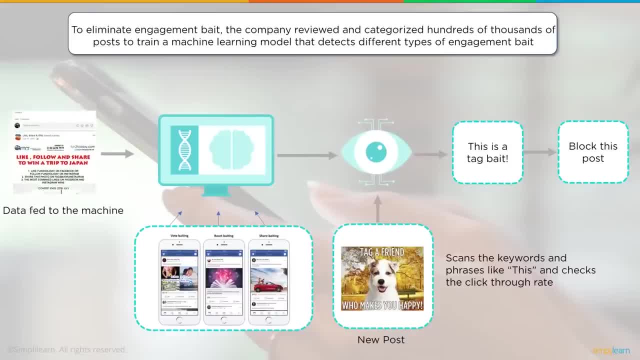 using Facebook, but this is, of course, across all the different social media. They have different tools. they're building And the Facebook scroll GIF will be replaced. a virus coming in there. It notices that there's a certain setup with Facebook and it's able to. 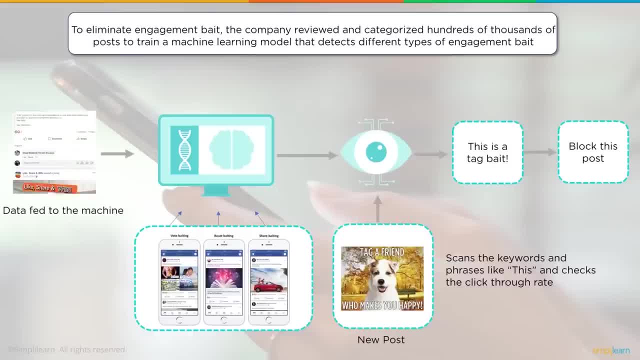 replace it And they have like: vote baiting, react baiting, share baiting, They have all these different. these are kind of general titles, but there certainly are a lot of way of baiting you to go in there and click on something, So they fed all this. This data was fed into the machine. 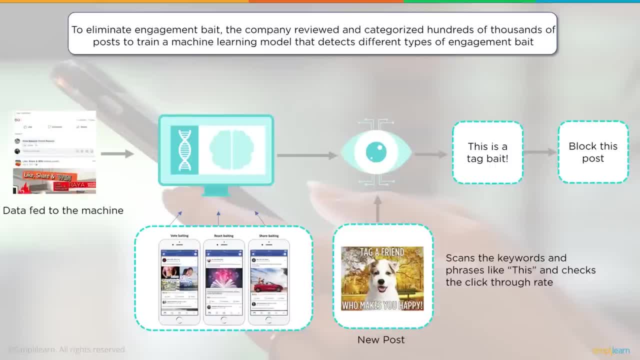 and then they have the new post. The new post comes up that takes over part of the Facebook setup, And that's what you're looking at. You're looking at this new post that's replaced like a virus has replaced that. So what Facebook did to eliminate this is they start scanning for. 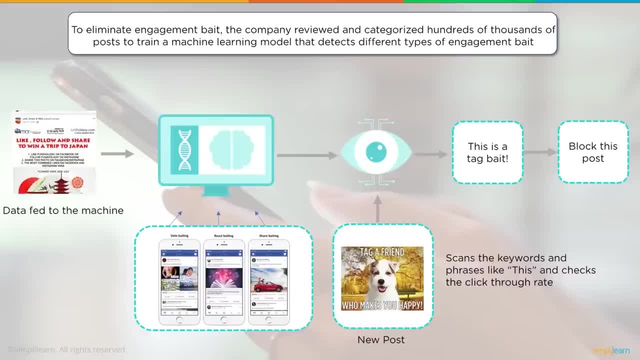 keywords and phrases like this and checks the click-through rate, So it starts looking for people who are clicking through it without even looking at it or clicking through it. It's not something that normally would be clicked through Once Facebook has scanned for these keywords and 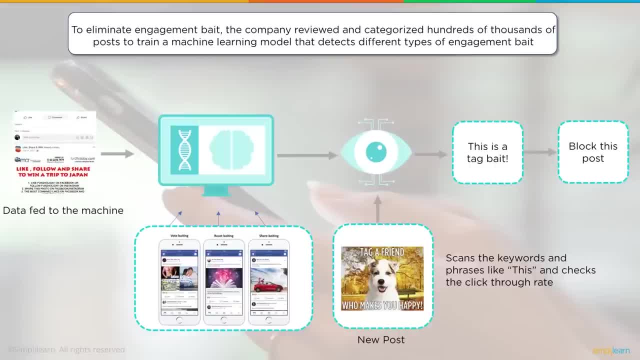 phrases. it is now able to identify the spam coming in And this makes your life easier, So you're not getting spammed. It's not like walking through an airport, And in a lot of countries you have like hundreds of people trying to. 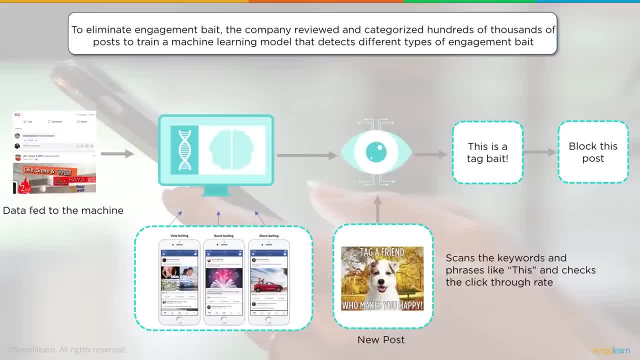 case we have. we're using facebook, but this is, of course, across all the different social media they have. different tools are building and the facebook scroll gif will be replaced. kind of like a virus coming in there. it notices that there's a certain setup with facebook and it's able to. 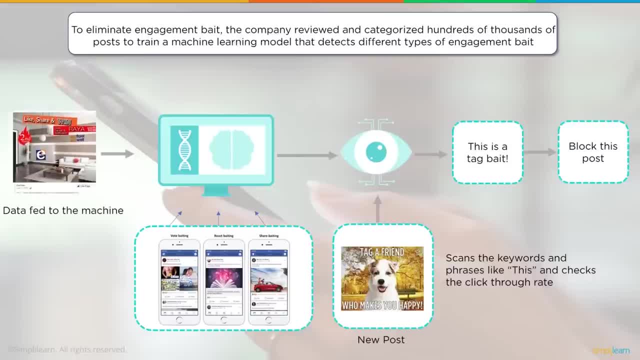 eliminate this and they have like: vote baiting, react baiting, share baiting. they have all these different. these are kind of general titles, but there certainly are a lot of way of baiting you to go in there and click on something so they fed all this. this data was fed into the machine. 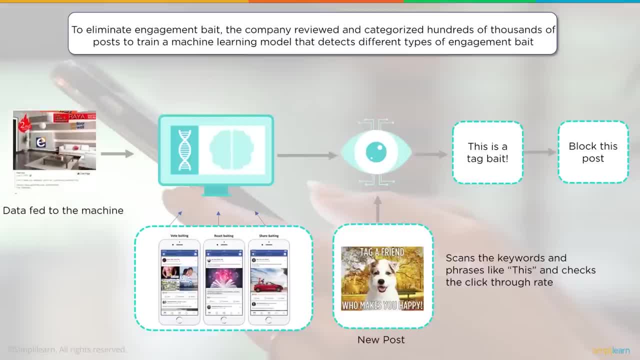 and then they have the new post. the new post comes up that takes over part of the facebook setup, and that's what you're looking at. you're looking at this new post that's replaced like a virus has replaced that. so what facebook did to eliminate this is they start scanning for keywords. 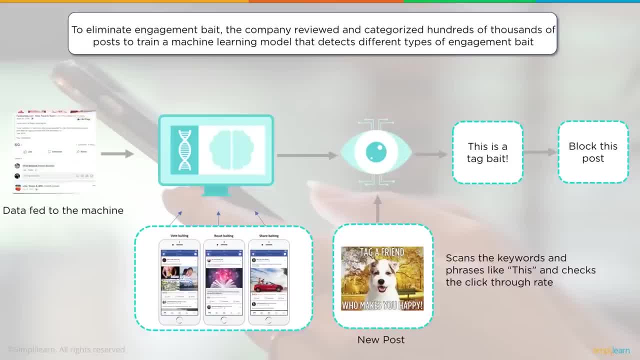 and phrases like this and checks the click-through rate, so it starts looking for people who are clicking through it without even looking at it or clicking through it. it's not something that normally would be clicked through. once facebook has scanned for these keywords and phrases, it is now able to identify the spam coming in, and this makes your 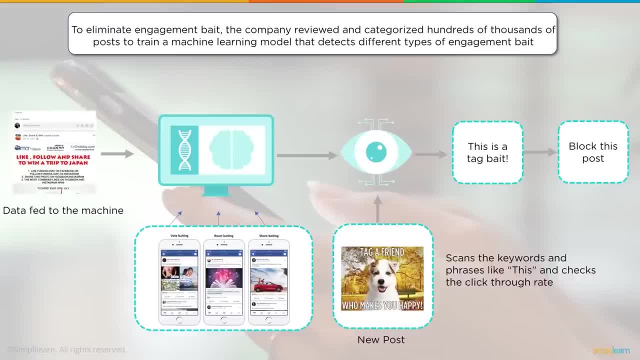 life easier so you're not getting spammed. it's not like walking through an airport, and in a lot of countries you have like hundreds of people trying to sell you timeshare. come join us. sign up for this eliminates that annoyance, so now you can just enjoy your facebook and your cat pictures, or 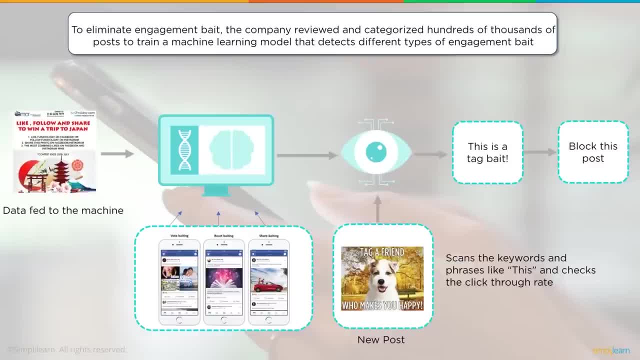 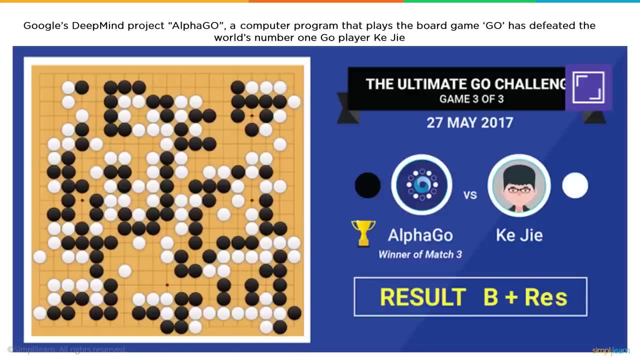 pictures. mine is family. certainly people like their cat pictures too. another good example is google's deep mind project alpha go, a computer program that plays a board game. go has defeated the world's number one go player- and i hope i say his name right- kiji the ultimate go challenge game. 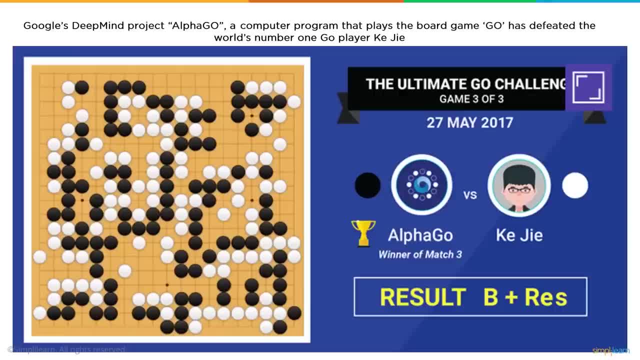 of three of three was on may 27, 2017, so that was just last year that this happened, and what makes this so important is that you know, go is just is a game, so it's not like you're driving a car or something in our real world, but they are using games to learn how to get the machine learning. 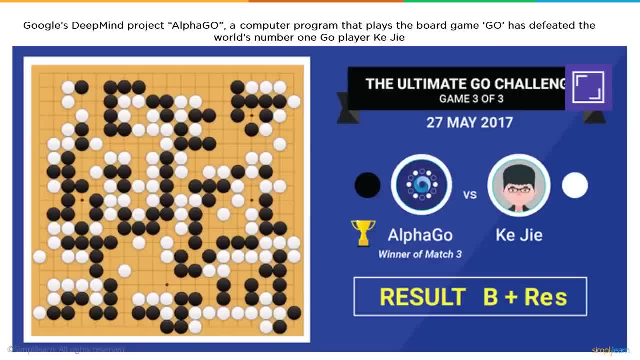 program to learn. they want it to learn how to learn, and that is a huge step. a lot of this is still in its infant stage as far as development, as we saw what happened with the- as i referred to earlier- the uber cars: they lost their whole division because they jumped ahead too fast. 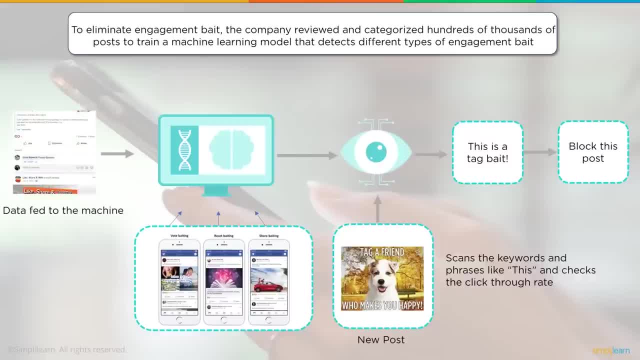 sell you timeshare. Come join us. Sign up for this. It eliminates that annoyingness. So now you can just enjoy your Facebook and your cat pictures- Or maybe it's your family pictures- Mine is family. Certainly, people like their cat pictures too. Another good example is Google's. 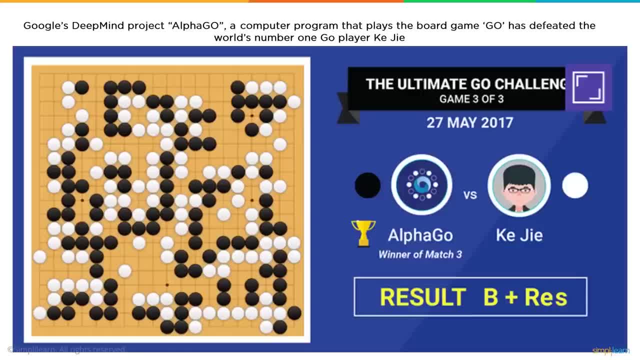 DeepMind project. AlphaGo, A computer program that plays a board game, Go, has defeated the world's number one Go player And I hope I say his name right- Kiji. The ultimate Go challenge game of three of three was on May 27th 2017.. 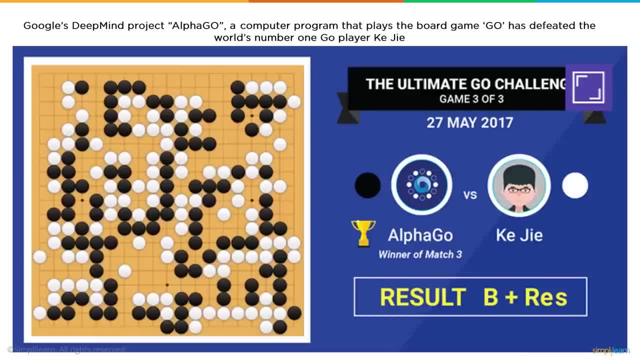 You canjου Como Kerx Cook, Not well past that. it was just last year that this happened, And what makes this so important is that Go is just is a game, So it's not like you're driving a car or something in our real world, But they are. 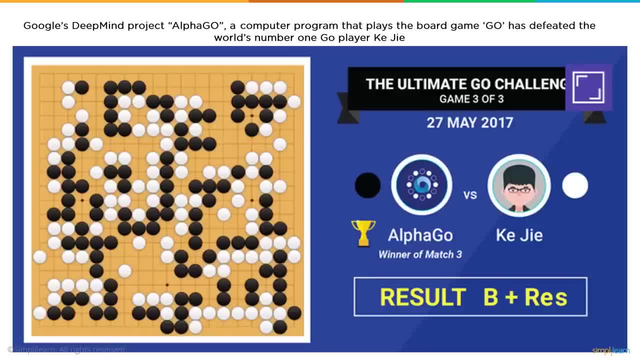 using games to learn how to get the machine learning program to learn. They want it to learn how to learn, And that is a huge step. A lot of this is still at its infant stage as far as development, as we saw What happened with the- as I referred to earlier, the Uber cars. They lost their whole division because they weren't loaded enough. And it's not like cta. Google didn't offer any jobs for said drop in Google folks because I think they didn't have the time. toody Me think it was став. then steps back up for you. Was that anatorsis, of course, For the game, Fr minister, This is the problem. 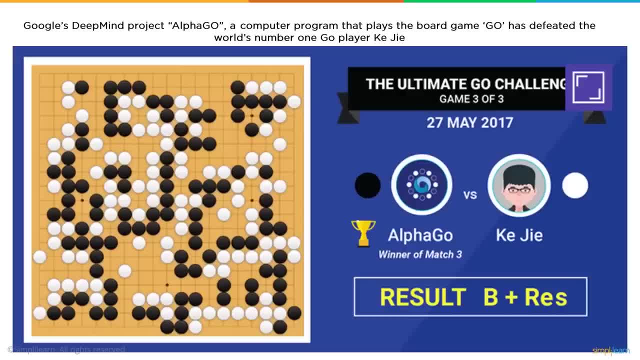 because they jumped ahead too fast. So still an infant stage. but boy is this like the beginning of just an amazing world that is automated in ways we can't even imagine what tomorrow's going to look like. We've looked at a lot of examples of machine learning. 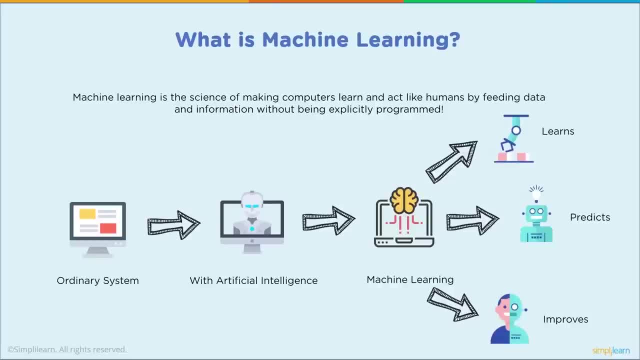 so let's see if we can give a little bit more of a concrete definition. What is machine learning? Machine learning is the science of making computers learn and act like humans by feeding data and information without being explicitly programmed. And we see, here we have a nice little diagram. 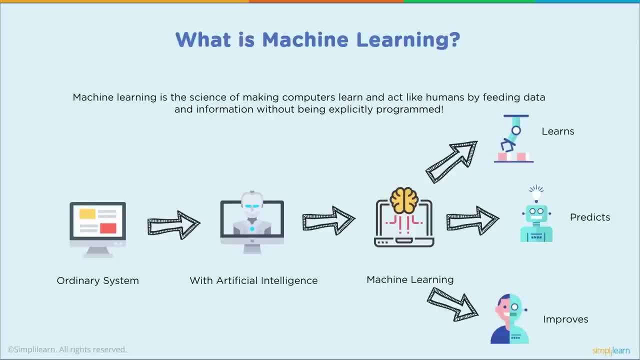 where we have our ordinary system. Your computer nowadays can even run a lot of this stuff on a cell phone, because cell phones have advanced so much. And then, with artificial intelligence and machine learning, it now takes the data and it learns from what happened before. 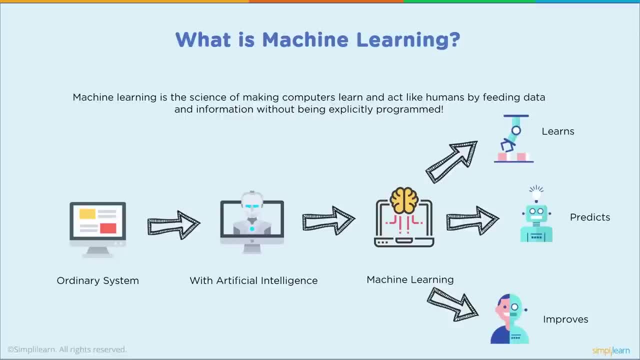 and then it predicts what's going to come next and then really the biggest part right now in machine learning that's going on is it improves on that. How do we find a new solution? So we go from descriptive where it's learning. 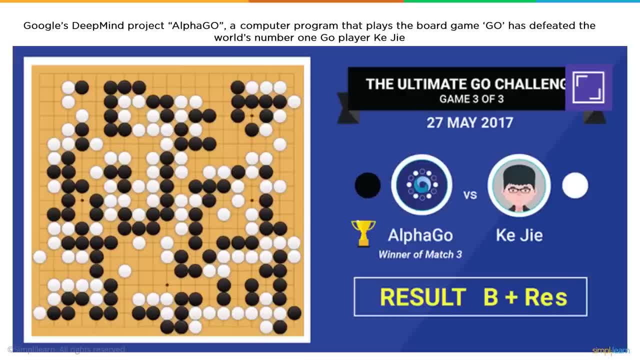 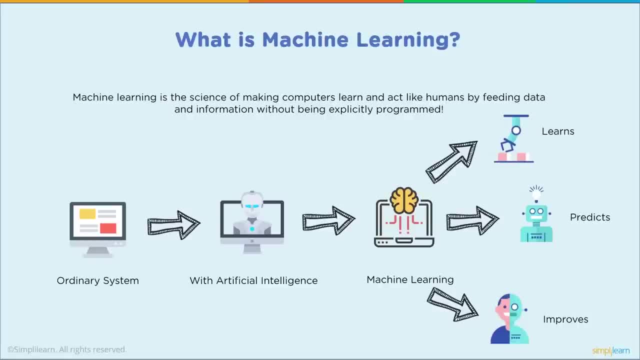 so still an infant stage, but boy is this like the beginning of just an amazing world that is automated in ways we can't even imagine. we can't even imagine, we can't even imagine, we can't even even imagine what tomorrow is going to look like. we've looked at a lot of examples of machine. 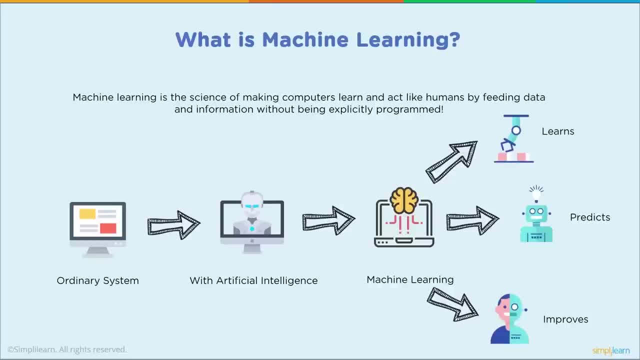 learning. so let's see if we can give a little bit more of a concrete definition. what is machine learning? machine learning is the science of making computers learn and act like humans by feeding data and information without being explicitly programmed. we see, here we have a nice little. 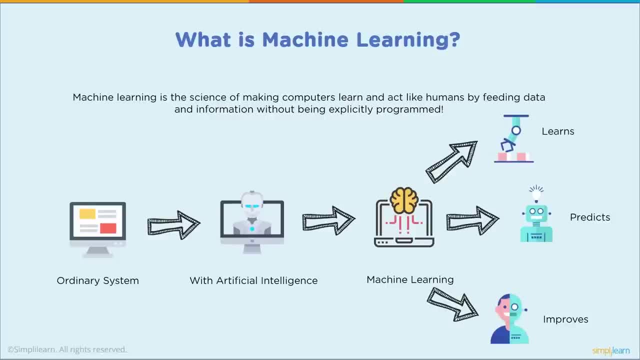 diagram where we have our ordinary system and your computer. nowadays you can even run a lot of the stuff on a cell phone, because cell phones advance so much. and then, with our artificial intelligence and machine learning, it now takes the data and it learns from what happened before and then it predicts what's going to come next. and then really the biggest part, right. 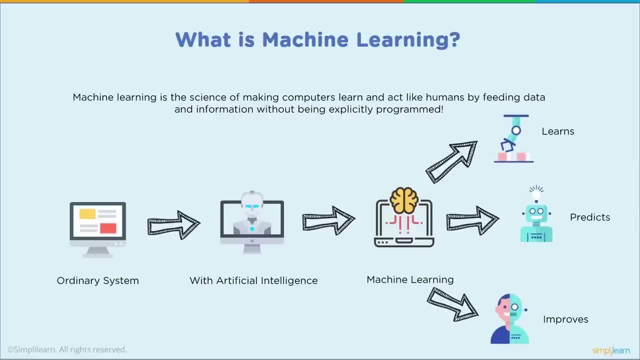 now in machine learning that's going on. is it improves on that? how do we find a new solution? so we go from descriptive, where it's learning about stuff and understanding how it fits together, to predicting what it's going to do, to post scripting, coming up with a new solution, and 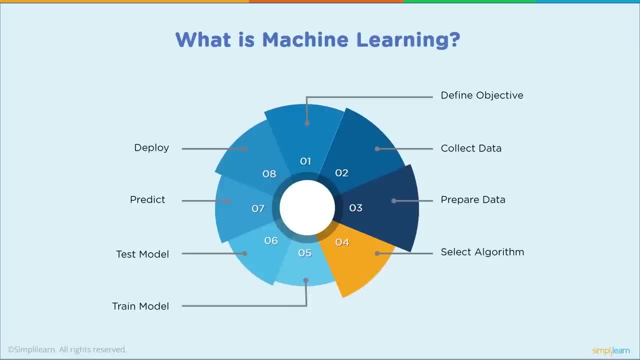 when we're working on machine learning. there's a number of different ways to do that, so we're going to do a number of different diagrams that people have posted for what steps to go through. a lot of it might be very domain specific. so if you're working on photo identification versus language versus 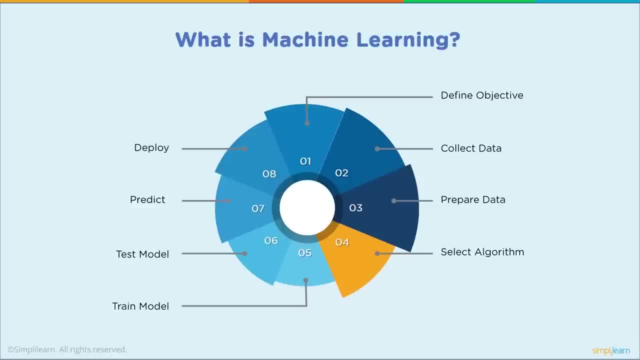 medical or physics. some of these are switched around a little bit or new things are put in the very specific to the domain. this is kind of a very general diagram. first you want to define your objective. very important to know what it is you're wanting to predict. then you're going to be. 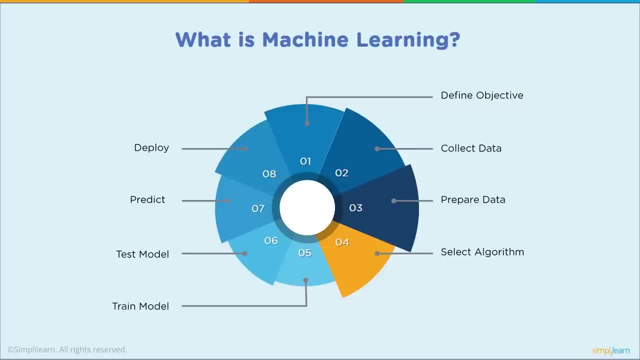 collecting the data. so once you've defined an objective, you need to collect the data matches. You spend a lot of time in data science, collecting data and the next step, preparing the data. You got to make sure that your data is clean going in. There's the old saying: bad data in bad. 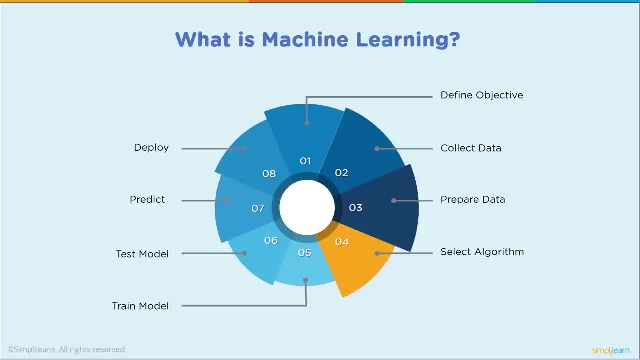 answer out or bad data out, And then, once you've gone through and we've cleaned all this stuff coming in, then you're going to select the algorithm. Which algorithm are you going to use? You're going to train that algorithm. In this case, I think we're going to be working with SVM, the support. 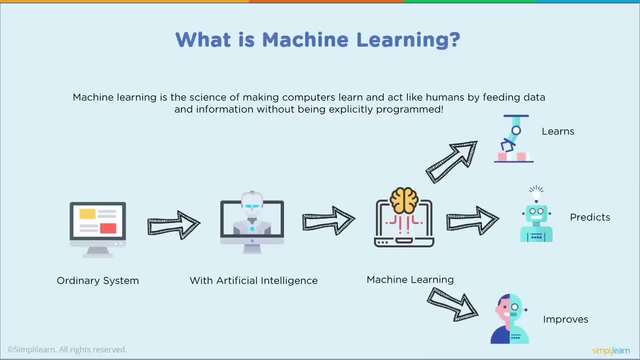 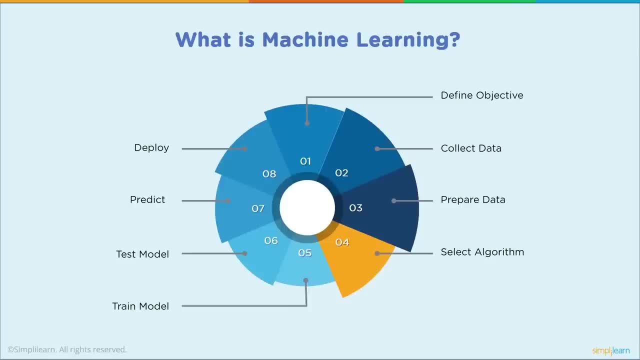 learning about stuff and understanding how it fits together, to predicting what it's going to do, to postscripting, coming up with a new solution, And when we're working on machine learning. there's a number of different diagrams that people have posted. 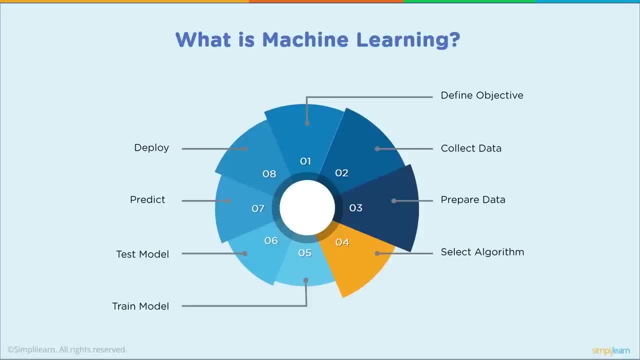 for what steps to go through. A lot of it might be very domain-specific. So if you're working on photo identification versus language, versus medical or physics, some of these are switched around a little bit, or new things are put in that are very specific to the domain. 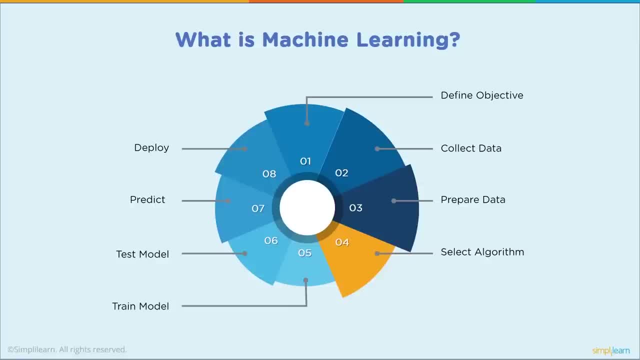 This is kind of very different, but it's a very general diagram. First you want to define your objective- Very important to know what it is you're wanting to predict. Then you're going to be collecting the data. So once you've defined an objective, 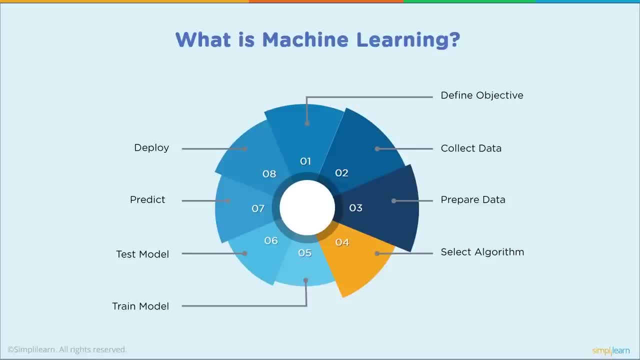 you need to collect the data that matches. You spend a lot of time in data science, collecting data and the next step, preparing the data. You've got to make sure that your data is clean going in. There's the old saying: bad data in, bad answer out or bad data out. 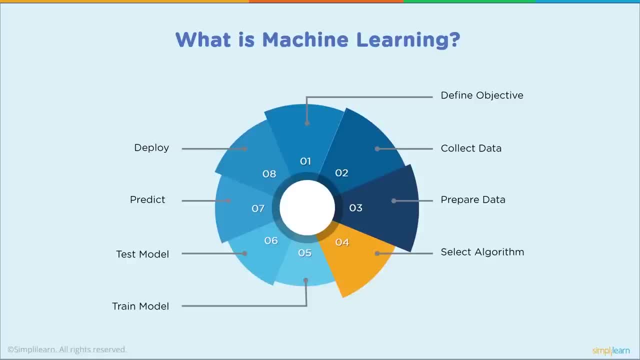 And then, once you've gone through and we've cleaned all this stuff coming in, then you're going to be able to go back and look at the data. And then, once you've gone through and we've cleaned all this stuff coming in, then you're going to be able to go back and look at the data. 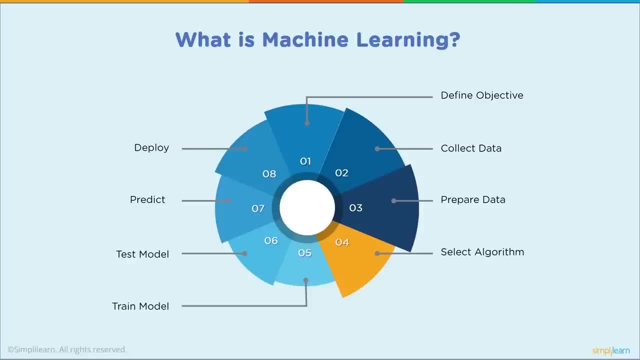 Then you're going to select the algorithm. Which algorithm are you going to use? You're going to train that algorithm. In this case, I think we're going to be working with SVM, the support vector machine. Then you have to test the model. 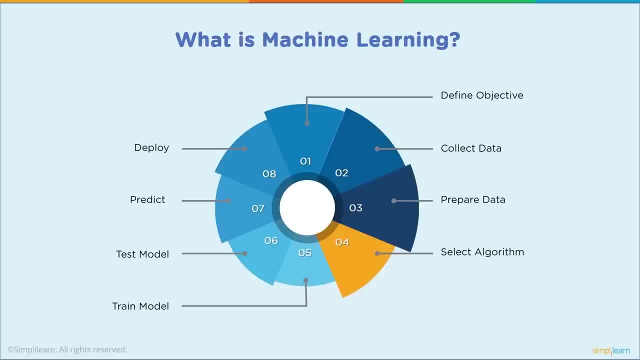 Does this model work? Is this a valid model for what we're doing? And then, once you've tested it, you want to run your prediction. You want to run your prediction or your choice, or whatever output it's going to come up with. 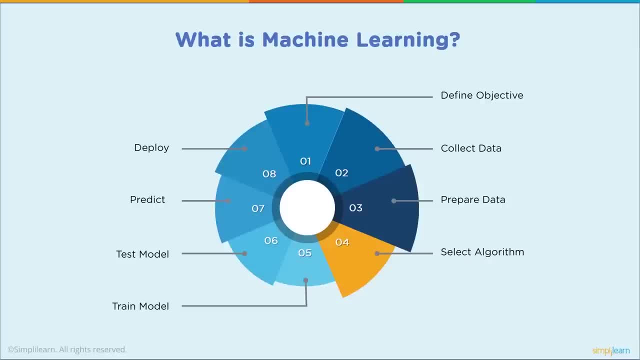 And then once everything is set and you've done lots of testing, then you want to go ahead and deploy the model. Remember I said domain specific. This is very general as far as the scope of doing something. A lot of models you get halfway through. 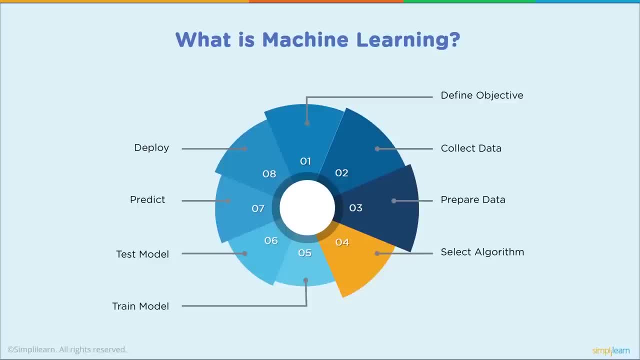 and you realize that your data is missing something and you have to go collect new data because you've run a test in here. someplace along the line, You're saying, hey, I'm not really getting the answers I need. So there's a lot of things that are domain specific. 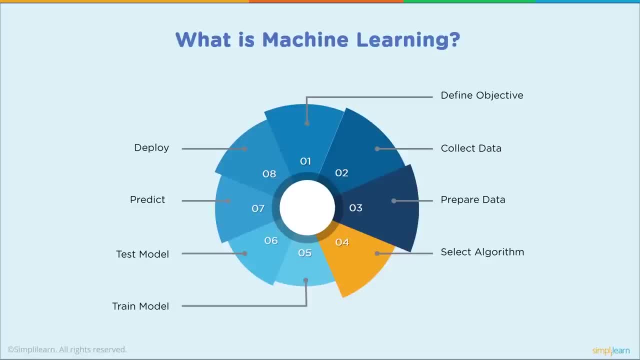 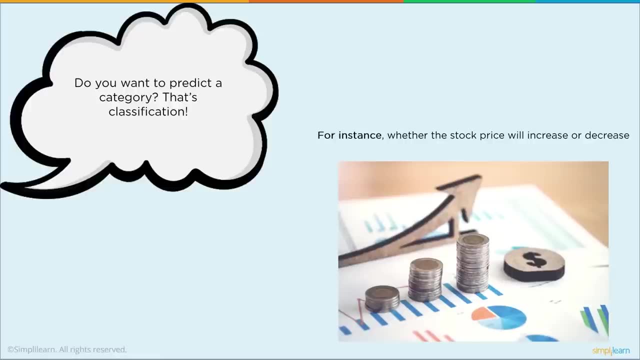 that become part of this model. This is a very general model, but it's a very good model to start with And we do have some basic divisions of what machine learning does. that's important to know. For instance, do you want to predict a category? 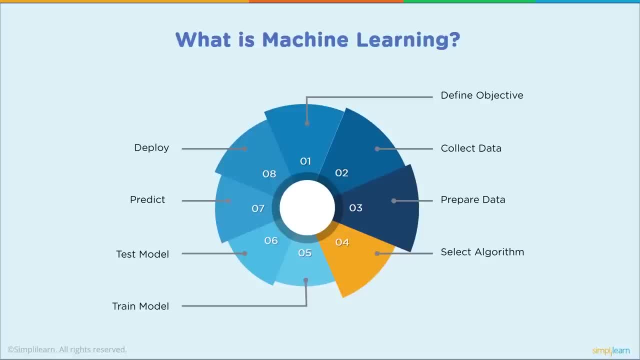 vector machine, Then you have to test the model. Does this model work? Is this a valid model for what we're doing? And then, once you've tested it, you want to run your prediction. You want to run your prediction or your choice, or whatever output is going to come up with. And then, once everything 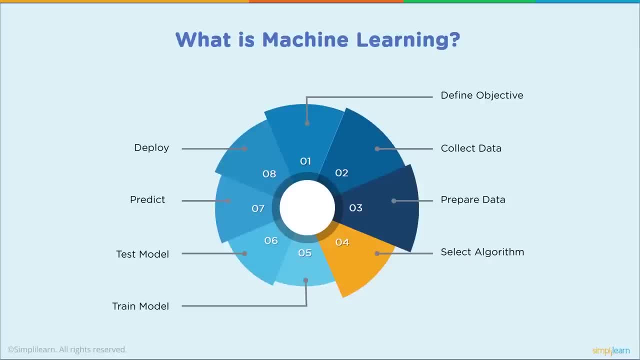 is set and you've done lots of testing, then you want to go ahead and deploy the model. Remember I said domain specific. This is very general as far as the scope of doing something. A lot of models. you get halfway through and you realize that your data is missing something and you have to go. 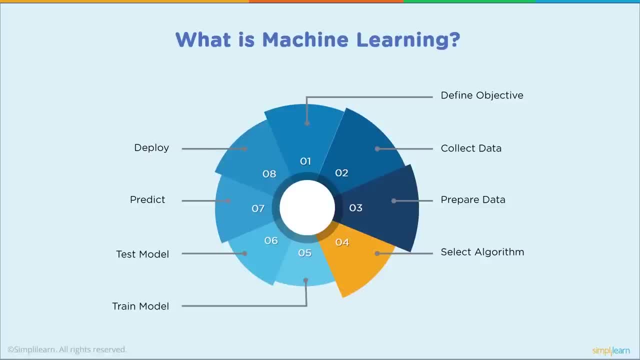 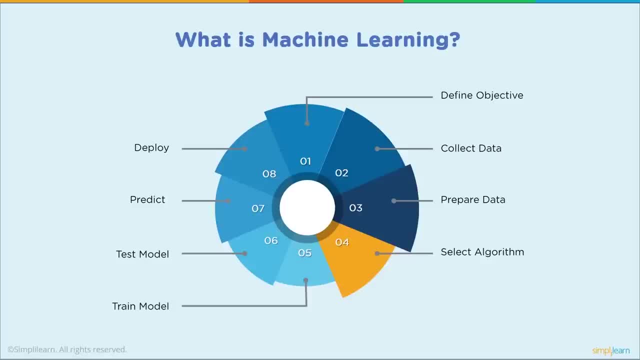 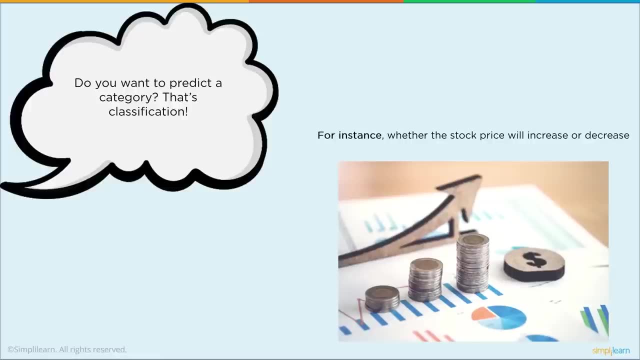 become part of this model. This is a very general model, but it's a very good model to start with And we do have some basic divisions of what machine learning does. that's important to know. For instance, do you want to predict a category? Well, if you're categorizing thing, that's. 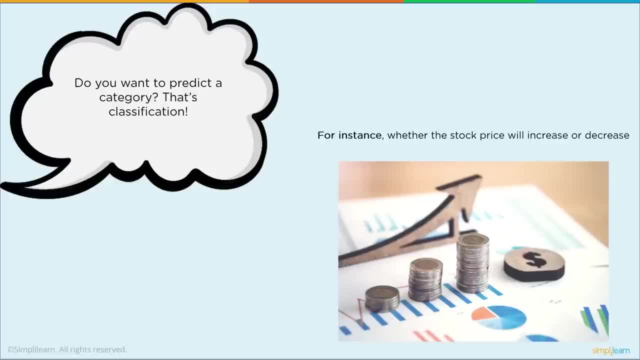 classification, For instance whether the stock price will increase or decrease. So in other words, I'm looking for a yes, no answer: Is it going up Or is it going down? And in that case we'd actually say: is it going up, True? If it's not, 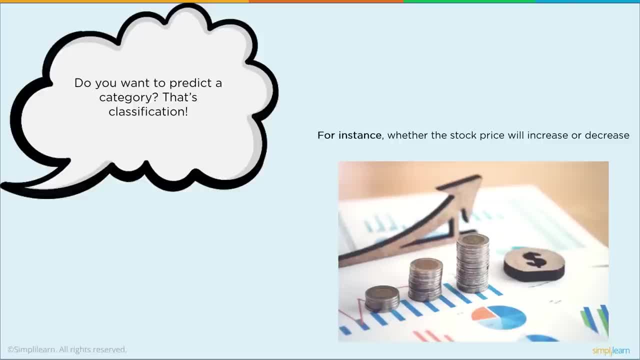 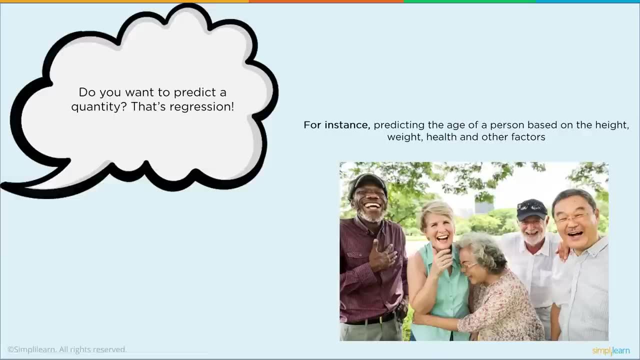 going up. it's false Meaning. it's going down. This way it's a yes, no, Zero one. Do you want to predict a quantity? That's regression. So remember, we just did classification, Now we're looking at regression. These are the two major divisions in what data is doing. For instance, 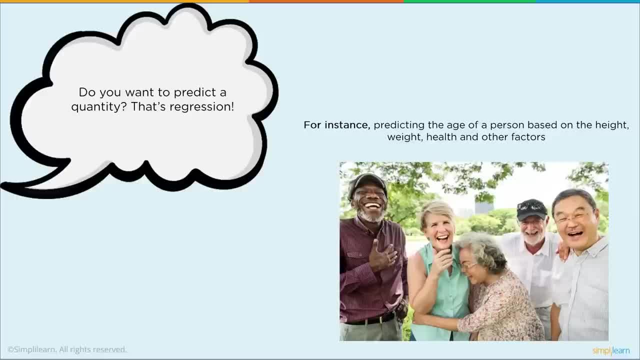 predicting the age of a person based on the height, weight, health and other factors. So, based on these different factors, you might guess how old a person is. And then there are a lot of domain, specific things Like: do you want to detect an anomaly? That's anomaly detection, This is. 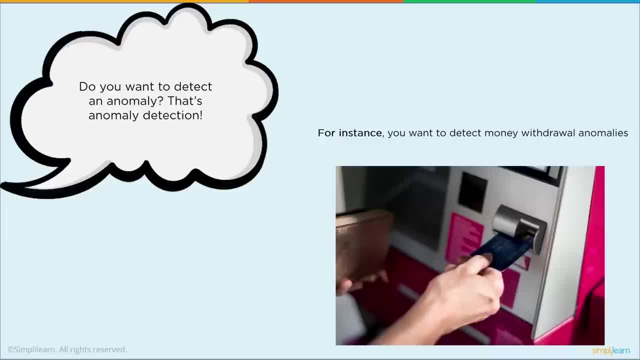 actually very popular right now. For instance, you want to detect money withdrawal anomalies. You want to know when someone's making a withdrawal that might not be their own account. We've actually brought this up because this is really big right now. If you're predicting the stock, whether to 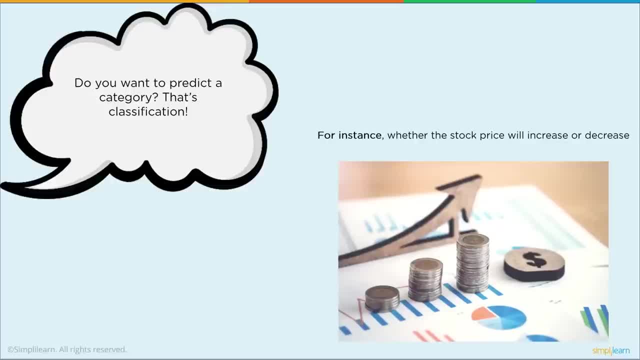 Well, if you're categorizing, that's classification, For instance, whether the stock price will increase or decrease. So, in other words, I'm looking for a yes-no answer: Is it going up or is it going down? And in that case we'd actually say: 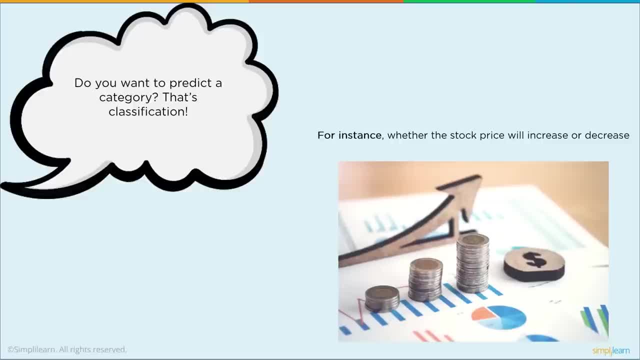 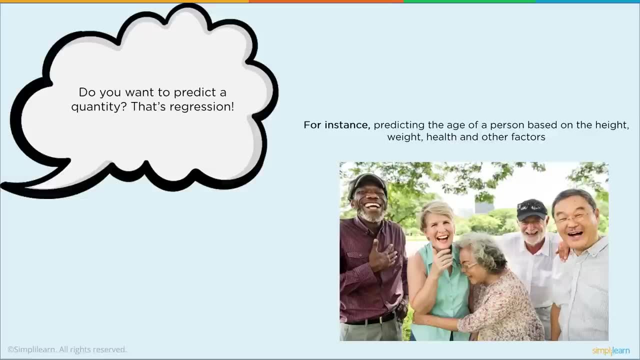 is it going up? True? If it's not going up, it's false, meaning it's going down. This way, it's a yes-no 0-1.. Do you want to predict a quantity? That's regression. So remember, we just did classification. 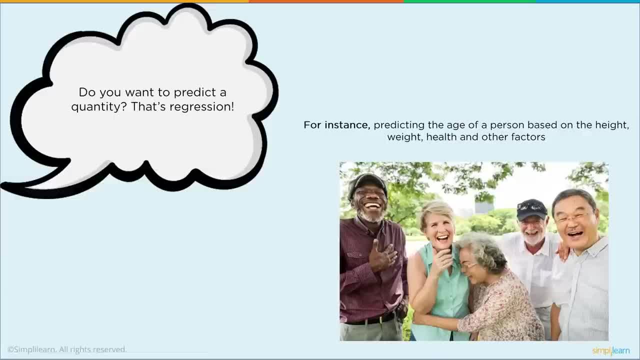 Now we're looking at regression. These are the two major divisions in what data is doing, For instance, predicting the age of a person based on the height, weight, health and other factors. So, based on these different factors, you might guess how old a person is. 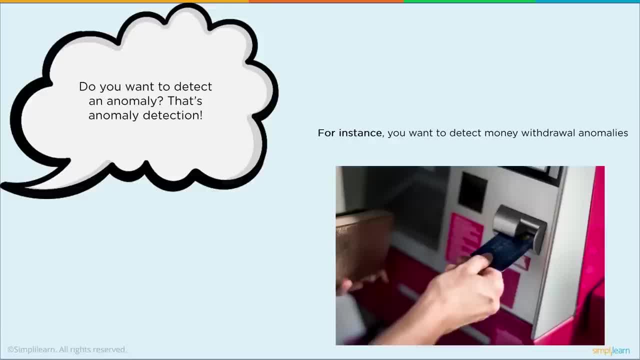 And then there are a lot of domain-specific things like: do you want to detect an anomaly? That's anomaly detection. This is actually very popular right now. For instance, you want to detect money withdrawal anomalies. You want to know when someone's making a withdrawal. 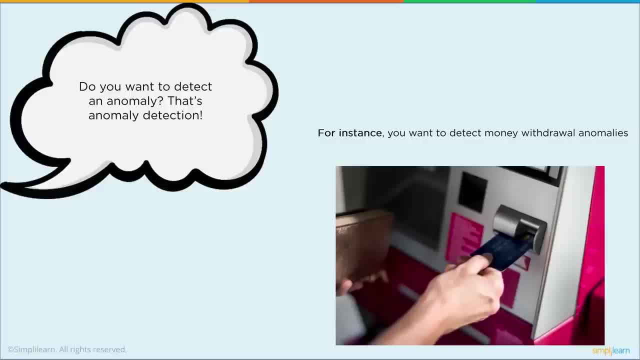 that might not be their own account. We've actually brought this up because this is really big right now. If you're predicting the stock- whether to buy stock or not- you want to be able to know if what's going on in the stock market is an anomaly. 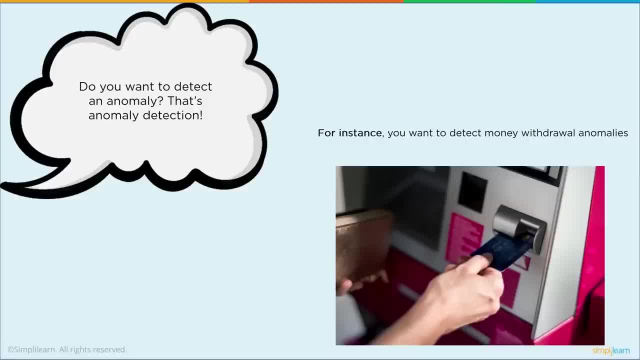 It's a different prediction model because something else is going on. You've got to pull out new information in there. Or is this just the norm? I'm going to get my normal return on my money invested, So being able to detect anomalies is very big in data science these days. 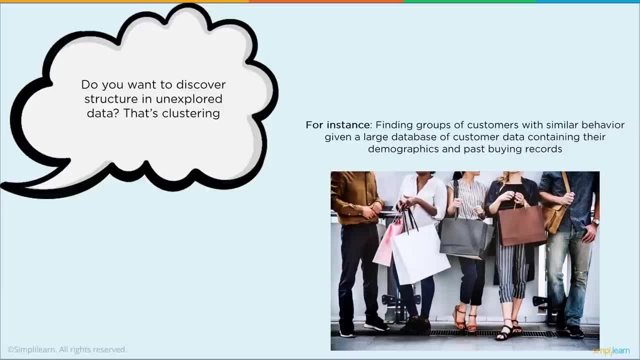 Another question that comes up, which is what we call untrained data, is: do you want to discover structure in unexplored data, And that's called clustering, For instance, finding groups of customers with similar behavior, given a large database of customer data? 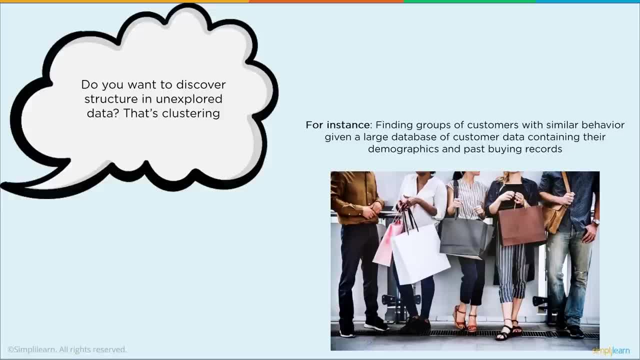 containing their demographics and past buying records. And in this case we might notice that anybody who's wearing a certain set of shoes goes shopping at certain stores, or whatever it is They're going to make certain purchases. By having that information, it helps us to market. 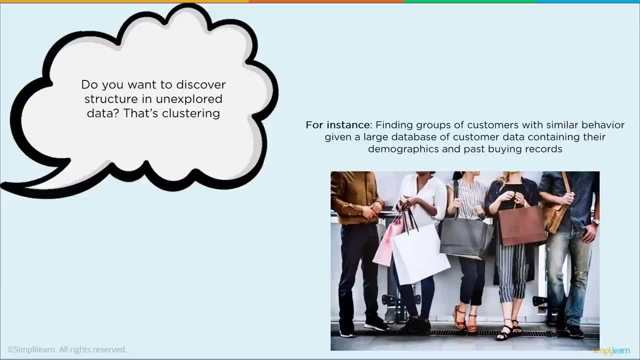 or group people together so that we can now explore that group and find out what it is we want to market to them. if you're in the marketing world- And that might also work in just about any arena- You might want to group people together. 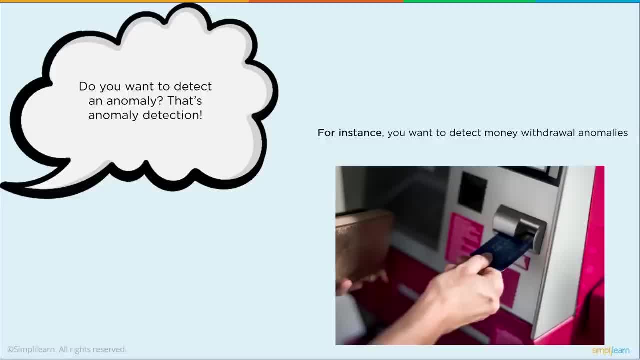 buy stock or not. You want to be able to know if what's going on in the stock market is an anomaly. Use a different prediction model because something else is going on. You got to pull out new information in there, Or is this just the way it is? You want to know what's going on in the 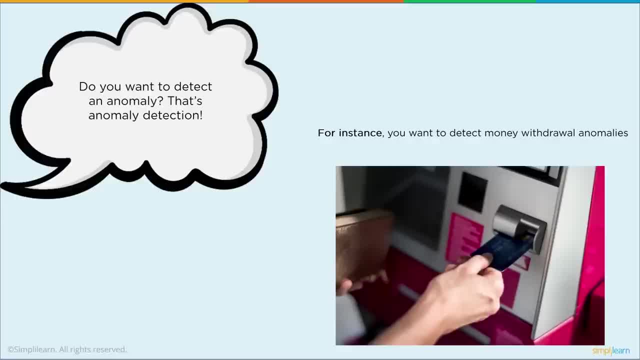 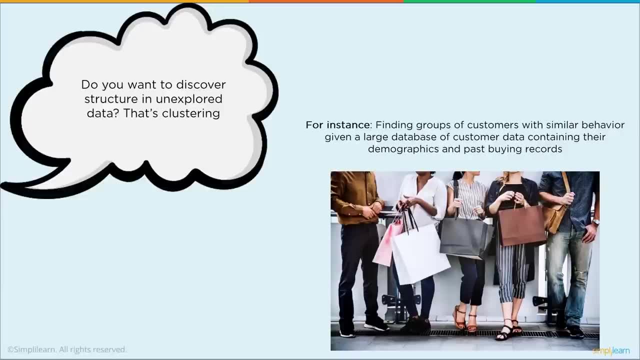 norm, I'm going to get my normal return on my money invested, So being able to detect anomalies is very big in data science these days. Another question that comes up, which is what we call untrained data, is: do you want to discover structure in unexplored data? And that's called. 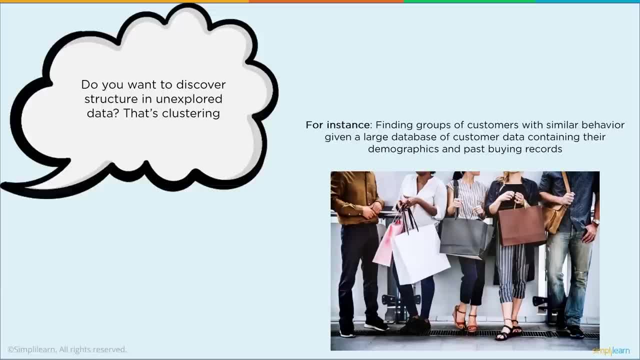 clustering, For instance, finding groups of customers with similar behavior, given a large database of customer data containing their demographics and past buying records. And in this case we might notice that in the past we've had a lot of customers that have been wearing certain sets of shoes, go shopping at certain stores Or whatever it is They're going. 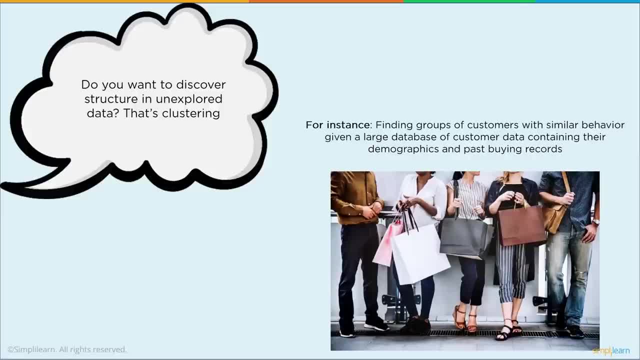 to make certain purchases By having that information. it helps us to market or group people together so that we can now explore that group and find out what it is we want to market to them. if you're in the marketing world- And that might also work in just about any arena- 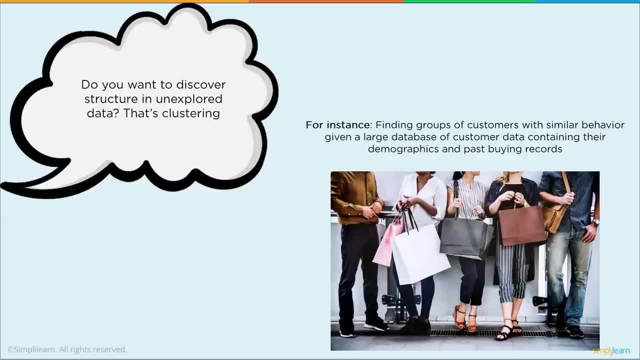 You might want to group people together, whether they're based on their different areas and investments and financial background, Whether you're going to give them a loan or not, before you even start looking at whether they're a valid customer for the bank you might want to look at. 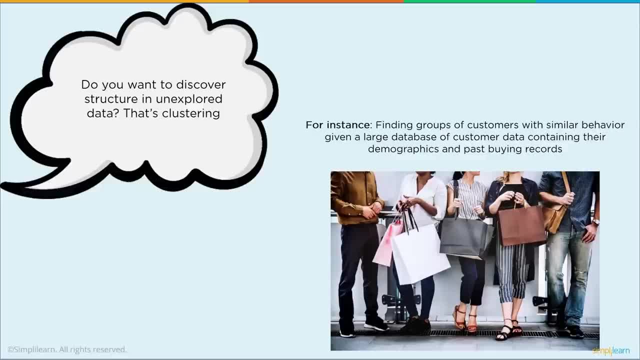 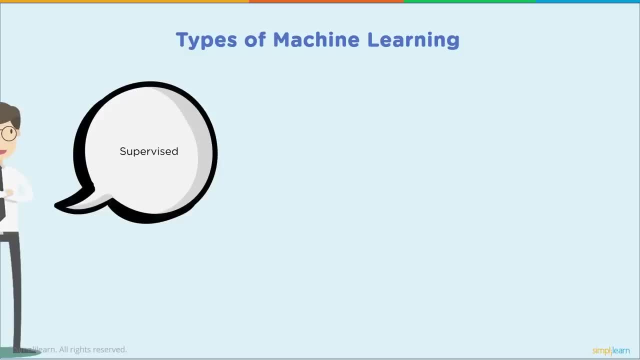 all these different areas and group them together, based on unknown data. So you're not, you don't know what the data is going to tell you, but you want to cluster people together that come together, And these last few bring us into the next topic, which is another way of dividing our types of 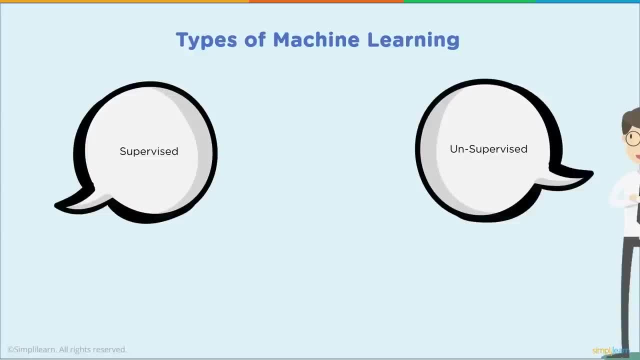 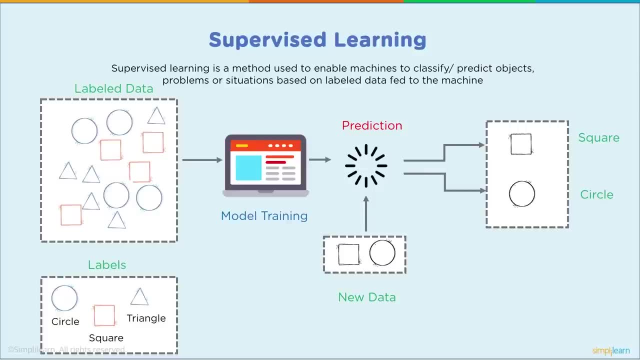 machine learning, and that is with supervised, unsupervised and reinforcement learning. Supervised learning is a method used to enable machines to classify, predict objects, problems or situations based on labeled data fed to the machine. And in here you see, we have a jungle. 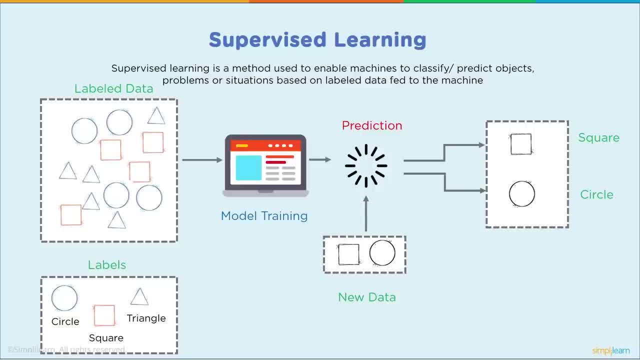 of data with circles, triangles and squares and we label them. We have what's a circle, what's a triangle, what's a square, and we have our model training and it trains it. so we know the answer. Very important when you're doing supervised learning: you already know the answer. 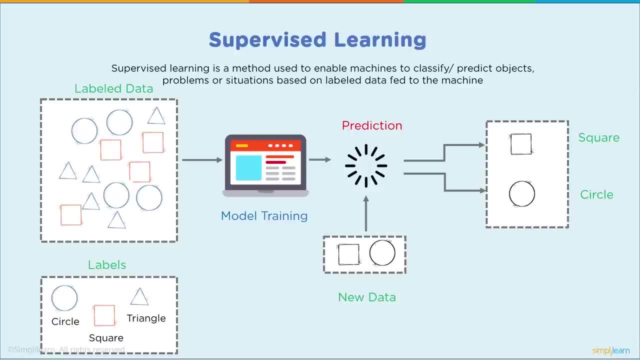 to a lot of your information coming in, So you have a huge group of data coming in and then you have a new data coming in. So we've trained our model. The model now knows the difference between a circle, a square, a triangle, and now that we've trained it, we can send in. 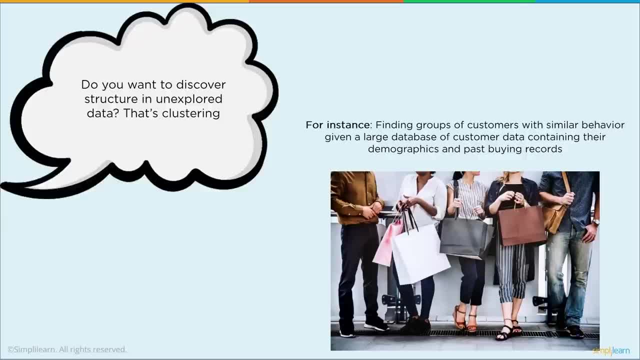 whether they're based on their different areas and investments and financial background, whether you're going to give them a loan or not. before you even start looking at whether they're a valid customer for the bank, You might want to look at all these different areas. 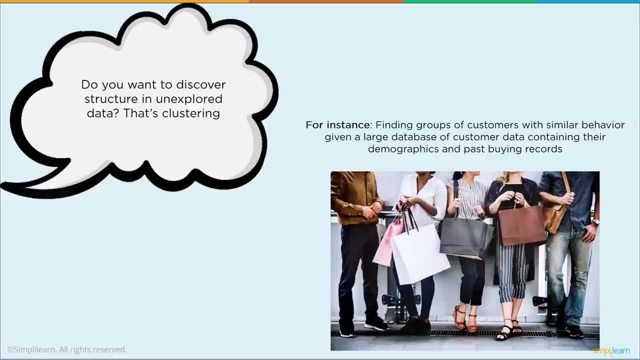 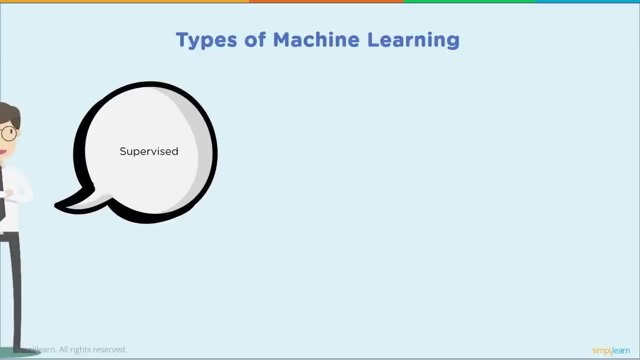 and group them together based on unknown data, So you don't know what the data is going to tell you. but you want to cluster people together that come together. And these last few bring us into the next topic, which is another way of dividing our types of machine learning. 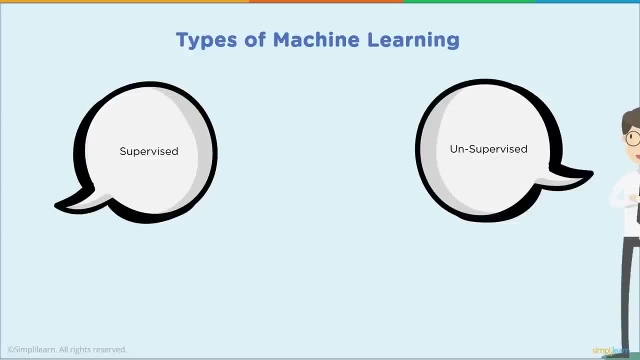 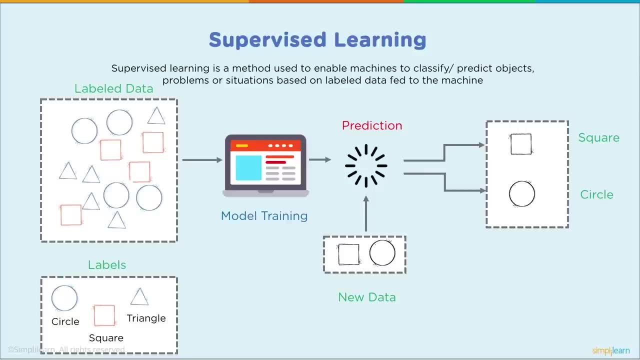 And that is with supervised, unsupervised, and supervised, supervised and reinforcement learning. Supervised learning is a method used to enable machines to classify, predict objects, problems or situations based on labeled data fed to the machine. And in here you see, we have a jumble of data with circles, triangles and squares, and we label them. We have 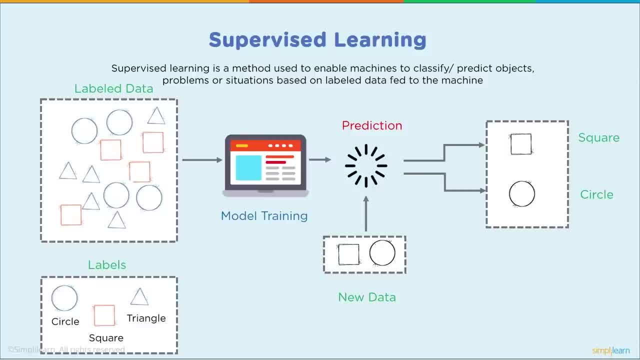 what's a circle, what's a triangle, what's a square? and we have our model training and it trains it, so we know the answer. Very important when you're doing supervised learning. you already know the answer to a lot of your information coming in. So you have a huge group of data coming in and then 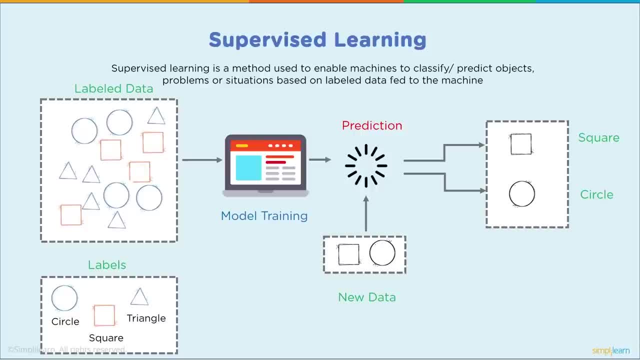 you have new data coming in, So we've trained our model. The model now knows the difference between a circle, a square, a triangle, and now that we've trained it, we can send in. in this case, a square and a circle goes in and it predicts that the top one's a square and the next one's a circle, And you 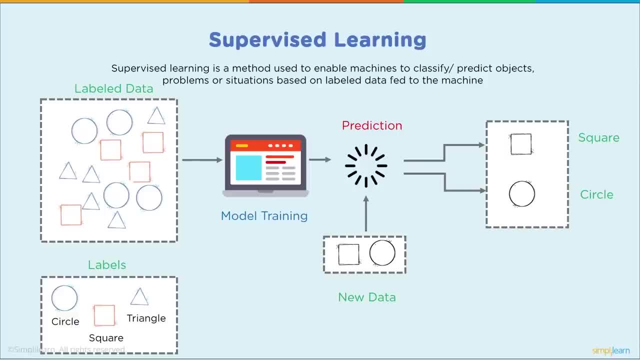 can see that this is being able to predict whether someone's going to default on a loan, because I was talking about banks earlier, Supervised learning on stock market. whether you're going to make money or not, that's always important And if you are looking to make a fortune in the stock, 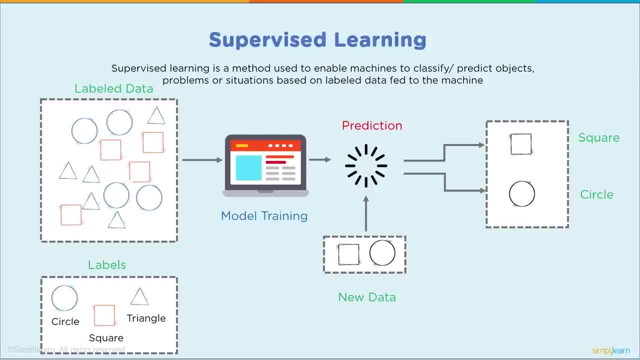 market keep in mind. it is very difficult to get all the data correct on the stock market. It is very. it fluctuates in ways you really hard to predict, So it's quite a roller coaster ride. if you're running machine learning on the stock market, You start realizing you really have to. 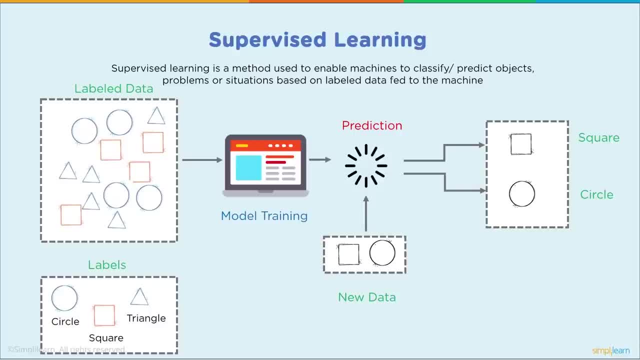 dig for new data. So we have supervised learning, and if you have supervised, we should need unsupervised learning. In unsupervised learning, machine learning model finds the hidden pattern in an unlabeled data. So in this case, instead of telling it what the circle is, 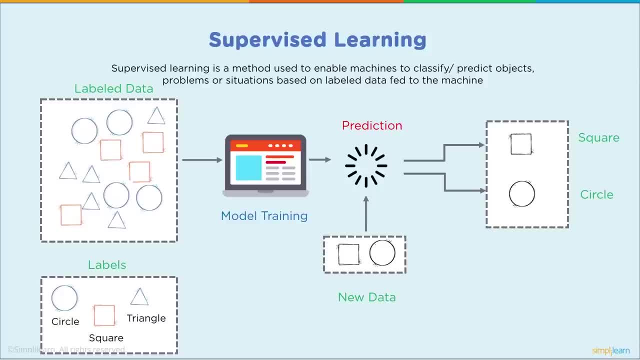 in this case, a square and a circle goes in and it predicts that the top one's a square and the next one's a circle, And you can see that this is being able to predict whether someone's going to default on a loan, because I was talking about banks earlier. Supervised learning on stock. 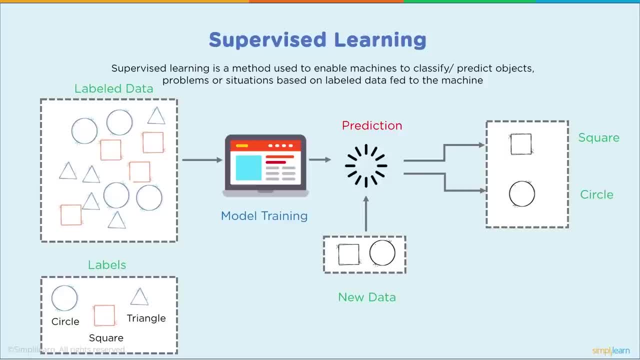 market. whether you're going to make money or not, that's always important And if you are looking to make a fortune in the stock market, keep that in mind. It is very difficult to get all the data correct on the stock market. It is very it fluctuates in. 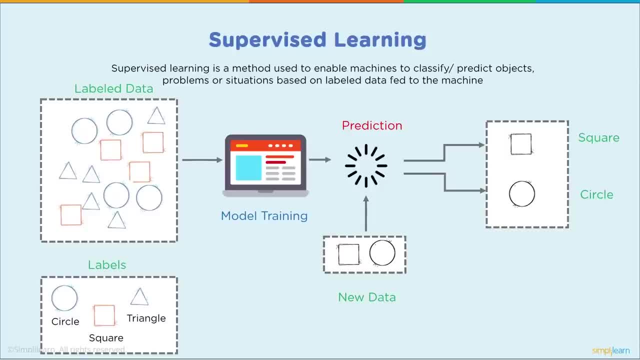 ways really hard to predict. So it's quite a roller coaster ride. If you're running machine learning on the stock market, you start realizing you really have to dig for new data. So we have supervised learning, and if you have supervised, we should need unsupervised learning In. 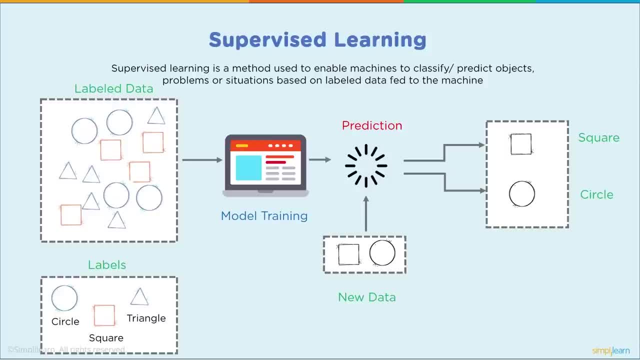 unsupervised learning. machine learning model finds the hidden pattern in an unlabeled data. So in this case, instead of telling it what the circle is and what a triangle is and what a square is, it goes in there, looks at them and says: 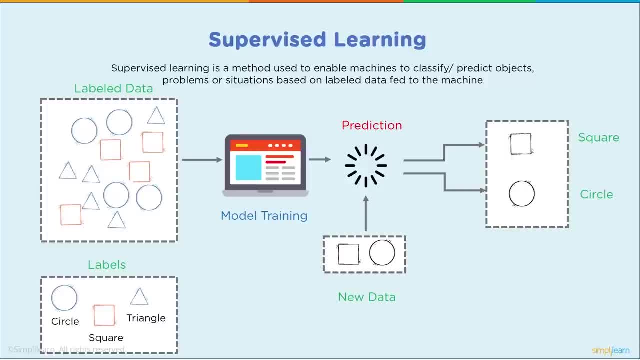 for whatever reason it groups them together. Maybe it'll group it by the number of corners And it notices that a number of them all have three corners, a number of them all have four corners and a number of them all have no corners, And it's able to filter those through and group them together. 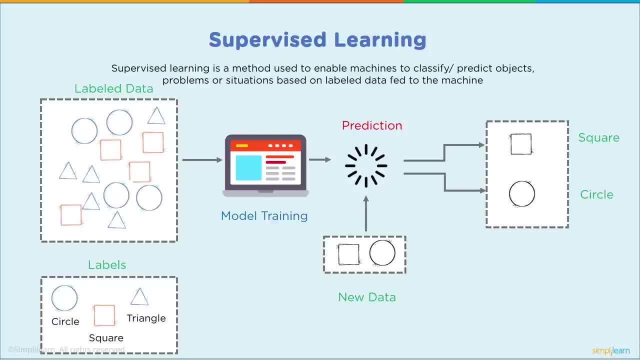 We talked about that earlier- with looking at a group of people who are out shopping. We want to group them together to find out what they have in common. And, of course, once you understand what people have in common, maybe you have one of the most important things in the stock market and you want to. 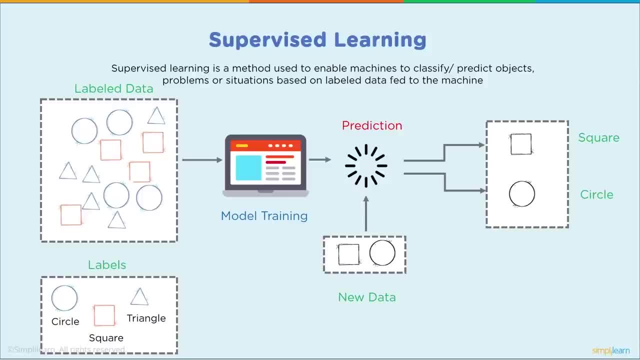 know who's a customer at your store, or you have five of them are customers at your store and they have a lot in common with five others who are not customers at your store. how do you market to those five who aren't customers at your store yet They fit the demographics of who's going to shop there? 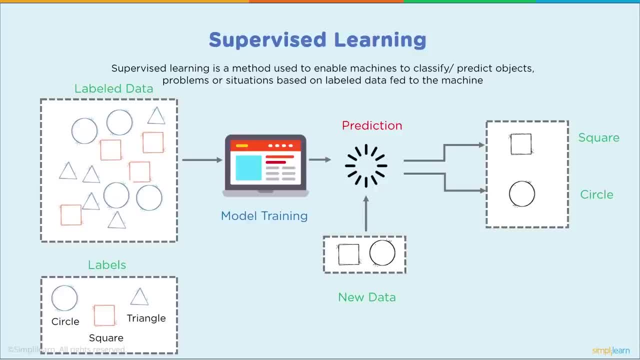 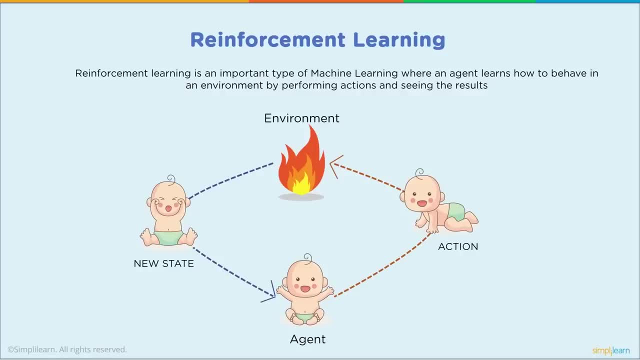 and you'd like them to shop at your store, not the one next door. Of course, this is a simplified version. You can see very easily the difference between a triangle and a circle, which might not be so easy in marketing. Reinforcement learning. Reinforcement learning is an important type of 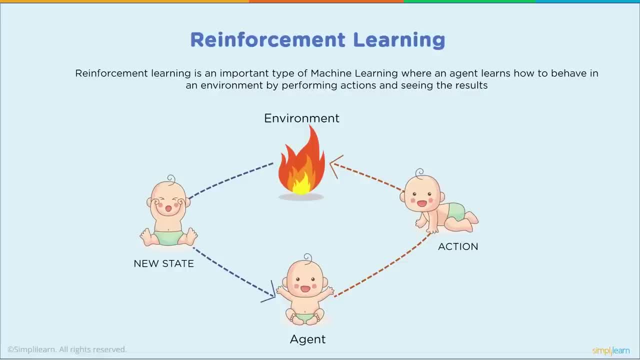 machine learning, where an agent learns how to behave in an environment by performing actions and seeing the result. We have here, in this case, a baby. It's actually great that they used an infant for this slide, because the reinforcement learning is very much in its 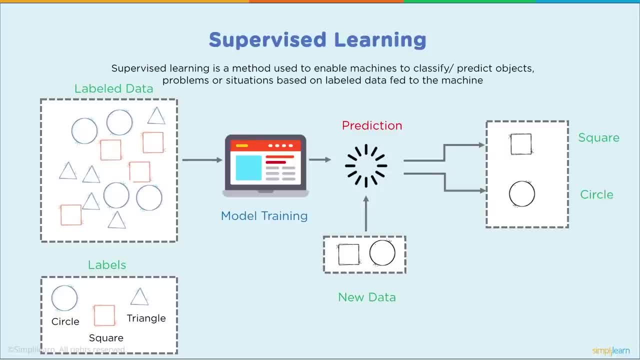 and what a triangle is and what a square is. it goes in there, looks at them and says, for whatever reason it groups them together. Maybe it'll group it by the number of corners And it notices that a number of them all have three corners, a number of them all have four corners and a number of them. 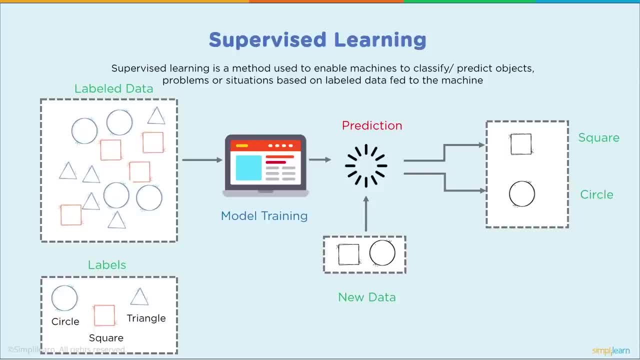 all have no corners And it's able to filter those through and group them together. We talked about that earlier, with looking at a group of people who are out shopping. We want to group them together so that they have in common And, of course, once you understand what people have in common, maybe 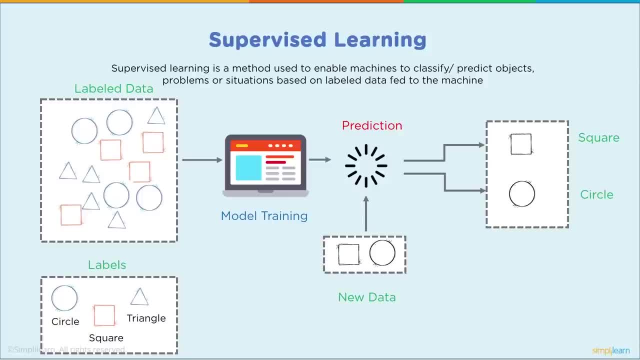 you have one of them who's a customer at your store, or you have five of them who are a customer at your store and they have a lot in common with five others who are not customers at your store. how do you market to those five who aren't customers at your store yet They fit the demographics of who's? 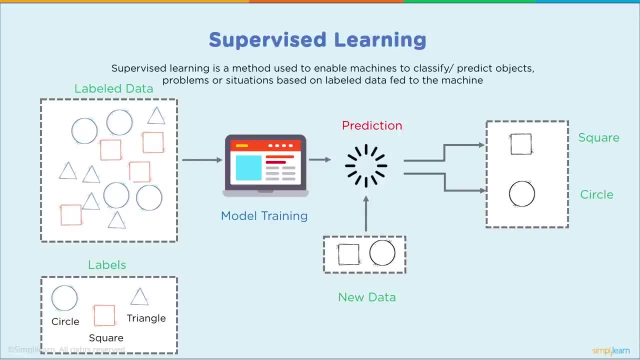 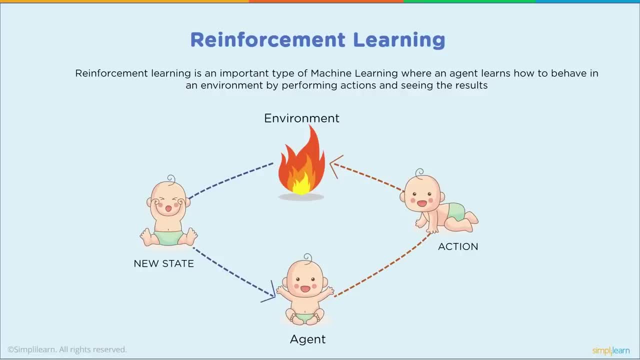 going to shop there and you'd like them to shop at your store, not the one next door. Of course, this is a simplified version. You can see very easily the difference between a triangle and a circle, which might not be so easy in marketing. Reinforcement learning. Reinforcement learning. 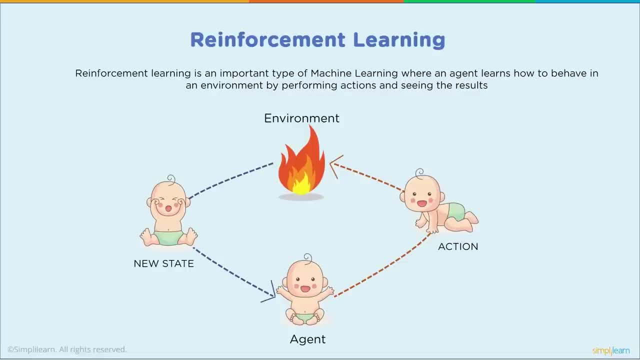 is an important type of machine learning where an agent learns how to behave in an environment by performing actions and seeing the result. We have here, in this case, a baby. It's actually great that they used an infant for this slide, because the reinforcement learning is very much in its 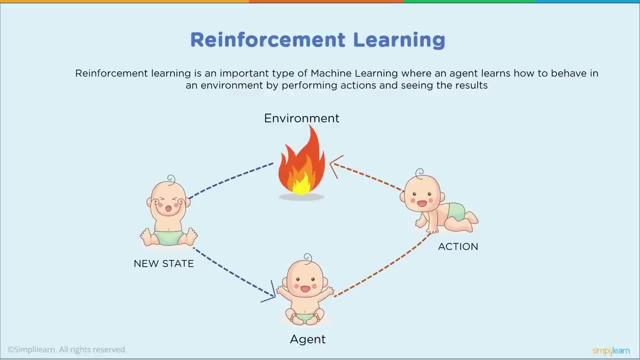 infant stages. But it's also probably the biggest machine learning demand out there right now or in the future it's going to be coming up over the next few years- is reinforcement learning and how to make that work for us. And you can see here where we have our action. I mean the action in 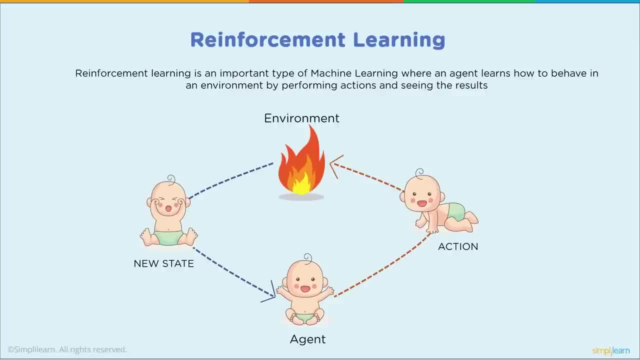 this one. it goes into the fire. Hopefully the baby didn't. it was just a little candle, not a giant fire pit like it looks like here. When the baby comes out and the new state is, the baby is sad and crying because they got burned on the fire And then maybe they take another action- The baby's 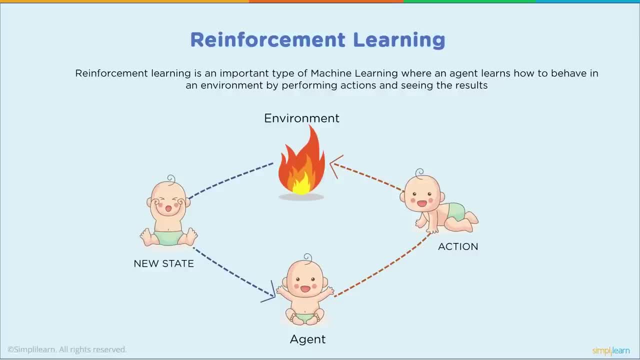 called the agent because it's the one taking the actions. And in this case they didn't go into the fire, They went a different direction and now the baby's happy and laughing and playing. Reinforcement learning is one of the ways we learn. We learn whether it is you know you burn yourself on the. 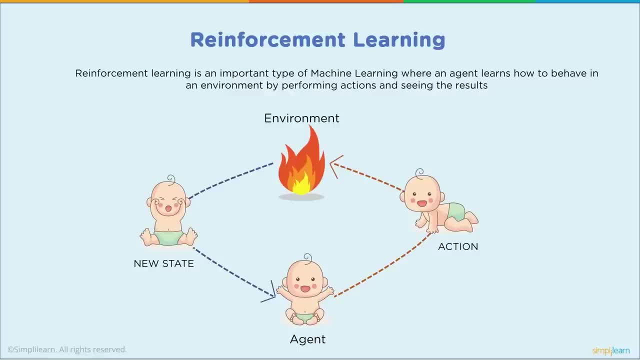 infant stages. but it's also probably the biggest machine learning demand out there right now or in the future It's going to be coming up over the next few years- is reinforcement learning and how to make that work for us, And you can see here where we have our action In the action in this. 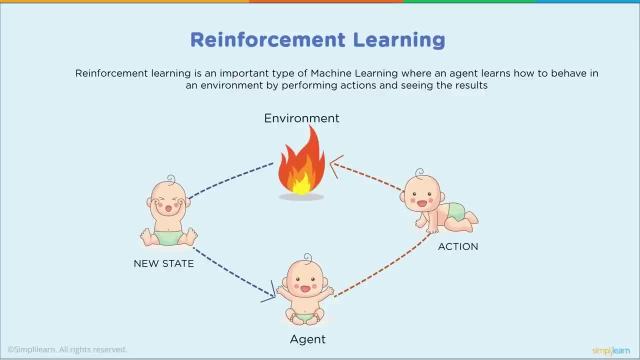 one, it goes into the fire. Hopefully the baby didn't. It was just a little candle, Not a giant fire pit like it looks like here. When the baby comes out and the new state is, the baby is sad and crying because they got burned on the fire And then maybe they take another action. The baby is 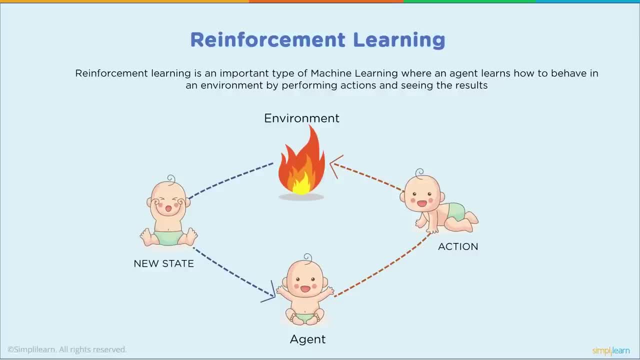 called the agent because it's the one taking the actions. And in this case they didn't go into the fire, They went a different direction and now the baby's happy and laughing and playing. Reinforcement learning is very easy to understand because that's how, as humans, that's one of the ways we learn. We 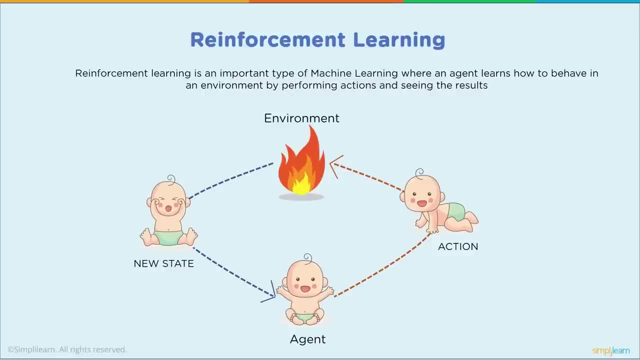 learn, whether it is you burn yourself on the stove. Don't do that anymore, Don't touch the stove. In the picture, being able to have a machine learning program or an AI be able to do this is huge, because now we're starting to learn how to learn. That's a big jump in the world of computer and machine. 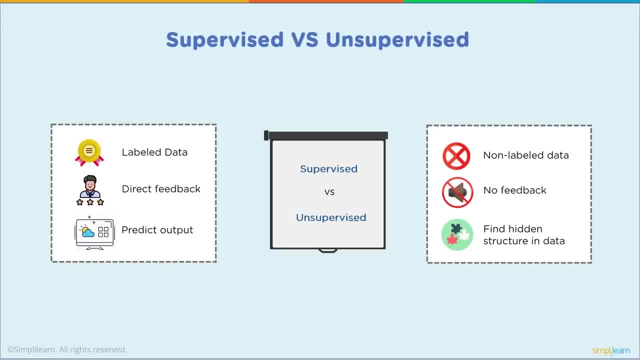 learning And we're going to go back and just kind of go back over supervised versus unsupervised learning. Understanding this is huge because this is going to come up in any project you're working on. We have in supervised learning, we have labeled data, We have direct feedback. So someone's 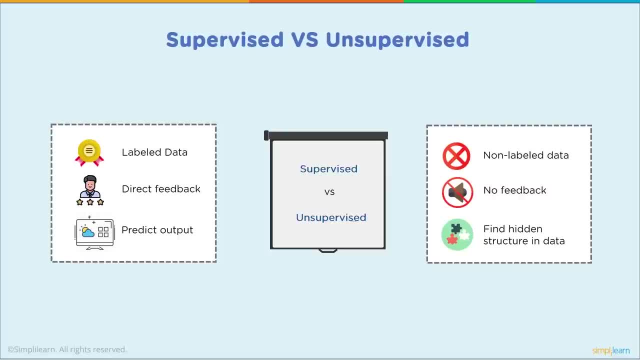 already gone in there and said, Yes, that's a triangle, No, that's not a triangle. And then you predict an outcome. So you have a nice prediction: This new set of data is coming in and we know what it's going to be. And then, with 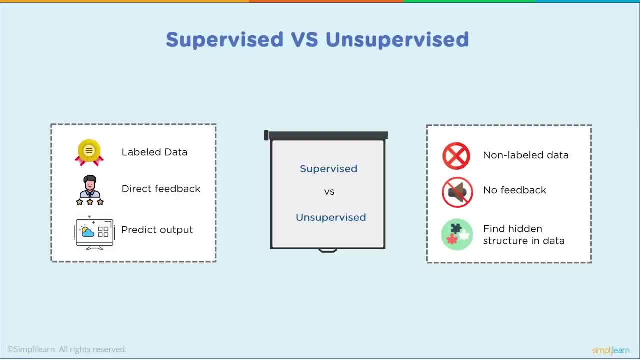 unsupervised training. it's not labeled, So we really don't know what it is. There's no feedback, So we're not telling it whether it's right or wrong. We're not telling it whether it's a triangle or a square. We're not telling it to go left or right. All we do is we're finding hidden structure. 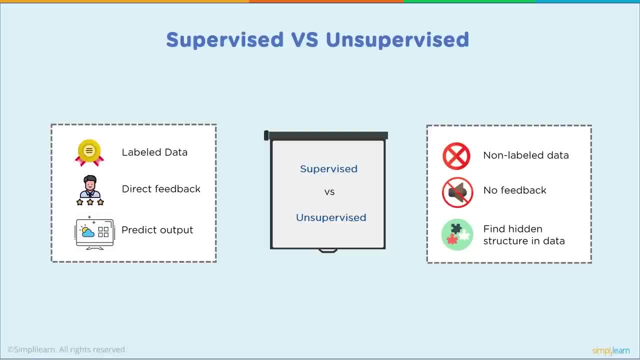 in the data, grouping the data together to find out what connects to each other, And then you can use these together. So imagine you have an image and you're not sure what you're looking for. So you go in and you have the unstructured data. Find all these things that. 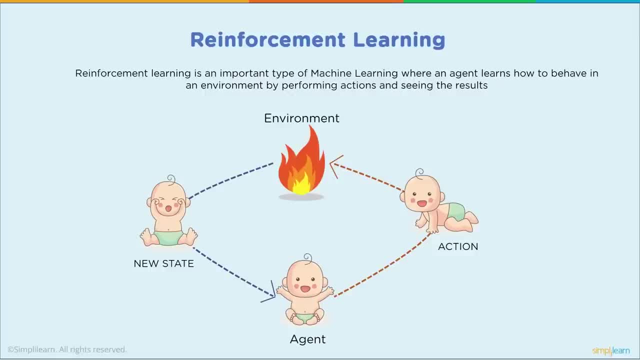 stove. don't do that anymore. Don't touch the stove. In the big picture, being able to have machine learning, programming or an AI be able to do this is huge because now we're starting to learn how to learn. That's a big jump in the world of computer and machine learning And we're going. 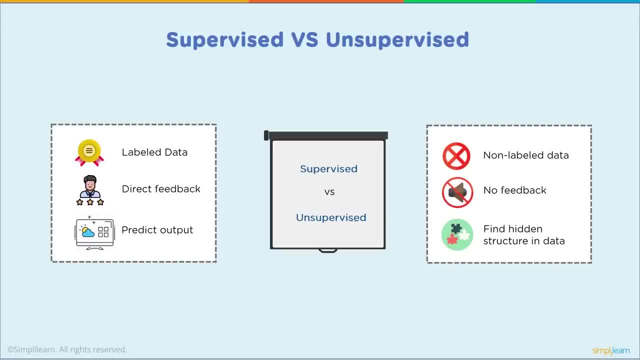 to go back and just kind of go back over supervised versus unsupervised learning, Understanding this is huge because this is going to come up in any future- And we're going to go back and just kind of go through every project you're working on We have in supervised learning, we have labeled 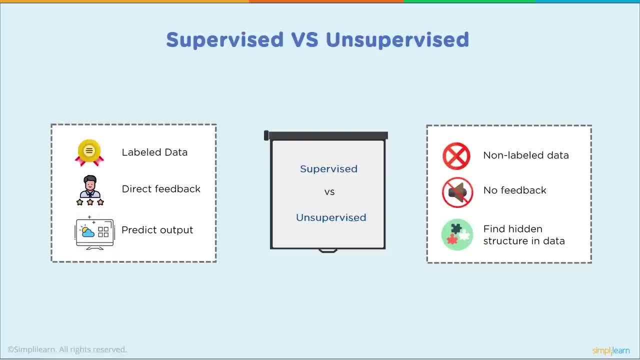 data. We have direct feedback. So someone's already gone in there and said, yes, that's a triangle, No, that's not a triangle. And then you predicted outcome. You have a nice prediction: This new set of data is coming in, and we know it is going to be, And then, with unsupervised training, it's not. 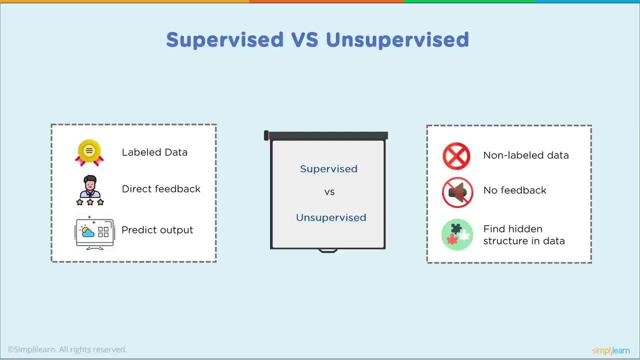 labeled, so we really don't know what it is. There's no feedback, So we're not telling it whether it's right or wrong. We're not telling it whether it's a triangle or a square. We're not telling it that it's a triangle or a square. So we're really going to go back and look at the data that's going. 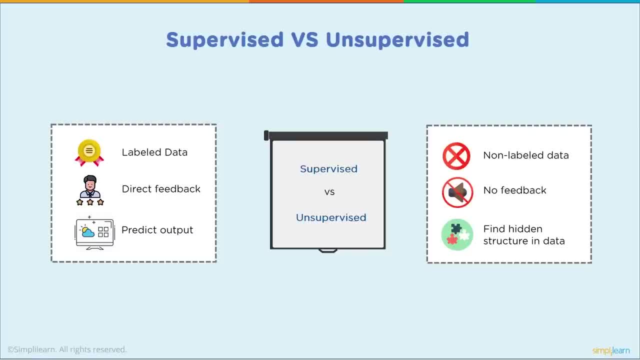 to have a positive effect and we're going to go back and just kind of go back and use it and we're telling it to go left or right. all we do is we're finding hidden structure in the data, grouping the data together to find out what connects to each other, and then 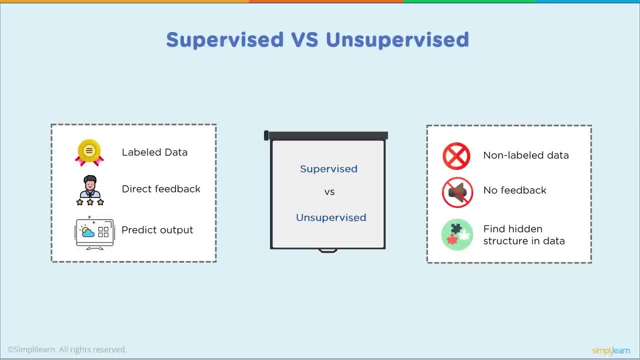 you can use these together. so imagine you have an image and you're not sure what you're looking for. so you go in and you have the unstructured data, find all these things that are connected together, and then somebody looks at those and labels them. now you can take that label data and program something to predict. 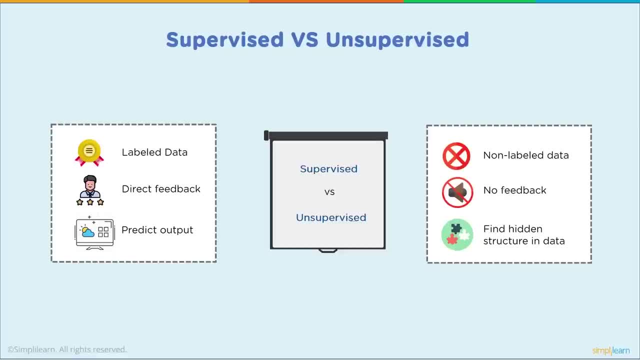 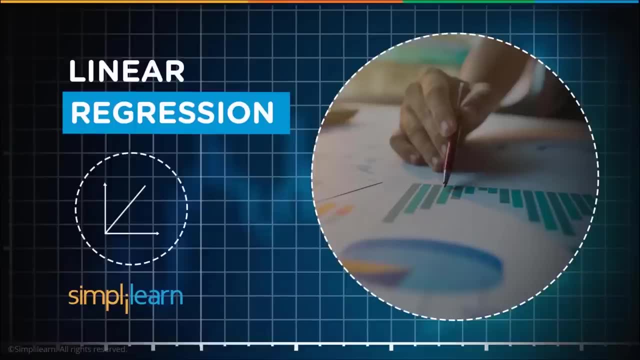 what's in the picture so you can see how they go back and forth and you can start connecting all these different tools together to make a bigger picture. let's look at an example of a common use for linear regression profit estimation of a company. if I was going to invest in a company, I would like to know how much. 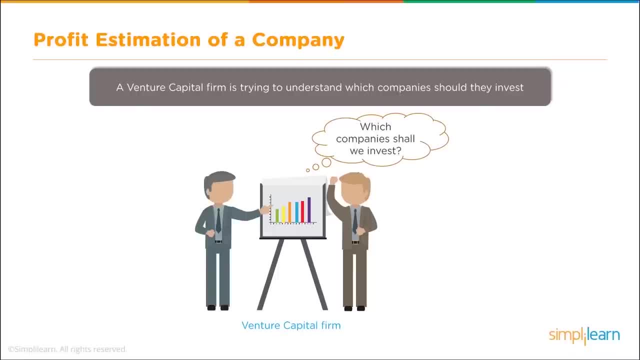 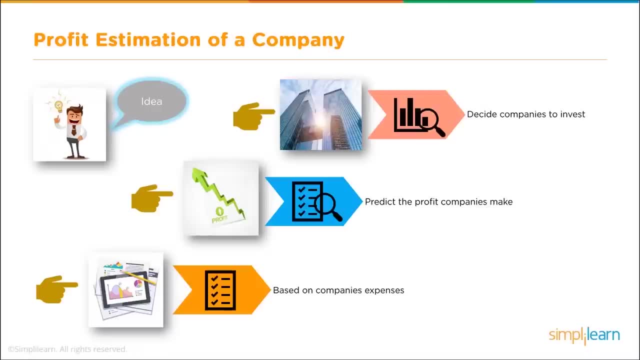 money I could expect to make. so we'll take a look at a venture capitalist firm and try to understand which companies they should invest in. so we'll take the idea that we need to decide the companies to invest in. we need to predict the profit the company makes and we're going to do it based on the company's expenses and 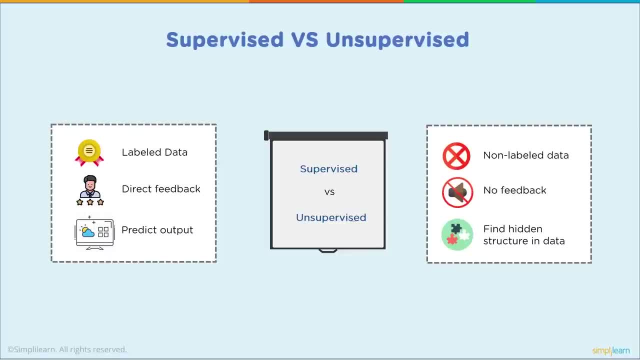 are connected together And then somebody looks at those and labels them. Now you can take that labeled data and program something to predict what's in the picture, So you can see how they go back and forth, and you can start connecting all these different tools together to make a 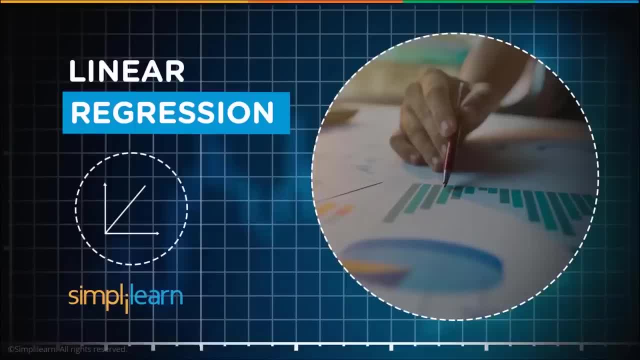 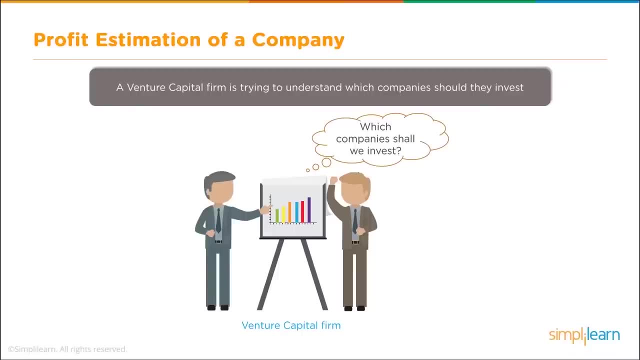 bigger picture. Let's look at an example of a common use for linear regression: Profit estimate, Estimation of a company. If I was going to invest in a company, I would like to know how much money I could expect to make. So we'll take a look at a venture capitalist firm and try to understand. 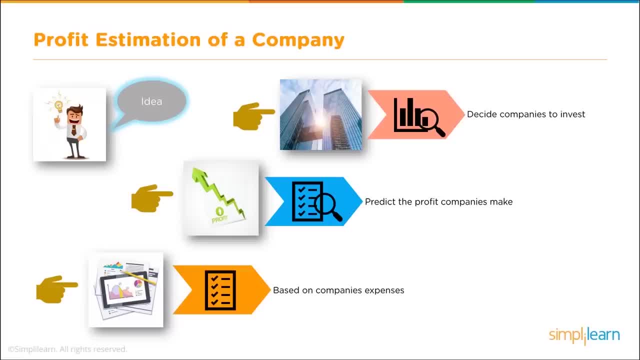 which companies they should invest in. So we'll take the idea that we need to decide the companies to invest in. We need to predict the profit the company makes, And we're going to do it based on the company's expenses, and even just a specific expense. In this case, we have our company. 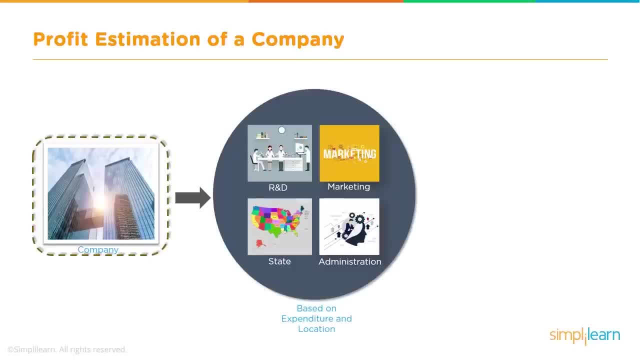 we have the different expenses. So we have our R&D, your research and development, We have our marketing, We might have the location, We might have what kind of administration is going through? Based on all this different information, we would like to calculate the profit. Now, in actuality, there's usually about 23 to 27 different markers. 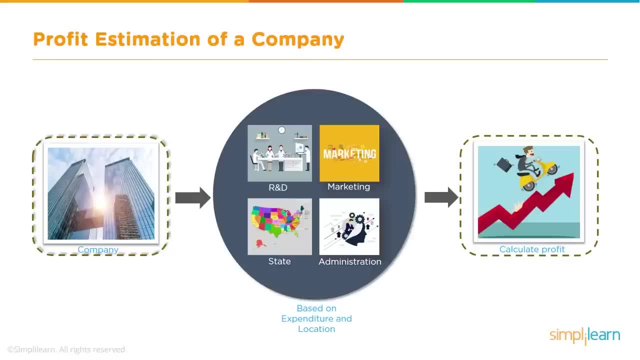 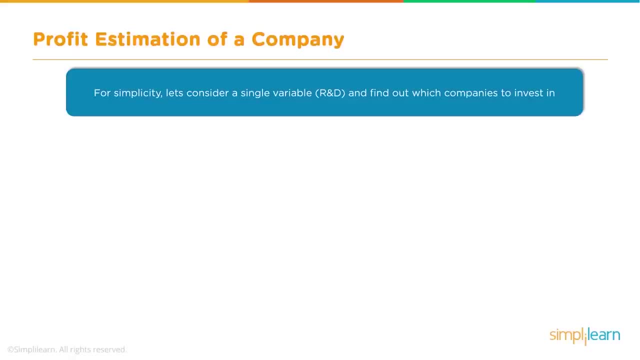 that they look at if they're a heavy duty investor. We're only going to take a look at one basic one. We're going to come in and, for simplicity, let's consider a single variable R&D and find out which companies to invest in based on that. So we take our R&D and we're. 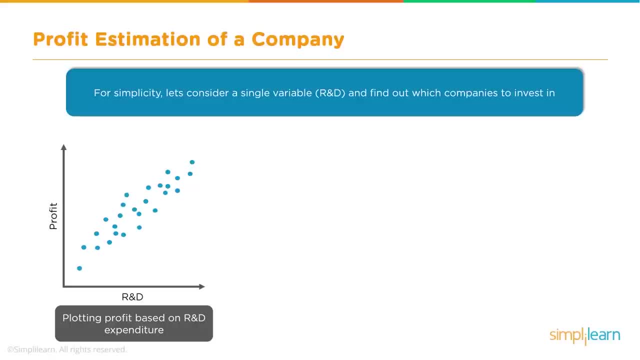 plotting the profit based on the R&D expenditure, how much money they put into the research and development, And then we look at the profit that goes with that. We can predict a line to estimate the profit. So we draw a line right through the data. When you look at that you can see how much. 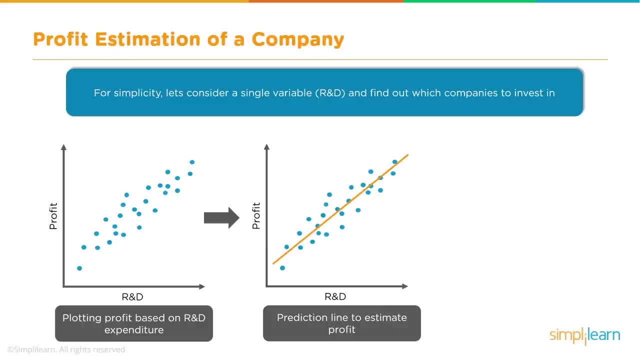 they invest in the R&D is a good marker as to how much profit they're going to have. We can also note that companies spending more on R&D make good profit, So let's invest in the ones that spend a higher rate in their R&D. Let's look at another example of machine learning Based on the amount. 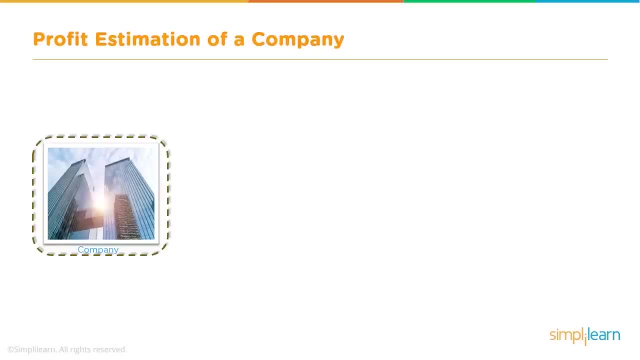 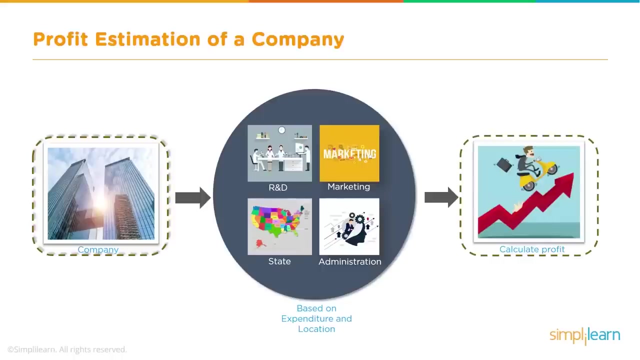 even just a specific expense. in this case, we have our company, we have the different expenses. so we have our R&D, which is your research and development. we have our marketing. we might have the location. we might have what kind of administration is going through? based on all this different information, we would 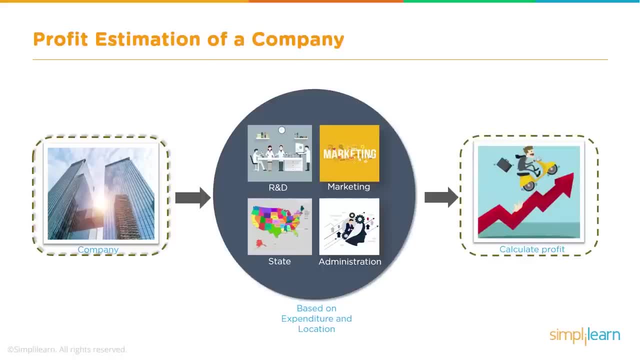 like to calculate the profit now. in actuality, there's usually about 23 to 27 different markers that they look at if they're a heavy-duty investor. we're only going to take a look at one basic one. we're going to come in and for 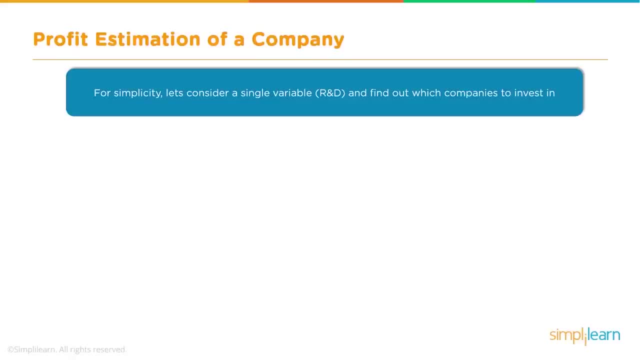 simplicity, let's consider a single variable R&D and find out which companies to invest in based on that. so we take our R&D, we're plotting the profit based on the R&D expenditure- how much money they put into the research and development- and then we look at the profit that goes with that. we can. 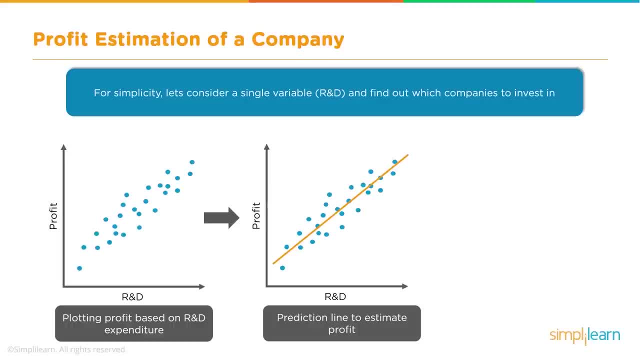 predict a line to estimate the profit, so we draw a line right through the data. when you look at that, you can see how much they invest in. the R&D is a good marker as to how much profit they're going to have. we also note that companies spending more on R&D make good profit, so let's 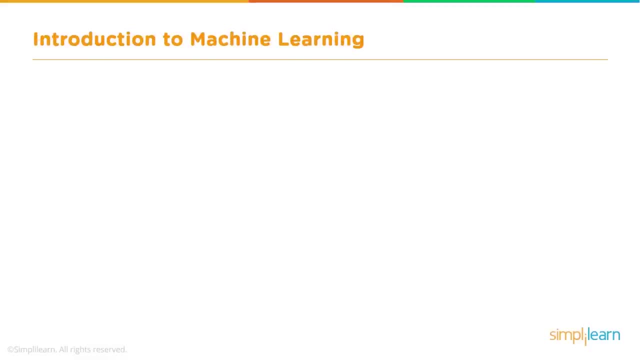 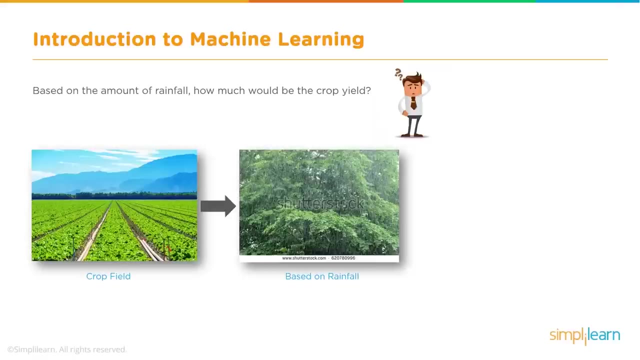 invest in the ones that spend a higher rate in their R&D. let's look at another example: machine learning based on the amount of rainfall. how much would be the crop yield? we here, we have our crops, we have a rainfall and we want to know how much we're going to get from our crops this year. so we're going to use two. 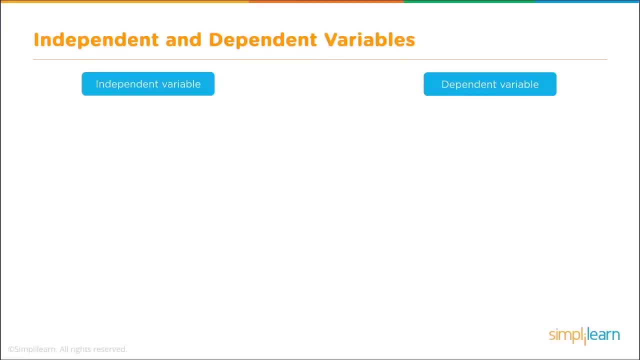 variables: independent and dependent. the independent variable is a variable whose value does not change by the effect of other variables and is used to manipulate the dependent variable. it is often denoted as X. in our example, rainfall is the independent variable. this is a wonderful example, because you can easily see that we can't. 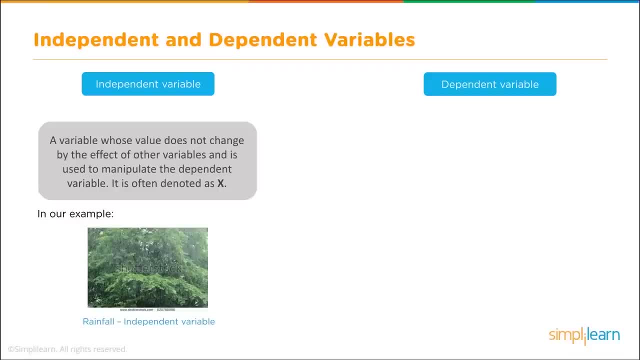 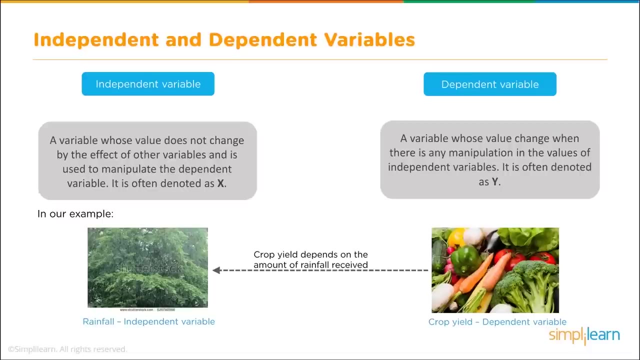 control the rain, but the rain does control the crop. so we talk about the independent variable controlling the dependent variable. let's define dependent variable as a variable whose value change when there is any manipulation- the values of the independent variables. it is often denoted as Y and you can see here our crop yield is dependent variable and it. 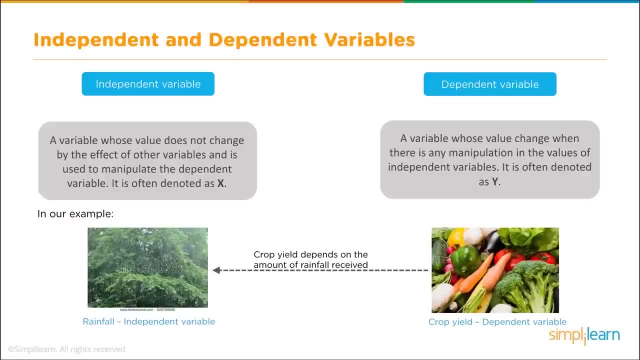 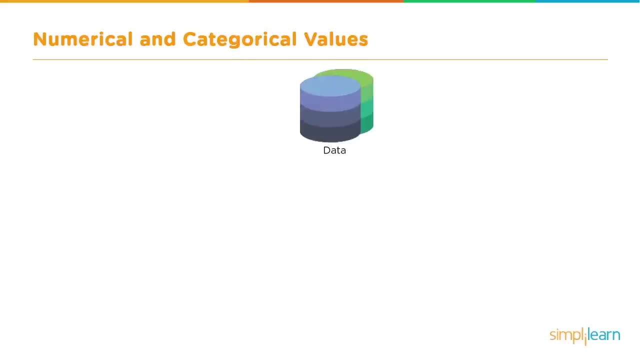 is dependent on the amount of rainfall received. now that we've taken a look at a real-life example, let's go a little bit into the theory and some definitions on machine learning and see how that fits together with linear regression, numerical and categorical values. let's take our data coming in. this is kind of random data from any kind of project we 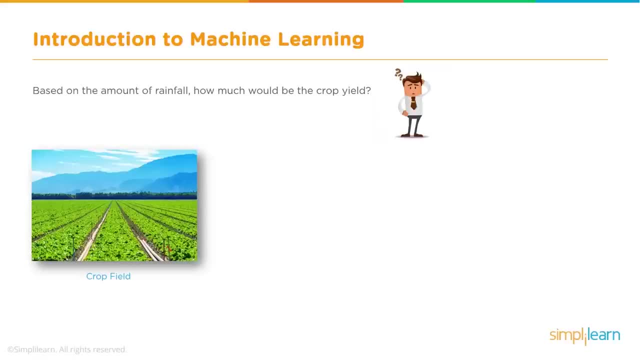 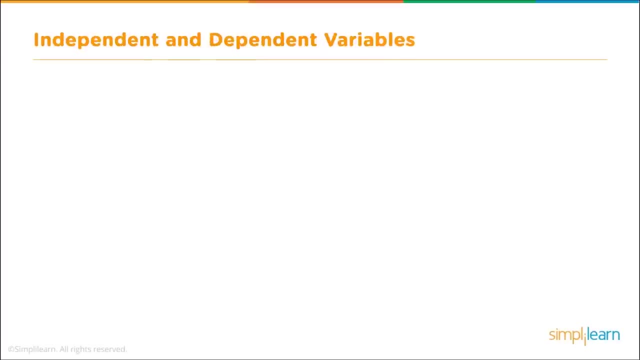 of rainfall, how much would be the crop yield? So here we have our crops, We have our rainfall And we want to know how much we're going to get from our crops this year. So we're going to use two variables: independent and dependent. The independent variable is a. 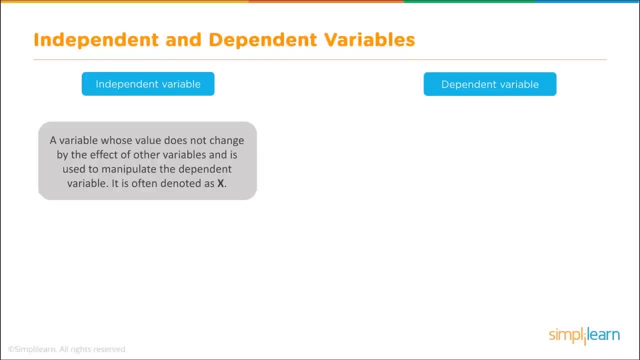 variable whose value does not change by the effect of other variables and is used to manipulate the dependent variable. It is often denoted as x. In our example, rainfall is the independent variable. This is a wonderful example, because you can easily see that we can't control the rain, but the rain does. 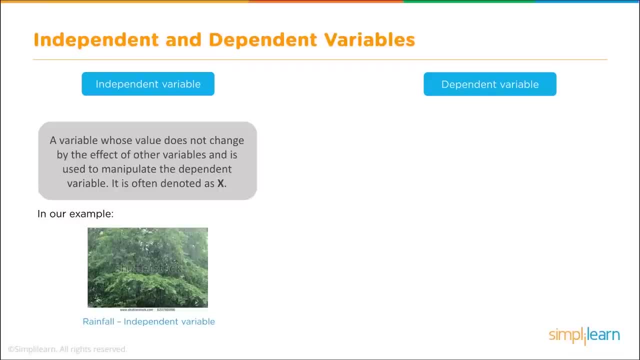 control the crop. So when we talk about the independent variable, controlling the dependent variable, let's define dependent variable as a variable whose value change when there is any manipulation: the values of the independent variables. It is often denoted as Y And you can see here our crop yield is 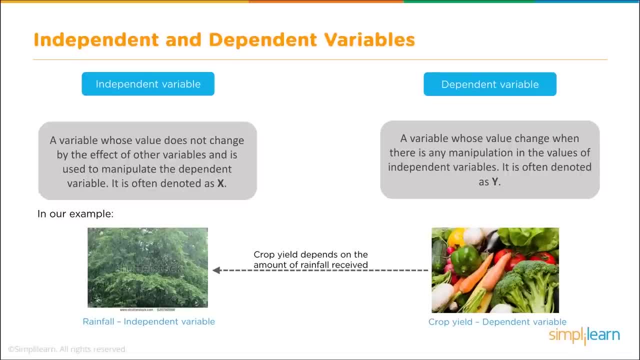 dependent variable and it is dependent on the amount of rainfall received. Now that we've taken a look at a real-life example, let's go a little bit into the theory and some definitions on machine learning and see how that fits together with linear regression, Numerical and categorical. 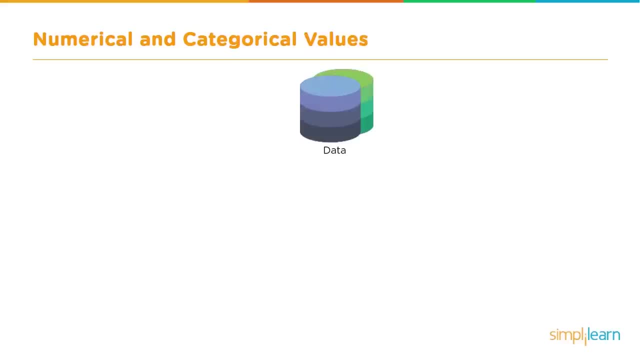 values. Let's take our data coming in. This is kind of random data from any kind of project. We want to divide it up into numerical and categorical. So numerical is numbers: age, salary, height, where categorical would be a description, the color, a dog's breed, gender. Categorical is: 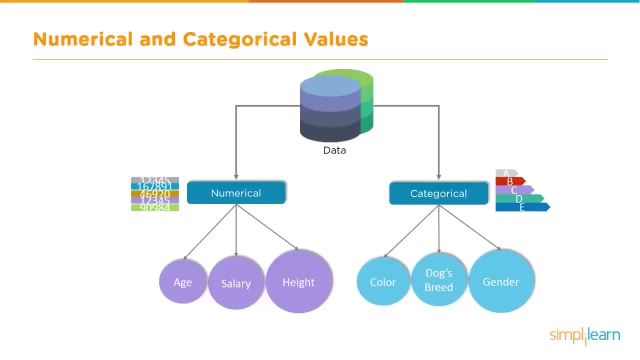 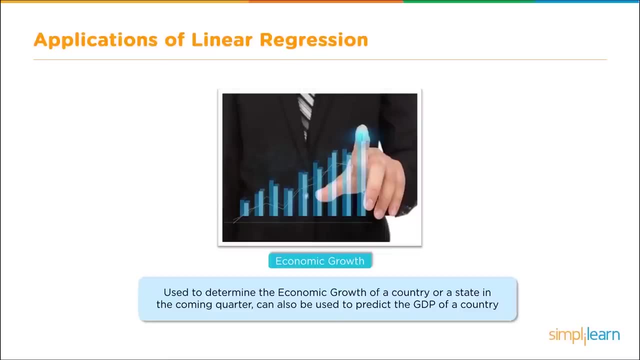 limited to very specific items where numerical is a range of information. Let's look at a few applications of linear regression. Economic growth, Used to determine the economic growth of a country or a state in the coming quarter, Can also be used to predict the GDP of a country. Product price Can be used to predict what would be the price of a. 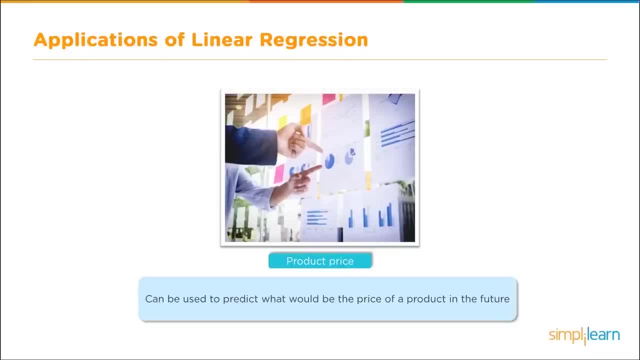 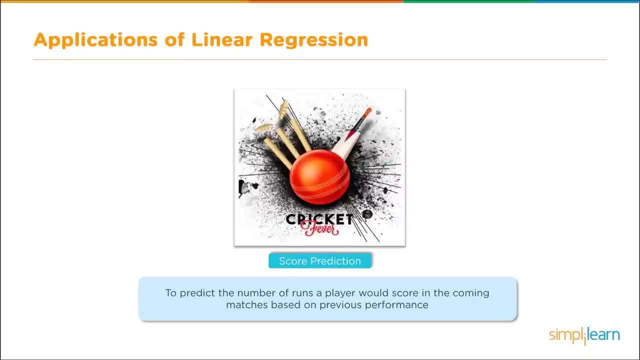 product in the future. We can guess whether it's going to go up or down. or should I buy today? Housing sales: To estimate the number of houses a builder would sell and what price in the coming months. Score predictions- Cricket fever: To predict the number of houses a builder would sell. 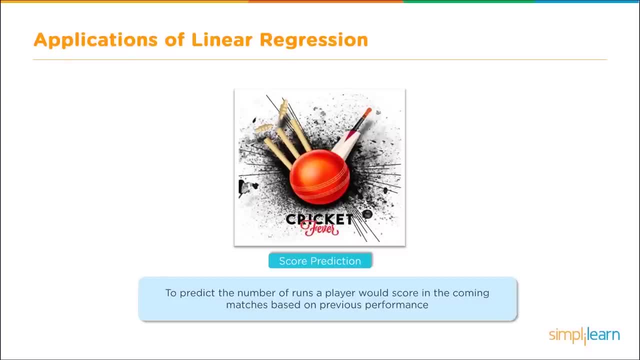 and what price in the coming months, The number of runs a player would score in the coming matches based on the previous performance. I'm sure you can figure out other applications you could use linear regression for. So let's jump in and let's understand linear regression and dig into the 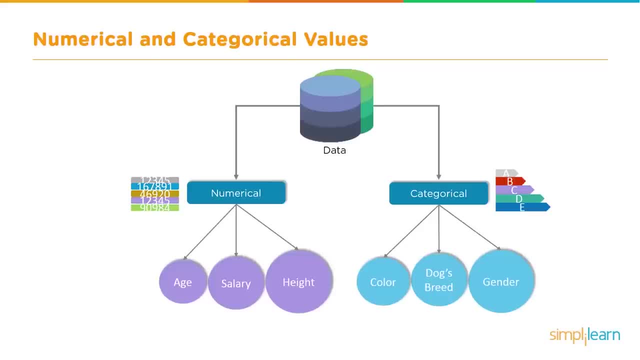 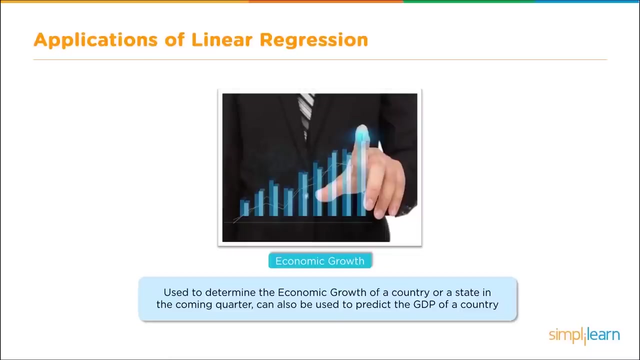 want to divide it up into numerical and categorical. so numerical is numbers- age, salary, height, where categorical would be a description, the color dogs, breed, gender. categorical is limited to very specific items, where numerical is a range of information. let's look at a few applications of linear regression economic growth used to determine the economic growth of a. 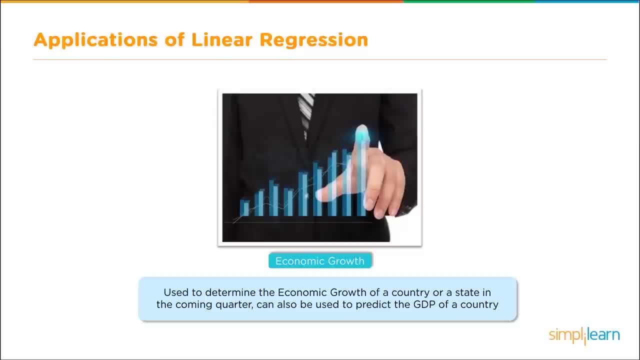 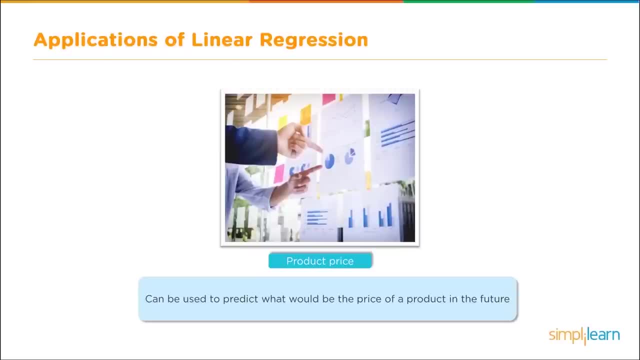 country or a state in the coming quarter can also be used to predict the GDP of a country. product price can be used to predict what would be the price of a product in the future. we can guess whether it's going to go up or down. or should I buy today? 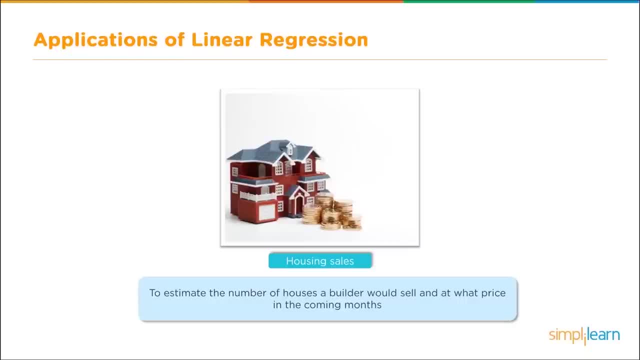 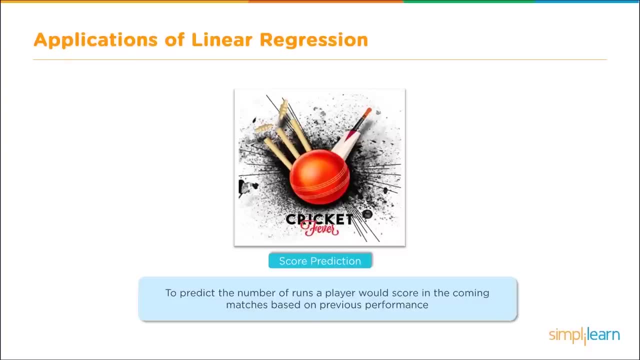 housing sales: to estimate the number of houses a builder would sell, and what price, in the coming months. score predictions- cricket fever: to predict the number of runs a player with score in the coming matches based on the previous performance. I'm sure you can figure out other applications you could use linear. 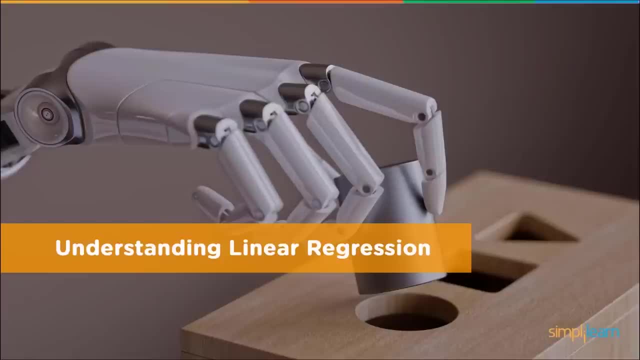 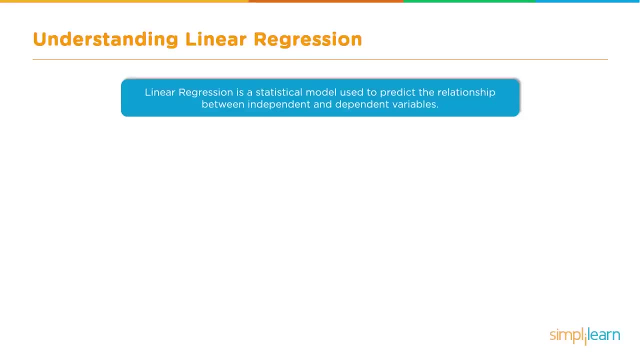 regression for. so let's jump in and let's understand linear regression and dig into the theory. understanding linear regression: linear regression is a statistical model used to predict the relationship between independent and dependent variables by examining two factors. the first, important one, is which variables in particular are significant predictors. 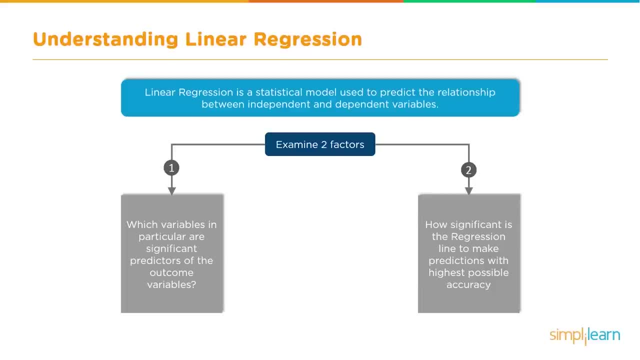 of the outcome variable, and the second one that we need to look at closely is: how significant is the regression line to make predictions with the highest possible accuracy? if it's inaccurate, we can't use it, so it's very important we find out the most accurate line we can get, since linear regression is based on. 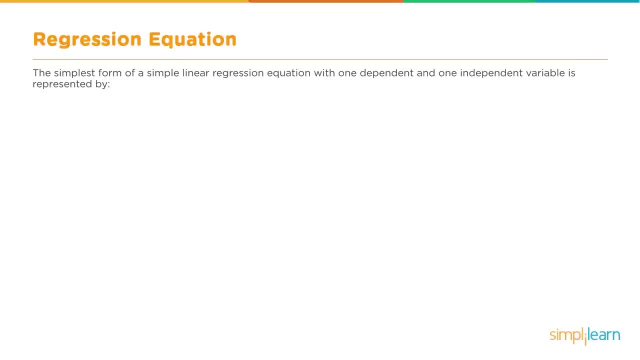 drawing a line through data. we're going to jump back and take a look at some Euclidean geometry. the simplest form of a simple linear regression equation with one dependent and one independent variable is represented by y equals m times x plus c. if you look at our model here, we plotted two points on here: x1 and y1, x2 and y2. 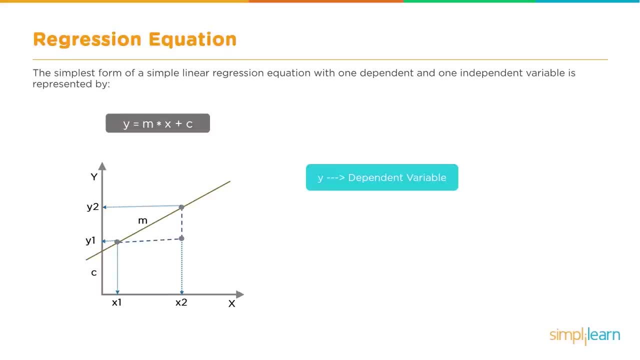 y being the dependent variable- remember that from before- and x being the independent variable. so y depends on whatever axis. m, in this case, is the slope of the line, where m equals the difference in the y2 minus y1 and x2 minus x1. and finally we have c, which is the coefficient of the. 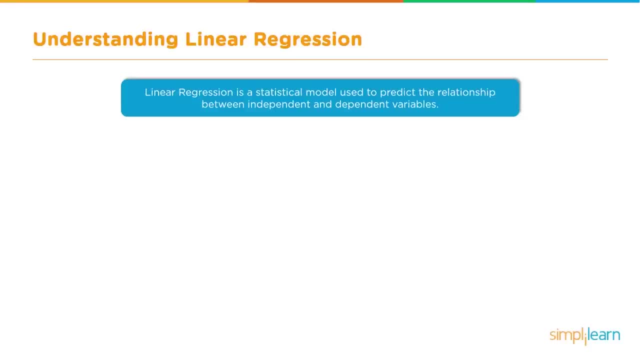 theory Understanding linear regression. Linear regression is the statistical model used to predict the relationship between independent and dependent variables by examining two factors. The first important one is which variables in particular are significant predictors of the outcome variable, And the second one that we need to look at closely. 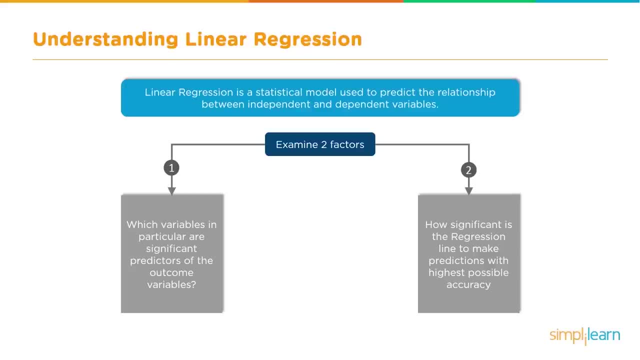 is: how significant is the regression line to make predictions with the highest possible accuracy? If it's inaccurate, we can't use it. so it's very important we find out the most accurate line we can get. Since linear regression is based on drawing a line through data, we're going to jump. 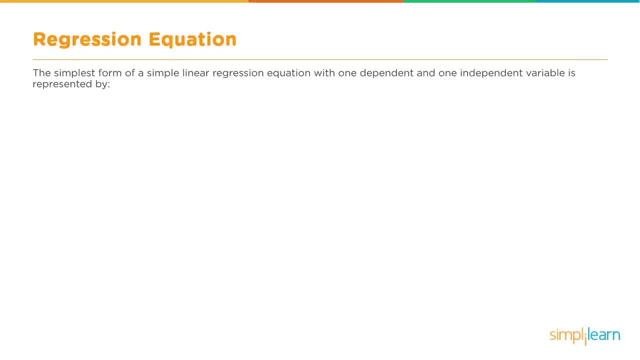 back and take a look at some Euclidean geometry. The simplest form of a simple linear regression equation with one dependent and one independent variable is linear regression. Linear regression is variable, is represented by: y equals m times x plus c. And if you look at our model here, we plotted two points on here: x1 and y1,, x2 and y2, y being the dependent variable- remember that from before- and x being the independent variable. So y depends on whatever x is. M in this case is the slope of the line where m equals the difference in the y2 minus y1. 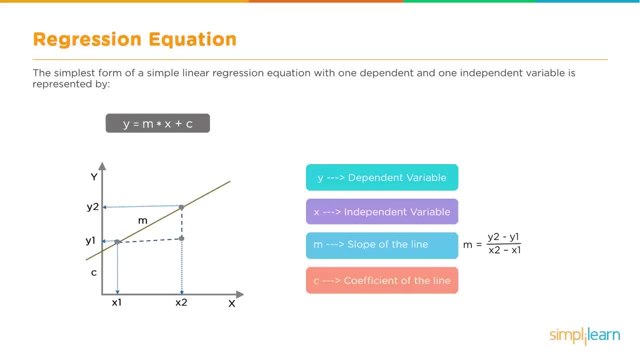 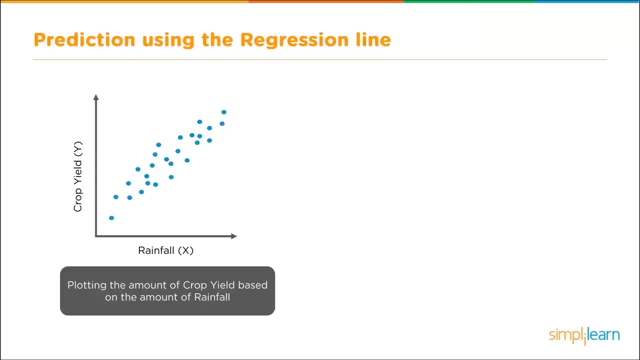 and x2 minus x1. And finally we have c, which is the coefficient of the line, or where it happens to cross the zero axes. Let's go back and look at an example we used earlier of linear regression. We're going to go back to plotting the amount of crop yield based on the amount of rainfall, And here we have our rainfall- Remember, we cannot change rainfall- And we have our crop yield, which is dependent on the rainfall. So we have our independent and our dependent variables. 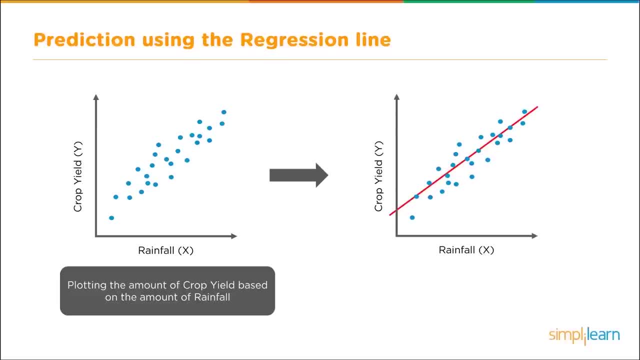 We're going to take this and draw a line through it as best we can, through the middle of the data, And then we look at that. we put the red point on the y-axis is the amount of crop yield you can expect for the amount of rainfall represented by the green dot. So if we have an idea what the rainfall is for this year and what's going on, then we can guess how good our crops are going to be. And we've created a nice line right through the middle to give us a nice mathematical formula. Let's take a look and see what the math looks like behind this. Let's look at the intuition behind the regression. 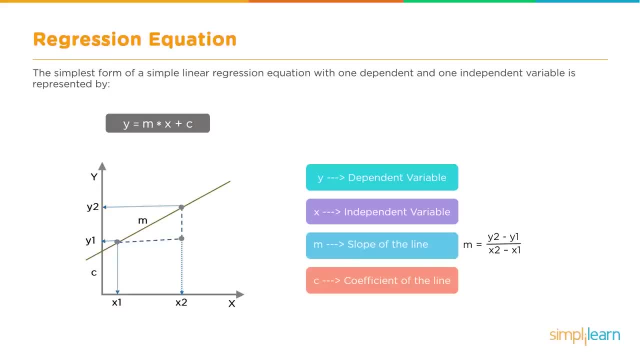 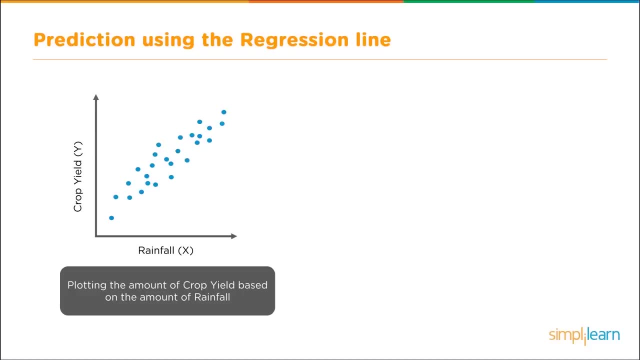 line or where happens to cross the zero axes. let's go back and look at an example we used earlier of linear regression. we're going to go back to plotting the amount of crop yield based on the amount of rainfall, and here we have our rainfall. remember, we cannot change rainfall. 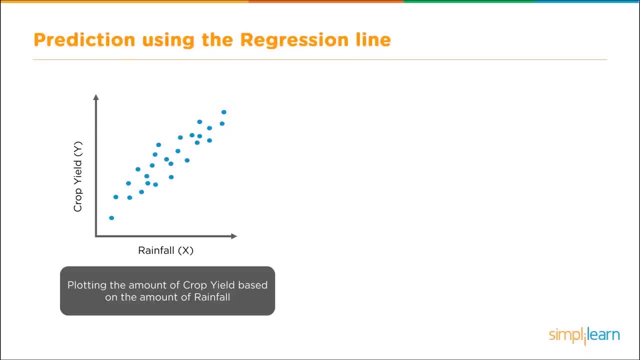 and we have our crop yield, which is dependent on the rainfall. so we have our independent and our dependent variables. we're going to take this and draw a line through it as best we can through the middle of the data, and we look at that. we put the red point on the y-axis is 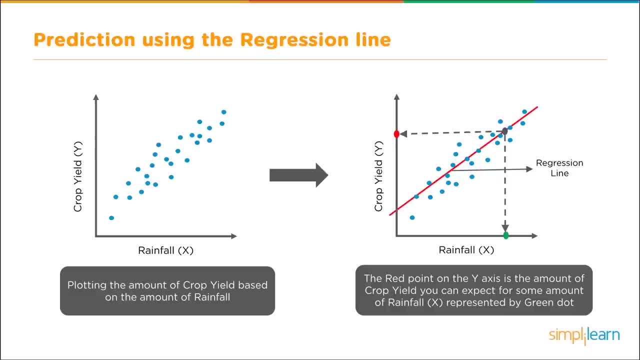 the amount of crop yield you can expect for the amount of rainfall represented by the green dot. so if we have an idea what the rainfall is for this year and what's going on, we can guess how good our crops are going to be. and we've created a nice line. 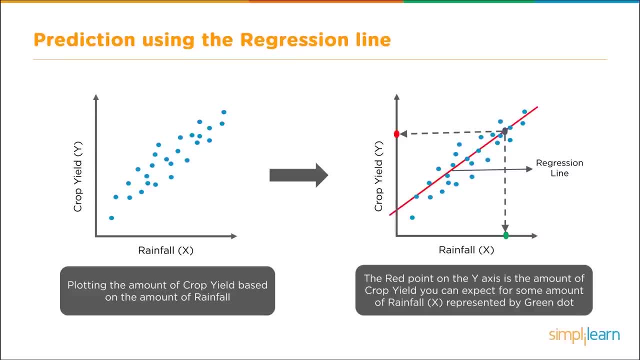 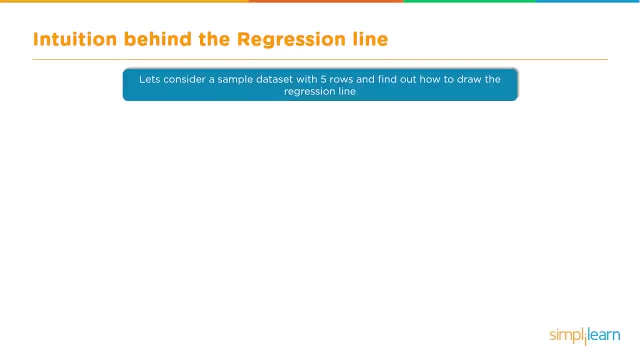 line right through the middle to give us a nice mathematical formula. Let's take a look and see what the math looks like behind this. Let's look at the intuition behind the regression line. Now, before we dive into the math and the formulas that go behind this and what's, 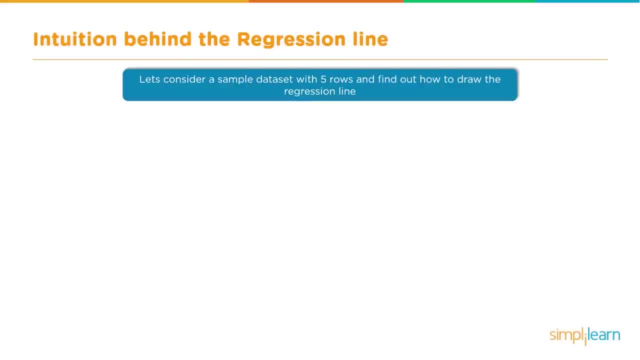 going on behind the scenes. I want you to note that when we get into the case study and we actually apply some Python script, that this math that you're going to see here is already done automatically for you. You don't have to have it memorized, It is. however. 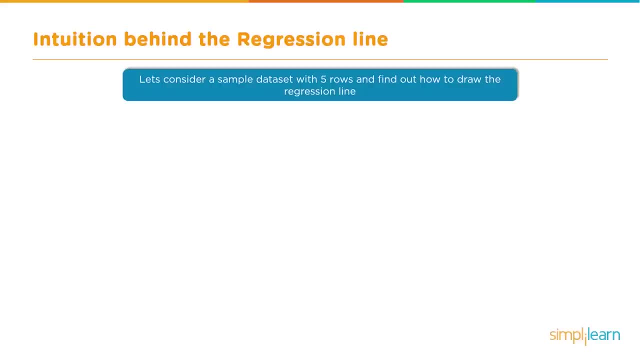 good to have an idea of what's going on, so if people reference the different terms, you'll know what they're talking about. Let's consider a sample data set with five rows and find out how to draw the regression line. We're only going to do five rows because if we did, 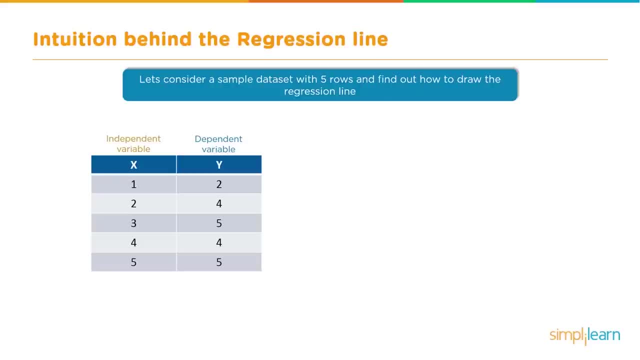 like the rainfall. with hundreds of points of data, that would be very hard to see what's going on with the mathematics. So we'll go ahead and create our own two sets of data and we have our independent variable, x, and our dependent variable, y, And when x was one, we got y equals two When x was. 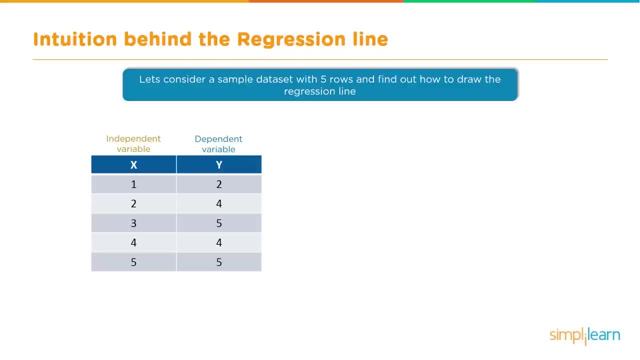 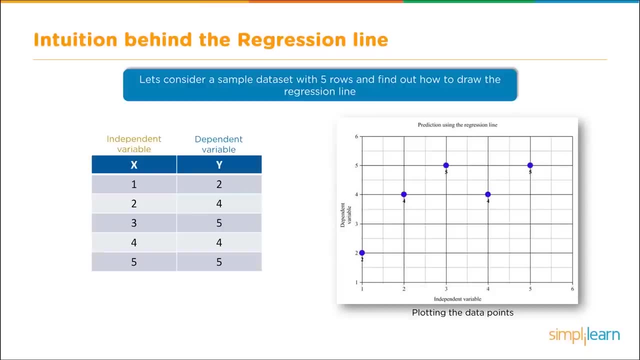 two, y was four, and so on and so on. If we go ahead and plot this data on a graph, we can see how it forms a nice line through the middle. You can see where it's kind of grouped, going upwards to the right. The next thing we want to know is what the means is of each. 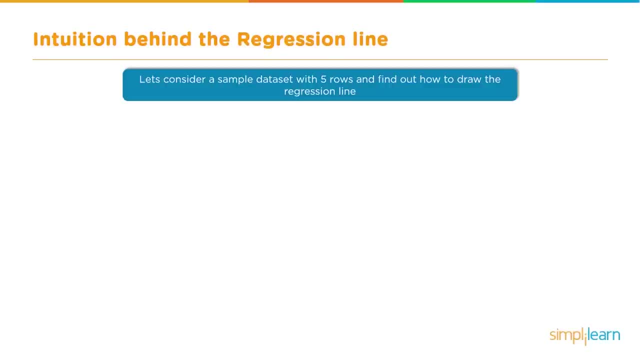 line. Now, before we dive into the math and the formulas that go behind this and what's going on behind the scenes, I want you to note that, when we get into the case study and we actually apply some Python script, that this math that you're going to see here is already done automatically for you. You don't have to have it memorized. It is, however, good to have an idea what's going on, So if people reference the different terms, you'll know what they're talking about. Let's consider a sample data set with five. 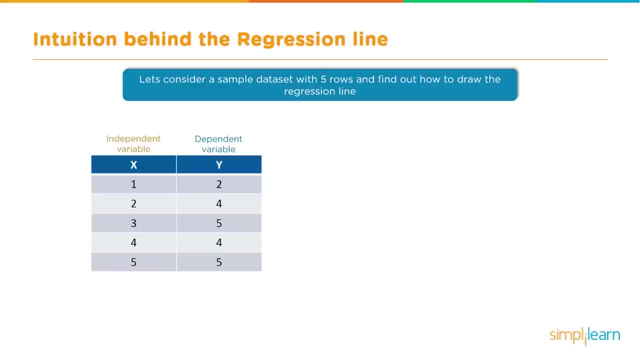 rows and find out how to draw the regression line. We're only going to do five rows because if we did, like the rainfall, with hundreds of points of data, that would be very hard to see what's going on with the mathematics. So we'll go ahead and create our own two sets of data And we have our independent variable, x, and our dependent variable, y. And when x was one, we got y equals two, When x was two, y was four, and so on and so on. If we go ahead and plot this data on a graph, 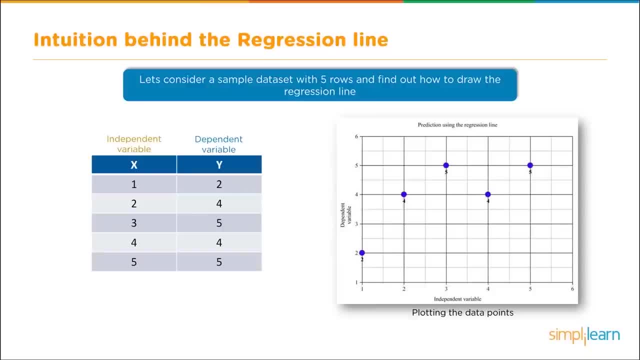 we can see how it forms a nice line through the middle. You can see where it's kind of grouped, going upwards to the right. The next thing we want to know is what the means is of each of the data coming in, the x and the y. The means doesn't mean anything other than the average. So we add up all the numbers and divide by the total. So one plus two plus three plus four plus five over five equals three, And the same for y. We get four. If we go ahead and plot the means on the graph, we'll see we get three comma four. 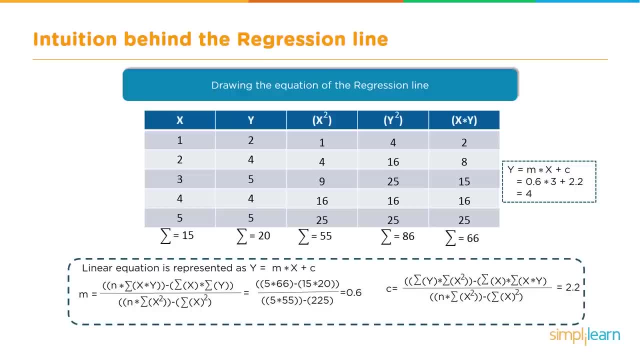 which draws a nice line down the middle, A good estimate. Here we're going to dig deeper into the math behind the regression line. Now remember before I said, you don't have to have all these formulas memorized or fully understand them, even though we're going to go into a little more detail of how it works. And if you're not a math whiz and you don't know, if you've never seen the sigma character before, which looks a little bit like an e that's opened up. that just means summation. That's all that is. So when you see the sigma character, it just means we're adding everything in 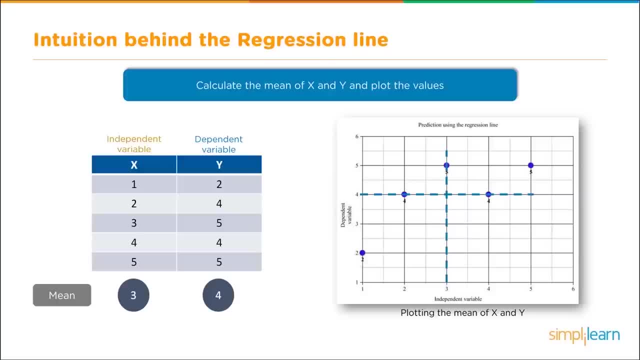 of the data coming in, the x and the y. The means doesn't mean anything other than the average. So we add up all the numbers and divide by the total. So one plus two plus three plus four plus five over five equals three, And the same for y: We get four If we go ahead. 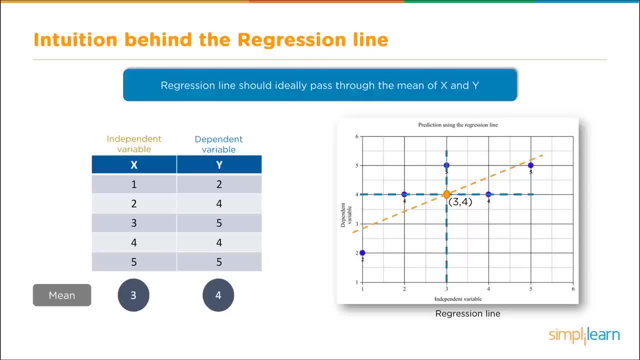 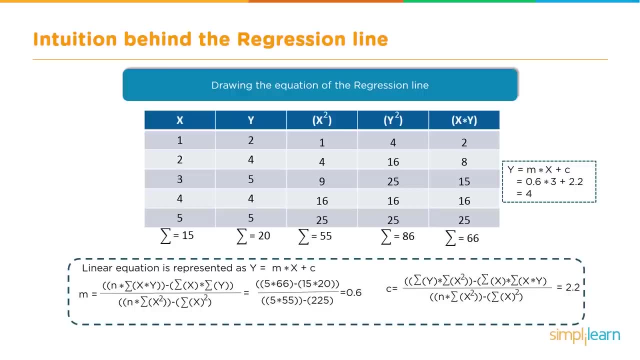 and plot the means on the graph, we'll see. we get three comma four, which draws a nice line down the middle, A good estimate. Here we're going to dig deeper into the math behind the regression line. Now remember before I said you don't have to have all these formulas. 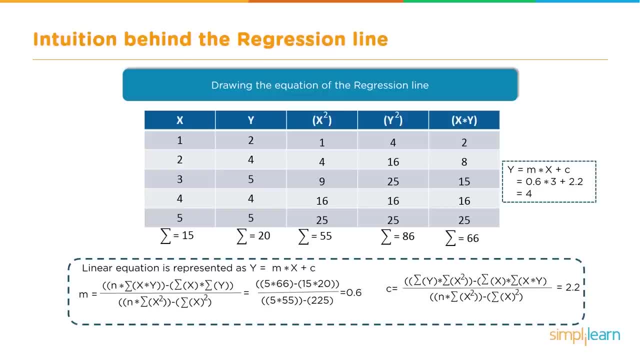 memorized or fully understand them, even though we're going to go into a little more detail of how it works. And if you're not a math whiz and you don't know, if you've never seen the sigma character before, which looks a little bit like an e, that's opened up that. 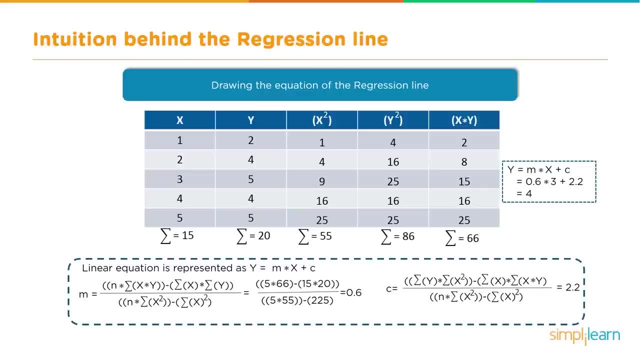 just means summation. That's all that is. So when you see the sigma character, it just means we're adding everything in that row, And for computers this is great because as a programmer you can easily iterate through each of the xy points and create all the information. 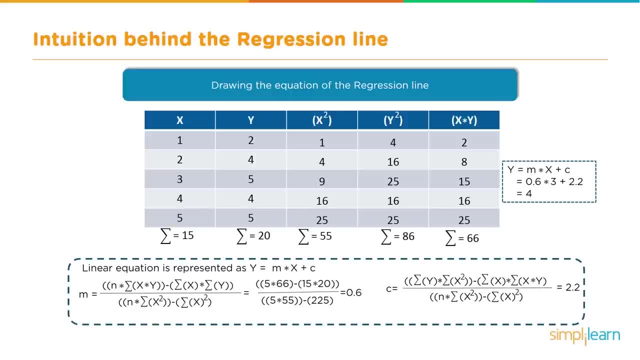 you need. So in the top half you can see where we've broken that down into pieces And as it goes through the first two points, it goes through the first two points and computes the squared value of x, the squared value of y and x times y, And then it takes 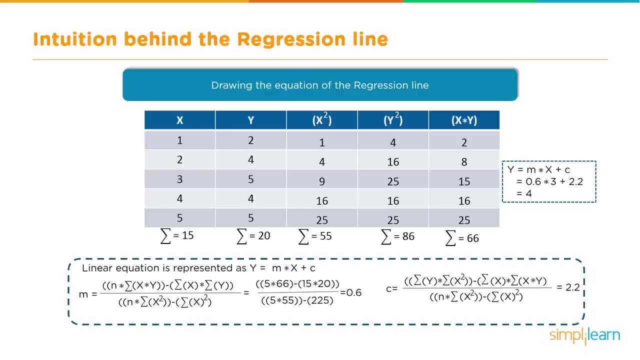 all of x and adds them up. all of y, adds them up. all of x squared, adds them up, and so on, and so on, And you can see we have: the sum is equal to 15,. the sum is equal to 20,. 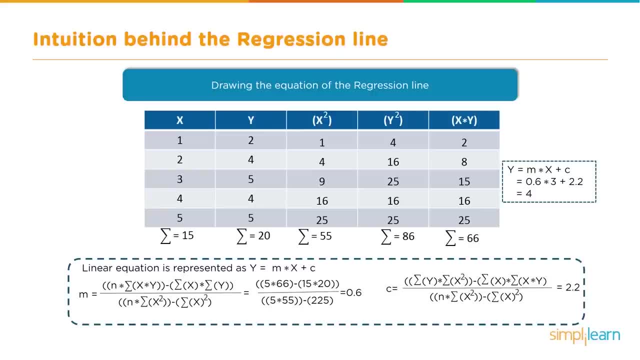 all the way up to x times y, where the sum equals 66.. This all comes from our formula for calculating a straight line where y equals the slope times x plus the coefficient c. So we go down below and we're going to compute minus x times y and we're going to compute. 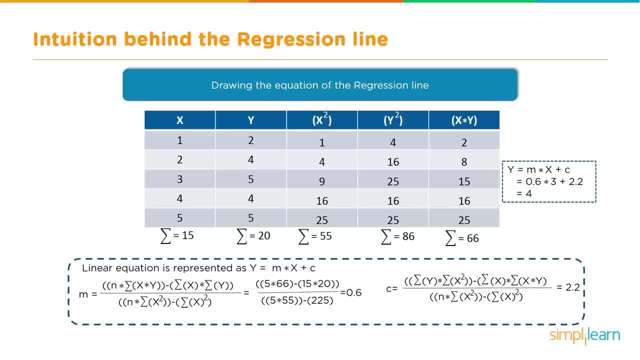 more like the averages of these, And we're going to explain exactly what that is in just a minute and where that information comes from. It's called the square means error, But we'll go into that in detail in a few minutes. All you need to do is look at the. 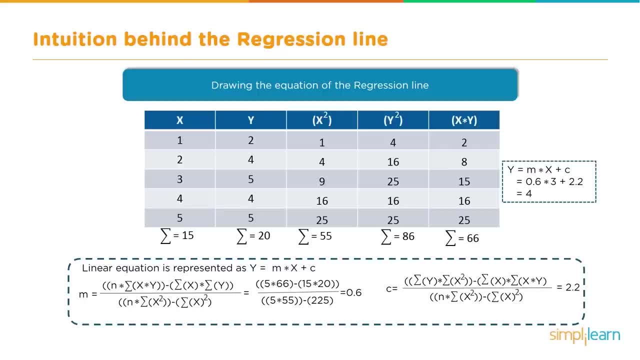 formula and see how we've gone about computing it line by line instead of trying to have a huge set of numbers pushed into it. And down here you'll see where the slope m equals and in the top part, if you read through the brackets, you have the number of data points. 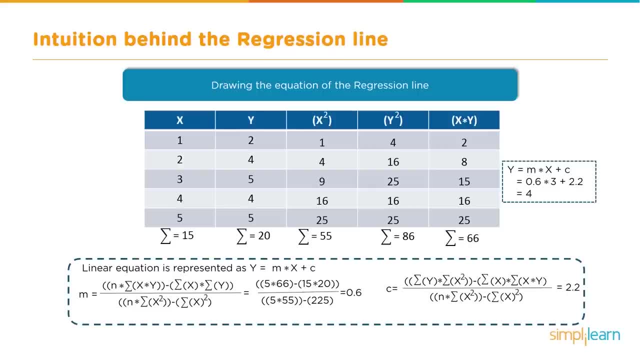 that row. And for computers this is great because as a programmer you can easily iterate through each of the xy points and create all the information you need. So in the top half you can see where we've broken that down into pieces. And as it goes through the first two points it computes the squared value of x, the squared value of y and x times y, And then it takes all of x and adds them up, All of y adds them up, All of x squared adds them up, and so on and so on And you can see we have the sum of equal to 15.. The sum is equal to 15.. 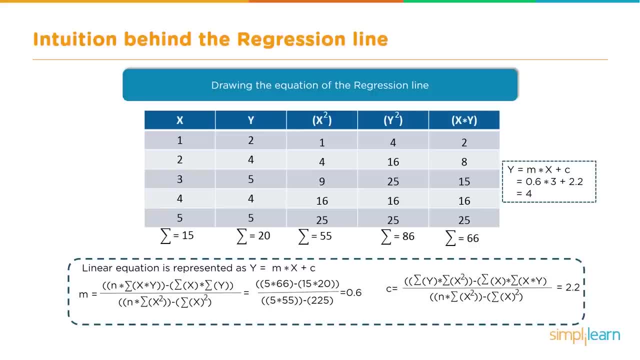 The sum is equal to 20.. All the way up to x times y, where the sum equals 66.. This all comes from our formula for calculating a straight line where y equals the slope times x plus the coefficient c. So we go down below and we're going to compute more like the averages of these And we're going to explain exactly what that is in just a minute and where that information comes from. It's called the square means error, But we'll go into that in detail in a few minutes. All you need to do is look at the formula and see how we've gone about computing it. 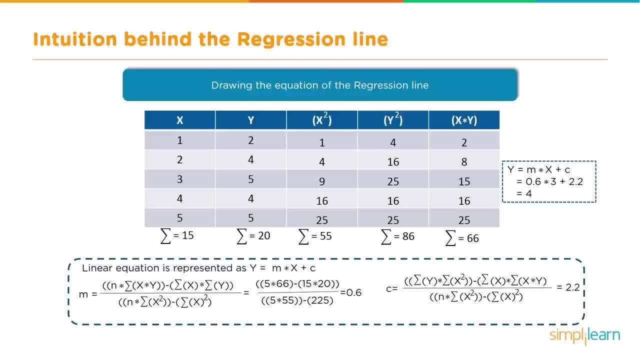 line by line instead of trying to have a huge set of numbers pushed into it. And down here you'll see where the slope m equals. And in the top part, if you read through the brackets, you have the number of data points times the sum of x times y, which we computed one line at a time there, And that's just the 66. And take all that and you subtract it from the sum of x times the sum of y, And those have both been computed, So you have 15 times 20.. 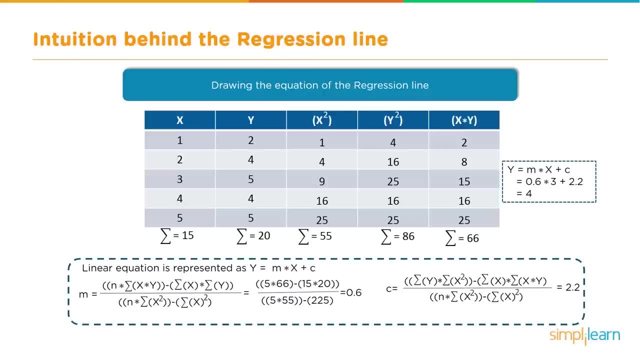 And on the bottom we have the number of lines times the sum of x squared, easily computed as 86 for the sum minus. I'll take all that and subtract the sum of x squared And we end up as we come across with our formula. you can plug in all those numbers, which is very easy to do on the computer. You don't have to do the math on a piece of paper or calculator- And you'll get a slope of 0.6.. And you'll get your c coefficient. If you continue to follow through that formula, you'll see it comes out as equal to 2.2.. 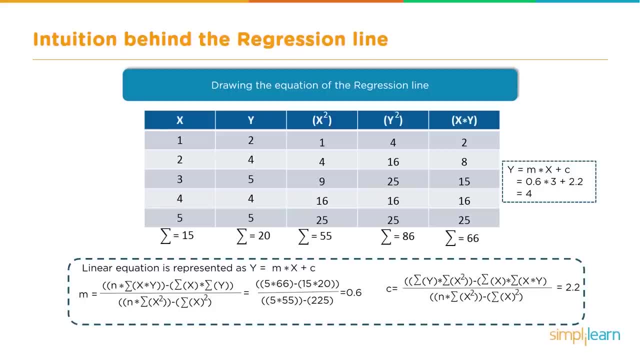 times The sum of x times y, which we computed one line at a time there, and that's just the 66. And take all that and you subtract it from the sum of x times the sum of y, And those have both been computed, So you have 15 times 20.. And on the bottom we have the. 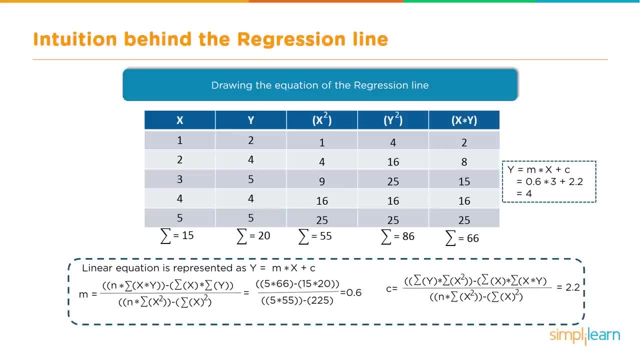 number of lines times the sum of x squared, easily computed as 86 for the sum minus. I'll take all that and subtract the sum of x squared And we end up as we come across with our formula. you can plug in all those numbers, which is very easy to do on the computer, You don't? 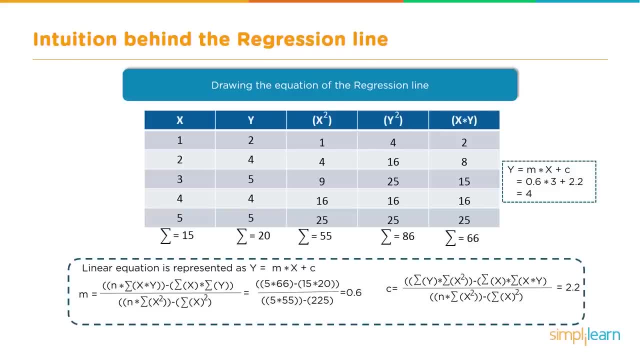 have to do the math on a piece of paper or a calculator And you'll get a slope of point six And you'll get your C coefficient. If you continue to follow through that formula, you'll see it comes out as equal to 2.2. 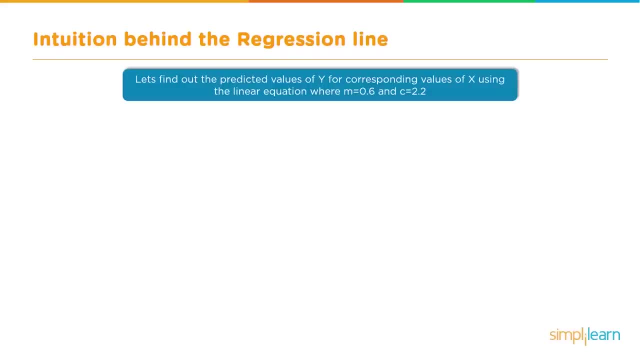 Continuing deeper into what's going behind the scenes, let's find out the predicted values of y for corresponding values of x using the linear equation where m equals point six and C equals two point two. We're going to take these values And we're going to go ahead. 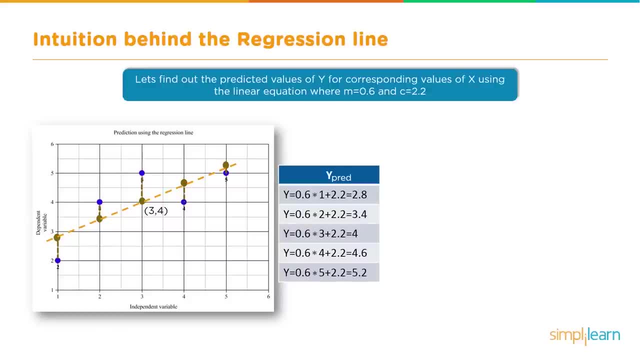 and plot them. We're going to predict them. So y equals 0.6 times where x equals 1, plus 2.2 equals 2.8, and so on and so on. And here the blue points represent the actual y values and the brown points. 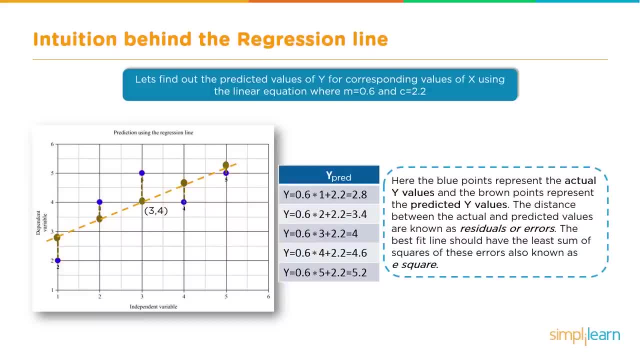 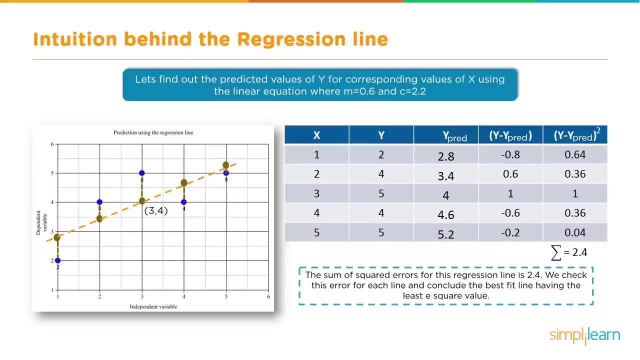 represent the predicted y values based on the model we created. The distance between the actual and predicted values is known as residuals or errors. The best fit line should have the least sum of squares of these errors, also known as e-square. If we put these into a nice chart, 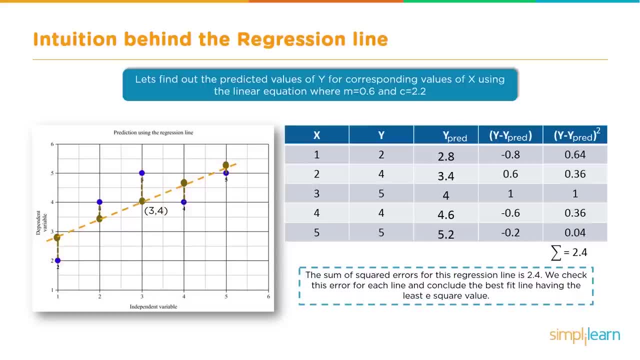 where you can see x and you can see y, what the actual values were, and you can see y predicted. you can easily see where we take y minus y predicted and we get an answer. What is the difference between those two? And if we square that y minus y prediction squared, we can then 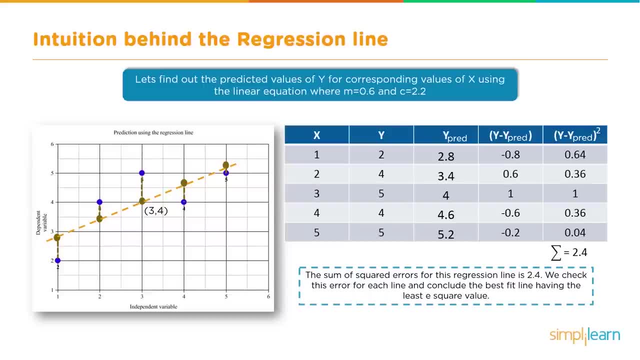 sum those squared values. That's where we get the 0.64 plus the 0.36 plus 1, all the way down until we have a summation equals 1.. So the sum of squared errors for this regression line is 2.4.. We check this error for each line. 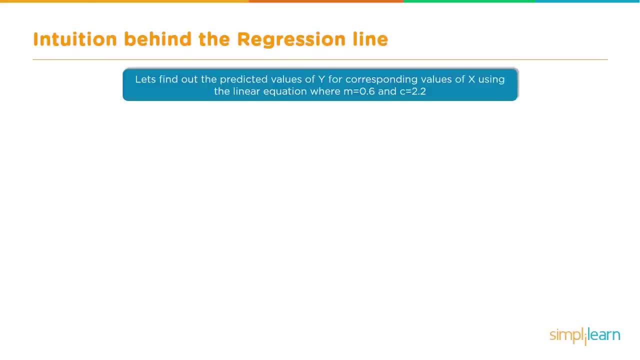 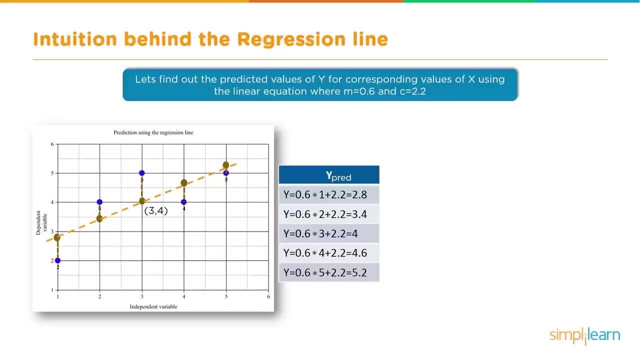 So, continuing deeper into what's going behind the scenes, let's find out the predicted values of y for corresponding values of x using the linear equation where m equals 0.6 and c equals 2.2.. We're going to take these values and we're going to go ahead and plot them. We're going to predict them. So y equals 0.6 times where x equals 1 plus 2.2 equals 2.8, so on and so on. And here the blue points represent the actual y values And the brown points represent the predicted values. 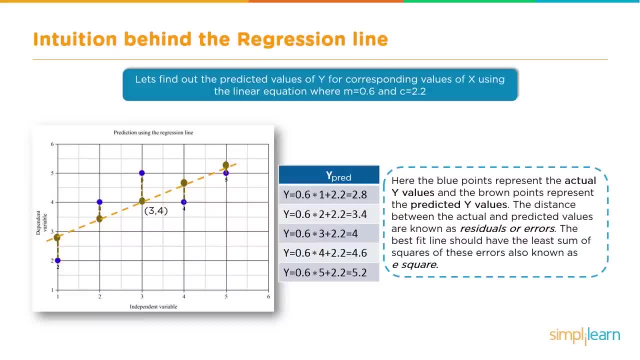 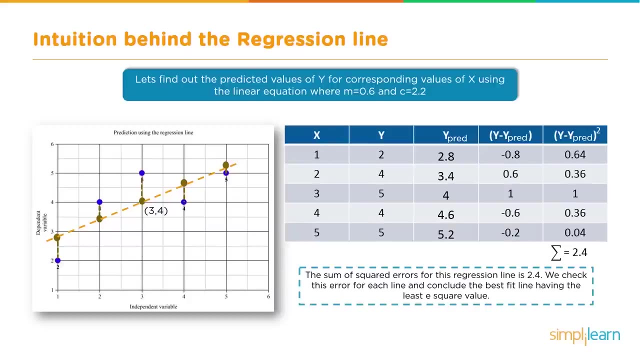 The distance between the actual and predicted values is known as residuals or errors. The best fit line should have the least sum of squares of these errors, also known as e squared. If we put these into a nice chart where you can see x and you can see y- what the actual values were and you can see y predicted- you can easily see where we take y minus y predicted and we get an answer. What is the difference between those two? 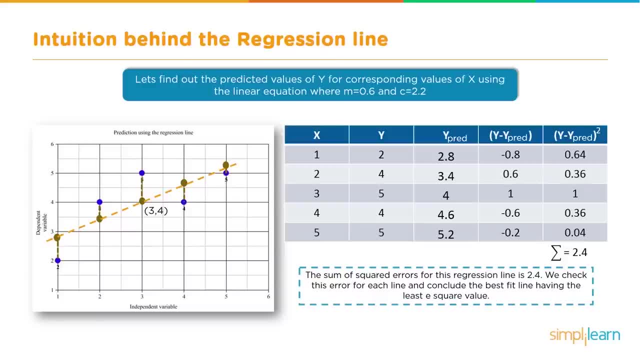 And if we square that y minus y- prediction squared, we can then sum those squared values. That's where we get the 0.64 plus the 0.36 plus 1, all the way down until we have a summation equals 2.4.. So the sum of squared errors for this regression line is 2.4.. We check this error for each line and conclude the best fit line having the least e squared value. 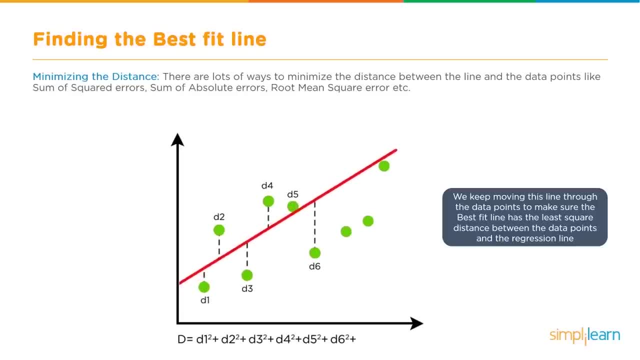 In a nice graphical representation. we can see here where we keep moving this line through the data points to make sure the best fit line has the least squared distance. Now we only looked at the most commonly used formula for minimizing the distance. There are lots of ways to minimize the distance between the line and the data points, like sum of squared errors, sum of absolute errors, root mean, square error, etc. 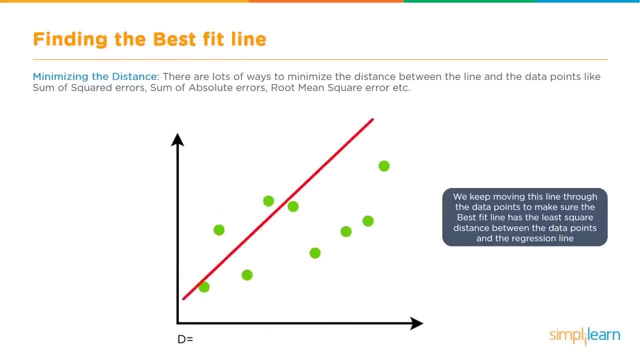 What you want to take away from this is: whatever formula is being used, you can easily, using a computer programming and iterating through the data, calculate the different parts of it. That way, these complicated formulas you see, with the different summations and absolute values, are easily computed, one piece at a time. 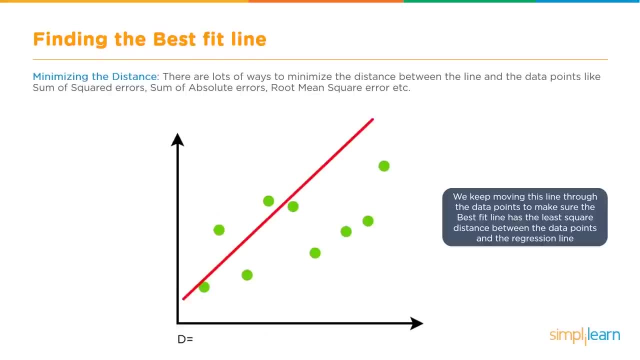 Up until this point, we've only been looking at two values: x and y. Well, in the real world, it's very rare that you only have two values when you're figuring out a solution. So let's move on to the next topic. 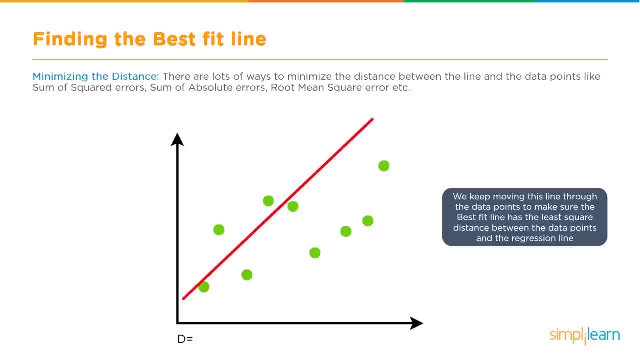 and conclude, the best fit line having the least e-square value In a nice graphical representation. we can see here where we keep moving this line through the data points to make sure the best fit line has the least squared distance between the data points and the regression line. Now we only 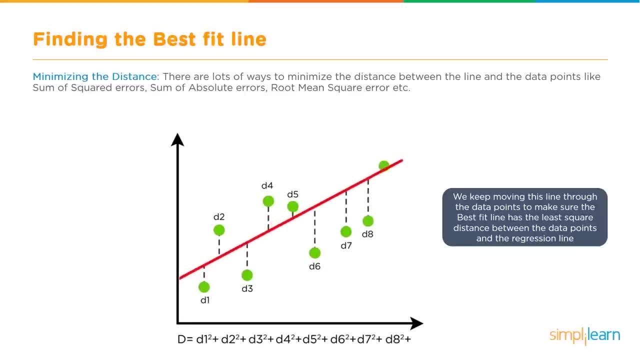 looked at the most commonly used formula for minimizing the distance. There are lots of ways to minimize the distance. We're going to look at the most commonly used formula for minimizing the distance between the line and the data points like sum of squared errors, sum of absolute errors. 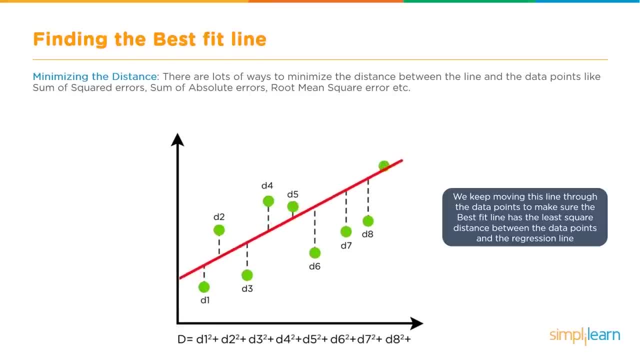 root mean square error, etc. What you want to take away from this is, whatever formula is being used, you can easily, using a computer programming and iterating through the data, calculate the different parts of it. That way, these complicated formulas you see, with the different summations and absolute. 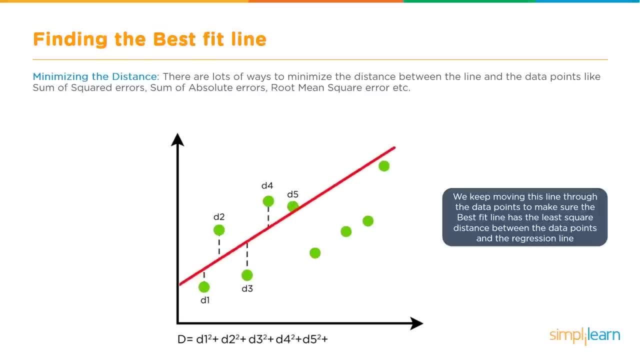 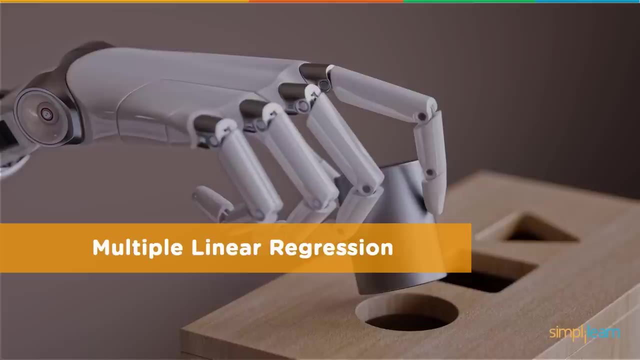 values are easily computed one piece at a time. Up until this point, we've only been looking at two values: X and y. Well, in the real world, it's very rare that you only have two values when you're figuring out a solution. So let's move on to the next topic: Multiple linear regression. Let's take a brief look at what happens. 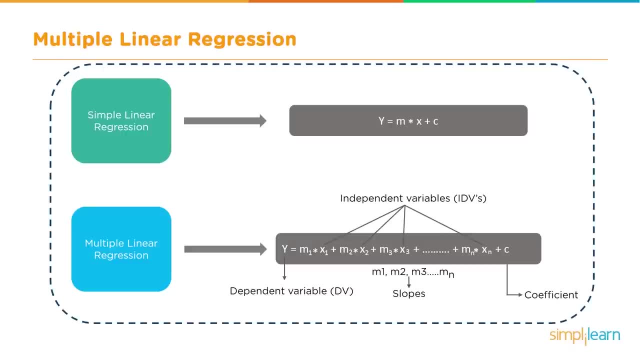 when you have multiple inputs. So in multiple linear regression we have. well, we'll start with the simple linear regression where we had y equals M plus X plus C and we're trying to find the value of Y. Now, with multiple linear regression, we have multiple variables coming in. So instead of having 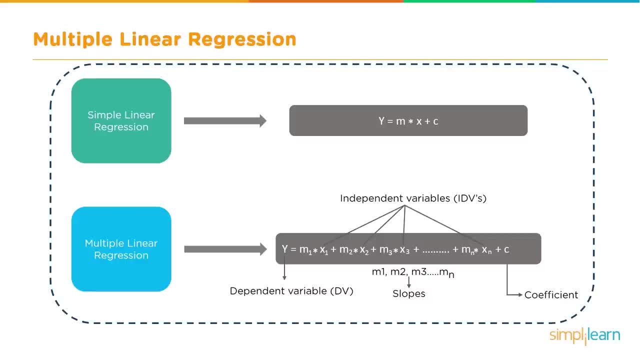 having just x. we have x1,, x2, x3.. And instead of having just one slope, each variable has its own slope attached to it. As you can see, here we have m1, m2,, m3, and we still just. 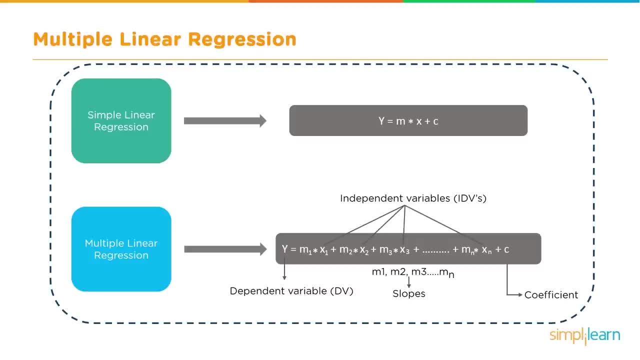 have the single coefficient. So when you're dealing with multiple linear regression, you basically take your single linear regression and you spread it out. So you have y equals m1 times x1 plus m2 times x2, so on all the way to m to the nth, x to the nth, and then 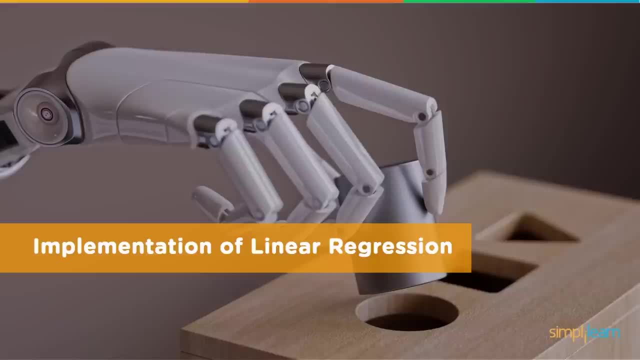 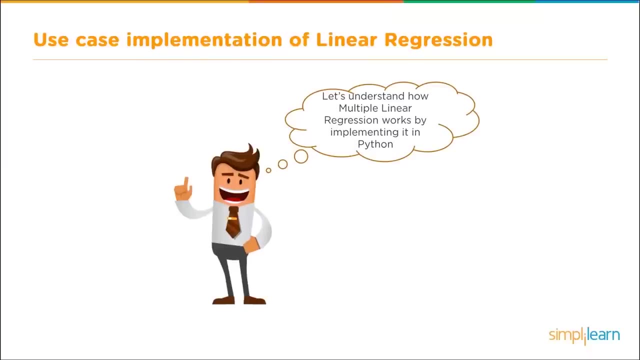 you add your coefficient on there. Implementation of linear regression: Now we get into my favorite part. Let's understand how multiple linear regression works by implementing it in Python. If you remember, before we were looking at a company and just based on its R&D trying. 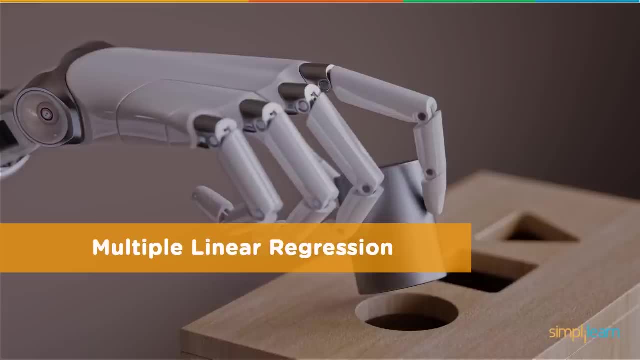 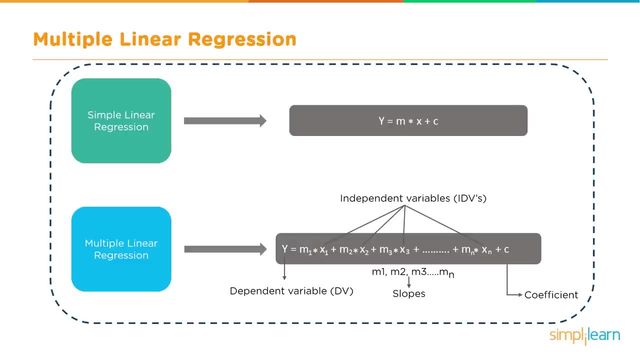 Multiple linear regression. Let's take a brief look at what happens when you have multiple inputs. So in multiple linear regression we have. well, we'll start with the simple linear regression Where we have the simple linear regression: had y equals m plus x plus c And we're trying to find the value of y. Now with multiple linear, 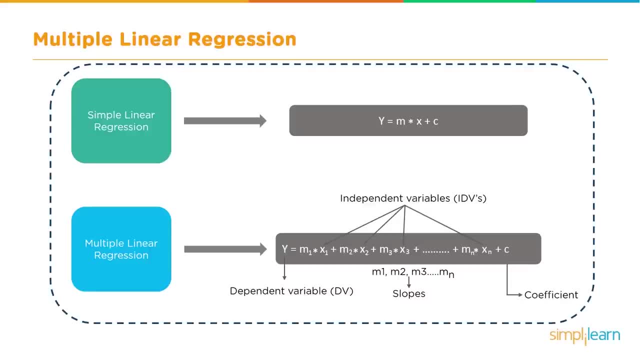 regression, we have multiple variables coming in. So instead of having just x, we have x1, x2, x3. And instead of having just one slope, each variable has its own slope attached to it. As you can see here, we have m1, m2, m3. And we still just have the single coefficient. So when you're dealing with 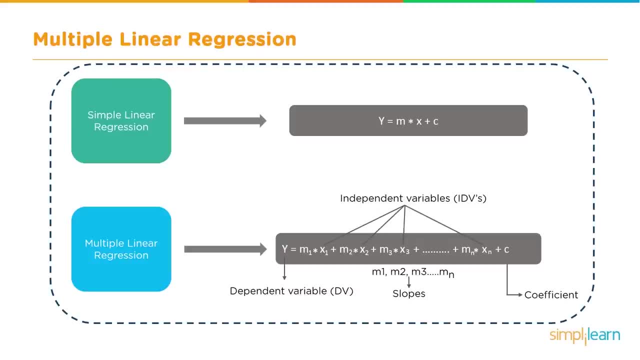 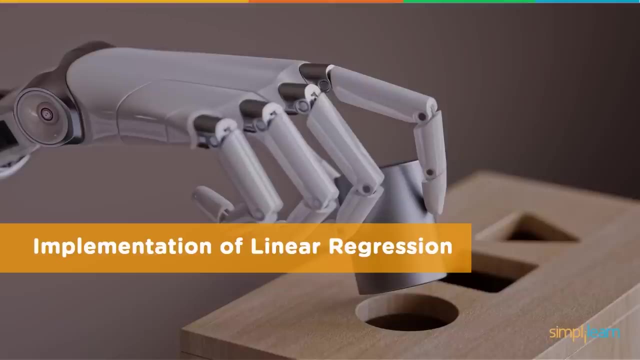 multiple linear regression. you basically take your single linear regression and you spread it out, So you have y equals m1 times x1, plus m2 times x2, so on all the way to m to the nth, x to the nth, and then you add your coefficient on there. Implementation of linear regression. Now we get. 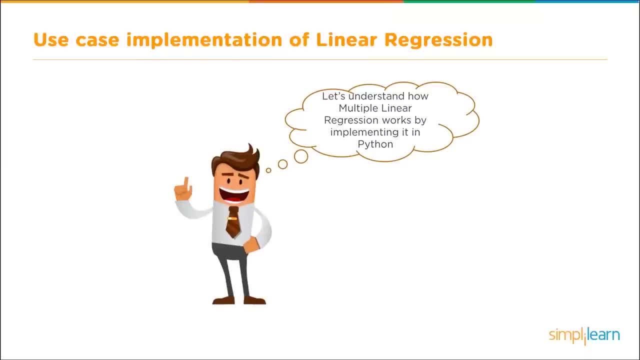 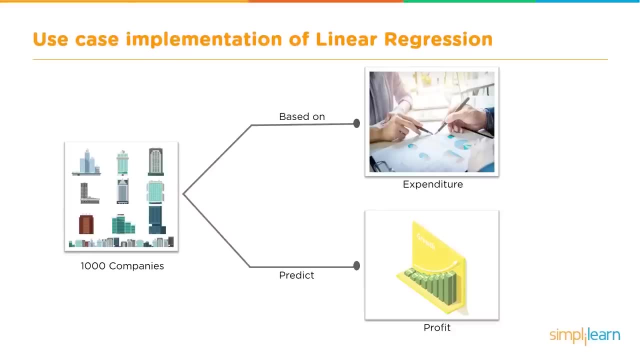 into my favorite part. Let's understand how multiple linear regression works by implementing it in Python. If you remember, before we were looking at a company and, just based on its R&D, trying to figure out its profit. We're going to start looking at the expenditure of the company. 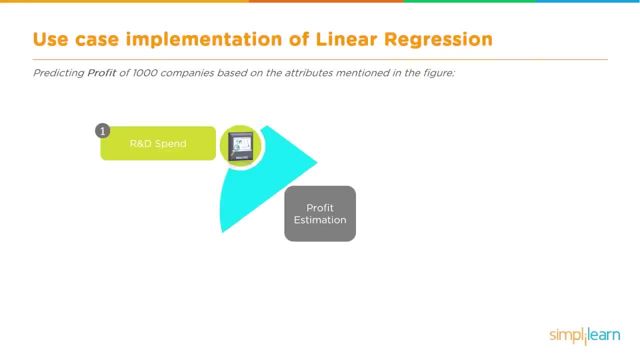 We're going to go back to that. We're going to predict its profit, But instead of predicting it just on the R&D, we're going to look at other factors like administration costs, marketing costs and so on, And from there we're going to see if we can figure out what the profit of that company. 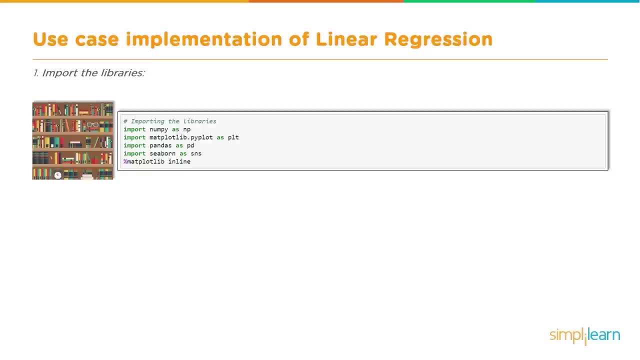 is going to be To start our coding. we're going to begin by importing some basic libraries And we're going to be looking through the data before we do any kind of linear regression. We're going to take a look at the data to see what we're playing with And we're going to take a look at. 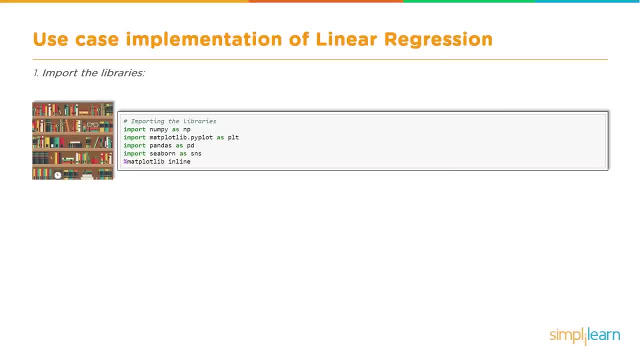 Then we'll go ahead and format the data to the format we need to be able to run it in the linear regression model, And then from there we'll go ahead and solve it and just see how valid our solution is. So let's start with importing the basic libraries. Now I'm going to be doing this. 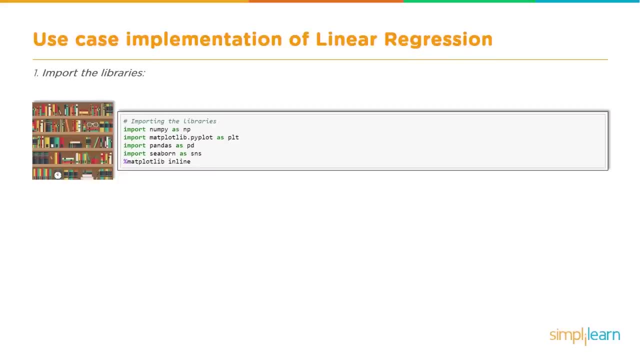 in Anaconda Jupyter Notebook, a very popular IDE. I enjoy it because it's such a visual to look at and it's so easy to use. Just any IDE for Python will work just fine for this. So break out your favorite Python IDE. So here we are in our Jupyter Notebook And we're going to start with a. 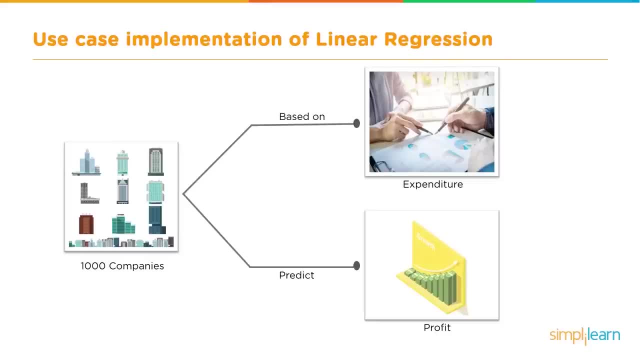 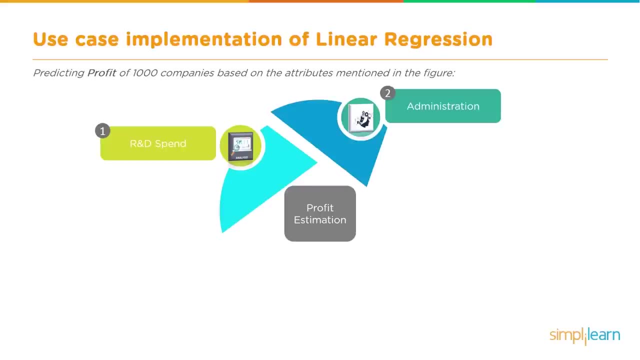 to figure out its profit. We're going to start looking at the expenditure of the company. We're going to go back to that. We're going to predict its profit. But instead of predicting it just on the R&D, we're going to look at other factors like administration costs, marketing. 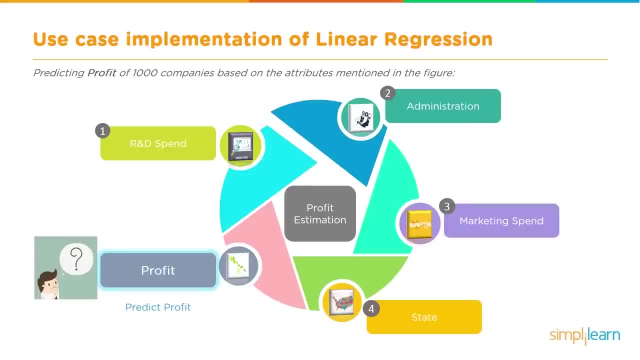 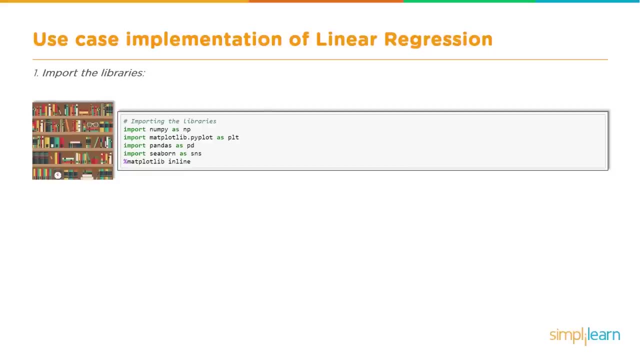 costs And so on, And from there we're going to see if we can figure out what the profit of that company is going to be. To start our coding, we're going to begin by importing some basic libraries And we're going to be looking through the data before we do any. 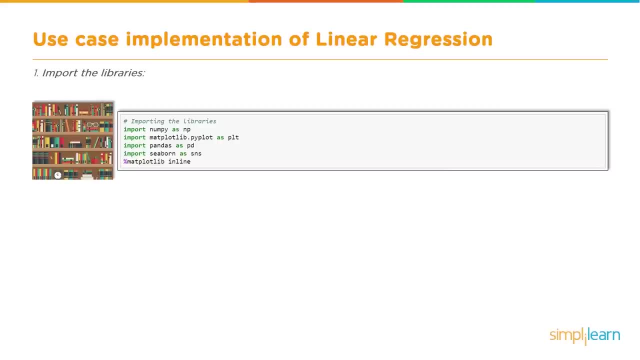 kind of linear regression. We're going to take a look at the data to see what we're playing with. Then we'll go ahead and format the data to the format we need to be able to run it in the linear regression model And then from there we'll go ahead and solve. 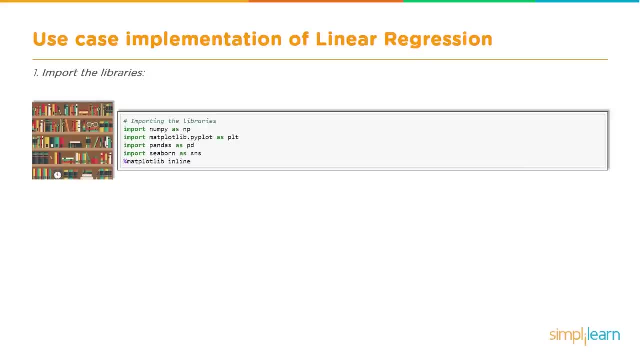 it and just see how valid our solution is. So let's start with importing the basic libraries. Now. I'm going to be doing this in Anaconda Jupyter Notebook, a very popular IDE. I enjoy it because it's such a visual to look at and so easy to use. Just any IDE for Python will. 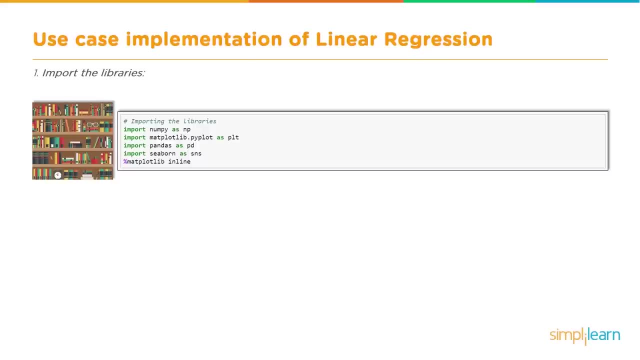 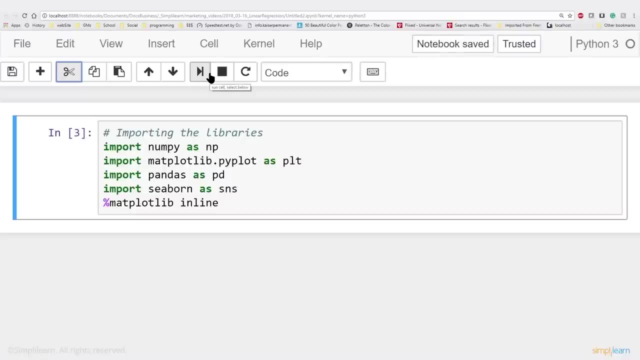 work just fine for this. So break out your favorite Python IDE. So here we are in our Jupyter Notebook. Let me go ahead and paste our first piece of code in there, And let's walk through what libraries we're importing. First we're going to import: 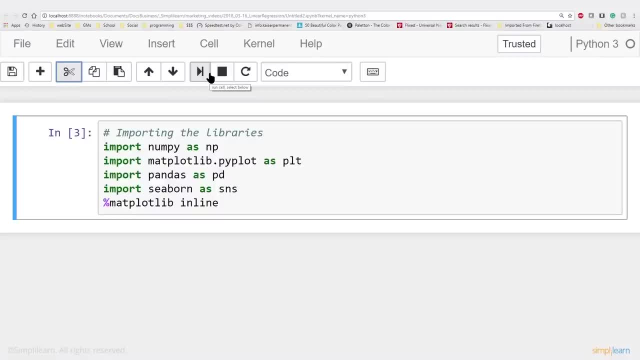 numpy as np. And then I want you to skip one line and look at import pandas as pd. These are very common tools that you need with most of your linear regression. The numpy, which stands for number Python, is usually denoted as np And you have to almost have. 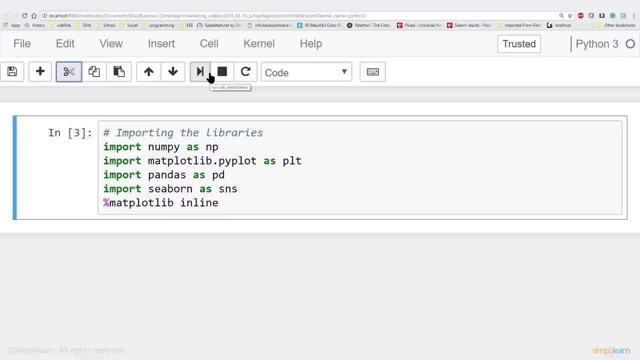 that for your sklearn toolbox, So you always import that right off the beginning, Pandas, although you don't have to have it for your sklearn libraries, it does such a wonderful job of importing data, setting it up into a data frame so we can manipulate it rather. 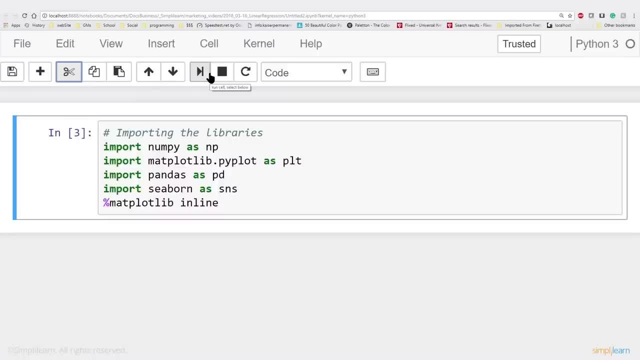 easily And it has a lot of tools also in addition to that. So we usually like to use the pandas when we can, And I'll show you what that looks like. The other three lines are for us to get a visual of this data and take a look at it. So we're going to import. 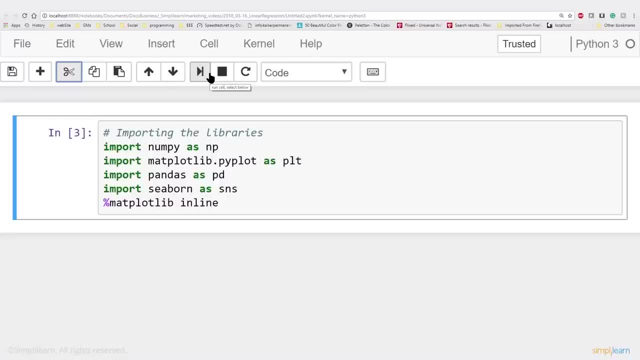 matplotlibrarypyplot as plt And then seaborn as sns. Seaborn works with the matplotlibrary, So you have to always import matplotlibrary and then seaborn sits on top of it And we'll take a look at what that looks like. You could use any of your own plotting libraries. you. 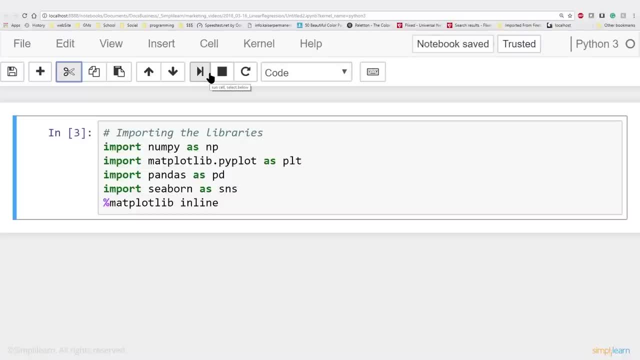 Jupyter Notebook. Let me go ahead and paste our first piece of code in there And let's walk through what libraries we're importing. First we're going to import numpy as np And then I want you to skip one line and look at import pandas as pd. These are very common tools that you need. 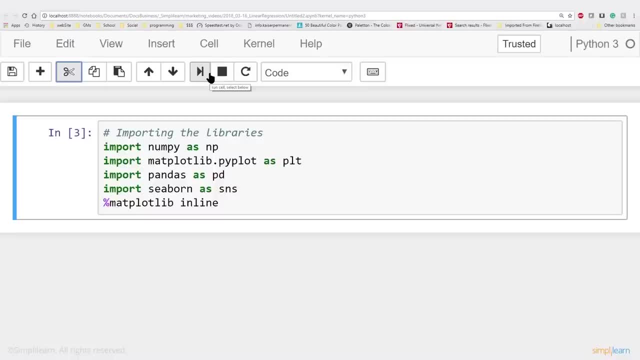 with most of your linear regression. The numpy, which stands for number. Python, is usually denoted as np, And you have to almost have that for your sklearn toolbox, So you always import that right off the beginning, Pandas. although you don't have to have it for your sklearn libraries, it does such. 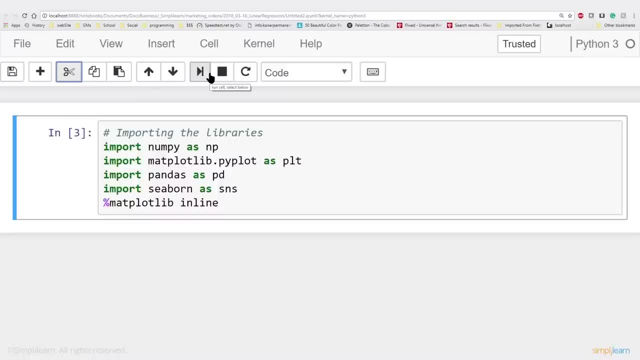 a wonderful job of importing data, setting it up into a data frame so we can manipulate it rather easily, And it has a lot of tools also in addition to that. So we usually like to use the pandas when we can, And I'll show you what that looks like. The other three lines are for us to get a visual of. 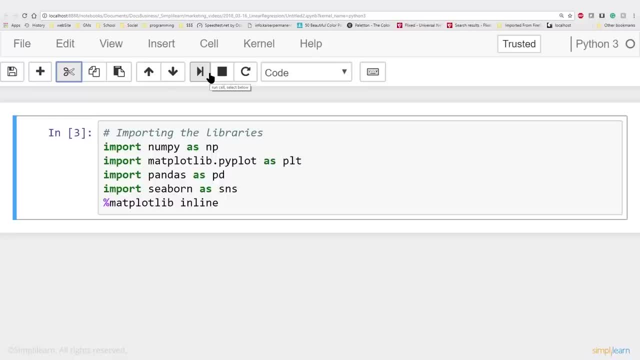 this data and take a look at it. So we're going to import matplotlibrarypyplot as plt And then sklearn as sns. sklearn works with the matplotlibrary, So you have to always import matplotlibrary and then sklearn sits on top of it, And we'll take a look at what that looks like. You could use any of your own. 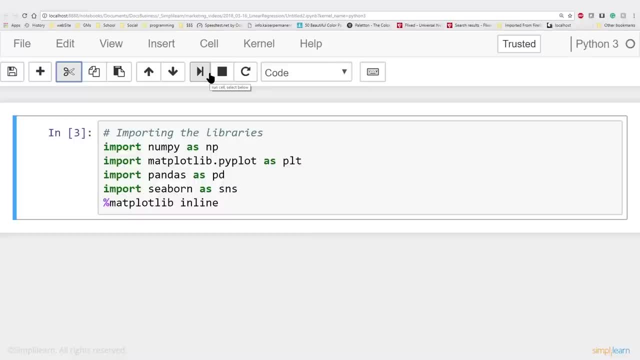 plotting libraries you want. There's all kinds of ways to look at the data. These are just very common ones. And the sklearn is so easy to use. it just looks beautiful. It's a nice representation that you can actually take and show somebody. And the final line is the amberson matplotlibrary inline. That is only because I'm 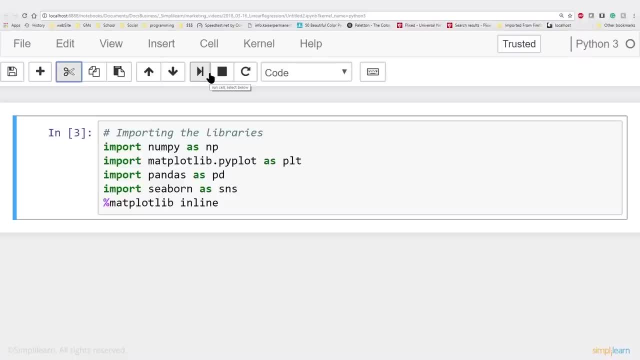 doing an inline IDE. My interface in the Anaconda Jupyter Notebook requires I put that in there or you're not going to be able to see the graph when it comes up. Let's go ahead and run this. It's not going to be that interesting. 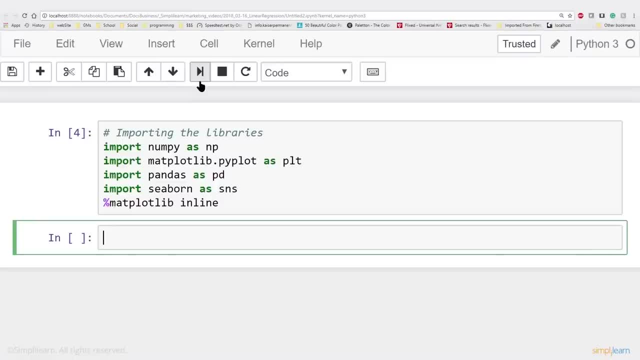 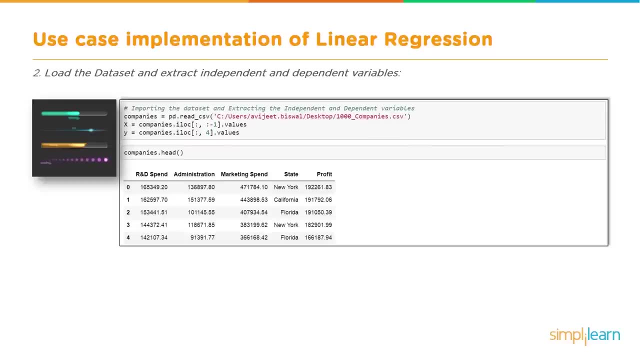 because we're just setting up variables. In fact, it's not going to do anything that we can see, but it is importing these different libraries and setup. The next step is load the data set and extract independent and dependent variables. Now here in the slide you'll see companies equals pdreadcsv and it has a long line there with the file at the end. 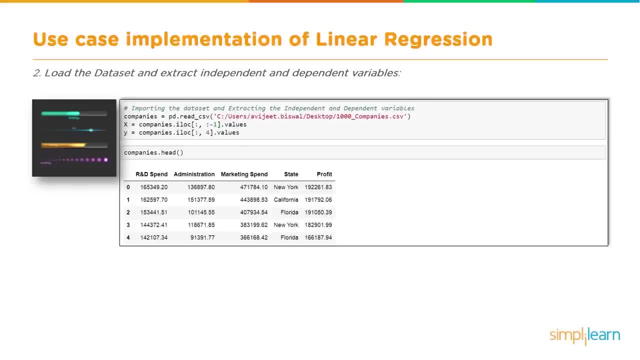 1000companiescsv. You're going to have to change this to fit whatever setup you have, And the file that you're going to use is the file itself. you can request. Just go down to the commentary below this video and put a note in there, and 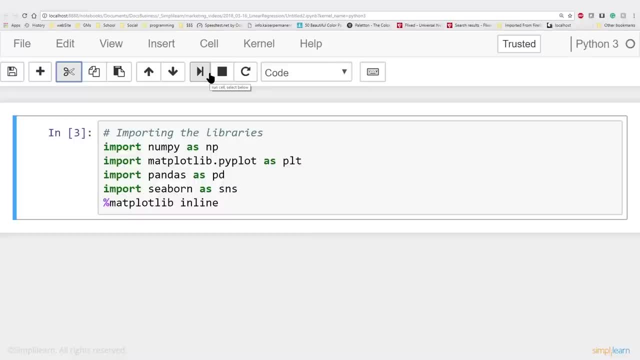 want. There's all kinds of ways to look at the data. These are just very common ones, and the seaborn is so easy to use that it just looks beautiful. It's a nice representation that you can actually take and show somebody, And the final line is the ambersand matplotlibrary. 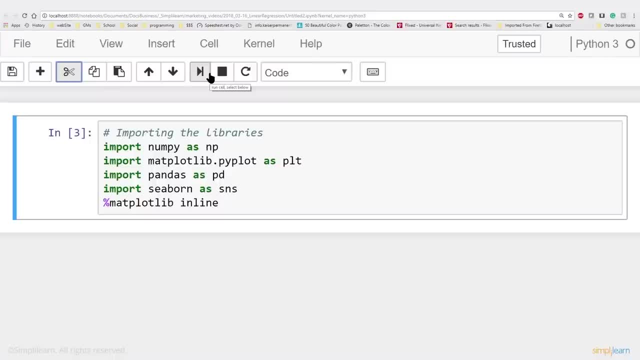 inline. That is only because I'm doing an inline IDE. My interface in the Anaconda Jupyter notebook requires I put that in there or you're not going to see the graph when it comes up. Let's go ahead and run this. It's not going to be that interesting because we're just 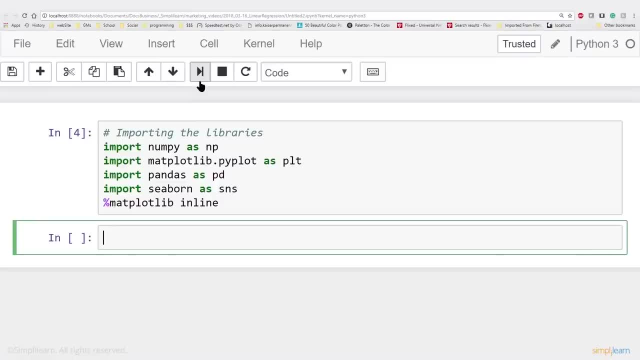 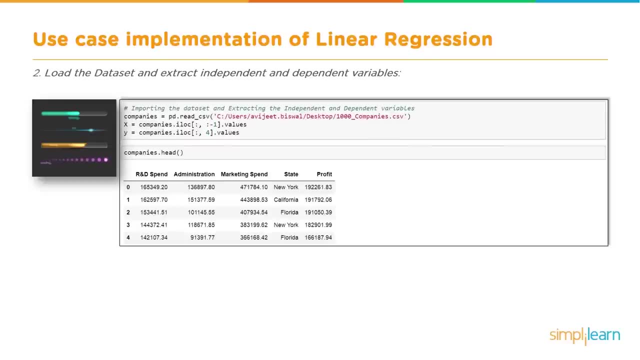 setting up variables. In fact, it's not going to do anything that we can see, but it is importing these different libraries and setup. The next step is load the data set and extract independent and dependent variables. Now here in the slide you'll see companies equals. 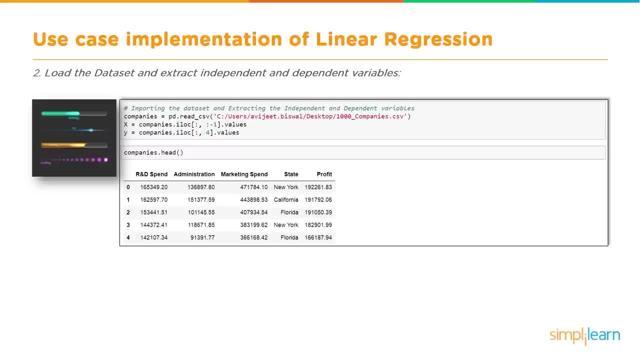 pdreadcsv and it has a long line there with the file at the end 1000companiescsv. You're going to have to change this to fit whatever setup you have And the file itself you can request. Just go down to the commentary below this video and put a note in there and simply. 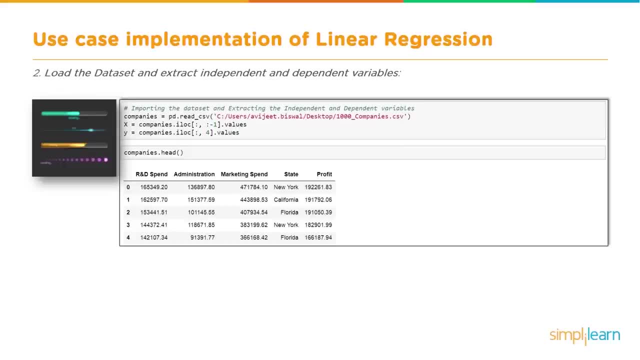 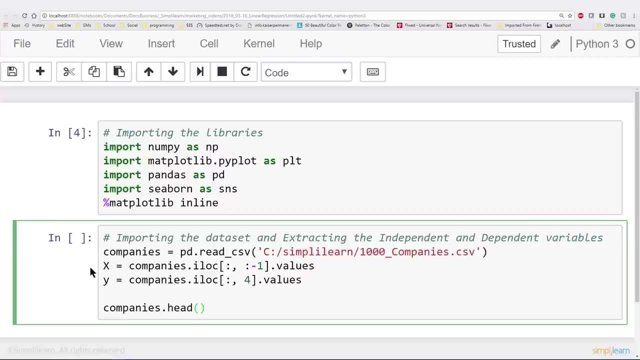 learn, we'll try to get in contact with you and supply you with that file so you can try this coding yourself. So we're going to add this code in here and we're going to see that they have companies equals pdreadcsv, and I've changed this path to match my computer. 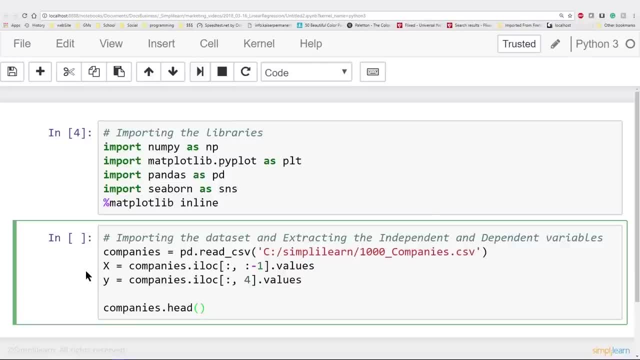 c colon slash, simply learn. slash 1000 underscore companies, dot, csv. And then below there we're going to set the x equals to companies under the i location and because this is companies is a pd data set, I can use this nice notation that says: take every row. that's what the 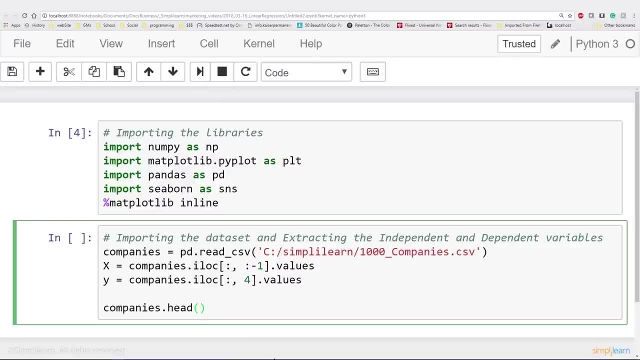 colon. the first colon is comma, except for the last column. That's what the second part is, where we have a colon minus one, values set into there. So x is no longer a data set, a pandas data set, but we can easily extract. 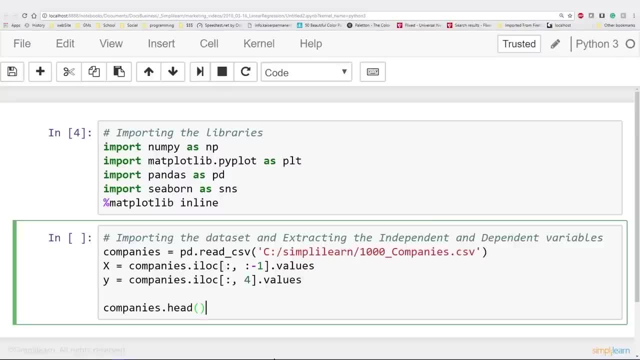 the data from our pandas data set with this notation, And then y we're going to set equal to the last row. Well, the question is going to be: what are we actually looking at? So let's go ahead and take a look at that, and we're going to look at the companieshead, which lists the first five rows of. 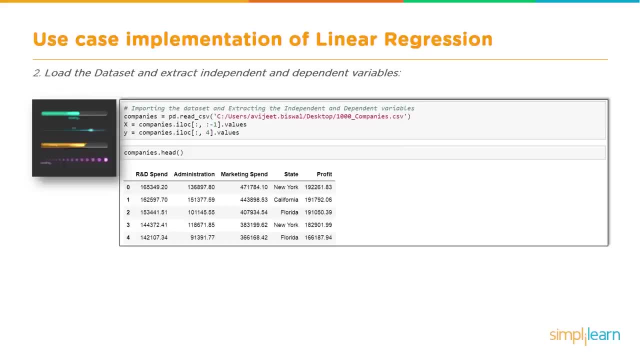 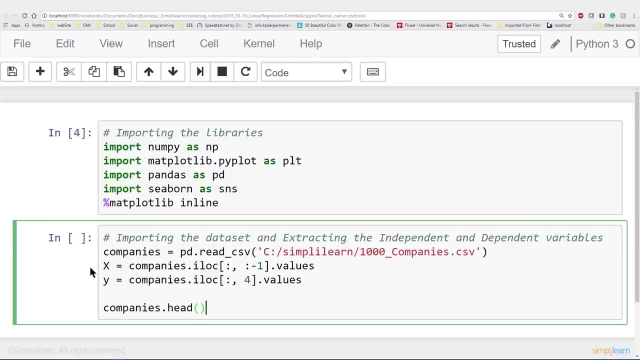 SimplyLearn will try to get in contact with you and supply you with that file so you can try this coding yourself. So we're going to add this code in here and we're going to see that I have companies equals pdreadercsv and I've 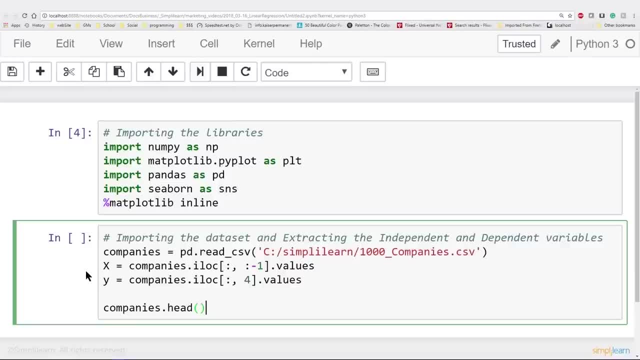 changed this path to match my computer C colon: slash, SimplyLearn. slash 1000 underscore companies, dot, csv, And then below there we're going to set the x equals to companies under the i location, And because this is companies is a pd data set, I can use this nice notation that says: take every row, that's what the colon. 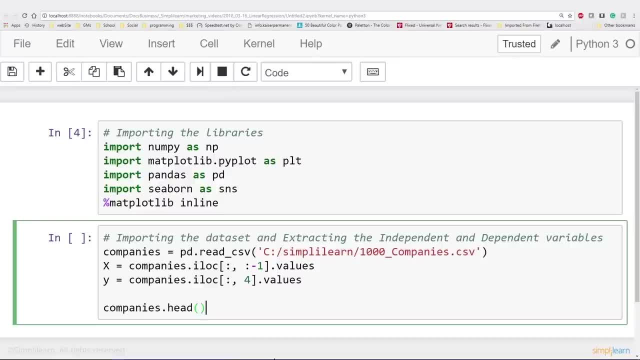 the first colon is comma, except for the last column. That's what the second part is, where we have a colon minus one And we want the values set into there. So x is no longer a data set, a pandas data set, But we can easily extract the data from our pandas. 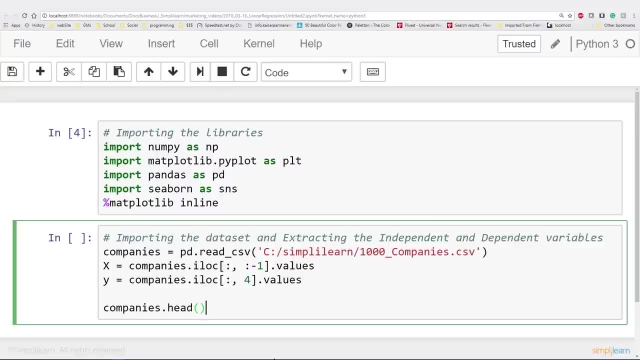 data set with this notation And then y we're going to set equal to the last row. Well, the question is going to be: what are we actually looking at? So let's go ahead and take a look at that, And we're going to look at the companies dot head, which lists the first five rows of data. 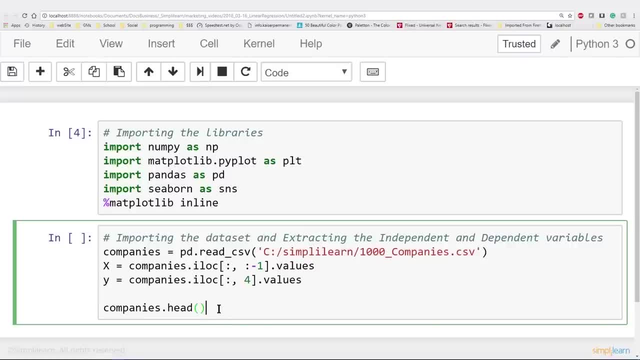 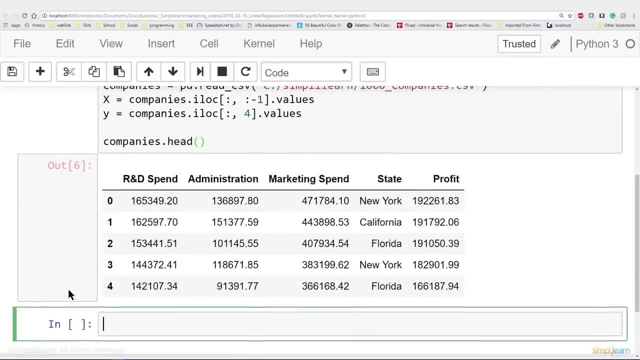 And I'll open up the file in just a second so you can see where that's coming from. But let's look at the data in here. as far as the way the pandas sees it, When I hit run, you'll see it breaks it out into a nice setup. This is what pandas- one of the things pandas is really good about- 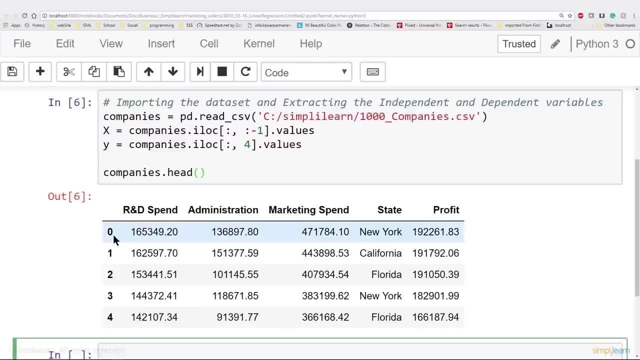 It looks just like an Excel spreadsheet. You have your rows And remember, when we're programming, we always start with zero, We don't start with one. So it shows the first five rows, It shows your columns. So, as you can see here, the first one is two. 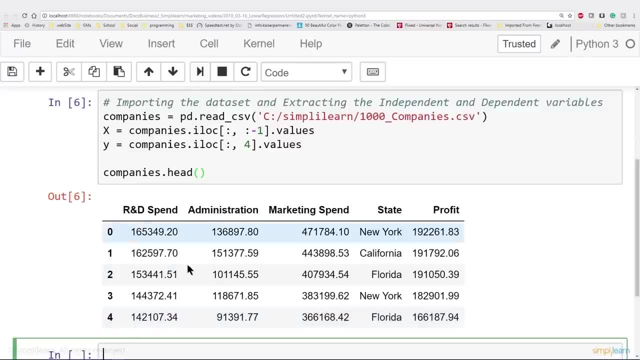 and then the second is zero, one, two, three, four, And then it shows your different columns- rn d, spend, administration, marketing spend, state profit- and even notes that the top are column names. It was never told that, but pandas is able to recognize a lot of things, that they're not the same as the data rows. 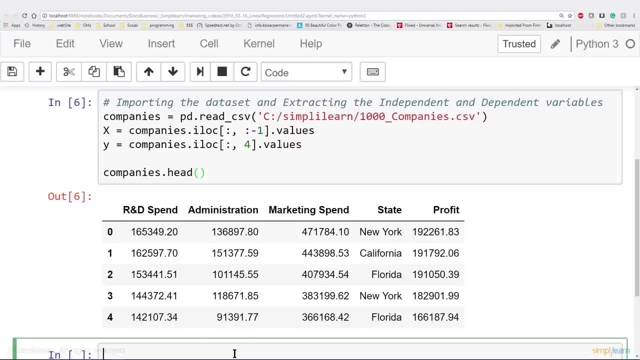 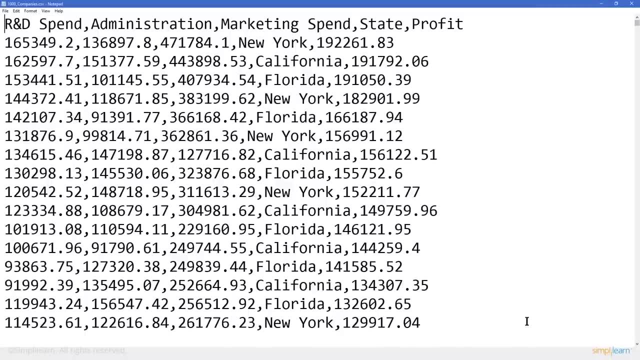 Why don't we go ahead and open this file up in a CSV so you can actually see the raw data? So here I've opened it up as a text editor And you can see at the top we have r n d spend. 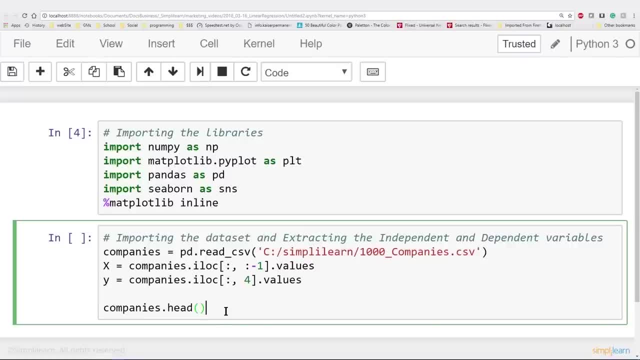 data And I'll open up the file in just a second so you can see where that's coming from. But let's look at the data in here as far as the way the pandas sees it, When I hit run, you'll see it breaks. 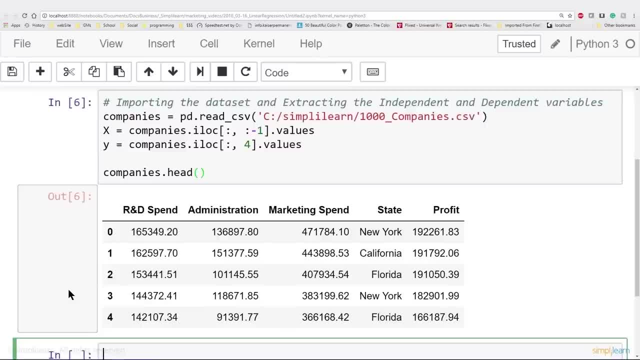 it out into a nice setup. This is what pandas- one of the things pandas is really good about- is it looks just like an excel spreadsheet. You have your rows and remember: when we're programming, we always start with zero, We don't start with one. So it shows the first five rows 0, 1, 2, 3, 4 and then 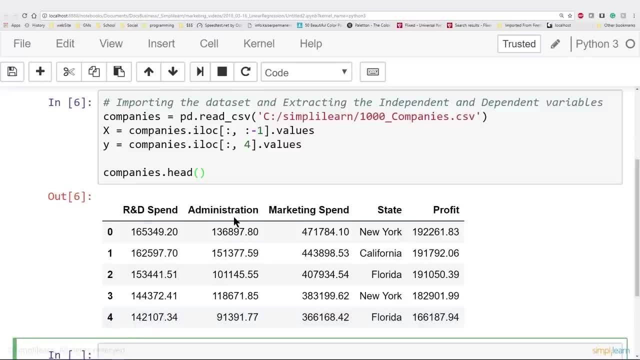 it shows your different columns: R&D spend, administration, marketing spend, state profit. It even notes that the top are column names. It was never told that, but pandas is able to recognize a lot of things that they're not the same as the data rows. Why don't we go ahead and open this file up in a CSV so you can? 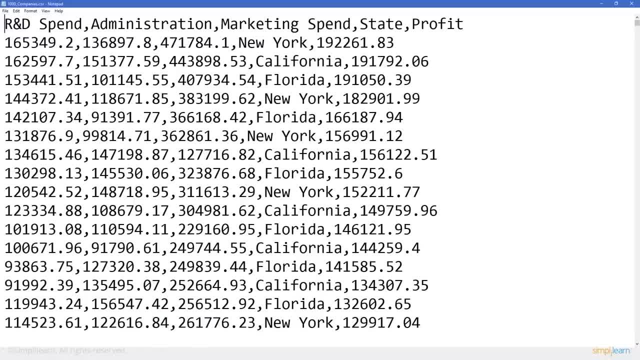 actually see the raw data. So here I've opened it up as a text editor and you can see at the top we have R&D spend comma, administration comma, marketing spend comma, state comma, profit carries, return. I don't know about you, but I'd go crazy trying to read files like this. That's why we use the pandas. 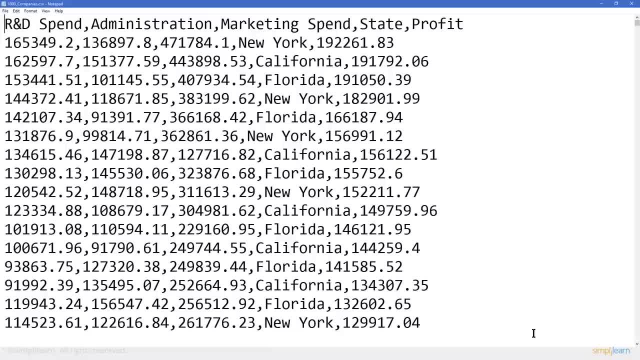 You could also open this up in an excel and it would separate it, since it is a comma separated variable file. But we don't want to look at this one. We want to look at something we can read rather easily. So let's flip back and take a look at that top part, the first. 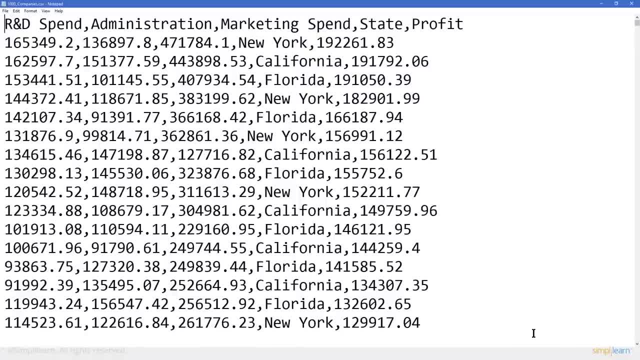 spend comma state comma profit carries return. I don't know about you, but I'd go crazy trying to read files like this. That's why we use the pandas. You could also open this up in an Excel and it would separate it, since it is a comma separated variable file. But we don't want to look at this. 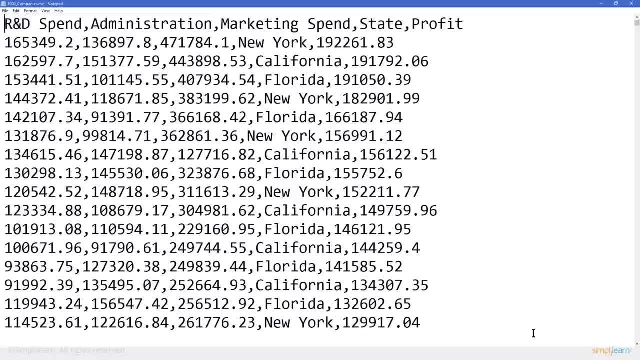 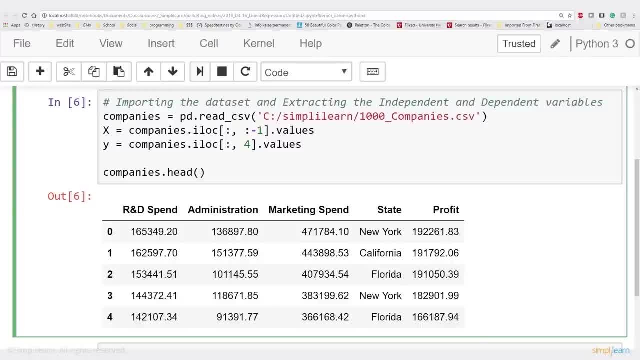 one. We want to look at something we can read rather easily. So let's flip back and take a look at that top part, the first five rows. Now, as nice as this format is where I can see the data, to me it doesn't mean a whole lot. Maybe you're an expert in business and investments and you understand. 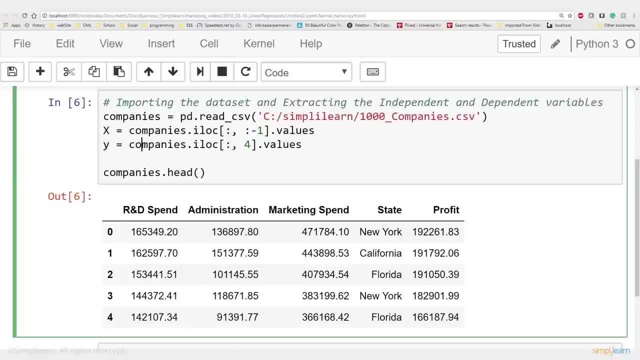 what? $165,349.20 compared to the administration cost of $136,897.80, so on and so on, helps to create the profit of $192,261.83.. That makes no sense to me whatsoever. no pun intended. So let's. 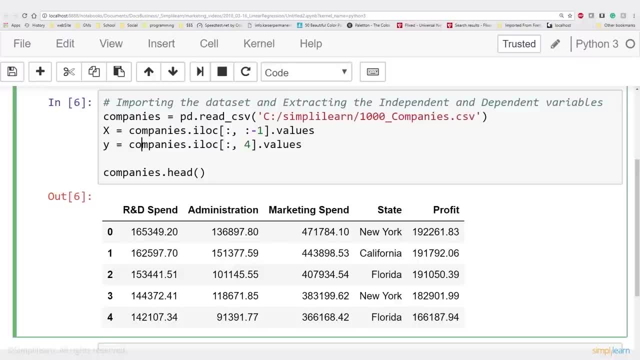 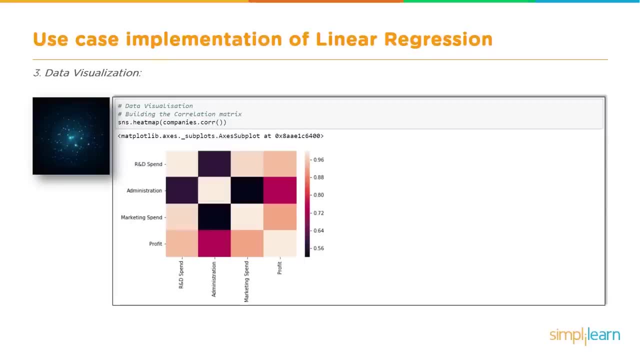 flip back here and take a look at our next set of code, where we're going to graph it so we can get a better understanding of our data and what it means. So at this point, we're going to use a single line of code To get a lot of information. so we can see where we're going with this, Let's go ahead and paste. 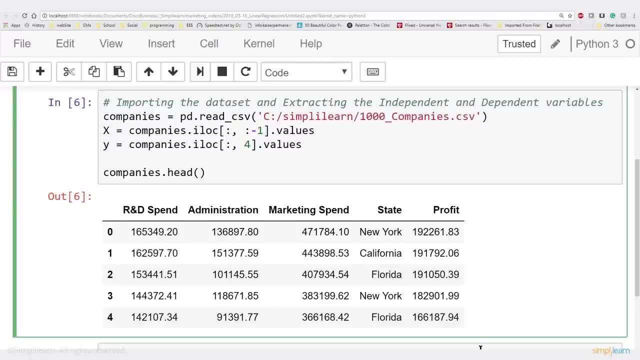 five rows. Now, as nice as this format is where I can see the data, to me it doesn't mean a whole lot. Maybe you're an expert in business and investments and you understand what. $165,349.20 compared to the administration cost of $136,897.80. so on, so on. It helps to create the. 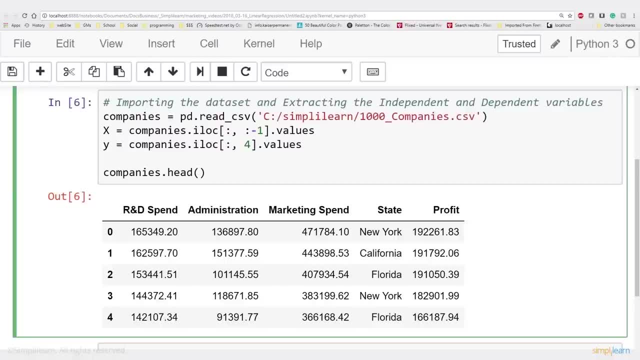 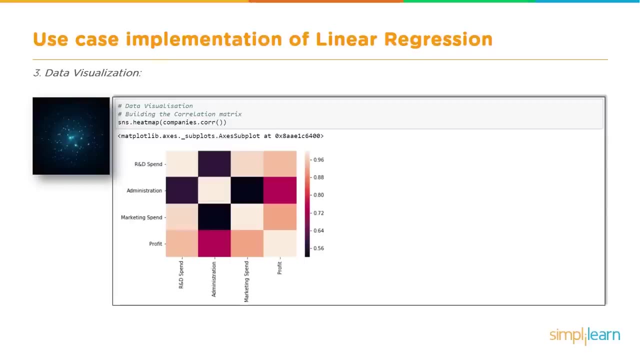 profit of $192,261.83.. That makes no sense to me whatsoever, No pun intended. So let's flip back here and take a look at our next set of code, where we're gonna graph it so we can get a better understanding of our data and what it means. So at this point we're gonna use a single line of code. 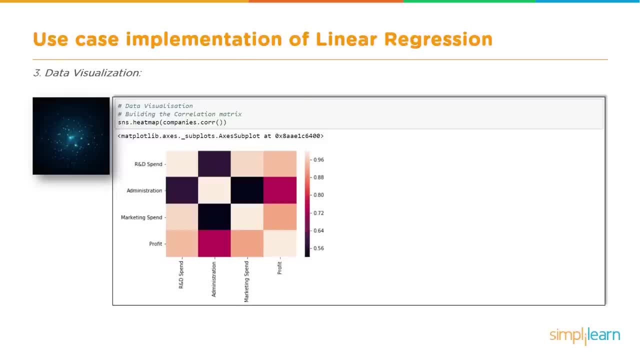 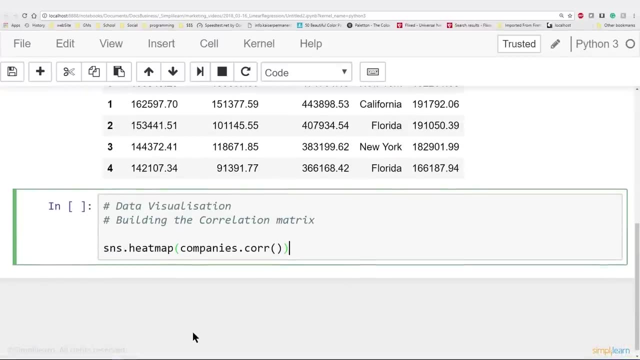 to get a lot of information. so we can see where we're going with this. Let's go ahead and paste that into our notebook and see what we got going, And so we have the visualization and again we're going to use a single line of code to get a lot of information. So what we're going to do is we're 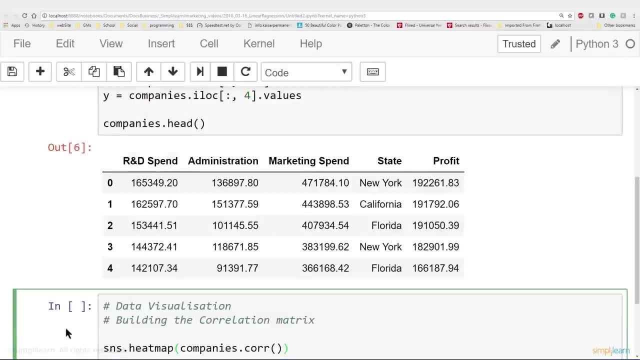 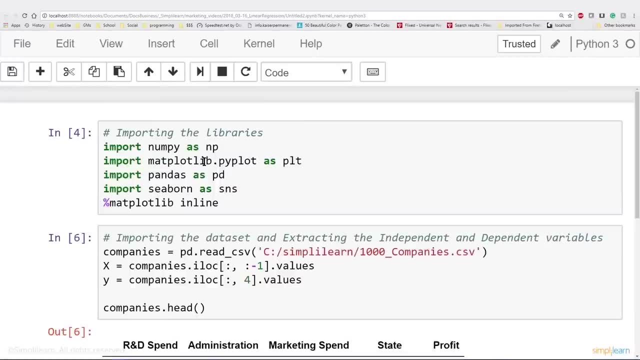 that into our notebook and see what we got going. And so we have the visualization and again we're using SNS, which is pandas. As you can see, we imported the matplotlibrarypyplot as PLT, which then the seaborn uses, And we imported the seaborn as SNS, And then that final line of code helps us. 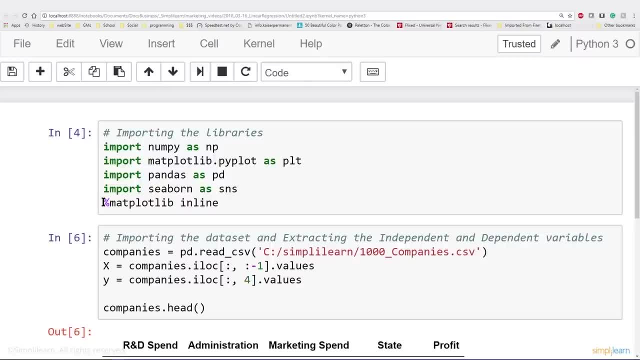 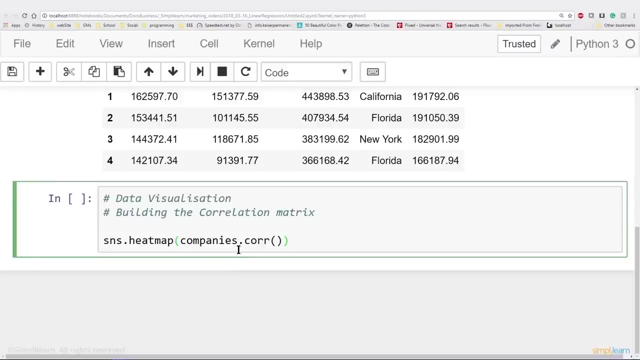 show this in our inline coding. Without this it wouldn't display and you could display it to a file And that's the matplotlibrary inline with the amber sign at the beginning. So here we come down to the single line of code. Seaborn is great because it actually recognizes the panda data frame, So I can just take the companiescore for coordinates. 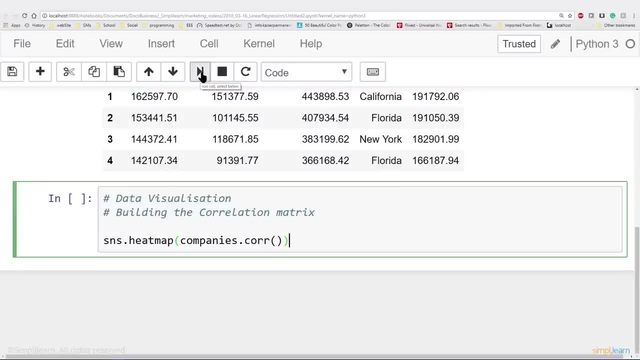 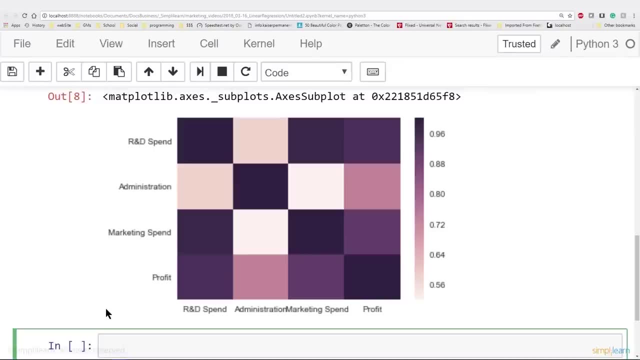 and then put that right into the seaborn. And when we run this, we get this beautiful plot. And let's just take a look at what this plot means. If you look at this plot on mine, the colors are probably a little more purplish and blue than the original one. We have the columns and the rows. 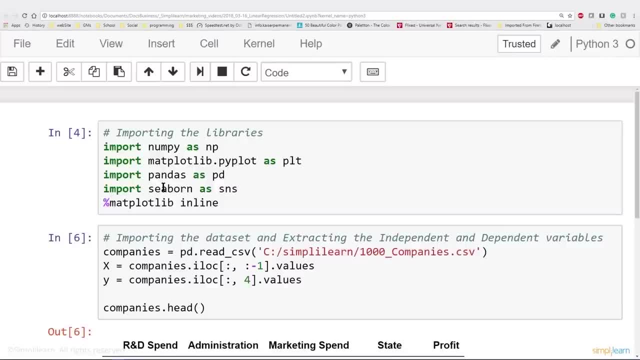 going to import the matplot librarypyplot as plt, which then the seaborn uses, And we imported the seaborn as sns, And then that final line of code helps us show this in our inline coding. Without this it wouldn't display and you could display it to a file and other means And that's the matplot. 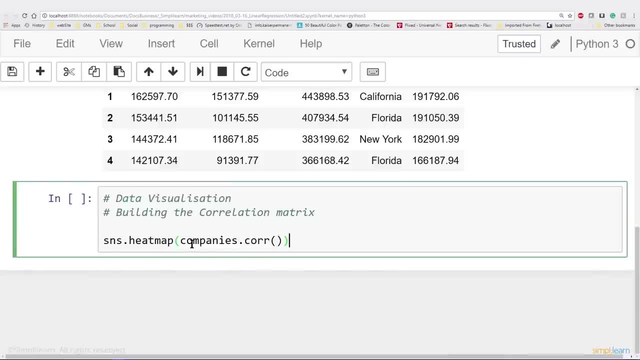 library inline with the amber sign at the beginning. So here we come down to the single line of code. Seaborn is great because it actually recognizes the panda data frame. So we're going to go to companiescore for coordinates And I can put that right into the seaborn. 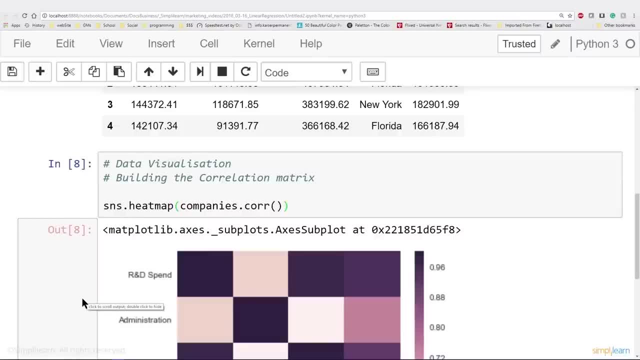 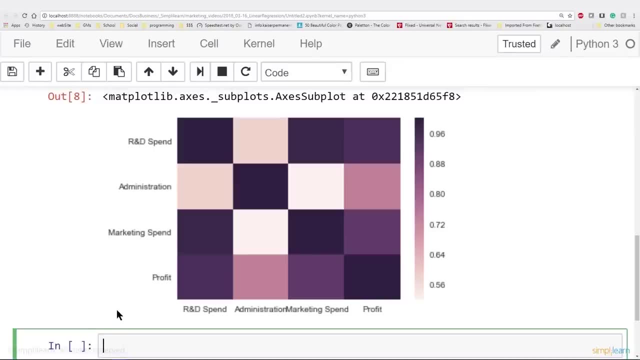 And when we run this, we get this beautiful plot. And let's just take a look at what this plot means. If you look at this plot on mine, the colors are probably a little bit more purplish and blue than the original one. We have the columns and the rows, We have r and d spending, We have administration. 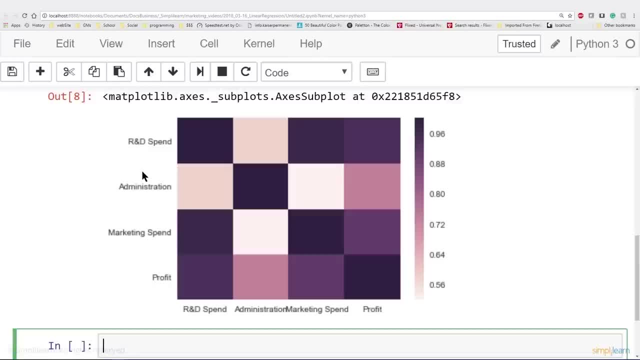 We have marketing spending and profit, And if you cross index any two of these, since we're interested in profit- If you cross index profit with profit, it's going to show up If you look at the scale on the right way up in the dark. Why? Because those are the same data. 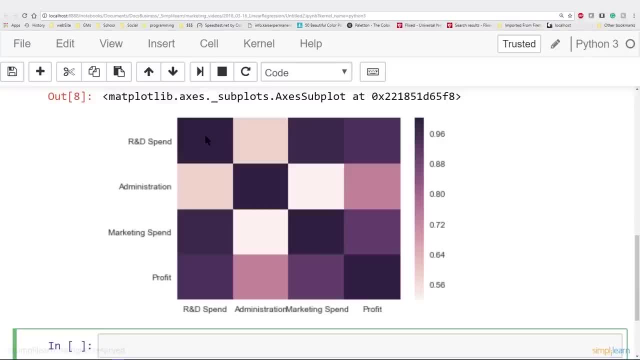 They have an exact correspondence. So r and d spending is going to be the same as r and d spending and the same thing with administration costs are. right down the middle You get this dark row, or dark diagonal row that shows that this is the highest corresponding data. that's exactly the same. 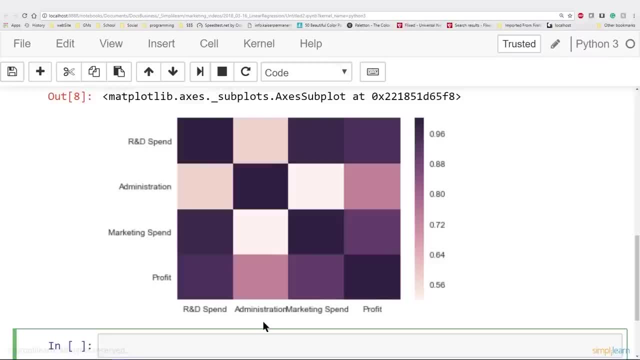 And as it becomes lighter, there's less connections between the data, So we can see with profit. And next it has a very high correlation with r and d spending, Which we looked at earlier, And it has a slightly less connection to marketing spending and even less to how much money we put. 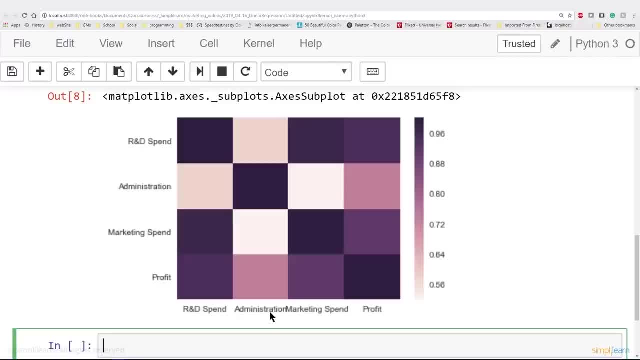 into the administration. So now that we have a nice look at the data, let's go ahead and dig in and create some actual useful linear regression models so that we can predict values and have a better profit. Now that we've taken a look at the visualization of this data, we're going 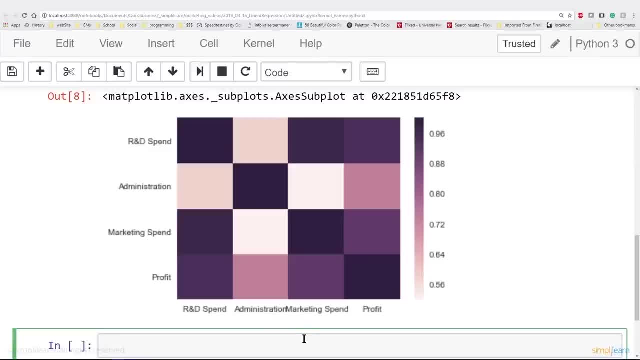 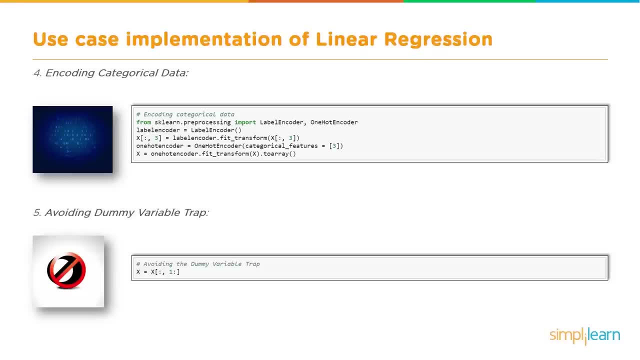 to move on to the next step. Instead of just having a pretty picture, we need to generate some hard data, Some hard values. So let's see what that looks like. We're going to set up our linear regression model in two steps. The first one is we need to prepare some of our 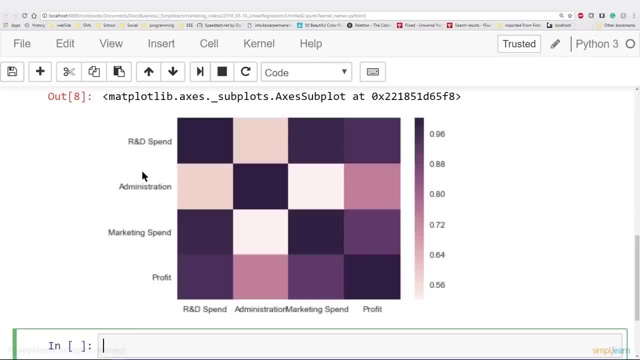 is: we have R&D spending, we have administration, we have marketing spending and profit. And if you cross-index any two of these- since we're interested in profit- if you cross-index profit with profit, it's going to show up if you look at the scale on the right way up in the dark. Why? Because those 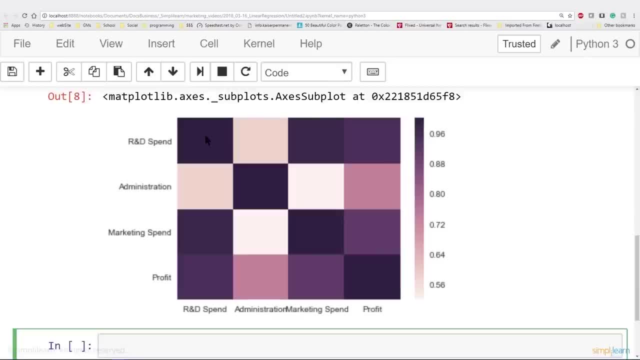 are the same data. They have an exact correspondence. So R&D spending is going to be the same as R&D spending and the same thing with administration costs. Right down the middle you get this dark row, or dark diagonal row that shows that this is the highest corresponding data. It's exactly the. 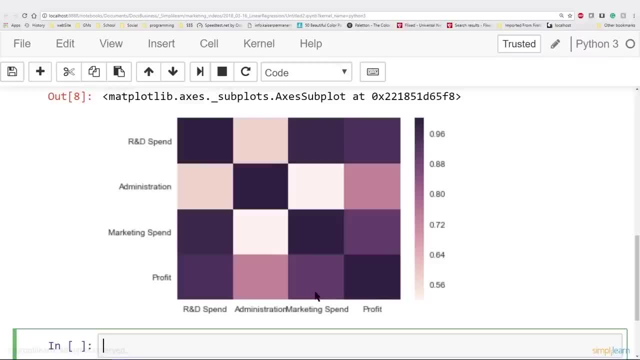 same And as it becomes lighter there's less connections between the data. So we can see: with profit, obviously profit is the same as profit And next it has a very high correlation with R&D spending, which we looked at earlier, And it has a slightly less connection to marketing spending. 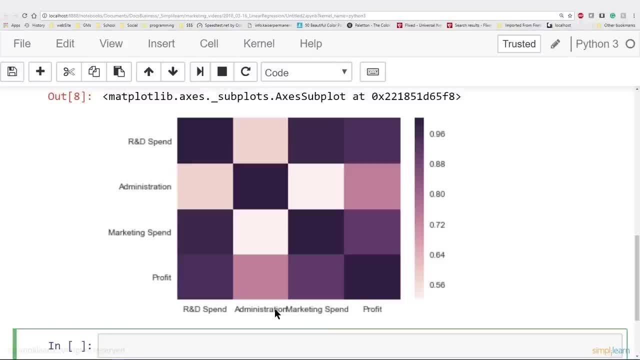 and even less to how much money we put into the administration. So, now that we have a nice look at the data, let's go ahead. Let's go ahead and dig in and create some actual useful linear regression models so that we can predict values and have a better profit Now that we've taken a look at the visualization of this. 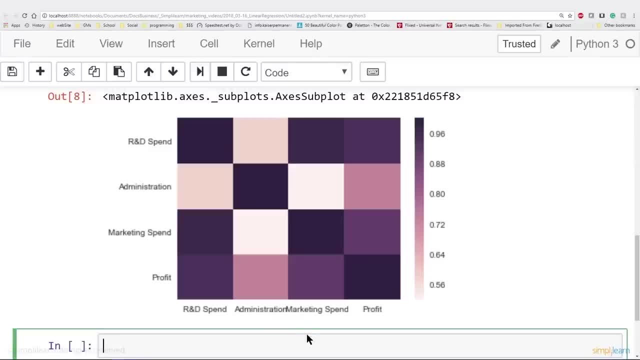 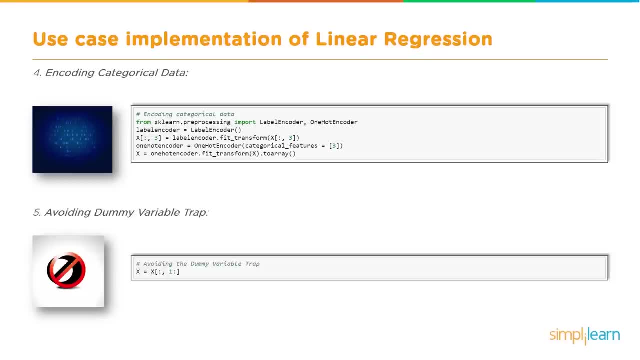 data. we're going to move on to the next step. Instead of just having a pretty picture, we need to generate some hard data, some hard values. So let's see what that looks like. We're going to set up our linear regression model in two steps. The first one is we need to prepare some of our data. 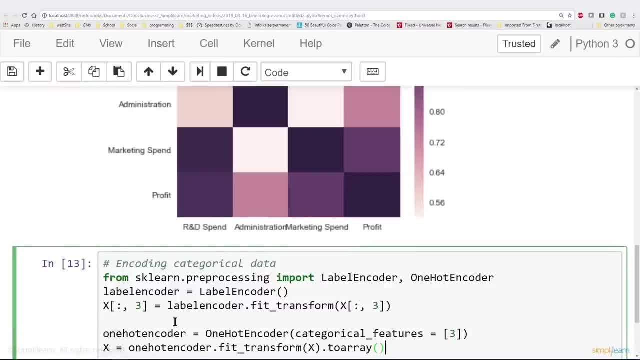 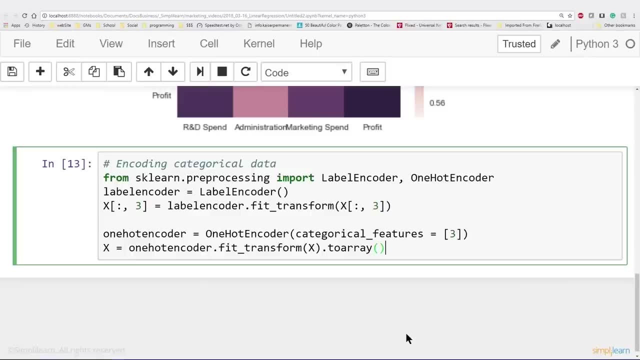 so it fits correctly. And let's go ahead and paste this code into our Jupyter notebook. And what we're bringing in is we're going to bring in the sklearn preprocessing, where we're going to import the label encoder and the one hot encoder To use the label encoder. we're going to create a variable. 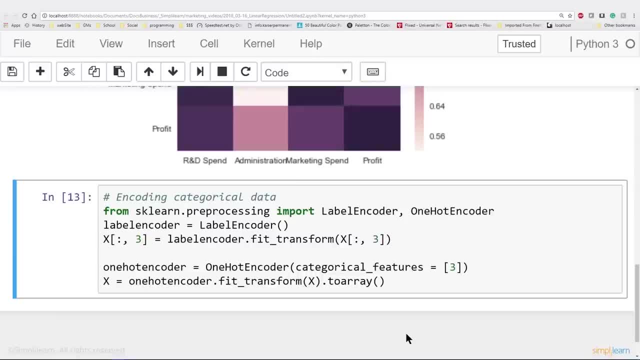 called label encoder and set it equal to capital L label capital E encoder. This creates a class that we can reuse for transferring the labels back and forth. Now about now, you should ask: what labels are we talking about? Let's go take a look at the data we processed before and see what I'm. 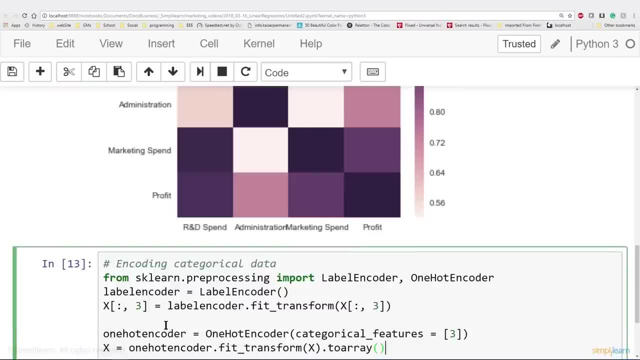 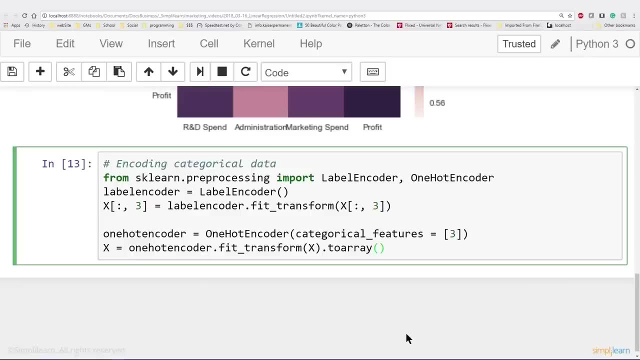 data so it fits correctly. And let's go ahead and paste this code into our Jupyter notebook. And what we're bringing in is we're going to bring in the sklearn pre-processing Where we're going to import the label encoder and the one hot encoder To use the label encoder. 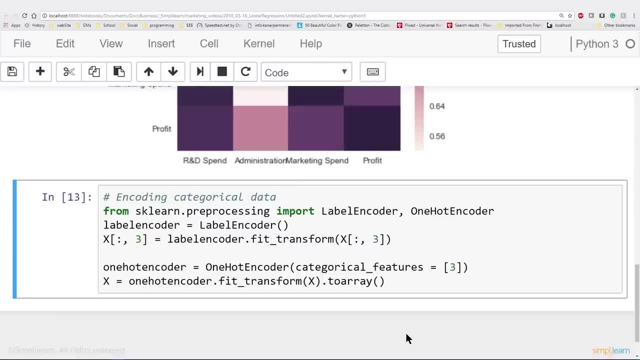 we're going to create a variable called label encoder and set it equal to capital L, capital E encoder. This creates a class that we can reuse for transferring the labels back and forth. Now about now, you should ask: what labels are we talking about? Let's go take a look at the 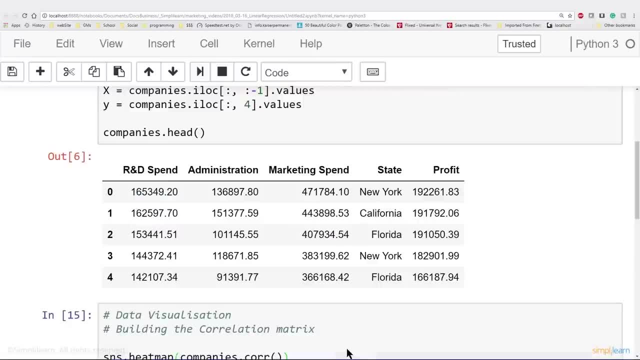 data we processed before and see what I'm talking about here. If you remember, when we did the companieshead, we printed the top five rows of data. We have our columns going across. We have column zero, which is R&D spending, Column one, which is administration, Column two, which is 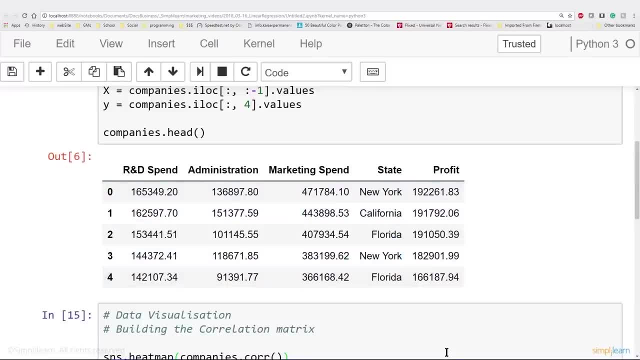 marketing spending. And column three is state, And you'll see that we have a lot of data Under state. we have New York, California, Florida, Now to do a linear regression model. it doesn't know how to process New York. It knows how to process a number. So the first thing we're going 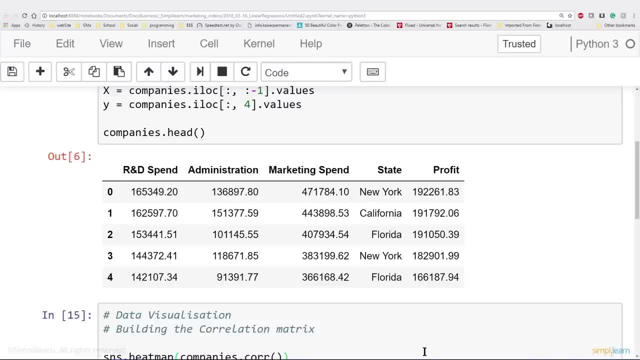 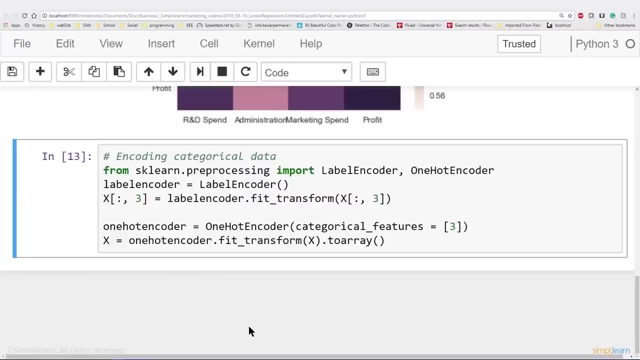 to do is we're going to change that- New York, California and Florida- and we're going to change those to numbers. That's what this line of code does. here X equals, and then it has the colon comma, three in brackets. The first part. the colon comma, means that we're going to look at all the 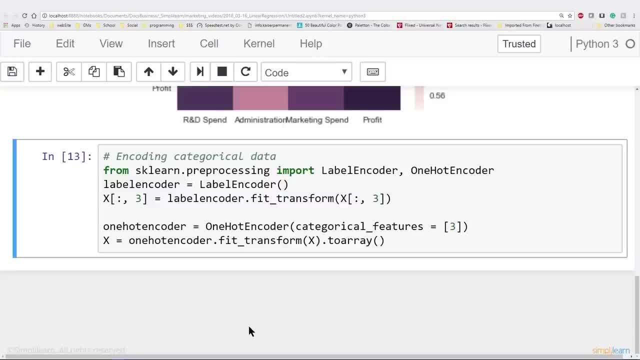 different rows, So we're going to keep them all together. But the only row we're going to edit is the third row And in there we're going to take the label coder and we're going to fit and transform the X- also the third row. So we're going to take that third row. We're going to set it equal to a. 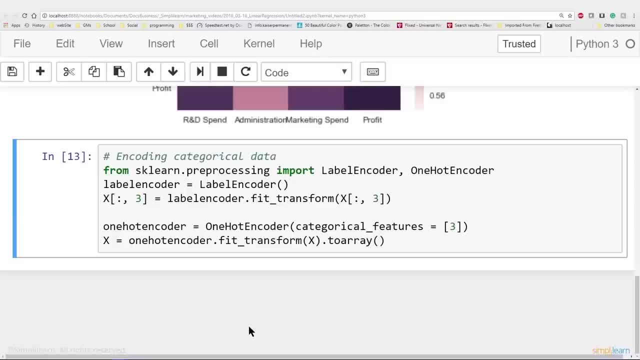 transformation, And that transformation basically tells it that instead of having a New York, it has a zero, or one or a two. And then, finally, we need to do a one hot encoder which equals one hot encoder categorical features, equals three. And then we take the X and we go ahead and do that equal to one hot. 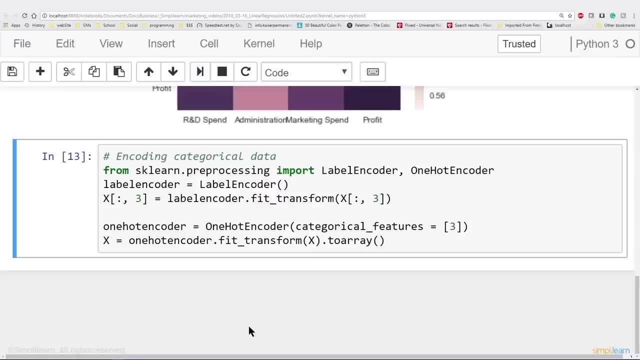 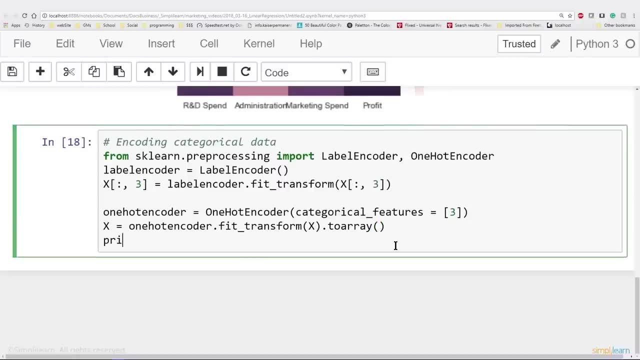 encoder, fit, transform X, So we're going to take the X and we're going to set it equal to array. This final transformation preps our data for us, so it's completely set the way we need it. It's just a row of numbers, Even. 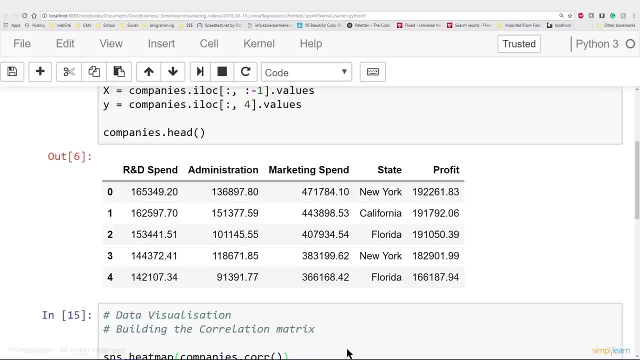 talking about here. If you remember, when we did the companieshead and we processed the labels, we printed the top five rows of data. We have our columns going across. We have column 0,, which is R&D spending, Column 1,, which is administration, Column 2,, which is marketing spending, And column 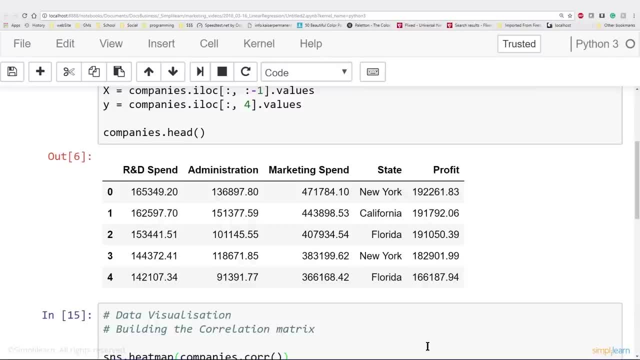 3 is state And you'll see, under state we have New York, California, Florida. Now to do a linear regression model, it doesn't know how to process New York, It knows how to process a number. So the first thing we're going to do is we're going to change that: New York, California and Florida. 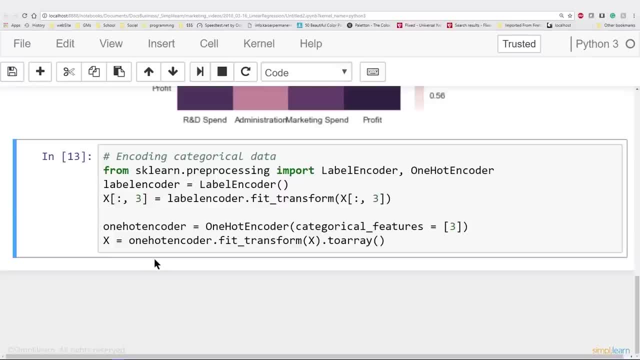 and we're going to change those to numbers. That's the first thing we're going to do is we're going to change that New York, California and Florida and we're going to change those to numbers. That's what this line of code does. here X equals, and then it has the colon comma 3 in brackets The. 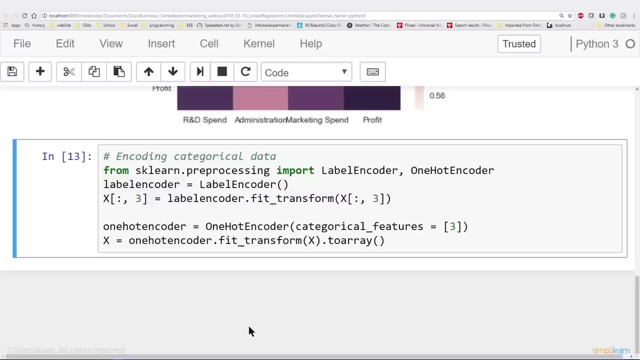 first part. the colon comma means that we're going to look at all the different rows, So we're going to keep them all together. But the only row we're going to edit is the third row And in there we're going to take the label coder and we're going to fit and transform the X, also the third. 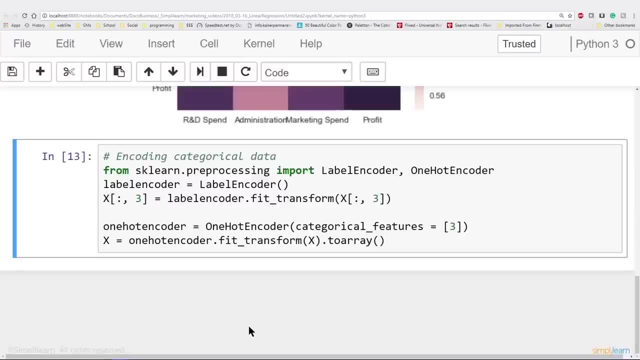 row. So we're going to take that third row, we're going to set it equal to a transformation And that transformation basically tells it that instead of having a New York, it has a Z or a 1, or a 2.. And then, finally, we need to do a one hot encoder which equals one hot encoder. 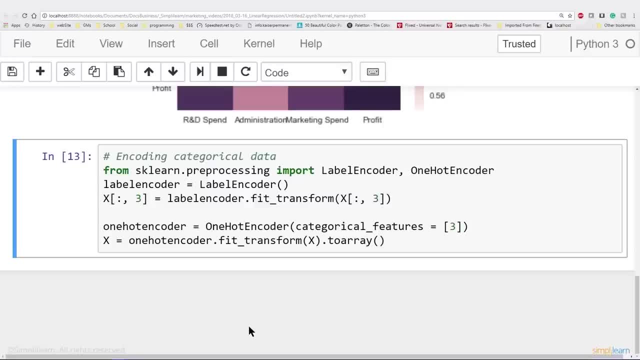 categorical features equals 3.. And then we take the X and we go ahead and do that. equal to one hot encoder, fit. transform X to array. This final transformation preps our data for us, so it's completely set the way. we need it as just a row of numbers. Even though it's not in here, let's go. 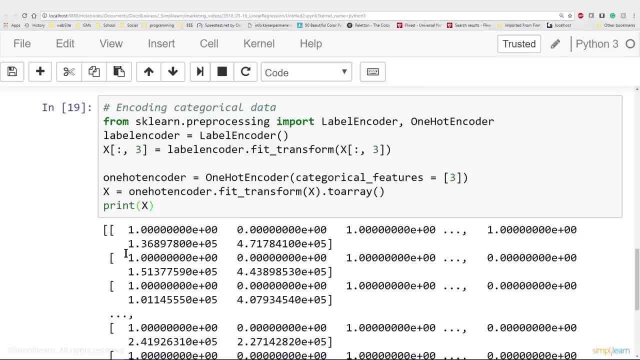 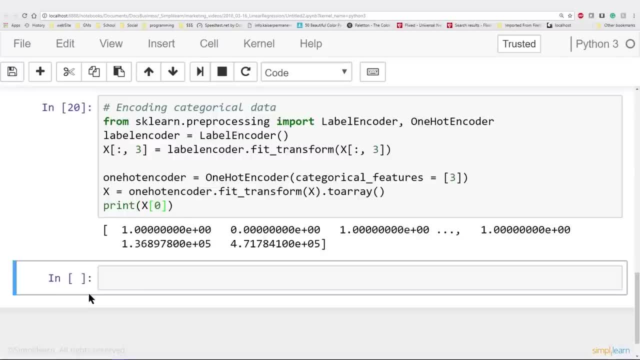 ahead and print X and just take a look at what this data is doing, You'll see you have an array of arrays and then each array is going to have an array of arrays And then each array is going to be a row of numbers. And if I go ahead and just do row zero, you'll see I have a nice organized. 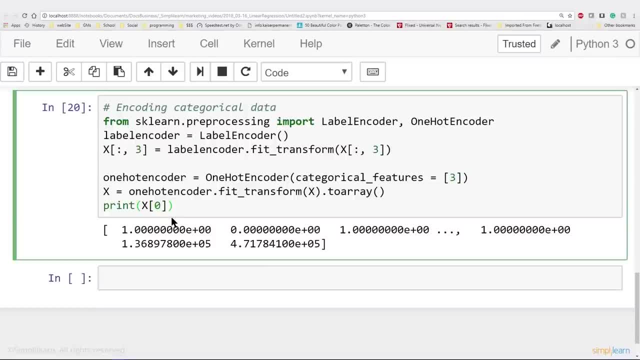 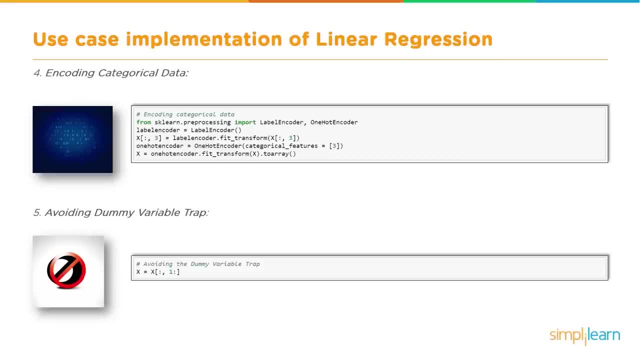 row of numbers that the computer now understands. We'll go ahead and take this out there, because it doesn't mean a whole lot to us. it's just a row of numbers. Next, on setting up our data, we have avoiding dummy variable trap. This is very important. Why? Because the computer has automatically 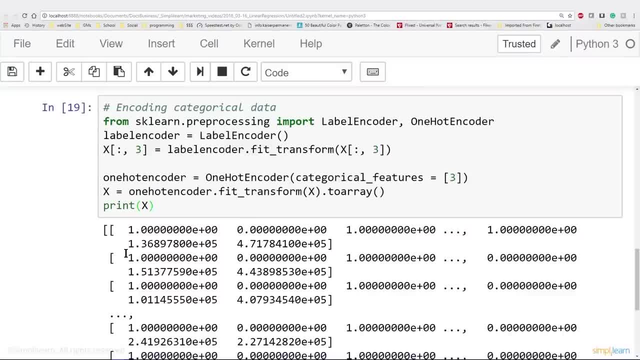 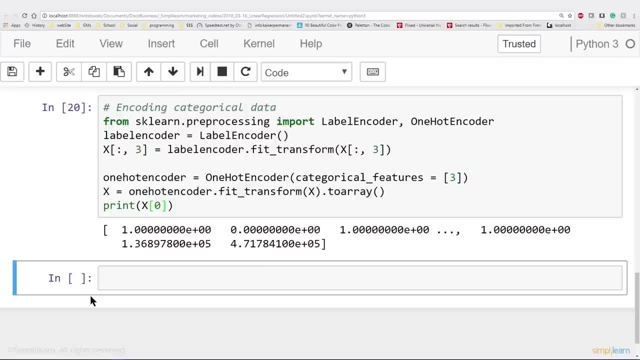 though it's not in here. let's go ahead and print X and just take a look at what this data is doing. You'll see you have an array of arrays and then each array is a row of numbers. And if I go ahead and just do row zero, you'll see I have a nice organized row of numbers that the computer now 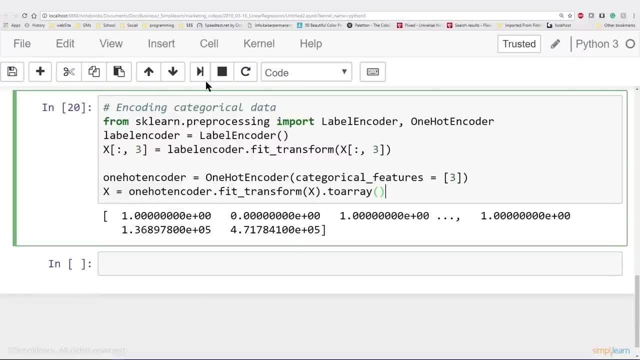 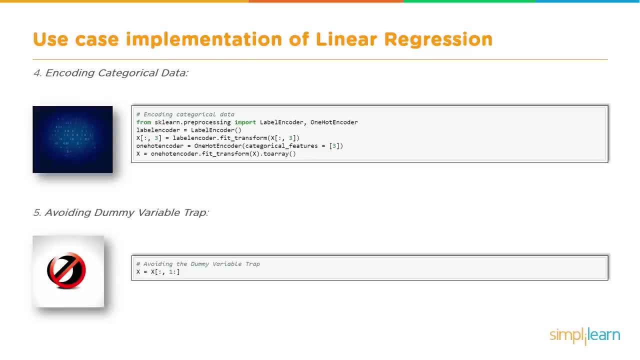 understands, We'll go ahead and take this out there, because it doesn't mean a whole lot to us. It's just a row of numbers And what we need to do is to take this array out there and then we do a little test test. We're going to take the X and we'll go ahead and paste those into our. 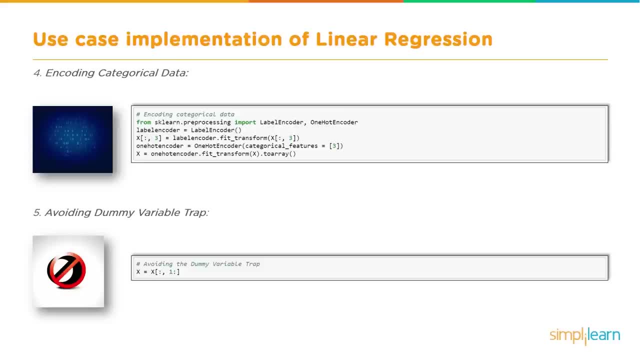 code And, as you'll notice, what you need to do is to take the X and you're going to go ahead and paste that into the data So that we can paste that into our code, And what we need to do is to run the same process. we're going to set it to two. we're going to pass the last row. 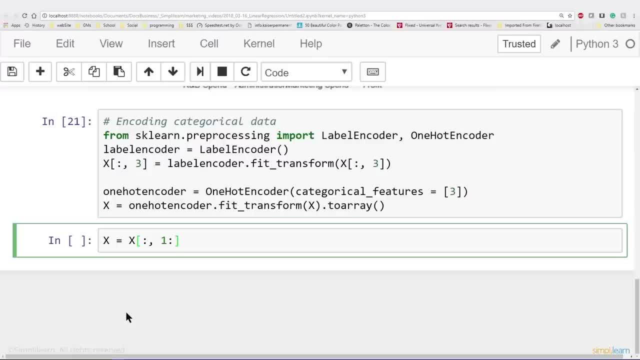 we're going to pass the last column and we're going to put the first row and then we're going one colon. All this is doing is removing that one extra column. we put in there when we did our one hot encoder and our label encoding. Let's go ahead and run that. And now we get. 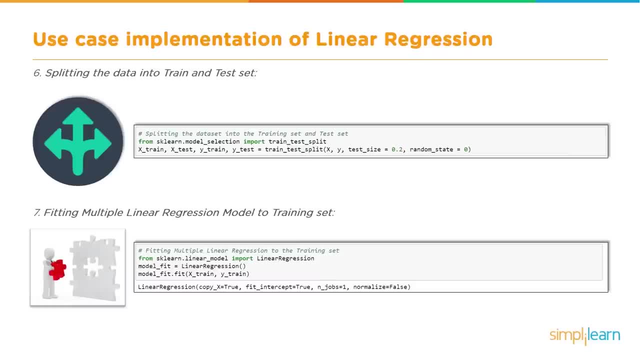 to create our linear regression model And let's see what that looks like here, And we're going to do that in two steps. The first step is going to be in splitting the data. Now, whenever we create a predictive model of data, we always want to split it up, so we have a 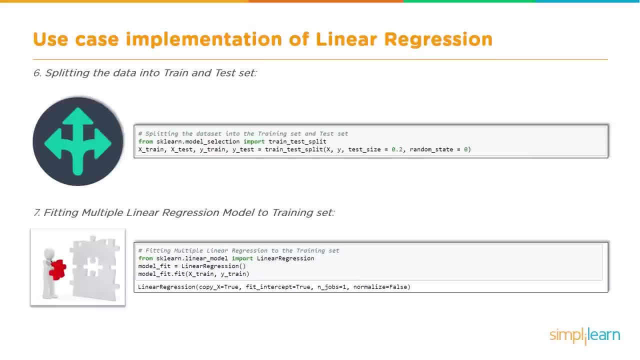 training set and we have a testing set. That's very important, otherwise we'd be very unethical- without testing it to see how good our fit is, And then we'll go ahead and create our multiple linear regression model and train it and set it up. Let's go ahead and paste. 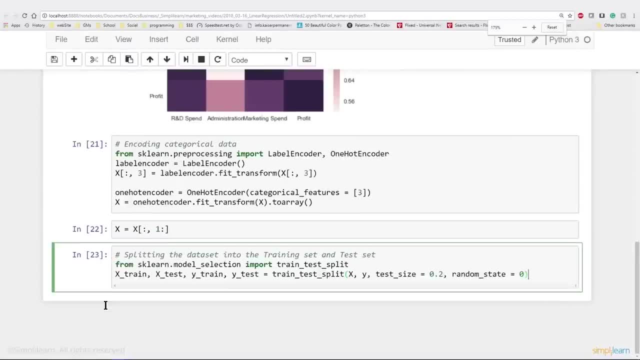 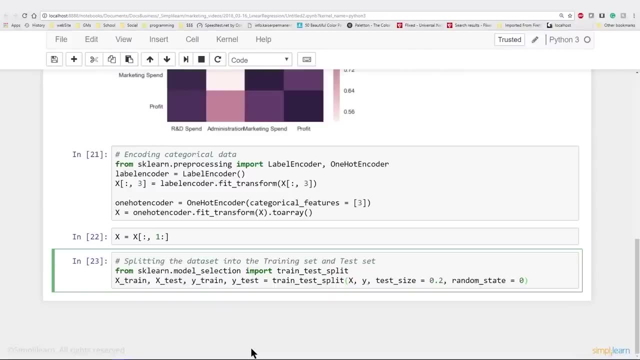 this next piece of code in here And I'll go ahead and shrink it down a size or two so it all fits on one line. So from the sklearn module selection we're going to import train test split And you'll see that we've created four completely different variables. We have 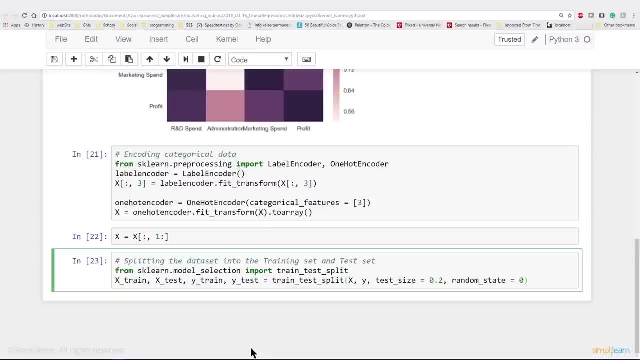 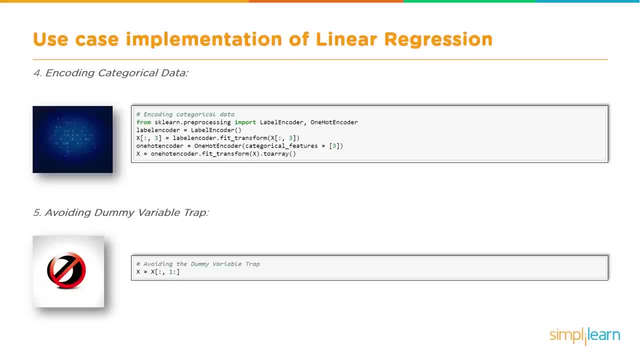 transformed our header into the setup and it's automatically transferred all these different variables. So, when we did the indexing, we did the indexing, we did the numbering, we did the encoder. The encoder created two columns And what we need to do is just have the one, because it 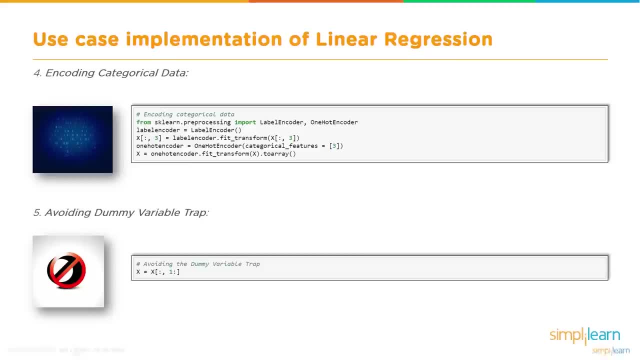 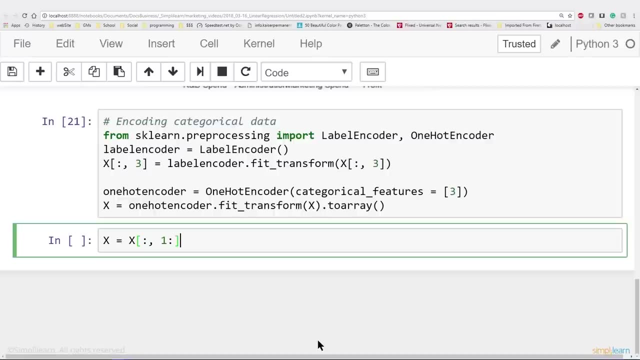 has both the variable and the name. That's what this piece of code does here. Let's go ahead and paste this in here and we have X equals X colon, comma, one colon. All this is doing is removing that one extra column we put in there when we did our one hot encoder and our label encoding. Let's go. 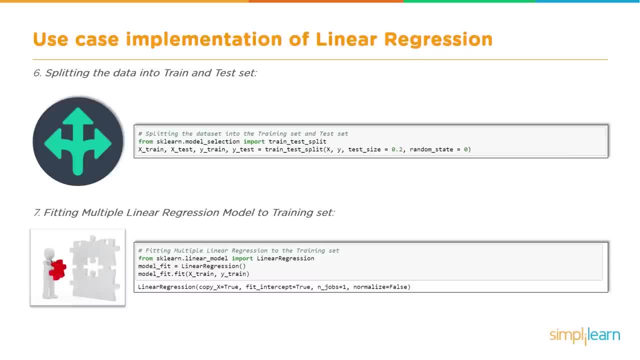 ahead and run that And now we get to create our linear regression model And let's see what that looks like here. So we're going to go ahead and split it up into two steps. The first step is going to be in splitting the data Now. 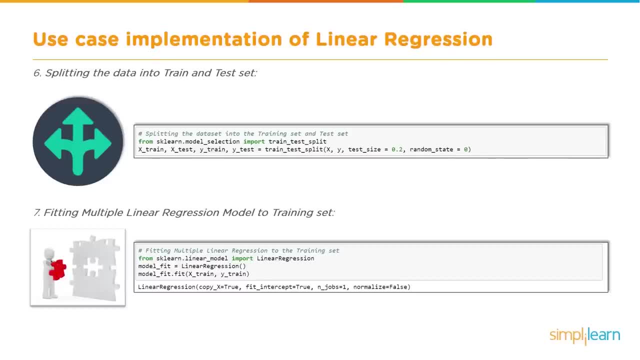 whenever we create a predictive model of data, we always want to split it up. so we have a training set and we have a testing set. That's very important, Otherwise we'd be very unethical without testing it to see how good our fit is. 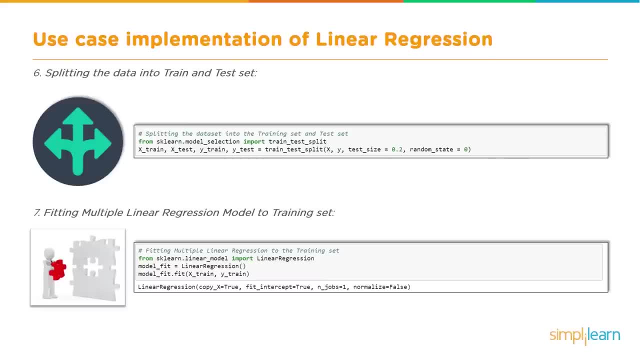 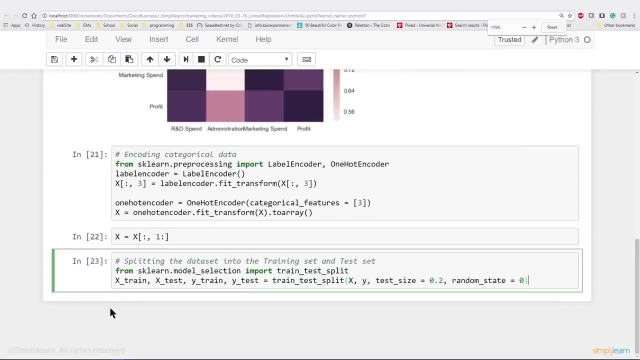 And then we'll go ahead and create our multiple linear regression model and train it and set it up. Let's go ahead and paste this next piece of code in here And I'll go ahead and shrink it down a size or two so it all fits on one. 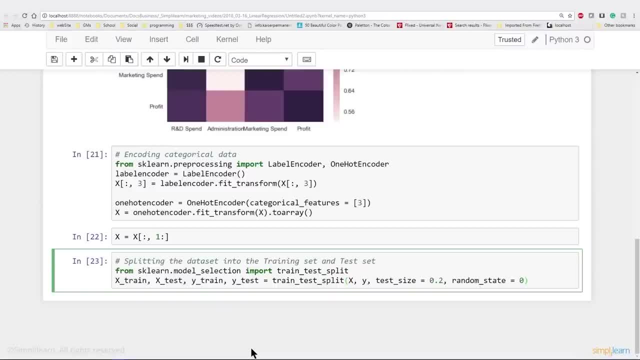 line. So from the sklearn model selection we're going to import train test split And you'll see that we created four completely different variables. We have capital X train, Capital X test, Smaller case y train, Smaller case y test. That is the standard way that they usually reference these when we're doing different models. 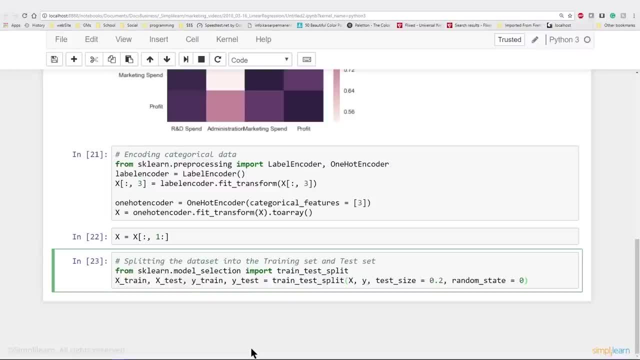 You usually see that as capital. X, You see the train and the test and the lower case, y, What this is. X is our data going in, That's our r index, dspin or administration or marketing, and then y, which we're training, is the answer, that's the. 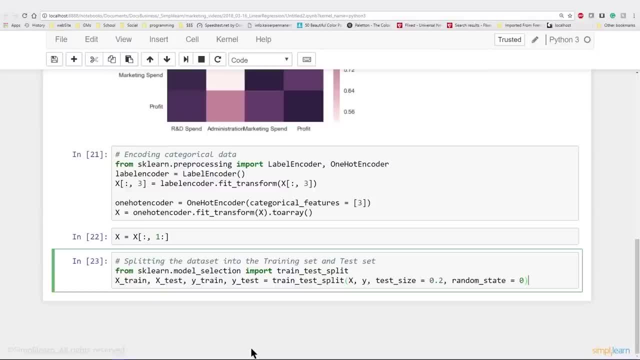 profit, because we want to know the profit of an unknown entity. that's what we're going to shoot for in this tutorial. the next part: train test split. we take x and we take y. we've already created those. x has the columns with the data in it and y has a column with profit in it, and then 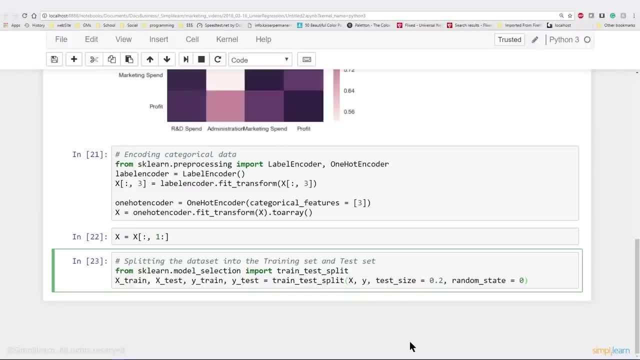 we're going to set the test size equals 0.2. that basically means 20 percent. so 20 percent of the rows are going to be tested. we're going to put them off to the side. so since we're using a thousand lines of data, that means that 200 of those lines we're going to hold off to the side to test for. 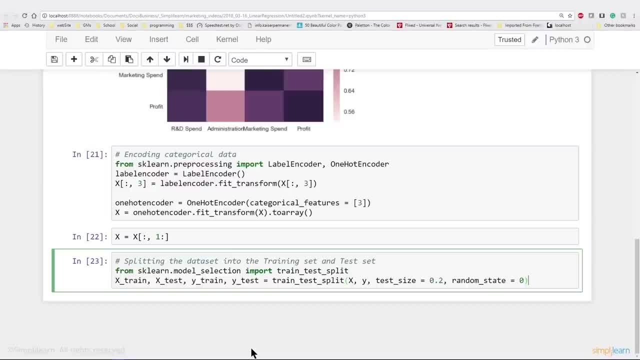 you see the train and the test and the lowercase y. What this is is: X- is our data going in, That's our R&D spin, our administration, our marketing. And then Y, which we're training, is the answer, That's the profit, Because we want to know the profit of an unknown entity. 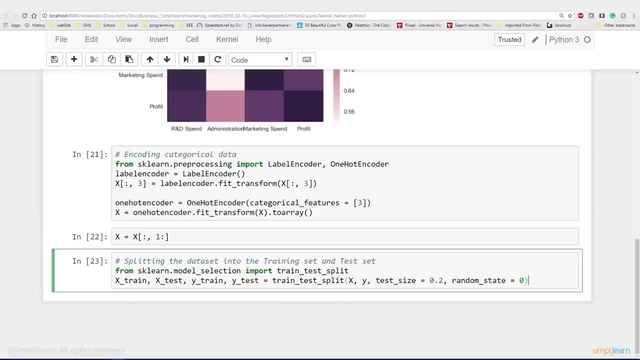 That's what we're going to shoot for in this tutorial. The next part: train test split. we take X and we take Y. We've already created those. X has the columns with the data in it and Y has a column with profit in it, And then 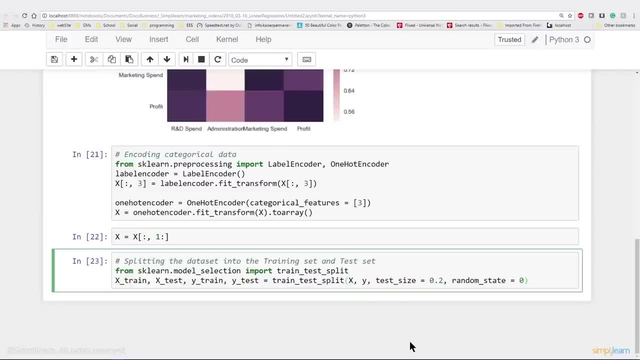 we're going to set the test size equals 0.2.. That basically means 20%. So 20% of the rows are going to be tested. We're going to put them off to the side. So since we're using a thousand lines of data, that means that 200 of those lines we're going to hold off. 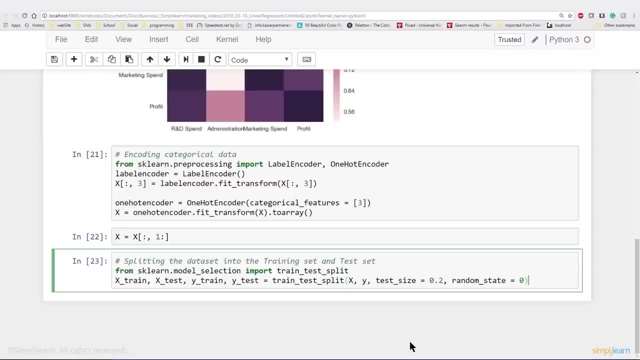 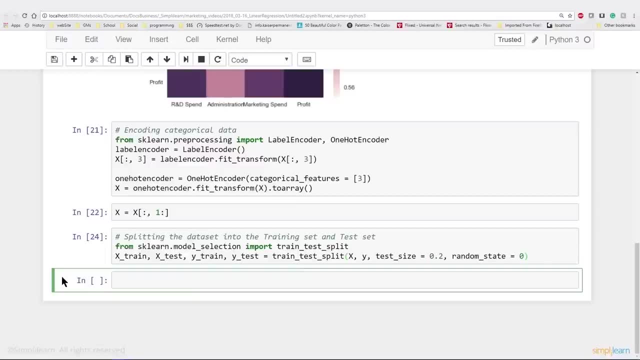 to the side to test for later. And then the random state equals zero. We're going to randomize which ones it picks to hold off to the side. We'll go ahead and run this. It's not overly exciting because it's setting up our variables. But the next. 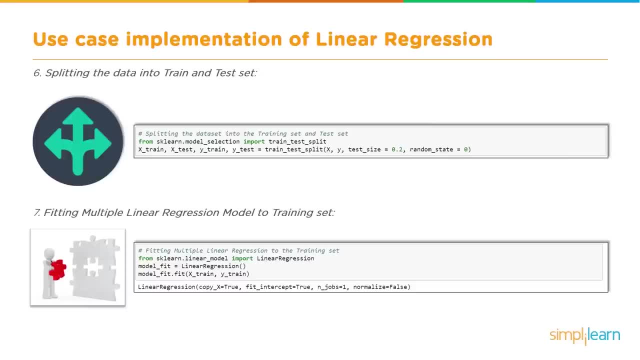 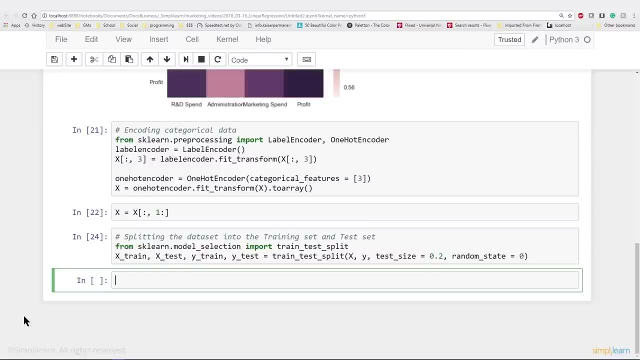 step is the next step. we actually create our linear regression model. Now that we got to the linear regression model, we get that next piece of the puzzle. Let's go ahead and put that code in there and walk through it. So here we go, We're going to paste it in. 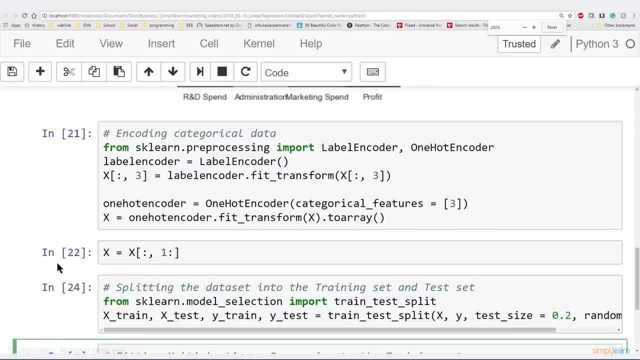 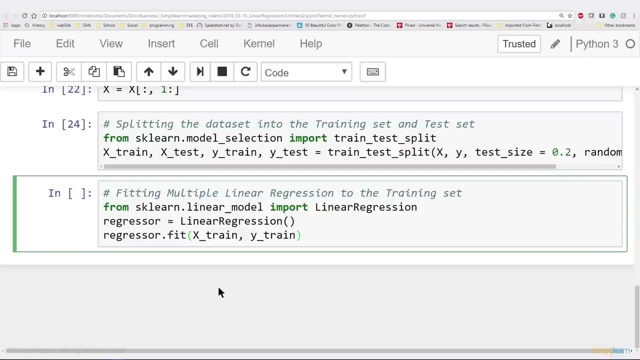 there And let's go ahead. and since this is a shorter line of code, let's zoom up there so we can get a good look. And we have from the sklearnlinear underscore model. we're going to import linear regression. Now. I don't know if you recall from earlier when we were doing all the math. let's go. 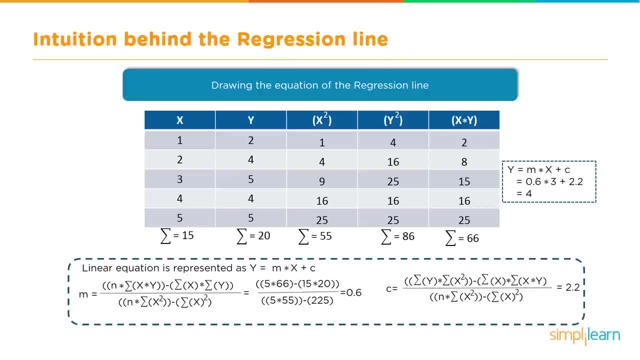 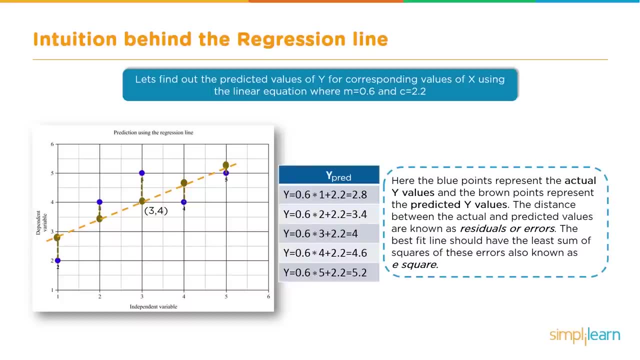 ahead and flip back there and take a look at that. Do you remember this, where we had this long formula on the bottom and we were doing all this summization And then we also looked at setting it up with the different lines, And then we also looked all the way? 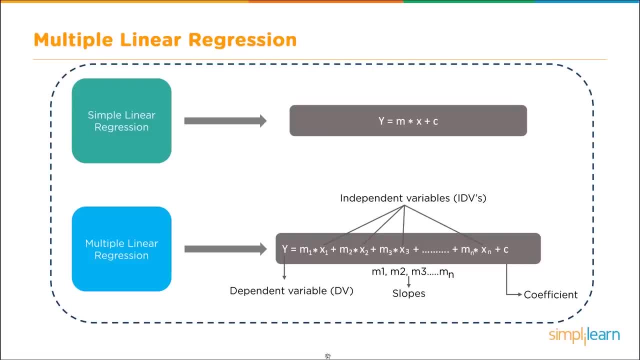 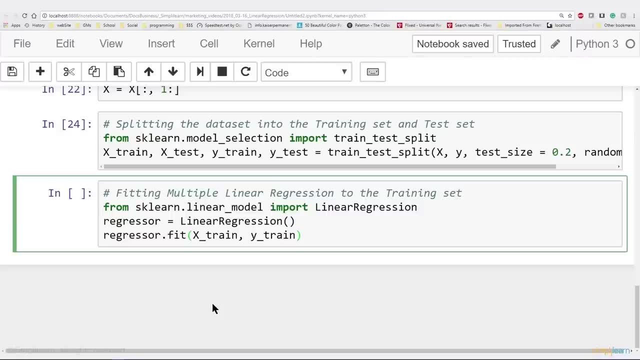 down to multiple linear regression, where we're adding all those formulas together. All of that is wrapped up in this one section. So what's going on here is I'm going to create a variable called regressor, And the regressor equals the linear regression. 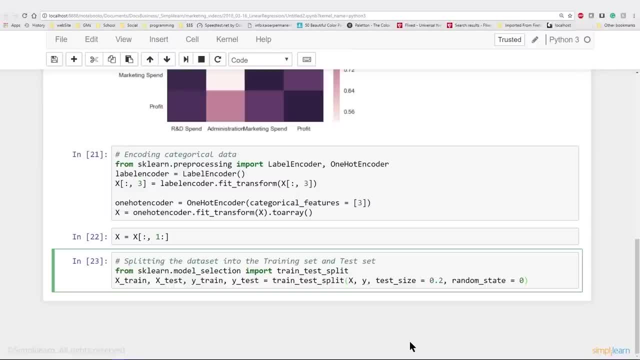 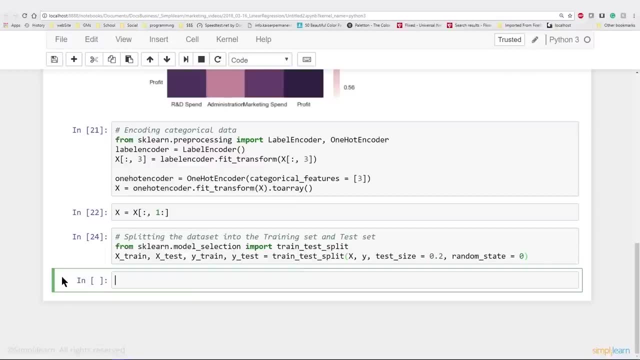 later, and then the random state equals zero. we're going to randomize which ones it picks to hold off to the side. we'll go ahead and run this. it's not overly exciting, so, setting up our variables, but the next step is the next step. we actually create our linear regression model. now that we got to the 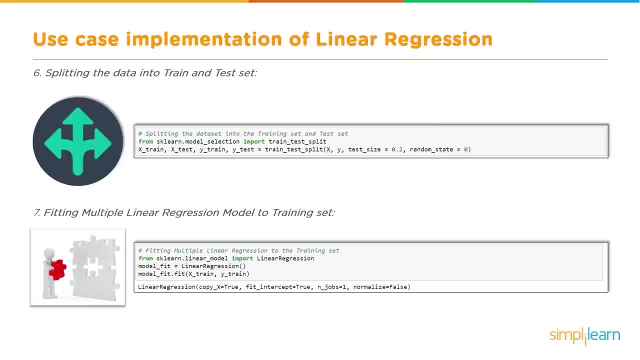 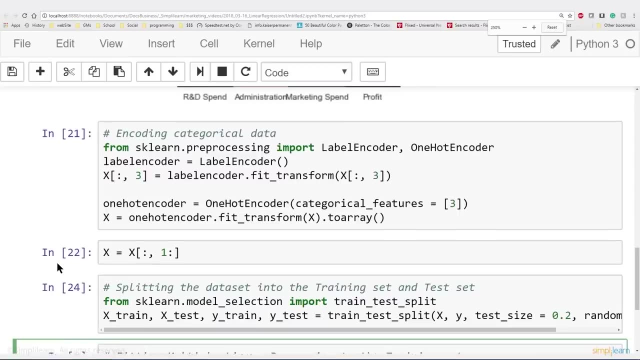 linear regression model, we get that next piece of the puzzle. let's go ahead and put that code in there and walk through it. so here we go, we're going to paste it in there and let's go ahead. and since this is a shorter line of code, let's zoom up there so we can get a good look, and we have from the sklearnlinear. 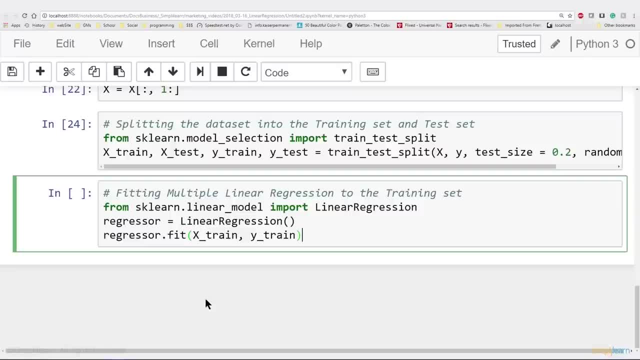 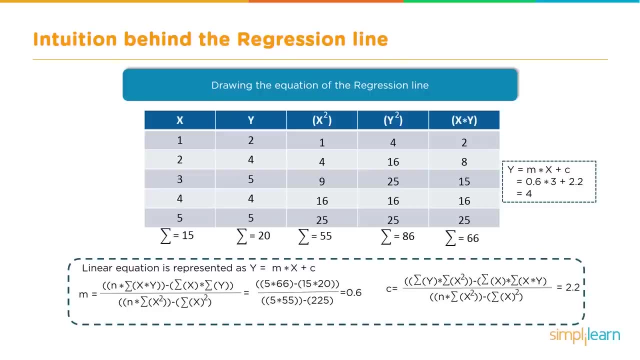 underscore model. we're going to import linear regression now. i don't know if you recall from earlier when we were doing all the math. let's go ahead and flip back there and take a look at that. do you remember this where we had this long formula on the bottom and we were doing all this? 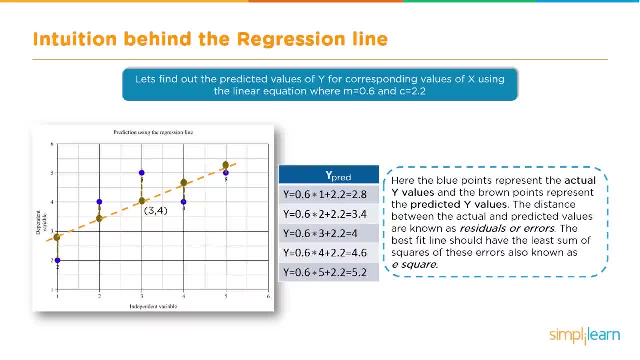 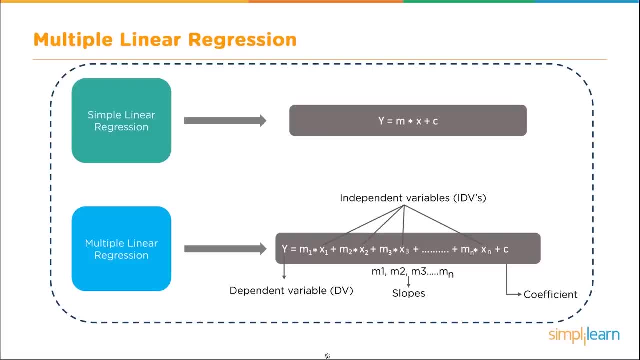 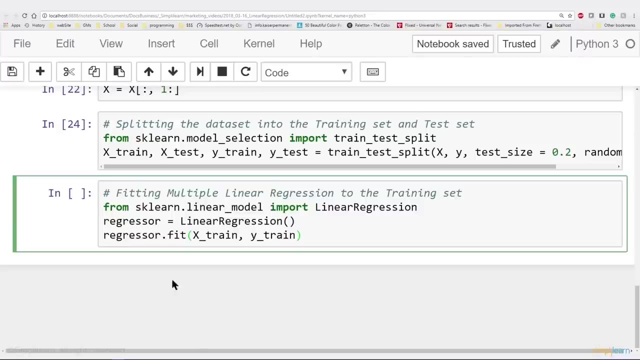 summization, and then we also looked at setting it up with the different lines, and then we also looked all the way down to multiple linear regression, where we're adding all those formulas together. all of that is wrapped up in this one section. so what's going on here is i'm going to create a variable called regressor and the 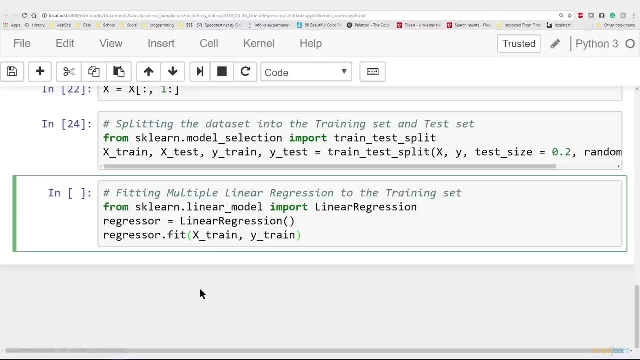 regressor equals the linear regression. that's a linear regression model that has all that math built in, so we don't have to have it all memorized or have to compute it individually. and then we do the regressorfit. in this case we do x train and y train because we're using the training data x. 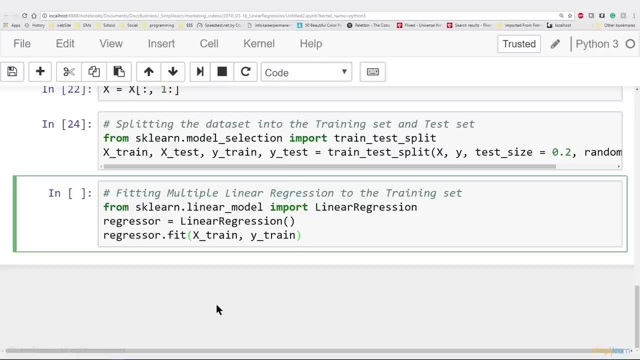 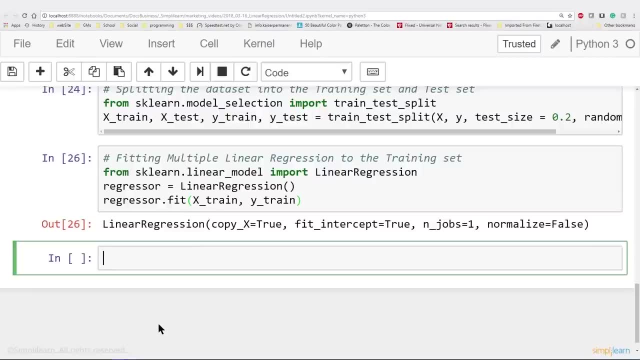 being the data in and y being profit. what we're looking at, all that math for us. so within one click and one line we've created the whole linear regression model and we fit the data to the linear regression model and you can see that when I run the regressor. 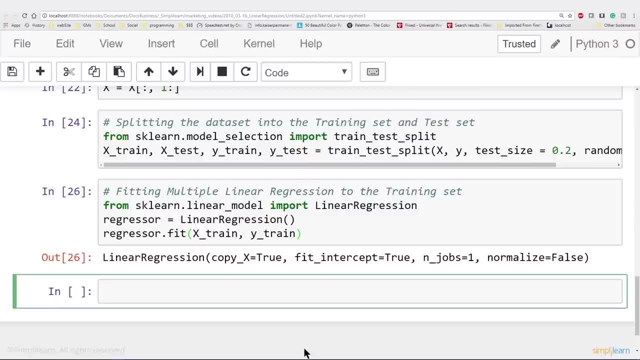 it gives an output- linear regression- it says: copy x equals true, fit intercept equals true. in jobs equal one, normalized equals false. it's just giving you some general information on what's going on with that regressor model. now that we've created our linear regression model, let's go ahead and 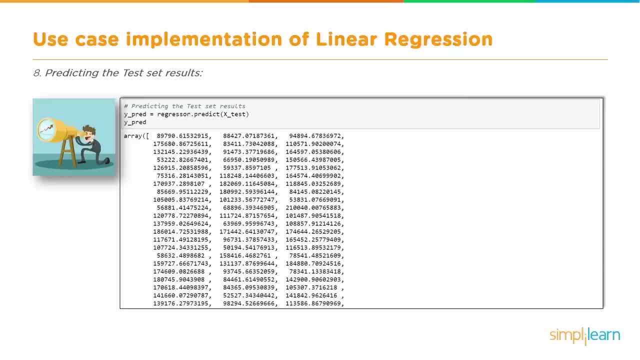 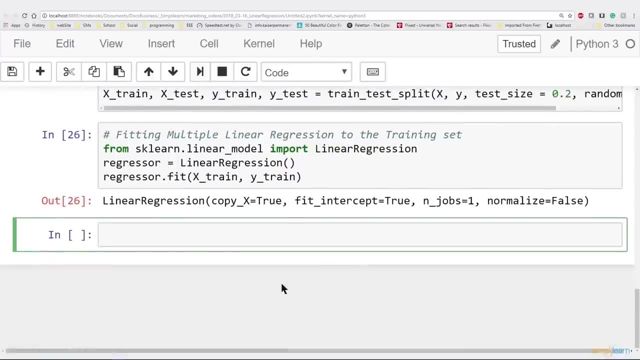 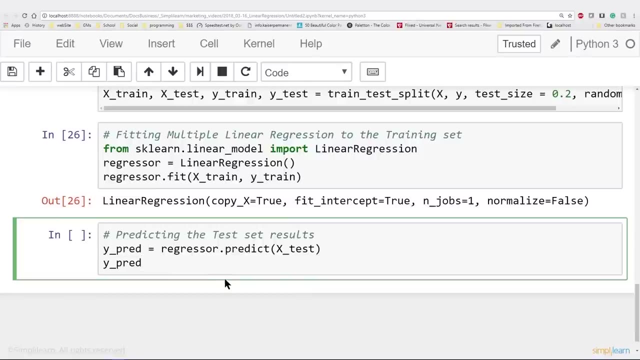 use it and, if you remember, we kept a bunch of data aside. so we're going to do a Y predict variable and we're going to put in the X test- and let's see what that looks like, scroll up a little bit, paste that in here. predicting the test set results. so here we have. Y predict equals regressor dot. 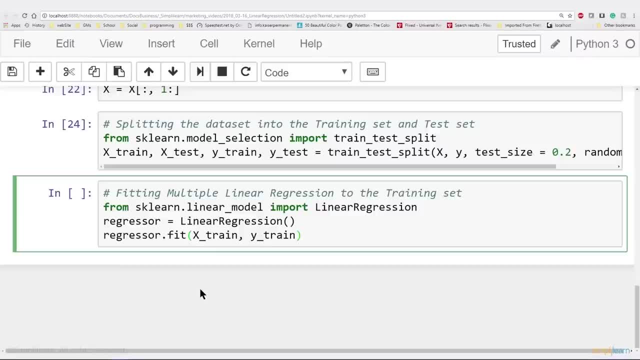 That's a linear regression model that has all that math built in, So we don't have to have it all memorized or have to compute it individually. And then we do the regressorfit. In this case we do xtrain and ytrain because we're using the training data, x being the 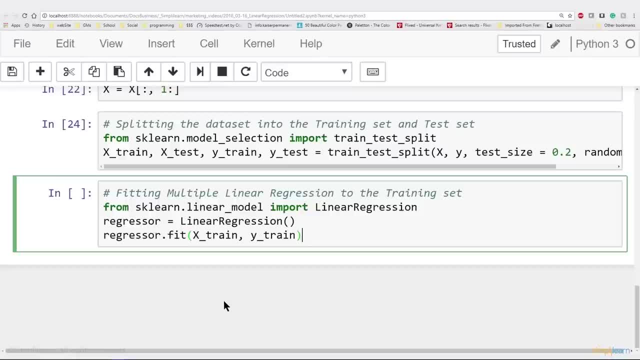 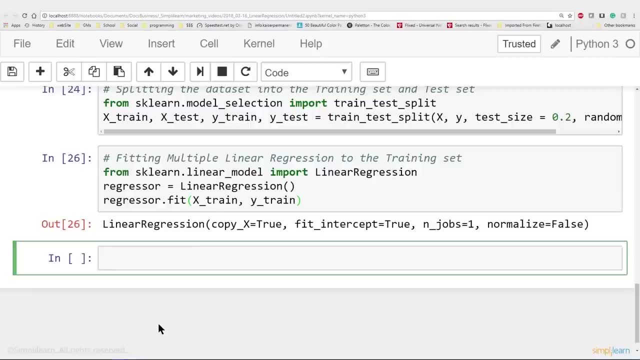 data in, and y being profit, what we're looking at And this does all that math for us. So within one click and one line we've created the whole linear regression model And we fit the data to the linear regression model And you can see that when I run the regressor it gives an. 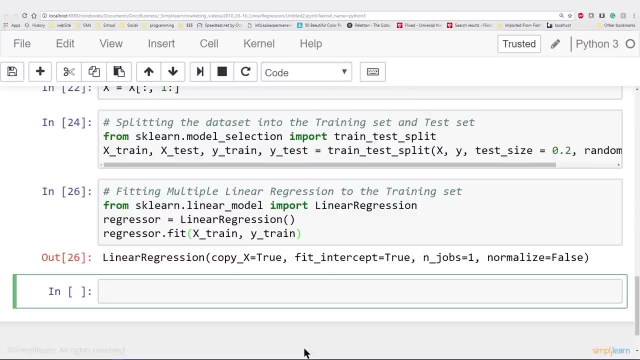 output linear regression. It says: copy x equals true, fit intercept equals true, in jobs equal one, normalized equals false. It's just giving you some general information on what's going on with that regressor model. Now that we've created our linear regression model, let's go ahead and use it And if you remember, we 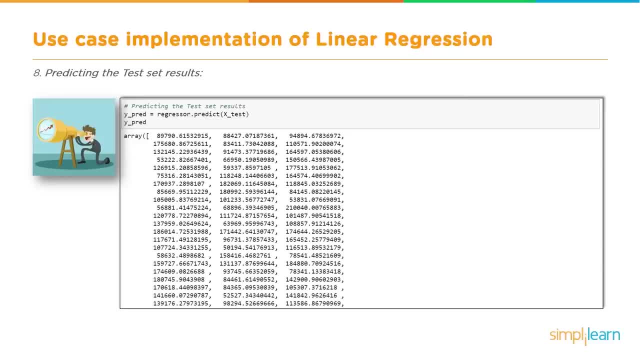 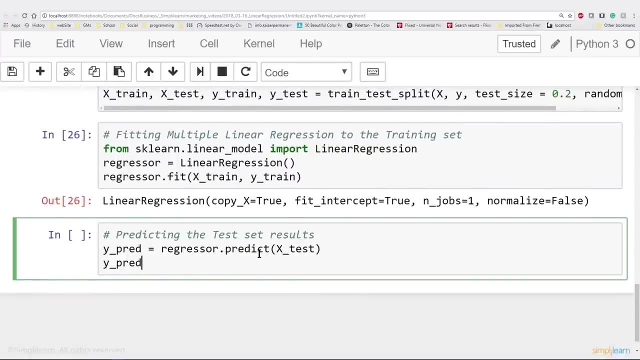 kept a bunch of data aside. So we're going to do a ypredict variable And we're going to put in the xtest And let's see what that looks like. Scroll up a little bit, Paste that in here. Predicting the test set. 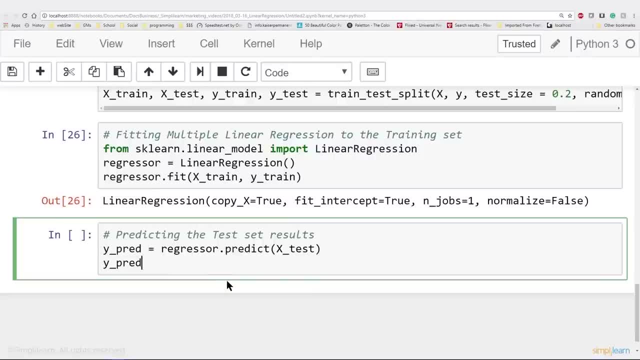 results. So here we have ypredict equals regressor dot predict xtest going in And this gives us ypredict. Now, because I'm in Jupyter inline, I can just put the variable up there And when I hit the run button, 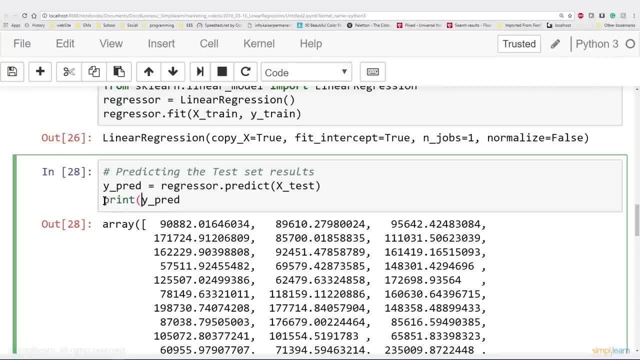 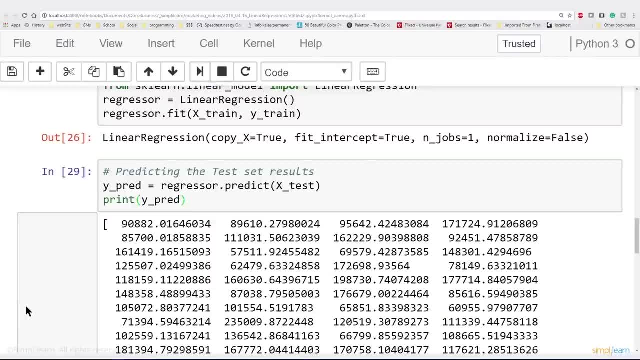 it'll print that array out. I could have just as easily done print ypredict. So if you're in a different IDE- that's not an inline setup like the Jupyter Notebook- you can do it this way: print ypredict And you'll see that for the 200 different test variables we kept off to the side, it's going to give us a. 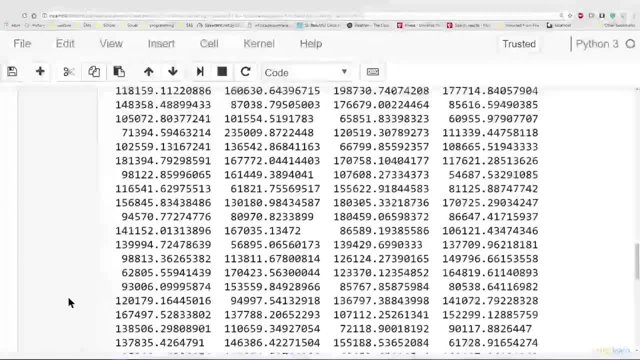 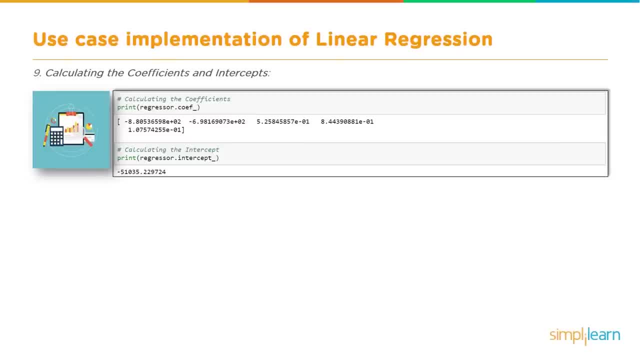 result: It's going to produce 200 answers. This is what it says the profit are for those 200 predictions. But let's don't stop there. Let's keep going and take a couple. look, We're going to take just a short detail here in calculating the coefficients and the intercepts. This gives us a 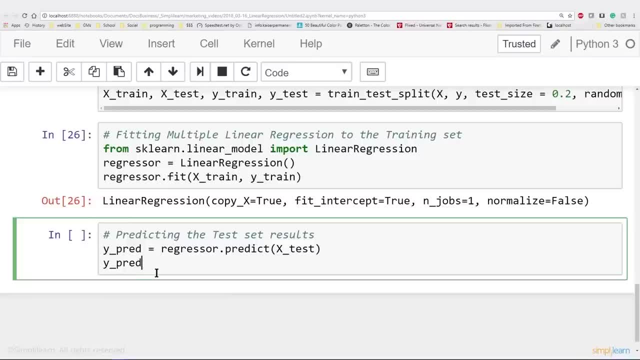 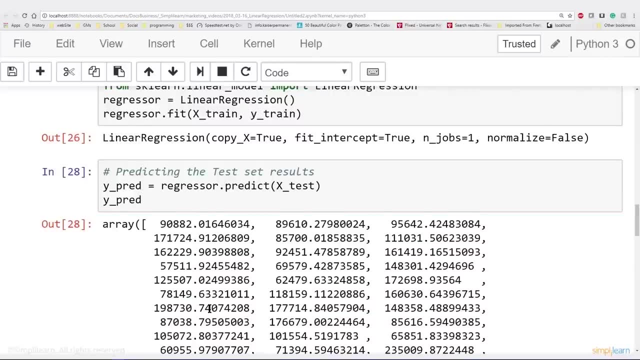 predict X test going in and this gives us Y predict. now, because I'm in Jupiter in line, I can just put the variable up there and when I hit the run button it'll print that array out. you, I could have just as easily done print Y predict. so if you're in a different IDE, that's not an. 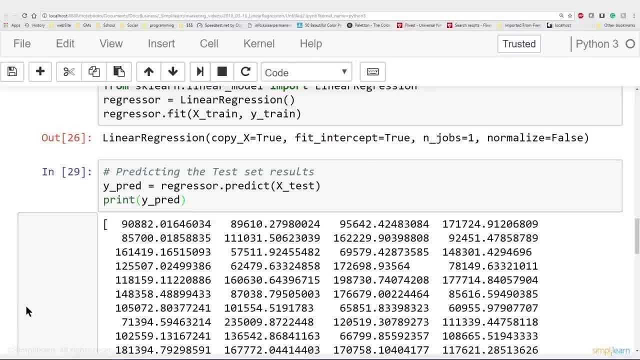 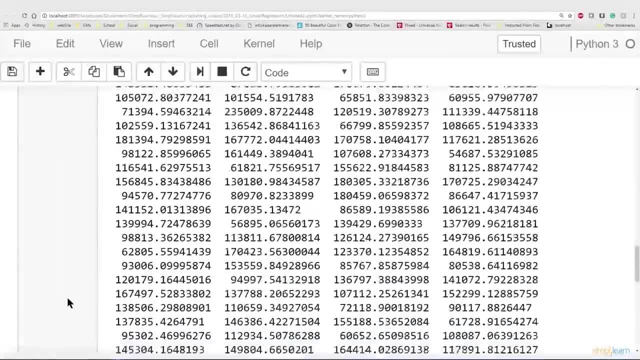 inline setup like the Jupiter notebook. you can do it this way: print Y, predict and you'll see that for the 200 different test variables we kept off to the side, it's going to produce 200 answers. this is what it says. the profit are for those 200 predictions. but let's don't 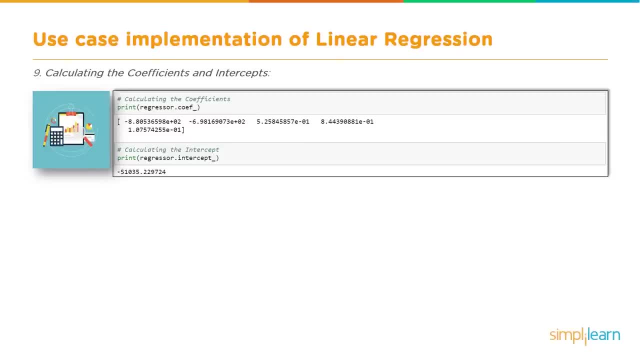 stop there, let's keep going and take a couple- look, we're gonna take this a short detail here- and calculating the coefficients and the intercepts. this gives us a quick flash and you can see that we've got a bunch of data that's going in and we've got a bunch of data. 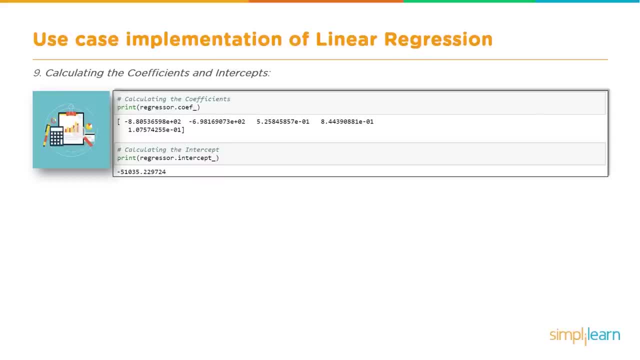 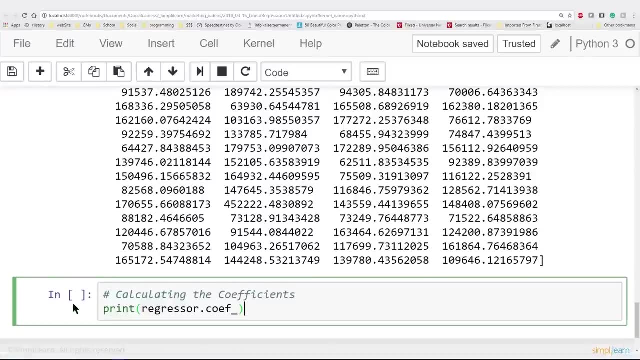 that's going in and we've got a bunch of data that's going out at what's going on behind the line. we're gonna take a short detour here and we're gonna be calculating the coefficient and intercepts so you can see what those look like. what's really nice about our regressor we created is it already? 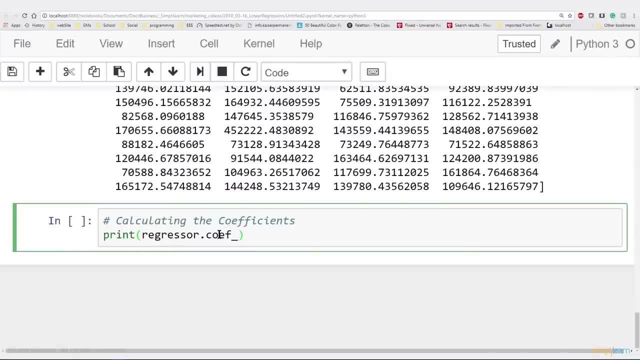 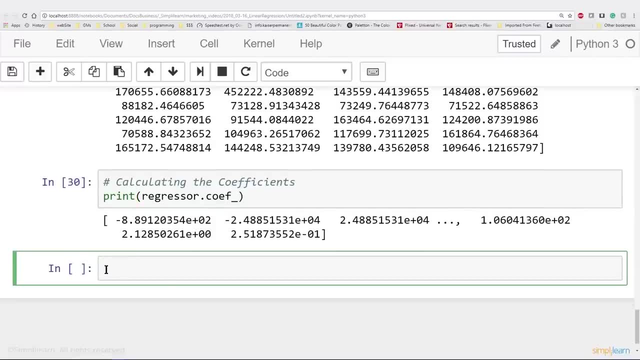 has a coefficients for us. we can simply just print regressor dot coefficient underscore. when I run this you'll see our coefficients here and if we can do the regressor coefficient, we can also do the regressor intercept. let's run that and take a look at that. this all came from the multiple. 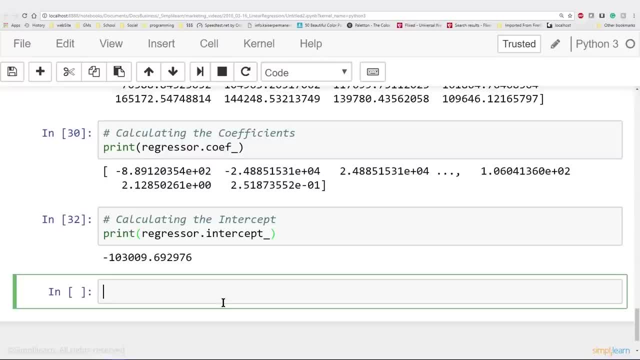 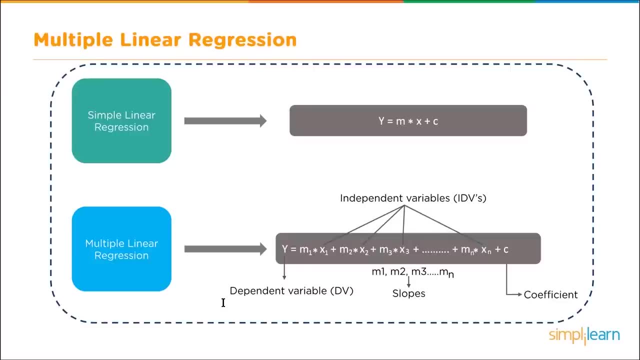 regression model and we'll flip over so you can remember where this is going into, where it's coming from. you can see the formula down here, where y equals m1 times x1 plus m2 times x2 and so on and so on, plus C, the coefficient, so these variables fit right into this formula. y equals: 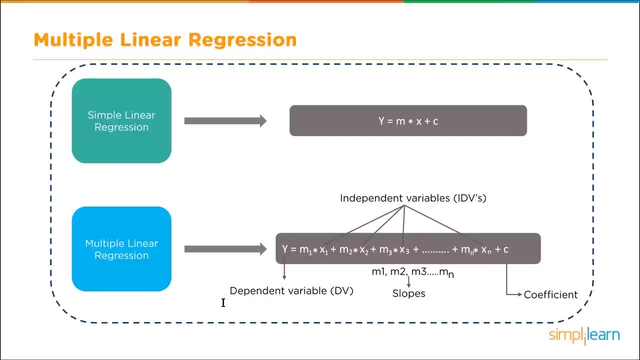 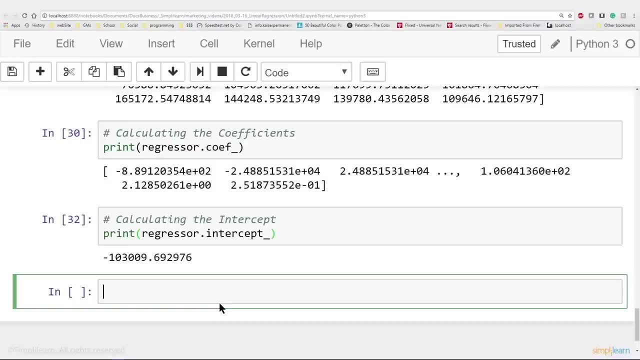 slope 1 times column 1 variable, plus slope 2 times column 2 variable, all the way to the M into the N and X to the N plus C the coefficient, or in this case you have minus eight point eight and nine to the power of two, etc. etc. times the first column and the second column in the third column. 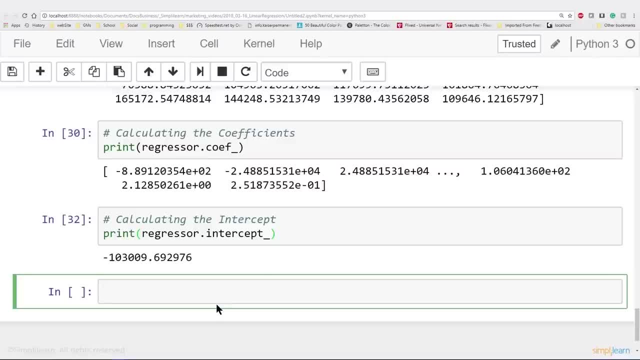 and then our intercept is the minus 1, 0, 3, 0 0, 9 point. boy gets kind of complicated when you look at it. this is why we don't do this by hand anymore. this is why we have the computer to make these. 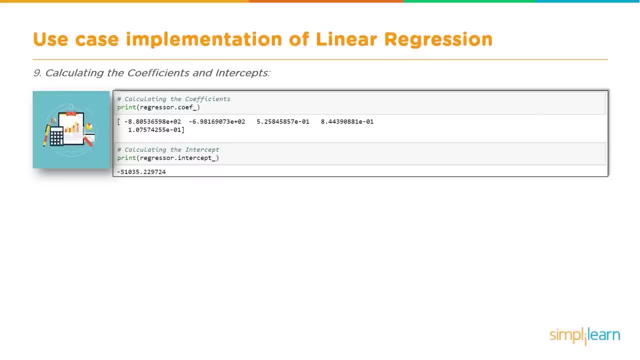 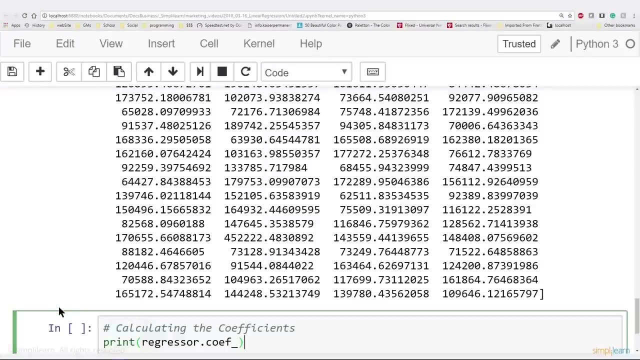 quick flash at what's going on behind the line. We're going to take a short detour here And we're going to be calculating the coefficient and intercepts So you can see what those look like. What's really nice about our regressor we created is it already has a coefficients for us And we 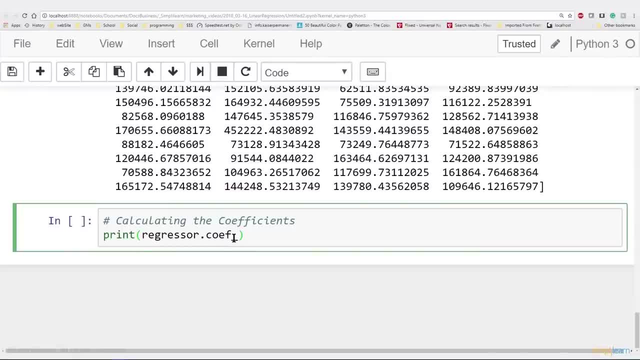 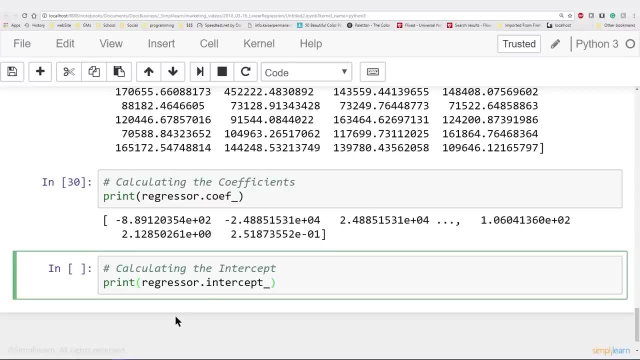 can simply just print regressorcoefficient underscore. When I run this, you'll see our coefficients here, And if we can do the regressor coefficient, we can also do the regressor intercept. Let's run that and take a look at that. This all came from the multiple regression model And we'll 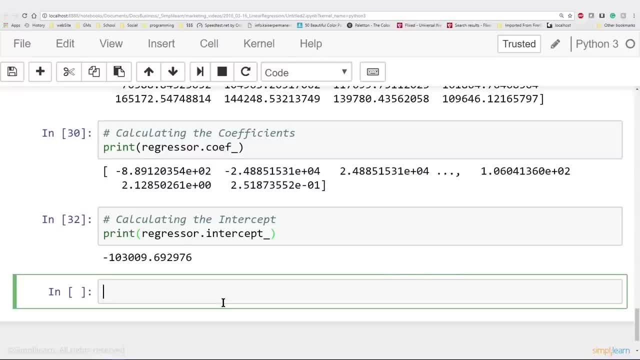 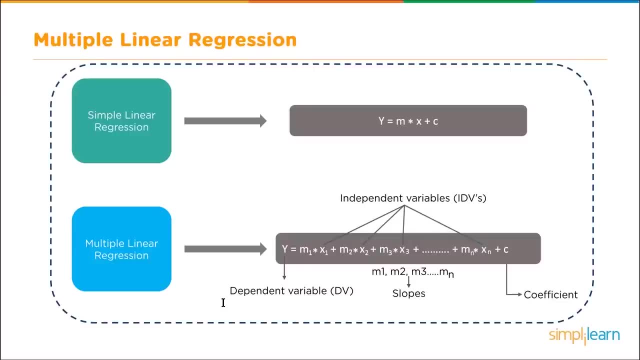 flip over so you can remember where this is going into and where it's coming from. You can see the formula down here, where y equals m1 times x1, plus m2 times x2, and so on and so on, plus c, the coefficient. So these variables are going to be the coefficients And we're going to print the. 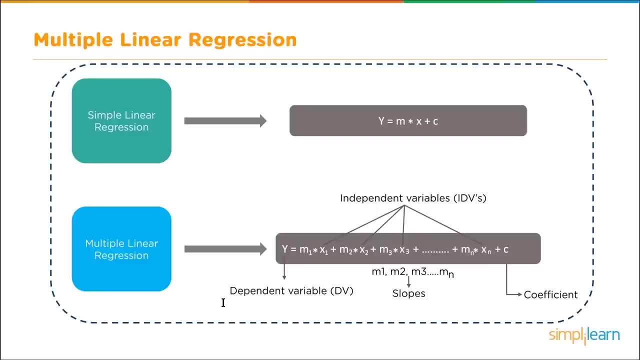 coefficients. And you can see that the coefficients fit right into this formula: Y equals slope one times column, one variable, plus slope two times column, two variable, all the way to the m, into the n and x to the n plus c the coefficient. Or in this case you have minus 8.89 to the power of two. 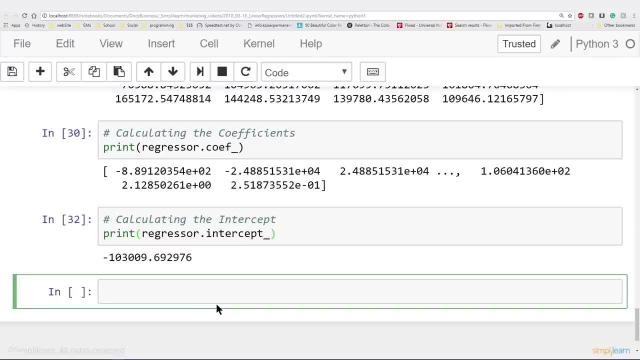 et cetera, et cetera, times the first column and the second column and the third column, And then our intercept is the minus 103009 point. Boy, it gets kind of complicated when you look at it. This is why we don't do this by hand anymore. This is why we don't do this by hand anymore. 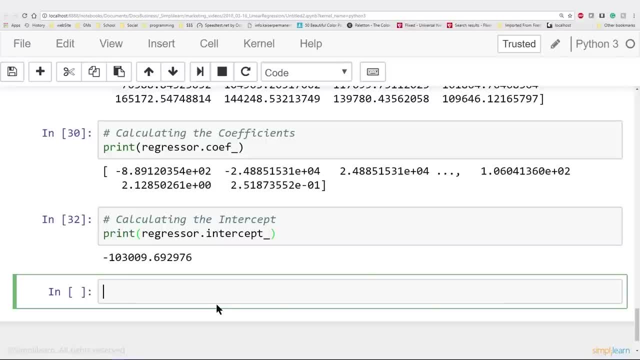 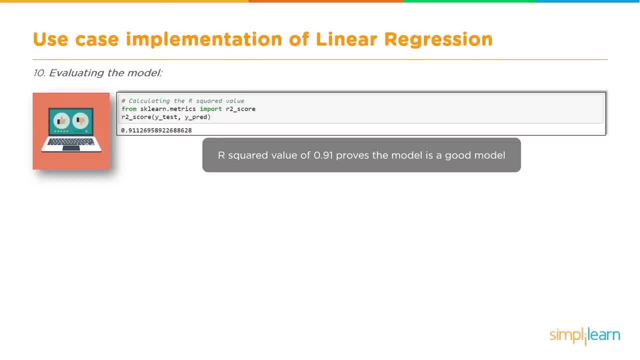 This is why we have the computer to make these calculations easy to understand and calculate. Now, I told you that was a short detour and we're coming towards the end of our script. As you remember, from the beginning I said, if we're going to divide this information, we have to make sure. 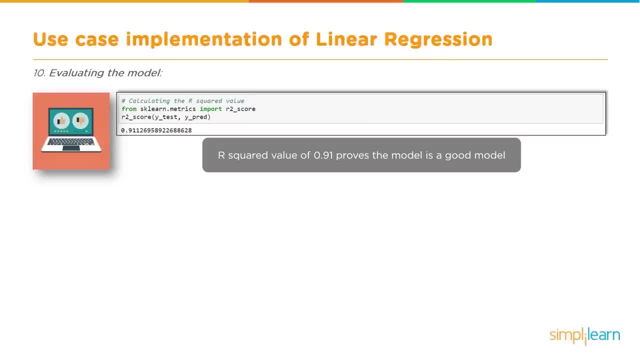 it's a valid model, that this model works and understand how good it works. So, calculating the r squared value, that's what we're going to use to predict how good our prediction is. And let's take a look at what that looks like in code. And so we're going to use this from sklearnmetrics. 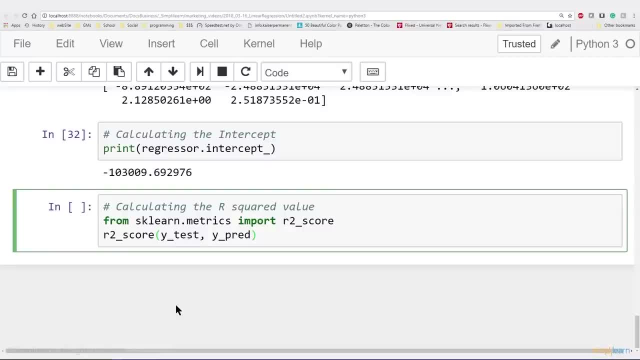 We're going to import r2 score. That's the r squared value. We're looking at the error. So in the r2 score we take our y test versus our y. predict Y test is the actual values we're testing. That was. 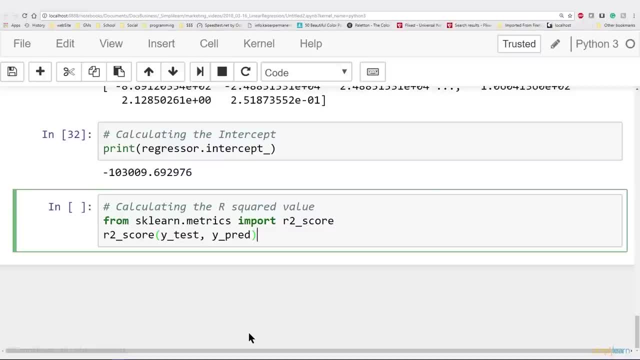 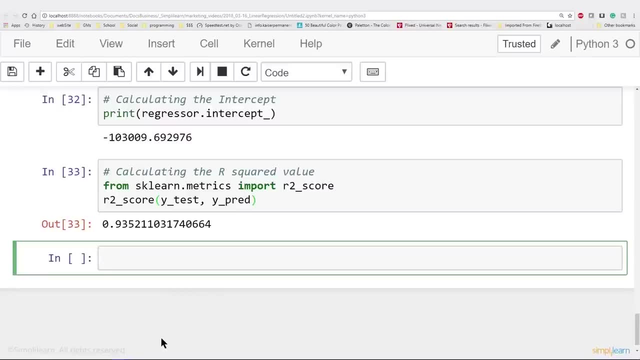 the one that was given to us that we know are true. The y predict of those 200 values is what we think it was true And when we go ahead and run this we see we get a 0.9352.. That's the r2 score. 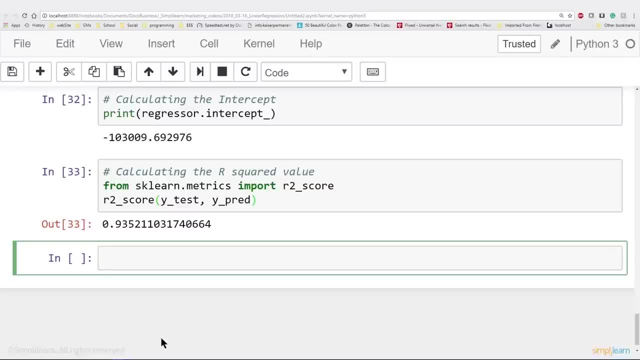 Now it's not exactly a straight percentage, So it's not saying it's 93% correct, But you do want that in the upper 90s. Oh and higher shows that this is a very valid prediction based on the r2 score And if r squared value of 0.91 or 92, as we got on our 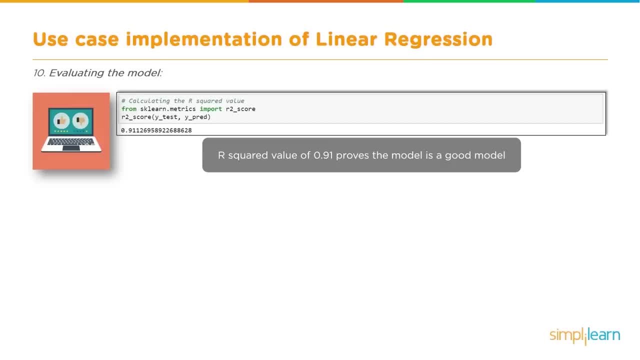 calculations easy to understand and calculate. now, I told you that was a short detour and we're coming towards the end of our script. as you remember, from the beginning I said, if we're going to divide this information, we have to make sure it's a valid model, that this 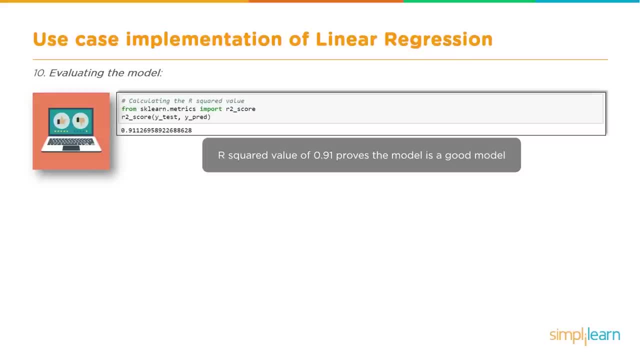 model works and understand how good it works. so, calculating the r-squared value, that's what we're going to use to predict how good our prediction is. and let's take a look at what that looks like in code. and so we're going to use this from sklearnmetrics we're going to import. 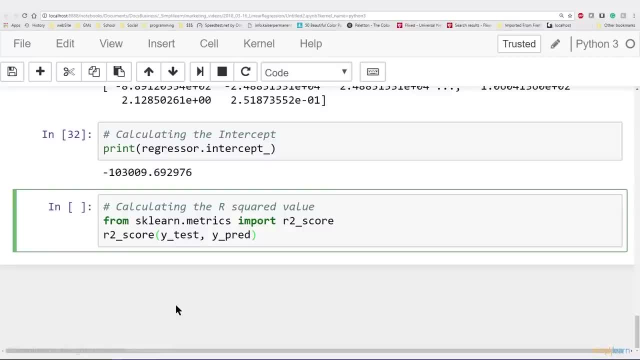 r2 score. that's the r-squared value. we're looking at the error. so in the r2 score we take our y test versus our y predict. y test is the actual values we're testing. that was the one that was given to us. we know are true. the y predict of those 200 values is what we think it was true and when. 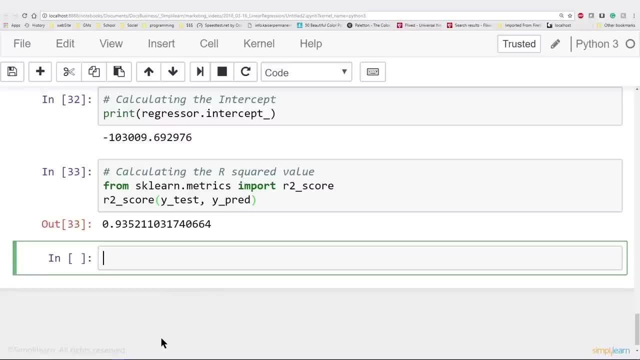 we go ahead and run this, we see we get a point nine, three, five, two. that's the r2 score. now it's not exactly a straight percentage, so it's not saying it's 93 percent correct, but you do want that in the upper 90s oh and higher shows that this is a very valid prediction based on the r2. 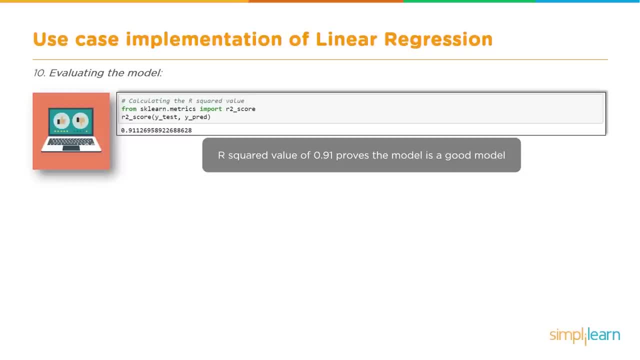 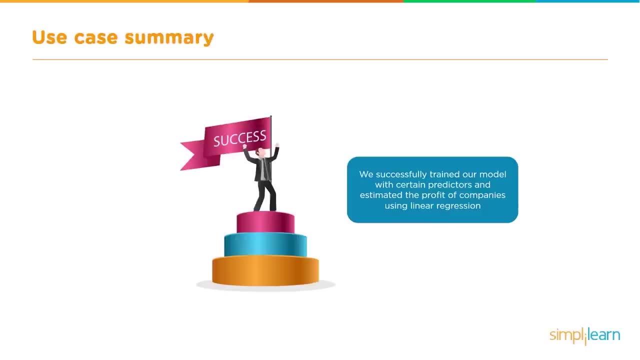 score and if r-squared value of 0.91 or 92 as we got on our model, remember it does have a random generation involved. this proves the model is a good model, which means success. yay, we successfully trained our model with certain predictors and estimated the profit of the companies using linear. 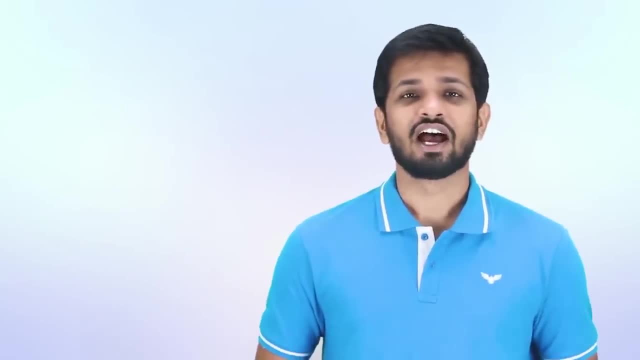 regression. thank you for a really great session, richard. i hope you guys found linear regression fun to learn. now let's get into some other machine learning algorithms. over to mohan. hello and welcome to the session on logistic regression. i am mohan kumar from simply learn what is logistic regression. 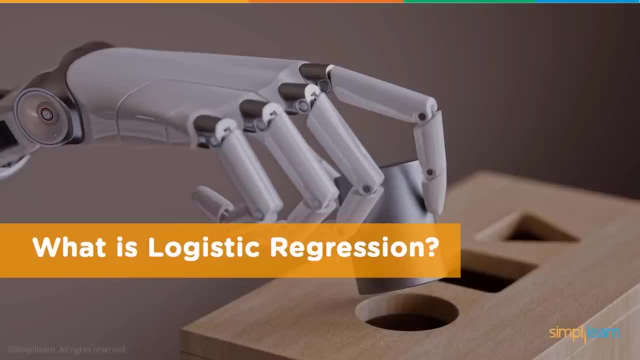 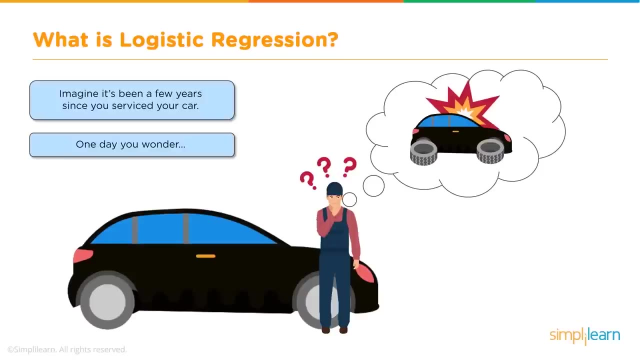 hello and welcome to the session on logistic regression. i am mohan kumar from simply learn what is logistic regression regression? As I mentioned earlier, logistic regression is an algorithm for performing binary classification. So let's take an example and see how this works. Let's say your car has not been. 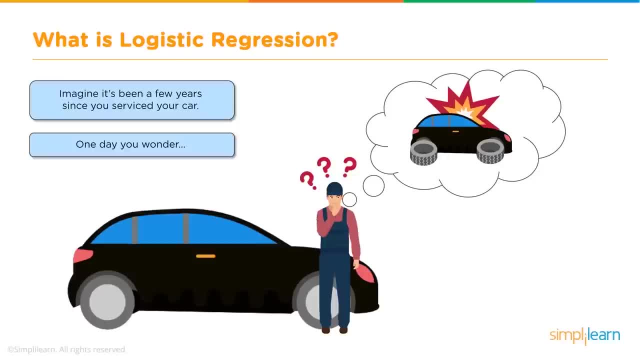 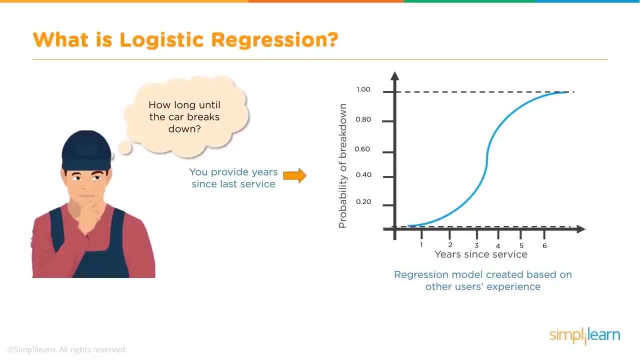 serviced for quite a few years and now you want to find out if it is going to break down in the near future. So this is like a classification problem: Find out whether your car will break down or not. So how are we going to perform this classification? So here's how it looks If we plot. 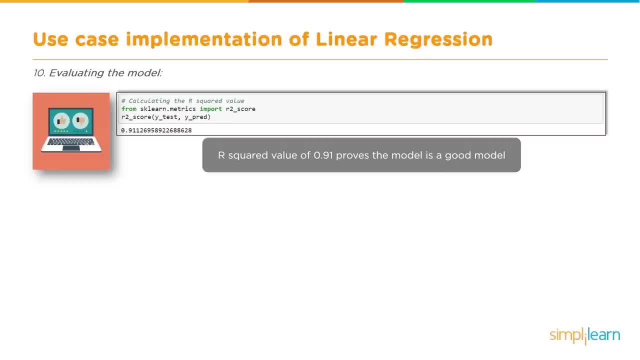 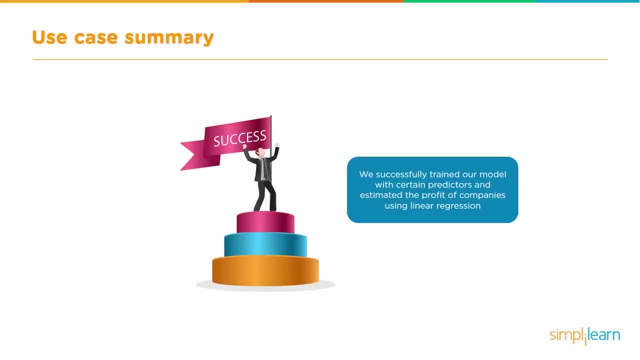 model. remember it does have a random generation involved. This proves the model is a good model, which means success. Yay, We successfully trained our model with certain predictors and estimated the profit of the companies using linear regression. Thank you for a really great session. 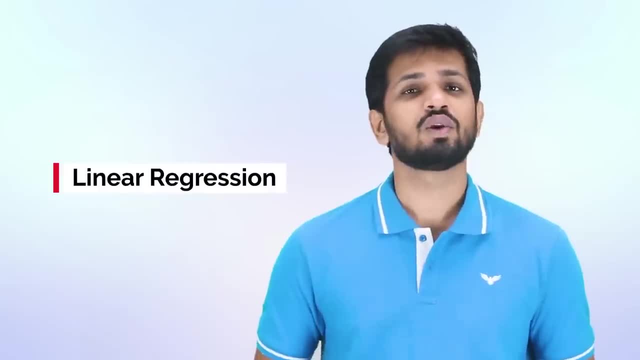 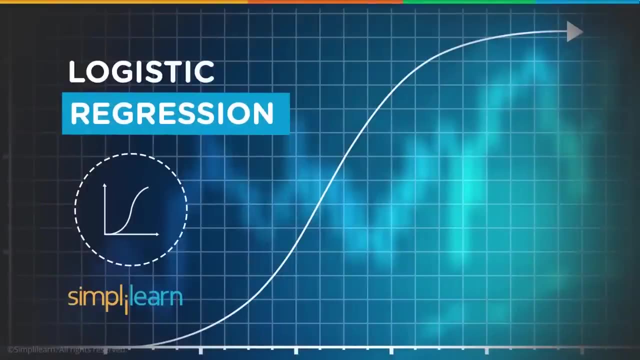 I hope you guys found linear regression fun to learn. Now let's get into some other machine learning algorithms. Over to Mohan. Hello and welcome to the session on logistic regression. I'm Mohan Kumar from Simply Learn What is logistic regression, As I mentioned earlier. 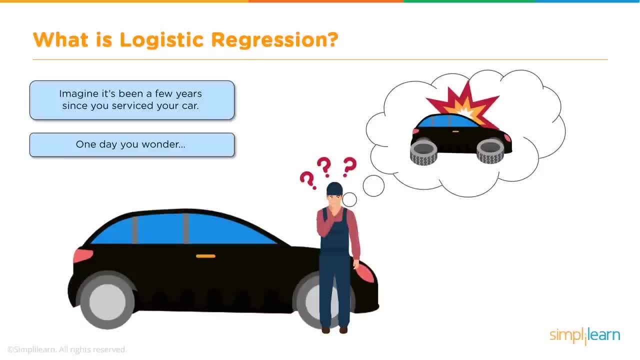 logistic regression is an algorithm for performing binary classification. So let's take an example and see how this works. Let's say your car has not been serviced for quite a few years And now you want to find out if it is going to break down in the near future. So this is like a classification. 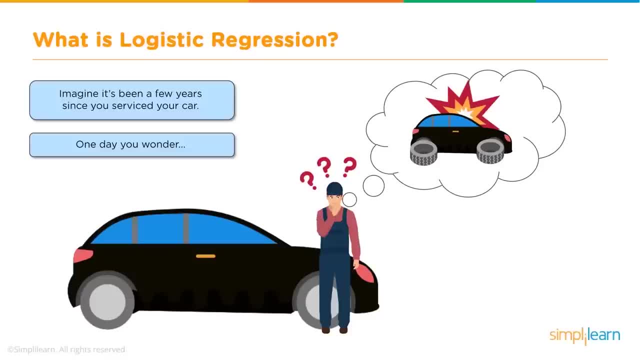 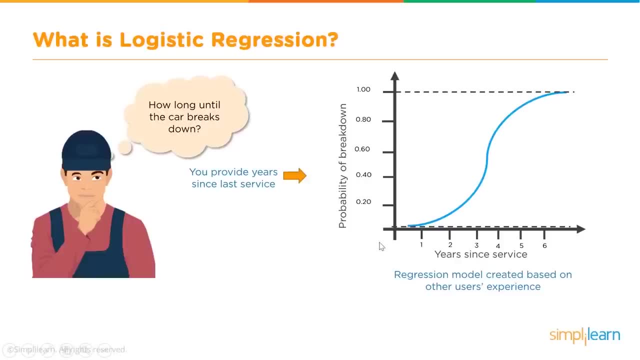 problem, Find out whether your car will break down or not. So how are we going to perform this classification? So here's how it looks. If we plot the information along the x and y axis, x is the number of years since the last service was performed and y is the probability of your. 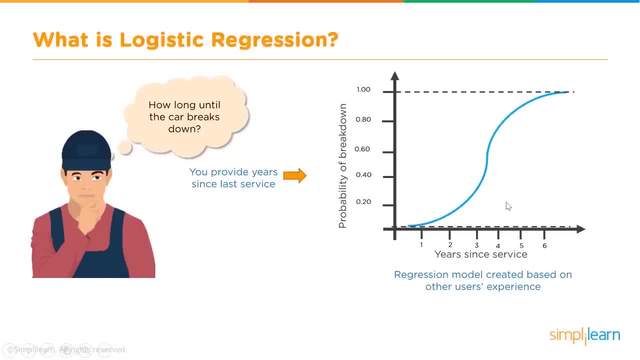 car breaking down And let's say this information was. this data, rather, was collected from several car users. It's not just your car, but several car users. So that is our labeled data. So the data has been collected and for the number of years and when the car broke. 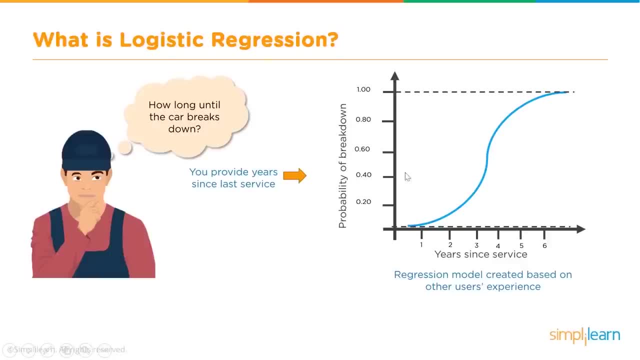 down and what was the probability. And that has been plotted along x and y axis. So this provides an idea. from this graph We can find out whether your car will break down or not. We'll see how The probability can go from zero to one. As you're aware, probability can be between zero and one. 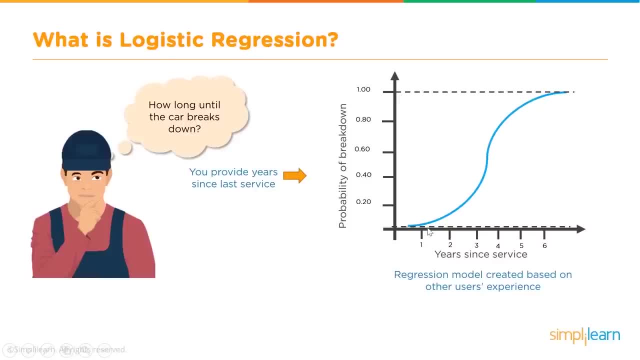 And, as we can imagine, it is intuitive as well. as the number of years are on the lower side, maybe one year, two years or three years till after the service, the chances of your car breaking down are very limited, right? So, for example, chances of your car breaking down, 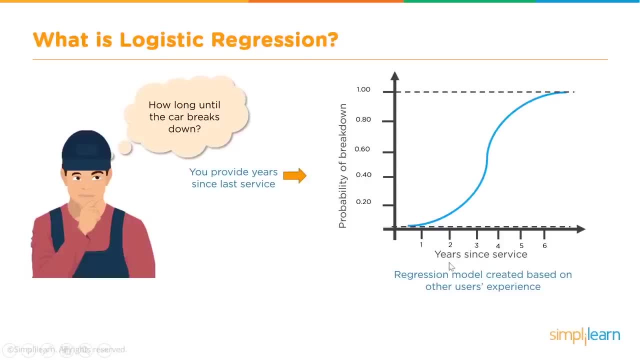 the information along the x and y axis: x is the number of years since the last service was performed and y is the probability of your car breaking down. And let's say, this information was, this data, rather, was collected from several car users. It's not just your car, but several car. 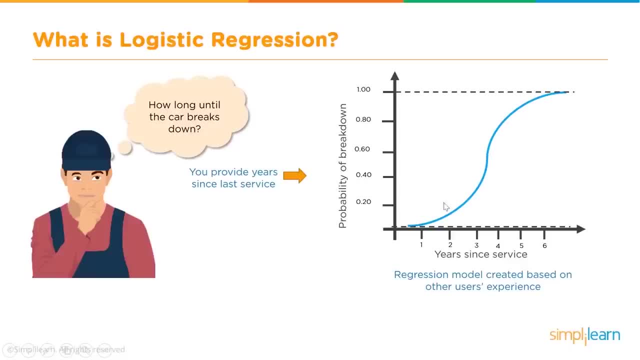 users. So that is our labeled data. So the data has been collected and for the number of years and when the car broke Down and what was the probability, and that has been plotted along x and y axis. So this provides an idea. from this graph We can find out whether your car will break down or not. We'll see how. 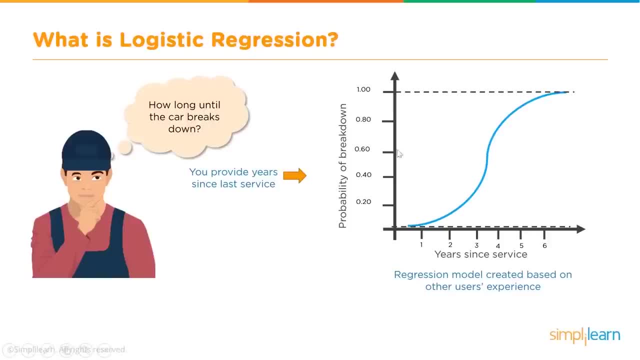 So, first of all, the probability can go from zero to one. As you are aware, probability can be between zero and one And, as we can imagine, it is intuitive as well, as the number of years are on the lower side, Maybe one year. 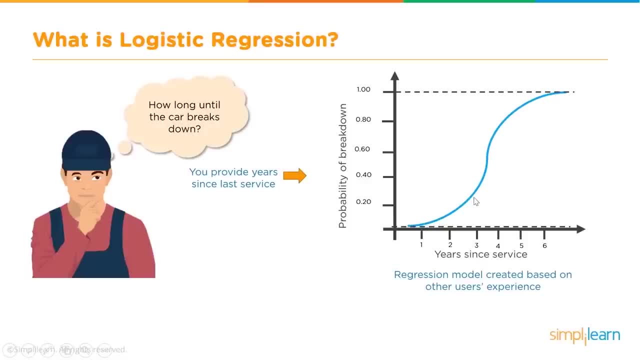 Two years or three years to after the service, the chances of your car breaking down are very limited, right? So, for example, chances of your car breaking down, the probability of your car breaking down within two years of your last service are 0.1 probability. Similarly, three years is. 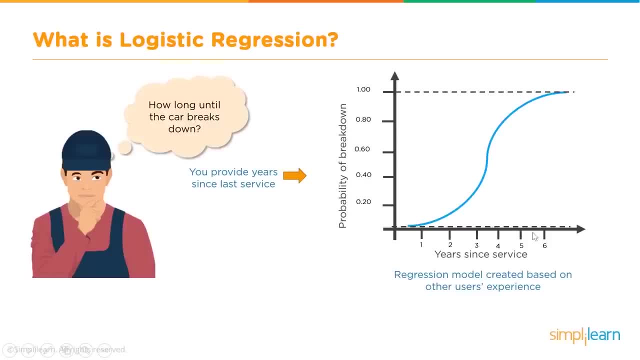 maybe 0.3 and so on, But as the number of years increases- let's say, if it was six or seven years- there is almost a certainty that your car is going to break down. That is what this graph shows. So this is an example of an application of the classification algorithm, And we will see. 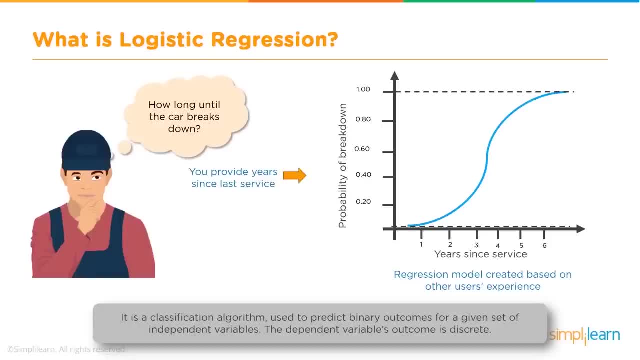 in little details how exactly logistic regression is applied here. One more thing needs to be added here is that the dependent variables outcome is discrete. So if we are talking about whether the car is going to break down or not, so that is a discrete value, the y that we are talking about. 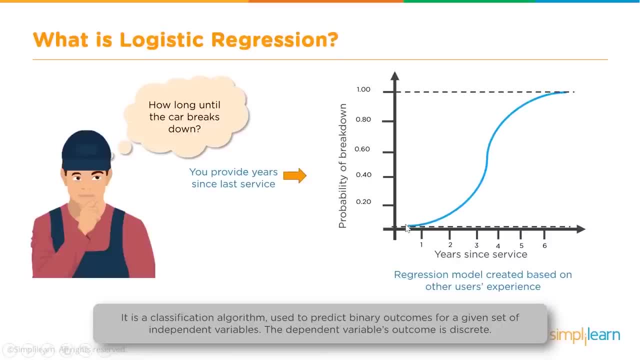 the dependent variable that we are talking about. what we are looking at is whether the car is going to break down or not, yes or no. That is what we are talking about. So here the outcome is discrete and not a continuous value. So this is how the logistic regression curve looks. Let me explain a 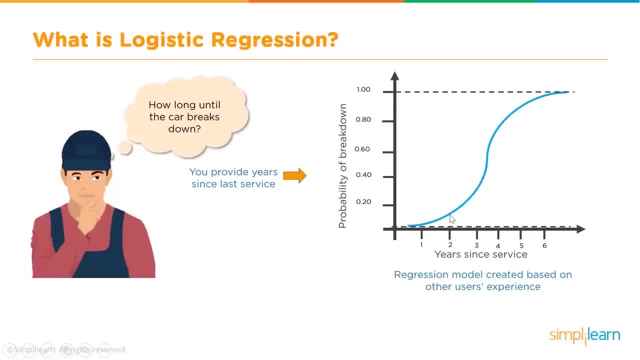 the probability of your car breaking down within two years of your last service are 0.1 probability. Similarly, three years is maybe 0.3, and so on. But as the number of years increases- let's say if it was six or seven years- there is almost a certainty that your car is going. 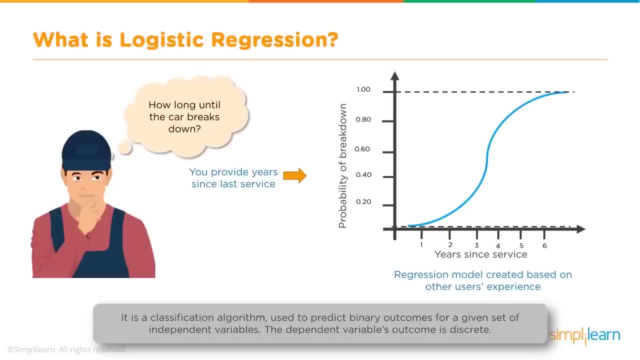 to break down, That is what this graph shows. So this is an example of an application of the classification algorithm, And we will see in little details how exactly logistic regression is applied here. One more thing needs to be added here is that the dependent variables 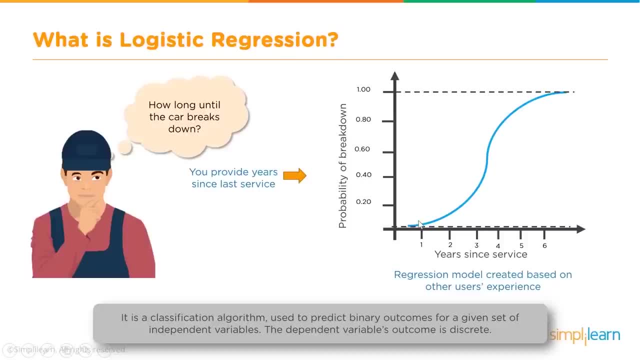 is discrete. So if we are talking about whether the car is going to break down or not, so that is a discrete value, the y that we are talking about, the dependent variable that we are talking about. what we are looking at is whether the car is going to break down or not, yes or no. 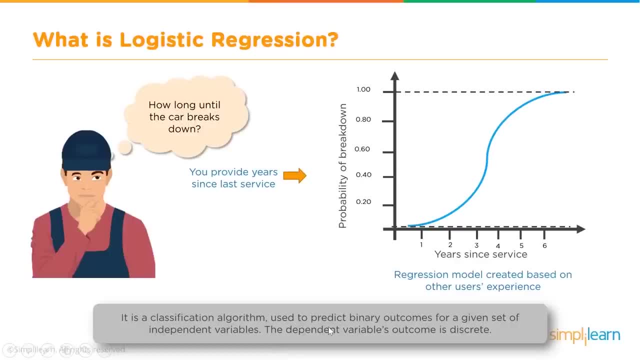 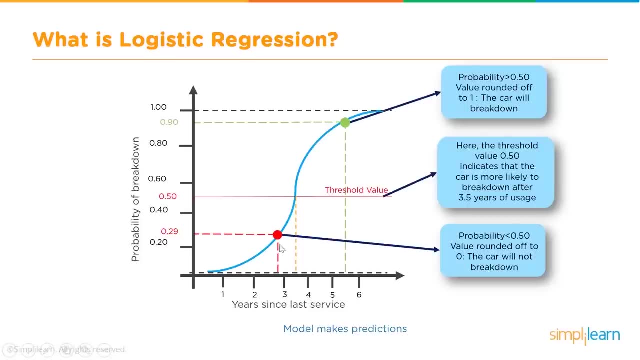 that is what we are talking about. So here the outcome is discrete and not a continuous value. So this is how the logistic regression curve looks. Let me explain a little bit what exactly we are going to determine the outcome. rather So, with a logistic regression curve, a threshold, 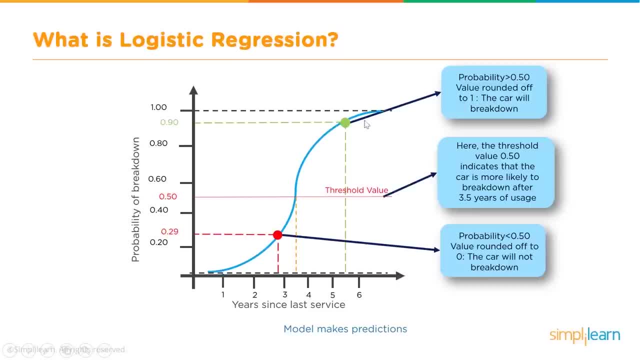 has to be set, saying that, because this is a probability calculation. remember, this is a probability calculation and the probability itself will not be 0 or 1.. But based on the probability, we need to decide what the outcome should be. So there has to be a threshold, like for example: 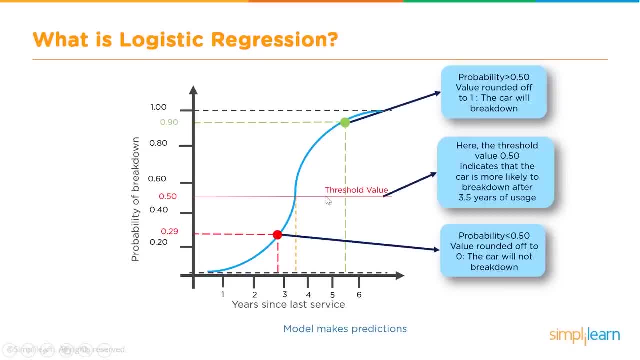 0.5 can be the threshold, let's say in this case. so any value of the probability below 0.5 is considered to be 0 and any value above 0.5 is considered to be 1.. so an output of, let's say, 0.8. 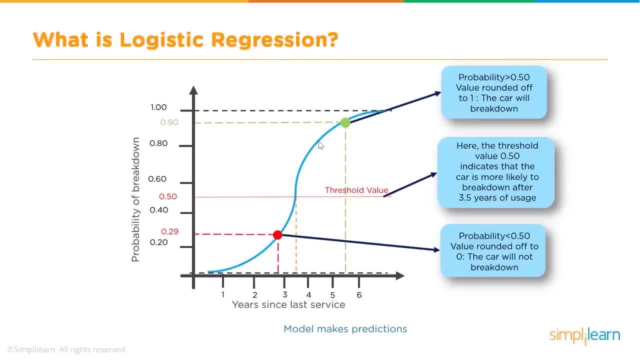 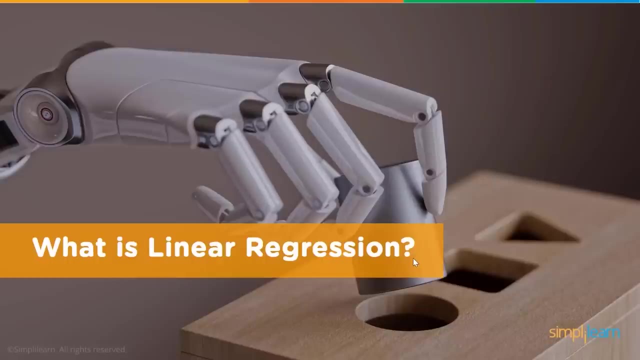 will mean that the car will break down. so that is considered as an output of 1, and let's say, an output of 0.29 is considered as 0, which means that the car will not break down. so that's the way legislation works. now let's do a quick comparison between logistic regression and linear regression. 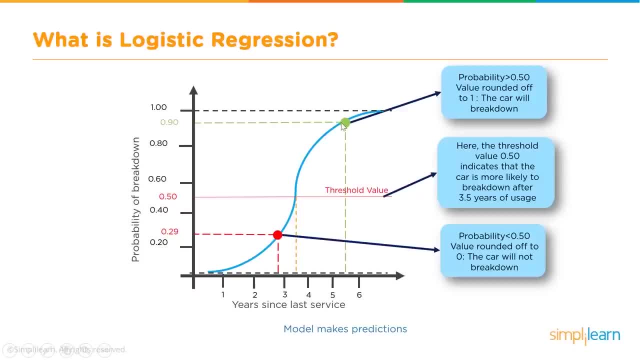 little bit. what exactly and how exactly we are going to determine the class, the outcome, rather. So, for a logistic regression curve, a threshold has to be set, saying that, because this is a probability calculation- remember, this is a probability calculation and the probability itself will not be zero or one, But based on the probability we need to decide. 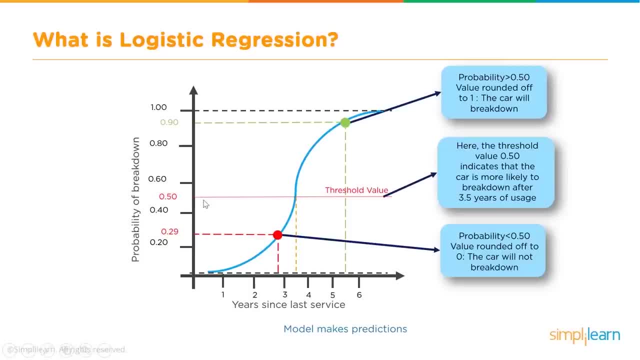 what the outcome should be. So there has to be a threshold, like, for example, 0.5 can be the threshold, let's say in this case. So any value of the probability below 0.5 is considered to be zero. 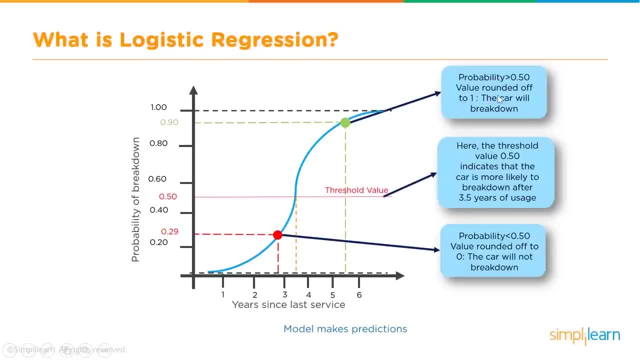 and any value above 0.5 is considered to be one. So an output of, let's say, 0.8 will mean that the car is going to break down or not. So this is how the logistic regression curve looks. So 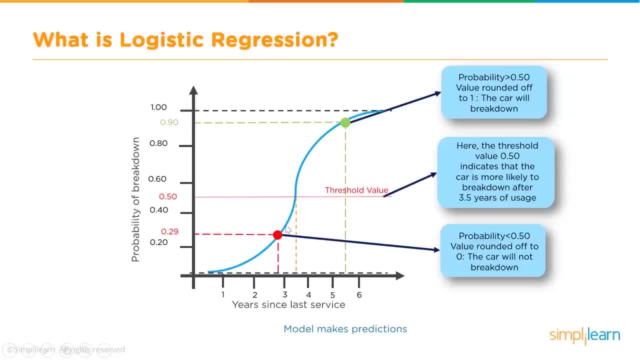 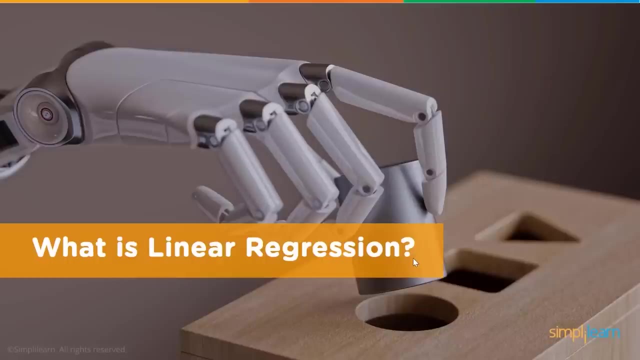 that is considered as an output of one. And let's say, an output of 0.29 is considered as zero, which means that the car will not break down. So that's the way logistic regression works. Now let's do a quick comparison between logistic regression and linear regression. 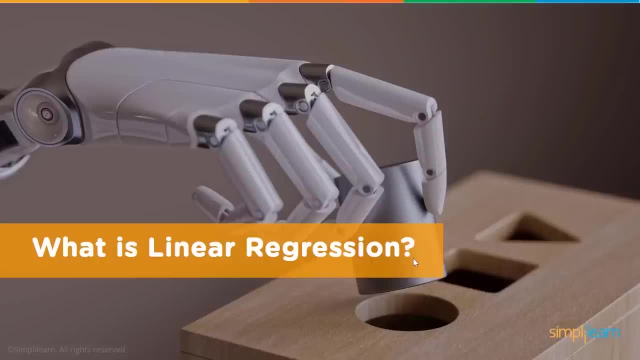 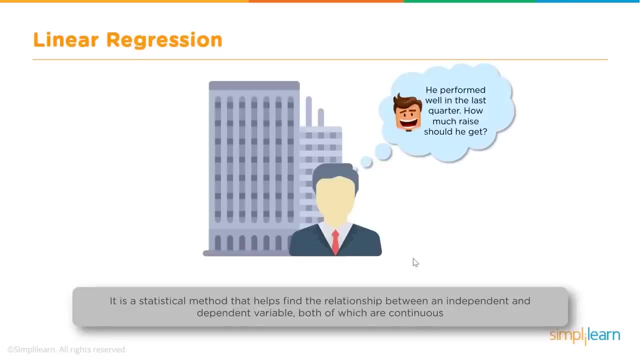 because they both have the term regression in them, So it can cause confusion. So let's try to remove that confusion. So what is linear regression? Linear regression is a process. it's, once again, an algorithm for supervised learning. However, here you're going to. 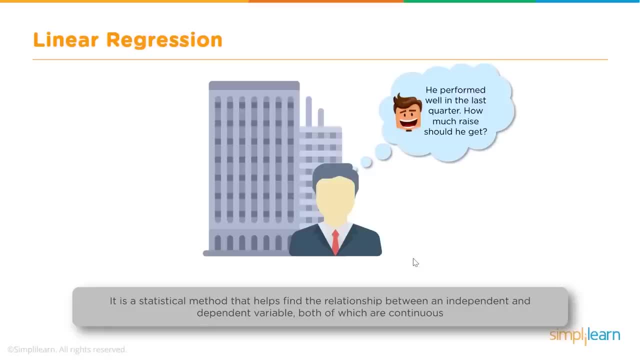 find a continuous value. you're going to determine a continuous value. It could be the price of a real estate property, It could be your hike- how much hike you're going to get- or it could be a stock price. These are all continuous values. These are not discrete. 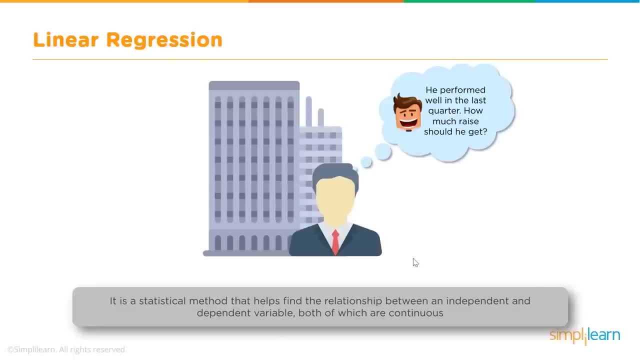 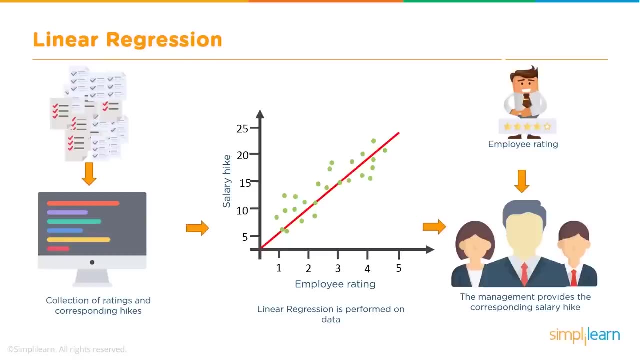 compared to a yes or a no kind of response that we are looking for in logistic regression. So this is one example of a linear regression. Let's say, at the HR team of a company tries to find out what should be the salary hike of an employee. 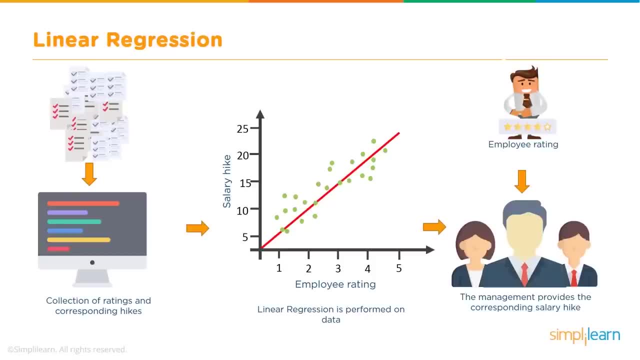 so they collect all the details of their existing employees, their ratings and their salary hikes. what has been given, and that is the labeled information that is available, and the system learns from us, it is trained and it learns from this labeled information so that, when a new employees, information is fed based on 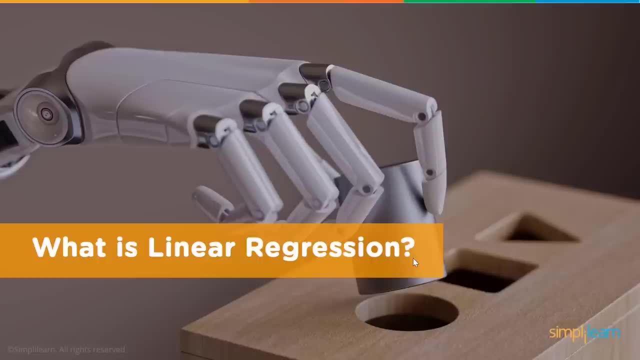 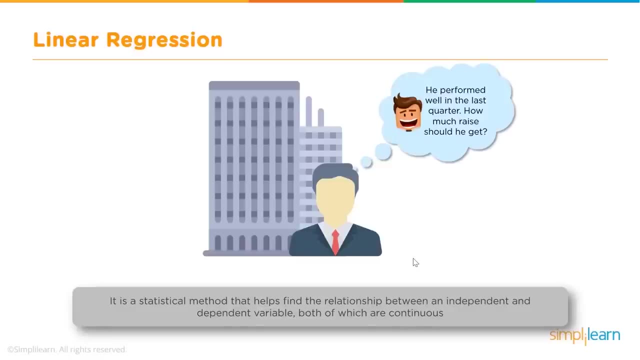 because they both have the term regression in them, so that can cause confusion, so let's try to remove that conclusion. so what is linear regression? linear regression is a process which, once again, an algorithm for supervised learning. however, here you are going to find a continuous value. you are 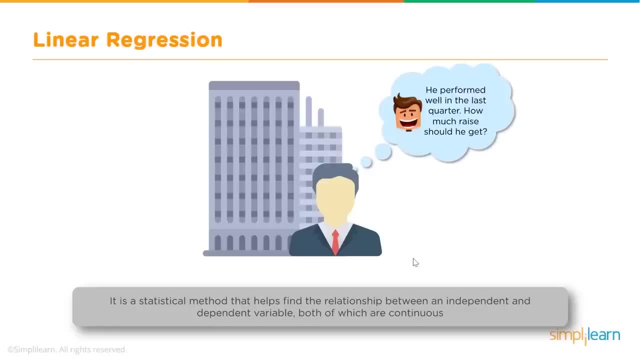 going to determine a continuous value. it could be the price of a real estate property property. it could be your hike- how much hike you're going to get- or it could be a stock price. These are all continuous values. these are not discrete compared to a yes or a no kind. 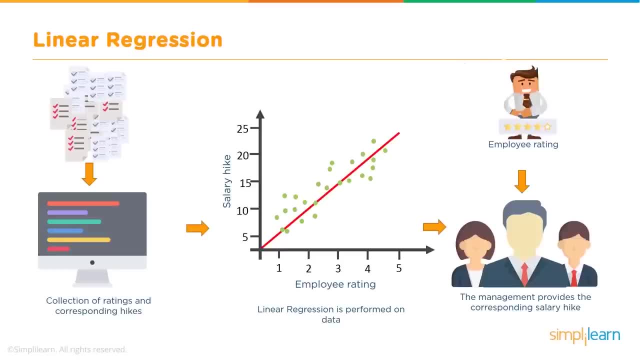 of response that we are looking for in logistic regression. So this is one example of a linear regression. Let's say the HR team of a company tries to find out what should be the salary hike of an employee, So they collect all the details of their existing employees, their ratings and their salary. 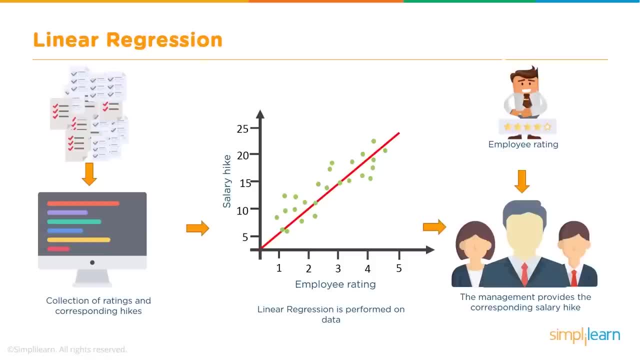 hikes what has been given, and that is the labeled information that is available, and the system learns from this. it is trained and it learns from this labeled information so that when a new employee's information is fed, based on the rating, it will determine what should be the hike. 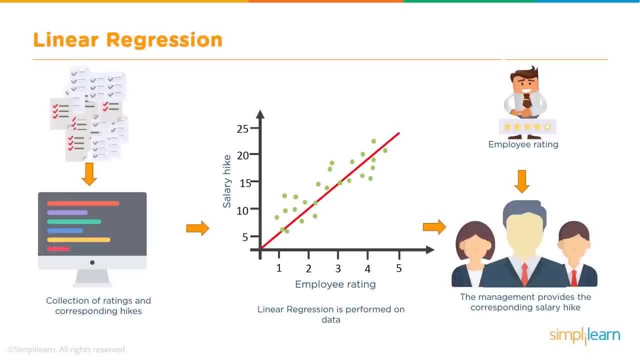 So this is a linear regression problem and a linear regression example. Now, salary is a continuous value. you can get 5000, 5500, 5600.. It is not discrete like a cat or a dog or an apple or a banana. 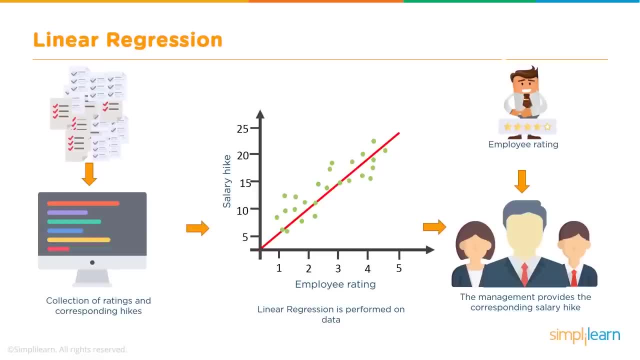 These are discrete, or a yes or a no, these are discrete values. So this way you're trying to find continuous values is where we use linear regression. So let's say, just to extend on this scenario, we now want to find out whether this employee 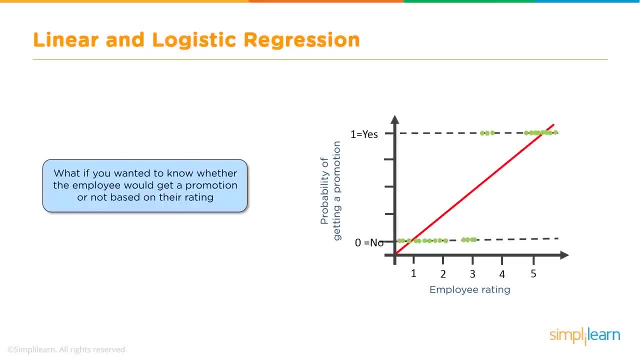 is going to get a promotion or not. So we want to find out- that is a discrete problem- a yes or no kind of a promotion. In this case, we actually cannot use linear regression, even though we may have labeled data. So this is the labeled data: 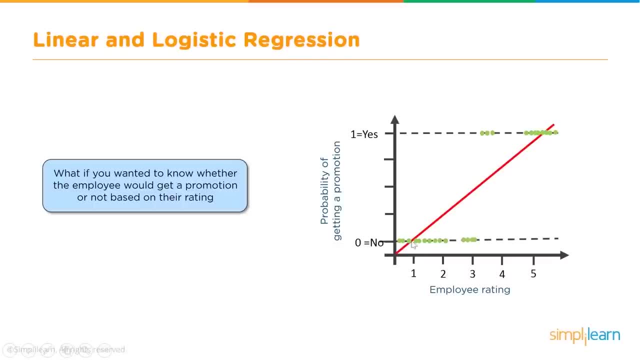 So, based on the employee rating, these are the ratings. and then some people got the promotion and this is the ratings for which people did not get promotion. that is a no, and this is the rating for which people got promotion. We just plotted the data about whether a person has got an employee has got promotion or 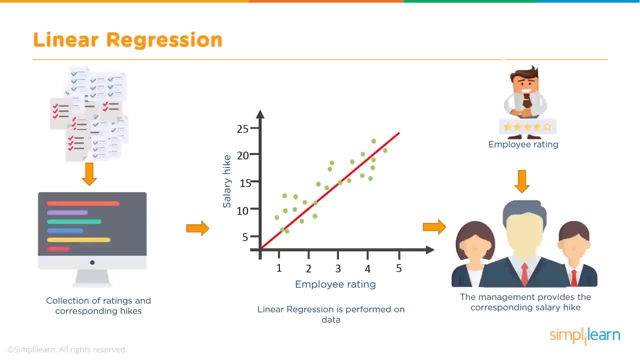 the rating, it will determine what should be the height. so this is a linear regression problem and a linear regression example. now, salary is a continuous value. you can get five thousand, five thousand, five hundred, five thousand, six hundred. it is not discrete, like a cat or a dog, or an apple or a. 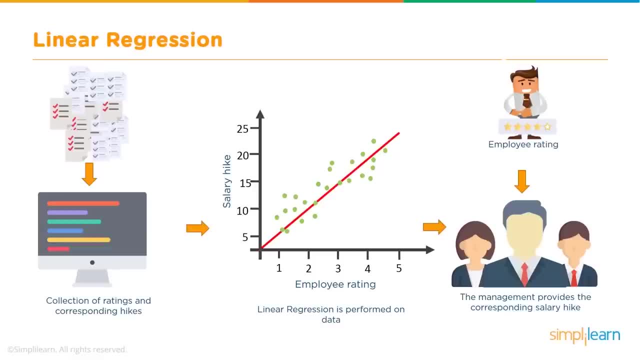 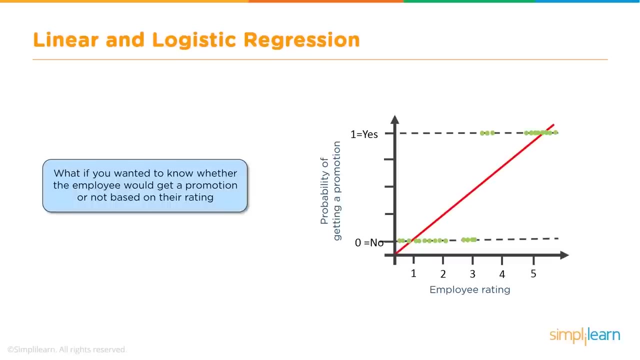 banana. these are discrete, or a yes or a no. these are discrete values, right? so this way you are trying to find continuous values is where we use linear regression. so let's say, just to extend on this scenario, we now want to find out whether this employee is going to get a. 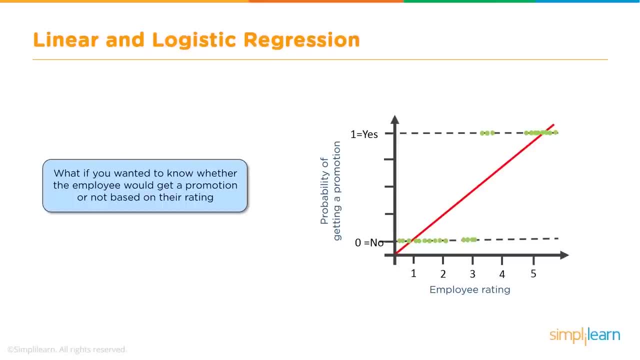 promotion or not, so we want to find out the week. that is a discrete problem, right, yes, or no kind of a problem? in this case, we actually cannot use linear regression, even though we may have labeled data. so this is the label data. so, based on the employee rating, these are the ratings. and then some people got 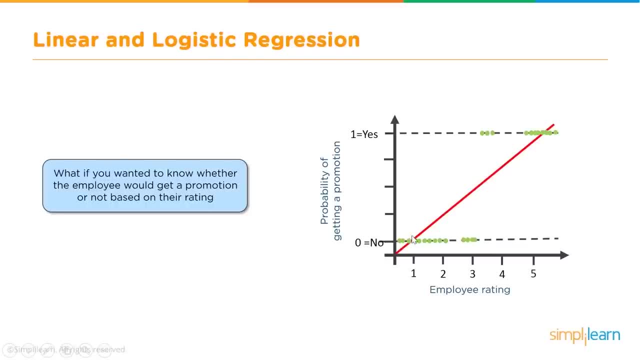 the promotion and this is the ratings for which people did not get promotion. that is a no and this is a rating for which people got promotion. we just plotted the data about whether a person has got an employers got promotion or not. yes, no, right, so there is nothing in between. and what is the employees rating? 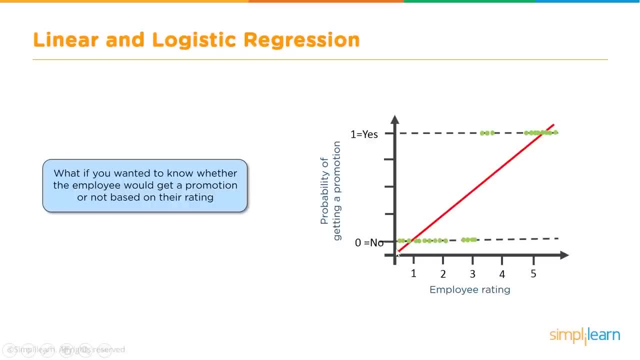 okay, and ratings can be continuous? that is not, but the output is discrete, in this case, whether employee got promotion, yes, no, okay. so if we try to plot that and we try to find a straight line, this is how it would look and, as you can see, doesn't look very right because looks like there will be a lot of errors. this 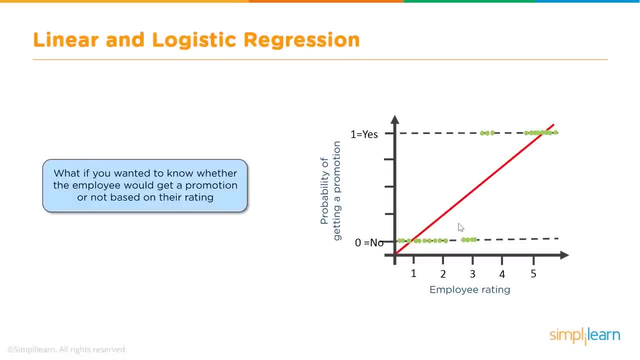 root mean square error, if you remember, for linear regression would be very, very high and also the the values cannot go beyond 0 or beyond 1, so the graph should probably look somewhat like this: click that 0 and 1, but still the straight line doesn't look right. 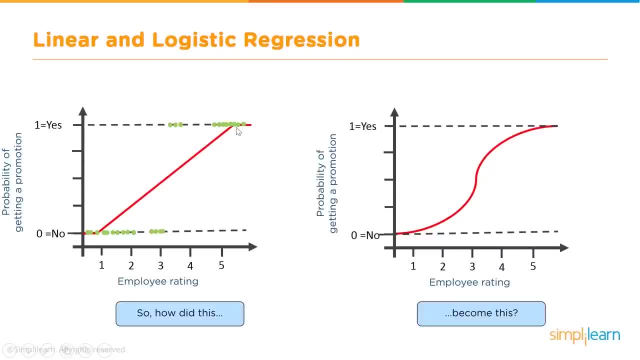 therefore, instead of using a linear equation, we need to come up with something different, and therefore the logistic regression model looks somewhat like this. so we calculate the probability and if we plot that probability, not in the form of a straight line, but we need to use some other equation. we will see very soon. 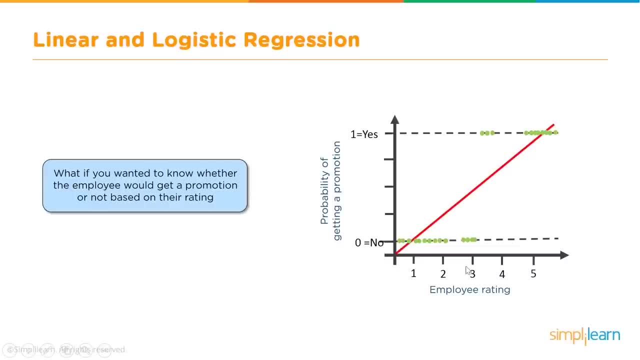 not? yes, no, right. So there is no promotion. There is nothing in between. and what is the employee's rating? and ratings can be continuous, That is not an issue. But the output is discrete in this case, whether employee got promotion, yes, no. 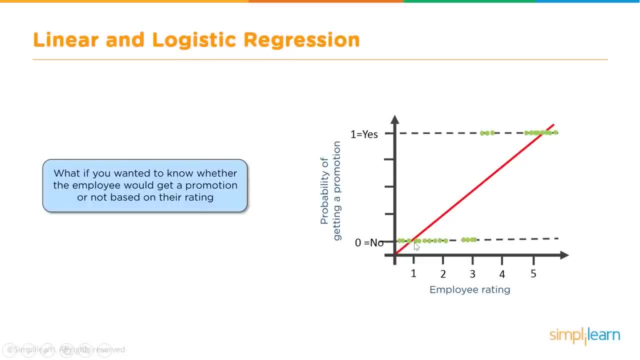 So if we try to plot that and we try to find a straight line, this is how it would look And, as you can see, it doesn't look very right because it looks like there will be a lot of errors. This root mean square error, if you remember, for linear regression would be very, very 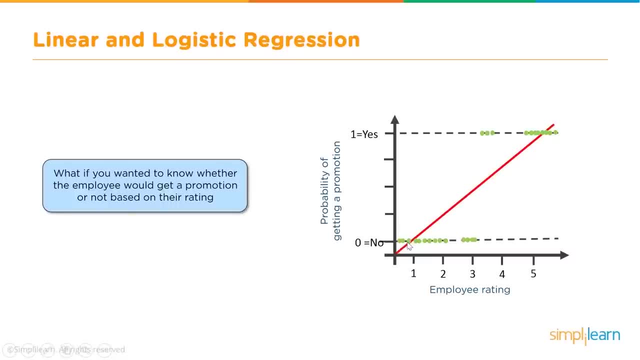 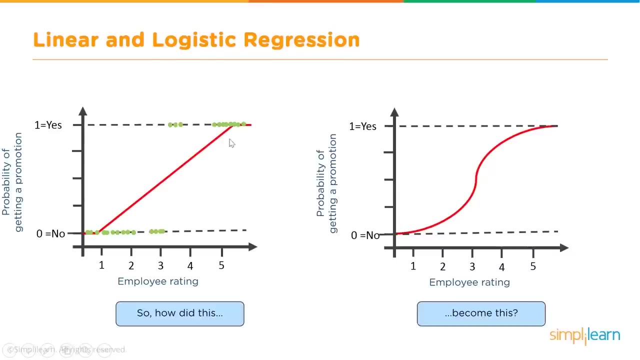 high, So the values cannot go beyond zero or beyond one. So the graph should probably look somewhat like this: clipped at zero and one, But still the straight line doesn't look right. Therefore, instead of using a linear equation, we need to come up with something different. 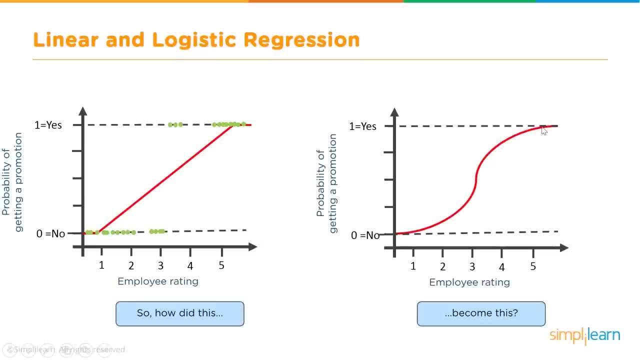 And therefore the logistic regression model looks somewhat like this. So we calculate the probability and if we plot that probability not in the proportion, it will be zero, And not in the form of a straight line, but we need to use some other equation. 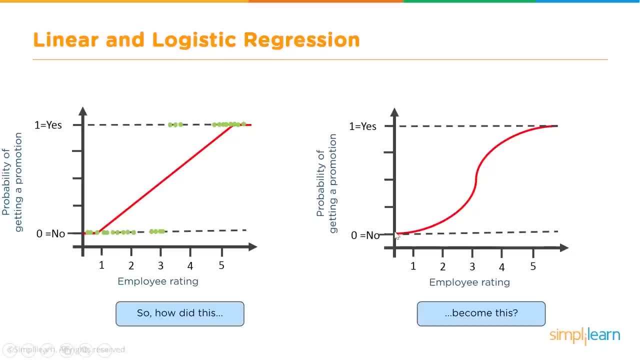 We will see very soon what that equation is. Then it is a gradual process. So you see here, people with some of these ratings are not getting any promotions, And then slowly, at certain rating, they get promotion. So that is a gradual process. 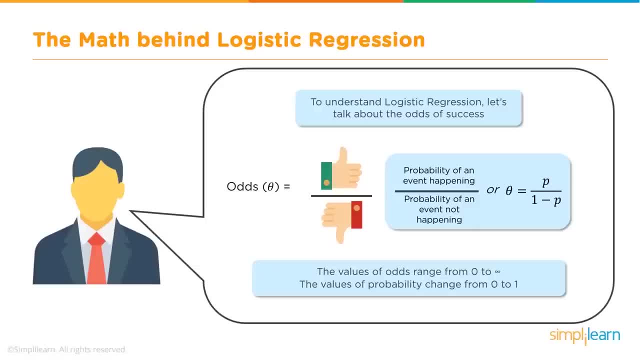 And this is how the math behind logistic regression looks. So we are trying to find the odds for a particular event happening. And this is the formula for finding the odds. So the probability of an event happening divided by the probability of the event not happening. 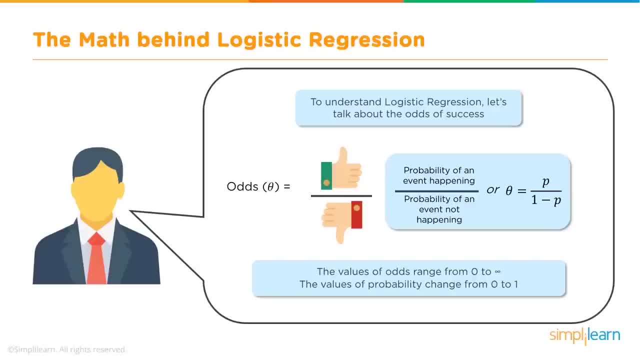 So p if it is the probability of the event happening- probability of the person getting a promotion- and divided by the probability of the person not getting a promotion, That is one minus p. This is how you measure the odds. Now, the values of the odds range from zero to infinity. 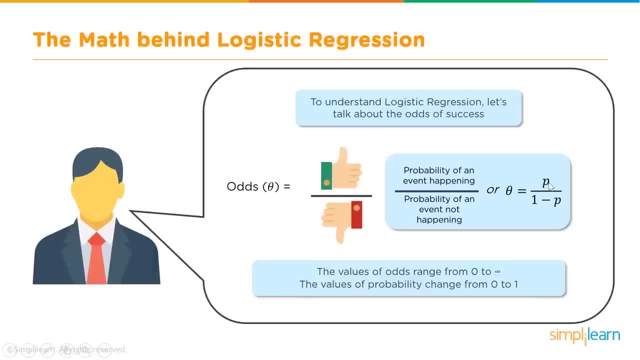 So when this probability is zero, Then the value of the odds is equal to zero, And when the probability becomes one, then the value of the odds is one by zero. That will be infinity, But the probability itself remains between zero and one. 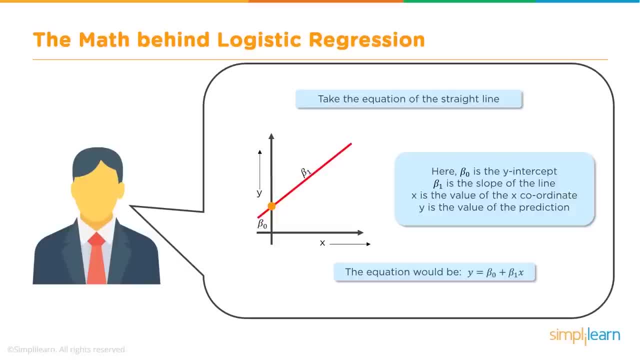 Now this is how an equation of a straight line looks. So y is equal to beta zero plus beta one, x, where beta zero is the y-intercept and beta one is the slope of the line. If we take the odds equation And take a log of p. 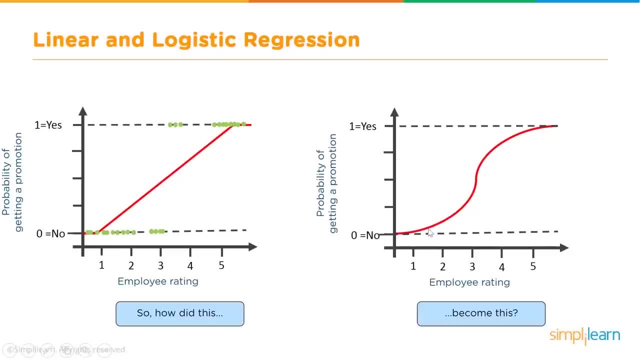 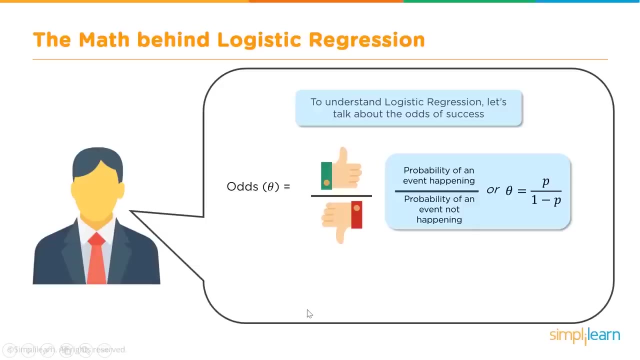 what that equation is, then it is a gradual process, right? so you see here, people with some of these ratings are not getting any promotions, and then, slowly, at certain rating, they get promotion. so that is a gradual process and this is how the math behind logistic regression looks. so we are trying to find the odds. 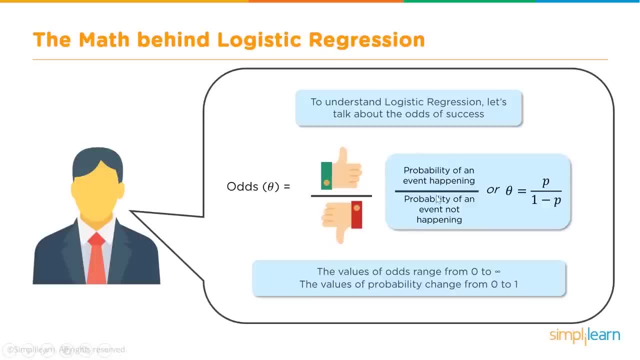 for a particular event happening and this is the formula for finding the odds. so the probability of an event happening divided by the probability of the event not happening. so P if it is the probability of the event happening, probability of the person getting promotion, and divided by the probability of the person not getting a promotion, that is 1 minus. 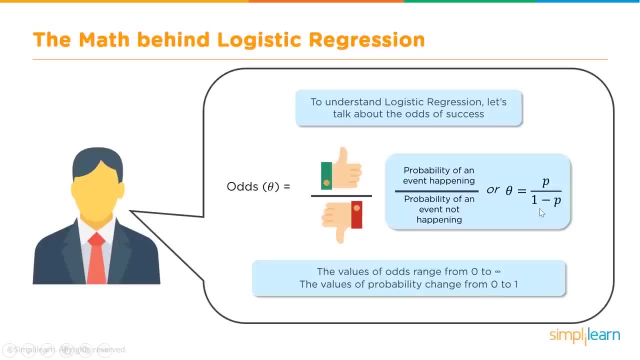 P. so this is how you measure the odds. now. the values of the odds range from 0 to infinity. so when this probability is 0, then the odds will. the value of the odds is equal to 0, and when the probability becomes 1, then the value of. 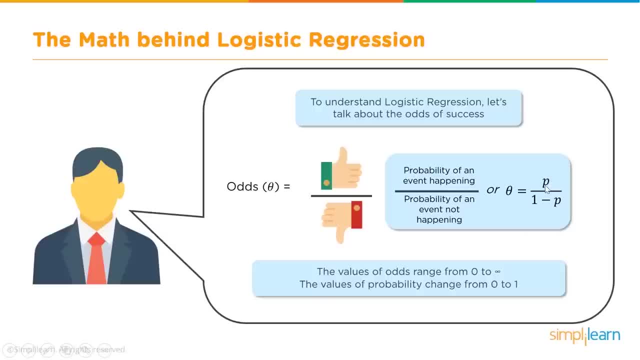 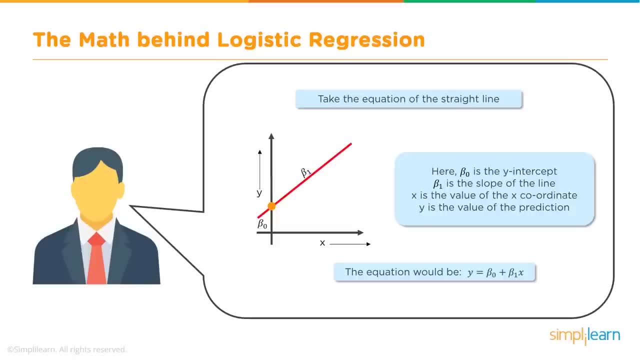 the odds is 1 by 0, that will be infinity, but the probability itself remains between 0 and 1.. now this is how an equation of a straight line looks. so y is equal to beta 0 plus beta 1, x, where beta 0 is the y intercept and beta 1 is the slope of the line. if we take the odds equation and take 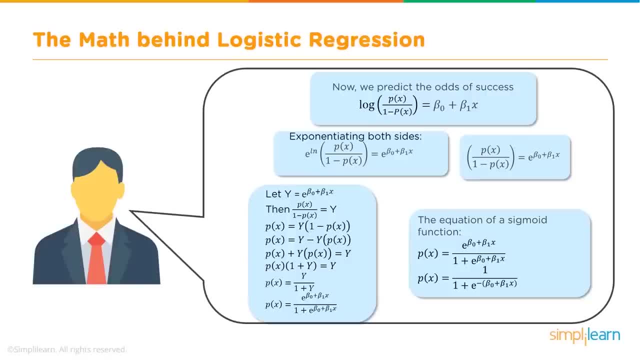 a log of both sides, then this would look somewhat like this, and the term logistic is actually derived from the fact that we are doing this. we take a log of px by 1 minus px. this is an extension of the calculation of odds that we have seen right and that is equal to beta 0 plus. 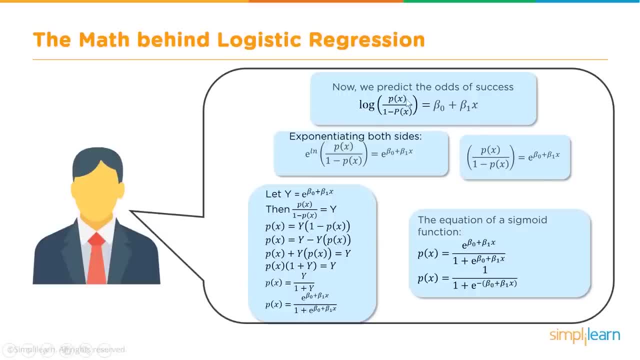 beta 1, x, which is the equation of the straight line. and now from here, if you want to find out the value of px, you will see we can take the exponential on both sides and then, if we solve that equation, we will get the equation of px like this: px is equal to 1 by 1 plus e to the power of. 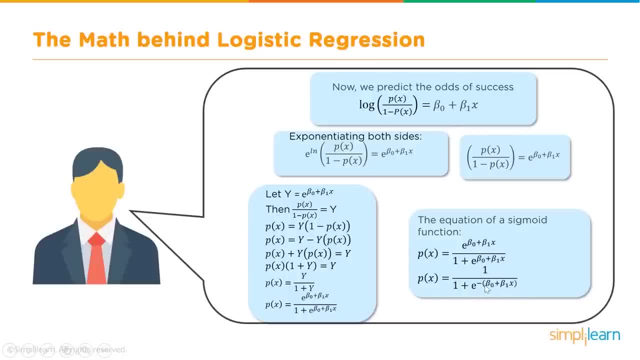 minus beta 0 plus beta 1 x, and recall this is nothing but the equation of the line which is equal to y. y is equal to beta 0 plus beta 1 x, so that this is the equation also known as the sigmoid function and this is the equation of the logistic regression. 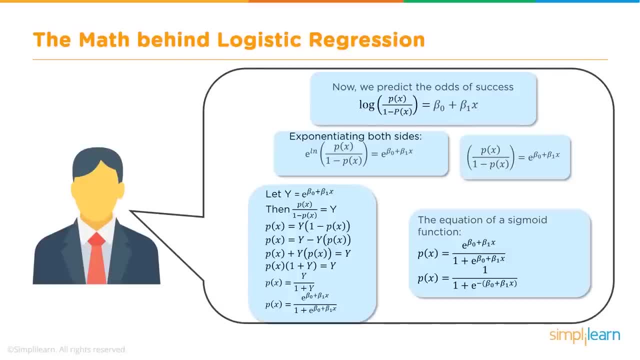 And then we get p, And then we get p Both sides. Then this would look somewhat like this, And the term logistic is actually derived from the fact that we are doing this. We take a log of p x by one minus p x. 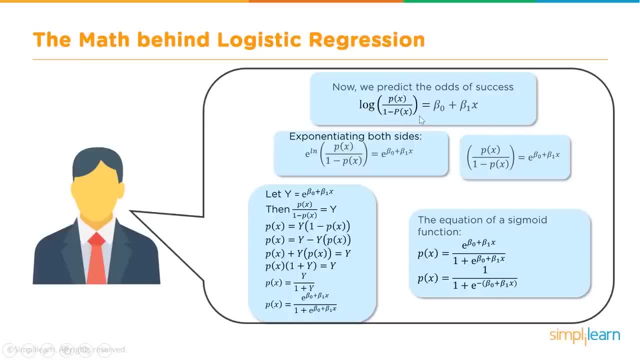 This is an extension of the calculation of odds that we have seen, And that is equal to beta zero plus beta one x, which is the equation of the straight line. And now, from here, if you want to find out the value of p x, 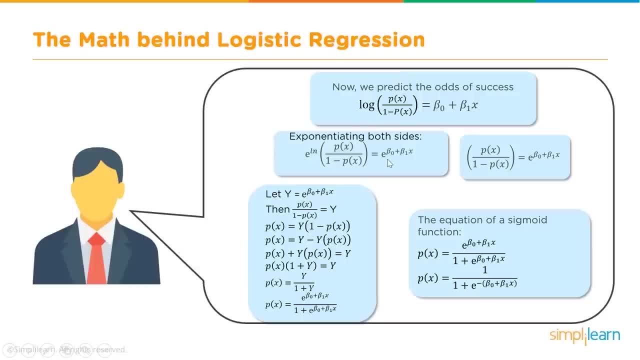 You will see, we can take the exponential on both sides. if we solve that equation, we will get the equation of px like this: px is equal to 1 by 1 plus e, to the power of minus beta 0 plus beta 1 x. and recall, this is nothing but the equation of the line which: 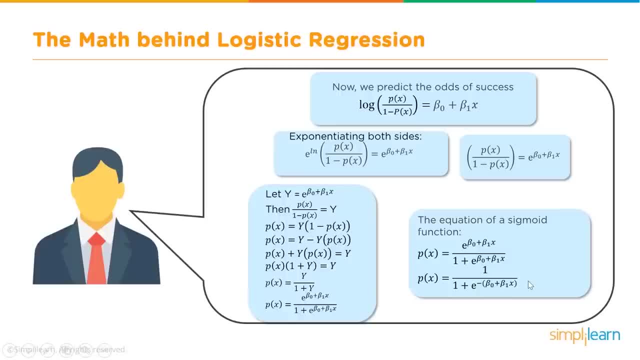 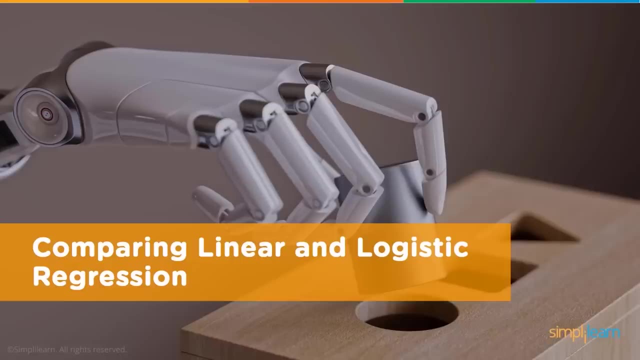 is equal to y, y is equal to beta 0 plus beta 1 x, so that this is the equation also known as the sigmoid function, and this is the equation of the logistic regression. all right, and if this is plotted, this is how the sigmoid curve is obtained. so let's compare linear and logistic regression. 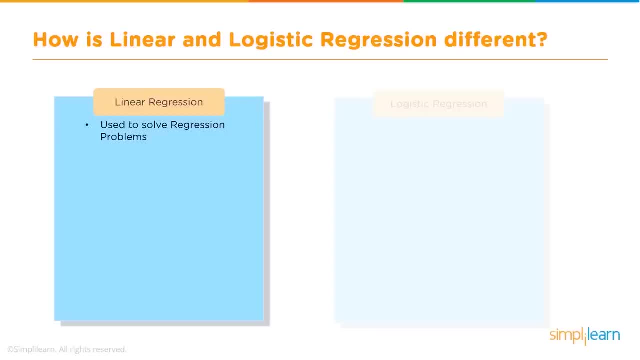 how they are different from each other. let's go back. so linear regression is solved or used to solve regression problems and logistic regression is used to solve classification problems. so both are called regression. but linear regression is used for solving regression problems where we predict continuous values, whereas logistic 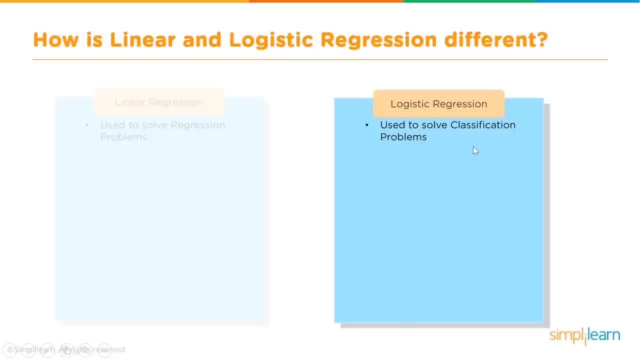 regression is used for solving classification problems where we have had to predict discrete values. the response variables in case of linear regression are continuous in nature, whereas here they are categorical or discrete in nature, and linear regression helps to estimate the dependent variable when there is a change in the independent variable, whereas here, in case of logistic. 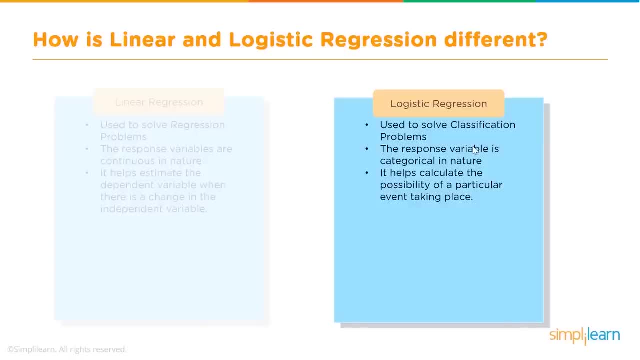 regression. it helps to calculate the probability or the possibility of a particular event happening, and linear regression, as the name suggests, is a straight line. that's why it's called linear regression, whereas logistic regression is a sigmoid function and the curve is. the shape of the curve is. 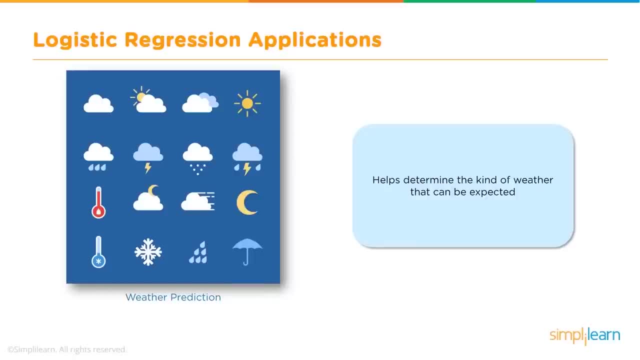 s, it's an s-shaped curve. this is another example of application of logistic regression in weather prediction: whether it's going to rain or not rain. now, keep in mind both are used in weather prediction if we want to find the discrete values like whether it's going to rain or not rain. 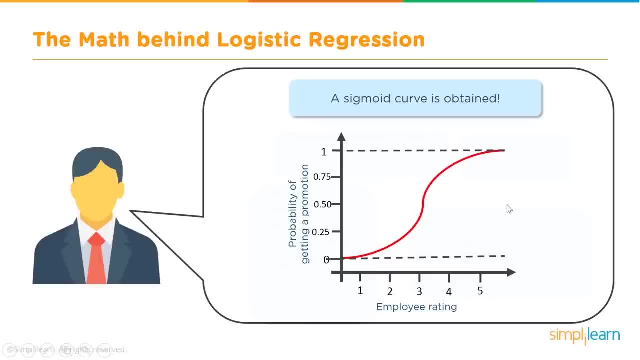 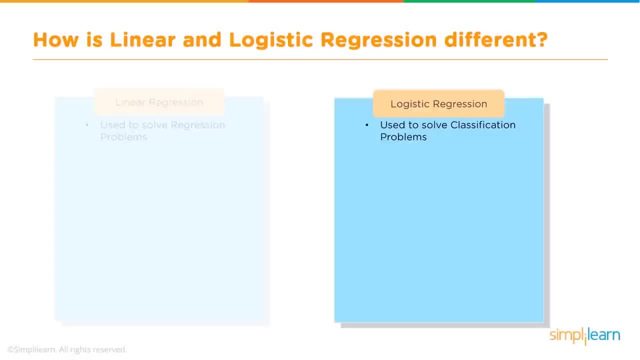 all right. and if this is plotted, this is how the sigmoid curve is obtained. so let's compare linear and logistic regression, how they are different from each other. let's go back. so linear regression is solved or used to solve regression problems and logistic regression is used to solve classification problems. so both are called. 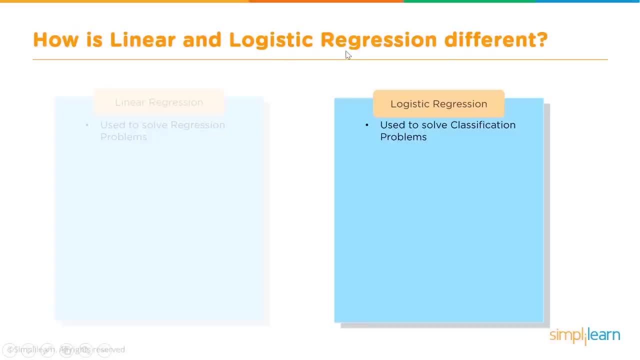 regression. but linear regression is used for solving regression problems where we predict continuous values, whereas logistic regression is used for solving classification problems where we have have to predict discrete values. the response variables in case of linear regression are continuous in nature, whereas here they are categorical or discrete in nature, and 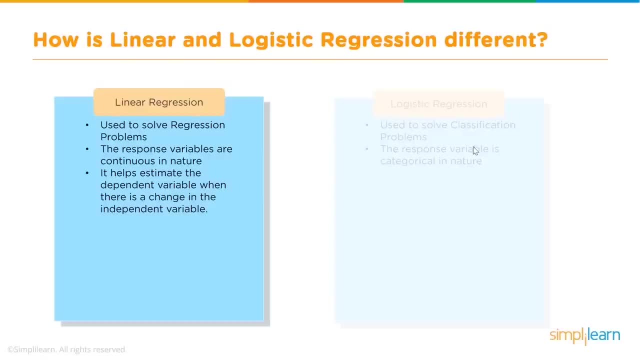 linear regression helps to estimate the dependent variable when there is a change in the independent variable, whereas here, in case of logistic regression, it helps to calculate the probability or the possibility of a particular event happening. and linear regression, as the name suggests, is a straight line. that's why it's called linear regression, whereas logistic regression is a sigmoid. 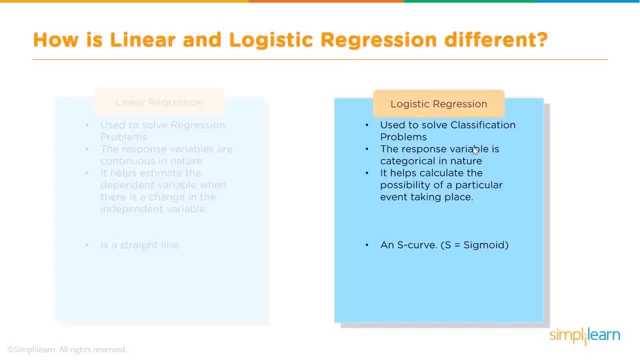 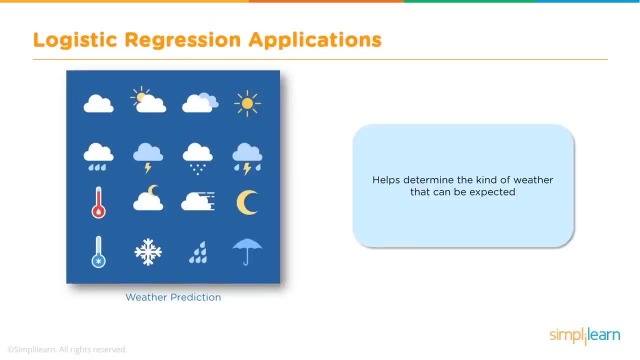 function and the curve is. the shape of the curve is s, it's an s-shaped curve. this is another example of linear regression. we're going to be studying linear regression, which is the vocal cleft. give us a way to navigate thistam flying downга. 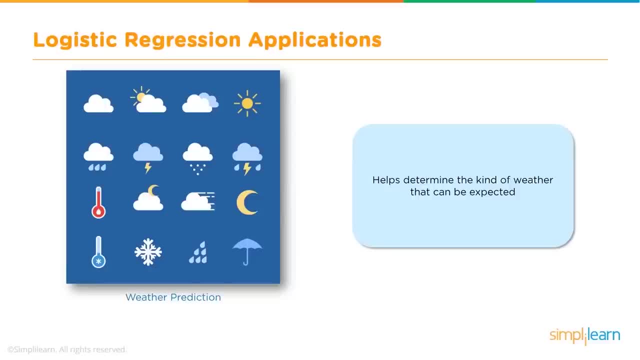 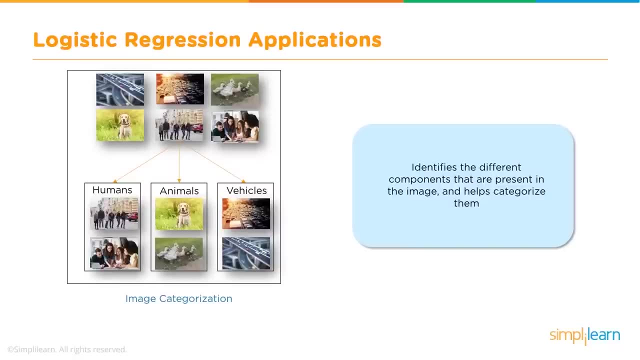 to reg to find the whether it's going to rain or not, whether it's going to be sunny or not, whether it's going to snow or not. These are all logistic regression examples. A few more examples: Classification of objects. This is again another example of logistic regression. 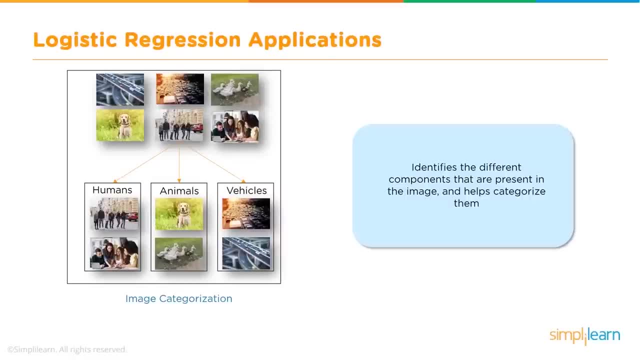 Now here, of course, one distinction is that these are multi-class classification, So logistic regression is not used in its original form, but it is used in a slightly different form. So we say: whether it is a dog or not a dog. I hope you understand. So, instead of saying: is it a dog or a cat or an elephant? 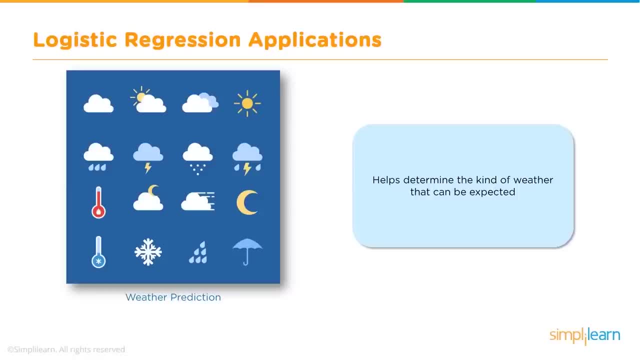 that is a classification problem. we use logistic regression. but if we want to determine what is going to be the temperature tomorrow, then we use linear regression. so just keep in mind that in weather prediction we actually use both. but these are some examples of logistic regression. so we want 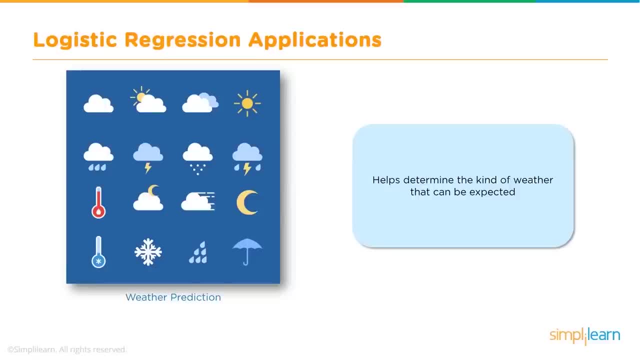 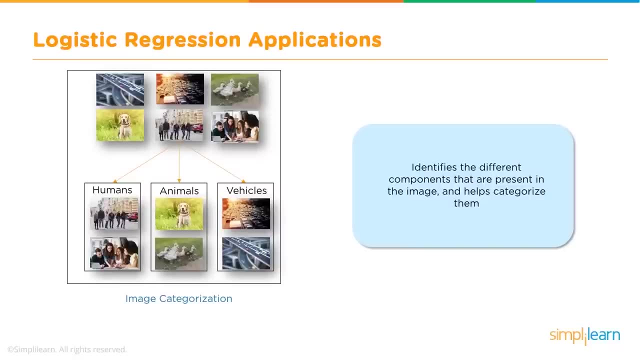 to find out whether it's going to rain or not, it's going to be sunny or not, it's going to snow or not. these are all logistic regression examples. a few more examples: classification of objects. this is a again another example of logistic regression, now here. of course, one distinction is that these are multi-class classification, so logistic regression. 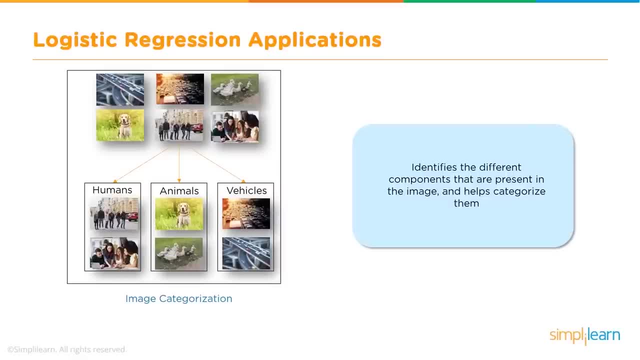 is not used in its original form, but it is used in a slightly different form. so we say whether it is a dog or not a dog. i hope you understand. so instead of saying is it a dog or a cat or elephant, we convert this into saying so because we need to keep it to binary classification. so we say: is it a dog? 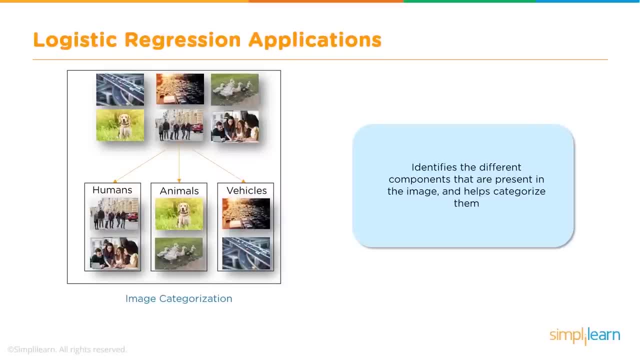 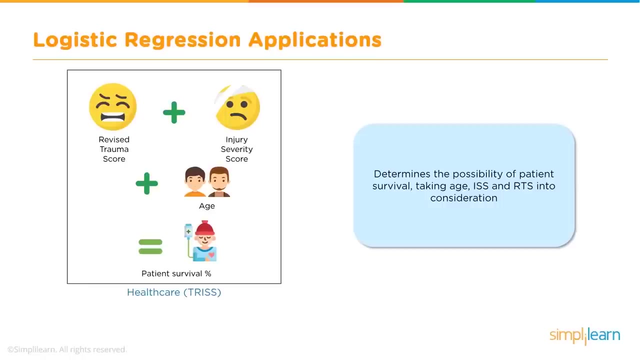 or not a dog, is it a cat or not a cat? so that's the way logistic regression can be used for classifying objects. otherwise, there are other techniques which can be used for performing multi-class classification. in healthcare, logistic regression is used to find the survival rate of a. 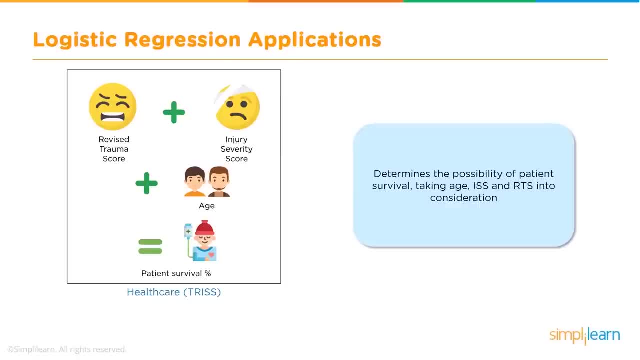 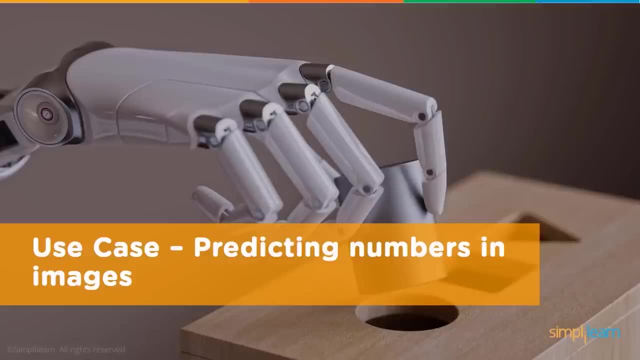 patient. so they take multiple parameters like trauma score and age and so on and so forth, and they try to predict the rate of survival. all right. now, finally, let's take an example and see how we can apply logistic regression to predict the number that is shown in the image. so this is. 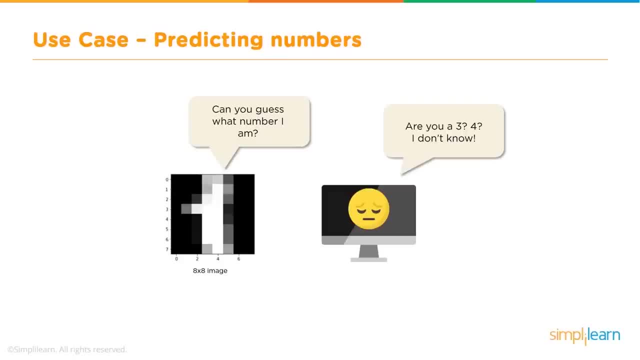 actually a live demo. i will take you into jupiter notebook and show the code, but before that let me take you through a couple of slides to explain what we are trying to do. so let's say you have an 8 by 8 image and there the image has a number one, two, three, four and you need to train your 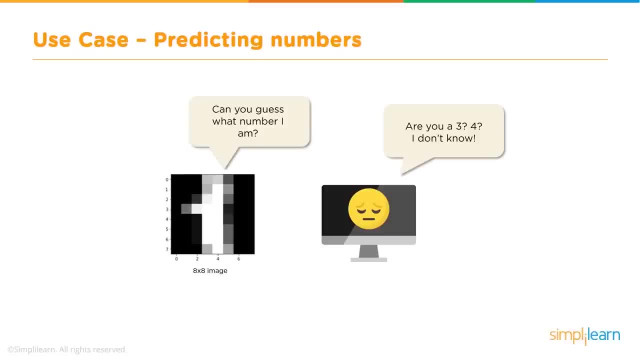 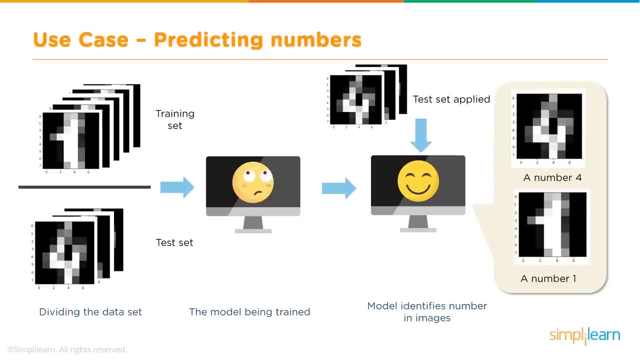 model to predict what this number is. so how do we do this? so the first thing is that we need to do is, obviously, in any machine learning process, you train your model. so in this case, we are using logistic regression, so, and then we provide a training set to train the model, and then we test. 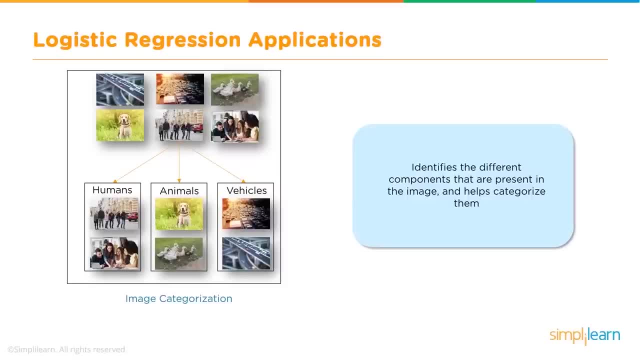 we convert this into saying So because we need to keep it to binary classification. So we say: is it a dog or not a dog, Is it a cat or not a cat? So that's the way logistic regression can be used for classifying. 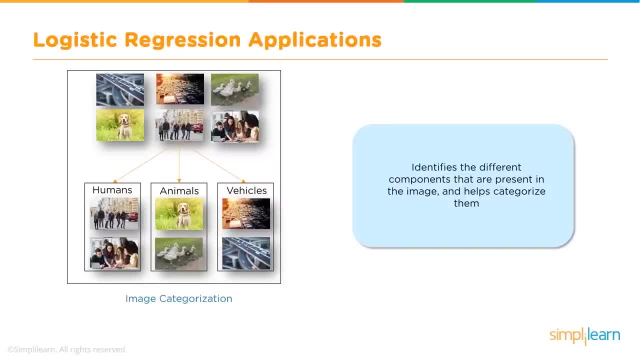 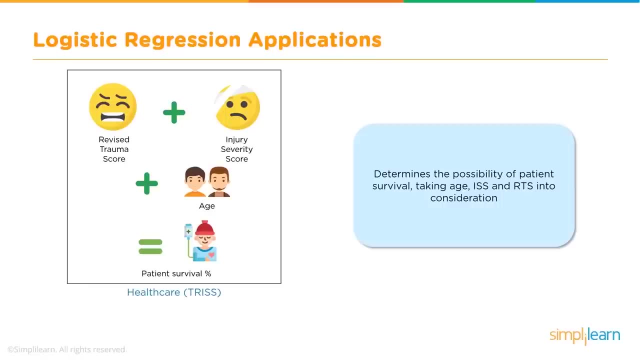 objects. Otherwise, there are other techniques which can be used for performing multi-class classification. In healthcare, logistic regression is used to find the survival rate of a patient. So they take multiple parameters like trauma score and age and so on and so forth, and they try to predict the rate of survival. 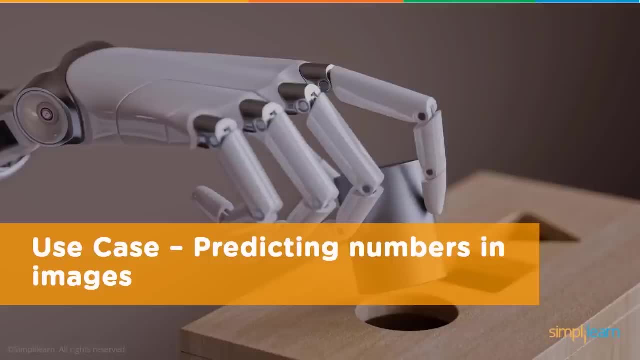 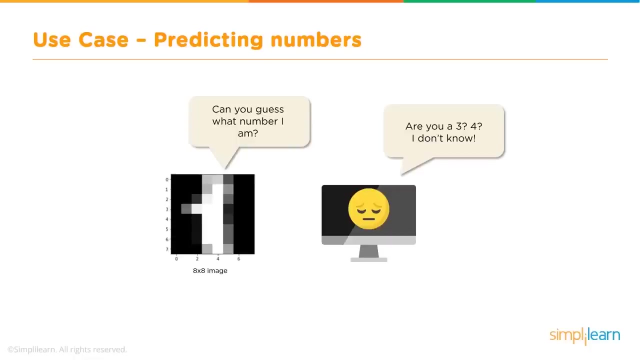 All right. Now, finally, let's take an example and see how we can apply logistic regression to predict the number that is shown in the image. So this is actually a live demo. I will take you into Jupyter notebook and show the code, But before that, let me take you through a couple of slides to explain what we are trying. 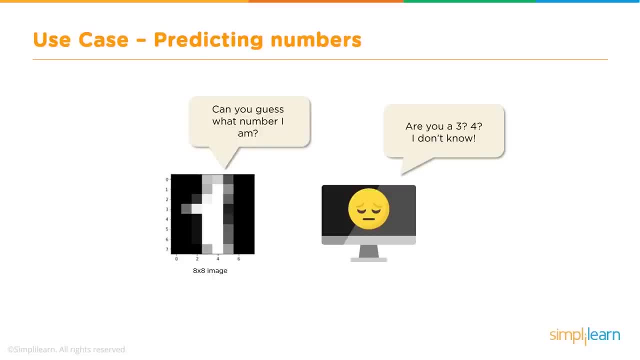 to do So. let's say you have an eight by eight image and the image has a number- one, two, three, four- and you need to train your model to predict what this number is. So how do we do this? So the first thing is obviously: in any 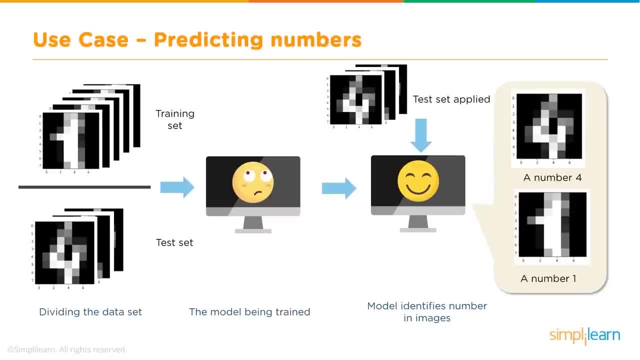 machine learning process. you train your model, So in this case, we are using logistic regression, So, and then we provide a training set to train the model, and then we test how accurate our model is with the test data, which means, like any machine learning process, we split our initial data into two parts. 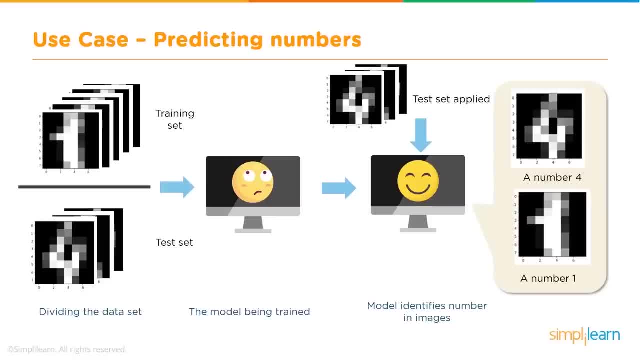 training set and test set. with the training set we train our model, and then, with the test set, we test the model till we get good accuracy and then we use it for for inference right. so that is typical methodology of training, testing and then deploying of machine learning models. so let's take a look at the code. 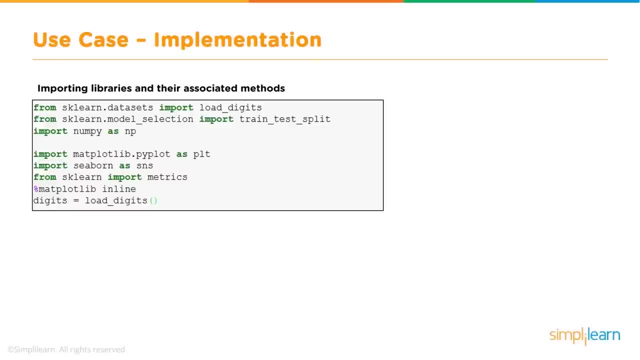 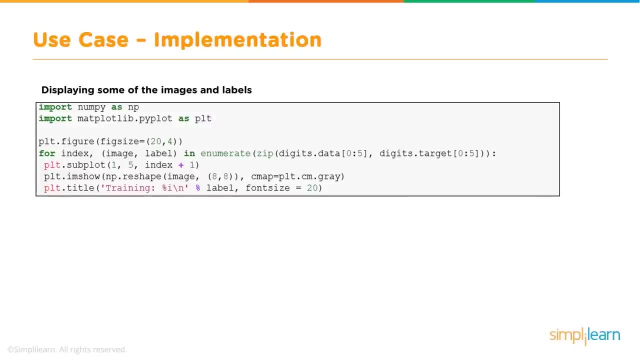 and see what we are doing. so I will not go line by line, but just take you through some of the blocks. so first thing we do is import all the libraries and then we basically take a look at the images and see what is the total number of images we can display using matplotlib. some of the images or a sample: 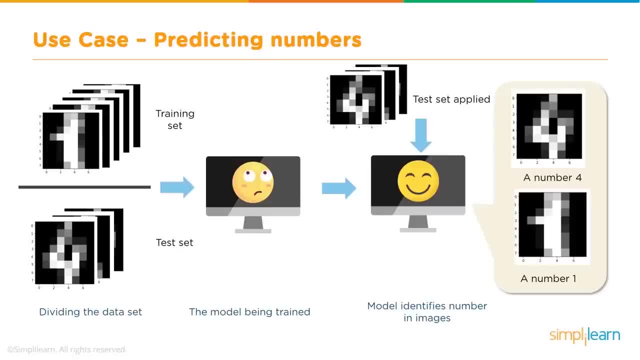 how accurate our model is with the test data, which means that, like any machine learning process, we split our initial data into two parts: training set and test set. with the training set, we train our model and then, with the test set, we test the model till we get good accuracy and then we use it. 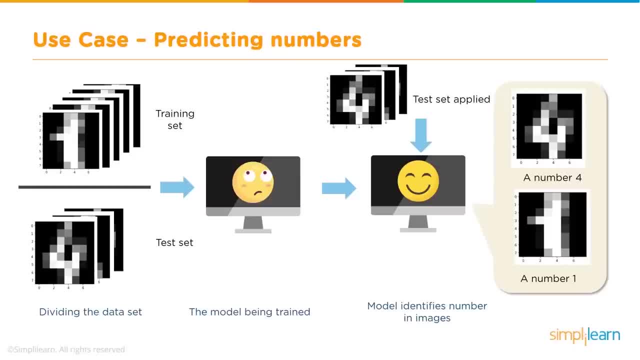 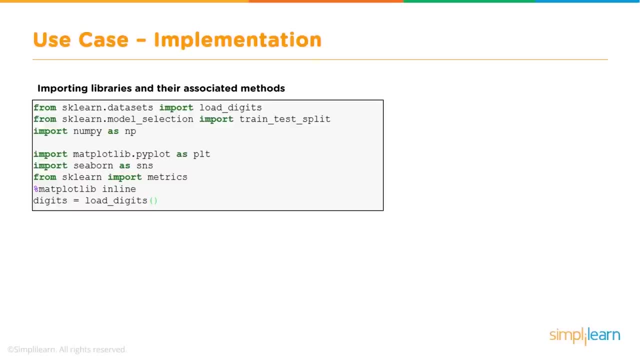 for for inference right. so that is typical methodology of training, testing and then deploying of machine learning modules. so let's take a look at the code and see what we are doing. so i will not go line by line, but just take you through some of the blocks. so first thing we do 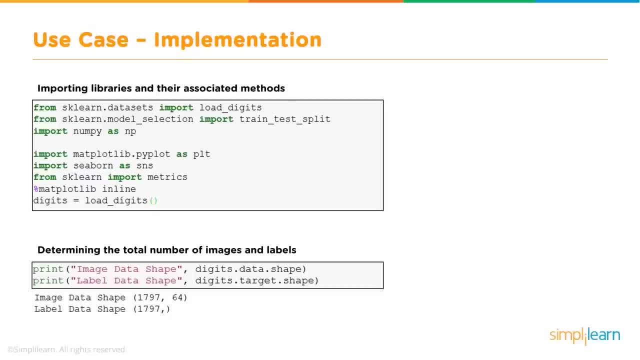 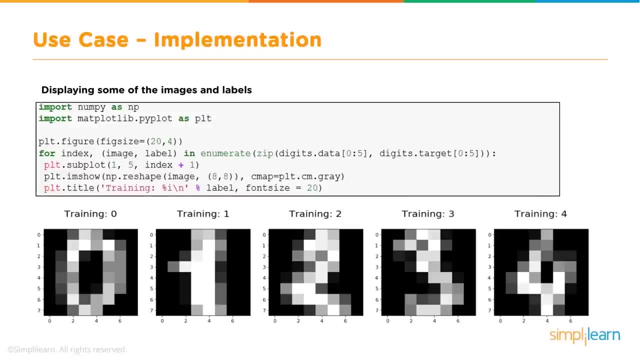 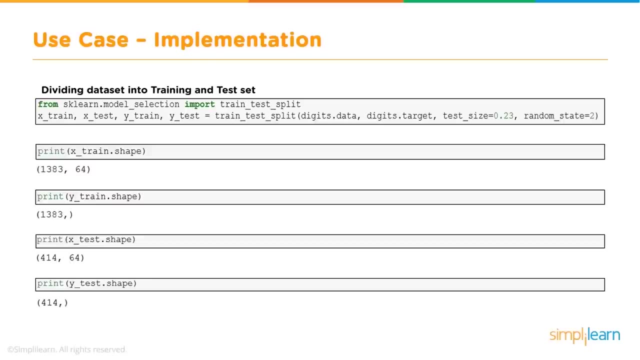 is import all the libraries and then we basically take a look at the images and see what is the total number of images we can display using matplotlib. some of the images, sample of these images- and then we split the data into training and test, as i mentioned earlier. 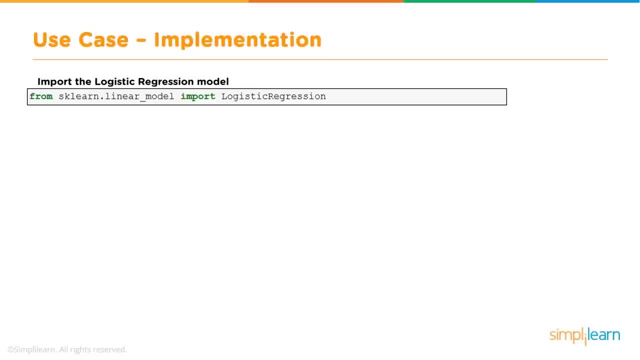 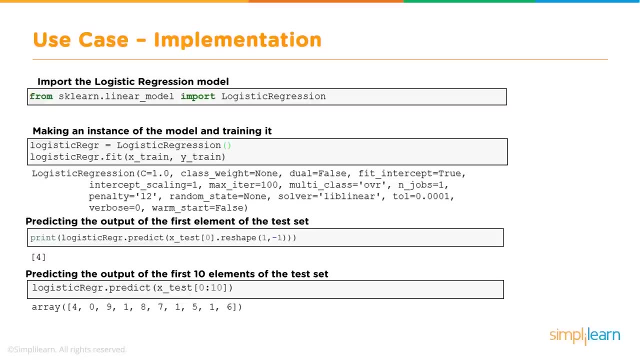 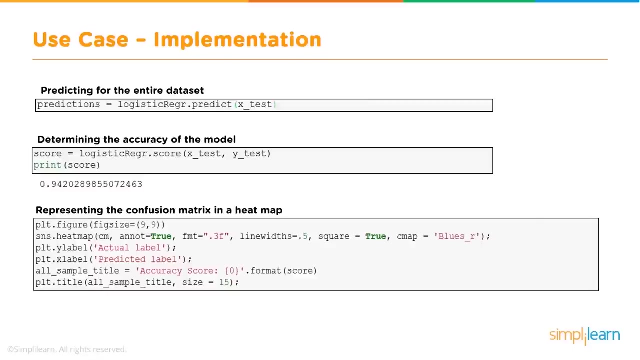 and we can do some exploratory analysis and then we build our model, we train our model with the training set and then we test it with our test set and find out how accurate our model is using the confusion matrix, the heat map, and use heat map for visualizing this and i will show you in. 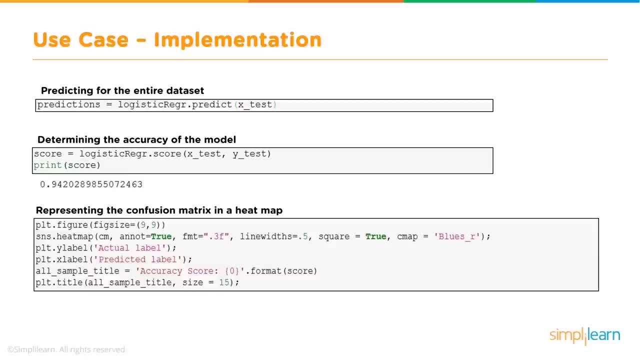 the code, what exactly is the confusion matrix and how it can be used for finding the accuracy. in our example we got, we get an accuracy of about 0.94, which is pretty good, or 94, which is pretty good, all right. so what is the confusion matrix? this? 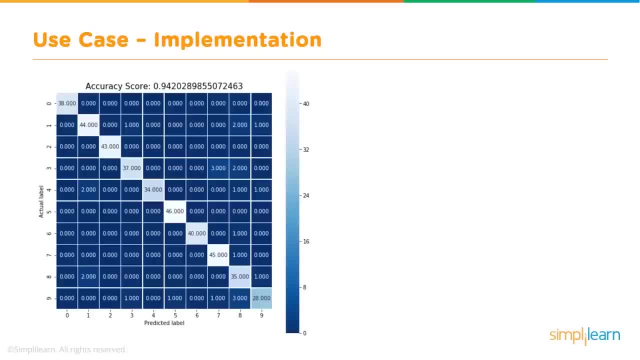 is an example of a confusion matrix and this is used for identifying the accuracy of a classification model like a logistic regression model. so the most important part in a confusion matrix is that first is the matrix- in this case we have some numbers, and then this is a matrix and the size of the 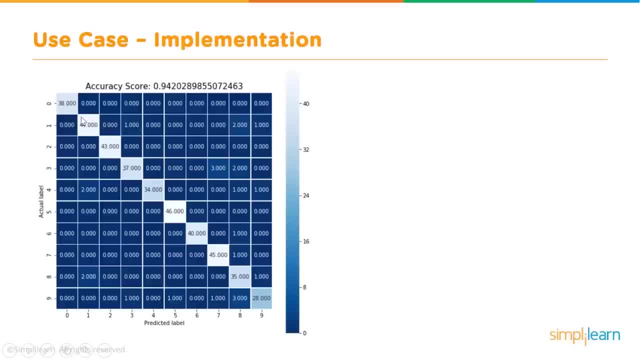 matrix depends on how many outputs we are expecting right. so the most important part here is that the model will be most accurate when we have the maximum numbers in its diagonal, like in this case. that's why it has almost 93- 94 percent, because the diagonals should have the maximum numbers and the 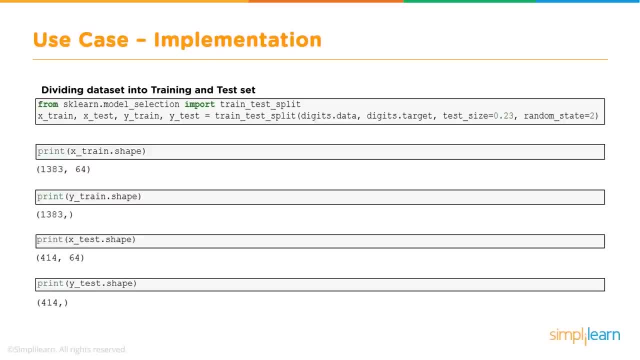 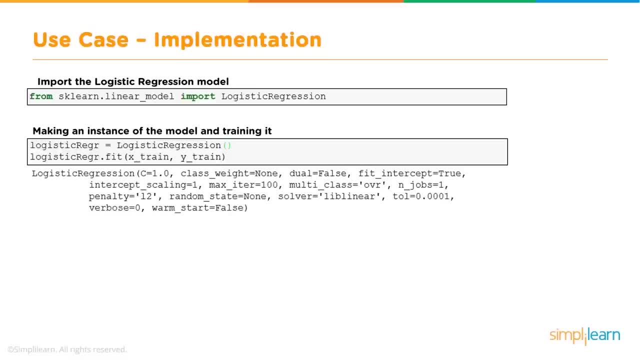 of these images and then we split the data into training and test, as I mentioned earlier, and we can do some exploratory analysis, and then we build our model, we train our model with the training set and then we test for the code in this particular set. gotta look like a few steps: ask for the code, if necessary, and then we test and, if necessary, take. 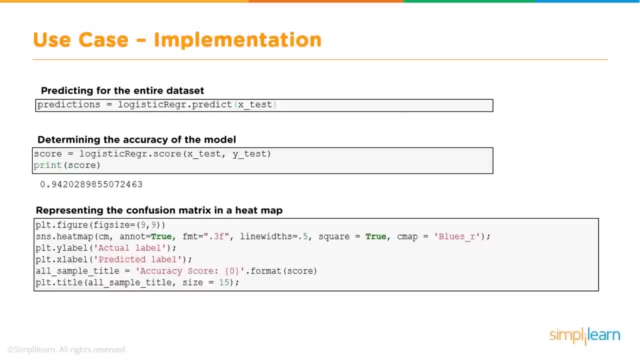 and we test for the code after the test. and then we test for the code, and then we test, test it with our test set and find out how accurate our model is, using the confusion matrix, the heat map, and use heat map for visualizing this and I will show you in the. 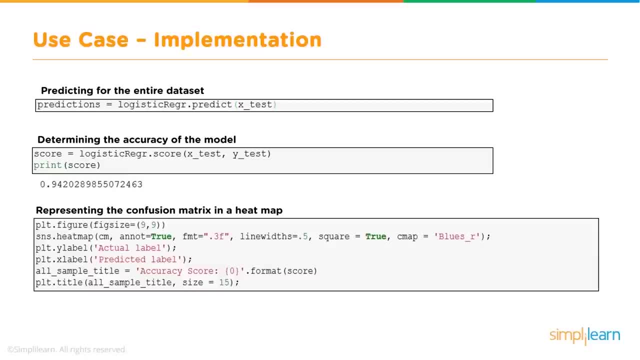 code, what exactly is the confusion matrix and how it can be used for finding the accuracy. In our example, we get an accuracy of about 0.94, which is pretty good, or 94%, which is pretty good, Alright. so what is the confusion matrix? 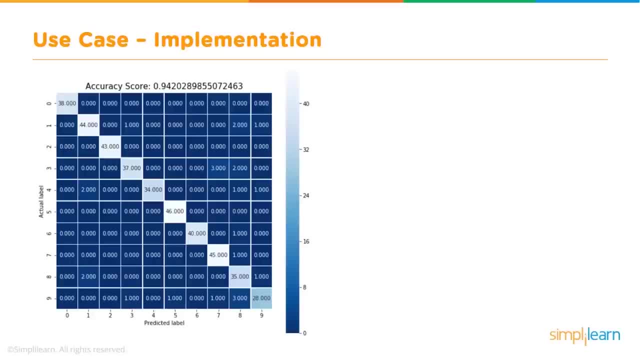 This is an example of a confusion matrix, and this is used for identifying the accuracy of a classification model, like a logistic regression model. So the most important part in a confusion matrix is that, first of all, as you can see, this is a matrix and the size of the matrix depends on how many outputs we are expecting. 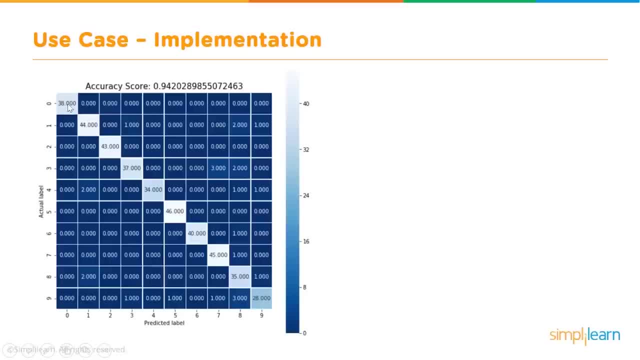 So the most important part here is that the model will be most accurate when we have the maximum numbers in its diagonal, like in this case. that's why it has almost 93, 94%, because the diagonals should have the maximum numbers and the others, other than diagonals, the cells. 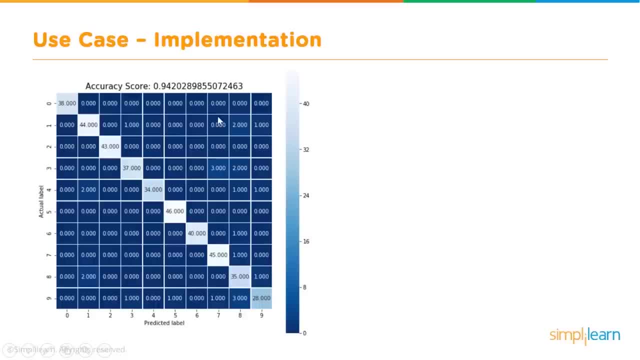 other than the diagonals should have very few numbers. So here that's what is happening. So there is a 2 here, there is a 1 here, but most of them are along the diagonal. What does this mean? This means that the number that has been found 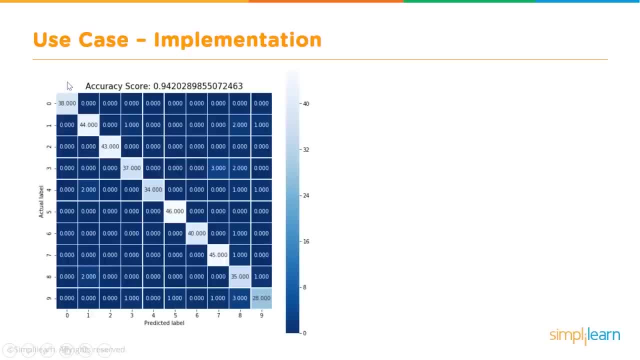 fed is 0 and the number that has been detected is also 0. So the predicted value and the actual value are the same. So, along the diagonals, that is true, which means that let's, let's, take this diagonal right. If the maximum number is here, that means that, like here in this case, it is 34, which means 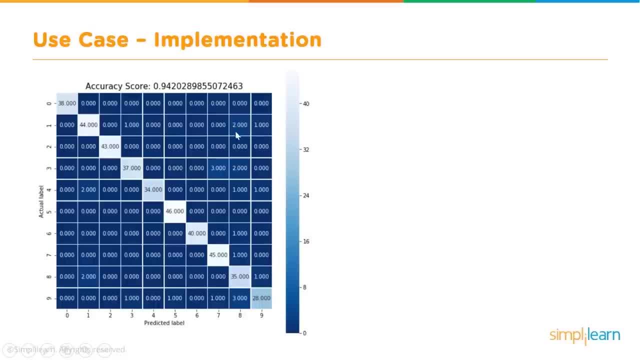 others, other than diagnostic cells, other than the diagonals, should have very few numbers. so if i see some other elements, then that video we're going to use that way. we're going to here. that's what is happening. so there is a two here, there are, there's a one here, but most of them. 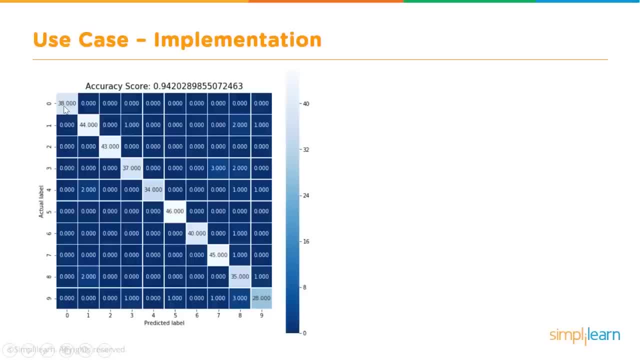 are along the diagonal this. what does this mean? this means that the number that has been fed is zero and the number that has been detected is also zero, so the predicted value and the actual value are the same. so, along the diagonals, that is true, which means that let's, let's take this diagonal. 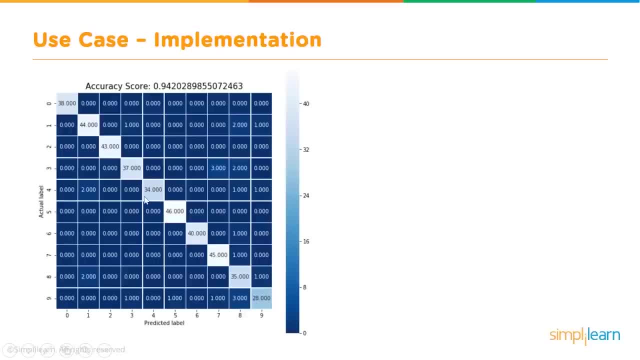 right, if the maximum number is here, that means that, uh, like here in this case, it is 34, which means that 34 of the images that have been fed- or rather, actually there are two misclassifications in there- so 36 images have been fed which have number four, and out of which 34 have been. 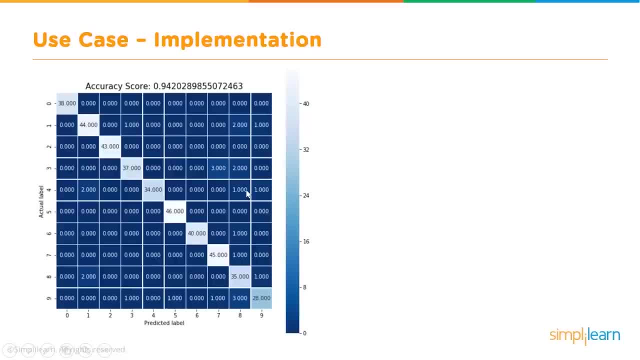 predicted correctly as number four, and one has been predicted as number eight and another one has been predicted as number nine. so these are two misclassifications. okay, so that is the meaning of saying that the maximum number should be in the diagonal. so if you have all of them, so for an ideal model which has, let's say, 100 accuracy, everything will be. 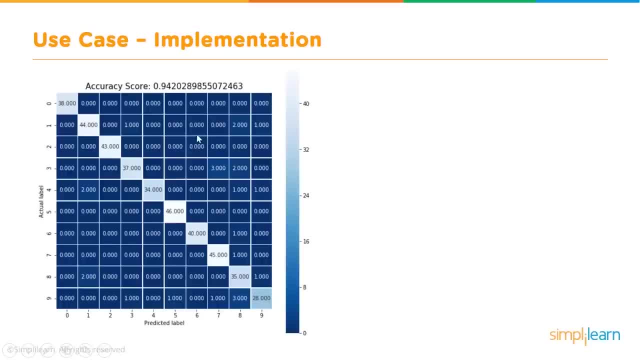 only in the diagonal. there will be no numbers other than zero in all other cells. but that is like a hundred percent accurate model. okay, so that's uh just of how to use this matrix. uh, how to use this uh confusion matrix. i know the name uh is a little funny sounding: confusion matrix. 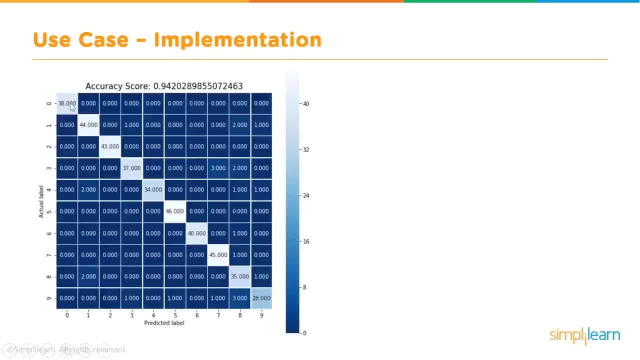 but actually it is not very confusing, it's very straightforward. so you are just plotting what has been predicted and what is the labeled information or what is the actual data. that's also known as the ground truth sometimes- okay, these are some fancy terms that are used, so 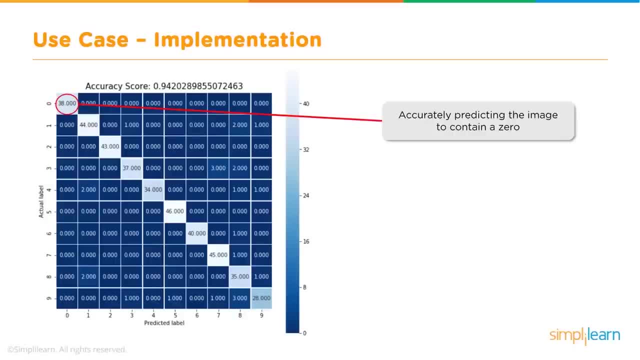 predicted label and the actual name. that's all it is okay. yeah, so we are showing a little bit more information here. so 38 have been predicted and here you will see that all of them have been predicted correctly. there have been 38 zeros and the predicted value and the 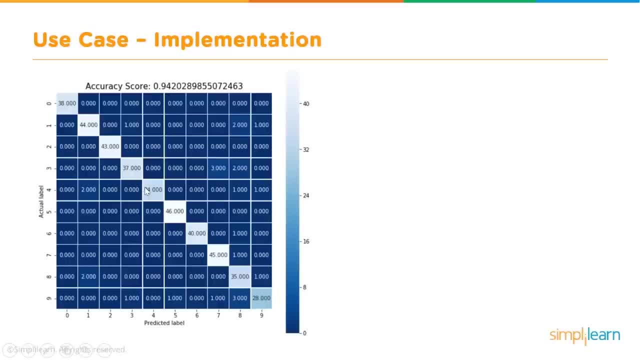 that 34 of the images that have been fed, or rather, actually there are two misclassifications in there, So 36 images have been fed. Each have number 4, and out of which 34 have been predicted correctly as number 4 and one. 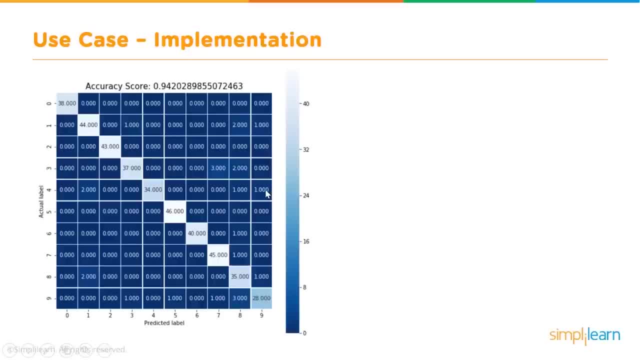 has been predicted as number 8 and another one has been predicted as number 9.. So these are two misclassifications. So that is the meaning of saying that the maximum number should be in the diagonal. So, if you have all of them, so for an ideal model which has, let's say, 100% accuracy, everything. 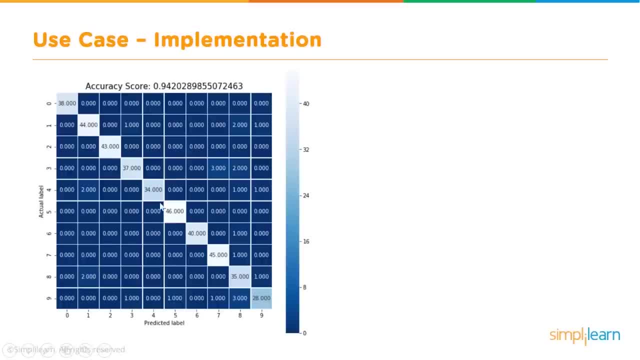 will be only in the diagonal. There will be no numbers other than 0 in all other cells. So that is like 100% accurate model. So that's just how to use this matrix, how to use this confusion matrix. I know the name is a little funny sounding- confusion matrix, but actually it is not very. 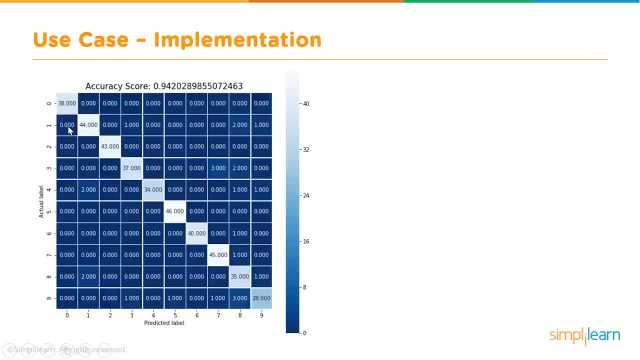 confusing. It's very straightforward. So you are just plotting what has been predicted and what is the label, information or what is the actual data. That's also known as the ground truth. sometimes These are some fancy terms that are used. So predicted label. 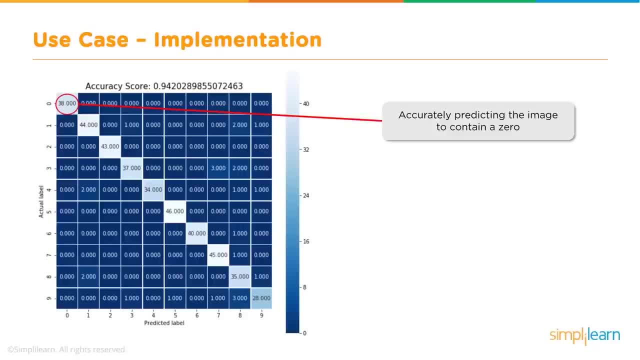 And actually that's all. it is OK. Yeah, So we are showing a little bit more information here. So 38 have been predicted and here you will see that all of them have been predicted correctly. There have been 38 zeros and the predicted value and the actual value is exactly the. 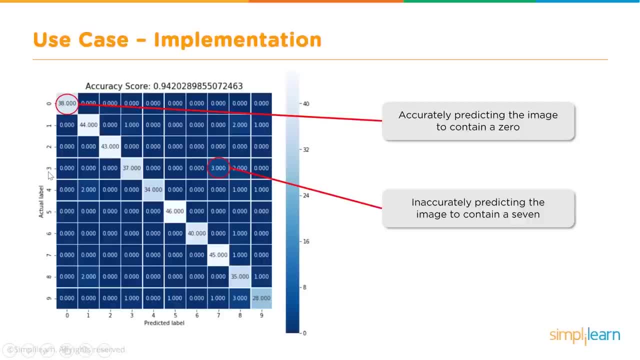 same, Whereas in this case, right it has. there are, I think, 37 plus 5, 42 have been fed the images. 42 images are of digit 3. And the accuracy is only 37 of them have been accurately predicted. three of them have been. 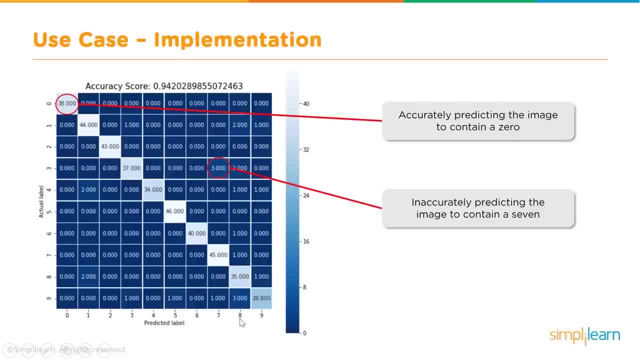 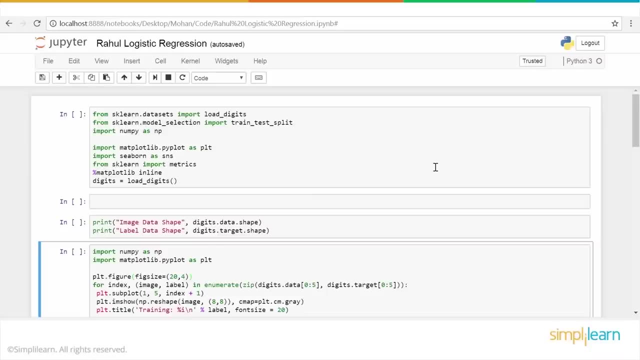 predicted as number seven, and two of them have been predicted as number eight, and so on and so forth. OK, All right. So with that let's go into Jupyter Notebook and see how the code looks. So this is the code in in Jupyter Notebook for logistic regression in this particular: 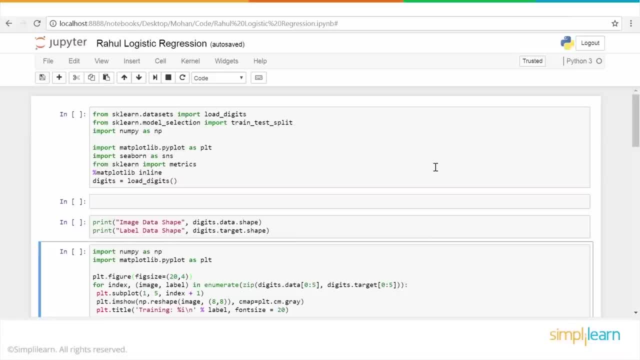 demo. What we are going to do is train our model To recognize Digits, Which are the images which have digits from, let's say, 0 to 5 or 0 to 9, and then we will see how well it is trained and whether it is able to predict these numbers correctly. 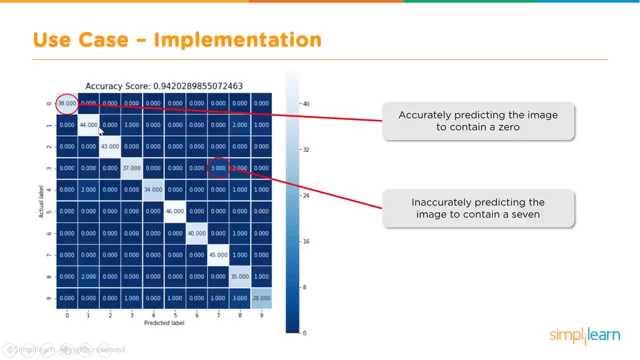 actual value is is exactly the same, whereas in this case, right, it has. uh, there are, i think, 37 plus five. yeah, 42 have been fed the images. 42 images are of digit 3 and the accuracy is only 37 of them have been accurately predicted. three of them have been predicted as number seven and two. 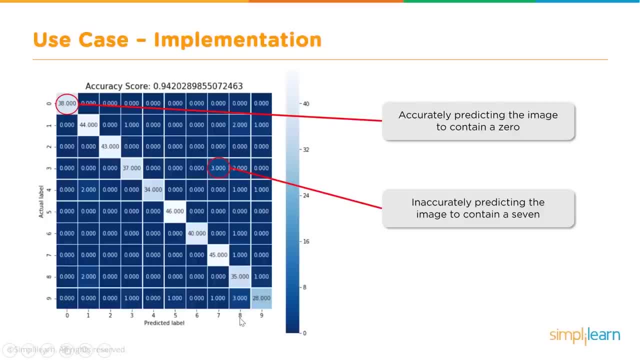 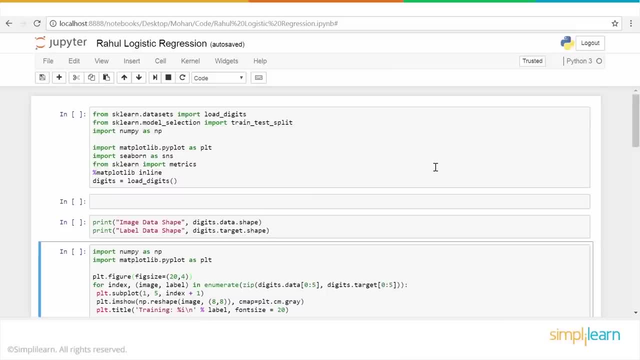 of them have been predicted as number eight, and so on and so forth. okay, all right. so with that, let's look and see how the code looks. so this is the code in in jupyter notebook for logistic regression in this particular demo, what we are going to do is train our model to recognize digits. 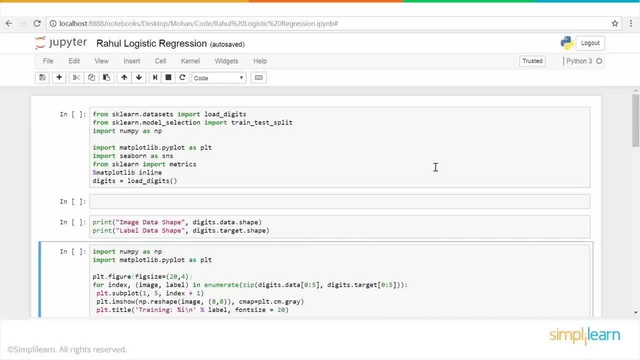 which are the images which have digits from, let's say, 0 to 5 or 0 to 9, and and then we will see how well it is trained and whether it is able to predict these numbers correctly or not. so let's get started. so the first part is, as usual, we are importing some libraries that are required. 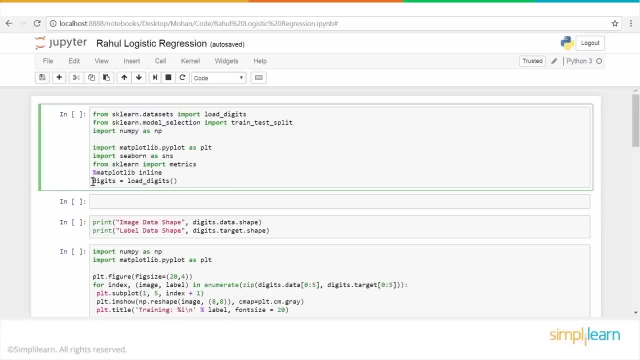 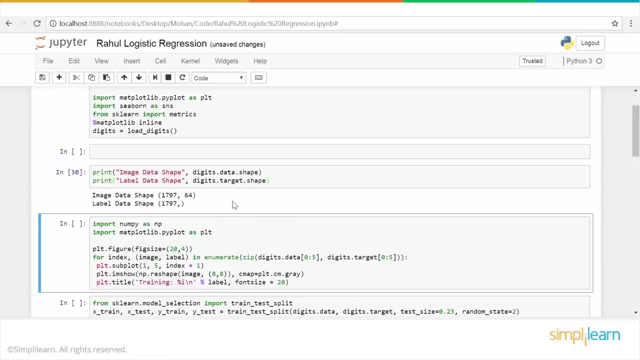 and then the last line and this block is to load the digits. so let's go ahead and run this code. then here we will visualize the shape of these uh digits so we can see here. if we take a look, this is how the shape is: 1797 by 64.. these are like 8 by 8. 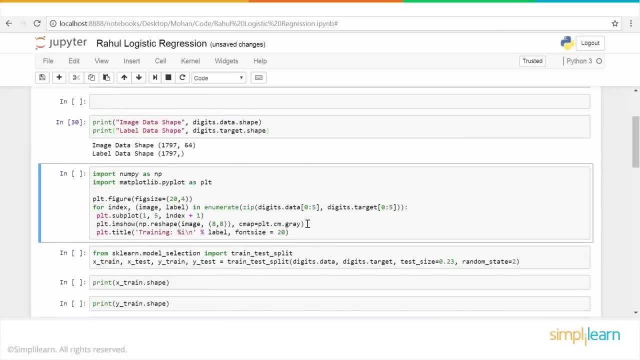 images. so that's that's what is reflected in this shape. now, from here onwards, we are basically once again importing some of the libraries that are required, like numpy and matplot, and we will take a look at some of the sample images that we have loaded. so this one for 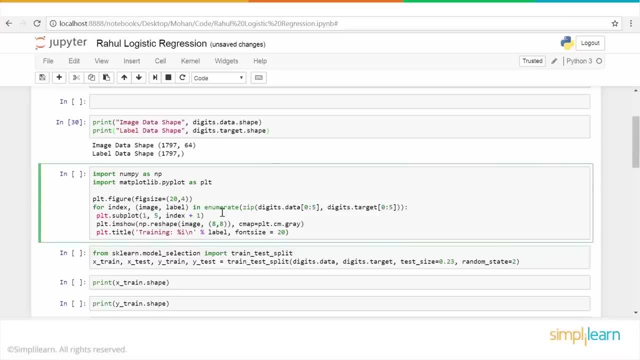 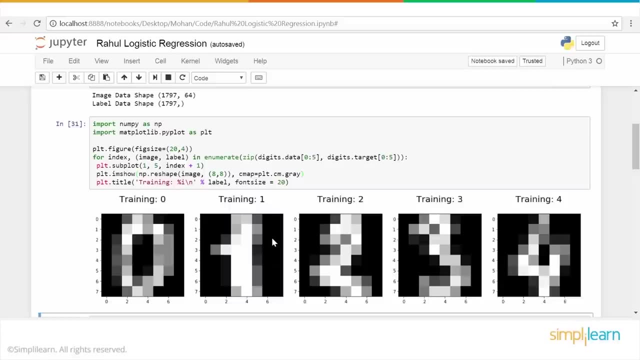 example, creates a figure and then we go ahead and take a few sample images to see how they look. so let me run this code and so that it becomes easy to understand. so these are about five images, sample images that we are looking at: zero, one, two, three, four. so this is. 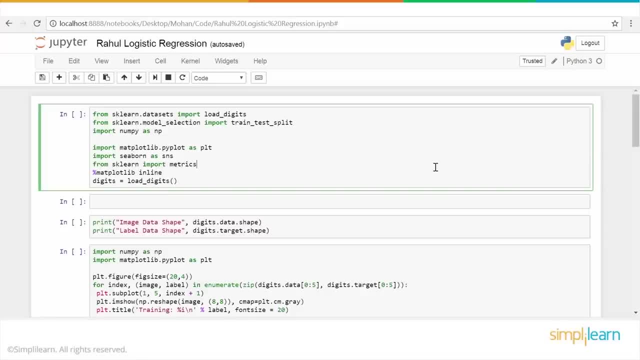 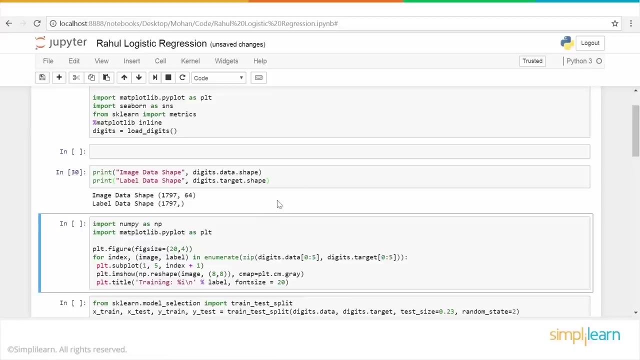 or not. So let's get started. So the first part is as usual. we are importing some libraries that are required, and then the last line and this block is to load the digits. So let's go ahead and run this code, Then here we will visualize the shape of these digits so we can see here if we take a look. 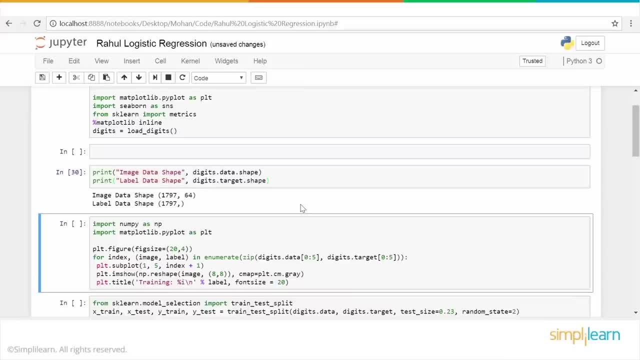 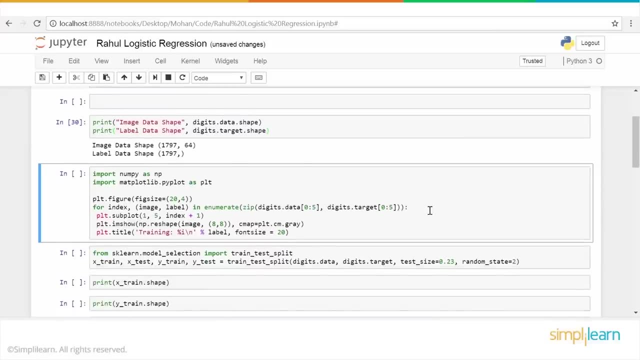 and this is how the shape is: 1797 by 64. These are like eight by eight images. So that's that's what is reflected in this shape. Now, from here onwards, we are basically once again importing some of the libraries that are required, like NumPy and Matplot. 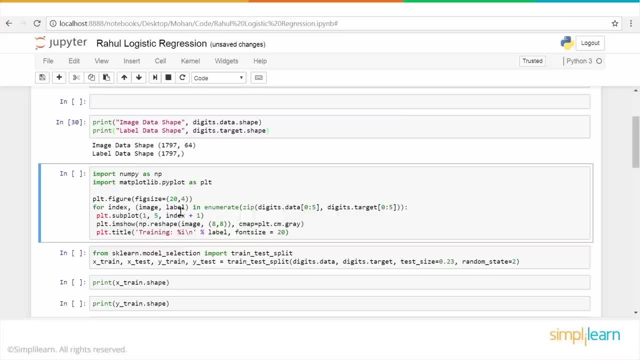 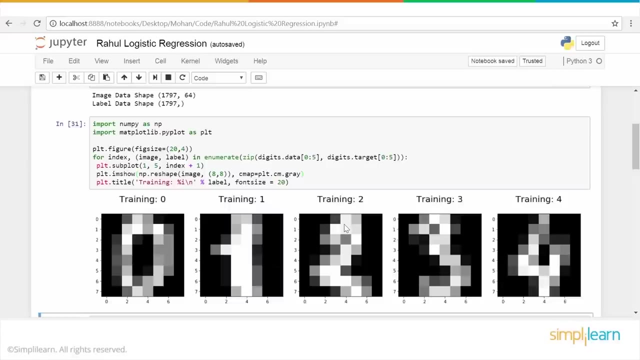 And we will take a look at Some of the Some of the sample images that we have loaded. So this one, for example, creates a figure and then we go ahead and take a few sample images to see how they look. So let me run this code and so that it becomes easy to understand. 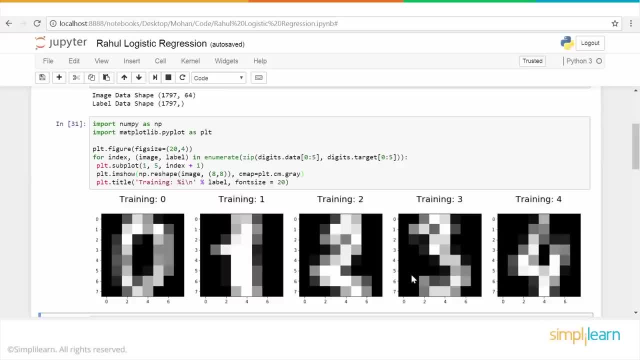 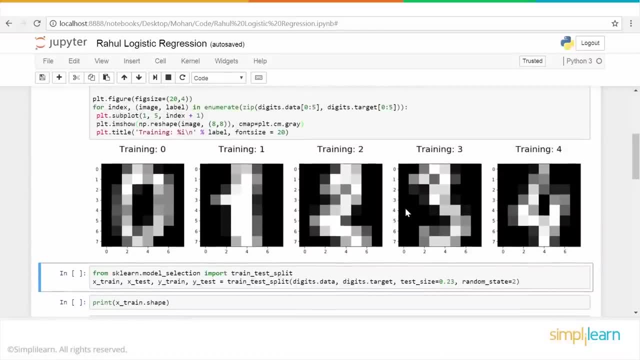 So these are about five images, sample images that we are looking at: 0, 1, 2, 3, 4.. So this is how the images, this is how the data is OK and based on this, we will actually train A logistic regression model and then we will test it and see how well it is able to recognize. 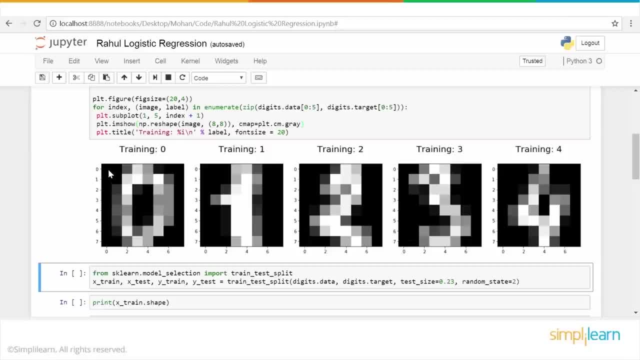 So the way it works is the pixel information. So, as you can see here, this is an eight by eight pixel kind of image and each pixel, whether it is activated or not activated, That is the information available for each pixel now, based on the pattern of this activation. 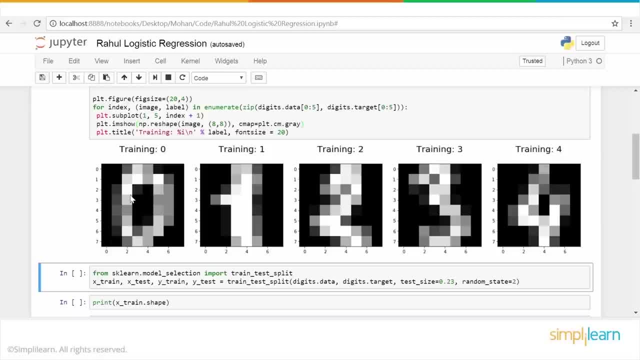 and non activation of the various pixels. This Is Identified As a zero, for example, Right, Similarly, as you can see. So overall, each of these numbers actually has a different pattern of the pixel activation, and that's pretty much that our model needs to learn. for which a number 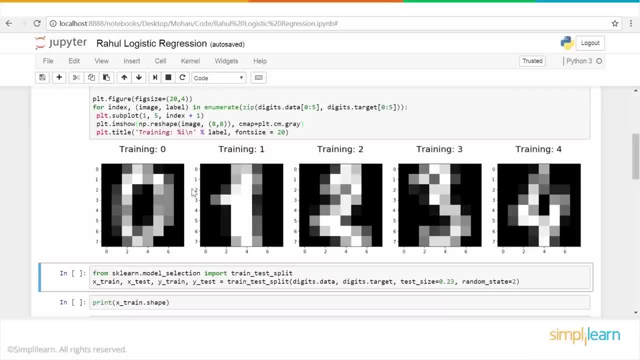 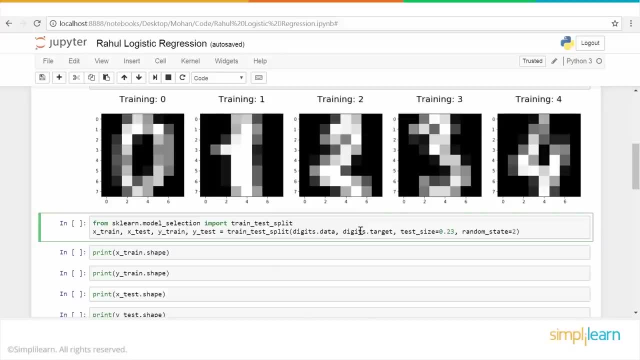 What is the pattern of the activation of the pixels? right, So that is what we are going to train our model. OK, So the first thing we need to do is to split our data into training, And This Is A split data set. 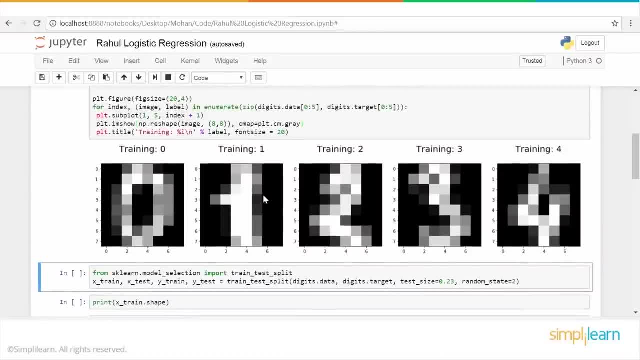 how the images. this is how the data is okay, and based on this we will actually train our logistic regression model and then we will test it and see how well it is able to recognize. so the way it works is the pixel information. so, as you can see here, this is an eight by eight pixel kind of a. 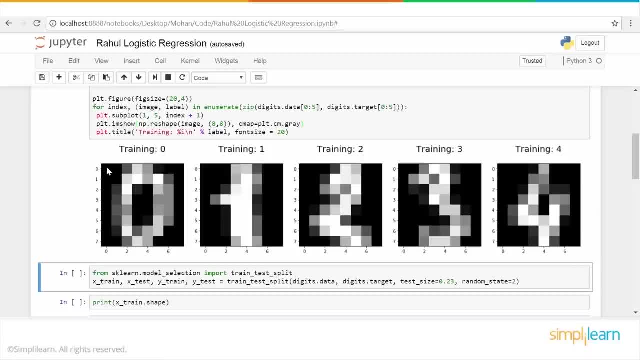 image and the each pixel, whether it is activated or not activated. that is the information available for each pixel. now, based on the pattern of this activation and non-activation of the various pixels, this will be identified as a zero, for example, right. similarly as you can see. so, overall, each of these numbers. 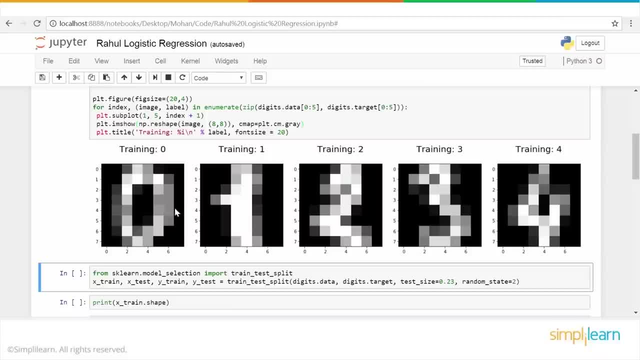 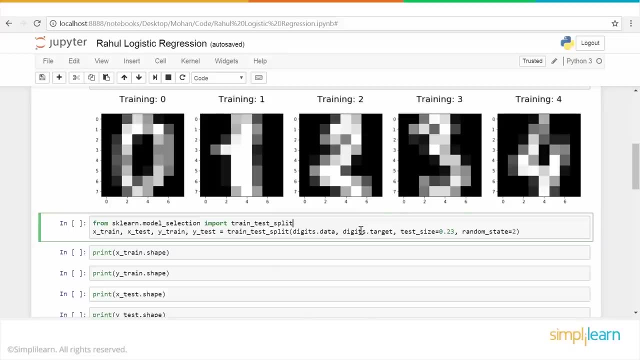 actually has a different pattern of the pixel activation, and that's pretty much that our model needs to learn. for which a number? what is the pattern of the activation of the pixels? right, so that is what we are going to train our model. okay, so the first thing we need to do is to split our data into training and test. 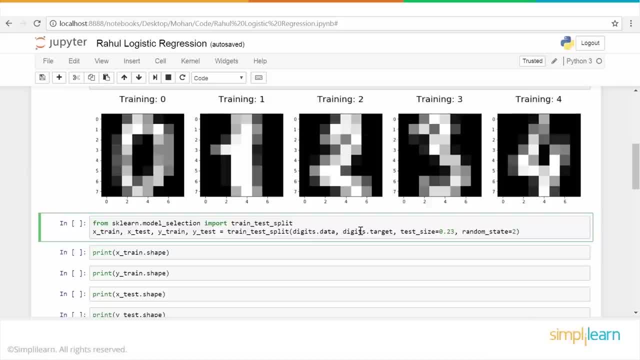 data set right. so whenever we perform any training, we split the data into training and test so that the training data set is used to train the system. so we pass this probably multiple times and then we test it with the test data set, and the split is usually in the form of the, and there are various 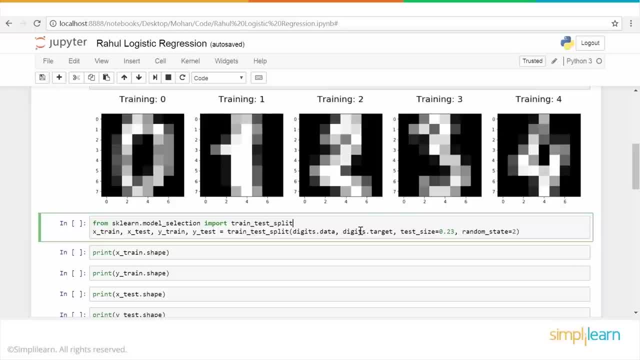 ways in which you can split this data. it is up to the individual preferences. in our case here we are splitting in the form of 23 and 77. so when we say test size as 20.23, that means 23 percent of that entire data is used for testing and the remaining 77 percent is used for training. so 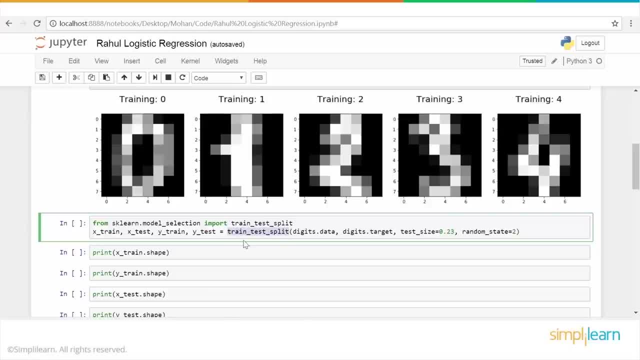 there is a readily available function which is called train test split, so we don't have to write any special code for the splitting. it will automatically split the data based on the proportion that we give here, which is test size. so we just give the test size automatically. 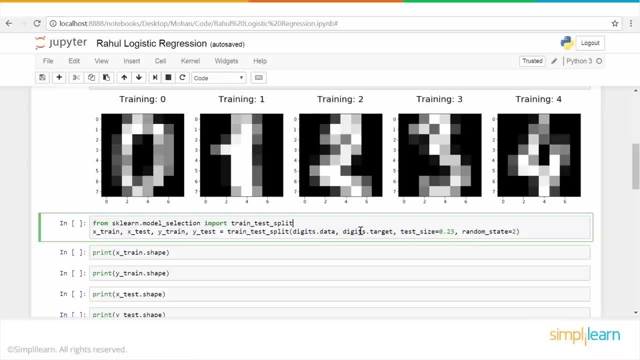 Right. So whenever we perform any training, we split the data into training and tests so that the training data set is used to train the system. So we pass this probably multiple times and then we test it with the test data set and the split is usually in the form of that and there are various ways in which you can split. 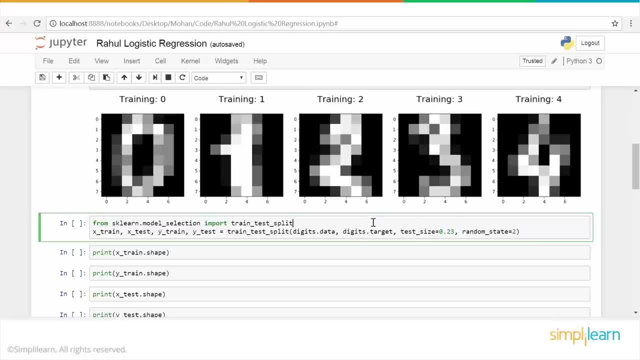 this data. It is up to the individual preferences. In our case, here we are splitting in the form of twenty three and seventy seven. So when we say test size as twenty point two three, That means twenty three percent of that entire data is used for testing and the remaining 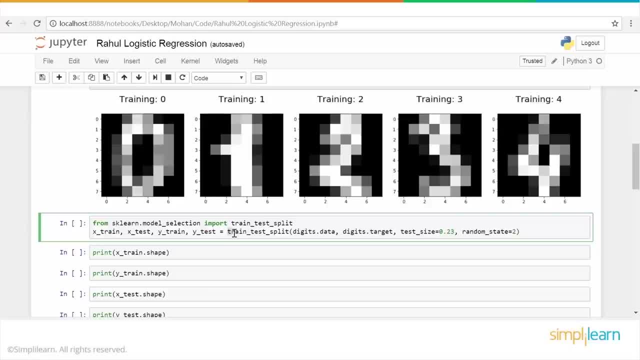 seventy seven percent is used for training. So there is a readily available function which is called train test split. So we don't have to write any special code for the splitting. It will automatically split the data based on the proportion that we give here, which. 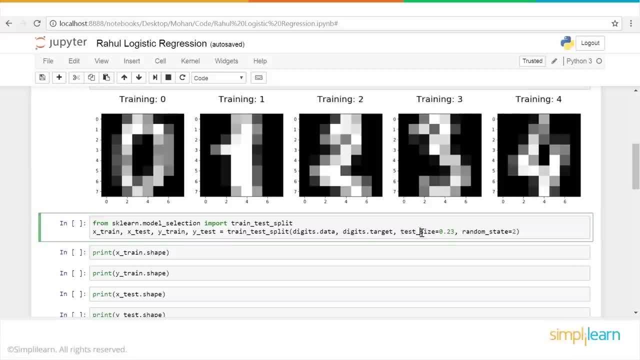 is test size. So we just give the test size, automatically training size will be determined and we pass the data that we want to split and the results will be stored in X underscore train and Y underscore train for the training data set. And what is X underscore train? 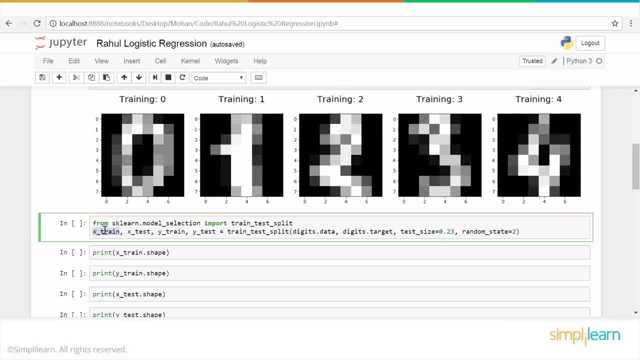 This: these are the features right, which is like the independent variable, and Y underscore train is the label right. So in this case, what happens is we have the input value, which is, Or the features value, which is in X underscore train, and since this is labeled data for each. 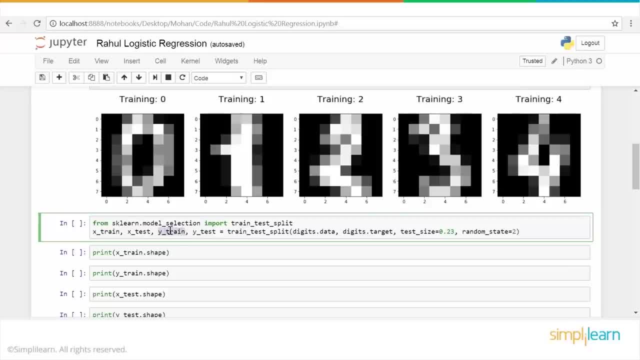 of them, each of the observations. we already have the label information saying whether this digit is a zero or a one or a two, so that this is what will be used for comparison to find out whether the system is able to recognize it correctly or there is an error. 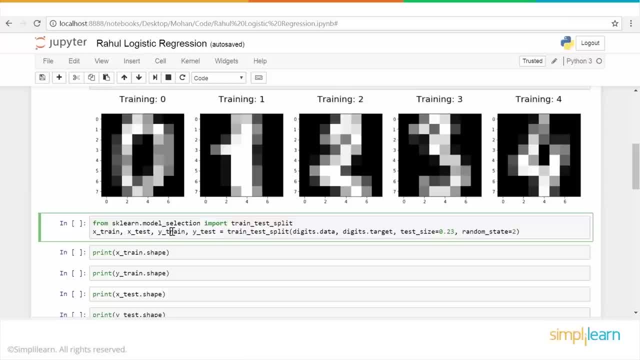 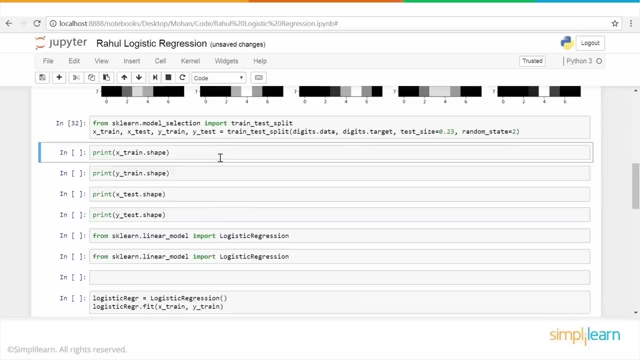 for each observation. it will compare with this right. So this is the label. So the same way, X underscore train, Y underscore train is for the training data set, X underscore test, Y underscore test is for the test data set. So let me go ahead and execute this code as well, and then we can go and check quickly. 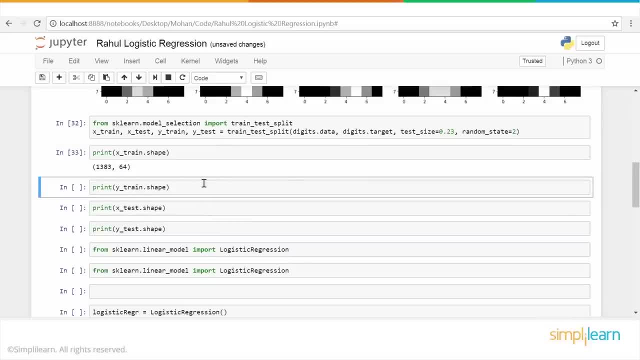 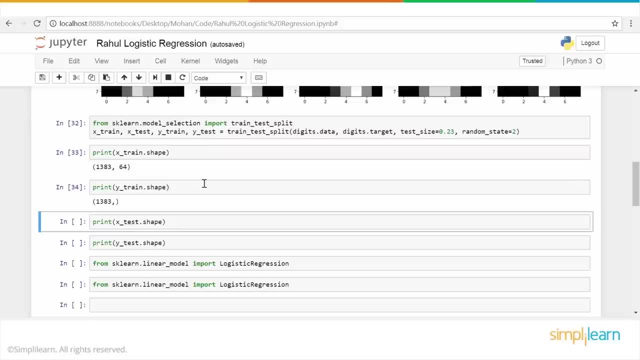 what is the? how many entries are there and in each of their? so? X underscore train, the shape is 1383 by 64, and Y underscore train has 1383, because there is nothing like the second part is not required here- And then X underscore. 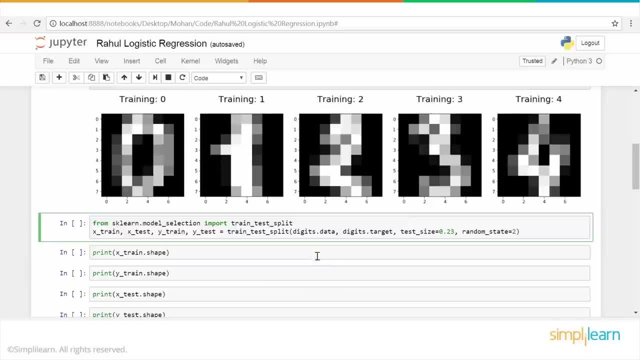 training size will be determined and we pass the data that we want to split and the. the results will be stored in x underscore train and y underscore train for the training data set. and what is x underscore train? this are: these are the features, right, which is like the independent variable, and y underscore train is the label, right. so in this case, what? 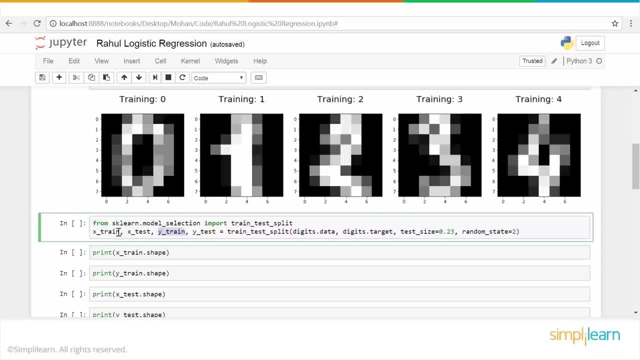 happens is we have the input value, which is, or the features value, which is in x underscore train, and since this is the labeled data for each of them, each of the observations, we already have the label information saying whether this digit is a 0 or a 1 or a 2. 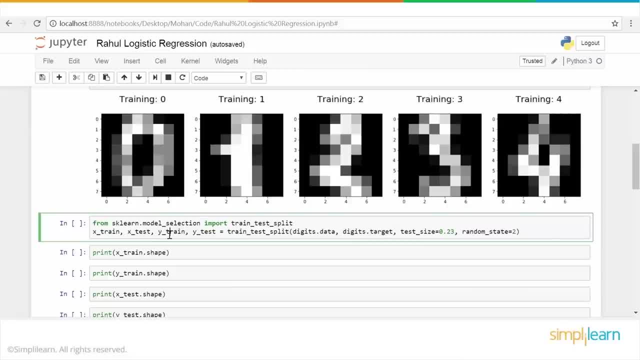 that this is what will be used for comparison to find out whether the the system is able to recognize it correctly or there is an error. for each observation, it will compare with this right. so this is the label. so the same way, x underscore train, y underscore train is for the. 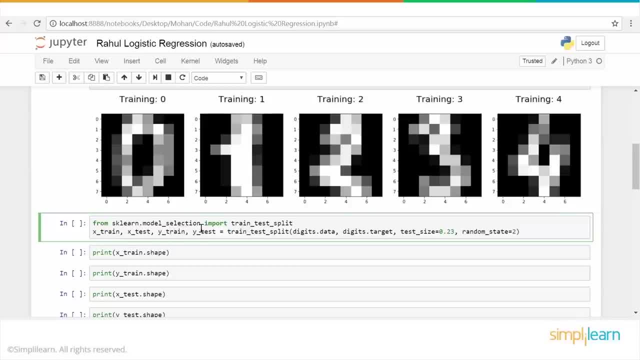 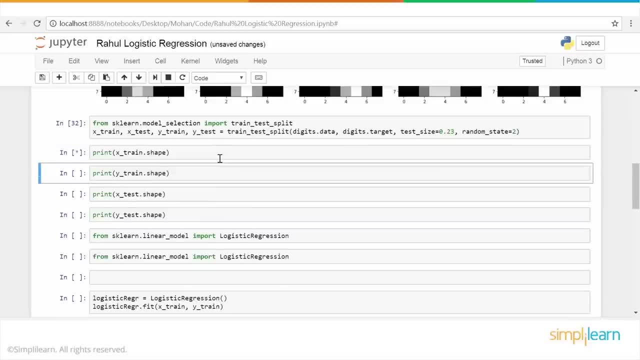 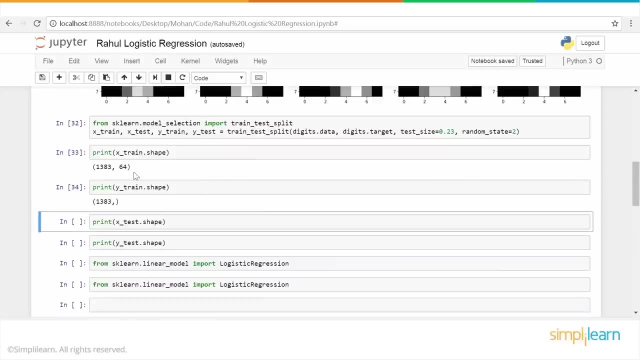 training data set. x underscore test. y underscore test is for the test data set. okay, so let me go ahead and execute this code as well, and then we can go and check quickly what is the. how many entries are there and in each of this? so x underscore train. the shape is 1383 by 64 and 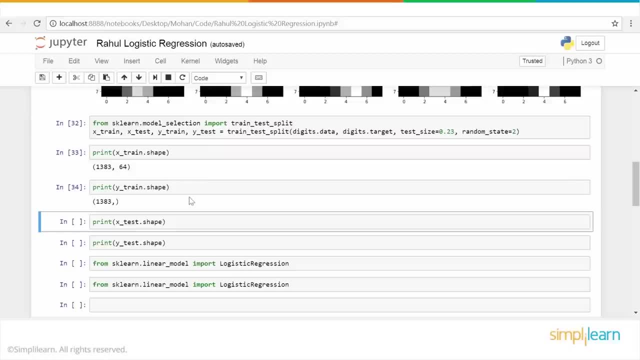 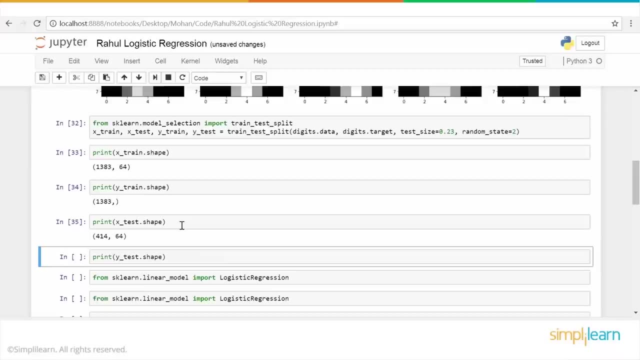 y underscore: train has 1383, because there is nothing like the second part is not required here. and then x underscore test shape we see is 414. so actually there are 414 observations in test and 1383 observations in train. so that's basically what these four lines of code are. 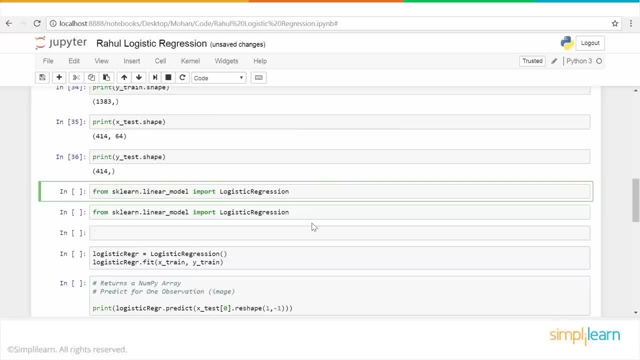 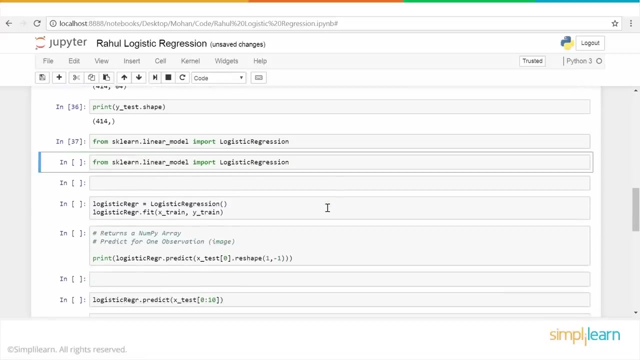 are saying: okay, then we import the logistic regression library and which is a part of scikit-learn, so we we don't have to implement the logistic regression process itself. we just call these the function and let me go ahead and execute that so that we have the logistic regression. 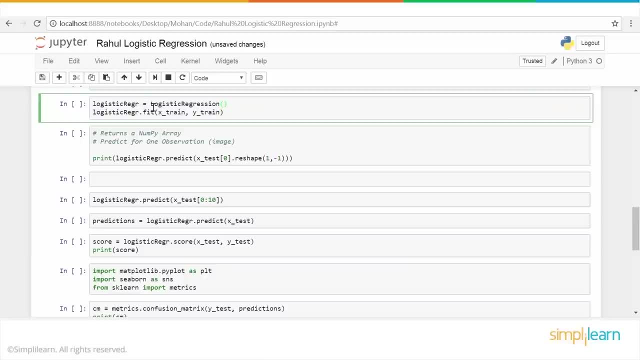 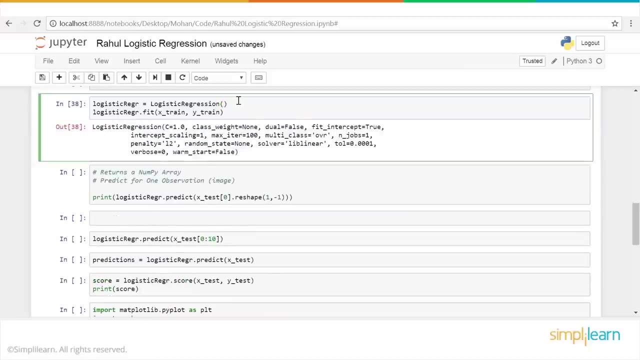 library imported. now we create an instance of logistic regression, right? so logistic regr is a is an instance of logistic regression, and when we create the model, we degrade it into a set of set of data set and this essentially creates our model, and then we use that for training our model. so let me first execute. 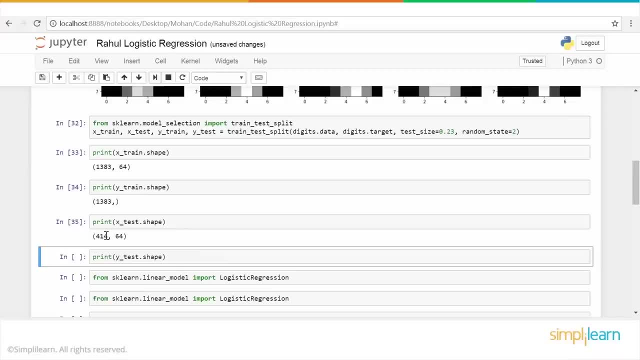 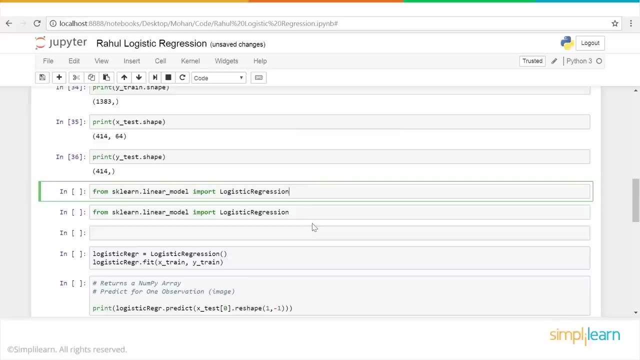 Test shape We see is 414. so actually there are 414 observations in test and 1383 observations in train. so that's basically what these four lines of code are saying. okay, then we import the logistic regression library and which is a part of scikit learn, so we don't have to implement. 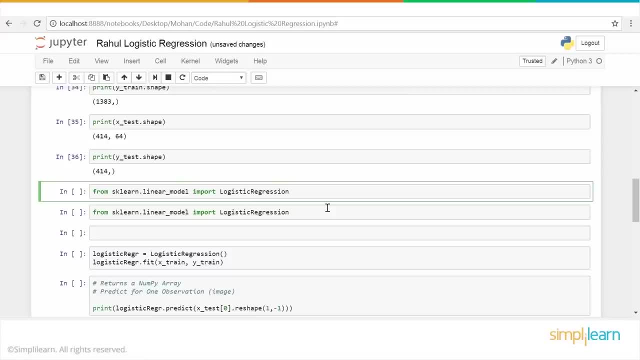 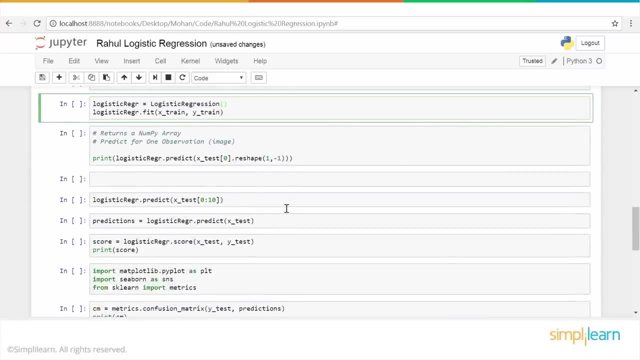 the logistic regression process itself. we just call these the function, and let me go ahead and execute that So that we have the logistic regression library imported. now we create an instance of logistic regression, right? so logistic regr is a is an instance of logistic regression. and then 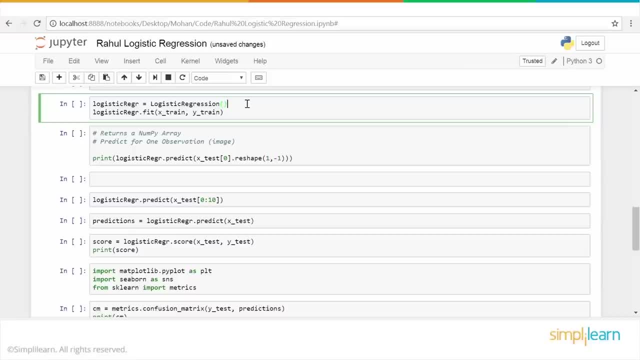 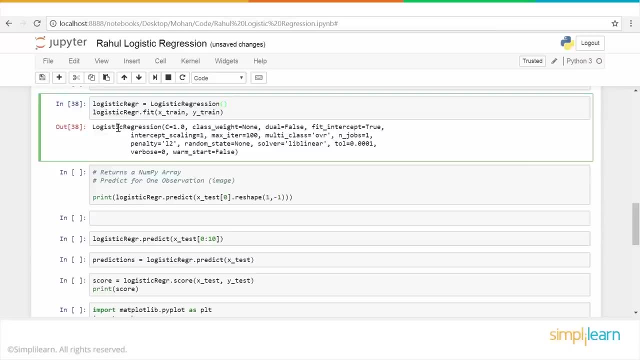 we use that for training our model. So let me first execute this code, so these two lines. so the first line basically creates an instance of logistic regression model, and then the second line is where we are passing our data, the training data set. Right, This is our the predictors and this is our target. we are passing this data set to train. 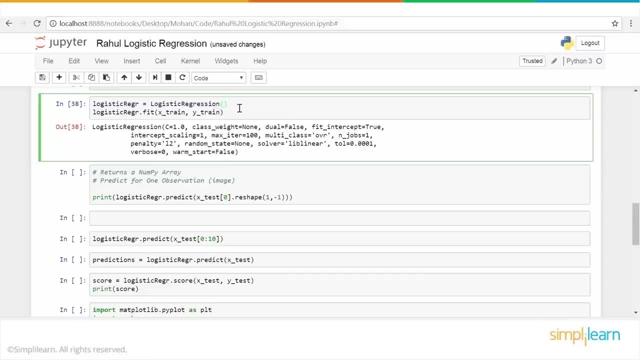 our model, All right. So once we do this, in this case the data is not large, but by and large the training is what takes usually a lot of time. So we spend in machine learning activities, in machine learning projects. we spend a lot of time for the training part of it. 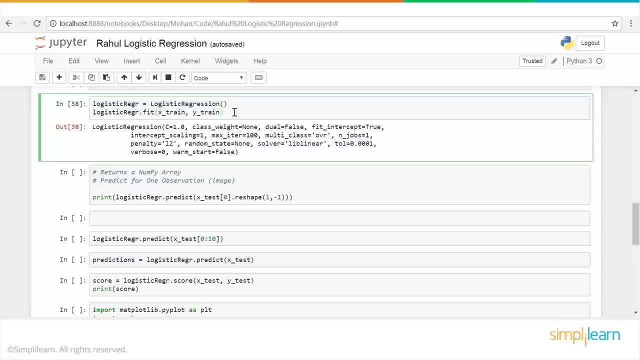 Okay, So here the data set is relatively small, so it was pretty quick. So all right. So our model has been trained using the training data set and we want to see how accurate this is. So what we'll do is we will test it out in, probably, faces. 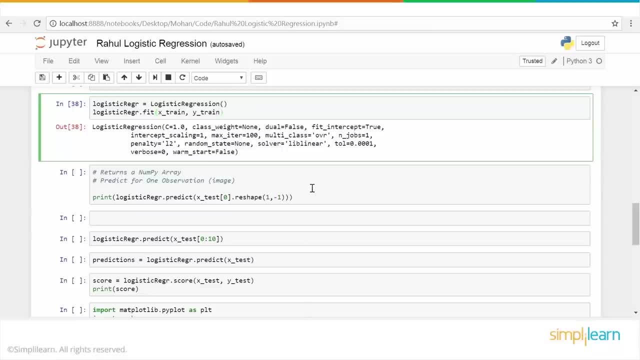 So let me first try out how well this is working for one image. Okay, I will just try it out with one image, my the first entry in my test data set, and see whether it is correctly predicting or not. So, and in order to test it, 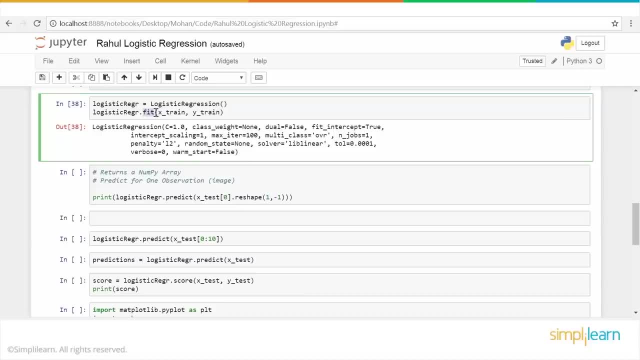 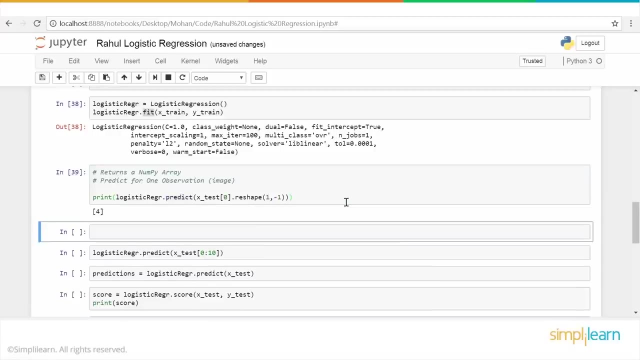 So for training purpose, We use the fit method. there is a method called fit, which is for training the model and once the training is done, if you want to test for a particular value, new input, you use the predict method. Okay, So let's run the predict method and we pass this particular image and we see that the 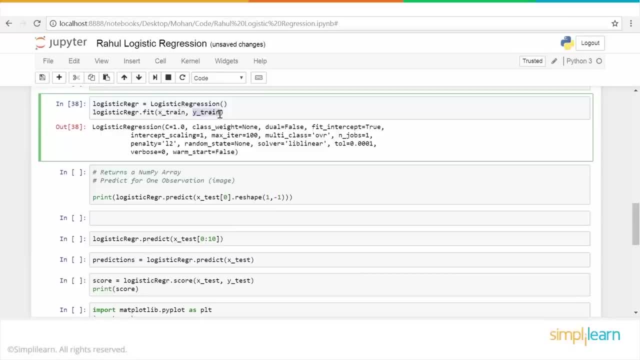 this code, so these two lines. so the first line basically creates an instance of logistic regression model, and then the second line: where is where we are passing our data, the training data set, and this is our the, the predictors, and, uh, this is our target. we are passing this dataset to train. 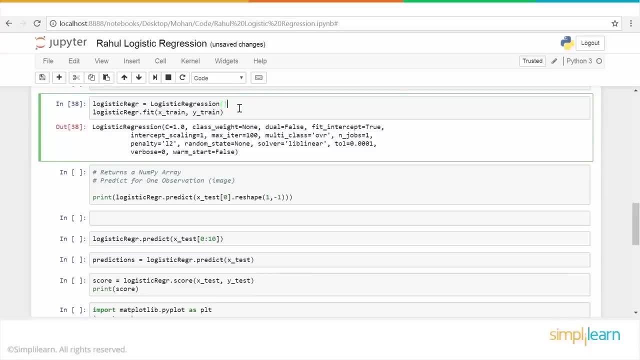 by and large, the training is what takes usually a lot of time. so we spend in machine learning activities, in machine learning projects, we spend a lot of time for the training part of it. okay, so here the data set is relatively small, so it was pretty quick. so all right. so now our model has. 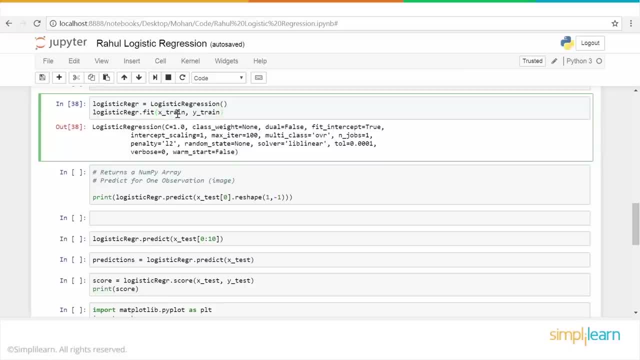 been trained using the training data set and we want to see how accurate this is. so what we'll do is we will test it out in, probably faces, so let me first try out how well this is working for one image. okay, i'll just try it out with one image- my the first entry in my test data set and see. 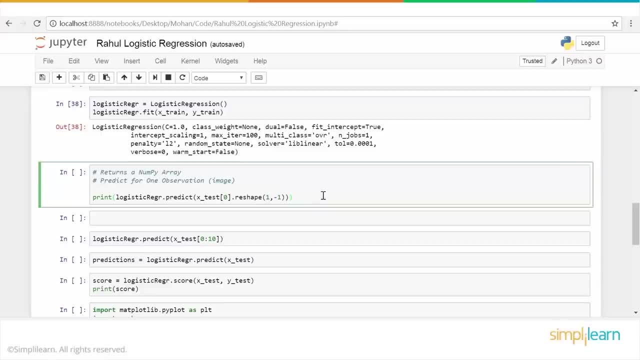 whether it is correctly predicting or not. so, and in order to test it, so for training purpose, we use the fit method. there is a method called fit, which is for training the model, and once the training is done, if you want to test for uh particular value- new input- you use the predict method. okay, so let's run the predict method and 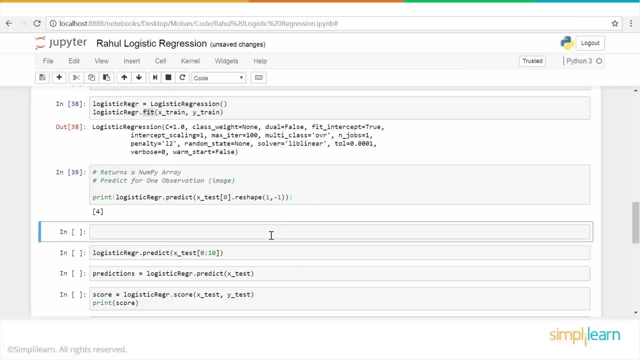 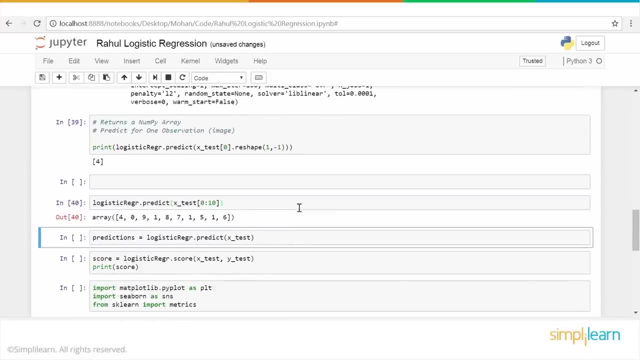 we pass this particular image and we see that the shape is, or the prediction is, four. so let's try a few more. let me see for the next 10. seems to be fine, so let me just go ahead and test the entire data set. okay, that's basically what we will do, so now we want to find out how accurately this has. 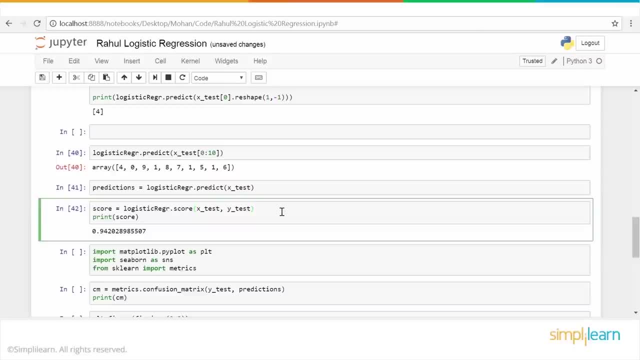 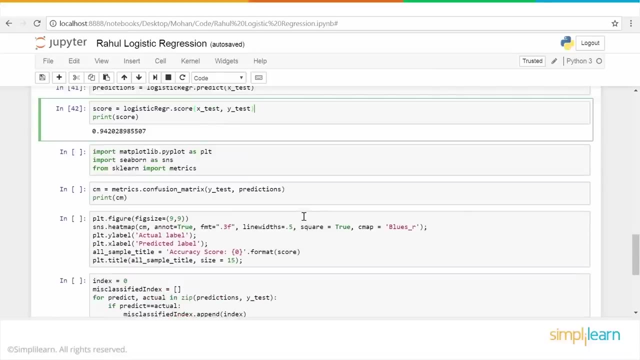 performed. so we use the score method to find what is the percentages of accuracy, and we see here that it has performed up to 94 percent accurate. okay, so that's on this part. now, what we can also do is we can um also see this accuracy using what is known as a confusion matrix. so let us go ahead. 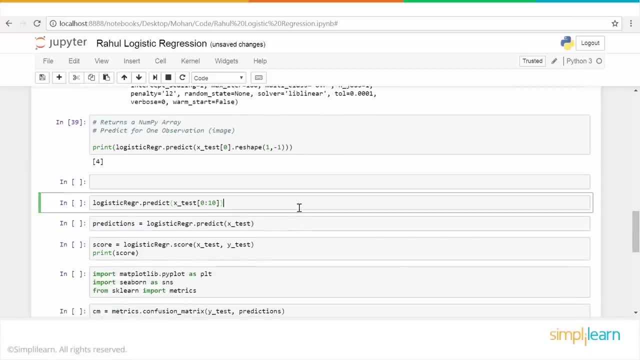 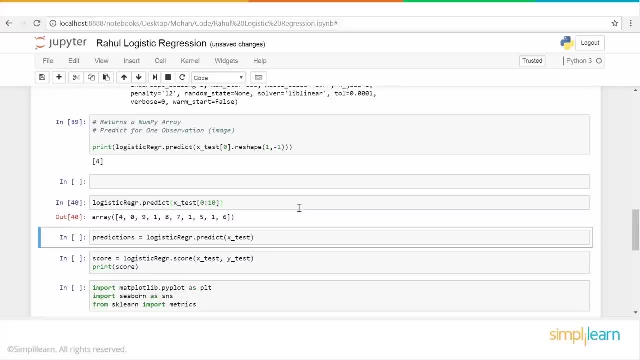 shape is already the prediction is for, so let's try a few more. Let me see for the next 10.. Seems to be fine, So let me just go ahead and test the entire data set. Okay, That's basically what we will do. 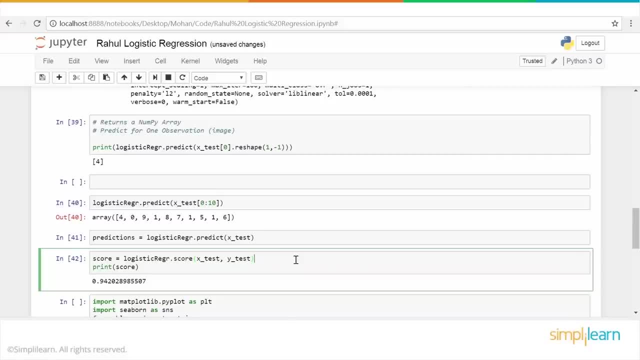 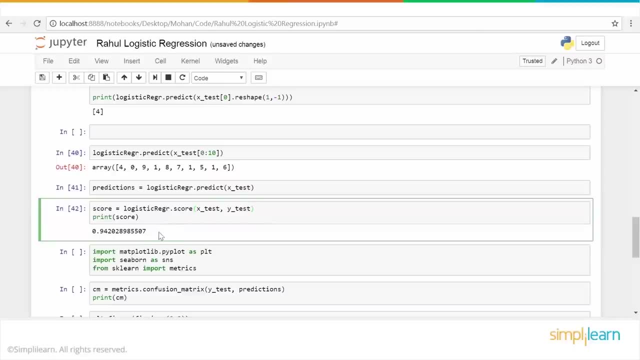 So now we want to find out how accurately this has performed. So we use the score method to find what is the percentages of accuracy, and we see here that it has performed up to 94% accurate. Okay, So that's on this part. 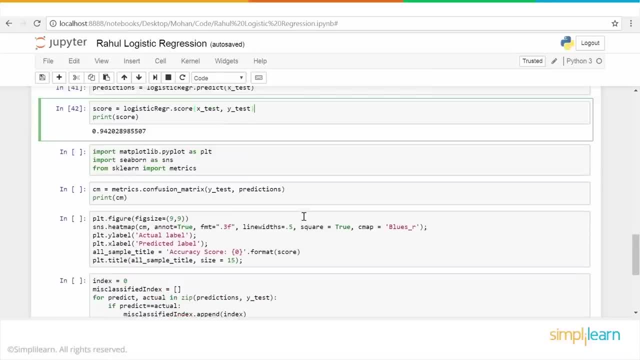 Now what we can also do is we can also see this accuracy using what is known as confusion matrix. So let us go ahead and try that as well, so that we can also visualize how well this model has done. So let me execute this piece of code, which will basically import some of the libraries. 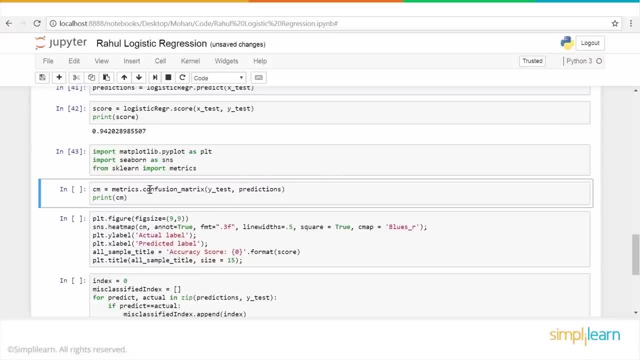 that are required and we basically create a confusion matrix and instance of confusion matrix by running confusion matrix and passing these values So we have. So Confusion underscore matrix method takes two parameters: One is the y underscore test and the other is the prediction. 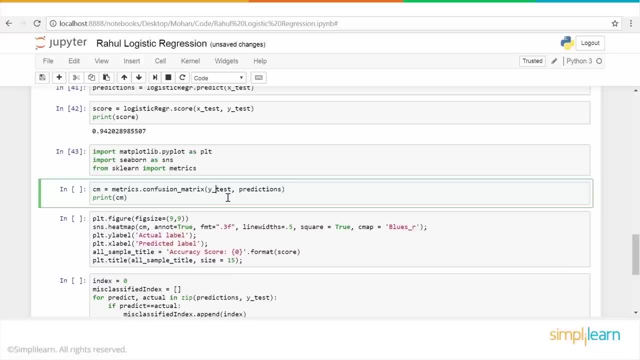 So what is the y underscore test? These are the labeled values which we already know for the test data set, and predictions are what the system has predicted for the test data set. Okay, So this is known to us and this is what the system has the model has generated. 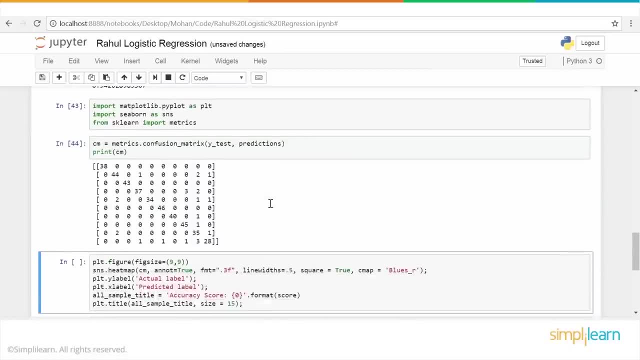 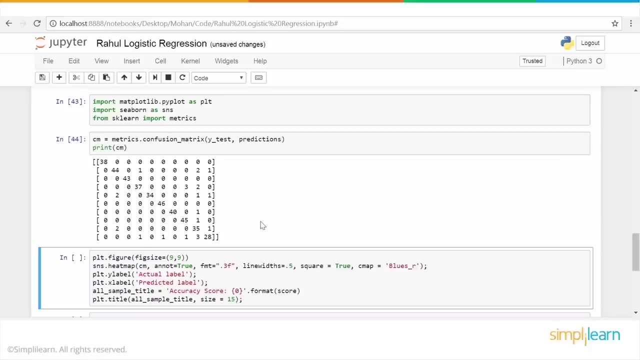 So we kind of create the Okay, The matrix and we will print it. and this is how the confusion matrix looks. as the name suggests, it is a matrix and the key point out here is that the accuracy of the model is determined by how many numbers are there in the diagonal. 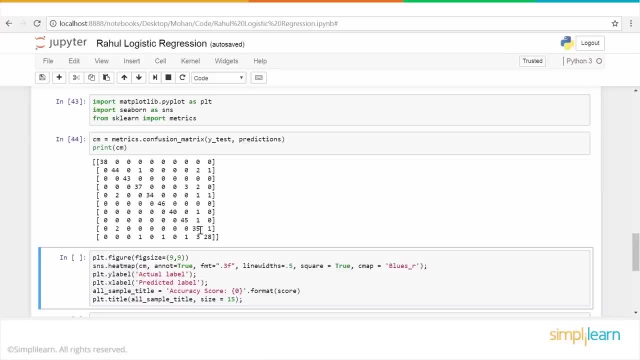 The more the numbers in the diagonal, the better the accuracy is Okay And, first of all, the total sum of all the numbers in this whole matrix is equal to the number of observations in the test data set. That is the first thing. 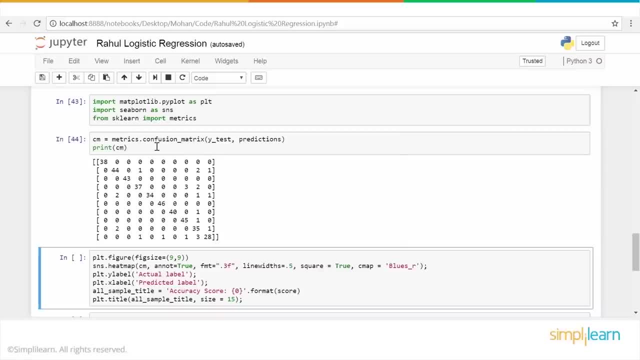 Right. So if you add up all these numbers that will be equal to the number of observations in the test data set, And then out of that the maximum number of them should be in the diagonal. That means the accuracy is pretty good. 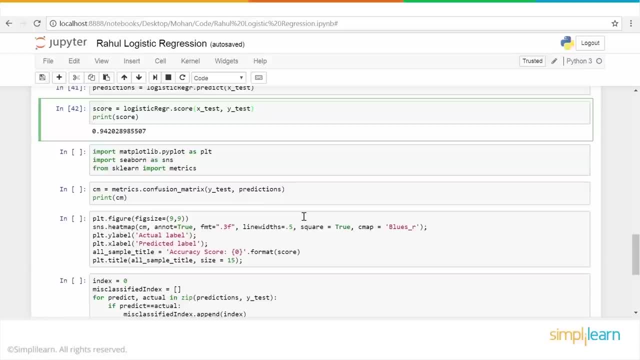 and try that as well, so that we can also visualize how well this model has done. so let me execute this piece of code, which will basically import some of the libraries that are required, and we we basically create a confusion matrix, an instance of confusion matrix, by running confusion. 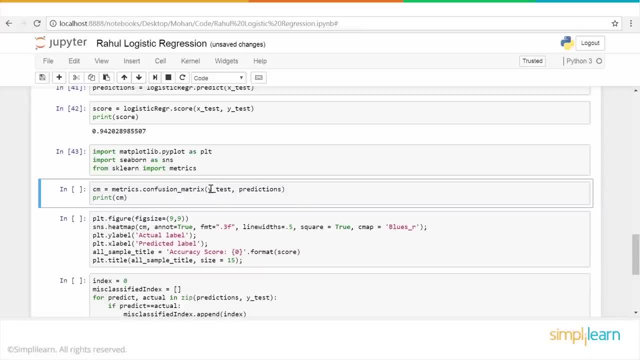 matrix and passing these values. so we have so this confusion. underscore matrix method takes two parameters. one is the y underscore test and the other is the prediction. so what is the y underscore value if the data is not? takes a set of a set of values which we already know for the test data. 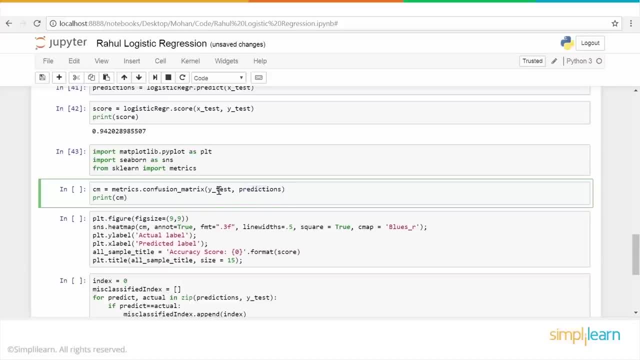 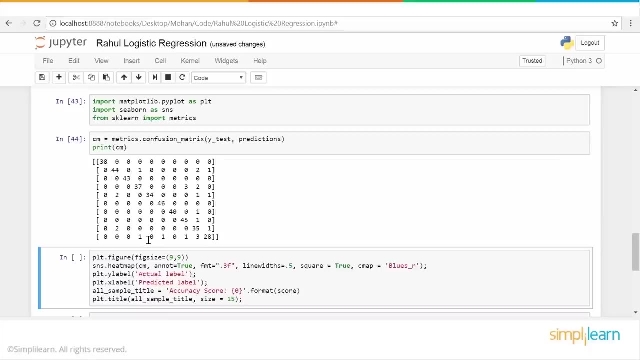 set and predictions are what the system has predicted for the test data set. okay, so this is known to us and this is what the system has, uh, the model has generated. so we kind of create the confusion matrix and we will print it and this is how the confusion matrix looks, as the name suggests. 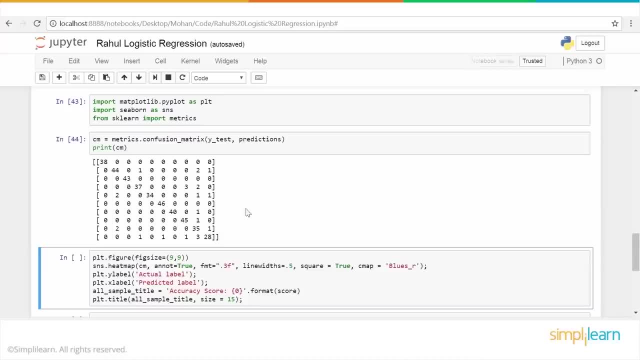 it is a matrix and model is determined by how many numbers are there in the diagonal. the more the numbers in the diagonal, the better. the accuracy is okay and, first of all, the total sum of all the numbers in this whole matrix is equal to the number of observations in the test data set. that is the first thing, right. 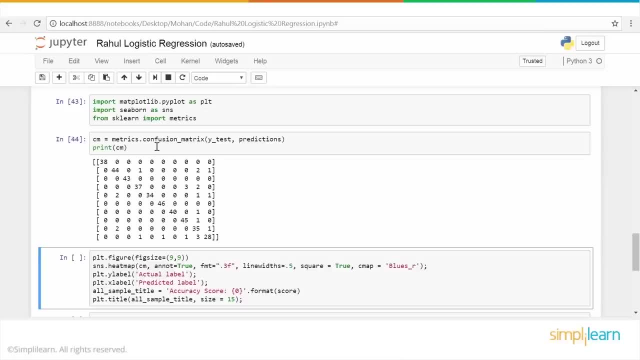 so if you add up all these numbers that will be equal to the number of observations in the test data set, and then out of that the maximum number of them should be in the diagonal. that means the accuracy is pretty good if the the numbers in the diagonal are less and in all other places there. 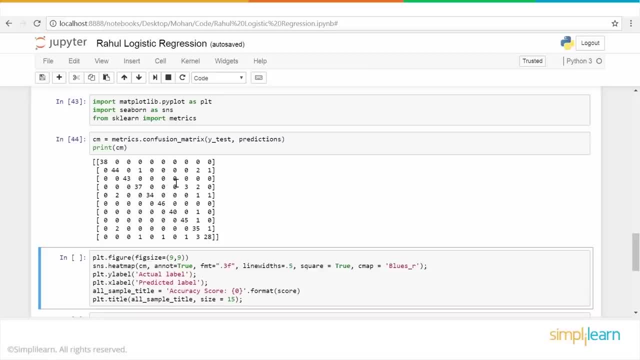 are a lot of numbers, which means the accuracy is very low. the diagonal indicates a correct prediction that this means that the actual value is same as the predicted value. here again: actual value, same as the predicted value, and so on. right. so the moment you see a number here, that means the actual. 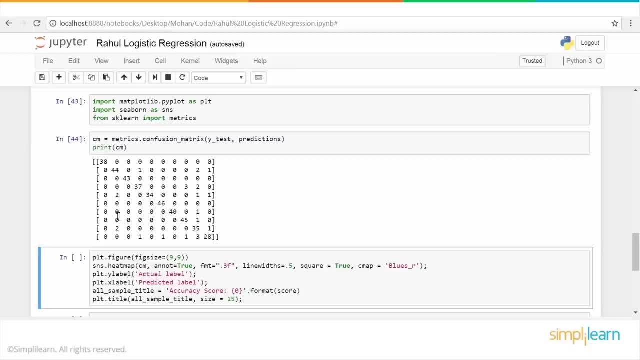 If the numbers in the diagonal are less- and in all other places there are a lot of numbers, which means the accuracy is very low- The diagonal indicates a correct prediction, that this means that the actual value is same as the predicted value. here Again, actual value is same as the predicted value, and so on, right? 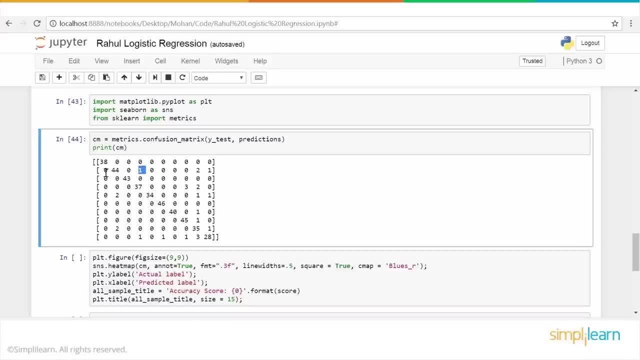 So the moment you see a number here, that means the actual value is something and the predicted value is something else, right? Similarly here: the actual value is something and the predicted value is something else. So that is basically how we read the confusion matrix. 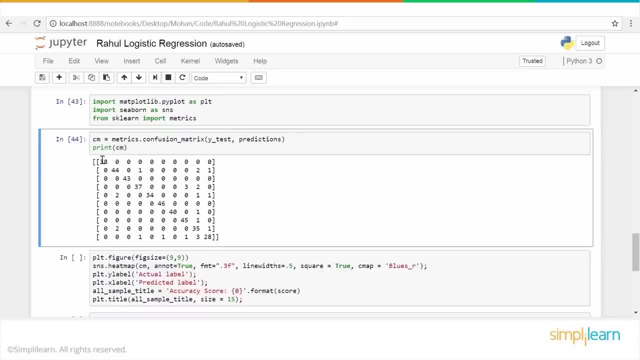 Now, how do we find the accuracy? You can actually add up the total values in the diagonal- So it's like 38 plus 44 plus 43 and so on- And divide that by the total number of test observations. that will give you the percentage. 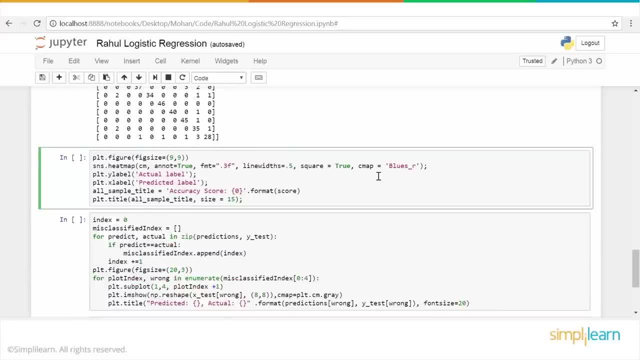 accuracy using a confusion matrix. Now let us visualize this confusion matrix in a slightly more sophisticated way, using a heat map. So we will create a heat map with some. we'll add some colors as well. It's a, it's like a more visually, visually more appealing. 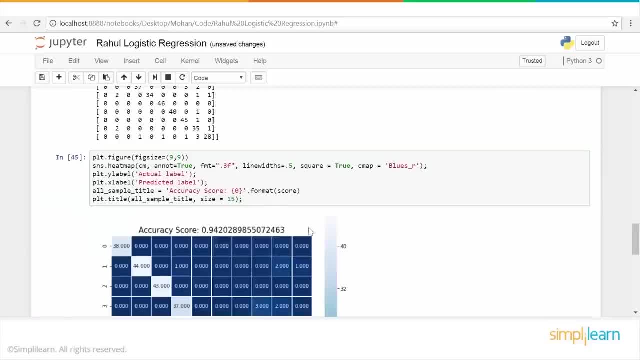 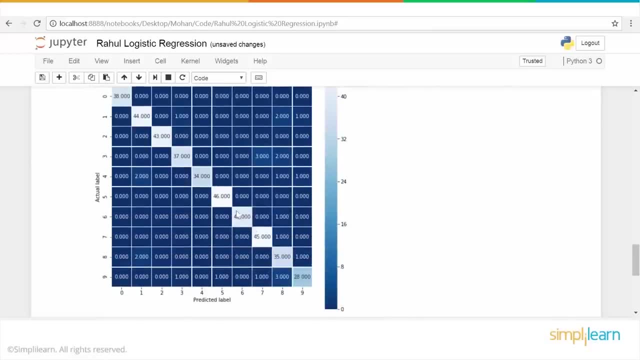 So that's the whole idea. So if we let me run this piece of code, And this is how The heat map uh looks, uh, and as you can see here, the diagonals again, uh are all the values, are here most of the values? 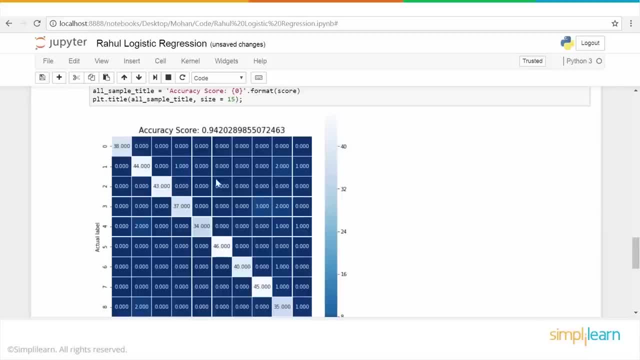 So, which means reasonably, this seems to be reasonably accurate. and yeah, basically the accuracy score is 94%. This is calculated, as I mentioned, by adding all these numbers divided by the total test value, So the total number of observations in test data set. 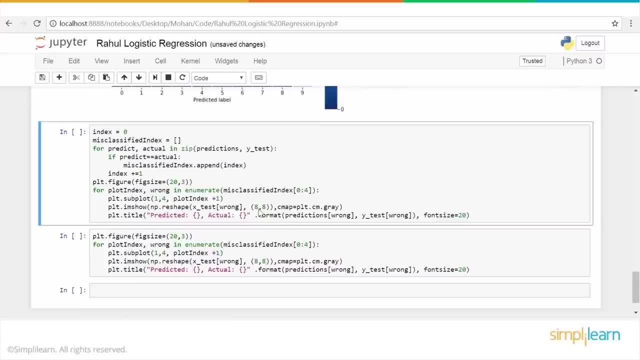 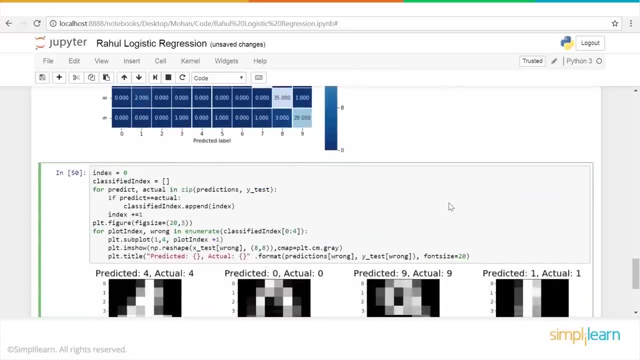 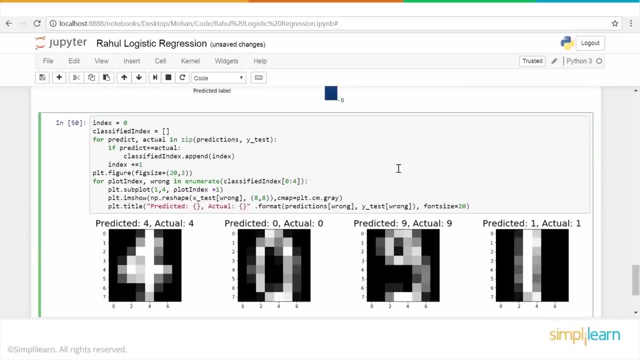 Okay, So This is The Acceleration, All right. So now that we have seen the confusion matrix, let's take a quick sample and see how well the system has classified and we will take a few examples of the data. So if we see here, we picked up randomly a few of them. 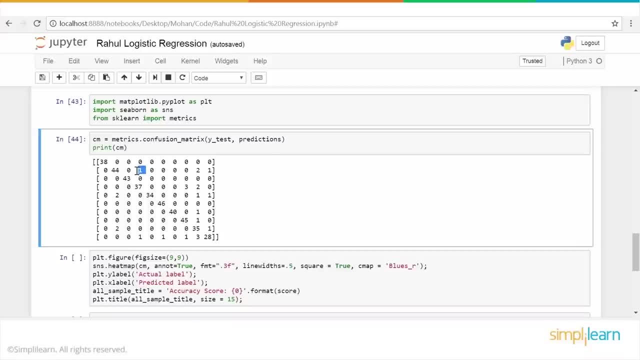 value is something and the predicted value is something else. right? similarly here, the actual value is something and the predicted value is something else. so that is basically how we read the confusion matrix. now how do we find the accuracy? you can actually add up the total values in the diagonal, so it's like: 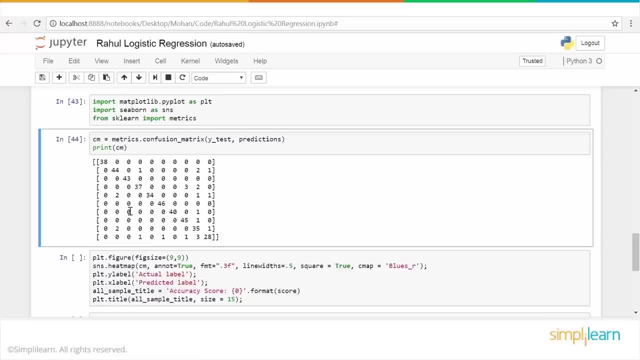 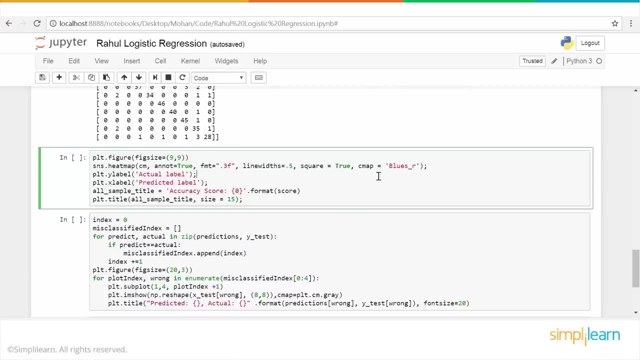 38 plus 44 plus 43 and so on, and divide that by the total number of test observations. that will give you the percentage accuracy using the configuration matrix. now let us visualize this confusion matrix in a slightly more sophisticated way, using a heat map. so we will create a heat map with some. we'll add some colors as well. it's 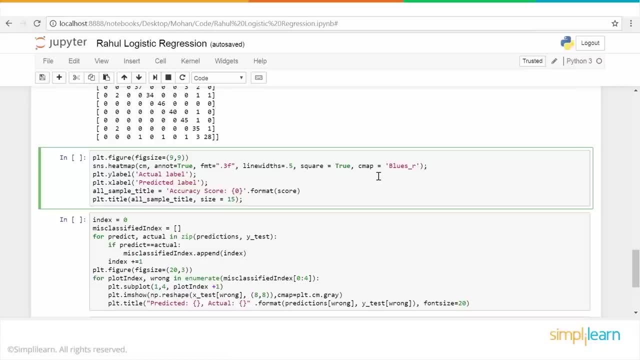 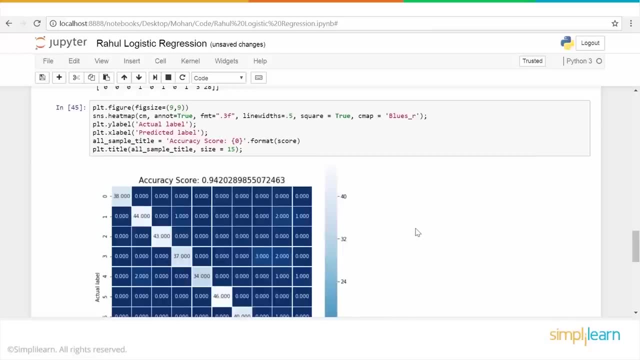 it's like a more visually, visually more appealing. so that's the whole idea. so if we let me run this piece of code and this is how the heat map looks, and as you can see here, the diagonals again are all the values are here. most of the 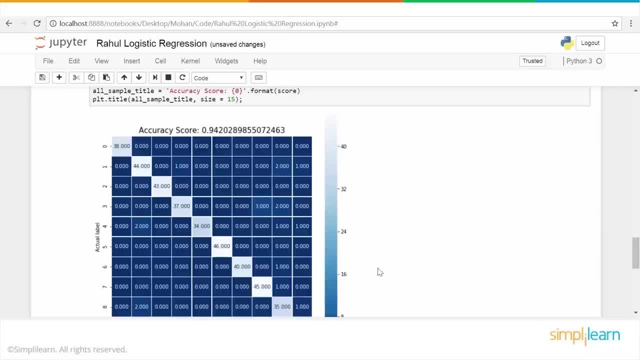 values. so, which means reasonably, this seems to be reasonably accurate and, yeah, basically the accuracy score is 94. this is calculated, as i mentioned, by adding all these numbers divided by the total test values or the total number of observations in test data set. okay, so this is the confusion matrix for. 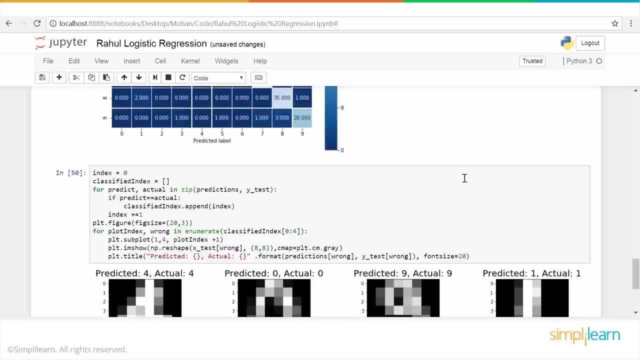 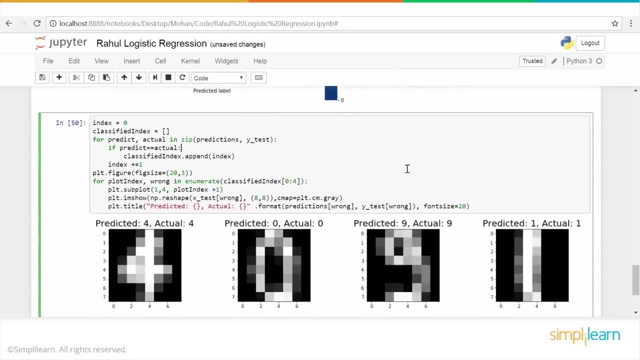 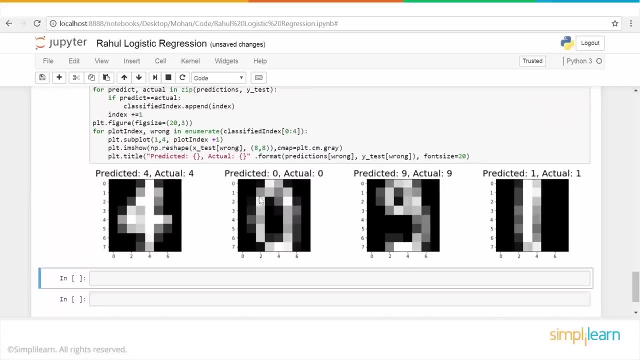 logistic regression. all right, so now that we have seen the confusion matrix, let's take a quick sample and see how well the system has classified and we will take a few examples of the data. so if we see here, we picked up randomly a few of them. so this is number four, which is the actual value, and also 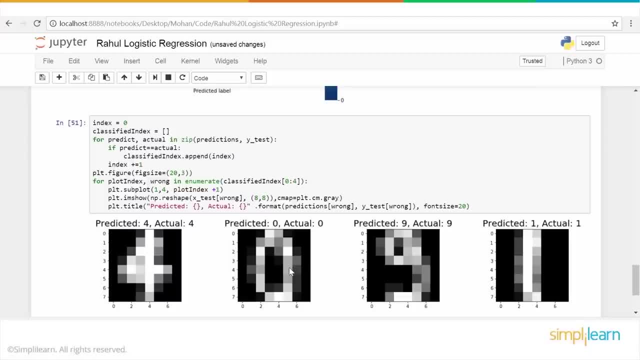 the predicted value. both are four. this is an image of zero, so the predicted value is also zero. actual values, of course zero. then this is the image of nine, so this has also been predicted correctly: nine and actually value is nine. and this is the image of one and again, this has been predicted correctly, as like the actual value. 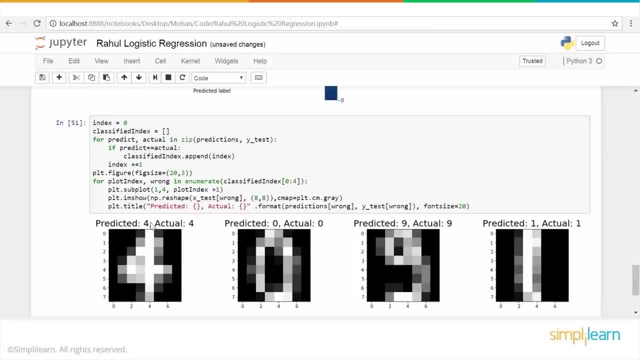 So this is a number four, which is the actual value and also the predicted value. Both are four. This is an image of a zero, So the predicted value is also zero. Okay, So actual values? of course zero. Then this is the image of nine. 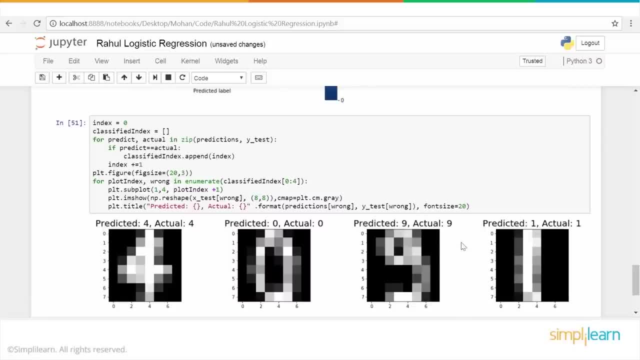 So this has also been predicted correctly: Nine and actual value is nine, And this is an image of one And again, this has been predicted correctly, as like the actual value. Okay, So this was a quick demo of logistic regression: how to use logistic regression to identify: 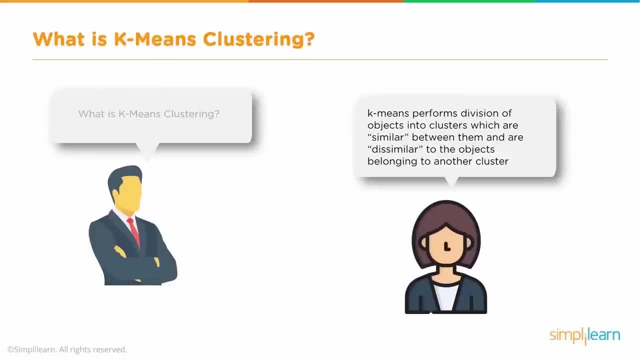 images. So what is K-means clustering? K-means clustering is an unsupervised Learning algorithm. In this case, you don't have labeled data, unlike in supervised learning. So you have a set of data and you want to group them. 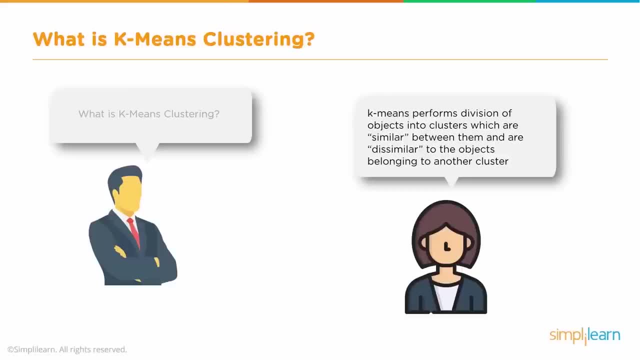 And, as the name suggests, you want to put them into clusters, which means objects that are similar in nature, similar in characteristics, need to be put together. So that's what K-means- clustering- is all about. The term K is basically is a number. 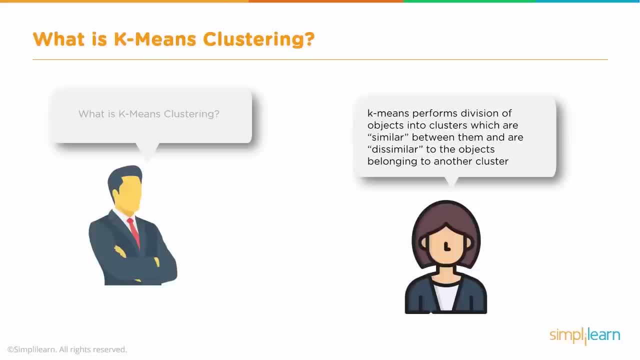 So we need to tell the system How many clusters we need to perform. So if K is equal to two, there will be two clusters. If K is equal to three, three clusters, and so on and so forth. That's what the K stands for. 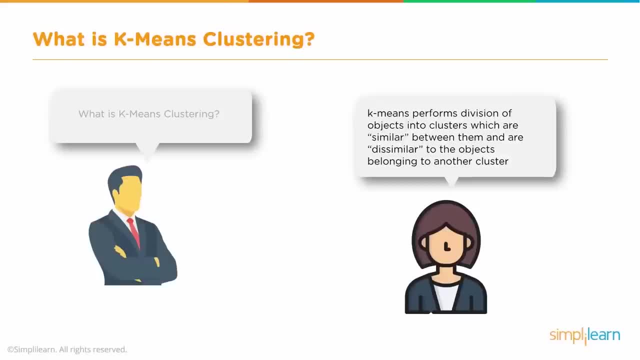 And of course, there is a way of finding out what is the best or optimum value of K for a given data. We will look at that. So that is K-means clustering. So let's take an example. K-means clustering is used in many, many scenarios. but let's take an example of cricket, the 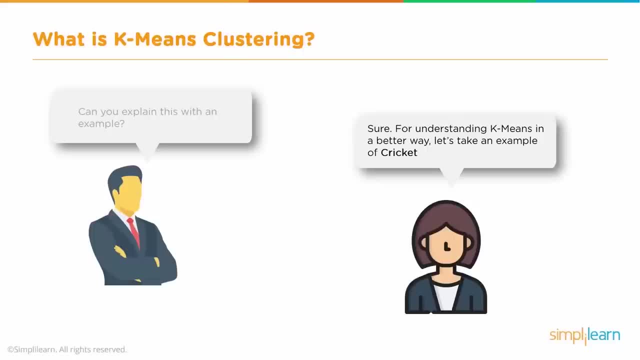 game of cricket. Let's say, you received Data of a lot of players from maybe all over the country or all over the world, And this data has information about the runs scored by the people or by the player and the wickets taken by the player. 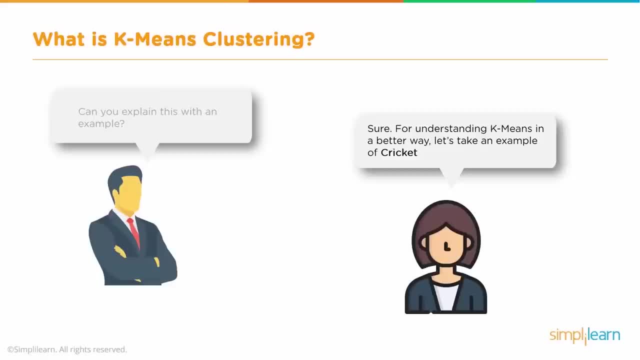 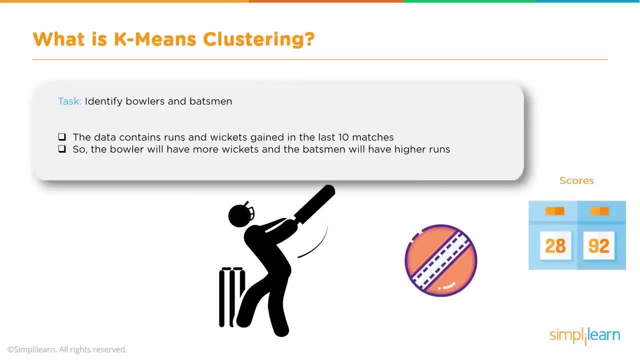 And, based on this information, we need to cluster this data into two clusters: batsmen and bowlers. So this is an interesting example. Let's see how we can perform this. So we have The data, which consists of primarily two characteristics, which is the runs and the wickets. 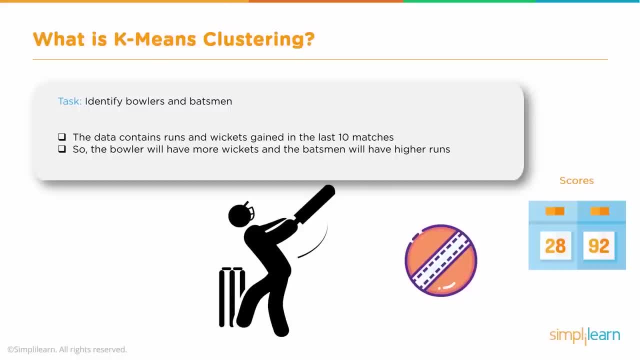 So the bowlers basically take wickets and the batsmen score runs. There will be, of course, a few bowlers who can score some runs And similarly, there will be some batsmen who will, who would have taken a few wickets. 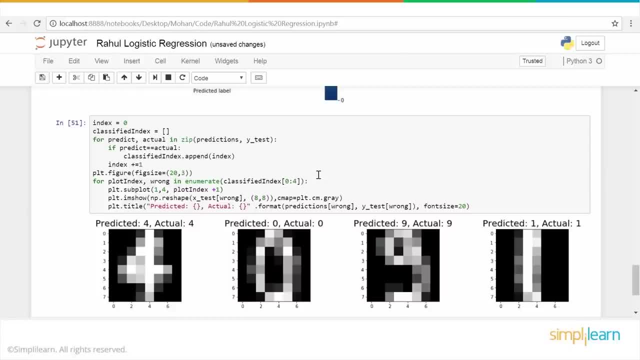 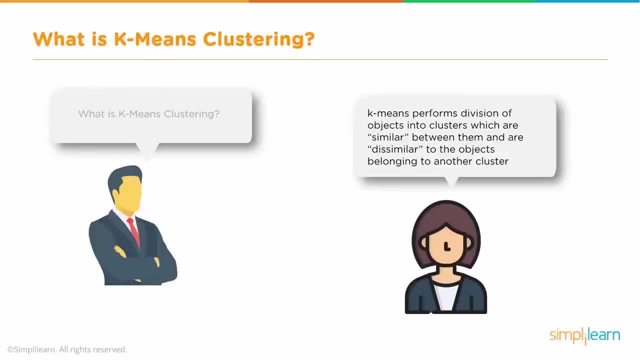 okay, so this was a quick demo of logistic regression- how to use logistic regression to identify images. so what is k-means clustering? k-means clustering is an unsupervised learning algorithm. in this case, you don't have labeled data, unlike in supervised learning, so you have a set of data. 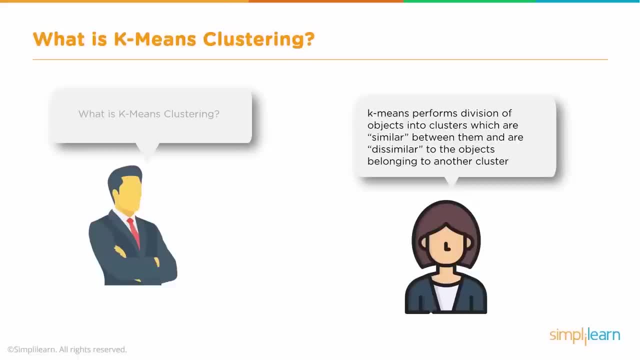 and you want to group them and, as the name suggests, you want to put them into clusters, which means objects that are similar in nature, similar in characteristics, need to be put together. so that's what k-means clustering is all about. the term k is basically is a number, so we need 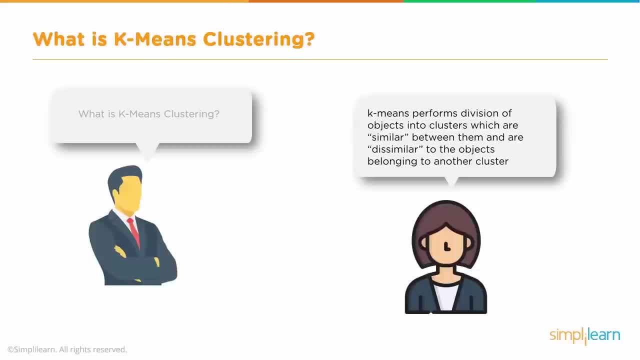 to tell the system how many clusters we need to perform. so if k is equal to two, there will be two clusters. if k is equal to three, three clusters, and so on and so forth. that's what the k stands for, and of course there is a way of finding out what is the best or optimum value of k for a. 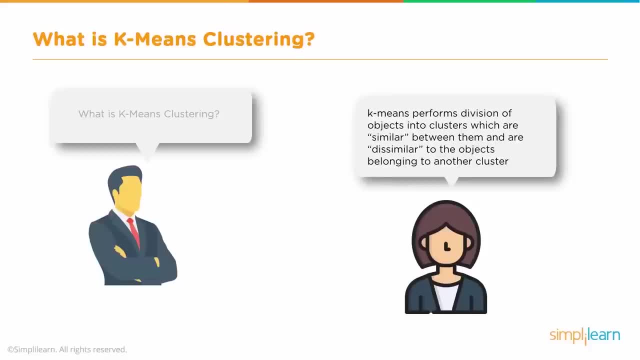 given data. we will look at that. so that is k-means clustering. so let's take an example. k-means clustering is used in many, many scenarios. but let's take an example of cricket, the game of cricket. let's say you received data of a lot of players from maybe all over the country or all. 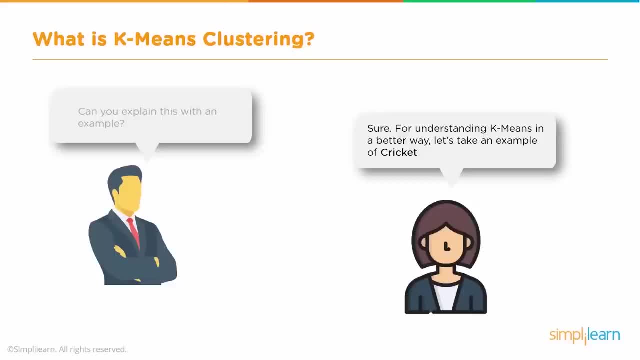 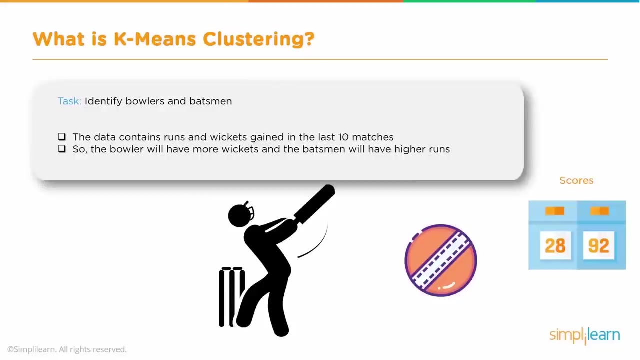 over the world, and this data has information about the runs scored by the people or by the player and the wickets taken by the player, and, based on this information, we need to cluster this data into two clusters: batsmen and bowlers. so this is an interesting example. let's see how we can perform this. so we have the data, which consists: 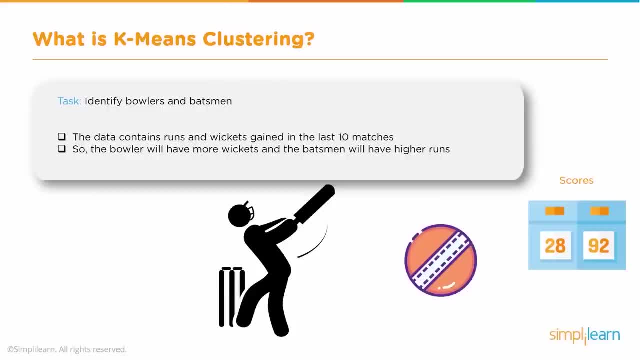 of primarily two characteristics, which is the runs and the wickets. so the bowlers basically take wickets and the batsmen score runs. there will be, of course, a few bowlers who can score some runs and similarly, there will be some batsmen who will, who would have taken a few wickets. but with this, 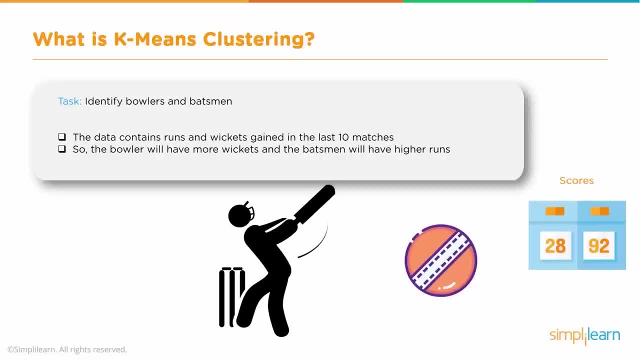 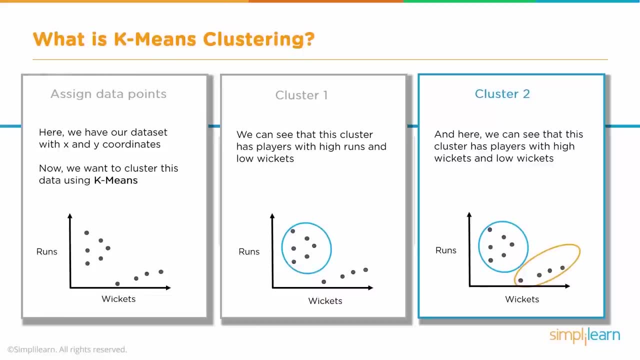 information. we want to cluster those players into batsmen and bowlers. so how does this work? let's say this is how the data is. so there are information. there is information on the y-axis about the runs scored and on the x-axis about the wickets taken by the players. so if we do a 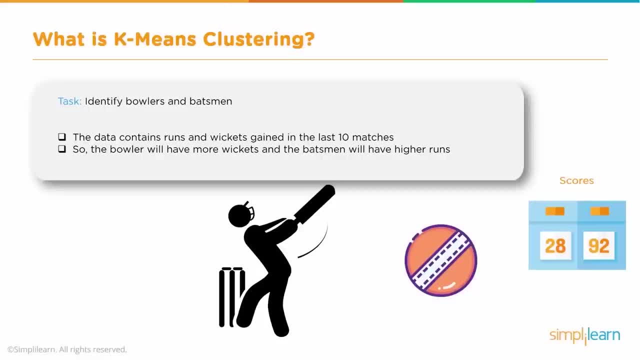 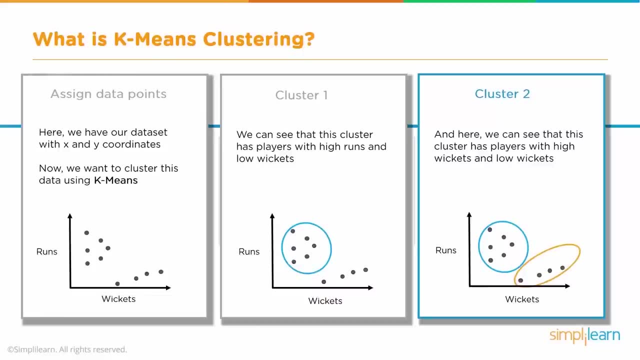 But with this information we want to cluster those players into batsmen and bowlers. So how does this work? Let's say this is how the data is For information: there is information on the Y axis about the runs scored and on the X. 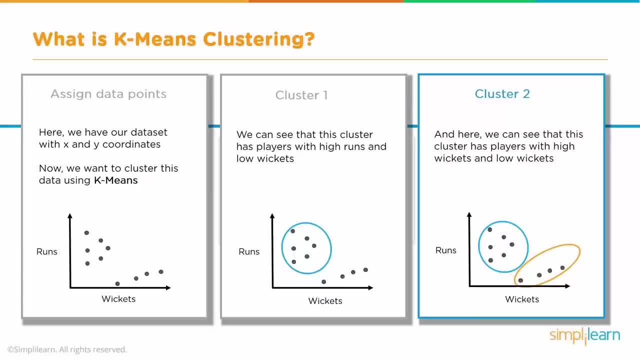 axis about the wickets taken by the players. So if we do a quick plot, this is how it would look, And when we do the clustering, we need to have the clusters, like shown in the third diagram out here. We need to have a cluster which consists of people who have scored high runs, which is 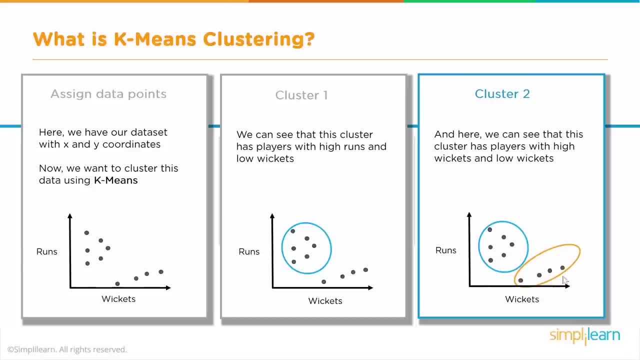 basically the batsmen, And then we need a cluster- Yeah, People who have taken a lot of wickets, which is typically the bowlers. There may be a certain amount of overlap, but we will not talk about it right now. So, with K-means clustering we will have here. 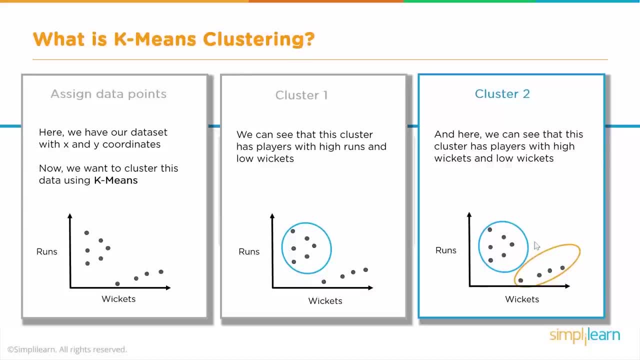 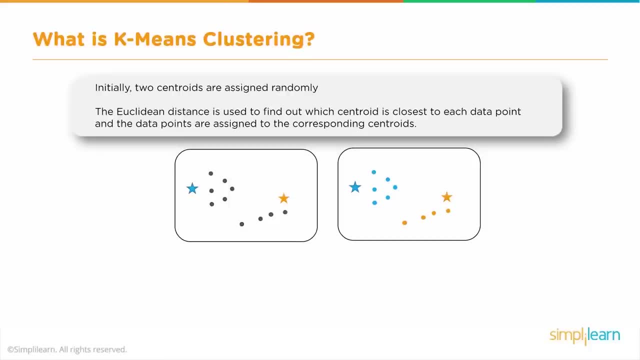 That means K is equal to two and we will have two clusters, which is batsmen and bowlers. So how does this work? The way it works is the first step in K-means clustering is the allocation of two centroids randomly, So two points are assigned. 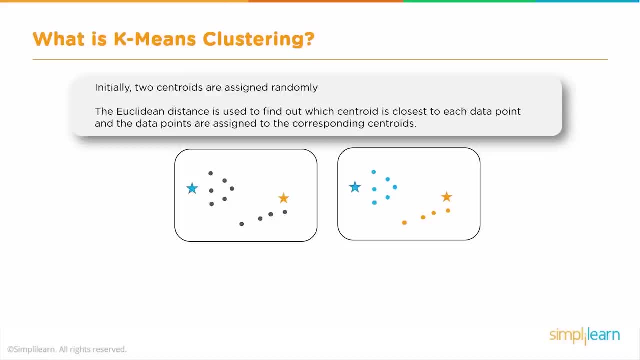 As so-called centroids. So in this case we want two clusters, which means K is equal to two. So two points have been randomly assigned as centroids. Keep in mind, these points can be anywhere. There are random points. They are not initially, they are not really the centroids. 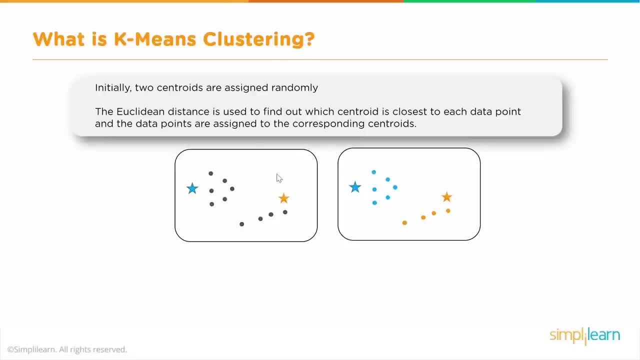 Centroid means it's a central point of a given data set, But in this case, when it starts off, it's not really the centroid. OK, so these points, though in our presentation here we have shown them one point closer. 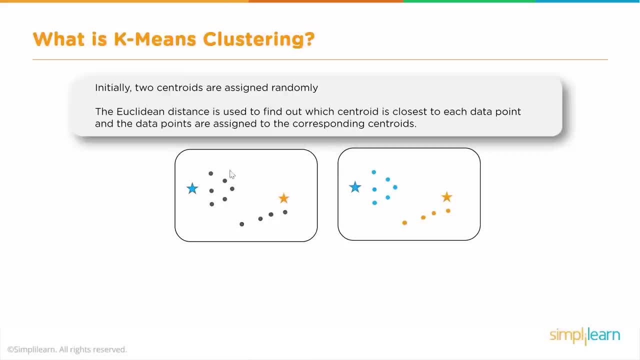 to these data points and another closer to these data points. They can be assigned randomly anywhere. OK, so that's the first step. The next step is to determine the distance of each of the data points from each of the randomly assigned centroids. So, for example, we take this point and find the distance from this centroid and the distance. 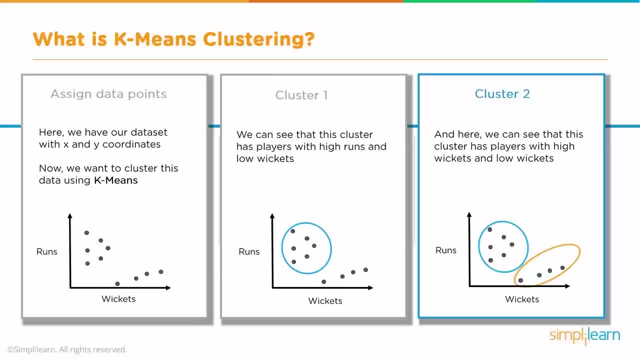 quick plot. this is how it would look, and when we do the clustering, we need to have the clusters like shown in the third diagram out here. we need to have a cluster which consists of people who have scored high runs, which is basically the batsman, and then we need a cluster with people. 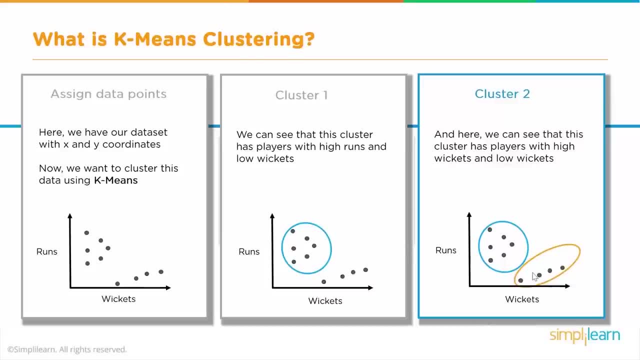 who have taken a lot of wickets, which is typically the bowlers. there may be a certain amount of overlap, but we will not talk about it right now. k-means clustering we will have here. that means k is equal to 2 and we will have two clusters which 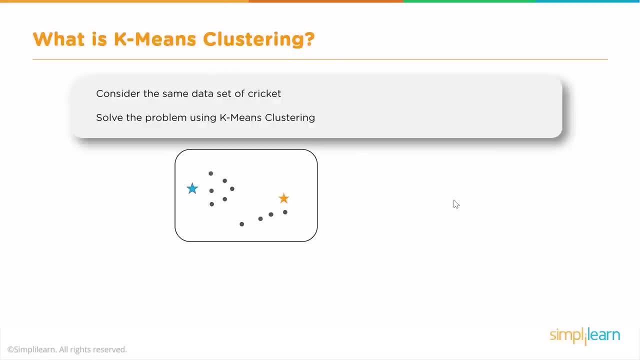 is batsman and bowlers. so how does this work? the way it works is the first step in k-means. clustering is the allocation of two centroids randomly, so two points are assigned as so-called centroids. so in this case we want two clusters, which means k is equal to two, so two points have. 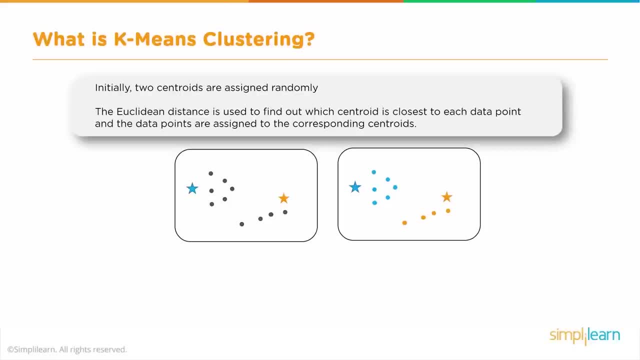 been randomly assigned as centroids. keep in mind these points can be anywhere. there are random points. they are not initially. they are not really the centroids. centroid means it's a central point of a given data set, but in this case, when it starts off, it's not really the centroid. 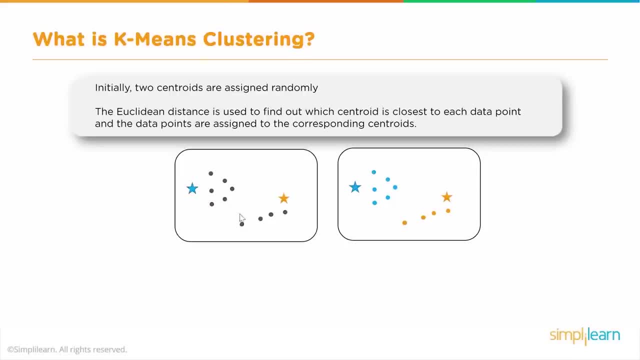 okay, so these points- though in our presentation here we have shown them one point closer to these data points and another closer to these data points- can be assigned randomly anywhere. okay, so that's the first step. the next step is to determine the distance of each of the data points from each of the randomly assigned centroids. so, for example, we: 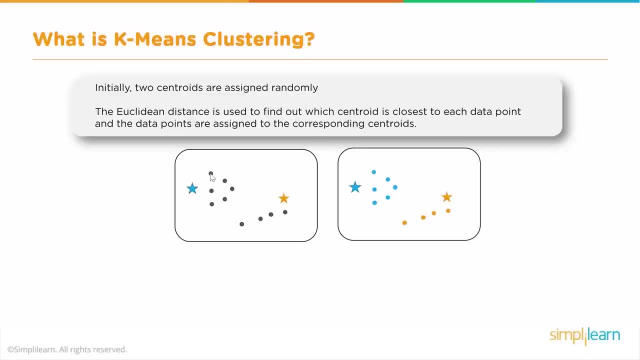 take this point and find the distance from this centroid and the distance from this centroid. this point is taken and the distance is found from this centroid and this and so on and so forth. so we can see that the distance is measured from both the centroids and then whichever distance is less. 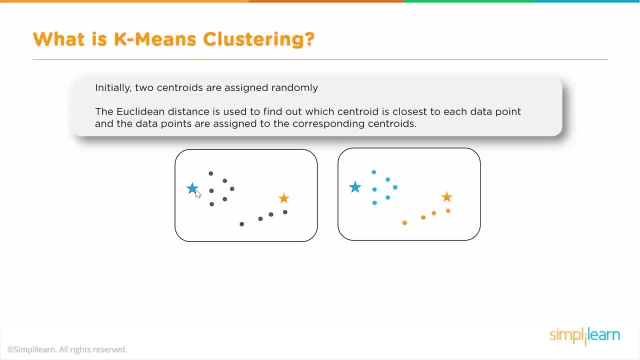 From this centroid, this point is taken and the distance is found from this centroid and this centroid, and so on and so forth. So for every point the distance is measured from both the centroids, and then whichever distance is less, that point is assigned to that centroid. 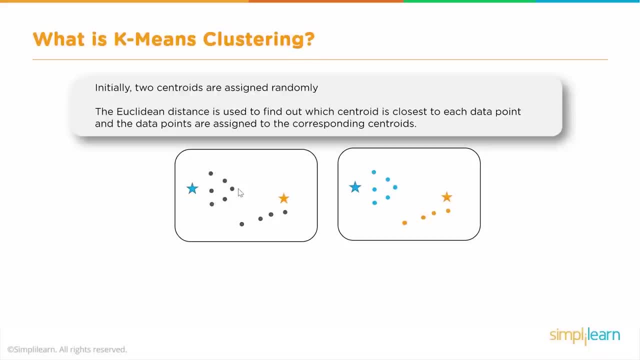 So, for example, in this case, visually, it is very obvious that all these data points are assigned to this centroid and all these data points are assigned to this centroid, And that's what is represented Here in blue color and in this yellow color. the next step is to actually determine the 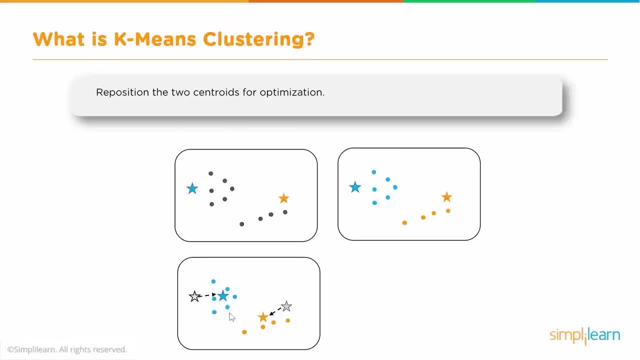 central point or the actual centroid for these two clusters. So we have this one initial cluster, this one initial cluster, But, as you can see, these points are not really the centroid. Centroid means it should be the central position of this dataset, central position of this. 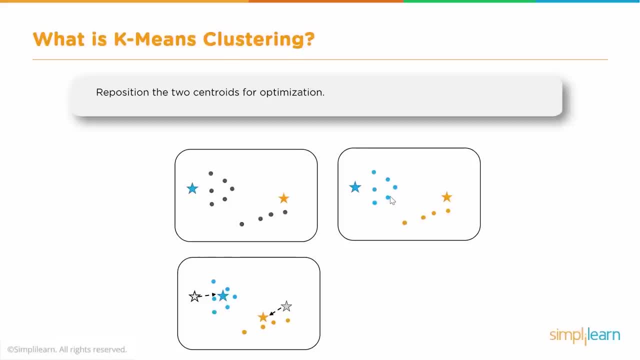 dataset. So that is what needs to be determined as the next step, Central point or the actual centroid is determined and the original randomly allocated centroid is repositioned to the actual centroid of these new clusters And this process is actually repeated. Now what might happen is some of these points may get reallocated. 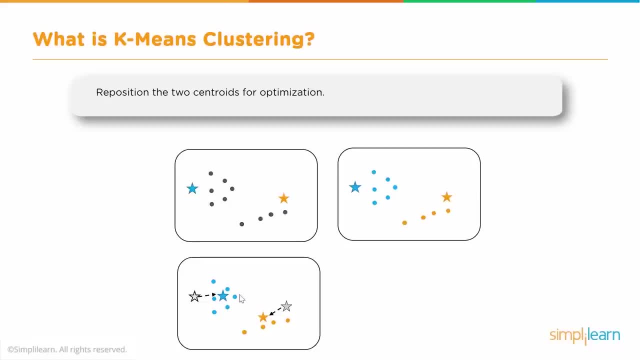 In our example. that is not happening probably, But it may so happen that the distance is found between each of these data points. once again, with these centroids, If it is required, some points may be reallocated. We will see that in a later example. 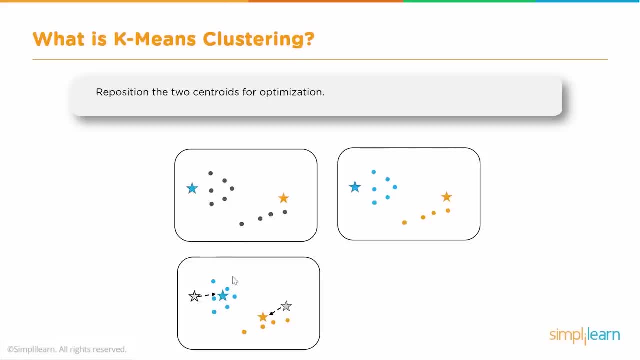 But for now we will keep it simple. So this process is continued till the centroid repositioning stops And that is our final cluster. So this is our. so after iteration, we come to this position, this situation where the centroid doesn't need any more repositioning. 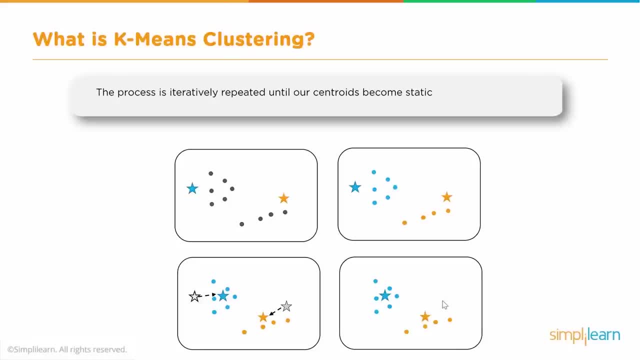 And that means our algorithm has converged, Convergence has occurred And we have the cluster, two clusters, We have the clusters with a centroid. So this process is repeated. The process of calculating the distance and repositioning the centroid is repeated till. 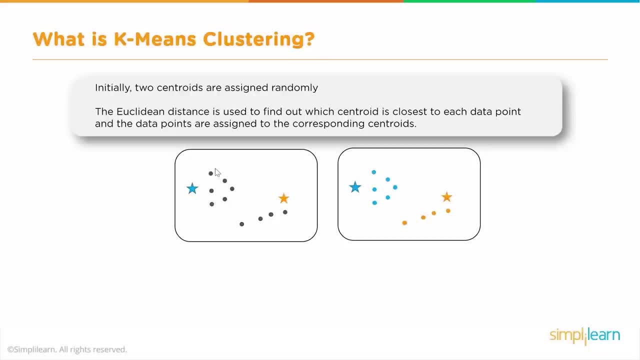 that point is assigned to that centroid. so, for example, in this case, visually it is very obvious that all these data points are assigned to this centroid and all these data points are assigned to this centroid. and that's what is represented here in blue color and in this yellow color, the 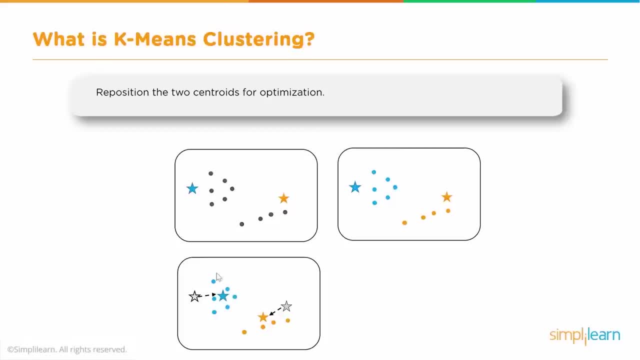 next step is to actually determine the central point or the actual centroid for these two points, two clusters. so we have this one initial cluster, this one initial cluster, but, as you can see, these points are not really the centroid. centroid means it should be the central position of this data set. 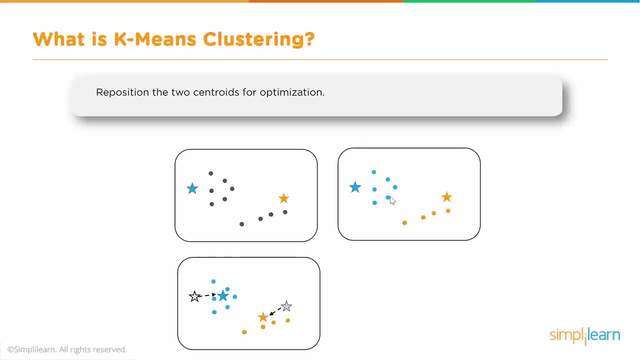 central position of this data set. so that is what needs to be determined as the next step. so the central point or the actual centroid is determined and the original, randomly allocated centroid is repositioned to the actual centroid of this new clusters, and this process is actually repeated. now what might happen is some of these points. 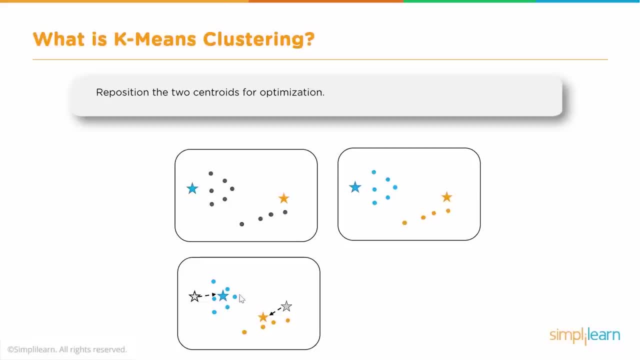 may get reallocated. in our example that is not happening, probably, but it may so happen that the distance is found between each of these data points, once again, with these centroids, and if there is, if it is required, some points may be reallocated. we will see that in a later example. 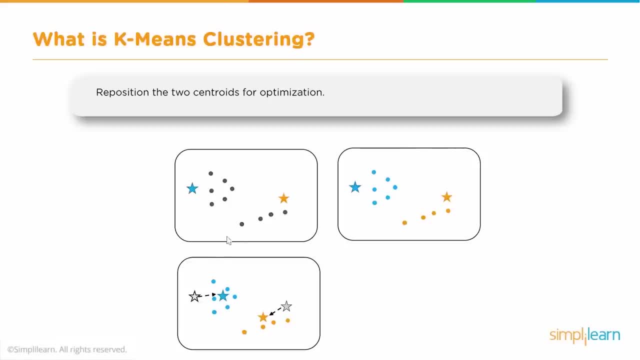 but for now we will keep it simple. so this process is continued till the centroid repositioning stops and that is our final cluster. so this is our. so after iteration, we come to this position, this situation where the centroid doesn't need any more repositioning. 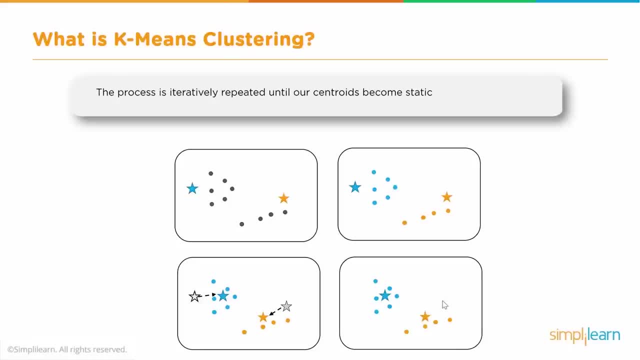 and that means our algorithm has converged, convergence has occurred and we have the cluster, two clusters, we have the clusters with a centroid. so this process is repeated, the process of calculating the distance and repositioning the centroid is repeated till the repositioning stops, which means that 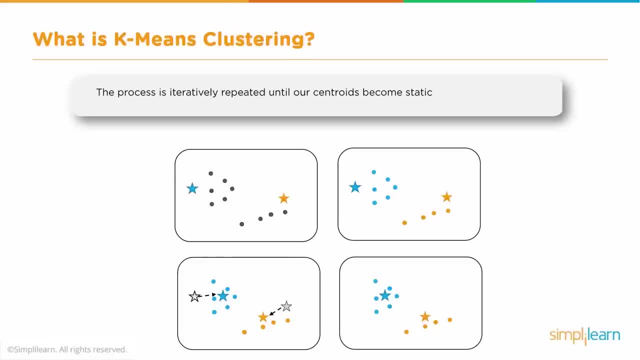 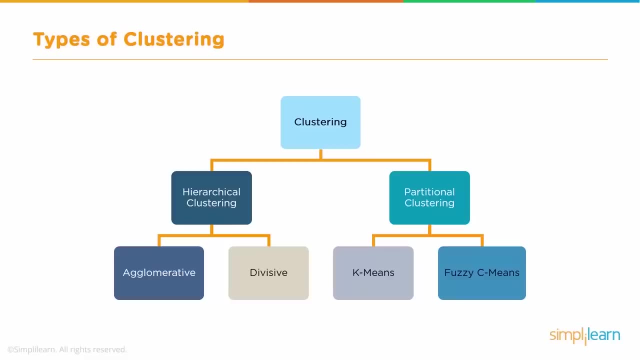 the algorithm has converged and we have the final cluster with the data points. what are the types of clustering? there are primarily two categories of clustering- hierarchical clustering and then partitional clustering- and each of these categories are further subdivided into agglomerative and divisive clustering, and k means and fuzzy c. 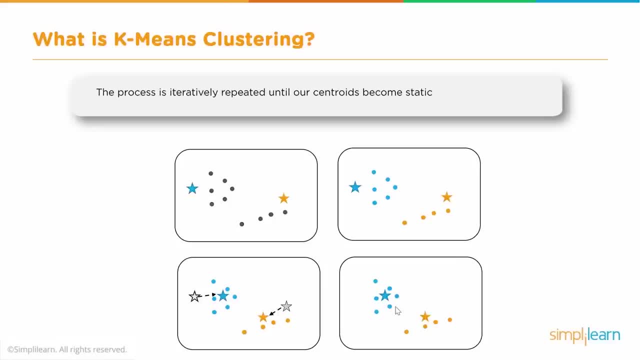 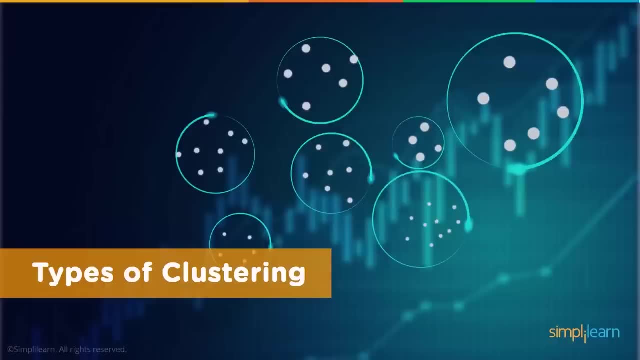 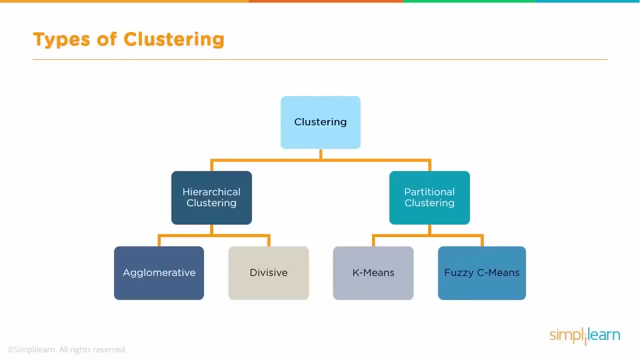 the repositioning stops, which means that the algorithm has converged And we have the final cluster with the data points. What are the types of clustering? There are primarily two categories of clustering: 1. Hierarchical clustering. 2. Partitional clustering. 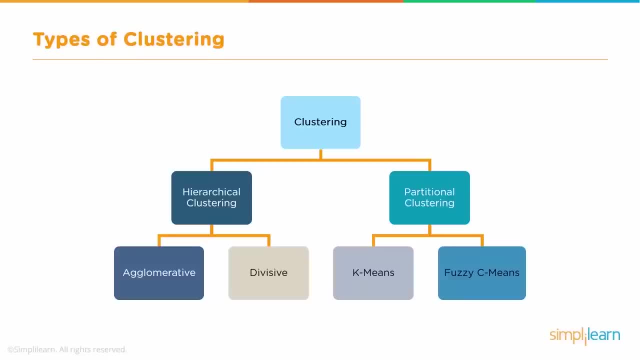 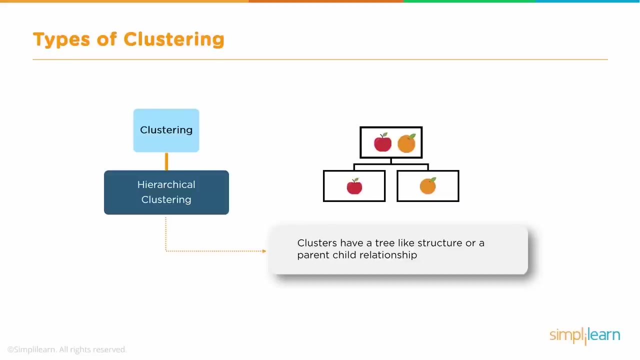 And each of these categories are further subdivided into agglomerative and divisive clustering, and k-means and fuzzy c-means clustering. Let's take a quick look at what each of these types of clustering are. In hierarchical clustering, the clusters have a tree-like structure, and hierarchical clustering 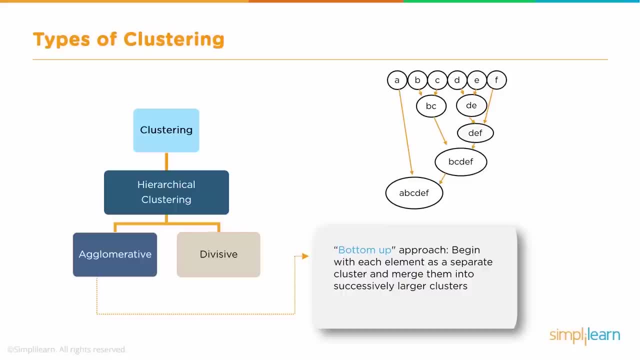 is further divided into agglomerative and divisive. 3. Agglomerative clustering: Agglomerative clustering is a bottom-up approach. We begin with each element as a separate cluster and merge them into successively larger clusters. For example, we have A, B, C, D, E, F. We start by combining B and C form one cluster. 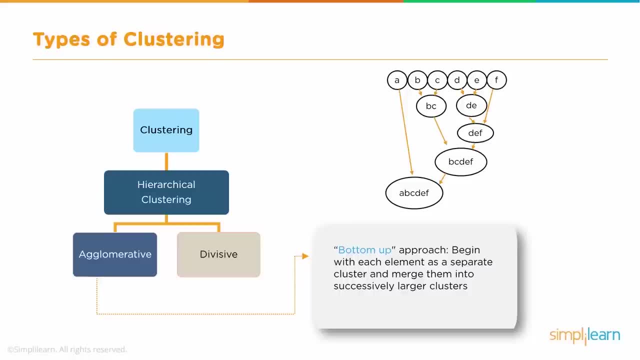 D and E form one more. then we combine D, E and F- one more bigger cluster, and then add B, C to that and then finally A to it. Compared to that, divisive clustering, or divisive clustering, is a top-down approach. 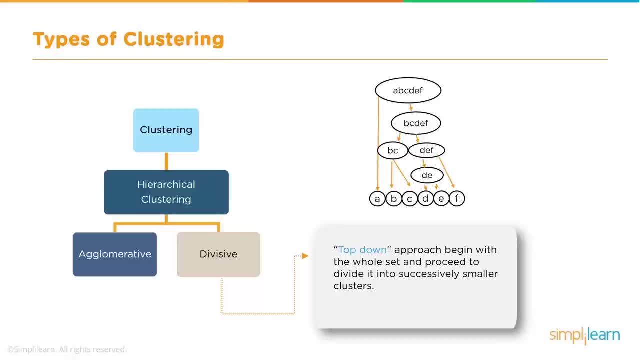 We begin with the whole set and proceed to divisive clustering. So we have A, B, C, D, E, F. We first take that as a single cluster and then break it down into A, B, C, D, E and F. 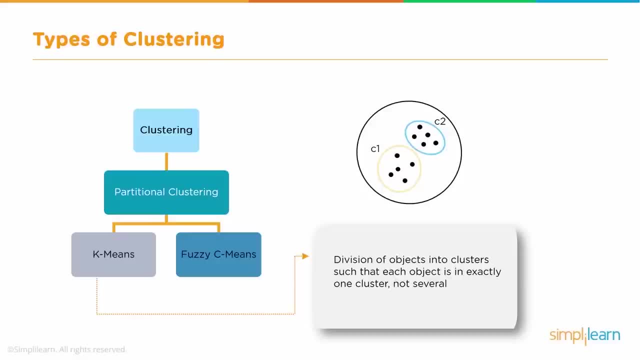 Then we have partitional clustering, split into two subtypes: k-means clustering and fuzzy c-means. In k-means clustering, the objects are divided into the number of clusters mentioned by the number k. That's where the k comes from. 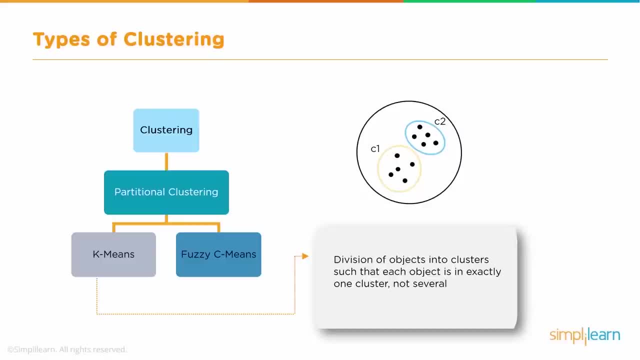 So if we say k is equal to two, the objects are divided into two clusters: C1 and C2.. And the way it is done is the features or characteristics are compared and all objects having similar characteristics are clubbed together. So that's how k-means clustering is done. 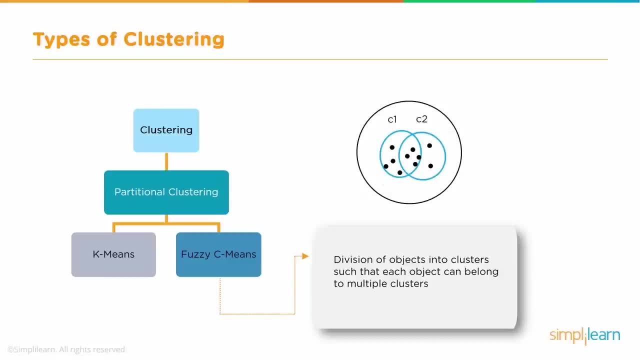 We will see it in more detail as we move forward. And fuzzy c-means is very similar to k-means in the sense that it clubs objects that have similar characteristics together. In k-means, clustering two objects cannot belong to, or any object a single object. 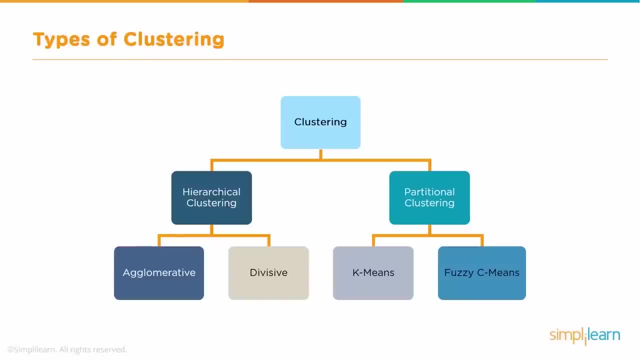 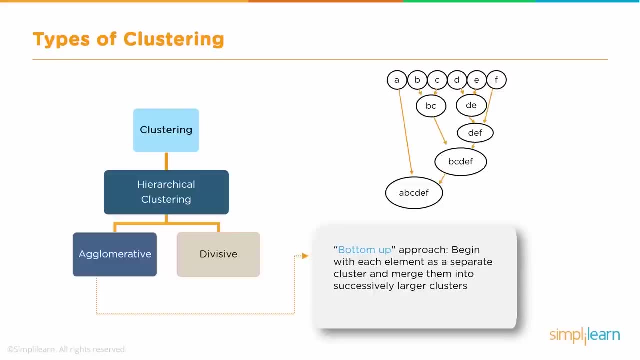 means clustering. let's take a quick look at what each of these types of clustering are. in hierarchical clustering, the clusters have a tree-like structure, and hierarchical clustering is further divided into agglomerative and divisive. agglomerative clustering is a bottom-up approach. we begin with each element as a separate cluster. 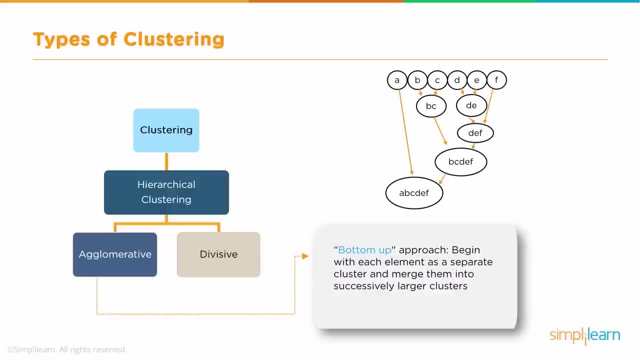 and merge them into successively larger clusters. so for example, we have a, b, c, d, e, f. we start by combining b and c form one cluster, d and e form one more. then we combine d, e and f- one more bigger cluster, and then add b, c to that and then finally a to it. compared to that divisive 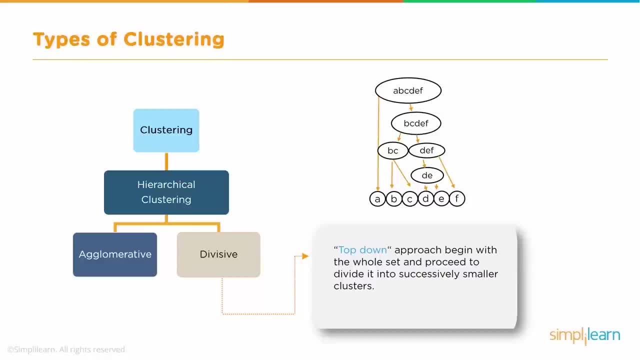 clustering or divisive clustering is a top-down approach. we begin with the whole set and proceed to divide it into successively smaller clusters. so we have a, b, c, d e, f. we first take that as a single cluster and then break it down into a, b, c, d, e and f. 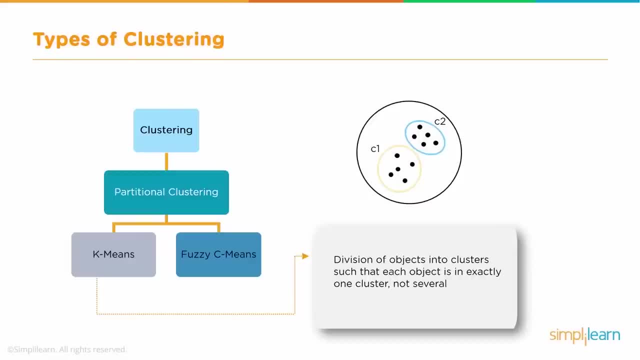 then we have partitional clustering, split into two subtypes: k-means clustering and fuzzy c-means. in k-means clustering the objects are divided into the number of clusters mentioned by the number k. that's where the k comes from. so if we say k is equal to 2, the objects are divided into. 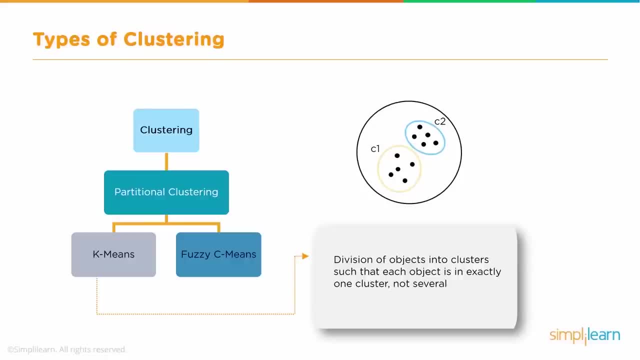 two clusters, c1 and c2, and the way it is done is the features or characteristics are compared and all objects having similar characteristics are clubbed together. so that's how k-means clustering is done. we will see it in more detail as we move forward, and fuzzy c-means is very 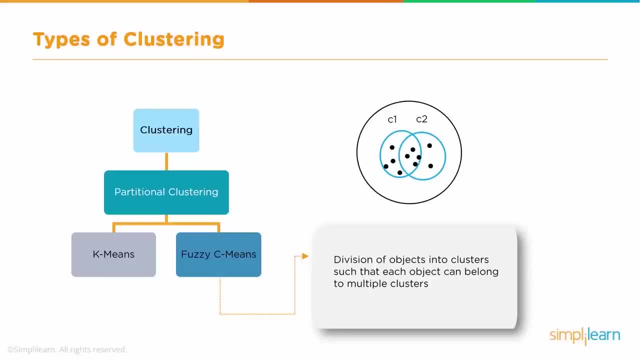 similar to k-means in the sense that it clubs objects that have similar characteristics together, but while in k-means clustering two objects cannot belong to or any object, a single object cannot belong to two different clusters. in c-means objects can belong to more than one cluster. 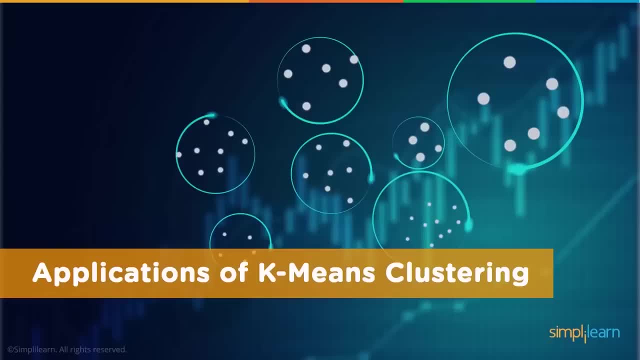 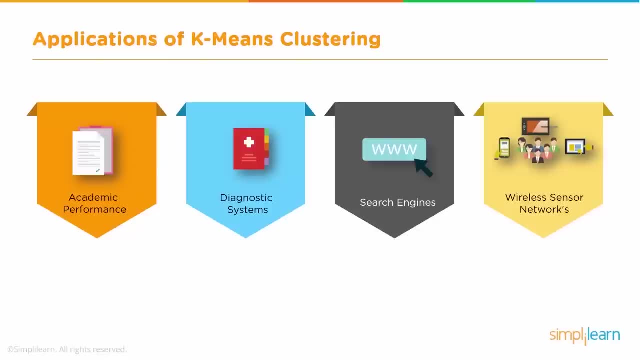 so that's how k-means clustering is done- is the primary difference between k-means and fuzzy c-means. so what are some of the applications of k-means clustering? k-means clustering is used in a variety of examples or variety of business. 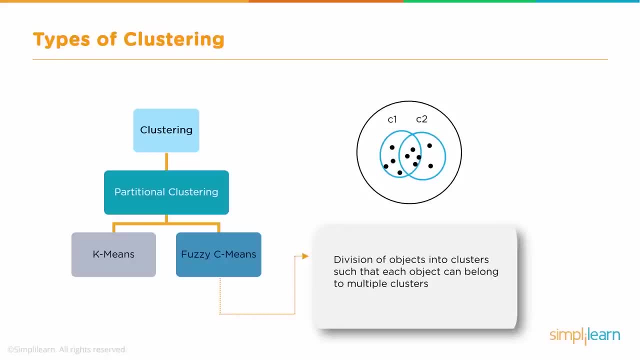 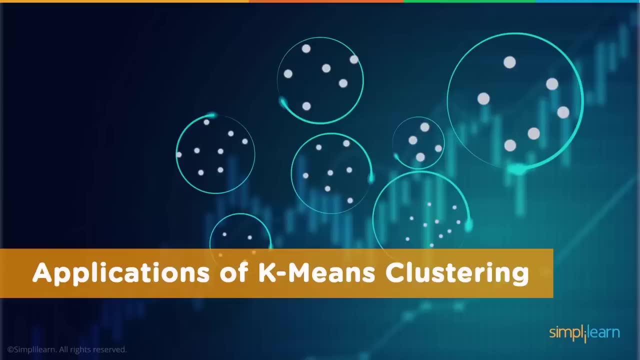 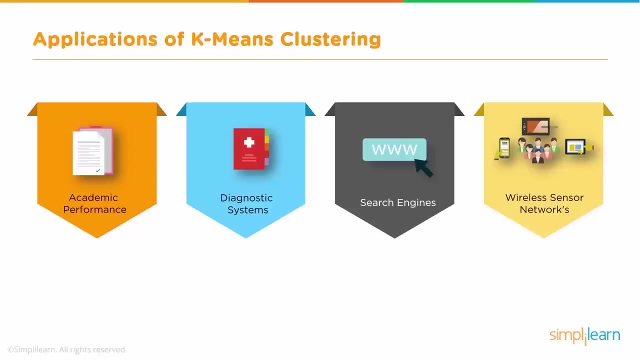 cannot belong to two different clusters. In c-means, objects can belong to more than one cluster. So that is the primary difference between k-means and fuzzy c-means. So what are some of the applications of k-means clustering? K-means clustering is used in a variety of examples or a variety of business cases in 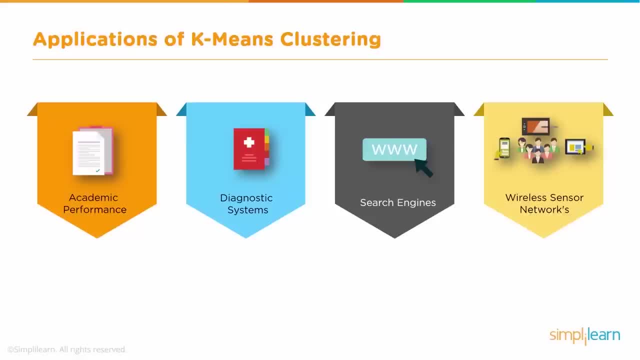 real life, starting from academic performance, diagnostic systems, search engines and so on. So let us take a little deeper look at each of these examples. Academic performance, So, based on the scores of the students, students are categorized into A, B, C and so on. 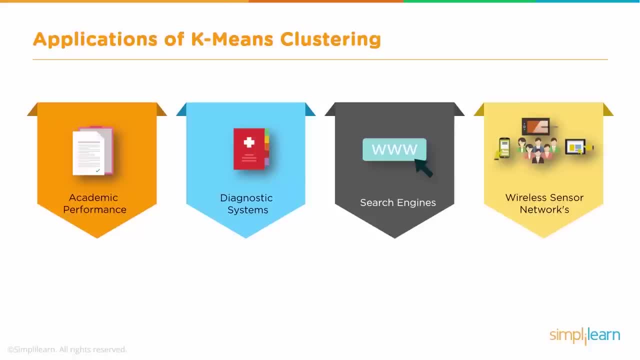 Clustering forms a backbone of search engines. When a search is performed, the search results need to be grouped together. The search engines very often use clustering to do this And, similarly, in case of wireless sensor networks, The clustering algorithm plays the role of finding the cluster heads, which collects. 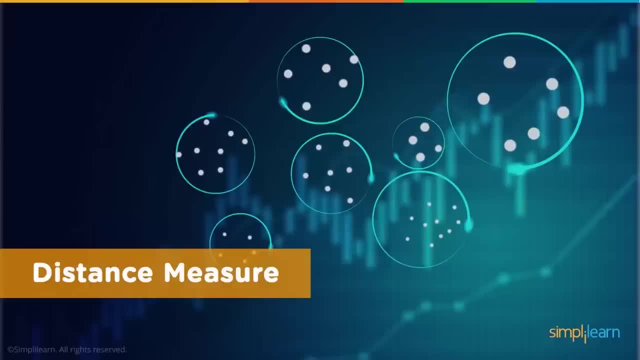 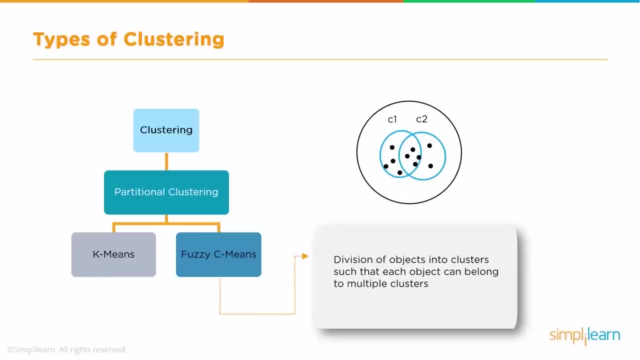 all the data in its respective cluster. So clustering, especially k-means clustering- uses distance measure, So let's take a look at what is distance measure. So, while these are the different types of clustering, in this video, we will focus on 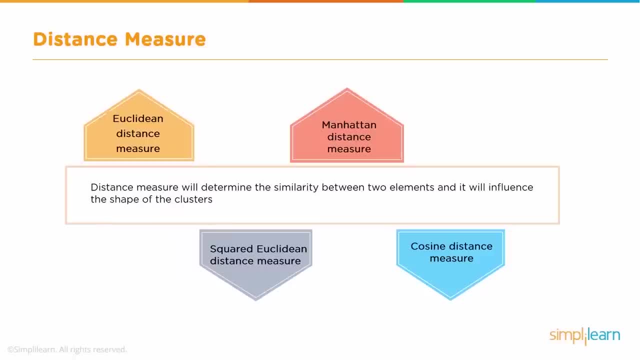 k-means clustering. So distance measure tells how similar some objects are. So the similarity is measured. So the similarity is measured using what is known as distance measure. And what are the various types of distance measures? There is Euclidean distance, There is Manhattan distance. 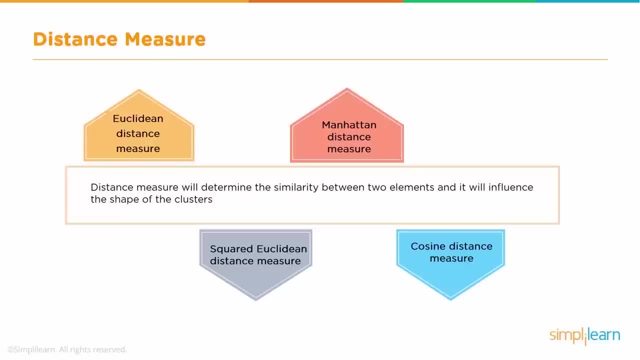 Then we have squared Euclidean distance measure and cosine distance measure. These are some of the distance measures supported by k-means clustering. Let's take a look at each of these. What is Euclidean distance measure? This is nothing but the distance between two points. 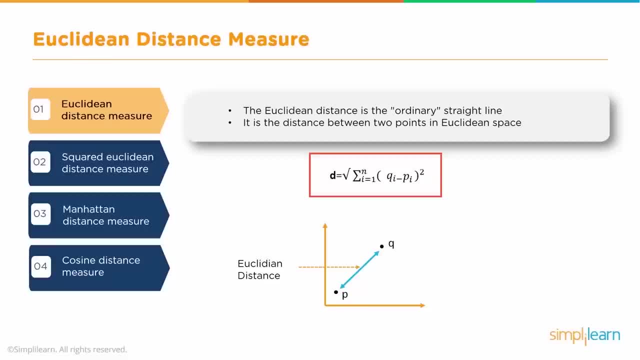 So we have learned in high school How to find the distance between two points. This is a little sophisticated formula for that, but we know a simpler one is: square root of y2 minus y1, whole square plus x2 minus x1, whole square. 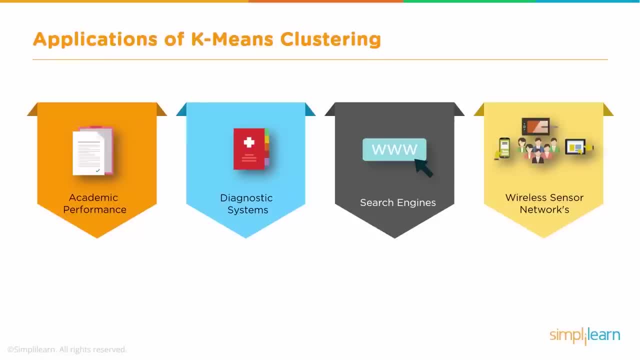 cases in real life, starting from academic performance, diagnostic systems, search engines and wireless sensor networks, and many more. so let us take a little deeper look at each of these examples. academic performance, so, based on the scores of the students, students are categorized into a, b, c and so on. clustering forms the backbone of search engines when a search is performed. the. 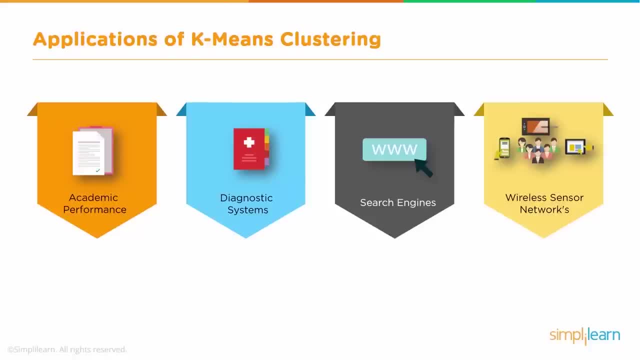 search results need to be grouped together. the search engines very often use clustering to do this and similarly, in case of wireless sensor networks, the clustering algorithm plays the role of finding the cluster heads, which collects all the data, and the data are the cluster heads in its respective cluster. so clustering especially k-means- clustering uses distance measure, so let's 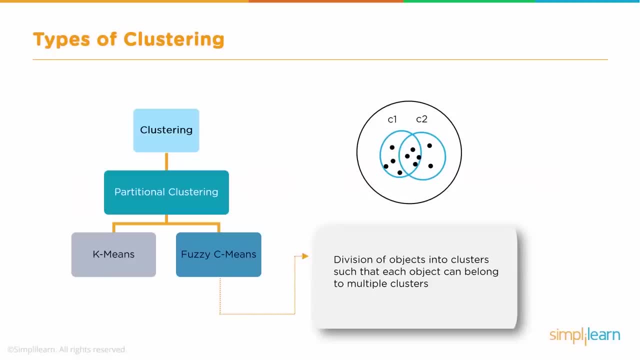 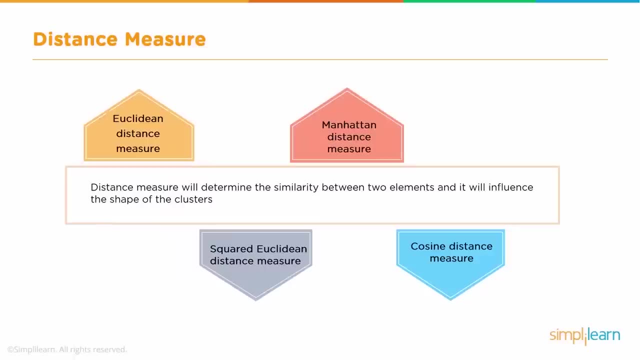 take a look at what is distance measure. so, while these are the different types of clustering, in this video we will focus on k-means clustering. so distance measure tells how similar some objects are. so the similarity is measured using what is known as distance measure. and what are the various? 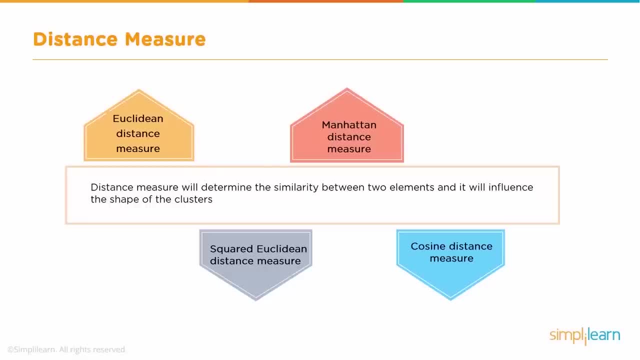 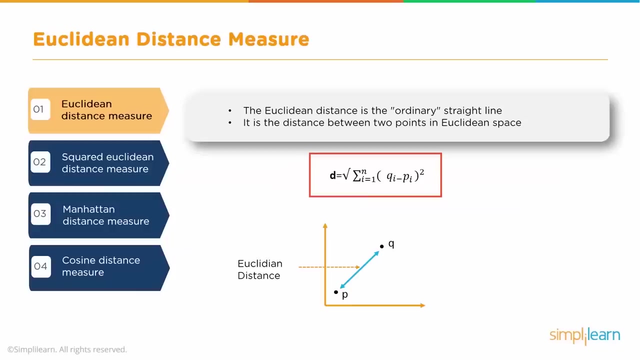 types of distance measures. there is euclidean distance, there is manhattan distance, then we have squared euclidean distance measure and cosine distance measure. these are some of the distance measures supported by k-means clustering. let's take a look at each of these. what is euclidean? 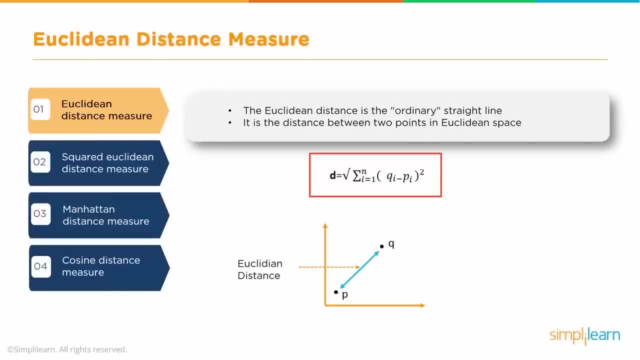 distance measure. this is nothing but the distance between two points. so we have learnt in high school how to find the distance between two points. this is a little sophisticated formula for that, but we know a simpler one. is square root of y2 minus y1 whole. square plus x2 minus x1 whole. 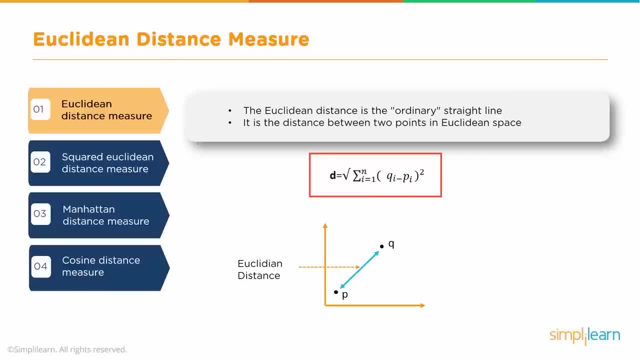 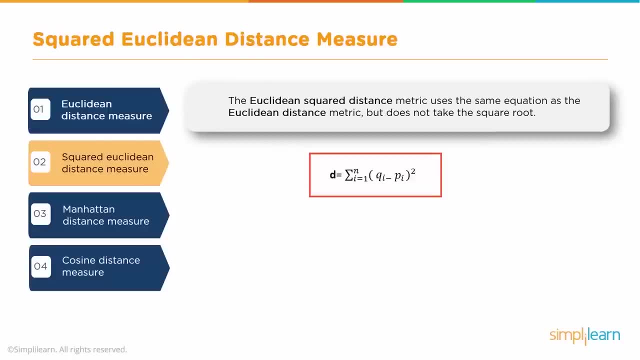 square. so this is an extension of that formula. so that is the euclidean distance between two points. what is the squared euclidean distance measure? it's nothing but the square of the euclidean distance, as the name suggests. so instead of taking the square root, we leave the square as it is, and then 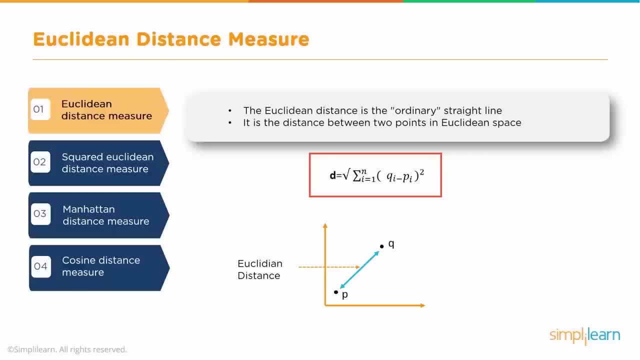 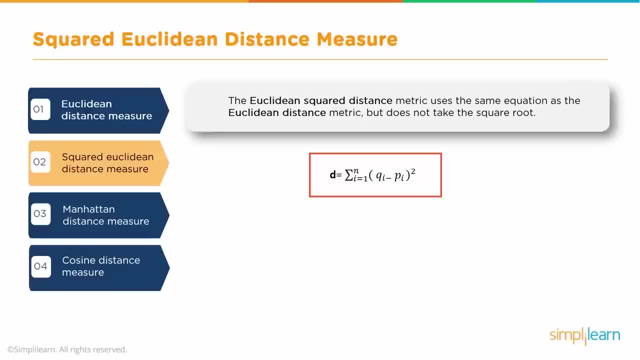 So this is an extension of that formula. So that is the Euclidean distance between two points. What is the squared Euclidean distance measure? It's nothing but the square of the Euclidean distance. as the name suggests, Instead of taking the square root, we leave the square as it is. 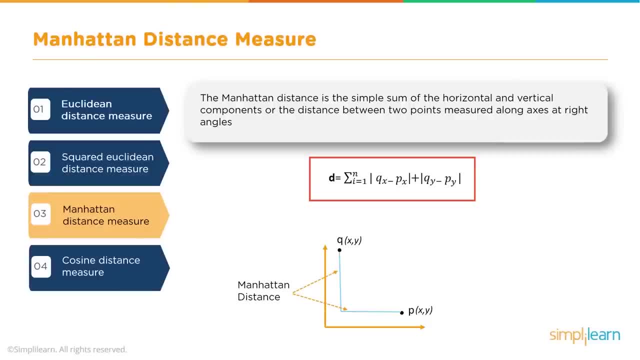 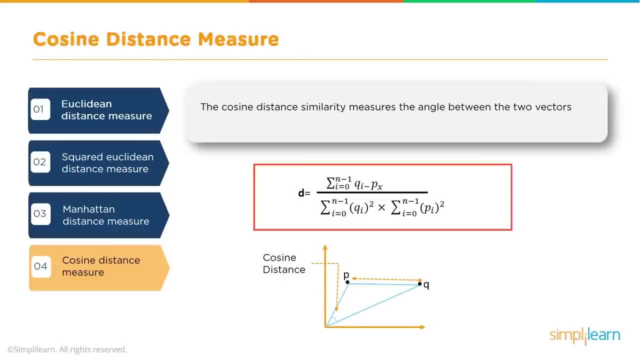 And then we have Manhattan distance measure. In case of Manhattan distance, it is the sum of the distances across the x-axis and the y-axis, And note that we are taking the absolute value so that the negative values don't come into play. So that is the Manhattan distance measure. 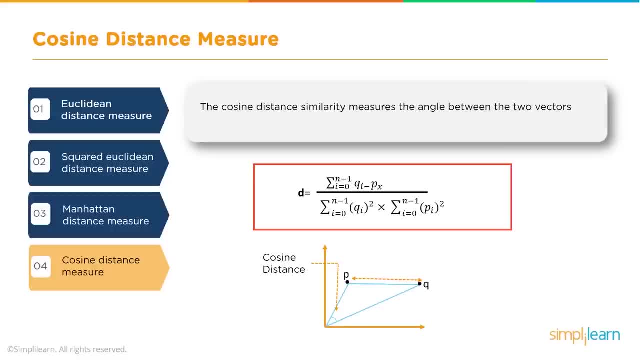 Then we have cosine distance measure. In this case we take the angle between the two vectors Formed by joining two points, Formed by joining the points from the origin. So that is the cosine distance measure. Okay, so that was a quick overview about the various distance measures that are supported. 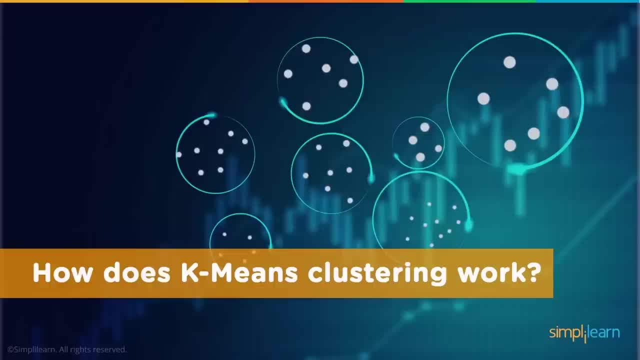 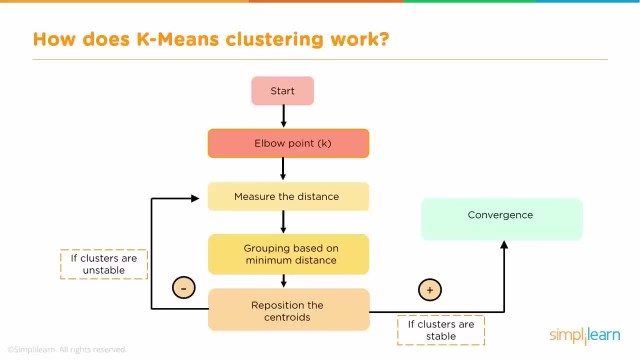 by k-means. Now let's go and check how exactly k-means clustering works. Okay, so this is how k-means clustering works. This is like a flow chart of the whole process. There is a starting point and then we specify the number of clusters that we want. 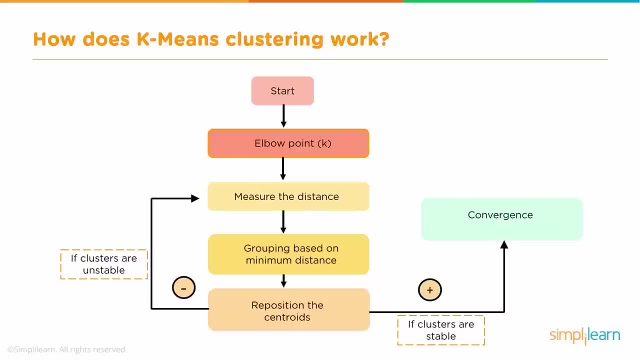 Now there are a couple of ways of doing this. We can do by trial and error. So we specify a certain number, Maybe k is equal to 3 or 4 or 5 to start with, And then as we progress, we keep changing until we get the best clusters. 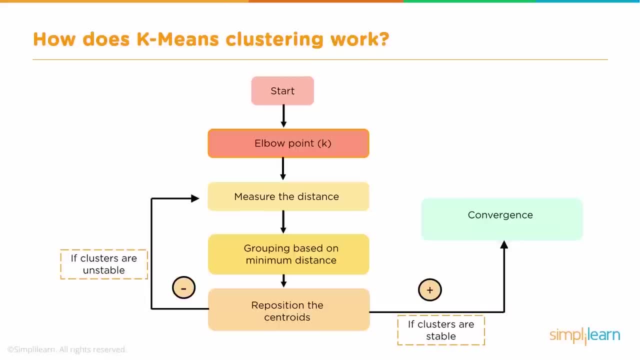 Or there is a technique called Elbow technique, whereby we can determine the value of k. What should be the best value of k? How many clusters should be formed? So once we have the value of k, we specify that And then the system works. 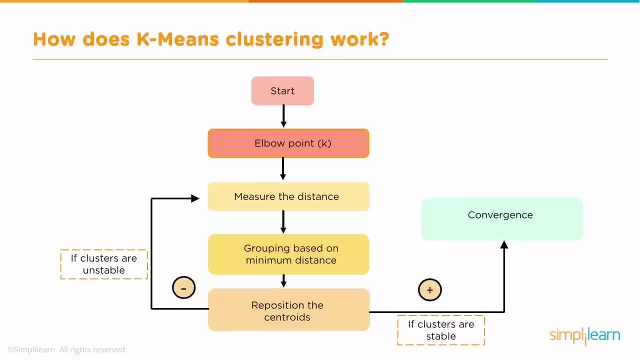 will assign that many centroids. so it picks randomly that to start with, randomly that many points that are considered to be the centroids of these clusters, and then it measures the distance of each of the data points from these centroids and assigns those points to the corresponding centroid, from which. 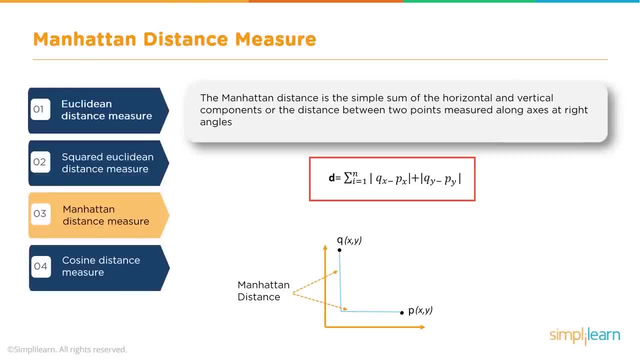 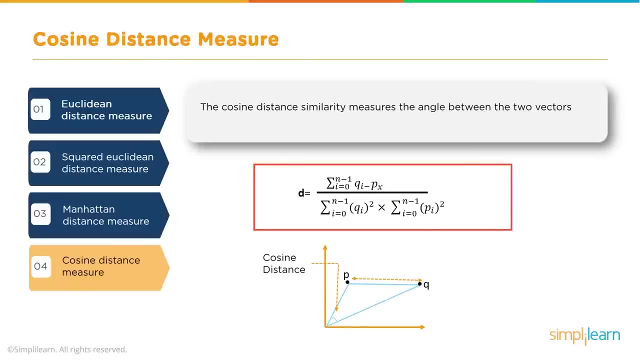 Manhattan distance measure. in case of manhattan distance, it is the sum of the distances across the x-axis and the y-axis, and note that we are taking the absolute value so that the negative values don't come into play. so that is the manhattan distance measure. then we have 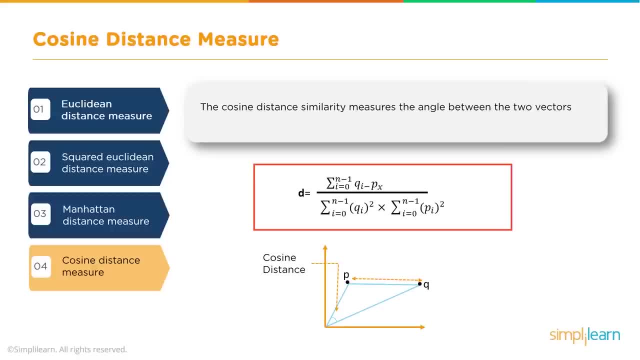 cosine distance measure. in this case, we take the angle between the two vectors formed by joining the points from the origin. so that is the cosine distance measure. okay, so that was a quick overview about the various distance measures that are supported by k-means. now let's go. 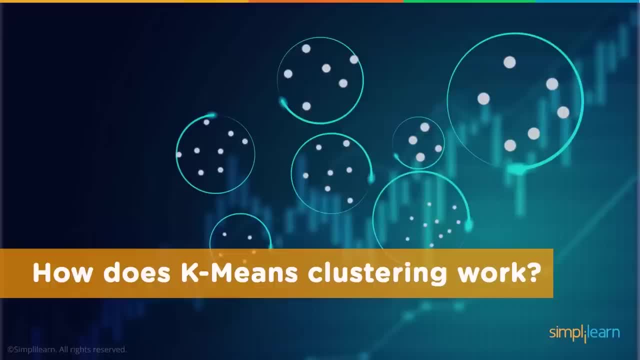 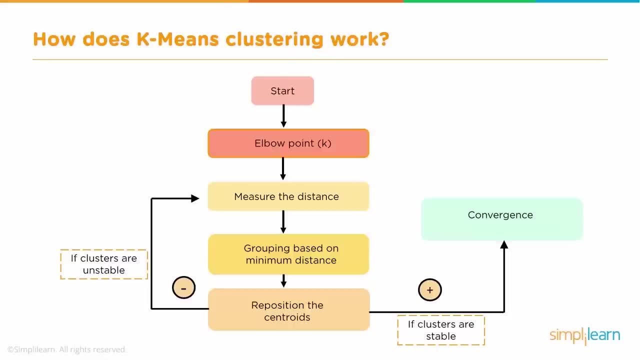 and check how exactly k-means clustering works. okay, so this is how k-means clustering works. this is like a flow chart of the whole process. there is a starting point and then we specify the number of clusters that we want. now there are a couple of ways of doing this. we can do by trial and error, so 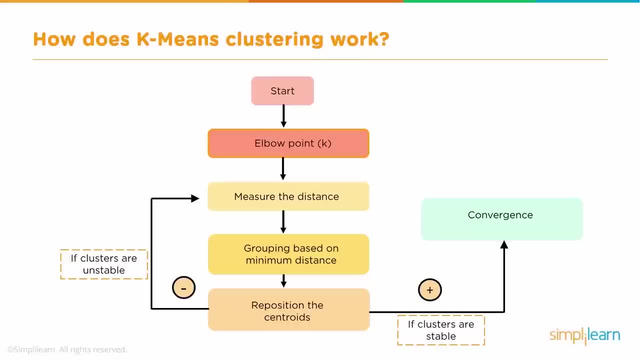 a certain number. maybe k is equal to 3 or 4 or 5 to start with, and then, as we progress, we keep changing until we get the best clusters. or there is a technique called elbow technique, whereby we can determine the value of k. what should be the best value of k? how many clusters should be formed? 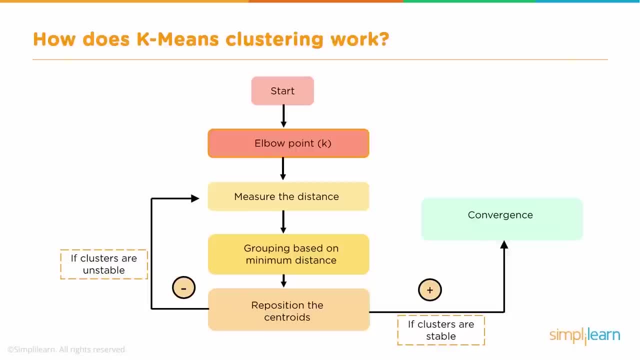 so once we have the value of k, we specify that and then the system will assign that many centroids. so k is equal to 3 or 4 or 5 to start with, and k is equal to 3 or 5 to start with, and k is equal to 3 or 5 to start with. 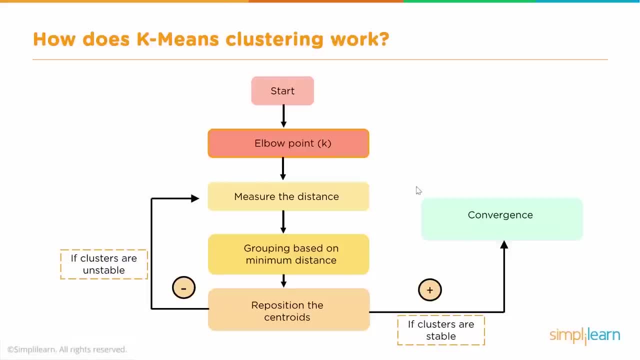 and then it measures the distance of each of the data points from these centroids and assigns those points to the corresponding centroid from which the distance is minimum. so each data point will be assigned to the centroid which is closest to it, and thereby we have k number of initial clusters. 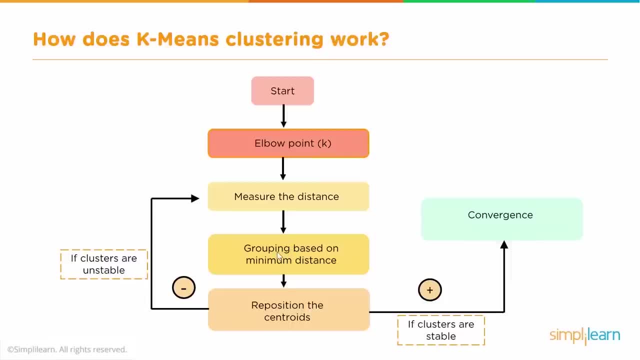 this is not the final clusters. the next step it does is for the new groups, for the clusters that have been formed, it calculates the mean position, thereby calculates the new centroid position. the position of the centroid moves compared to the randomly allocated one, so it's an iterative. 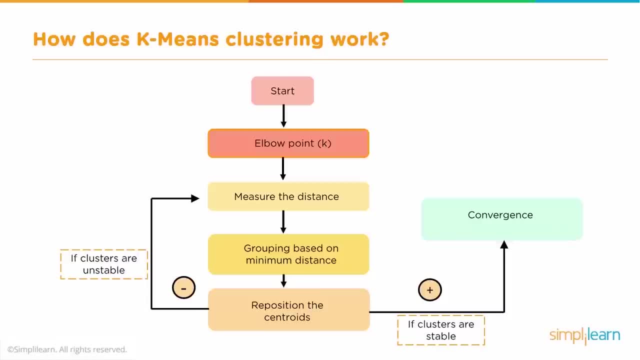 the distance is minimum, so each data point will be assigned to the centroid which is closest to it, and thereby we have K number of initial clusters. however, this is not the final clusters. the next step it does is for the new groups. for the clusters that have been formed, it calculates the mean position. 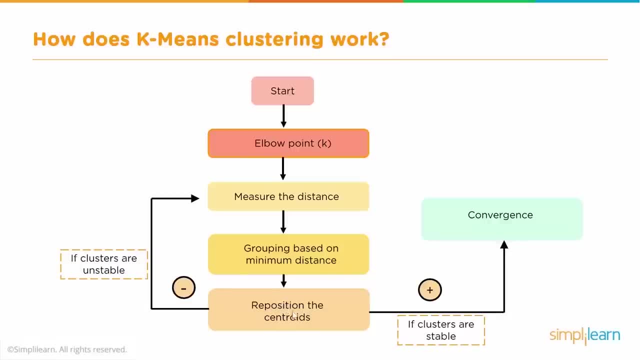 thereby calculates the new centroid position. the position of the centroid moves compared to the randomly allocated one, so it's an iterative process. once again, it is a process of calculating the position of the centroid. and then it again: the distance of each point is measured from this new centroid point and 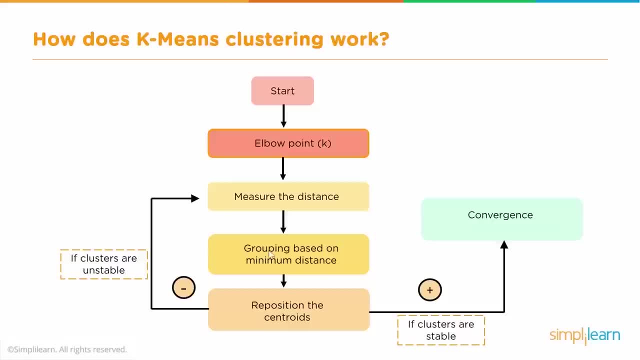 if required, the data points are reallocated to the new centroids and the mean position or the new centroid is calculated once again. if the centroid moves, then the iteration continues, which means the convergence has not happened, the clustering has not converged. so as long as there is a movement of the 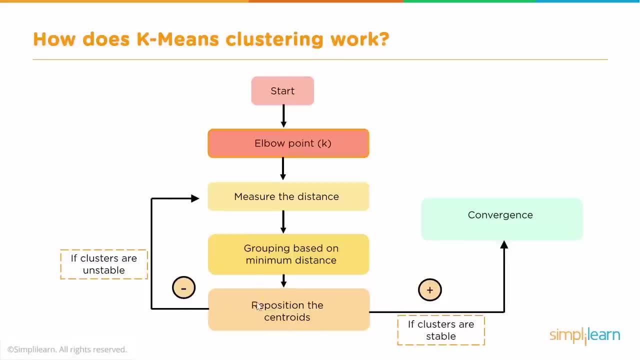 centroid. this iteration keeps happening, but once the centroid stops moving, which means that the cluster has converged or the clustering process has converged- that will be the end result. so now we have the final position of the centroid and the data points are allocated accordingly to the closest centroid. I know it's a little difficult to understand from this. 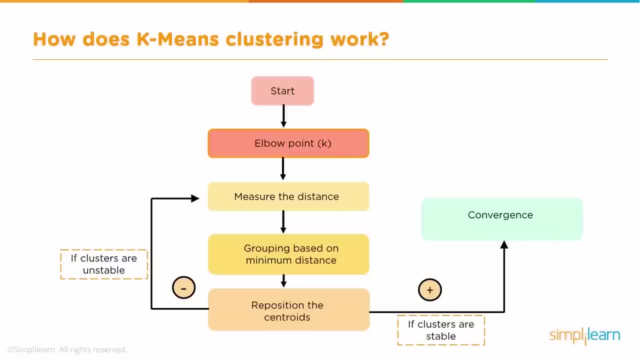 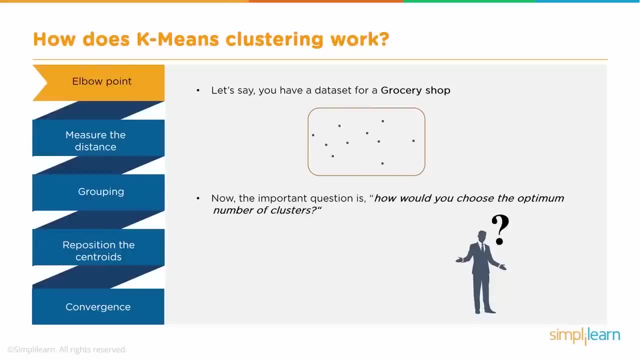 simple flowchart. so let's do a little bit of visualization and see if we can explain it better. let's take an example. if we have a simple flow chart like this, have a data set for a grocery shop. so let's say we have a data set for a grocery shop and now we 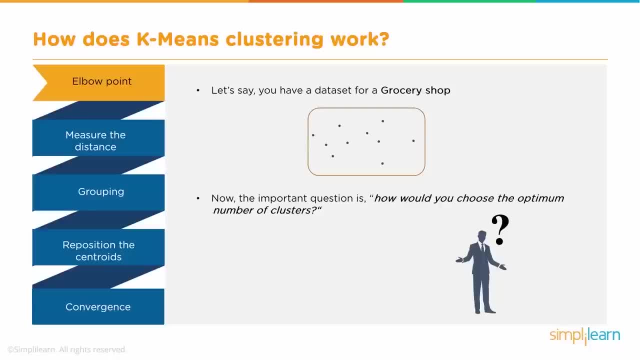 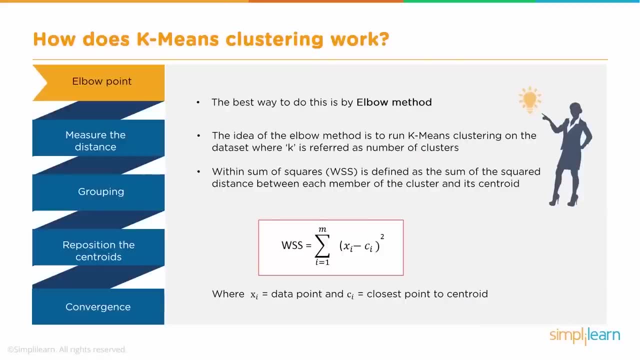 want to find out how many clusters. this has to be spread across. so how do we find the optimum number of clusters? there is a technique called the elbow method. so when these clusters are formed, there is a parameter called within sum of squares, and the lower this value is, the better the cluster. 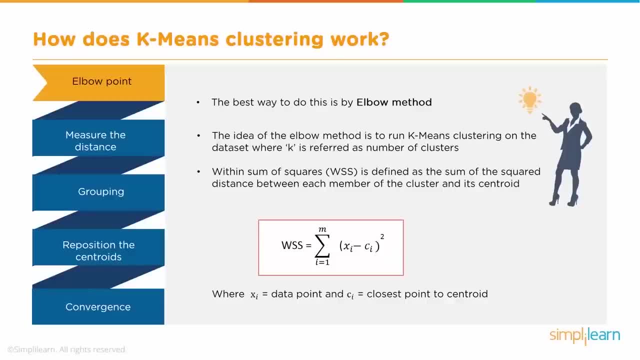 is. that means all these points are very close to each other. so we use this within sum of squares as a measure to find the optimum number of clusters that can be formed for a given data set. so we create clusters, or we let the system create clusters of a variety of numbers, maybe of 10. 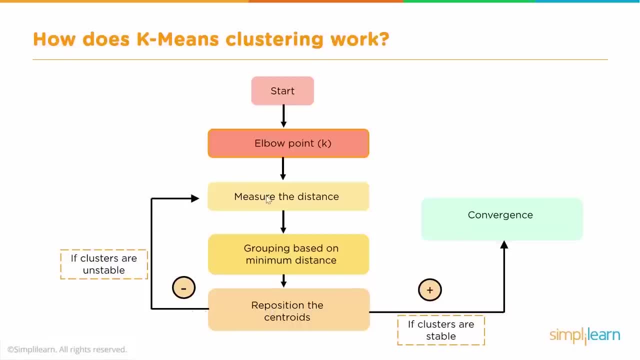 process. once again, the distance of each point is measured from this new centroid point and, if required, the data points are kept on the same position. so the distance of each point must be measured from any point of this new centroid point and the distance of each point must be measured. 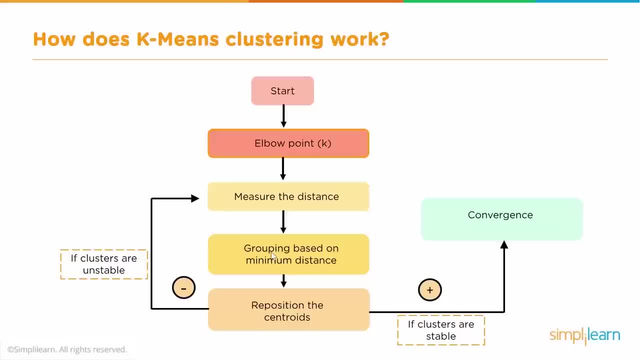 reallocated to the new centroids and the mean position or the new centroid is calculated once again. if the centroid moves, then the iteration continues, which means the convergence has not happened, the clustering has not converged. so as long as there is a movement of the centroid, this iteration keeps happening. but once the centroid stops moving, which means that the cluster, 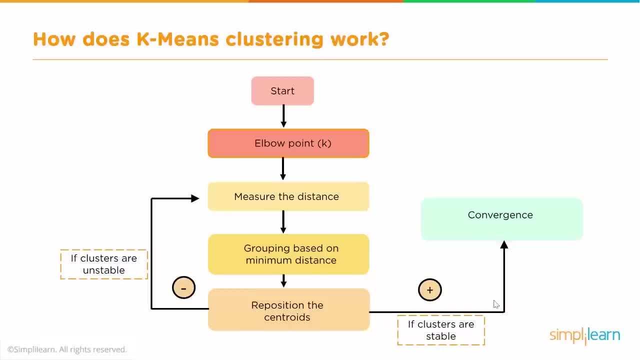 has converged or the clustering process has converged. that will be the end result. so now we have the final position of the centroid and the data points are allocated accordingly to the closest centroid. i know it's a little difficult to understand from this simple flowchart, so let's. 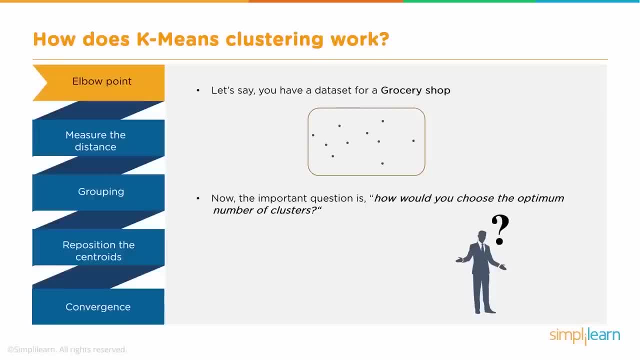 do a little bit of visualization and see if we can explain it better. let's take an example: if we have a data set for a grocery shop. so let's say we have a data set for a grocery shop and now we want to find out how many clusters this has to be. 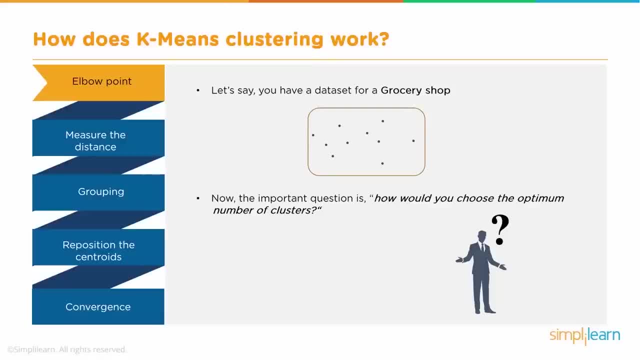 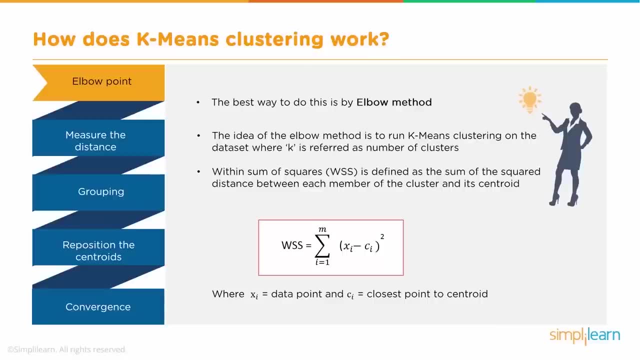 spread across. so how do we find the optimum number of clusters? there is a technique called the elbow method. so when these clusters are formed, there is a parameter called within sum of squares, and the lower this value is, the better the cluster is. that means all these points are very close to each. 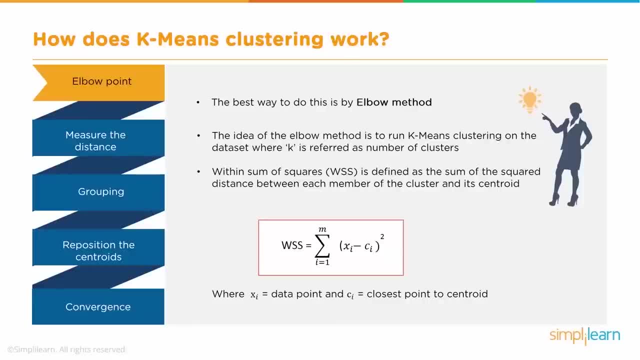 other. so we use this within sum of squares as a measure to find the optimum number of clusters that can be formed for a given data set. so we create clusters, or we let the system create clusters of a variety of numbers, maybe of 10, 10 clusters, and for each value of k, the within ss. 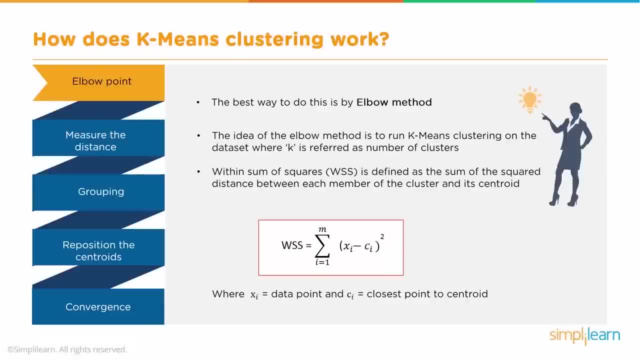 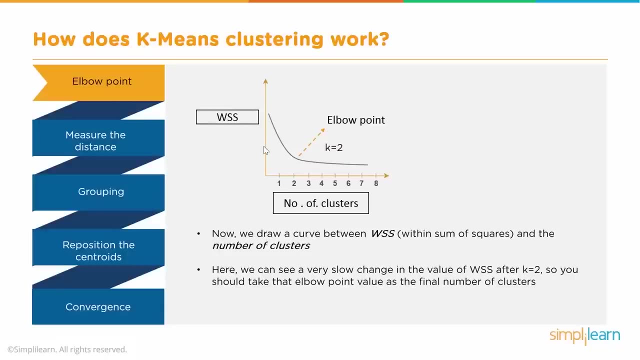 is measured and the value of k, which has the least amount of within ss or wss, that is taken as the optimum value of k. so this is the diagrammatic representation. so we have on the y-axis the within sum of squares or wss, and on the x-axis we have the number of clusters. so, as you, 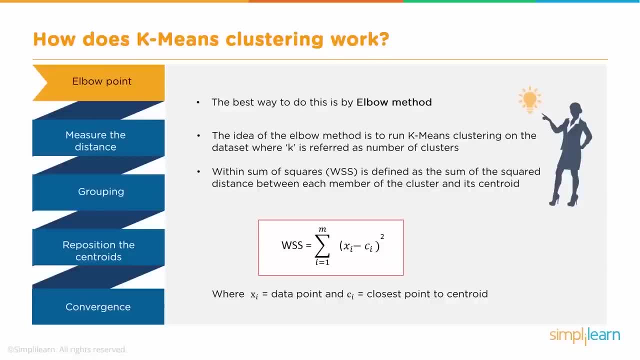 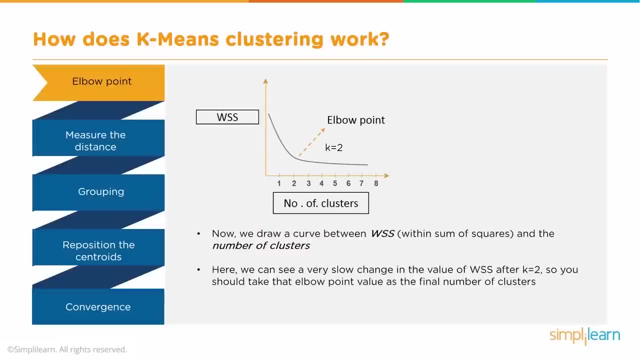 10 clusters and for each value of k, the within ss is a measured and the value of k which has the least amount of within ss or wss, that is taken as the optimum value of k. so this is the diagrammatic representation. so we have on the y-axis the 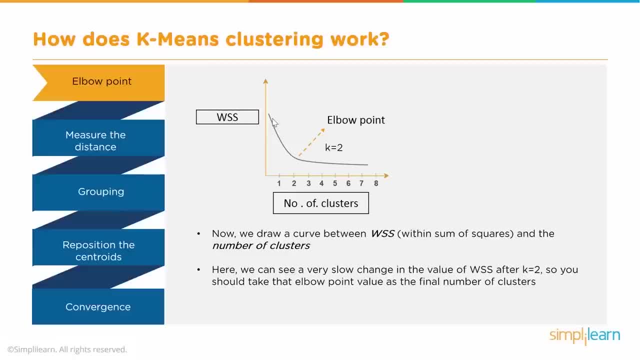 within sum of squares, or wss, and on the x-axis we have the number of clusters. so, as you can imagine, if you have, k is equal to 1, which means all the data points are in a single cluster, the within ss value will be very high because they are probably scattered all over the moment you split. 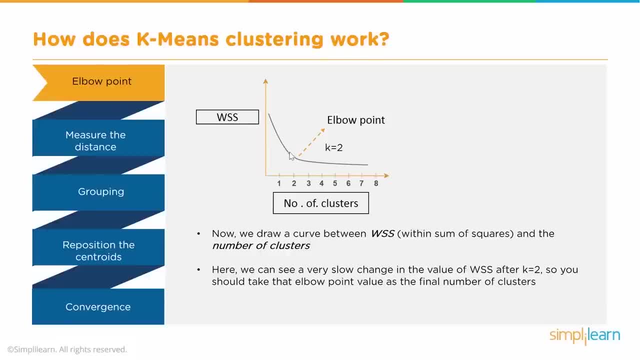 it into two, there will be a drastic fall in the within ss value. that's what is represented here. but then as the value of k increases, the decrease, the rate of decrease will not be so high. it will continue to decrease, but probably the rate of decrease will not be high. 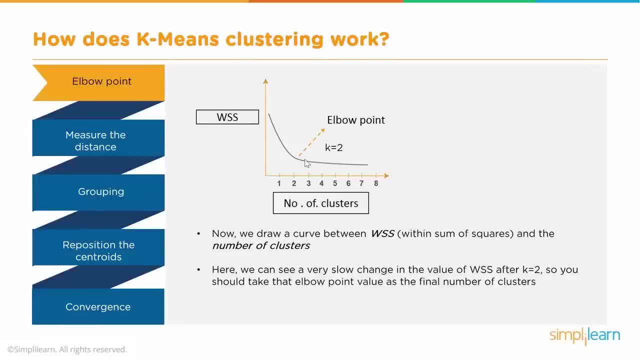 so that gives us an idea. so from here we get an idea. for example, the optimum value of k should be either 2 or 3 or at the most 4, but beyond that increasing the number of clusters is not dramatically changing the value in wss, because 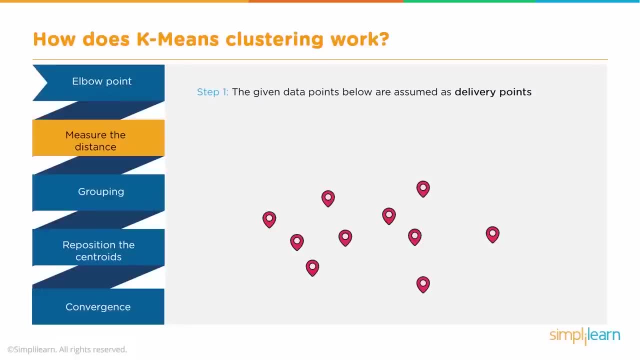 that pretty much gets stabilized. okay, now that we have got the value of k, and let's assume that these are our delivery points, the next step is basically to assign two centroids randomly. so we will be assigning the centroids as the points that are closest to c1 and c2 are the centroids. 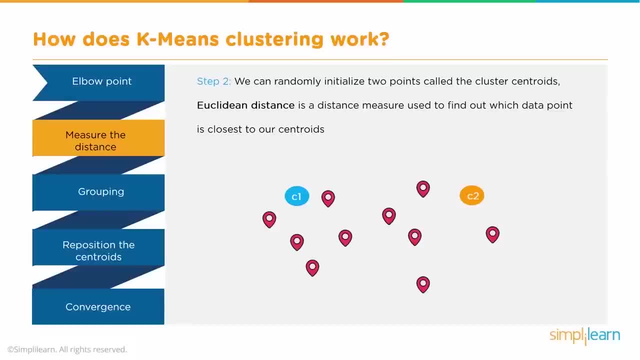 assigned randomly. now the distance of each location from the centroid is measured and each point is assigned to the centroid which is closest to it. so, for example, these points are very obvious, that these are closest to c1, whereas this point is far away from c2. so these points will be assigned. 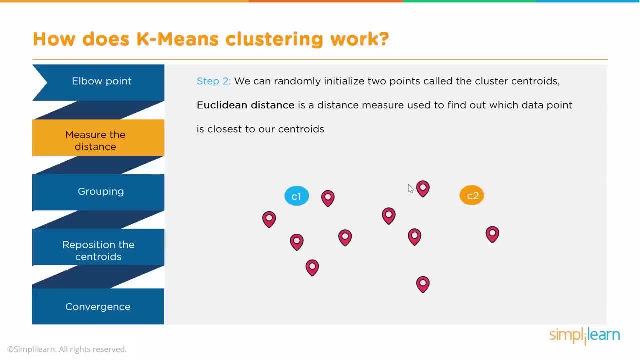 which are close to c1 will be assigned to c1, which are close to C2 will be assigned to C2 and then. so this is the how the initial grouping is done. this is part of C1 and this is part of C2. then the next. 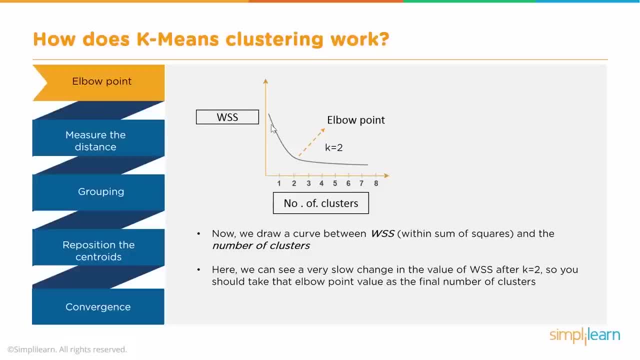 can imagine if you have k is equal to 1, which means all the data points are in a single cluster: the within ss and the within sum of squares. so we have a minimum value of k. so we use the same value will be very high because they are probably scattered all over The moment you split it into. 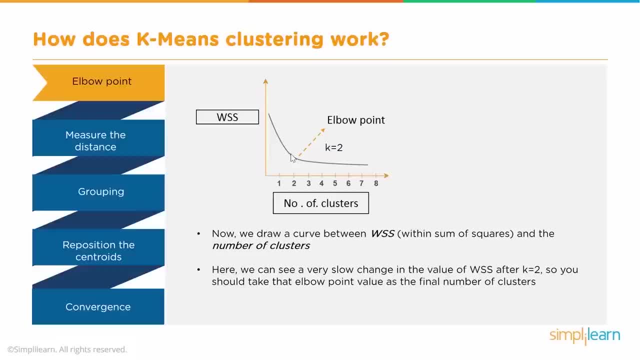 2, there will be a drastic fall in the within SS value. That's what is represented here. But then as the value of k increases, the decrease, the rate of decrease will not be so high. It will continue to decrease, but probably the rate of decrease will not be high. So that gives us an. 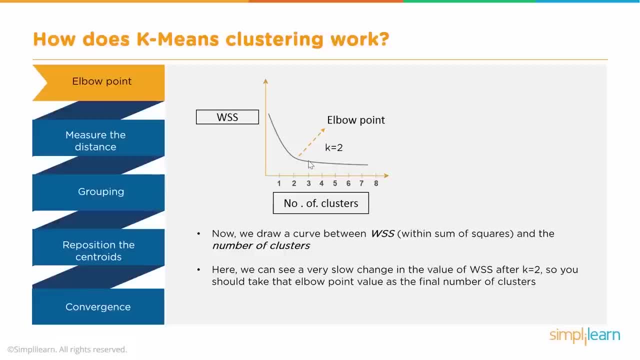 idea. So from here we get an idea. for example, the optimum value of k should be either 2 or 3 or at the most 4.. But beyond that, increasing the number of clusters is not dramatically changing the value in WSS, because that pretty much gets stabilized. Okay, now that we have got the value, 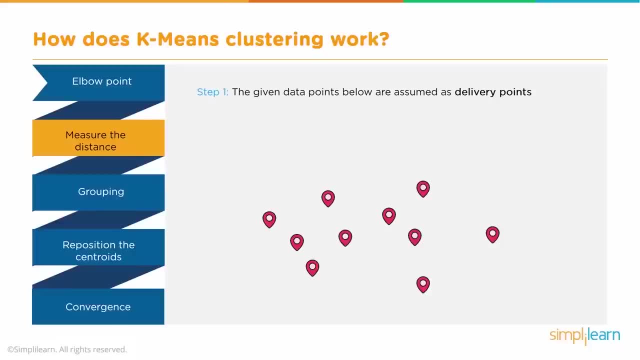 of k, and let's assume that these are our delivery points. the next step is basically to assign the value of k to the value of k. So let's assume that these are our delivery points. So let's assume that these are our delivery points. So let's assume that these are our delivery points. 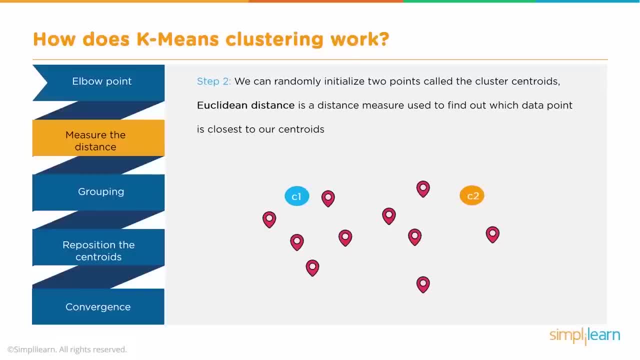 Two centroids randomly. So let's say c1 and c2 are the centroids assigned randomly. Now the distance of each location from the centroid is measured and each point is assigned to the centroid which is closest to it. So, for example, these points are very obvious that these are closest to c1, whereas 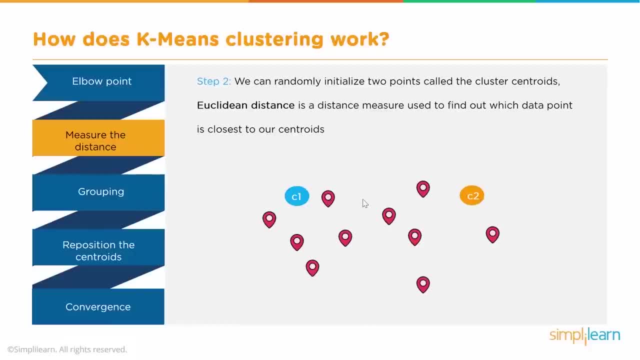 this point is far away from c2.. So these points will be assigned. which are close to c1 will be assigned to c1, and these points or locations which are close to c2 will be assigned to c2.. And then. so this is how the initial grouping is done. This is part of c1, and this is part of c2.. Then, 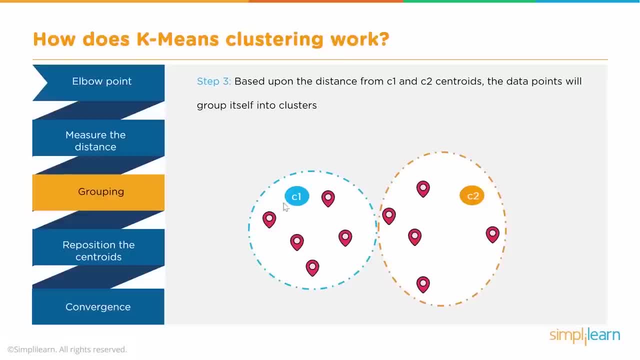 the next step is to calculate the actual centroid of this data because, remember, c1 and c2 are not the centroids, They have been randomly assigned points and only thing that has been done was the data points which are closest to them have been assigned to them. But now, in this step, the actual centroid will be calculated, which may: 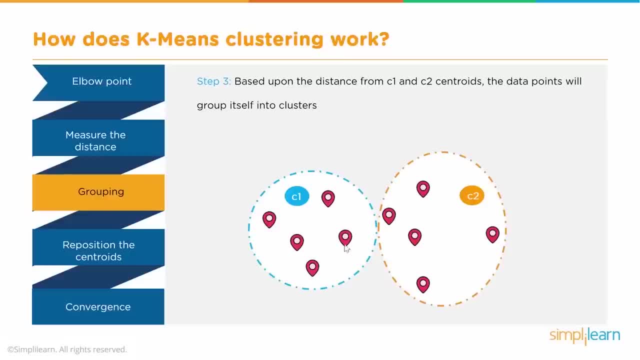 step is to calculate the actual centroid of this data because, remember, C1 and C2 are not the centroids. they've been randomly assigned points and only thing that has been done was the data points which are closest to them have been assigned to them. but now, in this step, the actual centroid will be calculated. 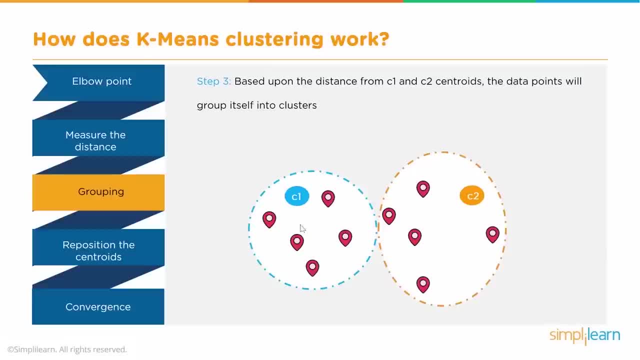 which may be for each of these data sets somewhere in the middle. so that's like the mean point. that will be calculated and the centroid will actually be positioned or repositioned there. same with C2. so the new centroid for this group is C2 in this new position and C1 is in this new position once again. the 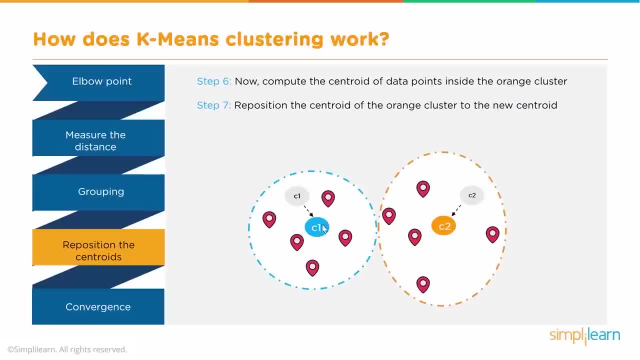 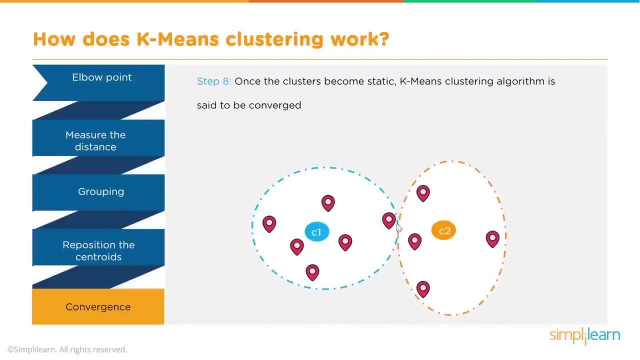 distance of each of the data points is calculated from these centroids. now, remember, it's not necessary that the distance still remains the or each of these data points still remain in the same group. by recalculating the distance, it may be possible that some points get reallocated like: so see this, so this. 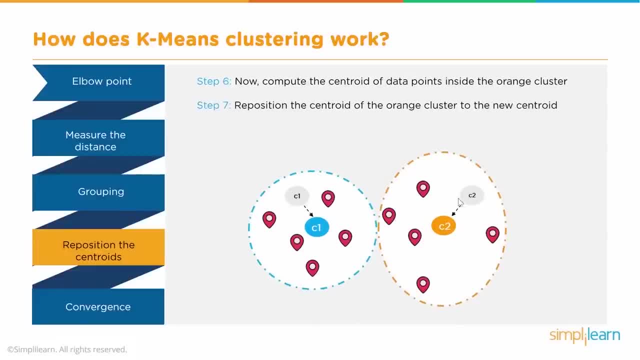 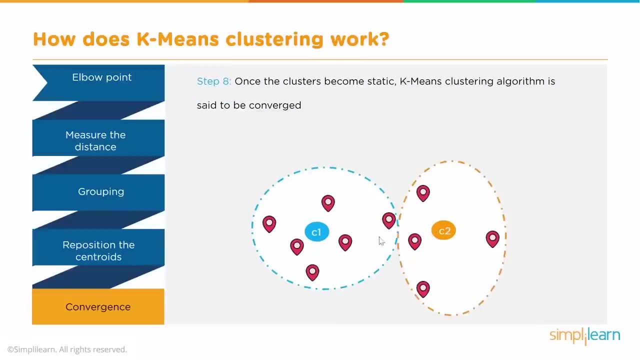 point earlier was closer to C2 because C2 was here. but after recalculating repositioning, it is observed that this is closer to C1 than C2. so this is the new group. so some points will be reassigned and again the centroid will be calculated. 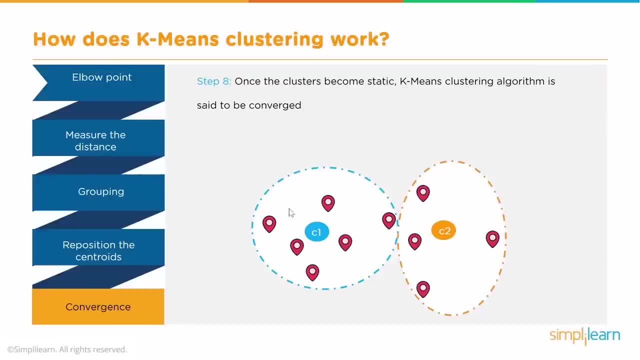 and if the centroid doesn't change, so that is a repetitive process, iterative process, and if the centroid doesn't change, once the centroid stops changing, that means the algorithm has converged and this is our final cluster, with this as the centroid, C1 and C2 as the centroids. these data points as a part of 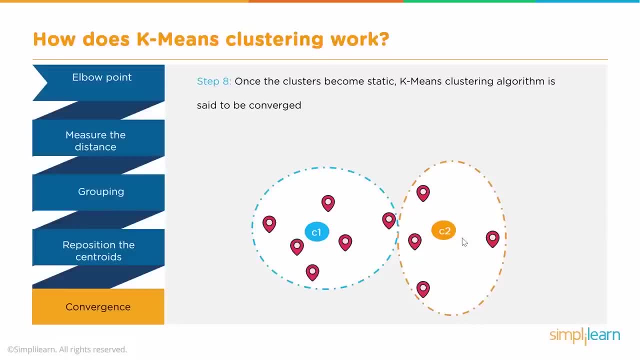 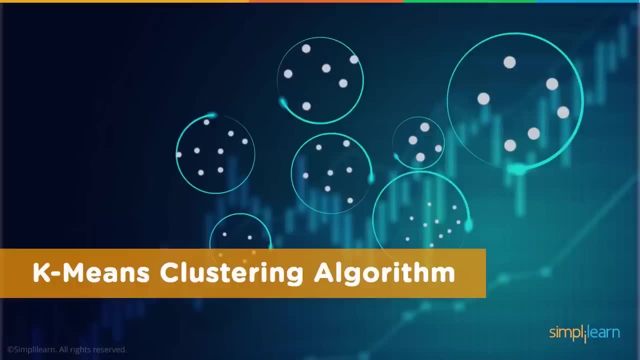 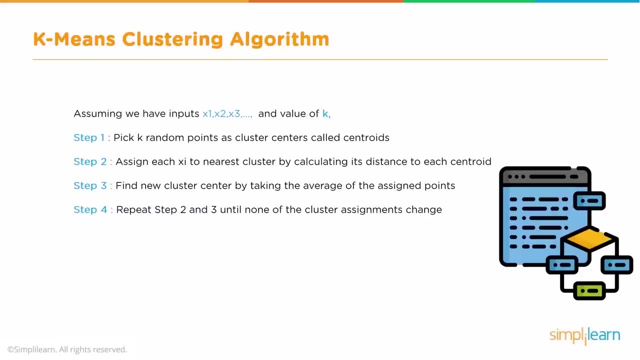 each cluster. so I hope this helps in understanding the whole process, iterative process of k-means clustering. so let's take a look at the k-means clustering algorithm. let's say we have x1, x2, x3, n number of points as our inputs and we want to split this into k clusters, or we want to 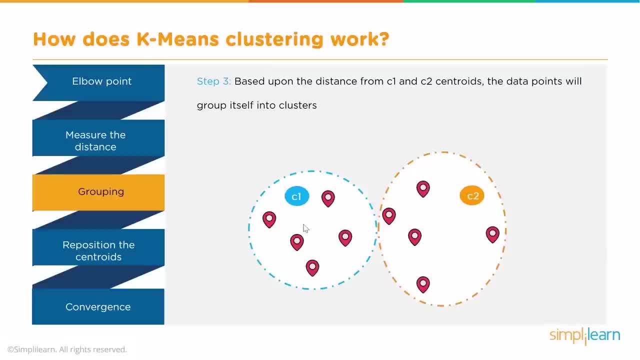 be for each of these data sets somewhere in the middle. So that's like the mean point that will be calculated And the centroid will actually be positioned or repositioned there. Same with c2.. So the new centroid for this group is c2 in this new position and c1 is in this new position Once. 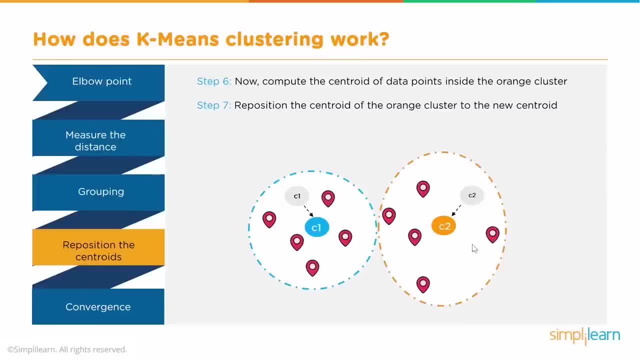 again, the distance of each of the data points is calculated from these centroids. Now remember, it's not necessary that the distance still remains the or each of these data points still remain in the same group. By recalculating the distance, it may be possible that some points. 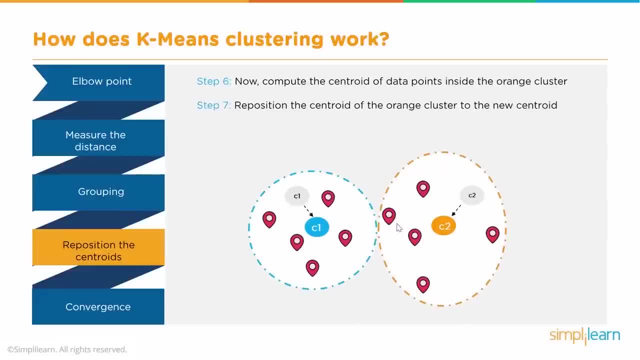 get reallocated like. so You see this. So this point earlier was closer to c2 because c2 was here. But after recalculating, repositioning, it is observed that this is closer to c1 than c2.. So this is the new. 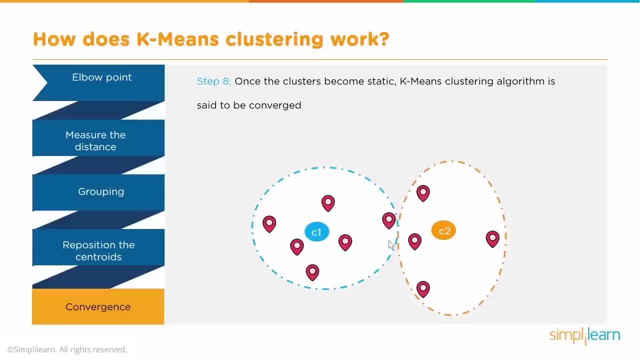 grouping. So some points will be reassigned And again the centroid will be calculated. And if the centroid doesn't change, so that is a repetitive process, iterative process- And if the centroid doesn't change, once the centroid stops changing, that means the algorithm has converged And this 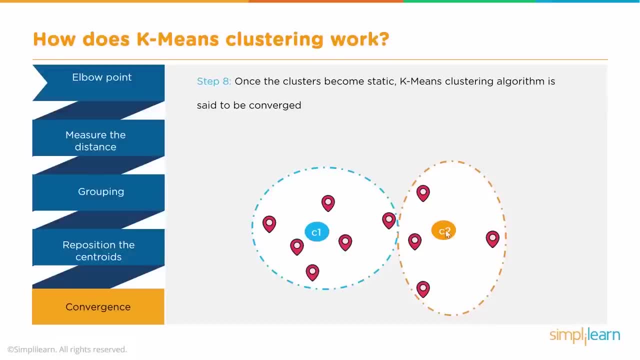 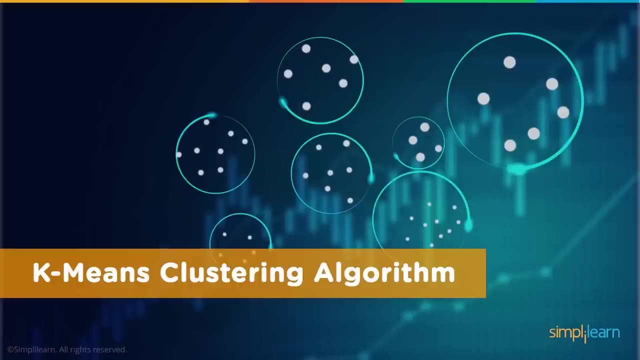 is our final cluster, With this as the centroid, c1 and c2 as the centroids, these data points as a part of each cluster. So I hope this helps in understanding the whole process. So let's take a look at the k-means clustering algorithm. Let's say we have x1, x2, x3, n number of 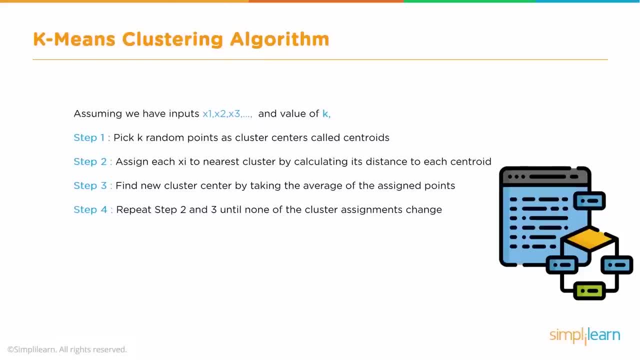 points as our inputs And we want to split this into k clusters or we want to create k clusters. So the first step is to randomly pick k points and call them centroids. They are not real centroids because centroid is supposed to be a centroid. 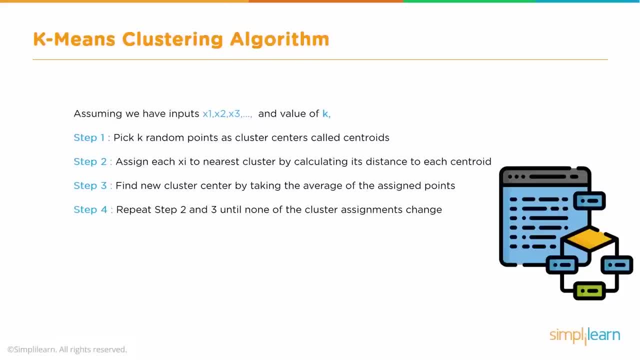 But they are just called centroids And we calculate the distance of each and every input point from each of the centroids. So the distance of x1 from c1, from c2, c3, each of the distances we calculate And then find out which distance is the lowest and assign x1 to that particular. 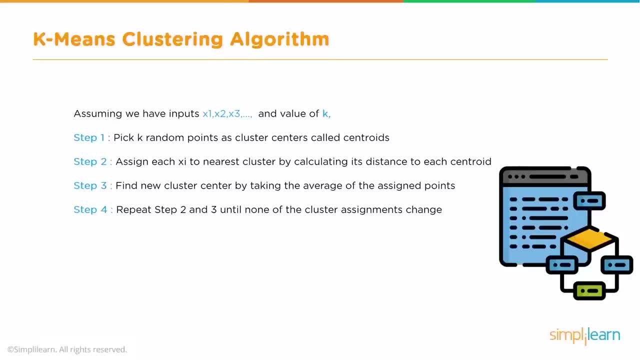 create k clusters. so the first step is to randomly pick k points and call them centroids. they are not real centroids, because centroid is supposed to be a center point, but they are just called centroids and we calculate the distance of each and every input point from each of the centroids, so the distance of x1 from C1, from C2, C3, each of. 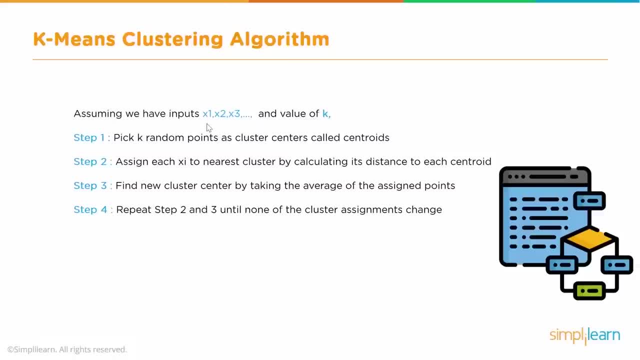 the distances we calculate and then find out which distance is the lowest and assign x1 to that particular random centroid. repeat that process for x2, its distance from each of the centroid- c1, c2, c3, up to ck- and find which is the lowest distance. and 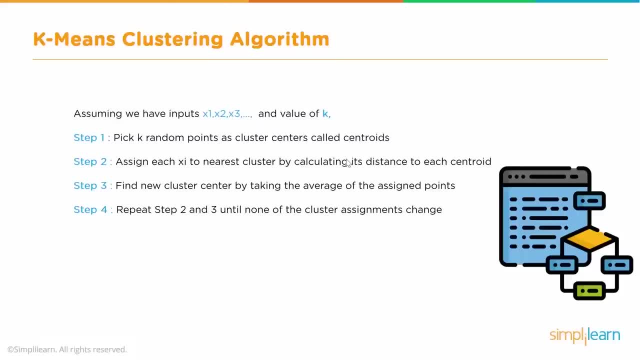 assign x2 to that particular centroid, same with x3, and so on. so that is the first round of assignment. that is done. now we have k groups, because there are. we have assigned the value of k, so there are k centroids, and so there are k groups. all these inputs have been split into k groups. 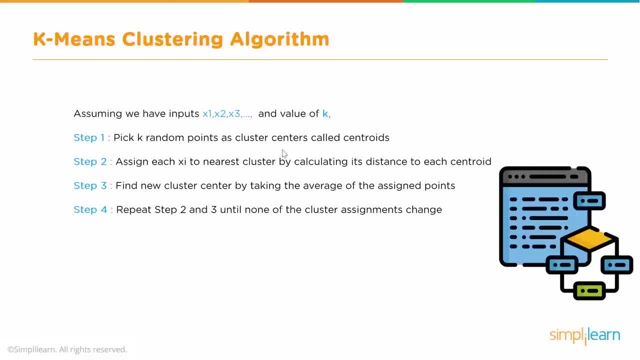 remember, remember. we pick the centroids randomly, so they are not real centroids. so now what we have to do? we have to calculate the actual centroids for each of these groups, which is like the mean position, which means that the position of the randomly selected centroids will now change, and 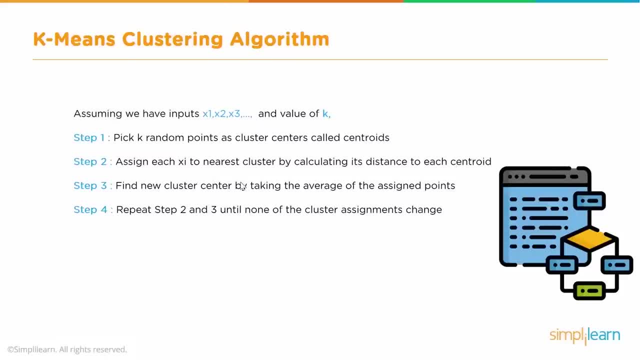 they will be the main positions of this newly formed k groups. and once that is done, we once again repeat this process, step 2 and 3. so we again calculate the distance of x1 from the centroid c1, c2, c3, and then see which. 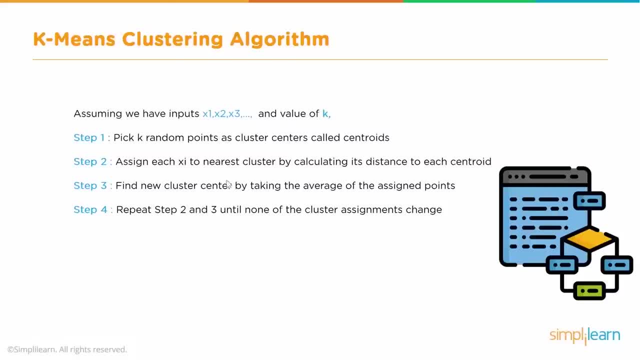 is the lowest value and assign x1 to that. calculate the distance of x2 from c1, c2, c3 or whatever up to ck and find whichever is the lowest distance and assign x2 again that centroid and so on. in this process there may be some reassignment. x1 pro was probably assigned. 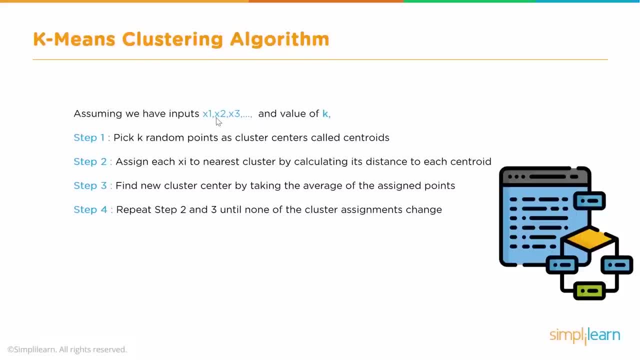 random centroid. Repeat that process for x2.. Calculate its distance from each of the centroids c1,, c2, c3, up to ck And find which is the lowest distance and assign x2 to that particular centroid, Same with x3 and so on, So that 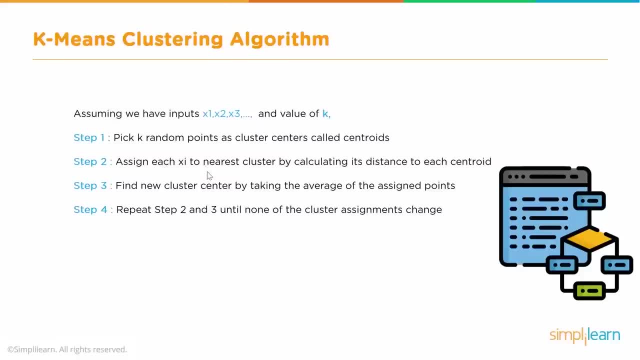 is the first round of assignment that is done. Now we have k groups, because there are. we have assigned the value of k, So there are k centroids And so there are k groups. All these inputs have been split into k groups. However, remember we picked the centroids randomly, So they are not real centroids. 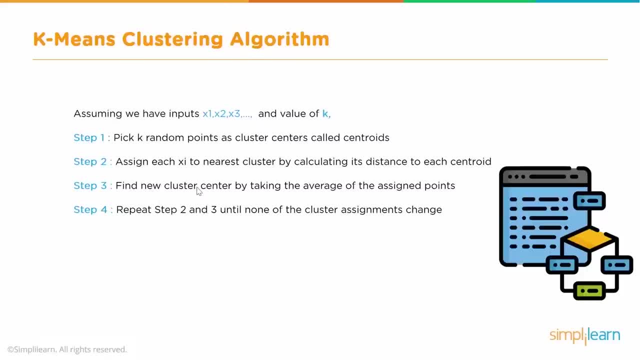 So now what we have to do? we have to calculate the actual centroids for each of these groups, which is like the mean position, which means that the position of the randomly selected centroids will now change And they will be the mean positions of this newly formed k. 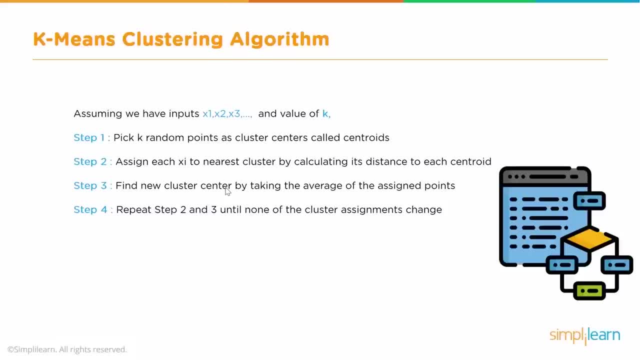 groups. And once that is done, we once again repeat the process of calculating the distance right? So this is what we are doing as a part of step 4.. We repeat step 2 and 3. So we again calculate the distance of x1 from the centroid. 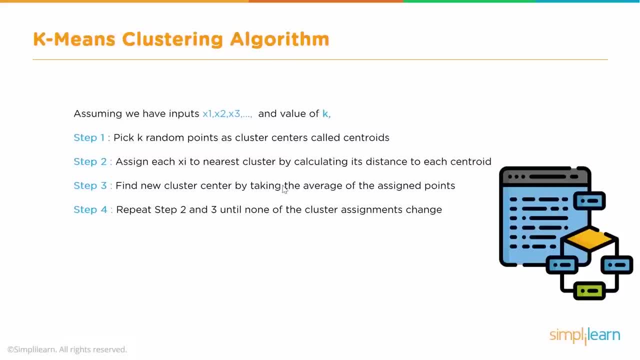 c1,, c2,, c3, and then c, which is the lowest value, and assign x1 to that. Calculate the distance of x2 from c1,, c2, c3 or whatever up to ck, and find whichever is the lowest. 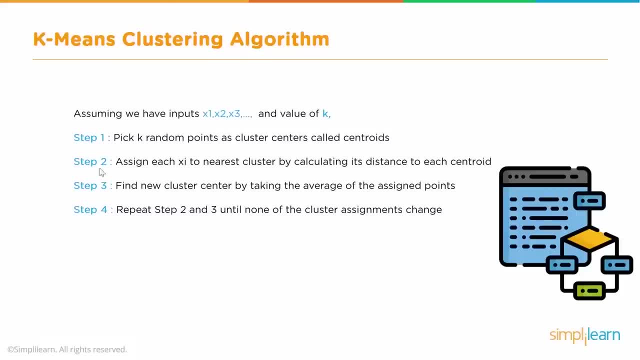 distance, And then x2 to that centroid and so on. In this process there may be some reassignment. x1 was probably assigned to cluster c2. And after doing this calculation maybe now x1 is assigned to c1. So that kind of reallocation may happen. So we repeat the steps 2 and 3. 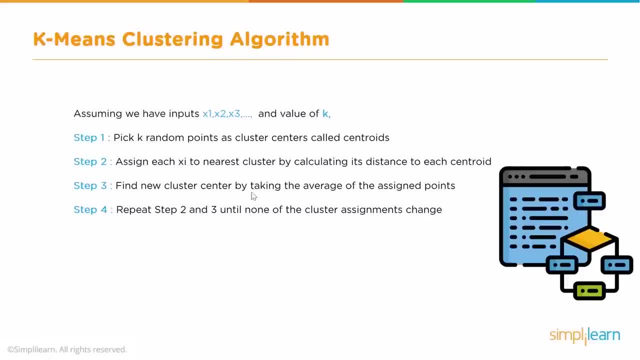 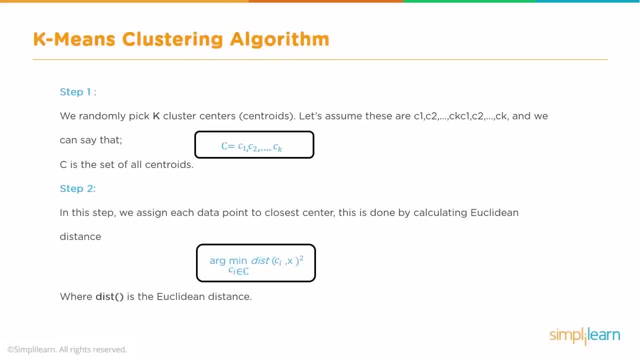 till, the position of the centroids don't change or stop changing, And that's when we have convergence. So let's take a detailed look at each of these steps. So we randomly pick k cluster centers. We call them centroids because they are not initially. 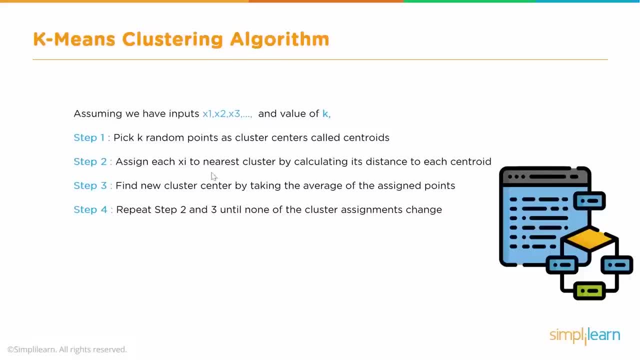 to cluster c2 and after doing this calculation, maybe now x1 is assigned to c1, so that kind of reallocation may happen. so we repeat the steps two and three till the position of the centroids don't change or stop changing, and that's when we have convergence. so let's take a detailed look at. 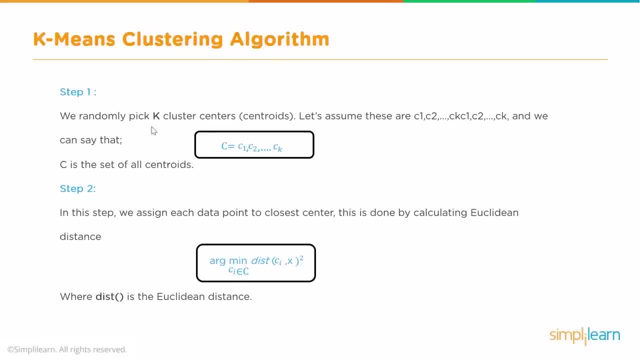 each of these steps. so we randomly pick k cluster centers. we call them centroids because they are not initially, they are not really the centroids, so we let us name them c1, c2, up to ck. and then, step two, we assign each data point to the closest center. so what we do? we calculate the distance of 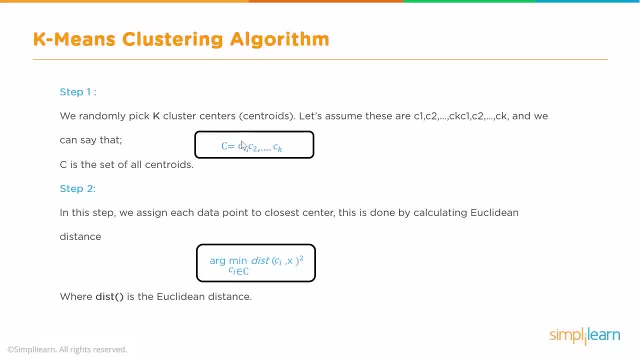 each x value from each c value. so the distance between x 1, c, 1, distance between x, x1, c2, x1, c3, and then we find which is the lowest value. right, that's the minimum value. we find and assign x1 to that particular centroid. then we go next to x2, find the distance of x2 from c1. 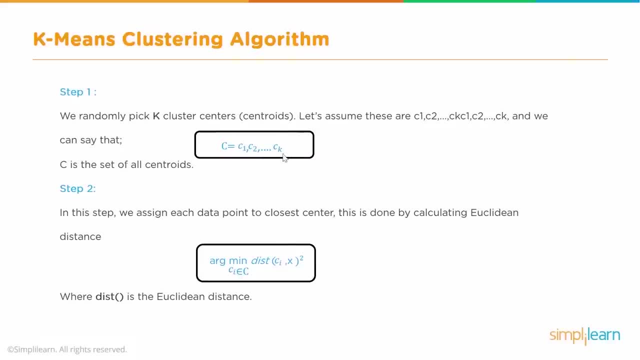 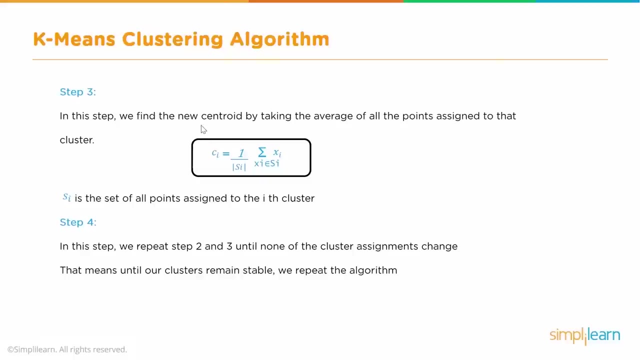 x2 from c2, x2 from c3 and so on up to ck and then assign it to the point or to the centroid which has the lowest value, and so on. so that is step number two. in step number three we now find the actual centroid for each group. so what has happened as a part of step number two? we now have all the 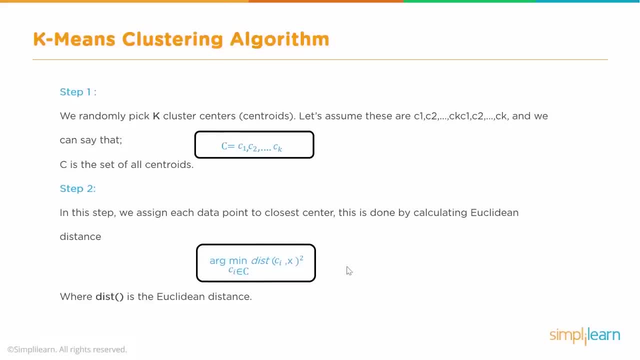 points, all the data points grouped into k groups because we we wanted to create k clusters, right? so we have k groups, each one may be having a certain number of input values. they need not be equally distributed by that. so we have k groups, each one may be having a certain number of input values. they need not be. 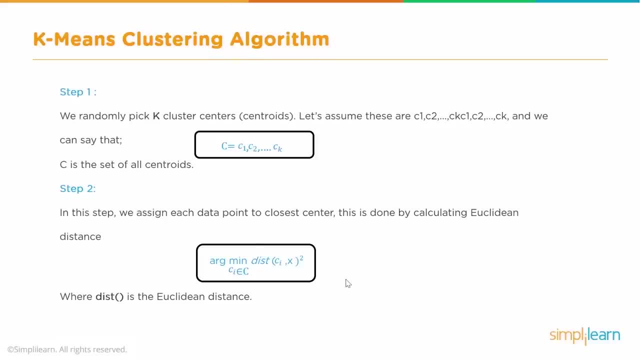 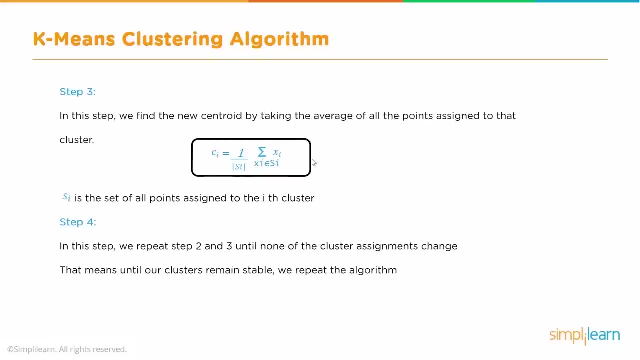 based on the distance, we will have k groups, but remember, the initial values of the c1, c2 were not really the centroids of these groups. right, we assign them randomly. so now, in step three, we actually calculate the centroid of each group, which means the original point which we thought. 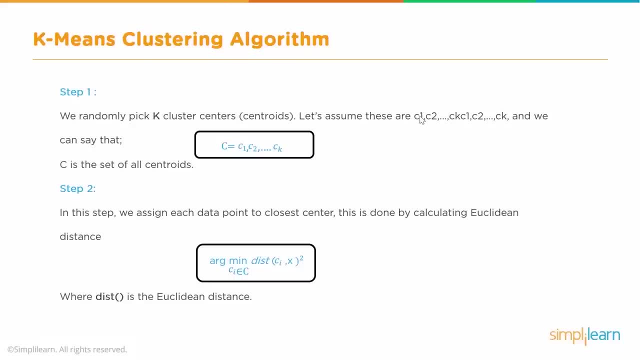 they are not really the centroids. So we let us name them c1, c2, up to ck. And then step 2, we assign each data point to the closest center. So what we do? we calculate the distance of each x value from each c value. So the distance between x1, c1, distance between 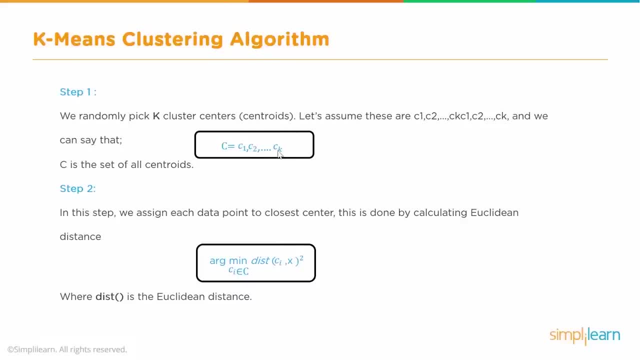 x1, c2, x1, c3. And then we find which is the lowest value, That's the minimum value. we find And assign x1 to that particular centroid. Then we go next to x2.. Find the distance of x2 from c1, x2 from c2, x2 from c3 and so on up to ck And then assign it. 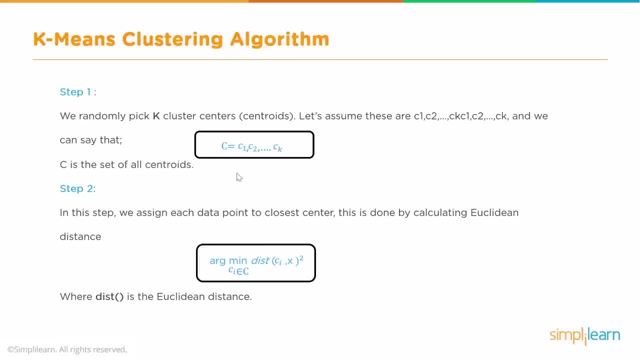 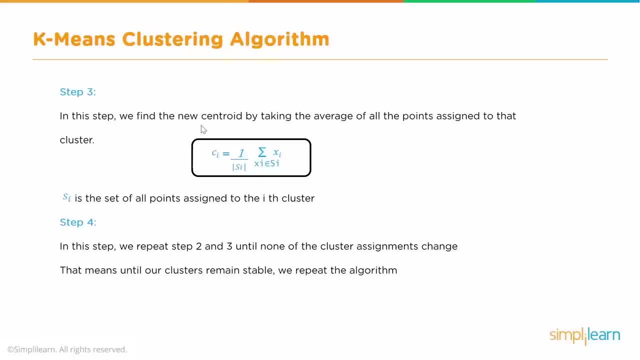 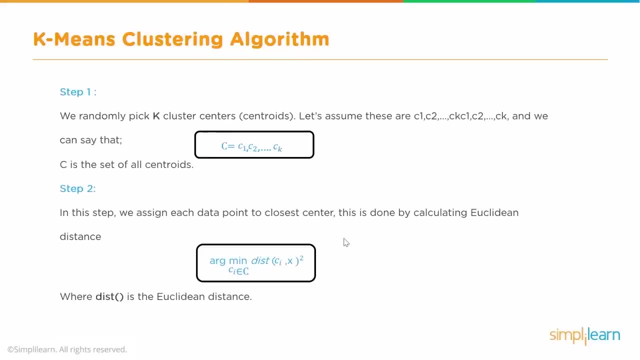 to the point or to the centroid which has the lowest value, and so on. So that is step number 2.. We now find the actual centroid for each group. So what has happened? As a part of step number 2, we now have all the points, all the data points, grouped into k groups, because we wanted 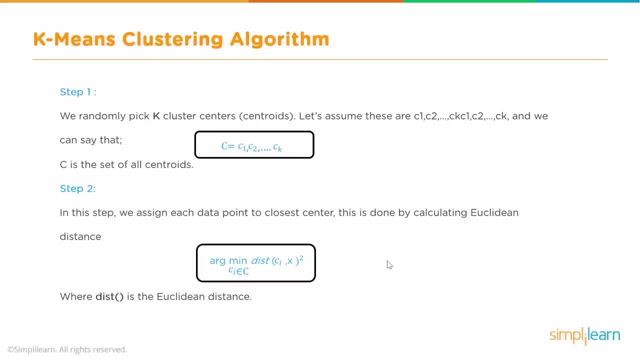 to create k clusters, right. So we have k groups. Each one may be having a certain number of input values. They need not be equally distributed. by the way, Based on the distance we will have k groups, But remember, the initial values of the c1, c2 were not really the centroids of these groups, right? 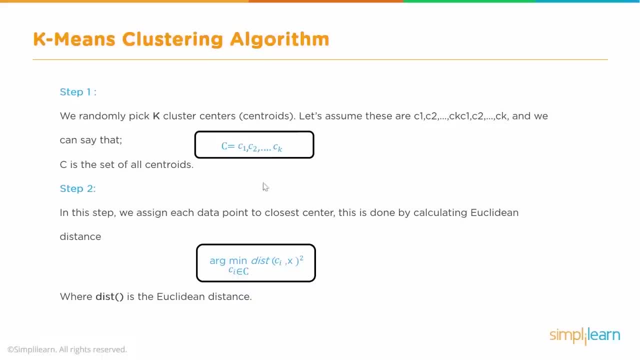 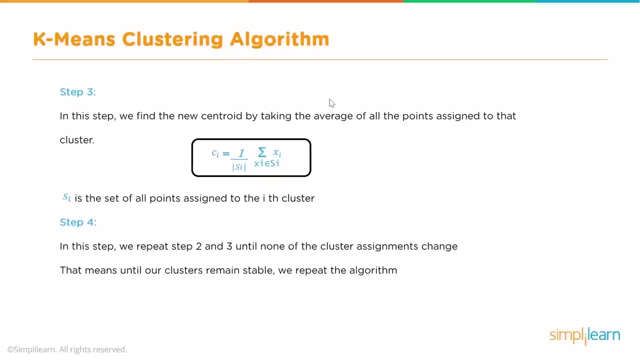 We assigned them randomly. So now, in step 3, we actually calculate the centroid of each group, which means the original point, which we thought was the centroid, will shift to the new position, which is the actual centroid for each of these groups. Okay, And we again. 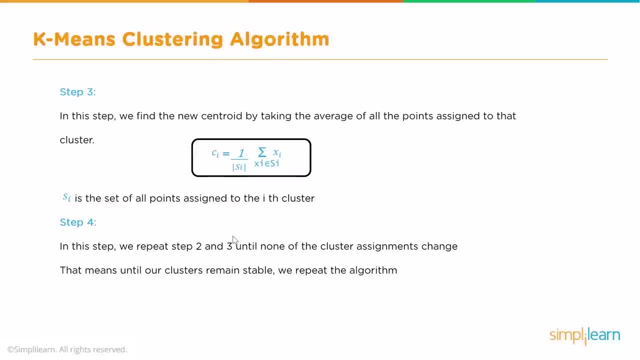 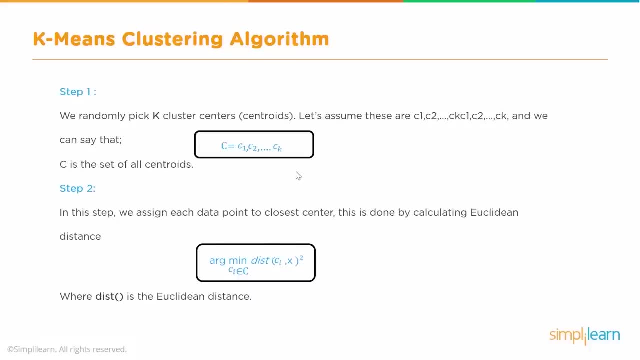 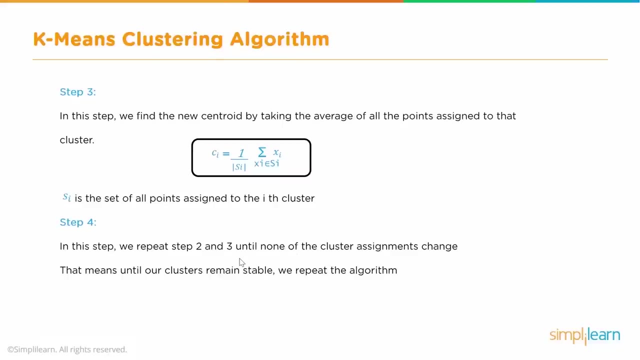 calculate the distance. So we go back to step 2.. Step 2. Which is what? We calculate again, the distance of each of these points from the newly positioned centroids And, if required, we reassign these points to the new centroids. So, as I said earlier, 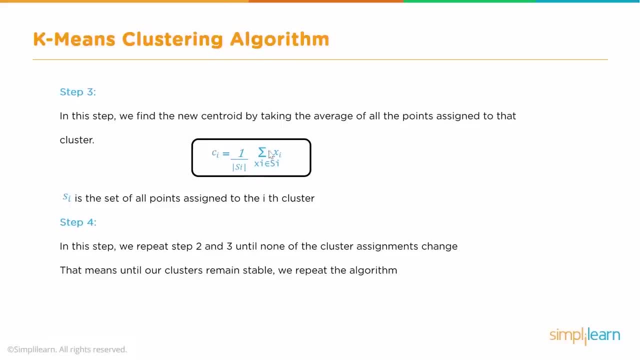 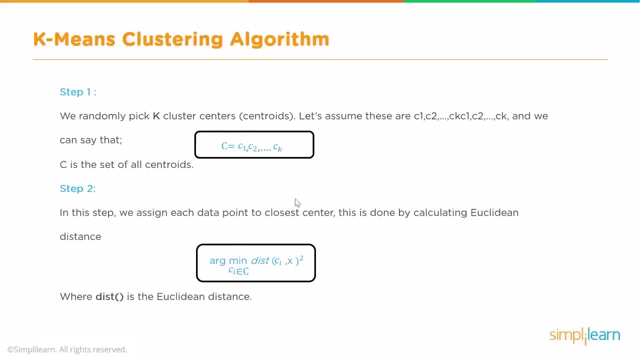 was the centroid will shift to the new position, which is the actual centroid for each of these groups. okay, and we again calculate the distance. so we go back to step two, which is what we calculate again, the distance of each of these points from the newly positioned centroids and, if required, we reassign. 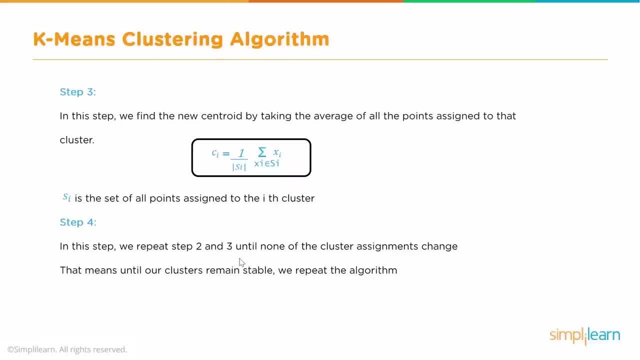 these points to the new centroids. so, as i said earlier, there may be a reallocation. so we now have a new set or a new group. we still have k groups, but the number of i terms and the actual assignment may be different from what was in step two here. okay, so that might. 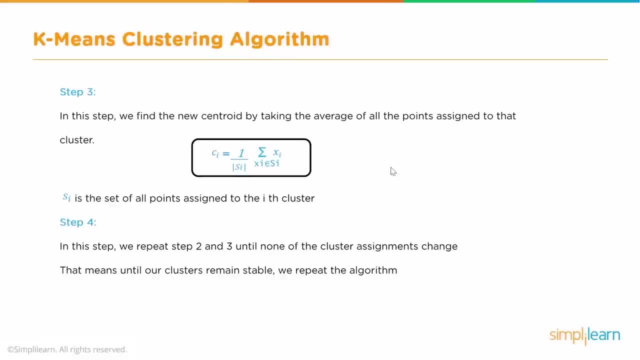 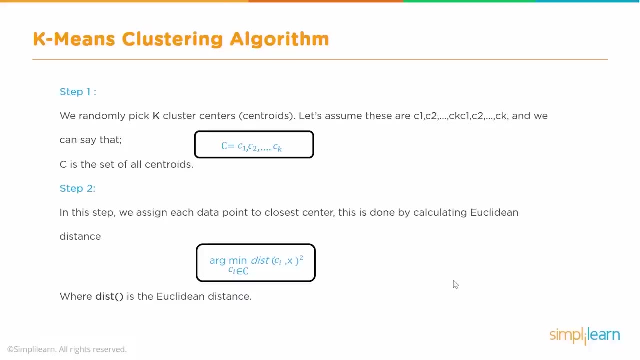 change. then we perform step three once again to find the new centroid of this new group. so we have again a new set of clusters, new centroids and new assignments. we repeat this step two again. once again we find, and then it is possible that after iterating through three, 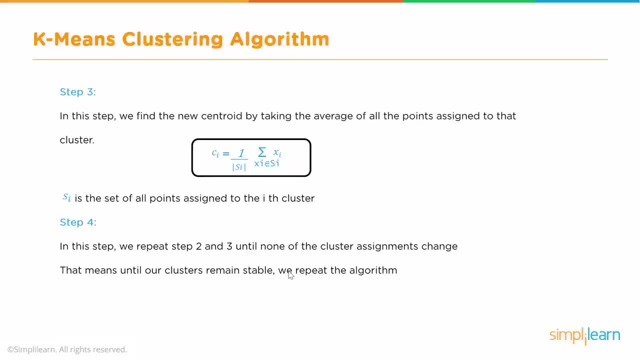 or four or five times, the centroid will stop moving, in the sense that when you calculate the new value of the centroid, that will be same as the original value or there will be very marginal change. so that is when we say convergence has occurred and that is our final cluster, that's. 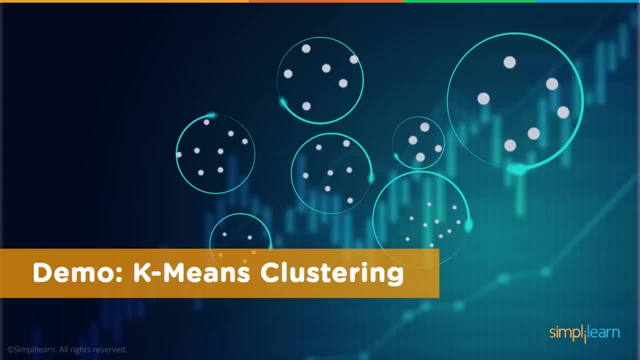 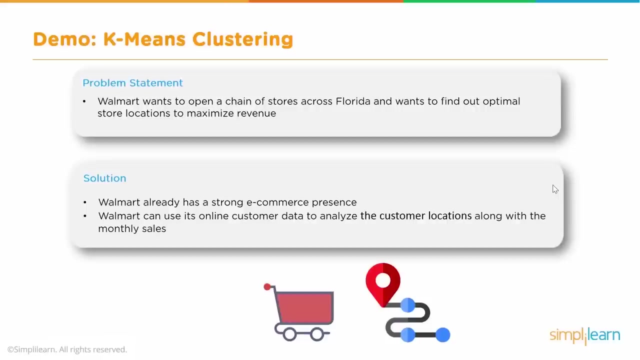 the formation of the final cluster. all right, so let's see a couple of demos of k-means clustering. we actually see some live demos in python notebook, using python notebook. but before that, let's find out what's the problem that we are trying to solve. the problem statement is: let's say, Walmart wants 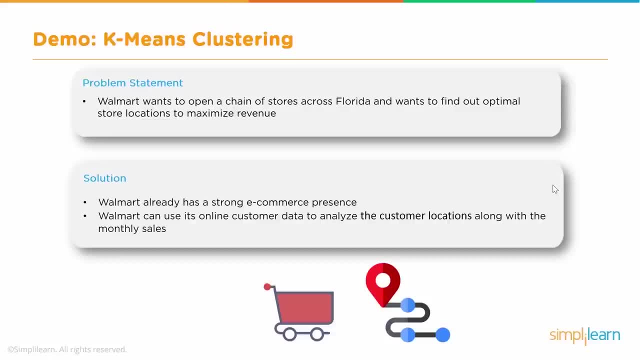 to open a chain of stores across the state of Florida and it wants to find the optimal store locations. now the issue here is: if they open too many stores close to each other, obviously the they will not make profit. but if they, if the stores are too far apart, then they will not have enough sales. so how do they optimize this? 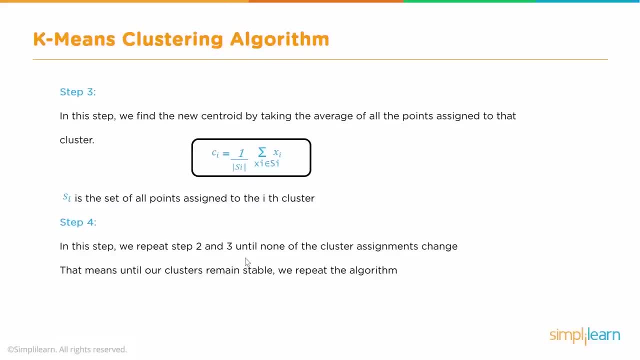 there may be a reallocation. So we now have a new set or a new group. We still have k groups, but the number of items and the actual assignment may be different from what was in step two here. Okay, so that might change. Then we perform step three once again to find: 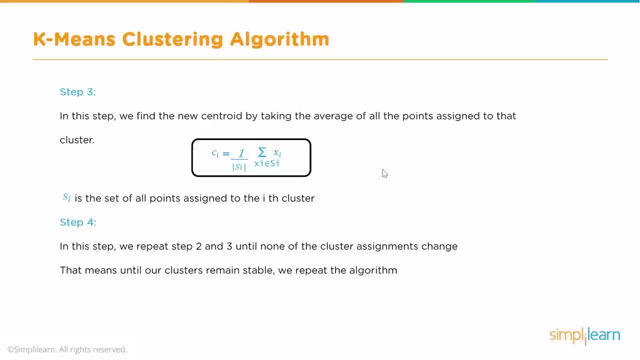 the new centroid of this new group. So we have again a new set of clusters, new centroids and new assignments. We repeat this step two again. Once again we find, and then it is possible- that after iterating through three or four or five times, the centroid will stop moving in the sense. 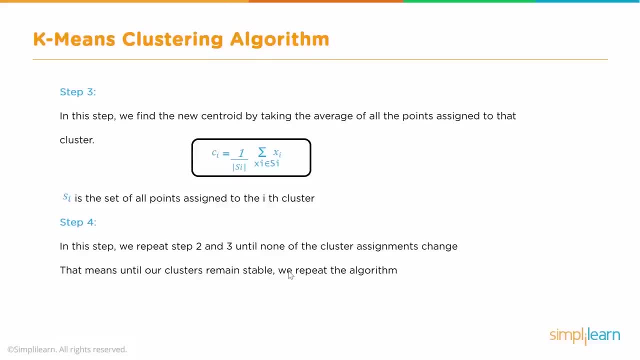 that when you calculate the new value of the centroid, that will be same as the original value or there will be very marginal change. So that is when we say convergence has occurred and that is our final cluster, That's the formation of the final cluster. All right, so let's see a couple. 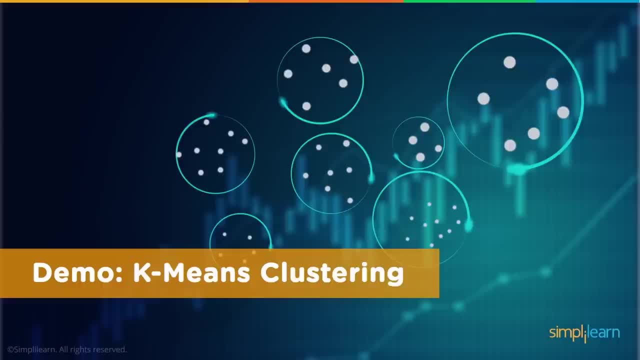 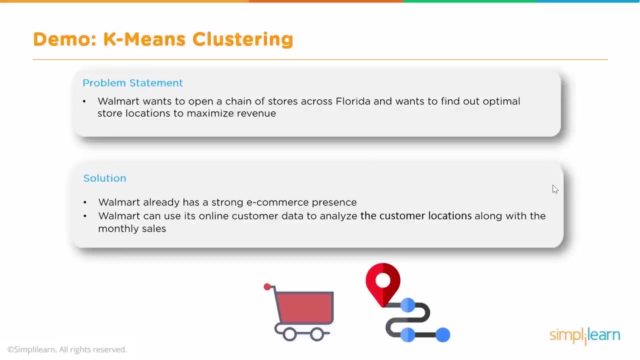 of demos of a K-Means clustering. We will actually see some live demos in Python Notebook using Python Notebook. But before that let's find out what's the problem that we are trying to solve. The problem statement is: let's say, Walmart wants to open a chain of stores across the state of 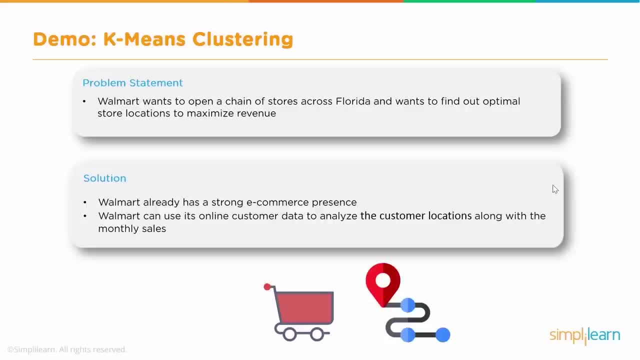 Florida and it wants to find the optimal store locations. Now the issue here is: if they open too many stores close to each other, obviously they will not make profit, But if the stores are too far apart, then they will not have enough sales. So how do 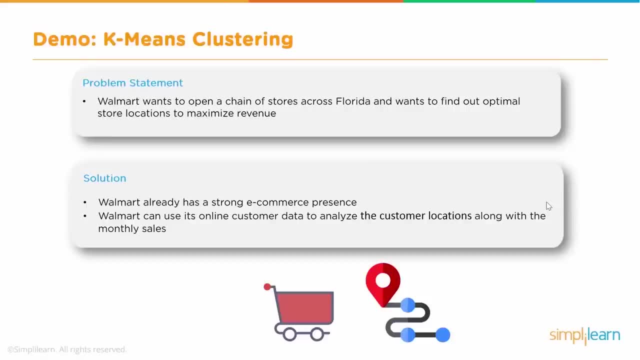 they optimize this Now for an organization like Walmart, which is an e-commerce giant. they already have the addresses of their customers in their database, So they can actually use this information or this data and use K-Means clustering to find the optimal location Now, before we. 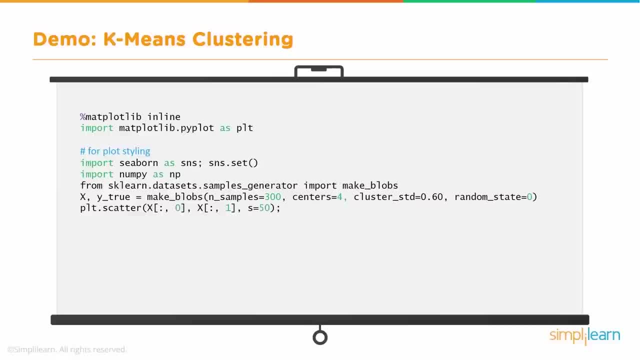 go into the Python Notebook and show you the live code. I wanted to take you through very quickly a summary of the code in the slides and then we will go into the Python Notebook. So in this block we are basically importing all the required libraries like NumPy, Matplotlib and so on. 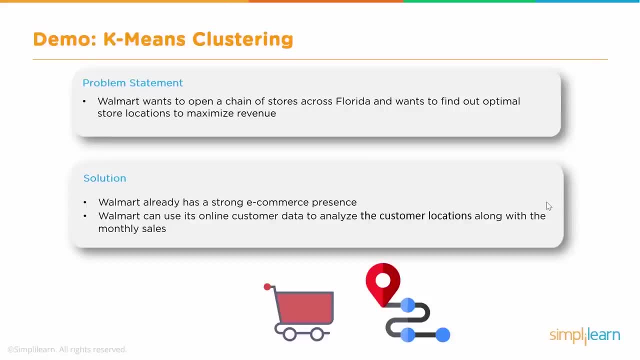 now for an organization like Walmart, which is an e-commerce giant. they already have the addresses of their customers in their database, so they can actually use this information or this data and use k-means clustering to find the optimal location. now, before we go into the python notebook, 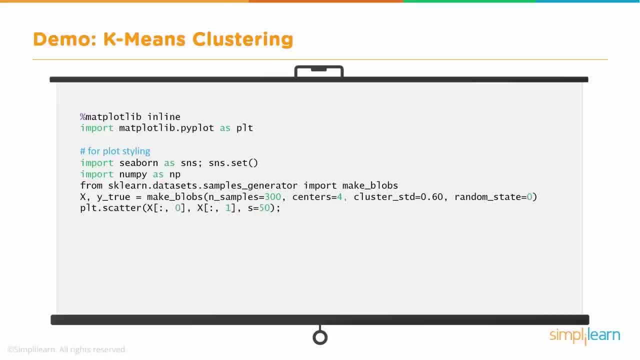 and show you the live code. I wanted to take you through very quickly a summary of the code in the slides and then we will go into the python notebook. so in this block we are basically importing all the required libraries like numpy, matplotlib and so on, and we are loading the data. 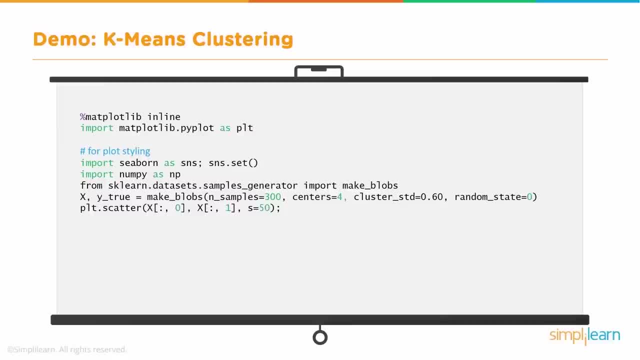 that is available in the form of, let's say, the addresses. for simplicity's sake we will just take as some data points. then the next thing we do is quickly do a scatter plot to see how they are related to each other with respect to each other. so in the scatter plot we see that there are a few. 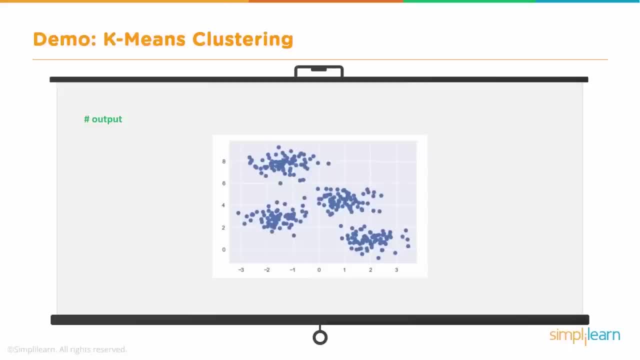 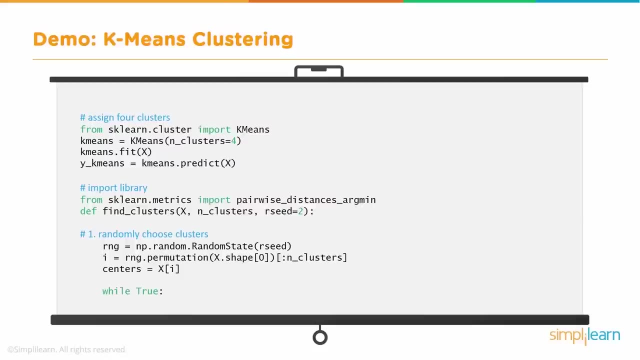 distinct groups already being formed, so you can actually get an idea about how the cluster would look and how many clusters, what is the optimal number of clusters? and then starts the actual k-means clustering process. so we will assign each of these points to the centroids and then check whether they are the optimal distance. 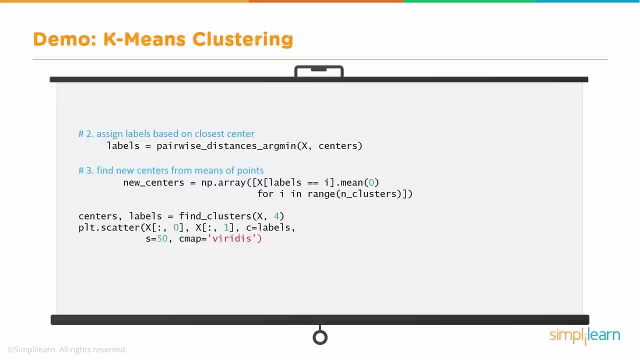 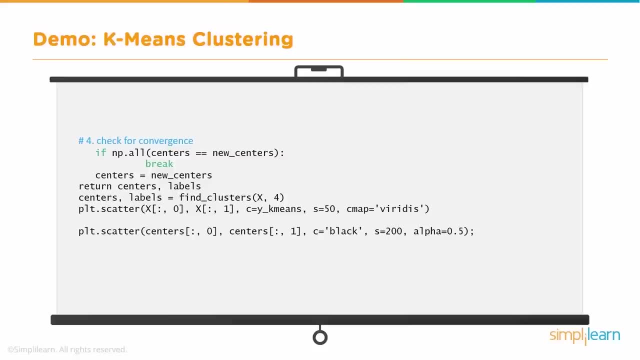 which is the shortest distance, and assign each of the points- data points, to the centroids and then go through this iterative process till the whole process converges and finally we get an output like this: so we have four distinct clusters, and which is, if we can say that this is how the 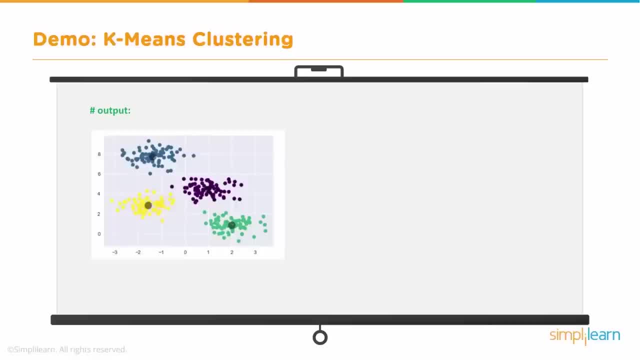 population is probably distributed across Florida state and the centroids are like the location where the store should be, the optimum location where the store should be. so that's the way we determine the best locations for the store and that's how we can help Walmart find the best locations for the stores in. 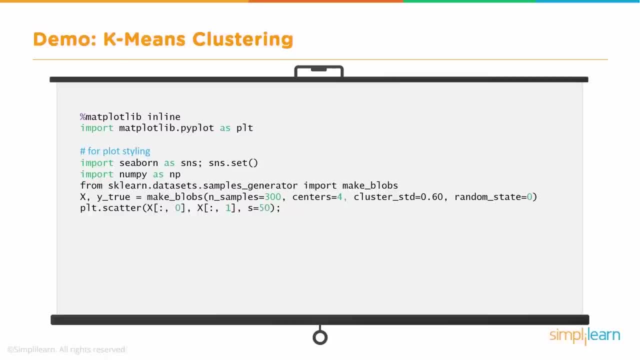 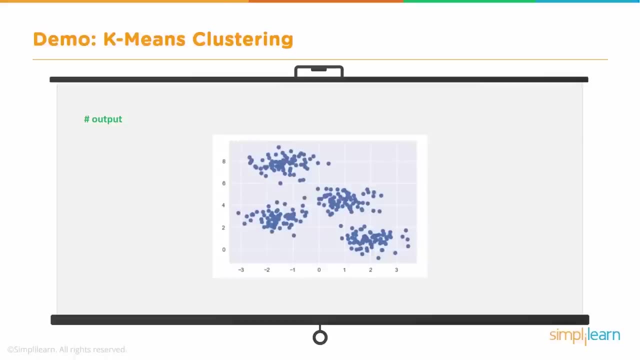 And we are loading the data that is available in the form of, let's say, the addresses. for simplicity's sake, we will just take them as some data points. Then the next thing we do is quickly do a scatter plot to see how they are related to each other with respect to each other. 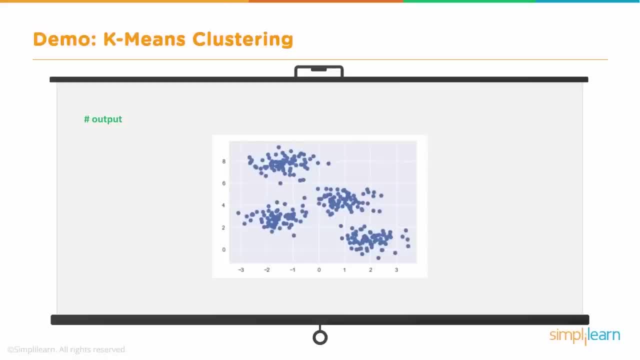 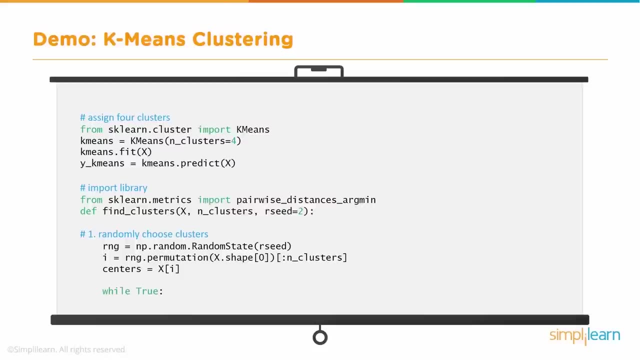 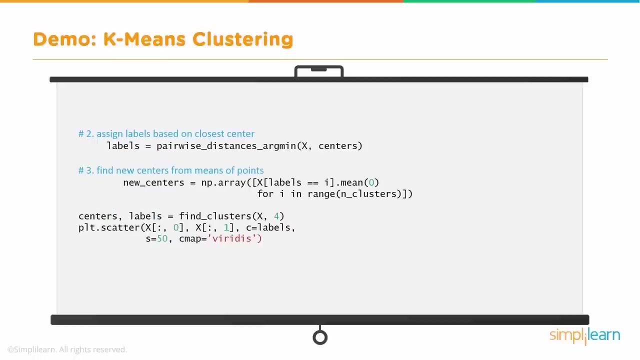 So in the scatter plot we see that there are a few distinct groups already being formed, So you can actually get an idea about how the cluster would look and how many clusters, what is the optimal number of clusters? And then starts the actual clustering process. So we will assign each of these points to the centroids and then check. 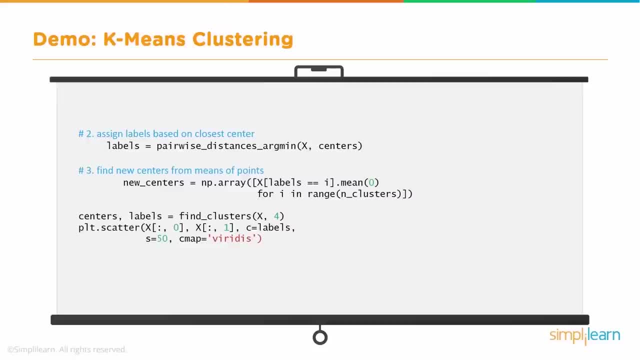 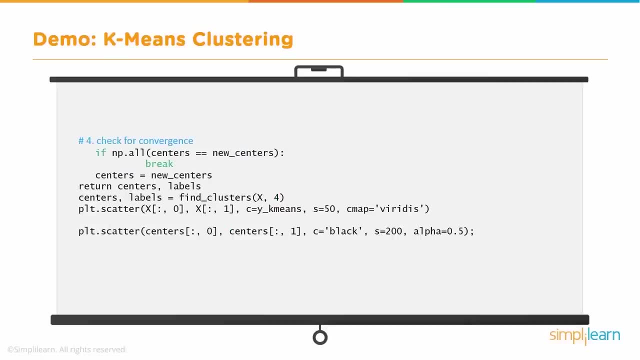 whether they are the optimal distance, which is the shortest distance, and assign each of the points- data points- to the centroids and then go through this iterative process till the whole process converges And finally we get an output like this: So we have four distinct clusters and 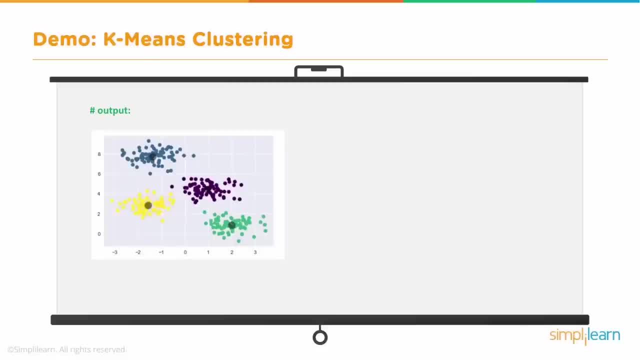 which is, if we can say that this is how the population is probably distributed across Florida State, And these centroids are like the location where the store should be, the optimum location where the store should be. So that's the way we determine the best locations for the store And that's how we 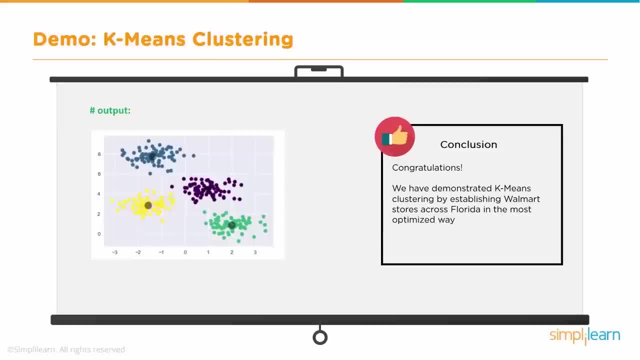 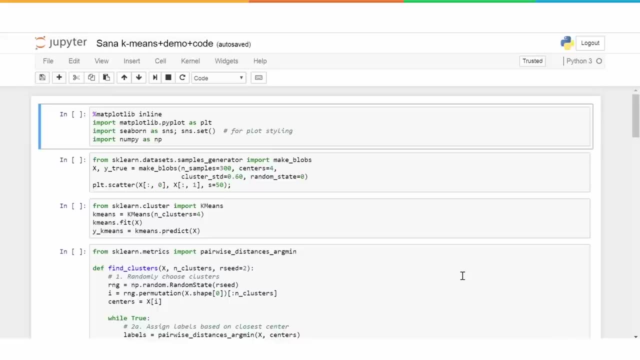 can help Walmart find the best locations for their stores in Florida. So now let's take this into the Python notebook. Let's see how this looks when we are learning running the code live. All right, So this is the code for K-means clustering in Jupiter notebook. We have a 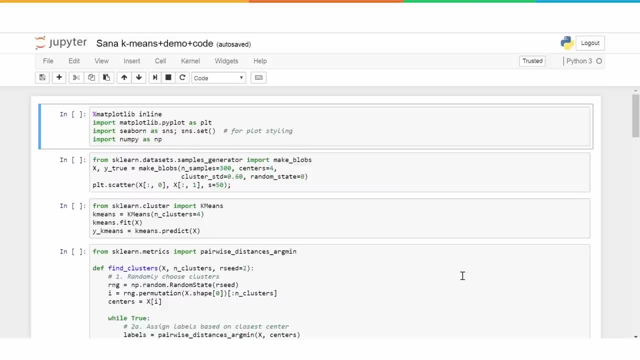 few examples here, which we will demonstrate how K-means clustering is used, And even there is a small implementation of K-means clustering as well. Okay, So, let's get started. Okay, So this block is basically importing the various libraries that are required, like matplotlib. 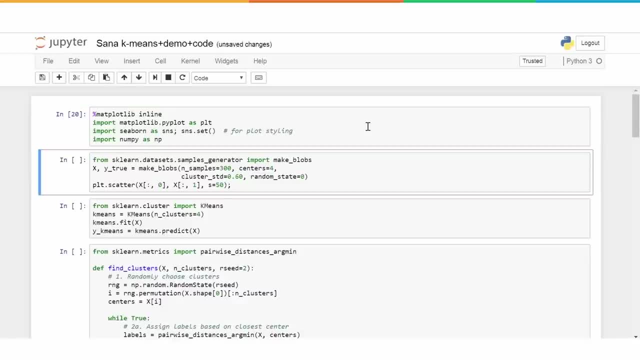 numpy and so on and so forth, which would be used as a part of the code. Then we are going and creating blobs which are similar to clusters. Now this is a very neat feature which is available in scikit-learn. Make blobs is a nice feature. 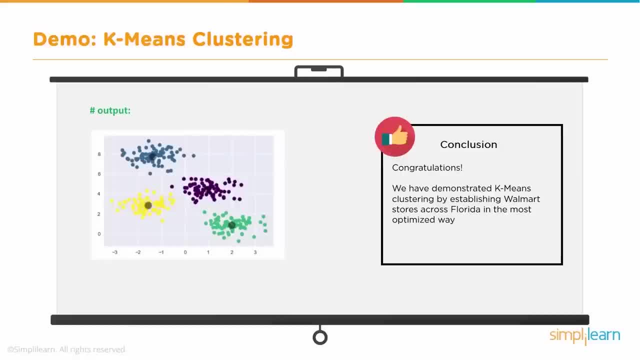 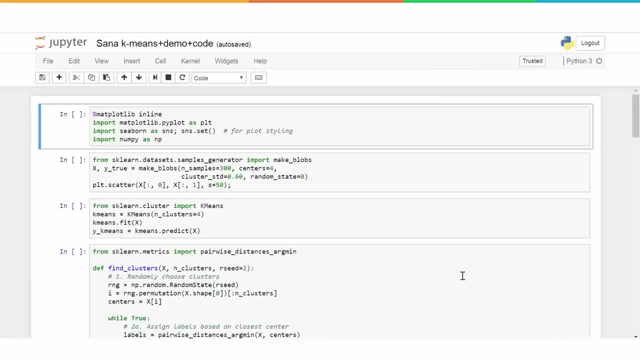 Florida. so now let's take this into python notebook. let's see how this looks when we are learning code live. all right, so this is the code for k-means clustering in jupyter notebook. we have a few examples here which we will demonstrate how k-means clustering is used, and even there is a 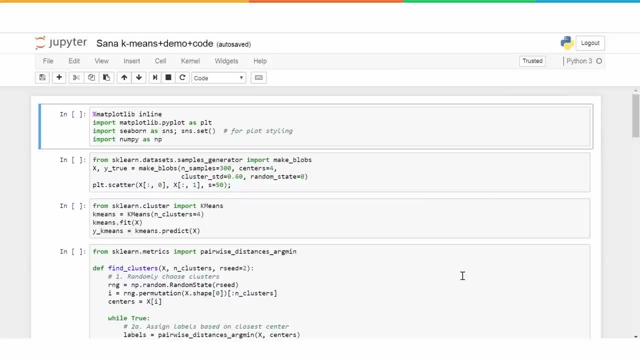 small implementation of k-means clustering as well. okay, so let's get started. okay, so this block is basically importing the various libraries that are required, like matplotlib and numpy and so on and so forth, which would be used as a part of the code. then we are going and creating blobs, which 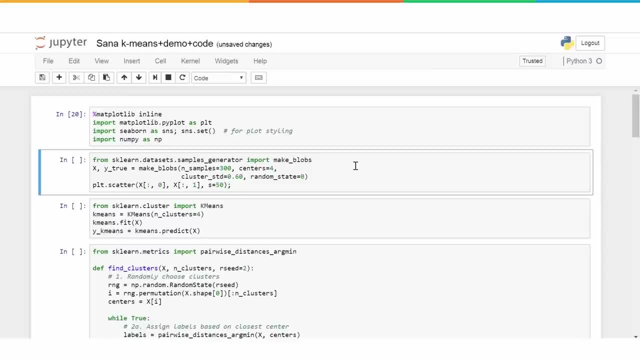 are similar to clusters. now this is a very neat feature which is available in scikit-learn. make blobs is a nice feature which creates clusters of data sets, so that's a wonderful functionality that is readily available for us to create some test data kind of thing. okay, so that's exactly. 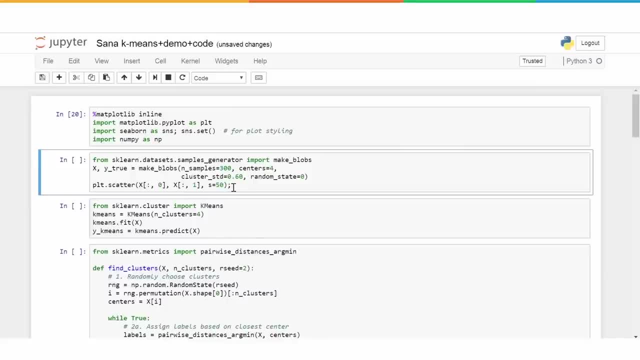 what we are doing here: we are using, make blobs and we can specify how many clusters we want. so centers we are mentioning here, so it will go ahead, and so we just mentioned four, so it will go ahead and create some test data for us, and this is. 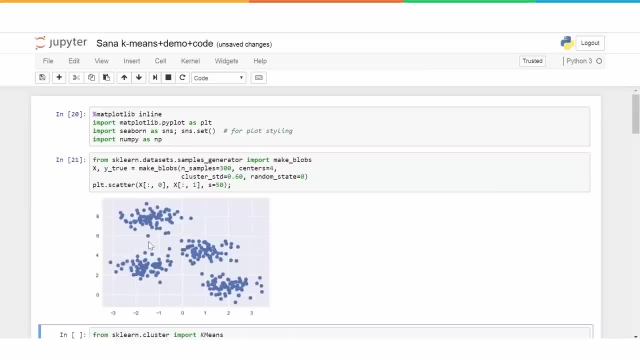 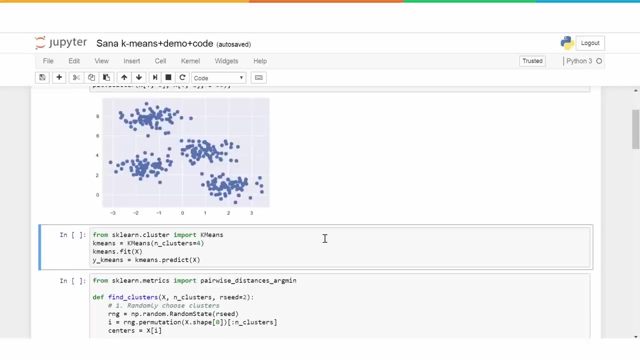 how it looks. as you can see visually also, we can figure out that there are four distinct classes or clusters in this data set, and that is what make blobs actually provides. now, from here onwards, we will basically run the standard k-means functionality that is readily available, so we really don't have to. 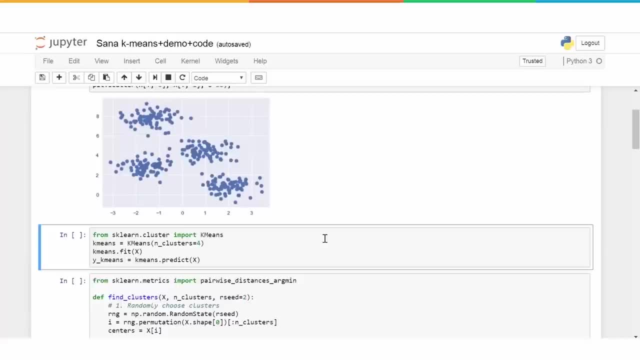 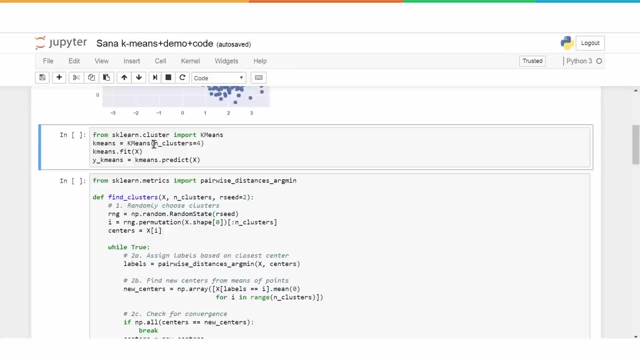 implement k-means itself. the k-means functionality or the function is readily available. you just need to feed the data and we'll create the clusters. so this is the code for that. we import k-means and then we create an instance of k-means and we specify the value of k. this n underscore clusters. 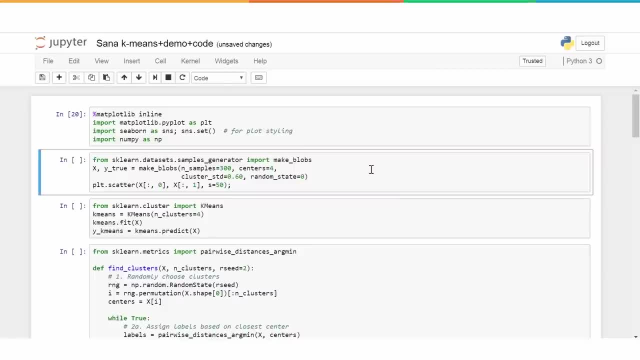 which creates clusters of data sets. So that's a wonderful functionality that is readily available for us to create some test data kind of thing. Okay, So that's exactly what we are doing here. We are using make blobs and we can specify how many clusters we want. So centers we are mentioning. 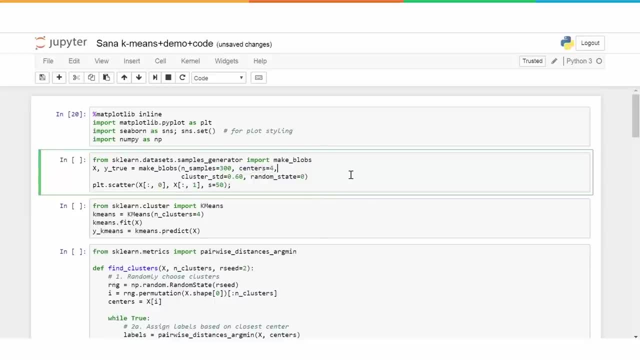 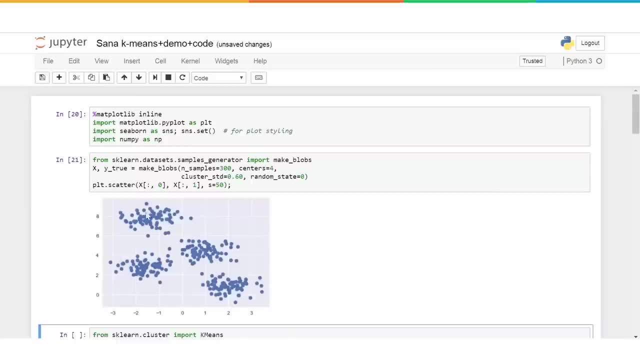 here. So it will go ahead. and so we just mentioned four. So it will go ahead and create some test data for us And this is how it looks, as you can see Visually also, we can figure out that there are four distinct classes or clusters in this data set, And that is what make blobs actually provides. 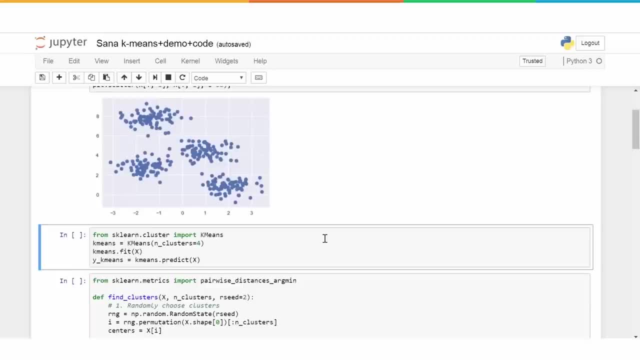 Now, from here onwards, we will basically run the standard kmeans functionality. that is readily available, So we really don't have to implement kmeans itself. The kmeans functionality or the function is readily available. You just need to feed the data and we'll create the clusters. So 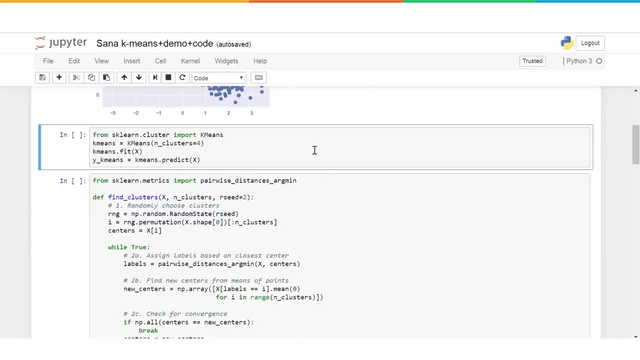 this is the code for that. We import kmeans and then we create an instance of kmeans and we specify for clusters is the value of k. Remember: k means in, k means k is basically the number of clusters that you want to create and it is a integer value. So this is where we are. 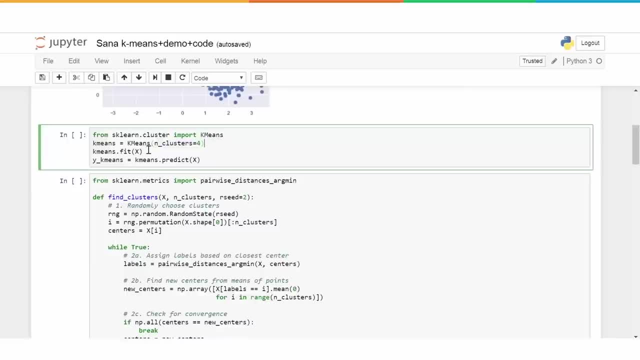 specifying that. So we have, k is equal to 4 and so that instance is created. We take that instance and, as with any other machine learning functionality, fit is what we use, the function or the method. rather, fit is what we use to train the model. Here there is no. 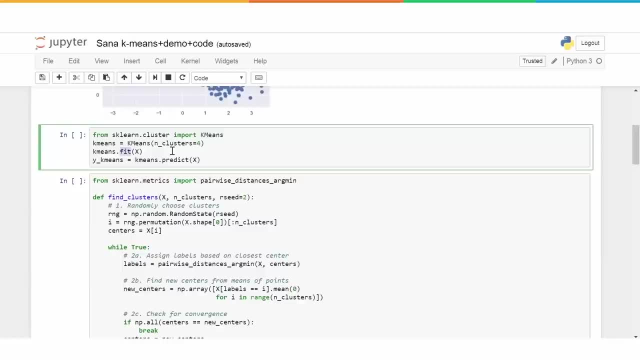 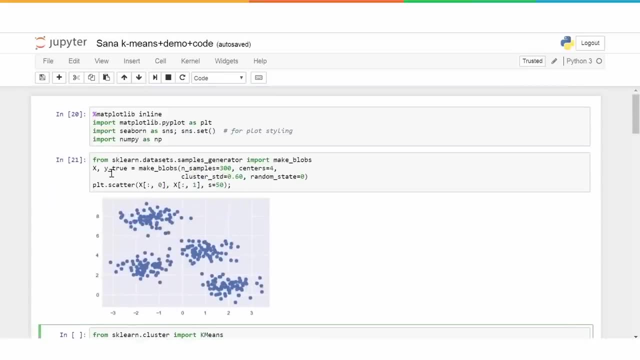 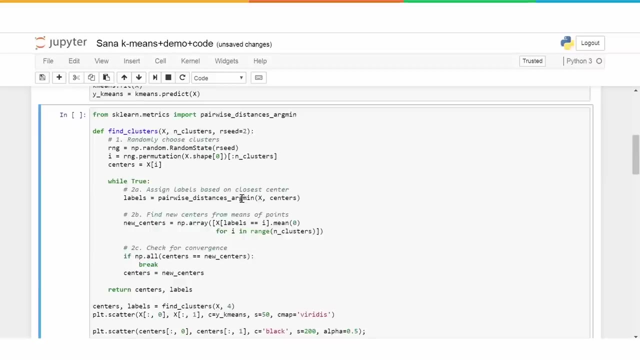 real training kind of thing. but that is the call. So we are calling fit and we are just passing the data. So X has the values, the data that has been created, right? So that is what we are passing here And this will go ahead and create the clusters and then 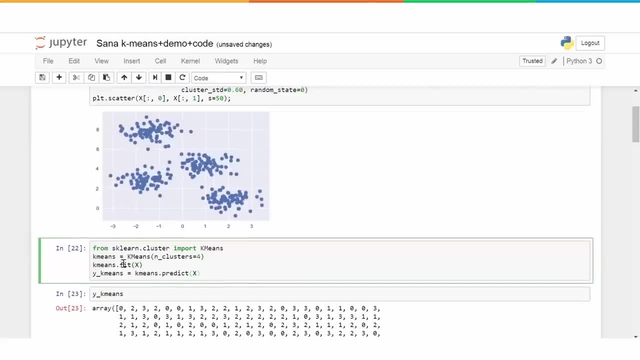 we are using. After doing fit, we run the predict, which basically assigns each of these observations which cluster it belongs to. all right, so it will name the clusters. maybe this is cluster one, this is two, three and so on, or i will actually start from zero cluster. 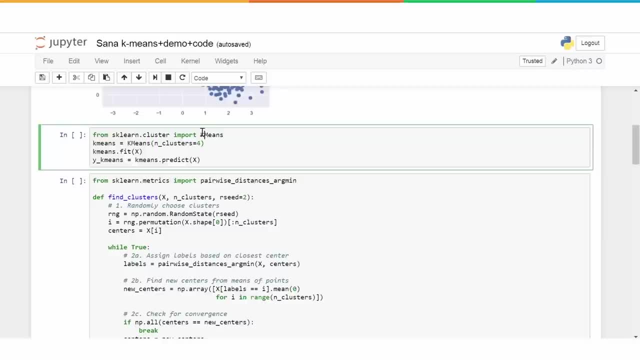 is the value of k. remember the value of k is the value of k and we specify the value of k and we remember k means in, k means k is basically the number of clusters that you want to create and it is a integer value. so this is where we are specifying that. so we have: k is equal to 4. 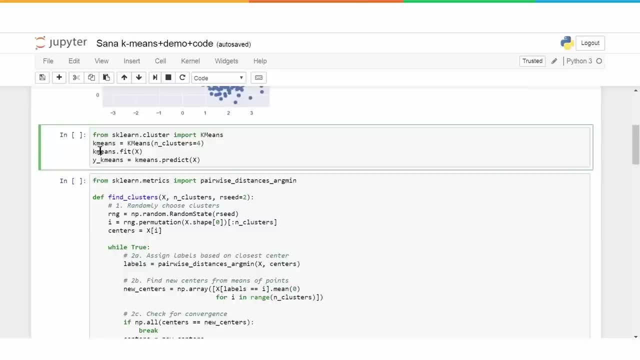 and so that instance is created. we take that instance and, as with any other machine learning functionality, fit is what we use, the function or the method. rather, fit is what we use to train the model. here there is no real training kind of thing, but that's the call. okay, so we are calling fit and what we are doing here. we are just passing the. 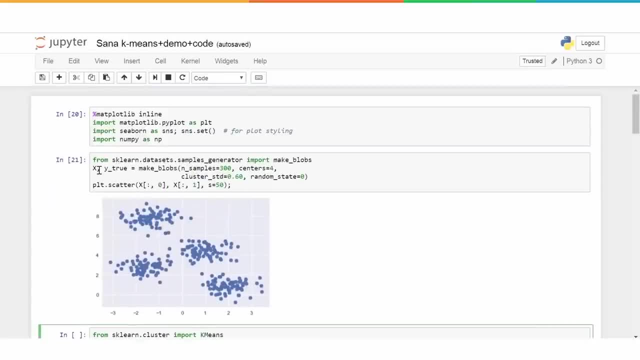 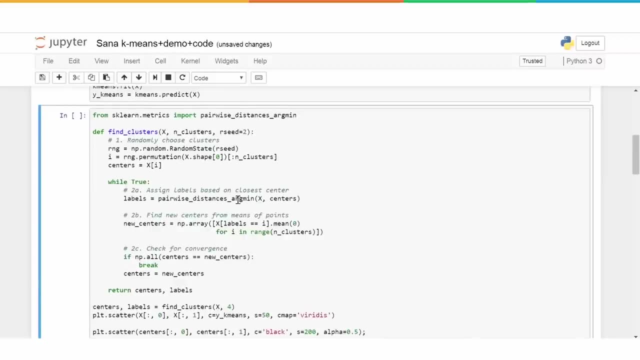 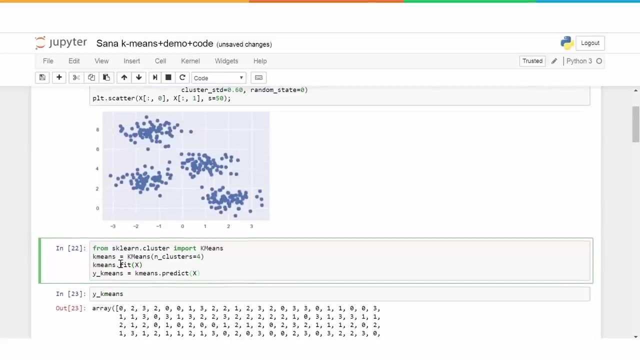 data. so x has these values, the data that has been created, right? so that is what we are passing here and this will go ahead and create the clusters and then we are using, after doing fit, we run the predict, which basically assigns for each of these observations which cluster it belongs to. all right, so it will name the clusters. maybe this is cluster one. this. 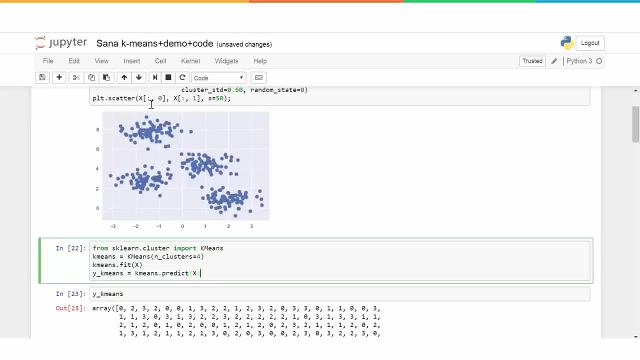 is two, three and so on, or I will actually start from zero cluster zero one, two and three maybe, and then for each of the observations it will assign, based on which cluster it belongs to, it will assign a value so that is stored in y underscore. k means when we call predict that 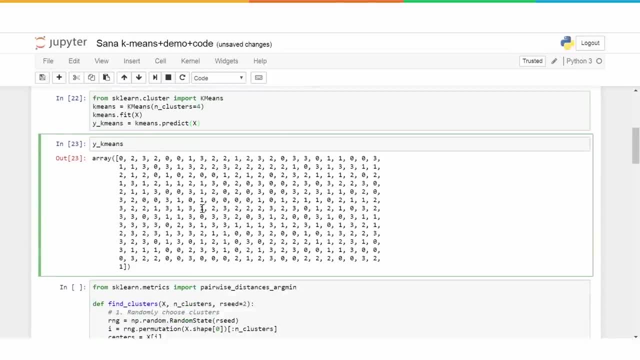 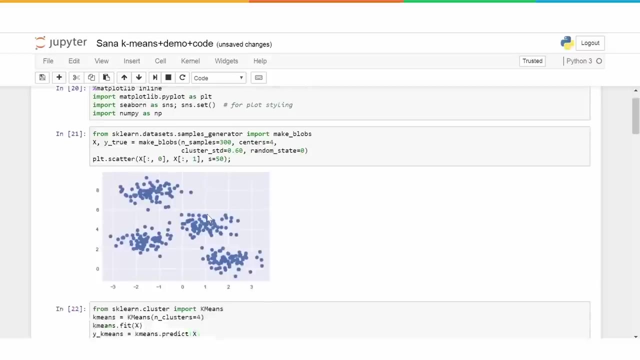 is what it does and we can take a quick look at these: uh, y, underscore, k means or with the cluster numbers that have been assigned for each observation. so this is the cluster number assigned for observation one, maybe this is for observation two, observation three and so on. so we have how many about? I think, 300 samples right. so all the 300 samples. 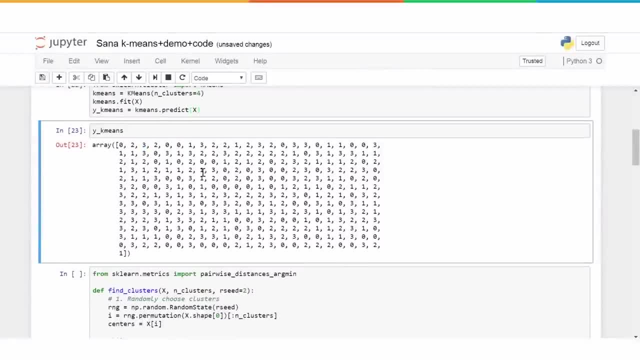 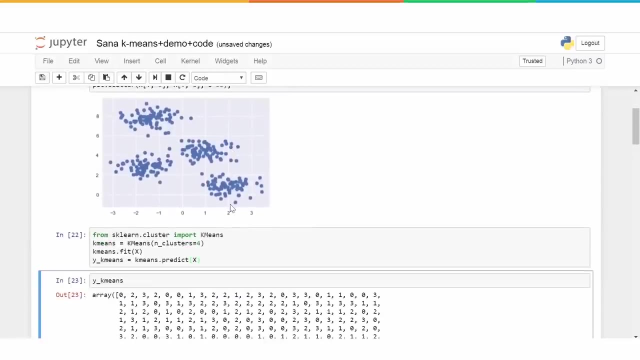 there are 300 values here. each of them, the cluster number is given, and the cluster number goes from zero to three. so there are four clusters, so the numbers go from zero, one, two, three. so that's what is seen here. okay now, so this was a quick example of generating some dummy data and 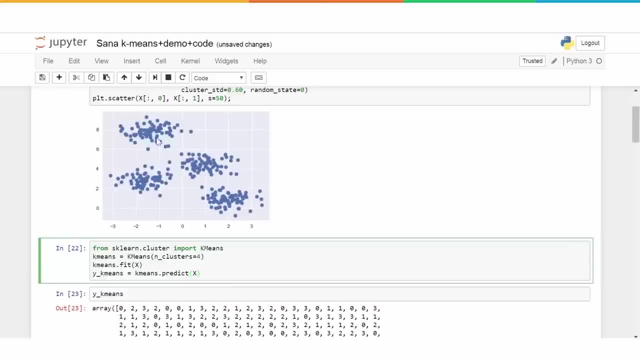 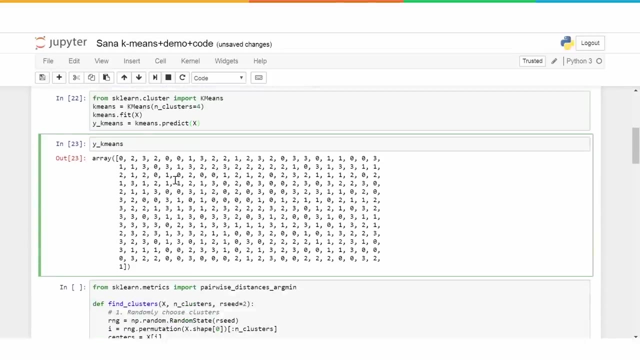 zero, one, two and three maybe, and then for each of the observations it will assign based on which cluster it belongs to, it will assign a value, so that is stored in. y underscore k means: when we call predict, that is what it does, and we can take a quick look at these. y underscore k means or: 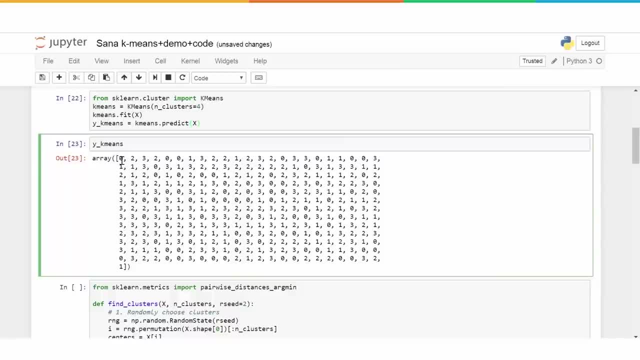 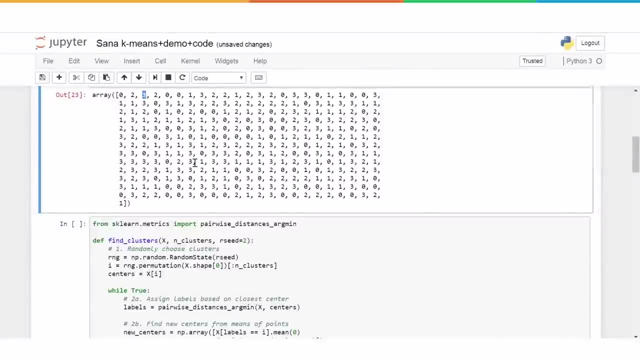 with the cluster numbers that have been assigned for each observation. so this is the cluster number assigned for observation one. maybe this is for observation two, observation three and so on. so we have how many about? i think 300 samples, right. so all the 300 samples. there are 300 values here. 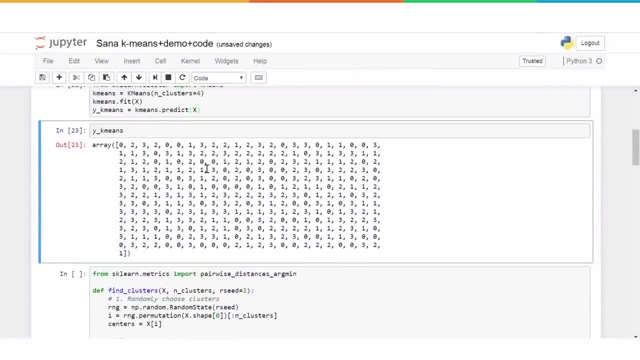 each of them the cluster number is given, and the cluster number goes from zero to a plus five plus five minus six minus a plus four minus a plus five plus five minus a plus to three. so there are four clusters. so the numbers go from zero one, two, three. so that's what is. 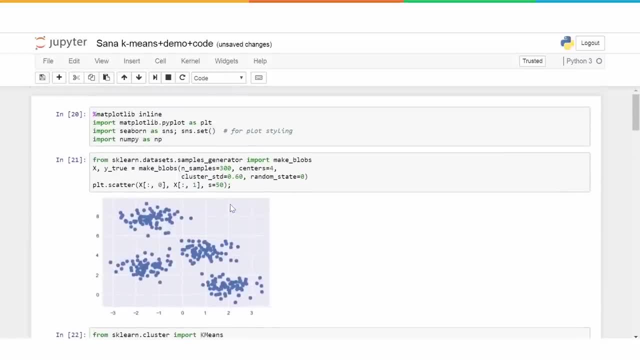 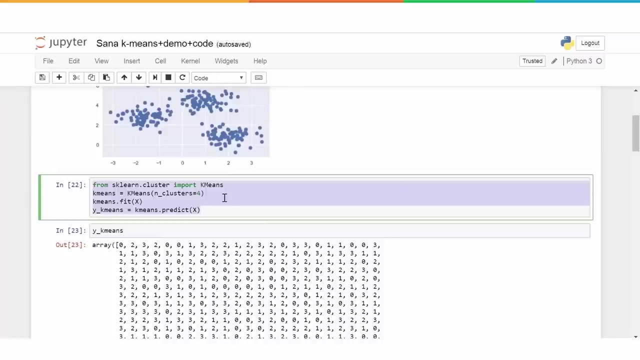 seen here. okay now, so this was a quick example of generating some dummy data and then clustering that. okay, and this can be applied: if you have proper data, you can just load it up into x, for example here, and then run the game. so this is the central part of the k-means clustering program. 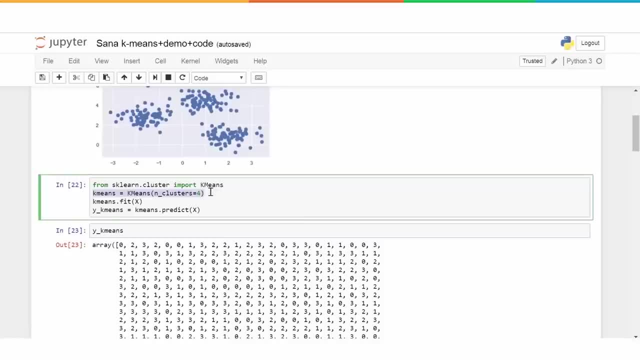 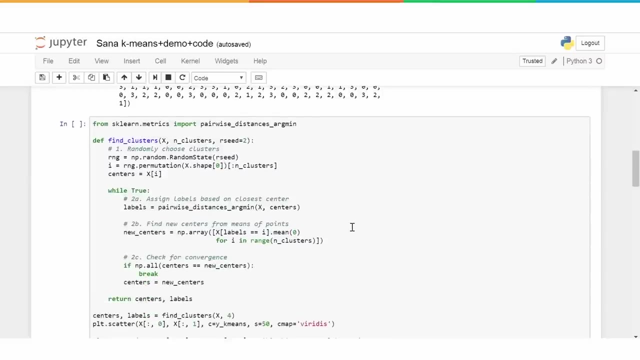 example. so you basically create an instance and you mention how many clusters you want by specifying this parameter and underscore clusters and that is also the value of k, and then pass the data to get the values. now the next section of this code is the implementation of a k-means. 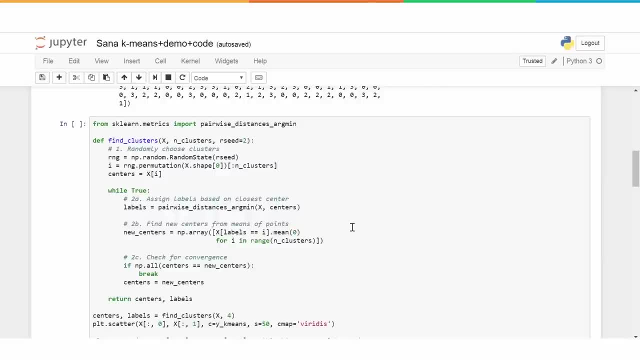 now this is kind of a rough implementation of the k-means algorithm, so we will just walk you through. i will walk you through the code at each step, what it is doing, and then we will see a couple of more examples of how k-means clustering can be used in maybe some real 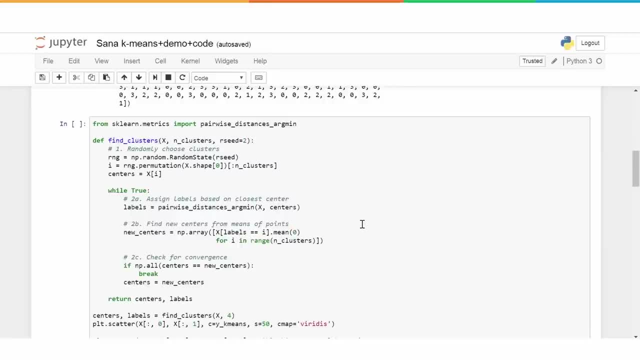 life examples, real life use cases, all right. so in this case, here, what we are doing is basically implementing k-means clustering, and there is a function for a library calculates for a given two pairs of points. it will calculate the, the distance between them and see which one is the. 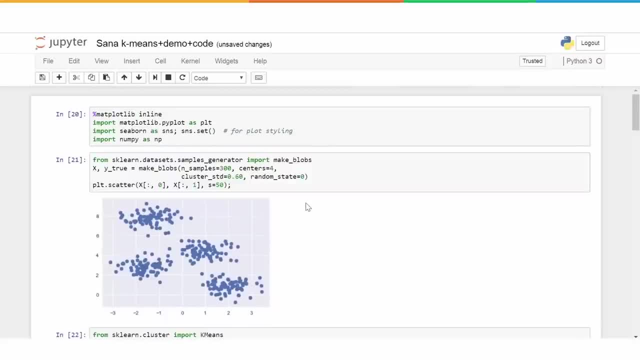 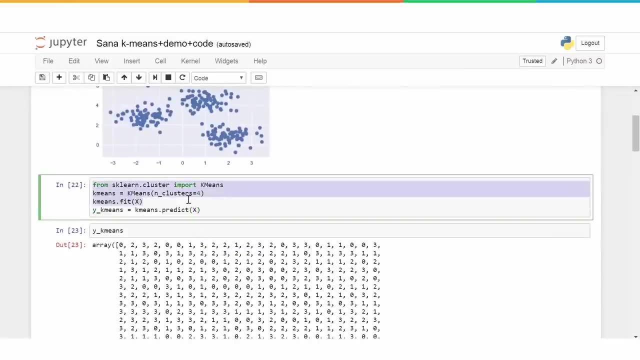 then clustering. that okay, and this can be applied. if you have proper data, you can just load it up into x, for example here, and then run the game. so this is the central part of the k-means clustering program example. so you basically create an instance and you mention how many clusters. 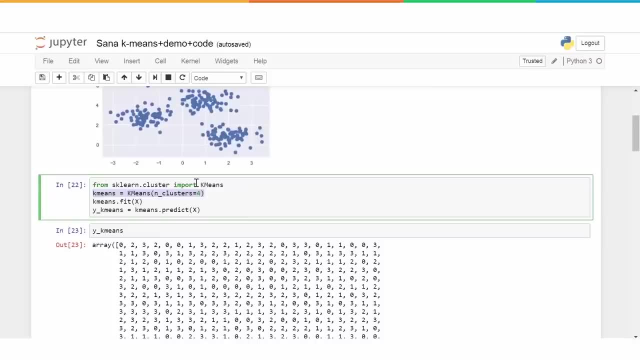 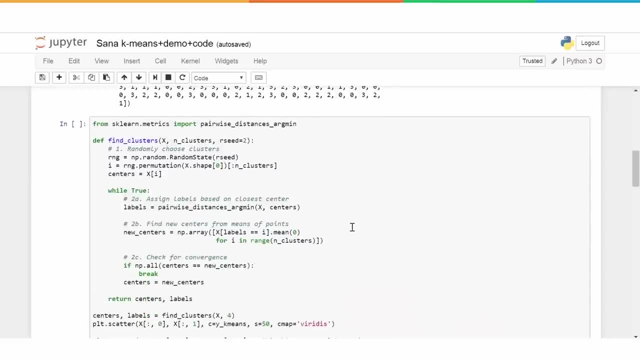 you want by specifying this parameter and underscore clusters and that is also the value, okay, and then pass the data to get the values. now the next section of this code is the implementation of a k-means. now, this is kind of a rough implementation of the k-means algorithm, so 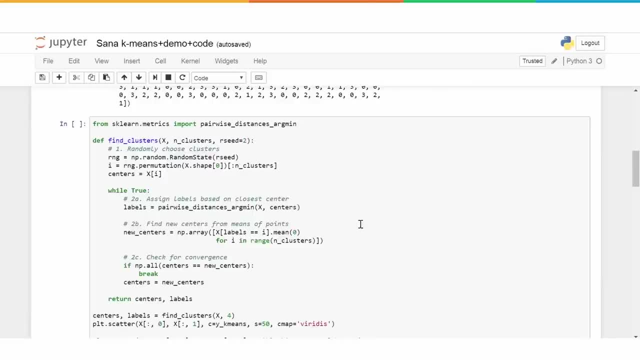 we will just walk you through. I will walk you through the code at each step, what it is doing, and then we will see a couple of more examples of how k-means clustering can be used in. maybe some real life examples, real life use cases. all right, so in this, 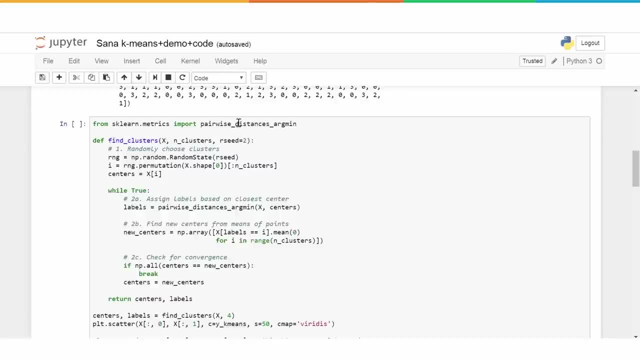 case. here, what we are doing is basically implementing k-means clustering, and there is a function for a library calculates for a given two pairs of points. it will calculate the, the distance between them and see which one is the closest, and so on. so this is like. 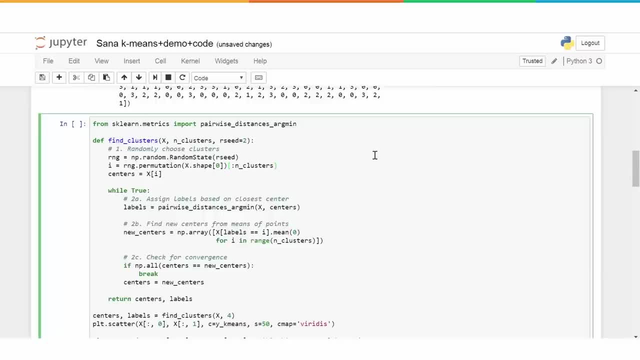 this is pretty much like what k-means does, right? so it calculates the distance of each point or each data set from predefined centroid and then, based on whichever is the lowest, this particular data point is assigned to that centroid. so that is basically available as a standard function and we will be using that here. so, as explained in the slides, the first step. 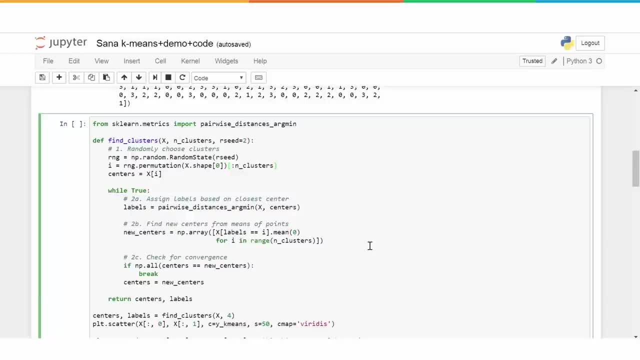 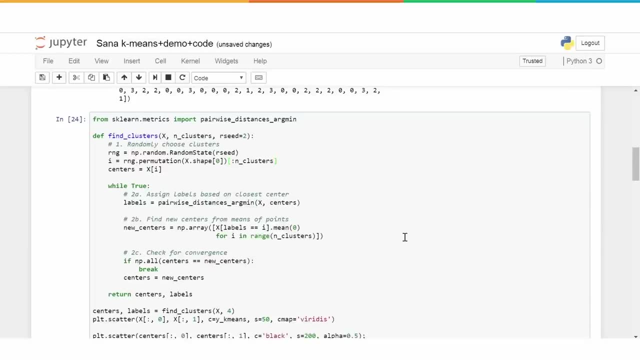 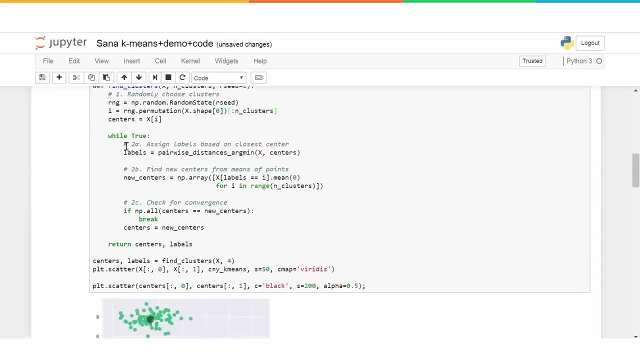 that is done in case of k-means clustering is to randomly assign some centroids. so as a first step we randomly allocate a couple of centroids which we call- here we are calling- as centers, and then we put this in a loop and we take it through an iterative process for each of the data points. we first 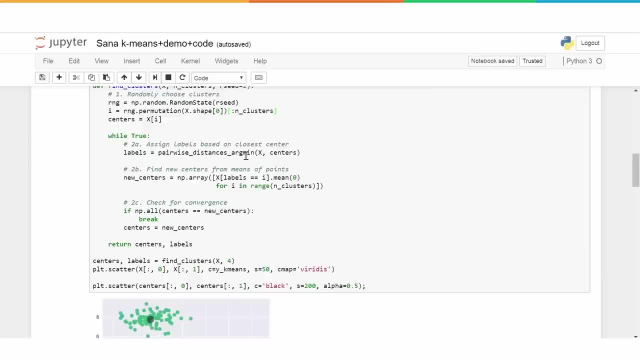 find out using this function, pairwise distance argument for each of the points. we find out which one, which center or which randomly selected centroid is the closest and accordingly we assign the data or the data point to that particular centroid or cluster. and once that is done, for all. 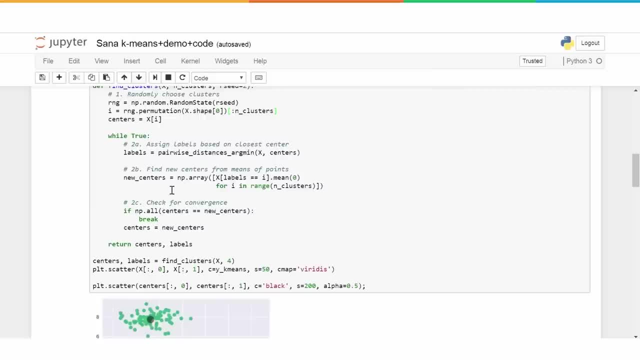 the data points. we calculate the new centroid by finding out the mean position, with the center position right. so we calculate the new centroid and then we check if the new centroid is the coordinates or the position is the same as the previous centroid. the positions we will compare and if it is the same, that means 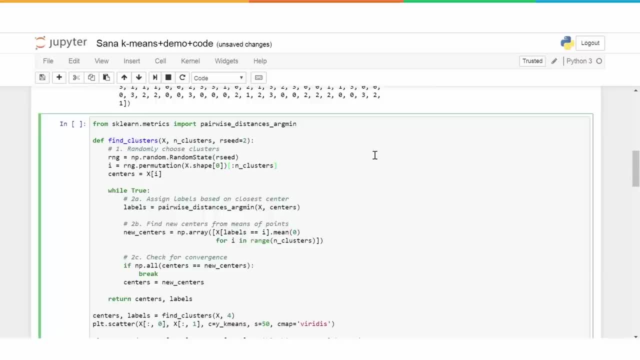 closest, and so on. so this is like. this is pretty much like what k-means does, right? so it calculates the distance of each point or each data set from predefined centroid and then, based on whichever is the lowest, this particular data point is assigned to that percent, right? so that is basically available as a standard function, and 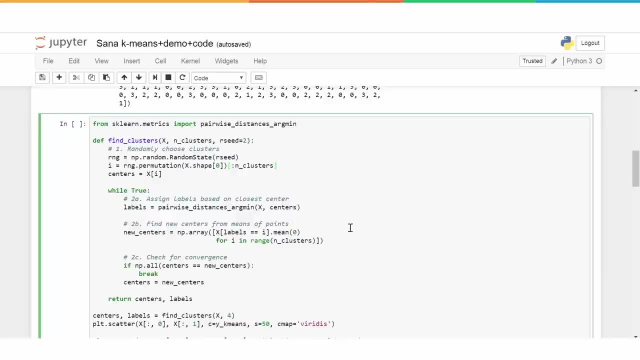 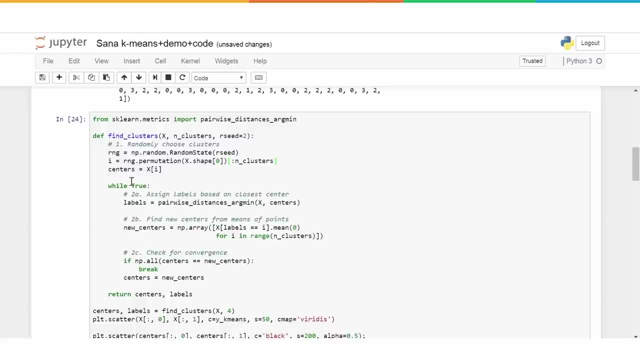 we will be using that here. so, as explained in the slides, the first step that is done in case of k-means clustering is to randomly assign some centroids. so, as a first step, we randomly allocate a couple of centroids which we call. here we are calling as: 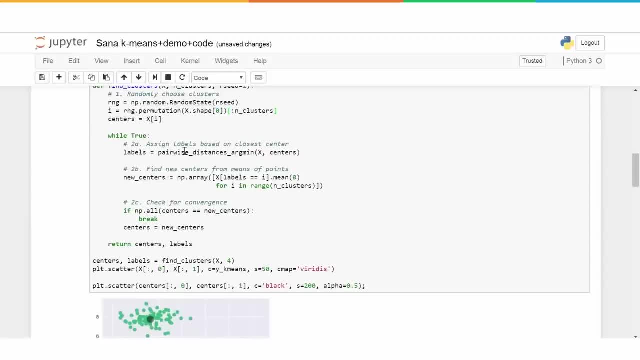 centers, and then we put this in a loop and we take it through an iterative process. for each of the data points, we first find out using this function, pairwise distance argument. for each of the points, we find out which one, which center or which randomly selected centroid is the closest, and 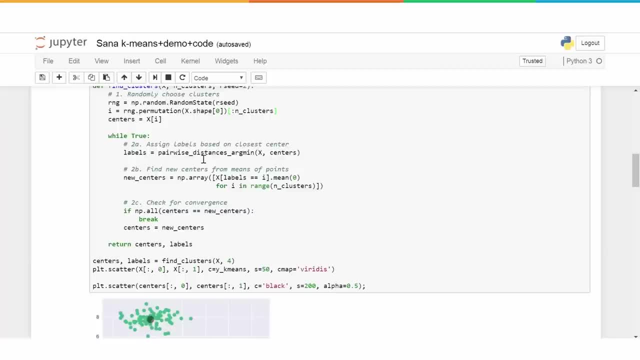 we assign that data or the data point to that particular centroid or cluster and once that is done for all the data points, we calculate the new centroid by finding out the mean position, with the center position right. so we calculate the new centroid and then we check if the new centroid 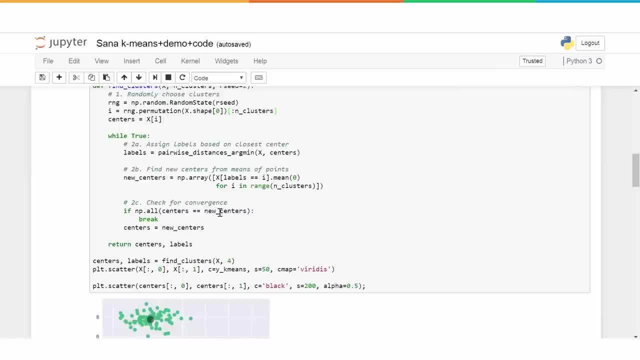 is the coordinates or the position is the same as the previous centroid, the positions, we will come here. and if it is the same, that means the process has converged. so remember, we do this process till these centroids or the centroid doesn't move anymore, right? so the centroid gets relocated each 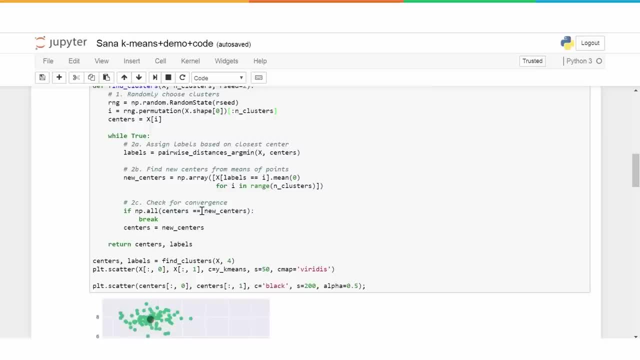 time this reallocation is done, so the moment it doesn't change anymore. the position of the centroid doesn't change anymore. we know that convergence has occurred. so till then. so you see, here this is like an infinite loop. while true is an infinite loop, it only takes when the centers are the same, the new center and the old center positions are the same, and 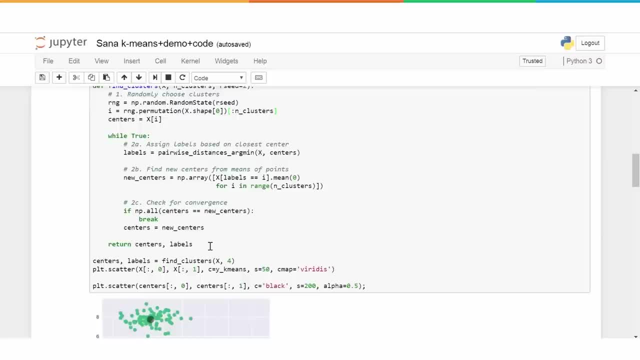 once that is done, we return the centers and the labels. now, of course, as explained, this is not a very sophisticated and advanced implementation, very basic implementation, because one of the flaws in this is that sometimes what happens is the centroid, the position, will keep moving, but in the change will be very minor. so in that case, also with that is actually. 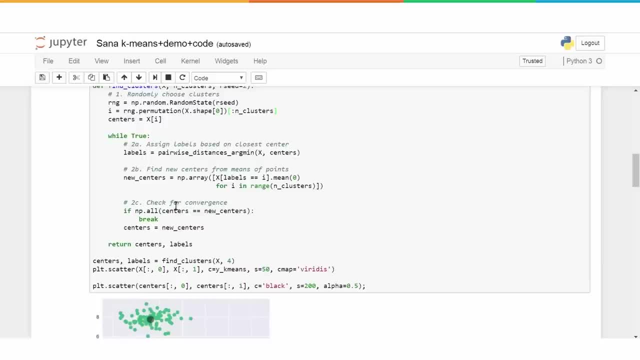 the process has converged. so remember, we do this process till these centroids or the centroid doesn't move anymore, right? so the centroid gets relocated each time this relocation is done. so the moment it doesn't change anymore, the position of the centroid doesn't change anymore. we know that. 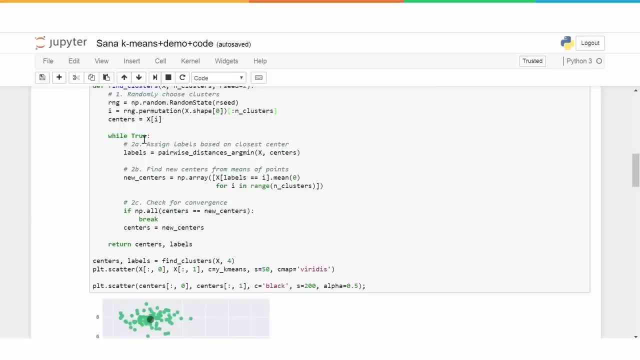 convergence has occurred. so till then. so you see, here this is like an infinite loop. while true is an infinite loop, it only breaks when the centers are the same, the new center and the old center, positions are the same, and once that is done, we return the centers and the labels. 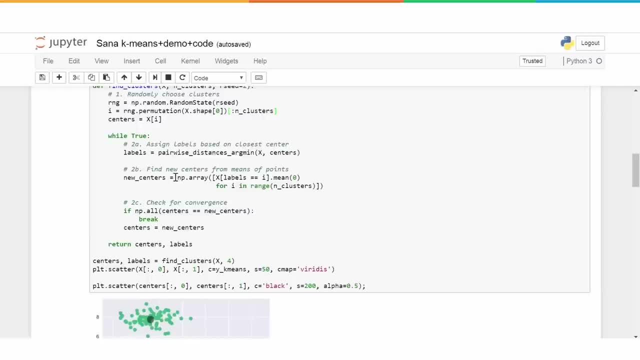 course, as explained, this is not a very sophisticated and advanced implementation, very basic implementation, because one of the flaws in this is that sometimes what happens is the centroid, the position, will keep moving, but in the change will be very minor. so in that case, also with that is actually. 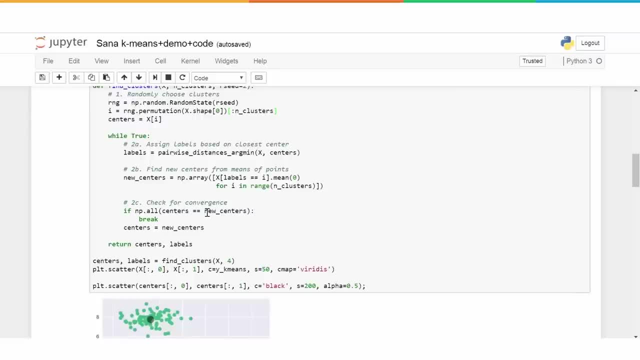 convergence right. so, for example, the change is 0.0001, we can consider that as convergence. otherwise, what will happen is this will either take forever or it will be never ending. so that's a small flaw here. so that is something. additional checks may have to be added here, but again, as 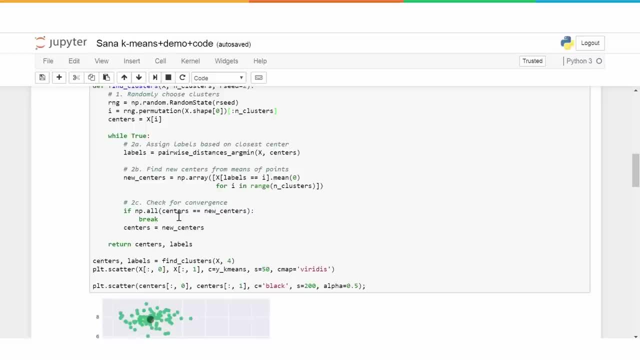 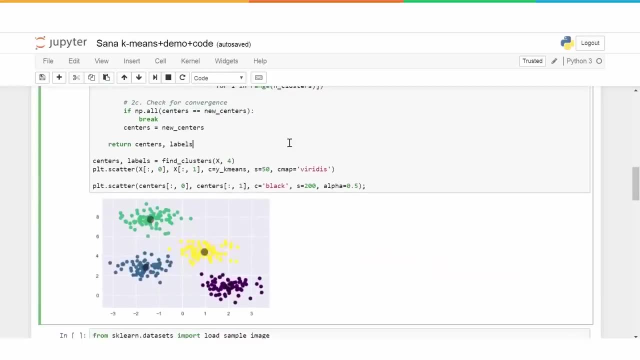 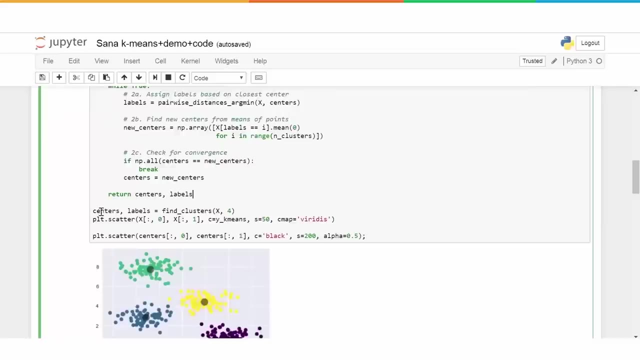 mentioned, this is not the most sophisticated implementation. this is like a kind of a rough implementation of the k-means clustering. okay, so if we execute this code, this is what we get as the output. so this is the definition of this particular function, and then we call that find. 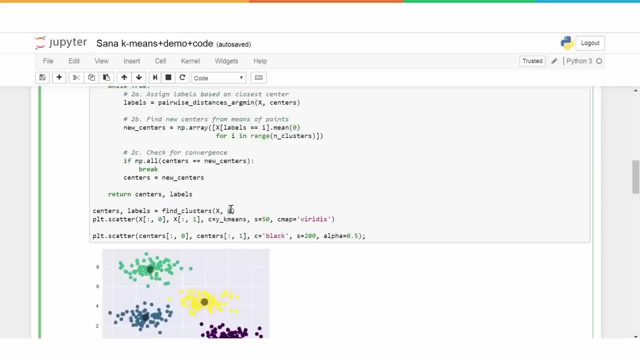 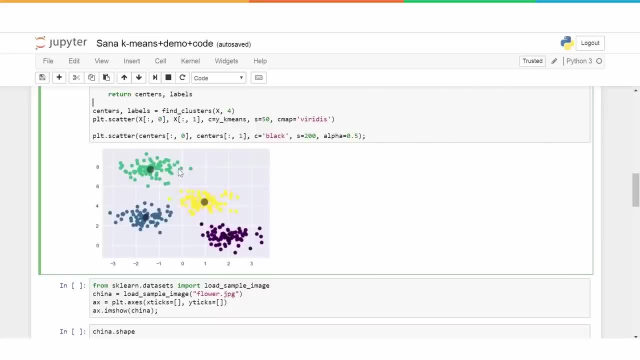 under score clusters and we pass our data, x, and the number of clusters, which is four, and if we run that and plot it, this is the output that we get. so this is, of course. each cluster is represented by a different color, so we have a cluster in green color, yellow color and so on and so forth, and 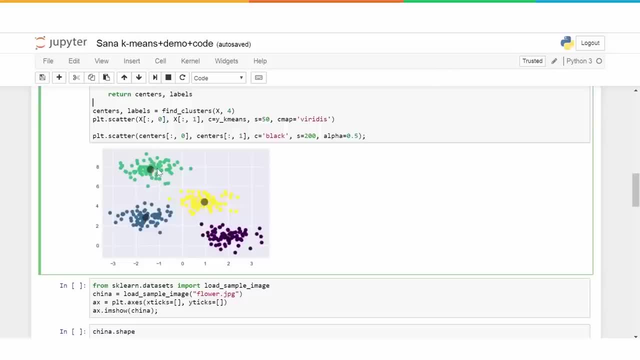 these big points here, these are the centroids, is the final position of the centroids and, as you can see, visually also, this appears like a kind of a center of all these points here, right. similarly, this is the center of all these points here, and so on. so this is the example, or this is an example of a 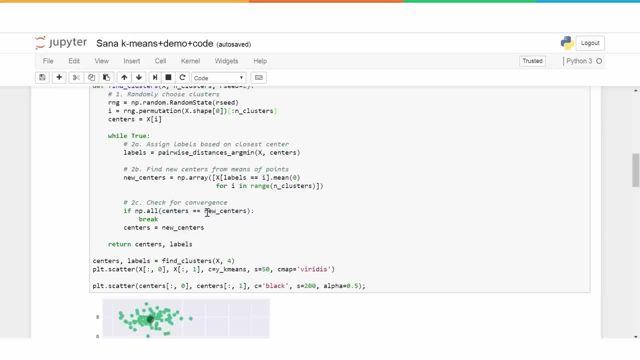 right. so, for example, the change is 0.0001. we can consider that as convergence. otherwise, what will happen is this will either take forever or it will be never ending. so that's a small flaw here. so that is something. additional checks may have to be added here. but again, as mentioned, this is. 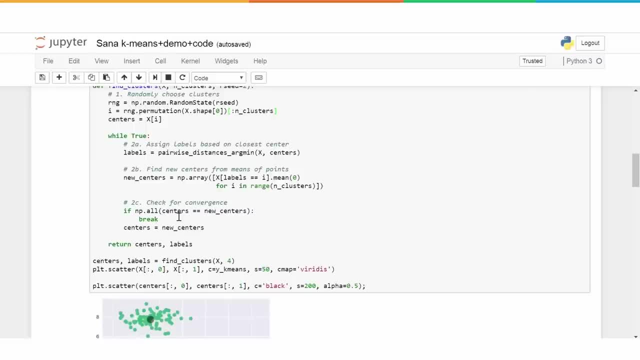 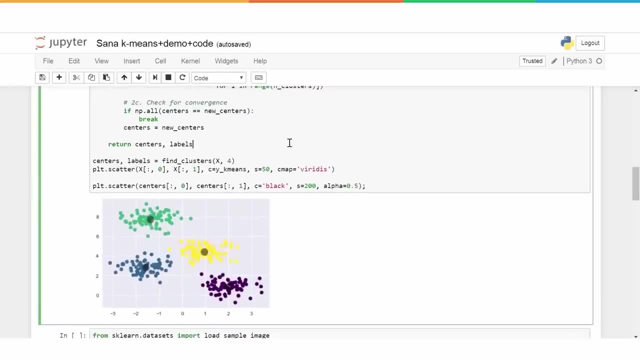 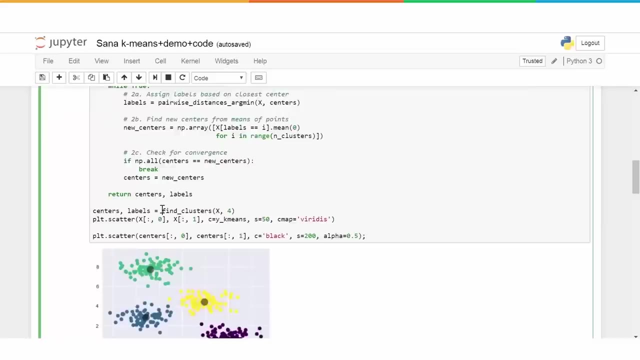 not the most sophisticated implementation. this is like a kind of a rough implementation of the k-means clustering. okay, so if we execute this code, this is what we get as the output. so this is the definition of this particular function, and then we call that: find underscore clusters. 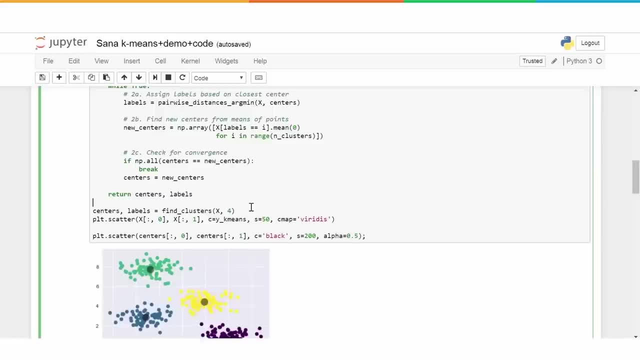 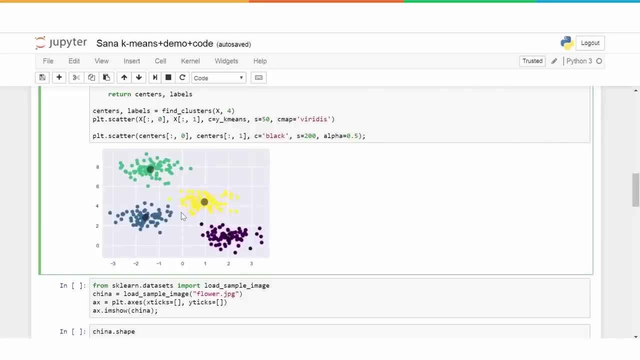 and we pass our data, x, and the number of clusters, which is four, and if we run that and plot it, this is the output that we get. so this is, of course. each cluster is represented by a different color, so we have a cluster in green color, yellow color and so on and so forth, and these big points here. 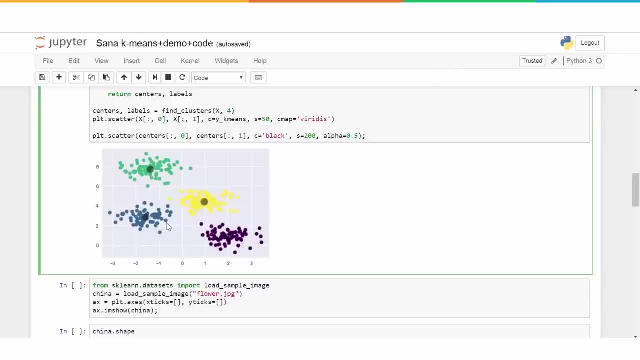 these are the centroids, this is the final position of the centroids and, as you can see, visually also the center of the cluster appears like a kind of a center of all these points here, right. similarly, this is like the center of all these points here and so on. so this is the example or this is an 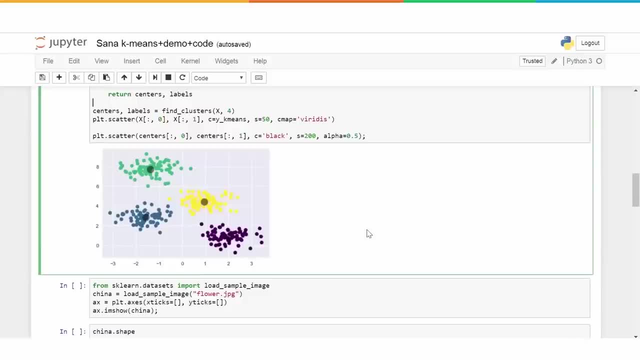 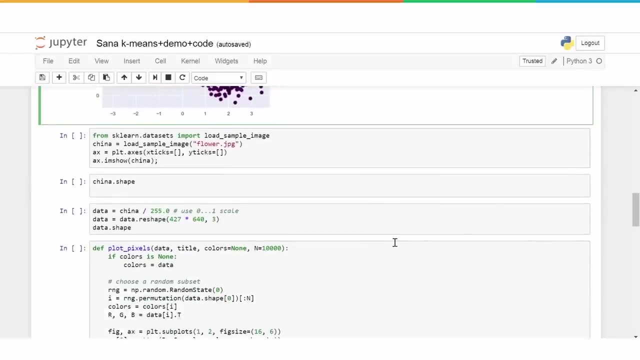 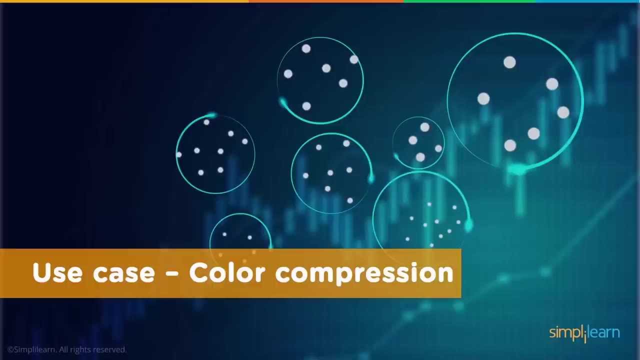 example of a implementation of k-means clustering and next we will move on to see a couple of examples of how k-means clustering is used in maybe some real-life scenarios or use cases. in the next example or demo, we are going to see how we can use k-means clustering to perform color compression. we will 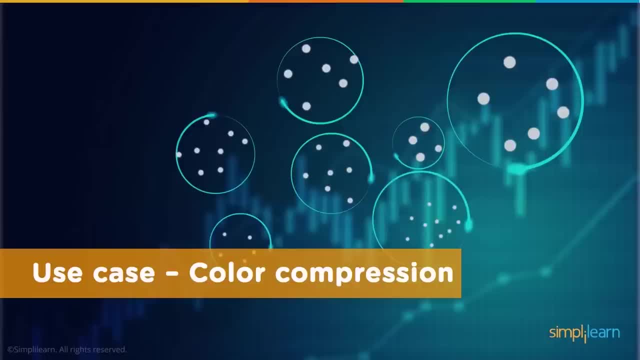 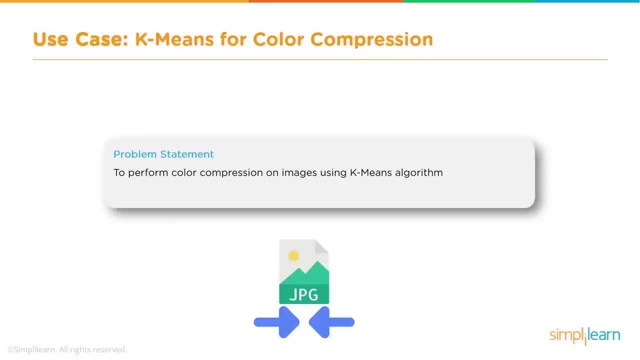 take a couple of images, so there will be two examples and we will try to use k-means clustering to compress the colors. this is a common situation in image processing, when you have an image with millions of colors but then you cannot render it on some devices which may not have enough memory. 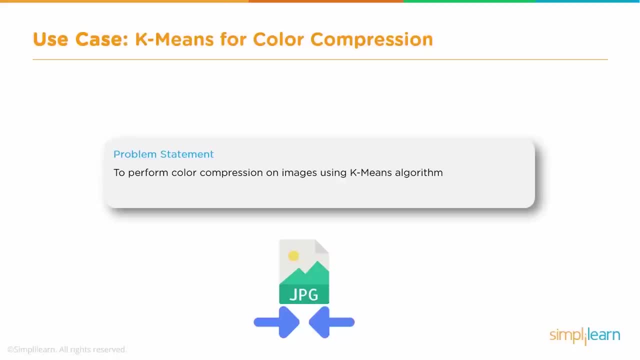 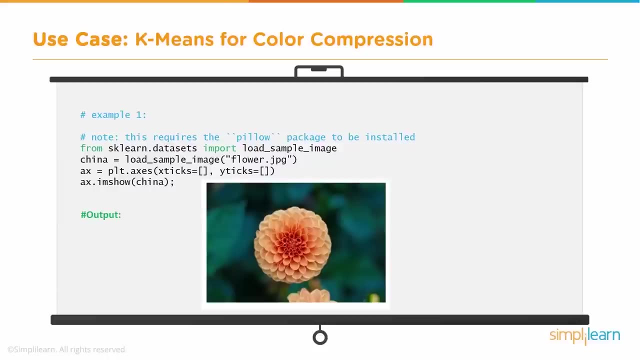 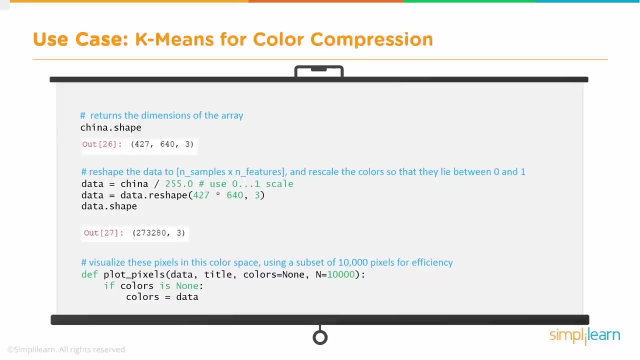 so that is the scenario where where something like this can be used. so before again we go into the python notebook, let's take a look at quickly the the code. as usual, we import the libraries and then we import the image and then we will flatten it. so the reshaping is basically: we have the image. 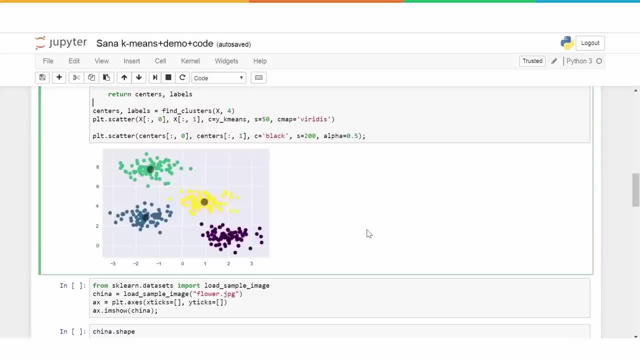 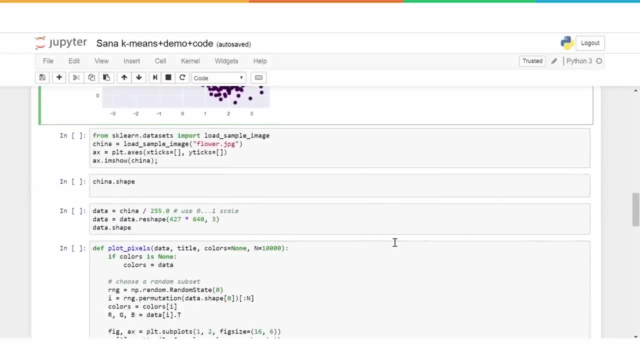 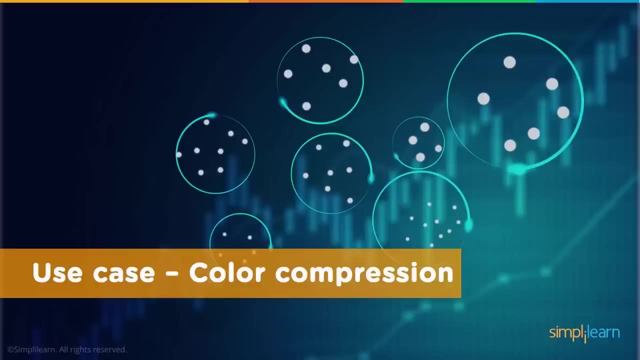 implementation of k-means clustering, and next we will move on to see a couple of examples of how k-means clustering is used in maybe some real life scenarios or use cases. in the next example or demo, we are going to see how we can use k-means clustering to perform color compression. 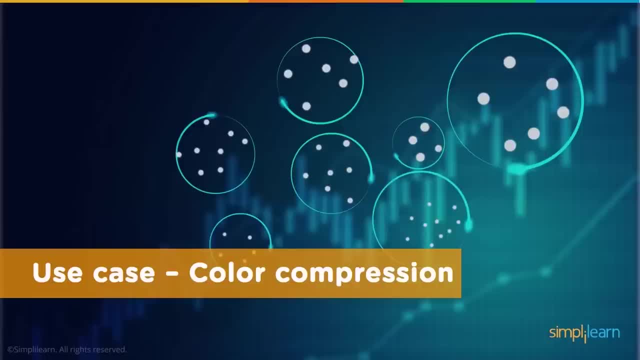 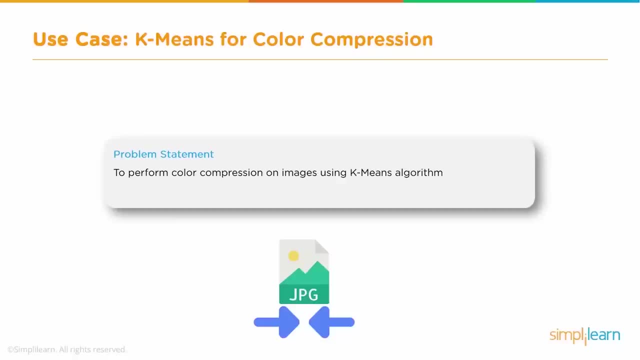 we will take a couple of images, so there will be two examples and we will try to use k-means- clustering- to compress the colors. this is a common situation in image processing, when you have an image with millions of colors but then you cannot render it on some devices which may not have enough. 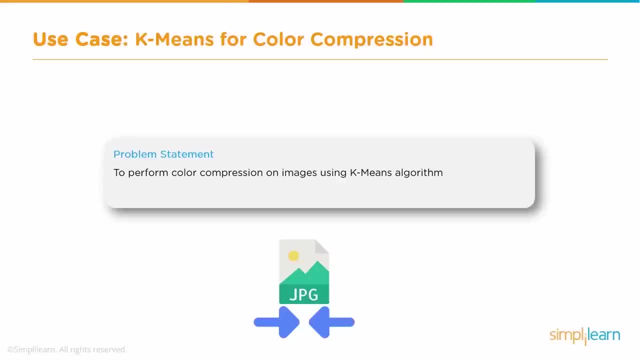 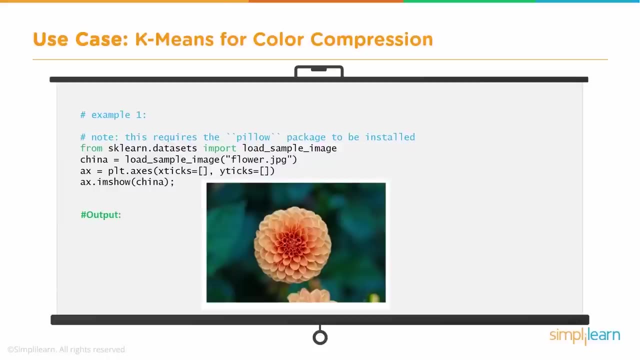 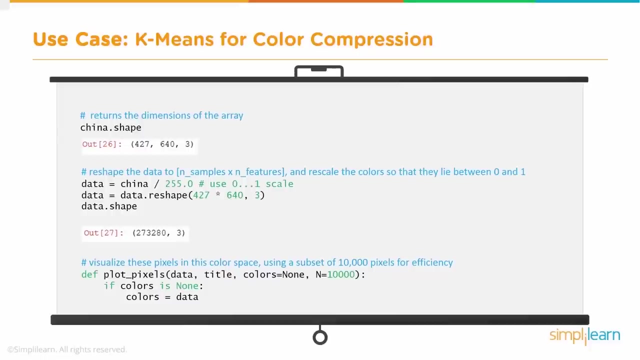 memory. so that is the scenario where where something like this can be used. so before again we go into the python notebook, let's take a look at quickly the the code. as usual, we import the libraries and then we import the image and then we will flatten it. so the reshaping is basically: we have the image. 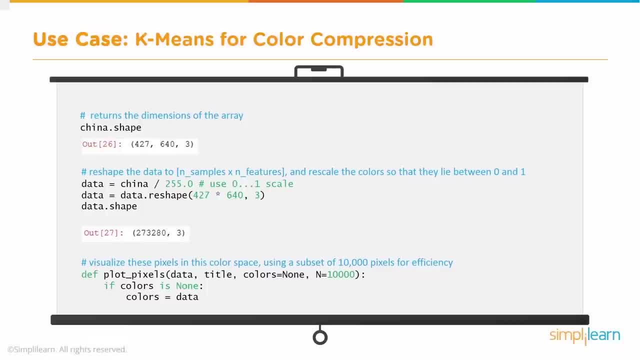 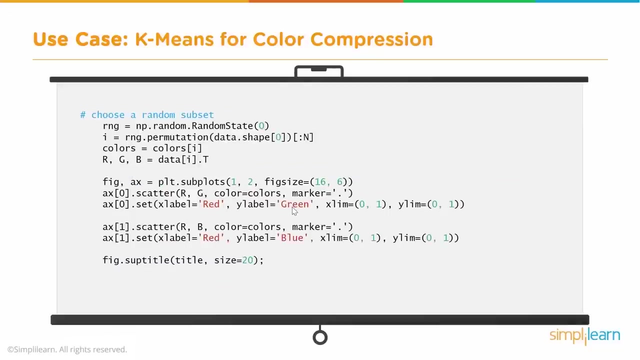 information is stored in the form of pixels, and if the image is like, for example, 427 by 640 and it has three colors- so that's the overall dimension of the of the initial image- we just reshape it and then feed this to our algorithm and this will then create clusters of only 16. 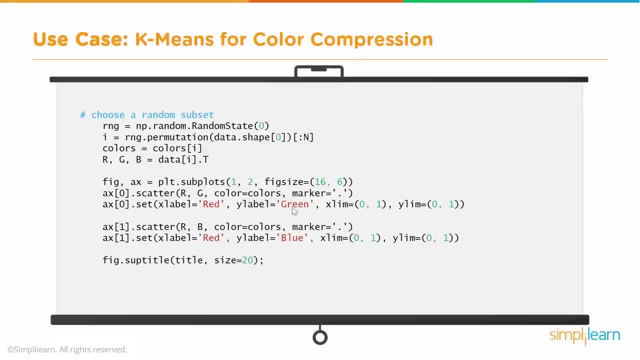 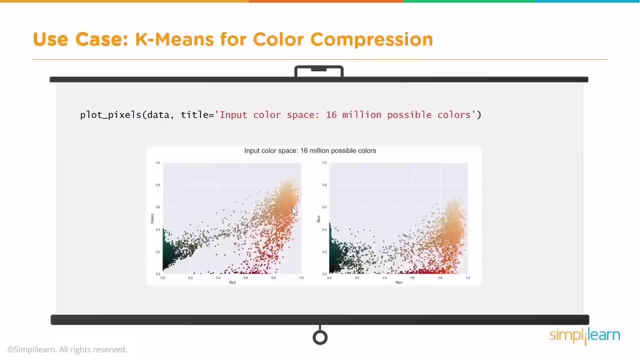 clusters. so this, this colors. there are millions of colors and now we need to bring it down to 16 colors, so we use: k is equal to 16 and this is a. when we visualize, this is how it looks. there are- these are all about 16 million possible colors. the 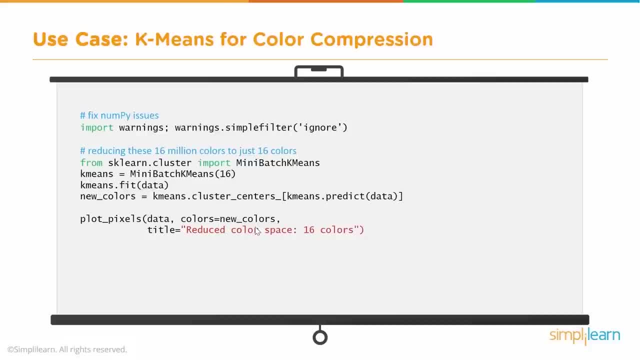 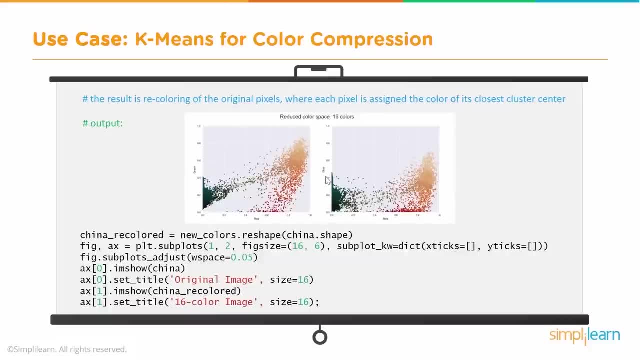 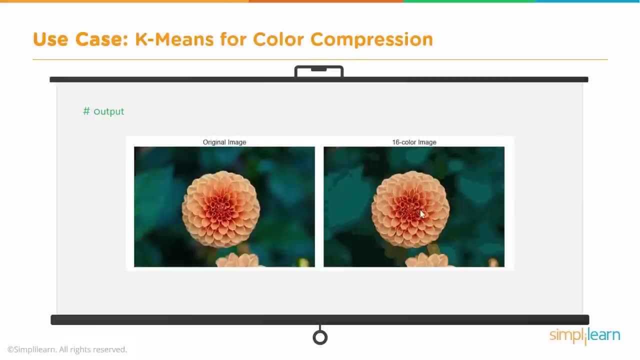 input color space has 16 million possible colors and we just some compress it to 16 colors. so this is how it would look when we compress it to 16 colors and this is how the original image looks and after compression to 16 colors. this is a the new image looks. as you can see, there is not a lot. 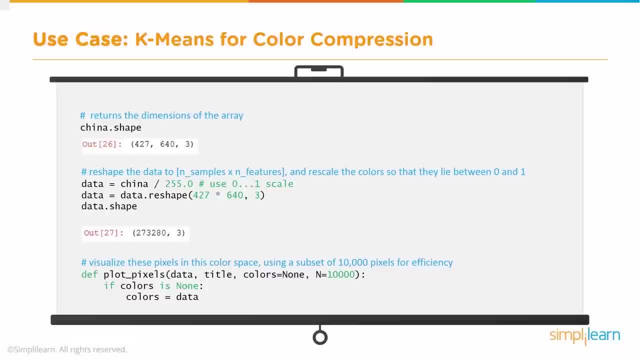 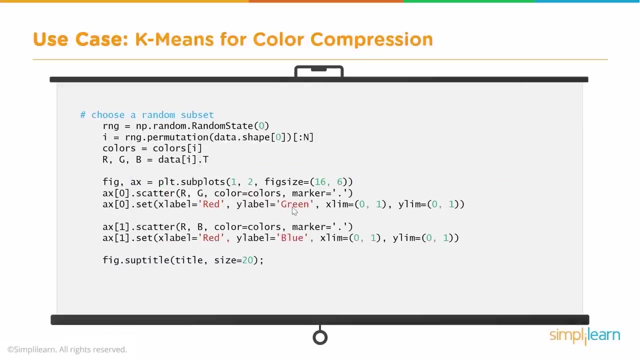 information is stored in the form of pixels and if the images like, for example, 427 by six, 40 and it has three colors, so that's the overall dimension of the of the initial image- we just reshape it and then feed this to our algorithm and this will then create clusters of only 16. 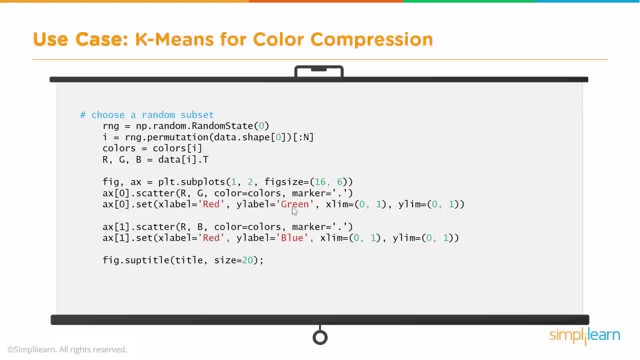 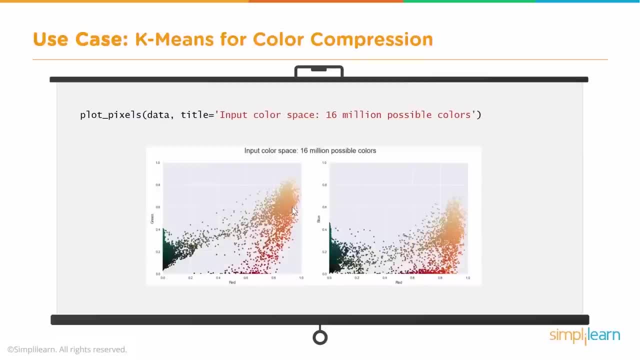 clusters. so this, this colors. there are millions of colors and now we need to bring it down to 16 colors, so we use: k is equal to 16 and this is a little bit more complex than the original image. so when we visualize, this is how it looks there. 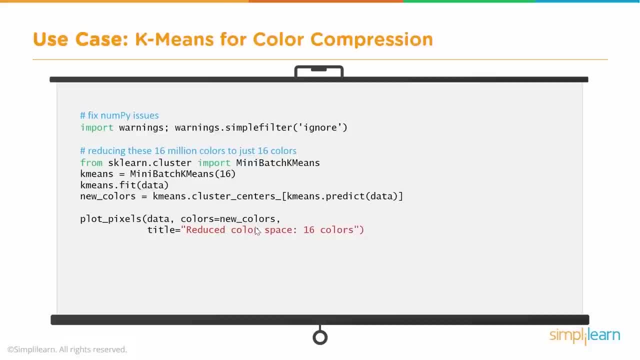 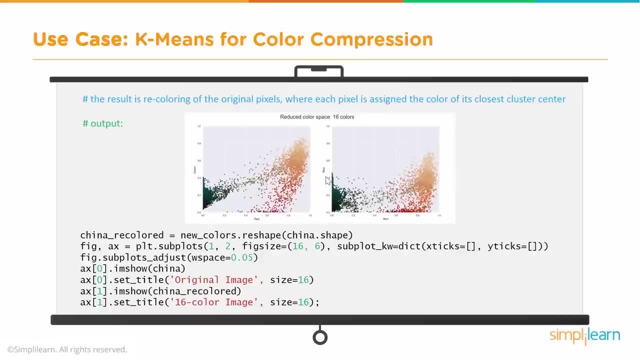 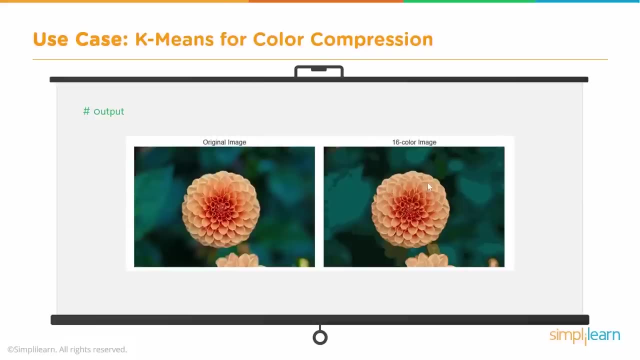 are. these are all about 16 million possible colors. the input color space has 16 million possible colors and we just sub compress it to 16 colors. so this is how it would look when we compress it to 16 colors and this is how the original image looks and after compression to 16. 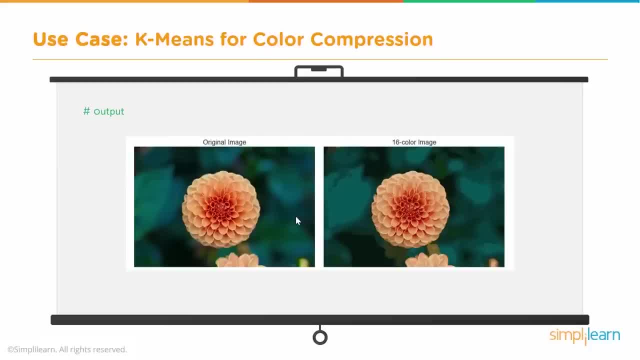 colors. this is how the new image looks. as you can see, there is not a lot of color that has been lost, though the image quality is definitely reduced a little bit. so this is an example which we are going to now see in python notebook. let's go into the python. 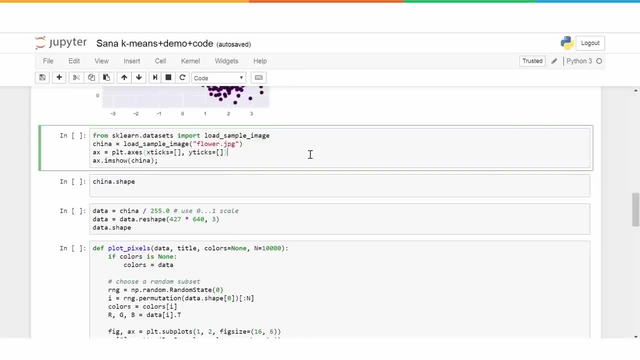 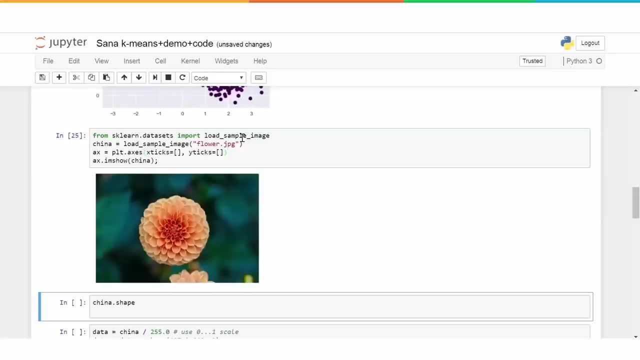 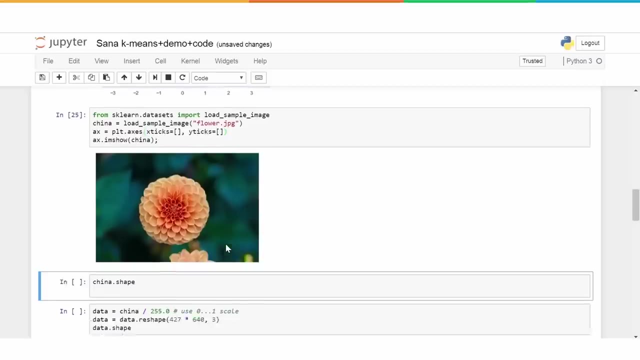 and once again, as always, we will import some libraries and load this image called flowerjpg. okay, so let we load that and this is how it looks. this is the original image, which has, i think, 16 million colors, and this is the shape of this image, which is basically what is the shape is. 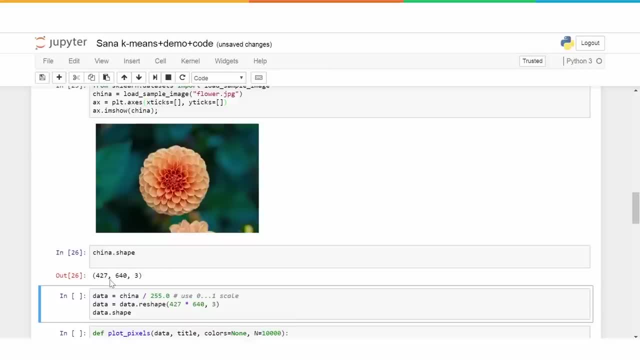 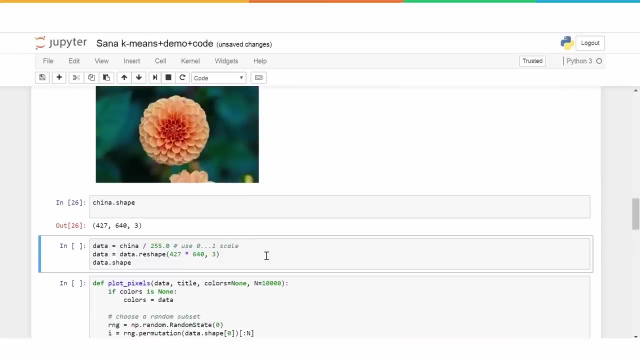 nothing but the overall size, right. so this is 427 pixel by 640 pixel, and then there are three layers, which is this. three basically is for rgb, which is red, green, blue. so color image will have that right. so that is the shape of this. now what we need to do is data. let's take a look at how data is looking. 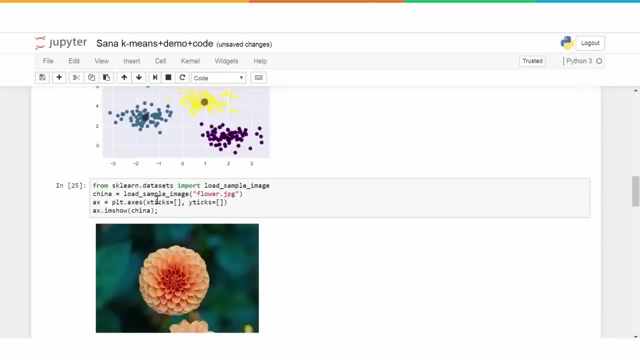 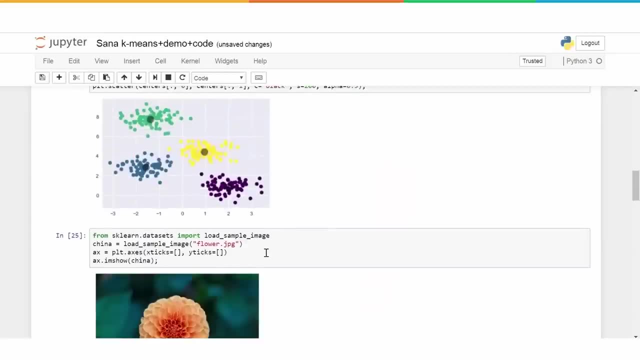 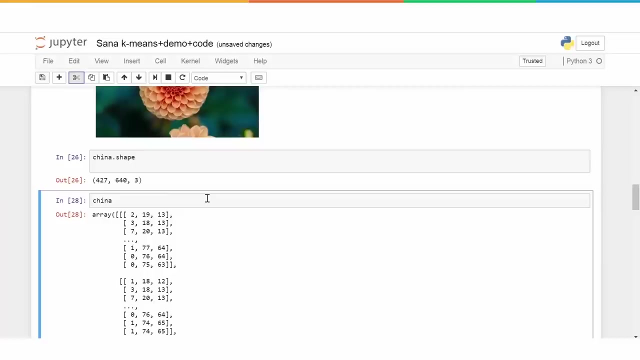 and so this is how we have the data to store and show you what is in data. basically, we have captured this information. so data is what? let me just show you here. all right, so let's take a look at china. what are the values in china? and if we see here, this is how. 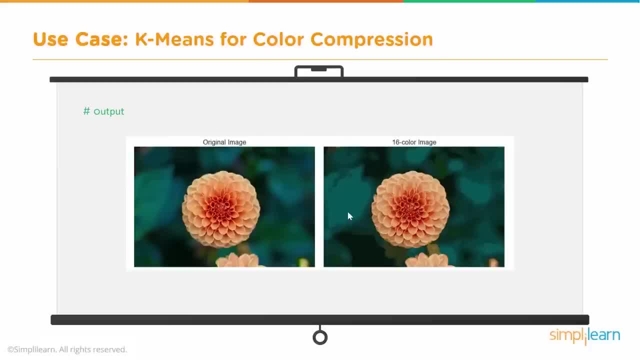 of information that has been given to the image when we compress it to 16 colors. so we have to been lost, though the image quality is definitely reduced a little bit. so this is an example which we are going to now see in Python notebook. let's go into the 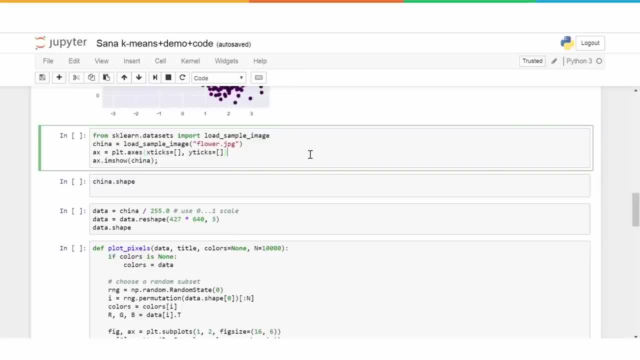 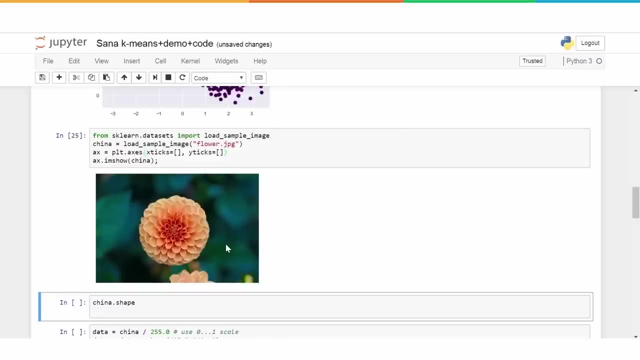 Python and once again, as always, we will import some libraries and load this image called flower dot JPG. okay, so let me load that and this is how it looks. this is the original image, which has, I think, 16 million colors, and this is the shape of this image, which is basically what is. the shape is nothing but the. 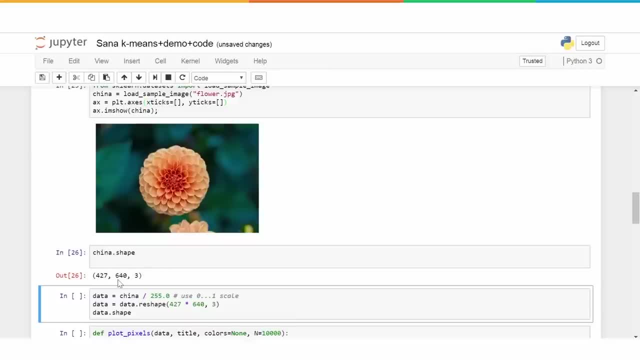 overall size, right. so this is 427 pixel by 640 pixel, and then there are three layers, which is this. three, basically, is for RGB, which is red, green, blue. so color image will have that right. so that is the shape of this. now what we need to do. 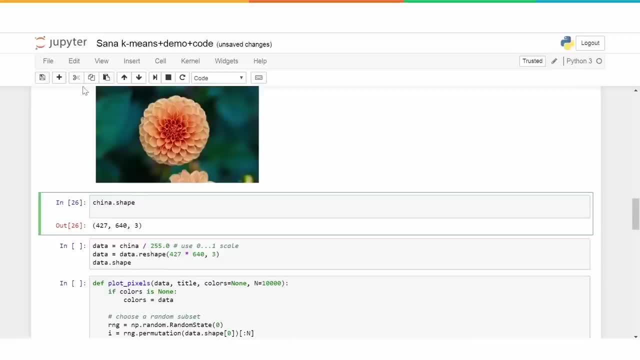 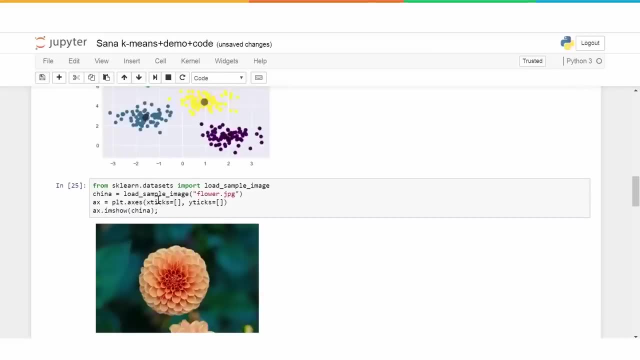 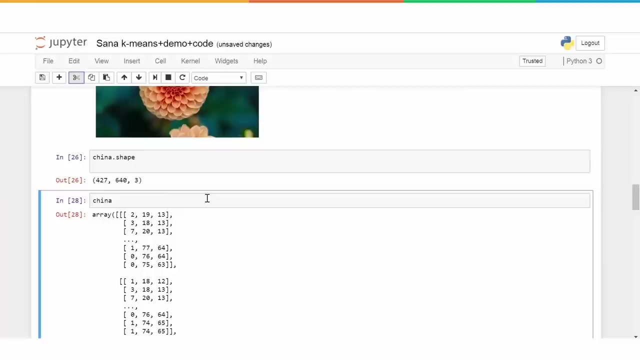 is data. let's take a look at how data is looking. so let me just create a new cell and show you what is in data. basically, we have captured this information, so data is what let me just show you here. all right, so let's take a look at China. what are the values in China? and if we 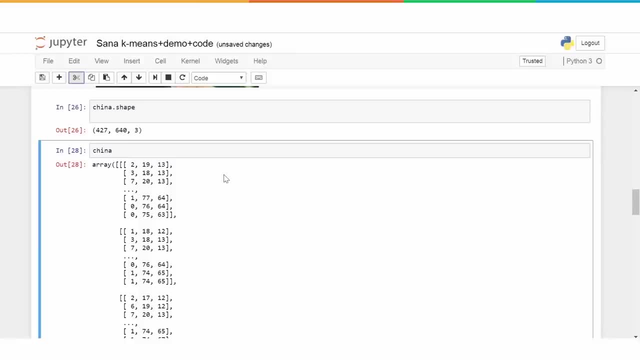 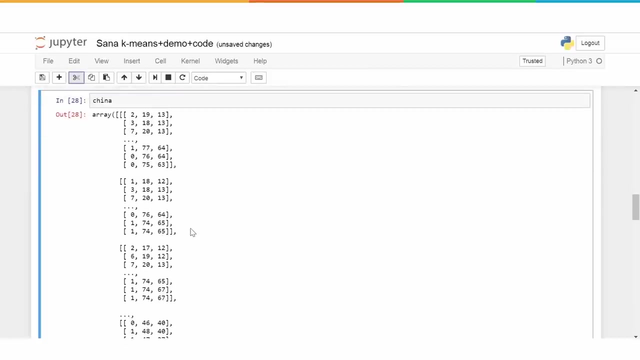 see here. this is how the data is stored. this is nothing but the pixel values. okay, so this is like a matrix, and each one has about for for this 427 by 640 pixels. all right, so this is how it looks. now. the issue here is: these values are large, the numbers are a lot, so we 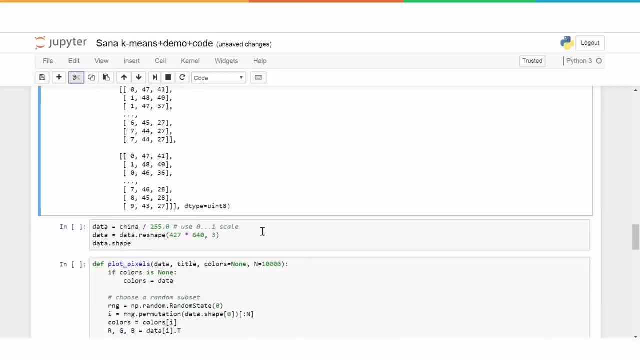 need to normalize them to between 0 and 1, right? so that's why we will basically create one more variable, which is data, which will contain the values between 0 and 1, and the way to do that is divided by 255. so we divide China by 255 and we get the. 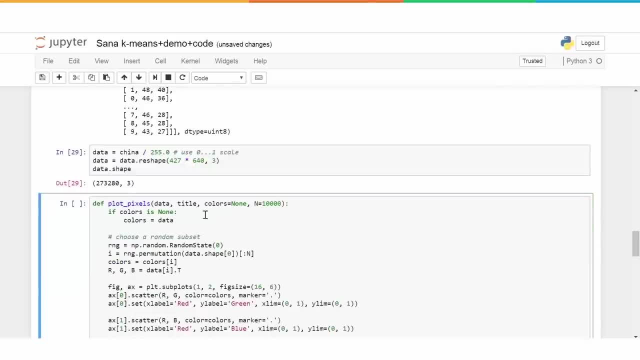 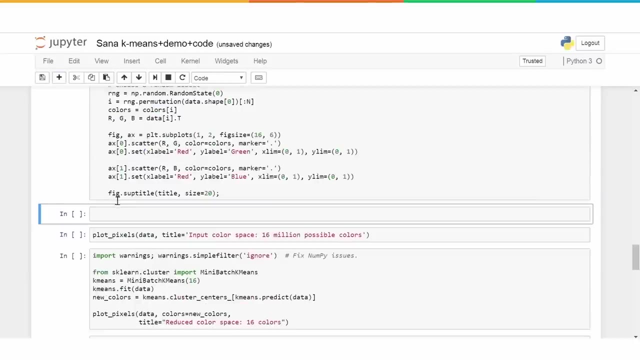 the new values in data. So let's just run this piece of code And this is the shape. So we now have also. Yeah, what we have done is we changed, using reshape, we converted into the three dimensional, into a two dimensional data set. And let us also take a look at how. let me just insert: 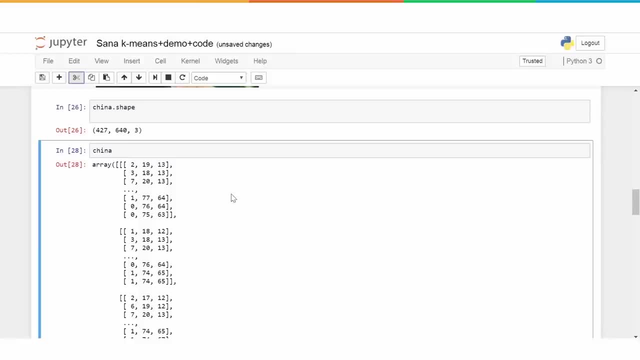 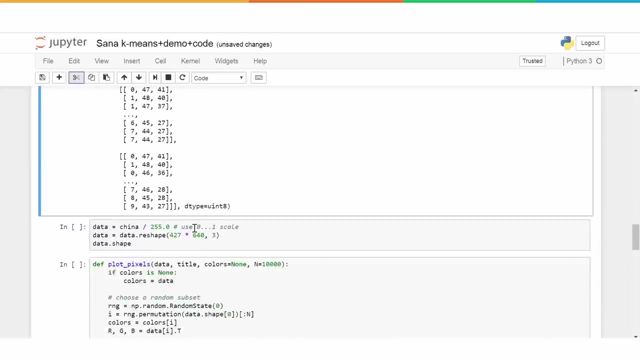 the data is stored. this is nothing but the pixel values. okay, so this is like a matrix, and each one by 640 pixels. all right, so this is how it looks. now, the issue here is: these values are large, the numbers are large, so we need to normalize them to between 0 and 1, right? so that's why we will. 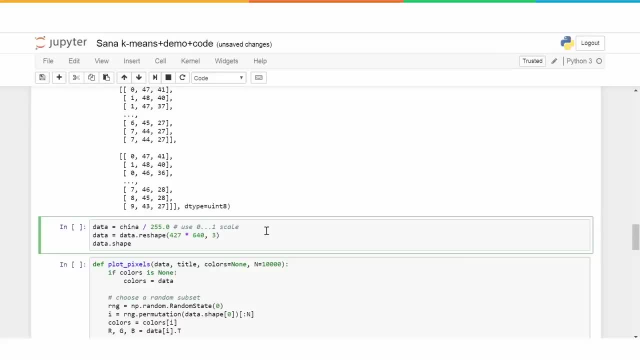 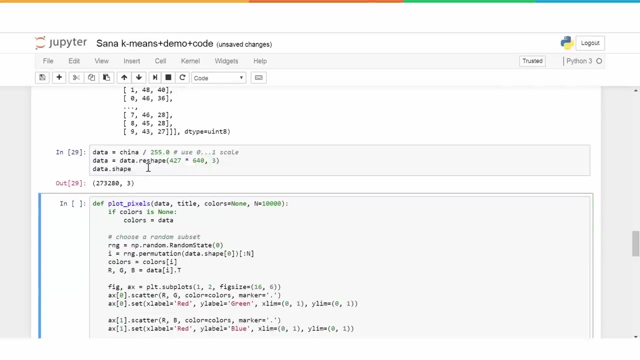 basically create one more variable, which is data, which will contain the values between 0 and 1, and the way to do that is divide by 255. so we divide china by 255 and we get the new values in data. so let's just run this piece of code and this is the shape. so we now have also. yeah, what we have. 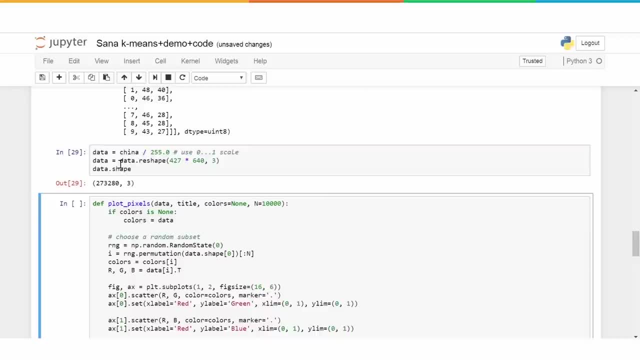 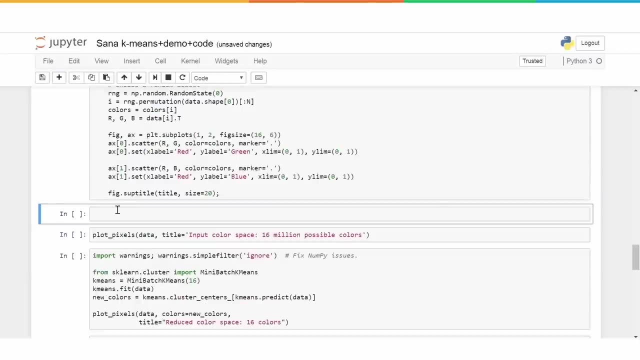 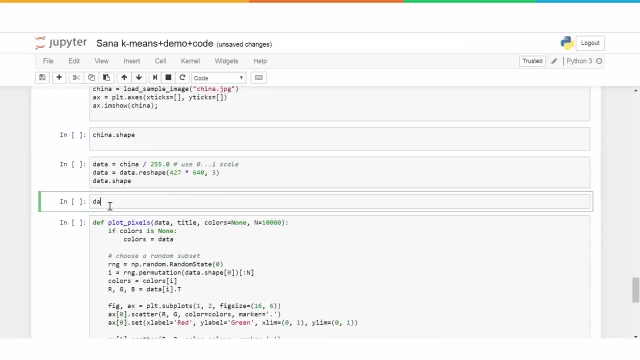 done is we changed, using reshape, we convert it into the three-dimensional, into a two-dimensional data set, and let us also take a look at how. let me just insert, probably, a cell here and take a look at how data is looking. all right, so this is how data is looking and now you see, this is the 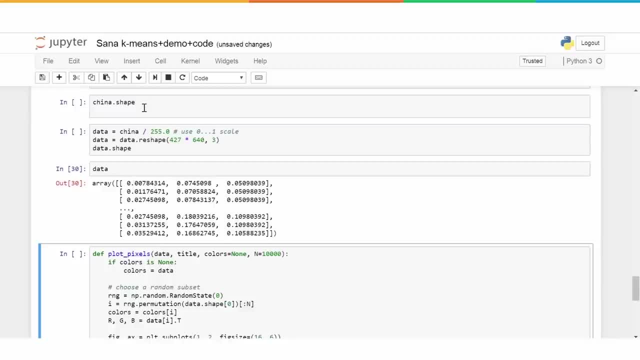 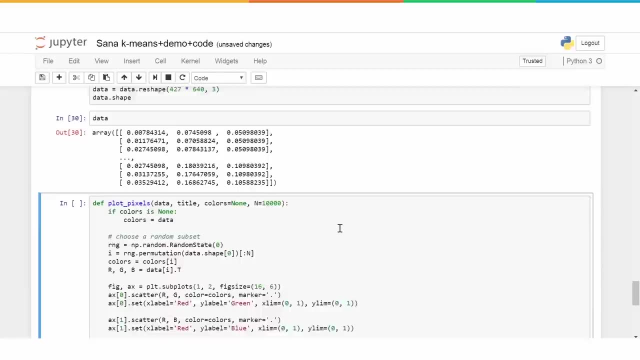 values are the values of the data. so let's just take a look at how data is looking. and now you are between 0 and 1, right? so if you earlier noticed, in case of china the values were large numbers. now everything is between 0 and 1. this is one of the things we need to do, all right? so 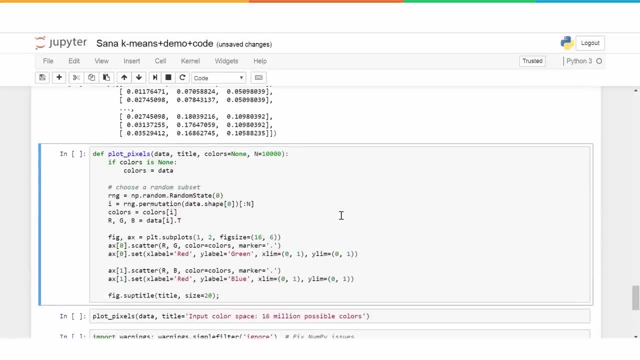 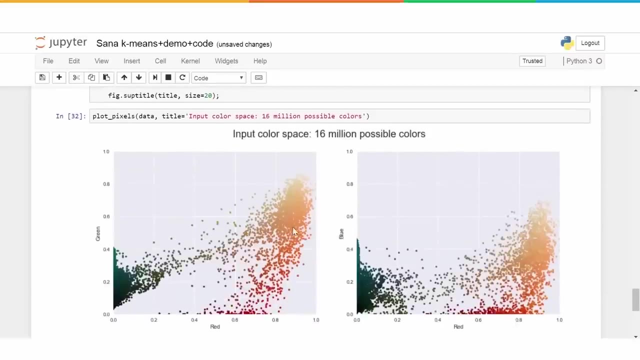 after that, the next thing that we need to do is to visualize this, and we can take random set of maybe 10 000 points and plot it and check and see how this looks. so let us just plot this, and so this is how the original, the color, the pixel distribution. 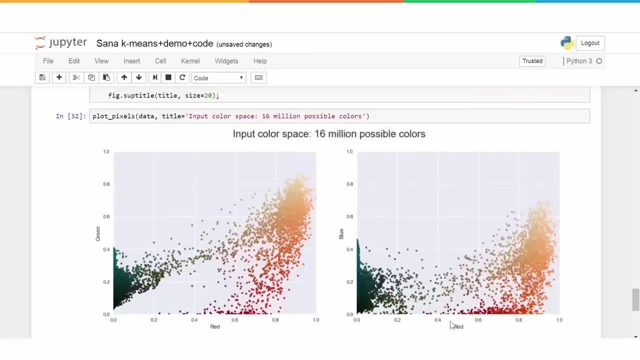 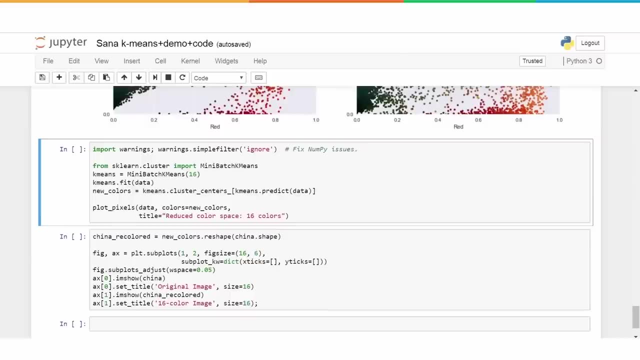 is, these are two plots: one is red against green and another is red against blue, and this is the original distribution of the color. so, then, what we will do is we will use k-means clustering to create just 16 clusters for the various colors, and then apply that to the image. now what will? 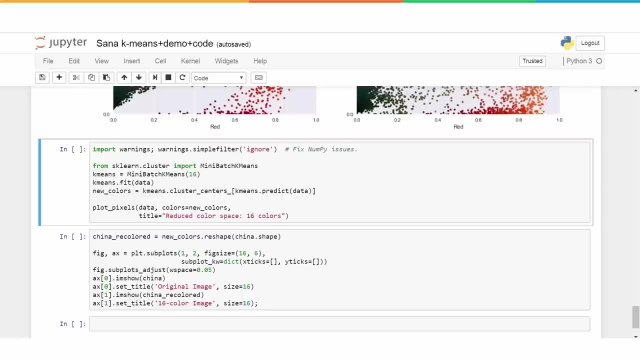 happen is, since the data is large, because there are millions of colors, using regular k-means may be a little time consuming, so there is another version of k-means which is mini batch k-means, so we will use that, which is which processes in the overall concept remains. 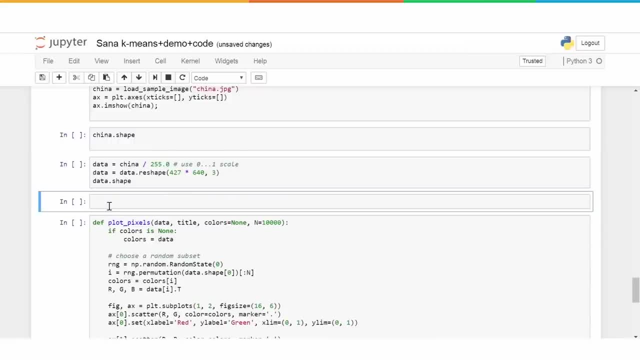 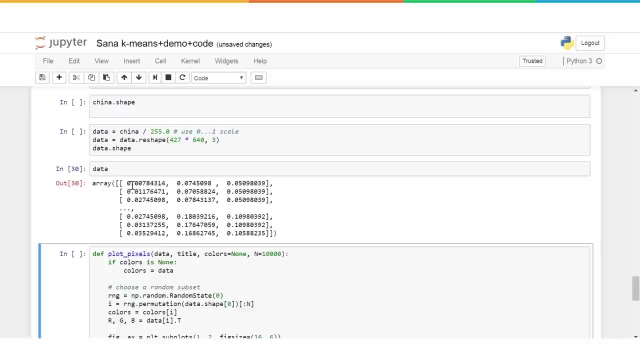 probably a cell here- and take a look at how data is looking. So this is how data is looking, And now you see, this is the values are between zero and one, right. So if you earlier noticed, in case of China, the values were large numbers. Now everything is between zero and one. this is one. 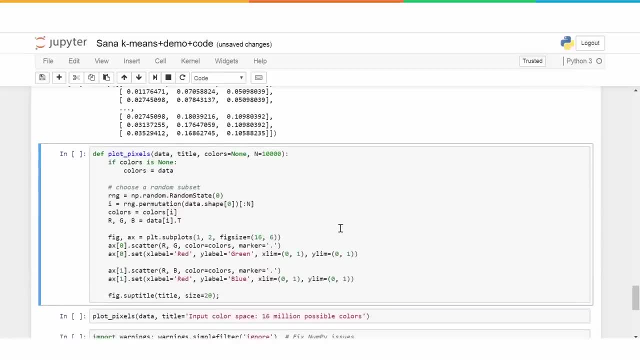 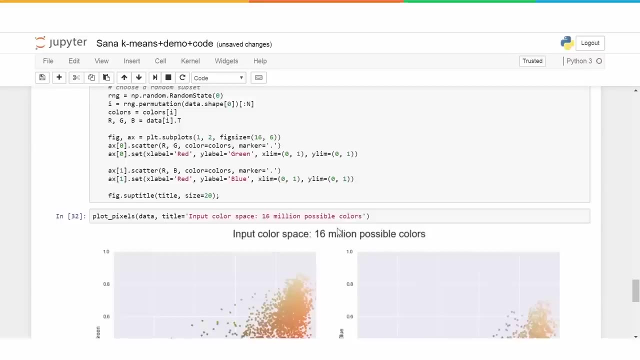 of the things we need to do. Alright, so after that, the next thing that we need to do is to visualize this, And we can take random set of maybe 10,000 points and plot it and check and see how this looks. So let us just plot this, And so this is how. 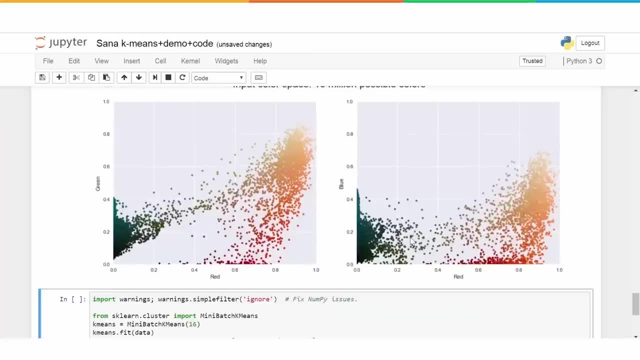 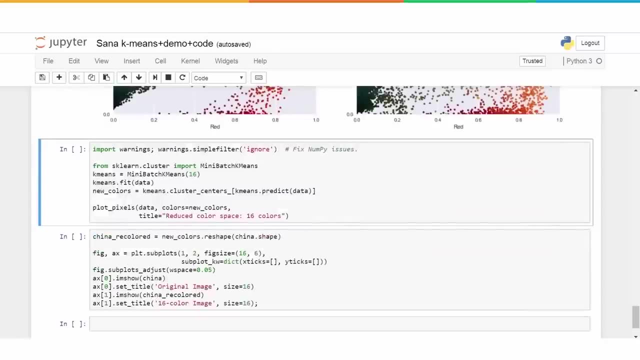 the original the color. the pixel distribution is: these are two plots: one is red against green and another is red against blue, And this is the original distribution of the color. So, then, what we will do is we will use k means clustering- to create just 16 clusters for the various colors. 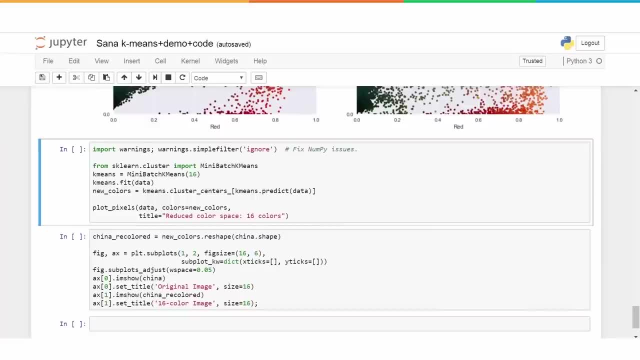 and then apply that to the image. Now what will happen is, since the data is large, because there are millions of colors- using regular k means maybe a little time consuming, So there is another version of k means which is called mini batch k means, So we will use that. 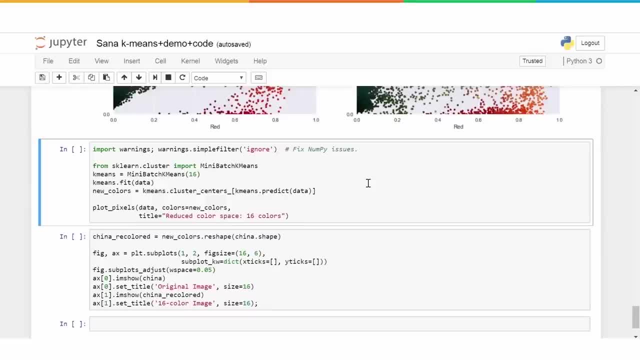 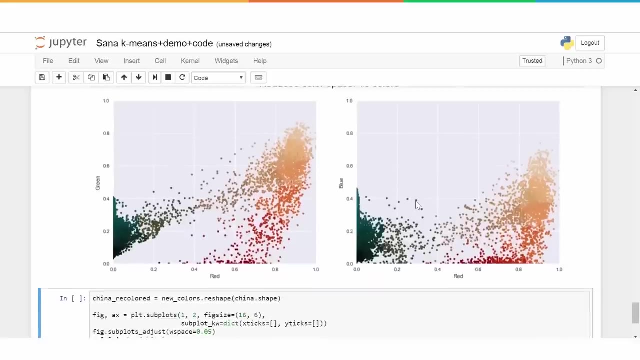 which is which processes in the overall concept remains the same, but this basically processes it in smaller batches. That's the only thing, okay, so the results will pretty much be the same. So let's go ahead and execute this piece of code and also visualize this so that we can see that there 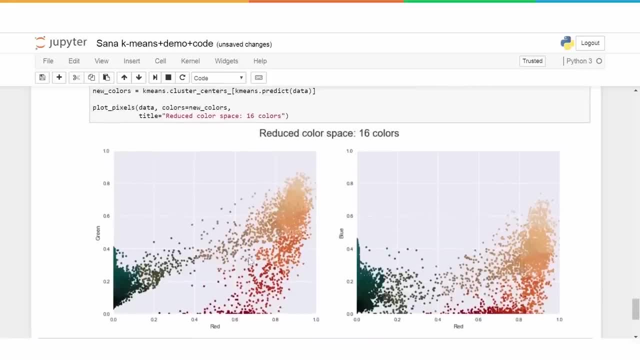 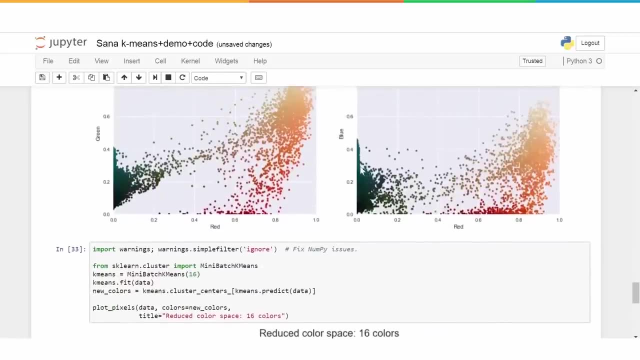 are these. this is how the 16 colors would look. So this is red against green, and this is red against blue, And this is red against green, And this is red against blue And this is red against blue. There is quite a bit of similarity between this original color schema and the new one. 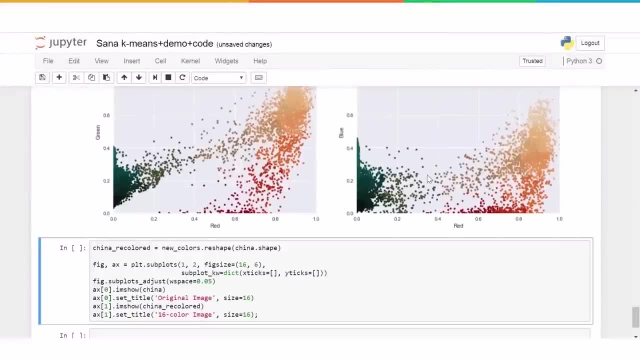 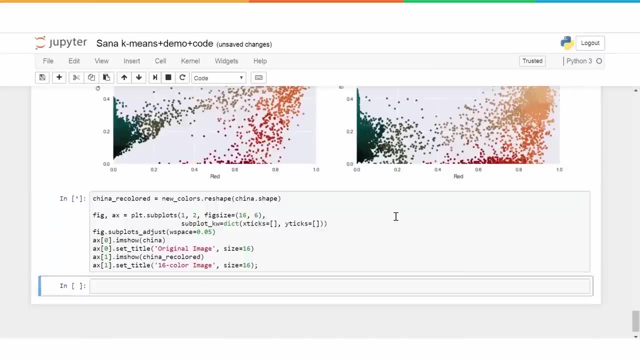 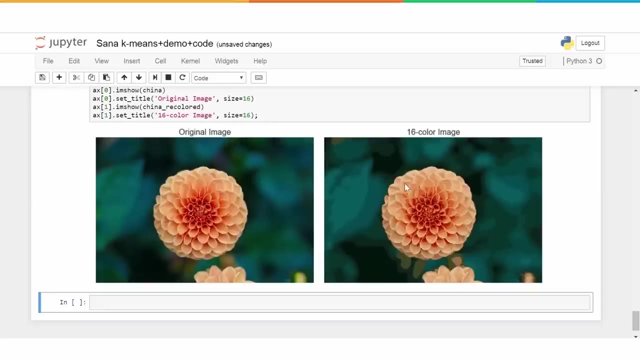 right, So it doesn't look very, very completely different or anything like that. Now we apply this- the newly created colors- to the image And we can take a look how this is looking. now we can compare both the images. So this is our original image and this is our new image. So, as you can, 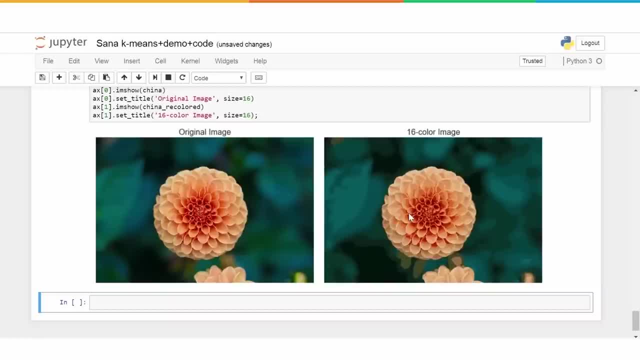 see there is not a lot of information that has been lost. It pretty much looks like the original image. Yes, we can see that. for example, here there is a little bit. it appears a little dullish compared to this one, right, because we kind of took off some. 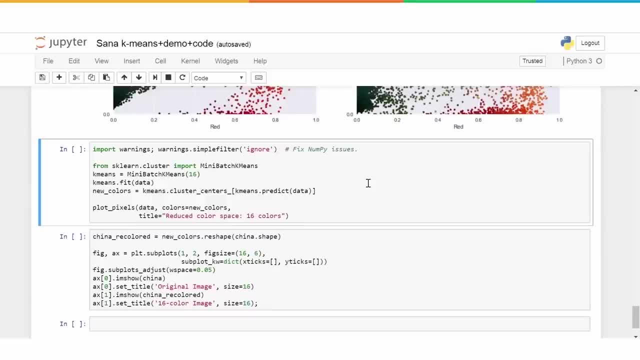 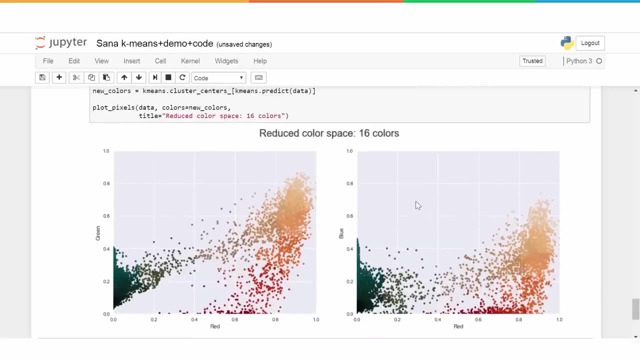 the same, but this basically processes it in smaller batches. that's the only thing, okay, so the results will pretty much be the same. so let's go ahead and execute this piece of code and also visualize this so that we can see that there are these. this is how the 16 colors, uh, would look. 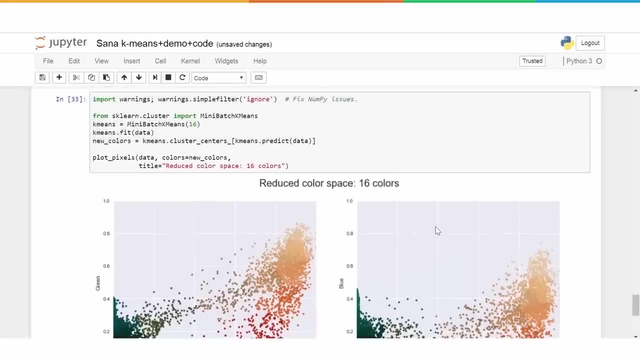 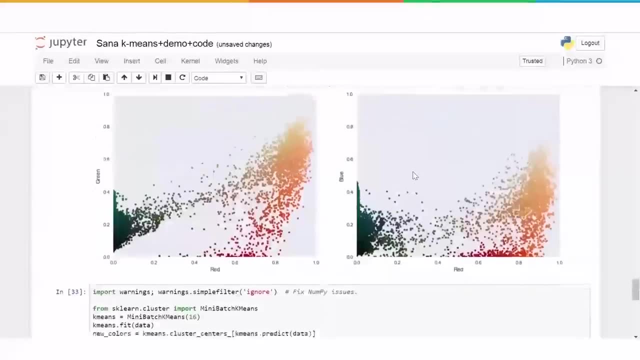 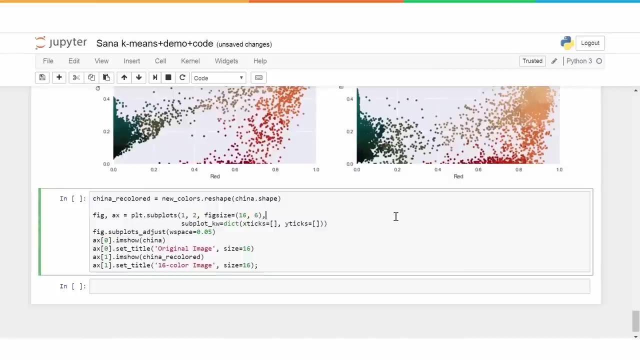 so this is red against green and this is red against blue. there is, uh, quite a bit of similar clarity between this original color schema and the new one, right, so it doesn't look very, very completely different, or anything like that. now we apply this- the newly created colors- to the image. 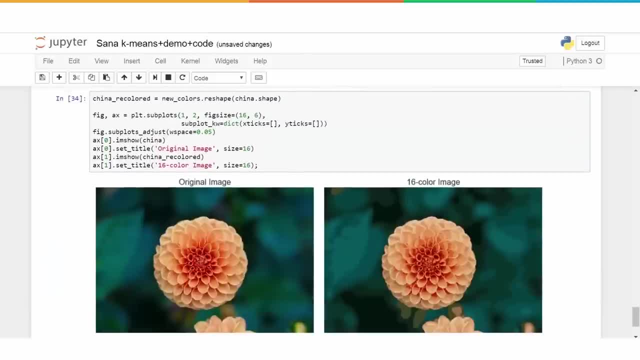 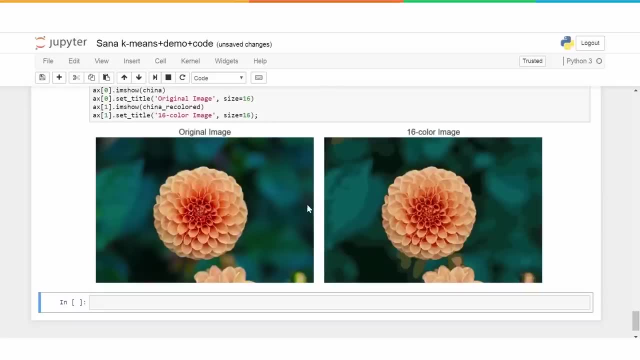 and we can take a look how this is looking. now we can compare both the images. so this is our original image and this is our new image. so, as you can see, there is not a lot of information that has been lost. it pretty much looks like the original. 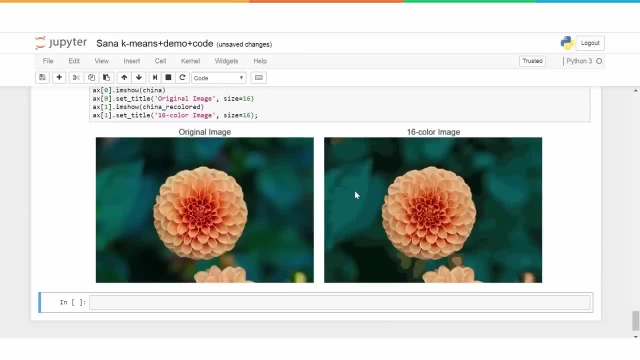 image. yes, we can see that, for example, here there is a little bit. it appears a little dullish compared to this one right, because we kind of took off some of the finer details of the color, but overall the high level information has been maintained. at the same time, the main advantage is that now this can. 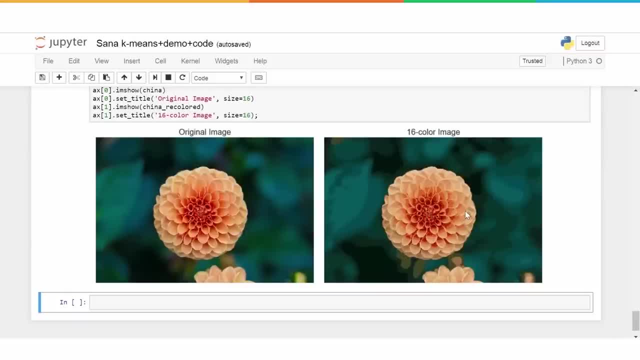 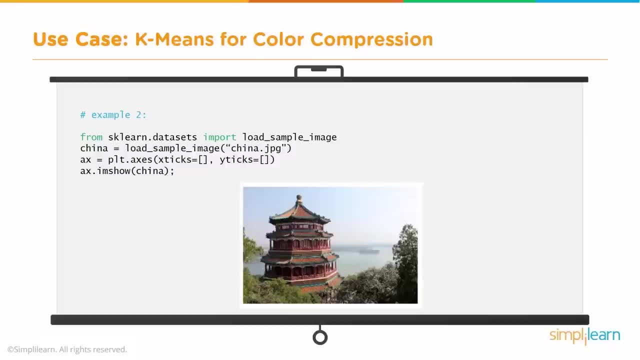 be. this is an image which can be rendered on a device which may not be that very sophisticated. now let's take one more example with a different image. in the second example, we will take an image of the summer palace in china and we repeat the same process. this is a high definition color image with millions of colors. 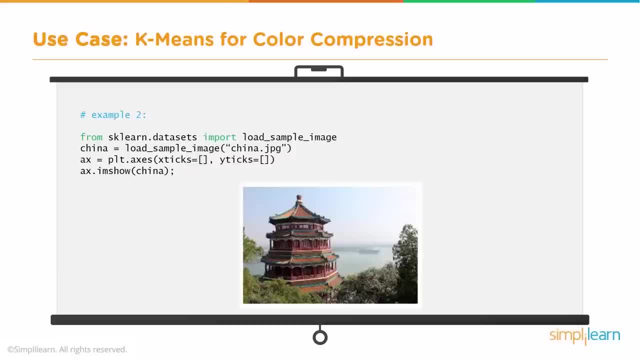 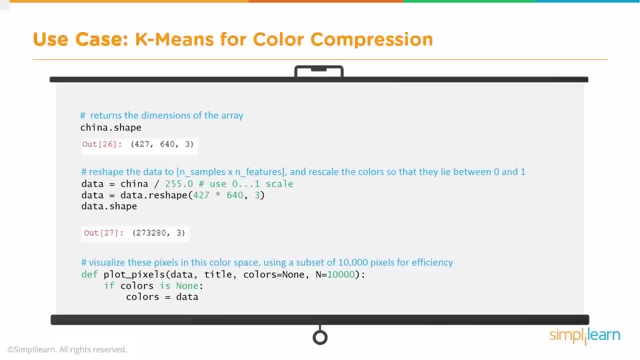 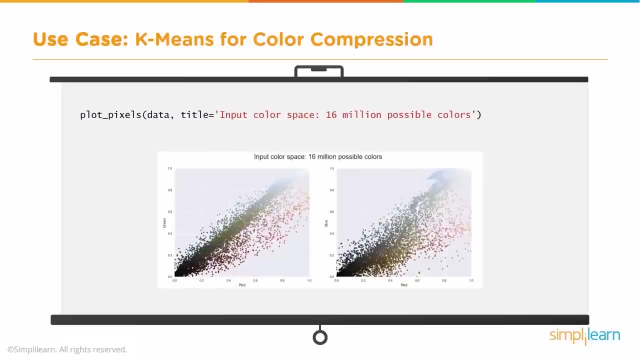 and also three-dimensional. now we will reduce that to 16 colors, using k-means clustering, and we do the same process like before. we reshape it and then we cluster the colors to 16, we render the image once again and we will see that the color, the quality of the image, 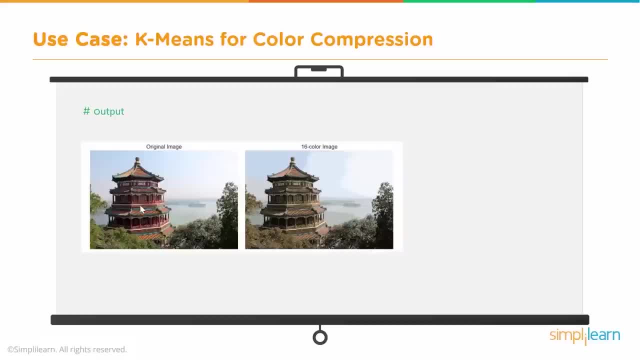 slightly deteriorates, as you can see here. this has much finer details in this which are probably missing here, but then that's the compromise, because there are some devices which may not be able to handle this kind of high density images. so let's run this code in python notebook. 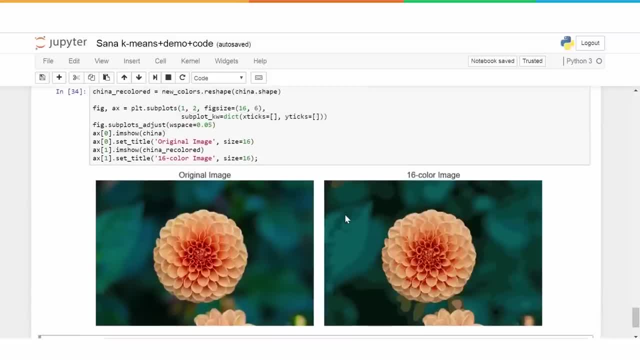 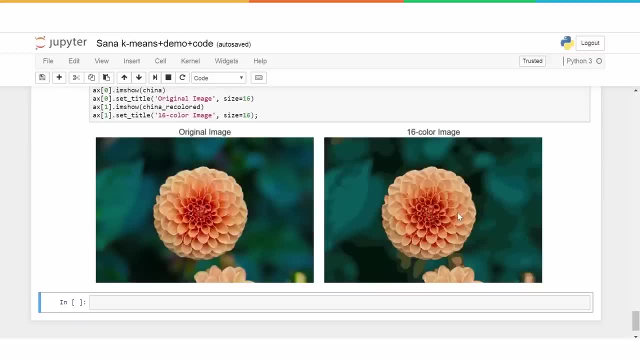 of the finer details of the color, But overall the high level information has been maintained. At the same time, the main advantage is that now this can be. this is an image which can be rendered on a device which may not be that very sophisticated. 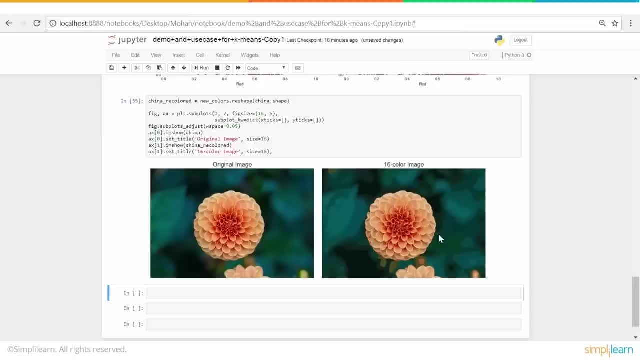 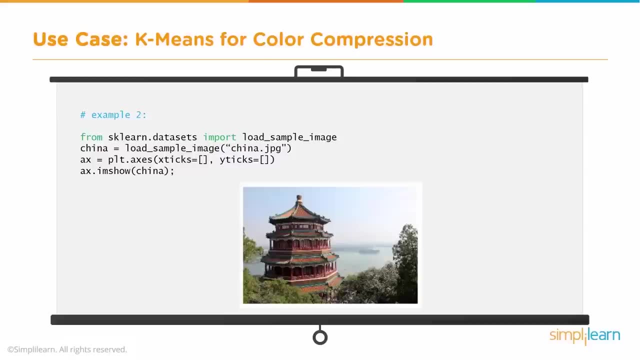 Now let's take one more example with a different image. In the second example, we will take an image of the Summer Palace in China And we repeat the same process. This is a high definition color image with millions of colors and also three dimensional. Now we will reduce that to 16 colors. 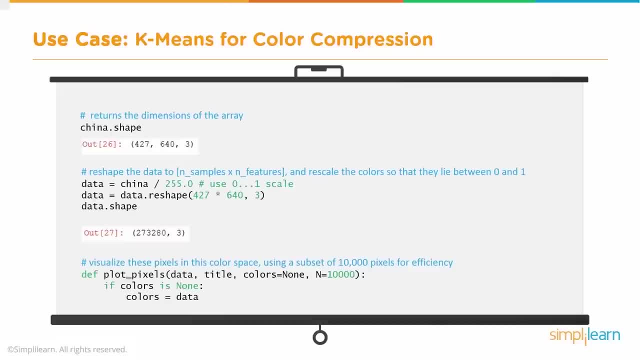 using k-means clustering. And we do the same process like before: we reshape it, and then we cluster it. And then we do the same process like before: we reshape it, And then we cluster it, And then we. And then we do the same process like before: we reshape it, And then we cluster it, And then we. 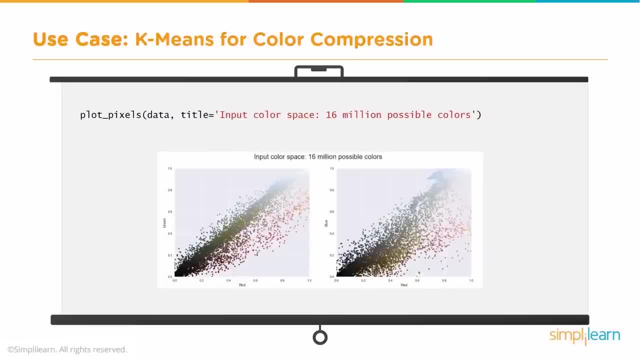 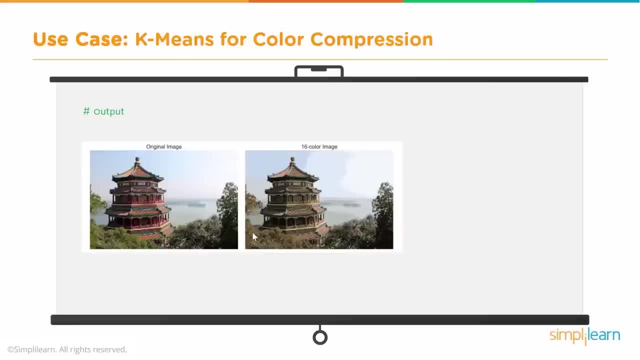 cluster the colors to 16.. And then we render the image once again And we will see that the color, the quality of the image slightly deteriorates. As you can see here, this has much finer details in this which are probably missing here. But then that's the compromise, because there are some. 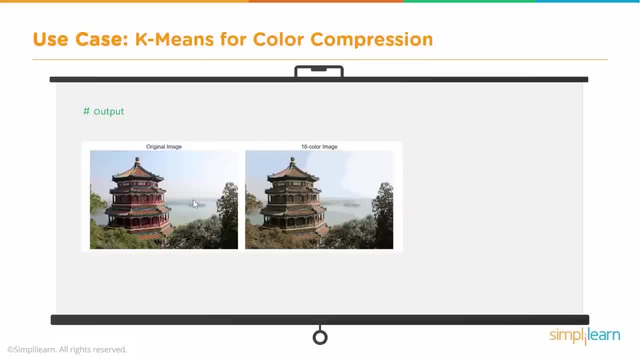 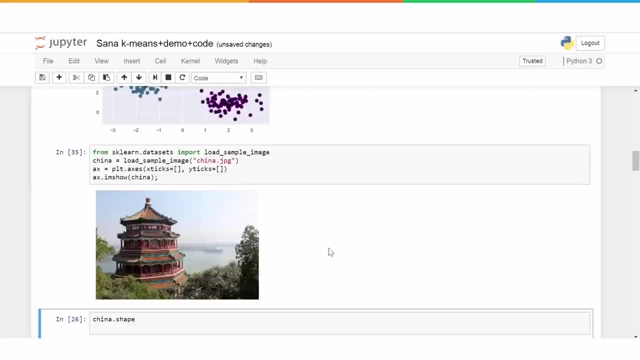 devices which may not be able to handle this kind of high density images. So let's run this code in Python notebook. Alright. so let's apply the same technique for another picture which is even more intricate and has probably much complicated color schema. So this is the image. Now, once again, we can take a look. 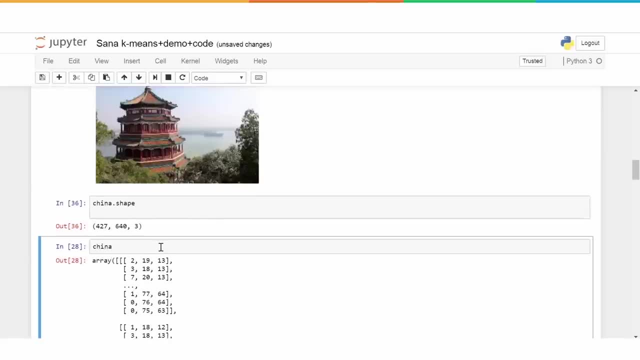 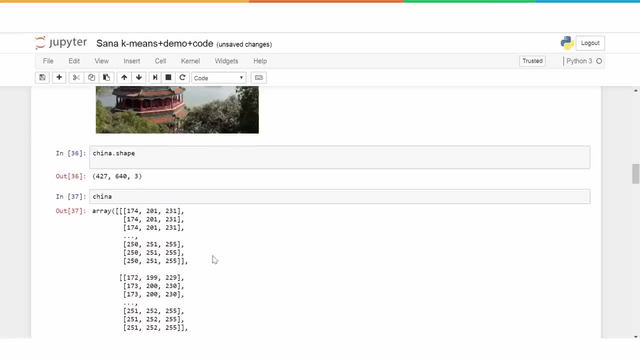 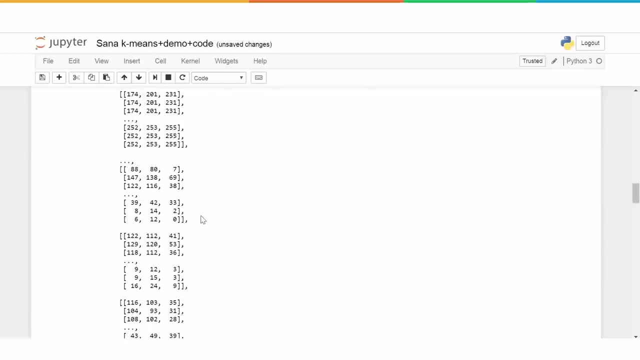 at the shape, which is 427 by 640 by three- And this is a new data- would look somewhat like this compared to the flower image. So we have some new values here And we will also bring this. as you can see, the numbers are much big, so we will have much bigger, So we will now. 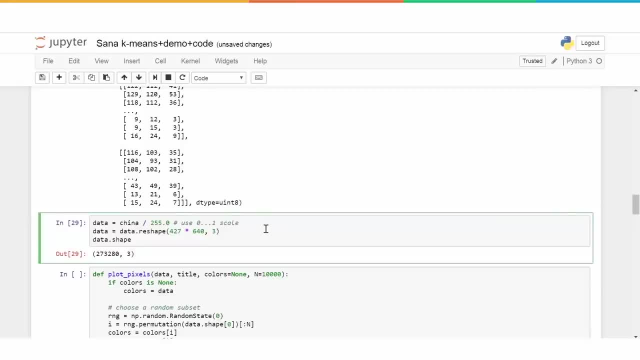 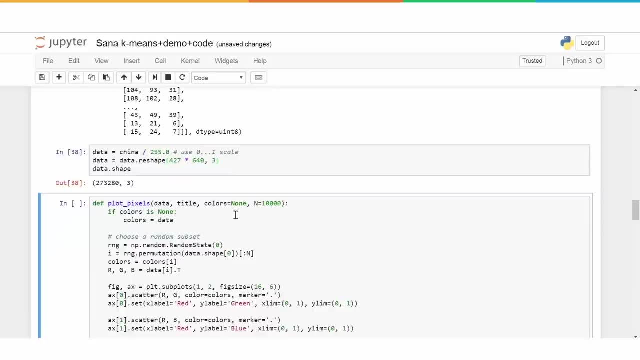 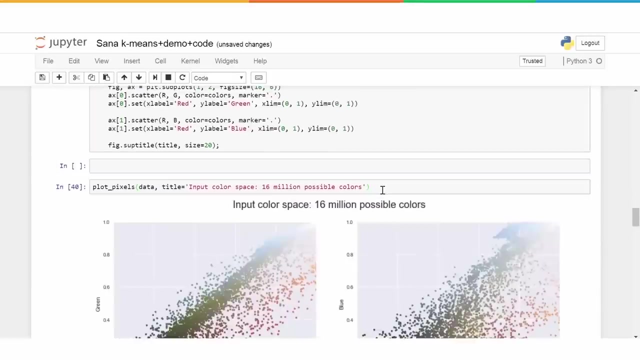 have to scale them down to values between zero and one, And that is done by dividing by 255.. So let's go ahead and do that And reshape it. Okay, so we get a two dimensional matrix And we will then, as a next step, we will go ahead and visualize this how it looks. There's the 16 colors And 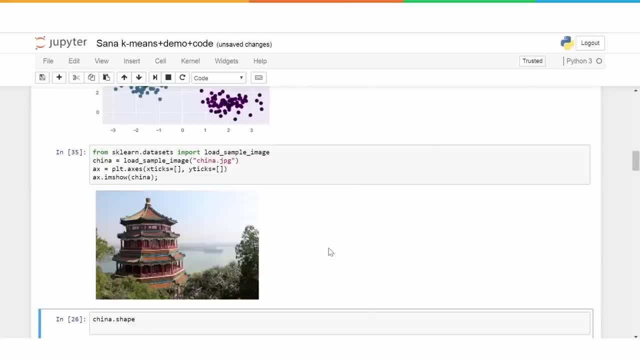 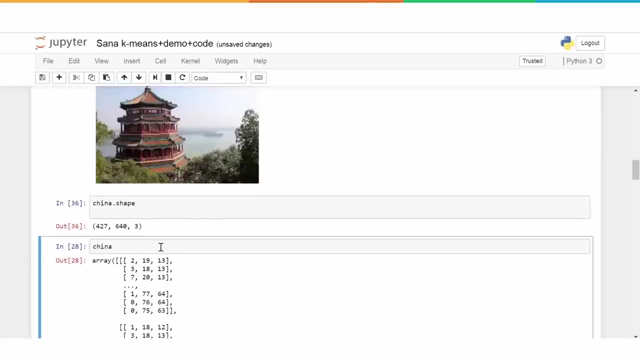 all right. so let's apply the same technique for another picture which is even more intricate and has probably much complicated color schema. so this is the image. now, once again, we can take a look at the shape, which is 427 by 640 by 3, and this is the new data. would look somewhat like this compared to the flower image. so we 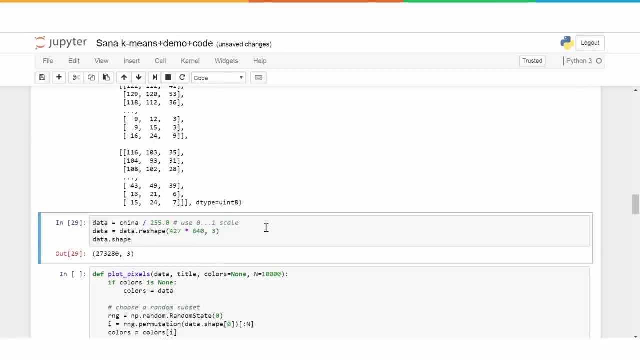 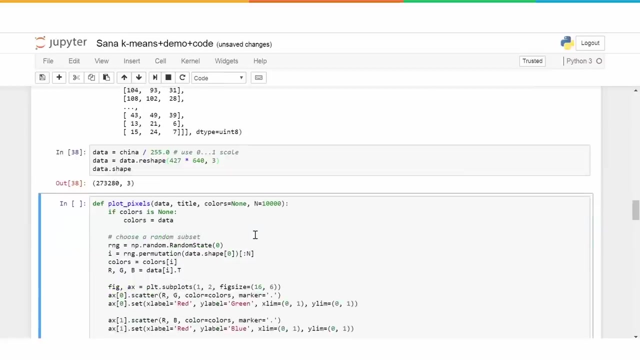 have some new values here and we will also bring this. as you can see, the numbers are much big, it's a much bigger, so we will now have to scale them down to values between 0 and 1, and that is done by dividing by 255. so let's go ahead and do that and reshape it. okay, so we get a two-dimensional matrix. 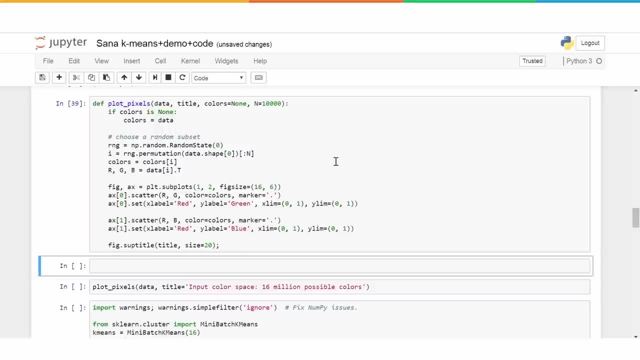 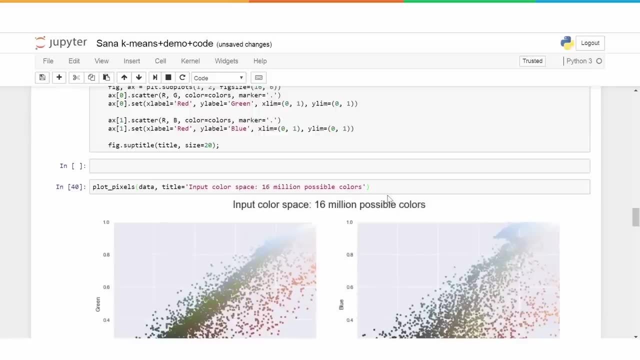 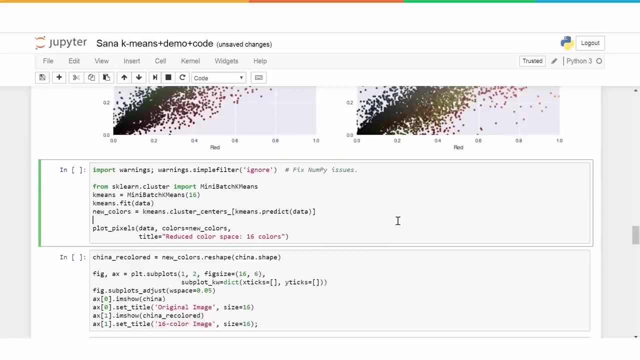 and we will then, as a next step, we will go ahead and visualize this how it looks, the 16 colors and this is basically how it would look, 16 million colors, and now we can create the clusters out of this, the 16 k-means clusters we will create. so this is how. 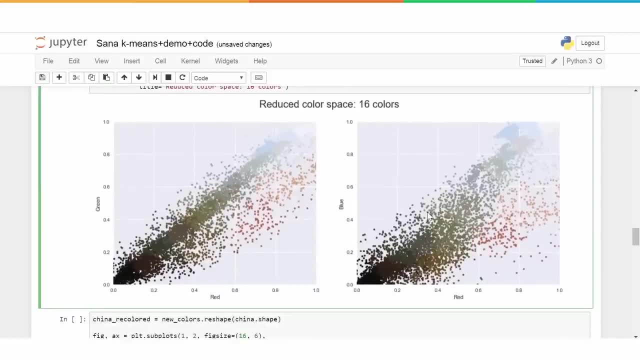 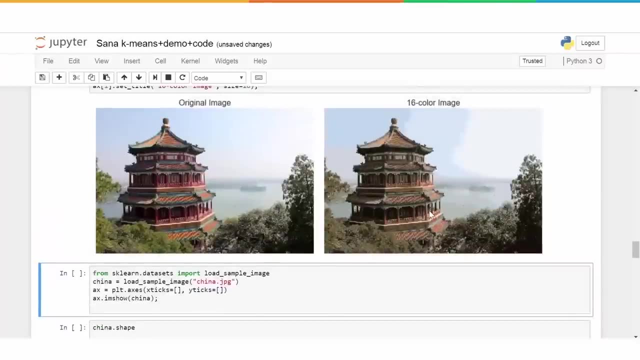 the distribution of the pixels would look with 16 colors, and then we go ahead and apply this and visualize how it is looking for with the new, just the 16 color. so, once again, as you can see, this looks much richer in color but at the same time- and this probably doesn't have, as we can see- it doesn't look as rich. 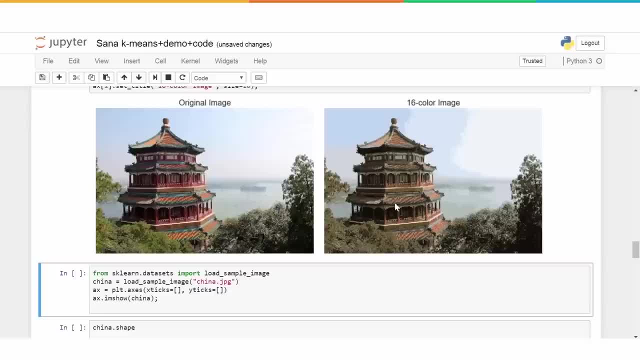 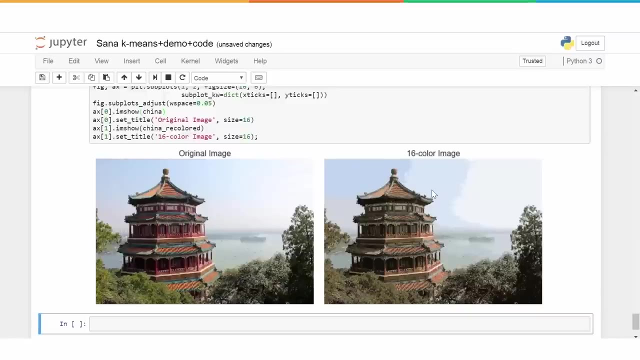 as this one, but nevertheless the information is not lost- the shape and all that stuff, and this can be also rendered on a slightly a device which is probably not that sophisticated. okay, so that's pretty much it. so we have seen two examples of how color compression can be done using k-means. 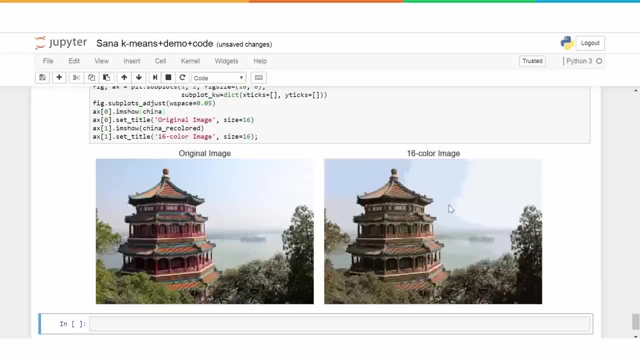 clustering and we have worked on a number of different cases of color compression and we have have also seen in the previous examples of how to implement k-means, the code to roughly how to implement k-means clustering and we use some sample data using blob to just execute the k-means. 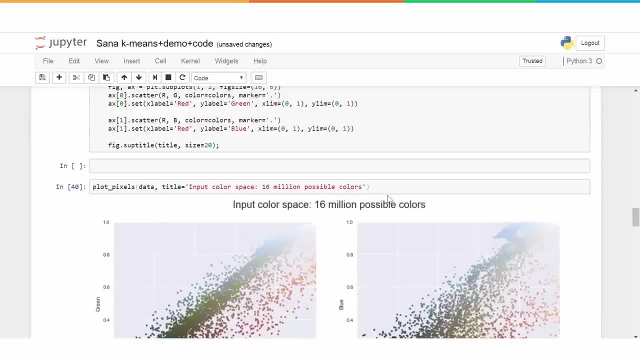 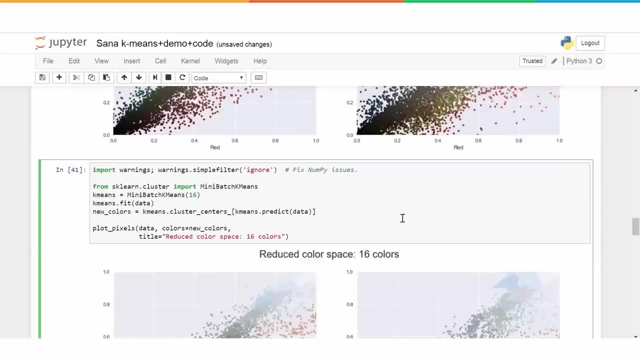 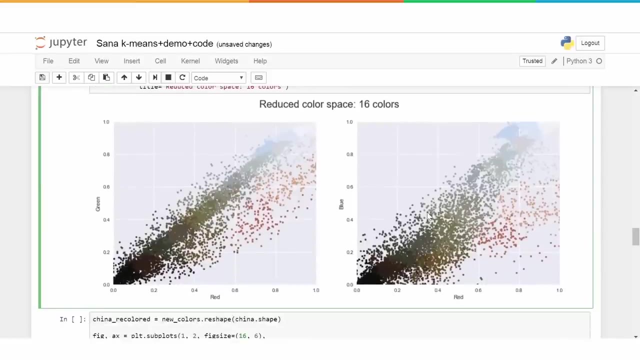 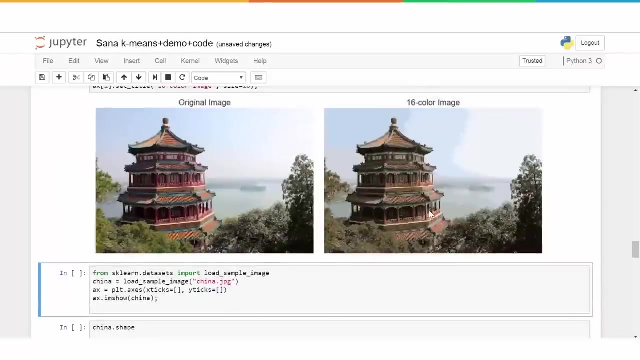 this is basically how it would look: 16 million colors, and Now we can create the clusters out of this. the 16 k means clusters we will create. So this is how the distribution of the pixels would look with 16 colors, And then we go ahead and apply this and visualize how it is looking. 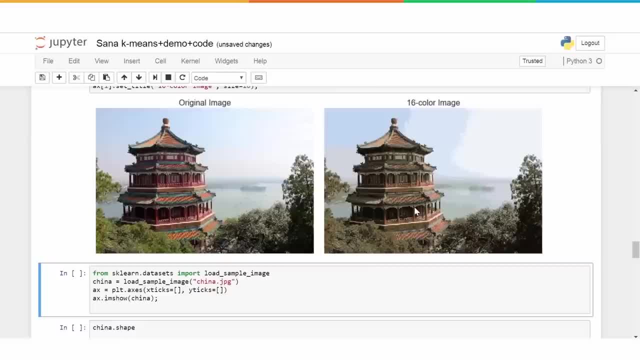 for, with the new, just the 16 colors. Again, as you can see, this looks much richer in color but at the same time- and this probably doesn't have, as we can see- it doesn't look as rich as this one. 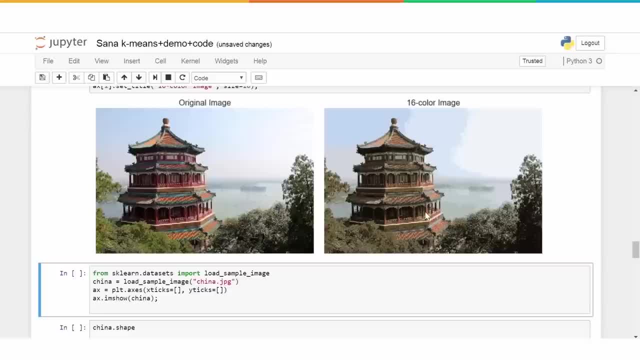 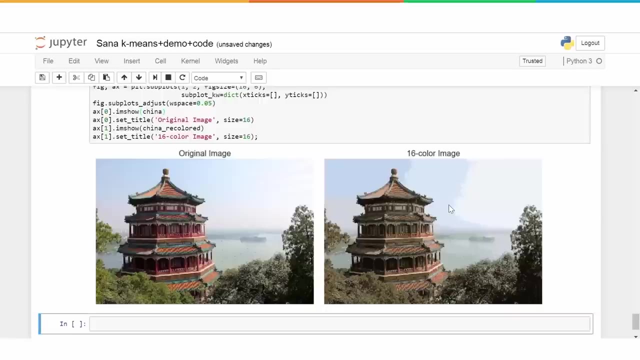 But nevertheless, the information is not lost. the shape and all that stuff, And this can be also rendered on a slightly a device which is probably not that sophisticated. Okay, so that's pretty much it. So we have seen two examples of how color compression can be done using k-means clustering. 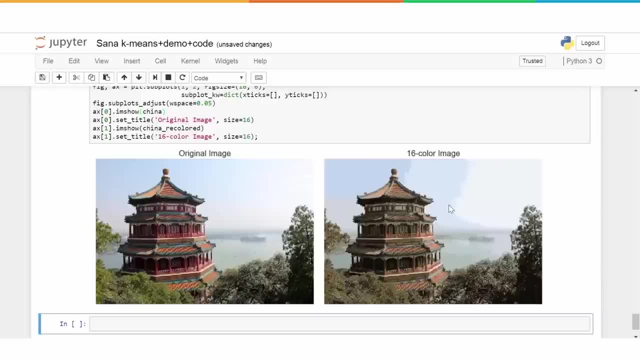 And we have also seen in the previous examples of how to implement k-means, the code to roughly how to implement k-means clustering And we use some sample data using blob to just execute the k-means clustering. Thank you, Mohan. 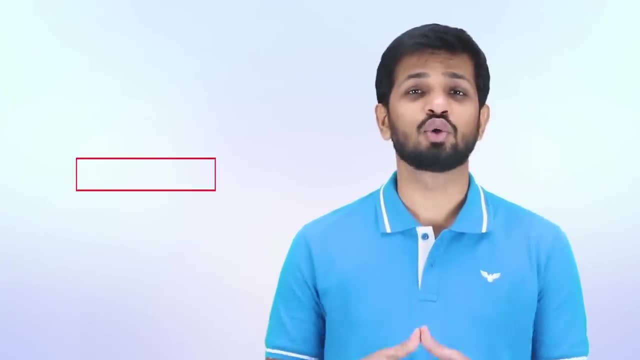 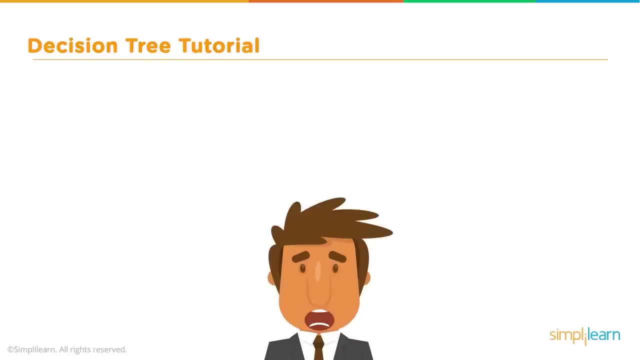 That was really informative. Now on to Richard, to help you learn more algorithms. So the decision tree, one of the many powerful tools in the machine learning library, begins with a problem. I think I have to buy a car. So in making this question, you want to go. how do I decide which one to buy? 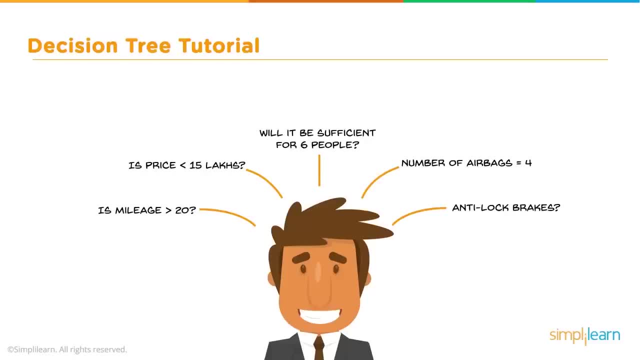 And you're going to start asking questions: Is the mileage greater than 20?? Is the price less than 15?? Will it be sufficient for six people? Does it have enough airbags, Anti-lock brakes- All these questions come up Then, as we feed all this data in, we make a decision. 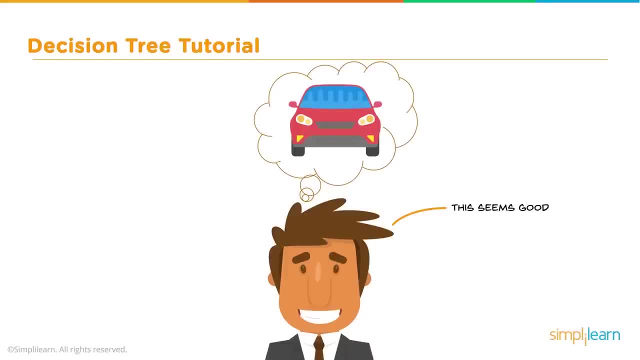 And that decision comes up: oh hey, this seems like a good idea. Here's a car, Here's a car, Here's this decision process using a decision tree. We're going to explore this, maybe not in buying a car, but in how to process data. 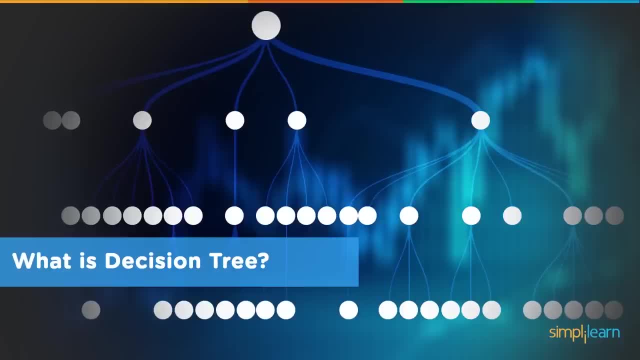 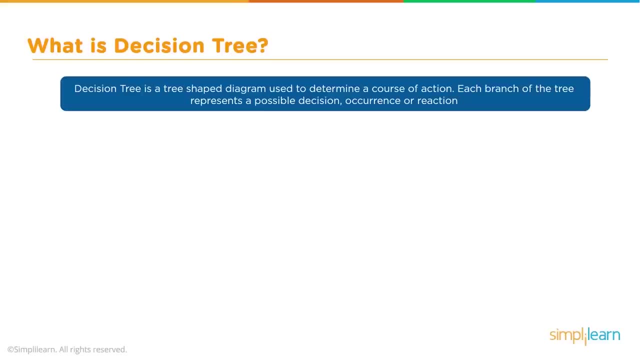 What is a decision tree? Let's go through a very simple example before we dig in deep. Decision tree is a tree-shaped diagram used to determine a course of action. Each branch of the tree represents a possible decision, occurrence or reaction. Let's start with a simple question. 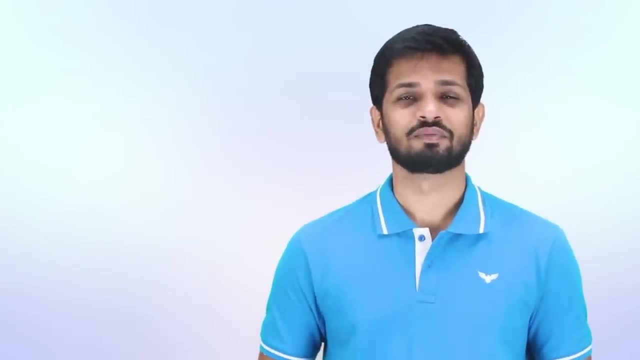 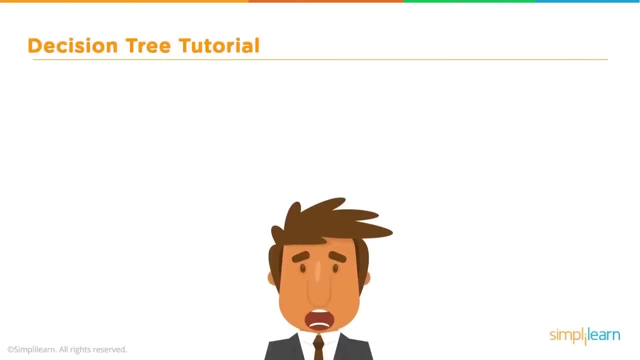 clustering. Thank you, Mohan, that was really informative. Now on to Richard, to help you learn more algorithms. So the decision tree, one of the many powerful tools in the machine learning library, begins with a problem. I think I have to buy a car. So in making this question, you want to know. 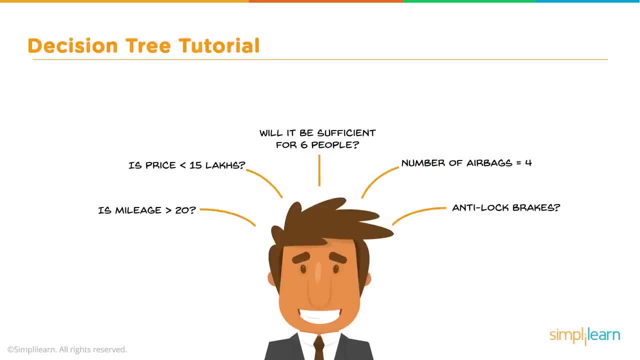 how do I decide which one to buy? and you're going to start asking questions: Is the mileage greater than 20? Is the price less than 15?? Will it be sufficient for six people? Does it have enough airbags, Anti-lock brakes? All these questions come up Then. as we feed all this data in, we make a 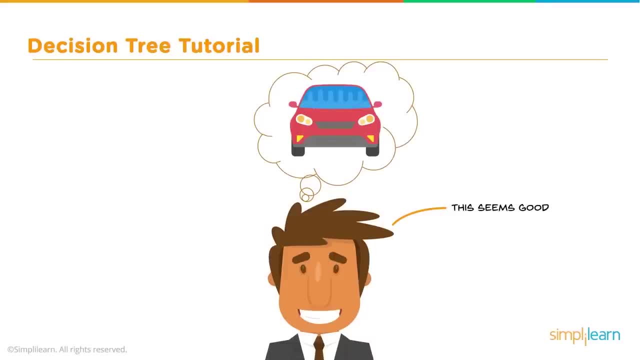 decision and that decision comes up: Oh hey, this seems like a good idea. Here's a car. So, as we go in through this decision process using a decision tree, we're going to explore this. maybe not in buying a car, but we're going to explore this in a decision tree. So we're going to explore this. 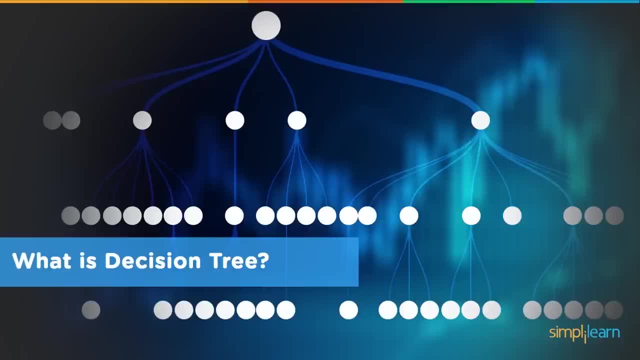 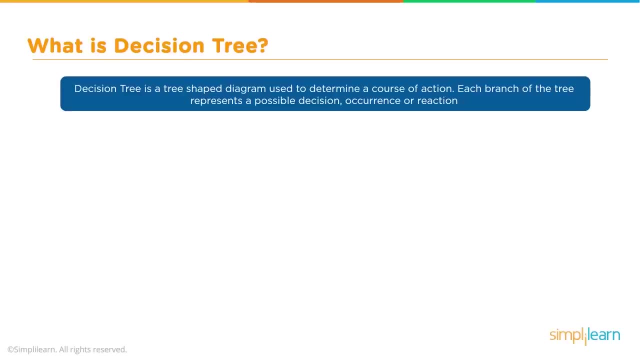 in how to process data. What is a decision tree? Let's go through a very simple example before we dig in deep. Decision tree is a tree-shaped diagram used to determine a course of action. Each branch of the tree represents a possible decision or occurrence or reaction. Let's start. 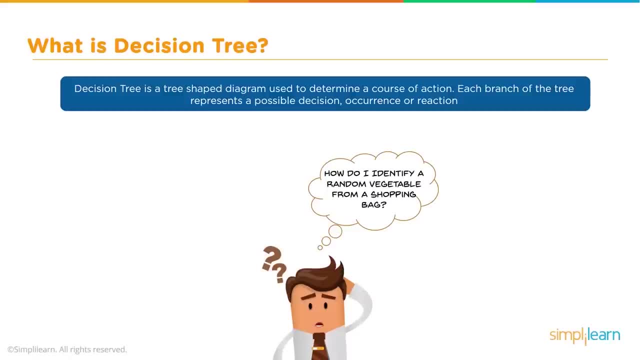 with a simple question: How to identify a random vegetable from a shopping bag. So we have this group of vegetables in here and we can start off by asking a simple question: Is it red? And if it's not, then it's going to be the purple fruit to the left, probably an eggplant. 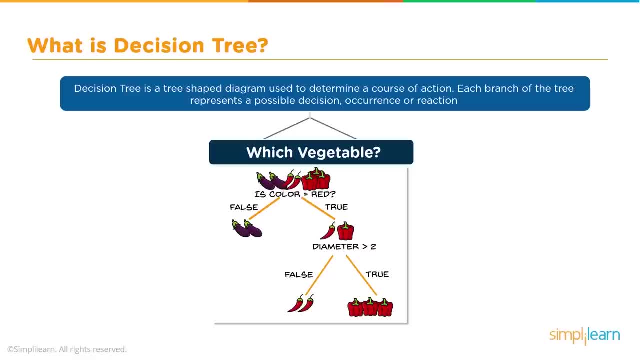 If it's true, it's going to be one of the red fruits. Is the diameter greater than two? If false, it's going to be a what looks to be a red chili, And if it's true, it's going to be a bell pepper. 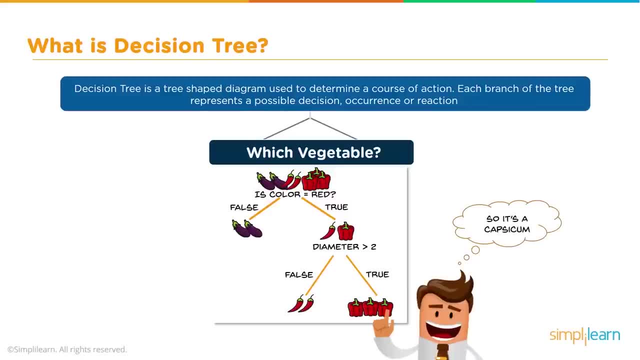 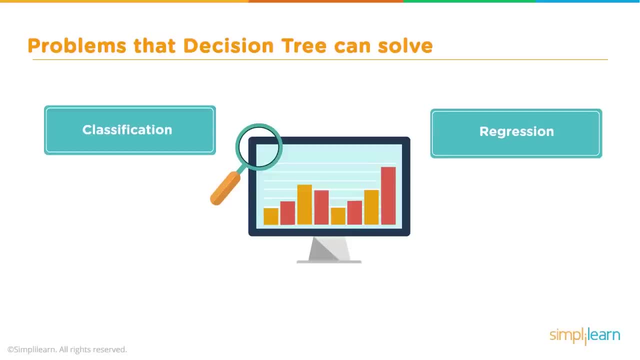 from the capsicum family, So it's a capsicum Problems that decision tree can solve. So let's look at the two different categories the decision tree can be used on. It can be used on the classification, the true, false, yes, no. and it can be used on regression, where we figure out what the 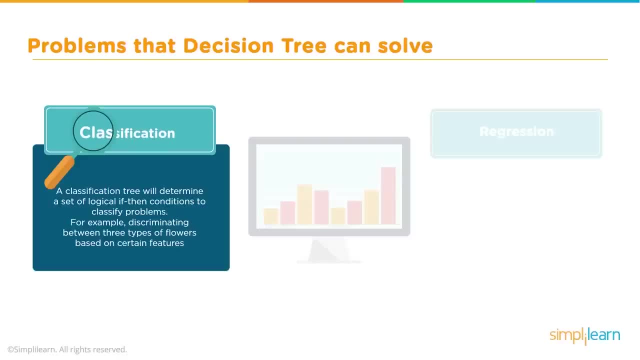 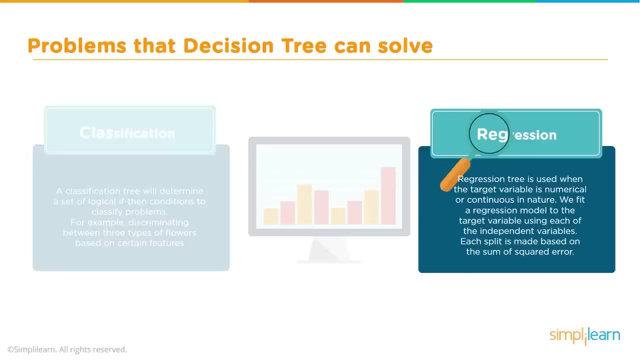 next value is in a series of numbers or a group of data. In classification, the classification tree will determine a set of logical, if then conditions to classify problems, For example, discriminating between three types of flowers based on certain features. In regression, a regression tree is used when the target variable is numerical. 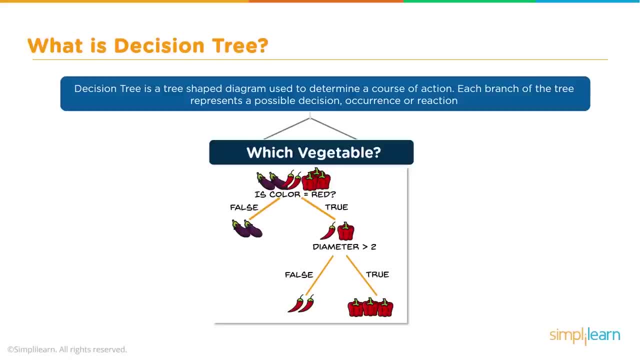 How do I identify a random vegetable from a shopping bag? So we have this group of vegetables in here And we can start off by asking a simple question: is it red? If it's not, then it's going to be the purple fruit to the left, probably an eggplant. 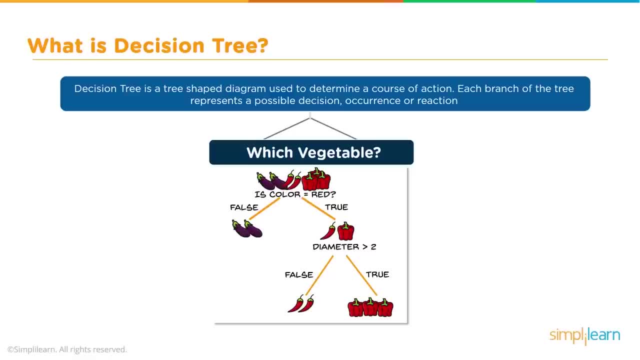 If it's true, it's going to be one of the red fruits. Is the diameter greater than two? If false, it's going to be what looks to be a red chili, And if it's true, it's going to be a bell pepper from the capsicum family. 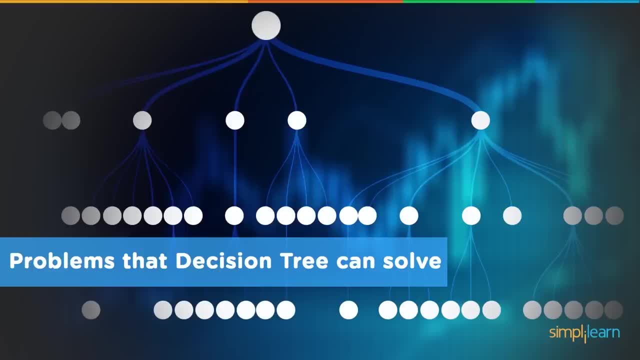 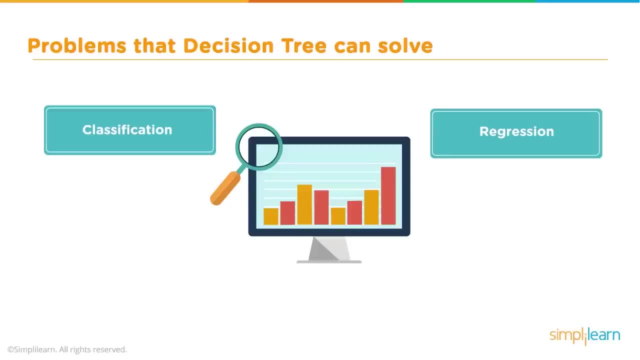 So it's a capsicum Problems that decision tree can solve. So let's look at the two different categories the decision tree can be used on. It can be used on the classification, the true, false, yes, no- And it can be used on regression. 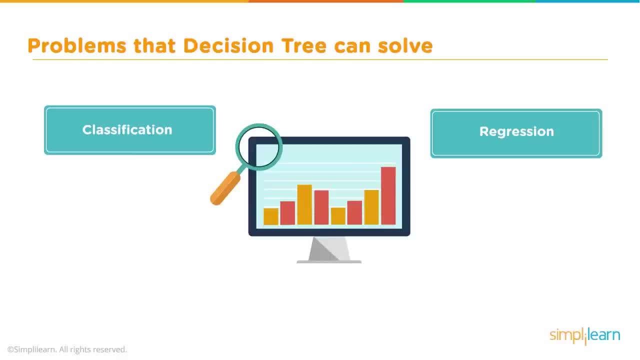 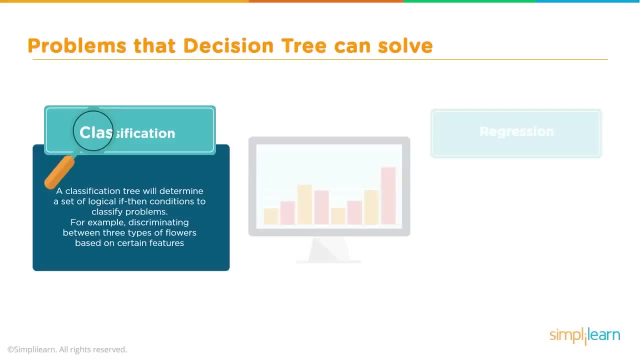 where we figure out what the next value is in a series of numbers or a group of data In classification. the classification tree will determine a set of logical if-then conditions to classify problems, For example, discriminating between three types of flowers based on certain features. 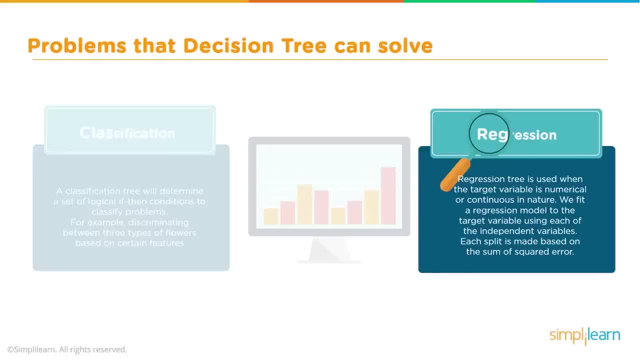 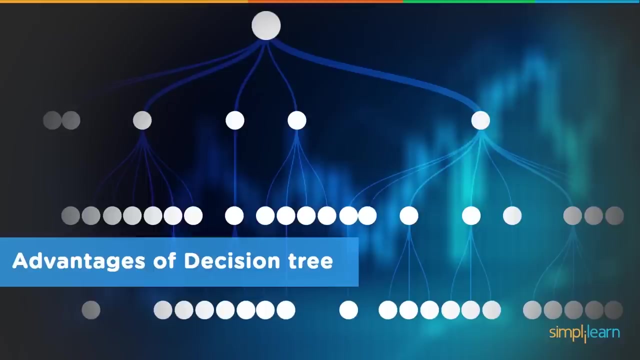 In regression. a regression tree is used when the target variable is numerical or continuous in nature. We fit the regression model to the target variable using each of the independent variables. Each split is made based on the sum of squared error. Before we dig deeper into the mechanics of the decision tree, 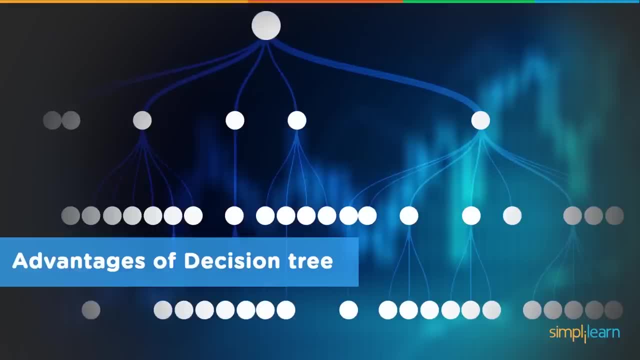 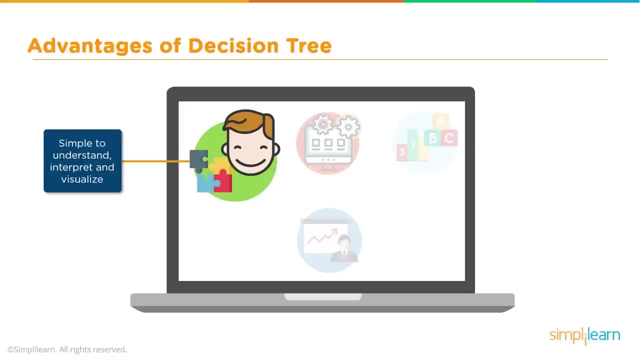 let's take a look at the advantages of using a decision tree And we'll also take a glimpse at the disadvantages. The first thing you'll notice is that it's simple to understand, interpret and visualize. It really shines here because you can see exactly what's going on in a decision tree. 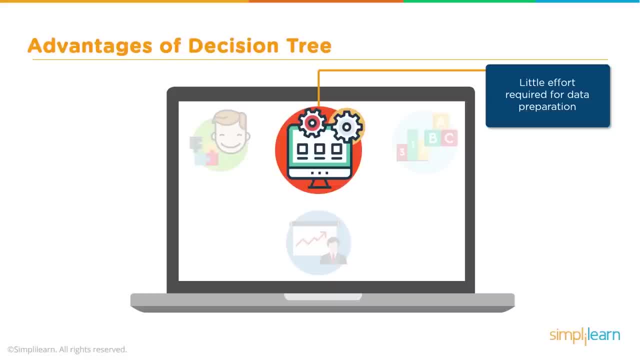 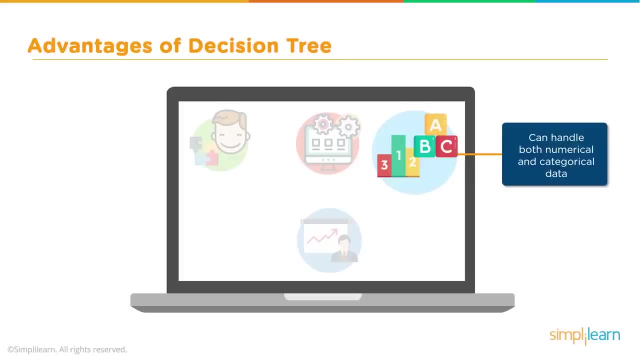 Little effort is required for data preparation, so you don't have to do special scaling. There's a lot of things you don't have to worry about when using a decision tree. It can handle both numerical and categorical data, as we discovered earlier. 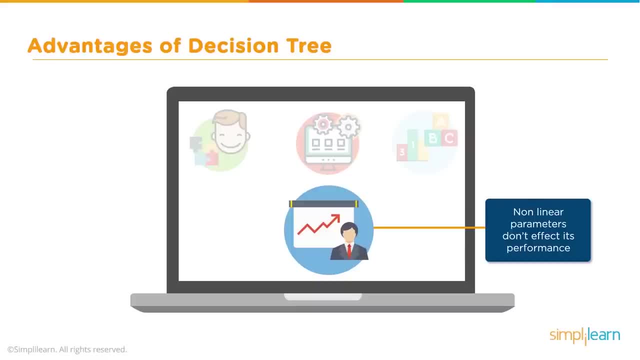 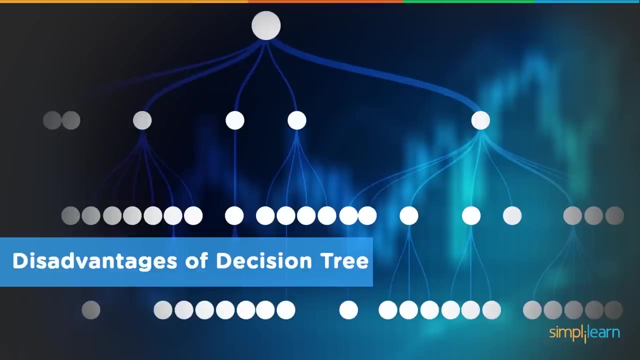 And nonlinear parameters don't affect its performance. So even if the data doesn't fit an easy curved graph, you can still use it to create an effective decision or prediction. If we're going to look at the advantages of a decision tree, we also need to understand the disadvantages of a decision tree. 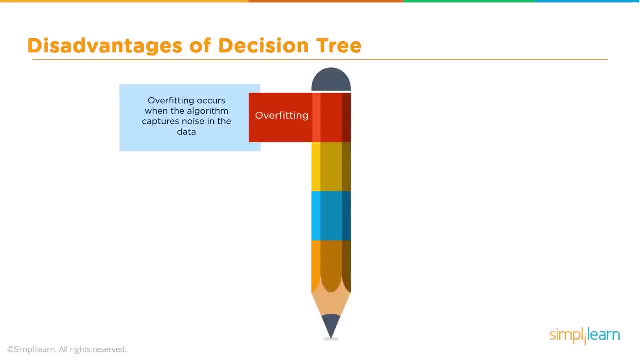 The first disadvantage is overfitting. Overfitting occurs when the algorithm captures noise in the data. That means you're solving for one specific instance instead of a general solution for all the data. High variance: The model can get unstable due to small variation in data. 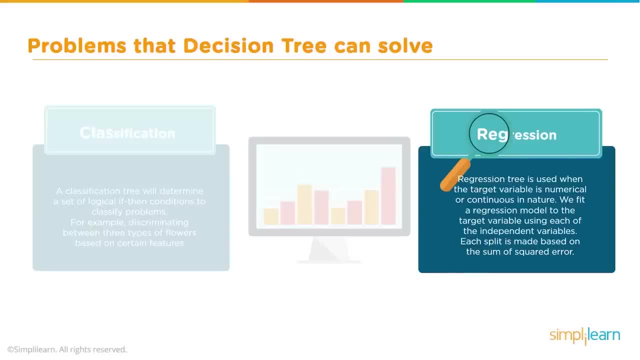 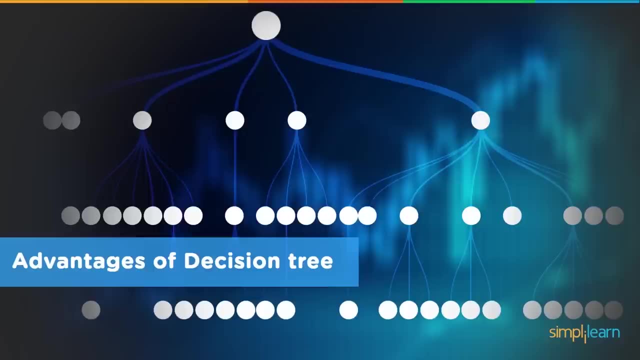 or continuous in nature. We fit the regression model to the target variable using each of the independent variables. Each split is made based on the sum of squared error. Before we dig deeper into the mechanics of the decision tree, let's take a look at the advantages of using a decision tree, and we'll also take a glimpse at the 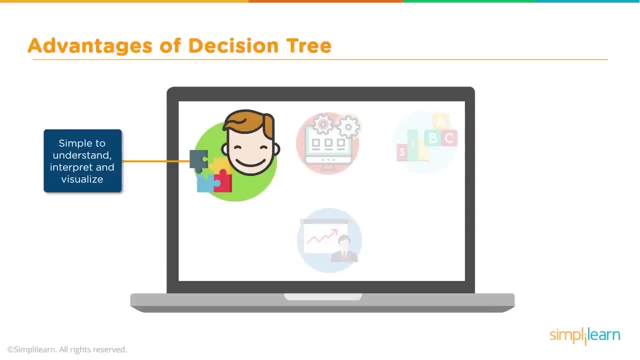 disadvantages. The first thing you'll notice is that it's simple to understand, interpret and visualize. It really shines here because you can see exactly what's going on in a decision tree. Little effort is required for data preparation, so you don't have to do special scaling. There's a lot of things you 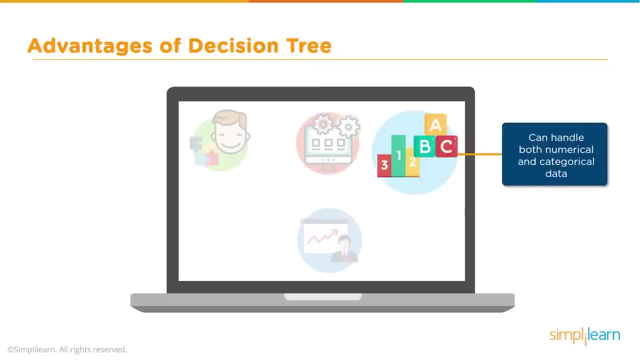 don't have to worry about when using a decision tree. It can handle both numerical and categorical data, as we discovered earlier, and non linear parameters don't affect its performance. So even if the data doesn't fit an easy curved graph, you can still use it to create an effective decision or prediction. 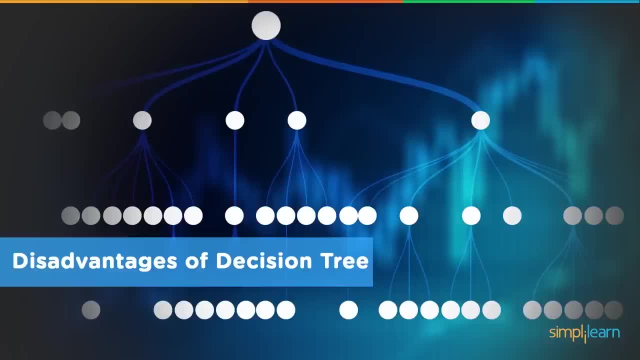 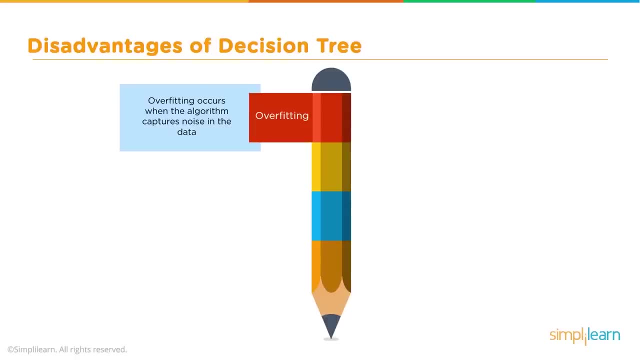 If we're going to look at the advantages of a decision tree, we also need to understand the disadvantages of a decision tree. The first disadvantage is overfitting. Overfitting occurs when the algorithm captures noise in the data. That means you're solving for one specific instance instead of a general solution for all the data. 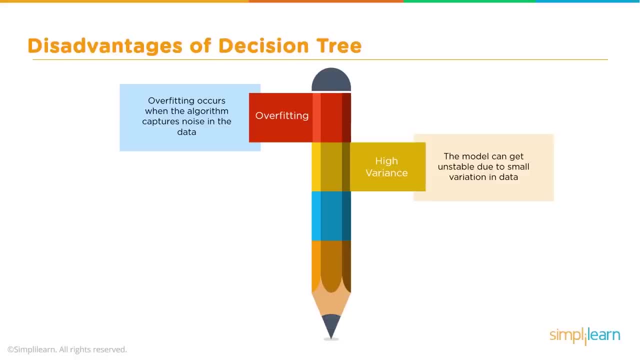 And this can lead to a small variation in the model. High variance: The model can get unstable due to small variation in data. Low bias tree: A highly complicated decision tree tends to have low bias, which makes it difficult for the model to work with new data. 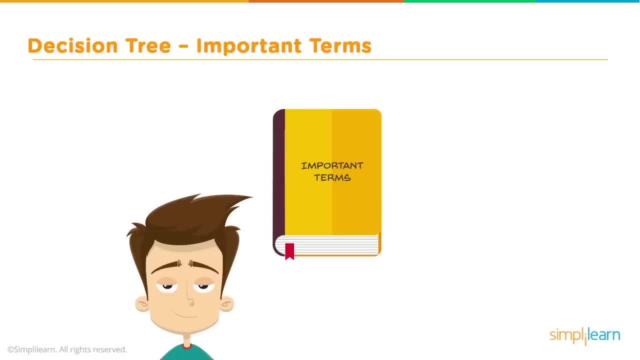 Decision tree: important terms. before we dive into further, we should look at some basic terms. We need to have some definitions to go with our decision trees in the different parts we're going to be using. We'll start with entropy. Entropy is a measure of randomness or unpredictability in a decision tree. It from the step of now in the in the year Dick's. 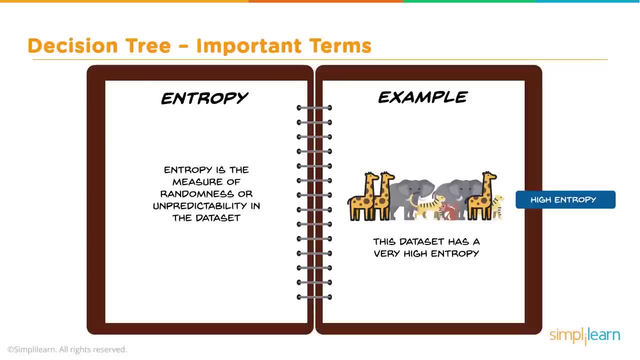 in the data set. For example, we have a group of animals. In this picture there's four different kinds of animals and this data set is considered to have a high entropy. You really can't pick out what kind of animal it is based on looking at just the four animals as a big clump of entities. 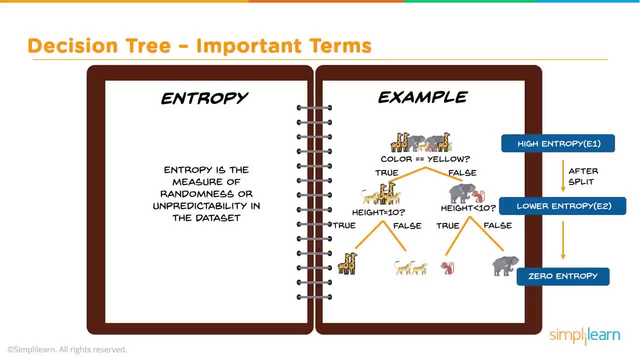 So, as we start splitting it into subgroups, we come up with our second definition, which is information gain. Information gain, it is a measure of decrease in entropy after the data set is split. So in this case, based on the color yellow, we've split one group of animals on one side as true. 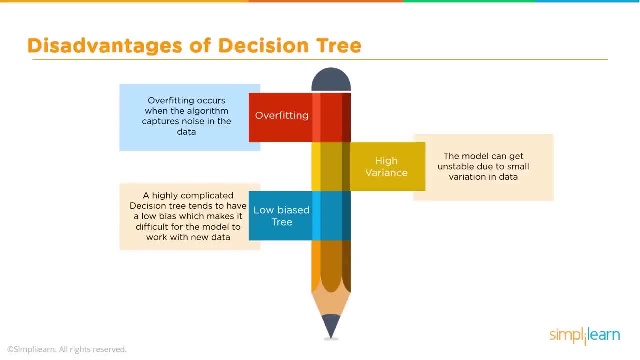 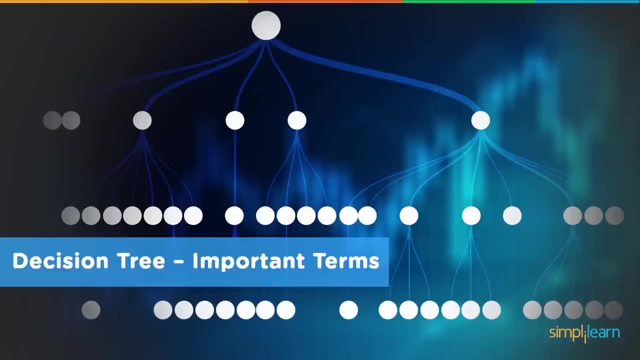 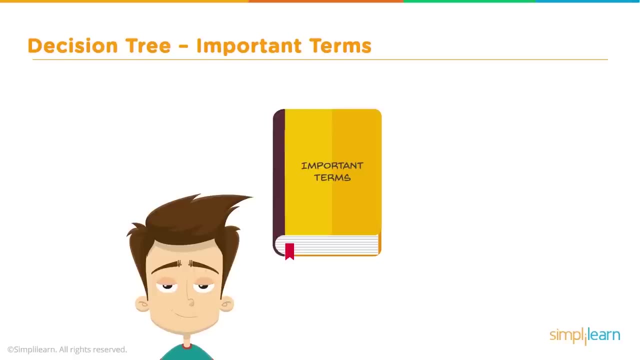 Low bias tree. A highly complicated decision tree tends to have a low bias, which makes it difficult for the model to work with new data. Decision tree important terms. Before we dive in further, we need to look at some basic terms. We need to have some definitions to go with our decision tree in the different 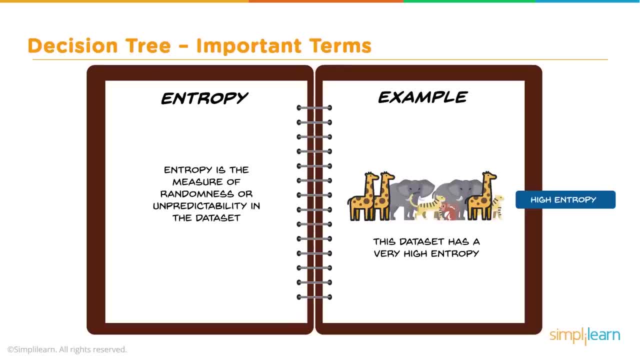 concepts we're going to be using. We'll start with entropy. Entropy is a measure of randomness or unpredictability in the data set. For example, we have a group of animals in this picture. There's four different kinds of animals and this data set is considered to have a high entropy. 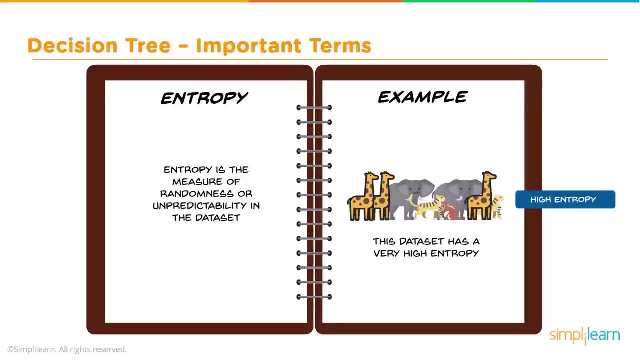 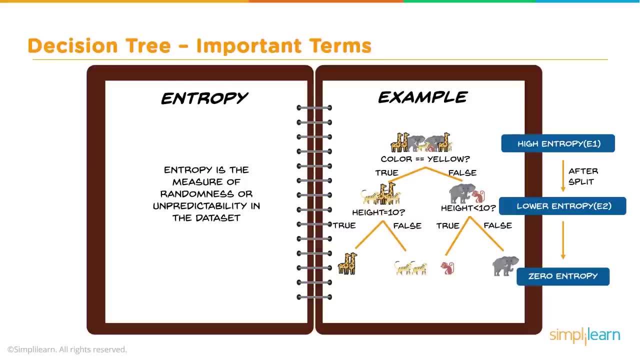 You really can't pick out what kind of animal it is based on looking at just the four animals as a big clump of entities. So as we start splitting it into subgroups, we come up with our second definition, which is information gain. 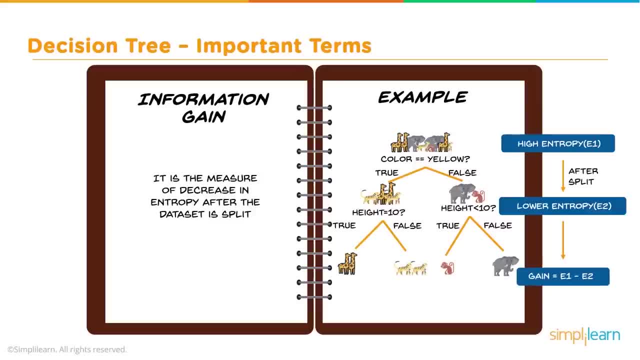 Information gain. It is a measure of decrease in entropy after the data set is split. So in this case, based on the color yellow, we've split one group of animals on one side as true and those who aren't yellow as false, As we continue down the yellow side. 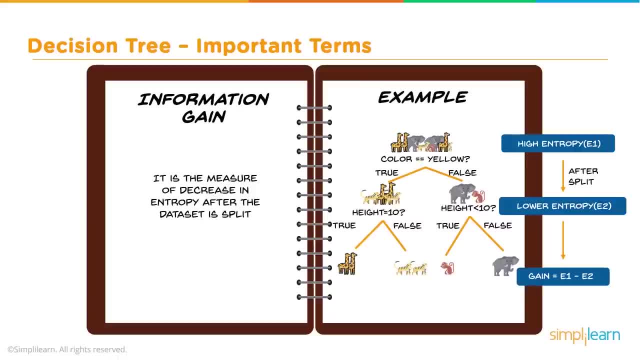 we split based on the height, true or false equals 10.. And on the other side, height is less than 10,, true or false. And as you see, as we split it, the entropy continues to be less and less and less. 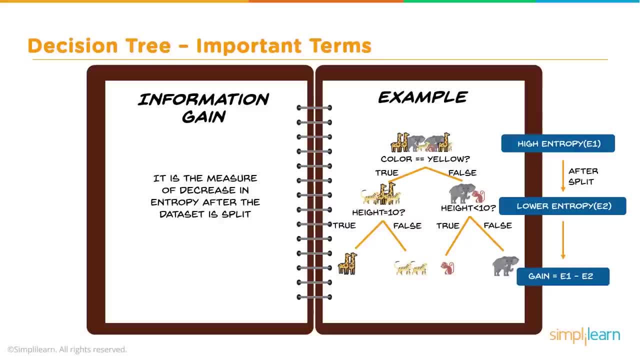 And so our information gain is simply the entropy E1 from the top and how it's changed to E2 in the bottom, And we'll look at the deeper math, although you really don't need to know a huge amount of math when you actually do the programming in Python, because they'll 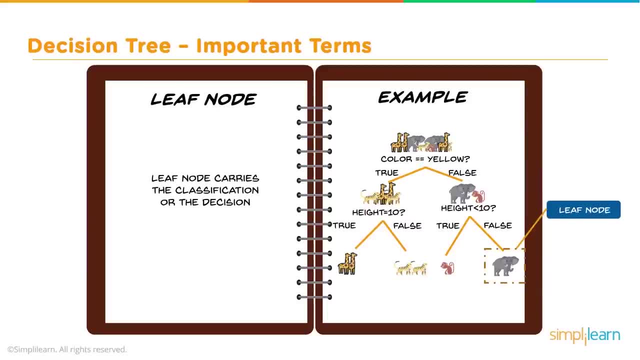 do it for you, but we'll look on the actual math at how they compute entropy. Finally, we went to the different parts of our tree and they call the leaf node. Leaf node carries the classification or the decision. So it's the final end at the bottom. 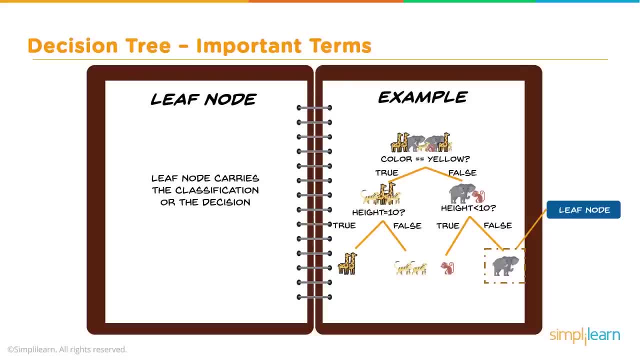 The decision node has two or more branches. This is where we're breaking the group up into different parts And finally you have the root node. The topmost decision node is known as the root node. How does a decision tree work? Wonder what kind of animals I'll get the jungle today. 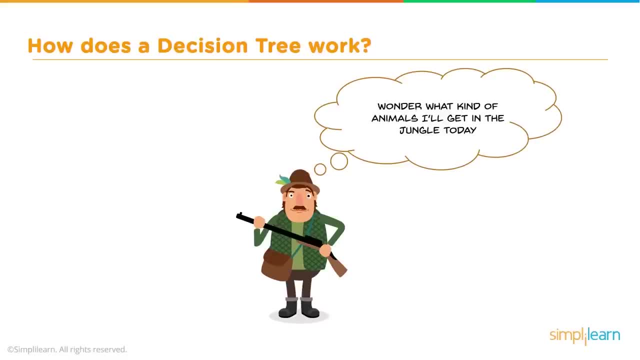 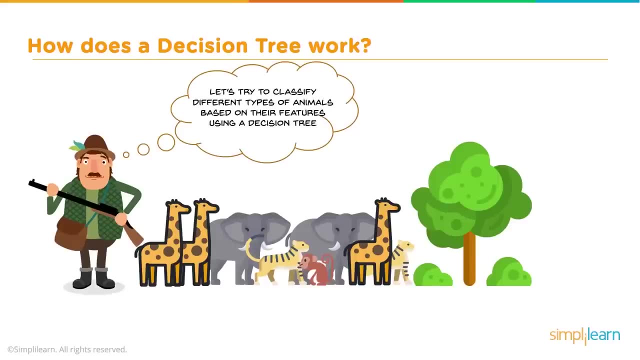 Maybe you're the hunter with the gun, or if you're more into photography, you're a photographer with a camera. So let's look at this group of animals and let's try to classify different types of animals based on their features, using a decision tree. 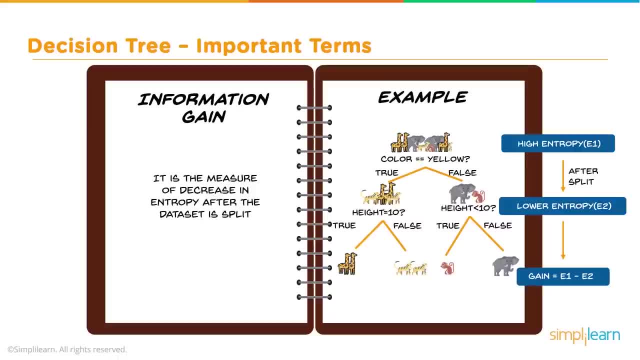 and those who aren't yellow as false. As we continue down the yellow side, we split based on the height. true or false equals 10, and on the other side, height is less than 10,- true or false. And as you see, as we split it, the entropy continues to be less and less and less, and so 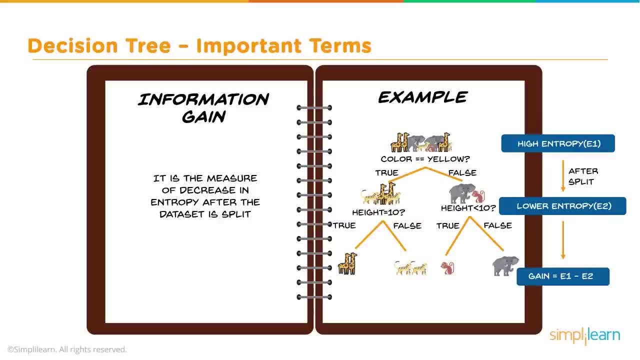 our information, gain is simply the entropy E1 from the top and how it's changed to E2 in the bottom, And we'll look at the deeper math, although you really don't need to know a huge amount of math when you actually do the programming in Python, because it'll do it for you. 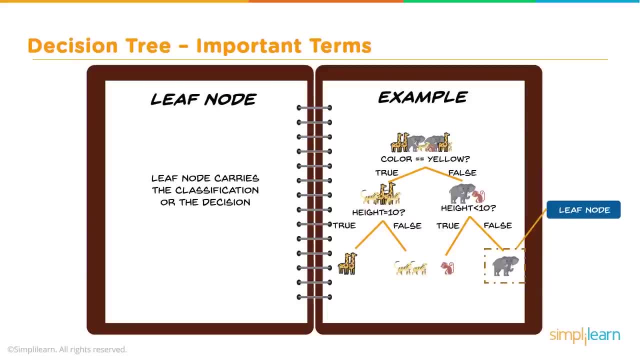 But we'll look on the actual math at how they compute entropy. Finally, we went over the different parts of our tree and they call the leaf node. Leaf node carries the classification or the decision, so it's the final end. at the bottom, The decision node has two or more branches. 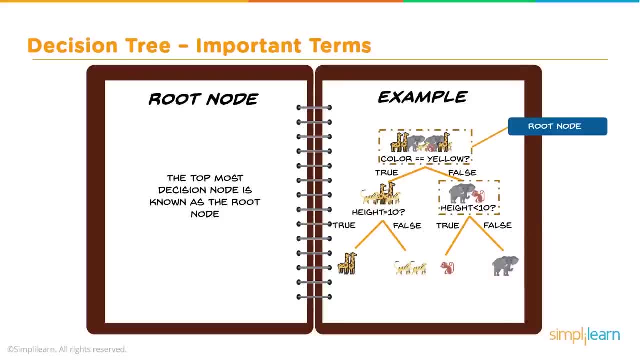 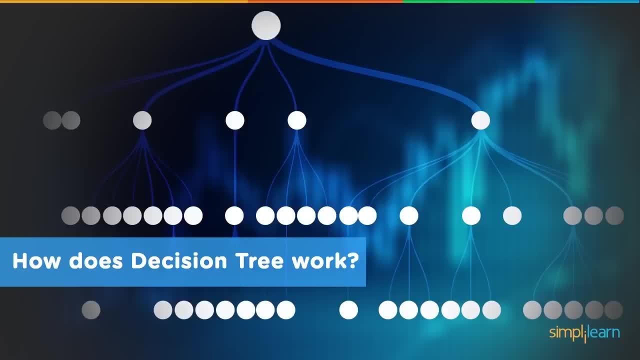 This is where we're breaking the group up into different parts And finally you have the root node. The topmost decision node is known as the root node. How does a decision node work? I wonder what kind of animals I'll get in the jungle today. Maybe you're the hunter with the gun. 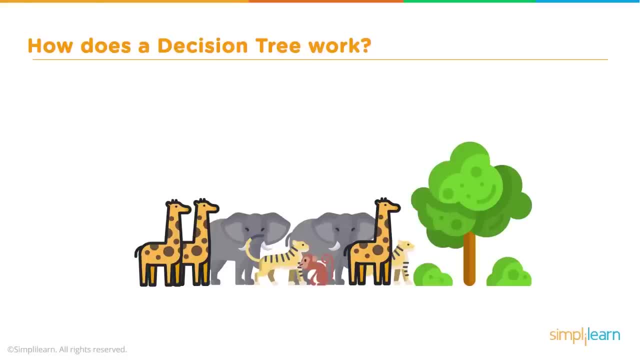 or if you're more into photography, you're a photographer with a camera. So let's look at this group of animals and let's try to classify different types of animals based on their features, using a decision tree. So the problem statement is to classify the different types of. 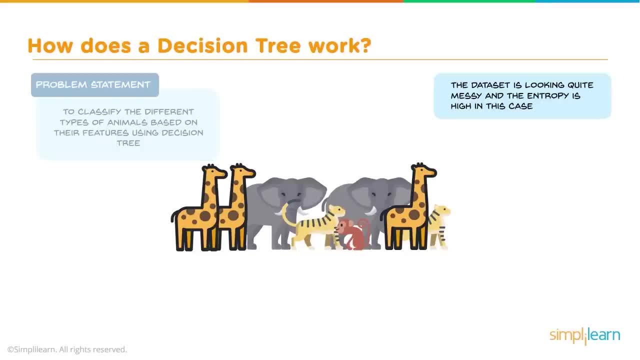 animals based on their features, using a decision tree. The data set is looking quite messy and the entropy is high in this case. So let's look at a training set or a training data set and we're looking at- we're looking at color, we're looking at height, and then we have our different animals. We have our 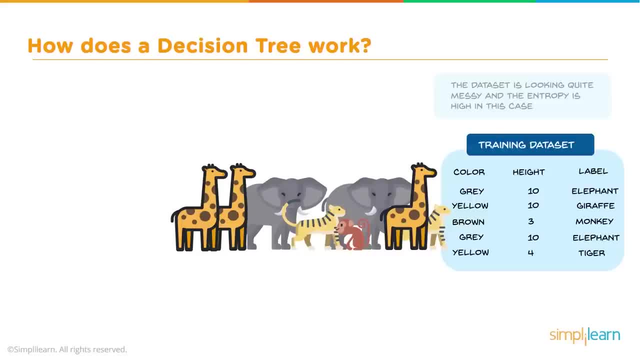 elephants, our giraffes, our monkeys and our tigers, And they're of different colors and shapes. Let's see what that looks like and how do we split the data. We have to frame the conditions that split the data in such a way that the information gain is the highest. Note gain is the measure of decrease. 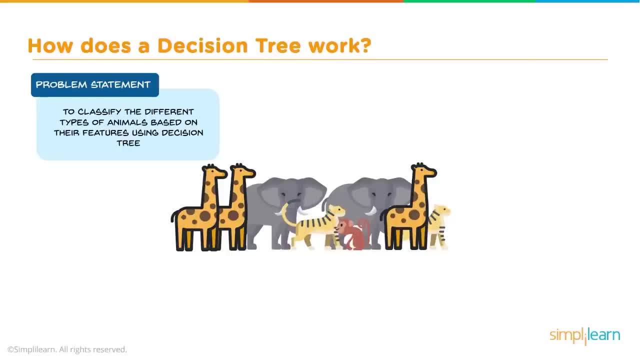 So the problem statement is to classify the different types of animals based on their features using a decision tree. The data set is looking quite messy and the entropy is high In this case, So let's look at a training set or a training data set. 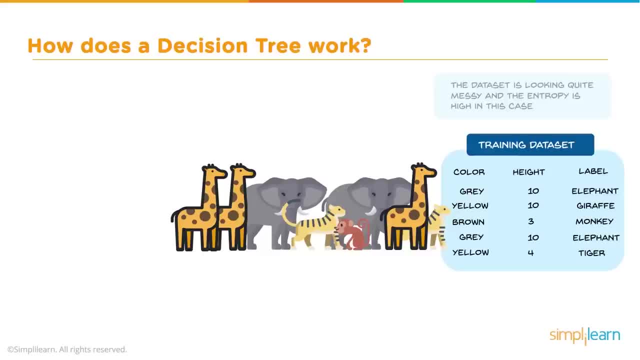 And we're looking at color, We're looking at height, And then we have our different animals. We have our elephants, our giraffes, our monkeys and our tigers, And they're of different colors and shapes. Let's see what that looks like. 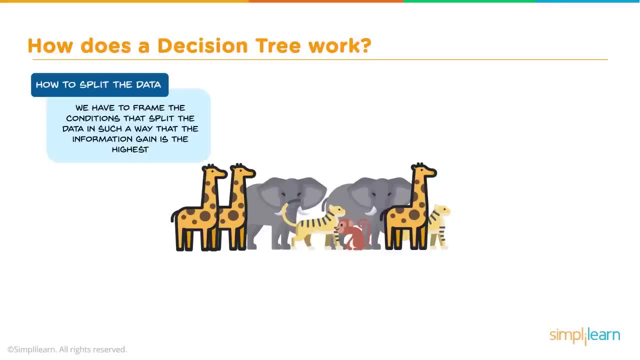 And how do we split the data? We have to frame the conditions that split the data in such a way that the information gain is the highest. Note gain is a measure of decrease in entropy after splitting, So the formula for entropy is the sum. that's what this symbol looks like. 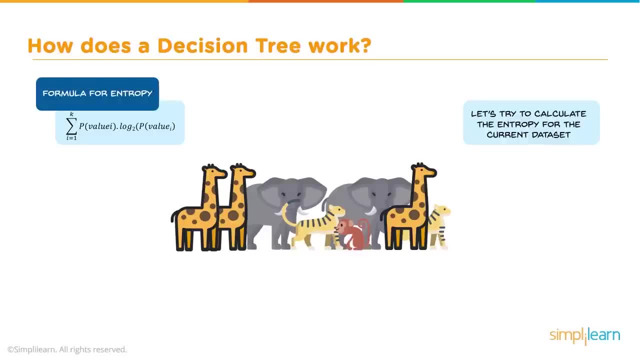 It looks like kind of like a funky E of K where I equals one to K. K would represent the number of animals, the different animals in there, where value or P value of I would be the percentage of that animal times the log base. two of the same: the percentage of that animal. 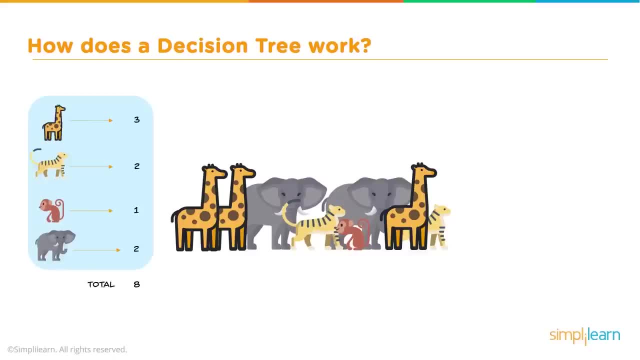 Let's try to calculate the entropy for the current data set and take a look at what that looks like. And don't be afraid of the math. Don't really have to memorize this math, Just be aware that this is there and this is what's going on in the background. 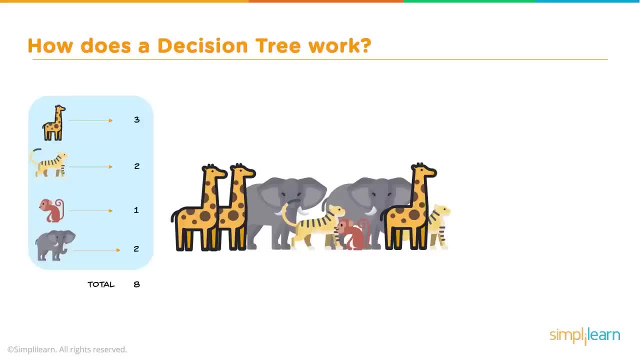 And so we have three giraffes, two tigers, one monkey, two elephants, a total of eight animals gathered. And if we plug that into the formula, we get an entropy that equals three over eight. So we have three giraffes, a total of eight times the log. 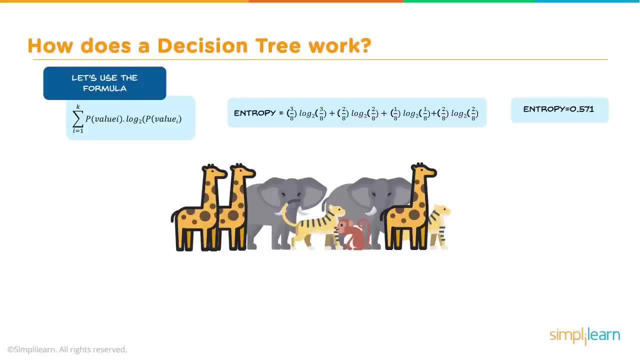 Usually they use base two on the log, So log base two of three over eight plus in this case let's say it's the elephants, two over eight, two elephants over a total of eight times log base two. two over eight plus one monkey. 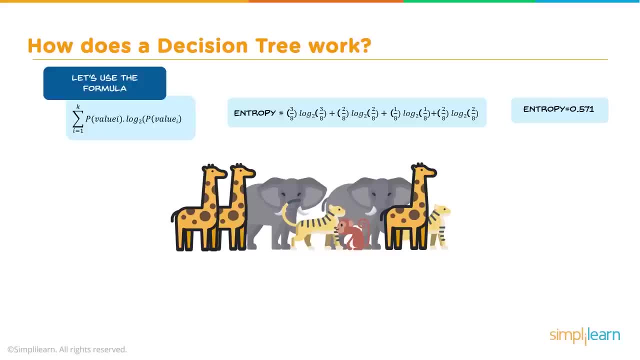 a total of eight log base two, one over eight and plus two over eight of the tigers Log base two over eight. And if we plug that into our computer or calculator- I obviously can't do logs in my head- we get an entropy equal to point five, seven, one. 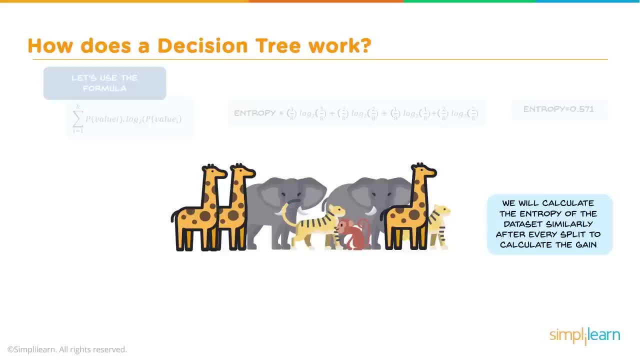 The program will actually calculate the entropy of the data set. similarly, after every split, to calculate the gain. Now, we're not going to go through each set, one at a time, to see what those numbers are. We just want you to be aware that this is a formula or the mathematics. 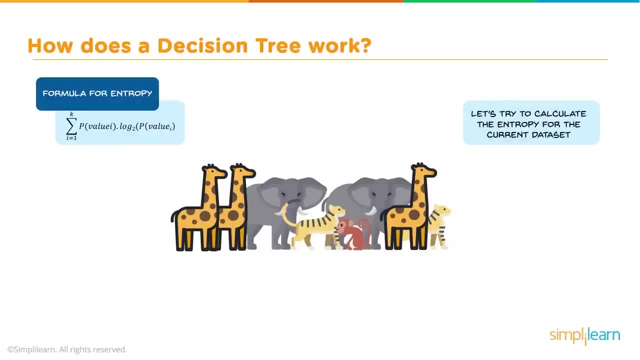 in entropy after splitting. So the formula for entropy is the sum. that's what this symbol looks like. that looks kind of like a funky E. that looks kind of like a funky E of K, where I equals 1 to K. K would represent the number of animals, the different animals in there, where value or p value of I would be the percentage of that animal times the log base 2 of the same, the percentage of that animal. 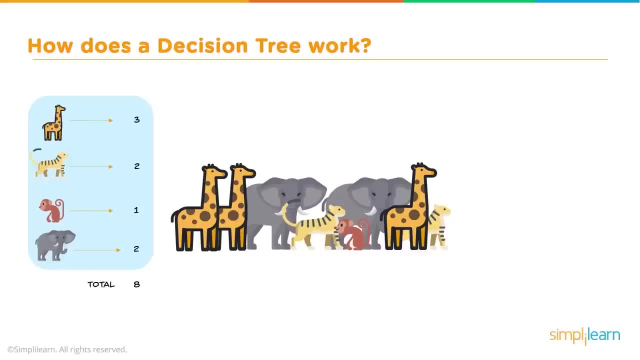 Let's try to calculate the entropy for the current data set and take a look at what that looks like. And don't be afraid of the math. You don't really have to memorize this math, Just be aware that it's there. and this is what's going on in the background. 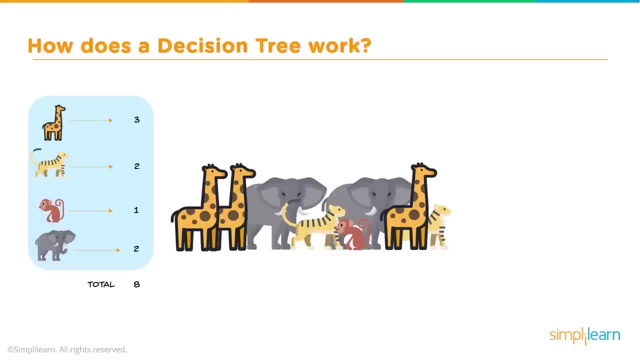 And so we have three giraffes, two tigers, one monkey, two elephants, a total of eight animals gathered. And if we plug that into the formula, we get an entropy that equals three over eight. So we have three giraffes, a total of eight times the log. 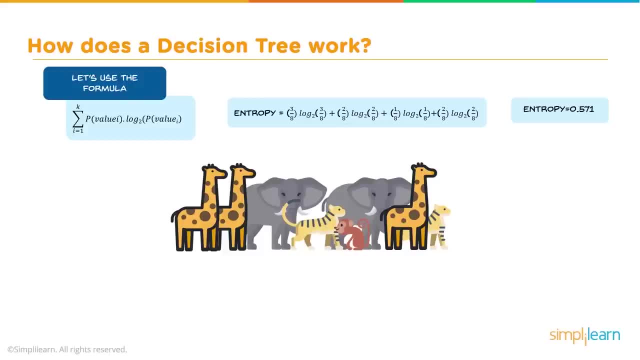 Usually they use base two on the log, So log base two of three over eight, plus in this case let's say it's the elephants two over eight. two elephants over a total of eight times log base two, two over eight plus one monkey over a total of eight. log base two: one over eight and plus two over eight. of the tigers: log base two over eight. 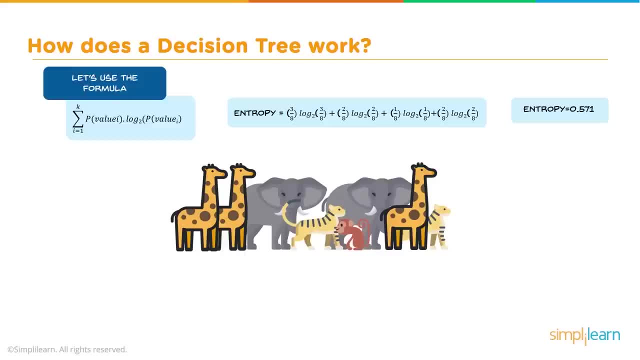 And if we plug that into our computer or calculator, I obviously can't do logs in my head. we get an entropy equal to 0.571.. The program will actually calculate the entropy of the data. We will use a data set. similarly, after every split to calculate the gain. 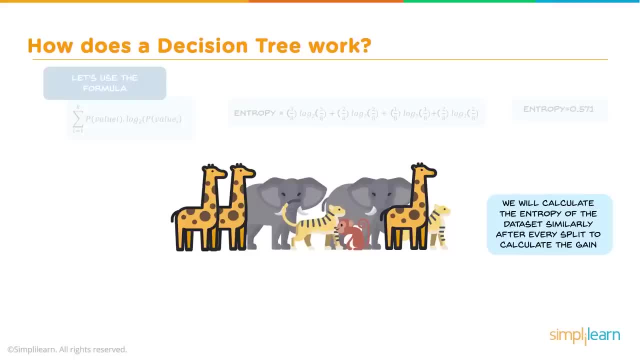 Now we're not going to go through each set, one at a time, to see what those numbers are. We just want you to be aware that this is a formula or the mathematics behind it. Gain can be calculated by finding the difference of the subsequent entropy values after a split. 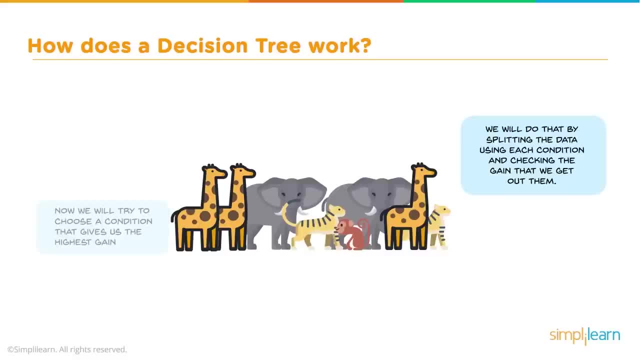 Now we will try to choose a condition that gives us the highest gain. We will do that by splitting the data using each condition and checking that the gain we get out of them- The condition that gives us the highest gain- will be used to make the first split. 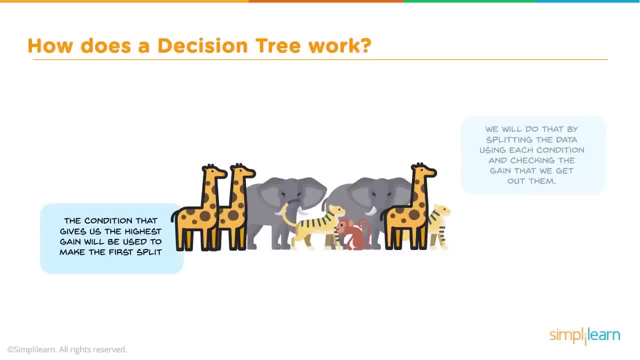 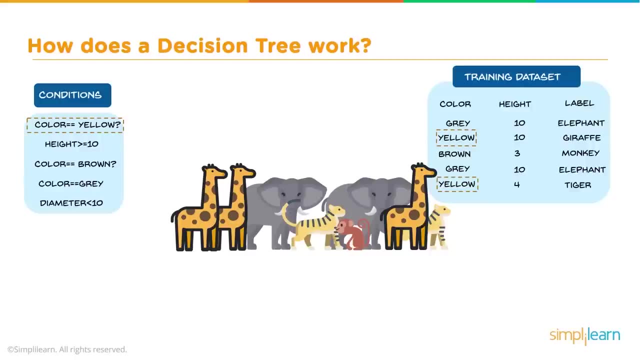 Can you guess what that first? The first split will be just by looking at this image. as a human, it's probably pretty easy to split it. Let's see if you're right. If you guessed the color yellow, you're correct. 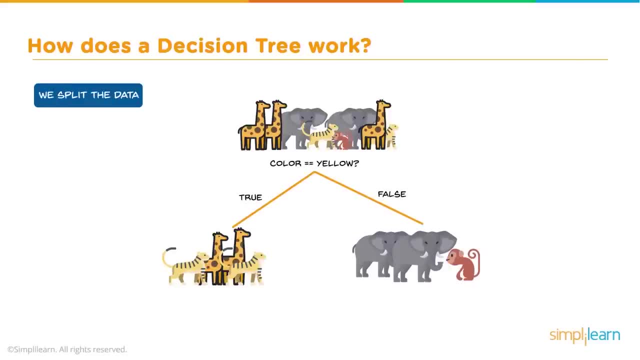 Let's say the condition that gives us the maximum gain is yellow. So we will split the data based on the color yellow. If it's true, that group of animals goes to the left. If it's false, it goes to the right. 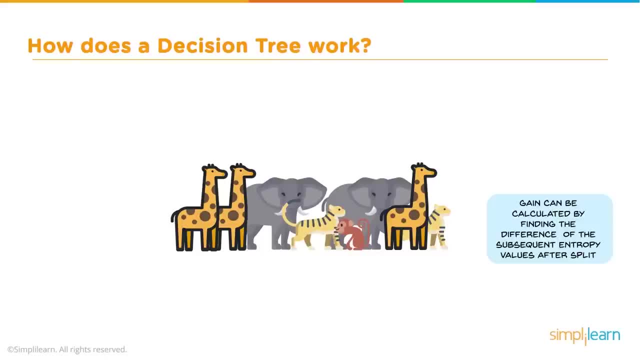 behind it. gain can be calculated by finding the difference of the subsequent entropy values after a split. Now we will try to choose a condition that gives us the highest gain. We will do that by splitting the data using each condition and checking that the gain we get out of them. 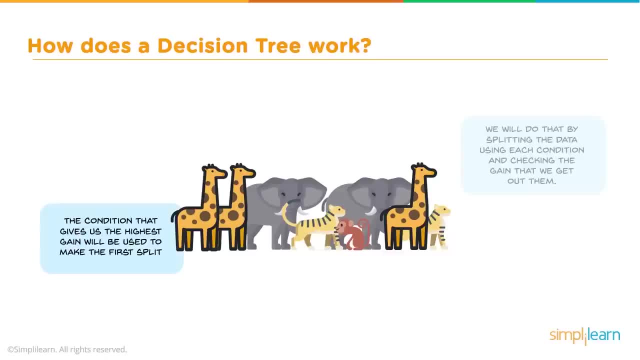 The condition that gives us the highest gain will be used to make the first split. Can you guess what that first split will be? Just by looking at this image, as a human is probably pretty easy to split it. Let's see if you're right. 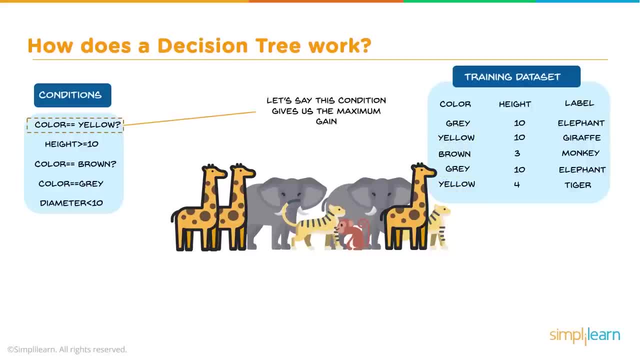 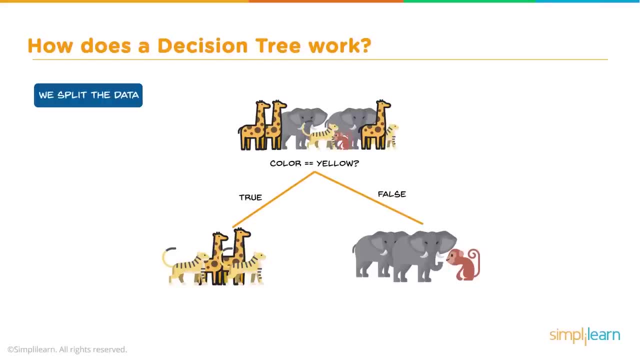 If you guessed the color yellow, you're correct. Let's say the condition that gives us the maximum gain is yellow. so we will split the data based on the color yellow. If it's true that group of animals goes to the left. 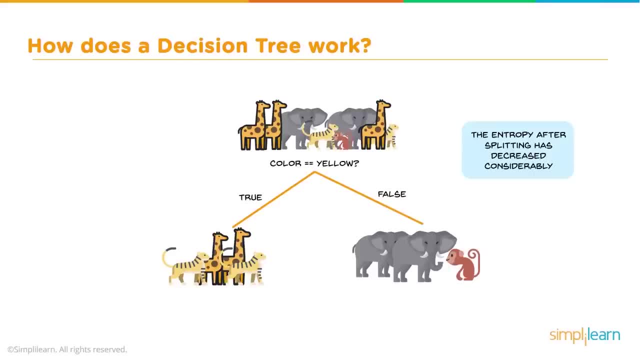 If it's false, it goes to the right. The entropy after the splitting has decreased considerably. However, we still need some splitting at both the branches to attain an entropy value equal to zero. So we decide to split both the nodes, using height as a condition. 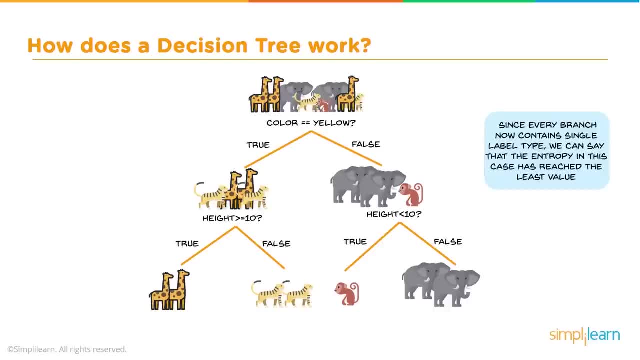 Since every branch now contains single label type, we can say that entropy, in this case, has reached the least value. And here you see, we have the giraffes, the tigers, the monkey and the elephants, all separated into their own groups. This tree can now predict all the classes. 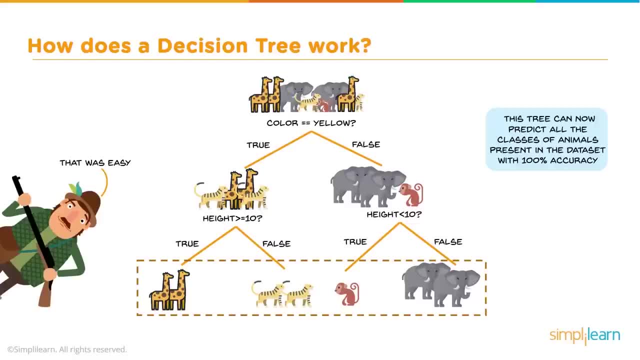 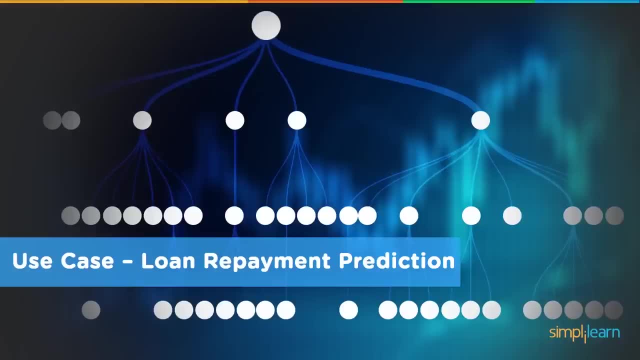 of animals present in the dataset with 100 percent accuracy. That was easy Use case loan repayment prediction. Let's get into my favorite part and open up some Python and see what the programming code and the scripting looks like. In here we're going to want to do a prediction. 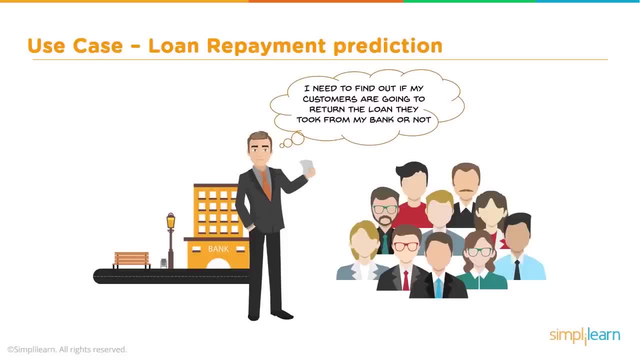 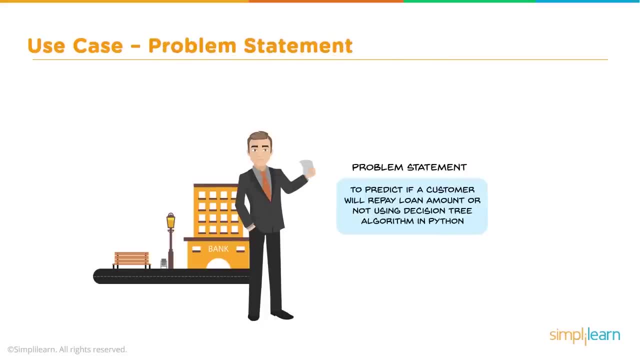 And we start with this individual here who's requesting to find out how good his customers are going to be, whether they're going to repay their loan or not for his bank. And from that we want to generate a problem statement to predict if a customer will repay loan amount or not. 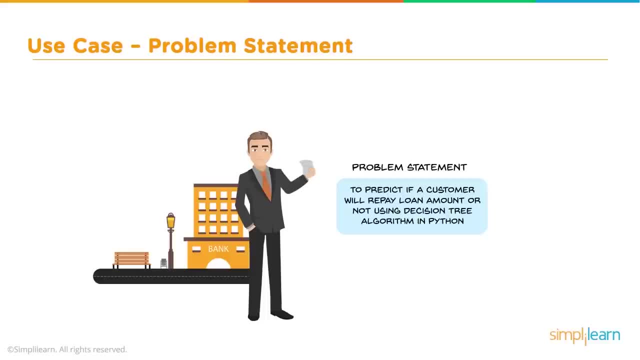 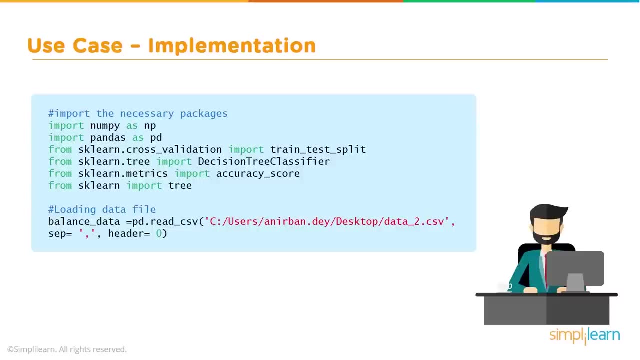 And then we're going to be using the decision tree algorithm in Python. Let's see what that looks like and let's dive into the code. In our first few steps of implementation, we're going to start by importing the necessary packages that we need from: 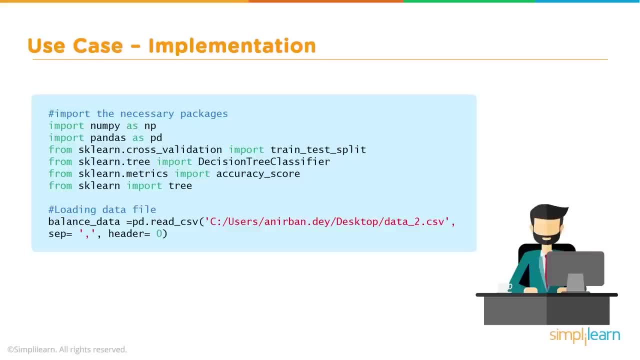 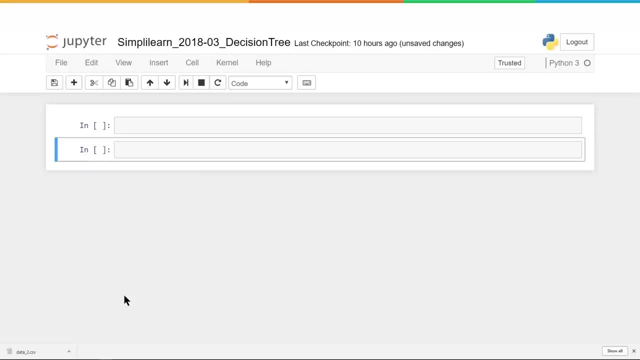 Python and we're going to load up our data and take a look at what the data looks like. So the first thing I need is I need something to edit my Python and run it in. So let's flip on over, And here I'm using the Anaconda. 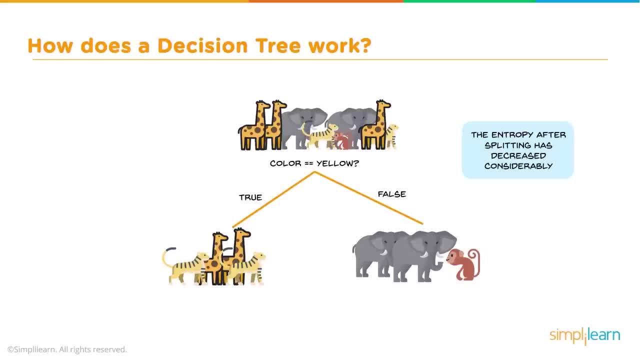 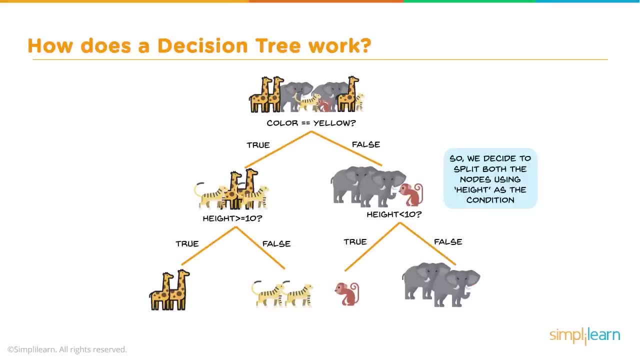 The entropy after the splitting has decreased considerably. However, we still need some splitting at both the branches to attain an entropy value equal to zero. So we decided to split both nodes using height as a condition. Since every branch now contains a single label type, we can say that entropy in this case has reached the least value. 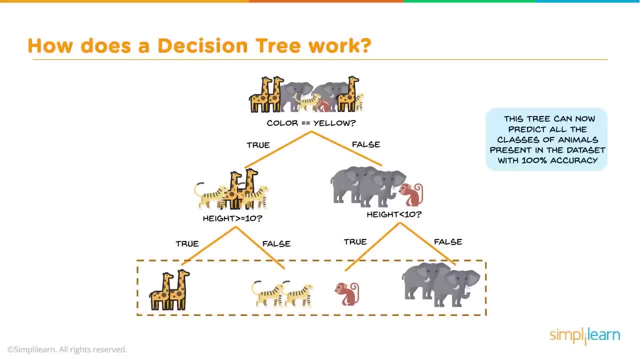 And here you see we have the giraffes, the tigers, the monkey and the elephants, all separated into their own groups. This tree can now predict all the classes of animals present in the data set with a hundred percent accuracy. That was easy. 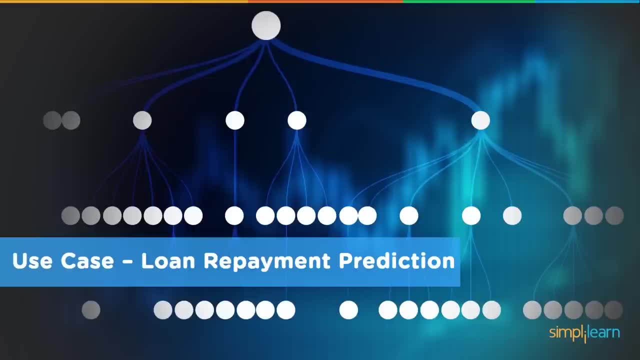 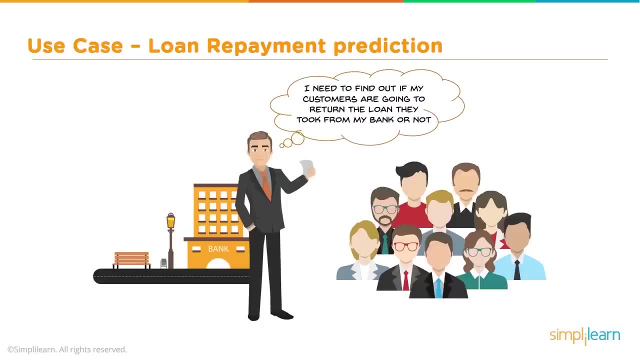 Use case: loan repayment prediction. Let's get into my favorite part and open up some Python and see what the programming code in the scripting looks like. In here we're going to want to do a prediction and we start with this individual here who's requesting to find out how good his customers are going to be, whether they're 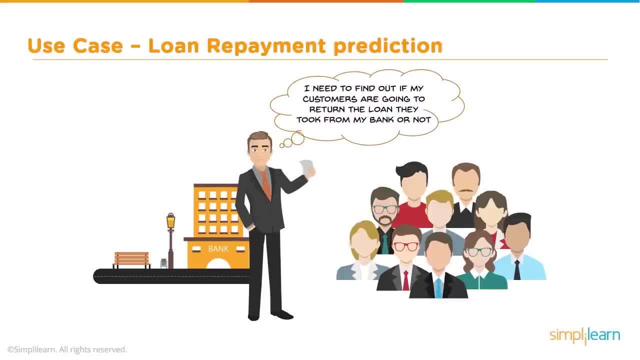 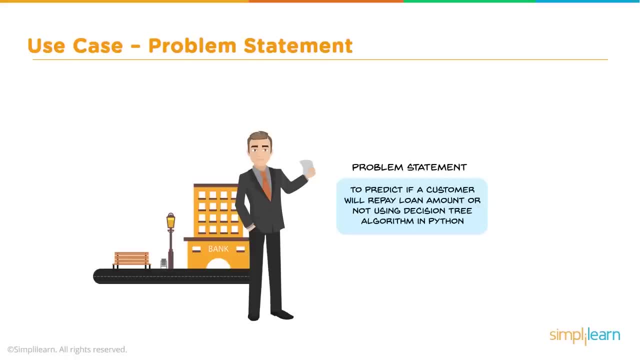 going to repay their loan or not for his bank, and from that we want to generate a problem statement to predict if a customer will repay loan amount or not, and then we're going to be using the decision tree algorithm in Python. Let's see what that looks like and let's dive into the code In our 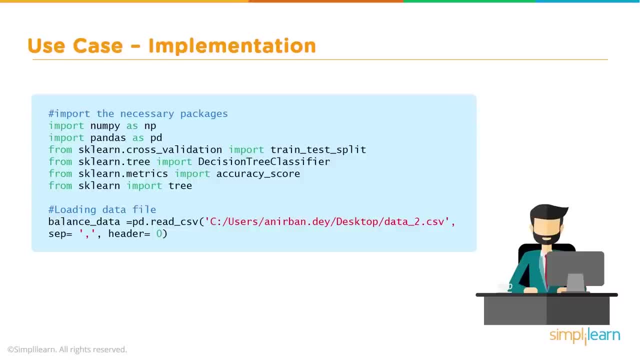 first few steps of implementation. we're going to start by importing the necessary packages that we need from Python, and we're going to load up our data and take a look at what the data looks like. So the first thing I need is I need something to edit my Python and run it in. So let's flip on. 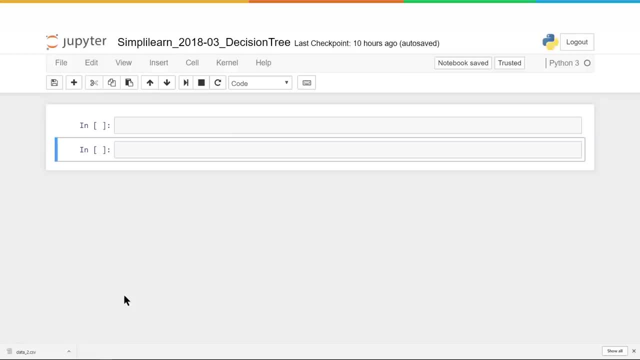 over, and here I'm using the Anaconda Jupyter notebook. Now you can use any Python IDE you like to run it in, but I find the Jupyter notebook's really nice for doing things on the fly, and let's go ahead and just paste that code in the beginning. and before we start, let's talk a little bit about. 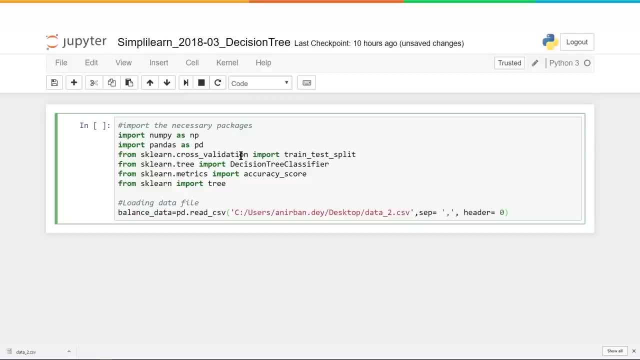 what we're bringing in, and then we're going to do a couple things in here. I have to make a couple changes as we go through This first part of the import. The first thing we bring in is numpy as np. That's very standard when 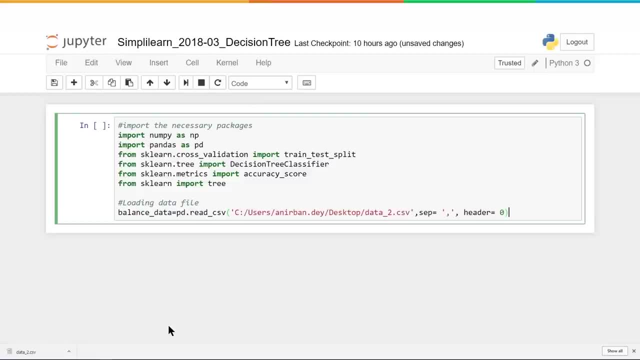 we're dealing with mathematics, especially with very complicated machine learning tools. You almost always see the numpy come in for your numbers. It's called number python. It has your mathematics in there. In this case we actually could take it out, but generally you'll need it. 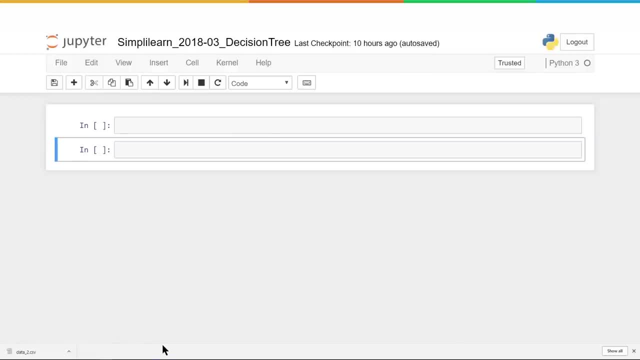 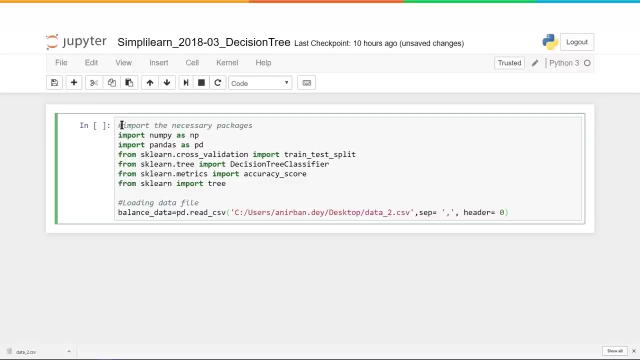 the Jupyter notebook. Now you can use any Python IDE you like to run it in, but I find the Jupyter notebooks really nice for doing things on the fly And let's go ahead and just paste that code in the beginning. And before we start, let's talk a little bit about what we're bringing in. 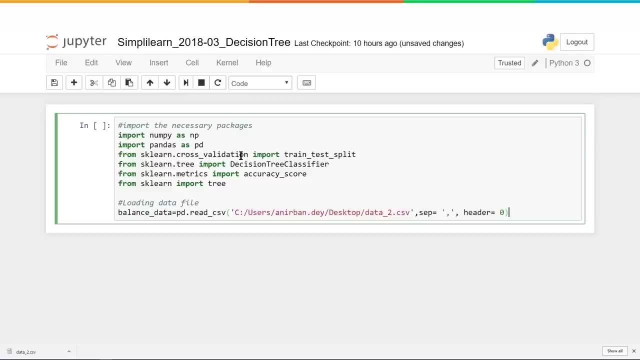 And then we're going to do a couple of things in here. We have to make a couple of changes as we go through this first part of the import. The first thing we bring in is numpy as NP. That's very standard when we're dealing. 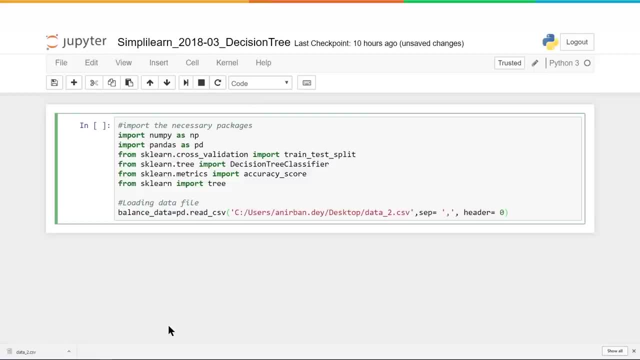 with mathematics, especially with very complicated machine learning tools. You see, the numpy come in for your numbers. It's called number Python. It has your mathematics in there. In this case we actually could take it out, But generally you'll need it for most of your different things you work with. 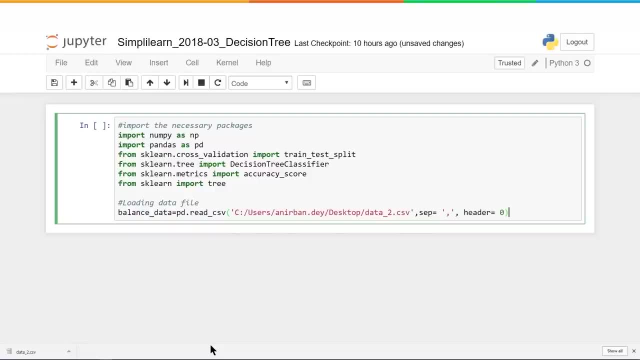 And then we're going to use pandas as PD. That's also a standard. The pandas is a data frame set up And you can liken this to taking your basic data and storing it in a way that looks like an Excel spreadsheet. So, as we come back to this, when you see NP or PD, those are very standard uses. 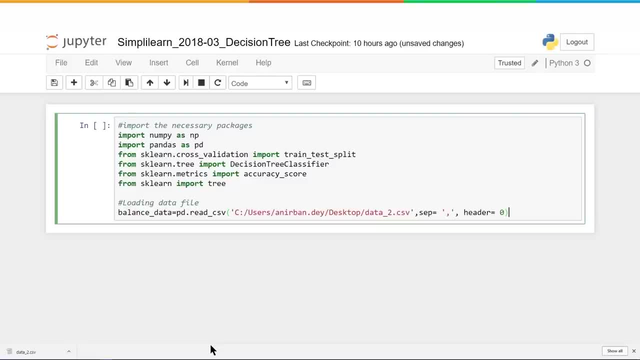 You'll know that that's the pandas And I'll show you a little bit more. when we explore the data in just a minute, Then we're going to need to split the data. So I'm going to bring in our train, test and split. 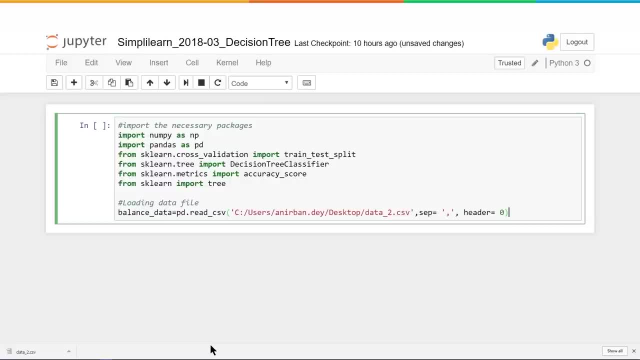 And this is coming from the sklearn package: cross-validation. In just a minute we're going to change that and we'll go over that too. And then there's also the sktree import decision tree classifier. That's the actual tool we're using. 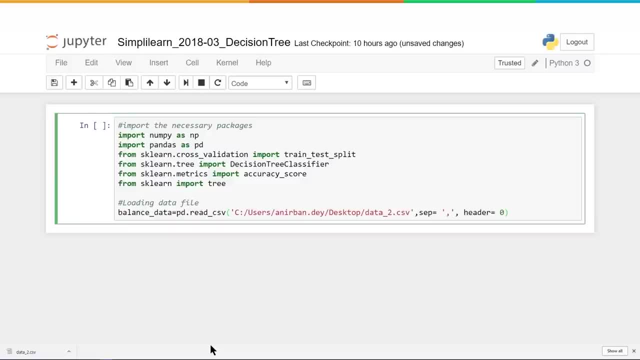 Remember I told you don't be afraid of the mathematics, It's going to be done for you. Well, the decision tree classifier has all that mathematics in there for you, So you don't have to figure it back out again. And then we have sklearn. 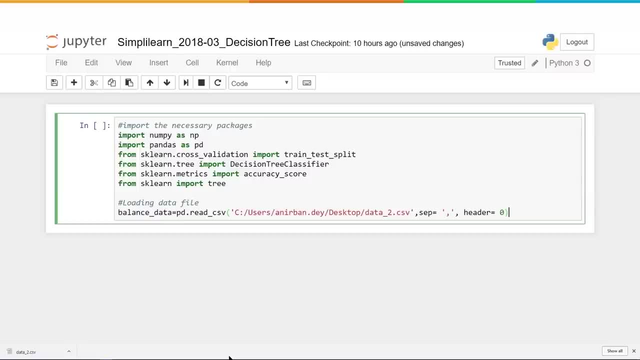 metrics for accuracy score. We need to score our setup. That's the whole reason we're splitting it between the training and testing data. And finally, we still need the sklearn import tree And that's just the basic tree function is needed for the decision tree classifier. 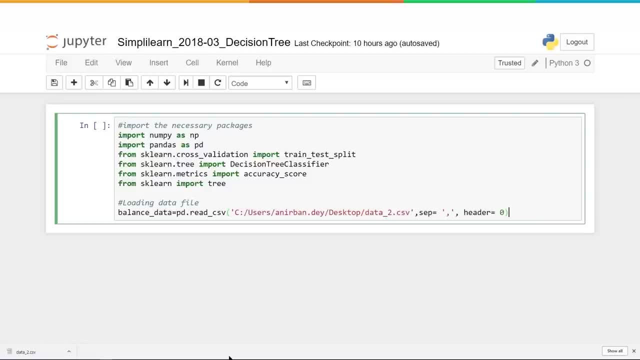 And finally, we're going to load our data down here and I'm going to run this And we're going to get two things on here: One, we're going to get an error and two, we're going to get a warning. 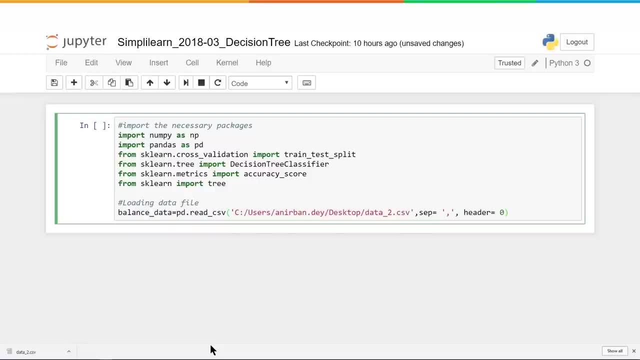 for most of your different things you work with, and then we're going to use pandas as pd. That's also a standard. The pandas is a data frame setup, and you can liken this to taking your basic data and storing it in a way that looks like an Excel spreadsheet. So, as we 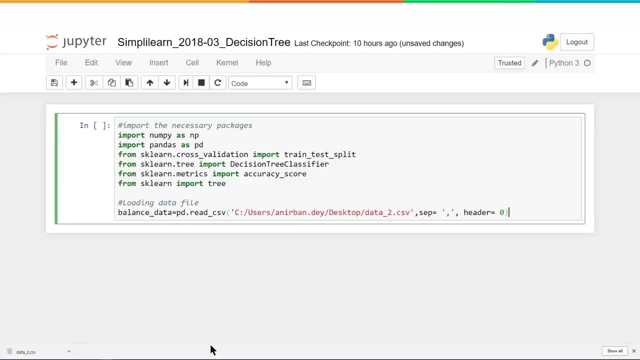 come back to this when you see np or pd. those are very standard uses. you'll know that that's the pandas and I'll show you a little bit more when we explore the data in just a minute. Then we're going to need to split the data. so I'm going to bring in our train, test and split and this is. 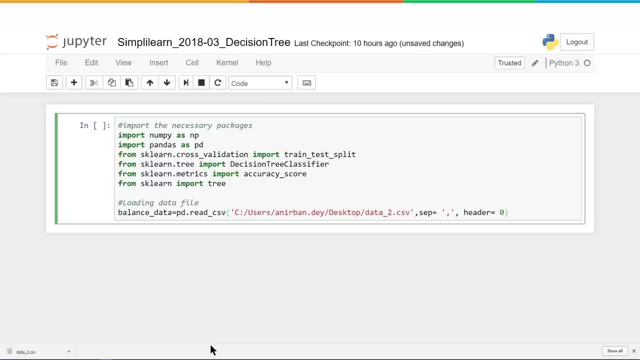 coming from the sklearn package: cross validation. In just a minute we're going to change that and we'll go over that too. and then there's also the sktree import decision tree classifier. That's the actual tool we're using. Remember I told you, don't be afraid of the mathematics. It's. 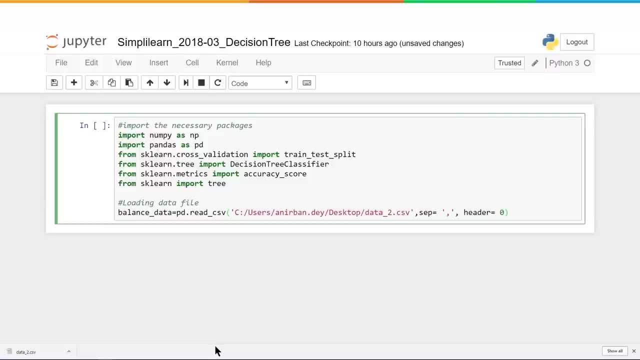 going to be done for you. Well, the decision tree classifier has all that mathematics in there for you, so you don't have to figure it back out again. and then we have sklearnmetrics for accuracy score. We need to score our setup. That's the whole reason. we're splitting it between the training and 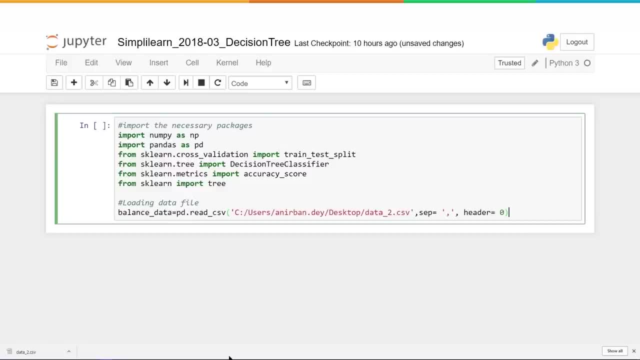 testing data. and finally, we still need the sklearn import tree, and that's just the basic tree function is needed for the decision tree classifier. and finally, we're going to load our data down here and we're going to get two things on here: One, we're going to get an error and two, we're going to get a. 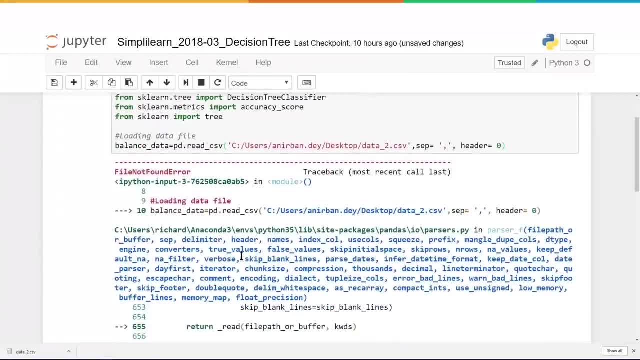 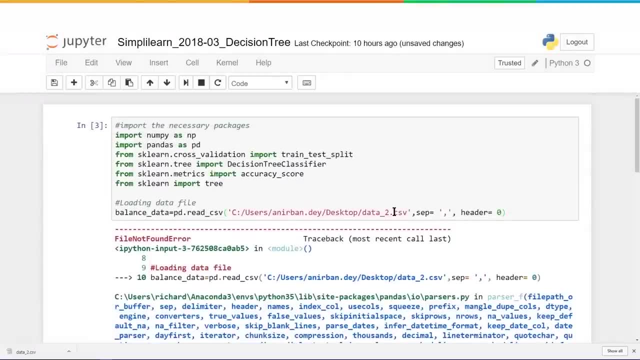 warning. Let's see what that looks like. So the first thing we had is we have an error. Why is this error here? Well, it's looking at this. it says I need to read a file and when this was written, the person who wrote it, this is their path where they stored the file. So let's go ahead and fix that. 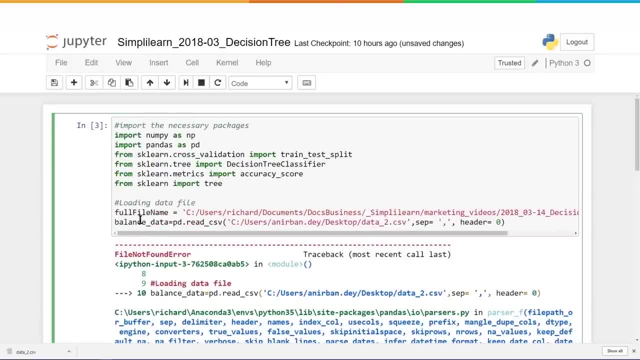 and I'm going to put in here my file path. I'm just going to call it full file name and you'll see it's on my C Drive and it's going to say file name and I'm going to put in here my file path and. 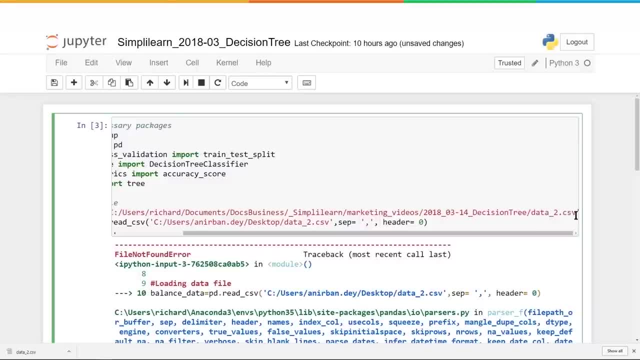 there's this very lengthy setup on here where I stored the data2.csv file. Don't worry too much about the full path, because on your computer it'll be different. The data2.csv file was generated by simplylearn. If you want a copy of that, you can comment down below and request it here in the. 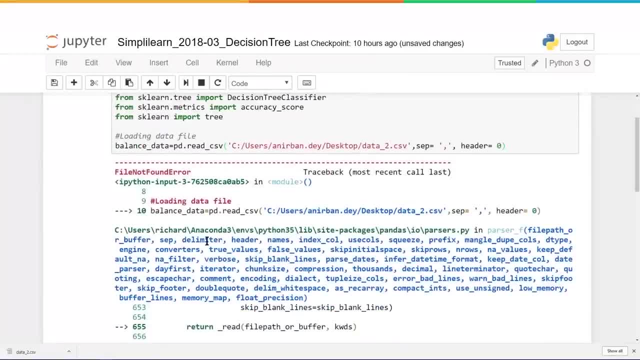 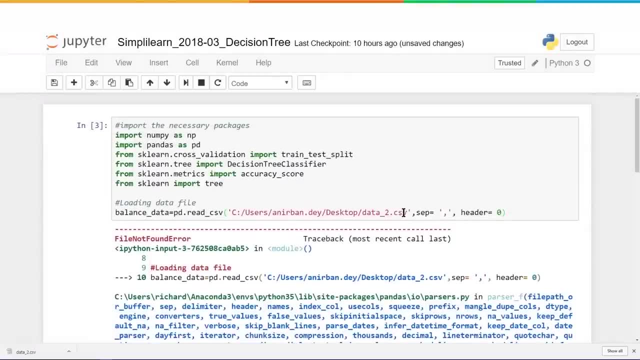 Let's see what that looks like. So the first thing we had is: we have an error. Why is this error here? Well, it's looking at this Because I need to read a file And when this was written, the person who wrote it. 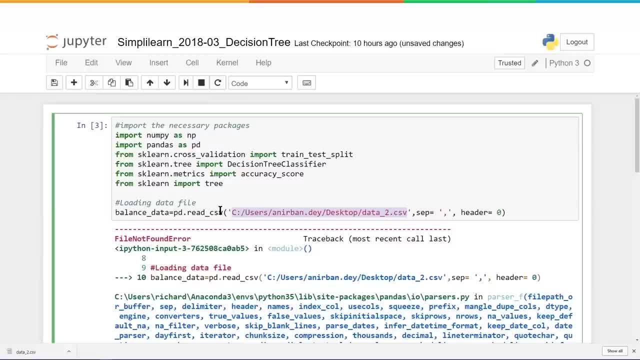 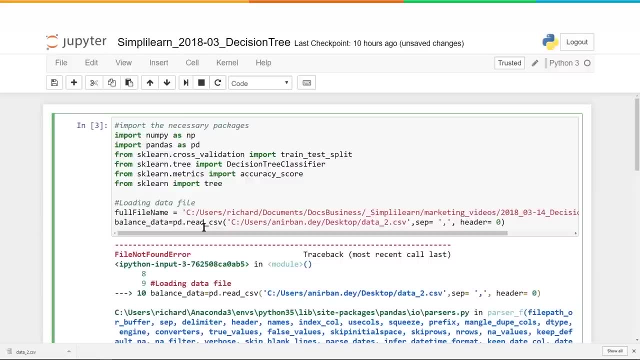 this is their path where they stored the file. So let's go ahead and fix that And I'm going to put in here my file path. I'm just going to call it full file name and you'll see. it's on my C drive and it's this very lengthy setup on here. 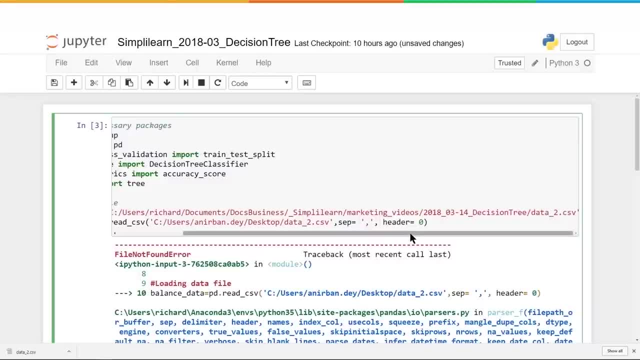 where I stored the data2.csv file. Don't worry too much about the full path, because on your computer it'll be different. The data.2csv file was generated by SimplyLearn. If you want a copy of that, you can comment down below and request it here in the YouTube. 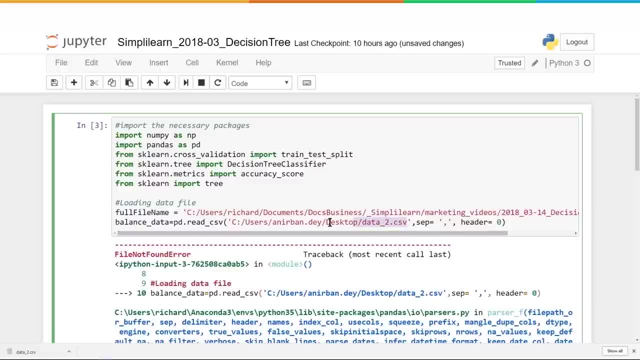 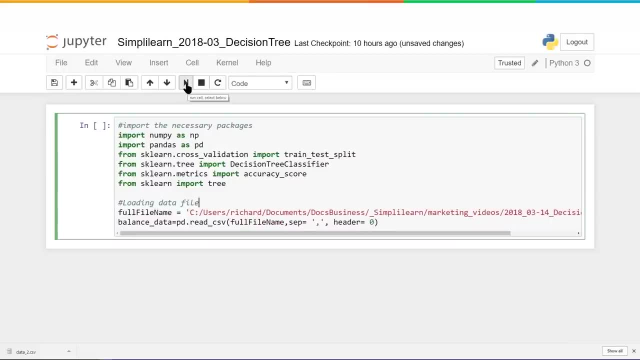 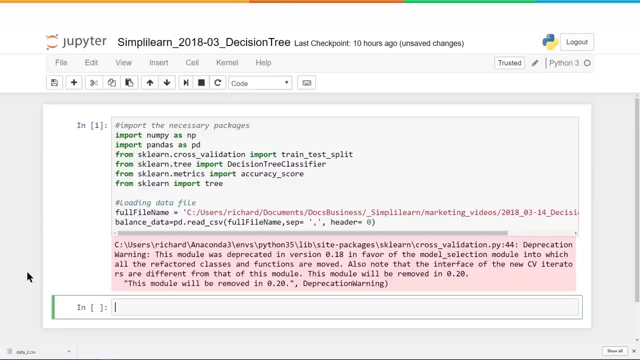 And then, if I'm going to give it a name- full file name- I want to go ahead and change it here to full file name. So let's go ahead and run it now and see what happens And we get a warning And when you're coding, understanding these different warnings and these different errors, 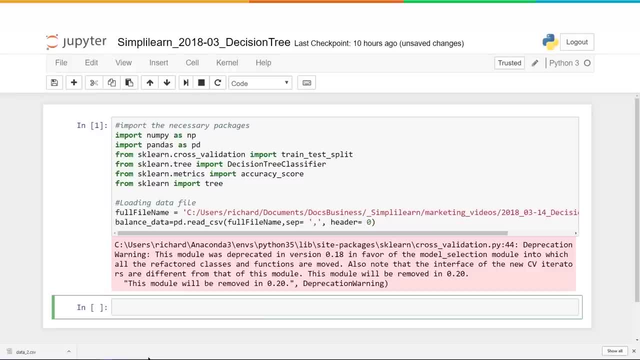 that come up is probably the hardest lesson to learn. So let's just go ahead and take a look at this and use this as a opportunity to understand what's going on here. If you read the warning, it says the cross validation is depreciated. 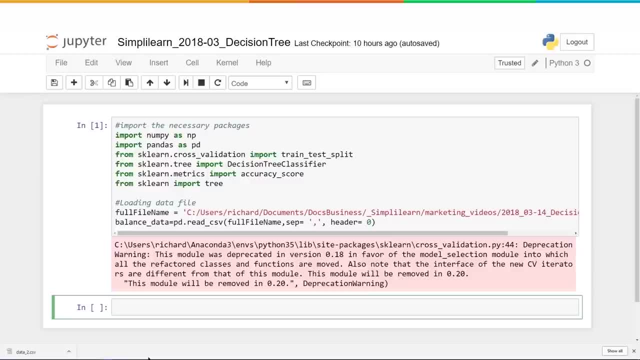 So it's a warning on. it's being removed and it's going to be moved in favor of the model selection. So if we go up here, we have sklearncrossvalidation And if you research this and go to the sklearn site, you'll find out that you can actually just swap it right in there with model selection. 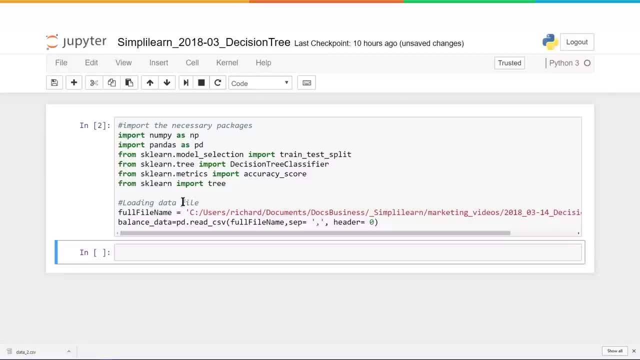 And so when I come in here and I run it again, that removes a warning. What they've done is they've had two different developers develop it in two different branches and then they decided to keep one of those and eventually get rid of the other one. 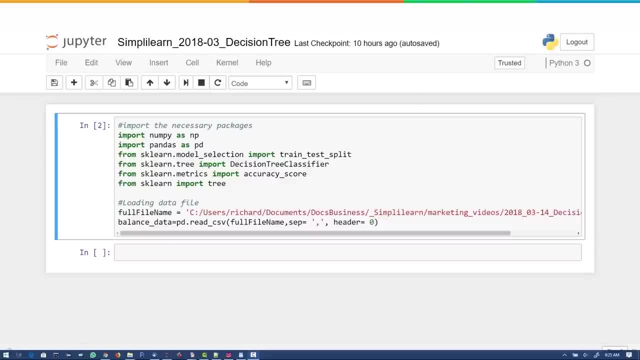 That's all that is, and very easy and quick to fix. Before we go any further, I went ahead and opened up the data from this file. Remember the data file we just loaded on here? the data underscore two dot csv. Let's talk a little bit more about that and see what that looks like. 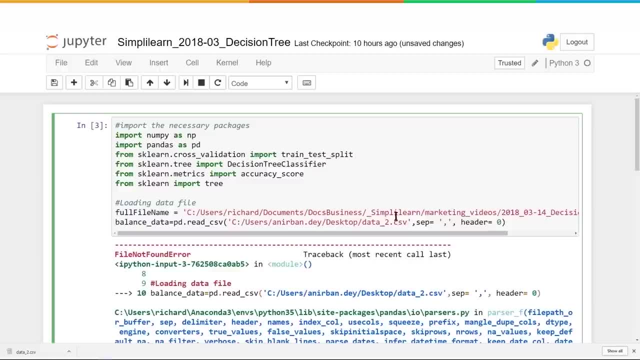 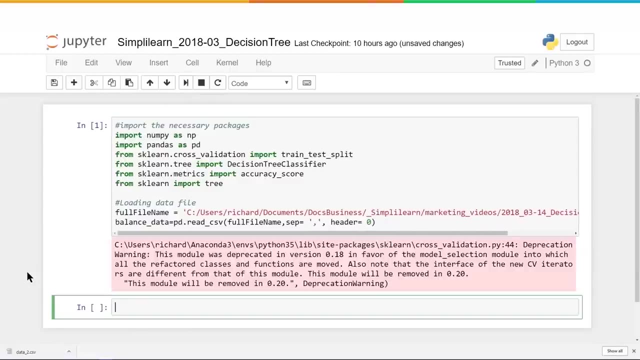 YouTube and then, if I'm going to give it a name- full file name- I want to go ahead and change it to my full file name. So let's go ahead and run it now and see what happens, And we get a warning When you're coding. understanding these different warnings and these different? 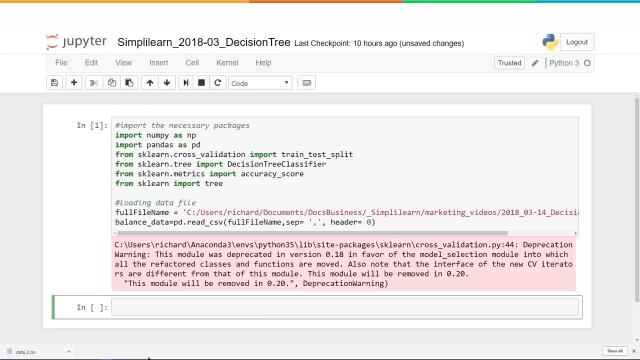 errors that come up is probably the hardest lesson to learn. So let's just go ahead and take a look at this and use this as a opportunity to understand what's going on here. If you read the warning, it says the cross validation is depreciated. So it's a warning on it's being removed And it's going to be moved. 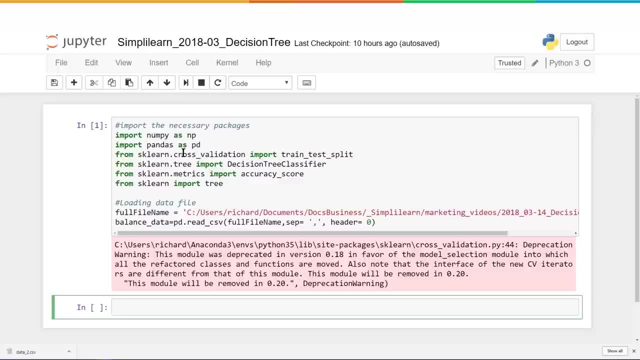 in favor of the model selection. So if we go up here, we have sklearn dot cross validation, and if you research this and go to the sklearn site, you'll find out that you can actually just swap it right in there with model selection. And so when I come in here and I run it again, that removes a warning. What? 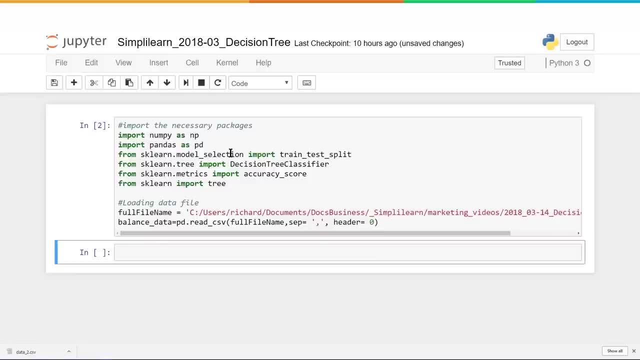 they've done is they've had two different developers develop it in two different branches, And then they decided to keep one of those and eventually get rid of the other one. That's all that is, And very easy and quick to fix. Before we go any further, I went ahead and opened up the data from 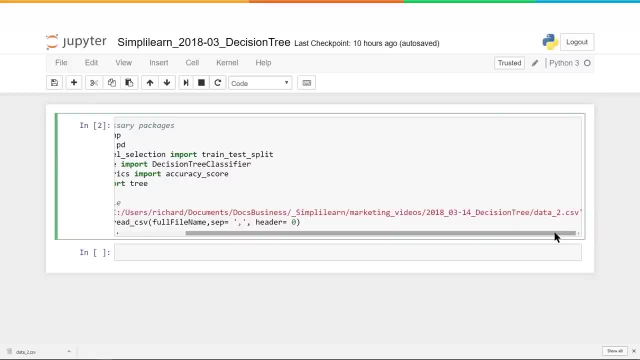 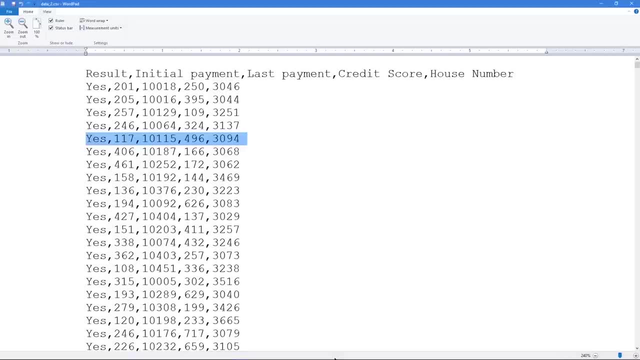 basic text file. You can see at the top they've created a header and it's got one, two, three, four, five columns and each column has data in it. And let me flip this over, because we're also gonna look at this in an actual spreadsheet, so you 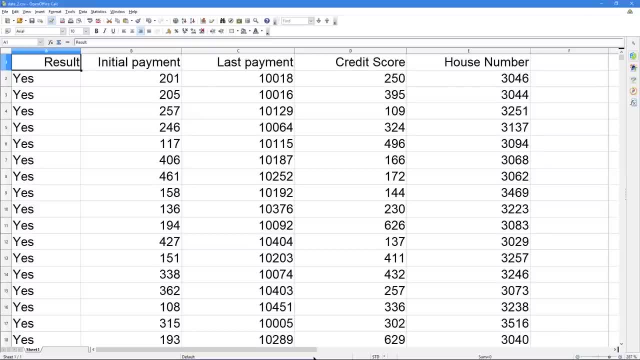 can see what that looks like And here I've opened it up in the OpenOffice calc, which is pretty much the same as Excel, and zoomed in and you can see we've got our columns and our rows of data A little easier to read. in here We have a 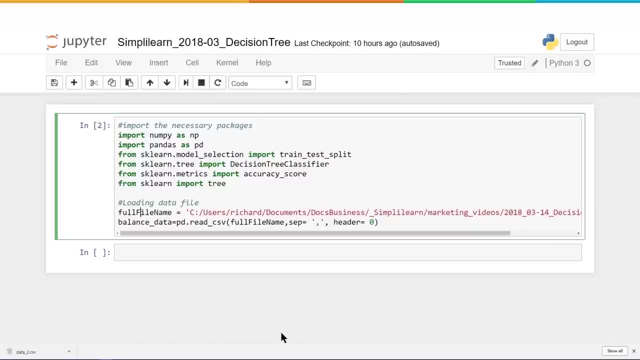 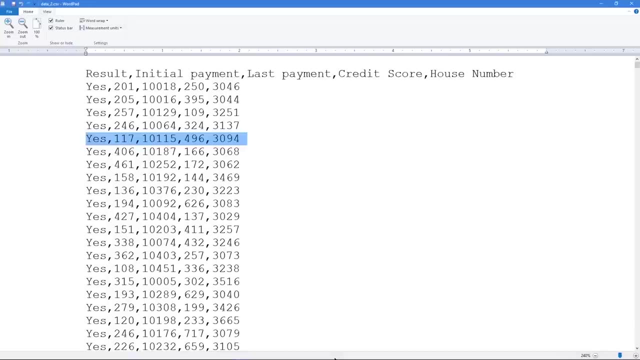 both as a text file, because it's a comma separated variable file- and in a spreadsheet. This is what it looks like as a basic text file. You can see at the top they've created a header and it's got one, two, three. 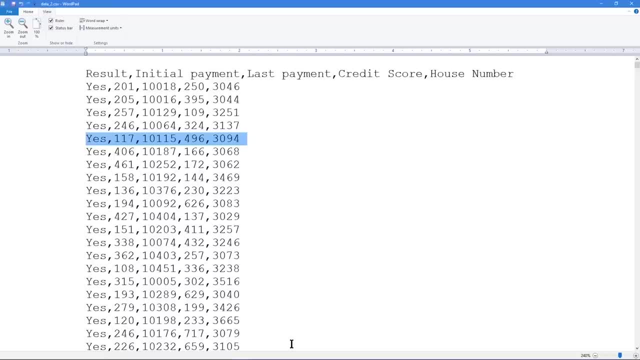 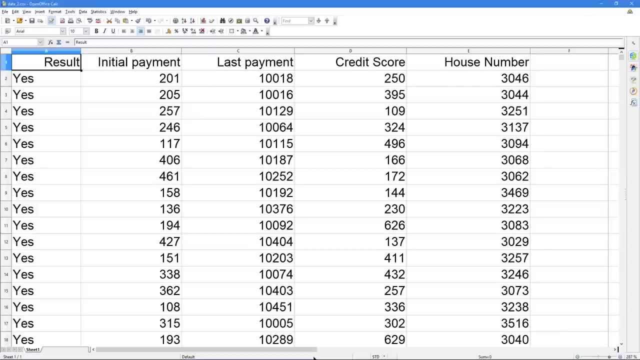 four, five columns and each column has data in it. And let me flip this over because we're also going to look at this in an actual spreadsheet. so you can see what that looks like. And here I've opened it up in the open office, calc. 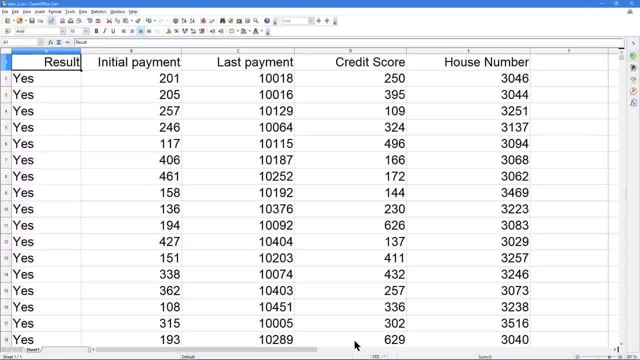 which is pretty much the same as Excel, and zoomed in And you can see we've got our columns and our rows of data a little easier to read. in here We have a result. Yes, yes, no, We have initial payment. last payment: credit score, house number. 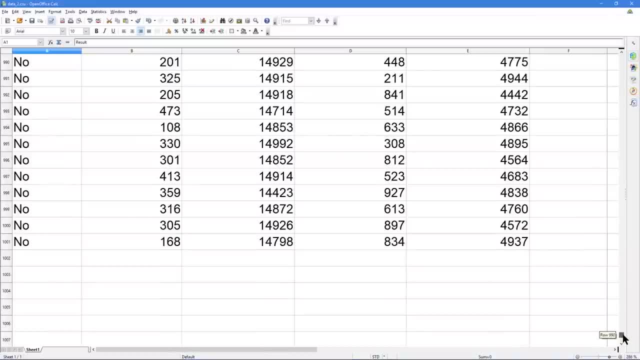 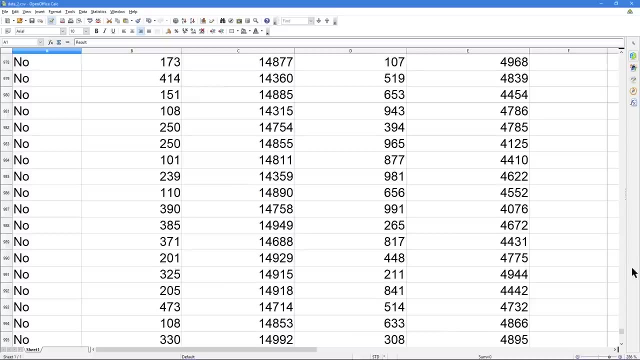 If we scroll way down, we'll see that this occupies a thousand and one lines of code or lines of data, with the first one being a column and then a thousand lines of data. Now, as a programmer, if you're looking at a small amount of data, 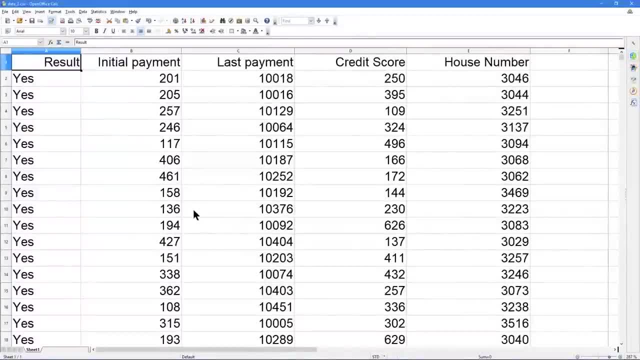 I usually start by pulling it up in different sources so I can see what I'm working with. But in larger data you won't have that option. It would just be too, too large. You need to either bring in a small amount that you can look at it like we're doing. 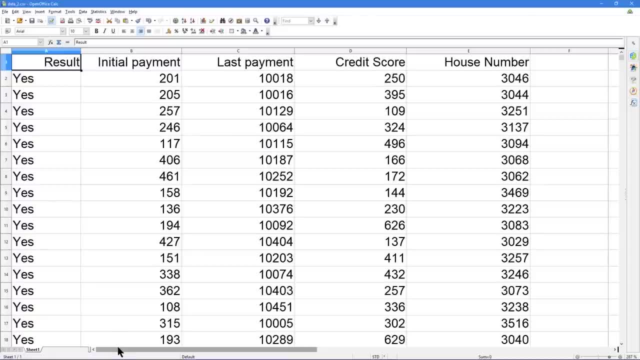 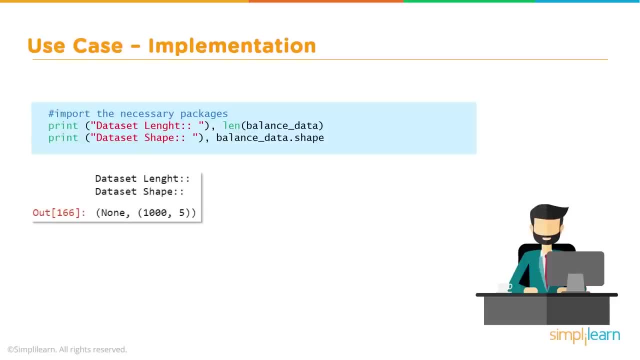 right now, or we can start looking at it through the Python code. So let's go ahead and move on and take the next couple of steps to explore the data in Python. Let's go ahead and see what it looks like in Python to print the length and the shape of the data. 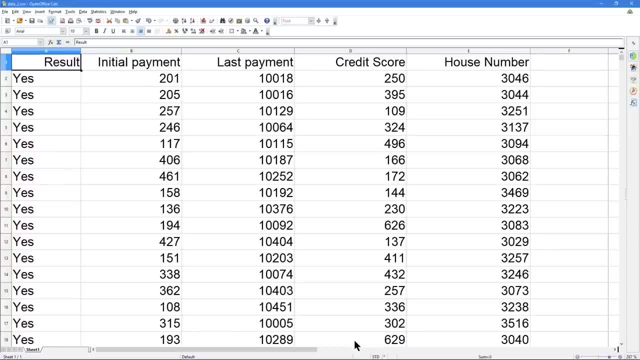 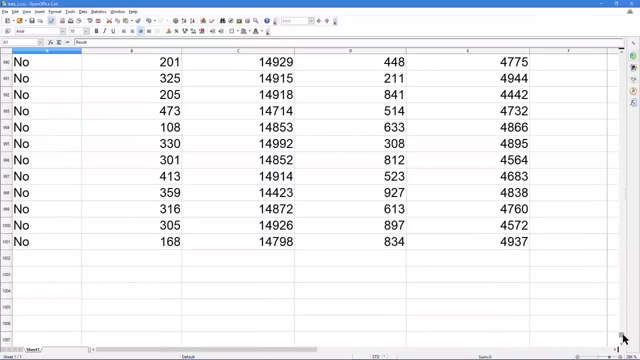 result: Yes, yes, no, We have initial payment, last payment. credit score house number. If we scroll way down, we'll see that this occupies a thousand and one lines of code or lines of data, with the first one being a column and then one thousand lines of data. 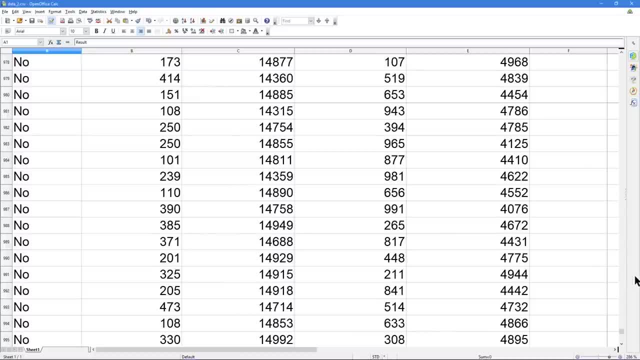 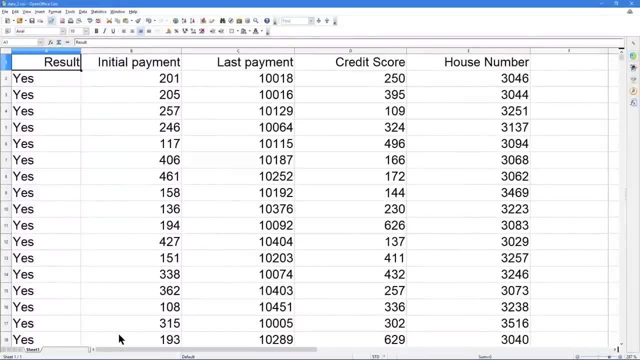 Now, as a programmer, if you're looking at a small amount of data, I usually start by pulling it up in different sources so I can see what I'm working with. But in larger data you won't have that option. There'll just be two large. So you need to either bring in a small amount that you can look at it like 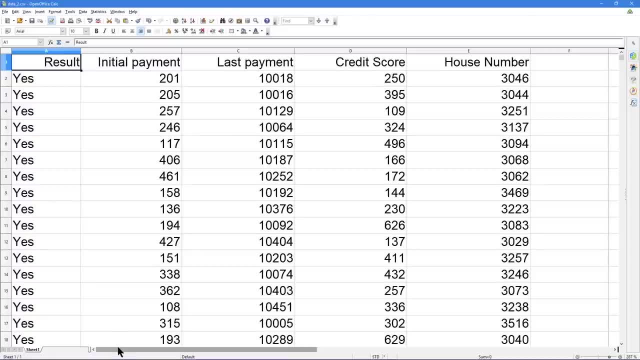 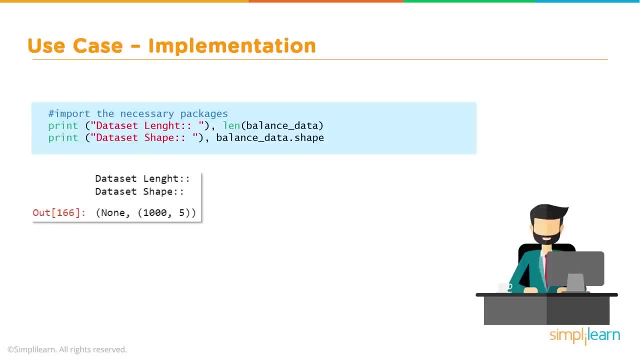 we're doing right now, or we can start looking at it through the Python code. So let's go ahead and move on and take the next couple steps to explore the data using Python. Let's go ahead and see what it looks like in Python to print the. 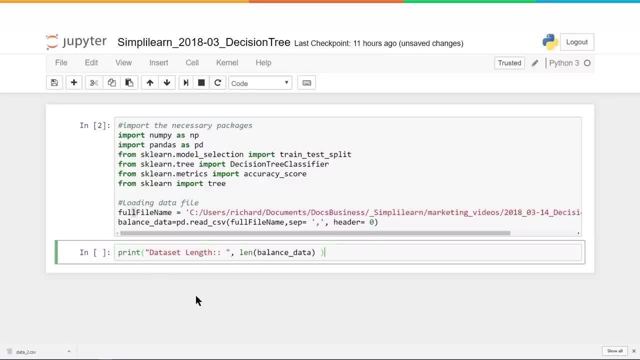 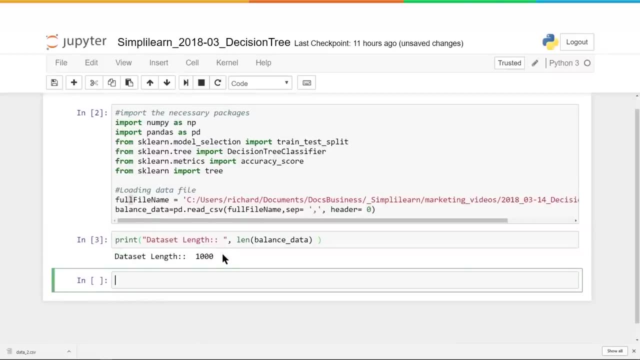 length and the shape of the data. So let's start by printing the length of the database. We can use a simple lin function from Python, And when I run this, you'll see that it's a thousand long. and that's what we expected. There's a lot of data in here. 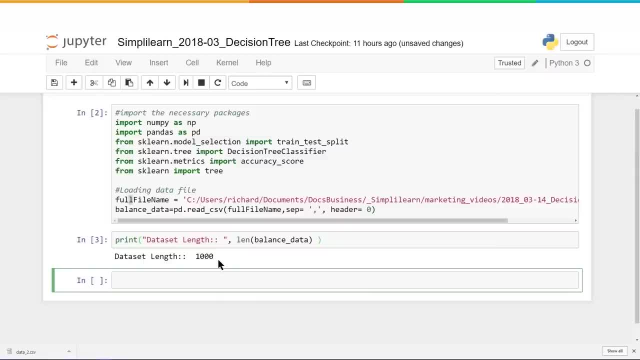 There's a thousand lines of data in there. if you subtract the column head. This is one of the nice things when we did the balance data from the Panda. read CSV. you'll see that the header is row zero, so it automatically removes a row and then shows the data separate. It does a good job sorting that data out for us. 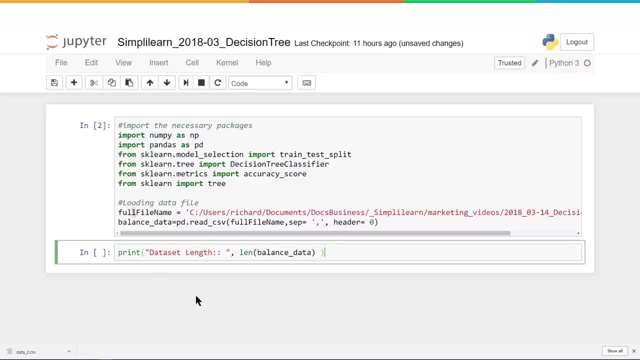 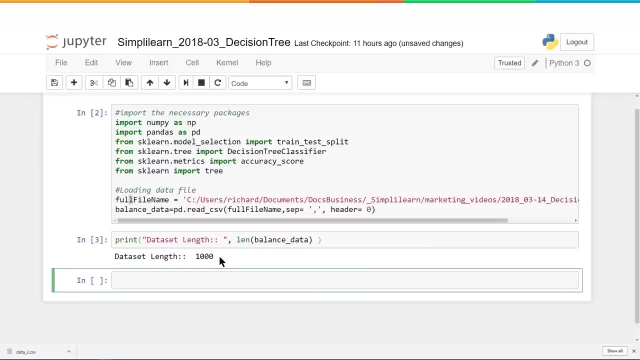 So let's start by printing the length of the database. We can use a simple lin function from Python, And when I run this, you'll see that it's a thousand long, And that's what we expected. There's a thousand lines of data in there if you subtract the column head. 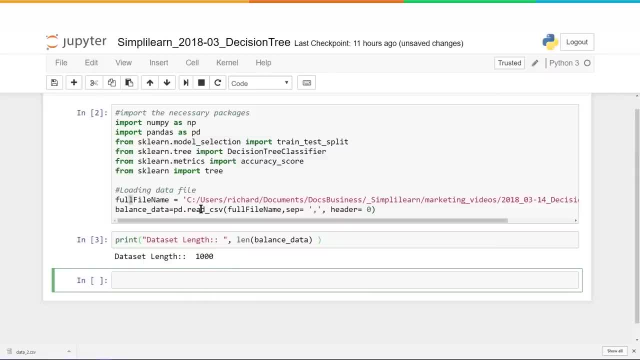 This is one of the nice things When we did the balance data from the Panda. read CSV. you'll see that the header is row zero, so it automatically removes a row And then shows the data separate. It does a good job sorting that data out for us. 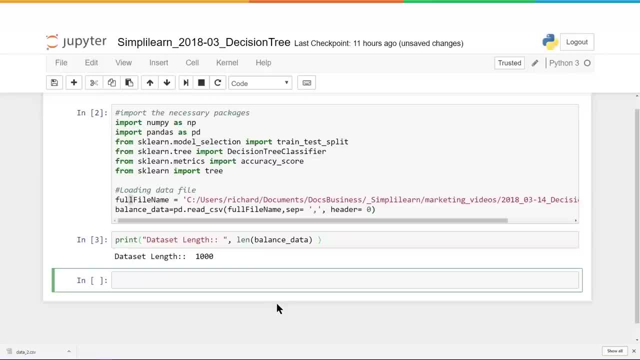 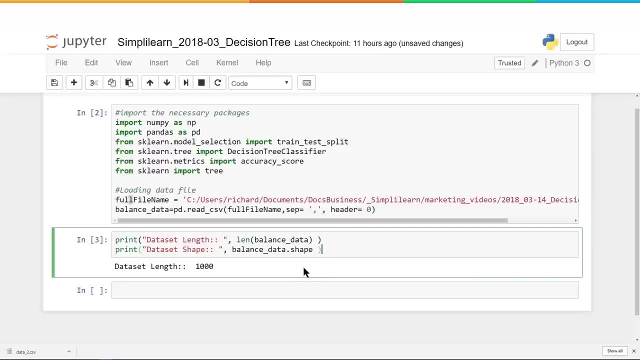 And then we can use a different function and let's take a look at that. And again, we're going to utilize the tools in Panda And since the balance underscore data was loaded as a Panda data frame, we can do a shape on it, And let's go ahead and run the shape and see what. 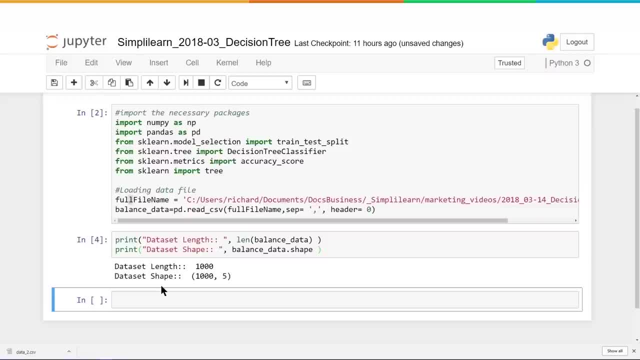 that looks like. What's nice about this shape is not only does it give me the length of the data- we have a thousand lines- it also tells me there's five columns. So we were looking at the data. we had five columns of data, And then 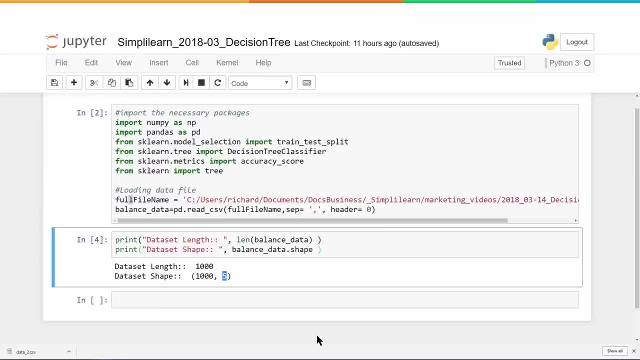 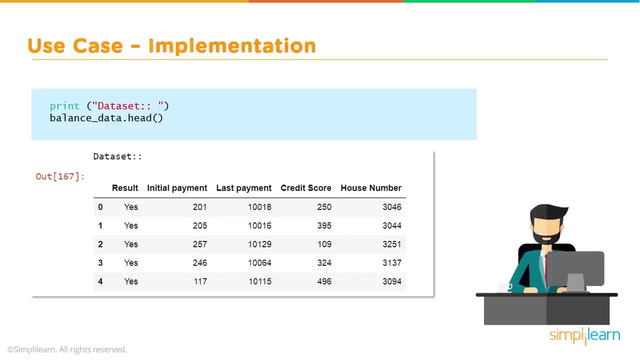 let's take one more step to explore the data using Python, And now that we've taken a look at the length and the shape, let's go ahead and use the Pandas module for head- Another beautiful thing in the data set that we can utilize. So 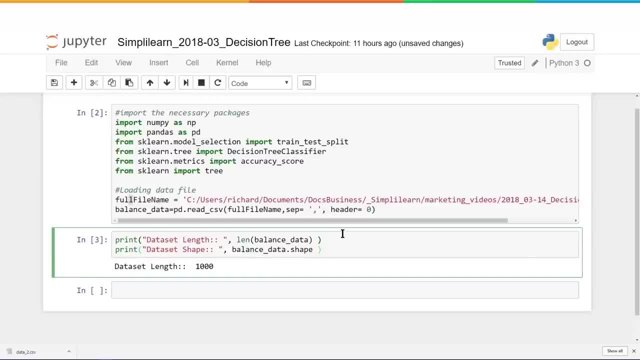 And then we can use a different function and let's take a look at that. And again, we're going to utilize the tools in Panda And since the balance underscore data was loaded as a Panda data frame, we can do a shape on it and let's go ahead and run the shape and see what that looks like. 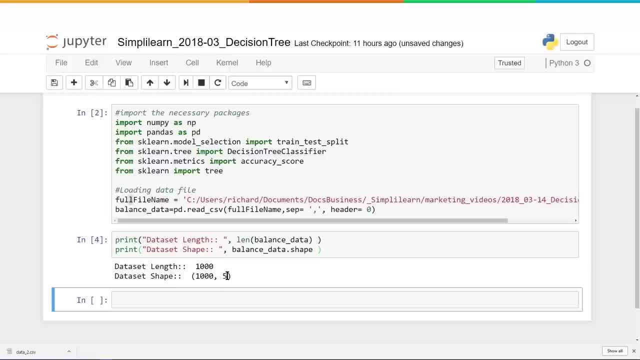 What's nice about the shape is not only does it give me the length of the data- we have a thousand lines- It also tells me there's five columns. So we were looking at the data. We had five columns of data. And then let's take one more step to explore the data using Python. 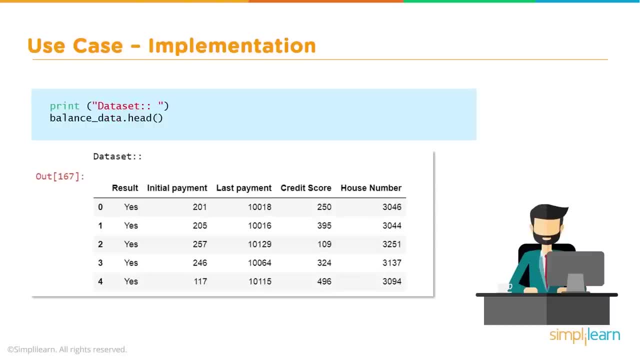 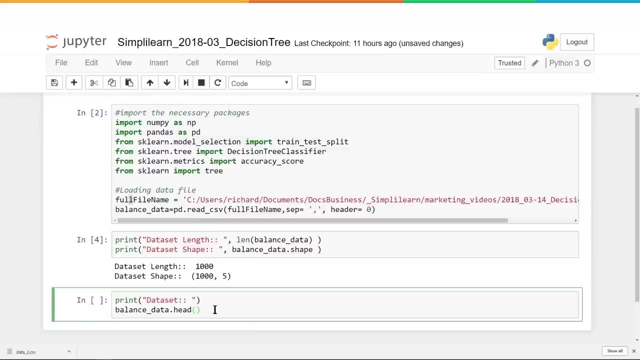 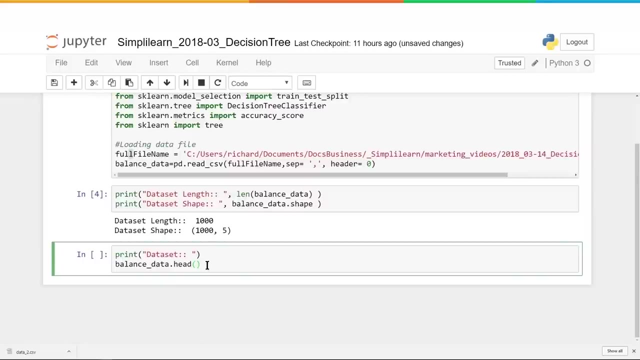 And now that we've taken a look at the length and the shape, let's go ahead and use the Pandas module for head- another beautiful thing in the data set that we can utilize. So let's put that on our sheet here And we have print data set and balance data dot head. 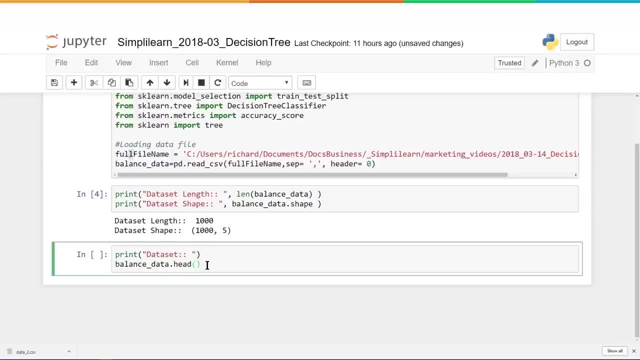 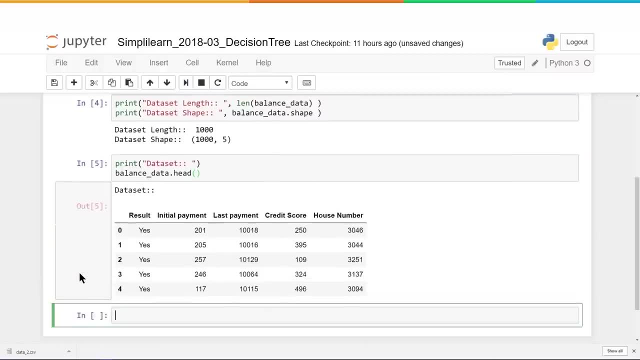 And this is a Pandas print statement of its own, So it has its own print feature in there. And then we went ahead and gave a label for our print job here of data set, just a simple print statement, And we run that and let's just take a closer look at that. 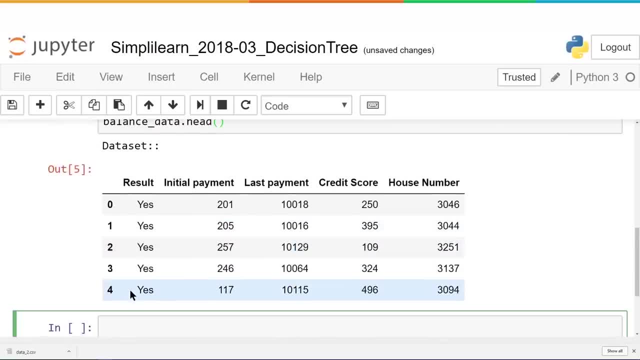 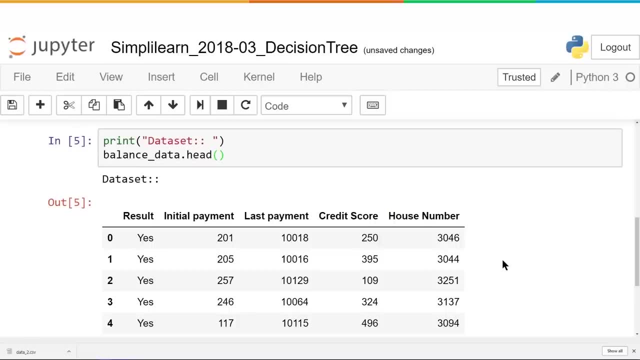 Let me zoom in here. There we go. Pandas does such a wonderful job of making this a very clean, readable data set, So you can look at the data. you can look at the column headers. You can have it when you put it as the head. 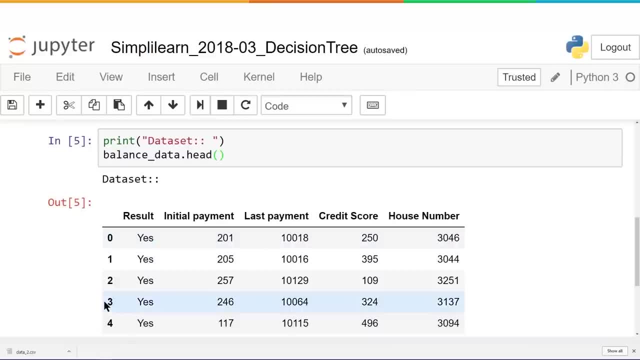 It pulls the first five lines of the data and we always start with zero. So we have five lines. We have zero. one, two, three, four, instead of one, two, three, four, five. That's a standard scripting and programming. 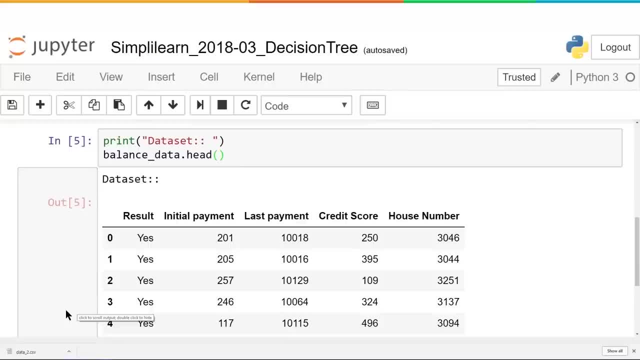 set is you want to start with the zero position, And that is what the data head does. It pulls the first five rows of data, puts it in a nice format that you can look at and view. very powerful tool to view the data. So, instead of having to flip and open up, 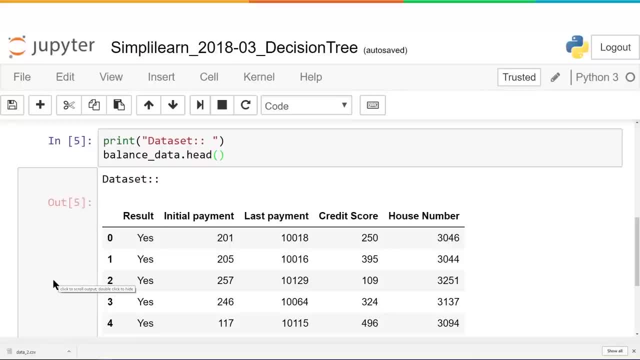 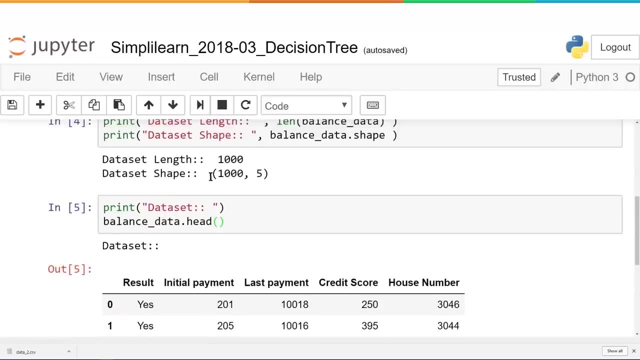 an Excel spreadsheet or open Office, Cal, or trying to look at a Word doc where it's all scrunched together and hard to read. you can now get a nice, open view of what you're working with. We're working with a shape of a thousand long, five wide. 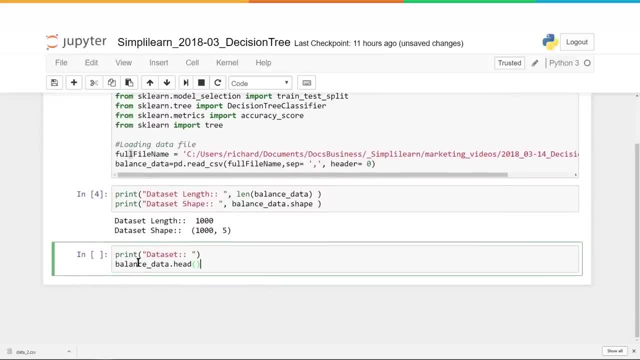 let's put that on our sheet here. And we have print data set and balance data dot head. And this is a Pandas print statement of its own, So it has its own print feature in there. And then we went ahead and gave a label for a print job. 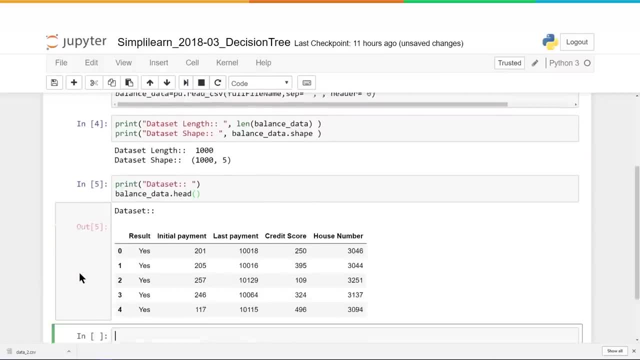 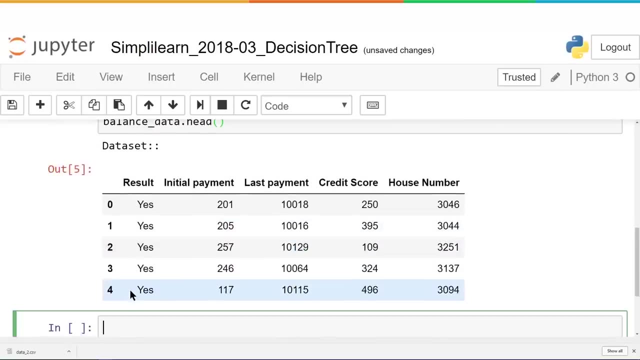 here of data set, Just a simple print statement, And when we run that and let's just take a closer look at that, Let me zoom in here. There we go. such a wonderful job of making this a very clean, readable data set so you can. 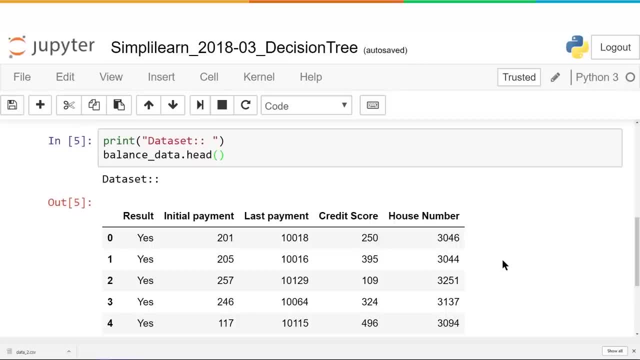 look at the data. you can look at the column headers. you can have it. when you put it as the head, it prints the first five lines of the data and we always start with zero. so we have five lines. we have zero. one, two, three, four instead of. 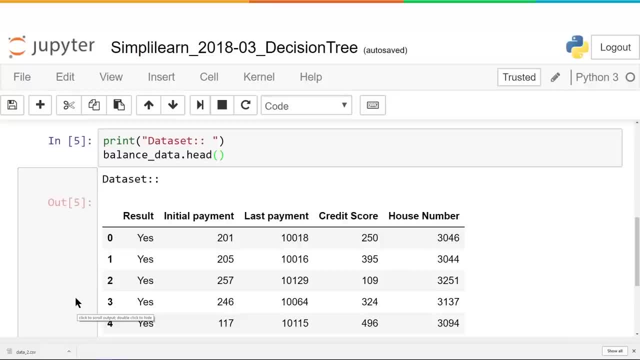 one, two, three, four, five. that's a standard scripting and programming set. is you want to start with the zero position? and that is what the data head does. it pulls the first five rows of data, puts in a nice format that you can look at and view. very powerful tool to view the data. so, instead of having to 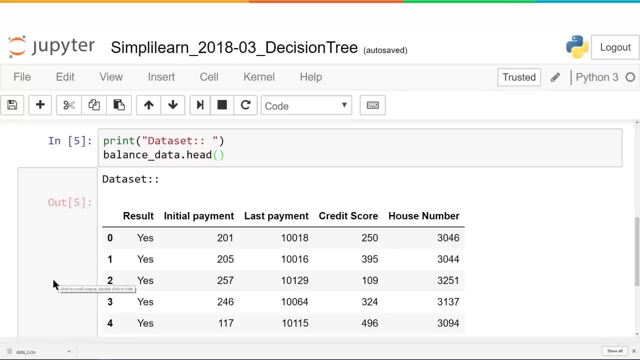 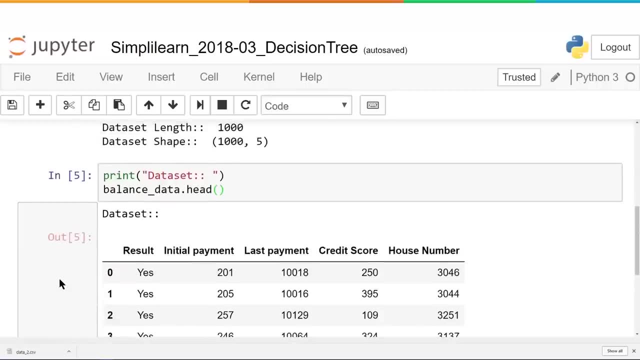 flip and open up an Excel spreadsheet or open office cal, or trying to look at a Word doc where it's all scrunched together and hard to read. you can now get a nice open view of what you're working with. we're working with the shape of a thousand long, five wide, so we have five columns and we do the full. 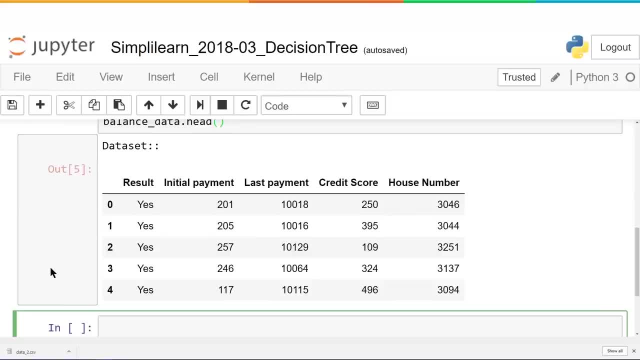 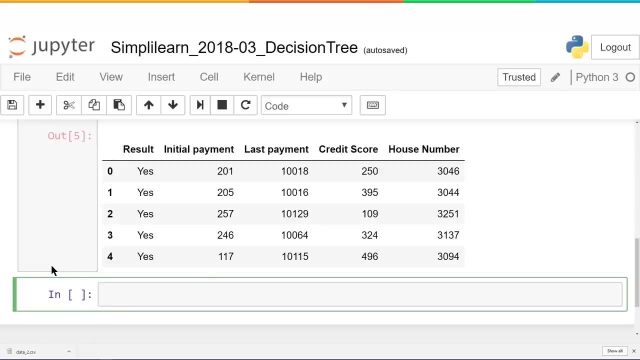 data head, you can actually see what this data looks like: the initial payment, last minute payment, credit scores, house number. So let's take this, now that we've explored the data, and let's start digging into the decision tree. So in our next step, 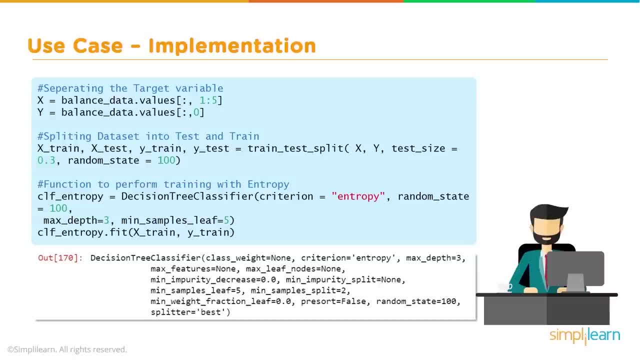 we're going to train and build our data tree and to do that we need to first separate the data out. We're going to separate into two groups so that we have something to actually train the data with and then we have some data on the side to test it, to see how good our model is. Remember, with any of the 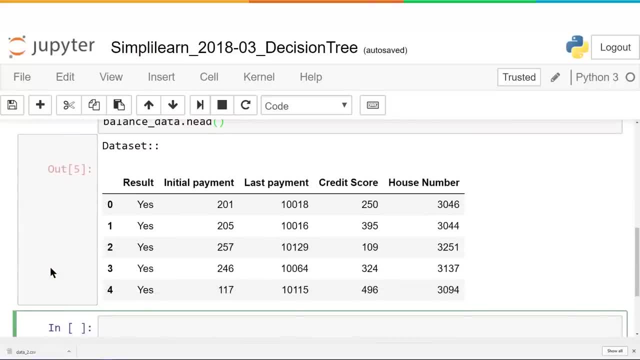 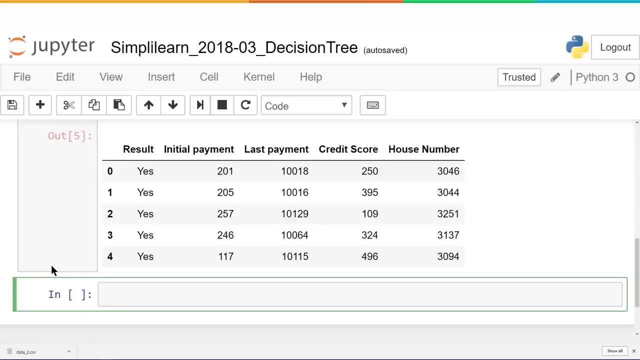 So we have five columns and we do the full data head. You can actually see what this data looks like: the initial payment, last payment, credit scores, house number. So let's take this, now that we've explored the data, and let's start digging into the decision tree. 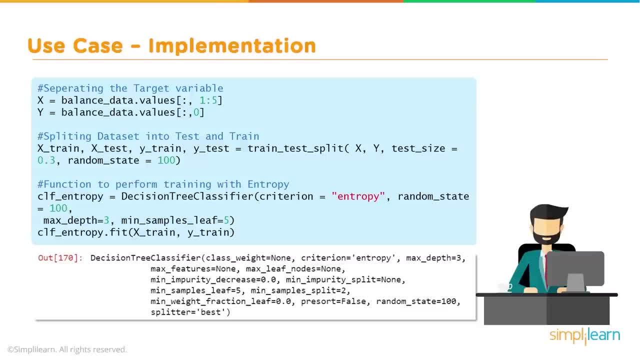 So in our next step we're going to train and build our data tree, And to do that we need to first separate the data out. We're going to separate into two groups so that we have something to actually train the data with. 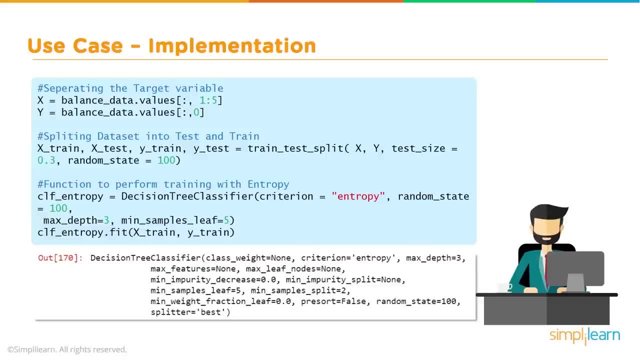 And then we have some data on the side to test it, to see how good our model is. Remember, with any of the machine learning you always want to have some kind of test set to weigh it against. So you know how good your model is when you distribute it. 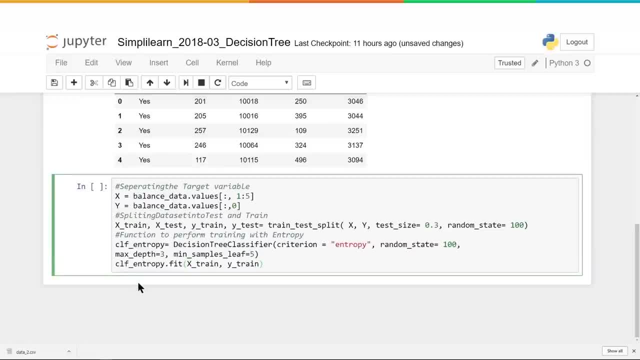 Let's go ahead and break this code down and look at it in pieces. So first we have our X and Y. Where do X and Y come from? Well, X is going to be our data and Y is going to be the answer or the target. You can look at it as source and target. 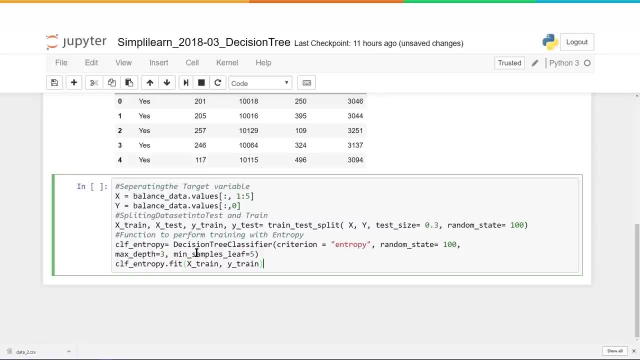 In this case, we're using X and Y to denote the data in and the data that we're actually trying to guess what the answer is going to be, And so to separate it we can simply put in: X equals the balance of the data values. 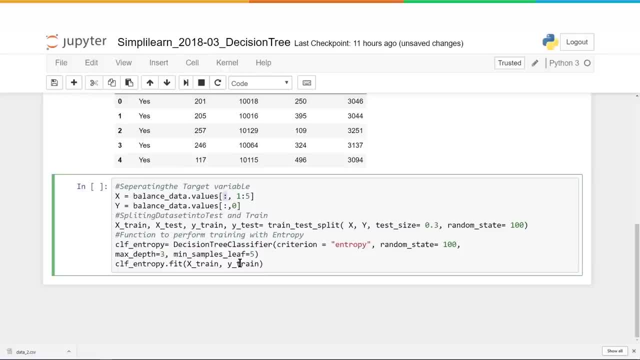 The first brackets means that we're going to select all the lines in the database, So it's all the data, And the second one says we're only going to look at columns one through five. Remember, we always start with zero. Zero is a yes or no. 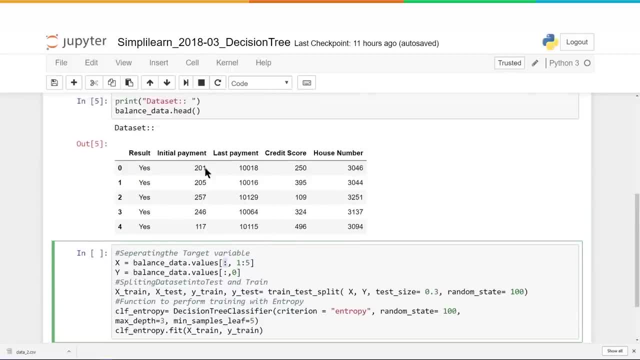 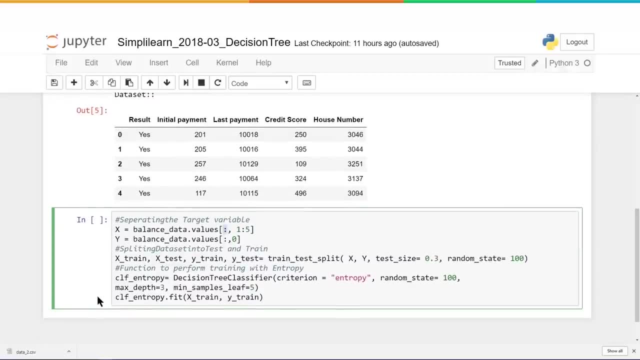 And that's whether the loan went default or not. So we want to start with one. If we go back up here, that's the initial payment And it goes all the way through the house number. Well, if we want to look at one through five, we can do the same thing for Y. 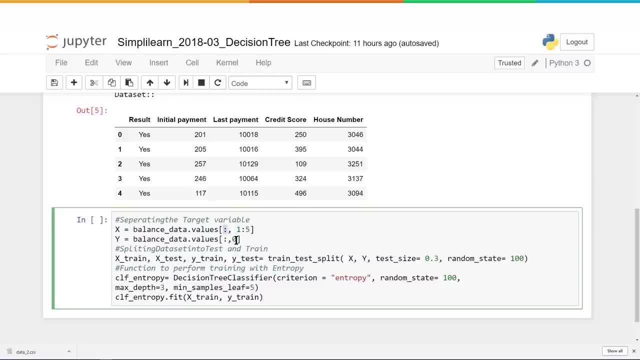 which is the answers, and we're going to set that just equal to the zero row. So it's just the zero row and then it's all rows going in there. So now we've divided this into two different data sets, one of them with the data. 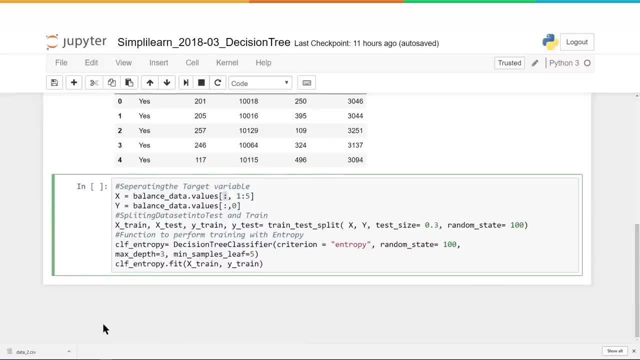 going in and one with the answers. Next, we need to split the data, And here you'll see that we have it split into four different parts. The first one is your X training your X test. your Y train your Y test. 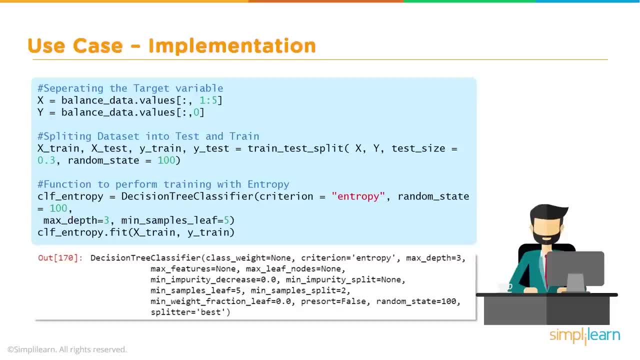 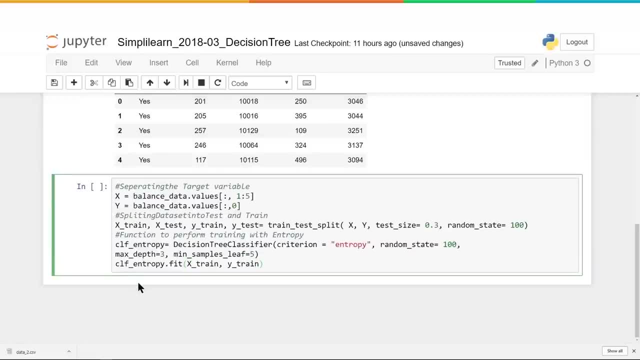 machine learning, you always want to have some kind of test set to weigh it against, so you know how good your model is when you distribute it. Let's go ahead and break this code down and look at it in pieces. So first we have our X and Y. 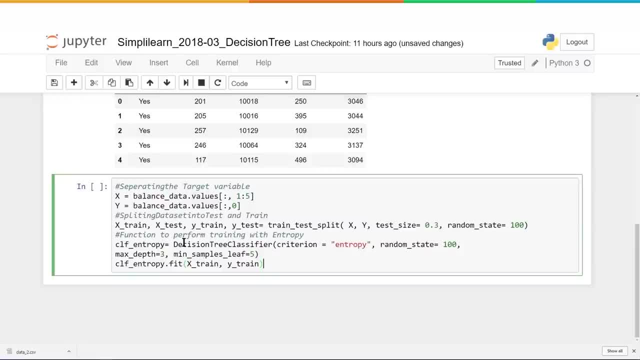 Where do X and Y come from? Well, X is going to be our data and Y is going to be the answer or the target. You can look at it: source and target. In this case, we're using X and Y to denote the data in and the data that we're actually. 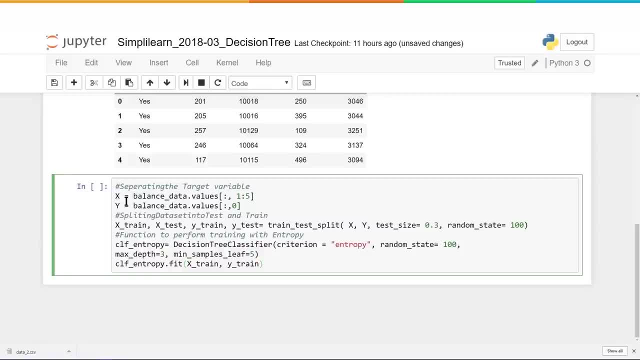 trying to guess what the answer is going to be, And so to separate it we can simply put in: X equals the balance of the data, datavalues. The first brackets means that we're going to select all the lines in the database, so it's all the data, And the second one says we're only going to 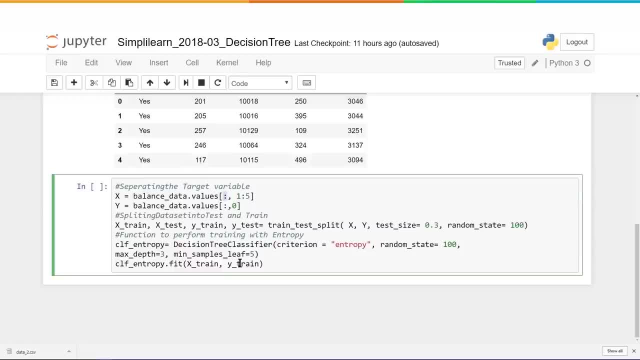 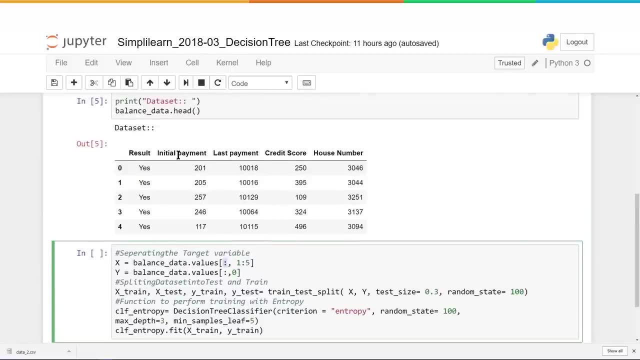 look at columns 1 through 5.. Remember, we always start with 0? 0 is a yes or no and that's whether the loan went default or not. So we want to start with 1.. If we go back up here, that's the initial payment and it goes all the way through the. 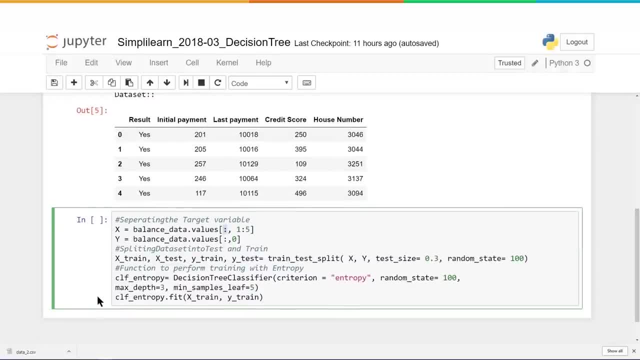 house number. Well, if we want to look at 1 through 5, we can do the same thing for Y, which is the answers, And we're going to set that just equal to the 0 row. So it's just the 0 row, and then it's all rows going in there. So now we've 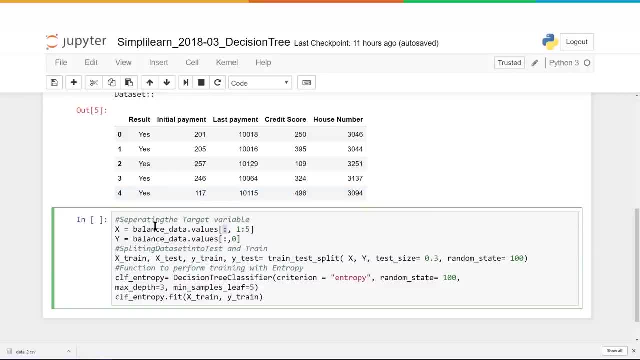 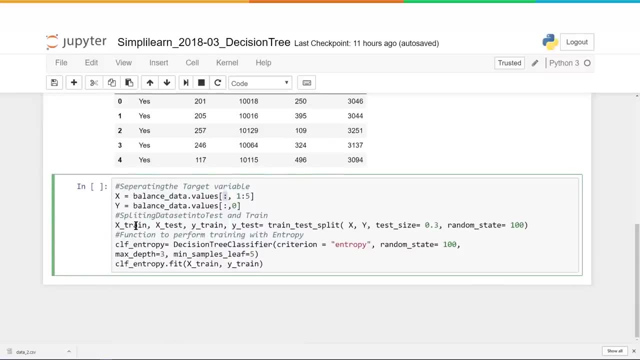 divided this into two different data sets, One of them with the data going in and one with the answers. Next we need to split the data, And here you'll see that we have it split into four different parts. The first one is your X training- your X test, your Y train, your Y test. 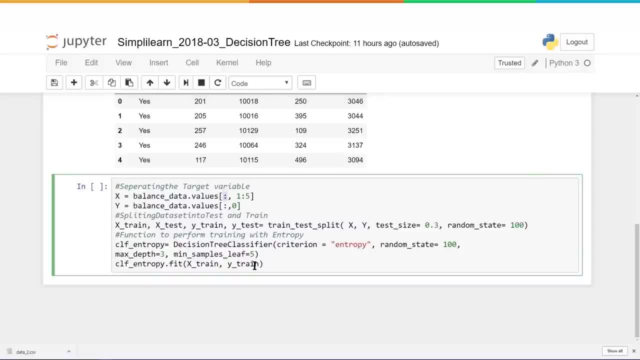 Simply put, we have X going in where we're going to train it and we have to know the answer to train it with. And then we have X test, where we're going to test that data And we have to know in the end, what the Y was supposed to be. 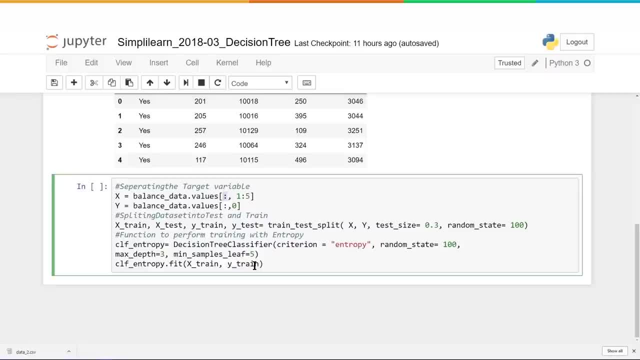 And that's where this train test split comes in that we loaded earlier in the modules. This does it all for us And you can see they set the test size equal to 0.3.. So it's roughly 30% will be used in the test And then we use a random state. so 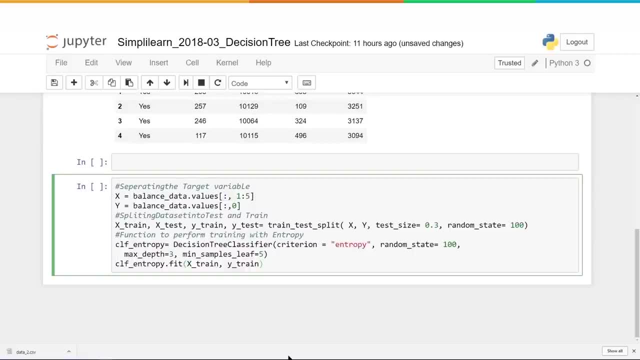 it's completely random which rows it takes out of there. And then finally we get to actually build our decision tree And they've called it here CLF, underscore entropy. That's the actual decision tree, or decision tree classifier, And in here they've added a couple variables which we'll explore in just a minute. And then 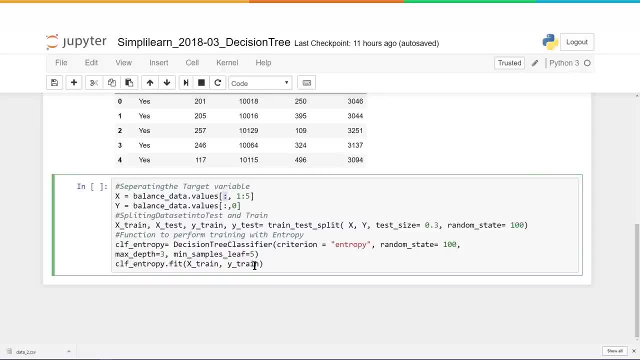 Simply put, we have X going in where we're going to train it and we have to know the answer to train it with. and then we have X test where we're going to use that data and we have to know, in the end, what the Y was supposed to be. 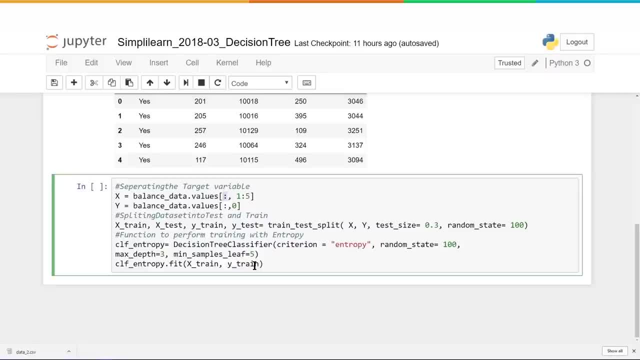 And that's where this train test split comes in that we loaded earlier in the modules. This does it all for us And you can see they set the test size equal to point three, So it's roughly 30 percent will be used in the test. 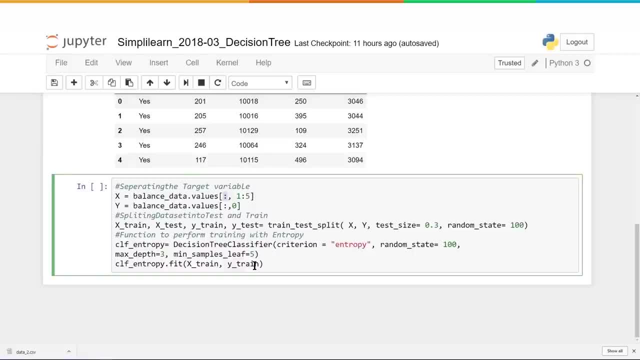 And then we use a random state, So it's completely random which rows it takes out of there. And then finally we get to actually build our decision tree And they've called it here CLF, underscore entropy. That's the actual decision tree or decision. 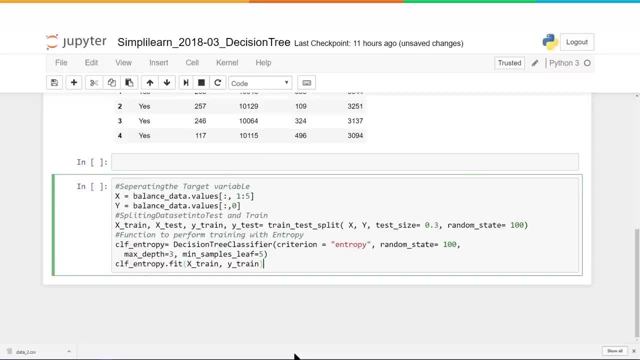 tree classifier, And in here they've added a couple of variables which we'll explore in just a minute. And then, finally, we need to fit the data to that. So we take our CLF entropy that we created and we fit the X train. 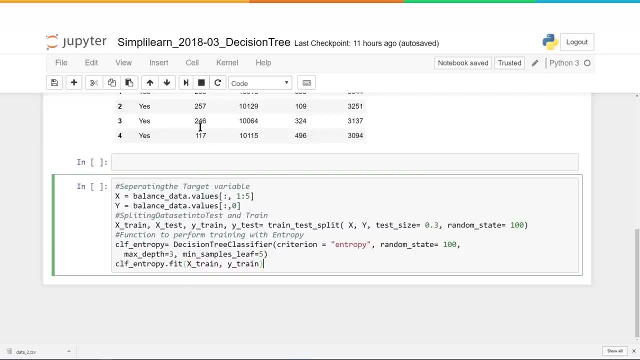 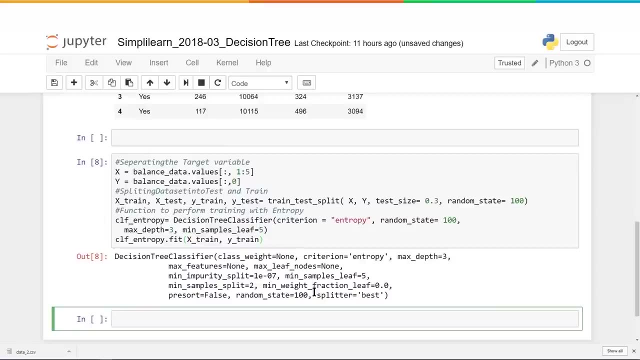 And since we know the answers for X train or the Y train, we go and put those in and let's go ahead and run this. And what most of these SKLearn modules do is when you set up the variable, in this case we set the CLF entropy: equal decision tree classifier. 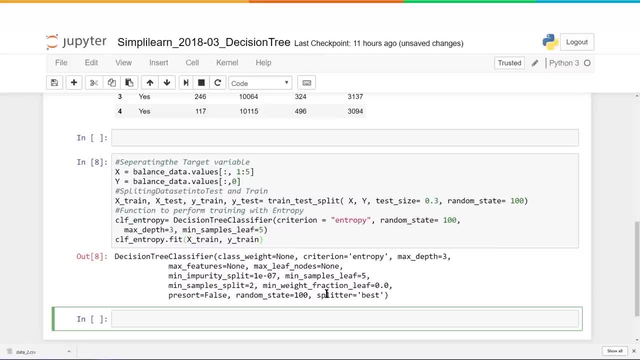 It automatically prints out what's in that decision tree. There's a lot of variables you can play with in here And it's quite beyond the scope of this tutorial to go through all of these and how they work. But we're working on entropy. 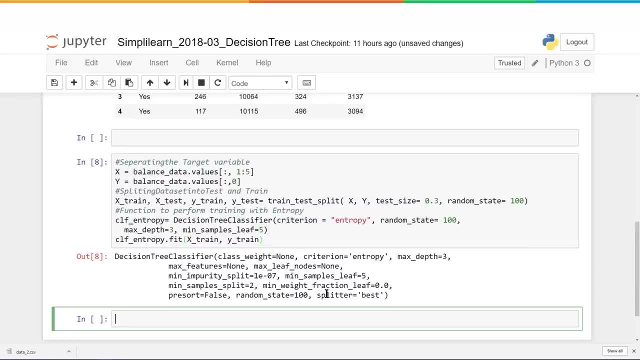 That's one of the options. We've added that it's completely a random state of 100.. So 100 percent And we have a max depth of three. Now the max depth, if you remember above when we were doing the different graphs of animals, means it's only going to go down three. 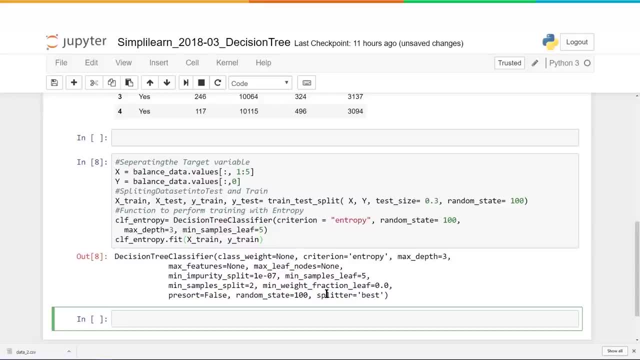 layers before it stops- and then we have minimal samples of leafs- is five, So it's going to have at least five leafs at the end. So we'll have at least three splits. We'll have no more than three layers and at least five in leafs, with the final. 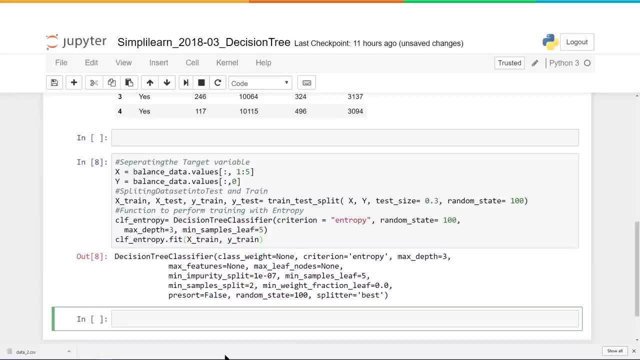 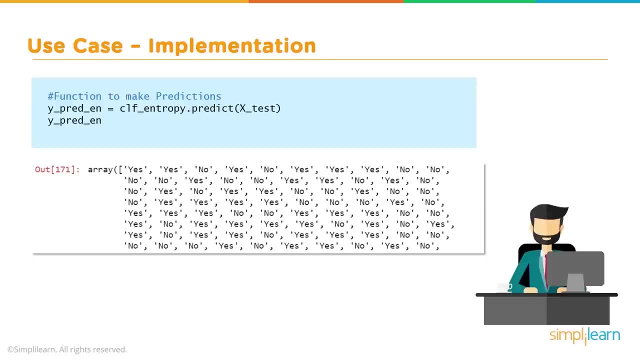 result at the bottom. now that we've created our decision tree classifier- not only created it, but trained it- Let's go ahead and apply it and see what that looks like. So let's go ahead and make a prediction and see what that looks like. 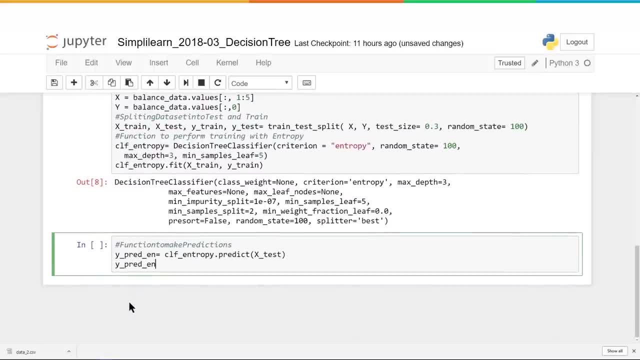 We're going to paste our predict code in here And before we run it, let's just take a quick look at what it's doing. here. We have a variable- Why predict it? Let's do, and we're going to use our variable, CLF entropy- that we created. 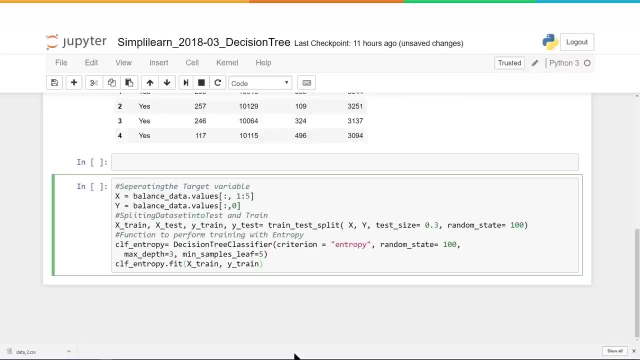 finally, we need to fit the data to that. So we take our CLF entropy that we created and we fit the X train And since we know the answers for X train or the Y train, we go ahead and put those in And let's go ahead and run this. 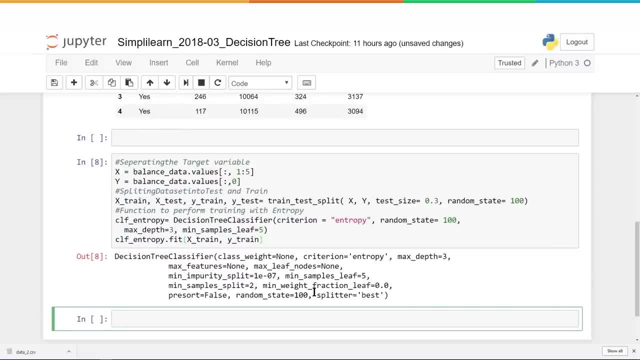 And what most of these sklearn modules do is when you set up the variable- in this case we set the CLF entropy equal to the decision tree classifier- it automatically prints out what's in that decision tree. There's a lot of variables you can play. 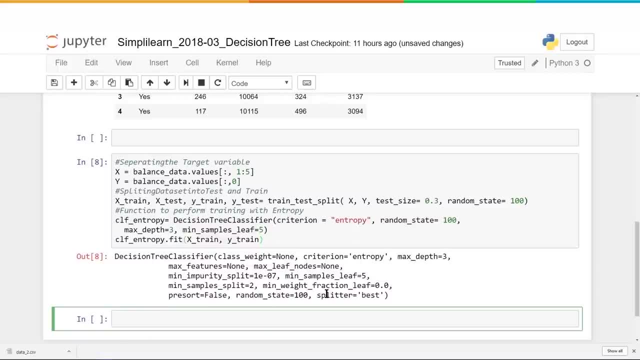 with in here And it's quite beyond the scope of this tutorial to go through all of these and how they work. But we're working on entropy. That's one of the options We've added that it's completely a random state of 100.. So 100%, and we've added 100% relative to this. 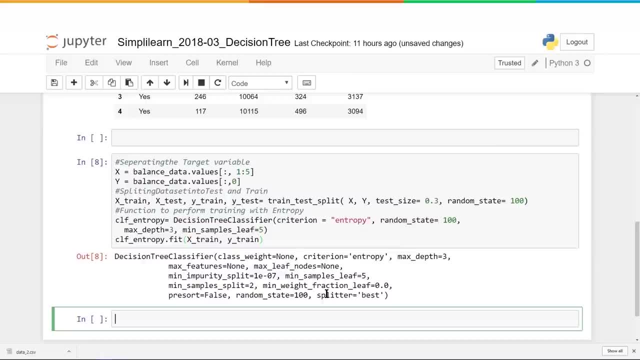 we have a max depth of three. Now the max depth- if you remember above when we were doing the different graphs of animals, means it's only gonna go down three layers before it stops, And then we have minimal samples of leaves- is five. 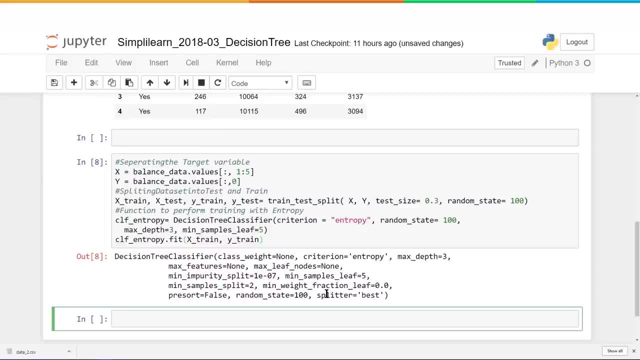 So it's gonna have at least five leaves at the end. So I'll have at least three splits, I'll have no more than three layers and at least five end leaves, with the final result at the bottom. Now that we've created our decision, tree classifier. 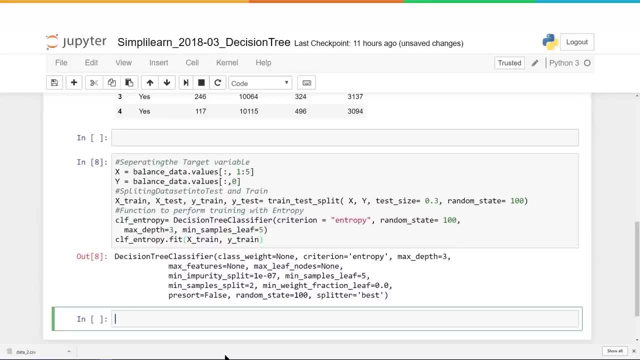 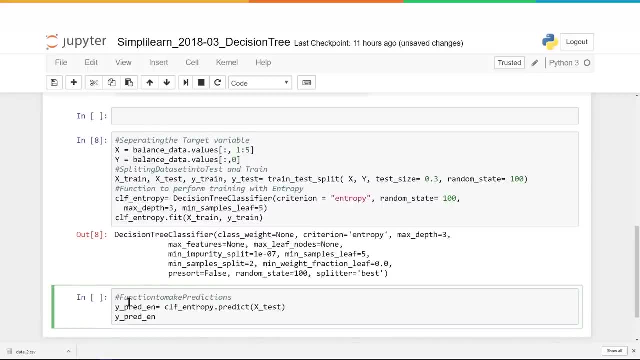 not only created it, but trained it. let's go ahead and apply it and see what that looks like. So let's go ahead and make a prediction and see what that looks like. We're gonna paste our predict code in here And, before we run it, 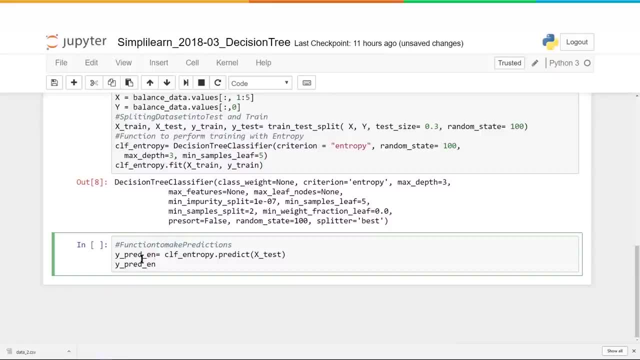 let's just take a quick look at what's it's doing here. We have a variable Y predict that we're gonna do And we're gonna use our variable CLF entropy that we created And then you'll see dot predict And it's very common in the SKLearn modules. 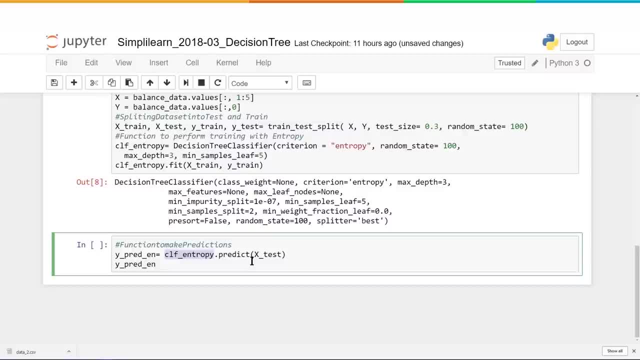 that their different tools have the predict when you're actually running a prediction. In this case, we're gonna put our X test data in here. Now, if you delivered this for use- an actual commercial use- and distributed it, this would be the new loans you're putting in here. 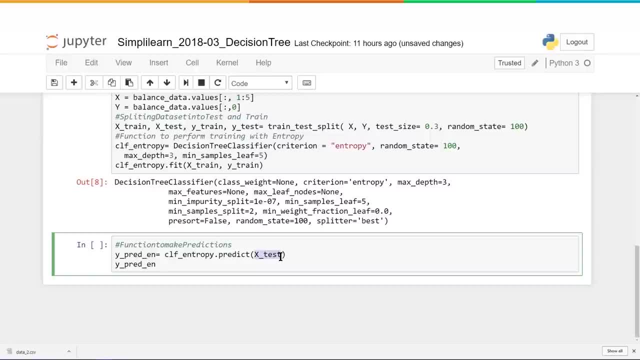 to guess whether the person's gonna pay them back or not. In this case, though, we need to test out the data and just see how good our sample is, how good of our tree does at predicting the loan payments. And finally, since Anaconda Jupyter Notebook works as a command line, 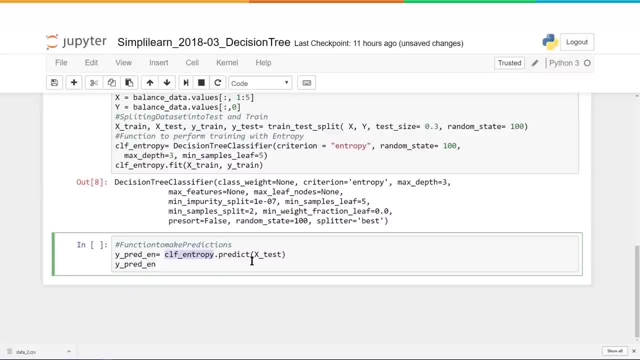 And then you'll see that predict- and it's very common in the SK learn modules that they're different tools- have the predict when you're actually running a prediction. in this case, we're going to put our X test data in here Now, if you delivered this for use and actual commercial use- and distributed it. 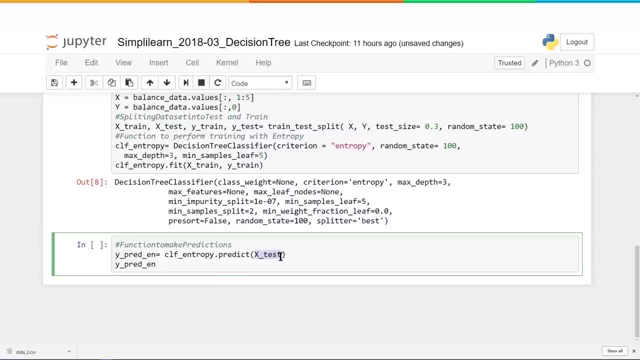 this would be the new loans you're putting in here- to guess Whether the person is going to be pay them back or not In this case. so we need to test out the data and just see how good our sample is, how good of our tree does at predicting the loan payments. 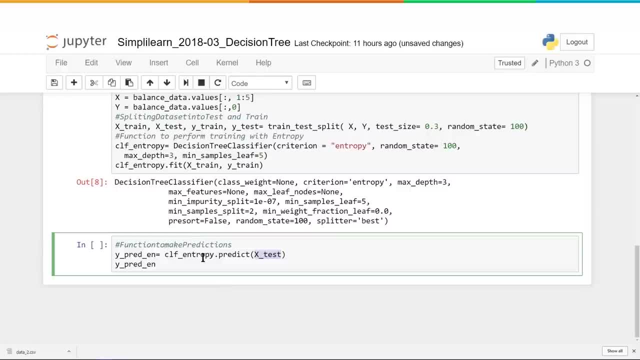 And finally, since Anaconda Jupyter Notebook works as a command line for Python, we can simply put the Y predict to print it. I could just as easily put the print And put brackets around Y predict to print it out and do that. 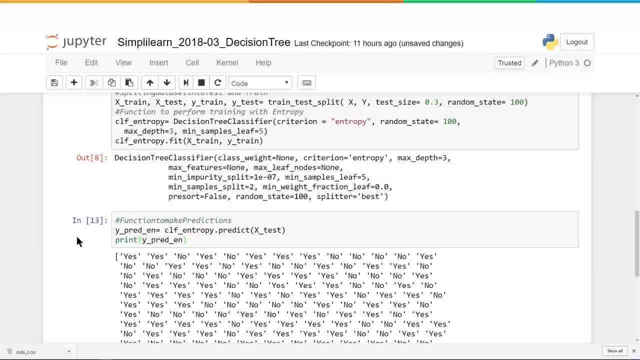 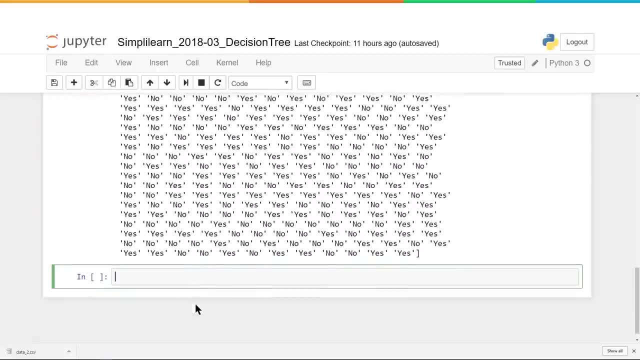 it doesn't matter which way you do it And you'll see right here that it runs a prediction. This is roughly 300 in here. Remember it's 30% of 1000.. So you should have about 300 answers in here. 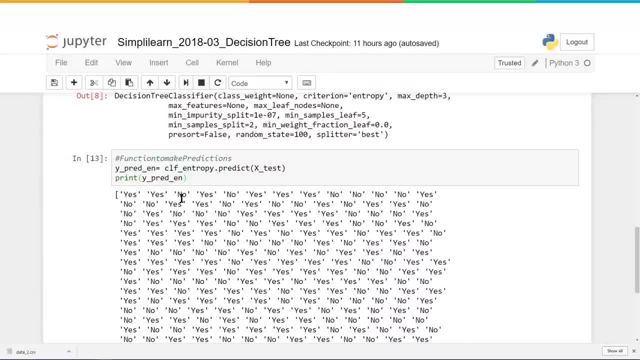 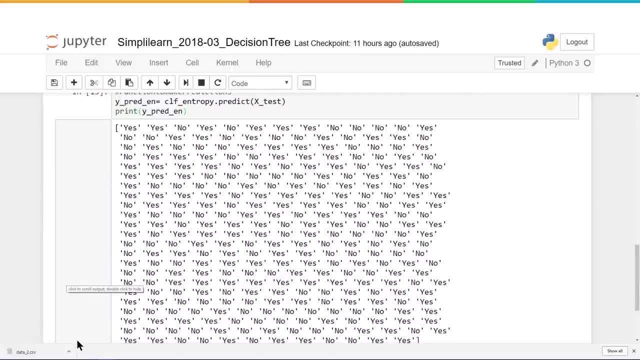 And this tells you which each one of those lines of our test went in there, And this is what our Y predict came out. So let's move on to the next step. We're going to take this data and try to figure out just how good a model we have. 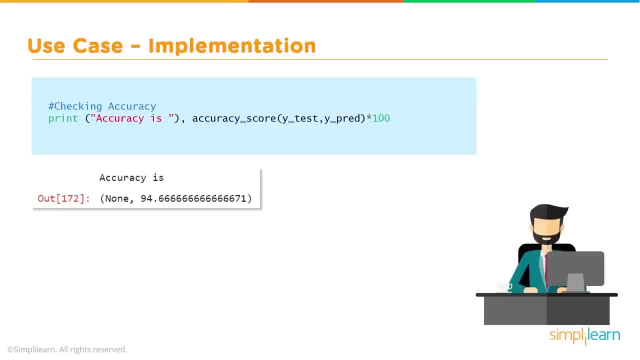 So here we go. Since SK learn does all the heavy lifting for you and all the math, we have a simple line of code To let us know what the accuracy is, And let's go ahead and go through that and see what that means and what that looks like. 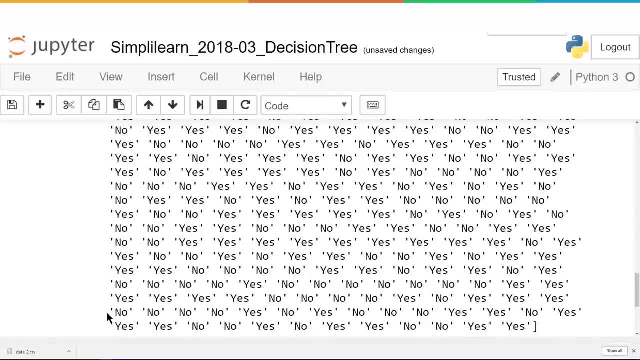 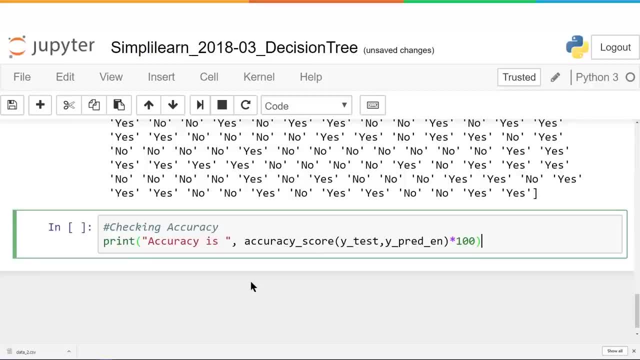 Let's go ahead and paste this in And let me zoom in a little bit. There we go, So you have a nice full picture And we'll see. here we're just going to do a print. accuracy is, And then we do the accuracy score. 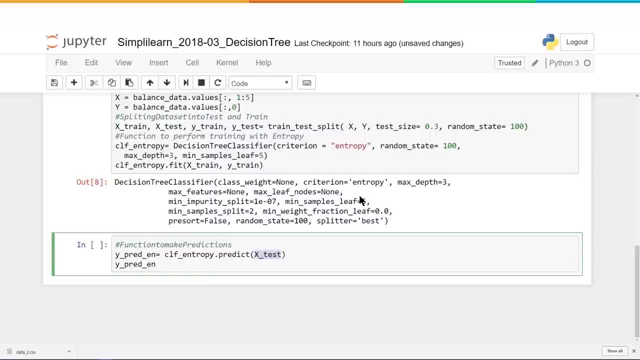 for Python we can simply put the Y predict E in to print it. I could just as easily have put the print and put brackets around Y predict E in to print it out. We'll go ahead and do that. It doesn't matter which way you do it. 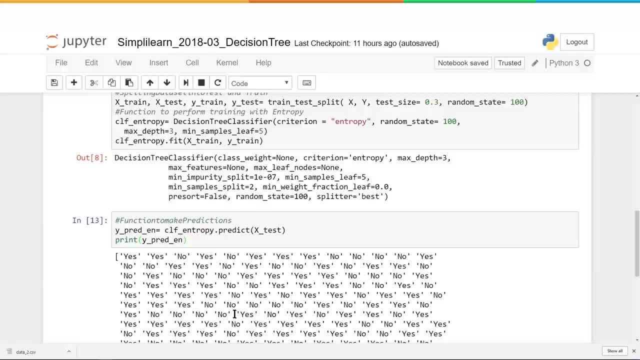 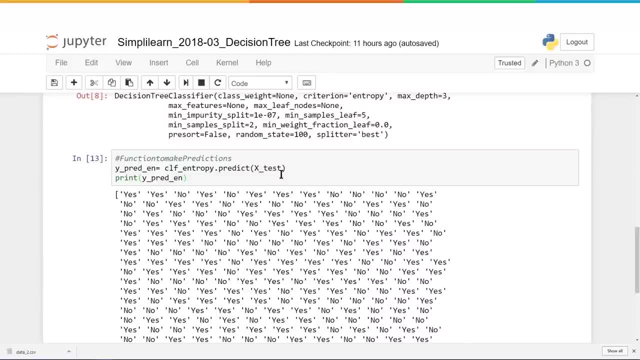 And you'll see right here that it runs a prediction. This is roughly 300 in here. Remember it's 30% of 1,000.. So you should have about 300 answers in here And this tells you which each one of those lines. 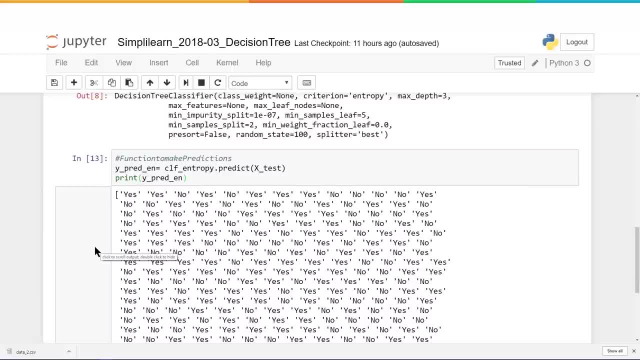 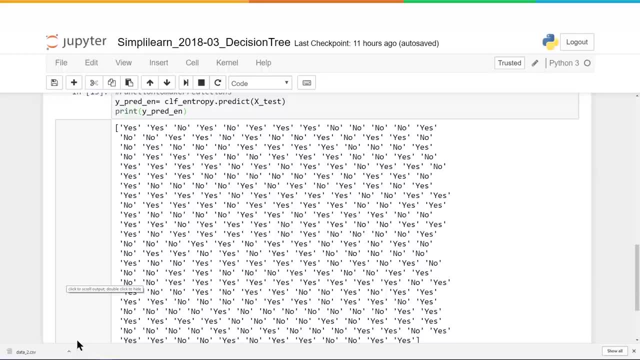 of our test went in there, And this is what our Y predict came out. So let's move on to the next step. We're gonna take this data and try to figure out just how good a model we have. So here we go. 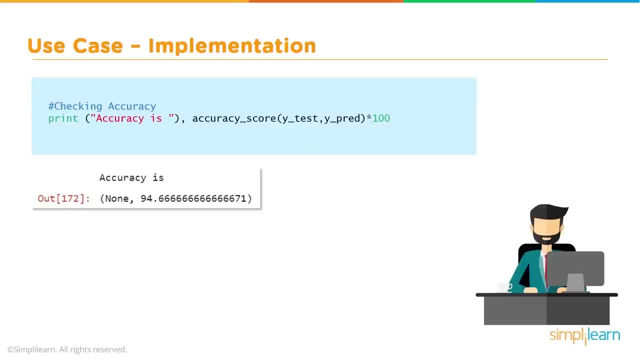 Since sklearn does all the heavy lifting for you and all the math, we have a simple line of code to let us know what the accuracy is, And let's go ahead and go through that and see what that means and what that looks like. Let's go ahead and paste this in. 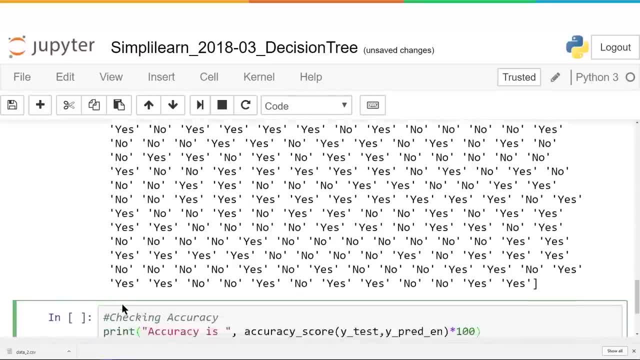 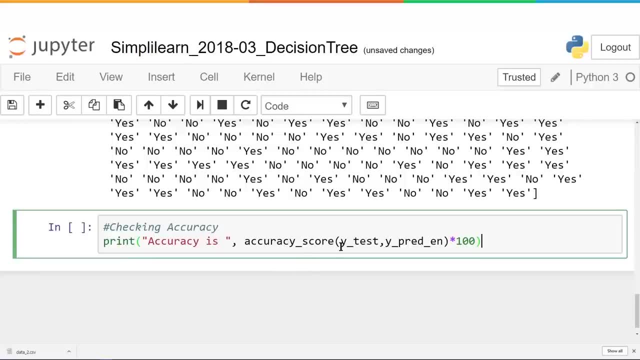 And let me zoom in a little bit. There we go. So you have a nice full picture And we'll see. here we're just gonna do a print. accuracy is, and then we do the accuracy score, And this was something we imported earlier. 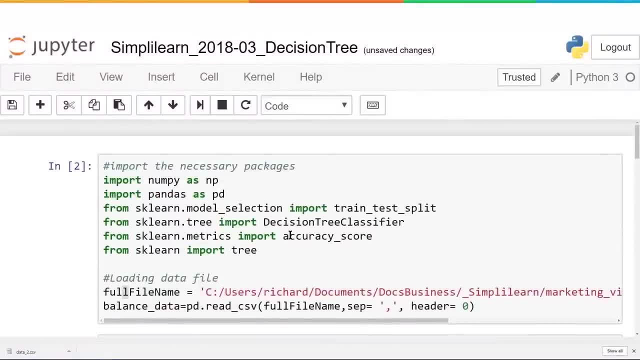 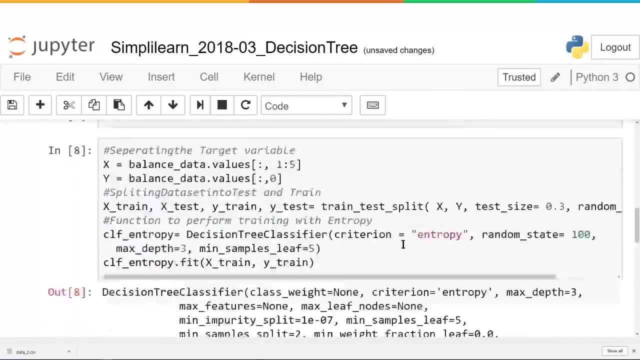 If you remember at the very beginning, let me just scroll up there real quick so you can see where that's coming from. That's coming from here, down here from sklearnmetrics import accuracy score And you could probably run a script, make your own script, to do this very easily. 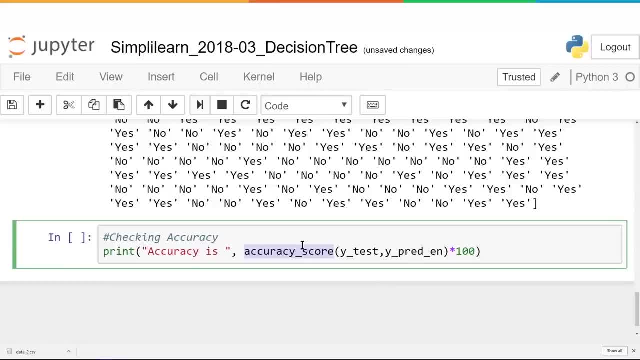 How accurate is it? How many out of 300 do we get right? And so we put in our y test. That's the one we ran the predict on. And then we put in our y predict en. That's the answers we got. 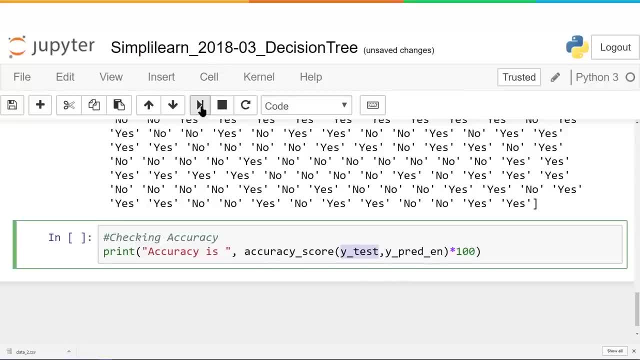 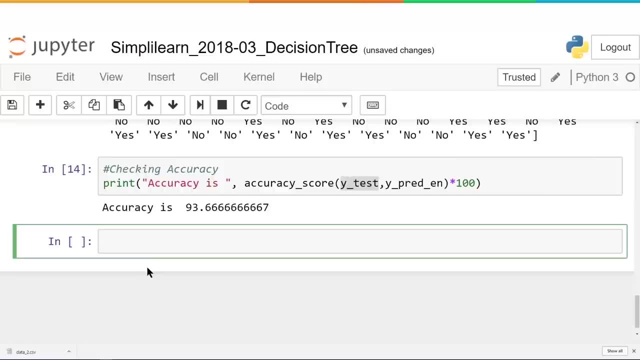 And we're just gonna multiply that by 100, because this is just gonna give us an answer as a decimal And we wanna see it as a percentage. And let's run that and see what it looks like And, if you see, here we got an accuracy of 93.66667.. 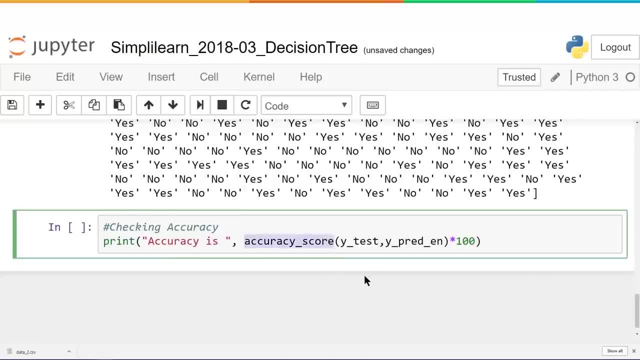 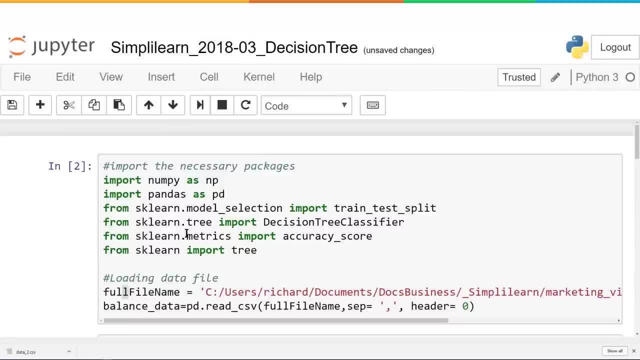 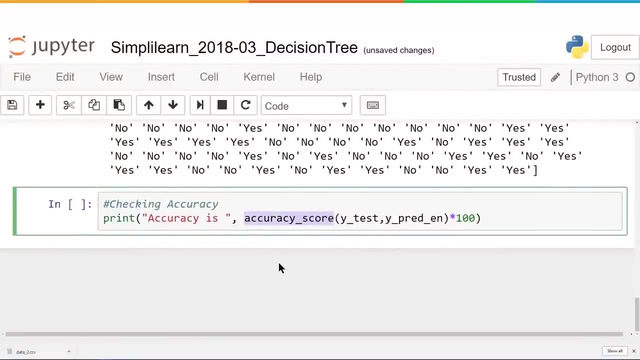 And this was something we imported earlier, If you remember, at the very beginning. Let me just scroll up there real quick so you can see where that's coming from. That's coming from here, down here, from SK. learn dot metrics, import accuracy score And you could probably run a script, make your own script, to do this very easily. 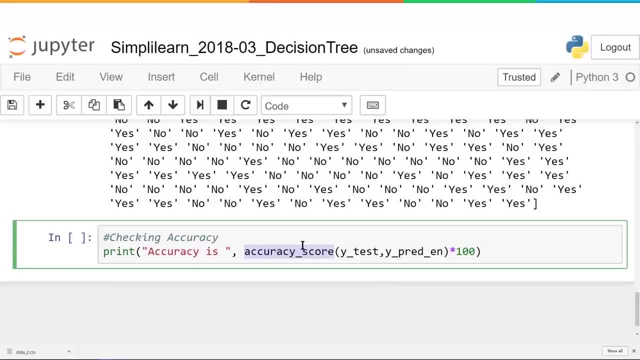 How accurate is it? How many out of 300 do we get right? And so we put in our y test. That's the one we ran the predict on. And then we put in our y predict en. That's the answers we got. 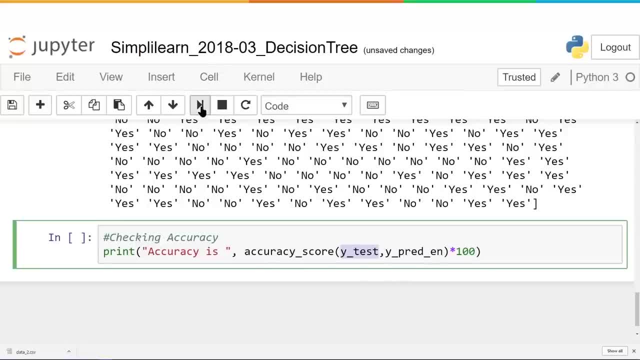 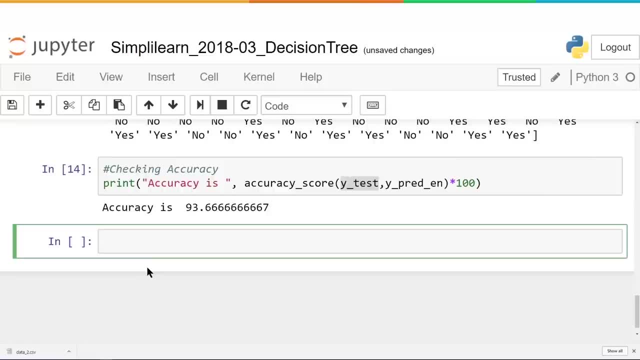 And we're just going to multiply that by 100, because this is just going to give us an answer as a decimal and we want to see it as a percentage. Let's run that and see what it looks like And if you see, here we got. 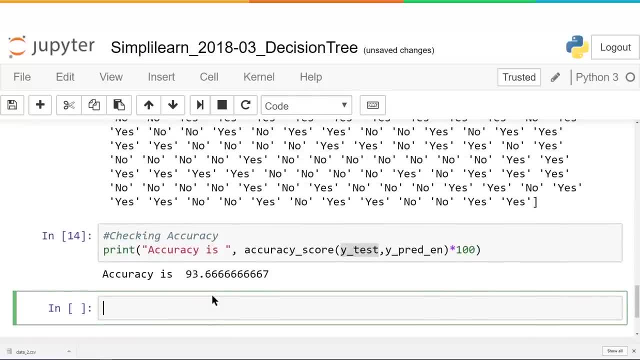 an accuracy of ninety three point six, six, six, six seven. So when we look at the number of loans and we look at how good our model fit, we can tell people it has about a ninety three point six fitting to it. So just a quick recap on that. 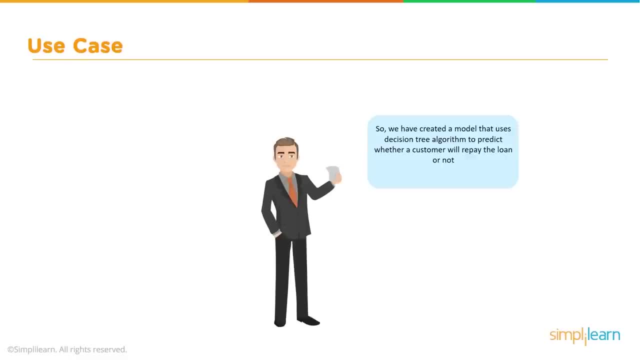 We now have accuracy set up on here, And so we have created a model that uses the decision tree algorithm to predict whether a customer will repay the loan or not. The accuracy of the model is about ninety four point six percent. The bank can now use this model to decide whether it should. 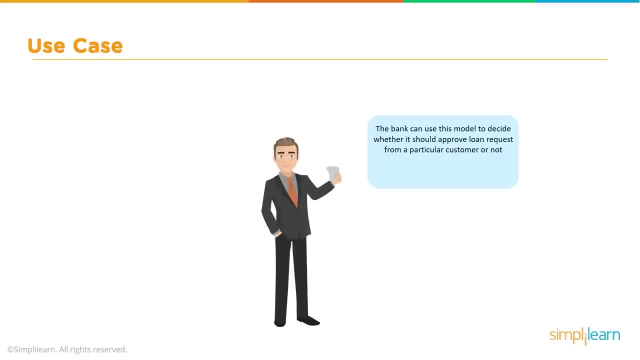 approve the loan request from a particular customer or not, And so this information is really powerful. We may not be able to, as individuals, understand all these numbers, because they have thousands of numbers that come in, But you can see that this is a smart decision for the bank to use a tool like 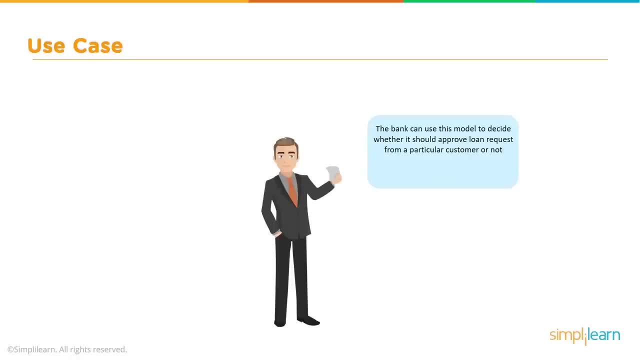 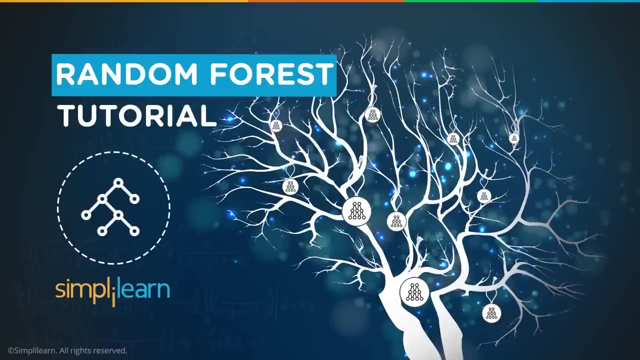 this to help them to predict how good their profits going to be off of the loan balances and how many are going to default or not. Today we're going to be looking at random forest, one of the many powerful tools in the machine learning library. 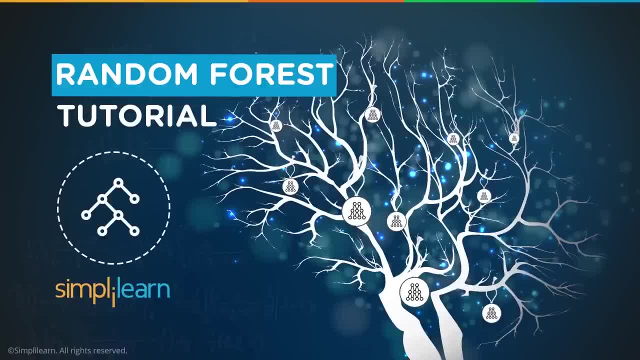 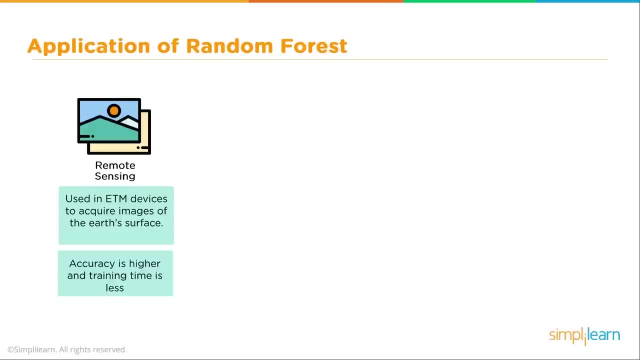 Before we dove into the topic, let's start by looking at a few of the uses for random forest Currently. today is used in remote sensing, For example. they're used in the ETM devices, If you're a space buff. 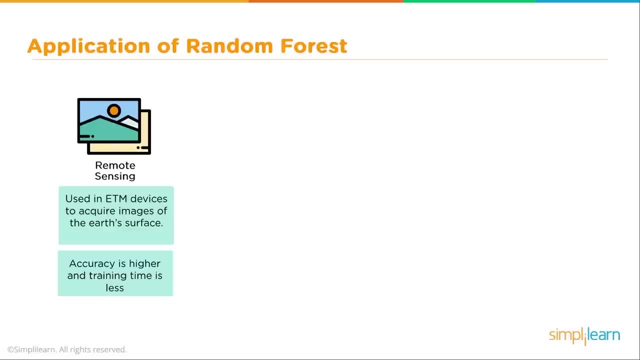 that's the enhanced thermatic mapper they use on satellites which see far outside the human spectrum for looking at land masses And they acquire images of the Earth's surface. The accuracy is higher and training time is less than many other machine learning tools out there. 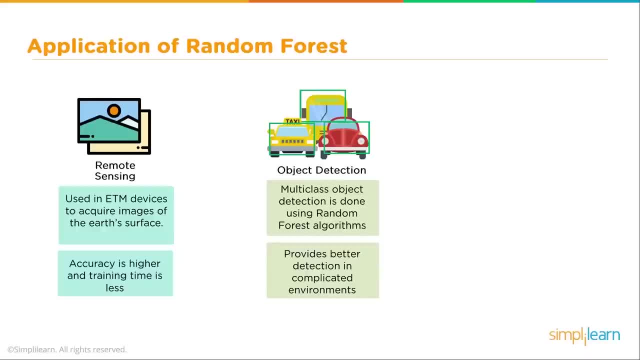 Also object detection. object detection is done using random forest algorithms. A good example is a traffic. We try to sort out the different cars, buses and things and it provides a better detection in complicated environments. It's very complicated up there. 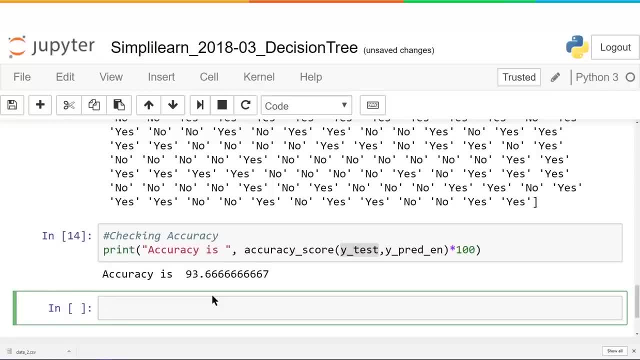 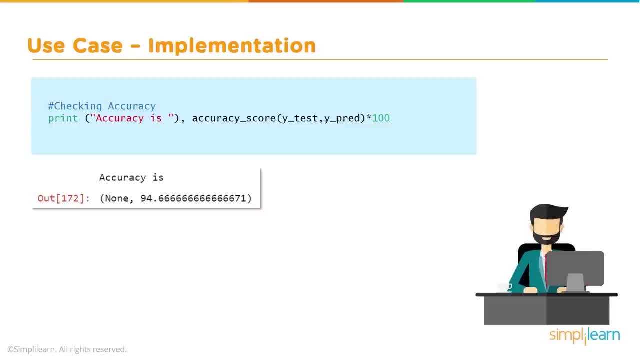 So when we look at the number of loans and we look at how good our model fit, we can tell people it has about a 93.66667. Fitting to it. So just a quick recap on that. We now have accuracy set up on here. 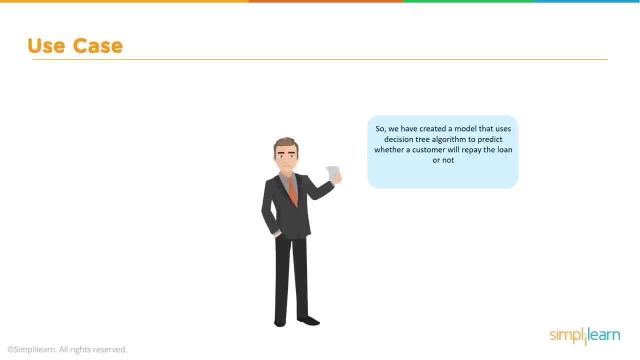 And so we have created a model that uses the decision tree algorithm to predict whether a customer will repay the loan or not. The accuracy of the model is about 94.6%. The bank can now use this model to decide whether it should approve the loan request. 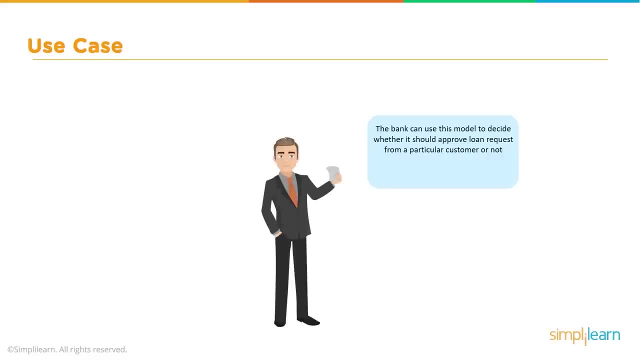 from a particular customer or not, And so this information is really powerful. We may not be able to, as individuals, understand all these numbers, because they have thousands of numbers that come in, But you can see that this is a smart decision for the bank to use a tool like this. 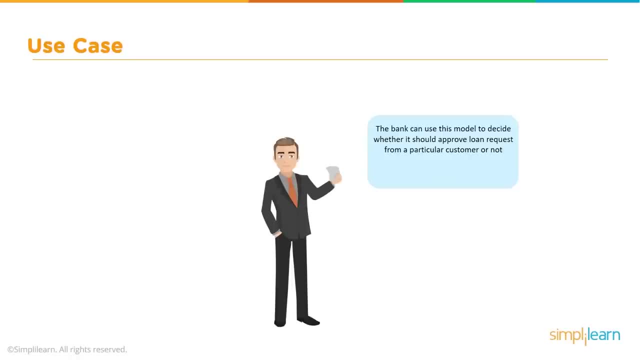 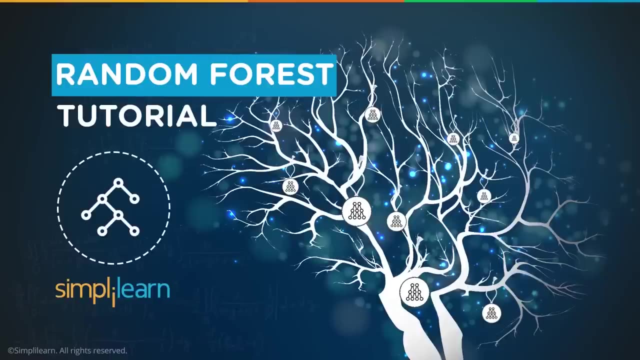 to help them to predict how good their profit's gonna be off of the loan balances and how many are gonna default or not. Today we're gonna be looking at Random Forest, one of the many powerful tools in the machine learning library, Before we dive into the topic. 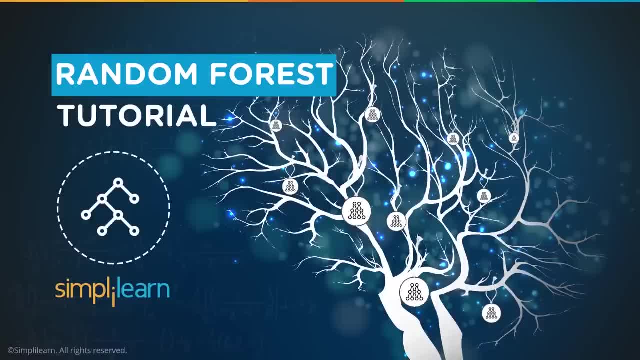 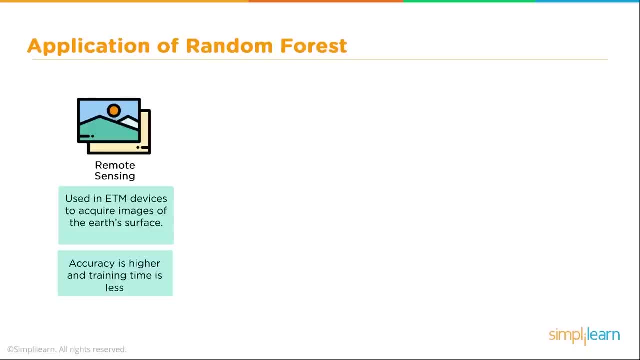 let's start by looking at a few of the uses for Random Forest Currently. today it's used in remote sensing, For example. they're used in the ETM devices. If you're a space buff, that's the Enhanced Thermatic Mapper they use on satellites. 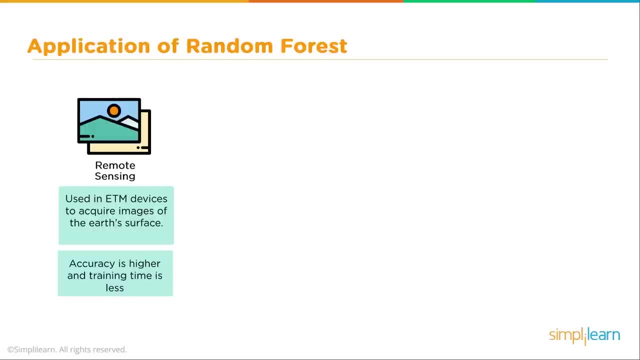 which see far outside the human spectrum for looking at land masses, And they acquire images of the Earth's surface. The accuracy is higher and training time is less than many other machine learning tools out there. Also, object detection- multi-class object detection- is done. 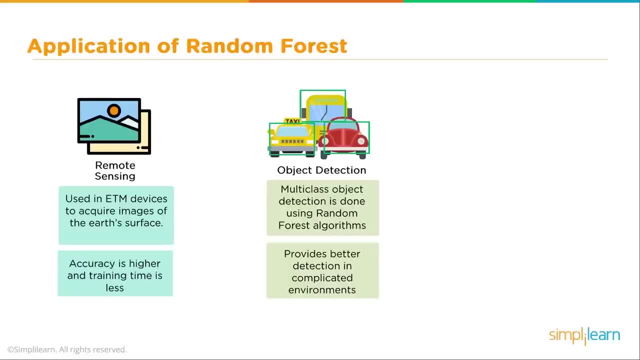 using Random Forest algorithms. A good example is traffic, where you're trying to sort out the different cars, buses and things, And it provides a better detection of what's going on up there. And then we have another example: Connect, And let's take a little closer look at Connect. 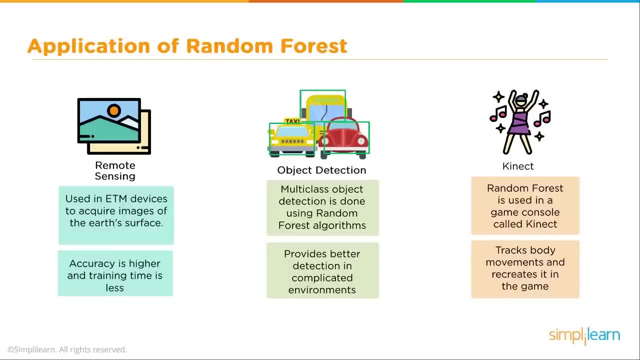 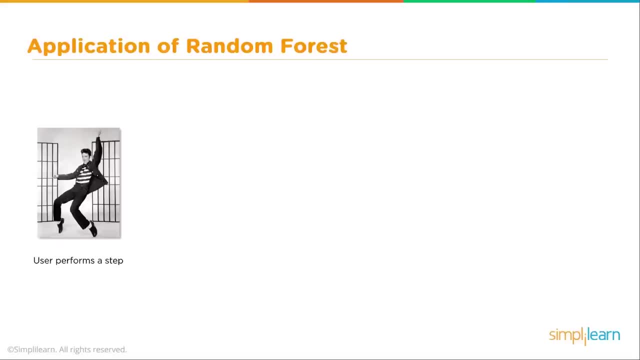 Connect. they use a Random Forest as part of the game console And what it does is it tracks the body movements and it recreates it in the game. And let's see what that looks like. We have a user who performs a step. 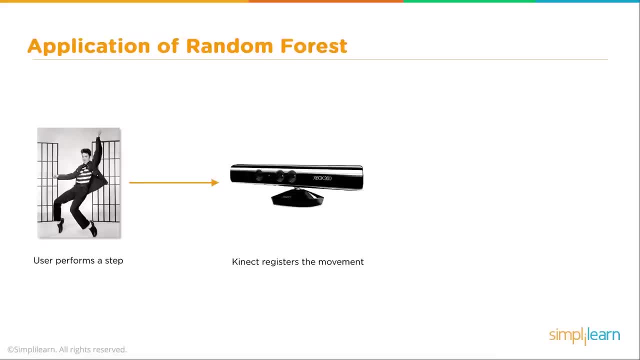 In this case it looks like Elvis Presley going there. That is then recorded so that Connect registers the movement And then it marks the user based on accuracy, And it looks like we have Prince going on. this one from Elvis Presley to Prince, that's great. 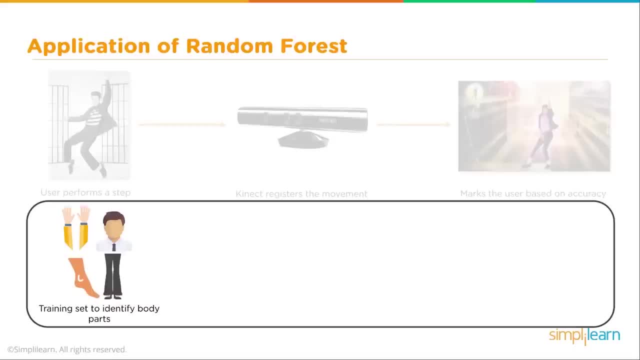 So it marks the user based on the accuracy. If we look at that a little closer, we have a training set to identify body parts. Where are the hands? where are the feet? what's going on with the body? That then goes into a Random Forest classifier. 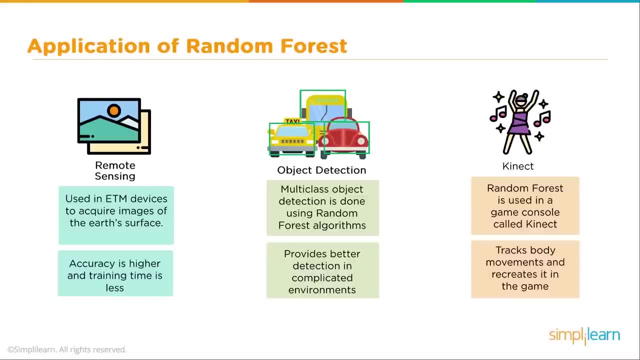 And then we have another example: connect. And let's take a little closer look at connect. connect, They use a random forest as part of the game console, And what it does is it tracks the body movements and it recreates it in the game. 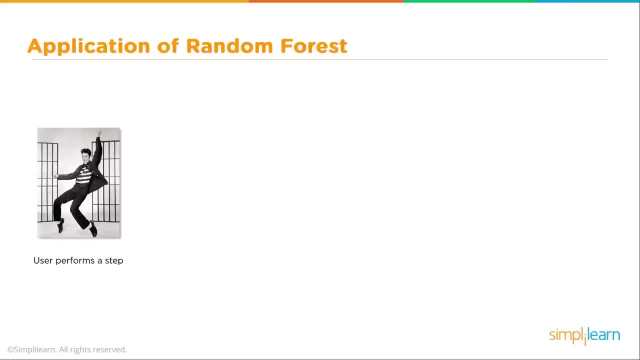 And let's see what that looks like. We have a user who performs a step- In this case it looks like Elvis Presley going there. That is then recorded, so that connect registers the movement And then it marks the user based on accuracy. 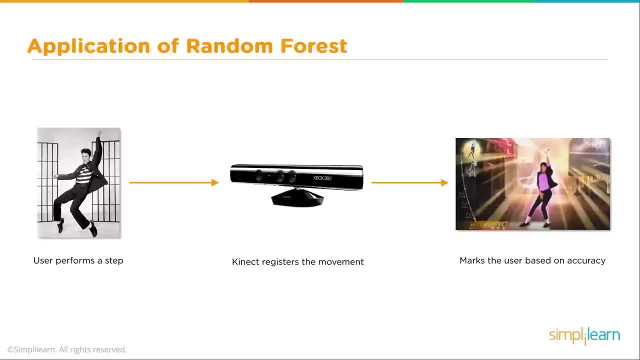 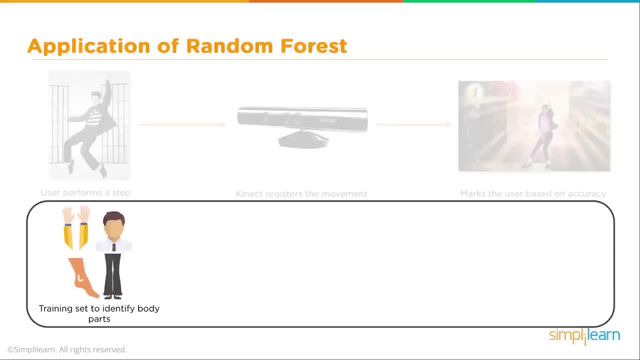 And it looks like we have prints going on this one from Elvis Presley to Prince. It's great. So marks user based on the accuracy. If we look at that a little closer, we have a training set to identify body parts: Where are the hands? Where are the feet? 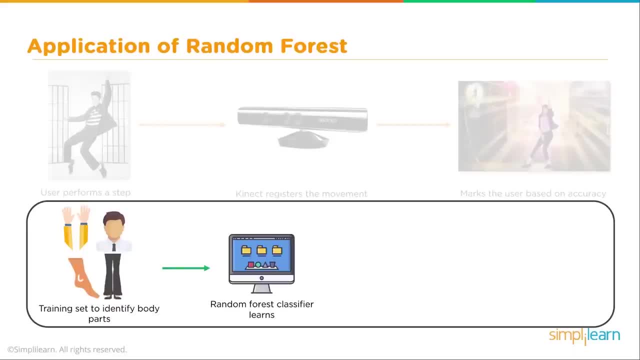 What's going on with the body That then goes into a random forest class of fire that learns from it once we've trained the classifier, and then identifies the body parts while the person's dancing. It's able to represent that in a computer format. 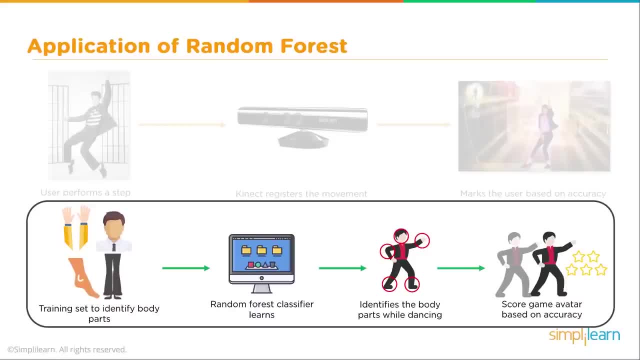 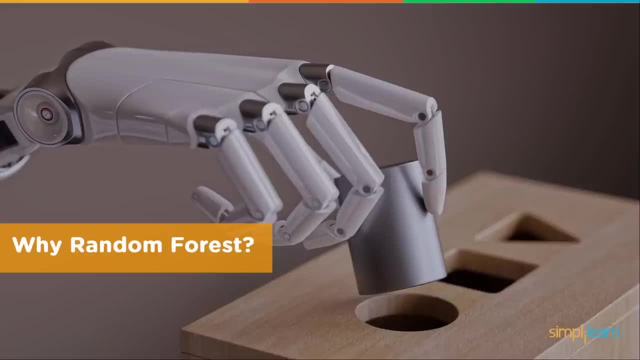 And then, based on that, it scores the game and how accurate you are as being Elvis Presley or Prince and you're dancing. Why random forest? It's always important to understand why we use this tool over the other ones. What are the benefits here? 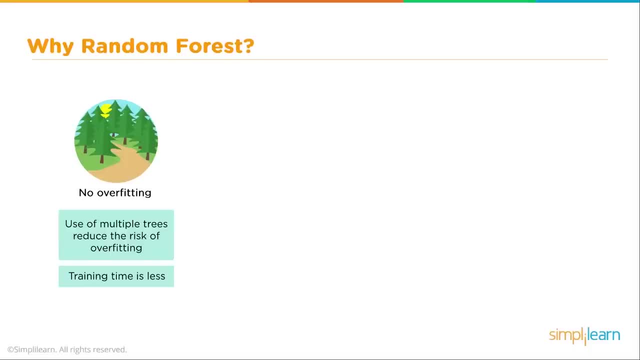 And so with the random forest. the first one is: there's no overfitting. If you use of multiple trees, reduce the risk of overfitting. Training time is less Overfitting means that we have fit the data so close to what we have as our. 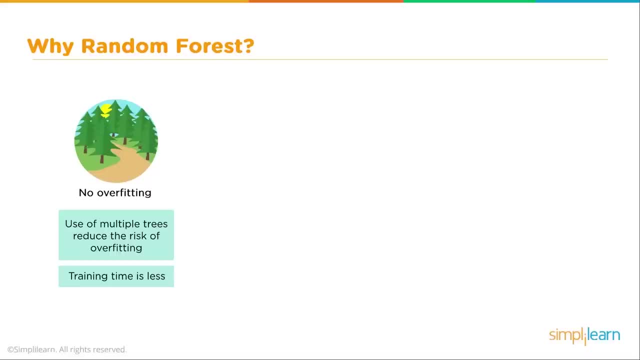 sample that we pick up on all the weird parts And instead of predicting the overall data, you're predicting the weird stuff which you don't want. High accuracy runs efficiently on large database For large data. it produces highly accurate predictions. In today's world of big. 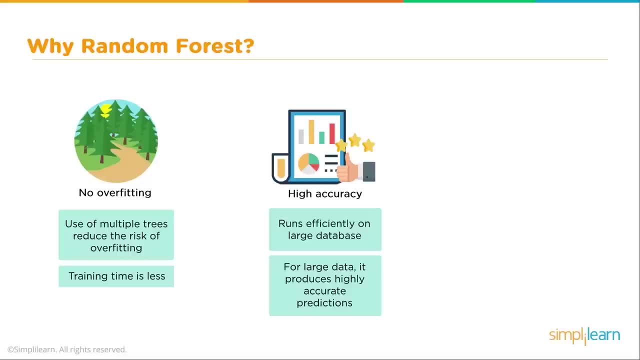 data. this is really important and this is probably where it really shines. This is where why random forest really comes in. It estimates missing data. Data in today's world is very messy, So when you have a random forest, it can maintain the accuracy when a large proportion of the data is missing. 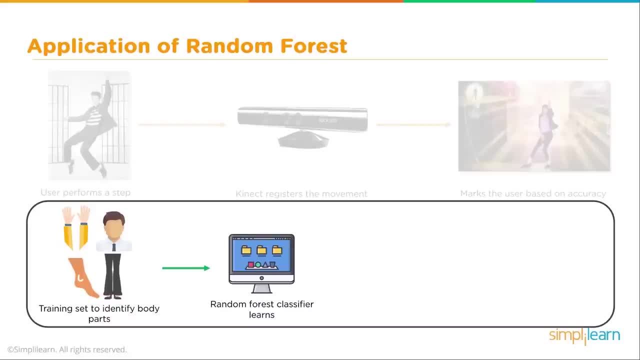 that learns from it Once we've trained the classifier. it then identifies the body parts while the person's dancing And it's able to represent that in a computer format And then, based on that, it scores the game. and how accurate you are as being Elvis Presley. 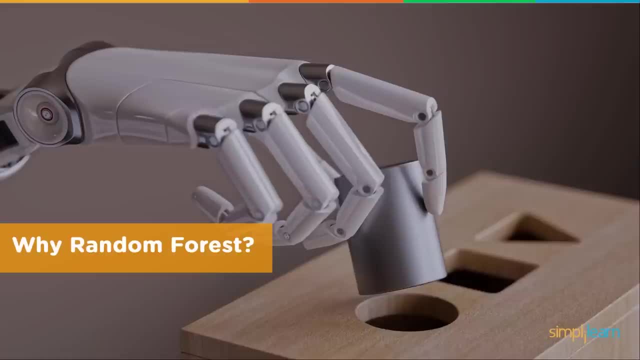 or Prince and you're dancing. Why Random Forest? It's always important to understand why we use this tool over the other ones. What are the benefits here And so with the Random Forest? the first one is there's no overfitting. 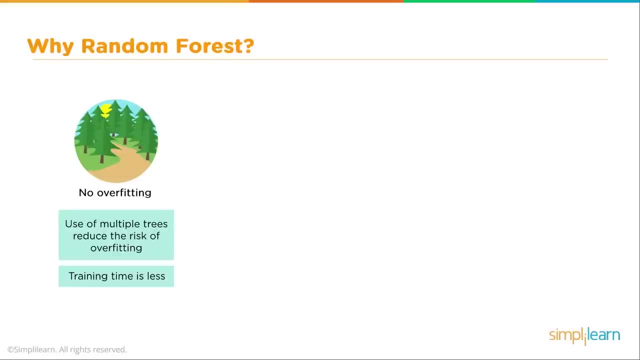 If you use of multiple trees, reduce the risk of overfitting. Training time is less. Overfitting means that we have fit the data so close to what we have as our sample that we pick up on all the weird parts And instead of predicting the overall data. 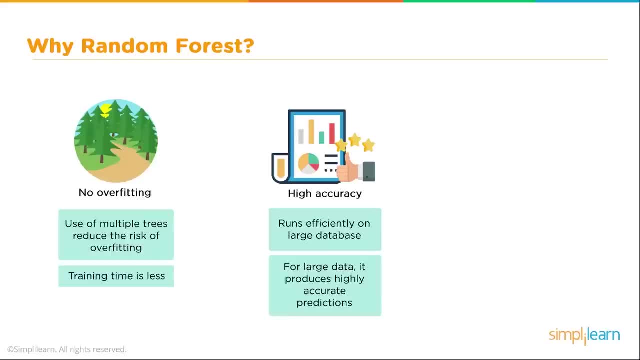 you're predicting the weird stuff which you don't want. High accuracy Runs efficiently on large database For large data. it produces highly accurate predictions. In today's world of big data, this is really important And this is probably where it really shines. 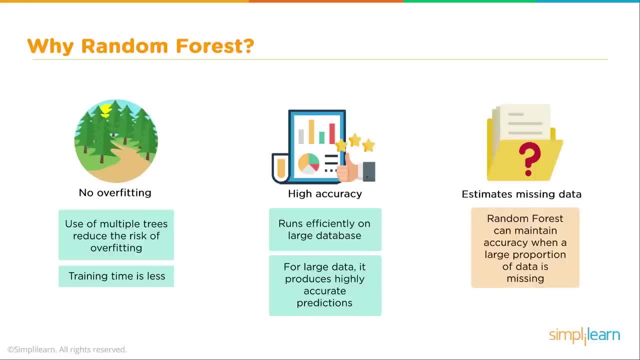 This is where why Random Forest really comes in. It estimates missing data. Data in today's world is very messy, So when you have a Random Forest, it can maintain the accuracy when a large proportion of the data is missing. What that means is if you have data that comes in. 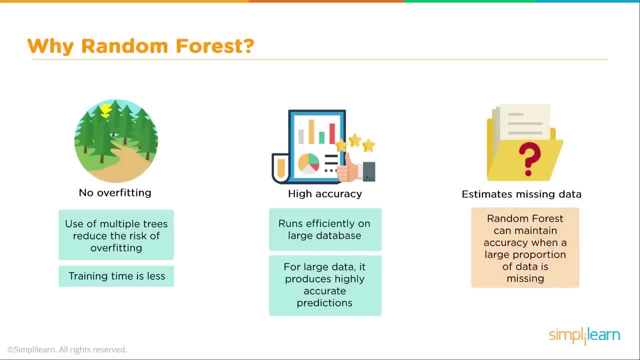 from five or six different areas and maybe they took one set of statistics in one area and they took a slightly different set of statistics in the other. so they have some of the same shared data, but one is missing, like the number of children in the house. if you're doing something over demographics, 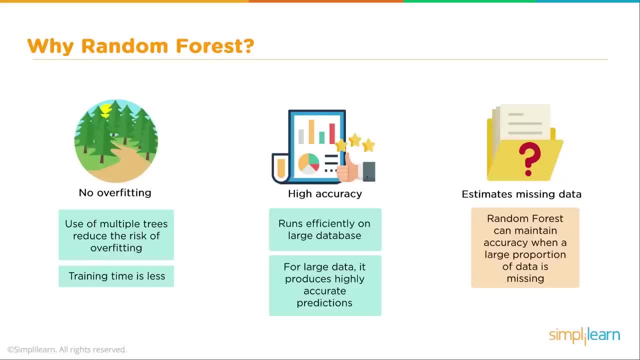 And the other one is missing- the size of the house. It will look at both of those separately and build two different trees, and then it can do a very good job of guessing which one fits better. even though it's missing that data, Let us dig deep into the theory of exactly how it works. 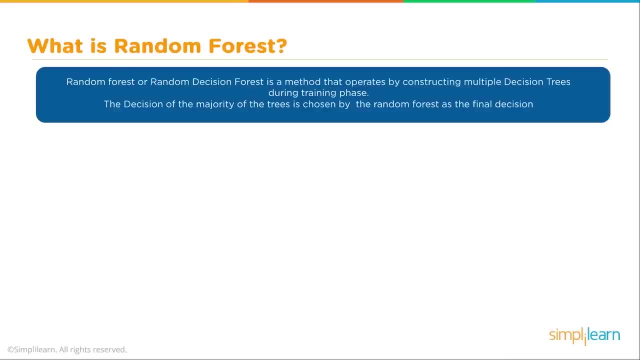 And let's look at what is Random Forest. Random Forest or Random Decision Forest is a method that operates by constructing multiple decision trees. The decision of the majority of the trees is chosen by the Random Forest as the final decision. And let's we have some nice graphics here. 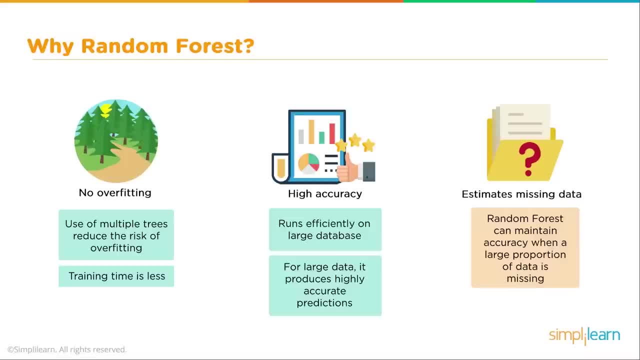 What that means is if you have data that comes in from five or six different areas and maybe they took one set of statistics in one area and they took a slightly different set of statistics in the other, so they have some of the same shared data. 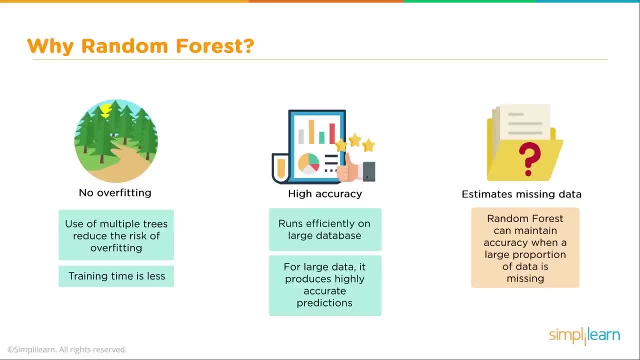 But one is missing, like the number of children in the house, If you're doing something over demographics, and the other one is missing- the size of the house. it will look at both of those separately and build two different trees and then it can do a very good job. 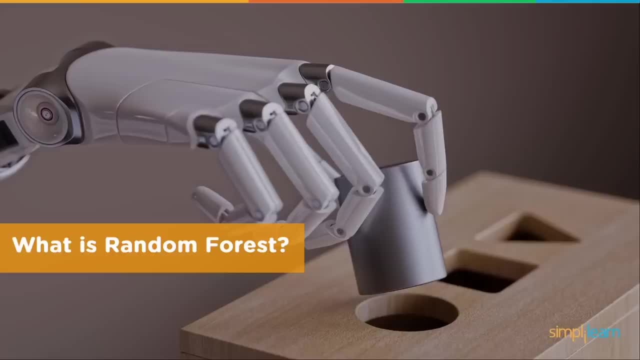 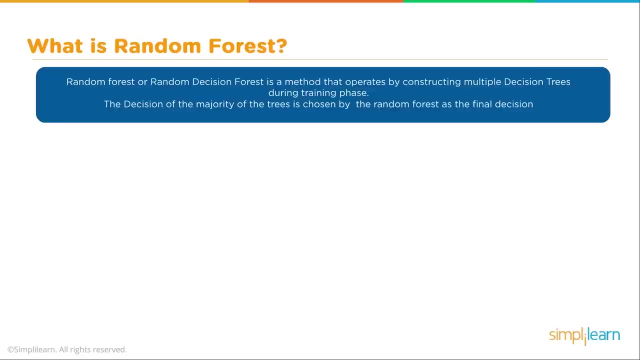 of guessing which one fits better, even though it's missing that data. Let us dig deep into the theory of exactly how it works And let's look at what is random forest. Random forest or random decision forest is a method that operates by constructing multiple decision trees. 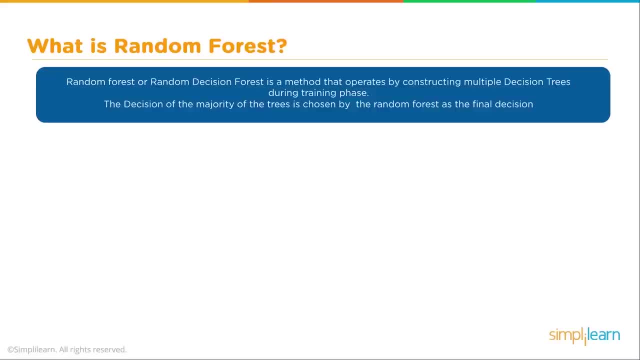 The decision of the majority of the trees is chosen by the random forest as the final decision. And we have some nice graphics here. We have a decision tree and they actually use a real tree to denote the decision tree, which I love, And given a random some kind of picture of a fruit. 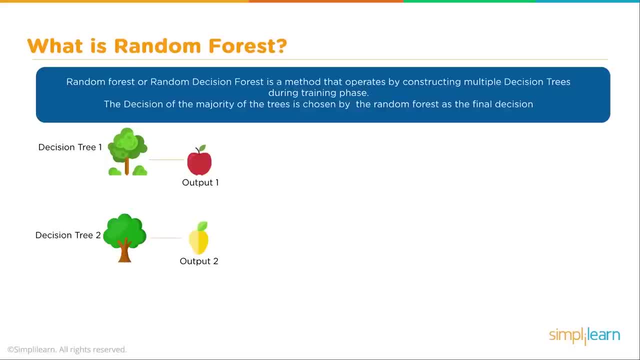 this decision tree decides that the output is it's an apple. And we have a decision tree two where we have that picture of the fruit goes in and this one decides that it's a lemon. and the decision tree tree gets another image and it decides it's an apple. 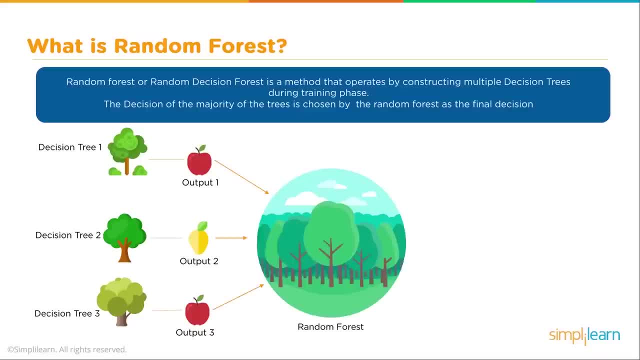 And then this all comes together in what they call the random forest. And this random forest then looks at it and says: OK, I got two votes for apple, one vote for lemon. the majority is apples, So the final decision is apples. 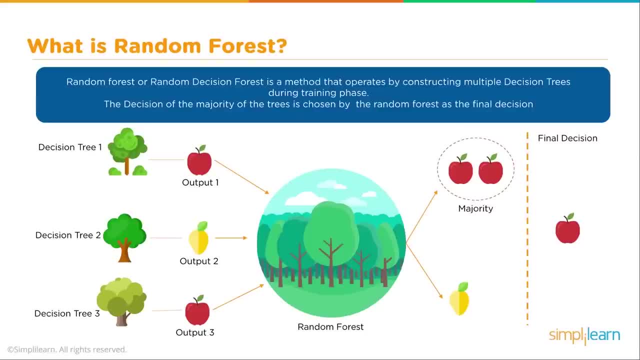 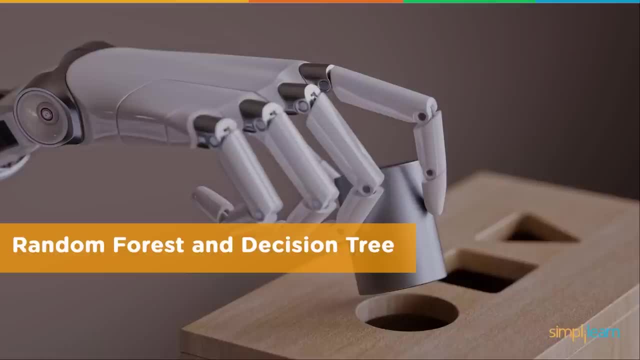 To understand how the random forest works, we first need to dig a little deeper and take a look at the random forest and the actual decision tree and how it builds that decision tree and, looking closer at how the individual decision trees work. We'll go ahead and continue. 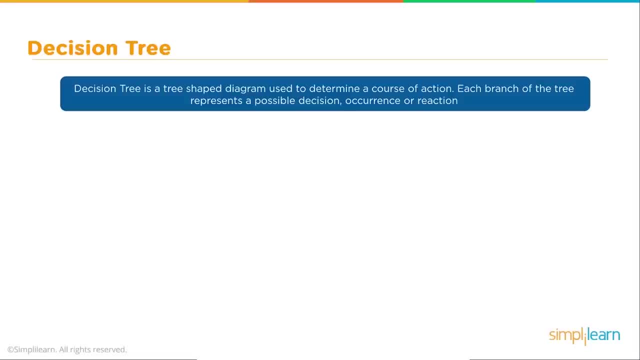 to use the fruit example, since we're talking about trees and forests. A decision tree is a tree shaped diagram used to determine a course of action. Each branch of the tree represents a possible decision, occurrence or reaction. So in here we have a bowl of fruit. 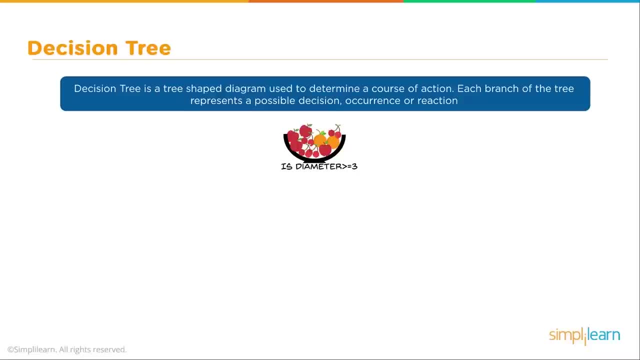 And if you look at that, it looks like they switched from lemons to oranges. We have oranges, cherries and apples And the first decision of the decision tree might be is a diameter greater than or equal to three, And if it says false, it knows that they're cherries, because everything else is bigger. 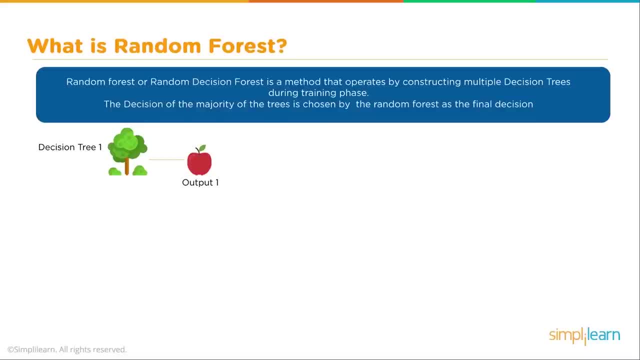 We have a decision tree, And they actually use a real tree to denote the decision tree, which I love, And, given a random, some kind of picture of a fruit, this decision tree decides that the output is it's an apple. And we have a decision tree two. 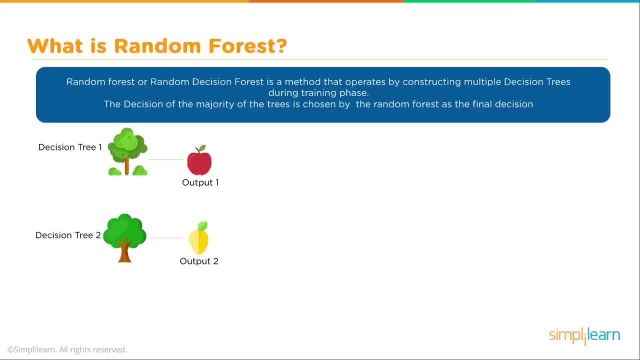 where we have that picture of the fruit goes in and this one decides that it's a lemon, And the decision tree three gets another image and it decides it's an apple. And then this all comes together in what they call the Random Forest. And this Random Forest then looks at it and says: 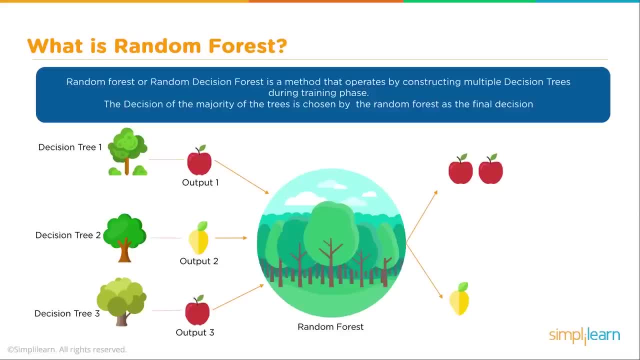 okay, I got two votes for apple, one vote for lemon. The majority is apples, so the final decision is apples. To understand how the Random Forest works, we first need to dig a little deeper and take a look at the Random Forest and the actual decision tree. 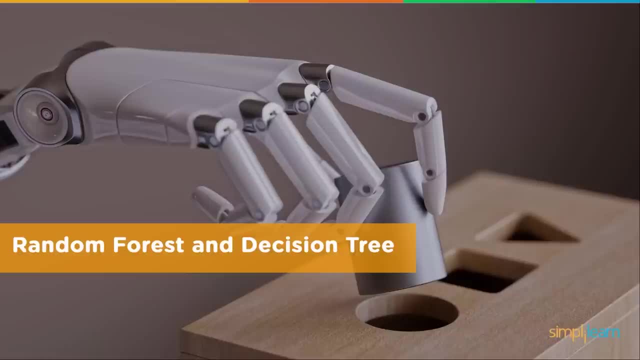 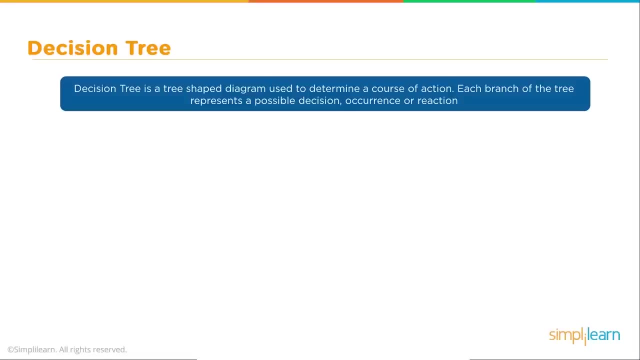 and how it builds that decision tree. In looking closer at how the individual decision trees work, we'll go ahead and continue to use the fruit example, since we're talking about trees and forests. A decision tree is a tree shaped diagram used to determine a course of action. 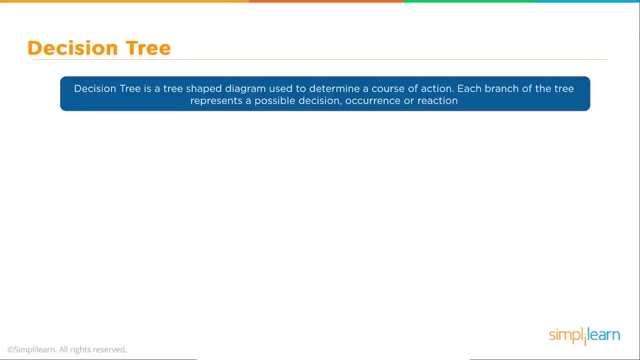 Each branch of the tree represents a possible decision, occurrence or reaction. So in here we have a bowl of fruit and if you look at that, it looks like they switched from lemons to oranges. We have oranges, cherries and apples. 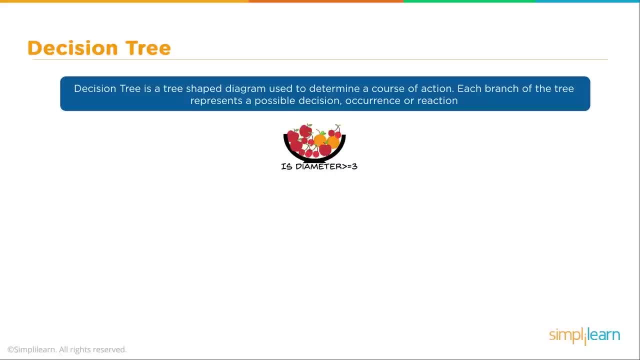 And the first decision of the decision tree might be: is the diameter greater than or equal to three. And if it says false, it knows that they're cherries, because everything else is bigger than that, So all the cherries fall into that decision. 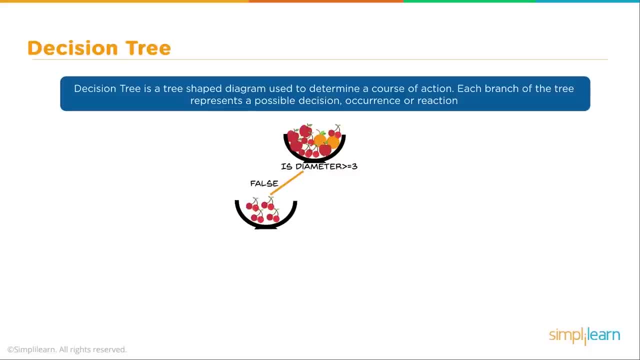 So we have all that data, we're training, We can look at that and we know that that's what's gonna come up. Is the color orange? Well, it goes. hmm, What about the red? Well, if it's true, then it comes out as the orange. 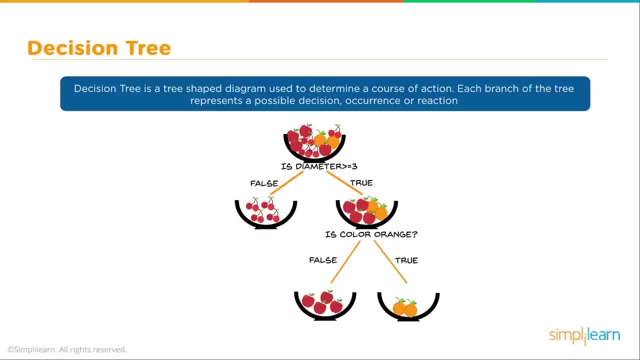 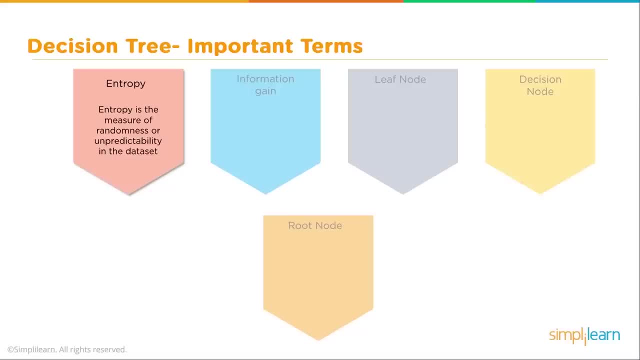 And if it's false, that leaves apples. So in this example, it sorts out the fruit in the bowl or the images of the fruit A decision tree. these are very important terms to know because these are very central to understanding the decision tree when working with them. 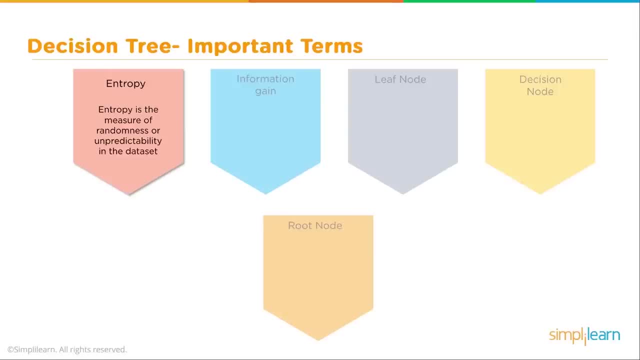 The first is entropy. Everything on the decision tree and how it makes a decision is based on entropy. Entropy is a measure of randomness or unpredictability in the data set. Then they also have information gain: the leaf node, the decision node and the root node. 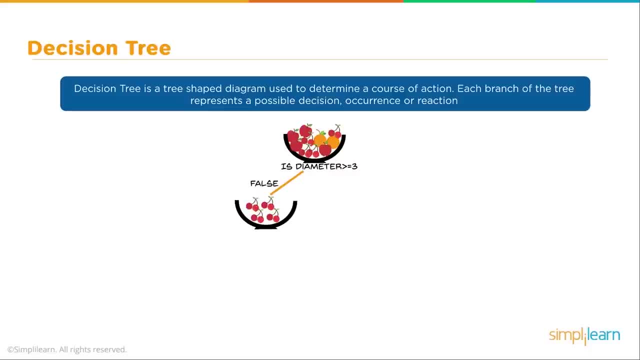 than that. So all the cherries fall into that decision. So we have all that data we're training, We can look at that. We know that that's what's going to come up. Is the color orange? Well, it goes. hmm, orange or red? 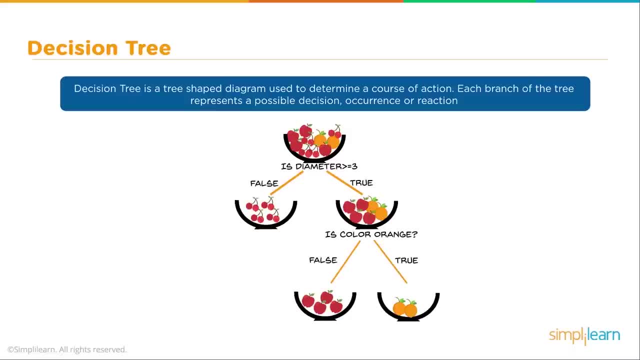 Well, if it's true, then it comes out as the orange, And if it's false, that leaves apples. So in this example it sorts out the fruit in the bowl or the images of the fruit A decision tree. these are very important terms to know because 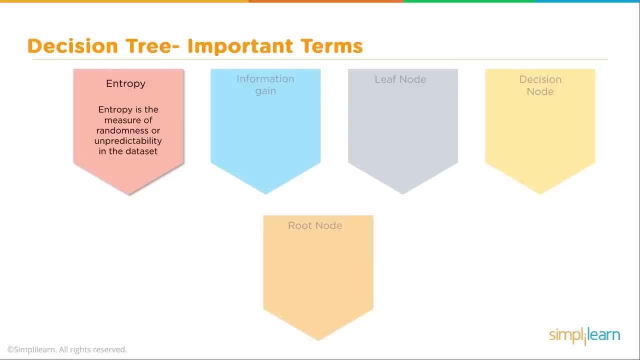 these are very central to understanding the decision tree when working with them. The first is entropy. Everything on the decision tree and how it makes a decision is based on entropy. Entropy is a measure of randomness or unpredictability in the data set. Then they also have information gain. 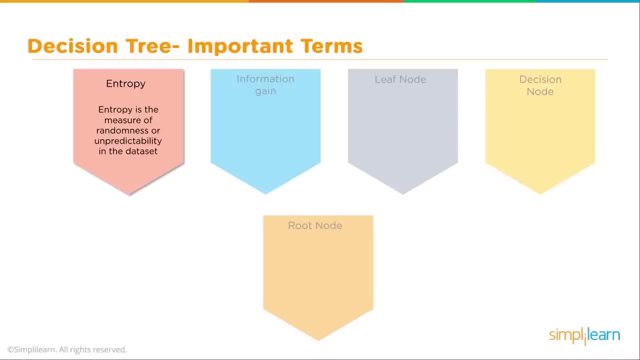 the leaf node, the decision node and the root node. We'll cover these other four terms as we go down the tree, But let's start with entropy. So, starting with entropy, we have here a high amount of randomness. What that means is that 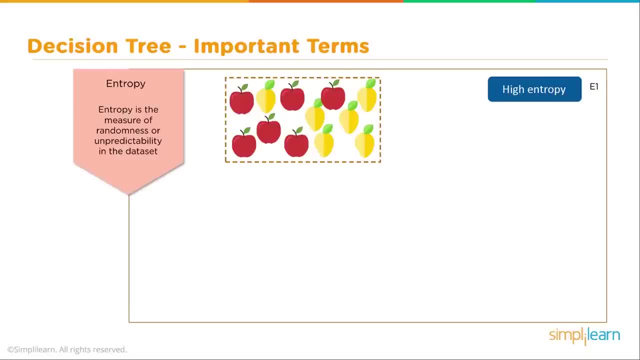 whatever is coming out of this decision, if it was going to guess based on this data, it wouldn't be able to tell you whether it's a lemon or an apple. It would just say it's a fruit. So the first thing we want to do is we want to split this apart and we take 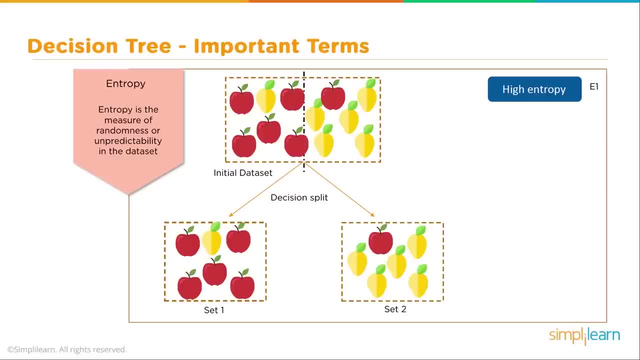 the initial data set. we're going to create a data set one and a data set two. We just split it in two And if you look at these new data sets after splitting them, the entropy of each of those sets is much less. 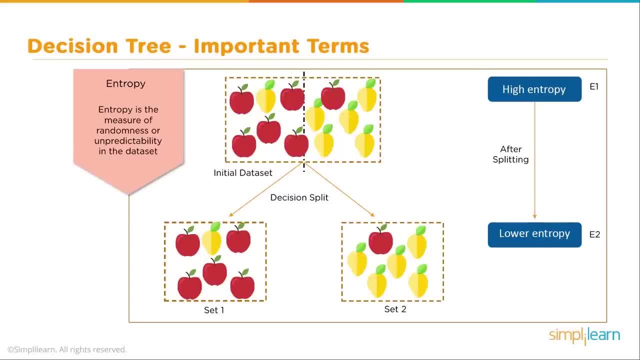 So for the first one, whatever comes in there, it's going to sort that data and it's going to say, OK, if this data goes this direction, it's probably an apple, And if it goes into the other direction it's probably a lemon. 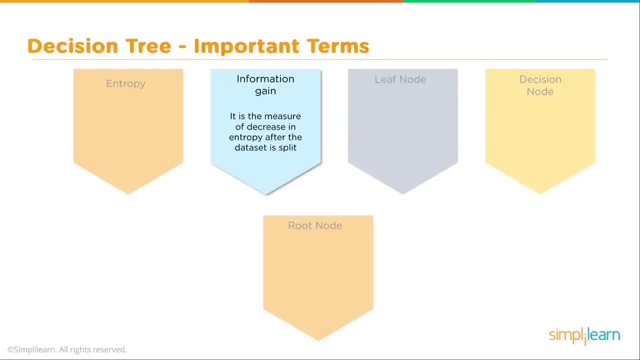 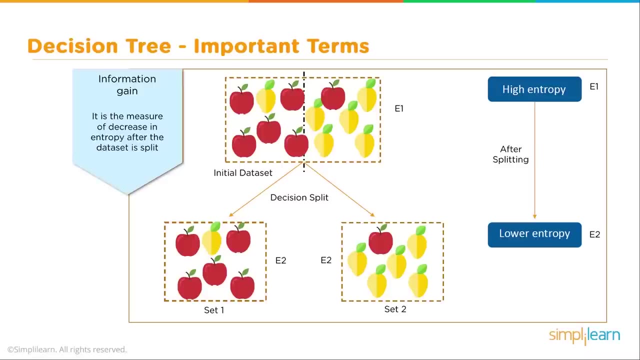 So that brings us up to information gain. It is the measure of decrease in the entropy after the data set is split. What that means in here is that we've gone from one set which has a very high entropy to two lower sets of entropy. 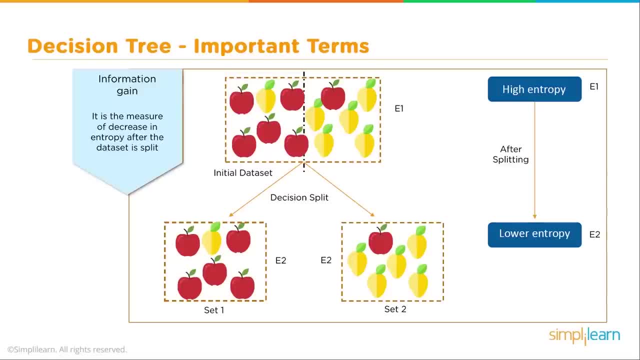 And we've added in the values of E1 for the first one and E2 for the second, two which are much lower, And so that information gain is increased greatly in this example, And so you can find that the information grain simply equals decision E1 minus E2.. 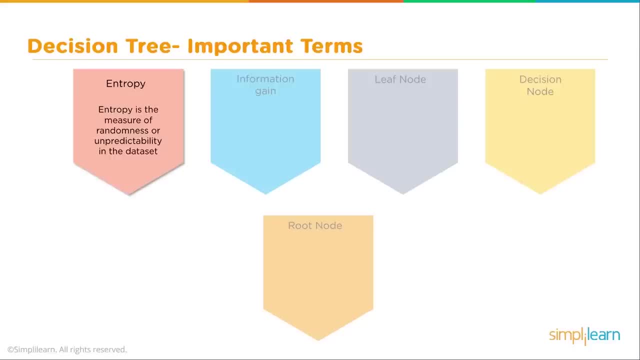 We'll cover these other four terms as we go down the tree, but let's start with entropy. So, starting with entropy, we have here a high amount of randomness. What that means is that whatever's coming out of this decision, if it was gonna guess based on this data, 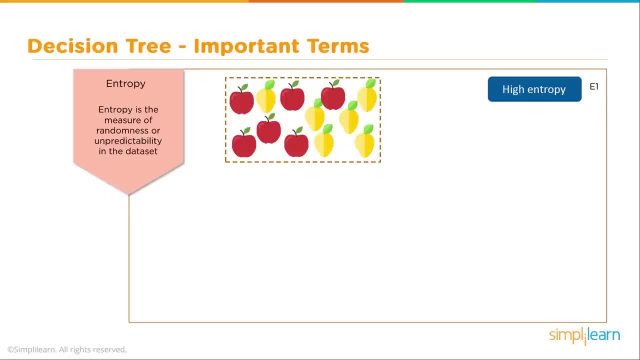 it wouldn't be able to tell you whether it's a lemon or an apple. It would just say it's a fruit. So the first thing we wanna do is we wanna split this apart And we take the initial data set and we're gonna create a data set one and a data set two. 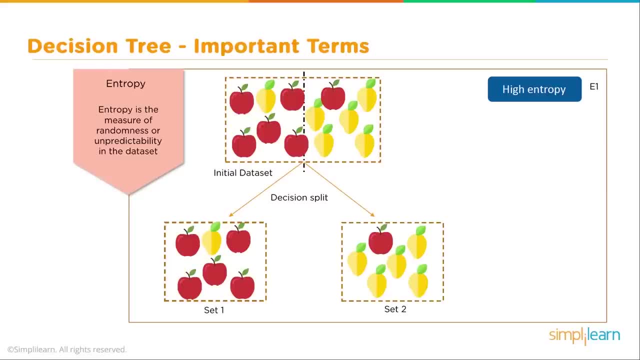 We just split it in two And if you look at these new data sets after splitting them, the entropy of each of those sets is much less. So for the first one, whatever comes in there, it's gonna sort that data and it's gonna say: 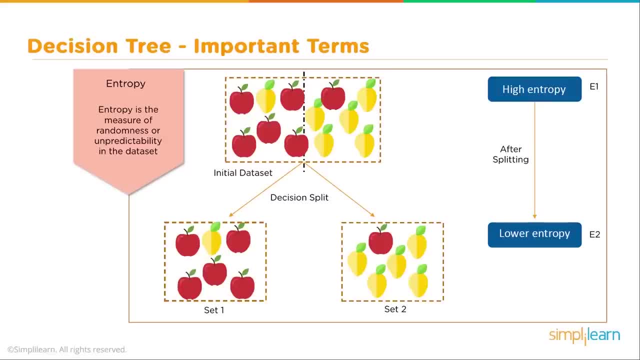 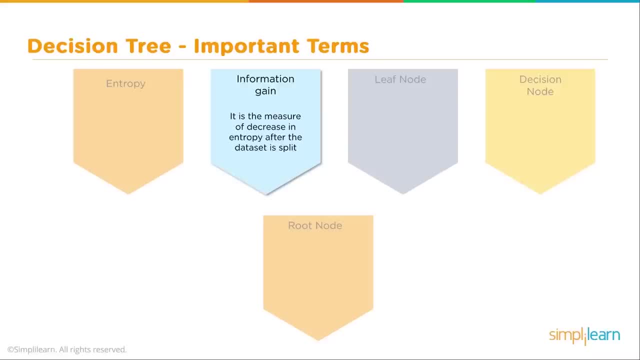 okay, if this data goes this direction, it's probably an apple, And if it goes into the other direction, it's probably a lemon. So that brings us up to information gain. So what does that mean? It is the measure of decrease in the entropy. 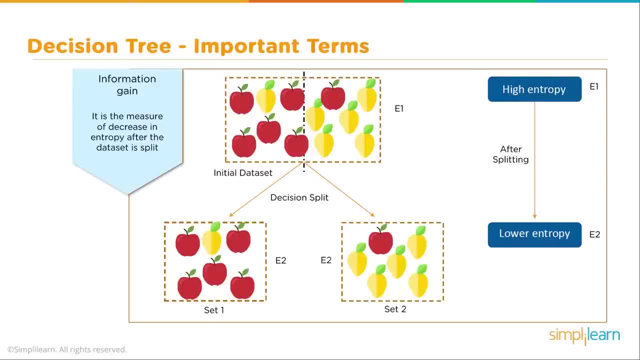 after the data set is split. What that means in here is that we've gone from one set which has a very high entropy to two lower sets of entropy And we've added in the values of E1 for the first one and E2 for the second, two which are much lower. 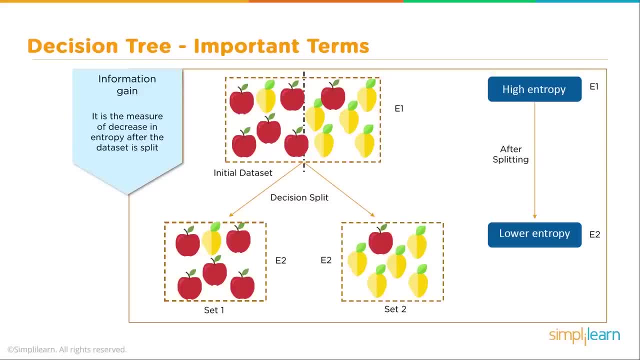 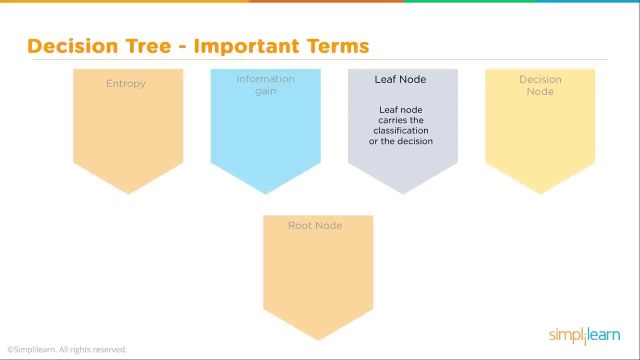 And so that information gain is increased greatly in this example, And so you can find that the information gain simply equals decision E1 minus E3.. As we're going down our list of definitions, we'll look at the leaf node, And the leaf node carries the classification or the decision. 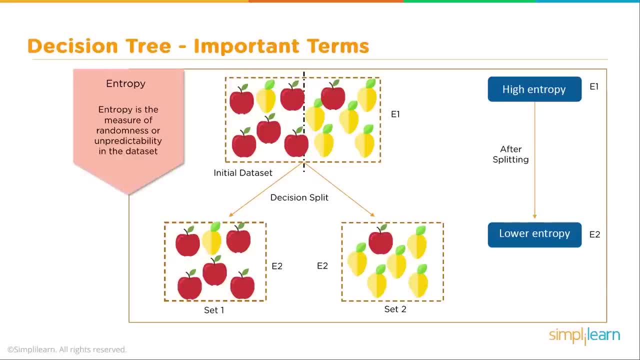 So we look down here to the leaf node, we finally get to our set one or our set two. When it comes down there and it says, okay, this object's gone into set one. if it's gone into set one, it's gonna be split by some means. 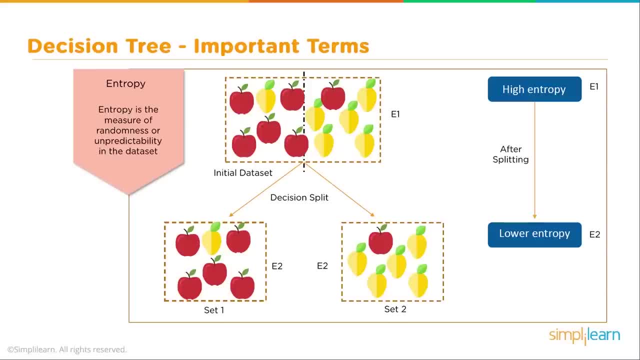 and we'll either end up with apples on the leaf node or a lemon on the leaf node, and on the right it'll be an apple or lemons. Those leaf nodes are those final decisions or classifications. That's the definition of leaf node in here. 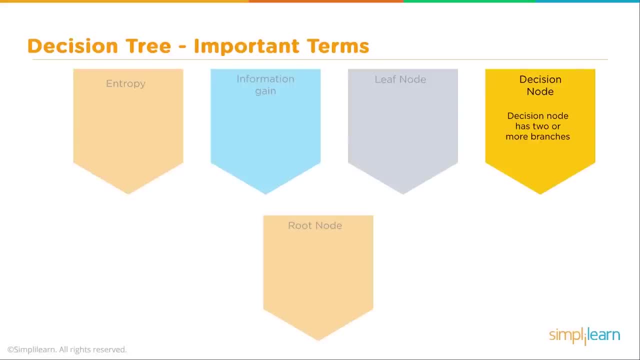 If we're gonna have a final leaf where we make the decision, we should have a name for the nodes above it and they call those decision nodes A decision node. decision node has two or more branches And you can see here where we have the five apples. 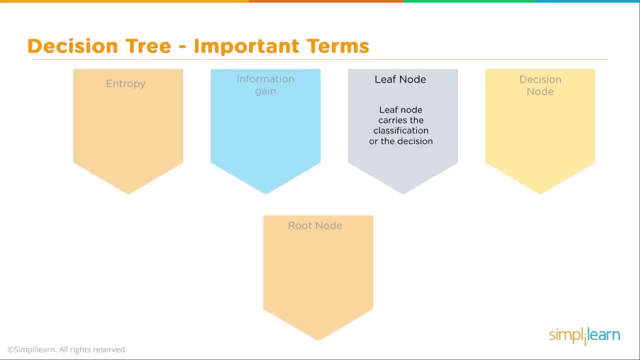 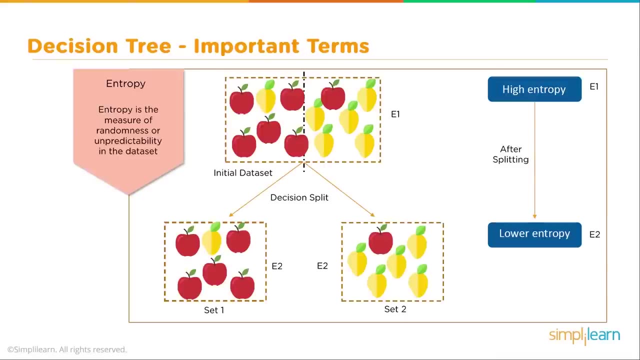 As we're going down our list of definitions, we'll look at the leaf node and the leaf node carries the classification or the decision. So we look down here to the leaf node. We finally get to our set one or set two when it comes down there and it says: OK. 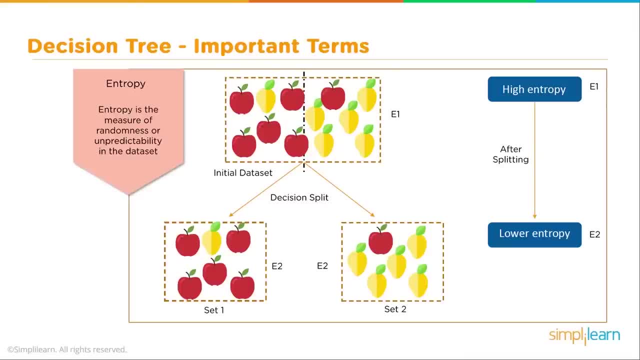 we've gone into set one. If it's gone into set one, it's going to be split by some means and we'll either end up with apples on the leaf node or a lemon on the leaf node, and on the right will either be an apple or 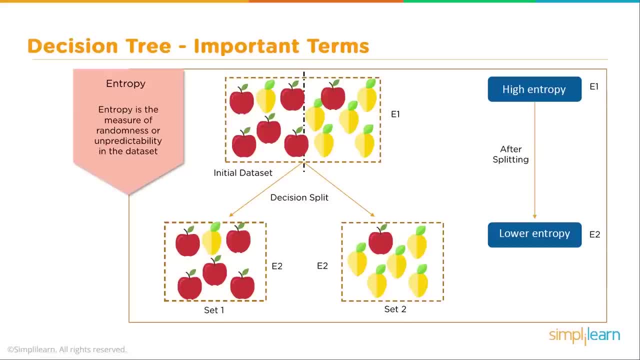 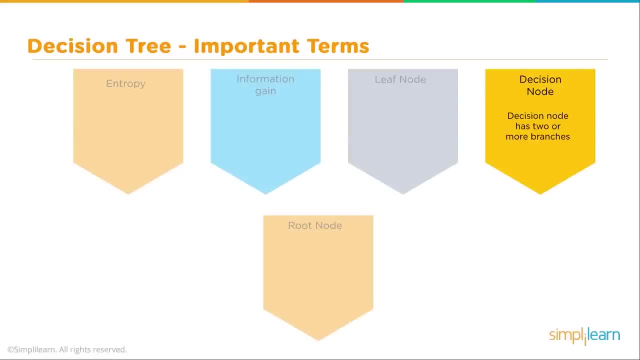 lemons. Those leaf nodes are those final decisions or classifications. That's the definition of leaf node in here. If we're going to have a final leaf where we make the decision, we should have a name for the nodes above it And they call those decision nodes A decision node. 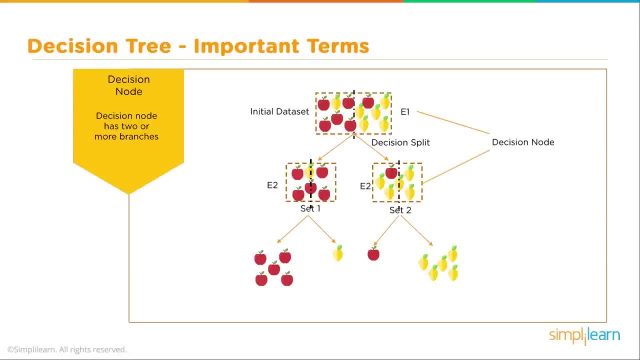 A decision node has two or more branches, and you can see here where we have the five apples and one lemon and in the other case, the five lemons and one apple. They have to make a choice of which tree it goes down, based on some kind. 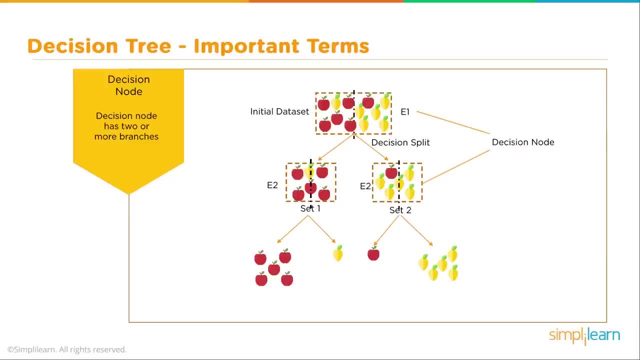 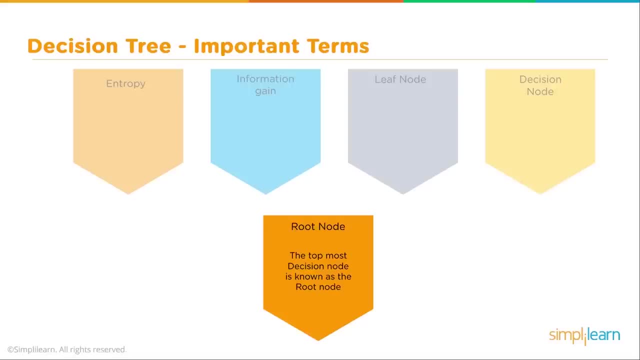 of measurement or information given to the tree. And that brings us to our last definition: The root node. the top, most decision node is known as the root node, And this is where you have all of your data and you have your first decision. it 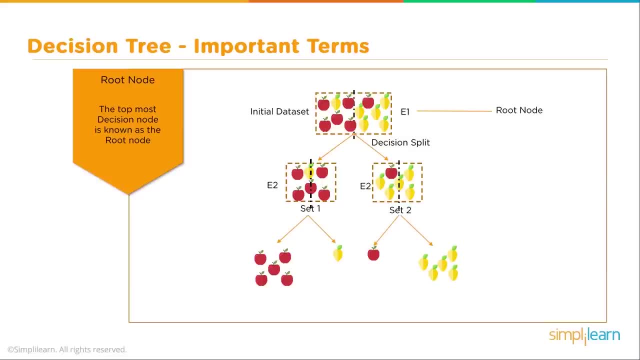 has to make. It has to be split in information. So far we've looked at a very general image with the fruit being split. Let's look and see exactly what that means to split the data And how do we make those decisions on there. 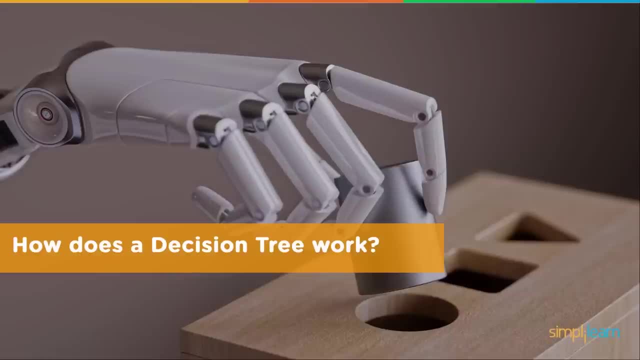 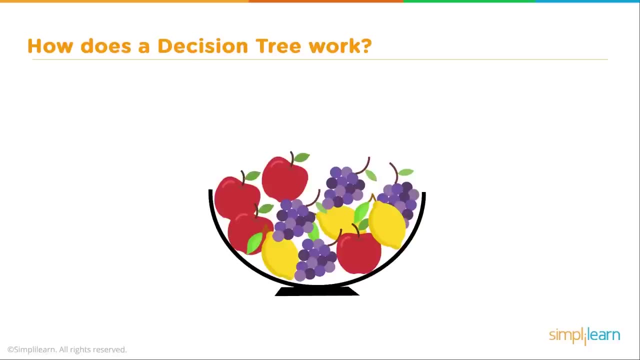 Let's go in there and find out how does a decision tree work. So let's try to understand this and let's use a simple example And we'll stay with the fruit. We have a bowl of fruit And so let's create a problem statement. 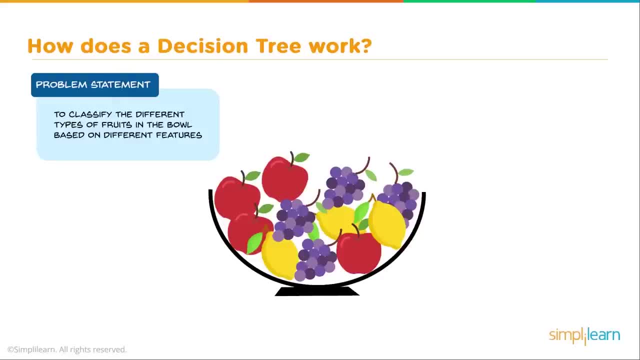 And the problem is we want to classify the different types of fruits in the bowl based on different features. The data set in the bowl is looking quite messy and the entropy is high in this case. So if this bowl was our decision maker, it wouldn't know what choice to make. 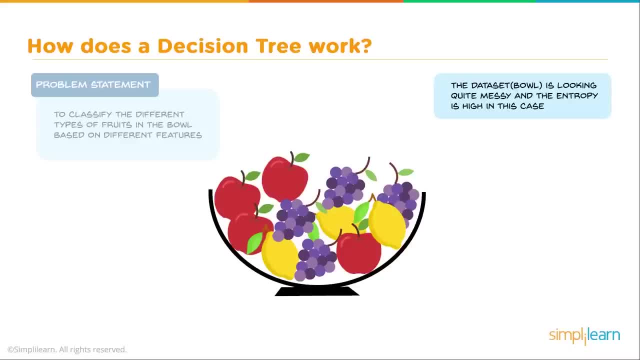 It has so many choices. Which one do you pick? Apple, grapes or lemons, And so we look in here we're going to start with a training set. So this is our data, that we're training our data with, And we have a number of options here. 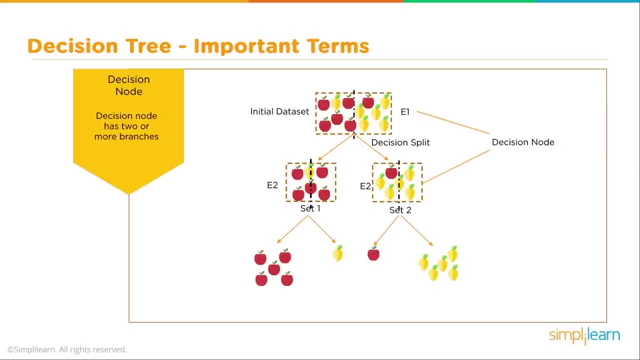 and one lemon, and in the other case, the five lemons and one apple. they have to make a choice of which tree it goes down, based on some kind of measurement or information given to the tree. And that brings us to our last definition. 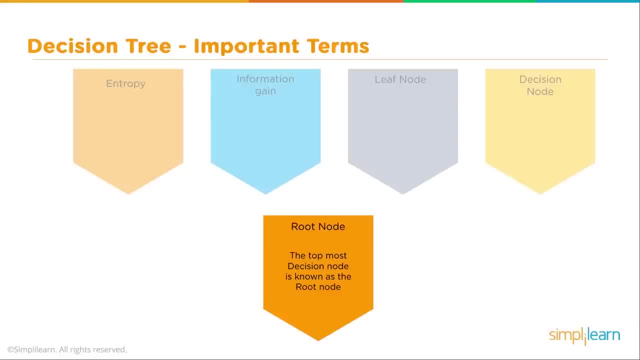 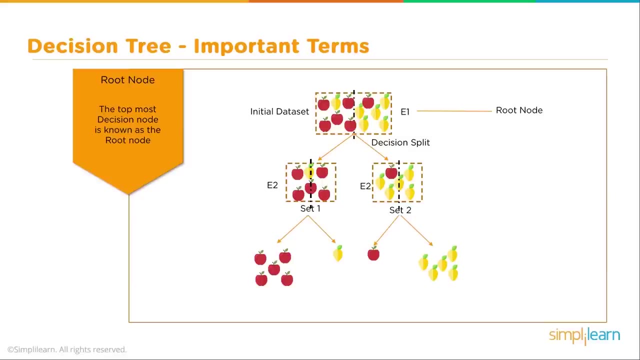 the root node. the topmost decision node is known as the root node And this is where you have all of your data and you have your first decision it has to make, or the first split in information. So far, we've looked at a very general image. 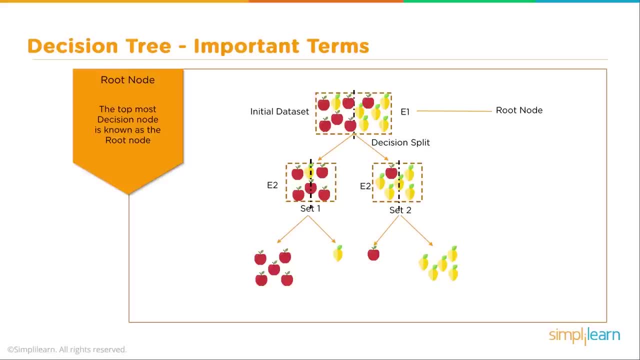 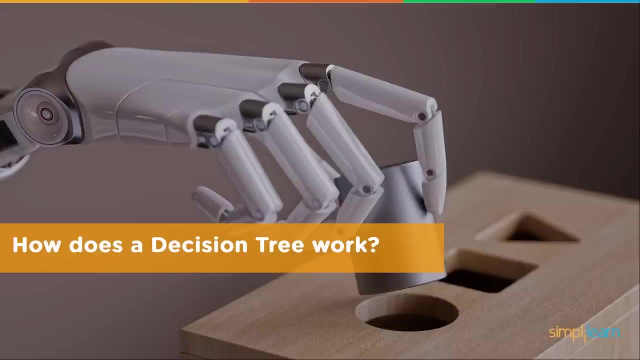 with the fruit being split. Let's look and see exactly what that means to split the data And how do we make those decisions on there. Let's go in there and find out. how does a decision tree work? So let's try to understand this. 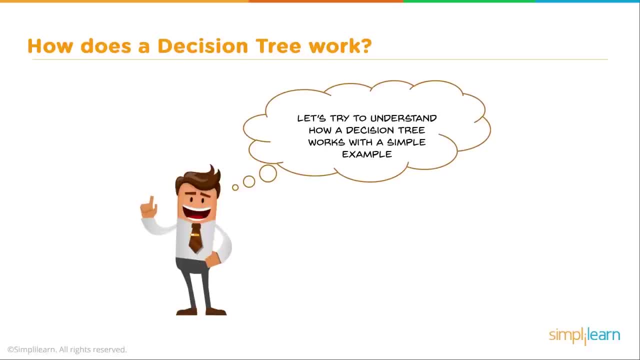 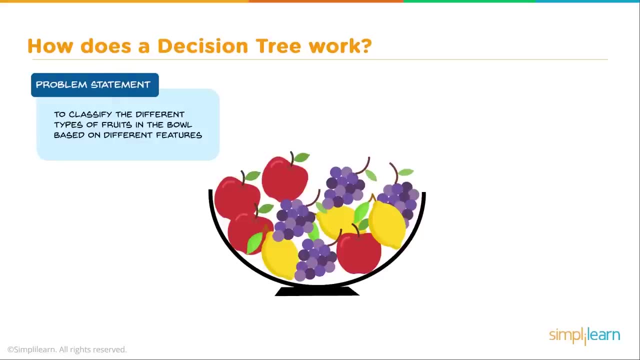 and let's use a simple example And we'll stay with the fruit. We have a bowl of fruit And so let's create a problem statement, And the problem is we want to classify the different types of fruits in the bowl based on different features. 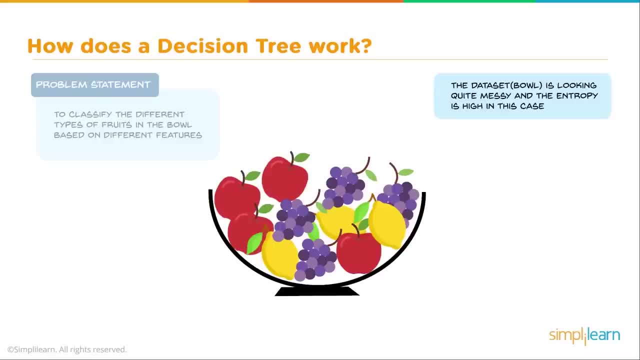 The data set in the bowl is looking quite messy and the entropy is high in this case. So if this, this bowl was our decision maker, it wouldn't know what choice to make. It has so many choices. Which one do you pick? 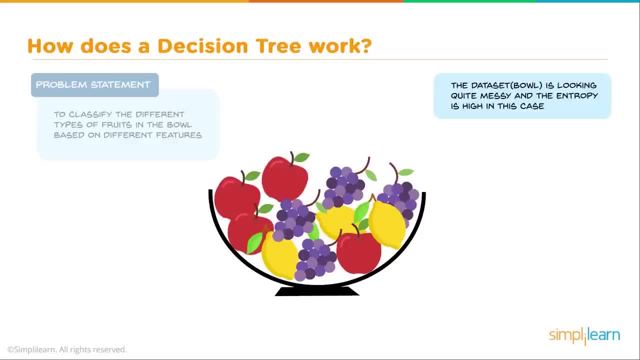 Apple, grapes or lemons, And so we look in here we're gonna start with a training set. So this is our data, that we're training our data with, And we have a number of options. here We have the color. 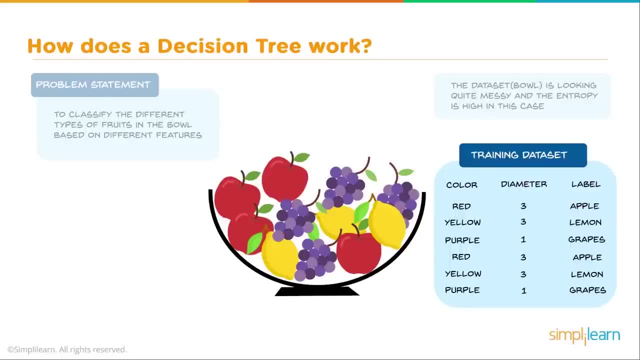 and under the color we have red, yellow, purple. We have a diameter three, three one, three three one, And we have a label: apple lemon grapes, apple lemon grapes. And how do we split the data? 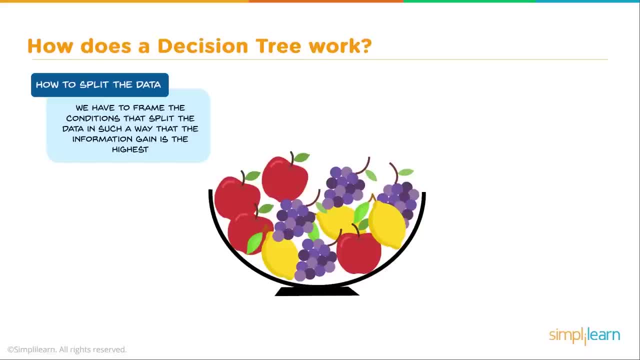 We're gonna frame the conditions to split the data in such a way that the information gain is the highest, And it's very key to note that we're looking for the best gain. We don't wanna just start sorting out the smallest piece in there. 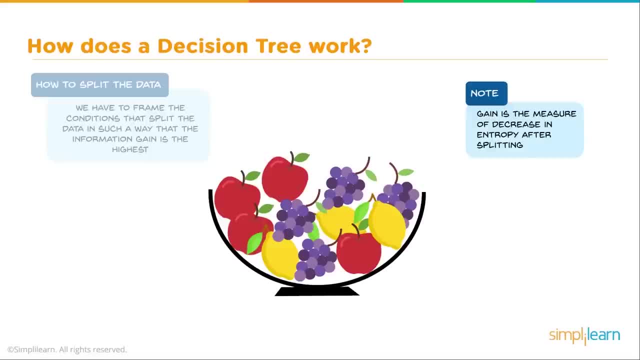 We wanna split it the biggest way we can, And so we measure this decrease in entropy. that's what they call it entropy. there's our entropy after splitting, And now we'll try to choose a condition that gives us the highest gain. 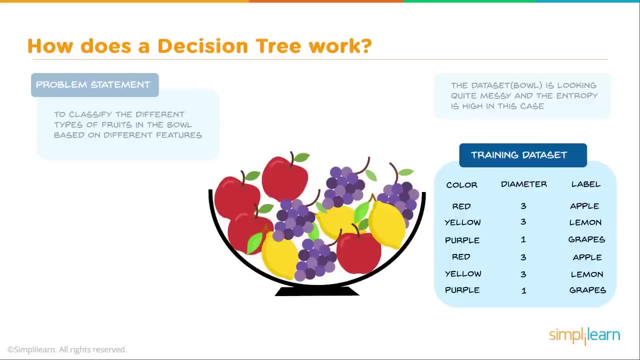 We have the color and under the color we have red, yellow, purple. we have a diameter: three, three one, three three one, And we have a label: apple lemon grapes, apple lemon grapes. And how do we split the data? 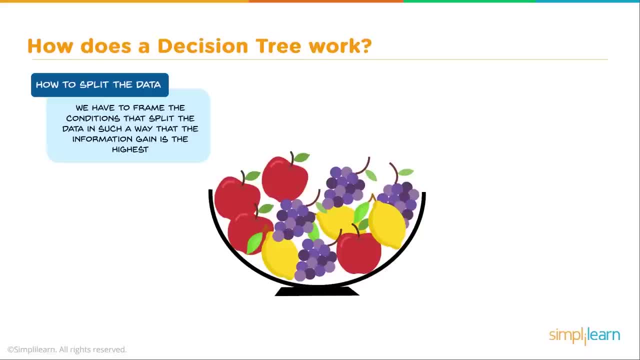 We have to frame the conditions to split the data in such a way that the information gain is the highest. That's very key to note that we're looking for the best gain. We don't want to just start sorting out the smallest piece in there. 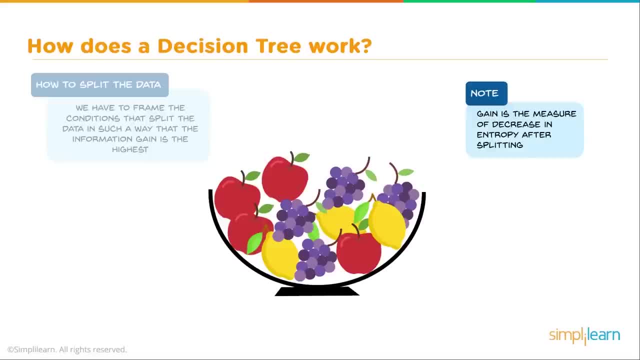 We want to split it the biggest way we can, And so we measure this decrease in entropy. That's what they call it Entropy. There's our entropy. We're splitting, And now we'll try to choose a condition that gives us the highest gain. 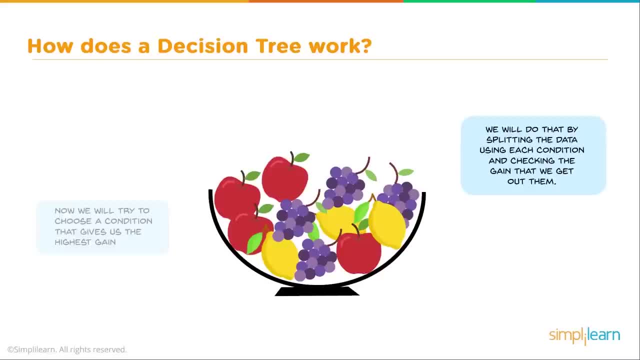 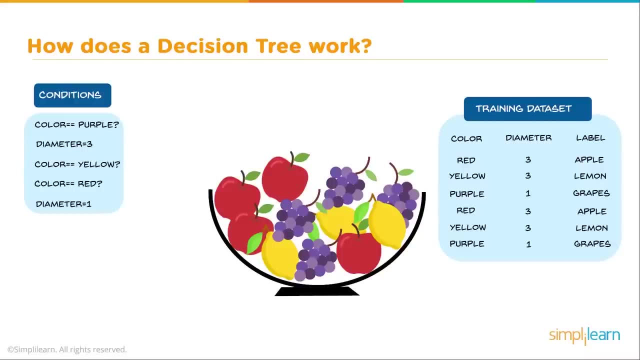 We will do that by splitting the data, using each condition and checking the gain that we get out of them. The conditions that give us the highest gain will be used to make the first split. So let's take a look at these different conditions. We have color, we have diameter. 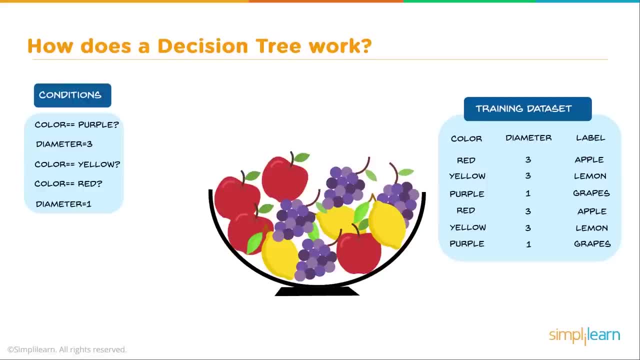 And if we look underneath that we have a couple of different values. We have: diameter equals three, color equals yellow, red, diameter equals one. And when we look at that you'll see over here we have one, two, three, four. 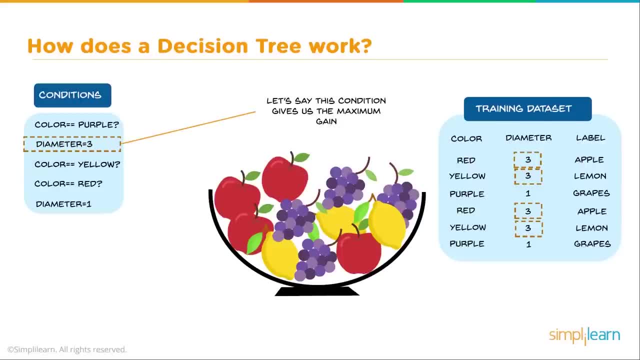 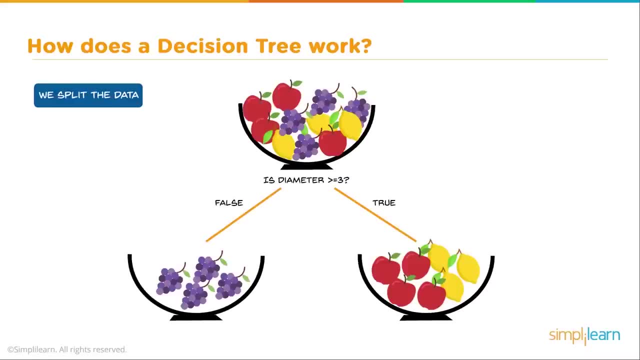 and three. That's a pretty hard selection. So let's say the condition gives us the maximum gain of three, So we have the most pieces fall into that range. So our first split from our decision node is we split the data based on the diameter. 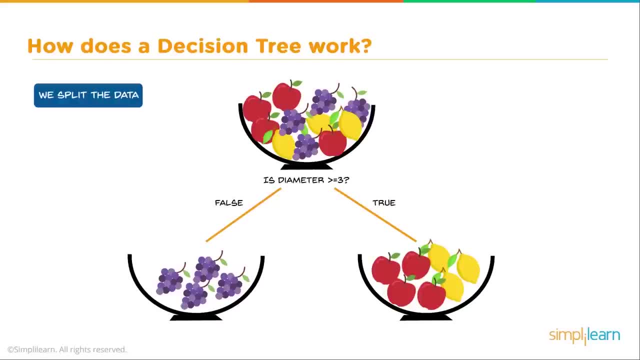 Is it greater than or equal to three? If it's not, that's false- It goes into the great bowl, And if it's true, it goes into a bowl full of lemon and apples. The entropy after splitting has decreased considerably, So now we can make two decisions. 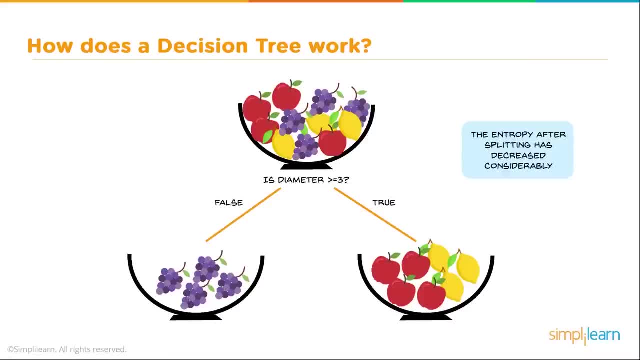 If you look at, they're very much less chaos going on there. This node has already attained an entropy value of zero. As you can see, there's only one kind of label left for this branch, So no further splitting is required for this node. 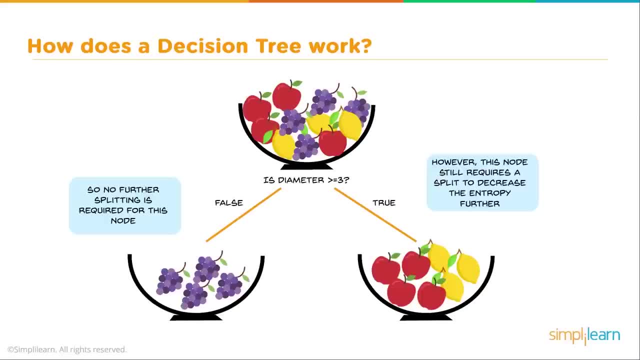 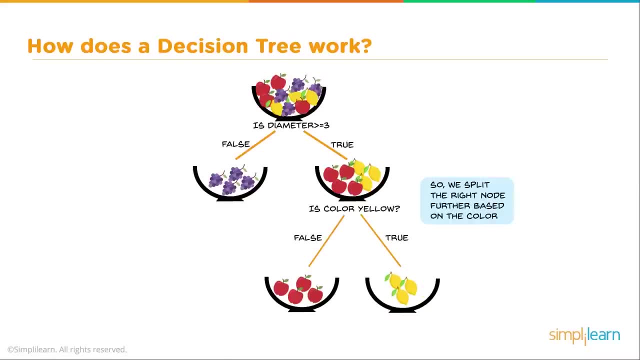 However, this node on the right is still requires a split to decrease the entropy further. So we split the right node further based on color. If you look at this, if I split it on color, that pretty much cuts it right down the middle. 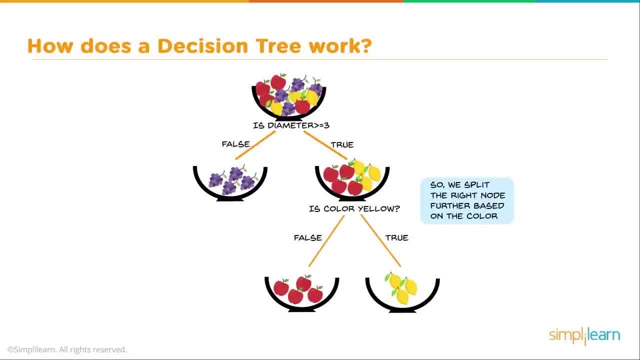 That's the only thing we have left, Based on our choices of color and diameter too, And if the color is yellow, it's going to go to the right bowl, And if it's false, it's going to go to the left bowl. 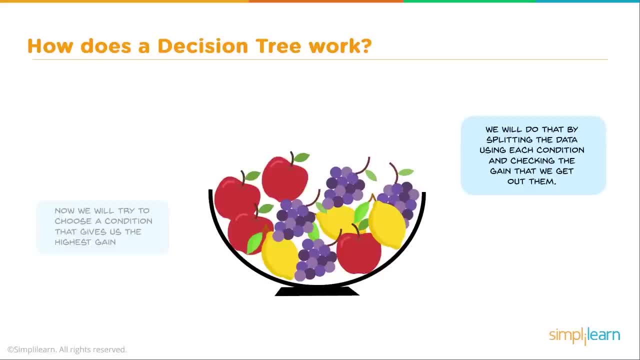 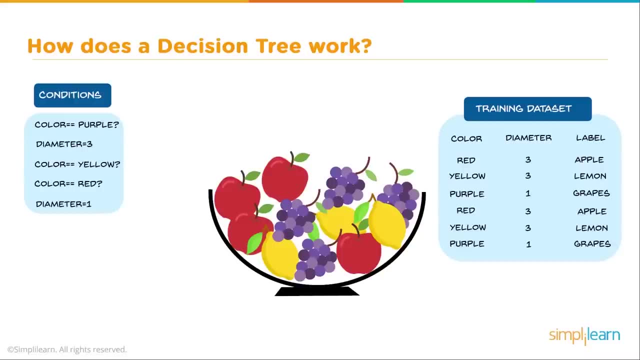 We will do that by splitting the data, using each condition and checking the gain that we get out of them. The conditions that give us the highest gain will be used to make the first split. So let's take a look at these different conditions. We have color, we have diameter. 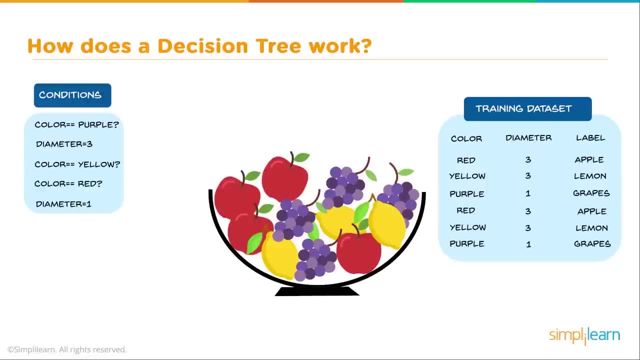 and if we look underneath that, we have a couple different values. We have: diameter equals three, color equals yellow, red, diameter equals one, And when we look at that, you'll see over here we have one, two, three, four, threes. 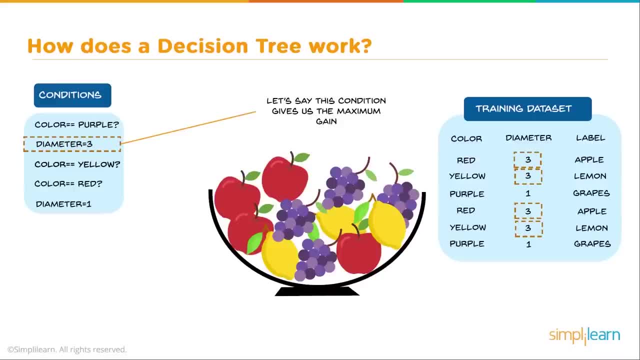 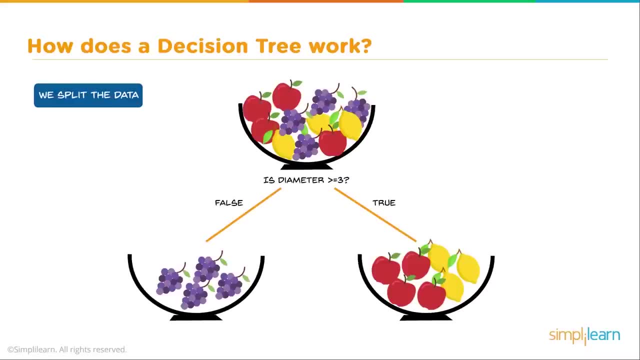 That's a pretty hard selection. So let's say the condition gives us the maximum gain of three, So we have the most pieces fall into that range. So our first split from our decision node is we split the data based on the diameter. Is it greater than or equal to three? 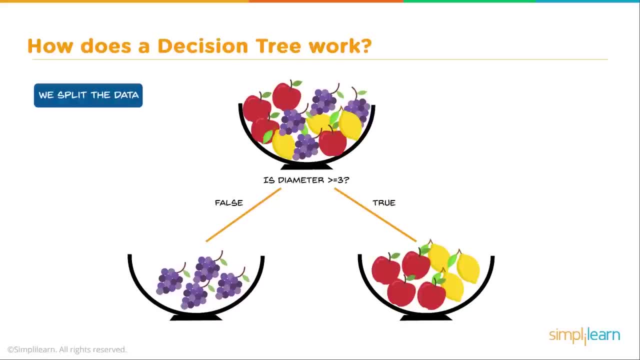 If it's not- that's false- it goes into the grape bowl, And if it's true, it goes into a bowl full of lemon and apples. The entropy after splitting has decreased considerably, So now we can make two decisions. If you look, there's very much less chaos going on there. 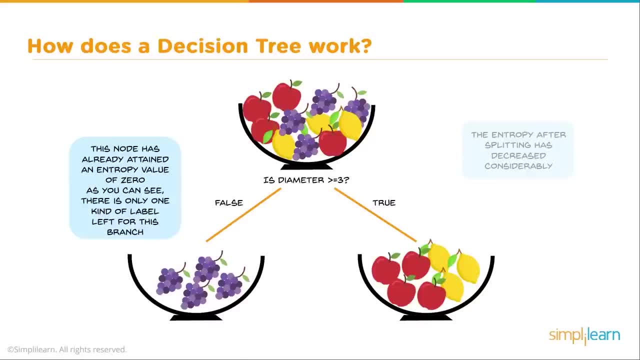 This node has already attained an entropy value of zero. as you can see, There's only one kind of label left for this branch, So no further splitting is required for this node. However, this node on the right still requires a split to decrease the entropy further. 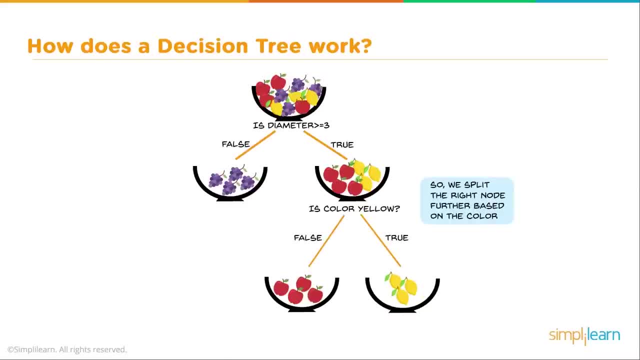 So we split the right node further based on color. If you look at this, if I split it on color, that pretty much cuts it right down the middle. That's the only thing we have left in our choices of color and diameter too. 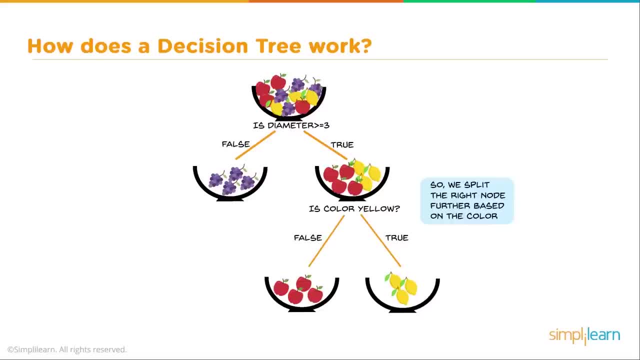 And if the color is yellow, it's gonna go to the right bowl, And if it's false, it's gonna go to the left bowl. So the entropy in this case is now zero. So now we have three bowls with zero entropy. 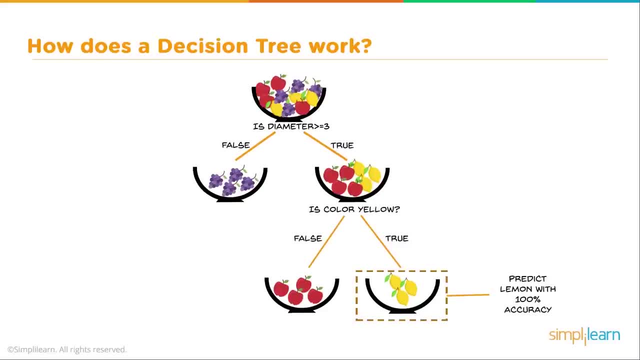 There's only one type of data in each one of those bowls. So we can predict a lemon with 100% accuracy And we can predict the apple also with 100% accuracy, along with our grapes up there. So we've looked at kind of a basic tree in our forest. 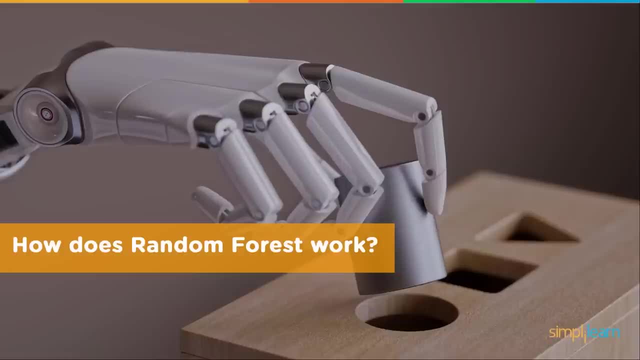 but what we really wanna know is: how does a random forest work as a whole? So to begin our random forest classifier, let's say we already have built three trees And we're gonna start with the first tree that looks like this, Just like we did in the example. 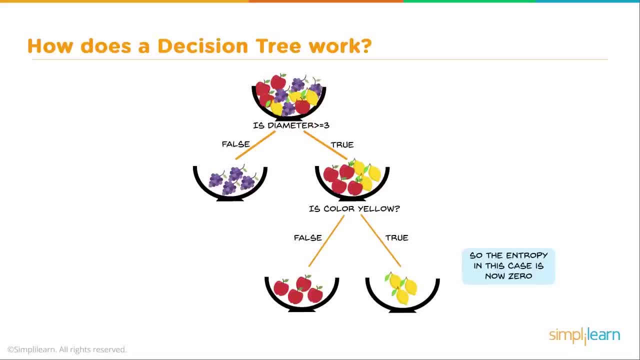 So the entropy in this case is now zero. So now we have three bowls with zero entropy. There's only one type of data in each one of those bowls, So we can predict a lemon with 100 percent accuracy and we can predict the apple. 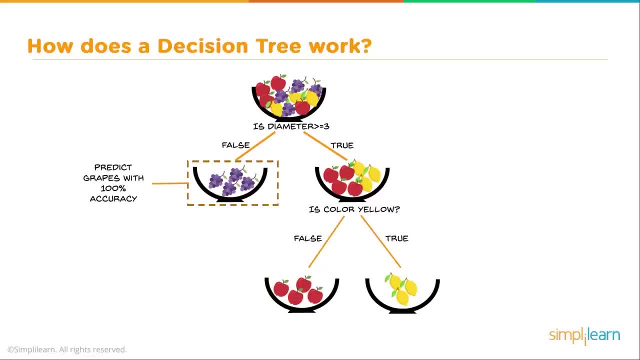 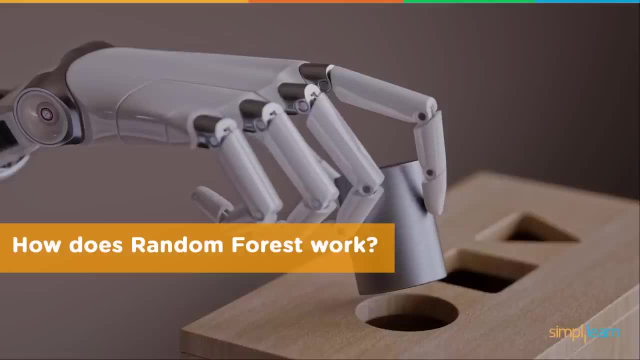 also with 100 percent accuracy, along with our grapes up there. So we've looked at kind of a basic tree in our forest. But what we really want to know is how does a random forest work as a whole? So to begin our random forest classifier. 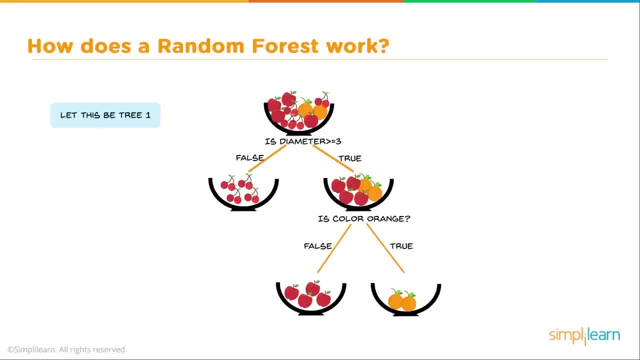 let's say we already have built three trees and we're going to start with the first tree that looks like this, just like we did in the example. This tree looks at the diameter If it's greater than or equal to three. it's true. 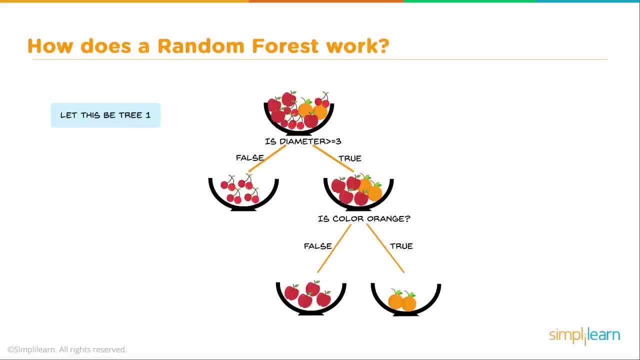 Otherwise it's false. So one side goes to the smaller diameter, one side goes to larger diameter. And if the color is orange, it's going to go to the right. True, We're using oranges now instead of lemons. And if it's red, it's going to go to the left. 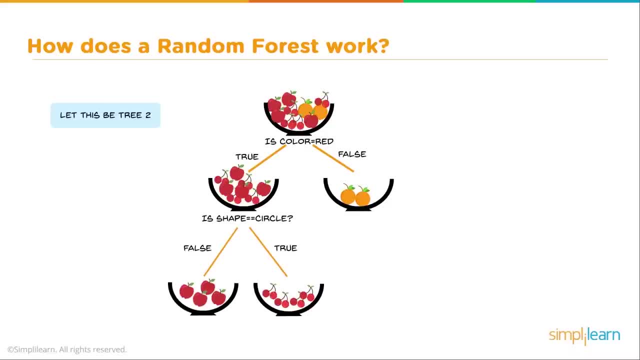 False. We build a second tree, very similar but split differently. Instead of the first one being split by a diameter, This one. when they created it. if you look at that first bowl, it has a lot of red objects. So it says, is the color red? 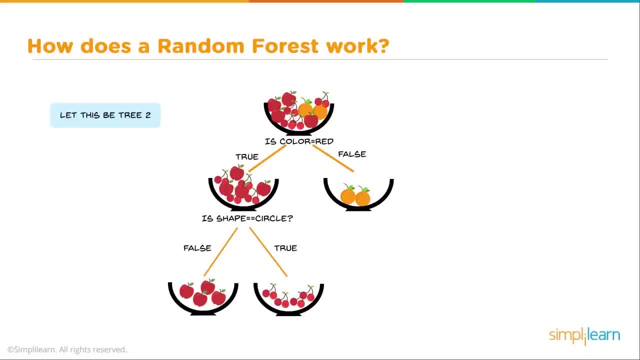 Because that's going to bring our entropy down the fastest. And so, of course, if it's true, it goes to the left, If it's false, it goes to the right, And then it looks at the shape: false or true, and so on and so on. 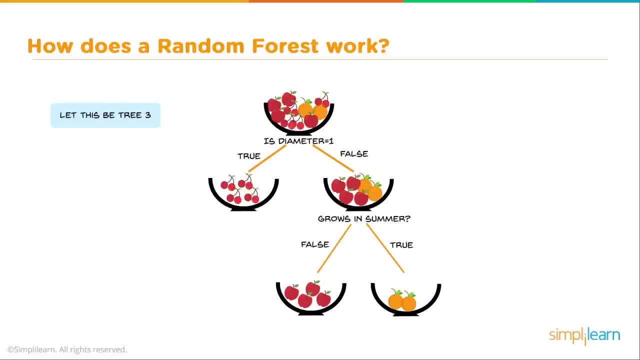 And tree three is the diameter equal to one, And it came up with this because there's a lot of cherries in this bowl, So that would be the biggest split on there is is the diameter equal to one. That's going to drop the entropy the quickest. 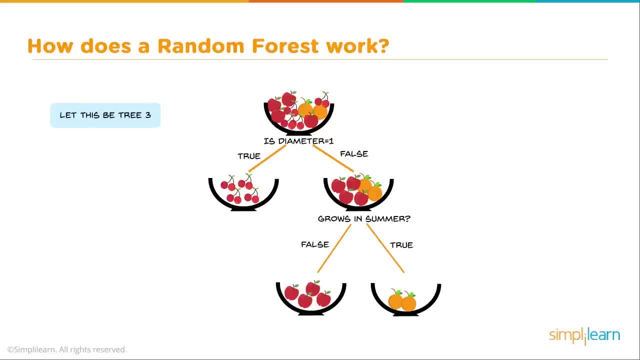 And, as you can see, it splits it into true. If it goes false- and they've added another category: does it grow in the summer? And if it's false, it goes off to the left. If it's true, it goes off to the right. 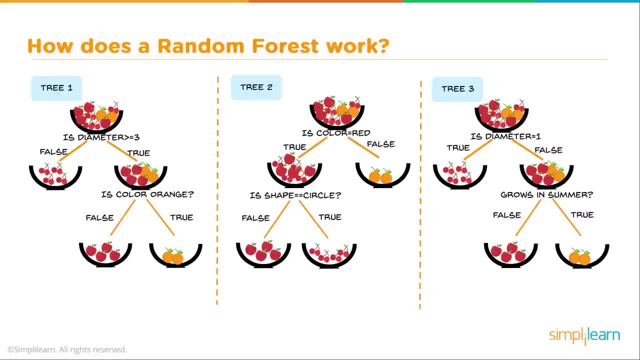 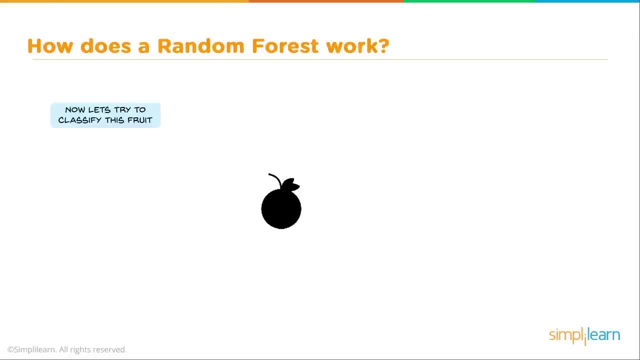 Let's go ahead and bring these three trees. You can see them all in one image. So this would be three completely different trees categorizing a fruit, and let's take a fruit. Now. let's try this And this fruit. if you look at it, we've blackened it out. 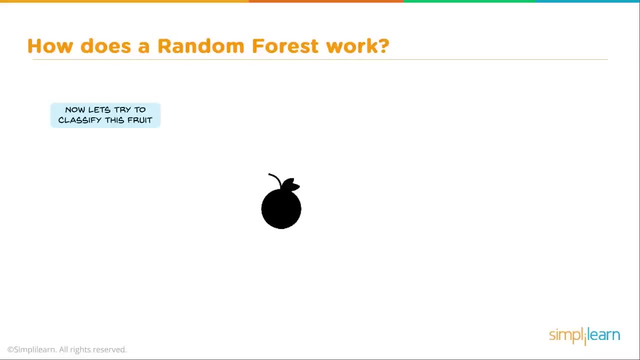 You can't see the color on it, So it's missing data. Remember, one of the things we talked about earlier is that a random forest works really good if you're missing data, if you're missing pieces. So this fruit has an image. 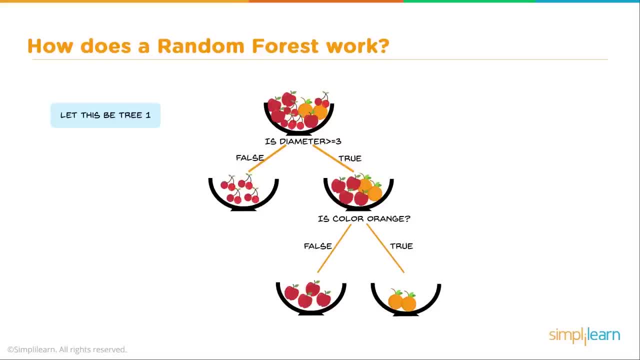 this tree looks at the diameter. If it's greater than or equal to three, it's true. otherwise it's false. So one side goes to the smaller diameter, one side goes to the larger diameter, And if the color is orange it's gonna go to the right, true? 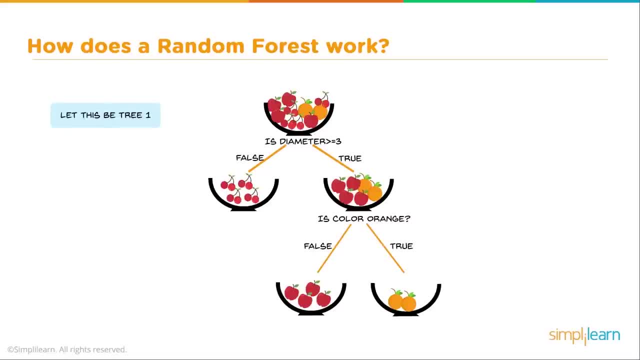 We're using oranges now instead of lemons, And if it's red it's gonna go to the left, false. We build a second tree, very similar, but it's split differently, Instead of the first one being split by a diameter. 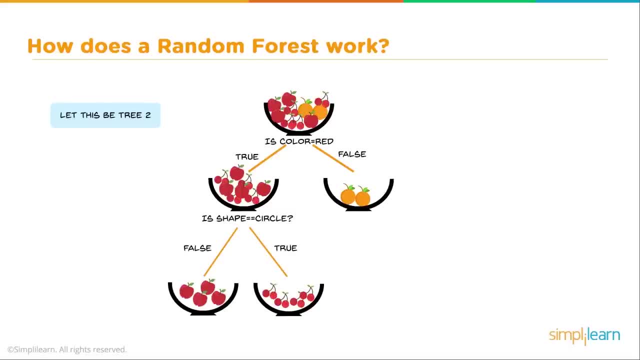 this one when they created it. if you look at that first bowl, it has a lot of red objects. So it says, is the color red Because that's gonna bring our entropy down the fastest? And so of course, if it's true, it goes to the left. 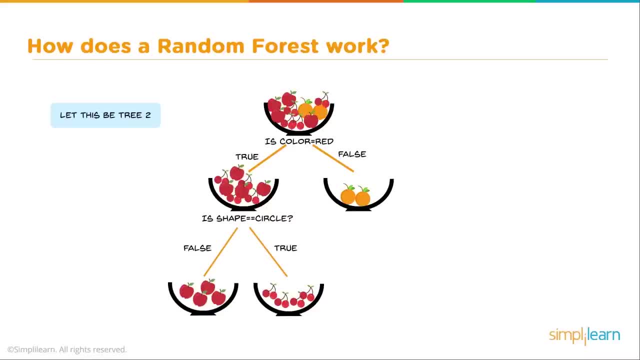 If it's false, it goes to the right And then it looks at the shape- false or true, and so on and so on. And tree three is the diameter equal to one, And it came up with this because there's a lot of cherries in this bowl. 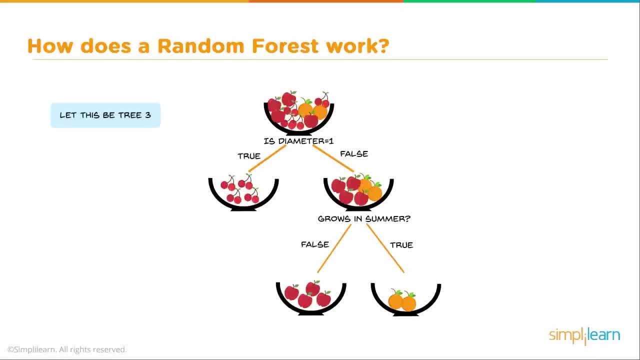 So that would be the biggest split on there is: is the diameter equal to one? That's gonna drop the entropy the quickest And, as you can see, it splits it into true If it goes false. and they've added another category: does it grow in the summer? 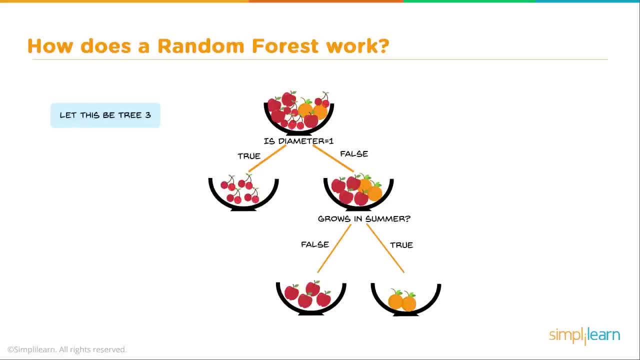 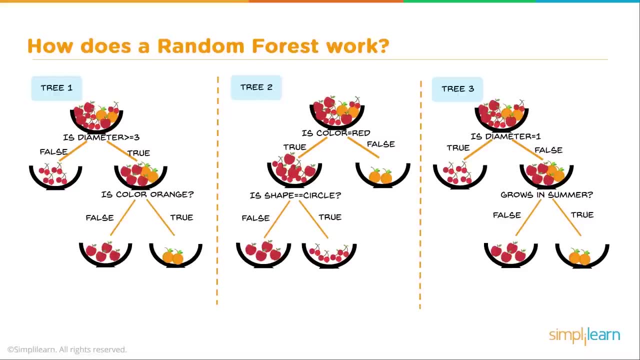 And if it's false, it goes off to the left. If it's true, it goes off to the right. Let's go ahead and bring these three trees. You can see them all in one image. So this would be three completely different trees. 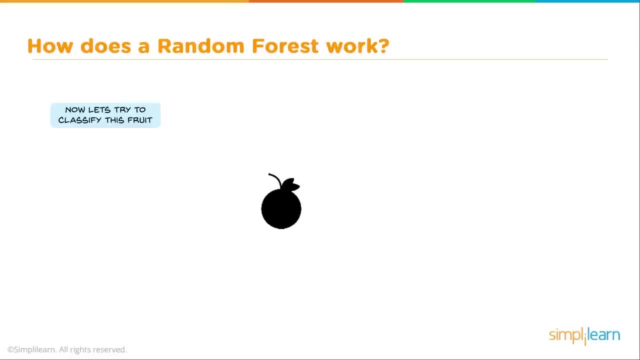 categorizing a fruit. And let's take a fruit Now. let's try this And this fruit. if you look at it, we've blackened it out. You can't see the color on it, So it's missing data. Remember one of the things we talked about earlier. 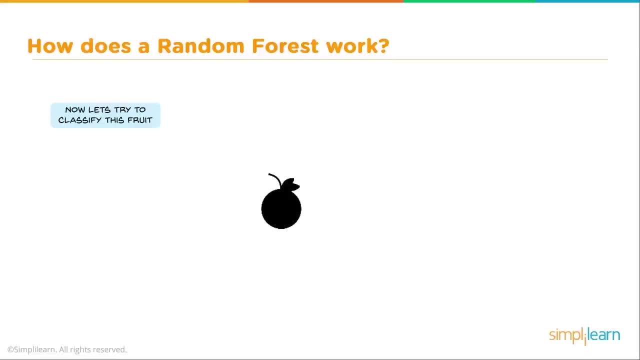 is that a random forest works really good if you're missing data, if you're missing pieces. So this fruit has an image, but maybe the person had a black and white camera when they took the picture And we're gonna take a look at this. 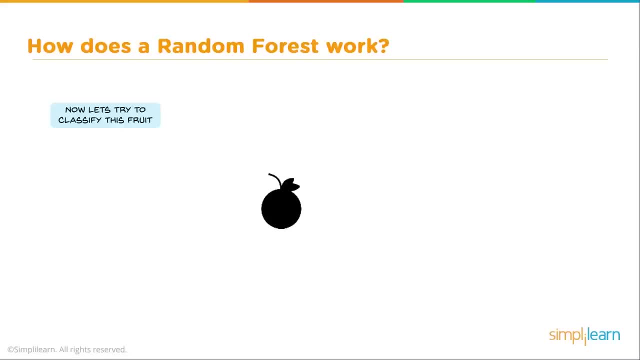 and it's gonna have. they put the color in there, So ignore the color down there. But the diameter equals three, We find out it grows in the summer. equals, yes, And the shape is a circle. And if you go to the right, 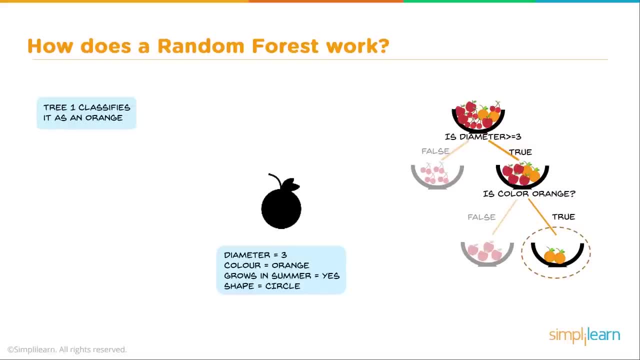 you can look at what one of the decision trees did. This is the third one. Is the diameter greater than or equal to three? Is the color orange? Well, it doesn't really know on this one, but if you look at the value it'd say true. 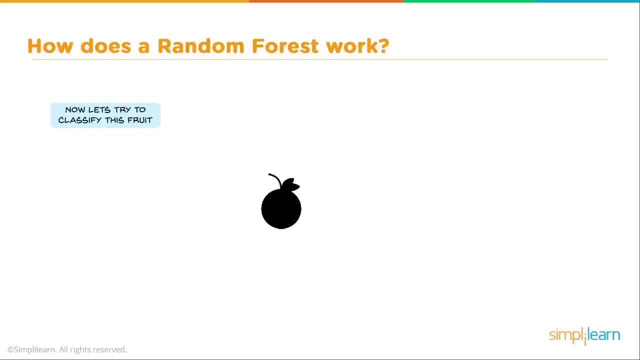 but maybe the person had a black and white camera when they took the picture And we're going to take a look at this and it's going to have they put the color in there, so ignore the color down there, But the diameter. 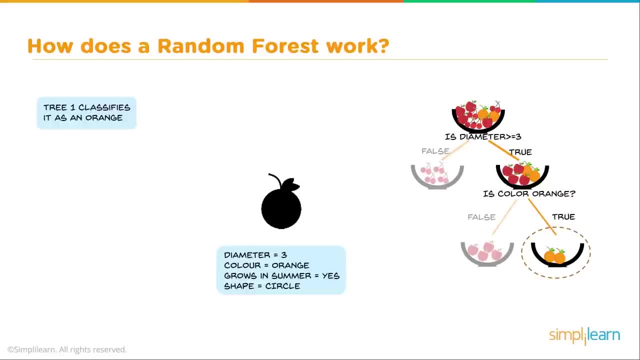 equals three. we find out it grows in the summer. equals yes, And the shape is a circle And if you go to the right you can look at what one of the decision trees did. This is the third one. Is the diameter greater than equal to three? 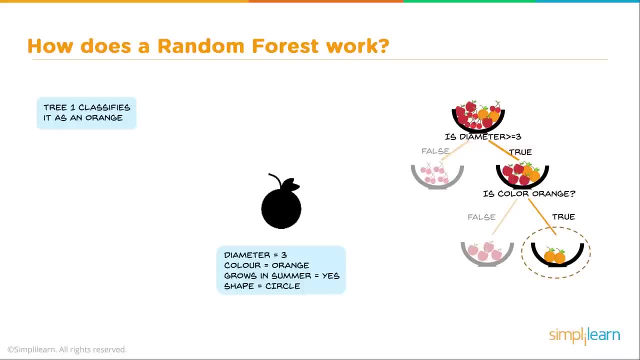 Is the color orange. Well, it doesn't really know on this one, but if you look at the value it'd say true and you go to the right Tree. two classifies it as: cherries Is the color equal. red Is the shape: a circle. 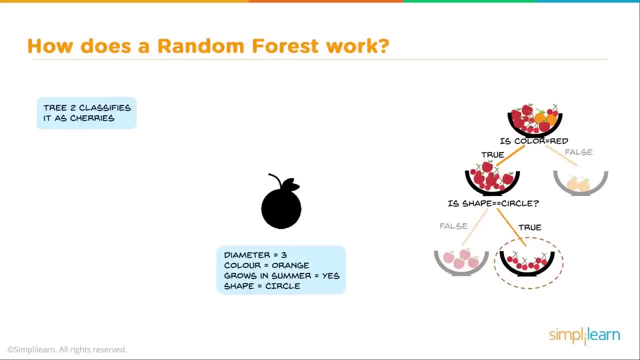 True, it is a circle. So this would look at it and say, oh, that's a cherry. And then we go to the other classifier and it says: is the diameter equal one? Well, that's false. Does it grow in the summer? 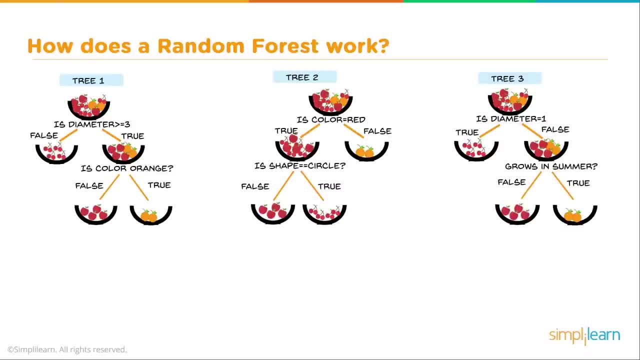 True. So it goes down and looks up as oranges. So how does this random forest work? The first one says it's an orange, The second one said it was a cherry And the third one says it's an orange. And you can guess if you have two oranges and one says it's a cherry. 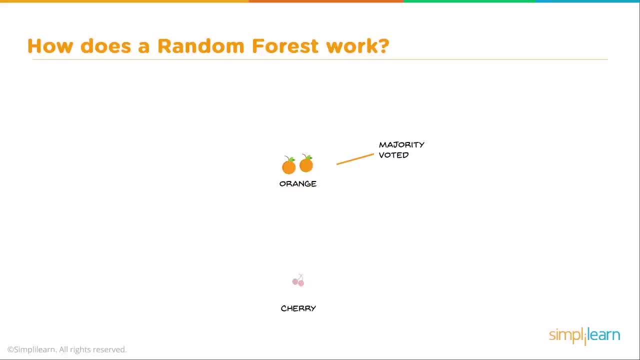 When you add that all together, the majority of the vote says orange, So the answer is it's classified as an orange, Even though we didn't know the color and we're missing data on it. I don't know about you, but I'm getting tired of fruit. 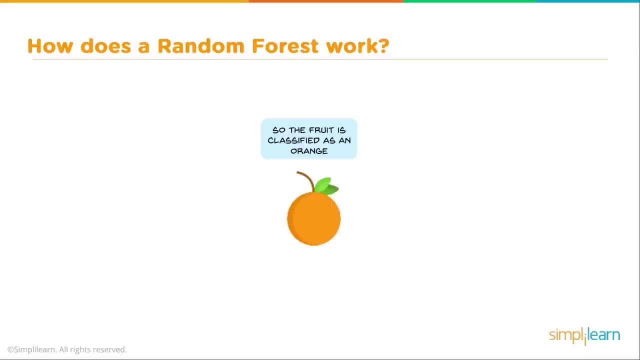 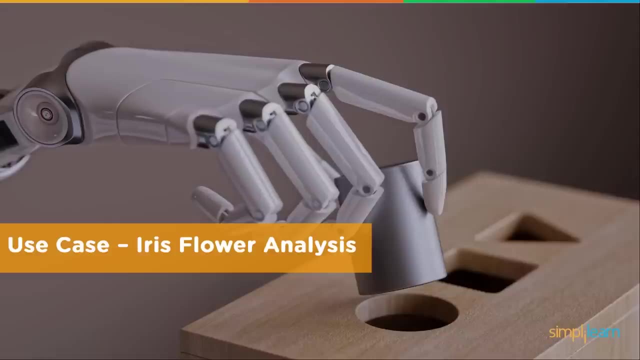 So let's switch, And I did promise you we'd start looking at a case example and get into some Python coding. Today we're going to use the case the iris flower analysis. This is the exciting part, as we roll up our sleeves and actually look at some Python coding. 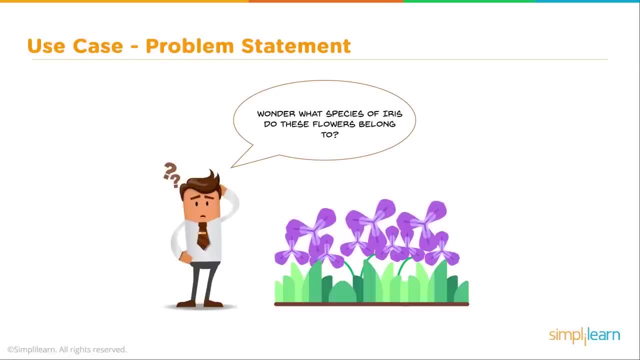 Before we start the Python coding, we need to go ahead and create a problem statement, Wonder: what species of iris do these flowers belong to? Let's try to predict the species of the flowers using machine learning in Python. Let's see how it can be done. 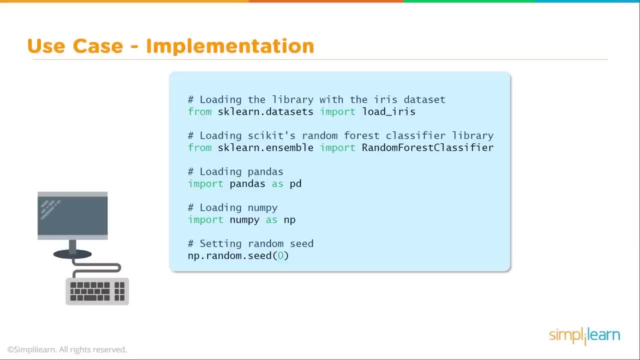 So here we begin to go ahead and implement our Python code, And you'll find that the first half of our implementation is all about organizing and exploring the data coming in. Let's go ahead and take this first step, which is loading the different modules into Python. 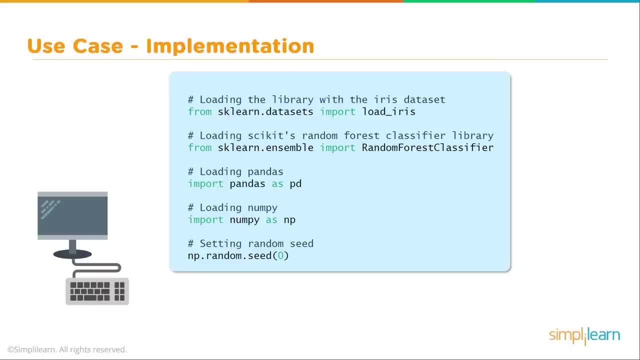 And let's go ahead and put that in our favorite editor. whatever your favorite editor is, In this case I'm going to be using the Anaconda, the Jupyter Notebook, which is one of my favorites. Certainly, there's Notepad++ and Eclipse. 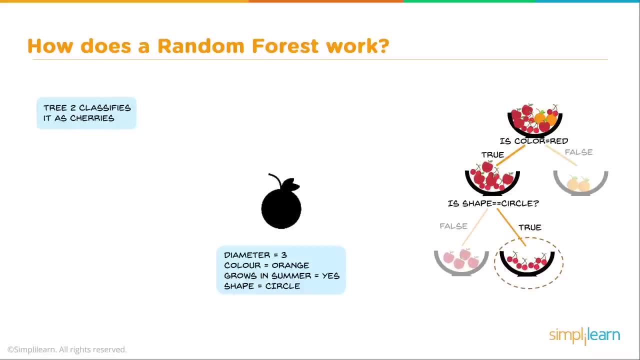 and it'd go to the right Tree. two: classifies it as cherries. Is the color equal red? Is the shape a circle? True, it is a circle. So this would look at it and say, oh, that's a cherry. 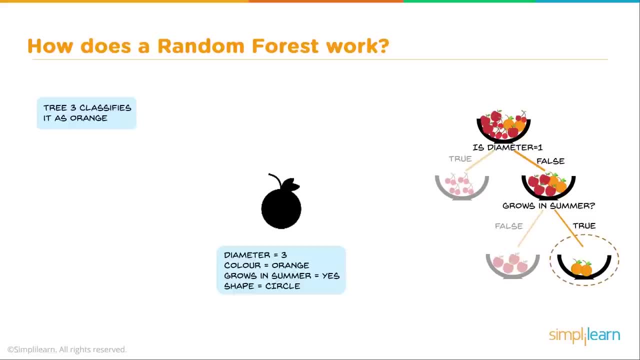 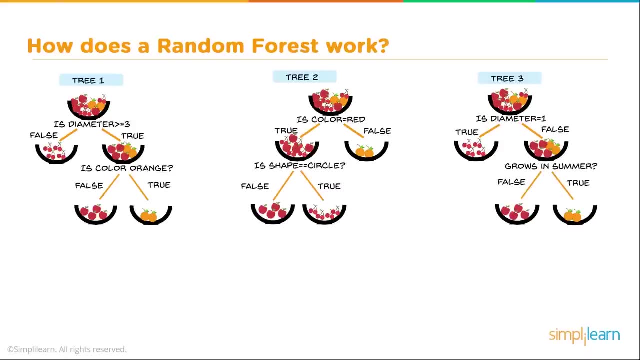 And then we go to the other classifier and it says: is the diameter equal one? Well, that's false. Does it grow in the summer? True, so it goes down and looks at as oranges. So how does this random forest work? 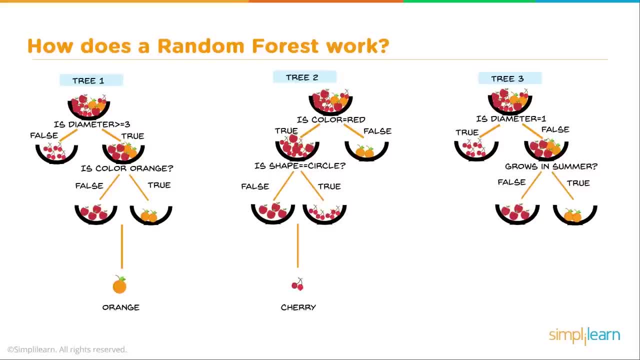 The first one says it's an orange, The second one said it was a cherry And the third one says, hmm, it's an orange. And you can guess that if you have two oranges and one says it's a cherry, when you add that all together, 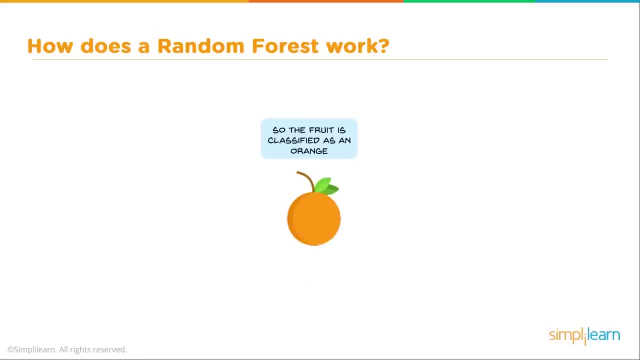 the majority of the vote says orange, So the answer is: it's classified as an orange, even though we didn't know the color and we're missing data on it. I don't know about you, but I'm getting tired of fruit, So let's switch, and I did promise you. 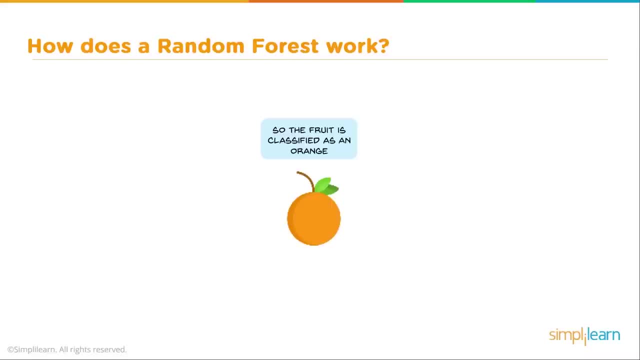 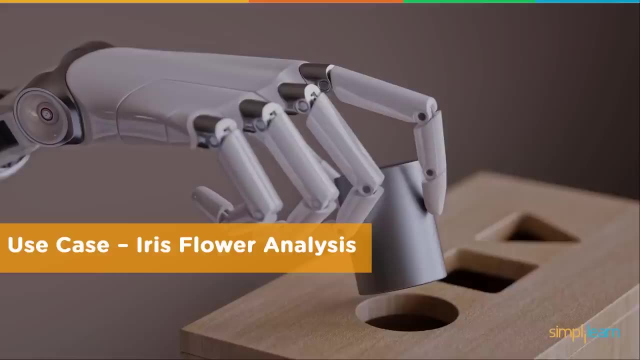 we'd start looking at a case example and get into some Python coding. Today we're gonna use the case the iris flower analysis. Ooh, this is the exciting part, as we roll up our sleeves and actually look at some Python coding. Before we start the Python coding: 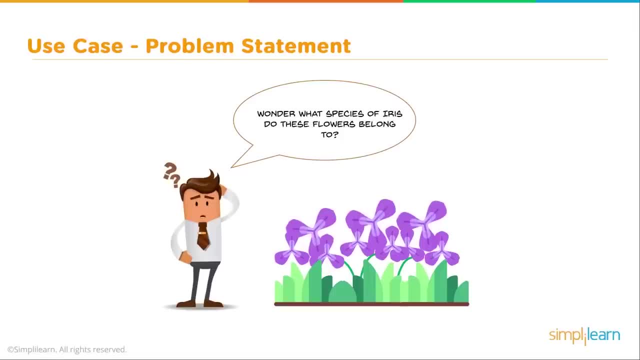 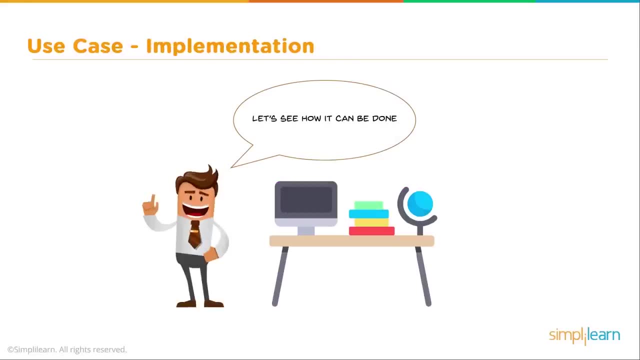 we need to go ahead and create a problem statement, Wonder: what species of iris do these flowers belong to? Let's try to predict the species of the flowers using machine learning in Python. Let's see how it can be done. So here we begin to go ahead and implement our Python code. 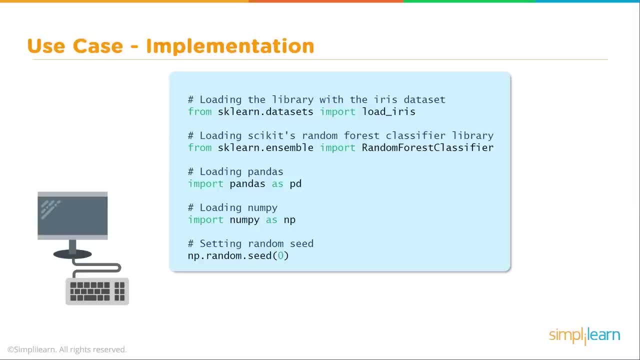 And you'll find that the first half of our implementation is all about organizing and exploring the data coming in. Let's go ahead and take this first step, which is loading the different modules into Python, and let's go ahead and put that in our favorite editor. 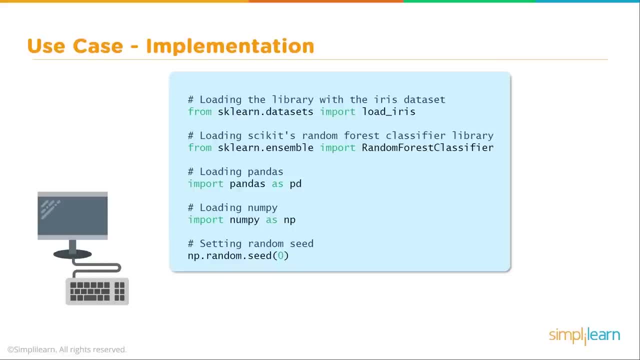 whatever your favorite editor is- In this case I'm gonna be using the Anaconda Jupyter Notebook, which is one of my favorites. Certainly there's Notepad++ and Eclipse and dozens of others, or just even using the Python terminal window. 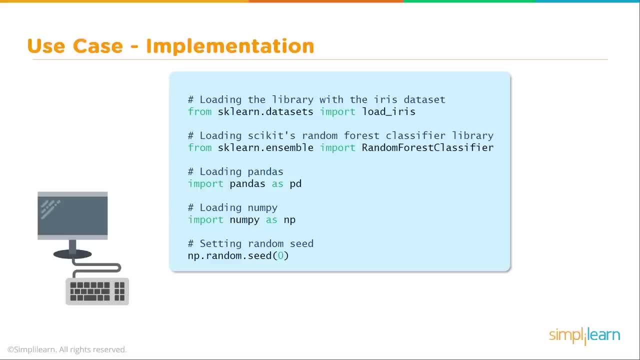 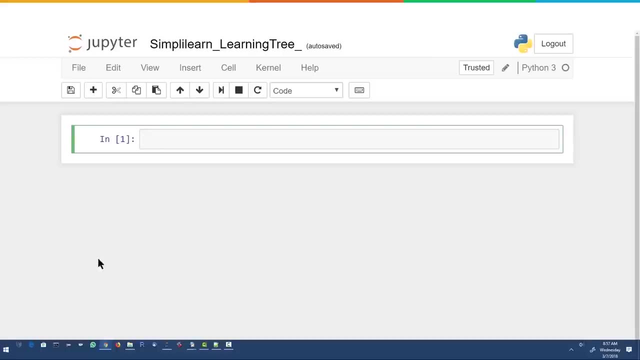 Any of those will work just fine to go ahead and explore this Python coding. So here we go. Let's go ahead and flip over to our Jupyter Notebook, And I've already opened up a new page for Python 3 code and I'm just gonna paste this right in there. 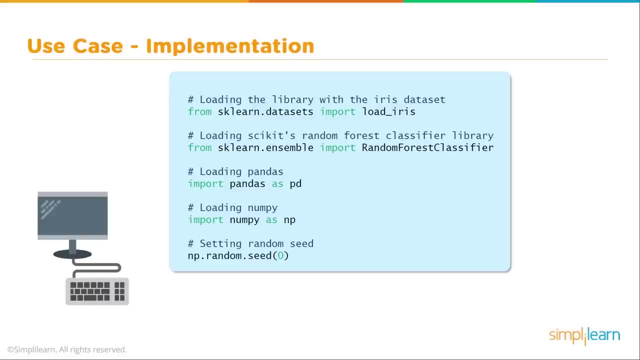 and dozens of others, or just even using the Python terminal window- Any of those will work just fine to go ahead and explore this Python coding. So here we go. Let's go ahead and flip over to our Jupyter Notebook, And I've already opened up a new page for Python 3 code. 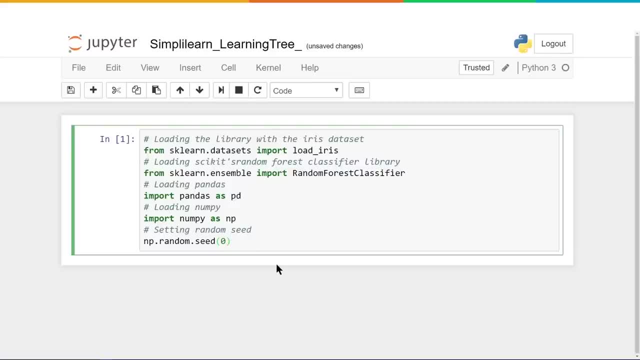 And I'm just going to paste this right in there And let's take a look and see what we're bringing into our Python. The first thing we're going to do is, from the sklearndata sets, import load iris. Now, this isn't the actual data. 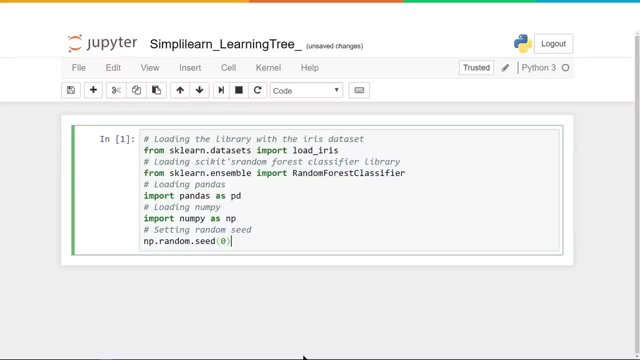 This is just the module that allows us to bring in the data, the load iris- And the iris is so popular- It's been around since 1936 when Ronald Fisher published a paper on it- And they're measuring the different parts of the flower and, based on those measurements, predicting what kind of flower it is. 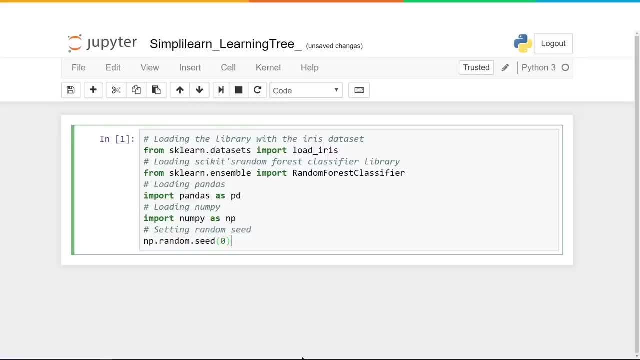 And then if we're going to do a random forest classifier, we need to go ahead and import a random forest classifier from the sklearn module. So sklearnonLine Ensemble, import random forest classifier, And then we want to bring in two more modules. 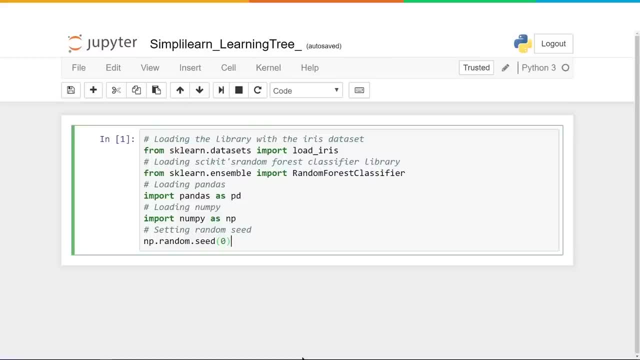 And these are probably the most commonly used modules in Python and data science. with any of the other modules that we bring in, And one is going to be pandas- We're going to import pandas as PD- PD is a common term used for pandas. 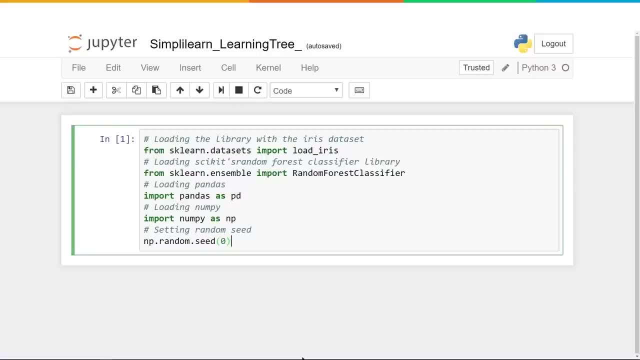 And pandas is basically creates a data format for us where when you create a pandas data frame, it looks like an Excel spreadsheet, And you'll see that in a minute when we start digging deeper into the code. Pandas is just wonderful because it plays nice with all the other modules in there. 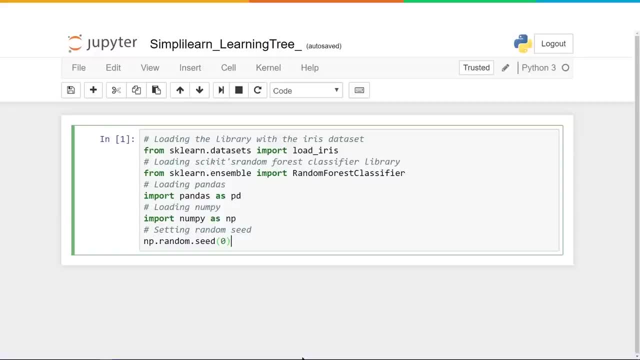 And then we have numpy, which is our numbers Python, And the numbers Python allows us to do different mathematical sets on here. We'll see right off the bat, We're going to take our NP and we're going to go ahead and seed the randomness with it. 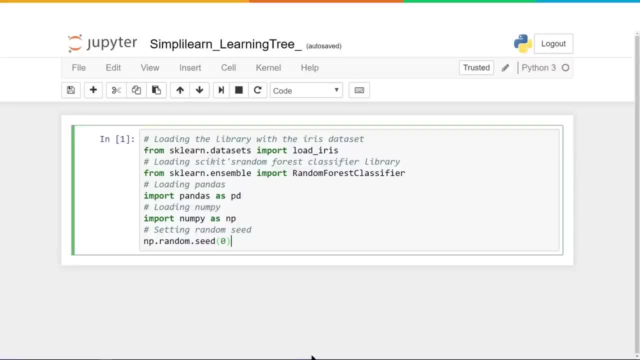 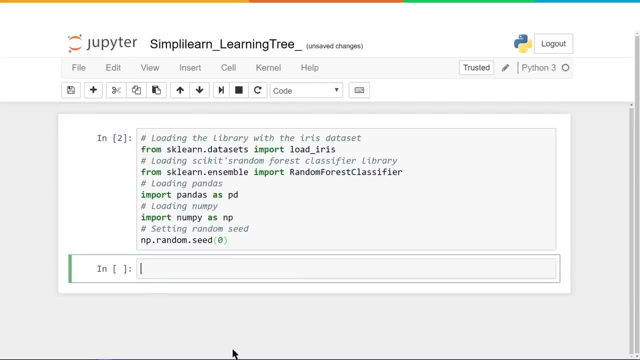 with zero, So nprandomseed is seeding that as zero. This code doesn't actually show anything. We're going to go ahead and run it, because I need to make sure I have all those loaded, And then let's take a look at the next module on here. 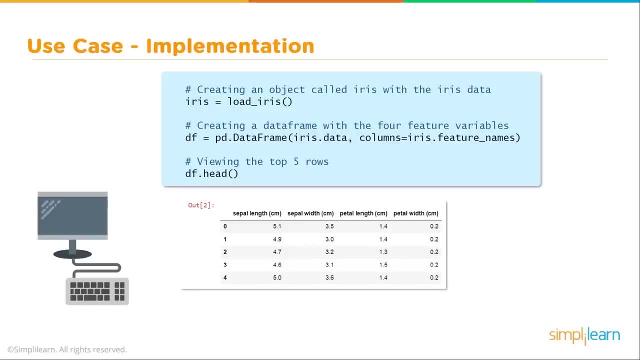 The next six slides, including this one, are all about exploring the data. Remember, I told you half of this is about looking at the data and getting it all set. So let's go ahead and take this code right here: the script. 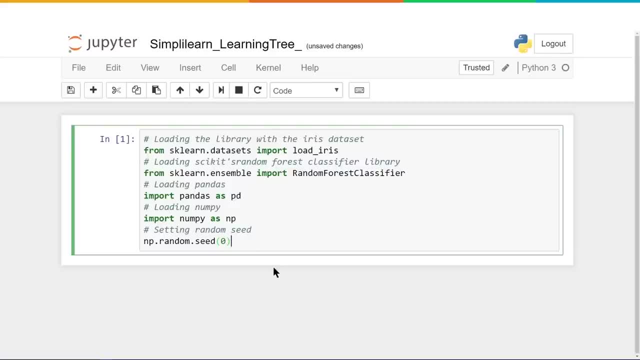 And let's take a look and see what we're bringing into our Python. The first thing we're gonna do is, from the sklearndatasets, import load iris. Now, this isn't the actual data. This is just the module that allows us to bring in the data, the load iris. 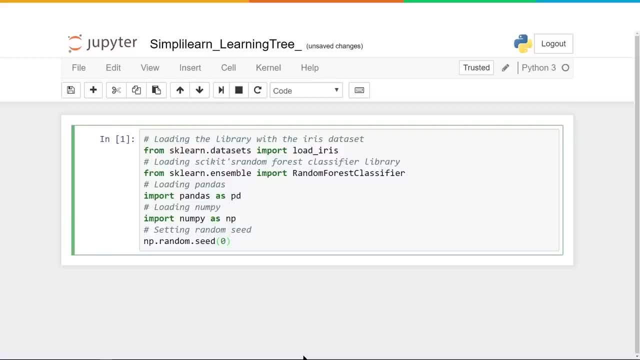 And the iris is so important and so popular. it's been around since 1936, when Ronald Fisher published a paper on it, And they're measuring the different parts of the flower And, based on those measurements, predicting what kind of flower it is. 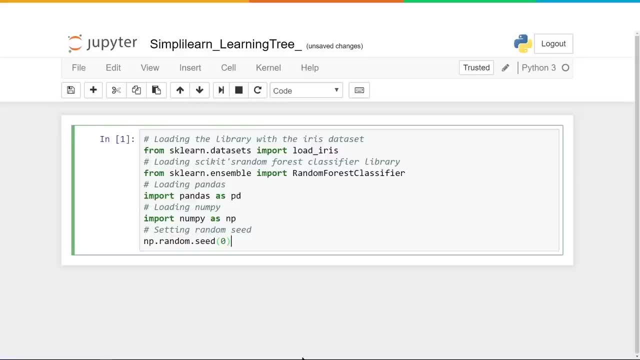 And then if we're gonna do a random forest classifier, we need to go ahead and import a random forest classifier from the sklearn module. So sklearnensemble, import random forest classifier. And then we wanna bring in two more modules And these are probably the most commonly used modules. 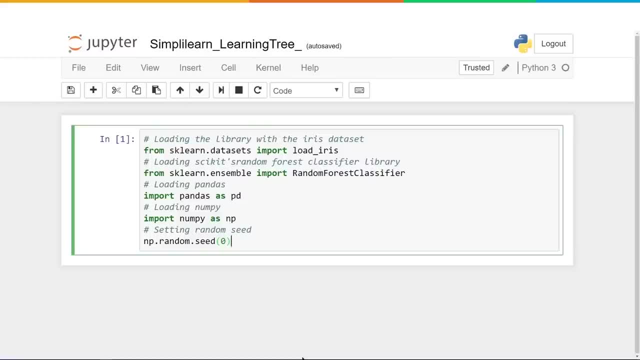 in Python and data science, With any of the other modules that we bring in, And one is gonna be pandas. We're gonna import pandas as pd- Pd is the common term used for pandas- And pandas is basically creates a data format for us. 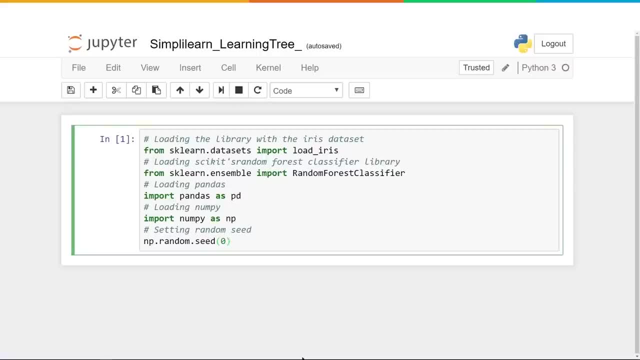 where, when you create a pandas data frame, it looks like an XScale spreadsheet, And you'll see that in a minute when we start digging deeper into the code. Panda is just wonderful because it plays nice with all the other modules in there. And then we have numpy, which is our numbers Python. 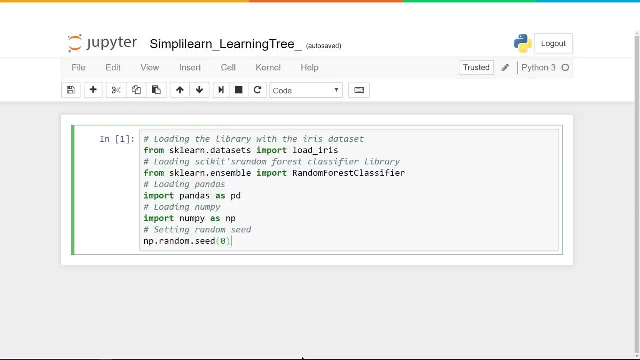 Numbers. Python allows us to do different mathematical sets on here. We'll see right off the bat, we're gonna take our np and we're gonna go ahead and seed the randomness with it with zero. So nprandomseed is seeding that as zero. 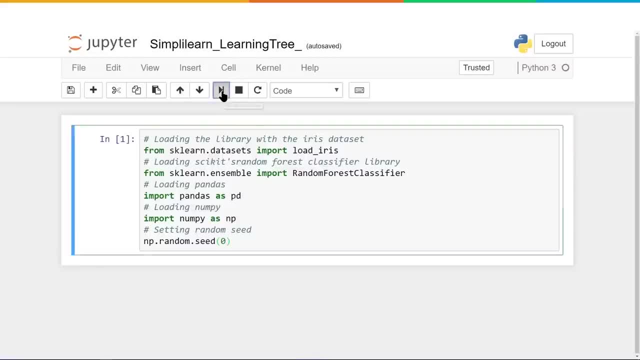 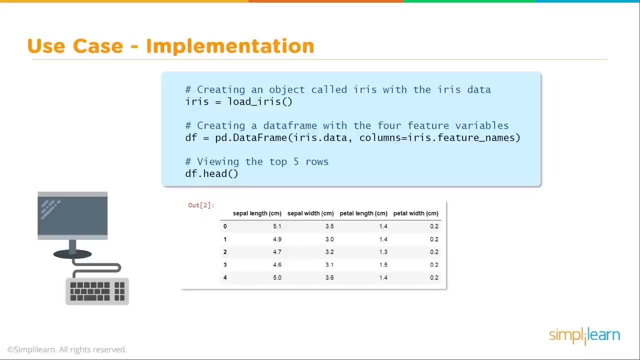 This code doesn't actually show anything. We're gonna go ahead and run it, cause I need to make sure I have all those loaded. And then let's take a look at the next module on here, The next six slides, including this one. 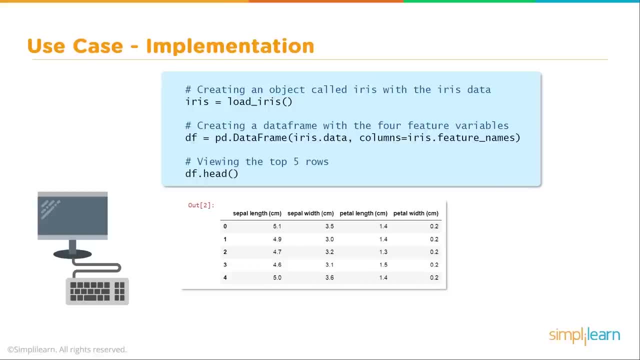 are all about exploring the data. Remember, I told you half of this is about looking at the data, getting it all set. So let's go ahead and take this code right here, the script, and let's get that over into our Jupyter notebook. 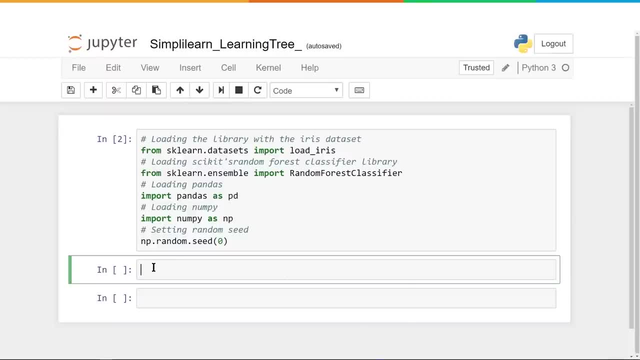 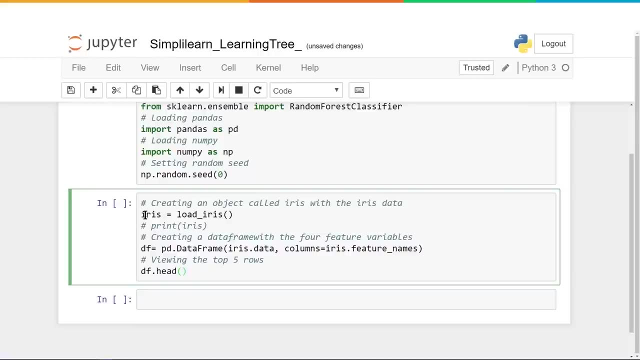 And here we go. we've gone ahead and run the imports And I'm gonna paste the code down here And let's take a look and see what's going on. The first thing we're doing is we're actually loading the iris data. 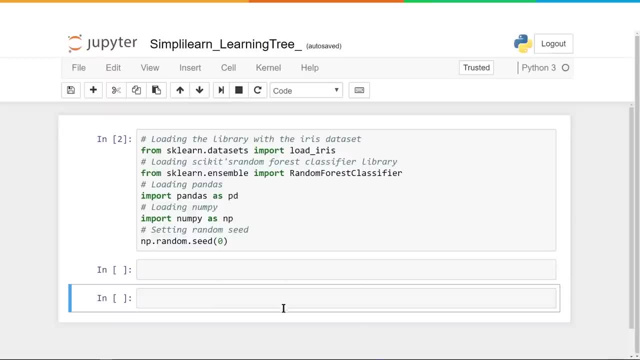 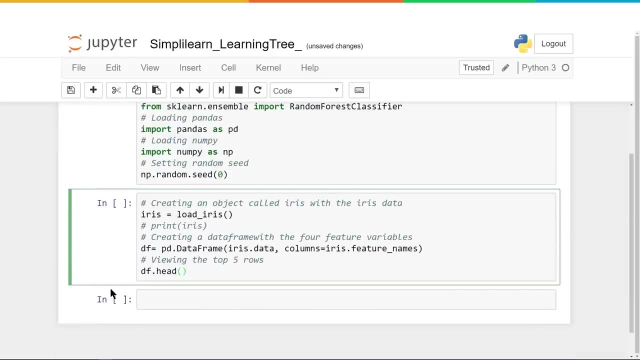 And let's get that over into our Jupyter notebook. And here we go. We've gone ahead and run the imports and I'm going to paste the code down here And let's take a look and see what's going on. The first thing we're doing is we're actually loading the 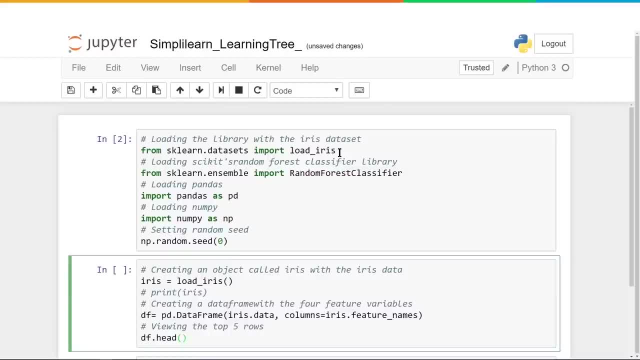 iris data and, if you remember, up here we loaded the module that tells it how to get the iris data. Now we're actually assigning that data to the variable iris And then we're going to go ahead and use the DF to define data frame. 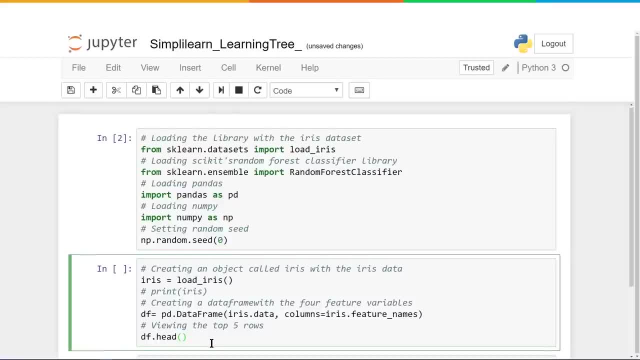 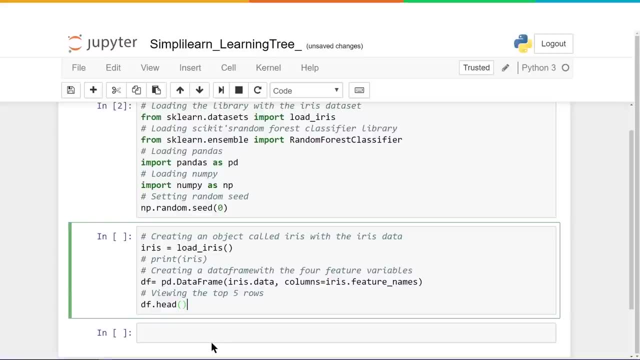 And that's going to equal PD And if you remember, that's pandas as PD. So that's our pandas and panda data frame. And then we're looking at iris data and columns equals iris feature names And we're going to do the DF head. 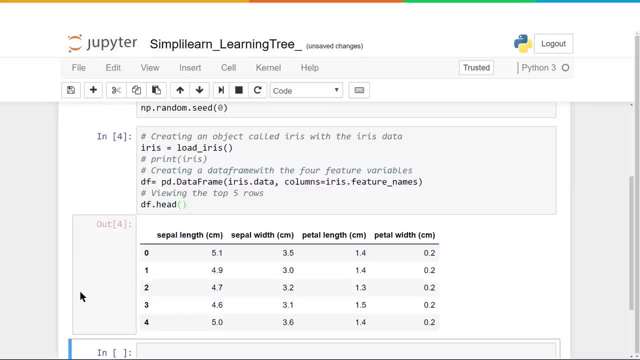 And let's run this So you can understand what's going on here. The first thing you want to notice is that our DF has created what looks like an Excel spreadsheet, And in this Excel spreadsheet we have set the columns, So up on the top you can see the four different columns. 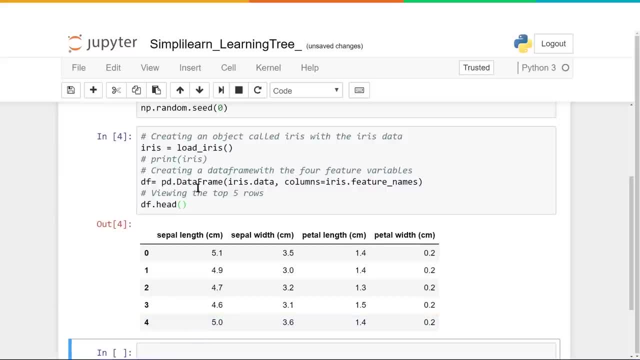 And then we have the data- iris data- down below. It's a little confusing without knowing where this data is coming from. So let's look at the bigger picture and I'm going to go print. I'm just going to change this for a moment. 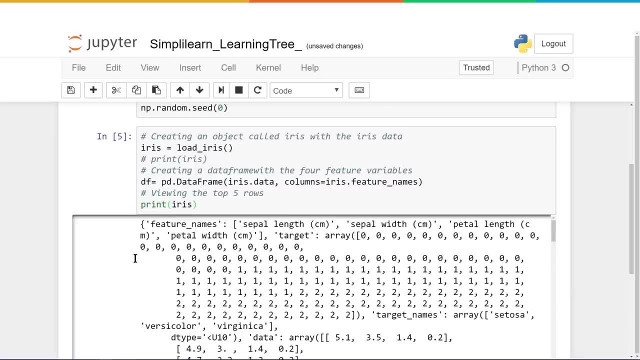 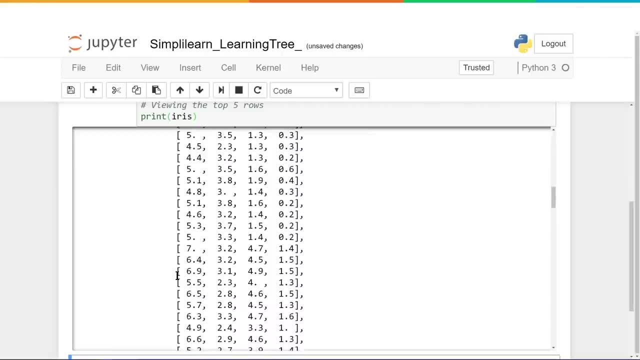 And we're going to print all of iris and see what that looks like. So when I print all of iris, I get this long list of information And you can scroll through here and see all the different titles on there. What's important to notice is that, first off, there's a brackets at the beginning. 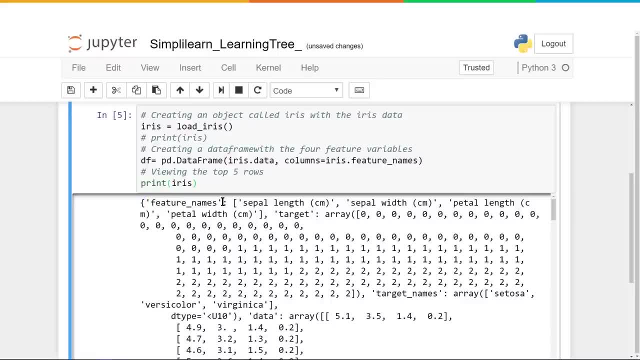 So this is a Python dictionary, And in a Python dictionary you'll have a key or a label And this label pulls up whatever information comes after it. So feature names, which we actually used over here for columns- is equal to an array of sepal length, sepal width. petal length, petal width. 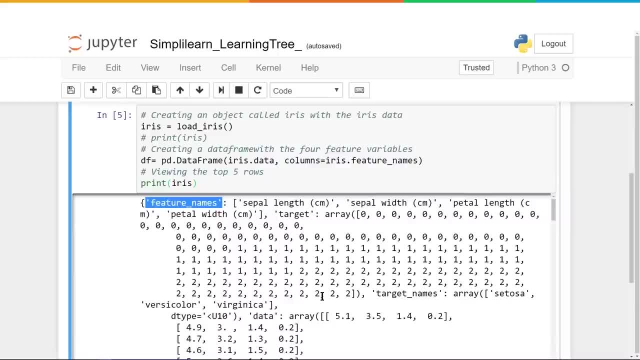 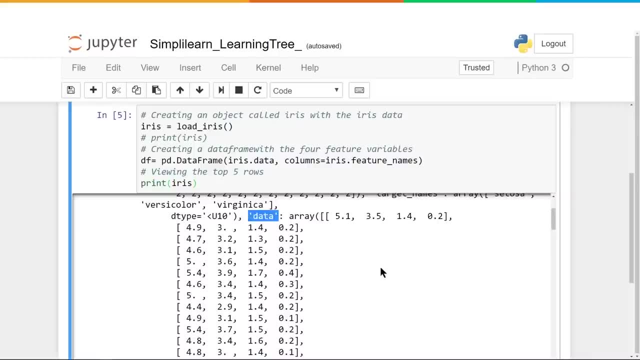 These are the different names they have for the four different columns And if you scroll down far enough, you'll also see data down here. Oh goodness, it came up right towards the top And data is equal to the different data we're looking at. 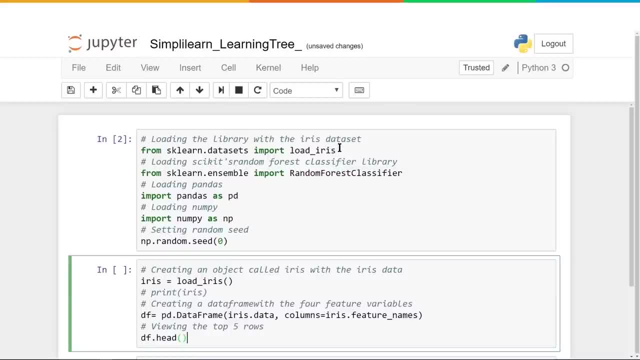 And, if you remember, up here we loaded the module that tells it how to get the iris data. Now we're actually assigning that data to the variable iris And then we're gonna go ahead and use the df to define data frame And that's gonna equal pd. 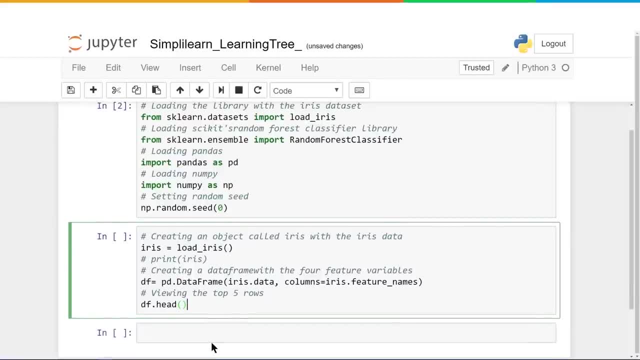 And, if you remember, that's pandas as pd. So that's our pandas And panda data frame. And then we're looking at iris data and columns equals iris feature names, And we're gonna do the df head And let's run this so you can understand. 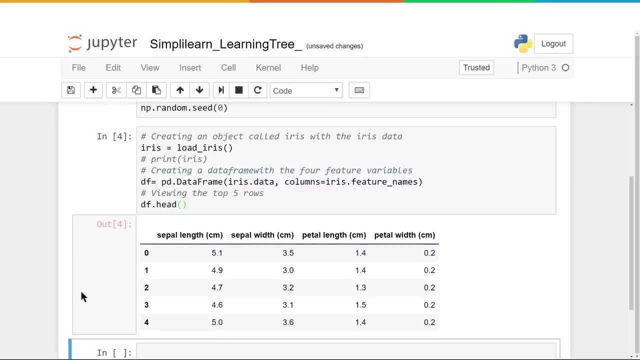 what's going on here? The first thing you wanna notice is that our df has created what looks like an Excel spreadsheet And in this Excel spreadsheet we have set the columns. So up on the top you can see the four different columns. 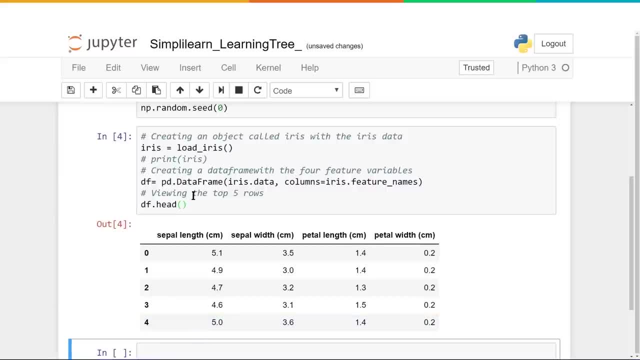 And then we have the data- irisdata- down below. It's a little confusing without knowing where this data is coming from. So let's look at the bigger picture And I'm gonna go print. I'm just gonna change this for a moment. 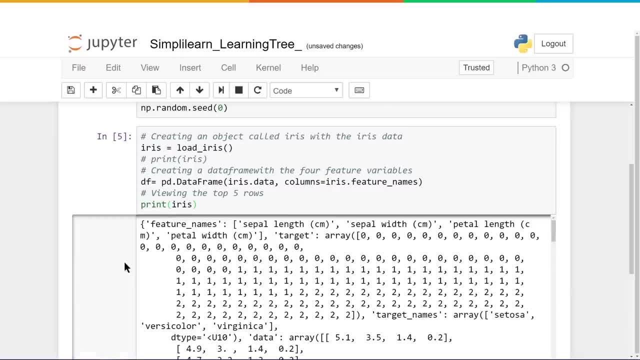 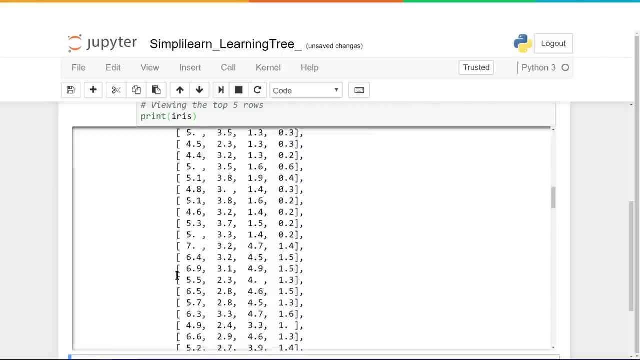 And we're gonna print all of iris and see what that looks like. So when I print all of iris, I get this long list of information And you can scroll through here and see all the different titles on there. What's important to notice is that, first off, 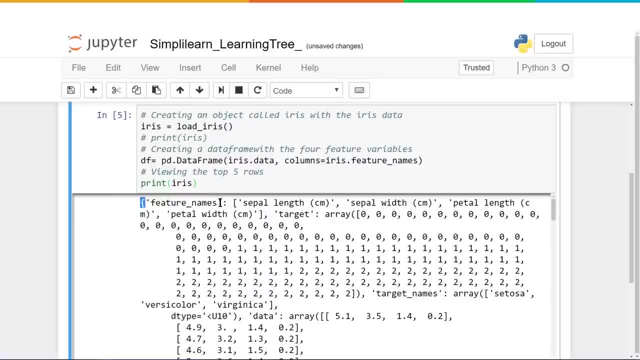 there's a brackets at the beginning. So this is a Python dictionary And in a Python dictionary you'll have a key or a label And this label pulls up whatever information comes after it. So feature names which we actually used over here. 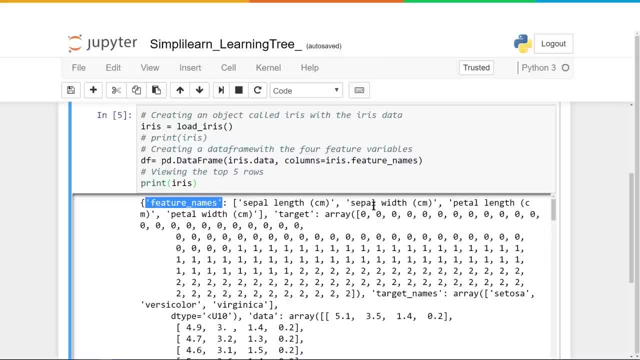 under columns is equal to an array of sepal length, sepal width, petal length, petal width. These are the different names they have for the four different columns And if you scroll down far enough you'll also see data down here. 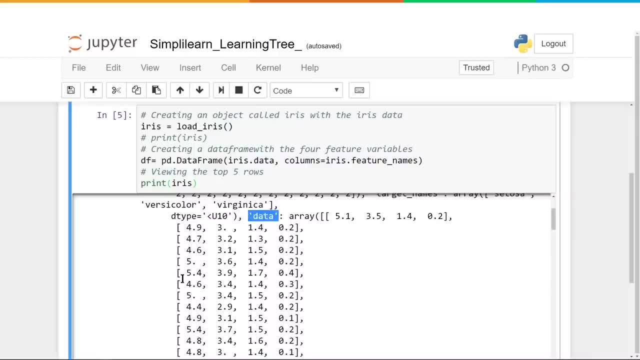 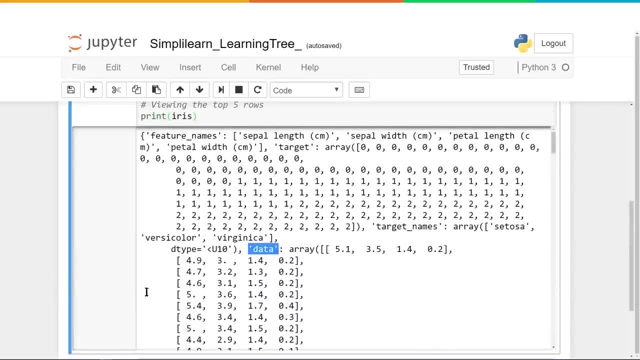 Oh goodness, it came up right towards the top And data is equal to the different data we're looking at Now. there's a lot of other things in here, like target- We're gonna be pulling that up in a minute- And there's also the names, the target names. 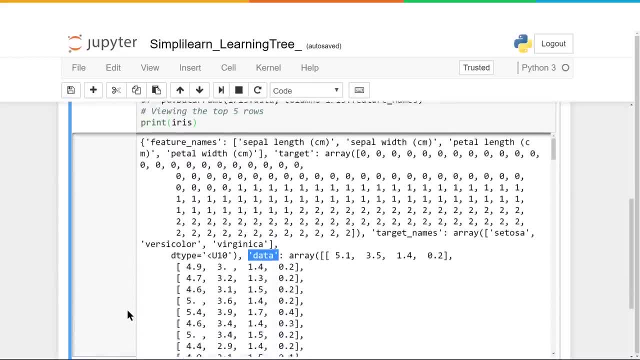 Now there's a lot of other things in here, like target- We're going to be pulling that up in a minute- And there's also the names, the target names, which is further down, And we'll show you that also in a minute. 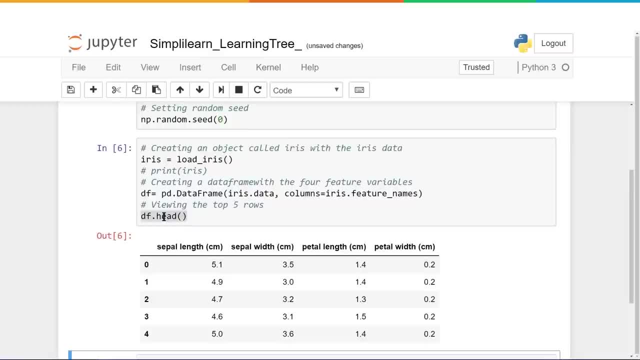 So let's go back to the head, And this is one of the neat features of pandas and panda data frames is, when you do dfhead or the panda data framehead, it'll print the first five lines of the data set in there, along with the headers. 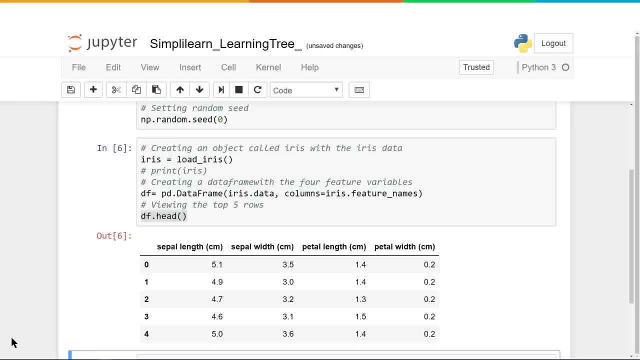 if you have it. In this case we have the column headers set to iris features And in here you'll see that we have 0,, 1,, 2,, 3, 4.. In Python, most arrays always start at zero. 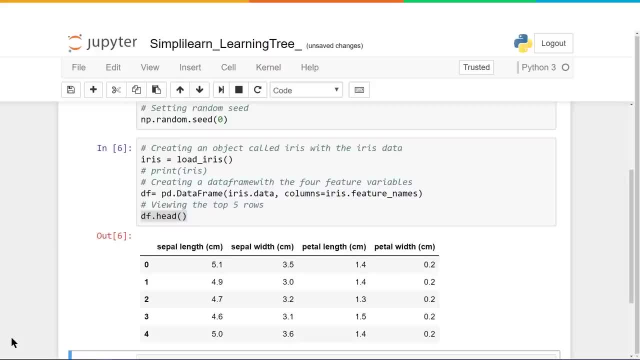 So when you look at the first five, it's going to be 0,, 1,, 2, 3, 4,, not 1, 2,, 3,, 4, 5.. So now we've got our iris data imported into a data frame. 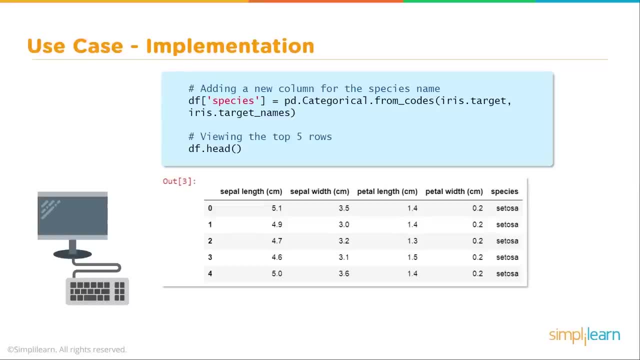 Let's take a look at the next piece of code in here, And so in this section here of the code, we're going to take a look at the target And let's go ahead and get this into our notebook, this piece of code. 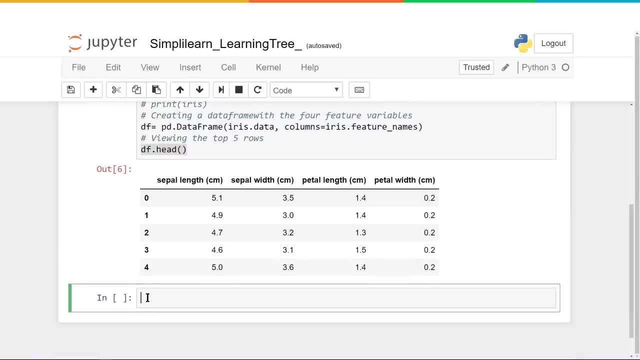 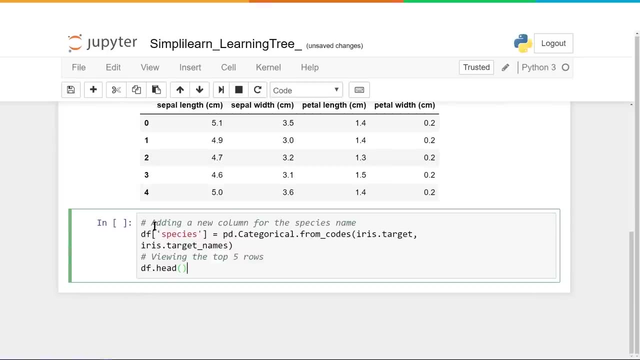 so we can discuss it a little bit more in detail. So here we are in our Jupyter notebook. I'm going to put the code in here And before I run it I want to look at a couple of things going on. So we have 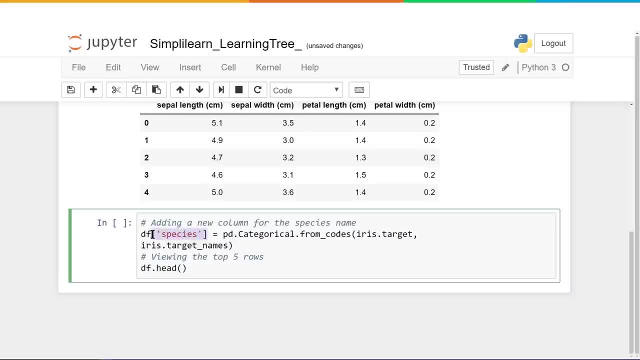 dfspecies. And this is interesting because right here you'll see where I have dfspecies in brackets, which is the key code for creating another column, And here we have iristarget. Now these are both in the pandas setup on here, So in pandas we can do either one. 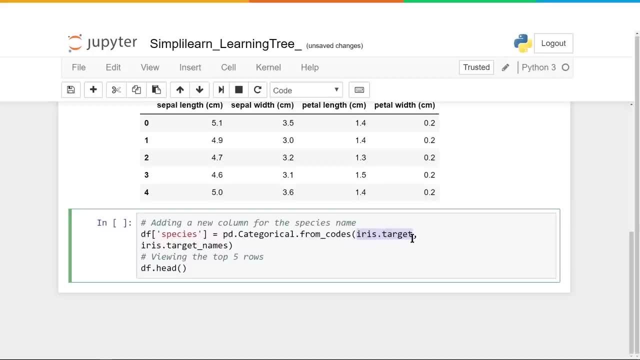 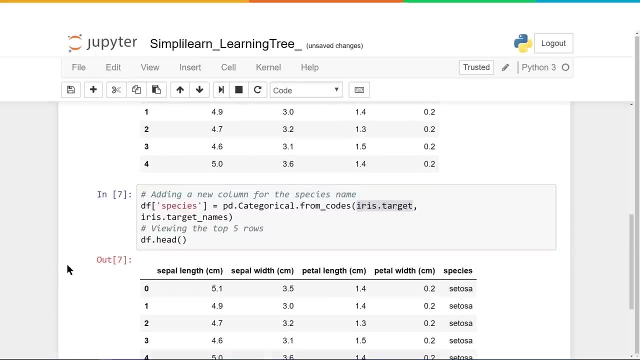 I could have just as easily done iris and then, in brackets, target. depending on what I'm working on, Both are acceptable. Let's go ahead and run this code and see how this changes, And what we've done is we've added the target from the iris data set. 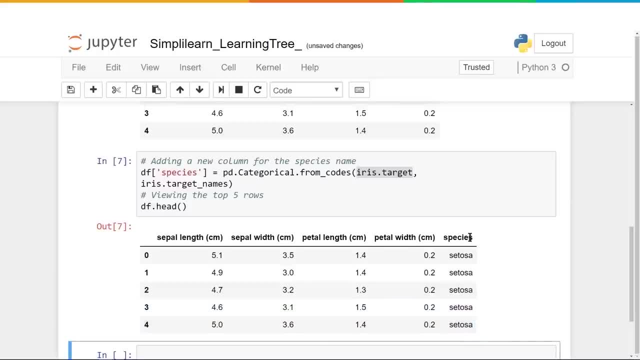 as another column on the end. Now, what species is? this is what we're trying to predict. So we have our data, which tells us the answer for all these different pieces, And then we've added a column with the answer. That way, when we do our final setup, we'll have the ability to program our 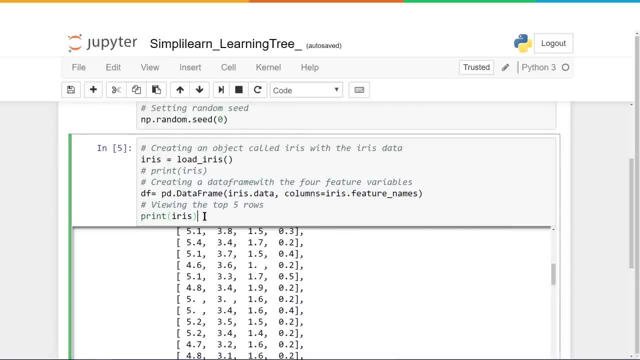 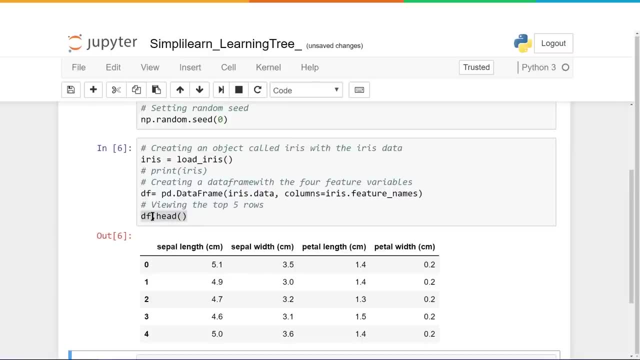 which is further down, And we'll show you that also in a minute. Let's go ahead and set that back to the head, And this is one of the neat features of pandas and panda data frames is when you do dfhead, or the panda data frame, dot head. 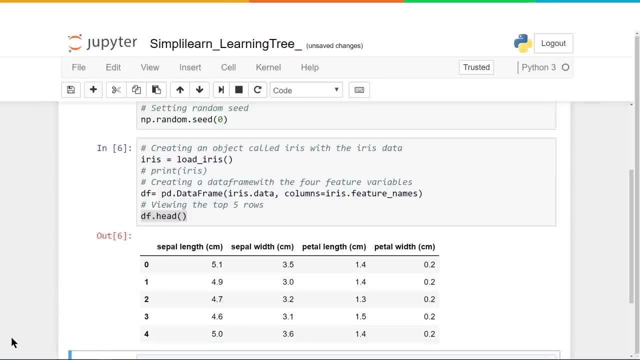 it'll print the first five lines of the data set in there, along with the headers, if you have them. In this case we have the column headers set to iris features And in here you'll see that we have 0,, 1,, 2,, 3,, 4.. 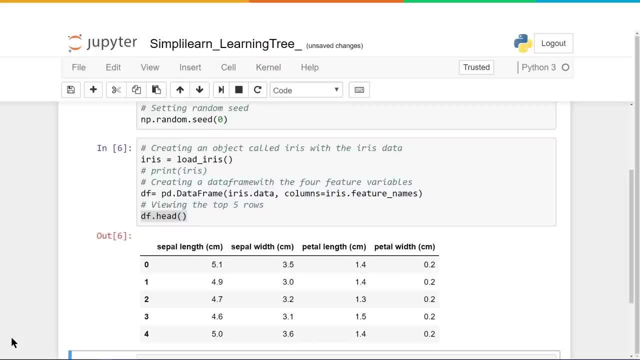 In Python, most arrays always start at zero. So when you look at the first five, it's gonna be 0, 1, 2, 3, 4, not 1, 2, 3, 4, 5.. 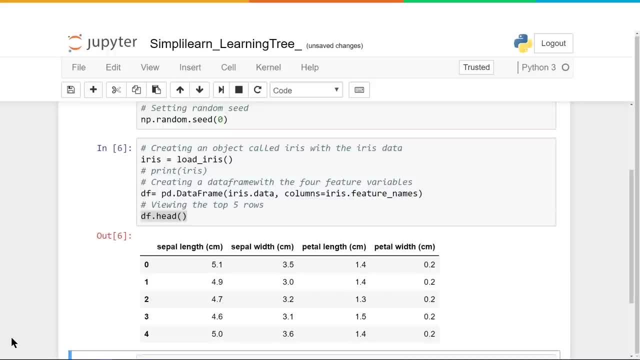 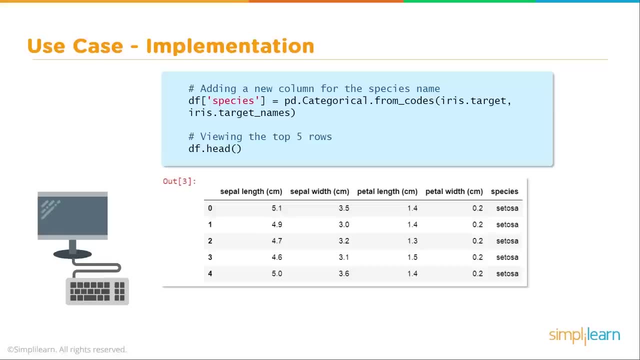 So now we've got our iris data imported into a data frame, Let's take a look at the next piece of code in here. And so in this section here of the code, we're gonna take a look at the target And let's go ahead and get this into our notebook. 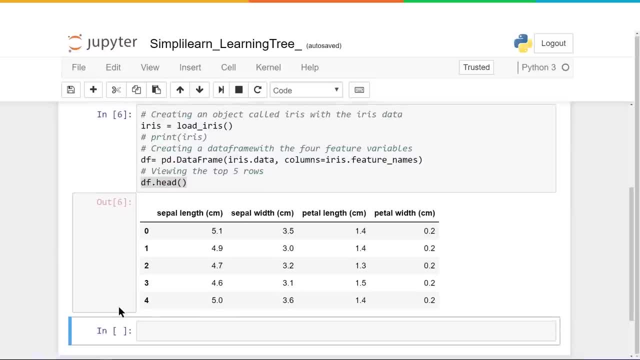 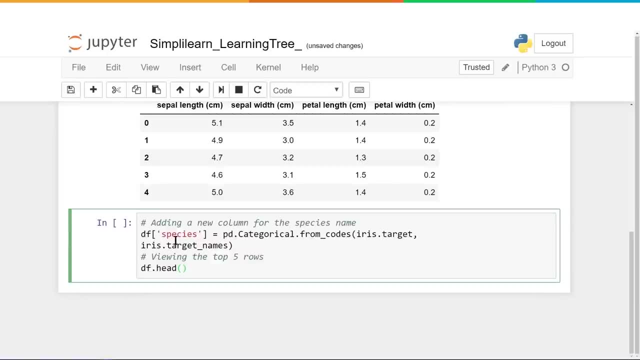 this piece of code so we can discuss it a little bit more in detail. So here we are in our Jupyter notebook. I'm gonna put the code in here And before I run it I wanna look at a couple things going on. 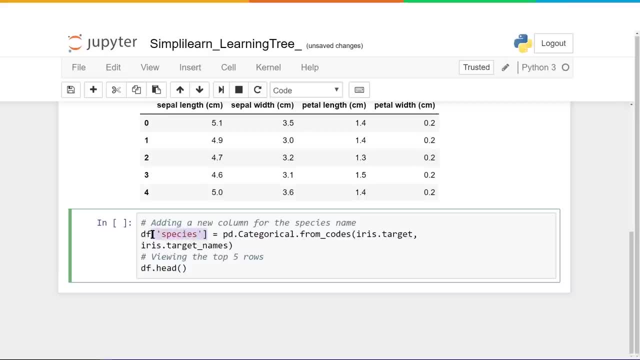 So we have a dfspecies- And this is interesting because right here you'll see where I have dfspecies in brackets, which is the key code for creating another column, And here we have iristarget. Now these are both in the pandas setup on here. 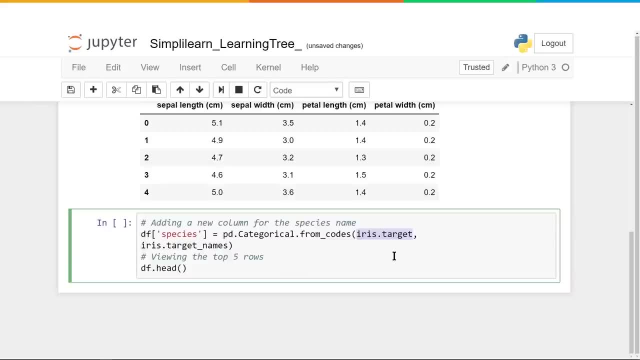 So in pandas we can do either one. I could have just as easily done iris and then in brackets, target, depending on what I'm working on, Both are acceptable. Let's go ahead and run this code and see how this changes. 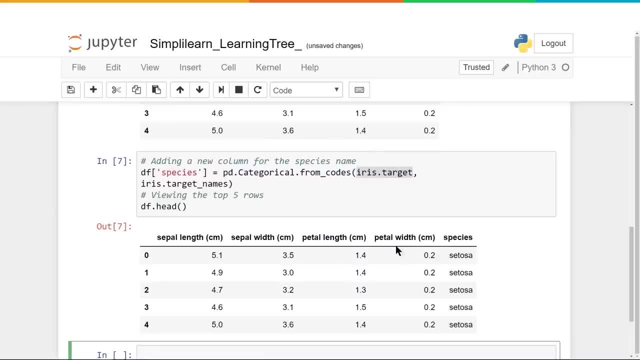 And what we've done is we've added the target from the iris data set as another column on the end. Now, what species is? this is what we're trying to predict. So we have our data, which tells us the answer for all these different pieces. 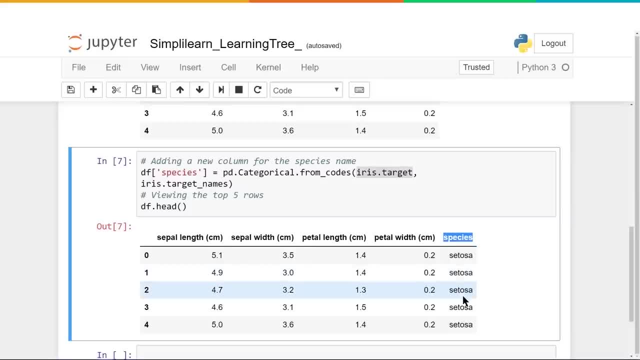 And then we've added a column with the answer. That way, when we do our final setup, we'll have the ability to program our neural network to look for this different data and know what a setosa is, or a vericolor, which we'll see in just a minute. 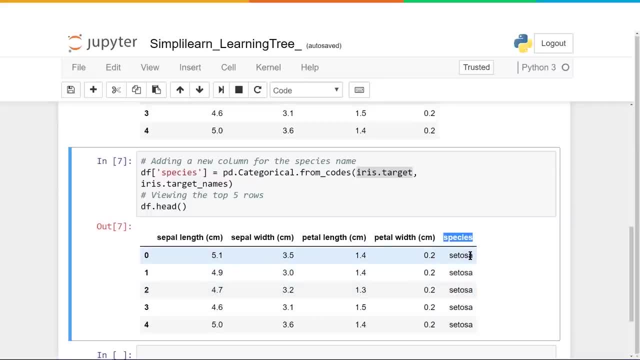 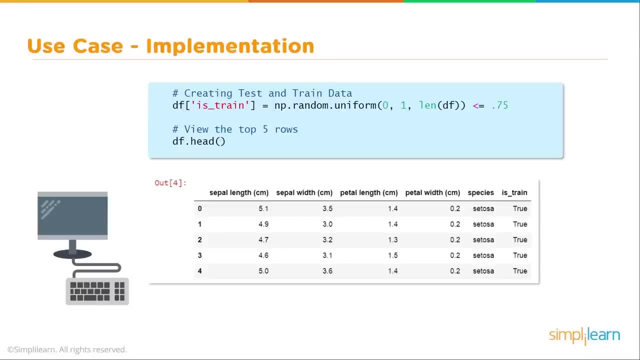 neural network to look for this different data and know what a setosa is, or a vericolor, which we'll see in just a minute- genica. Those are the three that are in there, And now we're going to add one more column. 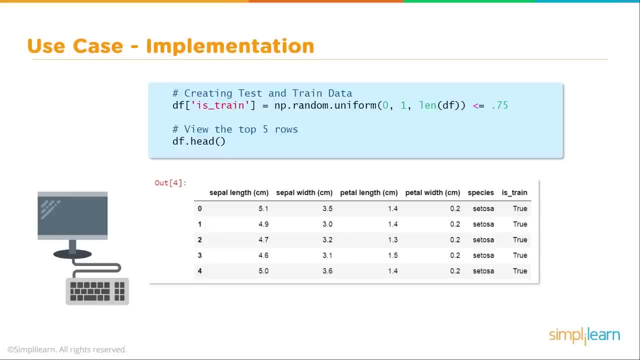 I know we're organizing all this data over and over again. It's kind of fun. There's a lot of ways to organize it. What's nice about putting everything onto one data frame is I can then do a printout and it shows me exactly what I'm looking at. 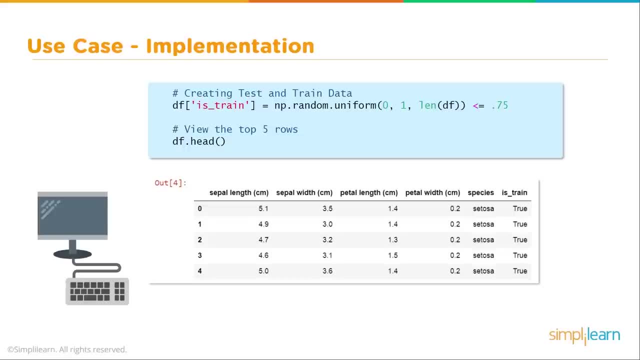 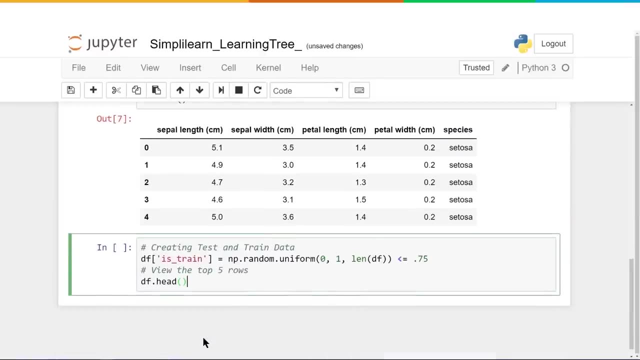 And I'll show you where that's different, where you can alter that and do it slightly differently. But let's go ahead and put this into our script up to that now. And here we go. We're going to put that down here. 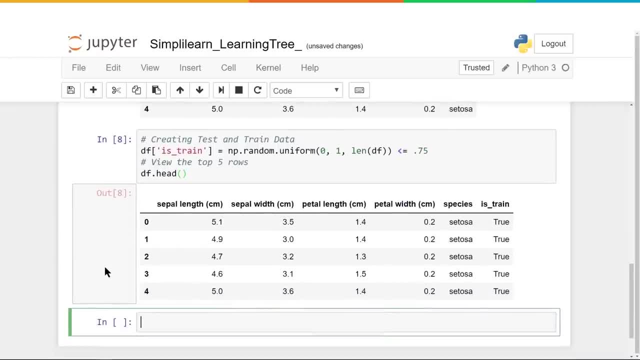 And we're going to run that. And let's talk a little bit about what we're doing Now. we're exploring data And one of the challenges is knowing how good your model is. Did your model work? And to do this, we need to split the data, and we split it into two different parts. 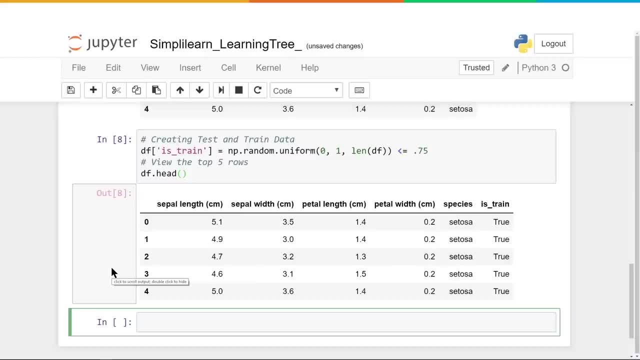 They usually call it the training and the testing, And so in here we're going to go ahead and put that in our database so you can see it clearly, And we've set it DF. Remember you can put brackets. This is creating another column. 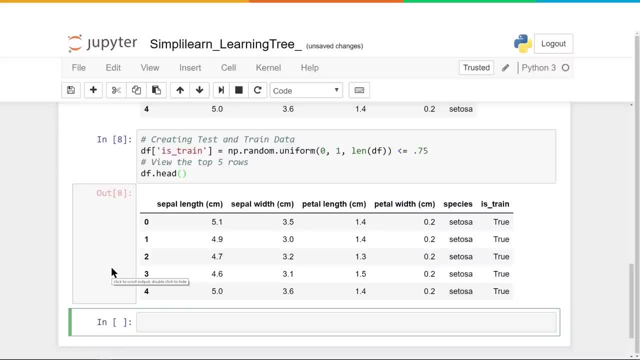 Is train, So we're going to use part of it for training, And this equals NP. remember that stands for numpy dot, random dot, uniform. So we're generating a random number between zero and one And we're going to do it for each of the rows. 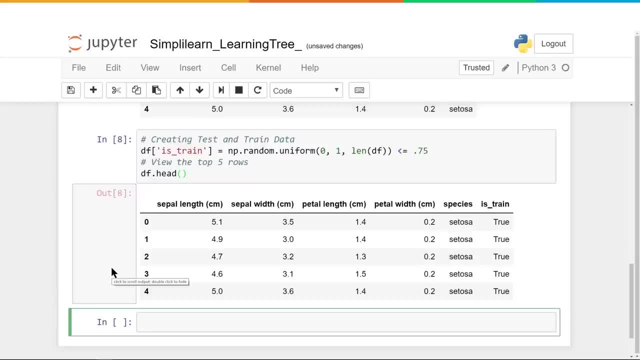 That's where the length DF comes from. So each row gets a generated number, And if it's less than 0.75, it's true, And if it's greater than 0.75, it's false. This means we're going to take 75 percent of the data roughly because there's a 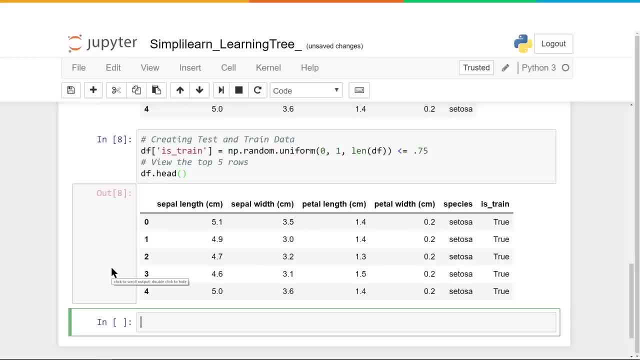 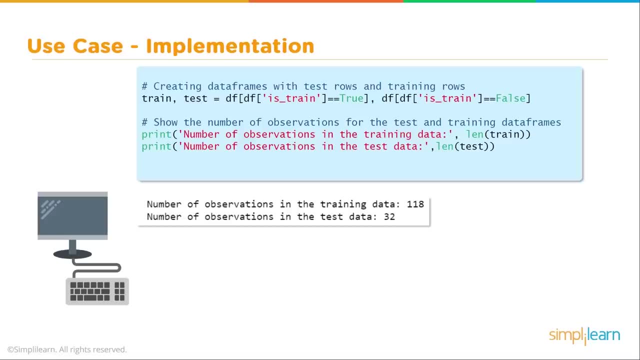 randomness involved and we're going to use that to train it. And then the other 25 percent we're going to hold off to the side and use that to test it later on. So let's flip back over and see what the next step is. 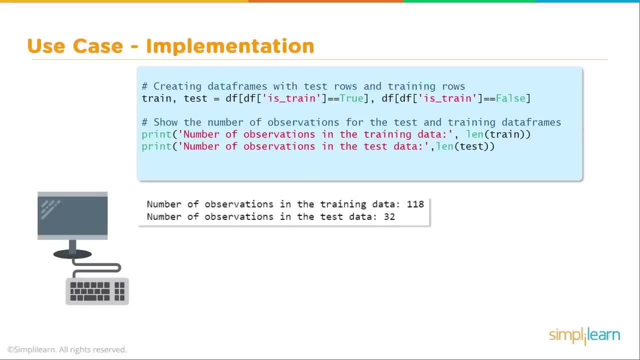 So now that we've labeled our database for which is training and which is testing, let's go ahead and sort that into two different variables- train and test, And let's take this code and let's bring it into our project. Here we go, Let's paste it on down here: 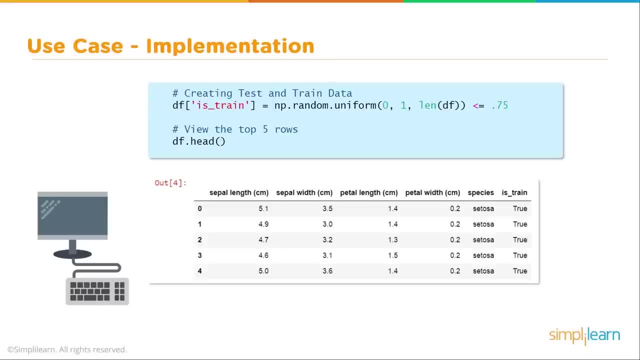 or a virginica. Those are the three that are in there, And now we're gonna add one more column. I know we're organizing all this data over and over again. it's kind of fun. There's a lot of ways to organize it. 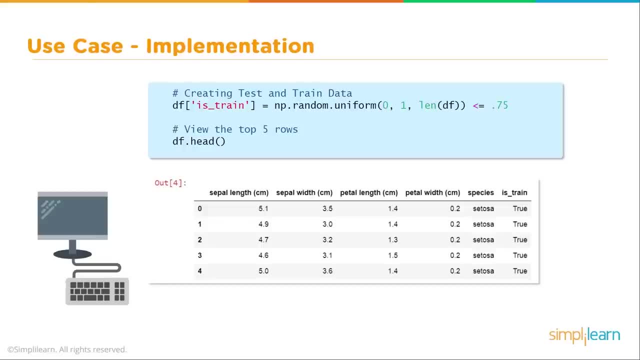 What's nice about putting everything onto one data frame is I can then do a printout and it shows me exactly what I'm looking at, And I'll show you where that's different, where you can alter that and do it slightly differently. But let's go ahead and put this into our script. up to that now. 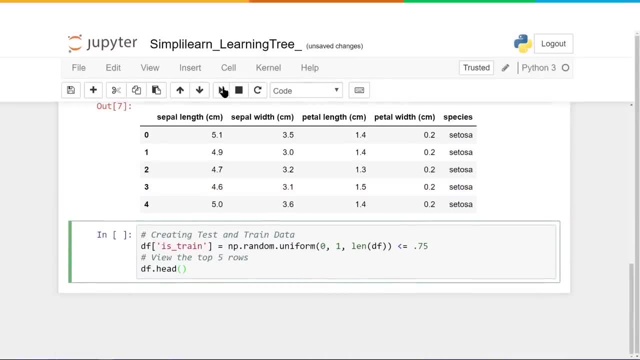 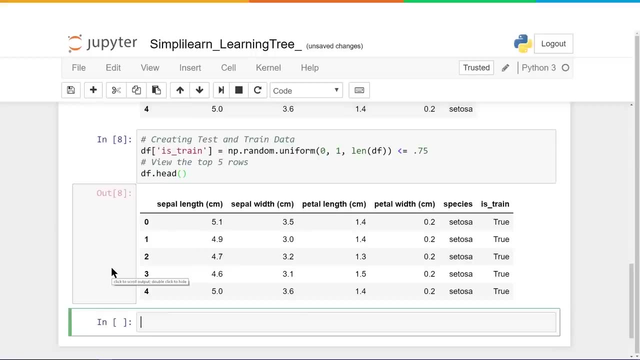 And here we go, we're gonna put that down here And we're gonna run that. And let's talk a little bit about what we're doing Now. we're exploring data And one of the challenges is knowing how good your model is. 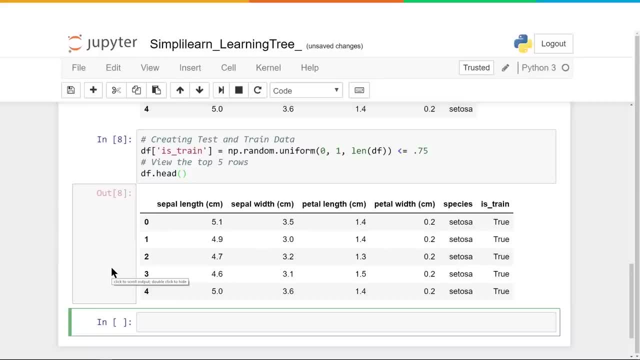 Did your model work, And to do this we need to split the data, And we split it into two different parts. They usually call it the training and the testing, And so in here we're gonna go ahead and put that in our database so you can see it clearly. 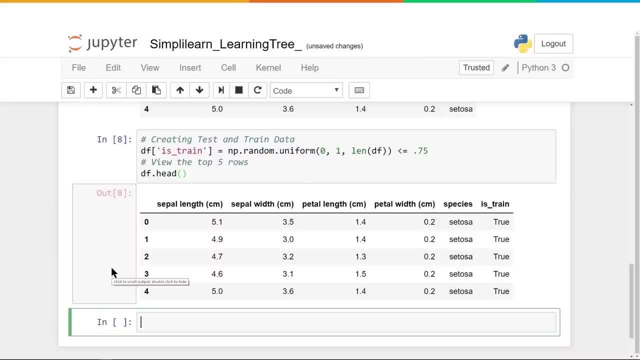 And we've set it df and remember you can put brackets. This is creating another column Is train, so we're gonna use part of it for training. And this equals np. remember that stands for numpy dot, random dot, uniform. So we're generating a random number between zero and one. 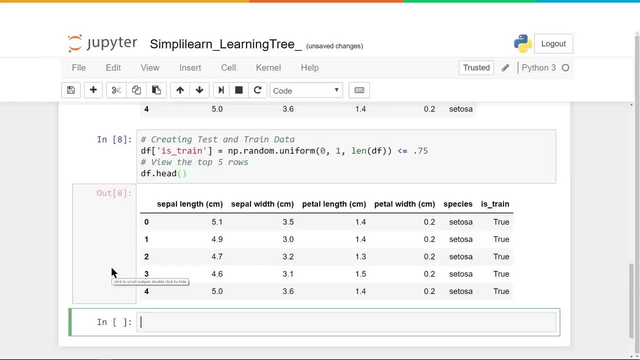 And we're gonna do it for each of the rows. That's where the length df comes from. So each row gets a generated number, And if it's less than .75, it's true, And if it's greater than .75, it's false. 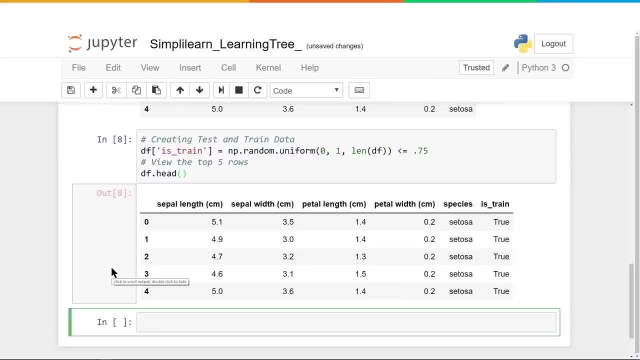 This means we're gonna take 75% of the data roughly, because there's a randomness involved And we're gonna use that to train it, And then the other 25% we're gonna hold off to the side and use that to test it later. 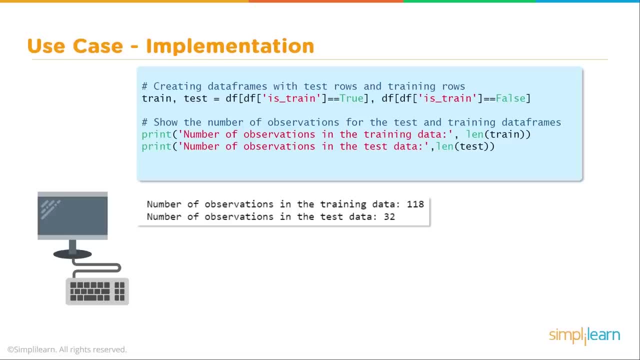 So let's flip back on over and see what the next step is. So, now that we've labeled our database for which is training and which is testing, let's go ahead and sort that in to two different variables, train and test, And let's take this code and let's bring it. 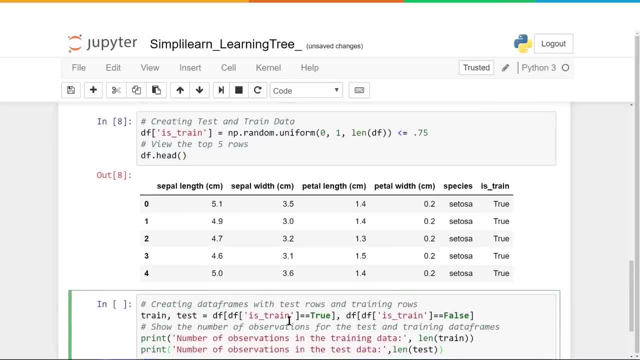 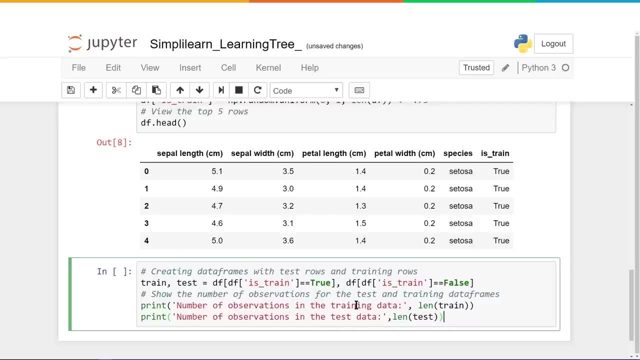 into our project And here we go, let's paste it on down here. And before I run this, let's just take a quick look of what's going on. here is we have up above we created- remember there's our dfhead. 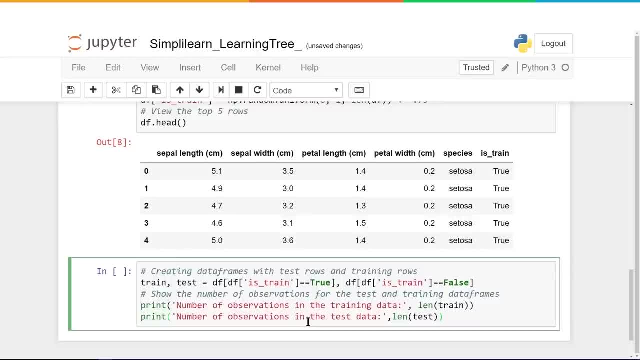 And before I run this, let's just take a quick look at what's going on here Is we have up above, we created- remember there's our defhead- which prints the first five rows, And we've added a column- is train at the end. 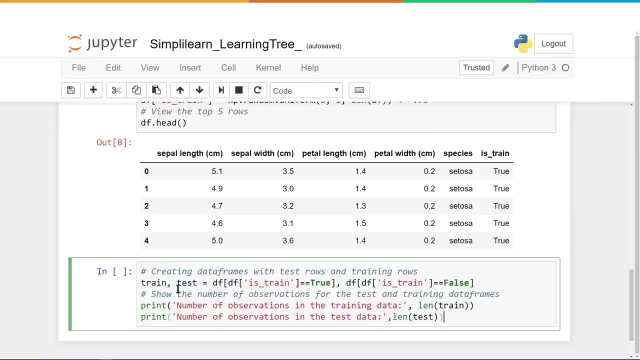 And so we're going to take that, We're going to create two variables, We're going to create two new data frames- One's called train, One's called test- 75 percent in train, 25 percent in test- And then to sort that out. 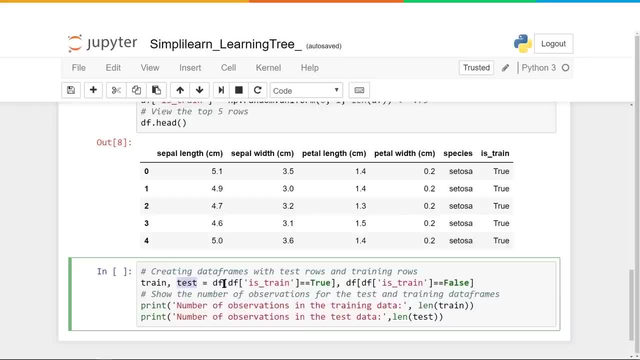 we're going to do that by doing DF, our original data frame, with the iris data in it. And if DF is trained equals true, that's going to go in the train, And if DF is trained equals false, it goes in the test. 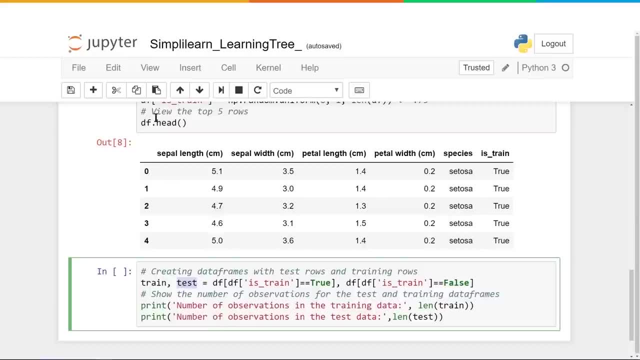 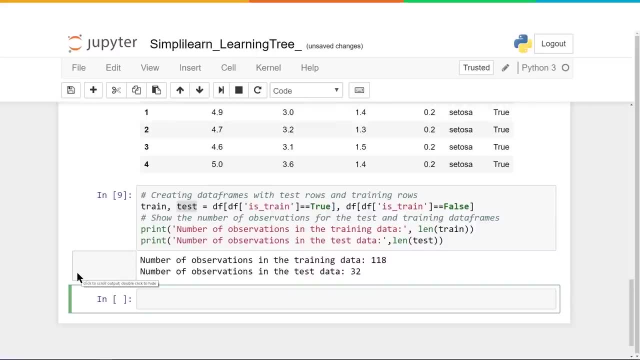 And so when I run this, we're going to print out the number in each one. Let's see what that looks like, And you'll see that it puts 118 in the training module and it puts 32 in the testing module, which lets us know that there was 150 lines of data in here. 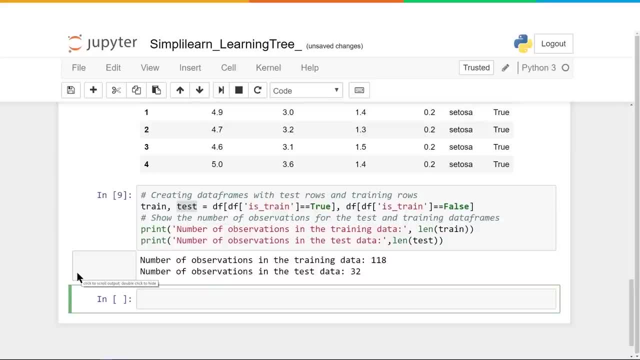 So if you went and looked at the original data, you could see that there's 150 lines and that's roughly 75 percent in one and 25 percent for us to test our model on afterward. So let's jump back to our code and see where this goes. 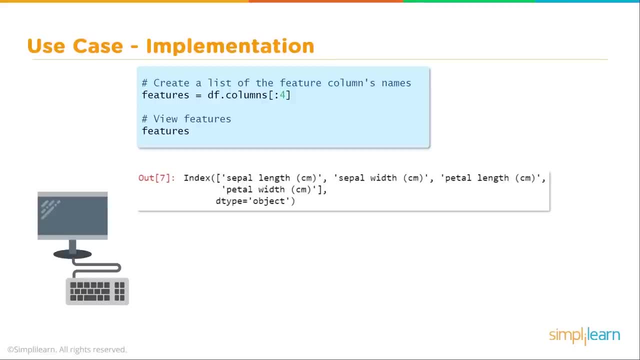 In the next two steps, we want to do one more thing with our data, and that's make it readable to humans. I don't know about you, but I hate looking at zeros and ones, So let's start with the features and let's go ahead and 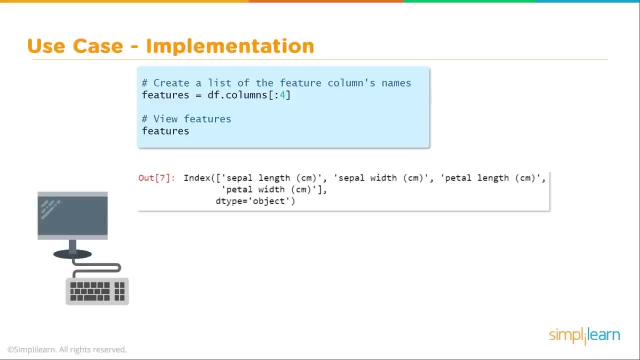 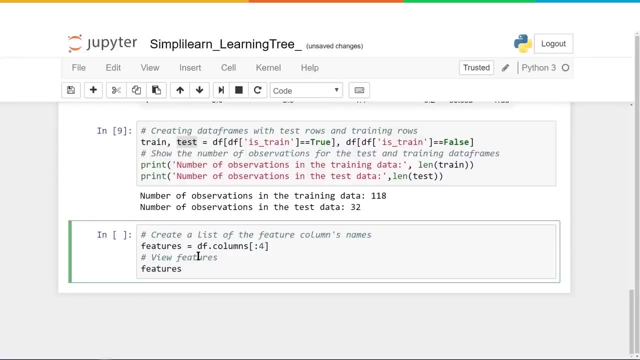 take those and make those readable to humans And let's put that in our code. Let's see, Here we go, Paste it in And you'll see, here we've done a couple very basic things. We know that the columns in our data frame- again, this is a panda thing. 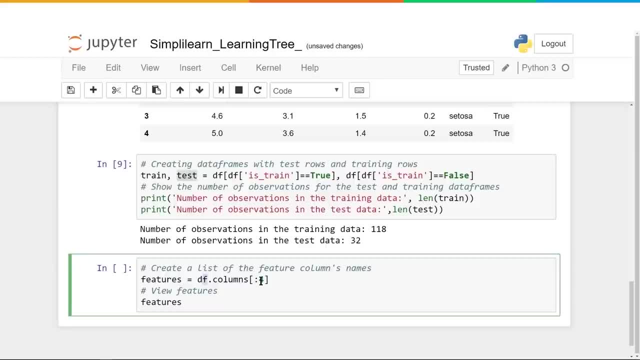 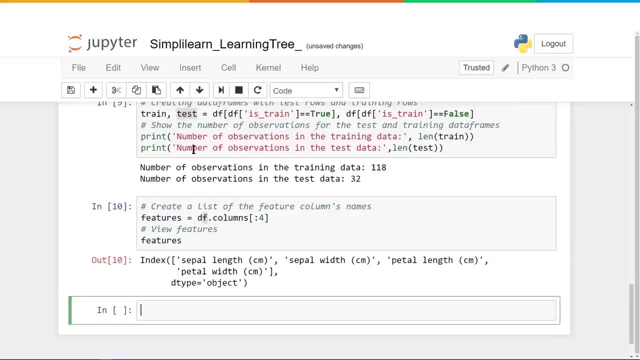 the DF columns, and we know the first four of them- 0,, 1,, 2, 3, that'd be the first four- are going to be the features or the titles of those columns, And so when I run this you'll see down here that it creates. 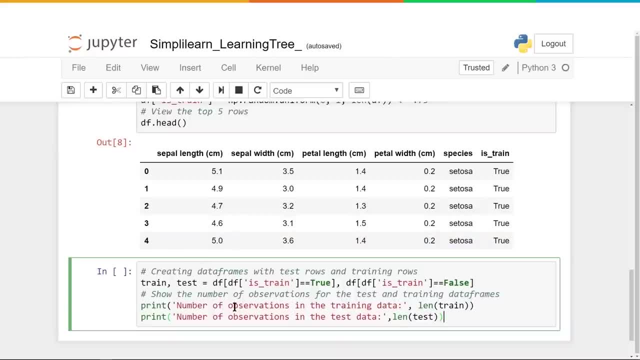 which prints the first five rows, And we've added a column- is train at the end. And so we're gonna take that. we're gonna create two variables, We're gonna create two new data frames. One's called train, one's called test. 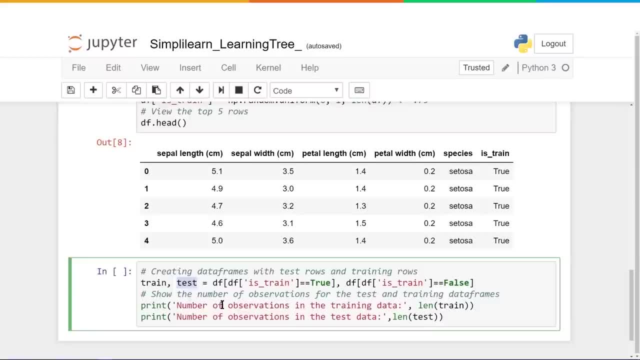 75% in train, 25% in test, And then to sort that out, we're gonna do that by doing df, our main original data frame, with the iris data in it. And if df is train equals, true, that's gonna go in the train. 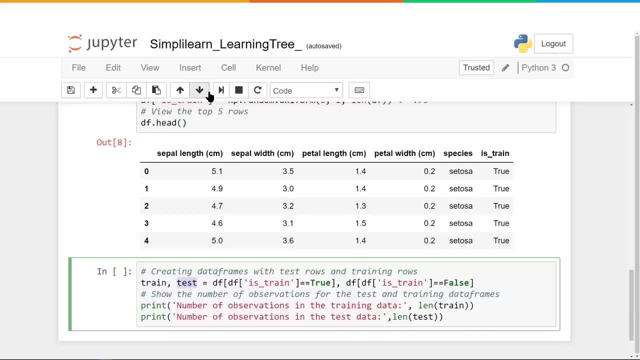 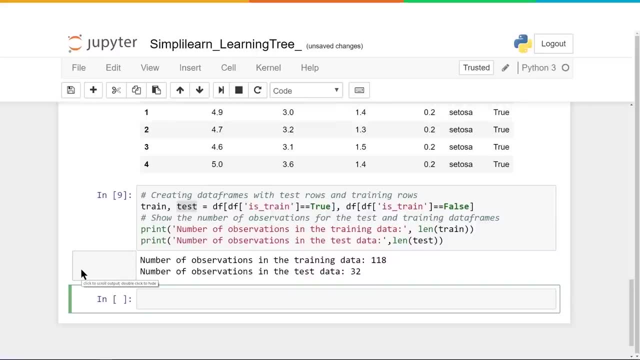 And if df is train equals false, it goes in the test, And so when I run this, we're gonna print out the number in each one. Let's see what that looks like, And you'll see that it puts 118 in the training module. 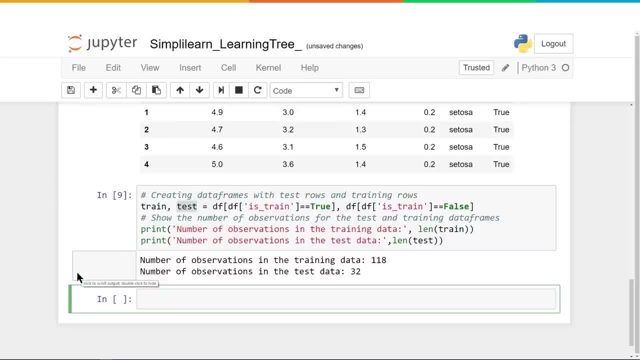 and it puts 32 in the testing module, which lets us know that there was 150 lines of data in here. So if you went and looked at the original data, you could see that there's 150 lines And that's roughly 75% in one. 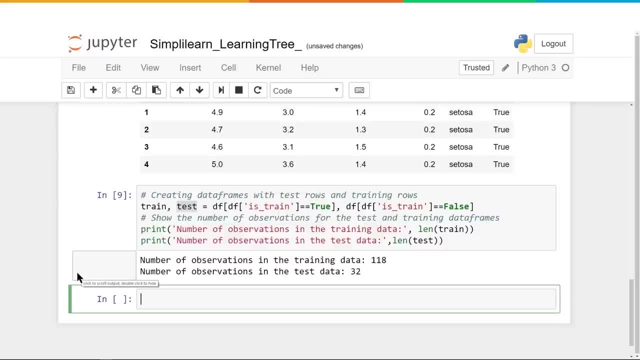 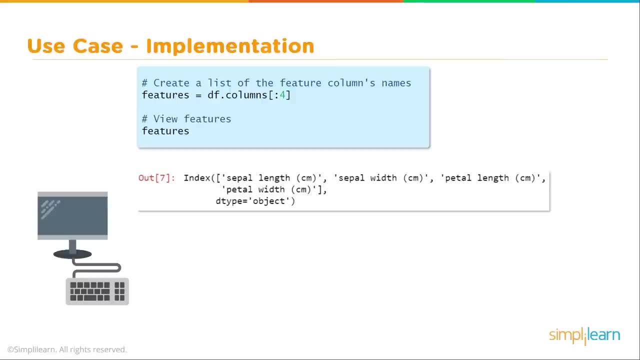 and 25% for us to test our model on afterward. So let's jump back to our code and see where this goes. In the next two steps, we wanna do one more thing with our data, and that's make it readable to humans. 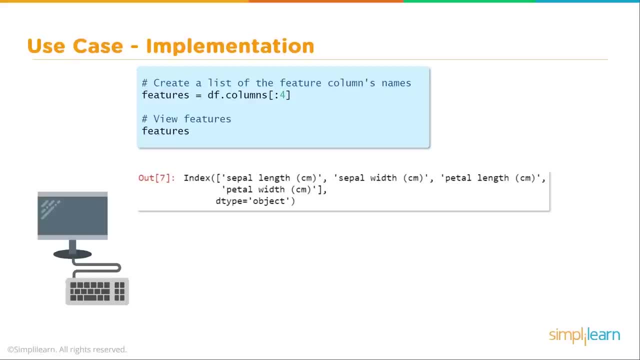 I don't know about you, but I hate looking at zeros and ones. So let's start with the features and let's go ahead and take those and make those readable to humans And let's put that in our code. Let's see, here we go, paste it in. 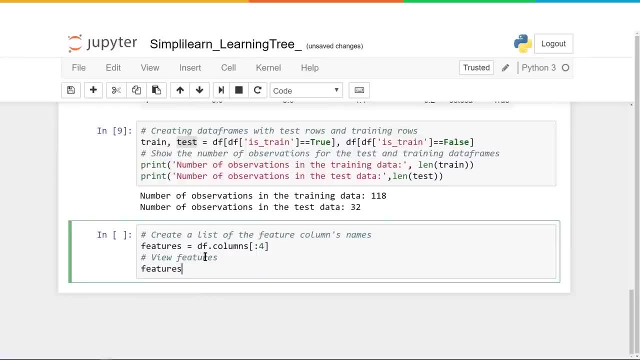 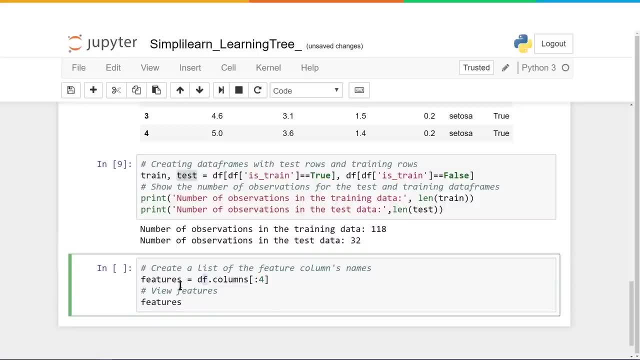 And you'll see here we've done a couple very basic things. We know that the columns in our data frame- again this is a panda thing- the DF columns, and we know the first four of them: zero one, two, three. that'd be the first four. 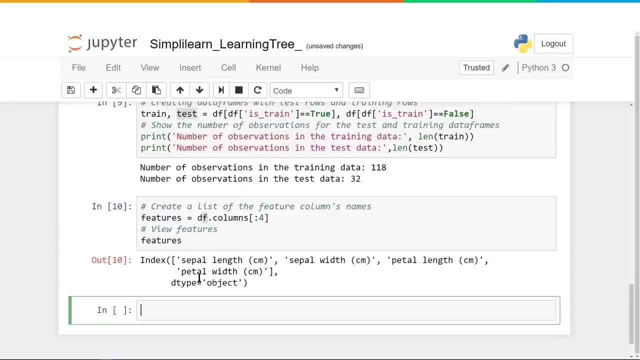 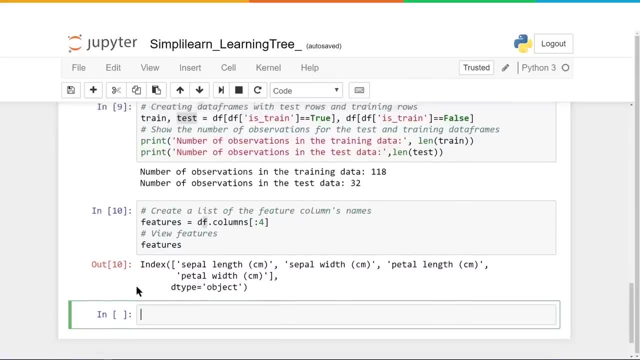 are gonna be the features or the titles of those columns, And so when I run this, you'll see down here that it creates an index: SEPA length, SEPA width, petal length and petal width, And this should be familiar. 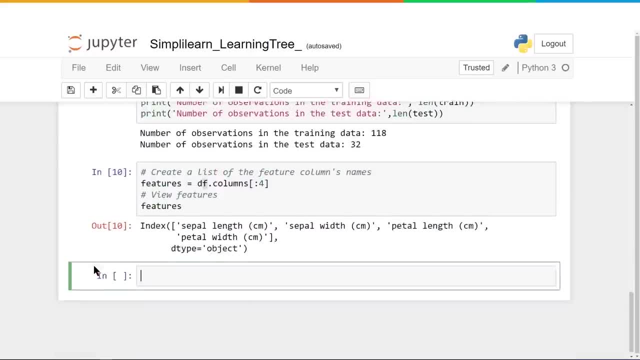 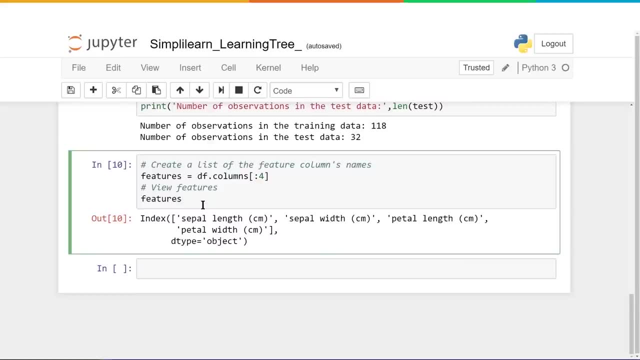 because if you look up here, here's our column titles going across, and here's the first four. One thing I want you to notice here is that when you're in a command line- whether it's Jupyter Notebook, or you're running command line in the terminal window, 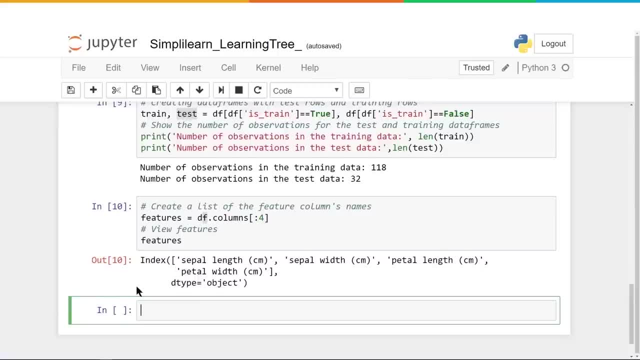 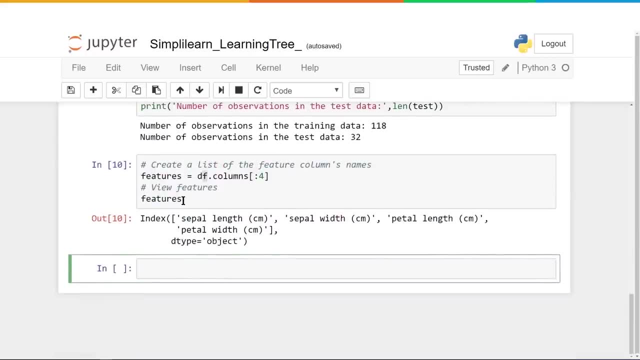 an index: SEPA length, SEPA width, petal length and petal width. And this should be familiar because if you look up here, here's our column titles going across, Here's the first four. One thing I want you to notice here is that when you're in a command line, 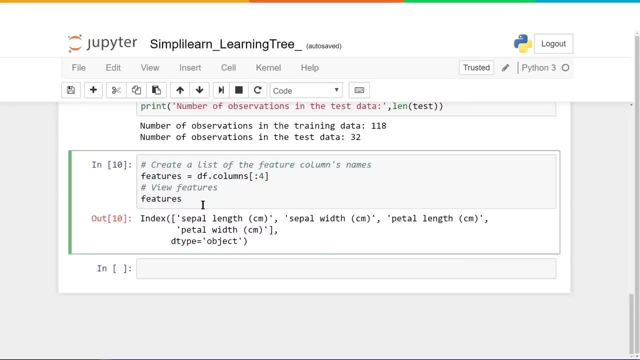 whether it's Jupyter Notebook or you're running command line in the terminal window. if you just put the name of it, it'll print it out. This is the same as doing print features, And the shorthand is you just put features in here. 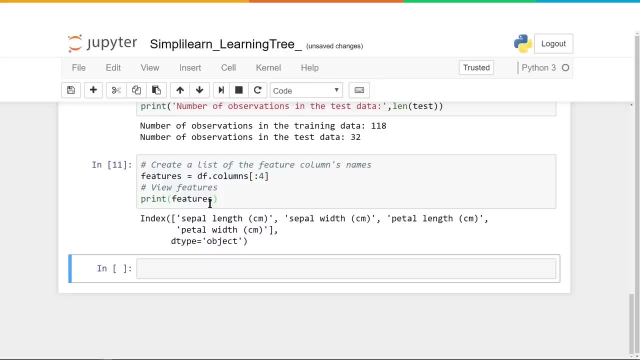 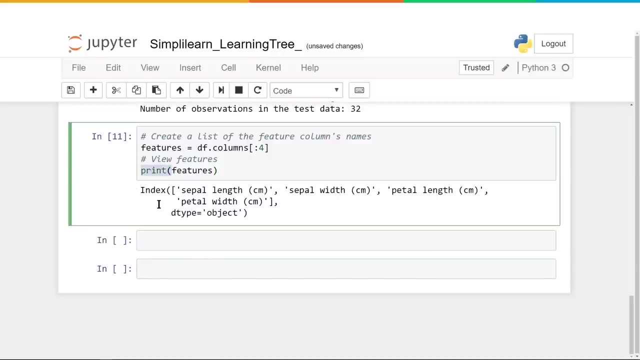 If you're actually writing a code and saving the script and running it by remote, you really need to put the print in there. But for this- and when I run it you'll see- it gives me the same thing. But for this we want to go ahead and we'll. 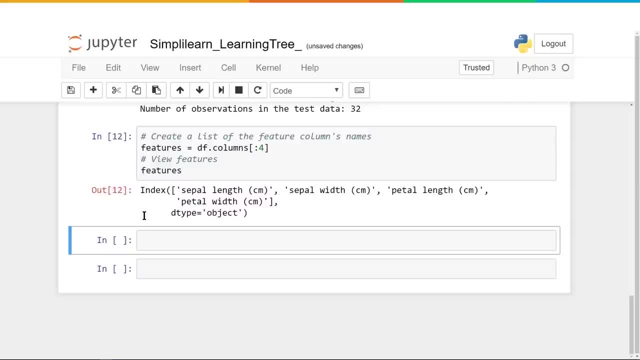 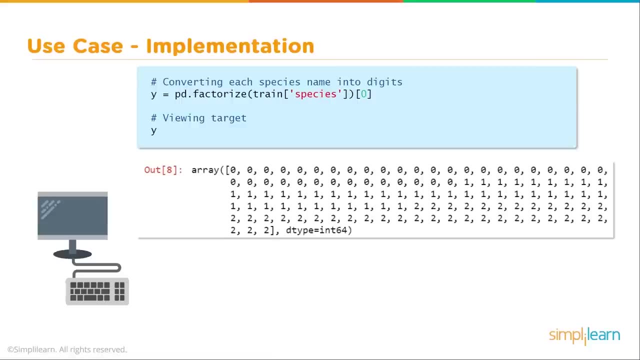 just leave it as features, because it doesn't really matter. And this is one of the fun thing about Jupyter Notebooks is I'm just building the code as we go, and then we need to go ahead and create the labels for the other part. So let's take a look and see what that 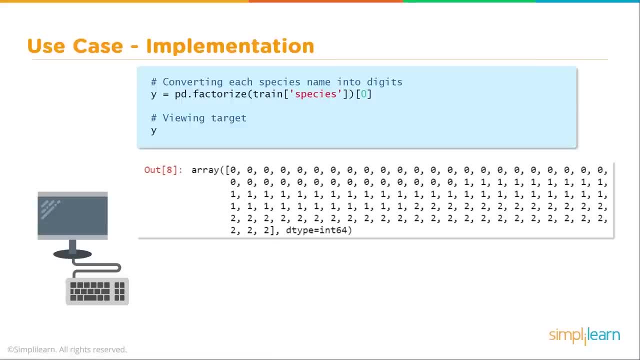 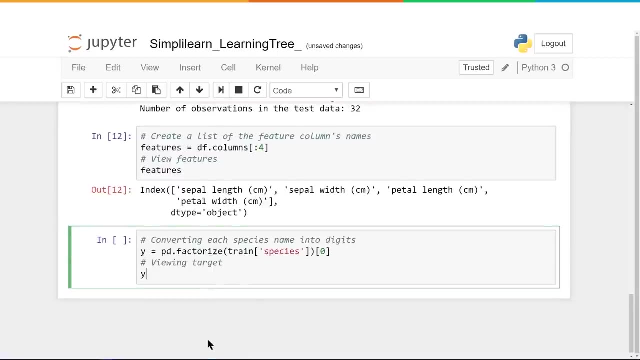 For our final step in prepping our data before we actually start running the training and the testing, is we're going to go ahead and convert the species on here into something the computer understands. So let's put this code into our script and see where that takes us. 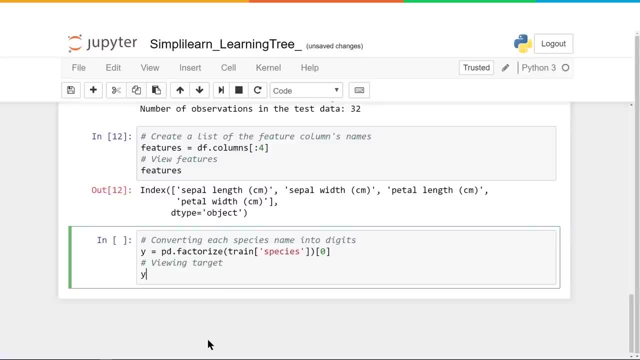 All right, here we go. We set Y equal to PD, dot factorize- train species of zero. So let's break this down just a little bit. We have our pandas right here. PD factorize- What's factorize doing? I'm going to come back to that in just a second. 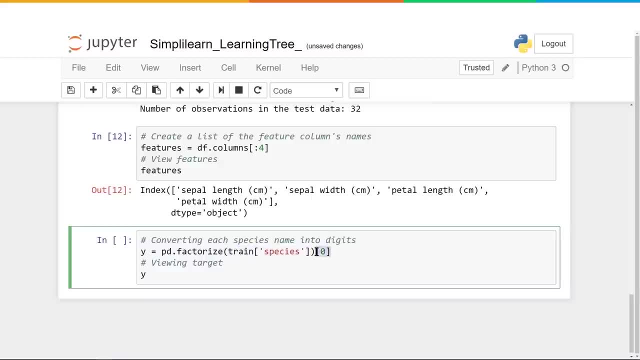 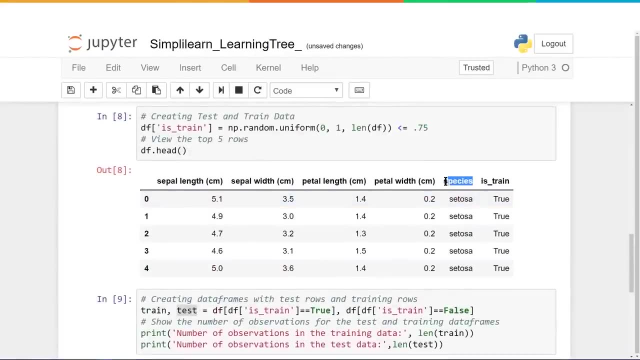 Let's look at what train species is and why. we're looking at the group zero on there And let's go up here And here is our species. Remember this: we created this whole column here for species And then it has setosa, setosa, setosa, setosa. 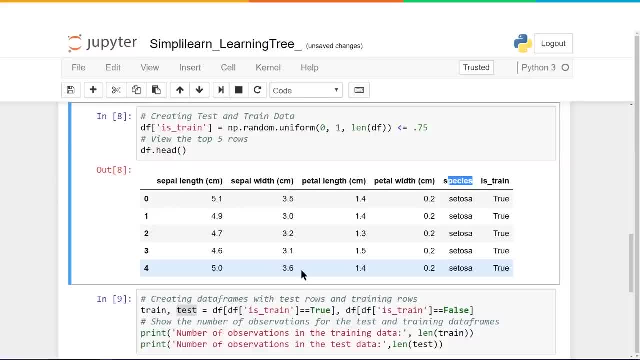 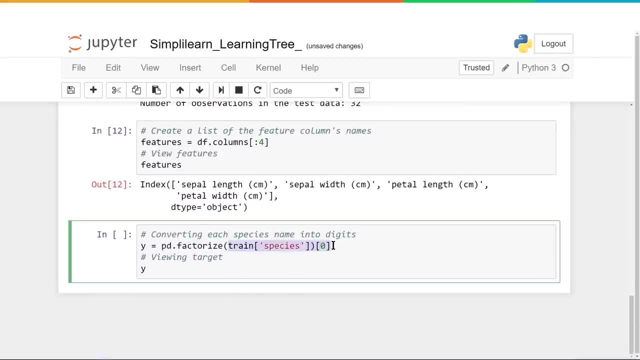 And if you scroll down enough, you'd also see virginica and vericolor. We need to convert that into something. the computer understands: zeros and ones, So the train species of zero, because this is in the format of an array of arrays. 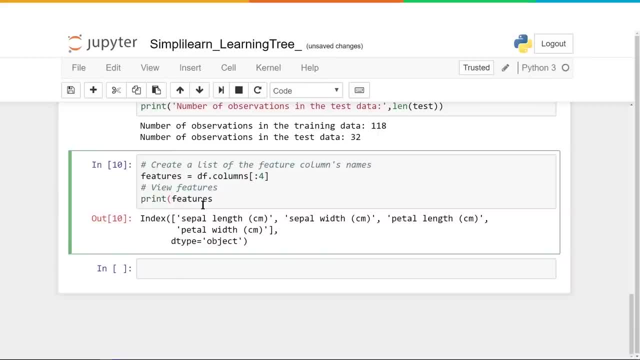 if you just put the name of it, it'll print it out. This is the same as doing print features, And the shorthand is you just put features in here If you're actually writing a code and saving the script and running it by remote. 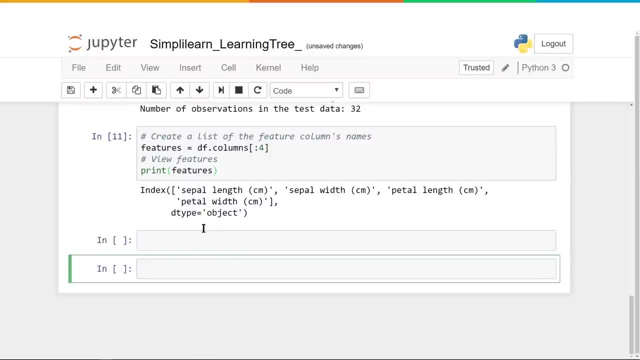 you really need to put the print in there. But for this, when I run it you'll see it gives me the same thing. But for this we wanna go ahead and we'll just leave it as features because it doesn't really matter. 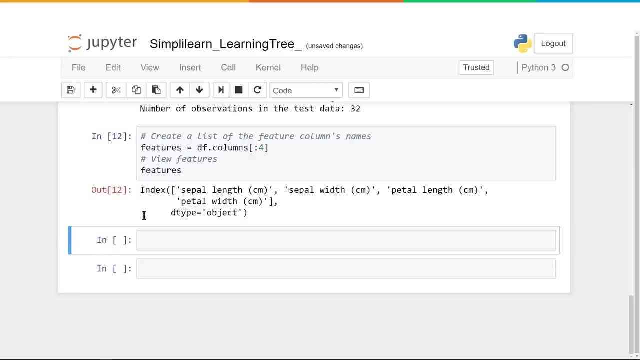 And this is one of the fun thing about Jupyter Notebooks is I'm just building the code as we go, And then we need to go ahead and create the labels for the other part. So let's take a look and see what that. 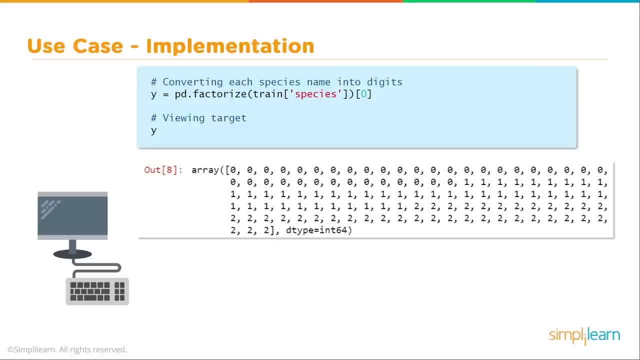 For our final step in prepping our data before we actually start running the training and the testing is we're gonna go ahead and convert the species on here into something the computer understands. So let's put this code into our script and see where that takes us. 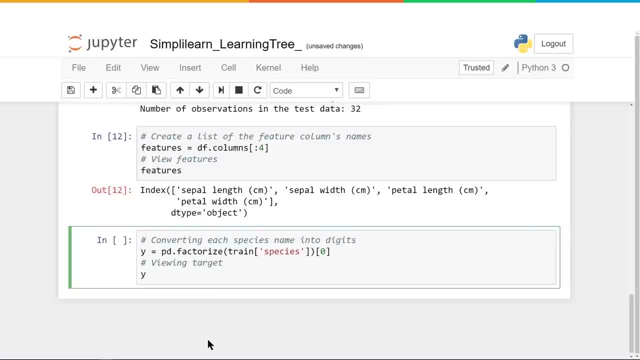 All right, here we go. Set y equal to pdfactorize, train species of zero. So let's break this down just a little bit. We have our pandas right here. pd: factorize- What's factorize doing? I'm gonna come back to that in just a second. 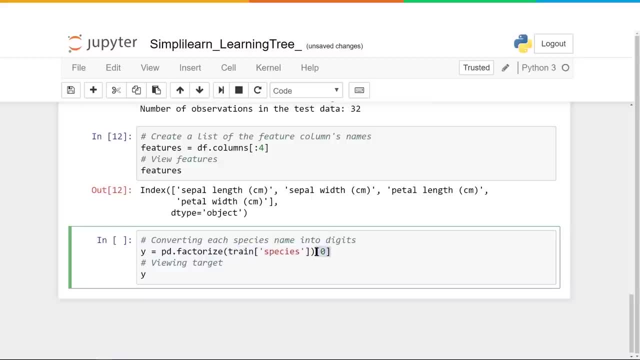 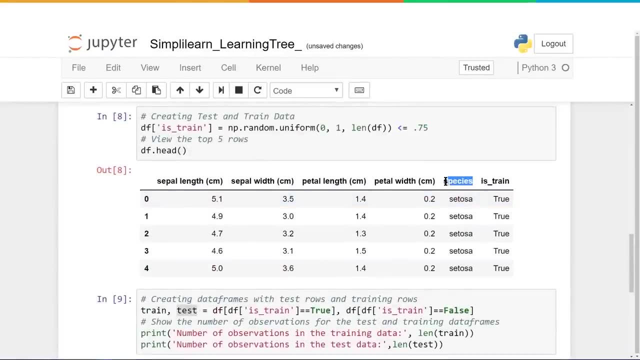 Let's look at what train species is and why. we're looking at the group zero on there And let's go up here and here is our species. Remember this: we created this whole column here for species and then it has setosa, setosa, setosa, setosa. 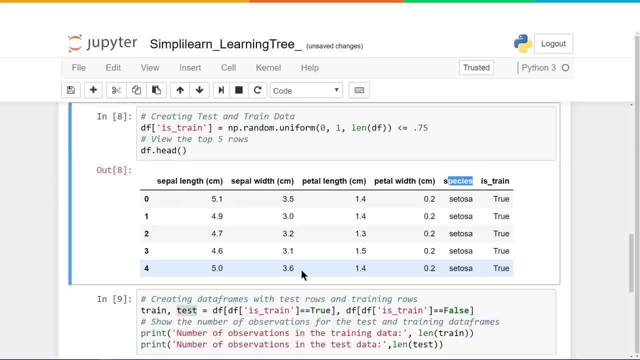 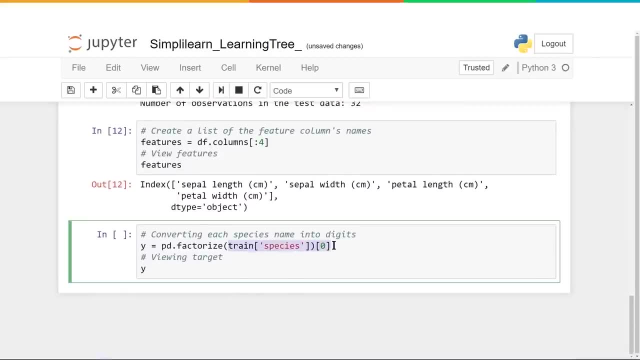 and if you scroll down enough, you'd also see virginica and vericolor. We need to convert that into something. the computer understands: zeros and ones, So the train species of zero, because this is in the format of an array of arrays. 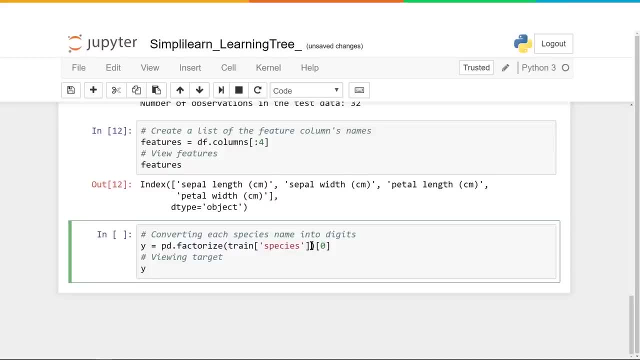 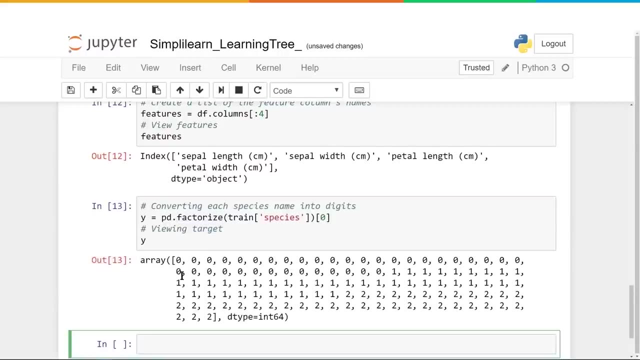 so you have to have the zero on the end, And then species is just that column. Factorize goes in there and looks at the fact that there's only three of them. So when I run this, you'll see that y generates an array. 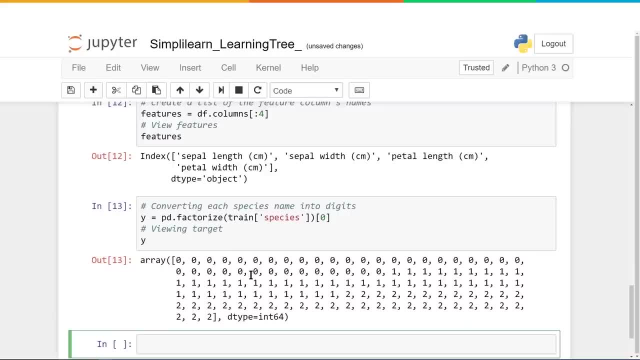 that's equal to. in this case it's the training set and it's zeros, ones and twos representing the three different kinds of flowers we have. So now we have something the computer understands and we have a nice table that we can read and understand. 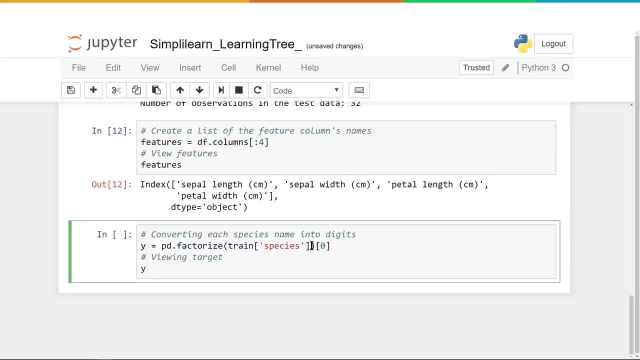 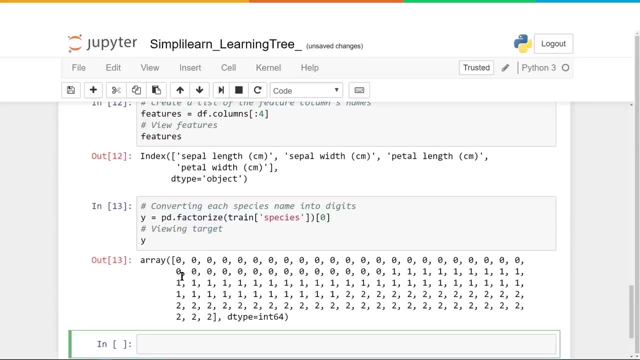 So you have to have the zero on the end and then species is just a column. factorize goes in there and looks at the fact that there's only three of them. So when I run this, you'll see that Y generates an array that's equal to in this: 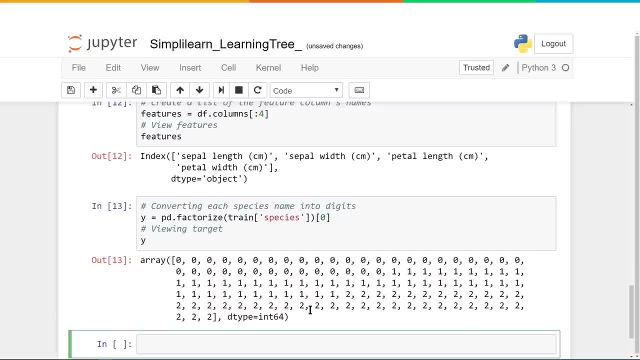 case it's a training set and it's zeros, ones and twos representing the three different kinds of flowers we have. So now we have something the computer understands and we have a nice table that we can read and understand, And now, finally, we get to actually start doing the predicting. 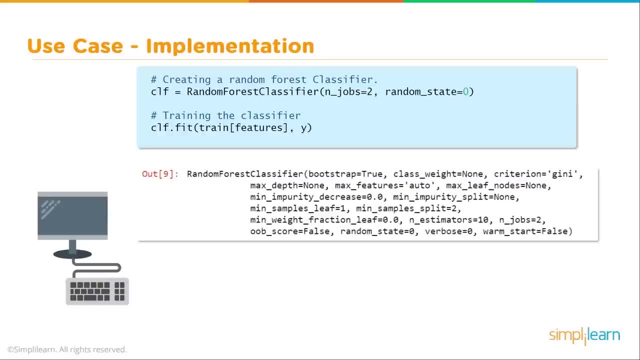 So here we go. We have two lines of code. Oh my goodness, That was a lot of work to get to two lines of code, But there is a lot in these two lines of code, So let's take a look and see what's going on here. 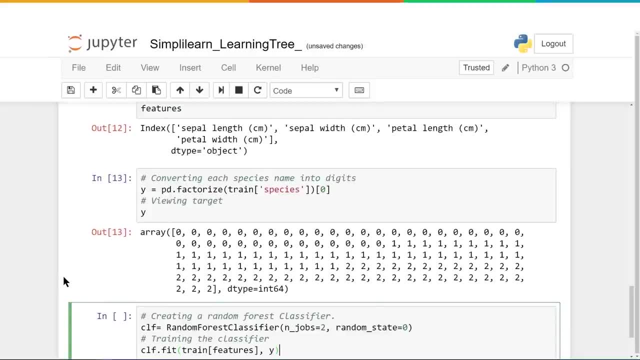 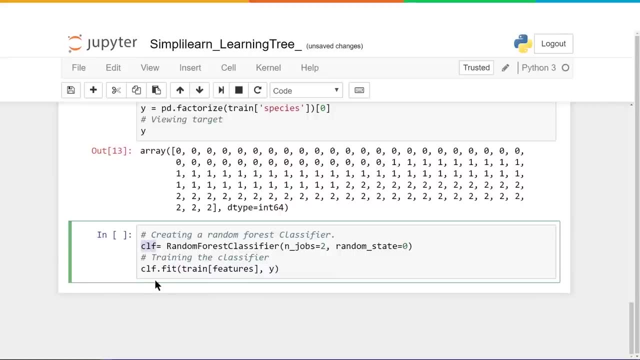 Put this into our full script that we're running, Let's paste this in here and let's take a look and see what this is We have. we're creating a variable, CLF, and we're going to set this equal to the random forest classifier, and we're passing two variables in here. 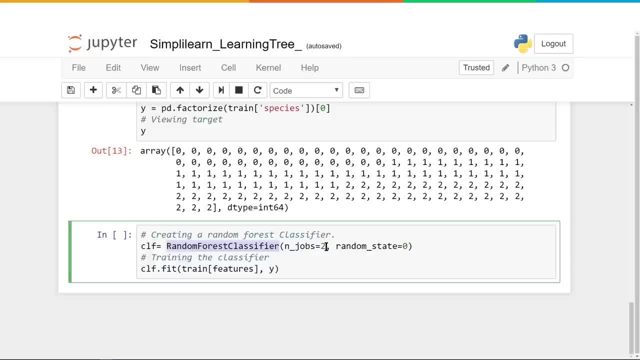 And there's a lot of variables you can play with. As far as these two are concerned, they're very standard in jobs. All that does is to prioritize it, Not something to really worry about. Usually, when you're doing this on your own computer, you do in: jobs equals two. 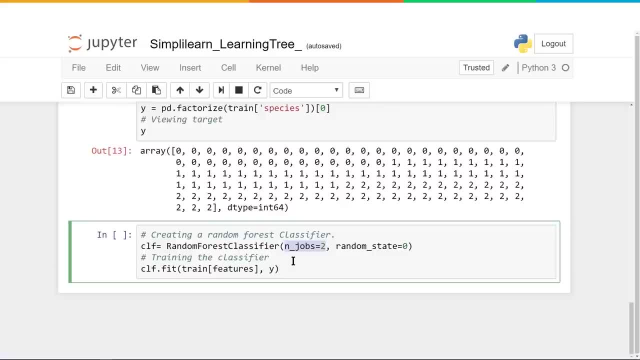 If you're working in a larger or big data and you need to prioritize it differently. this is what that number does, is it changes your priorities and how it's going to run across the system and things like that, And then the random state is just how it starts. 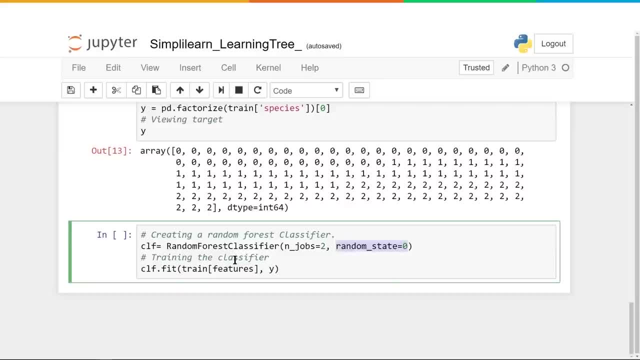 Zero is fine for here, But let's go ahead and run this. We also have CLF dot fit. train features comma why- And before we run it, let's talk about this a little bit more- CLF dot fit- So we're fitting, we're training it. 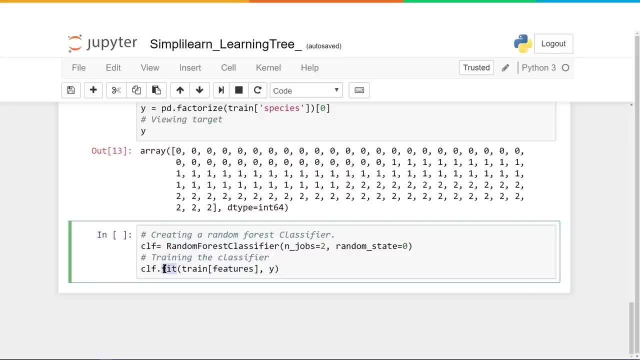 We are actually creating our random forest classifier right here. This is a code that does everything, And we're going to take our training set- Remember, we kept our test off to the side- and we're going to take our training set with the features, and then we're going to go ahead and put that in. 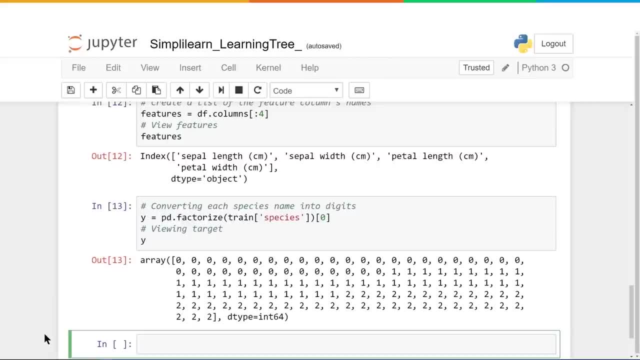 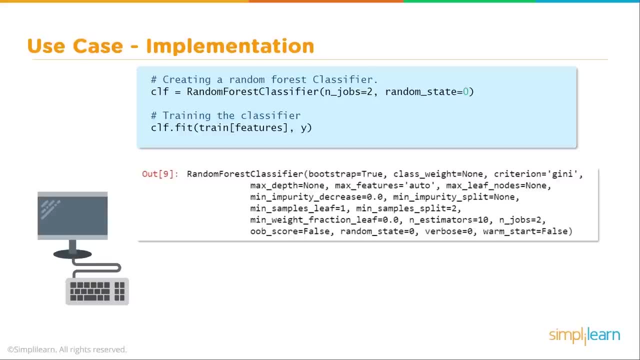 And now, finally, we get to actually start doing the predicting. So here we go. we have two lines of code. Oh, my goodness, that was a lot of work to get to two lines of code. So let's take a look and see what's going on here. 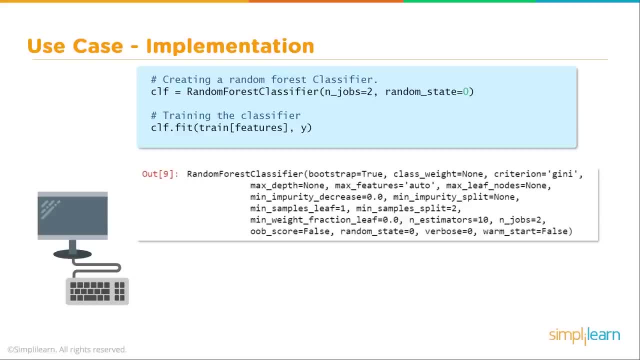 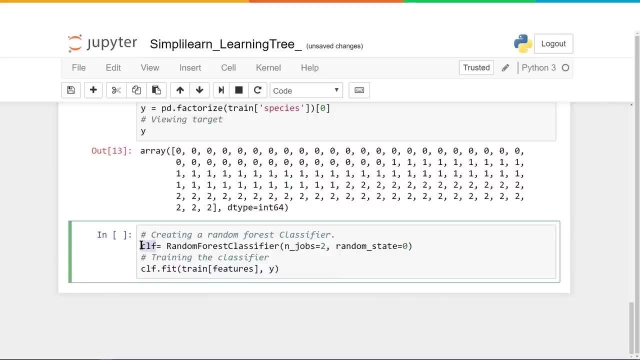 Put this into our full script that we're running And let's paste this in here And let's take a look and see what this is. We're creating a variable clf, and we're gonna set this equal to the random forest classifier. 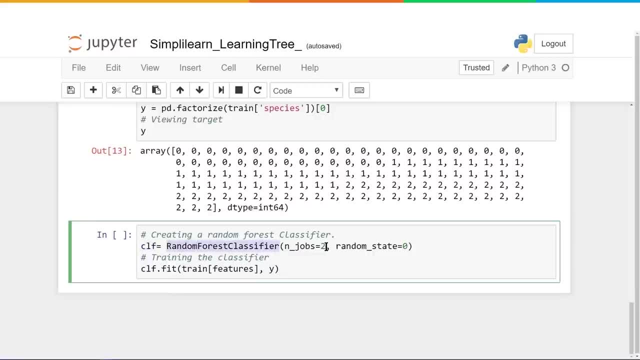 And we're passing two variables in here and there's a lot of variables you can play with As far as these two are concerned. they're very standard In jobs. all that does is to prioritize it, Not something to really worry about. 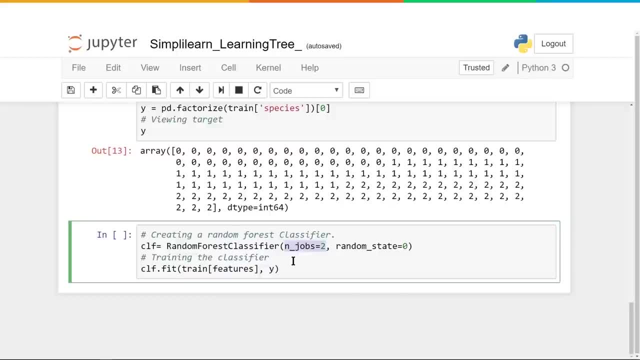 but it's something you can do. Usually, when you're doing this on your own computer, you do in jobs equals two. If you're working in a larger or big data and you need to prioritize it differently, this is what that number does. 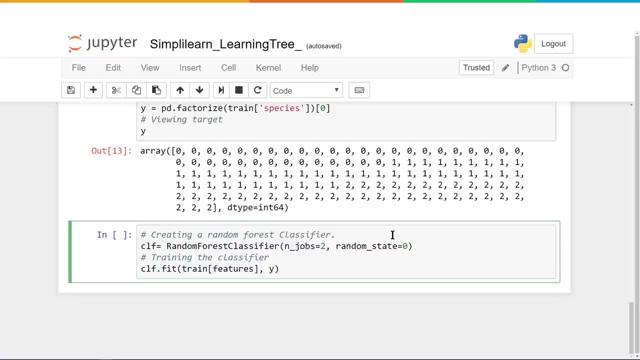 is it changes your priorities and how it's gonna run across the system and things like that, And then the random state is just how it starts. Zero's fine for here, But let's go ahead and run this. We also have clffit train features, comma y. 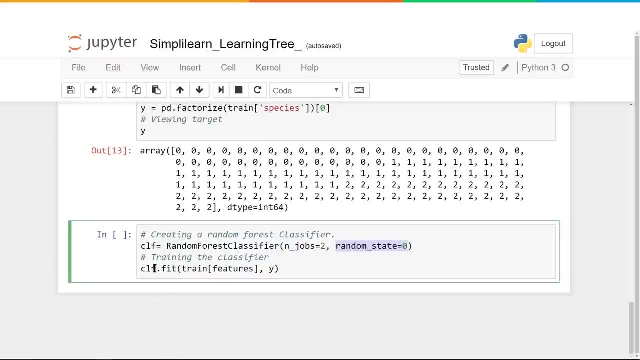 And before we run it, let's talk about this a little bit more clffit. So we're fitting, we're training it. We are actually creating our random forest classifier right here. This is the code that does everything, And we're gonna take our training set. 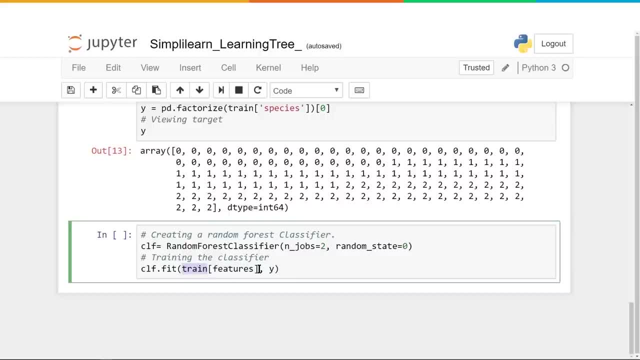 Remember, we kept our test off to the side And we're gonna take our training set with the features and then we're gonna go ahead and put that in. And here's our target: the y. So the y is zero one and two that we just created. 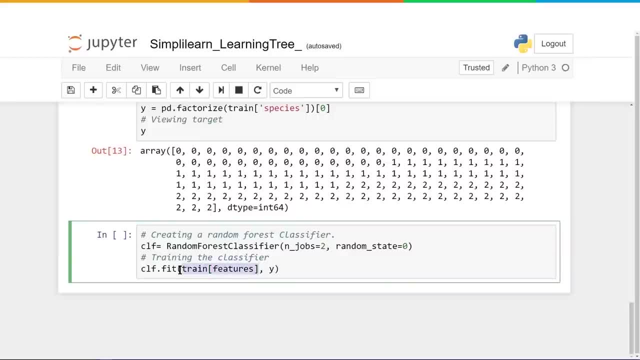 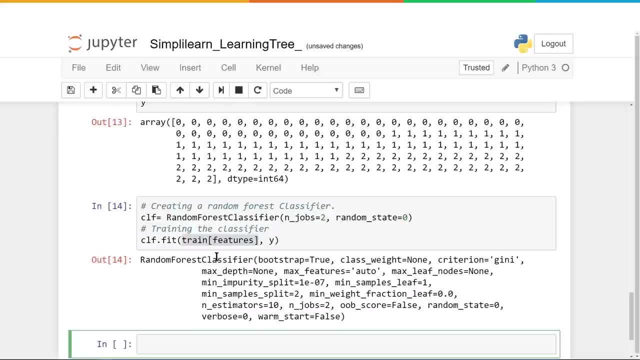 And the features is the actual data, The data going in that we put into the training set And let's go ahead and run that. And this is kind of an interesting thing because it printed out the random forest classifier and everything around it, And so when you're running this in your terminal window, 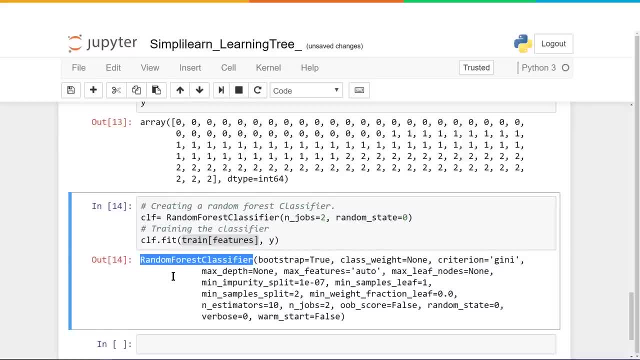 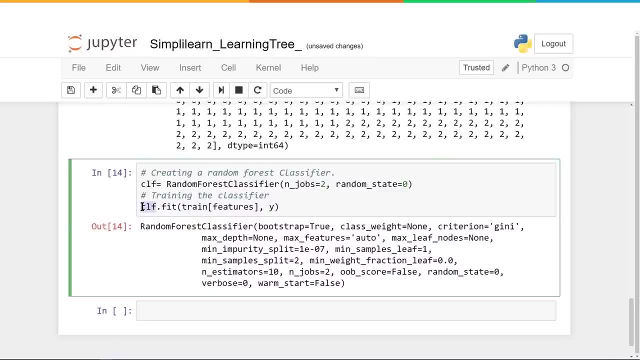 or in a script like this. this automatically treats this, just like when we were up here and I typed in y and it printed out y instead of print y. This does the same thing. It treats this as a variable and prints it out, But if you're actually running your code, 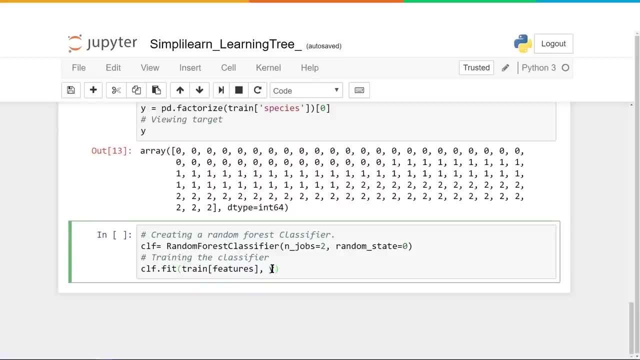 And here's our target, The Y. So the Y is zero one and two that we just created And the features is the actual data going in that we put into the training set And let's go ahead and run that, And this is kind of an interesting thing. 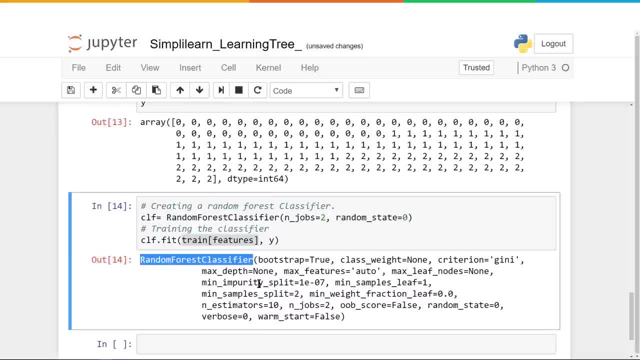 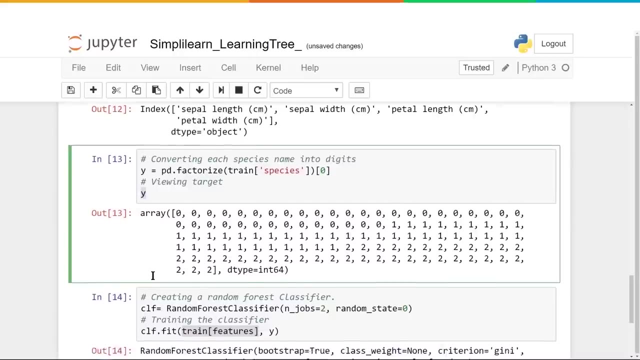 because it printed out the random forest classifier And everything around it, And so when you're running this in your terminal window or in a script like this, this automatically treats this like, just like when we were up here and I typed in Y and it printed out Y instead of print Y. 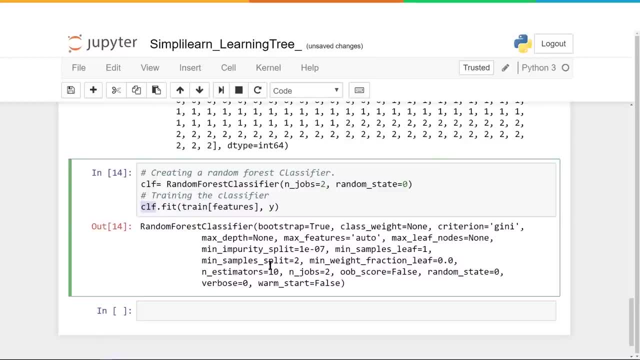 This does the same thing. It treats this as a variable and prints it out. But if you're actually running your code, that wouldn't be the case. And what is printed out is: it shows us all the different variables we can change And if we go down here, you can actually see in jobs equals two. 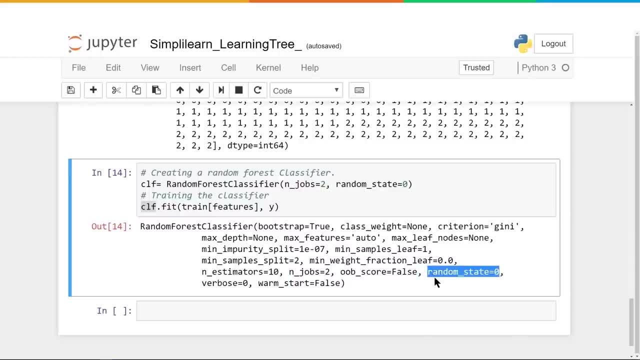 You can see the random state equals zero. Those are the two that we sent in there. You would really have to dig deep to find out all these different meanings of all these different settings on here. Some of them are self-explanatory If you kind of think about it a little bit like max features is auto. 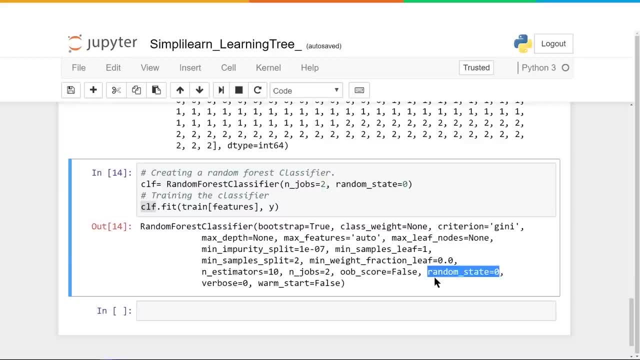 So all the features that we're putting in there is just going to automatically take all four of them. Whatever we send it, it'll take. Some of them might have so many features because you're processing words. There might be like one point four million features in there because you're doing. 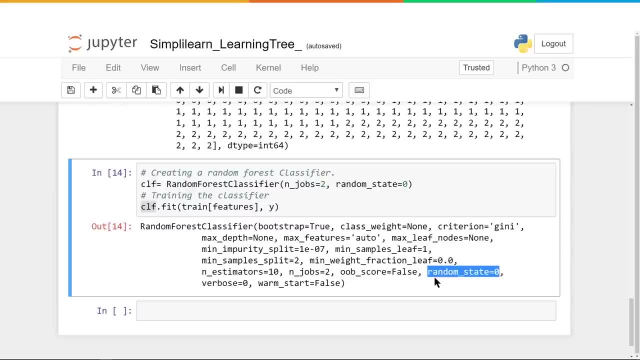 legal documents and that's how many different words are in there. At that point you probably want to limit the maximum features that you're going to process And leaf nodes- that's the end nodes. Remember we had the fruit and we're talking about the leaf nodes. 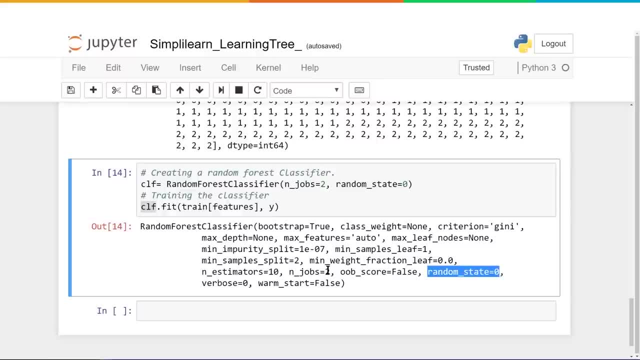 Like I said, there's a lot in this. We're looking at a lot of stuff here, So you might have- in this case there's probably only three leaf nodes, maybe four. You might have thousands of leaf nodes, at which point you do need to put a cap on that and say, OK, you can only go so far. 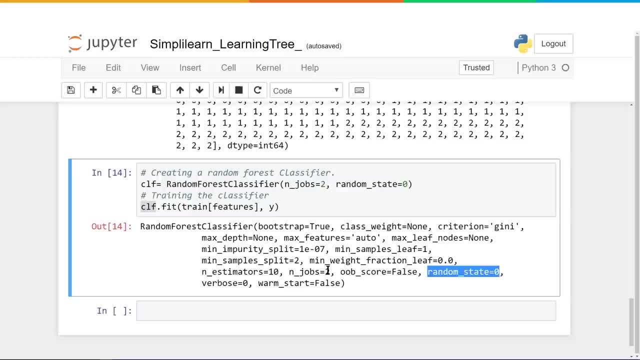 and then we're going to use all of our resources on processing this, And that really is what most of these are about is limiting the process and making sure we don't overwhelm a system. And there's some other settings in here. Again, we're not going to go over all of them. 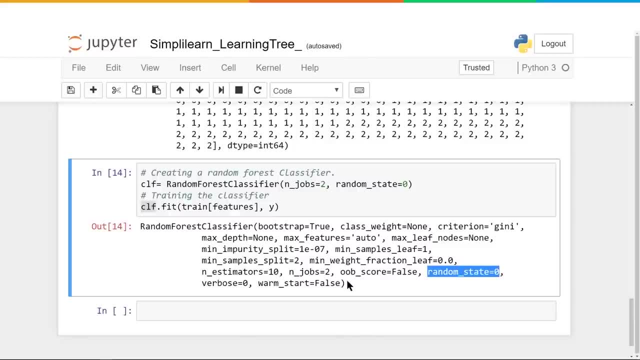 Warm start equals false. Warm start is if you're programming it one piece at a time externally, Since we're not, we're not going to have, like we're not going to, continually to train this particular learning tree. And again, like I said, there's a lot of things in here that you'll want to look. 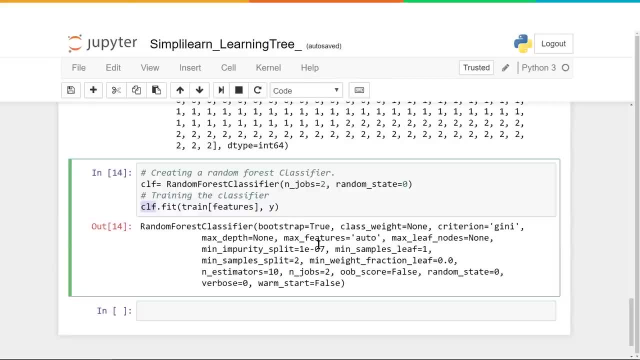 that wouldn't be the case And what it's printed out is. it shows us all the different variables we can change And if we go down here, you can actually see njobs equals two. You can see the random state equals zero. Those are the two that we sent in there. 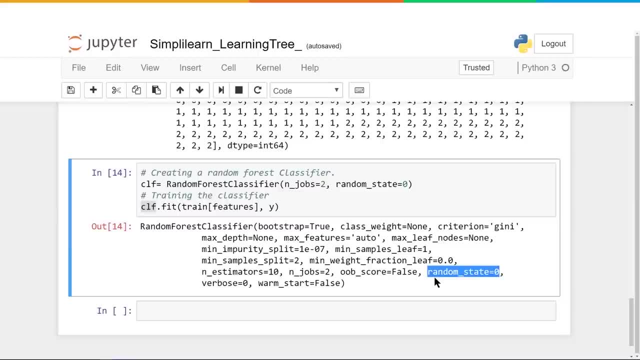 You would really have to dig deep to find out all these different meanings of all these different settings on here. Some of them are self-explanatory if you kind of think about it a little bit. like max features is auto, So all the features that we're putting in there. 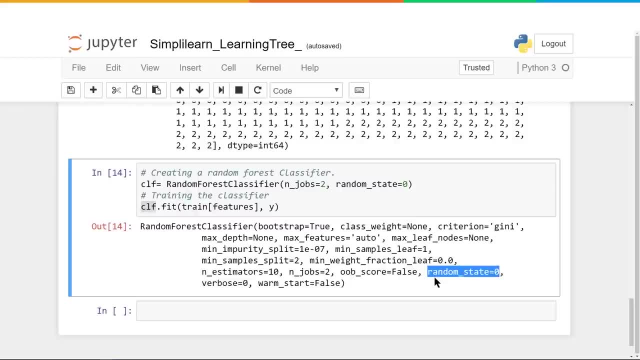 all four of them. whatever we send it, it'll take. Some of them might have so many features because you're processing words. there might be like 1.4 million features in there because you're doing legal documents and that's how many different words are in there. 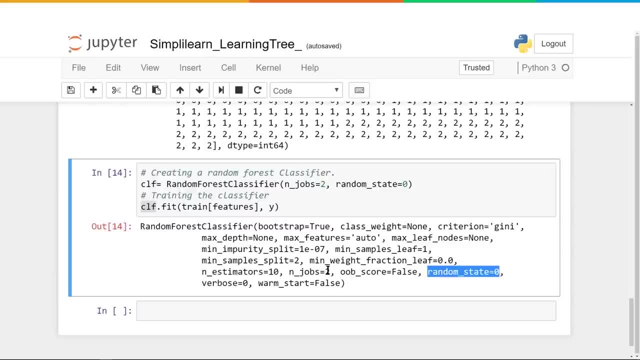 At that point you probably want to limit the maximum features that you're going to process And leaf nodes. that's the end nodes. Remember we had the fruit and we're talking about the leaf nodes. Like I said, there's a lot in this. 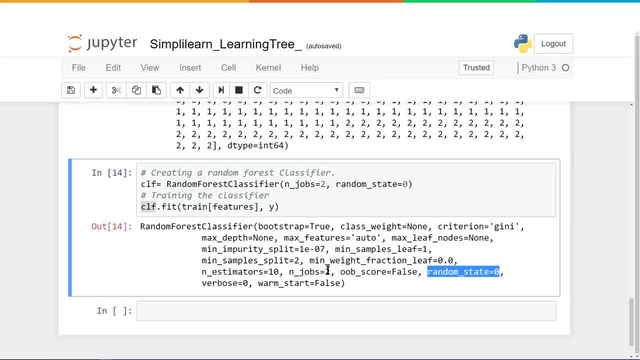 We're looking at a lot of stuff here, So you might have- in this case there's probably only, I think- three leaf nodes, maybe four. You might have thousands of leaf nodes, at which point you do need to put a cap on that. 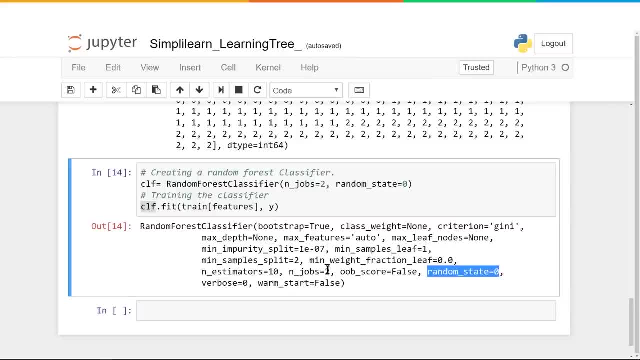 and say, okay, you can only go so far, and then we're going to use all of our resources on processing this, And that really is what most of these are about is limiting the process and making sure we don't overwhelm a system, And there's some other settings in here. 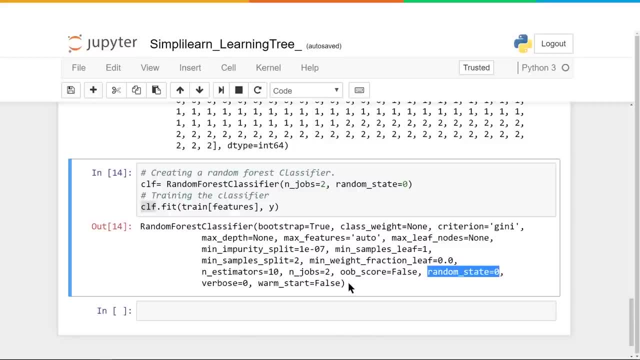 Again, we're not going to go over all of them. Warm start equals false, Warm start is if you're programming it one piece at a time externally. Since we're not, we're not going to have, we're not going to continually detrain. 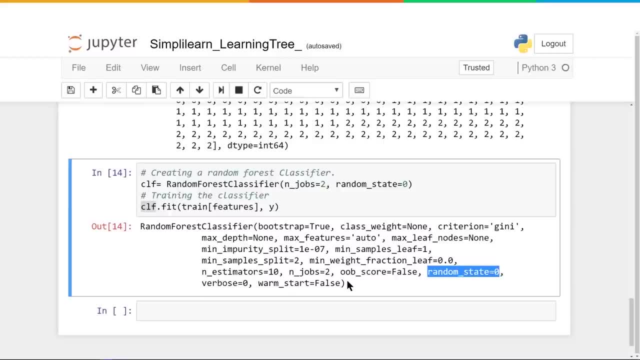 this particular learning tree, So there's a lot of things in here that you'll want to look up more detail from the sklearn, and if you're digging in deep and running a major project on here. For today, though, all we need to do 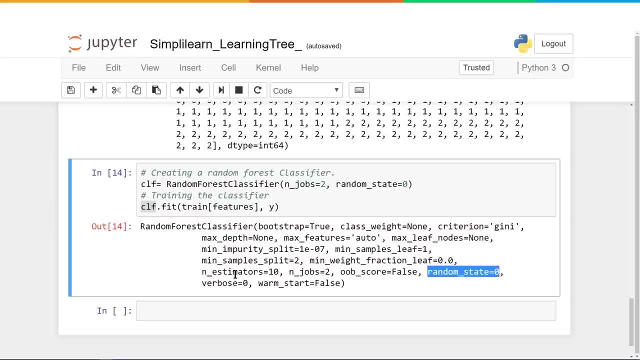 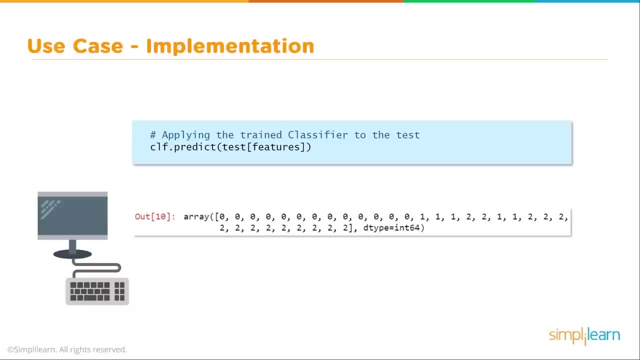 is fit, or train our features and our target Y. So now we have our training model. What's next? If we're going to create a model, we now need to test it. Remember we set aside the test feature- test group- 25% of the data. 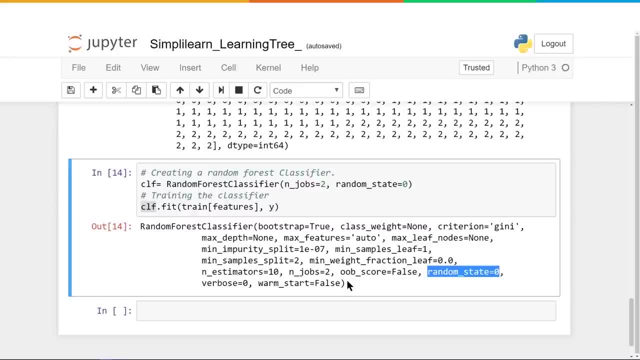 up more detail from the SKLearn and if you're digging in deep and running a major project on here. For today, though, all we need to do is fit or train our features and our target Y, So now we have our training model. 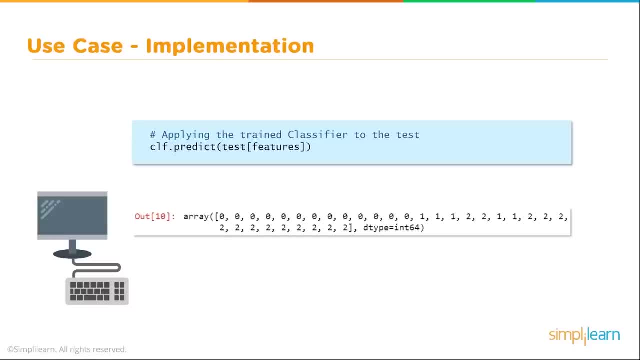 What's next? If we're going to create a model, we now need to test it. Remember, we set aside the test feature, test group- 25 percent of the data. So let's go ahead and take this code and let's put it into our script and see what. 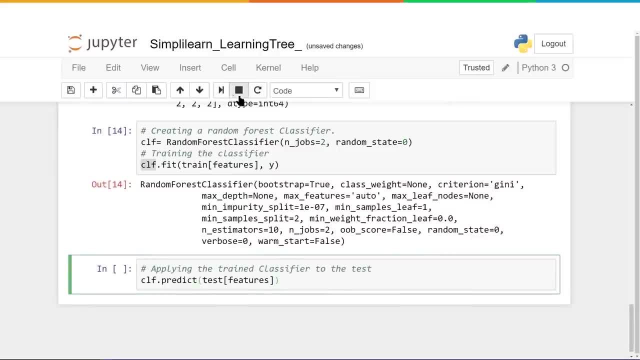 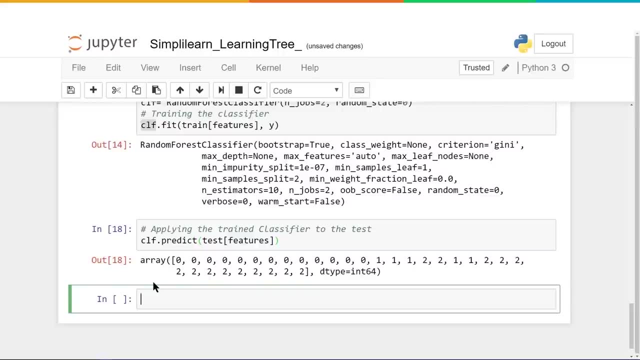 that looks like, Here we go And we're going to run this And it's going to come out with a bunch of zeros, ones and twos, which represents the three type of flowers: the setosa, the virginica and the versicolor. 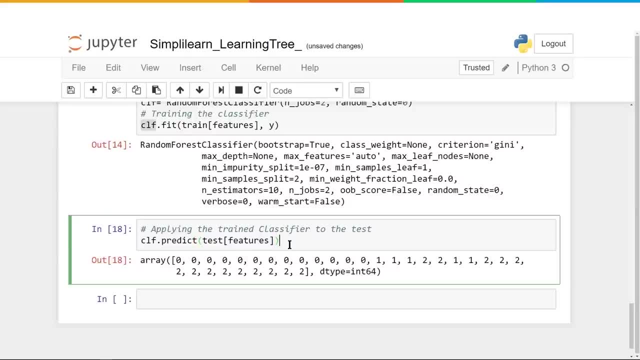 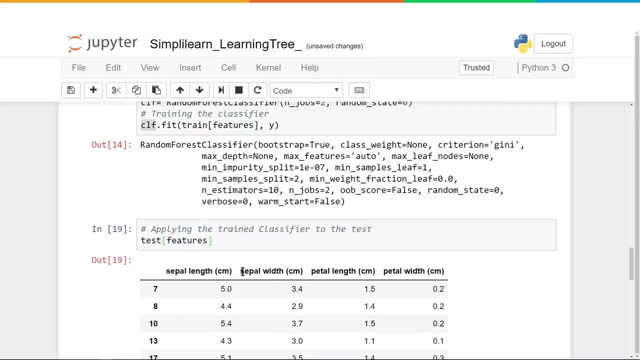 And what we're putting into our predict is the test features, And I always kind of like to know what it is I am looking at. So, real quick, we're going to do test features And remember features is an array of sepal length, sepal width, petal length, petal width. 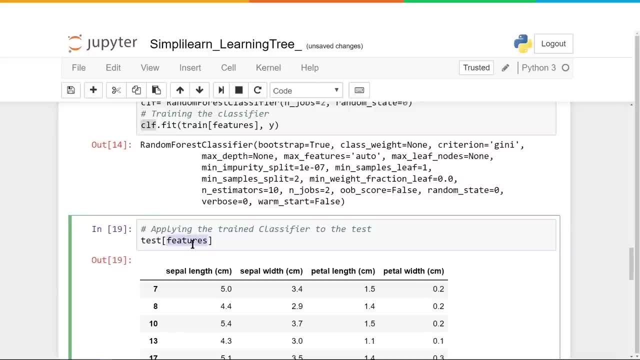 So when we put it in this way, it actually loads all these different columns that we loaded into features. So if we did just features, let me just do features in here So it features. looks like this is just playing with the, with Pandas data frames. 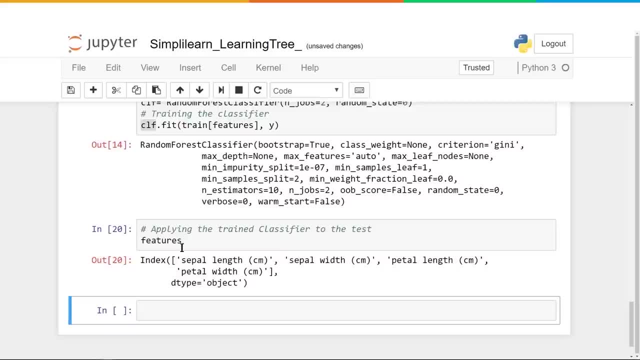 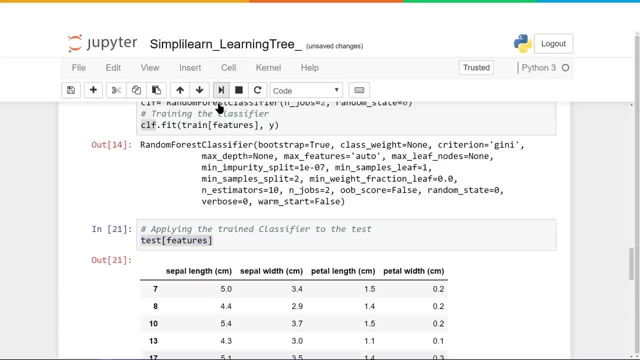 You'll see that it's an index. So when you put an index in like this Into test, features, into test- it then takes those columns and creates a Panda data frames from those columns and in this case we're going to go ahead and put those into our predict. 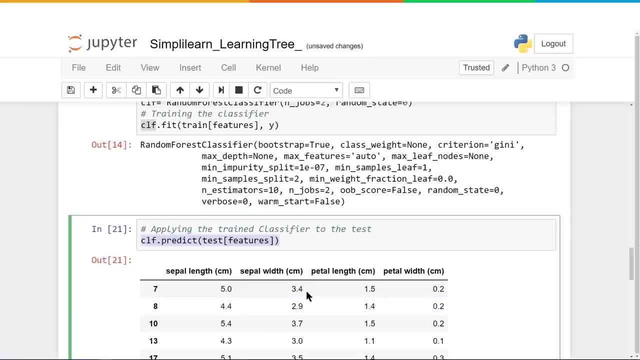 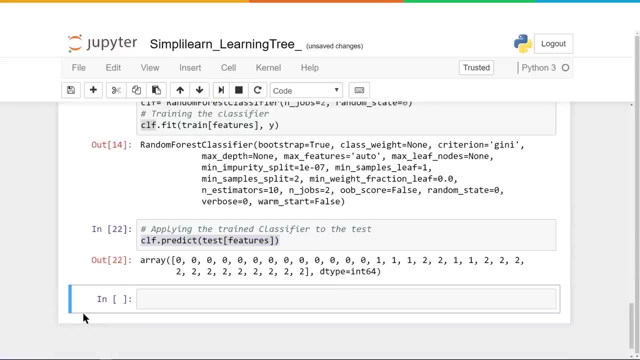 So we're going to put each one of these lines of data- the five point, oh, three point four, one point, five, point two- and we're going to put those in and we're going to predict what our new Forest classifier is going to come up with. and this is what it predicts. 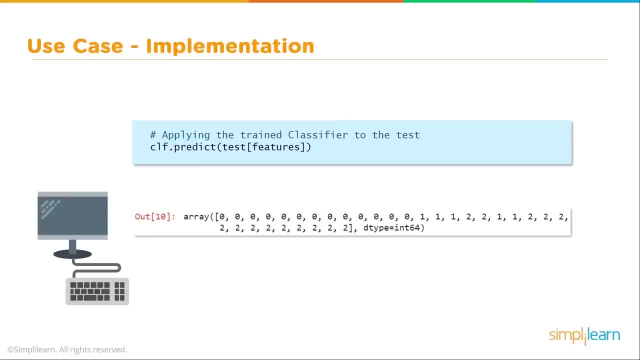 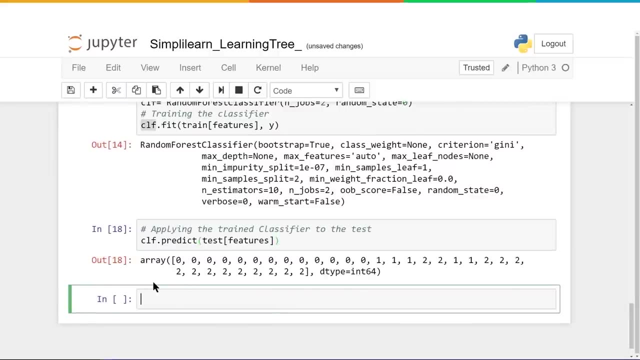 So let's go ahead and take this code and let's put it into our script and see what that looks like. Okay, here we go And we're going to run this and it's going to come out with a bunch of zeros, ones and twos. 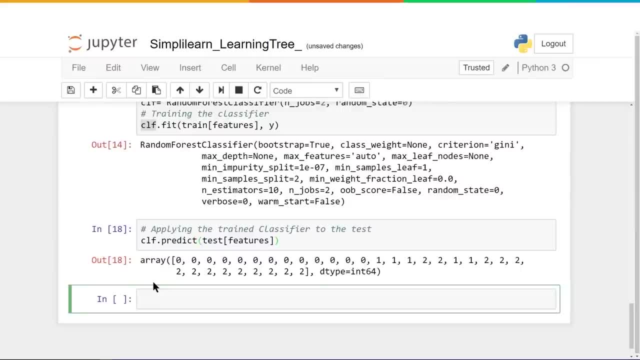 which represents the three types of flowers: The setosa, the virginica and the versicolor. And what we're putting into our predict is the test features, And I always kind of like to know what it is I am looking at. So, real quick, we're going to do. 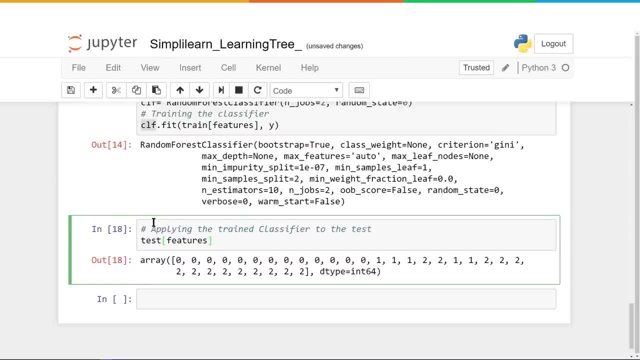 test features And remember, features is an array Of sepal length, sepal width, petal length, petal width. So when we put it in this way, it actually loads all these different columns that we loaded into features. So if we did just features, 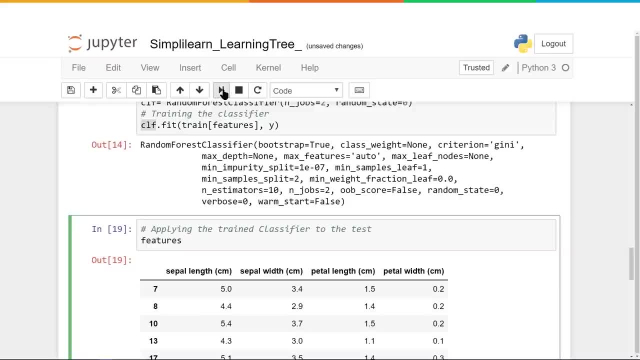 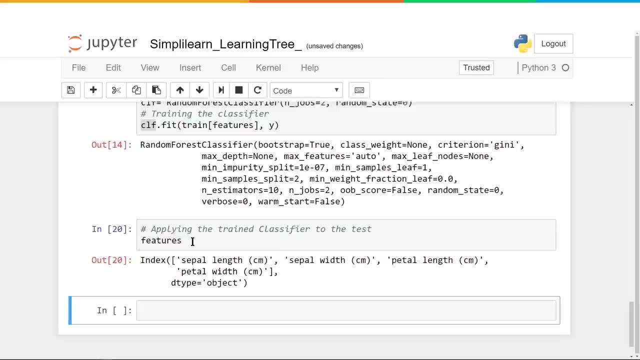 let me just do features in here so you can see what features looks like. This is just playing with Panda's data frames. You'll see that it's an index. So when you put an index in like this into test, features into test- 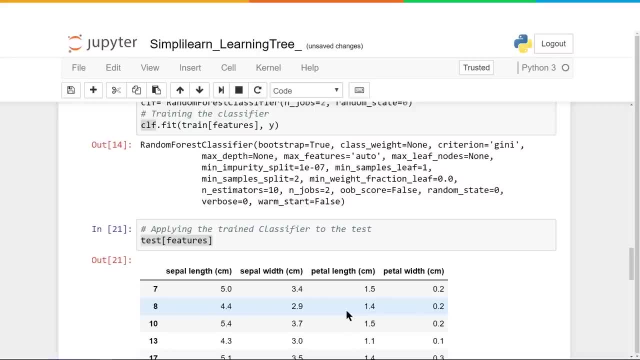 it takes those columns and creates a Panda data frame from those columns And in this case we're going to go ahead and put those into our predict. So we're going to put each one of these lines of data, the 5.0,. 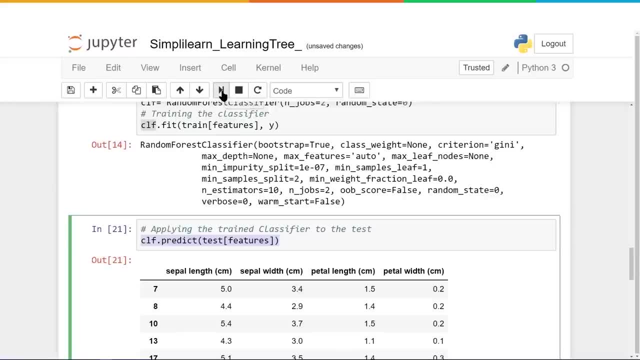 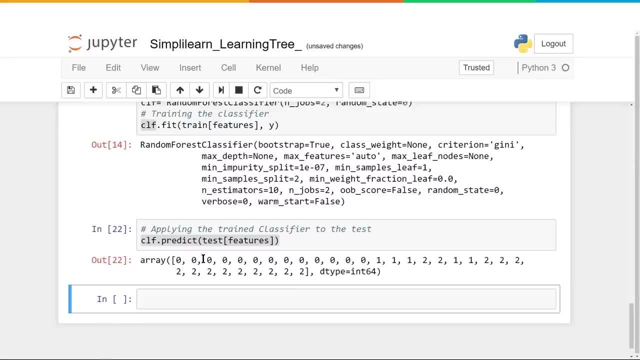 3.4, 1.5, 0.2, and we're going to put those in and we're going to predict what our new forest classifier is going to come up with. And this is what it predicts. It predicts 0, 0, 0, 1, 2, 1, 1, 2, 2, 2. 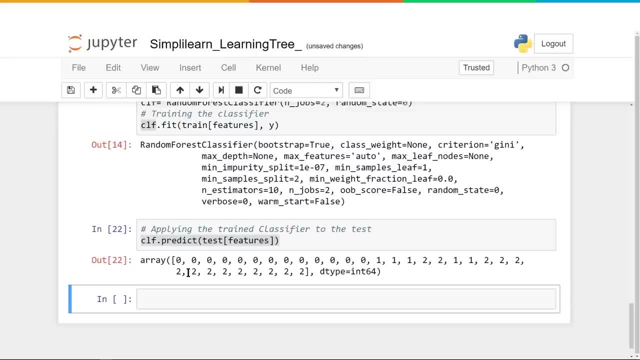 It predicts zero, zero, zero, one, two, one, one, two, two, two, And and again. this is the flower type, So Tosa, Virginia and Versicolor. So now that we've taken our test features, let's explore that, Let's see exactly what that data means to us. 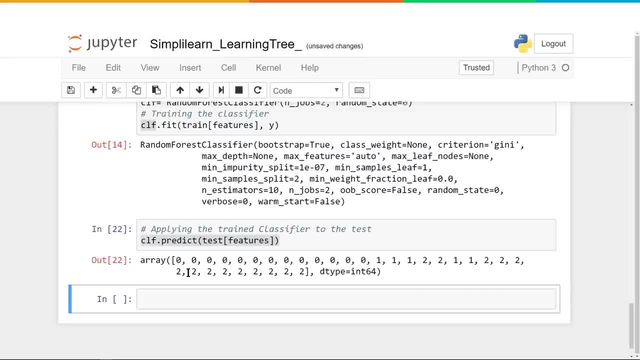 and again, this is the flower type: setosa, virginica and versicolor. So now that we've taken our test features, let's explore that. Let's see exactly what that data means to us. So the first thing we can do with, 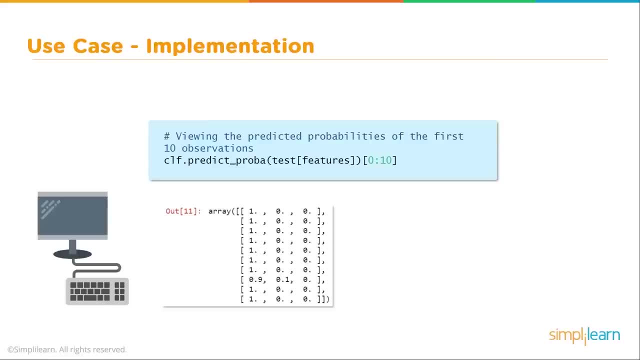 our predicts is. we can actually generate a different prediction model. When I say different, we're going to view it differently. It's not that the data itself is different. So let's take this next piece of code and put it into our script. 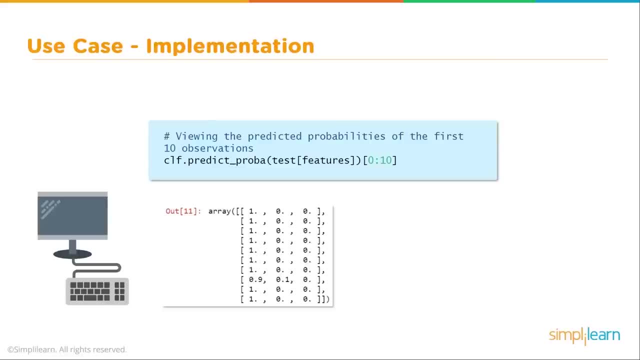 So the first thing we can do with our predicts is we can actually generate a different prediction model. when I say different, We're going to view it differently. It's not that the data itself is different. So let's take this next piece of code and put it into our script. 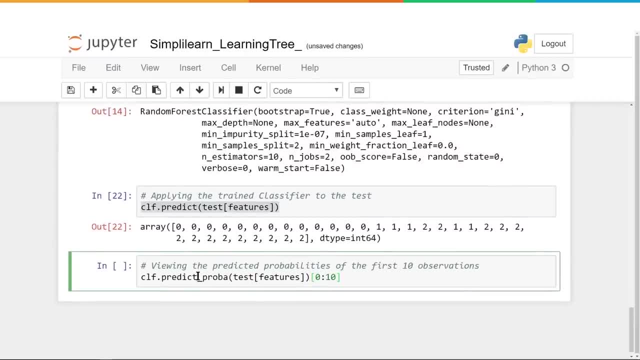 So we're pasting it in here and you'll see that we're doing predict and we've added underscore proba for probability. so there's our CLF predict probability. So we're running it just like we ran it up here, But this time, with this, we're going to get a slightly different result. 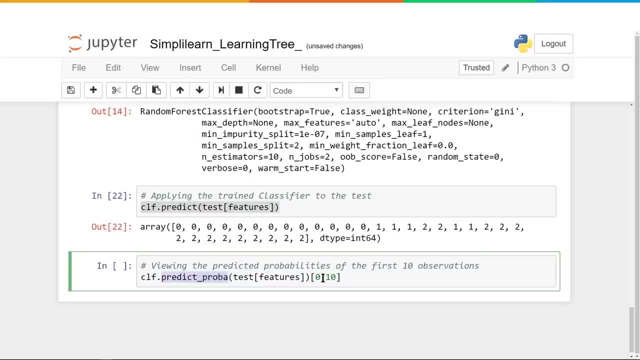 And we're only going to look at the first ten. So you'll see down here, instead of looking at all of them, which was what twenty seven? you'll see right down here that this generates a much larger field on the probability. 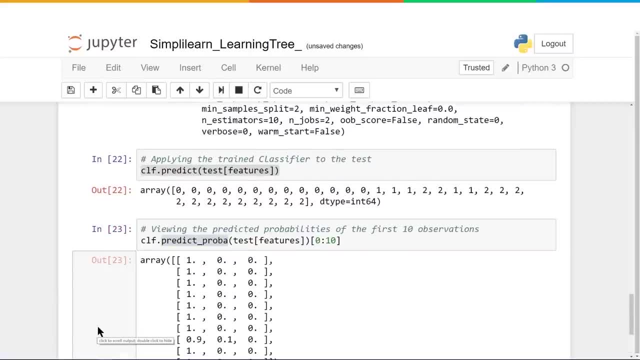 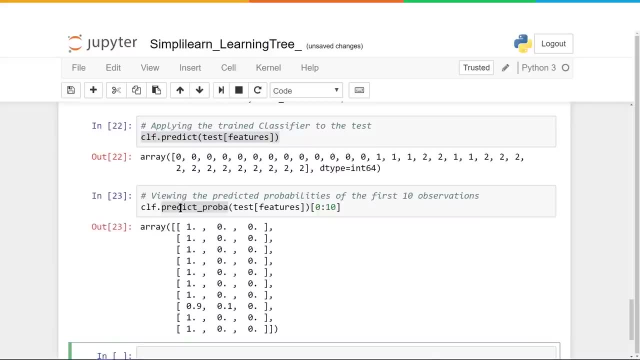 And let's take a look and see what that looks like and what that means. So when we do the predict underscore, proba for probability, it generates three numbers. So we had three leaf nodes at the end And if you remember from all the theory we did, this is the predictors. 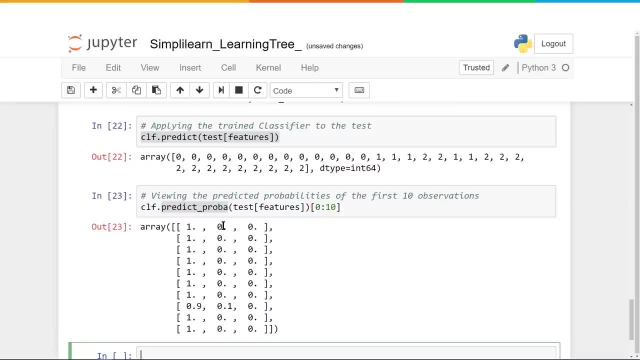 The first one is predicting a one for Tosa, The second one is predicting a zero for Virginica, and it predicts a zero for Versacolor, and so on, and so on, and so on. And let's you know what? I'm going to change this just a little bit. 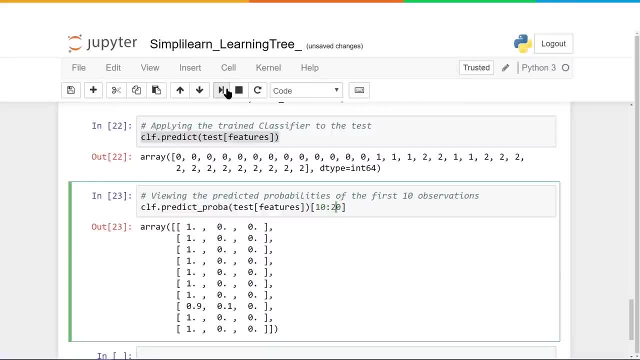 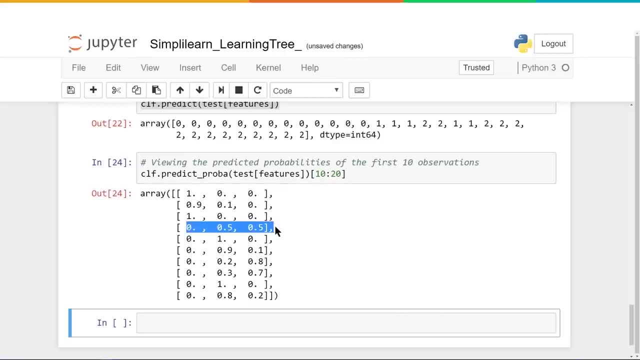 Let's look at ten to twenty, just because we can And we start to get a little different of data and you'll see right down here it gets to this one, this line, right here, and this line has zero, zero point five, zero point five. 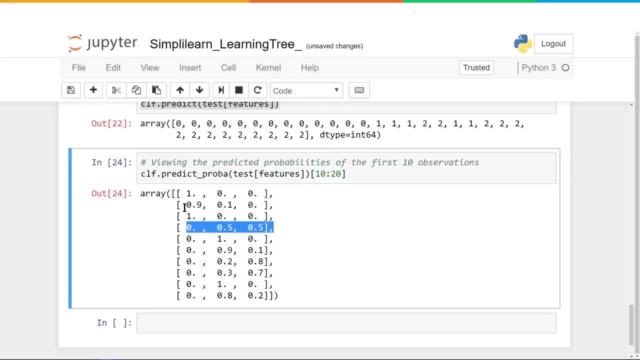 And so if we're going to vote and we have two equal votes, it's going to go with the first one. So it says Satosa gets zero votes, Virginica gets point five votes, Versacolor gets point five votes, But let's just go with the Virginica, since these two are equal, and so on and so on down the list. 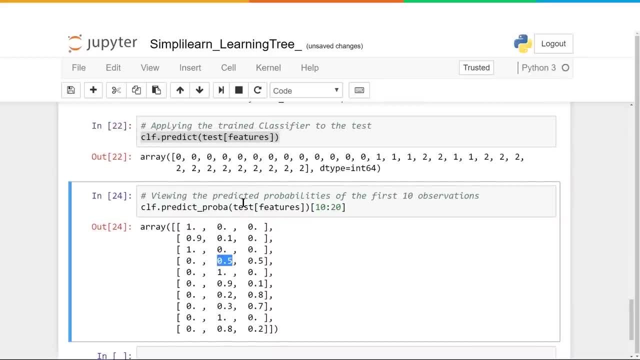 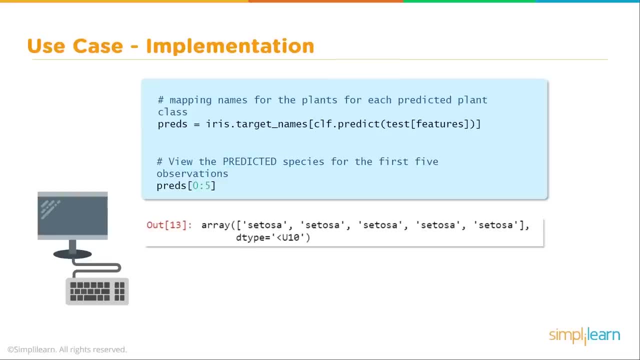 You can see how they vary on here. So now we've looked at both- how to do a basic predict of the features and we've looked at the predict probability. Let's see what's next on here. So now we want to go ahead and start mapping names for the plants. 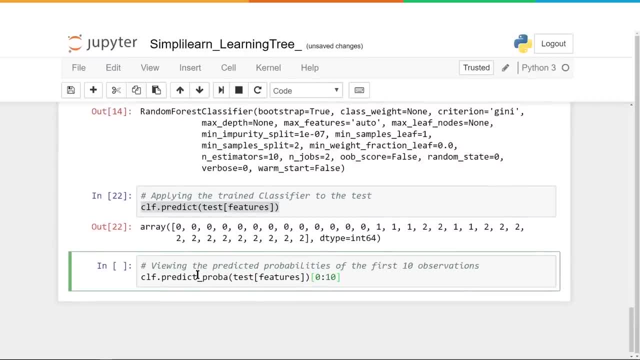 So we're pasting it in here and you're going to see that we're doing predict and we've added underscore proba for probability. So there's our clfpredict probability. So we're running it just like we ran it up here, but this: 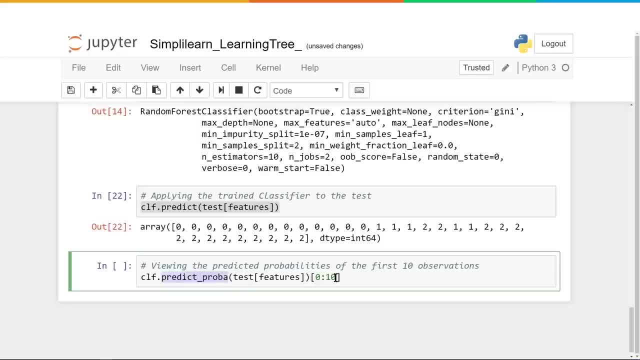 time. with this, we're going to get a slightly different result And we're only going to look at the first 10. So you'll see down here instead of looking at all of them, which was 27,. you'll see right down here. 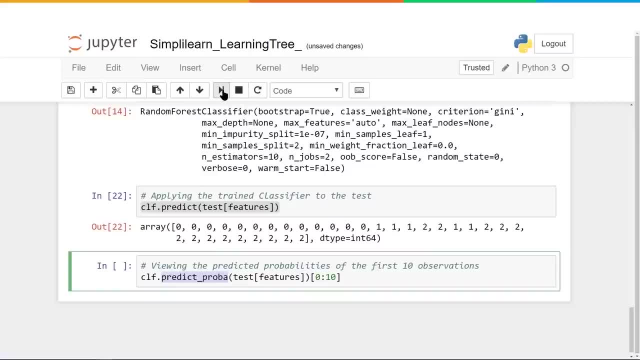 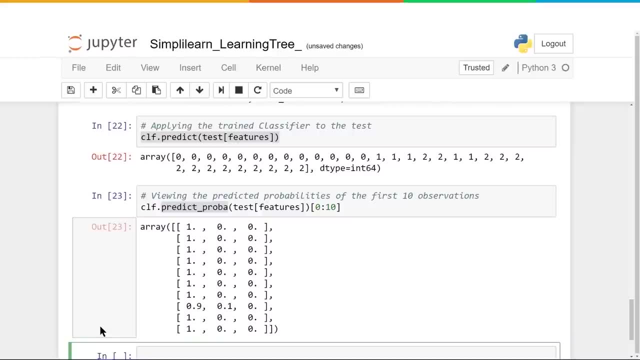 that this generates a much larger field on the probability And let's take a look and see what that looks like And what that means. So when we do the predict, underscore proba for probability, it generates three numbers, So we had three. 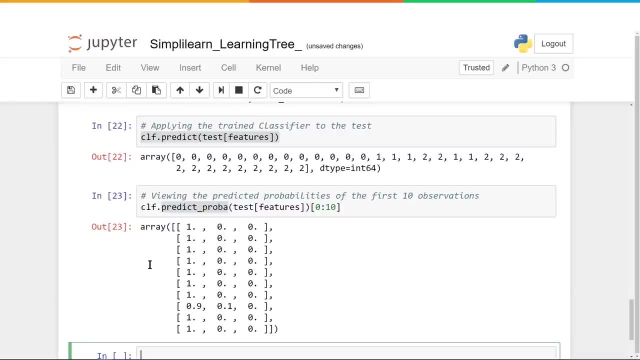 leaf nodes at the end. And if you remember from all the theory we did, this is the predictors. The first one is predicting a 1 for setosa, It predicts a 0 for virginica, And it predicts a 0 for versicolor, And so on and so on. 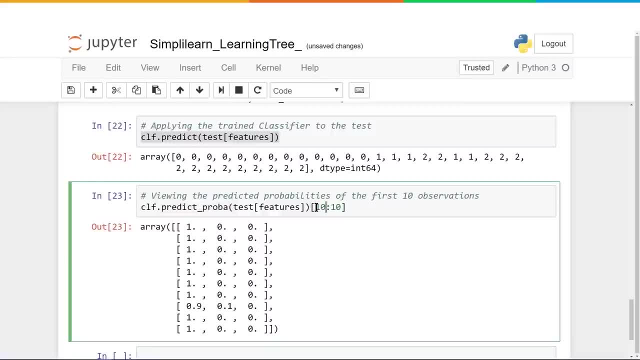 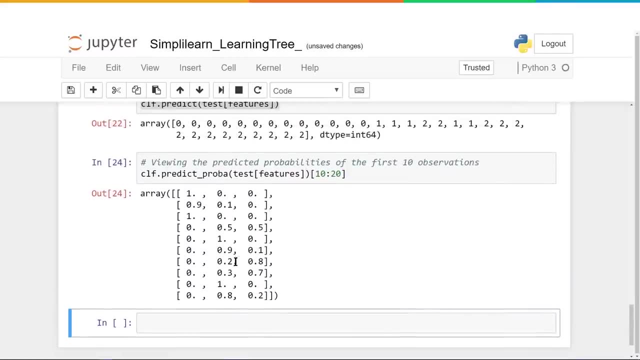 and so on. And let's you know what, I'm going to change this just a little bit. Let's look at 10 to 20, just because we can, And we start to get in a little different of data And you'll see, right down here it gets. 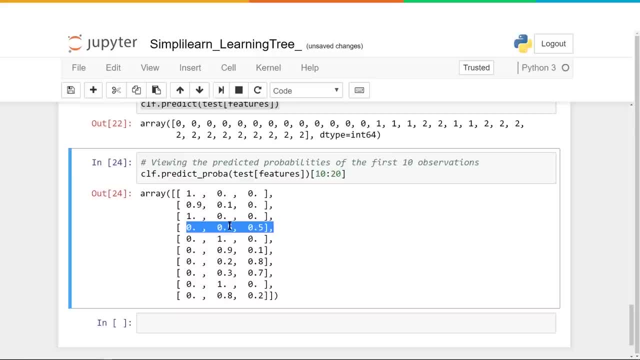 to this one, this line right here, And this line has 0,, 0.5,, 0.5. And so if we're going to vote and we have two equal votes, it's going to go with the first one. So it says: 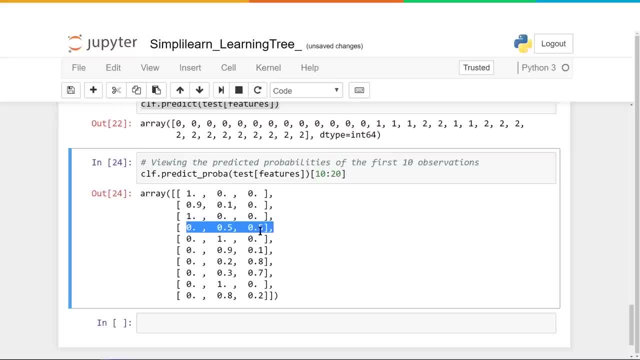 setosa gets 0 votes, virginica gets 0.5 votes, versicolor gets 0.5 votes, But let's just go with the virginica, since these two are equal, And so on and so on down the list. 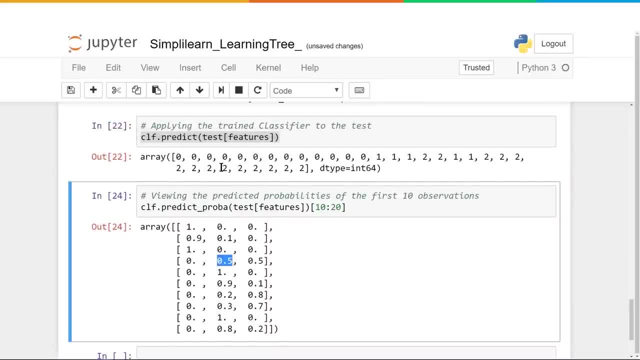 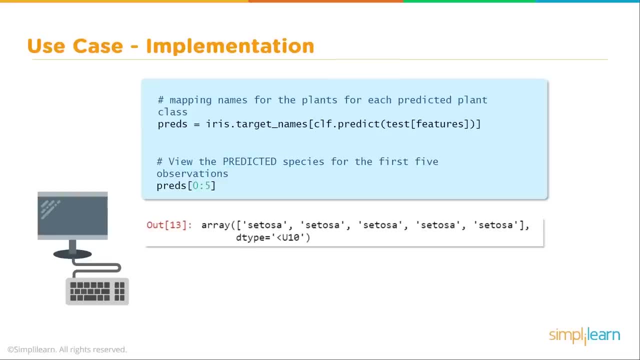 You can see how they vary on here. So now we've looked at both- how to do a basic predict of the features, and we've looked at the predict probability. Let's see what's next on here. So now we want to go ahead and start. 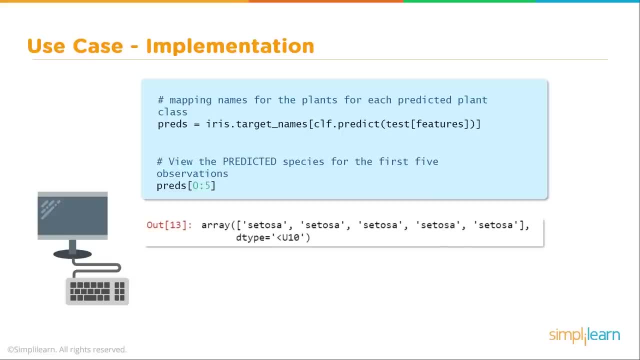 mapping names for the plants. We want to attach names so that it makes a little more sense for us, And that's what we're going to do in these next two steps. We're going to start by setting up our predictions and mapping them to the names. 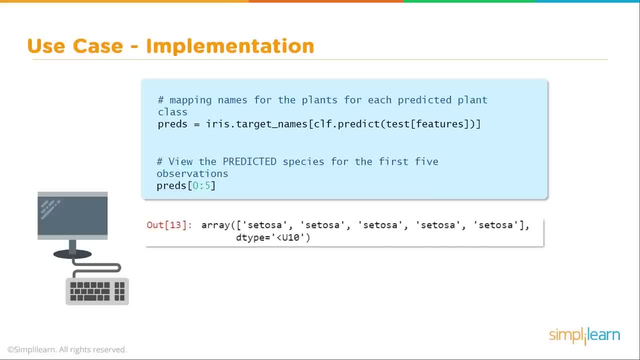 We want to attach names so that it makes a little more sense for us, and that's what we're going to do in these next two steps. We're going to start by setting up our predictions and mapping them to the name, So let's see what that looks like. 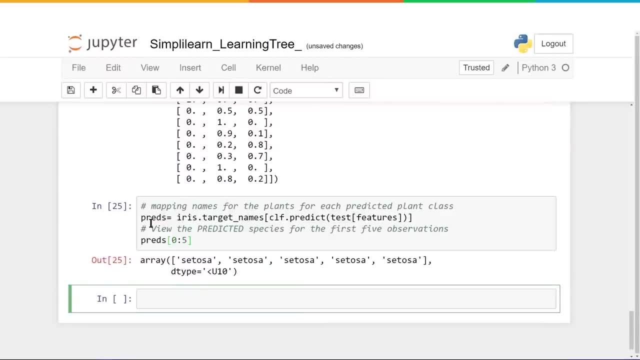 And let's go ahead and paste that code in here and run it, And this goes along with the next piece of code. So we'll skip through this quickly and then come back to it a little bit. So here's iris dot target names. 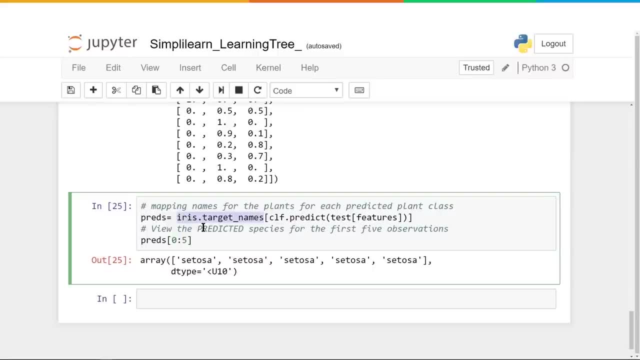 And, if you remember correctly, this was the names that we've been talking about this whole time: the setosa virginica versicolor. And then we're going to go ahead and do the prediction again. We could have just set a variable equal to this, instead of rerunning it each time. 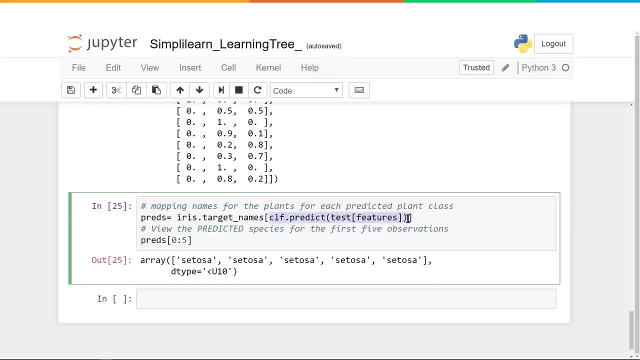 But we're going to run it again. clf dot- predict test features. Remember that returns the zeros, the ones and the twos, And then we're going to set that equal to predictions. So this time we're actually putting it in a variable. 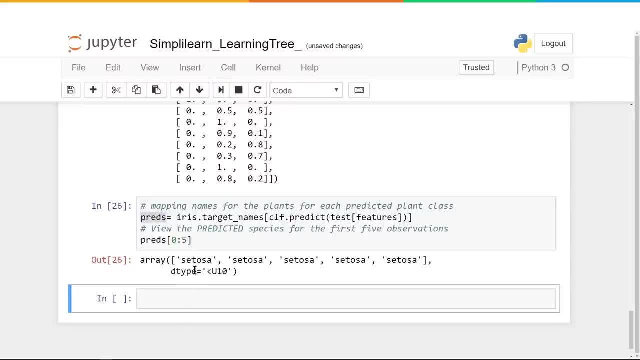 And when I run this it comes out as an array and the array is: setosa, setosa, setosa, setosa. We're only looking at the first five. We could actually do let's do the first 25, just so we can see a little bit more on there. 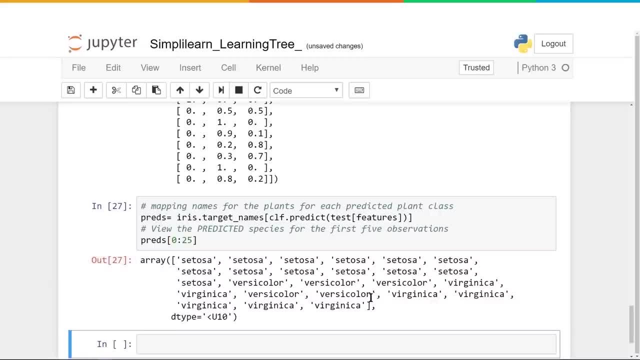 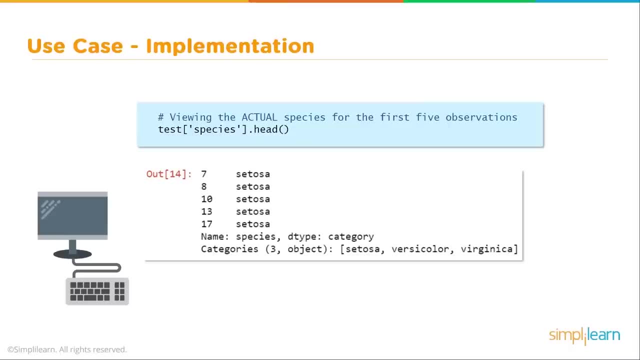 And you'll see that it starts mapping it to all the different flower types- the versicolor and the virginica in there- And let's see how this goes with the next one. So let's take a look at the top part of our species in here. 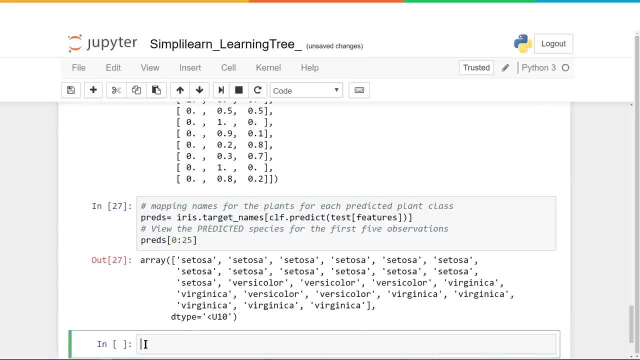 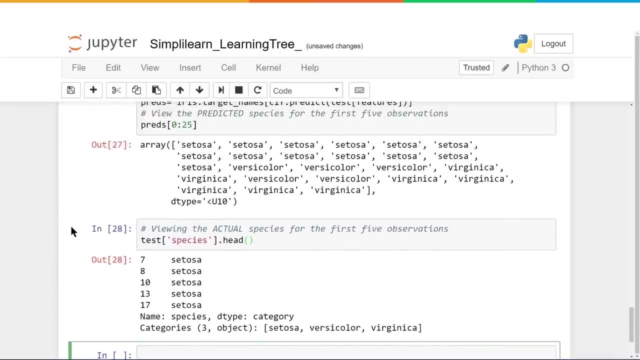 And we'll take this code and put it in our script. Let's put that down here and paste it. There we go And we'll go ahead and run it. And let's talk about both These sections of code here and how they go together. 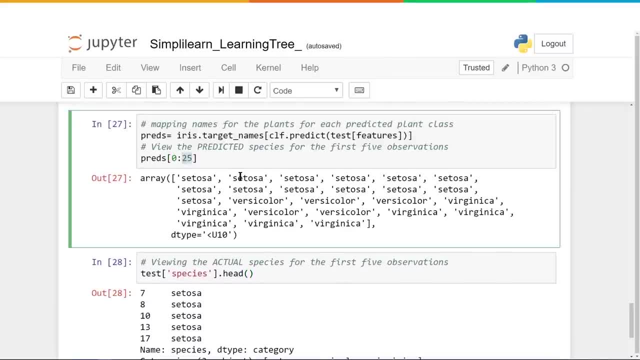 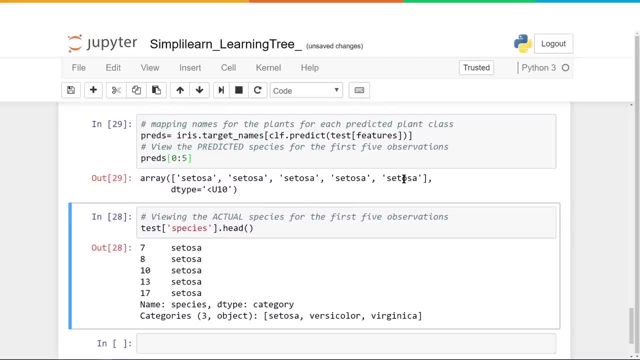 The first one is our predictions, And I went ahead and did predictions through 25.. Let's just do five, And so we have setosa, setosa, setosa, setosa. That's what we're predicting from our test model. 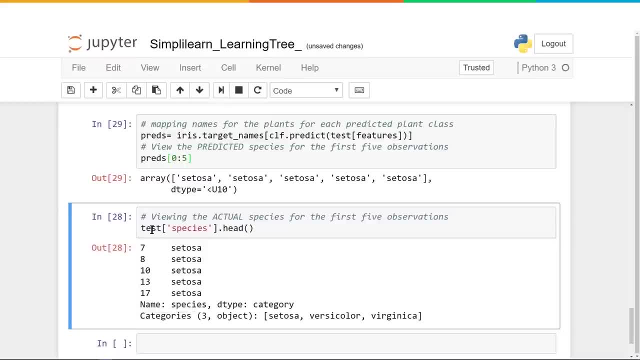 And then we come down here we look at test species. I remember I could have just done testspecieshead and you'll see, it says setosa, setosa, setosa, setosa And they match. So the first one is what our forest is doing. 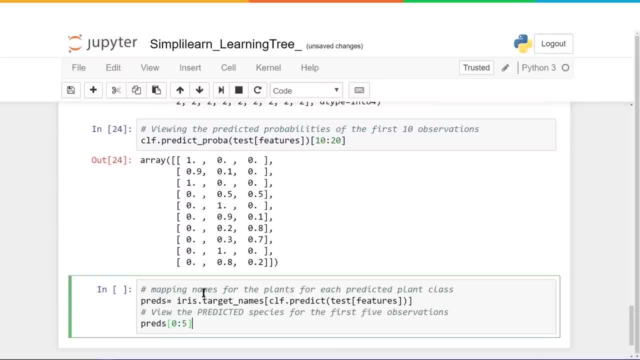 So let's see what that looks like And let's go ahead and paste that code in here and run it, And this goes along with the next piece of code. So we'll skip through this quickly and then come back to it a little bit. 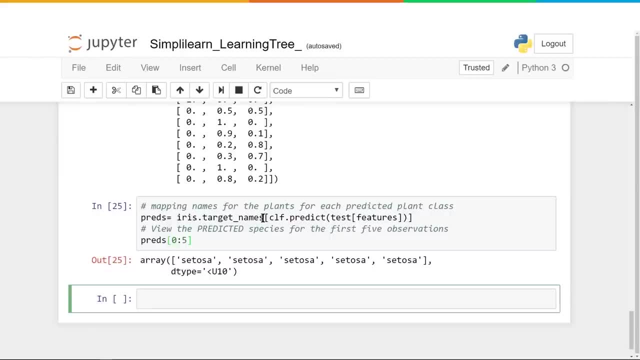 So here's iris dot target names And, if you remember correctly, this was the names that we've been talking about this whole time: The setosa virginica versicolor. And then we're going to go ahead and do the prediction again. 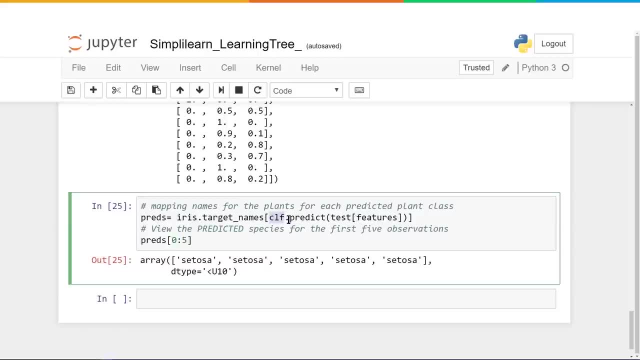 We could have just said a very variable equal to this, instead of re-running it each time, But we're going to go ahead and run it again. clf dot: predict test features. Remember that returns the zeros, the ones and the twos, And then we're going to set that. 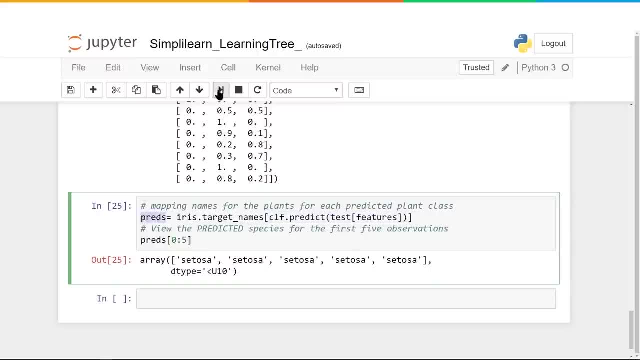 equal to predictions. So this time we're actually putting it in a variable And when I run this, it distributes and it comes out as an array And the array is: setosa, setosa, setosa, setosa, setosa. We're only looking at the 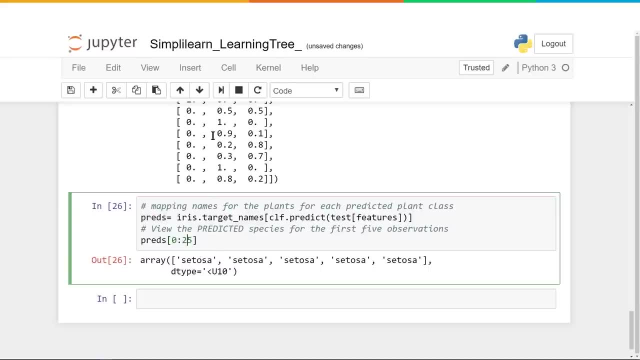 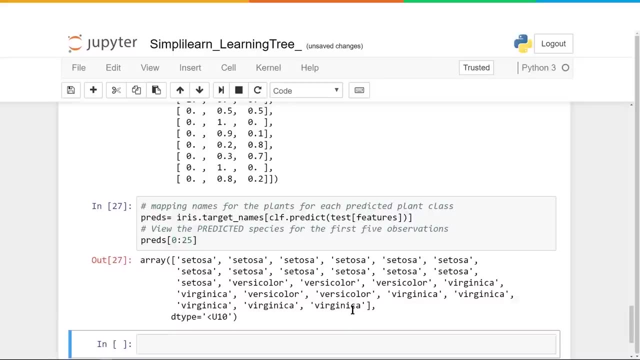 first five We could actually do. let's do the first 25, just so we can see a little bit more on there, And you'll see that it starts mapping it to all the different flower types- The versicolor and the virginica in there. 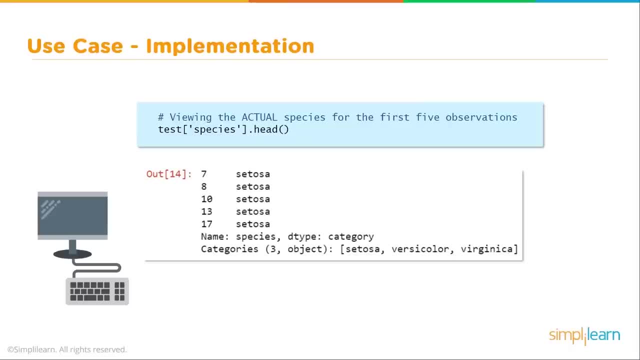 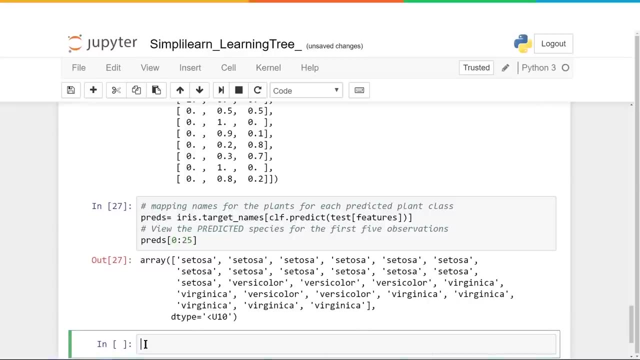 And let's see how this goes with the next one. So let's take a look at the top part of our species in here And we'll take this code and put it in our script And let's put that down here and paste it. 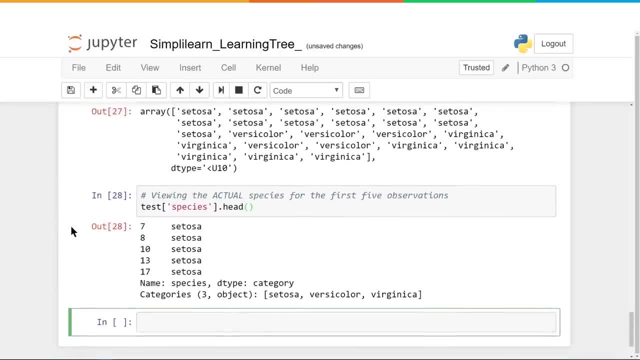 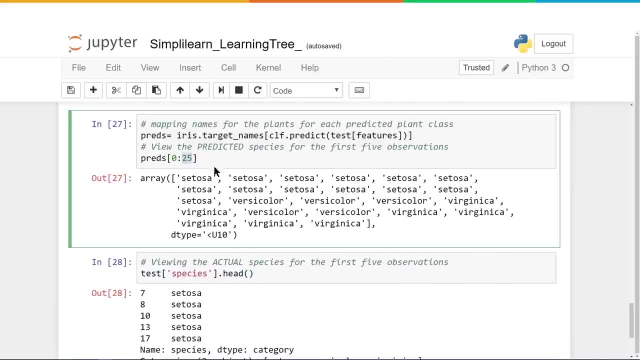 There we go, And we'll go ahead and run it, And let's talk about both these sections of code here And how they go together. The first one is our predictions, And I went ahead and did predictions through 25.. Let's just do 5.. 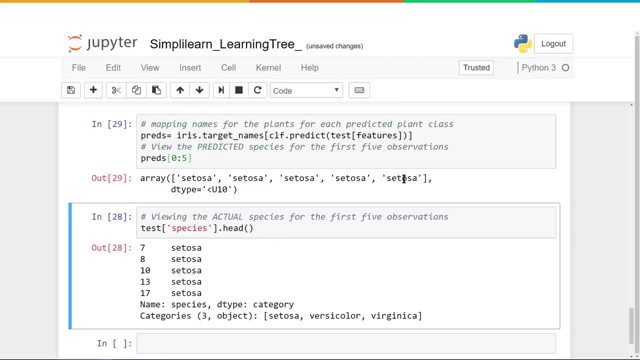 And so we have setosa setosa, setosa setosa. That's what we're predicting from our test model. And then we come down here and we look at test species And remember- I could have just done testspecieshead And you'll see, it says setosa setosa. 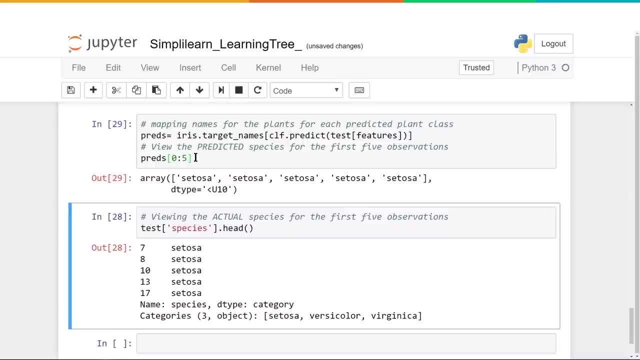 setosa, setosa And they match. So the first one is what our forest is doing And the second one is what the actual data is. Now we need to combine these so that we can understand what that means. We need to know how good our forest. 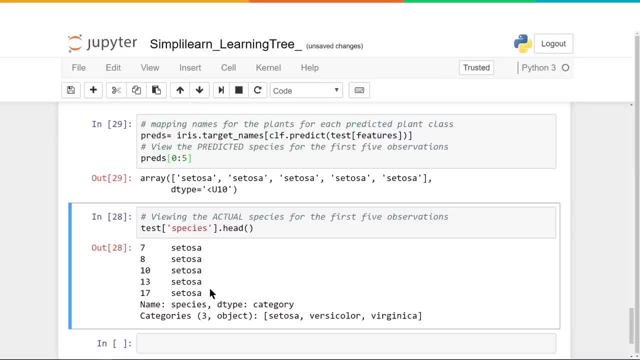 And the second one is what the actual data is. Now we need to combine these so that we can understand what that means. We need to know how good our forest is, how good it is at predicting the features. So that's where we come up to the next step, which is lots of fun. 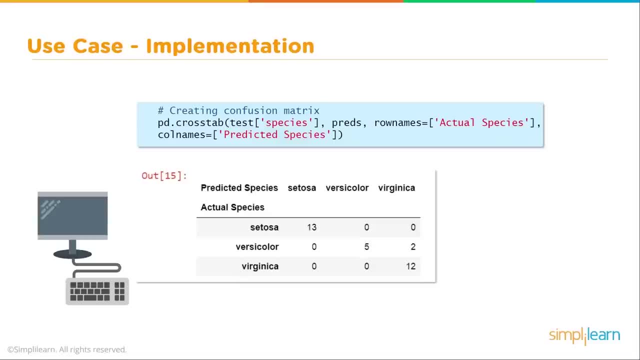 We're going to use a single line of code to combine our predictions and our actuals. So we have a nice chart to look at And let's go ahead and put that in our script in our Jupyter notebook here. Let's see, let's go ahead and paste that in. 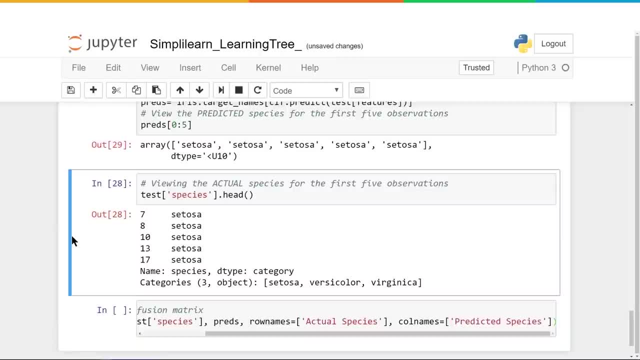 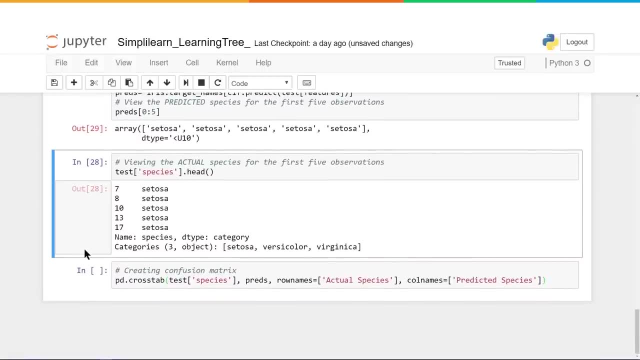 And then I'm going to, because I'm on the Jupyter notebook, I can do a control minus. You can see the whole line there. There we go, resize it And let's take a look and see what's going on here. 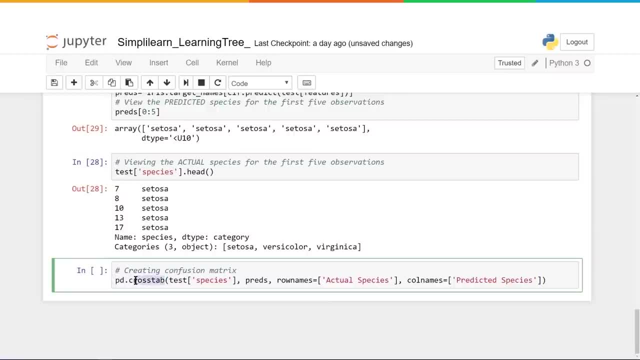 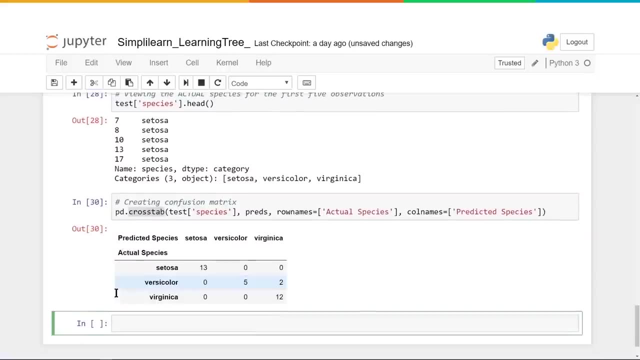 We're going to create in pandas- Remember, PD stands for pandas And we're doing a crosstab. This function takes two sets of data and creates a chart out of them, So when I run it you'll get a nice chart down here. 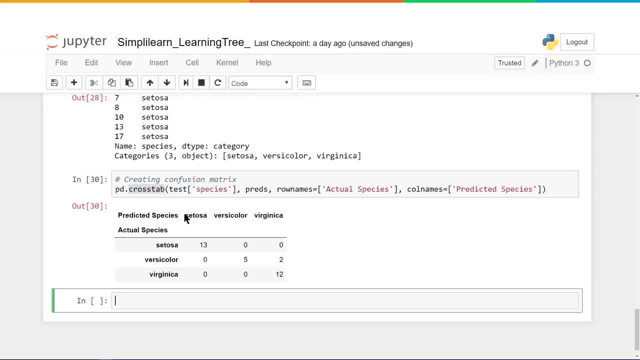 And we have the predicted species. So a crosstab: Across the top you'll see the Cetosa versicolor virginica and the actual species, Cetosa versicolor virginica. And so the way to read this chart. and let's go ahead and take a look on how to read this chart here. 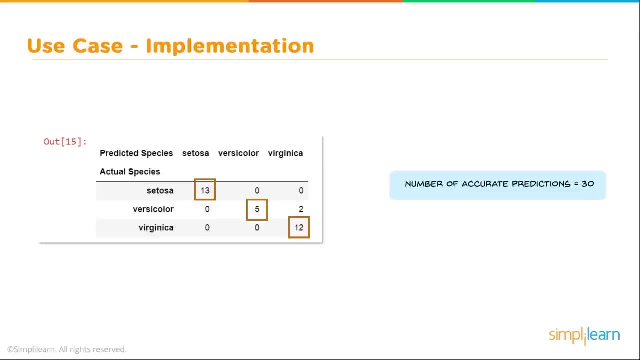 When you read this chart, you have Cetosa where they meet, you have versicolor where they meet, and you have virginica where they meet, And they're meeting where the actual and the predicted agree. So this is the number of accurate predictions. 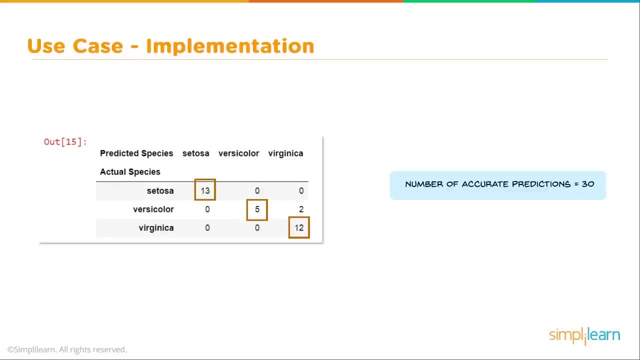 So in this case it equals 30. If you had 13 plus 5 plus 12, you get 30. And then we notice here where it says virginica, but it was supposed to be versicolor. This is inaccurate. 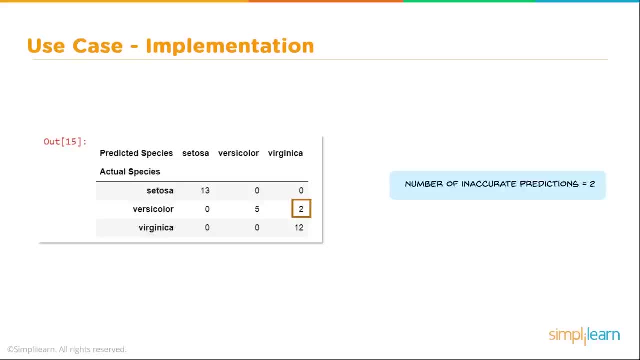 So now we have two: two inaccurate predictions and 30 accurate predictions. So we'll say that the model accuracy is 93. That's just 30 divided by 32. And if we multiply it by 100, we can say that it is 93 percent accurate. 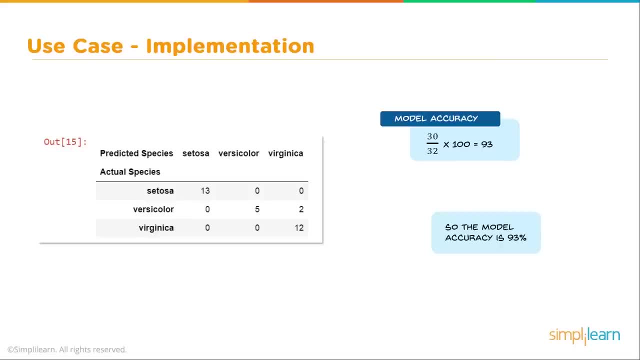 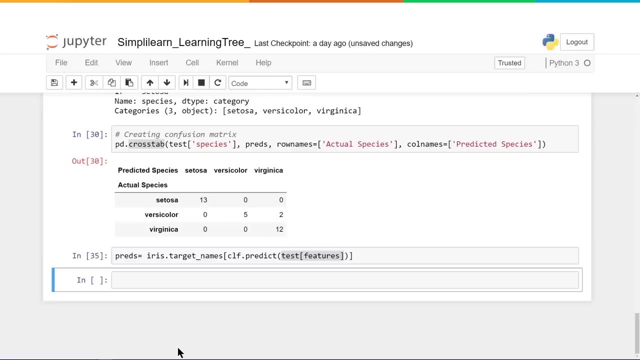 So we have a 93 percent accuracy with our model. I did want to add one more quick thing in here on our scripting before we wrap it up, So let's flip back on over to my script In here. we're going to take this line of code from up above: 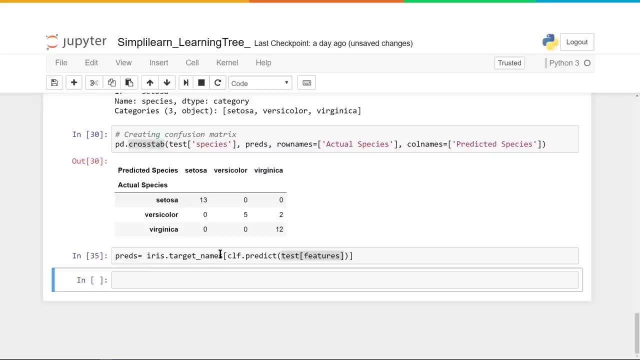 I don't know if you remember it, but predicts equals the iris dot target underscore names. So we're going to map it to the names and we're going to run the prediction and we read it on test features. But you know we're not just testing it. 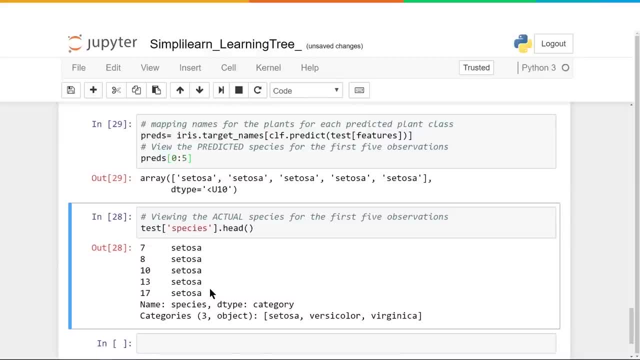 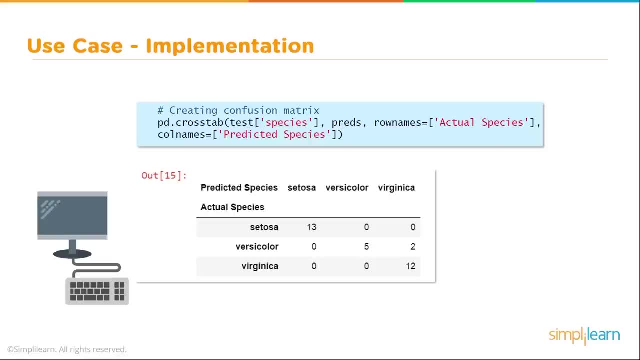 is How good it is at predicting the features. So that's where we come up to the next step, Which is lots of fun. We're going to use a single line of code to combine our predictions and our actuals, so we have a nice 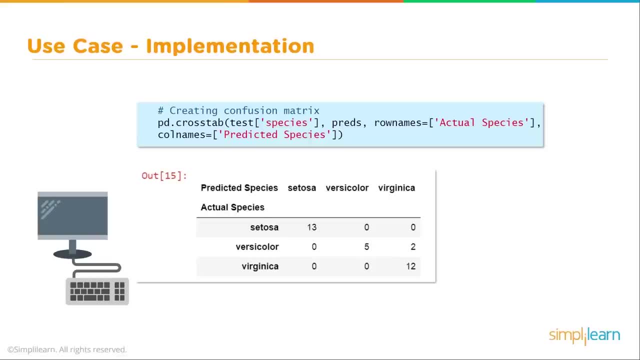 chart to look at. And let's go ahead and put that in our script, in our Jupyter Notebook here. Let's see, Let's go ahead and paste that in, And then I'm going to, because I'm on the Jupyter Notebook, I can do. 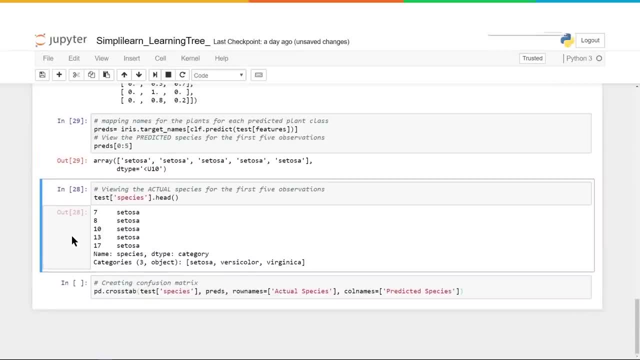 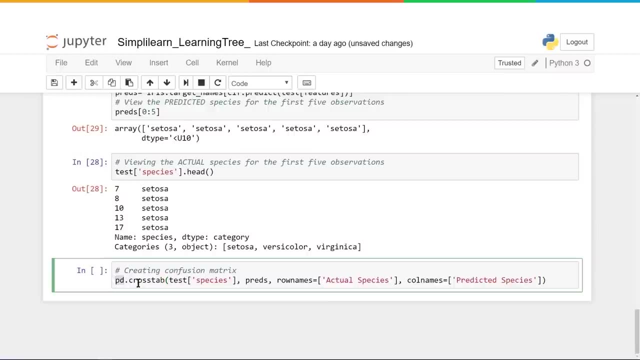 a control minus. You can see the whole line there. There we go, Resize it And let's take a look and see what's going on here. We're going to create in pandas- Remember, PD stands for pandas- And we're doing a crosstab. 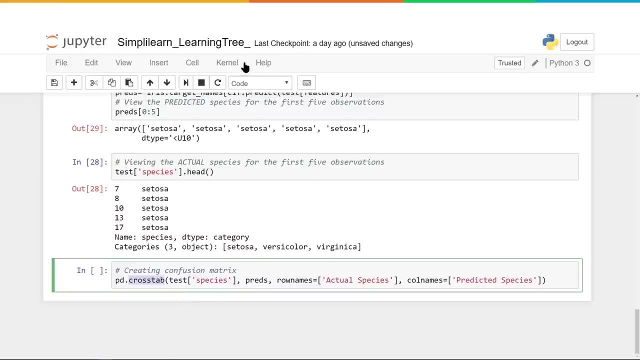 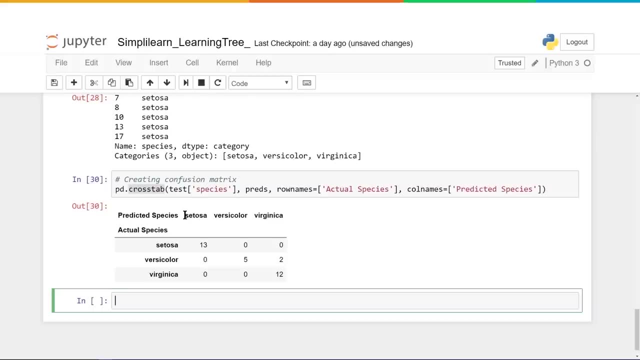 This function takes two sets of data and creates a chart out of them. So when I run it you'll get a nice chart down here And we have the predicted species. So across the top you'll see the setosa versicolor virginica. 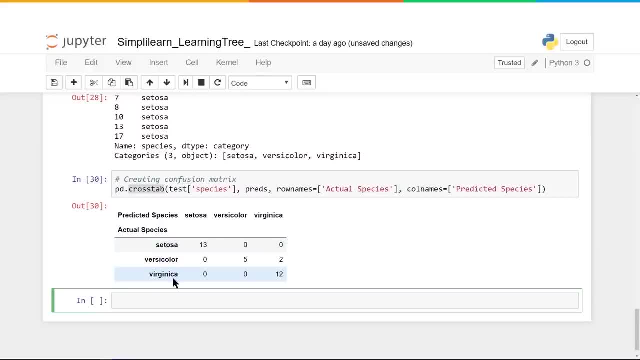 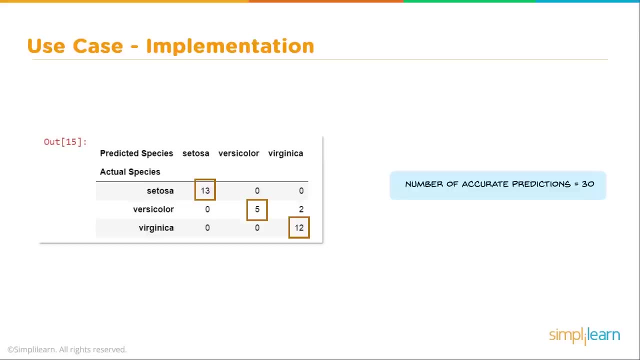 And the actual species, Setosa versicolor virginica. And so the way to read this chart, and let's go ahead and take a look on how to read this chart here: When you read this chart, you have setosa where they meet, You have versicolor where they meet. 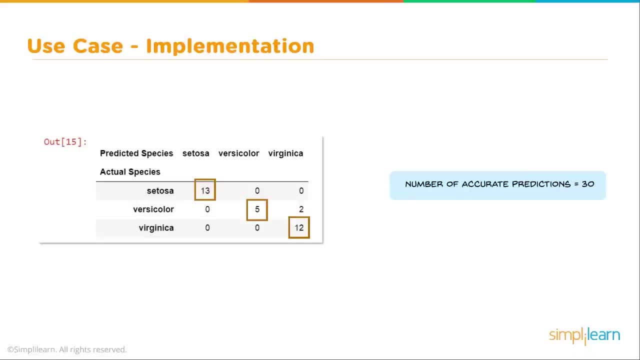 And you have virginica where they meet And they're meeting where the actual and the predicted agree. So this is the number of accurate predictions. So in this case it equals 30. If you add 13 plus 5 plus 12, you get 30.. 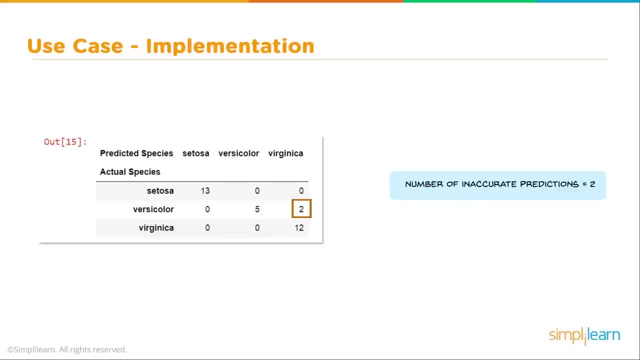 And then we notice here where it says virginica, but it was supposed to be versicolor. This is inaccurate. So now we have two: Two inaccurate predictions and 30 accurate predictions. So we'll say that the model accuracy is 93. That's just 30 divided by 32.. 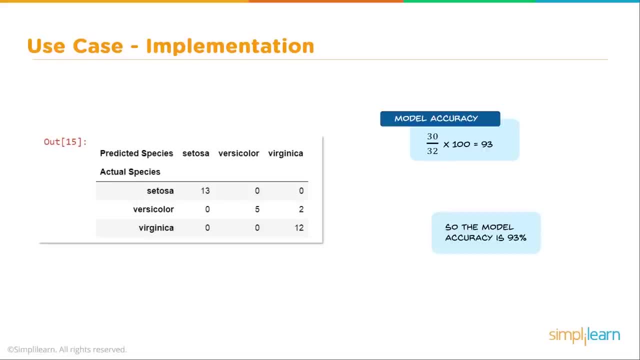 And if we multiply it by 100, we can say that it is 93% accurate. So we have a 93% accuracy with our model. I did want to add one more quick thing in here on our scripting before we wrap it up. 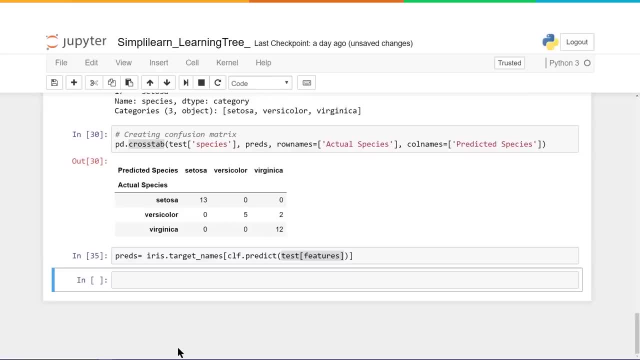 So let's flip back on over to my script. In here we're going to take this line of code from up above, Remember it. But predicts equals the iris dot target underscore names. So we're going to map it to the names And we're going to run the prediction. 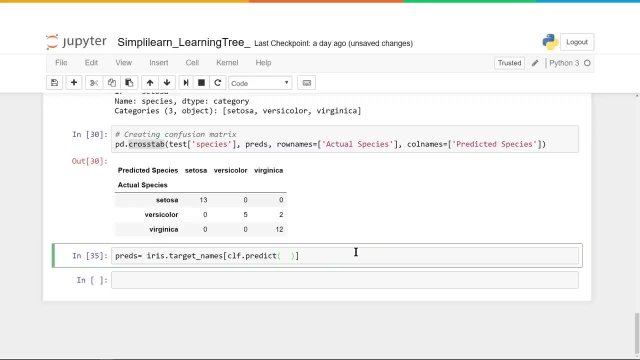 And we ran it on test features. But you know, we're not just testing it, We want to actually deploy it. So at this point I would go ahead and change this, And this is an array of arrays. This is really important when you're running these. 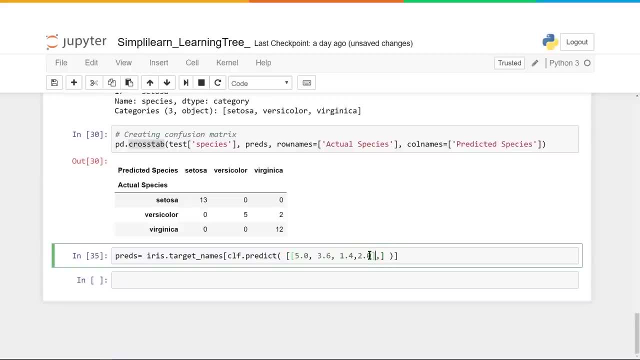 to know that. So you need the double brackets, And that could actually create data. Let's just do two flowers And we'll put two flowers in here, And then I actually want to see what the answer is. So let's go ahead and type in. 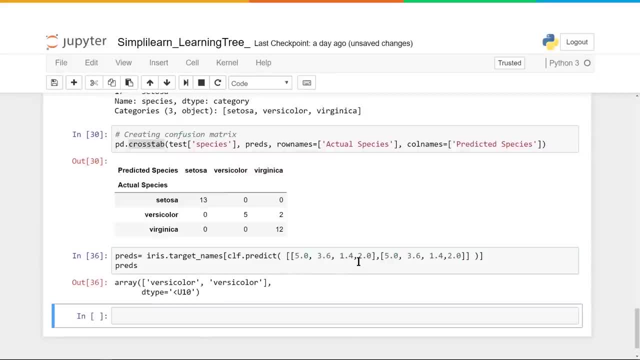 preds and print that out, And when I run this you'll see that I've now predicted two flowers that maybe I measured in my front yard as versicolor and versicolor- Not surprising, since I put the same data in for each one. This would be the actual. 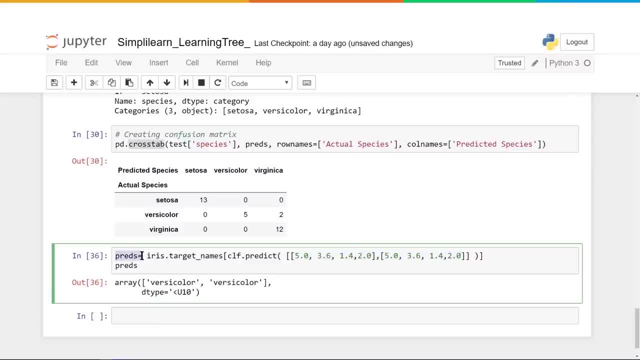 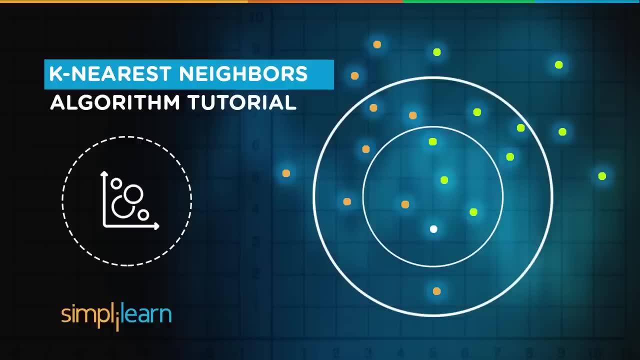 end product going out to be used on data that you don't know the answer for. So that's going to conclude our scripting part of this. Today we're going to cover the K nearest neighbors, a lot referred to as KNN, And KNN is really a. 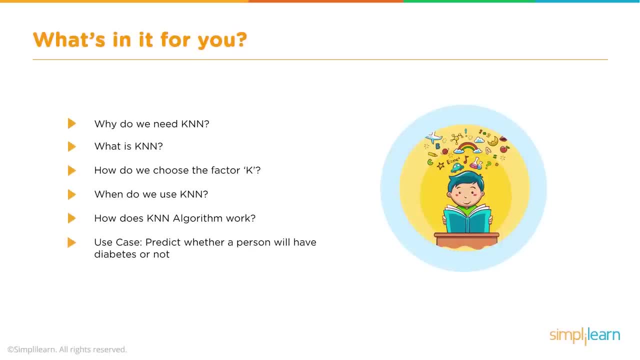 fundamental place to start in the machine learning. It's the basis of a lot of other things and just the logic behind it is easy to understand and incorporate it in other forms of machine learning. So today, what's in it for you? Why do we need KNN? 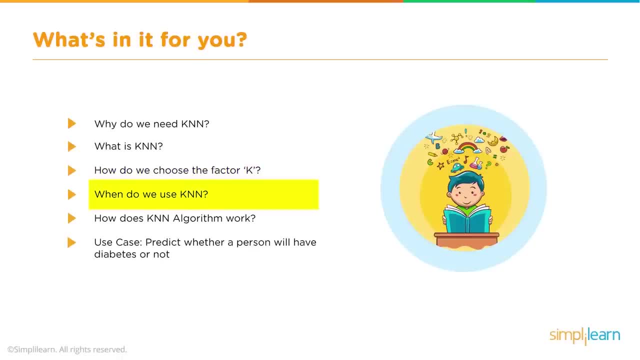 What is KNN? How do we choose the factor K? Why do we use KNN? How does KNN algorithm work? And then we'll dive into my favorite part, the use case: Predict whether your person will have diabetes or not. That is a very common 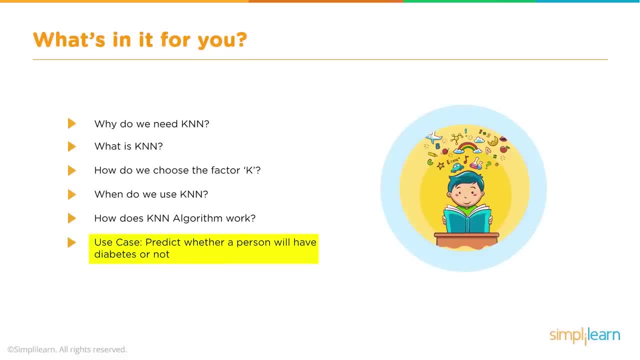 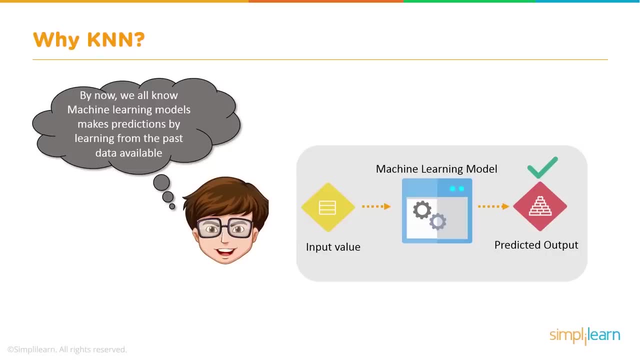 and popular used data set. as far as testing out models and learning how to use the different models in machine learning, By now we all know machine learning models make predictions by learning from the past data available. So we have our input values. our machine learning model builds on those. 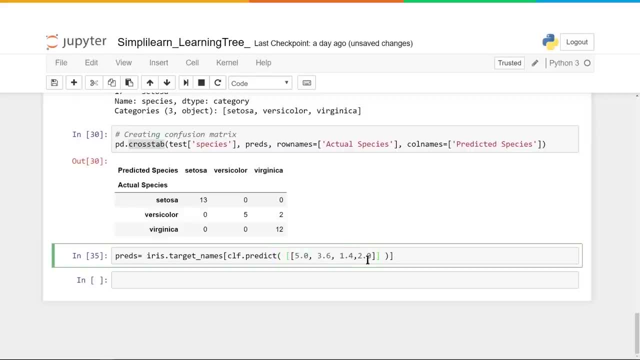 We want to actually deploy it. So at this point I would go ahead and change this, And this is an array of arrays. This is really important when you're running these to know that. so you need the double brackets and I could actually create data. 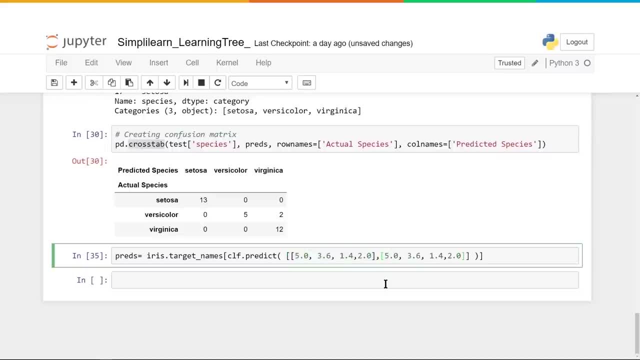 Maybe let's just do two flowers. So maybe I'm processing more data coming in and we'll put two flowers in here, And then I actually want to see what the answer is. So let's go ahead and type in Preds and print that out. 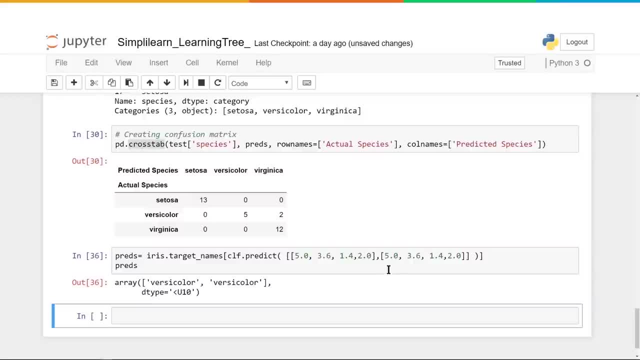 And when I run this, you'll see that I've now predicted two flowers that maybe I measured in my front yard as Versicolor and Versicolor- Not surprising, since I put the same data in for each one. This would be the actual end product going out to be used. 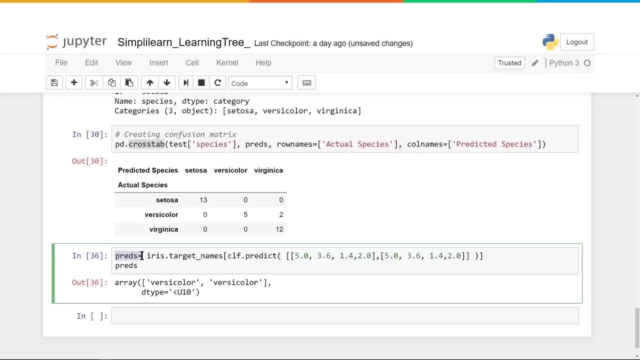 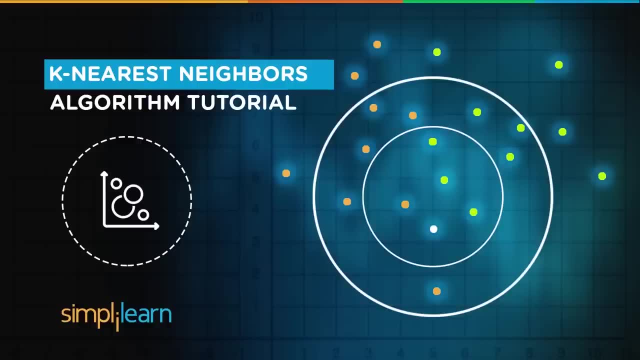 on data that you don't know the answer for. So that's going to conclude our scripting part of this. Today we're going to cover the K-nearest neighbors, a lot referred to as K-N-N, And K-N-N is really a fundamental place to start in the machine learning. 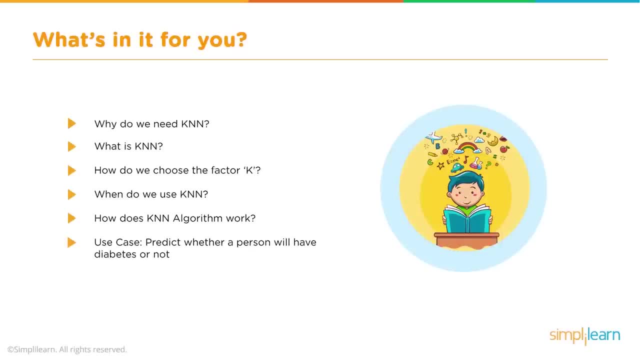 It's a basis of a lot of other things, And just the logic behind it is easy to understand and incorporate it in other forms of machine learning. So, today, what's in it for you? Why do we need K-N-N? What is K-N-N? 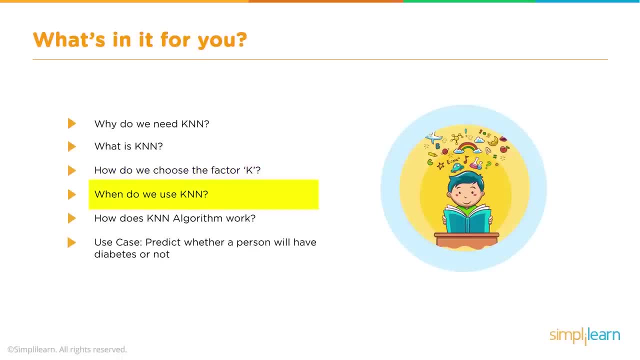 How do we choose the factor K? When do we use K-N-N? How does K-N-N algorithm work? And then we'll dive in to my favorite part: the use case Predict whether a person will have diabetes or not. That is a very common and popular used data set. as far as testing out models, 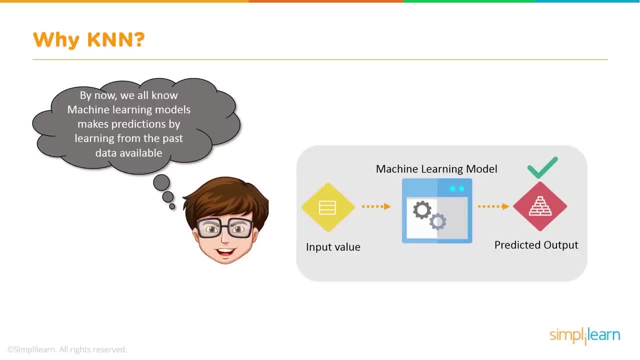 and learning how to use the different models in machine learning. By now we all know machine learning models make predictions by learning from the past data available. So we have our input values. Our machine learning model builds on those inputs of what we already know. 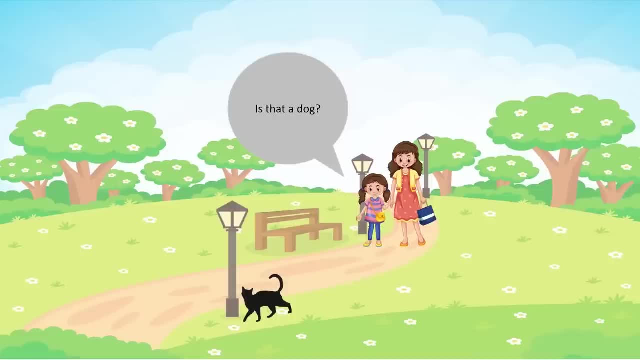 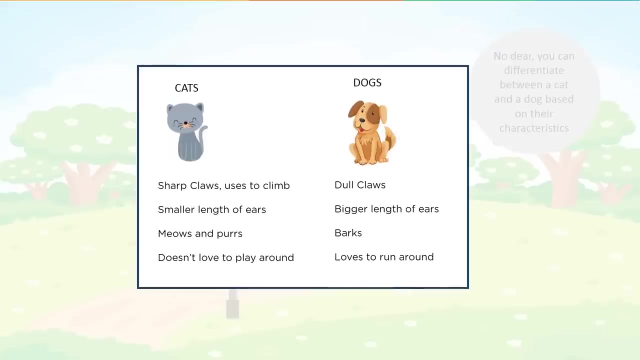 And then we use that to create a predicted output. Is that a dog? Little kid looking over there and watching the black cat cross their path? No dear, You can differentiate between a cat and a dog based on their characteristics: Cats- Cats have sharp claws. uses to climb. 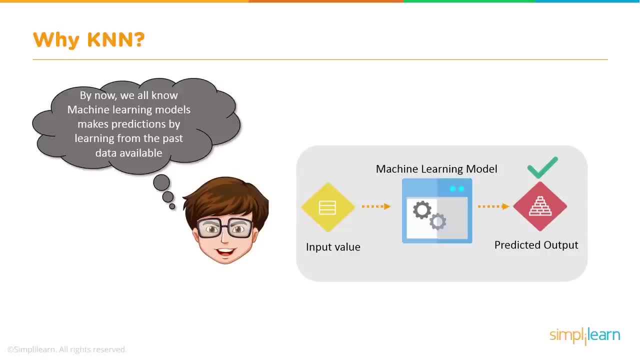 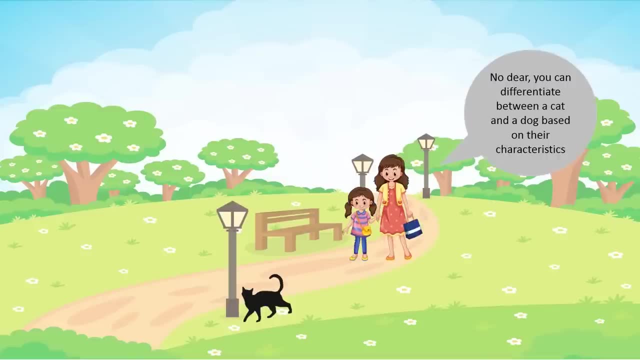 outputs of what we already know and then we use that to create a predicted output. Is that a dog? Little kid looking over there watching the black cat cross their path? No dear, you can differentiate between a cat and a dog based on their characteristics. 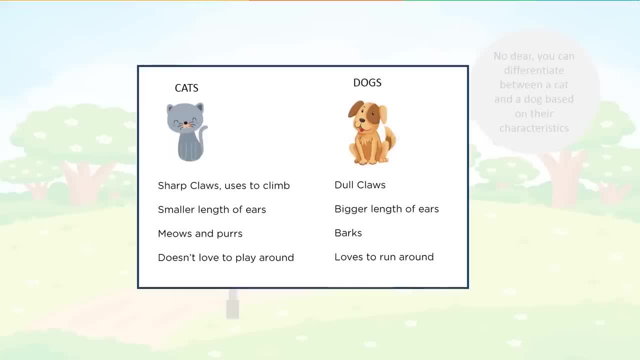 Cats: Cats have sharp claws, uses to climb, smaller length of ears, meows and purrs. doesn't love to play around. Dogs have dull claws, bigger length of ears, barks. loves to run around. I don't see a cat running around people. 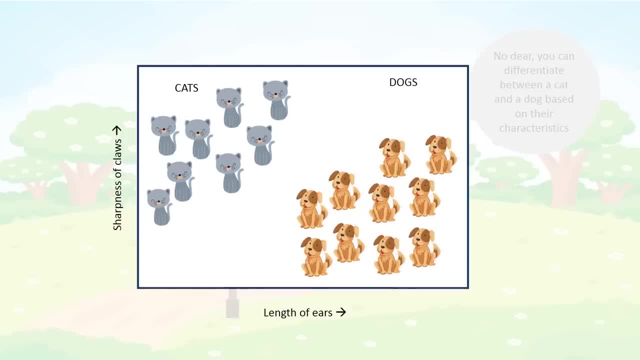 although I do have a cat that does that- where dogs do, And we can look at these and we can evaluate the sharpness of the claws- how sharp are their claws? and we can evaluate the length of the ears, and we can usually sort out cats from dogs based on even those. 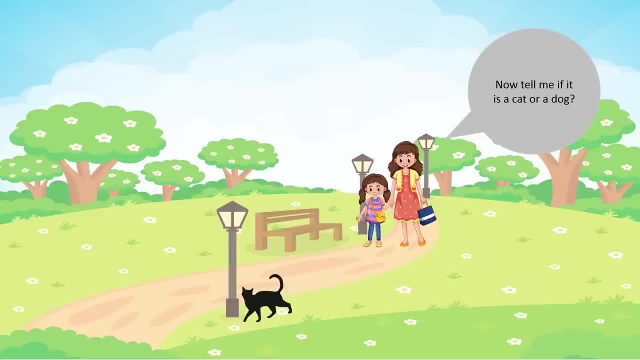 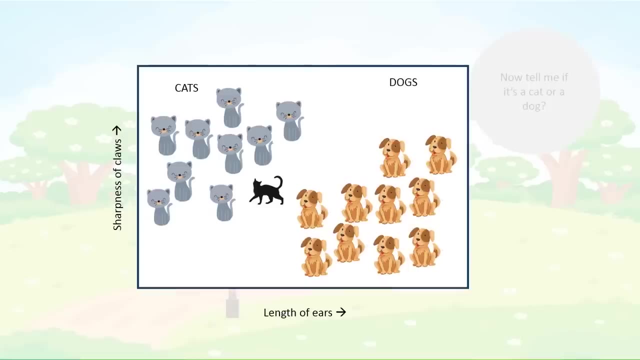 two characteristics. Now tell me if it is a cat or a dog. Odd question. usually little kids know cats and dogs by now, Unless they live in a place where there's not many cats or dogs. So if we look at the sharpness of the claws, 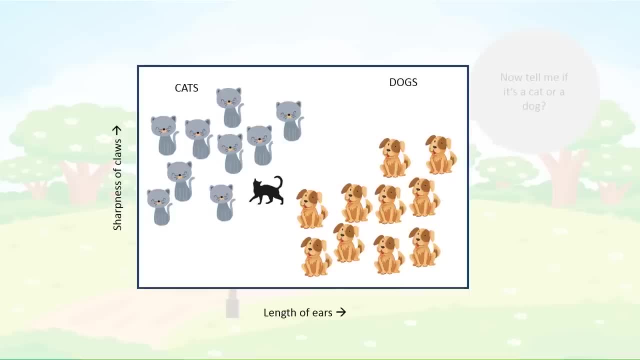 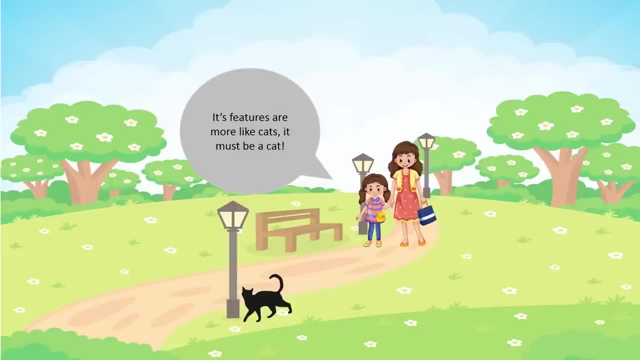 the length of the ears and we can see the cat has smaller ears and sharper claws than the other animals. Its features are more like cats. it must be a cat: Sharp claws, length of ears- and it goes in the cat group. Because KNN is based on 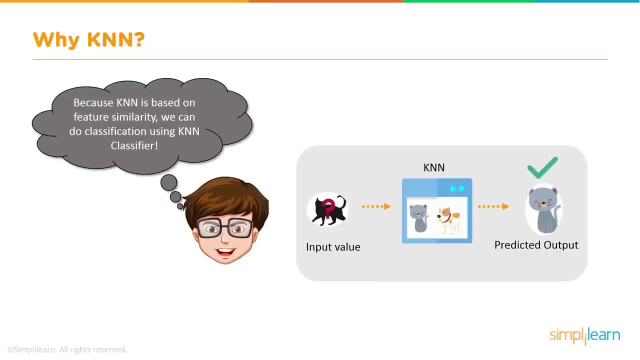 feature similarity. we can do classification using KNN classifier. So we have our input value, the picture of the black cat. it goes into our trained model and it predicts that this is a cat coming out. So what is KNN? What is the KNN algorithm? 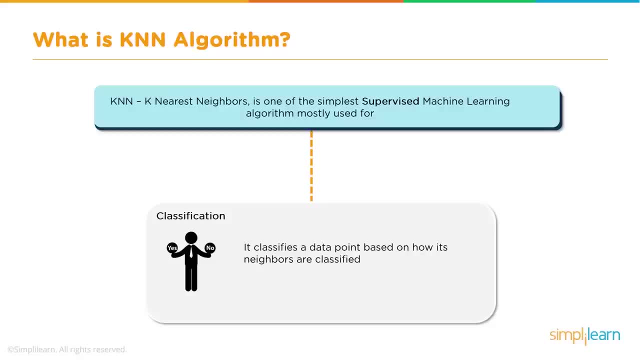 KNN nearest neighbors is what that stands for. It's one of the simplest supervised machine learning algorithms mostly used for classification. So we want to know: is this a dog or it's not a dog? Is it a cat or not a cat? 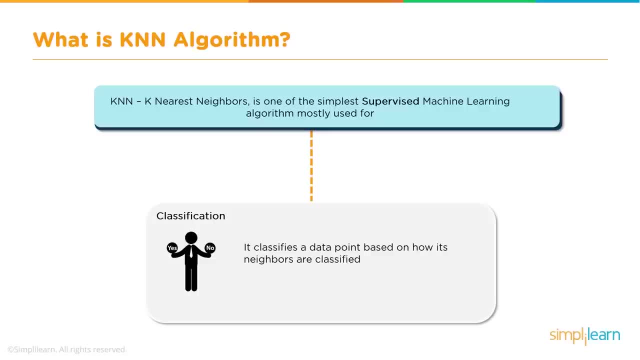 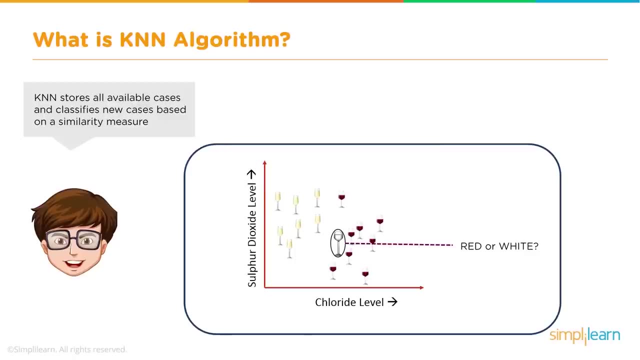 It classifies a data point based on how its neighbors are classified- KNN stores all available cases- and classifies new cases based on a similarity measure. And here we've gone from cats and dogs right into wine, another favorite of mine: KNN stores- all available cases. 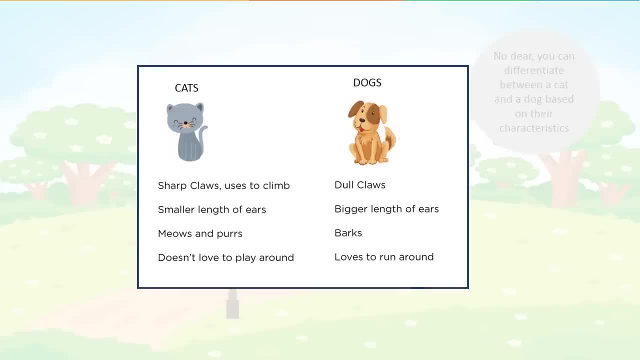 smaller length of ears, meows and purrs. doesn't love to play around. Dogs have dull claws. bigger length of ears. barks. loves to run around. You usually don't see a cat running around people, Although I do have a cat that does that where dogs do. 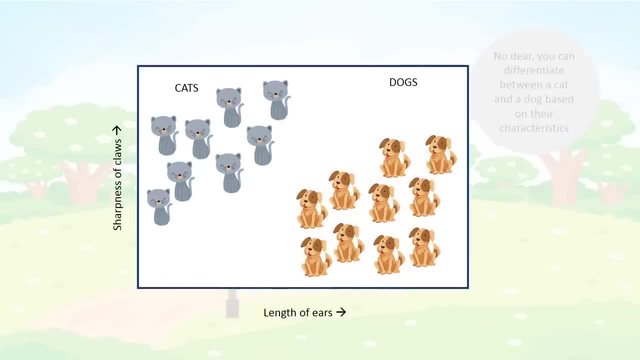 And we can look at these. We can say we can evaluate the sharpness of the claws- how sharp are their claws? and we can evaluate the length of the ears And we can usually sort out cats from dogs based on even those two characteristics. 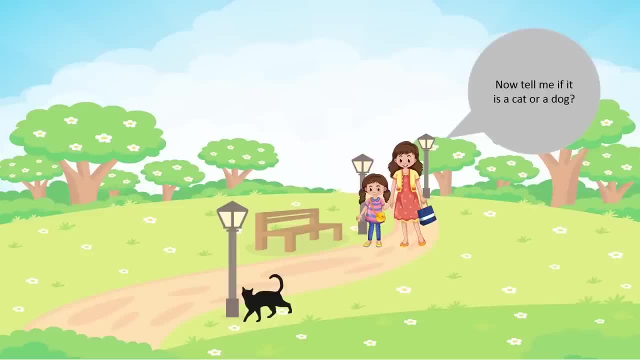 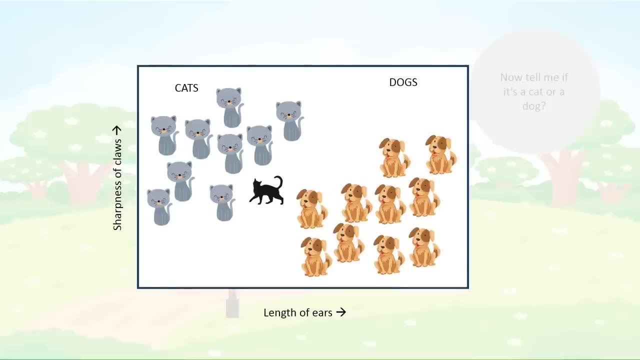 Now tell me if it is a cat or a dog, And I'd question. usually little kids know cats and dogs by now, Unless they live in a place where there's not many cats or dogs. So if we look at the sharpness of the claws, the length of the ears, 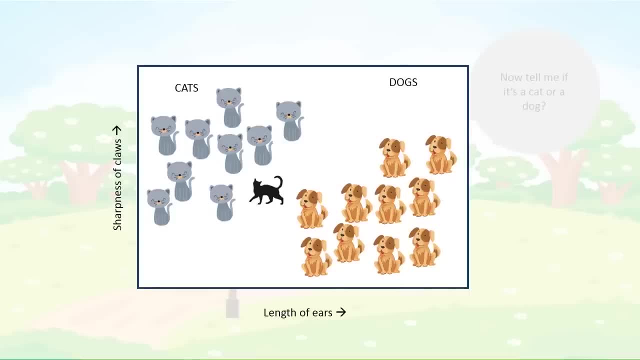 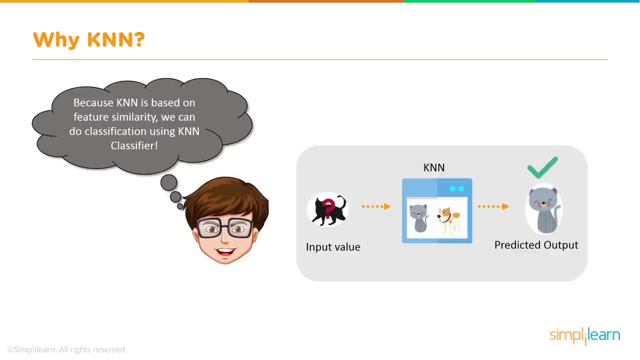 and we can see that the cat has smaller ears and sharper claws than the other animals. Its features are more like cats. It must be a cat- Sharp claws, length of ears- and it goes in the cat group. Because KNN is based on feature similarity, we can do classification using KNN classifier. 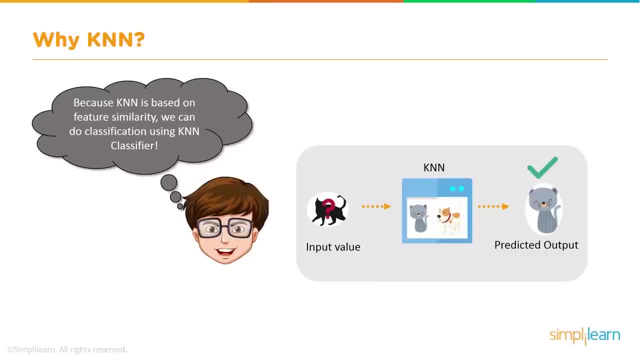 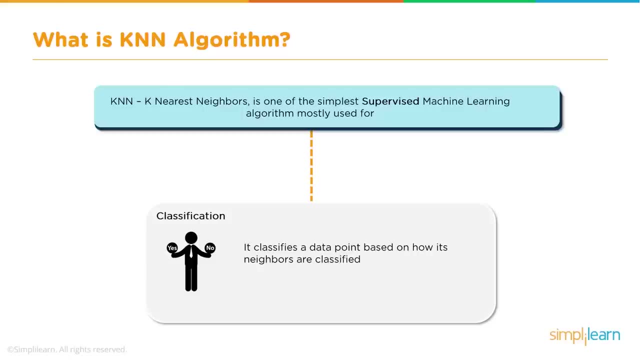 So we have our input value. This is the picture of the black cat. It goes into our trained model and it predicts that this is a cat coming out. So what is KNN? What is the KNN algorithm? K nearest neighbors is what that stands for. 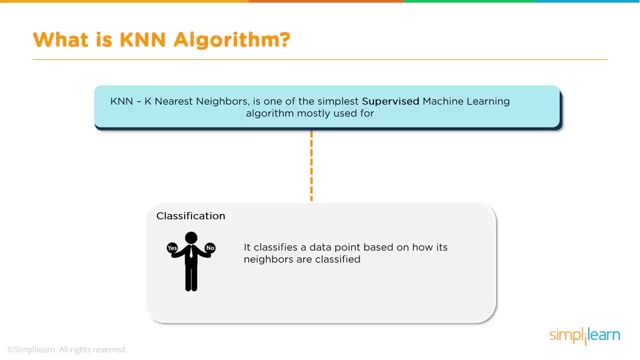 It's one of the simplest supervised machine learning algorithms mostly used for classification. So we want to know: is this a dog or it's not a dog? Is it a cat or not a cat? It classifies a data point based on how its neighbors are classified. 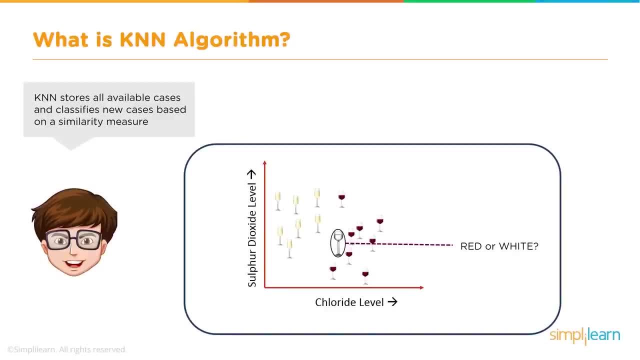 KNN stores all available cases and classifies new cases based on a similarity measure. And here we've gone from cats and dogs right into wine, another favorite of mine. KNN stores all available cases and classifies new cases based on a similarity measure. 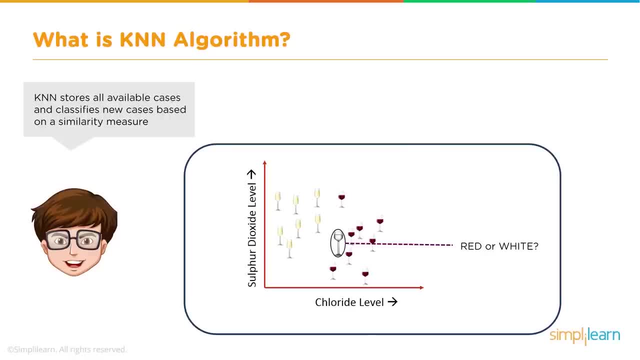 And here you see, we have a measurement of sulfur dioxide versus the chloride level and then the different wines they've tested and where they fall on that graph, based on how much sulfur dioxide and how much chloride. K in KNN is a perimeter that refers to the number of nearest neighbors to include. 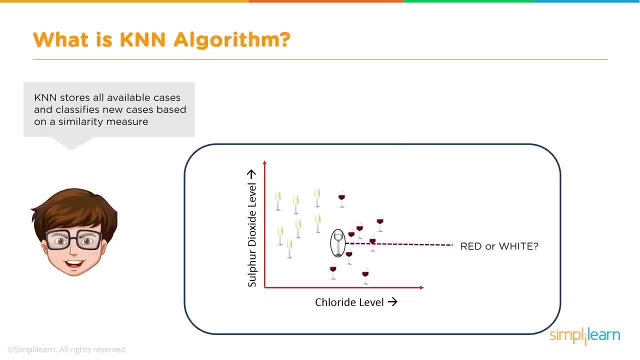 and classifies new cases based on a similarity measure. And here you see, we have a measurement of sulfur dioxide versus the chloride level and then the different wines they've tested and where they fall on that graph, based on how much sulfur dioxide and how much chloride. 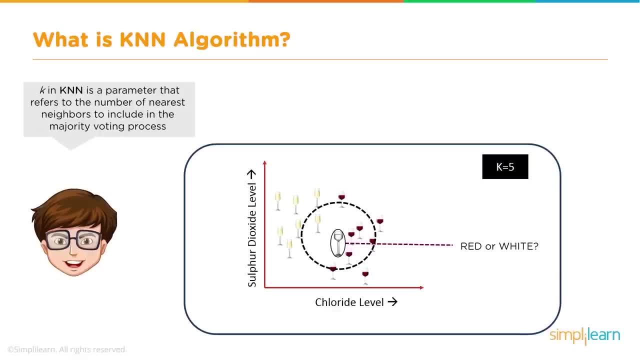 KNN is a perimeter that refers to the number of nearest neighbors to include in the majority of the voting process, And so if we had a new glass of wine there- red or white- we want to know what the neighbors are. In this case, we're going to put K equals 5.. 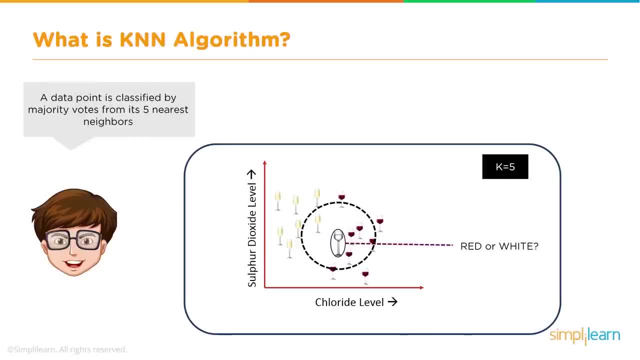 We'll talk about K in just a minute. A data point is classified by the majority of votes from its five nearest neighbors. Here, the unknown point would be classified as red, since four out of five neighbors are red. So how do we choose K? 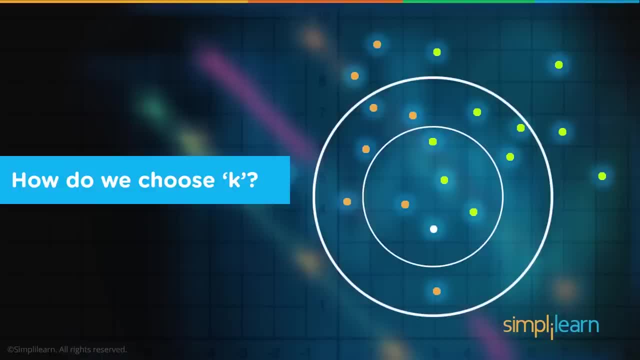 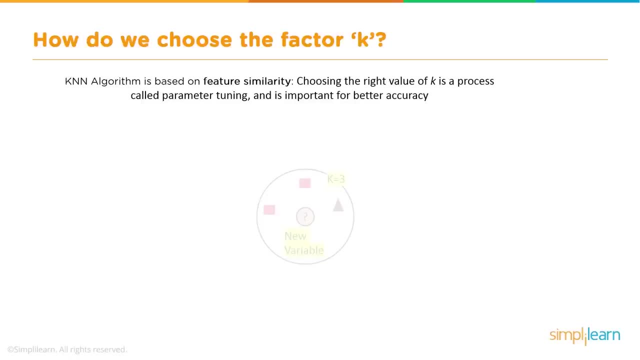 How do we know K equals 5? I mean, that was the value we put in there, so we're going to talk about it. How do we choose the factor K? KNN algorithm is based on feature similarity, Choosing the right value of K. 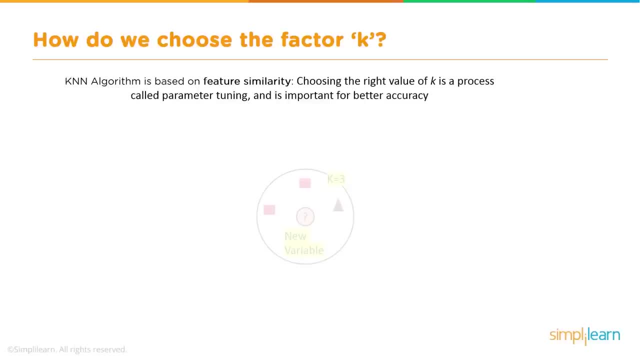 is a process called parameter tuning and is important for better accuracy. So at K equals 3, we can classify- we have a question mark in the middle- as either a square or not. Is it a square or is it, in this case, a triangle? And so if we set K equals to 3, 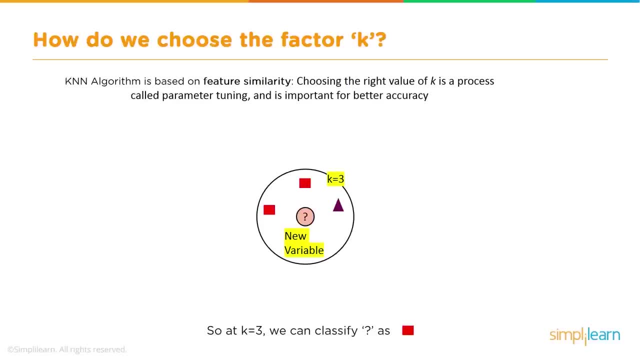 we're going to look at the three nearest neighbors. we're going to say this is a square And if we put K equals to 7, we classify as a triangle, depending on what the other data is around it And you can see as the K changes. 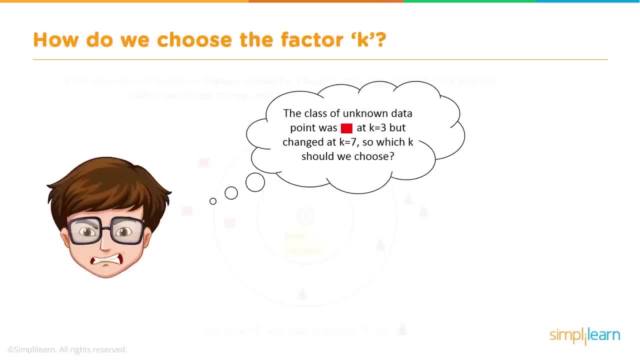 depending on where that point is. that drastically changes your answer And we jump here and we go. how do we choose the factor of K? You'll find this in all machine learning. When you look at factors, that's the face you get. It's like: oh my gosh, did I choose the right K? 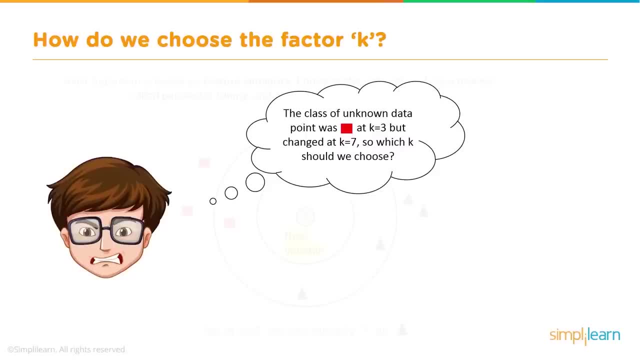 Did I set it right my values in whatever machine learning tool you're looking at, so that you don't have a huge bias in one direction or the other. And in terms of KNN- the number of K, if you choose it too low, the bias is based on. 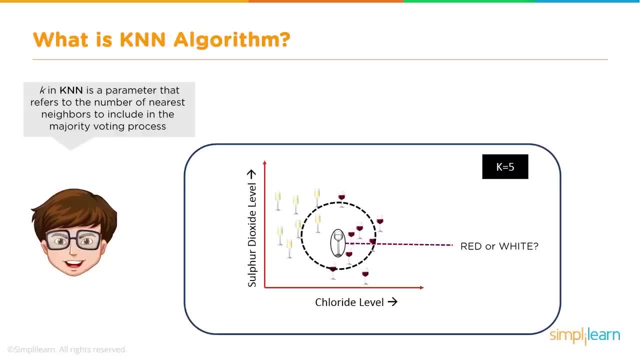 in the majority of the voting process, And so if we had a new glass of wine there, red or white, we want to know what the neighbors are. In this case, we're going to put K equals five. We'll talk about K in just a minute. 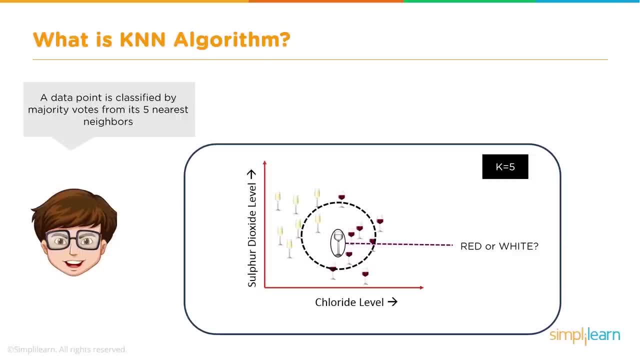 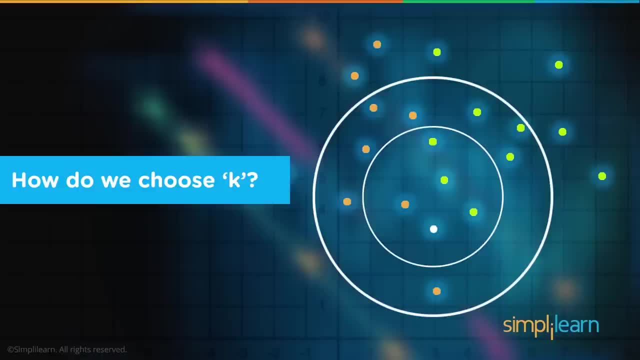 A data point is classified by the majority of votes from its five nearest neighbors. Here, the unknown point would be classified as red, since four out of five neighbors are red. So how do we choose K? How do we know K equals five? I mean, that was the value we put in there, so we're going to talk about it. 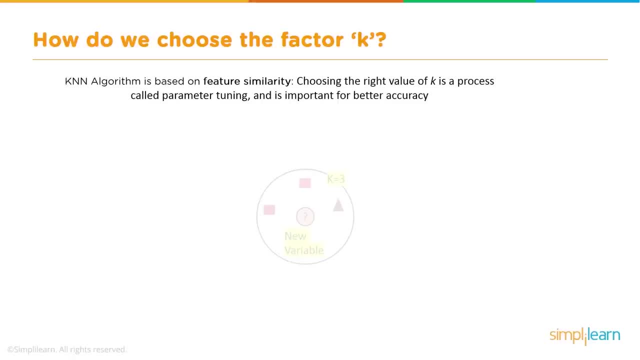 How do we choose the factor K? KNN algorithm is based on feature similarity. Choosing the right value of K is a process called parameter tuning and is important for better accuracy. So at K equals three, we can classify. we have a question mark in the middle. 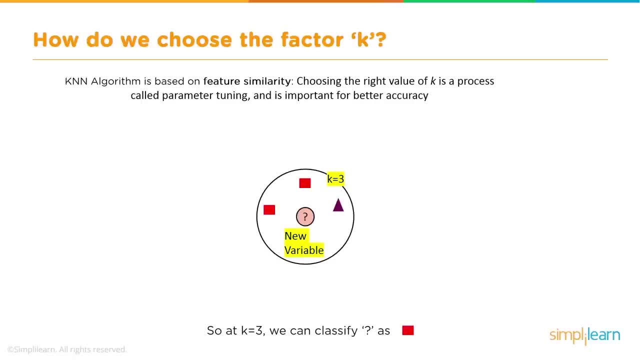 as either a square or not. Is it a square or is it, in this case, a triangle? And so if we set K equals to three, we're going to look at the three nearest neighbors. We're going to say: this is a square. 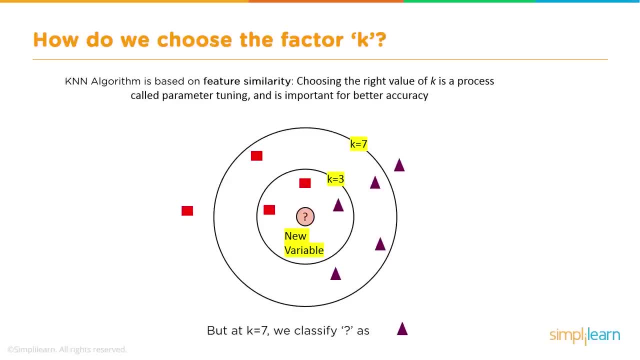 And if we put K equals to seven, we classify as a triangle depending on what the other data is around it And you can see as the K changes depending on where that point is. that drastically changes your answer And we jump. here we go. how do we choose the factor of K? 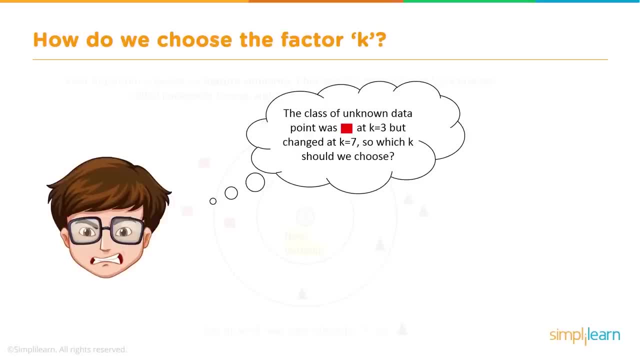 You'll find this in all machine learning. Choosing these factors, that's the face you get. It's like: oh my gosh, did I choose the right K? Did I set it right my values? in whatever machine learning tool you're looking at? 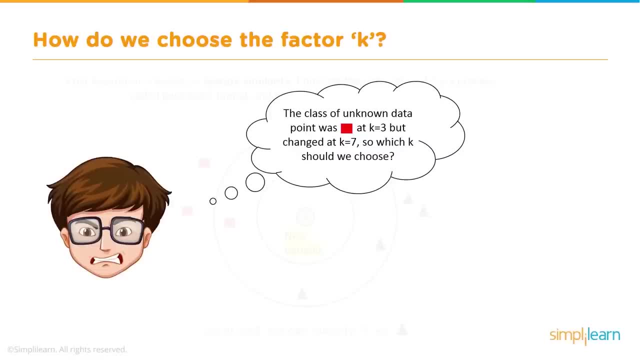 so that you don't have a huge bias in one direction or the other. And in terms of KNN, the number of K, if you choose it too low, the bias is based on. it's just too noisy, It's just right. next to a couple of things: 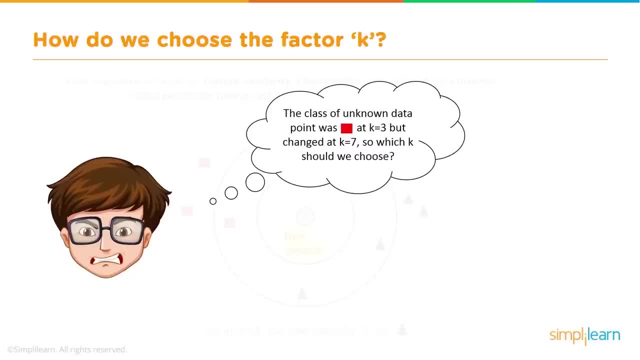 And it's going to pick those things and you might get a skewed answer And if your K is too big then it's going to take forever to process. So you're going to run into processing issues and resource issues. So what we do, the most common use- 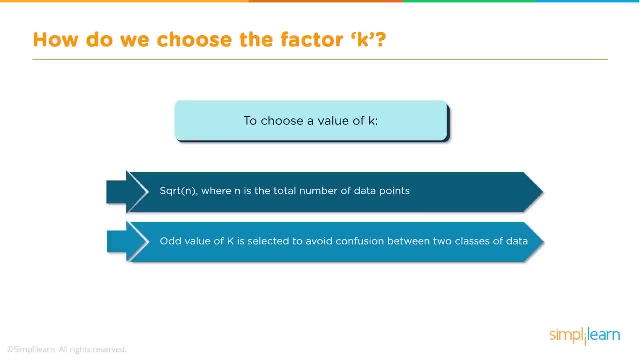 and there's other options for choosing. K is to use the square root of N. So it is a total number of values you have. You take the square root of it. In most cases you also if it's an even number. 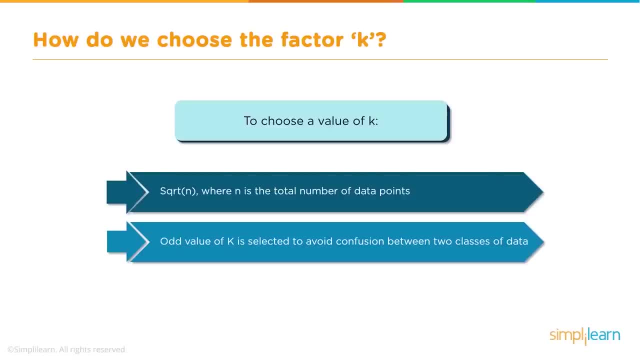 so if you're using, like in this case, squares and triangles, if it's even, you want to make your K value odd, That helps it select better. So, in other words, you're not going to have a balance between two different factors that are equal. 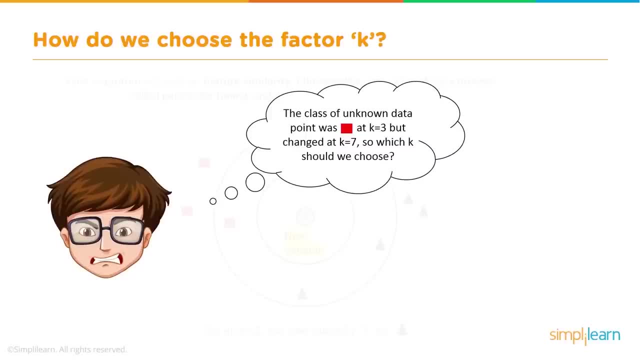 it's just too noisy. it's right next to a couple things and it's going to pick those things and you might get a skewed answer And if your K is too big you're going to have issues and resource issues. So what we do, the most common use. 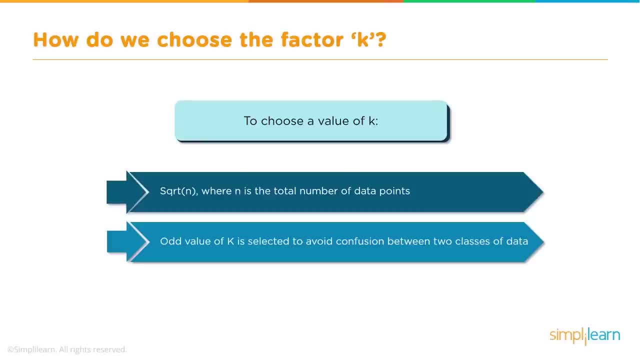 and there's other options for choosing. K is to use the square root of N. So N is the total number of values you have and you take the square root of it. In most cases you also if it's an even number. so if you're using squares and triangles, 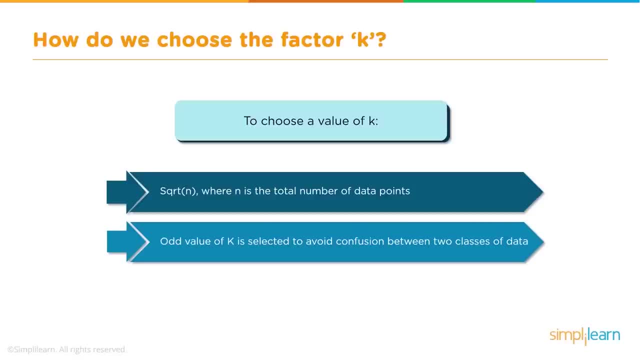 if it's even, you want to make your K value odd. That helps it select better. So in other words, you're not going to have a balance between two different factors that are equal. So usually take the square root of N and if it's even you, add one to it. 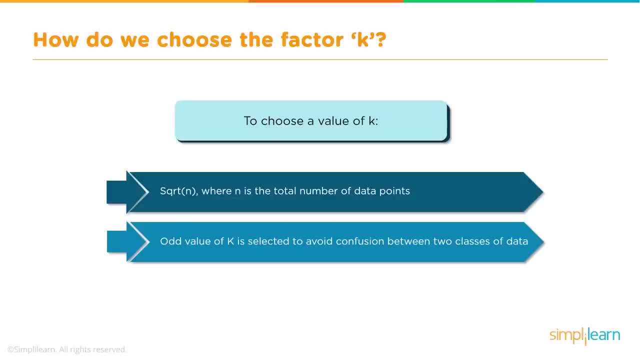 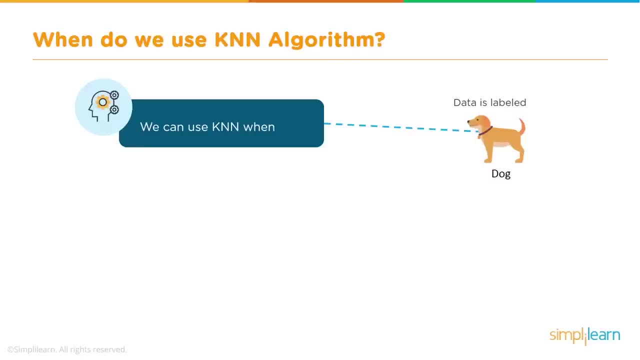 or subtract one from it, and that's where you get the K value from. That is the most common use and it's pretty solid. It works very well. When do we use KNN? We can use KNN when data is labeled, so you need a label on it. 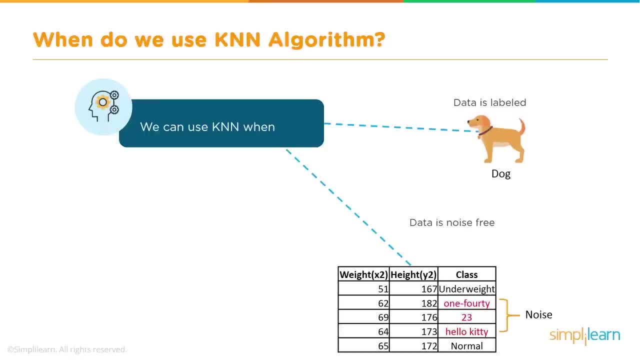 we know we have a group of pictures with dogs, dogs, cats, cats. Data is noise free and so you can see here when we have a class and we have, like, underweight 140,, 23,, hello, kitty, normal. that's pretty confusing. We have a high variety. 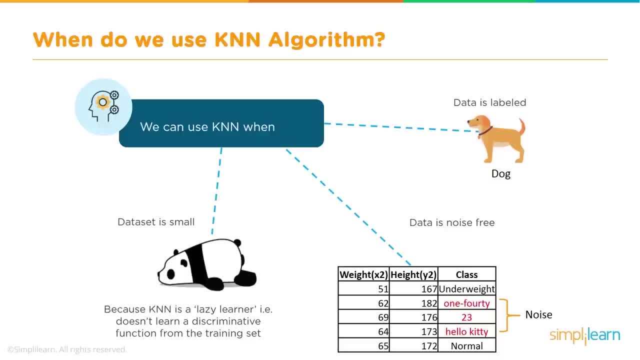 of K and N so it's very noisy and that would cause an issue. Data set is small, so we're usually working with smaller data sets where you might get into a gig of data if it's really clean, doesn't have a lot of noise because KNN is a lazy learner. 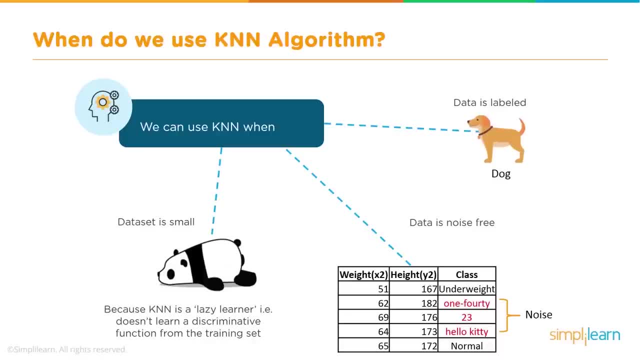 ie. it doesn't learn a discriminative function from the training set, so it's very lazy. so if you have very complicated data and you have a large amount of it, you're not going to use the KNN, but it's really great to get a place to start. 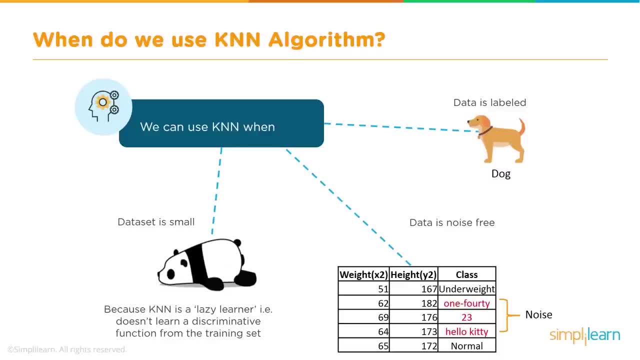 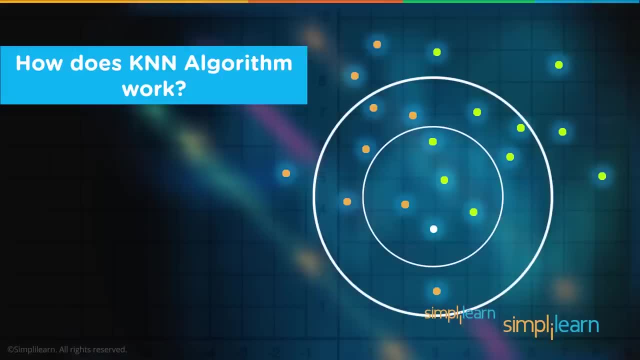 even with large data, you can sort out a small sample and get an idea of what that looks like and also just using for smaller data sets, KNN works really good. How does a KNN algorithm work? Consider a data set having two variables: height in centimeters and weight in. 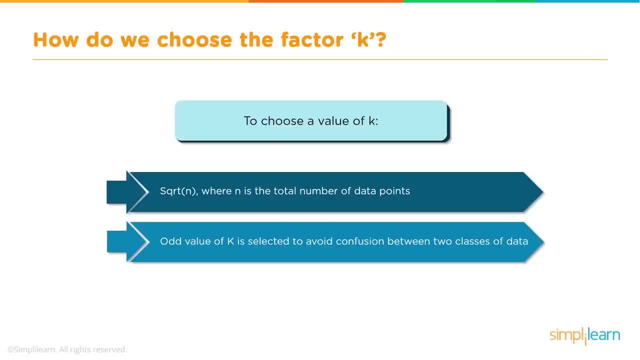 So usually take the square root of N And, if it's even you, add one to it or subtract one from it, And that's where you get the K value from. That is the most common use and it's pretty solid. It works very well. 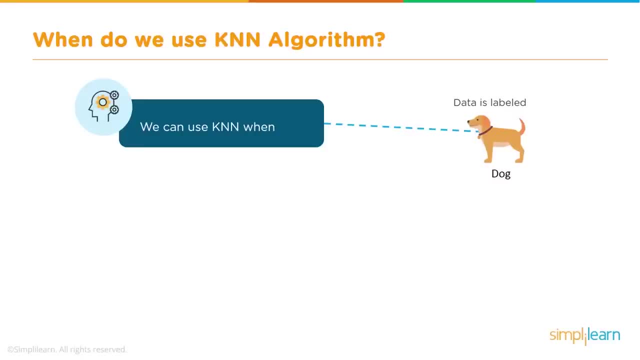 When do we use KNN? We can use KNN when data is labeled, So you need a label on it. We know we have a group of pictures with dogs, dogs, cats, cats. Data is noise free And so you can see here when we have a class and we have like underweight. 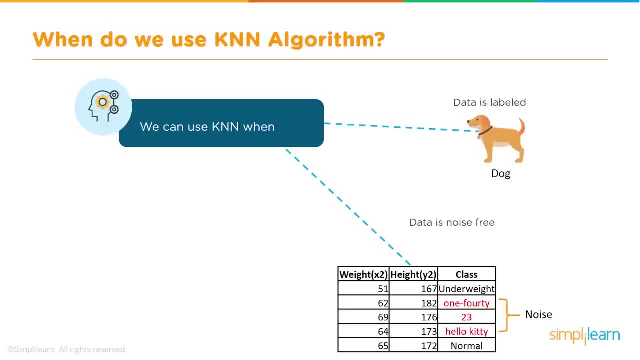 140, 23,. Hello Kitty, normal. that's pretty confusing. We have a high variety of data coming in So it's very noisy and that would cause an issue. Data set is small, So we're usually working with smaller data sets where you might get into a gig. 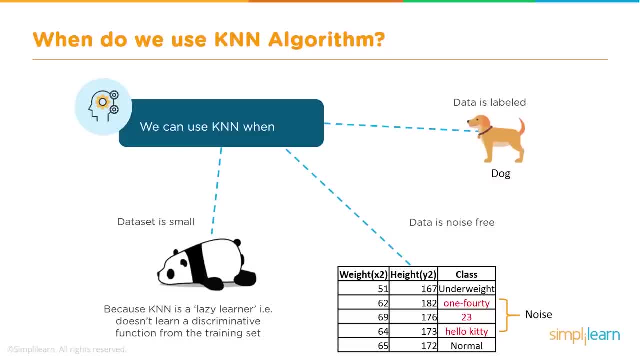 of data if it's really clean, doesn't have a lot of noise, Because KNN is a lazy learner, ie it doesn't learn a discriminative function from the training set, So it's very lazy. So if you have very 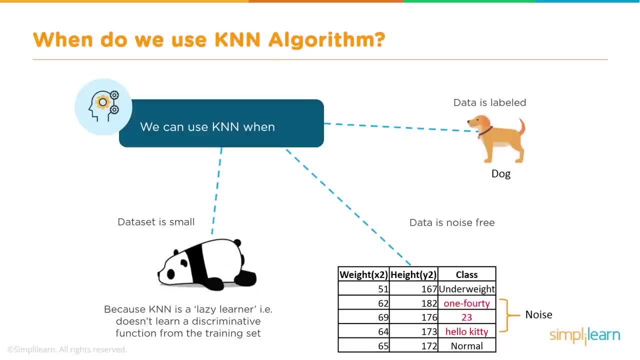 complicated data and you have a large amount of it. you're not going to use the KNN, but it's really great to get a place to start, Even with large data. you can sort out a small sample and get an idea of what that looks like, using the KNN and also just using for smaller data. 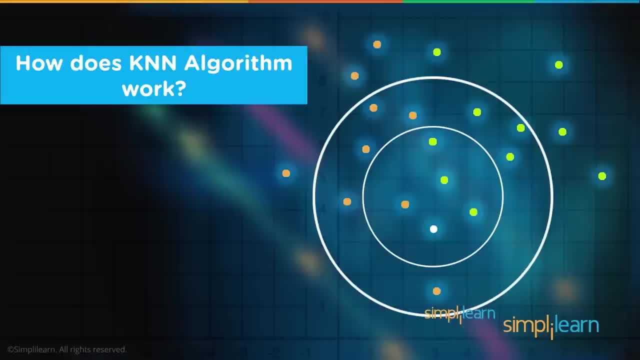 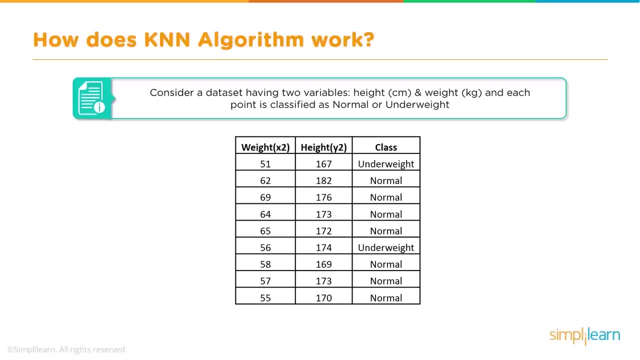 sets. KNN works really good. How does a KNN algorithm work? Consider a data set having two variables: height in centimeters and weight in kilograms, And each point is classified as normal or underweight. So we see, right here we have two variables. 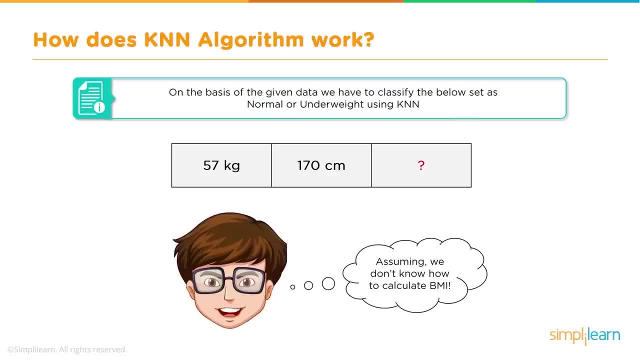 you know, true, false, or either normal or they're not, they're underweight. On the basis of the given data, we have to classify the below set as normal or underweight using KNN. So if we have new data coming in that says: 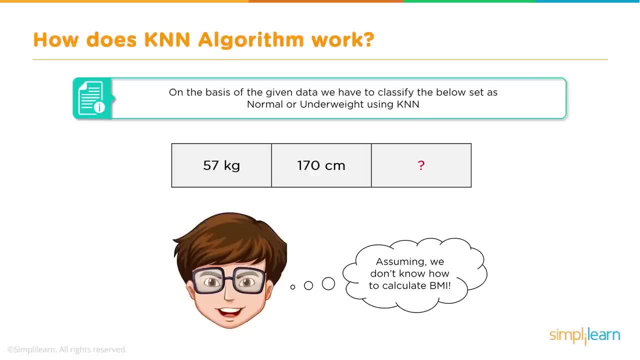 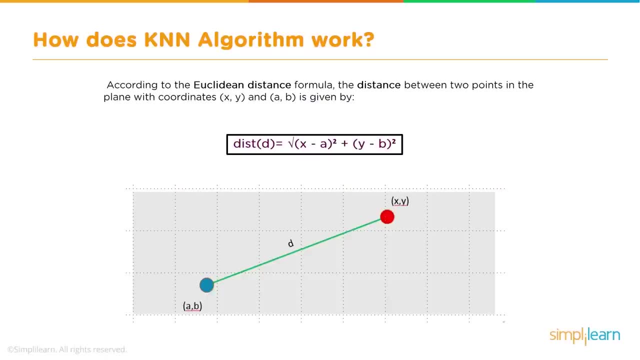 fifty seven kilograms and one hundred and seventy seven centimeters. is that going to be normal or underweight? To find the nearest neighbors, we'll calculate the Euclidean distance According to the Euclidean distance formula. the distance between two points in the plane with the coordinates X, Y and A B is given by: 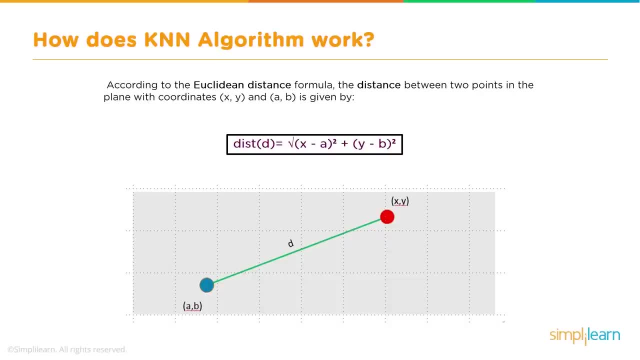 distance D equals the square root of X minus A squared, plus Y minus B squared, And you can remember that from the two edges of a triangle We're computing the third edge. since we know the X side and the Y side, Let's calculate it to understand clearly. 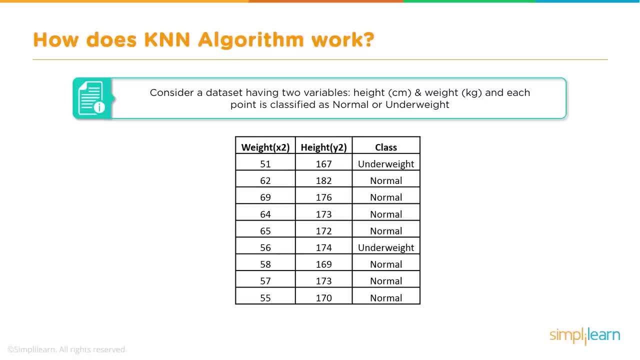 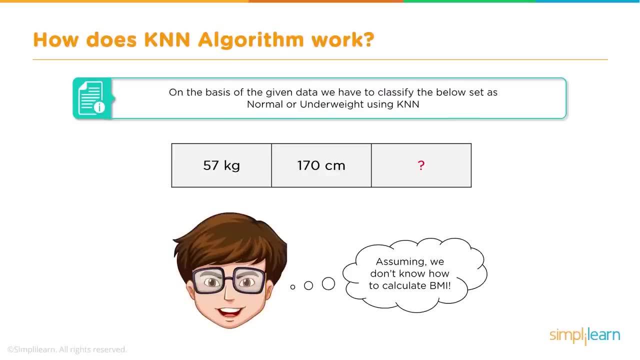 kilograms and each point is classified as normal or underweight. so we can see right here we have two variables: true, false. they're either normal or they're not. they're underweight. on the basis of the given data, we have to classify the below set. 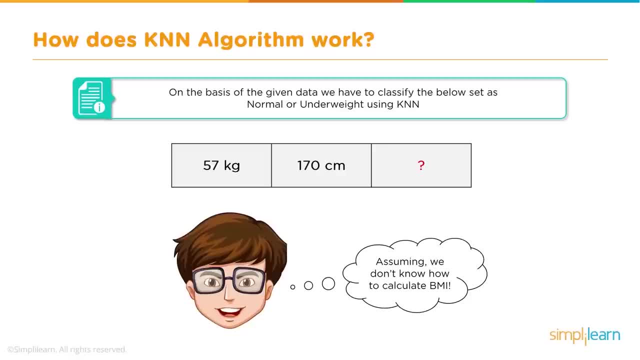 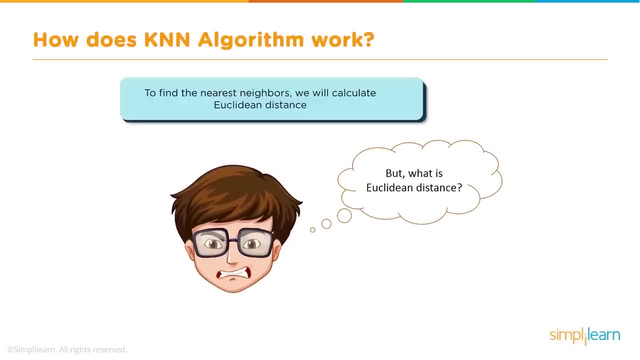 as normal or underweight using KNN. so if we have new data coming in that says 57 kilograms and 177 centimeters, is that going to be normal or underweight? to find the nearest neighbors, we'll calculate the Euclidean distance according to the Euclidean distance. 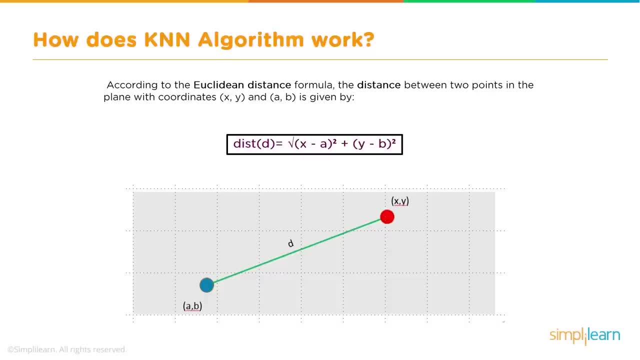 formula: the distance between two points in the plane with the coordinates is given by distance. d equals the square root of x minus a squared, plus y minus b squared. and you can remember that from the two edges of a triangle we're computing the third edge so that we know the x side. 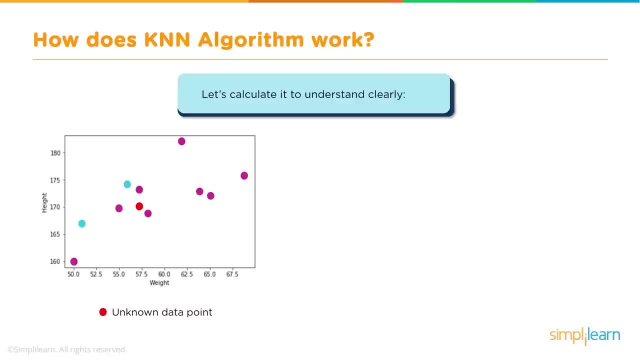 and the y side. let's calculate it to understand clearly. so we have our unknown point- we placed it there in red- and we have our other points where the data is scattered around the distance. d1 is the square root of 170 minus 167 squared, plus 57 minus 51 squared. 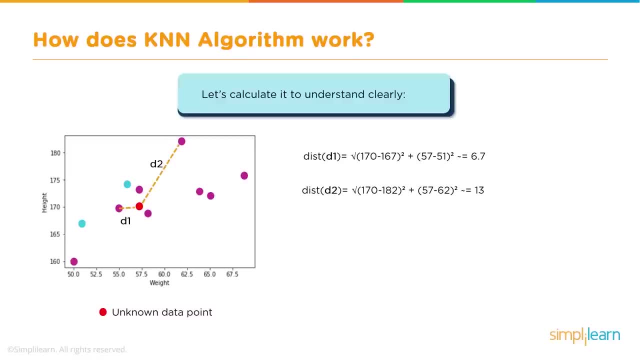 which is about 6.7, and distance 2 is about 13 and distance 3 is about 13.4. similarly, we will calculate the distance of unknown data point from all the points in the data set and because we're dealing with small amount of data, 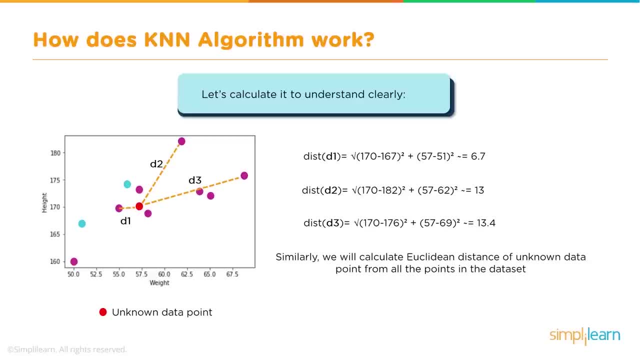 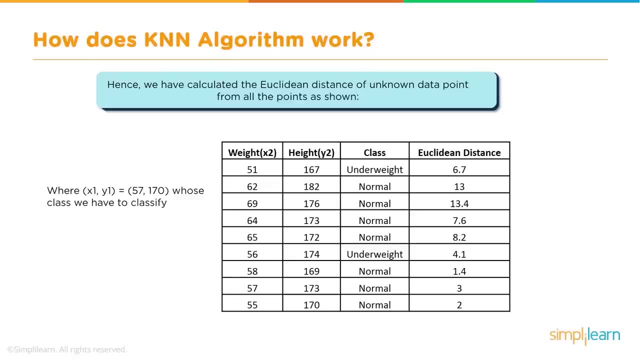 that's not that hard to do and it's actually pretty quick for a computer and it's not really complicated math. so you can just see how close is the data based on the Euclidean distance. hence we have calculated the Euclidean distance of unknown data point. 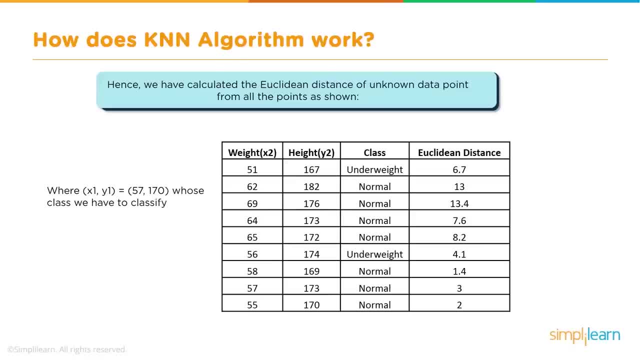 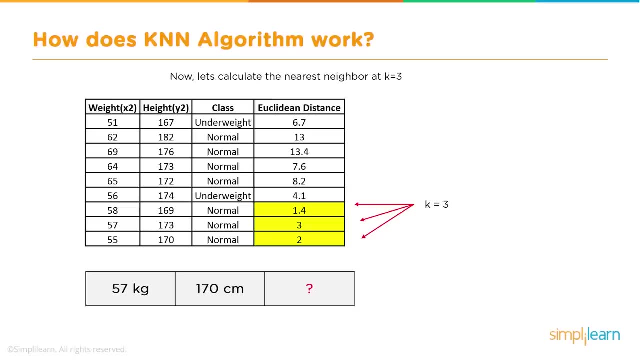 from all the points as shown, where x1 and y1 equal 57 and 170, whose class we have to classify. so now we're looking at that, we're saying, well, here's the Euclidean distance of neighbors. now let's calculate the nearest neighbor at: k equals 3. 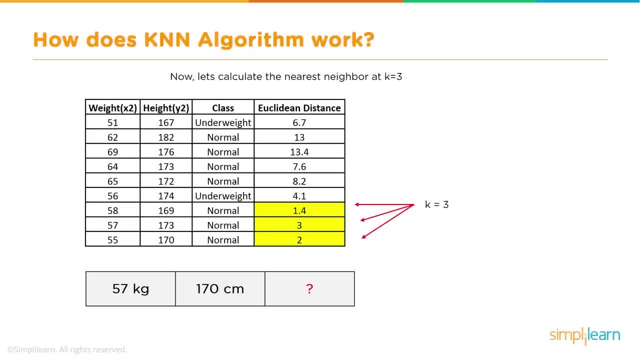 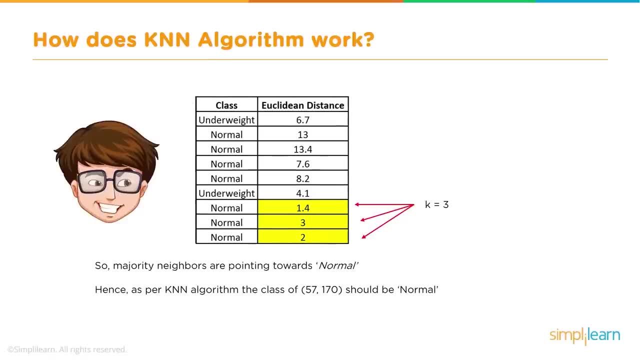 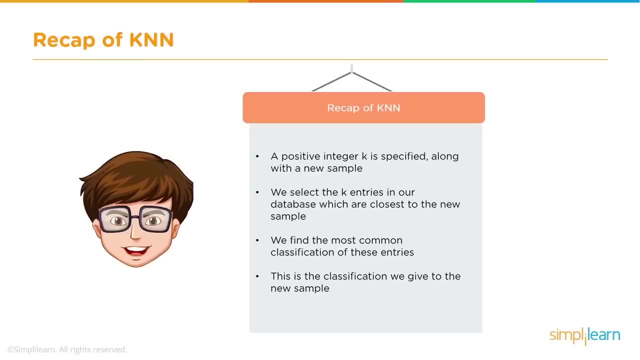 and we can see the three closest neighbors- puts them at normal and that's pretty self evident. when you look at this graph, it's pretty easy to say, okay, we're just voting normal, normal, normal. three votes for normal. this is going to be a normal weight, so majority of neighbors are pointing towards normal. 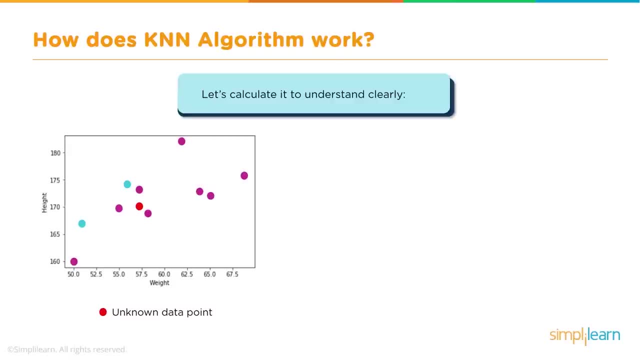 So we have our unknown point and we placed it there in red, and we have our other points where the data is scattered around The distance. D1 is a square root of one hundred and seventy minus one hundred and sixty seven squared, plus fifty seven minus fifty one squared, which is about six point seven. 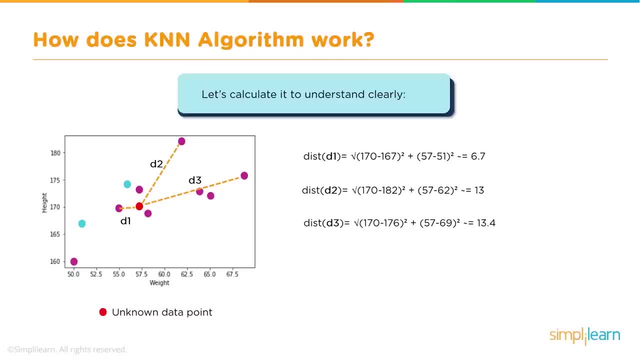 And distance two is about thirteen and distance three is about thirteen. point four: Similarly, we will calculate the Euclidean distance of unknown data point from all the points in the data set And because we're dealing with small amount of data, that's not that hard to do. 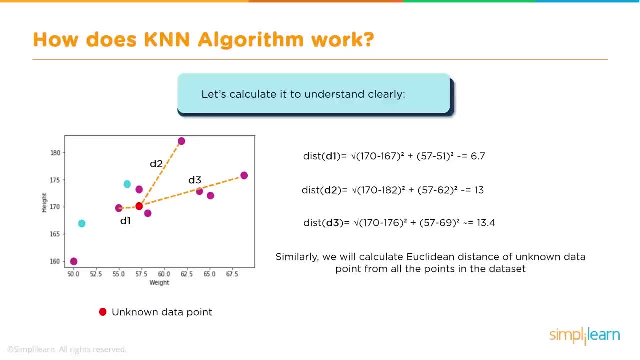 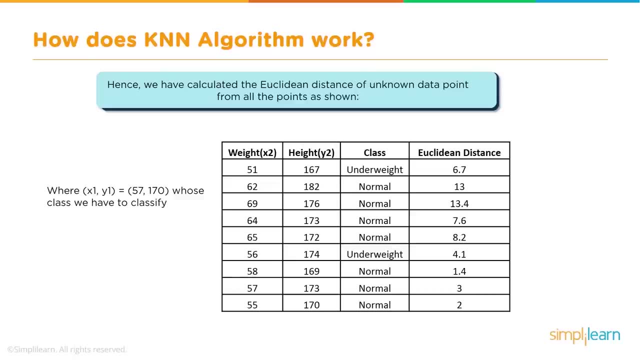 It's actually pretty quick for a computer and it's not really complicated math. You can just see how close is the data based on the Euclidean distance. Hence we have calculated the Euclidean distance of unknown data point from all the points as shown, where X1 and Y1 equal fifty seven and one hundred and seventy. 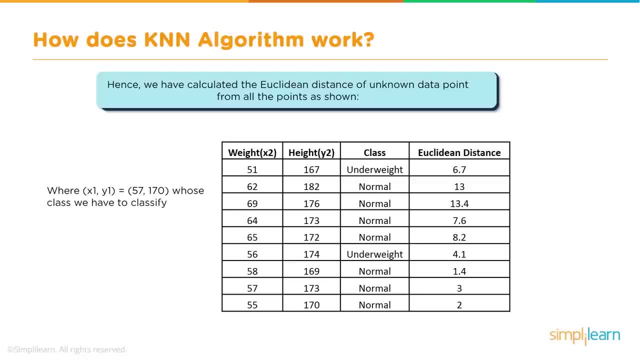 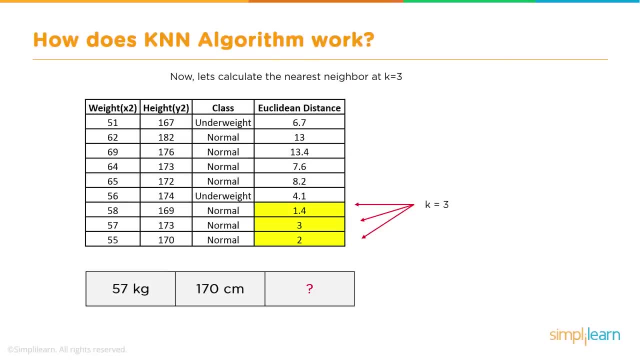 whose class we have to classify. So now we're looking at that, We're saying: well, here's the Euclidean distance. Who's going to be the closest neighbors? Now let's calculate the nearest neighbor at K equals three And we can see the three closest neighbors. puts them at normal. 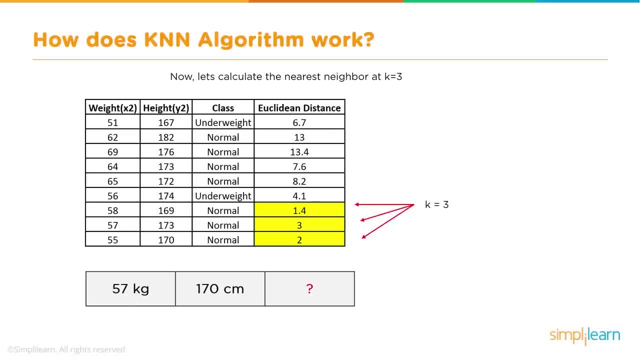 And that's pretty self-evident. When you look at this graph, it's pretty easy to say: OK, we're just voting Normal, normal, normal. three votes for normal. This is going to be a normal weight. So majority of neighbors are pointing. 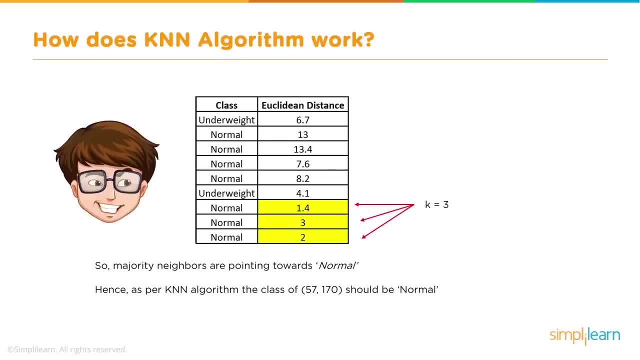 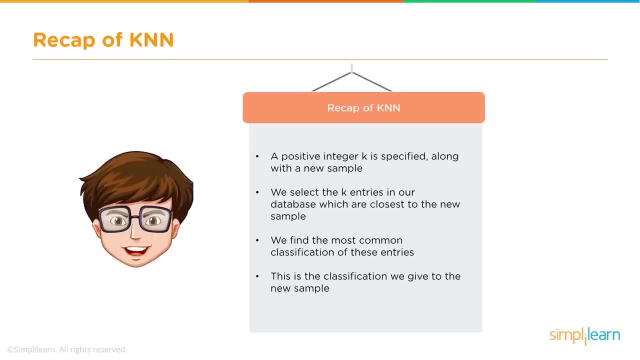 towards normal. Hence, as per K and N algorithm, the class of fifty seven one seventy should be normal. So a recap of K and N Positive integer K is specified along with a new sample. We select the K entries in our database which are closest to the new sample. 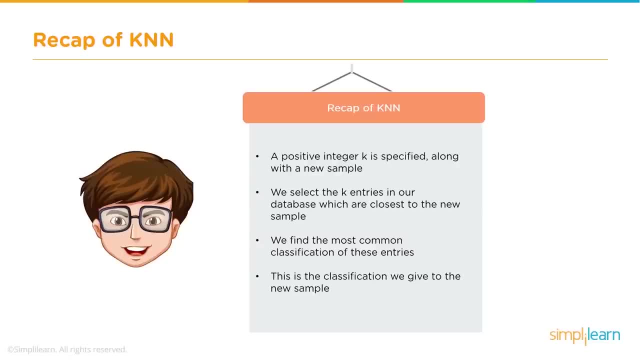 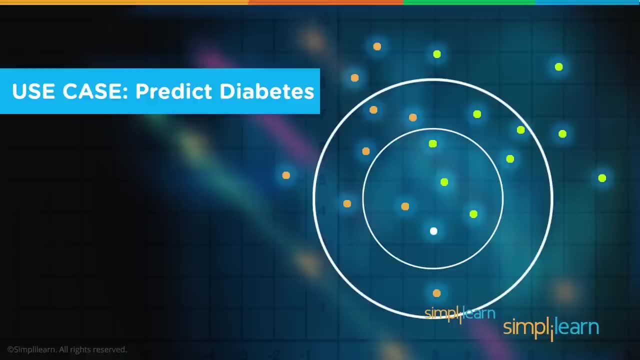 We find the most common classification of these entries. This is the classification we give to the new sample. So, as you can see, it's pretty straightforward. We're just looking for the closest things that match what we got. So let's take a look and see what that looks like in a use case. 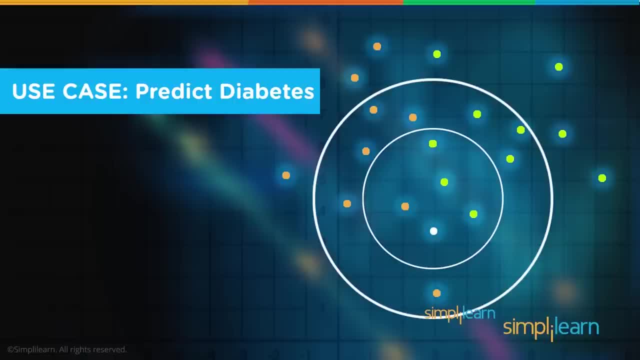 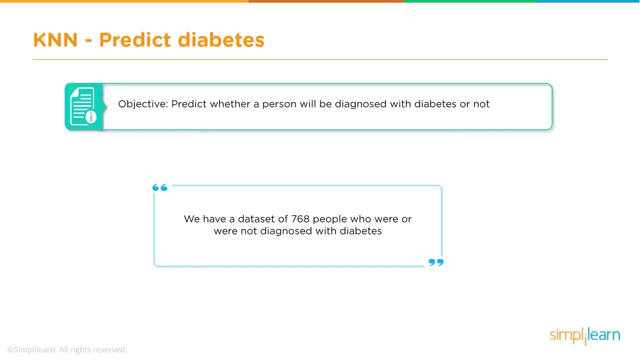 Python. So let's dive into the predict diabetes use case. So use case: predict diabetes. The objective: predict whether a person will be diagnosed with diabetes or not. We have a data set of seven hundred and sixty eight people who were or were not diagnosed with diabetes. 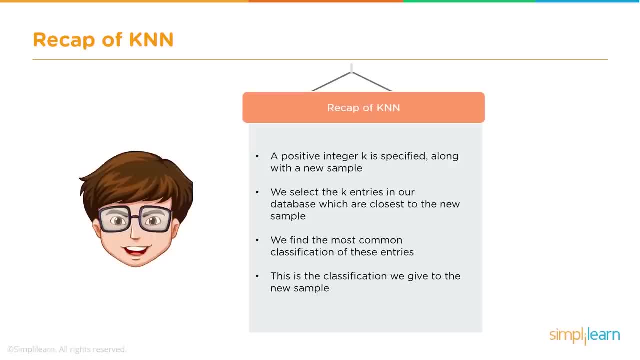 hence, as per KNN algorithm, the class of 57 170 should be normal and we can see the entries in our database which are closest to the new sample. we find the most common classification of these entries. this is the classification we give to the new sample. 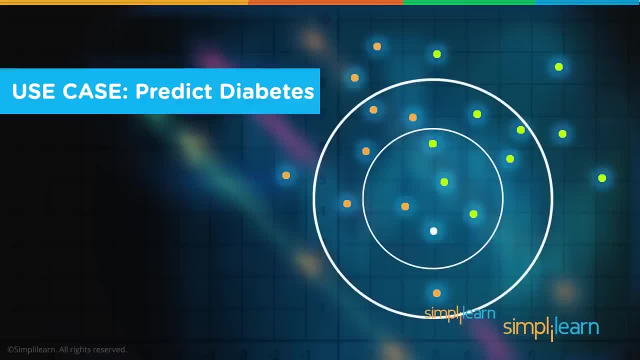 so, as you can see, it's pretty straight forward. we're just looking for the closest things that match what we got. so let's take a look and see what that looks like in a use case in python. so let's dive into the predict diabetes use case. 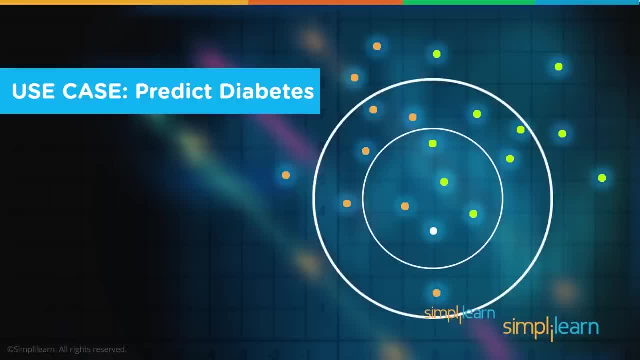 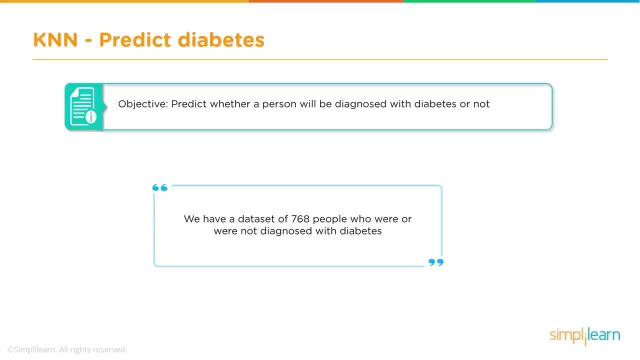 so use case: predict diabetes. the objective: predict whether a person will be diagnosed with diabetes or not. we have a data set up of 768 people who were or were not diagnosed with diabetes and let's go ahead and open that file and just take a look at that data. 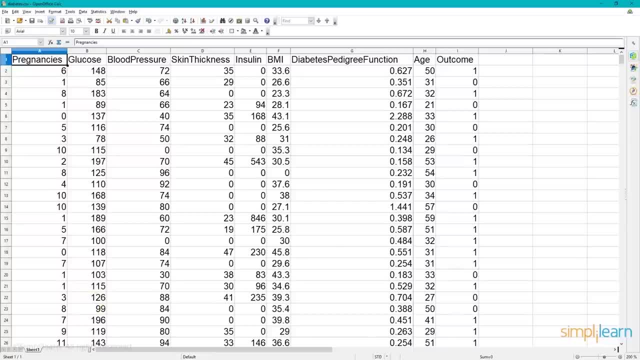 and this is in a simple spreadsheet format. the data itself is comma separated- very common set of data and it's also a very common way to get the data and you can see here we have columns A through I. that's what: 1, 2, 3, 4, 5, 6, 7, 8. 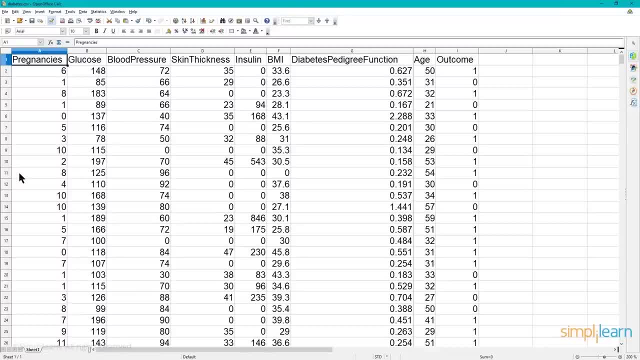 8 columns with a particular attribute, and then the 9th column is whether they have diabetes. as a data scientist, the first thing you should be looking at is insulin. well, you know, if someone has insulin, they have diabetes because that's why they're taking it. 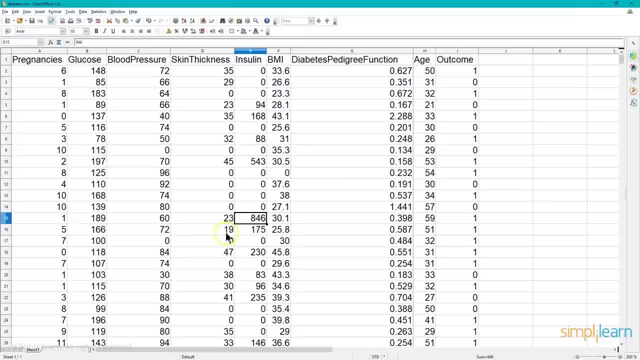 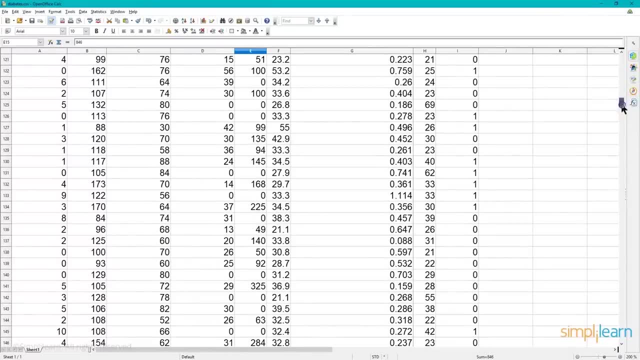 and that could cause issue in some of the machine learning packages. but for a very basic set up this works fine for doing the KNN and the next thing you notice is it didn't take very much to open it up. I can scroll down to the bottom of the data. 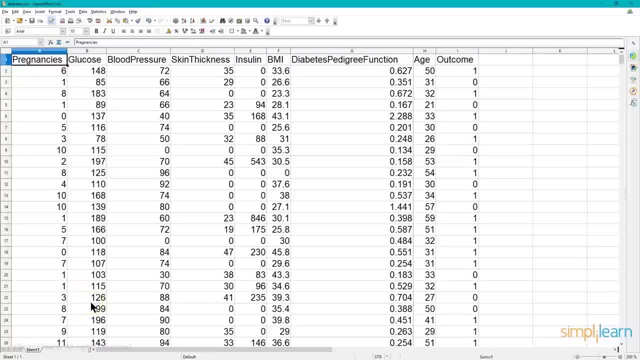 And let's go ahead and open that file and just take a look at that data. And this is in a simple spreadsheet format. The data itself is comma separated- very common set of data And it's also a very common way to get the data. 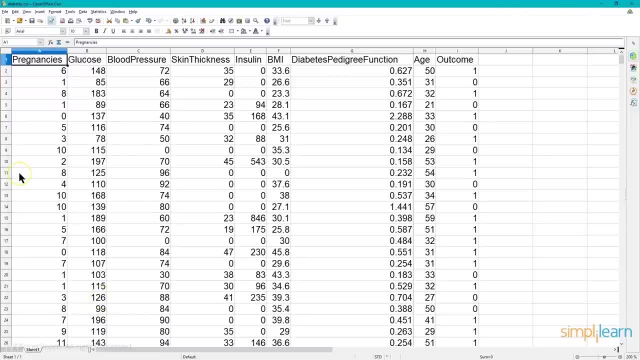 So, as you can see, here we have columns A through I. That's what one, two, three, four, five, six, seven, eight, eight columns with a particular attribute, And then the ninth column, which is the outcome, is whether they have diabetes. 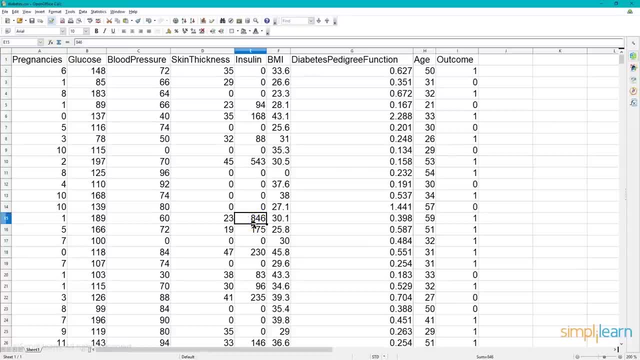 As a data scientist, the first thing you should be looking at is insulin. Well, you know, if someone has insulin, they have diabetes, because that's why they're taking it, And that could cause issue in some of the machine learning packages. 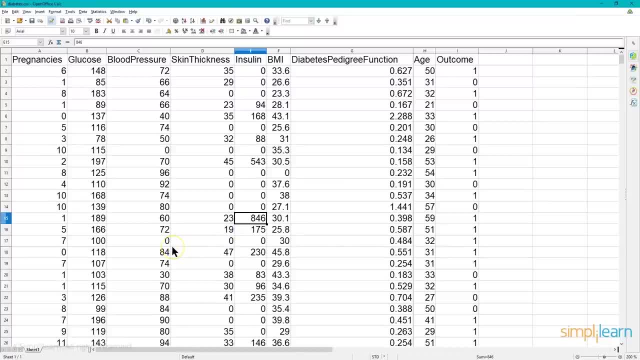 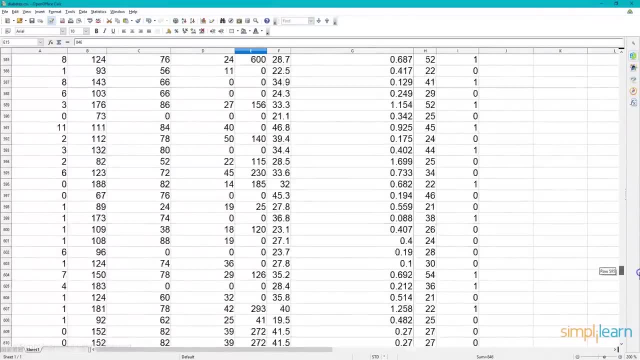 But for a very basic setup. this works fine for doing the KNN And the next thing you notice is that it didn't take very much to open it up. I can scroll down to the bottom of the data. There's seven hundred and sixty eight. 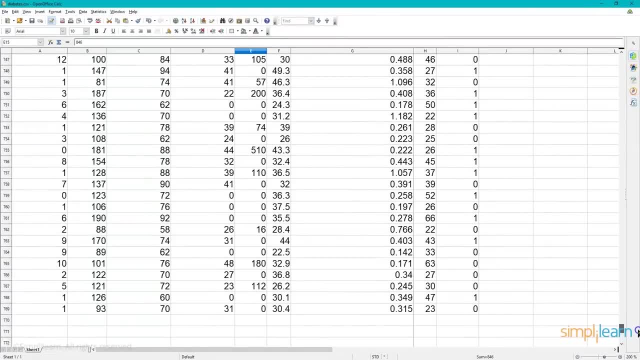 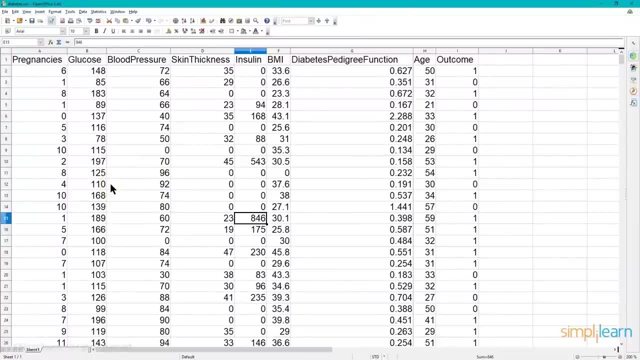 there's 768. it's pretty much a small data set. you know, at 769 I can easily fit this into my RAM on my computer. I can look at it, I can manipulate it and it's not going to really tax, just a regular desktop computer. you don't even need an enterprise version to run a lot of this. 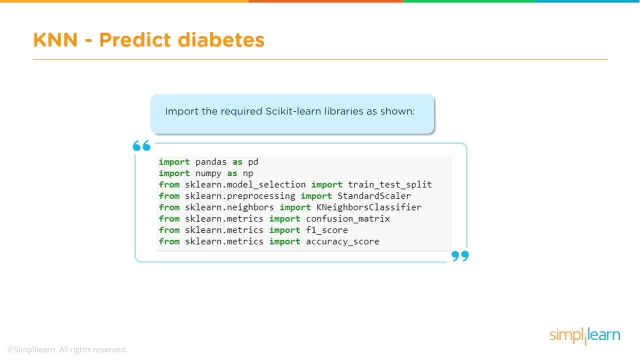 so let's start with importing all the tools we need, and before that, of course, we need to discuss what IDE I'm using. certainly, you can use any particular editor for Python, but I like to use, for doing very basic visual stuff, the Anaconda, which is great for doing. 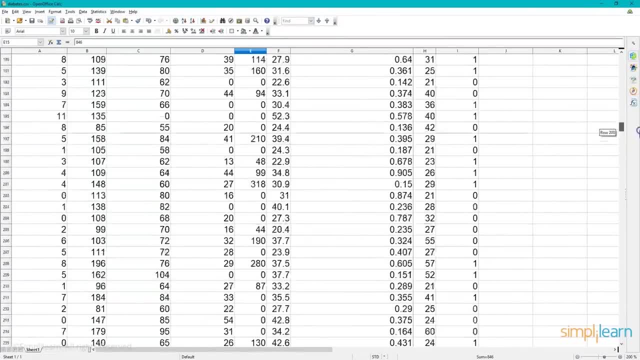 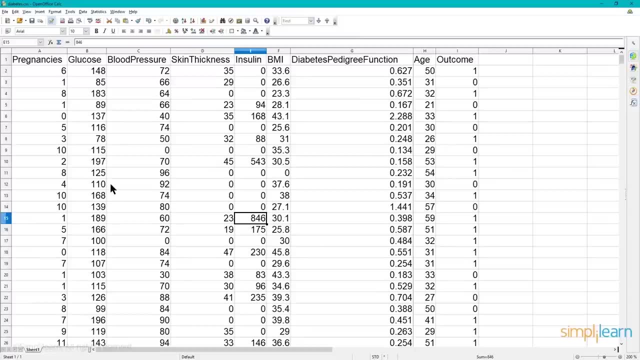 It's pretty much a small data set. You know it's seven hundred sixty nine. I can easily fit this into my RAM on my computer. I can look at it, I can manipulate it And it's not going to really tax, just a regular desktop computer. 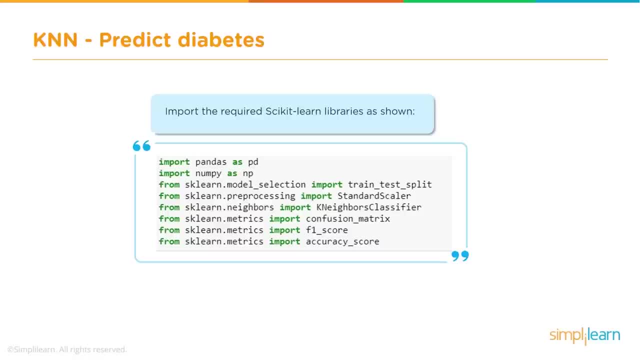 You don't even need an enterprise version to run a lot of this. So let's start with importing all the tools we need, And before that, of course, we need to discuss what IDE I'm using. Certainly can use any software for Python, but I like to use for doing very basic visual stuff. 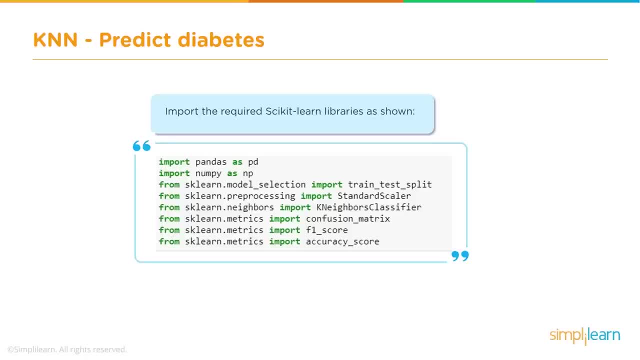 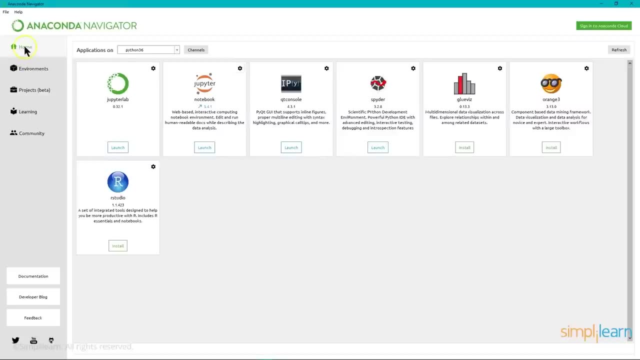 the Anaconda, which is great for doing demos with the Jupyter notebook, And just a quick view of the Anaconda navigator, which is the new release out there, which is really nice. You can see under home. I can choose my application. 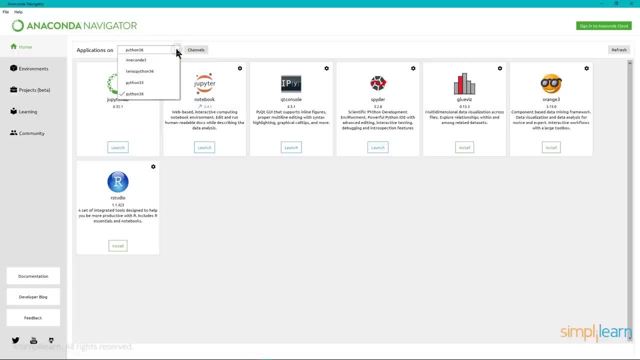 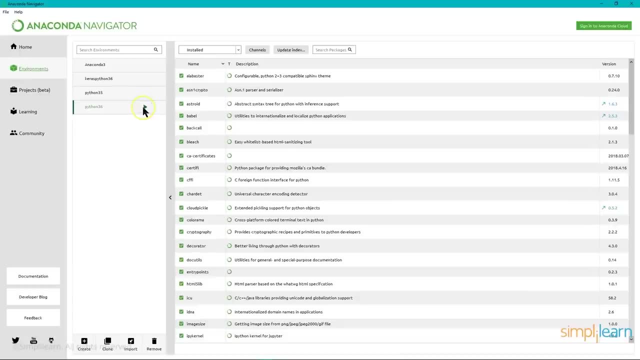 We're going to be using Python three six. I have a couple of different versions on this particular machine. If I go under environments, I can create a unique environment for each one, which is nice, And there's even a little button there where I can install different. 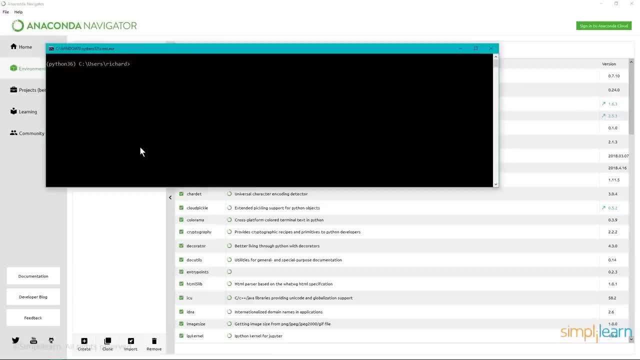 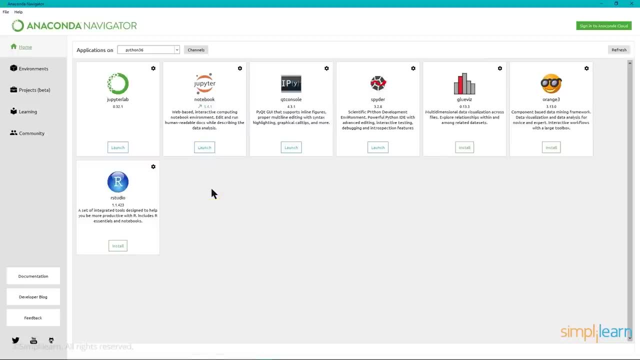 packages. so if I click on that button and open the terminal, I can then use a simple pip install to install different packages I'm working with. Let's go ahead and go back under home and we're going to launch our notebook And I've already, you know, kind of like the old cooking shows. 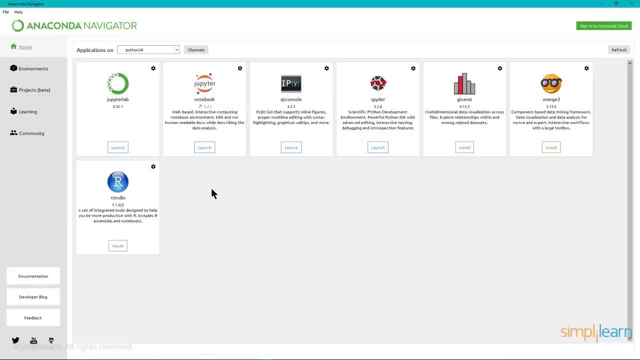 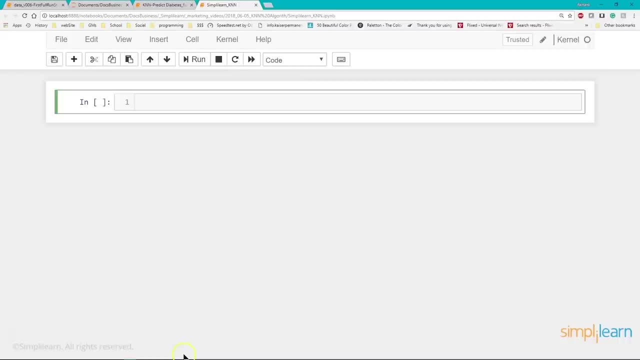 I've already prepared a lot of my stuff, so we don't have to wait for it to launch, because it takes a few minutes for it to open up a browser window. In this case, I'm going to open up Chrome because that's my default that I use. 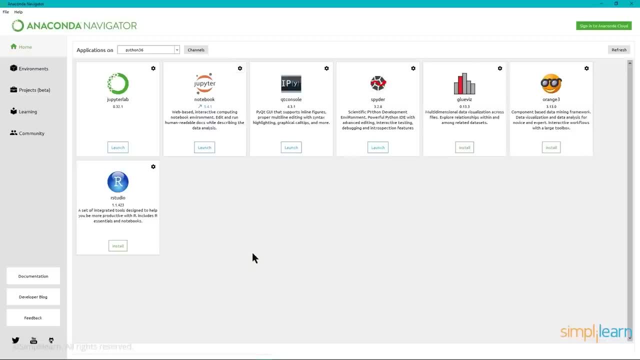 demos with the Jupyter notebook and just a quick view of the Anaconda Navigator, which is the new release out there, which is really nice you can see under home. I can choose my application. we're going to be using Python 3.6. I have a couple different versions on this particular machine. 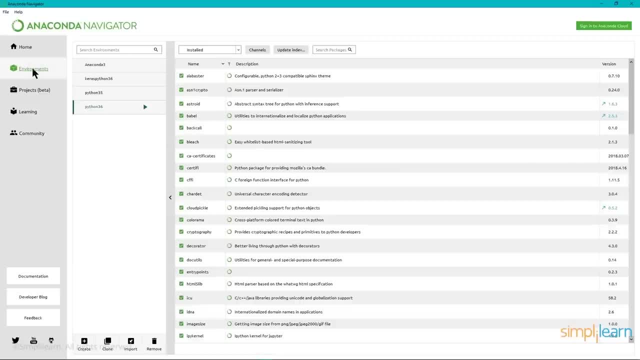 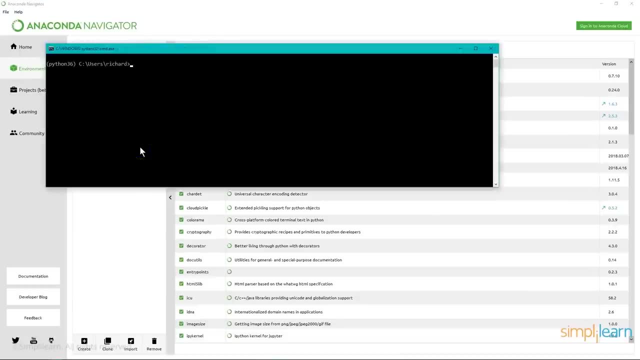 if I go under environments, I can create a unique environment for each one, which is nice, and there's even a little button there where I can install different packages. so if I click on that button and open the terminal, I can then use a simple pip install to install different packages I'm working with 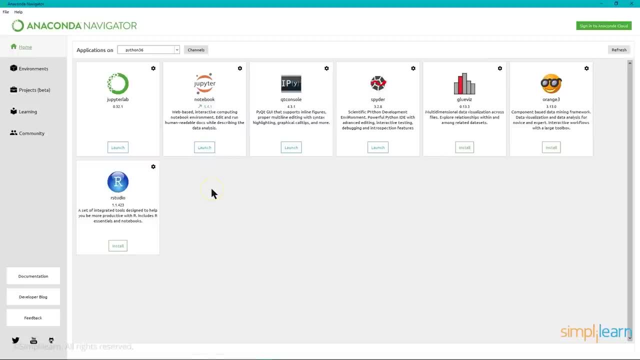 let's go ahead and go back under home and we're going to launch our notebook and I've already, kind of like the old cooking shows, I've already prepared a lot of my stuff, so we don't have to wait for it to launch, because it takes a few minutes for it to open up. 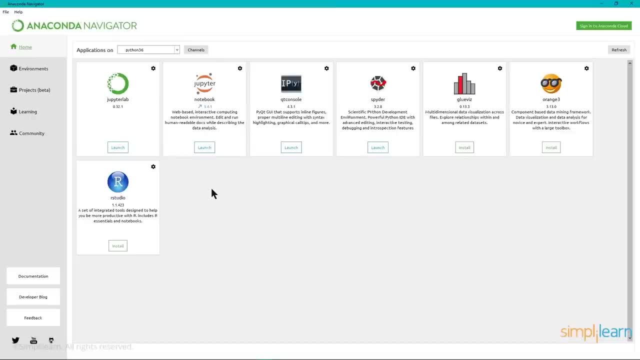 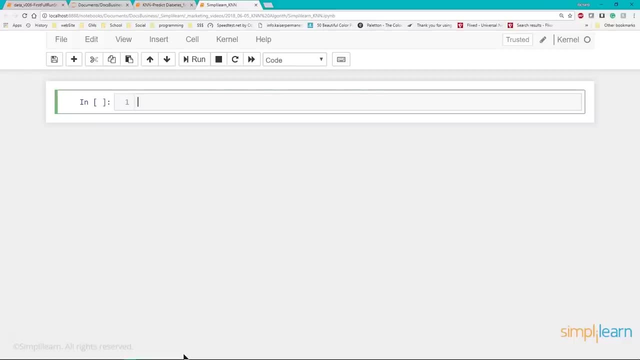 a browser window. in this case it's going to open up Chrome, because that's my default that I use, and since the script is pre-done, you'll see I have a number of windows open up, at the top the one we're working in. and since we're working on the 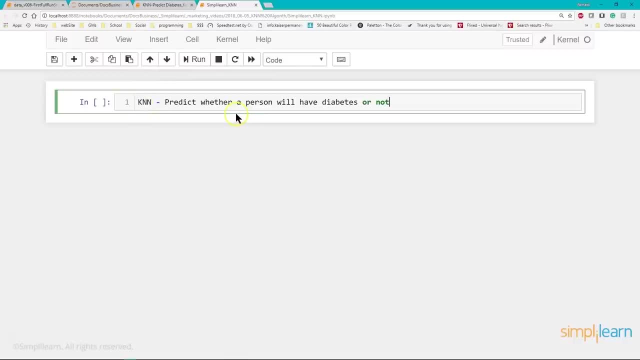 KNN predict whether a person will have diabetes or not. let's go ahead and put that title in there, and I'm also going to go up here and click on cell. actually, we want to go ahead and first insert a cell below and then I'm going to go back. 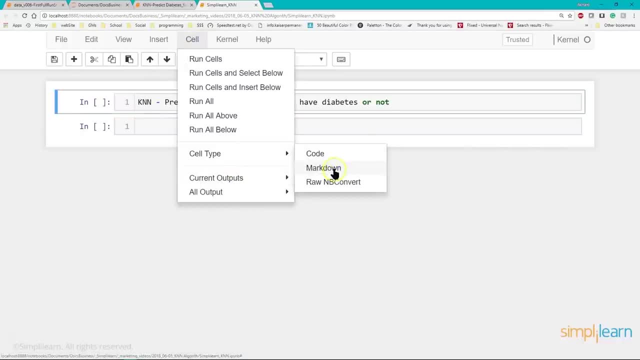 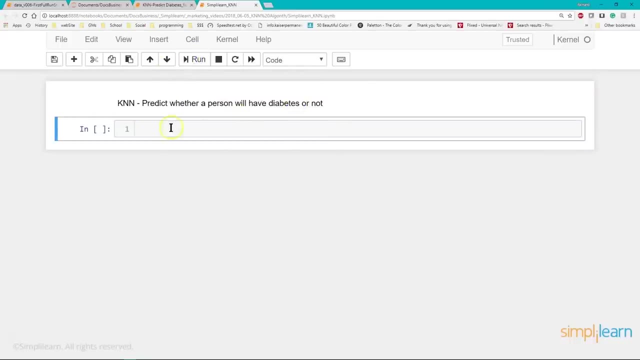 up to the top cell and I'm going to change the cell type to markdown. that means this is not going to run as Python it's a markdown language, so if I run this first one it comes up in nice big letters, which is kind of nice. remind us what we're. 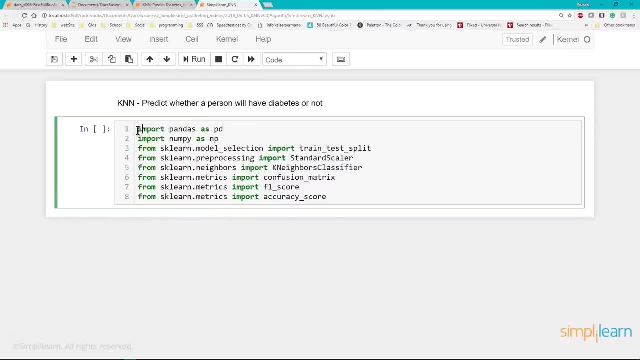 working on- and by now you should be familiar with doing all of our imports. we're going to import the pandas as pd import, numpy as np, pandas is the pandas data frame and numpy is the number array- very powerful tools to use in here. so we have our 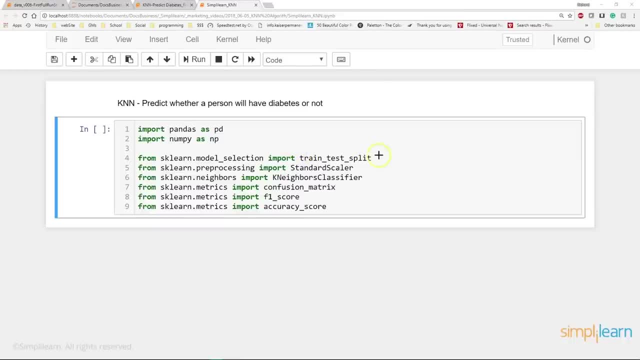 imports. so we've brought in our pandas, our numpy, our two general python tools, and then you can see over here we have our train test split. by now you should be familiar with splitting the data. we want to split part of it for training our thing and then training our particular model. 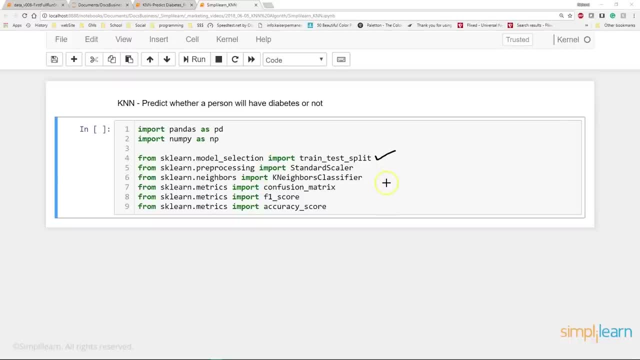 and then we want to go ahead and test the remaining data to see how good it is preprocessing a standard scalar preprocessor so we don't have a bias of really large numbers. remember in the data we had like number pregnancies isn't going to get very large. 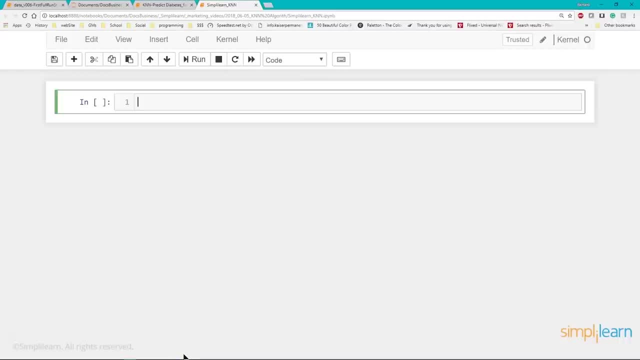 And since the script is pre-done, you'll see I have a number of windows open up at the top, the one we're working in. and since we're working in a KNN predict whether a person will have diabetes or not, Let's go and put that title in there. 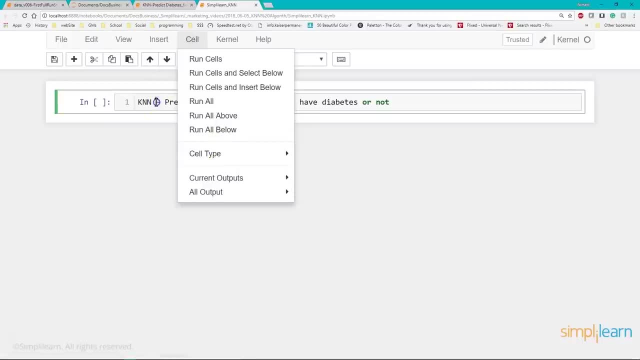 And I'm also going to go up here and click on cell. Actually, we want to go ahead and first insert a cell below and then I'm going to go back up to the top cell and I'm going to change the cell type to markdown. 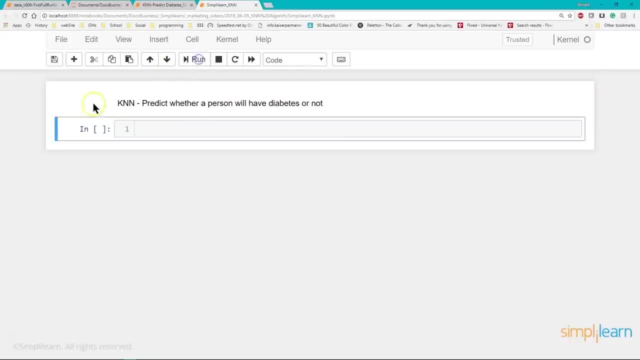 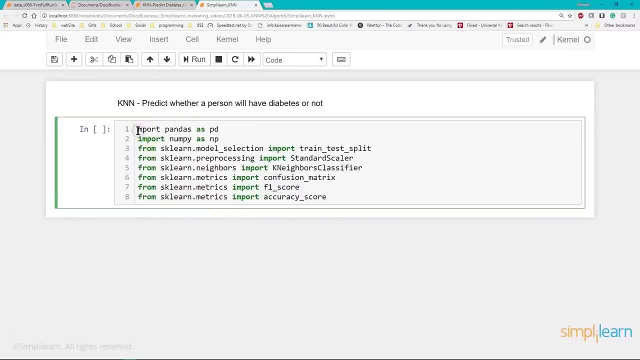 That means this is not going to run as Python It's a markdown language, So if I run this first one it comes up in nice big letters, which is kind of nice, Remind us what we're working on, And by now you should be familiar with doing all of our imports. 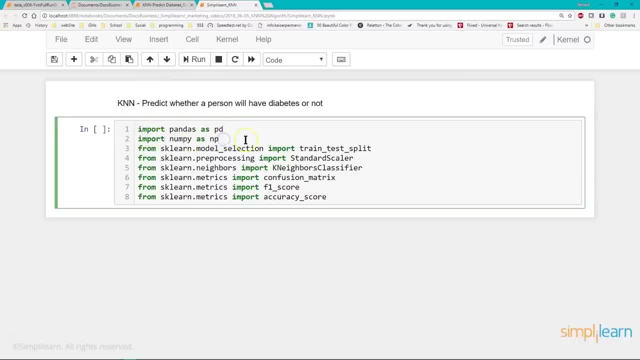 We're going to import the pandas as pd import, numpy as np. Pandas is the pandas data frame and numpy is a number array, Very powerful tools to use in here. So we have our imports. So we've brought in our pandas, our numpy, our two general Python tools. 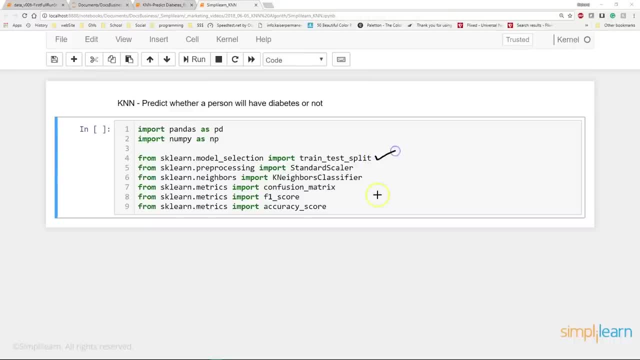 And then you can see over here we have our train test split. By now. you should be familiar with splitting the data. We want to split part of it for training our thing and then training our particular model, and then we want to go ahead and test the remaining data to see how good. 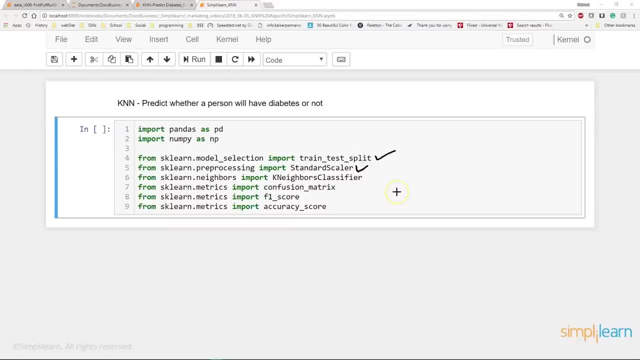 it is Pre-processing, a standard scalar pre-processor, So we don't have a bias of really large numbers. Remember, in the data we had like number pregnancies isn't going to get very large, where the amount of insulin they take and get up to 256, so 256 versus six, that will skew results. 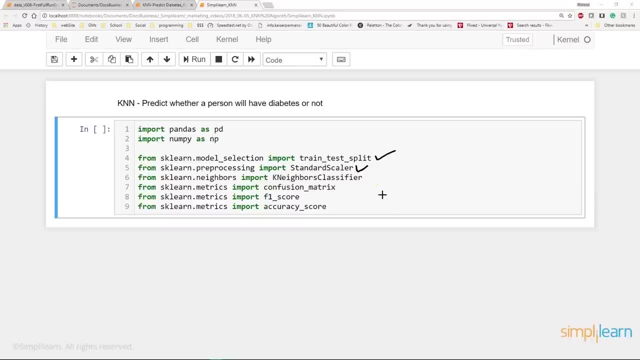 So we want to go ahead and change that so that they're all uniform between minus one and one. And then the actual tool. This is the K neighbors classifier we're going to use. And finally, the last three are three tools to test. all about testing our model. How good is it? 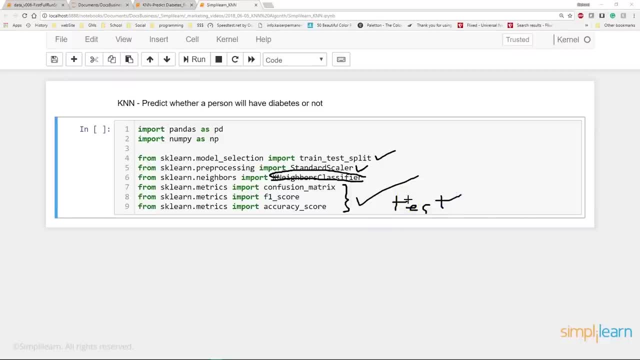 We just put down test on there and we have our confusion matrix, our F1 score and our accuracy. So we have our two general Python modules we're importing and then we have our six modules specific from the SK learn set up and then we do need to go ahead and run. 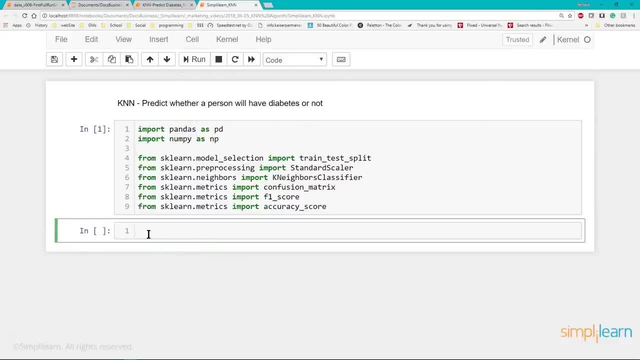 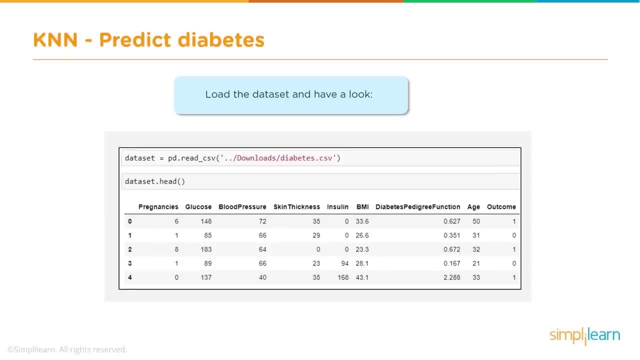 this so that these are actually imported. There we go And then move on to the next step, And so in this set, we're going to go ahead and load the database, We're going to use pandas- Remember pandas is PD- And we'll take 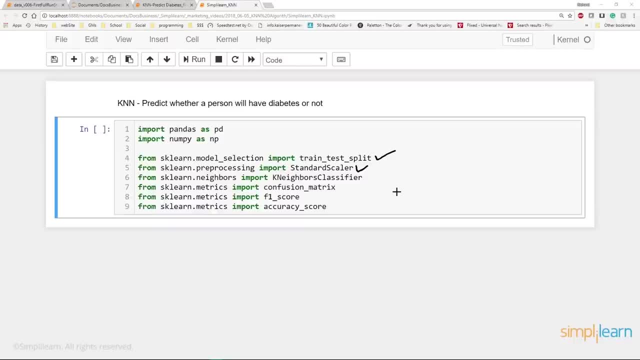 where the amount of insulin they take can get up to 256. so 256 versus six, that will skew results. so we want to go ahead and change that so that they're all uniform between minus one and one, and then the actual tool. this is the k neighbors. 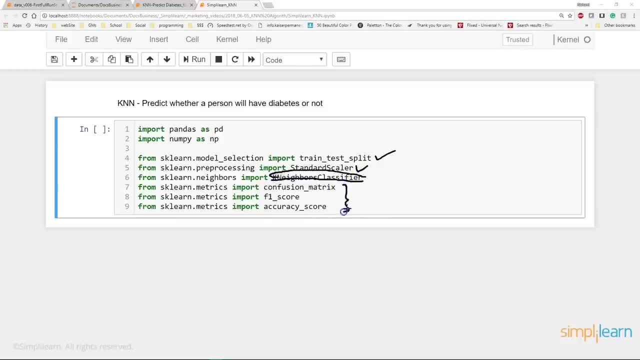 classifier we're going to use. and finally, the last three are three tools to test. all about testing our model. how good is it? we just put down test on there and we have our confusion matrix, our f1 score and our accuracy. so we have our two general python. 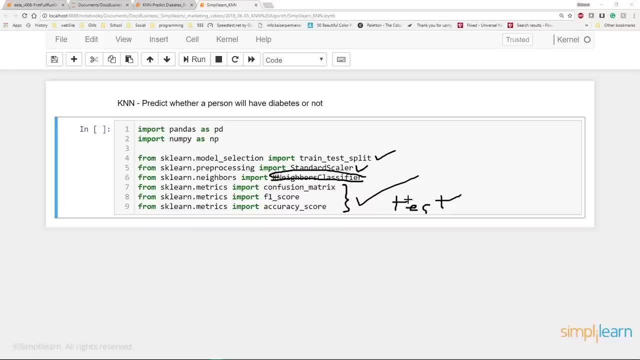 modules we're importing and they we have our six modules specific from the sk learn set up and then we do need to go ahead and run this, so these are actually imported. there we go and then move on to the next step and so in this set we're going to go ahead and load the database. 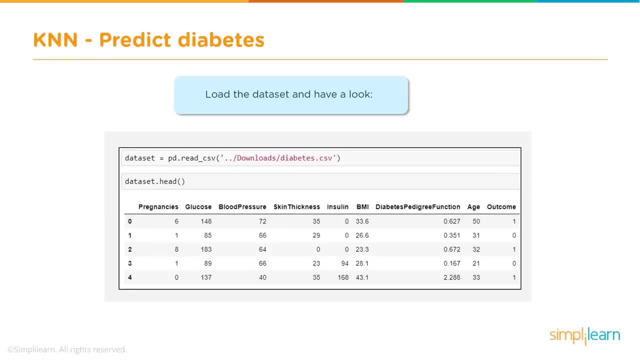 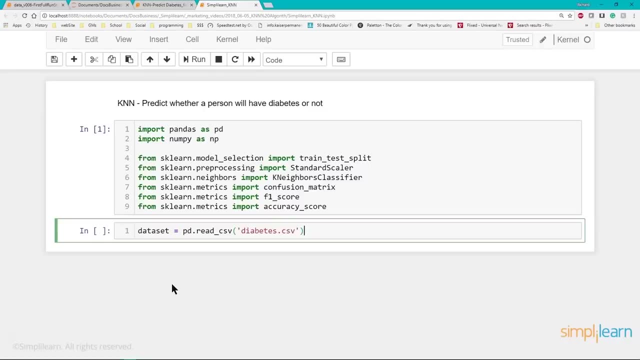 we're going to use pandas- remember pandas is pd- and we'll take a look at the data in python. we looked at it in a simple spreadsheet, but usually i like to also pull it up so that we can see what we're doing. so here's our data set. 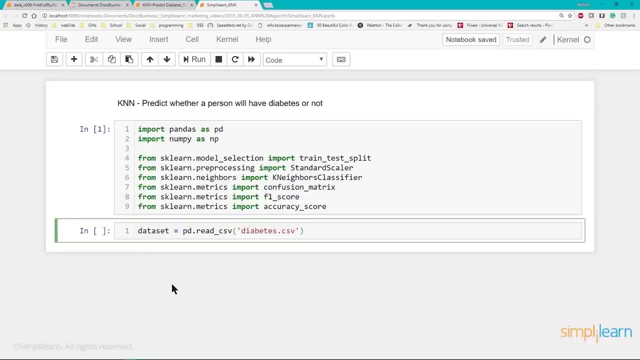 equals pd dot. read csv. that's a pandas command. and the diabetes folder i just put in the same folder where my ipython script is. if you put in a different folder you'd need the full length on there. we can also do a quick length of the data. 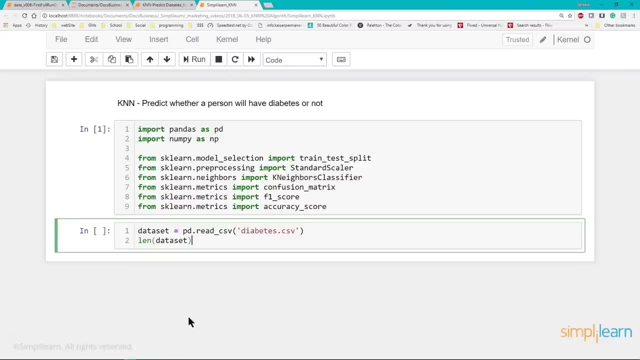 set. that is a simple python command. len for length, we might even let's go ahead and print that. we'll go print and if you do it on its own line, link that data set in the jupyter notebook. it'll automatically print it. but when you're in most of your different setups, 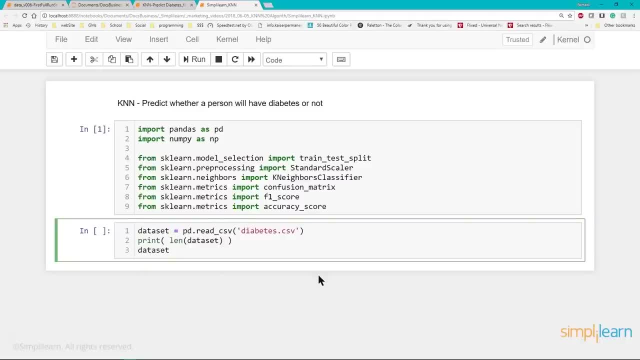 you want to do the print in front of there and then we want to take a look at the actual data set and since we're in pandas, we can simply do data set head and again. let's go ahead and add the print in there, if you put. 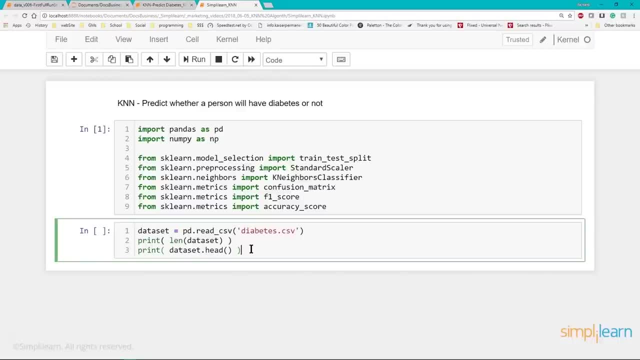 a bunch of these in a row. you know the data set one head, data set two head. it only prints out the last one, so i usually always like to keep the print statement in there. but because most projects only use one data frame- pandas data frame- doing it this way doesn't. 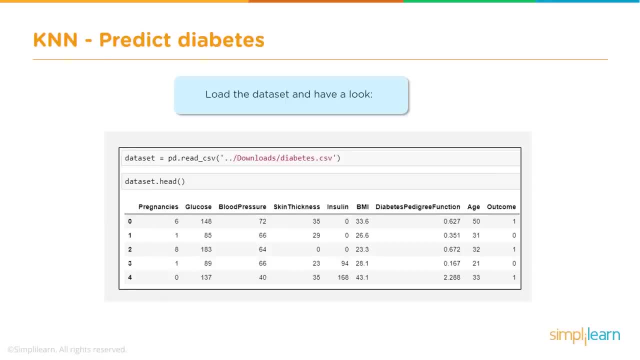 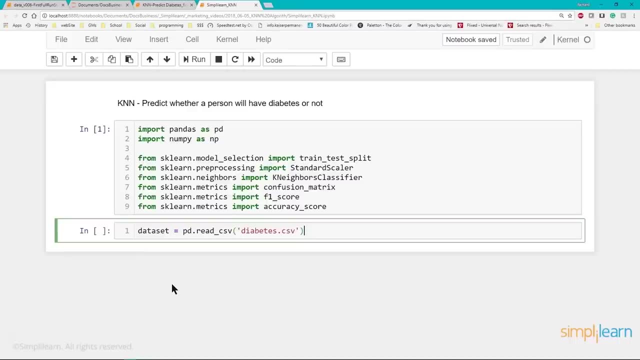 a look at the data in Python. We looked at it in a simple spreadsheet, but usually I like to also pull it up so that we can see what we're doing. So here's our data. set: equals pdreadcsv, That's a pandas command and the diabetes. 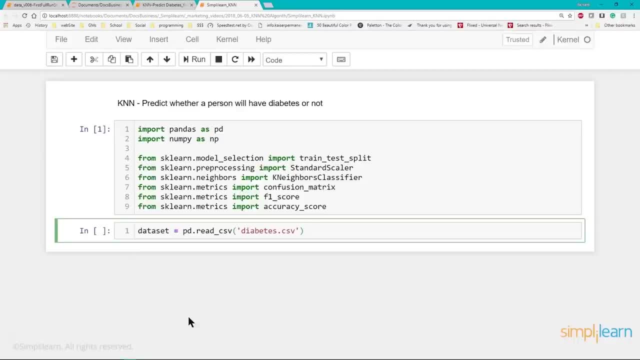 folder. I just put in the same folder where my IPython script is. If you put in a different folder you'd need the full length on there. We can also do a quick length of the data set. That is a simple Python command: len for length. 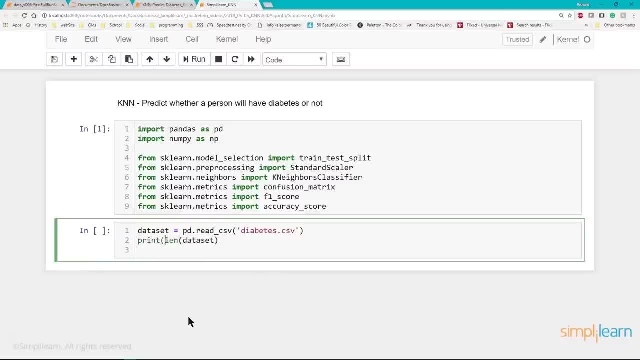 We might even just go ahead and print that. We'll go print And if you do it on its own line lengthdataset in the Jupyter Notebook, it'll automatically print it. But when you're in most of your different setups you want to do the print in front of there. 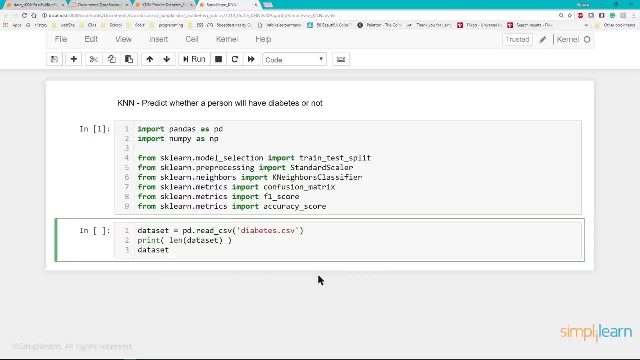 And then we want to take a look at the actual data set And since we're in pandas, we can simply do data set head And again. let's go ahead and add the print in there If you put a bunch of these in a row. 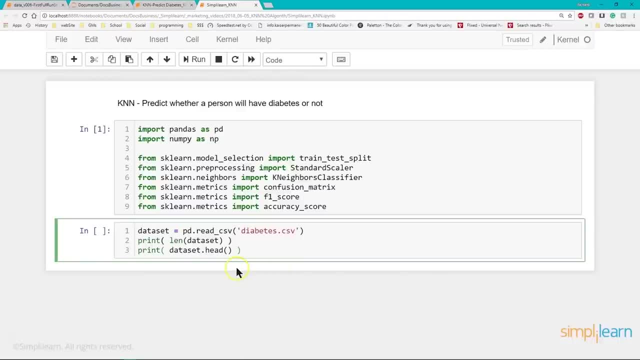 you know the data set one head, data set two head. it only prints out the last one. So I always like to keep the print statement in there. But because most projects only use one data frame, pandas data frame doing it this way. 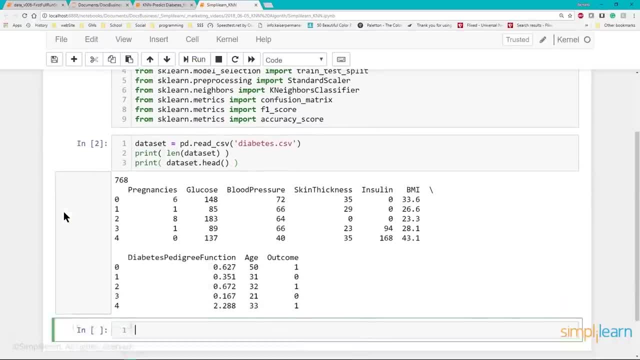 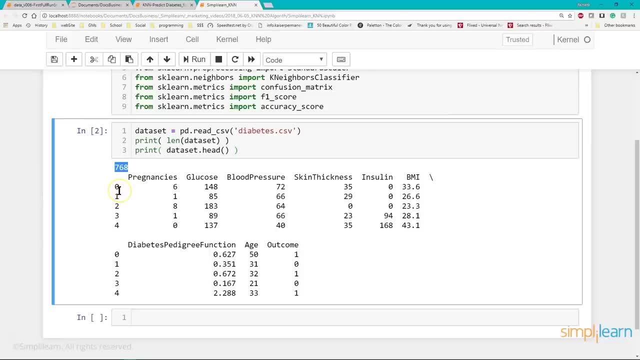 doesn't really matter. The other way works just fine And you can see when we hit the run button. we have the seven hundred and sixty eight lines which we knew and we have our pregnancies. It's automatically given a label on the left. 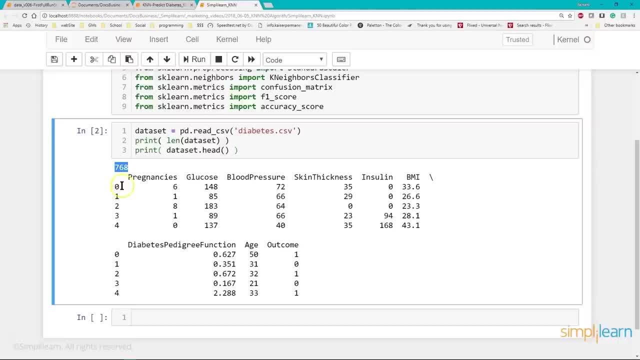 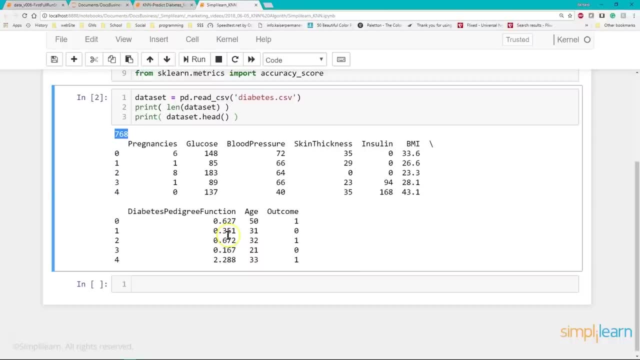 Remember, the head only shows the first five lines, So we have zero through four And just a quick look at the data You can see it matches what we looked at before. We have pregnancy, glucose blood pressure, all the way to age, and then the outcome. 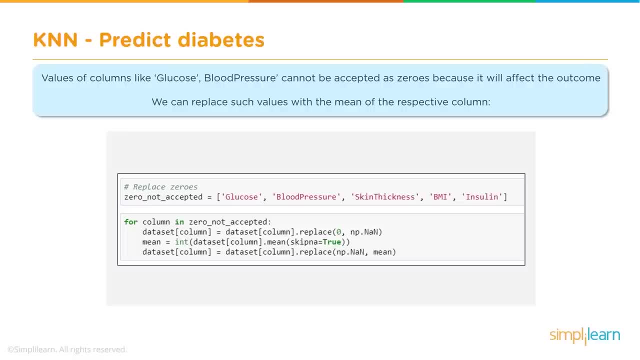 on the end, And we're going to do a couple of things in this next step. We're going to create a list of columns where we can't have zero. There's no such thing as zero skin thickness or zero blood pressure, zero glucose- any of those, you'd be dead. 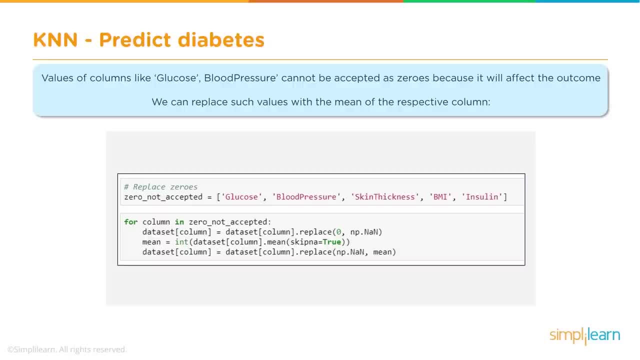 So not a really good factor if they don't, if they have a zero in there because they didn't have the data- And we'll take a look at that because we're going to start replacing that information with a couple of different things And let's see what that looks like. 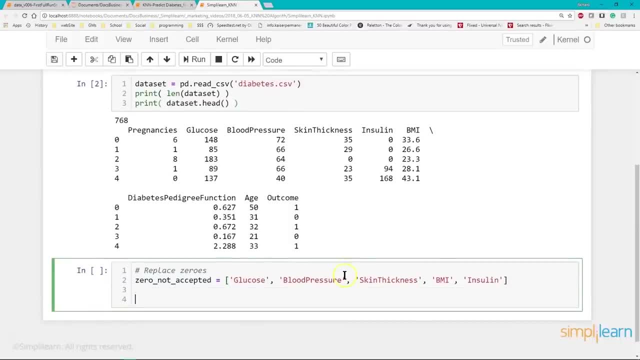 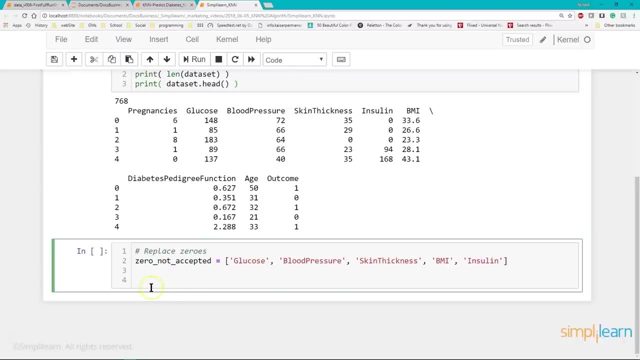 So first we create a nice list. As you can see, we have the values talked about: glucose, blood pressure, skin thickness, And this is a nice way when you're working with columns is to list the columns you need to do some kind of transformation on. 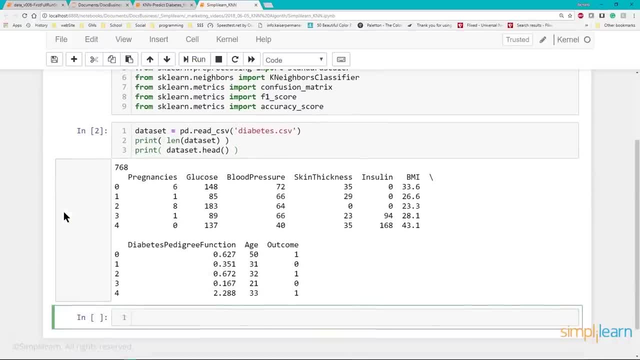 really matter. the other way works just fine and you can see when we hit the run button. we have the 768 lines which we knew and we have our pregnancies. it's automatically given a label on the left. remember, the head only shows the first five lines, so we have zero through four. 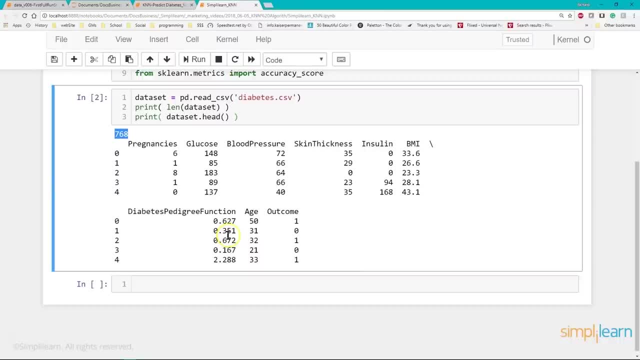 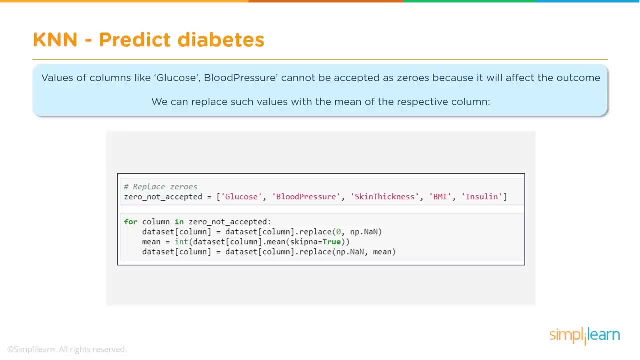 and just a quick look at the data. you can see it matches what we looked at before. we have pregnancy, glucose blood pressure, all the way to age, and then the outcome on the end, and we're going to do a couple things in this next step. we're going to create 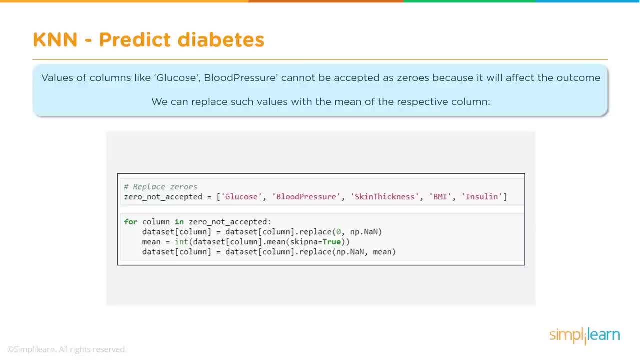 a list of columns where we can't have zero. there's no such thing as zero skin thickness or zero blood pressure, zero glucose- any of those, you'd be dead. so not a really good factor if they have a zero in there because they didn't have the data. 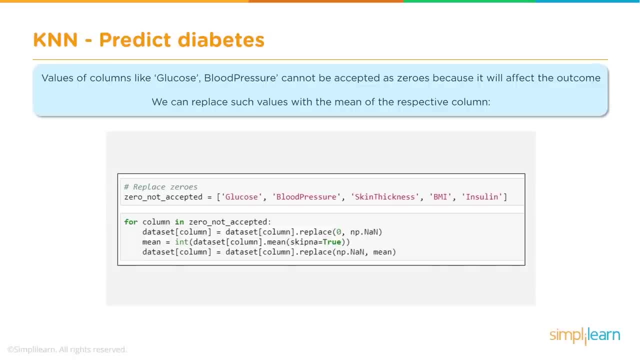 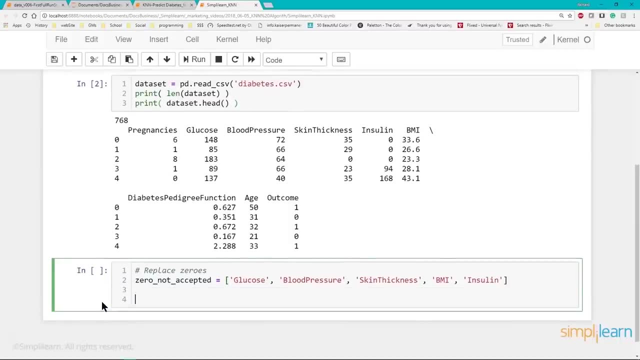 and we'll take a look at that, because we're going to start replacing that information with a couple of different things and let's see what that looks like. so first we create a nice list. as you can see, we have the values we talked about: glucose, blood pressure, skin thickness. 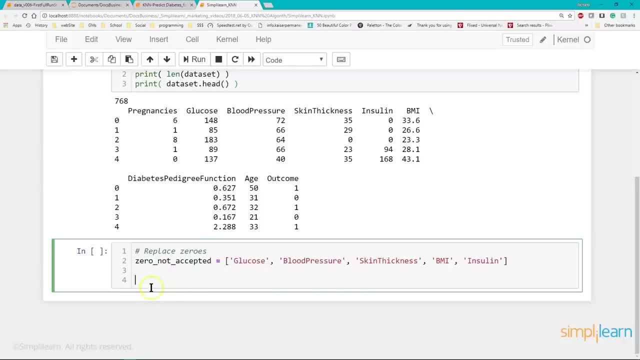 and this is a nice way when you're working with columns- is to list the columns you need to do some kind of transformation on a very common thing to do, and then for this particular setup, we certainly could use. there's some panda tools that will do a lot of this- where we can replace the 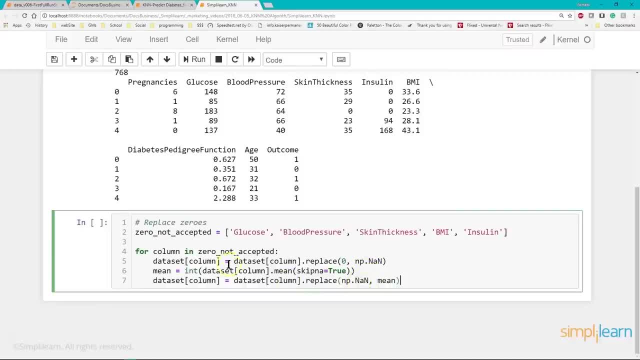 NA, but we're going to go ahead and do it as a data set column equals data set column. dot replace this is still pandas. you can do it direct. there's also one that you look for your NAN. a lot of different options in here, but the NAN numpy NAN. 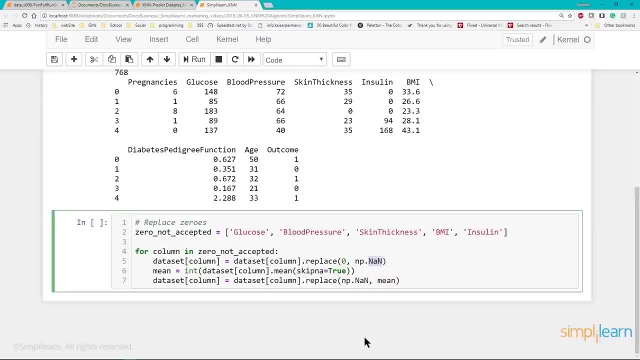 is what that stands for is: none doesn't exist. so the first thing we're doing here is we're replacing the zero with a numpy: none. there's no data there. that's what that says. that's what this is saying right here. so put the zero in and we're going to replace zeros with. 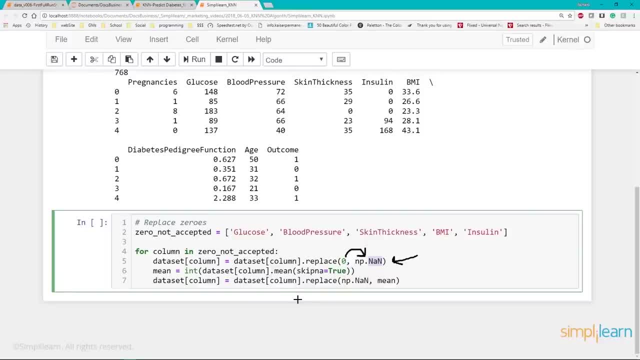 no data. so if it's a zero, that means the person's well, hopefully, not dead. hopefully just didn't get the data. the next thing we want to do is we're going to create the mean, which is the integer from the data set, from the column dot mean, where we skip NAs. 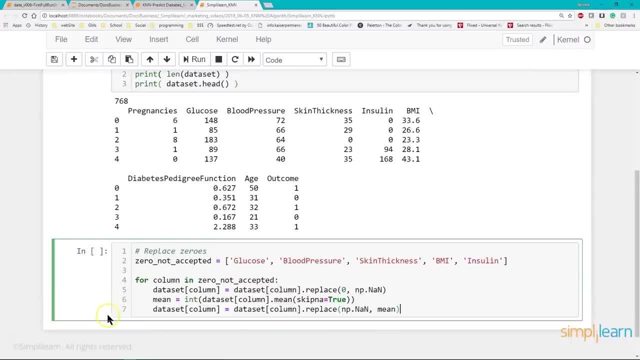 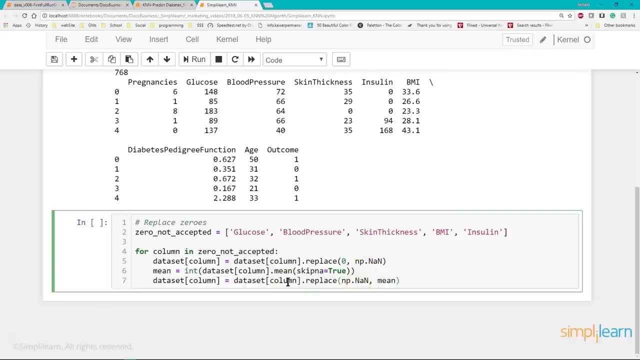 Very common thing to do, And then for this particular setup, we certainly could use the- there's some Panda tools that will do a lot of this- where we can replace the NA, But we're going to go ahead and do it as a data set column equals data set column. 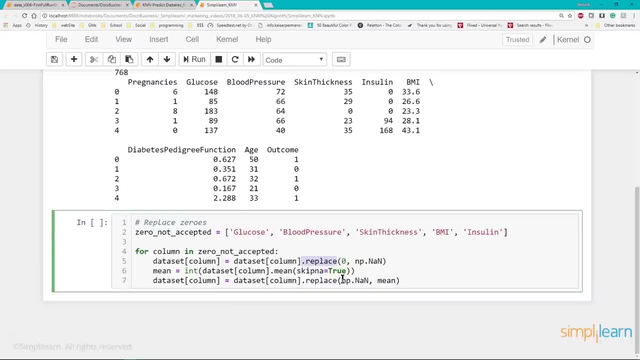 dot replace This is. this is still Pandas. You can do a direct. There's also one that you look for your NA in A lot of different options in here, But the NA in numpy NA is what that stands for is is none doesn't exist. 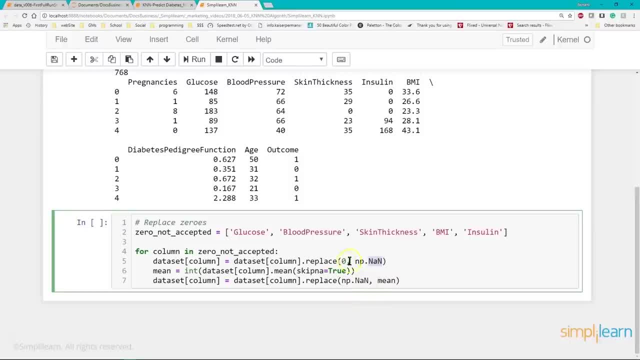 So the first thing we're doing here is we're replacing the zero with a numpy none. There's no data there. That's what that says. That's what this is saying right here. So put the zero in and we're going to play zeros with no data. 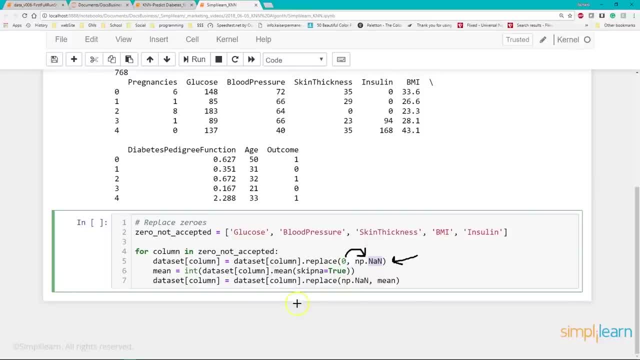 So if it's a zero, that means a person's well, hopefully not dead. Oh, they just didn't get the data. The next thing we want to do is we're going to create the mean, which is the integer data set from the column dot mean, where we skip NA's. 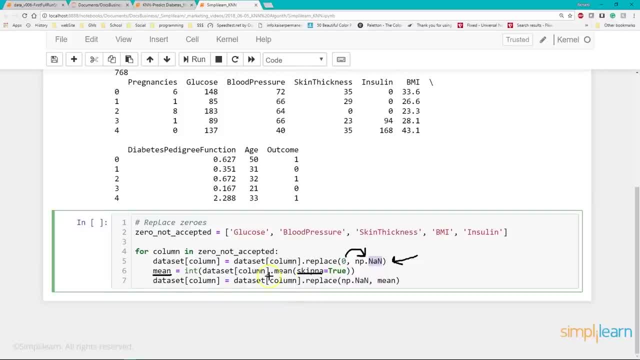 We can do that. That is a Pandas command there. The skip NA. So we're going to figure out the mean of that data set And then we're going to take that data set column and we're going to replace all the NPNAN with the means. Why did we do that? 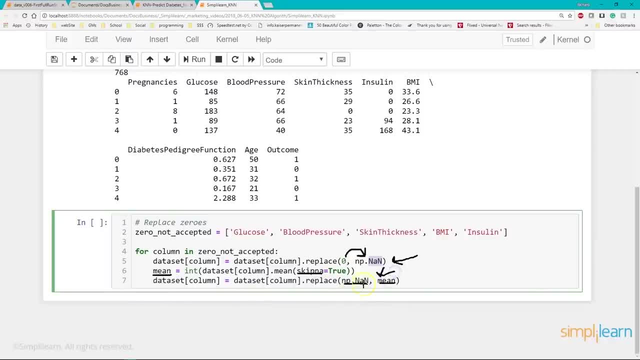 And we could have actually just taken this step and gone right down here and just replace zero and skip anything where you could. actually there's a way to skip zeros and then just replace all the zeros, But in this case we want to go ahead and do it this way. 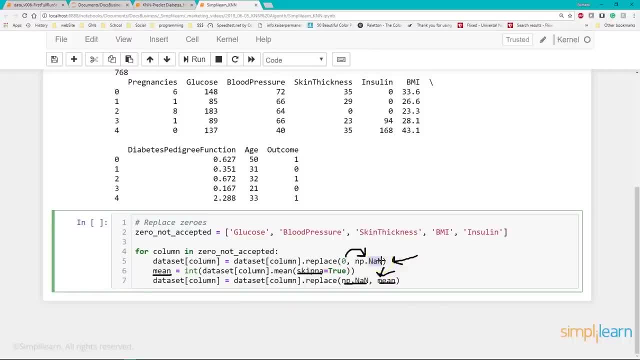 So you could See that we're switching this to a non-existent value and we're going to create the mean. Well, this is the average person. So if we don't know what it is, if they did not get the data- and the data is- 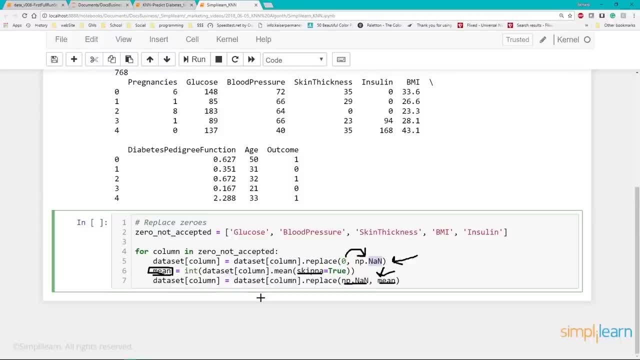 missing. one of the tricks is you replace it with the average, What is the most common data for that. This way you can still use the rest of those values to do your computation And it kind of just brings that particular value of those missing values out of the equation. 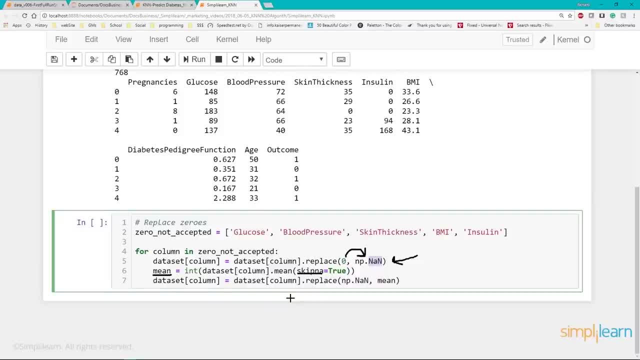 we can do that. that is a pandas command. there the skip NA. so we're going to figure out the mean of that data set and then we're going to take that data set column and we're going to replace all the NPNAN with the means. why did we? 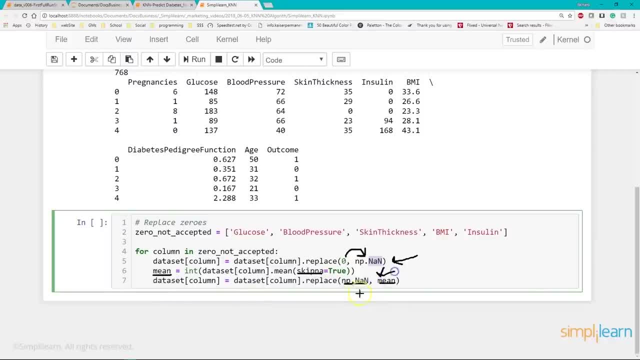 do that. we could have actually just taken this step and gone right down here and just replace zero and skip anything. where except you could actually there's a way to skip zeros and then just replace all the zeros. but in this case we want to go ahead and do it this way. 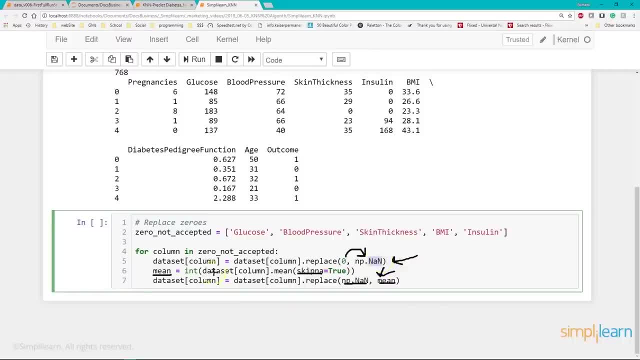 so you can see that we're switching this to a non-existent value and we're going to create the mean. well, this is the average person. so if we don't know what it is, if they did not get the data and the data is missing, one of the tricks is you replace. 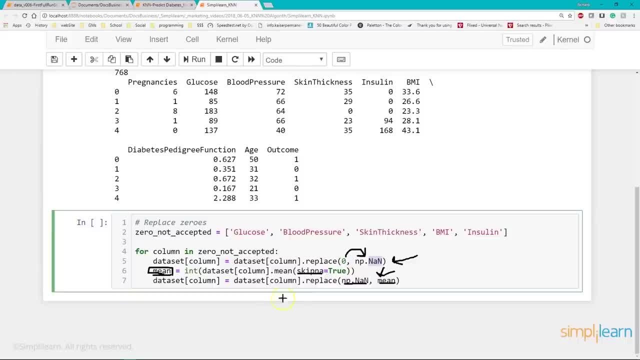 it with the average. what is the most common data for that? this way you can still use the rest of those values to do your computation and it kind of just brings that particular value of those missing values out of the equation. let's go ahead and take this and: 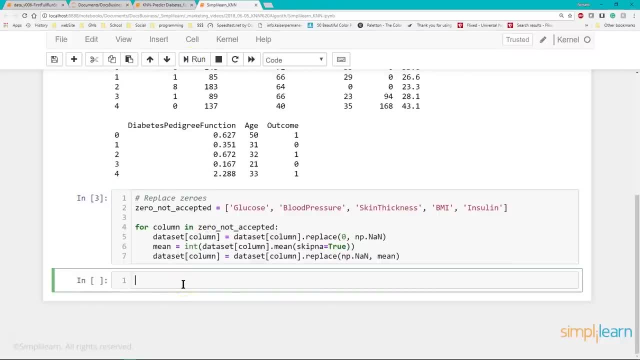 we'll go ahead and run. it doesn't actually do anything, so we're still preparing our data. if you want to see what that looks like, we don't have anything in the first few lines, so it's not going to show up, but we certainly could look at a row. let's do. 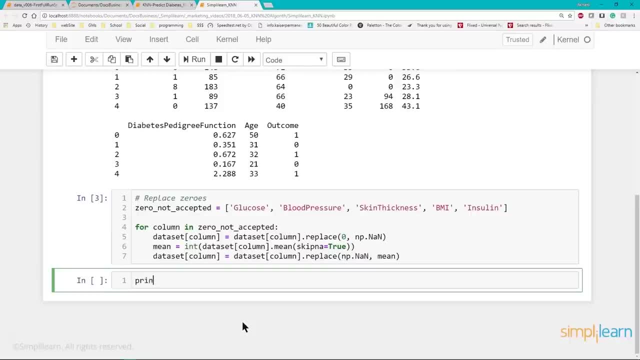 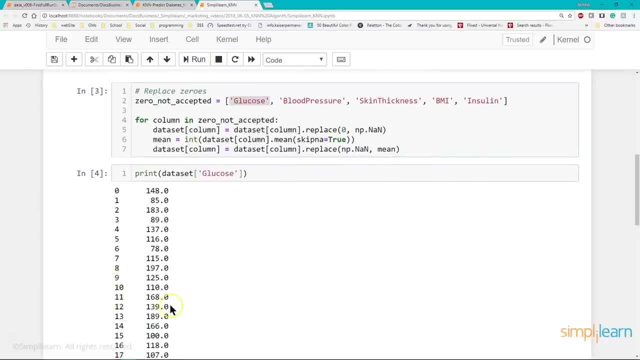 that let's go into our data set, let's print a data set and let's pick- in this case, let's just do glucose- and if I run this, this is going to print all the different glucose levels going down and we thankfully don't see anything in here that looks. 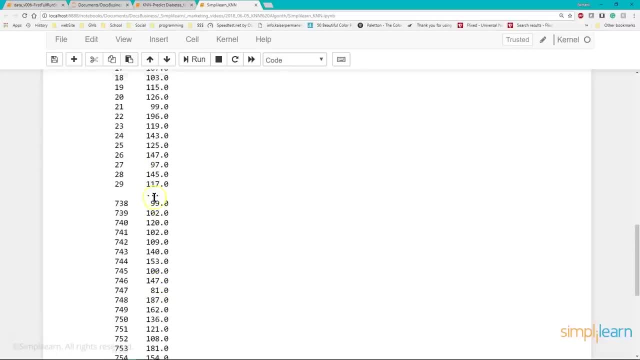 like missing data. at least on the ones it shows you can see it skipped a bunch in the middle. that's what it does: if you have too many lines in jupiter notebook, it'll skip a few and go on to the next in a data set. let me go. 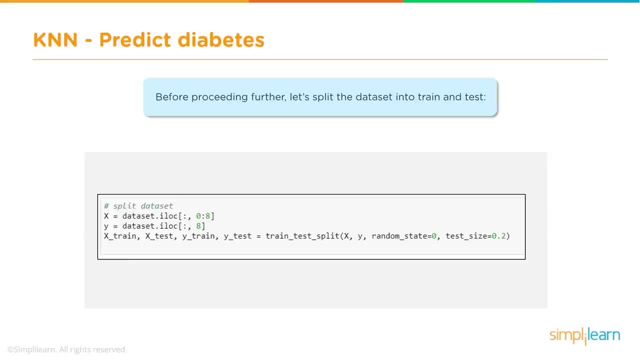 and remove this and we'll just zero out that. and, of course, before we do any processing, before proceeding any further, we need to split the data set into our train and testing data. that way we have something to train it with and something to test it on. and you're going to notice, we did a little something here with the. 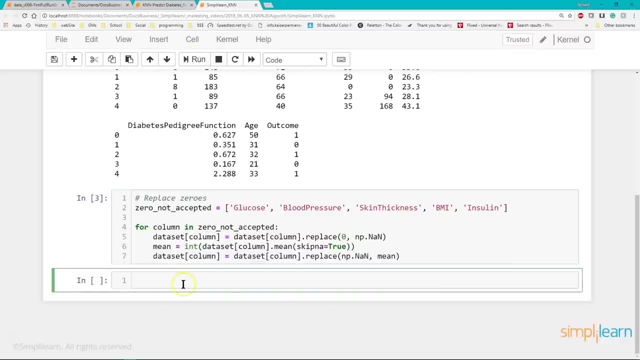 Let's go ahead and take this and we'll go ahead and run. it Doesn't actually do anything, so we're still preparing our data. If you want to see what that looks like, we don't have anything in the first few lines. 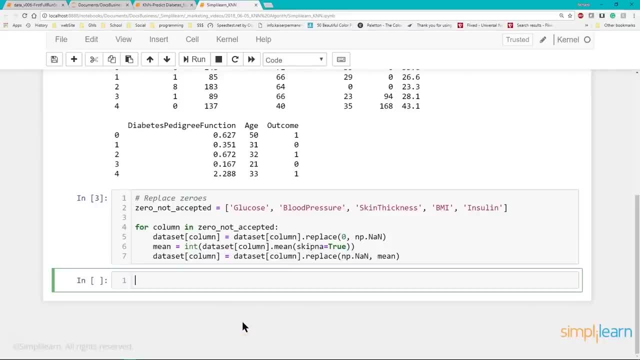 It's not going to show up, but we certainly could look at a row. Let's do that. Let's go into our data set, Let's print a data set and let's pick. in this case, let's just do glucose And if I run this, this is going to print all the different glucose levels going. 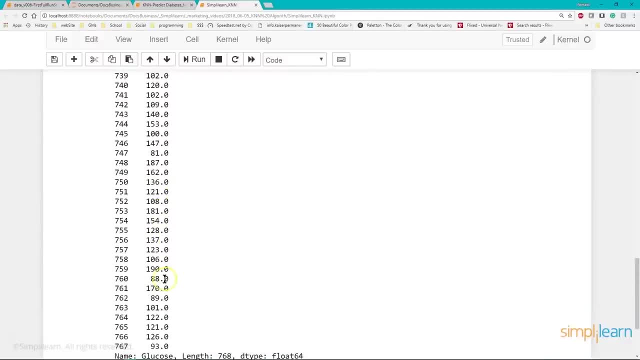 down and we thankfully don't see anything in here that looks like missing data, at least on the ones that shows you can see it skipped a bunch in the middle, Because that's what it does If you have too many lines in Jupyter Notebook. 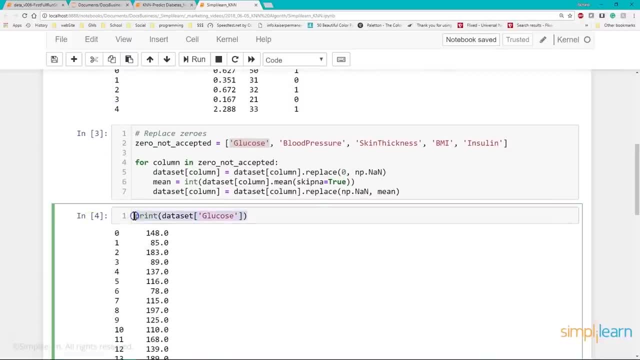 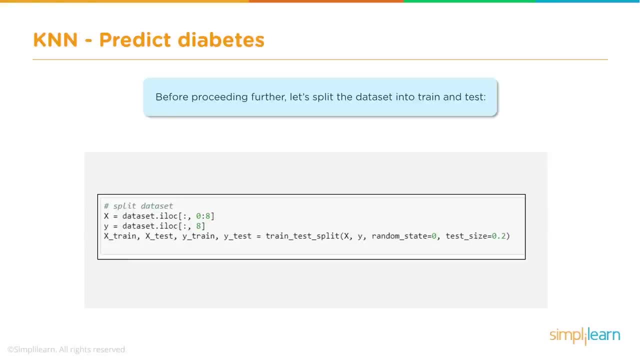 it'll skip a few and go on to the next in a data set. Let me go and remove this and we'll just zero out that. And, of course, before we do any processing, before proceeding any further, we need to split the data set into our train and testing data. 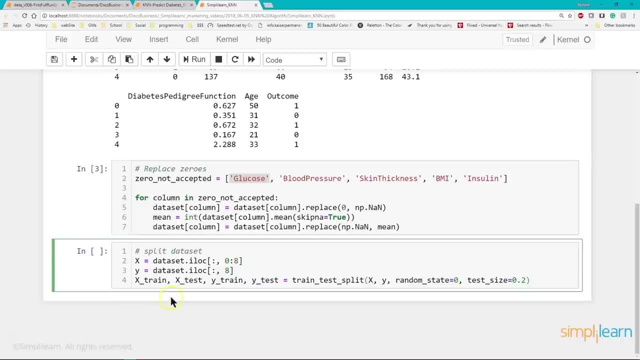 That way we have something to train it with and something to test it on. And you're going to notice, we did a little something here with the Pandas database code. There we go, my drawing tool. We've added in this right here, off the data set. 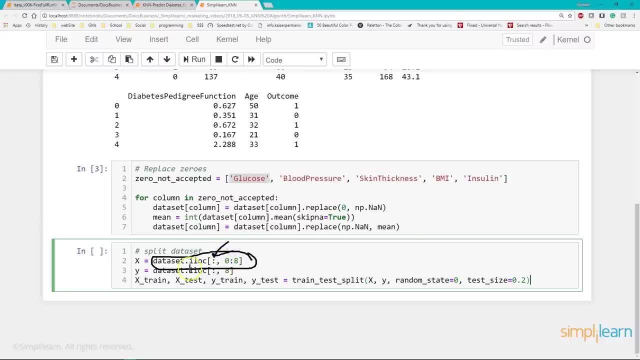 And what this says is that the first one in Pandas- this is from the PD Pandas- It's going to say, within the data set, we want to look at the I location and it is all rows. That's what that says. 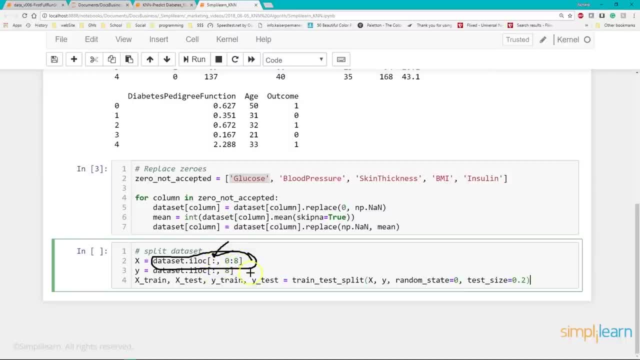 So we're going to keep all the rows, but we're only looking at zero columns, zero to eight. Remember column nine? Here? it is right up here. We put it in here as outcome. Well, that's not part of the training data. 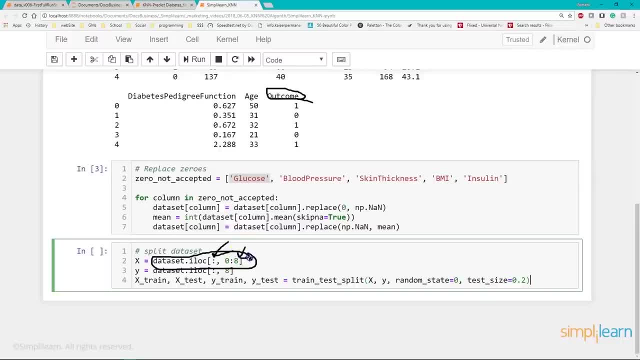 That's part of the answer. Yes, column nine, but it's listed as eight number eight. So zero to eight is nine columns. So eight is the value And when you see it in here, zero. this is actually zero to seven. 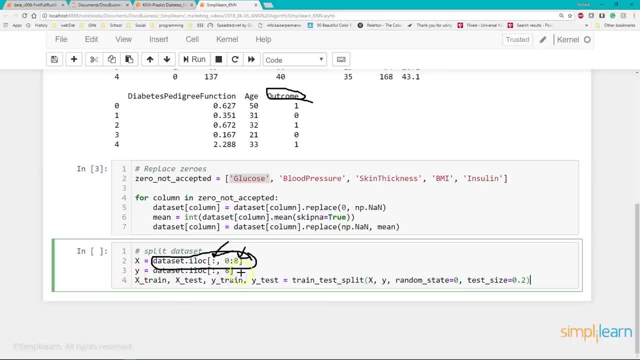 It doesn't include the last one. And then we go down here to Y, which is our answer, And we want just the last one, just column eight, And you can do it this way with this particular notation. And then, if you remember, we imported the train test split. 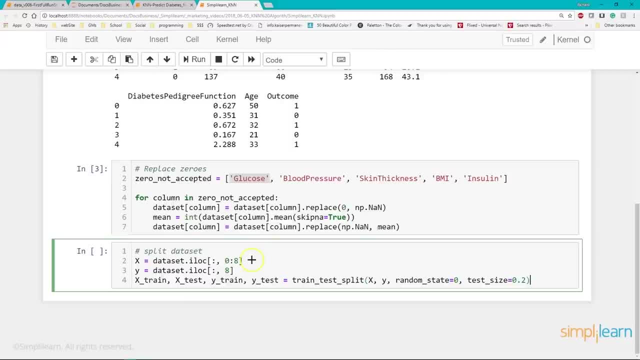 pandas database code. there we go, my drawing tool. we've added in this right here off the data set, and what this says is that the first one in pandas- this is from the pd pandas. it's going to say within the data set, we want to look at the i location. 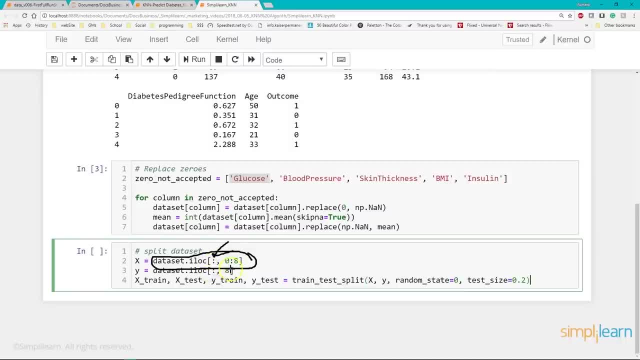 and it is all rows. that's what that says. so we're going to keep all the rows, but we're only looking at zero, column zero to eight. remember column nine? here it is right up here, we printed it in. here is outcome. well, that's not part of the training. 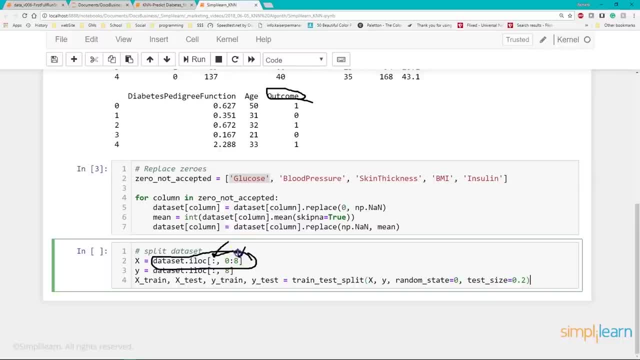 data. that's part of the answer. yes, column nine, but it's listed as eight number eight. so zero to eight is nine columns. so eight is the value and when you see it in here, zero. this is actually zero to seven. it doesn't include the last one. 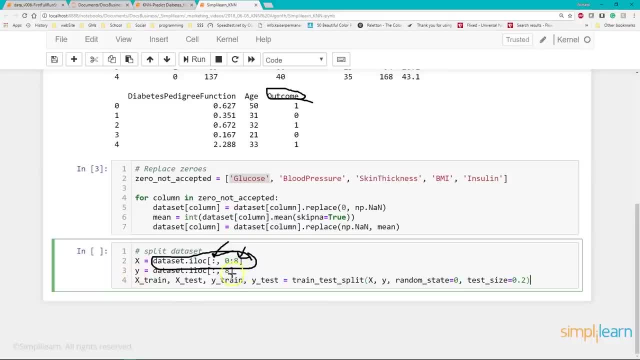 and then we go down here to y, which is our answer, and we want just the last one, just column eight, and you can do it this way with this particular notation. and then, if you remember, we imported the train test split. that's part of the sk learn. 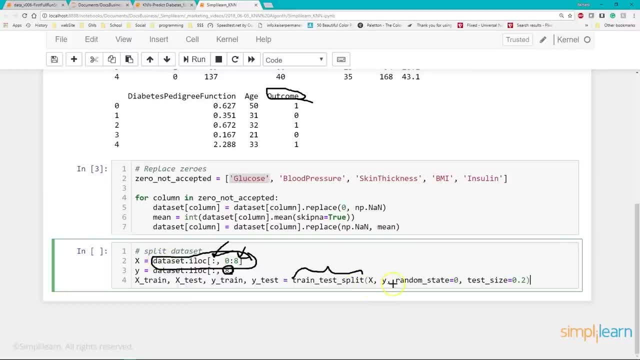 right there and we simply put in our x and our y. we're going to do random. state equals zero. you don't have to necessarily seed it. that's a seed number. i think the default is one when you seed it. i have to look that up. and then the 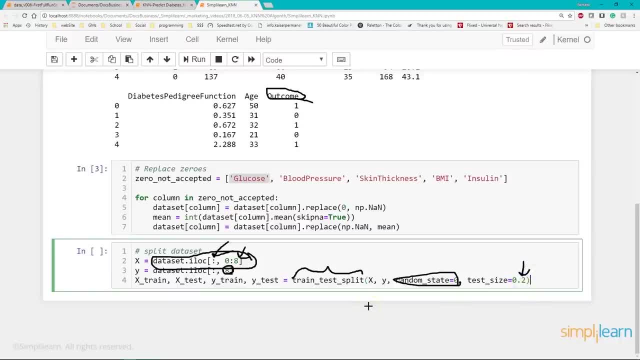 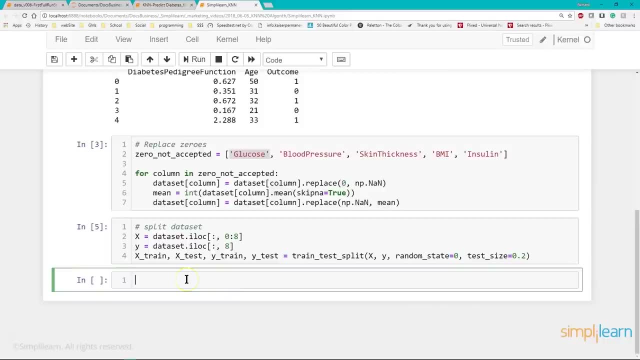 test size. test size is point two. that simply means we're going to take twenty percent of the data and put it aside so that we can test it later. that's all that is, and again we're going to run it. not very exciting. so far we haven't had any print. 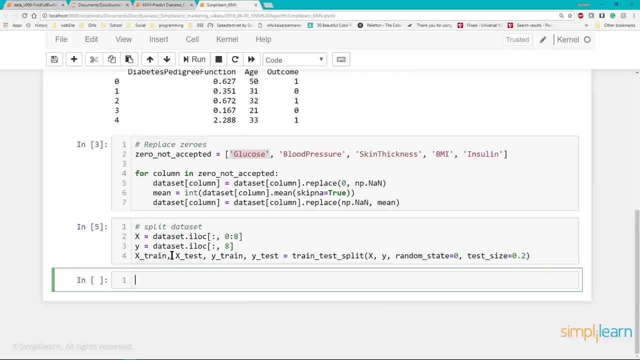 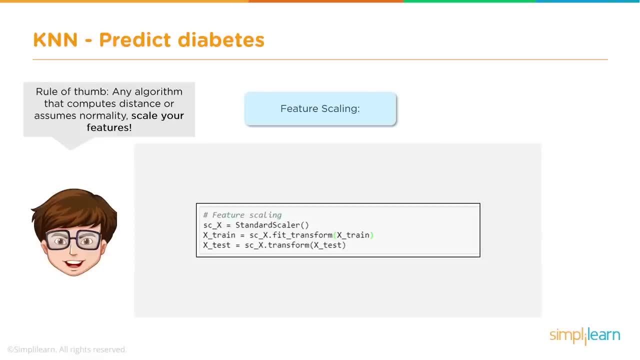 out other than to look at the data. but that is a lot of. this is prepping this data. once you prep it, the actual lines of code are quick and easy and we're almost there. but the actual running of our knn, we need to go ahead and do. 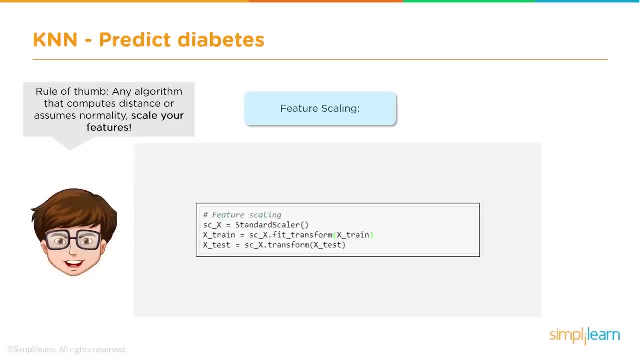 scale the data. if you remember correctly, we're fitting the data in a standard scalar, which means, instead of the data being from, you know, five to three hundred and three in one column, and the next column is one to six. we're going to set that all so that all the data 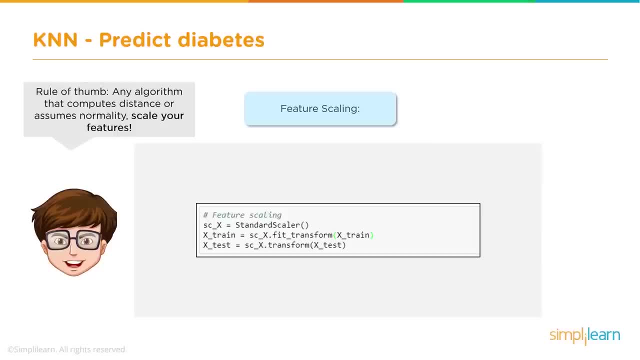 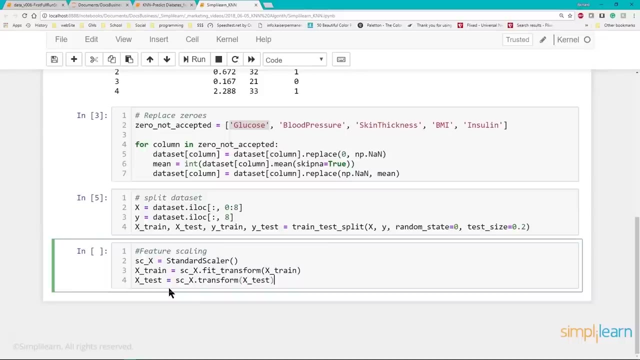 is between minus one and one. that's what that standard scalar does, keeps it standardized, and we only want to fit the scalar with the training set. but we want to make sure the testing set is the x test going in is also transformed, so it's processing it the same. so 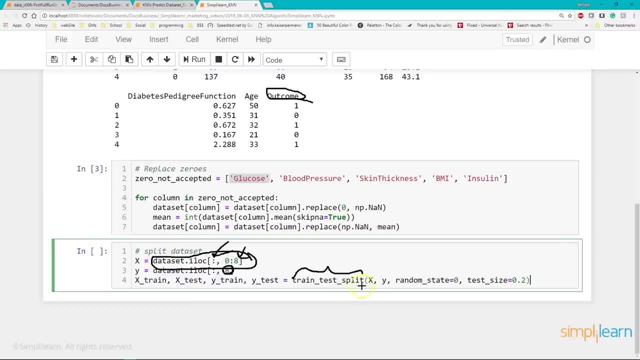 That's part of the SKLearn right there And we simply put in our X and our Y. We're going to do random state equals zero. You don't have to necessarily seed it. That's a seed number. I think the default is one when you seed it. 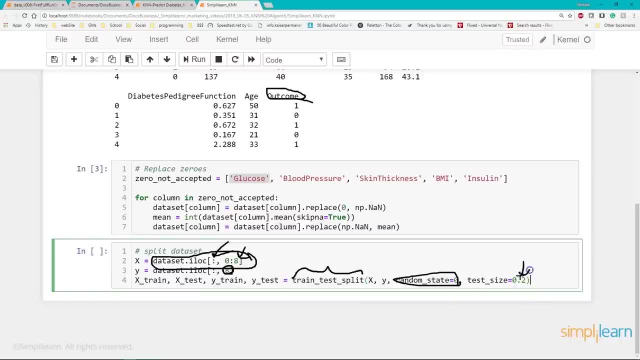 I'd have to look that up. And then the test size. test size is 0.2.. That simply means we're going to take 20% of the data and put it aside so that we can test it later. That's all that is. 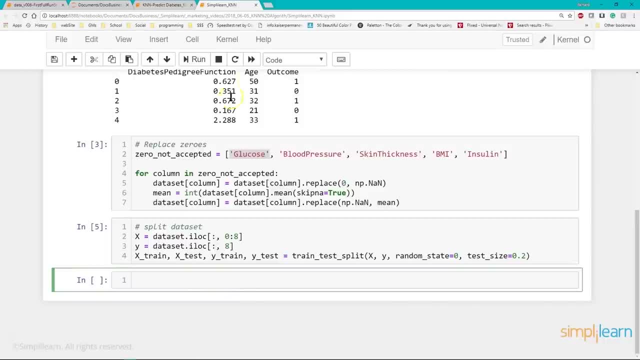 And again, we're going to run it. Not very exciting. So far we haven't had any printout other than to look at the data. But that is a lot of. this is prepping this data. Once you prep it, the actual lines of code are quick and easy. 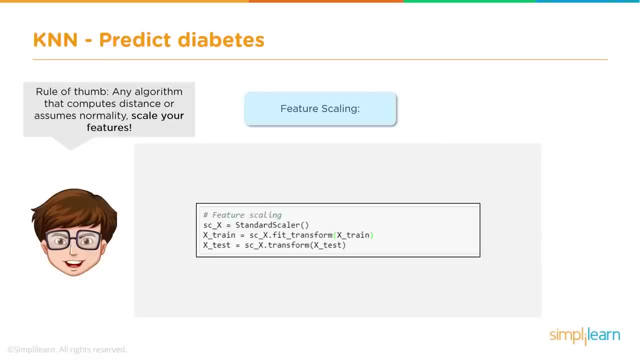 And we're almost there, But the actual running of our KNN. we need to go ahead and do a scale the data. If you remember correctly, we're fitting the data in a standard scaler, which means, instead of the data being from, you know, five to three hundred and three in one. 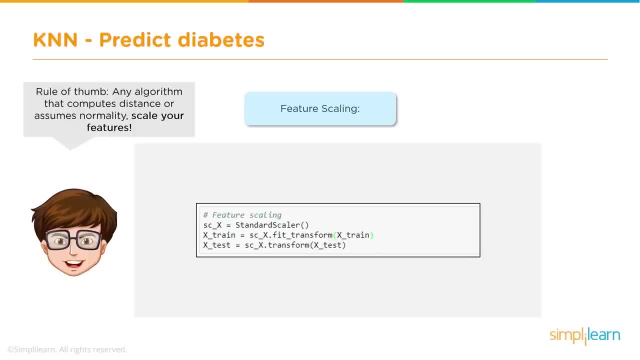 column and the next column is one to six. we're going to set that all so that all the data is between minus one and one. That's what that standard scaler does, Keeps it standardized, And we only want to fit the scaler with the training set. 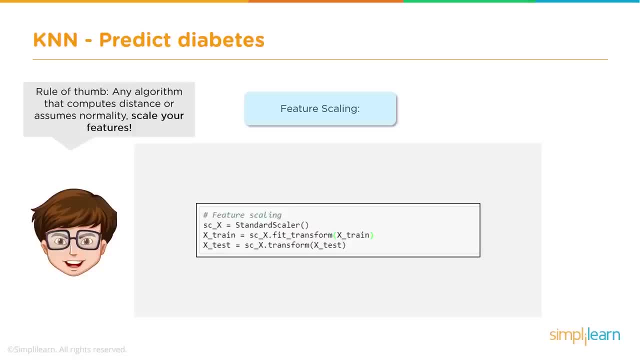 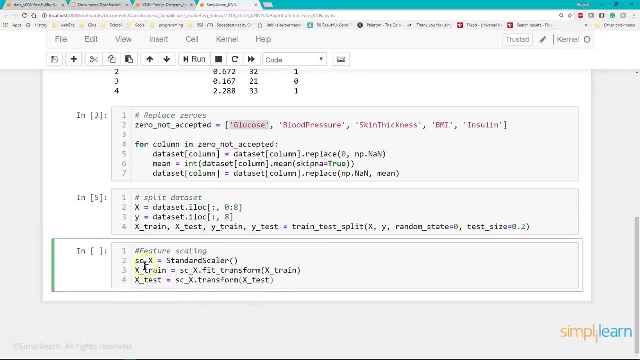 But we want to make sure the testing set is the X test going in is also transformed, So it's processing it the same. So here we go with our standard scaler. We're going to call it SC underscore X for the scaler And we're going to import the standard scaler into this variable. 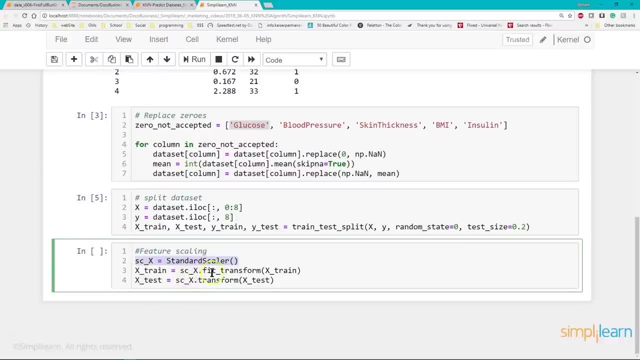 And then our X train equals SC, underscore X, dot, fit, transform. So we're creating the scaler on the X train variable And then our X test. we're also going to transform it. So we've trained and transformed the X train And then the X test isn't part of that training. 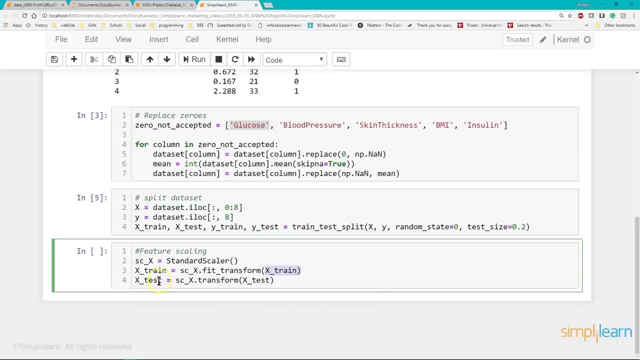 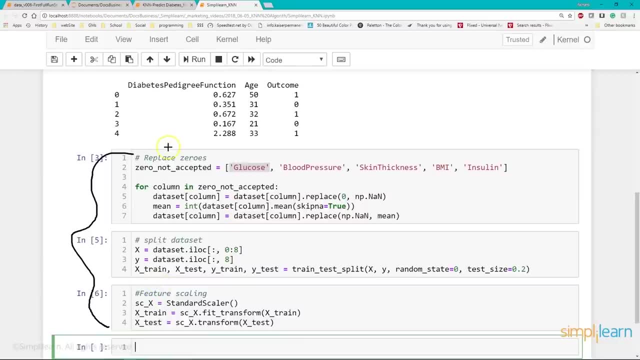 It isn't part of training the transformer. It just gets transformed. That's all it does. And again, we're going to go and run this And, if you look at this, we've now gone through these steps, all three of them. 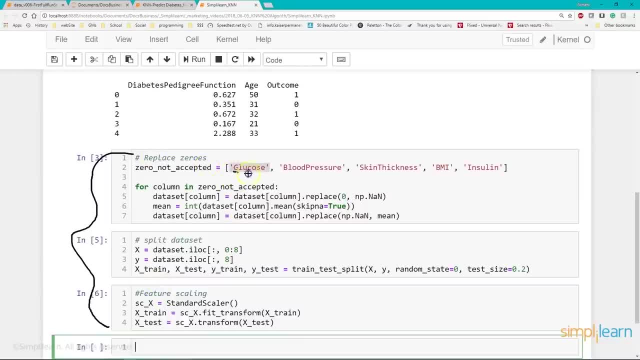 We've taken care of replacing our zeros for key columns that shouldn't be zero And we replace that with the means of those columns, that way that they fit right in with our data models. We've come down here and we split the data, So now we have our test data and our training data. 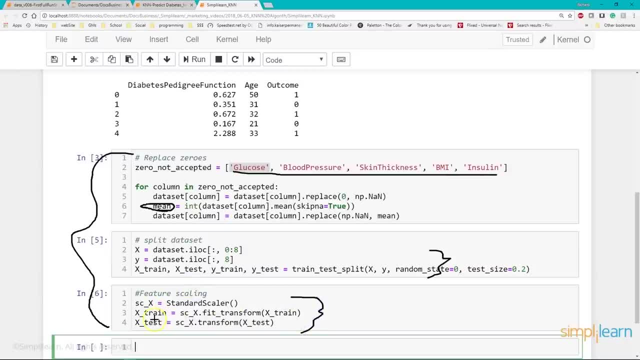 And then we've taken and we scaled the data. So all of our data going in? No, no, we don't. We don't train the Y part, The Y train and Y test. That never has to be trained. It's only the data going in. 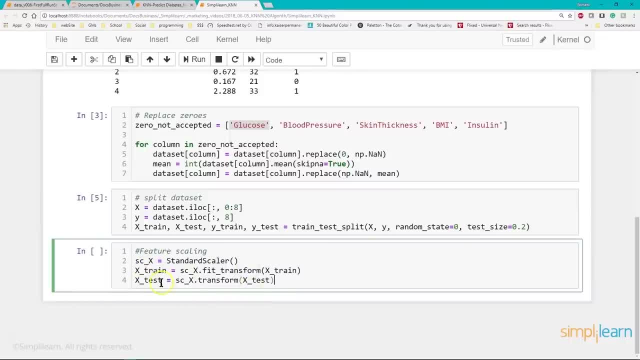 here we go with our standard scalar. we're going to call it sc underscore x for the scalar and we're going to import the standard scalar into this variable and then our x train equals sc underscore x, dot fit transform. so we're creating the scalar on the x train variable. 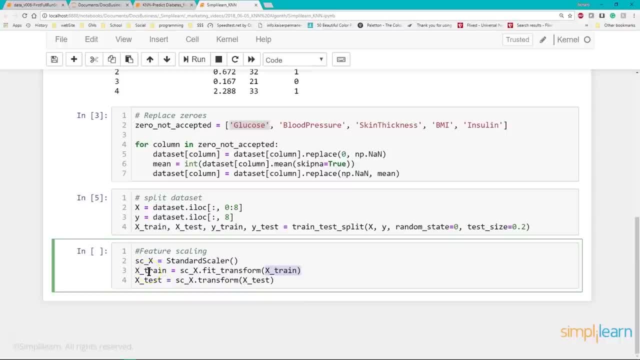 and then our x test. we're also going to transform it. so we've trained and transformed the x train and then the x test isn't part of that training. it isn't part of training the transformer. it just gets transformed. that's all it does, and again, we're going to go ahead and run. 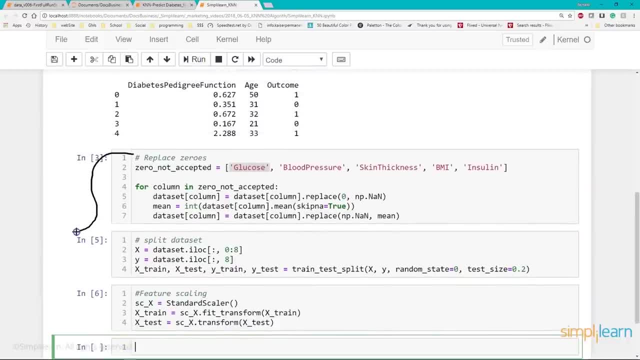 this and, if you look at this, we've now gone through these steps, all three of them. we've taken care of replacing our zeros for key columns that shouldn't be zero and we replace that with the means of those columns, that way that they fit right in with our data model. 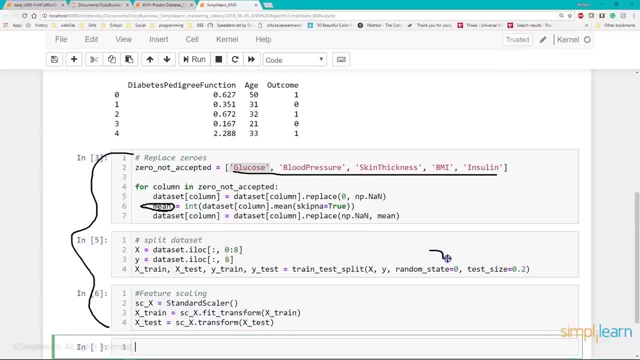 we've come down here and we've split the data, so now we have our test data and our training data and then we've taken and we've scaled the data, so all of our data going in now. no, we don't train the y part, the y train 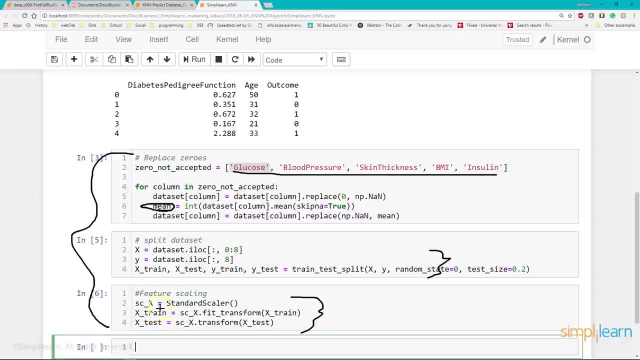 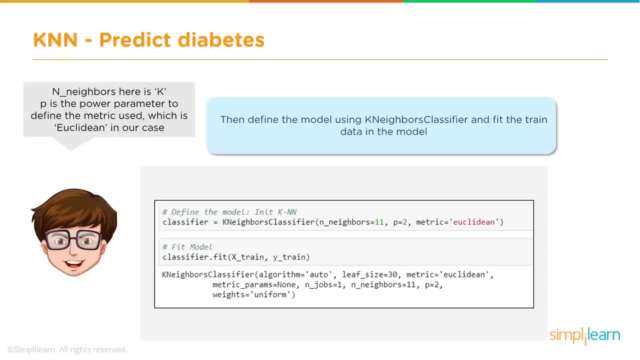 and y test. that never has to be trained, it's only the data going in. that's what we want to train in there. then define the model using k-neighbors classifier and fit the train data in the model. so we do all that data prep and you can. 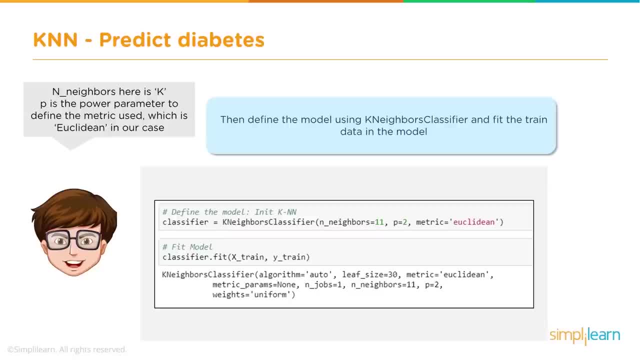 see down here we're only going to have a couple lines of code where we're actually building our model and training it. that's one of the cool things about python and how far we've come. it's such an exciting time to be in machine learning because there's so many 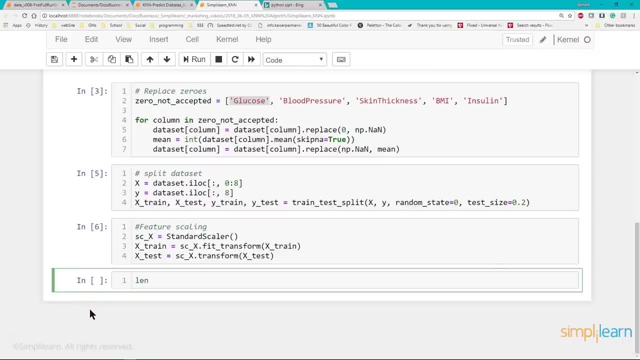 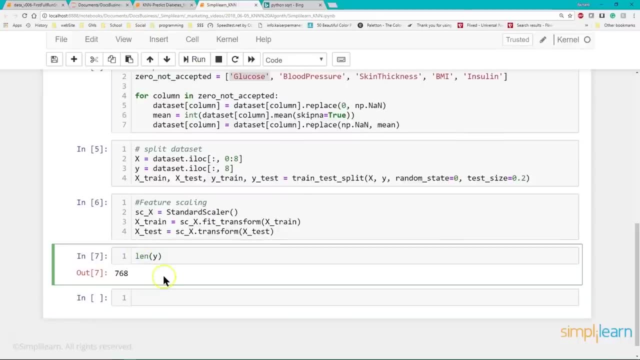 automated tools. let's see before we do this: let's do a quick length of and let's do y. we want. let's just do length of y and we get 768. and if we import math, we do math, dot square root. let's do y train. there we go. it's actually 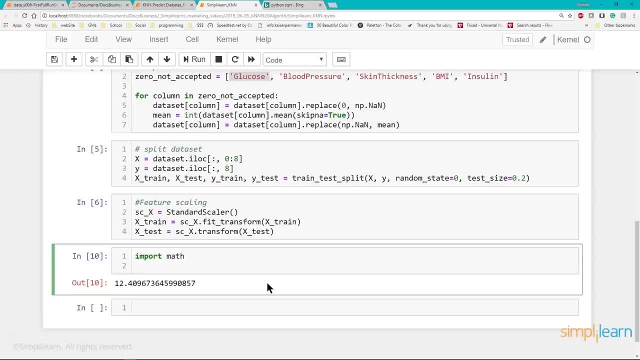 going to be x train. before we do this, let's go ahead and do import math and do math square root length of y test, and when i run that we get 12.409. i want to show you where this number comes from. we're about to use. 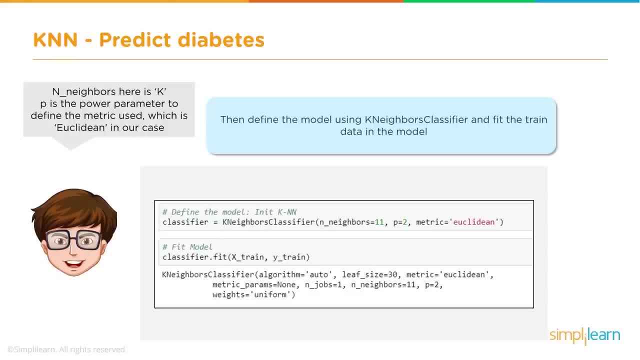 That's what we want to train in there. Then define the model using KNeighbors classifier and fit the train data in the model. So we do all that data prep And you can see down here we're only going to have a couple of lines. 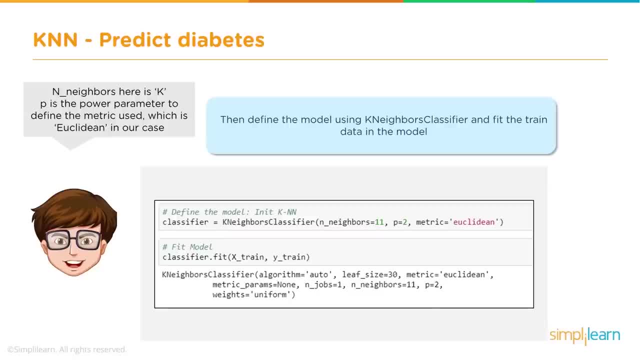 of code, where we're actually building our model and training it. That's one of the cool things about Python and how far we've come. It's such an exciting time to be in machine learning because there's so many automated tools. Let's see. before we do this, let's do a quick length of 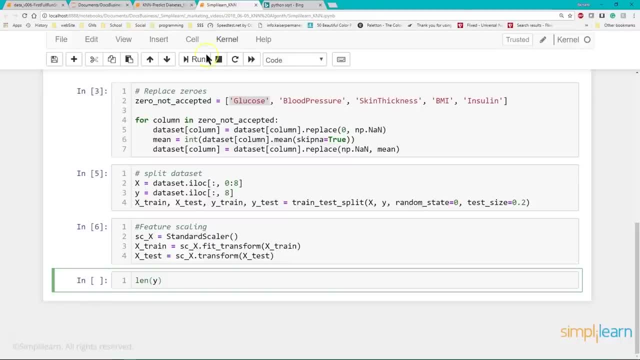 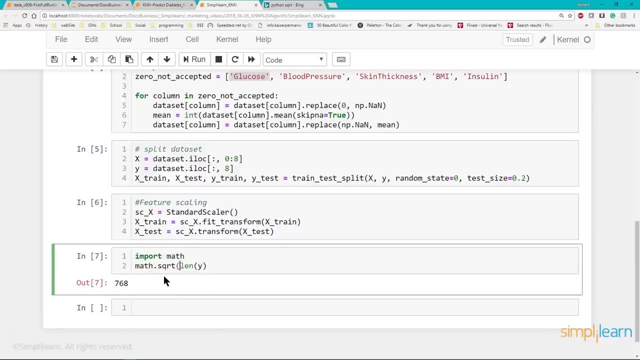 And let's do Y we want. let's just do length of Y and we get 768.. And if we import math, we do math dot square root. Let's do Y train. There we go. It's actually supposed to be X train. 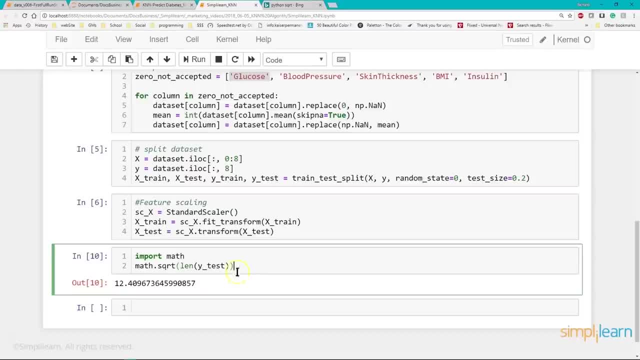 Before we do this, let's go ahead and do import math and do math square root length of Y test. And when I run that we get 12.409.. I want to show you where this number comes from. we're about to use. 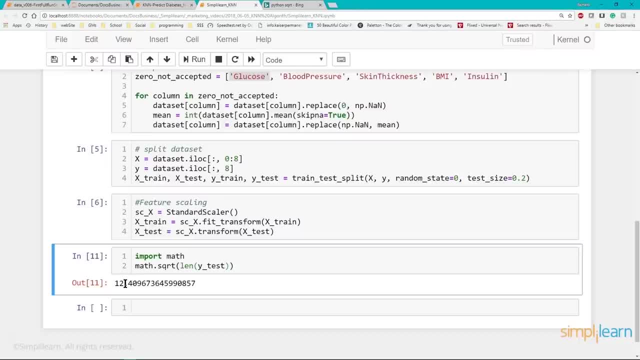 12 is an even number, So if you know, if you're ever voting on things, remember the neighbors all vote. Don't want to have an even number of neighbors voting, So we want to do something odd And let's just take one away. We'll make it 11.. 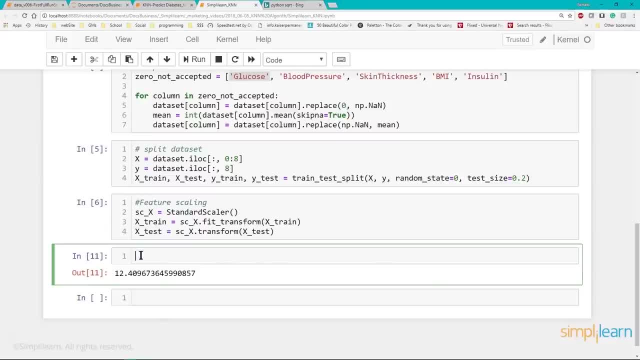 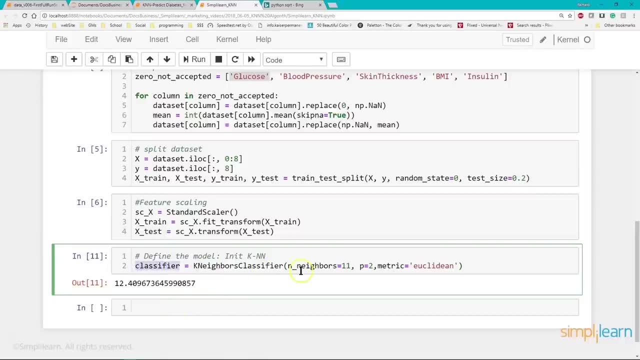 Let me delete this out of here. That's one of the reasons I love Jupyter Notebook, because you can flip around and do all kinds of things on the fly. So we'll go ahead and put in our classifier. We're creating our classifier now and it's going to be the K neighbors classifier. 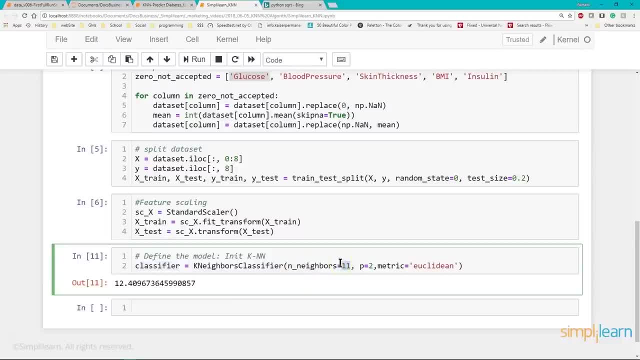 N neighbors equal 11.. Remember, we did 12 minus 1 for 11.. We have an odd number of neighbors. P equals 2, because we're looking for is it, are they diabetic or not? And we're using the Euclidean metric. 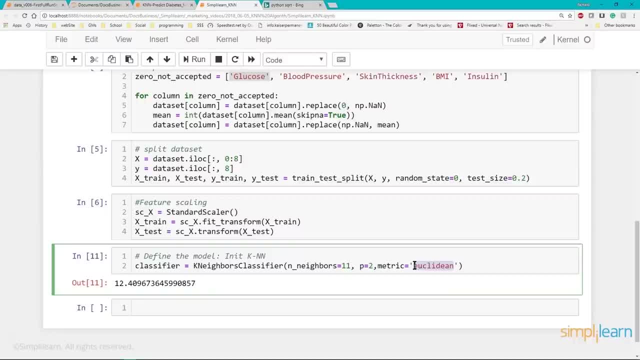 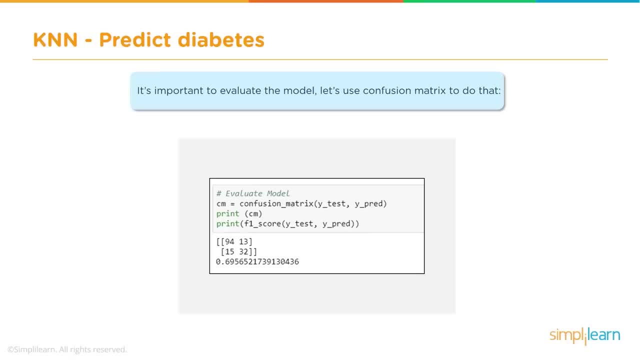 There are other means of measuring the distance. You could do like square. square means values. all kinds of measure this, But the Euclidean is the most common one and it works quite well. It's important to evaluate the model. Let's use the confusion matrix to do that. 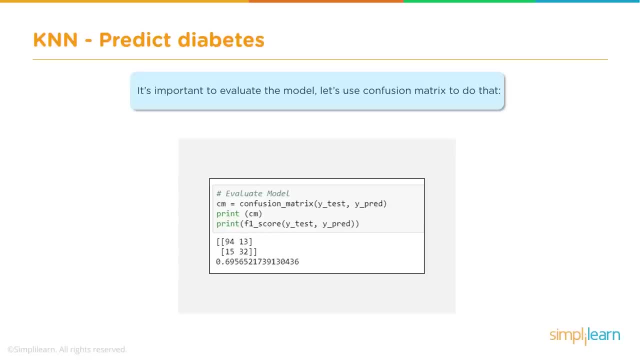 And we're going to use the confusion matrix Wonderful tool, And then we'll jump into the F1 score and, finally, accuracy score, which is probably the most commonly used quoted number when you go into a meeting or something like that. So let's go ahead and paste that in there. 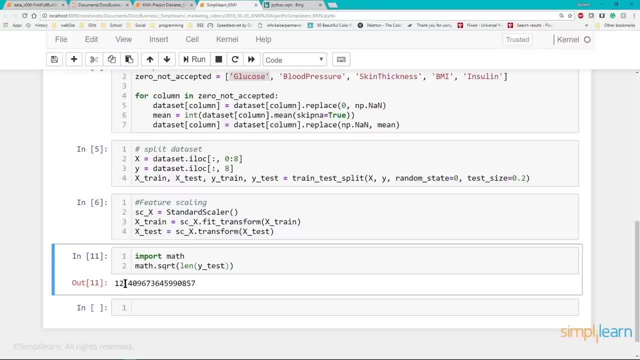 12 is an even number, so if you know, if you're ever voting on things, remember the neighbors all vote. don't want to have an even number of neighbors voting, so we want to do something odd and let's just take one away. we'll make it 11. let me delete this. 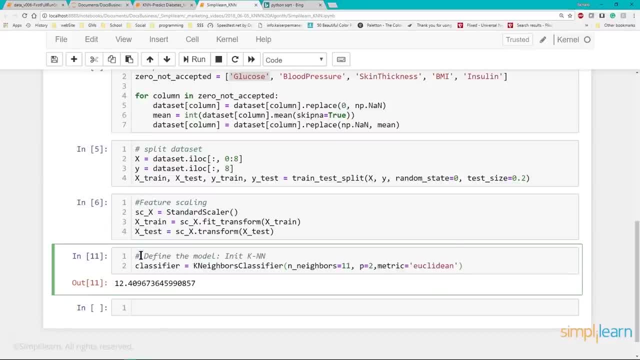 out of here. that's one of the reasons i love jupiter notebook, because you can flip around and do all kinds of things on the fly. so we'll go ahead and put in our classifier. we're creating our classifier now and it's going to be the k neighbors. 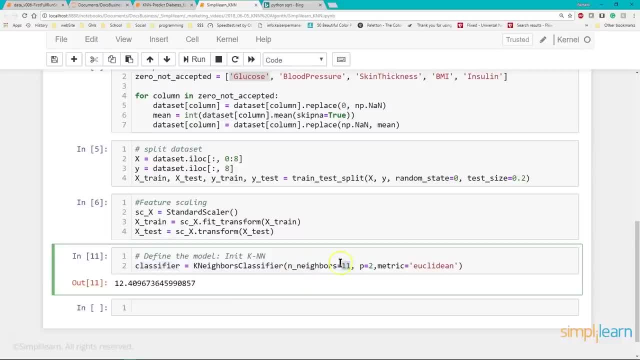 classifier: n neighbors equal 11. remember we did 12 minus 1 for 11, so we have an odd number of neighbors. p equals 2 because we're looking for is it, are they diabetic or not? and we're using the euclidean metric. there are. 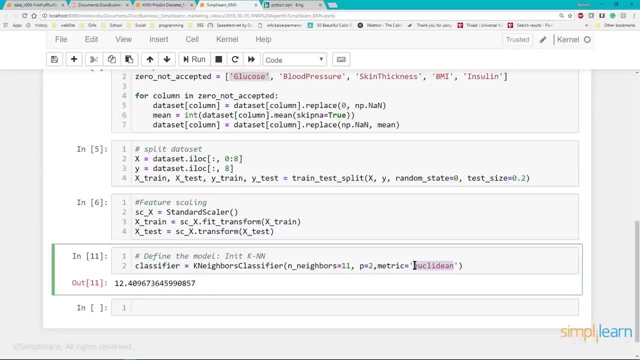 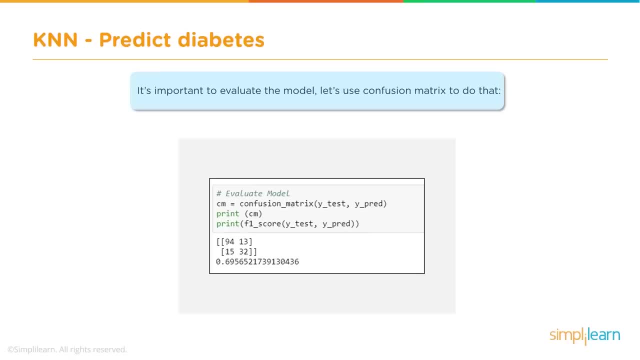 other means of measuring the distance. you could do like square. square means values, all kinds of measure this, but the euclidean is the most common one and it works quite well. it's important to evaluate the model. let's use the confusion matrix to do that, and we're going to use the confusion matrix. 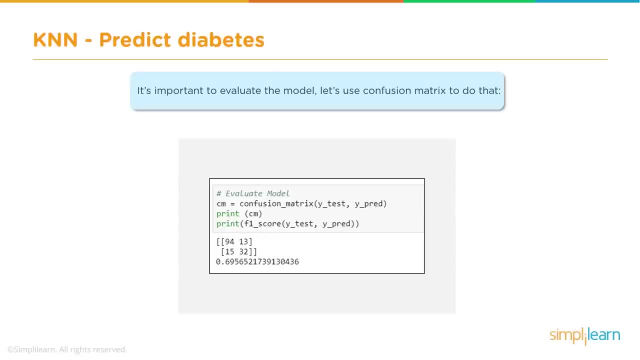 wonderful tool, and then we'll jump into the f1 score and, finally, accuracy score, which is probably the most commonly used quoted number when you go into a meeting or something like that. so let's go ahead and paste that in there and we'll set the cm equal to confusion. 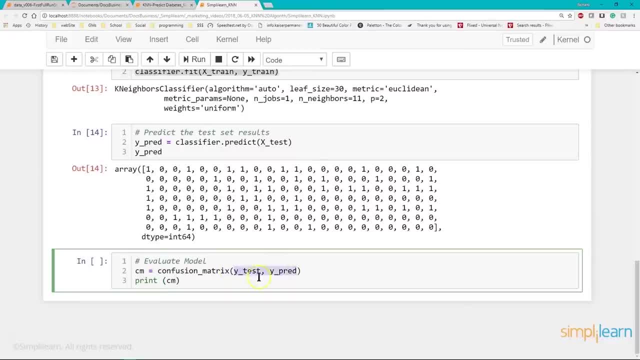 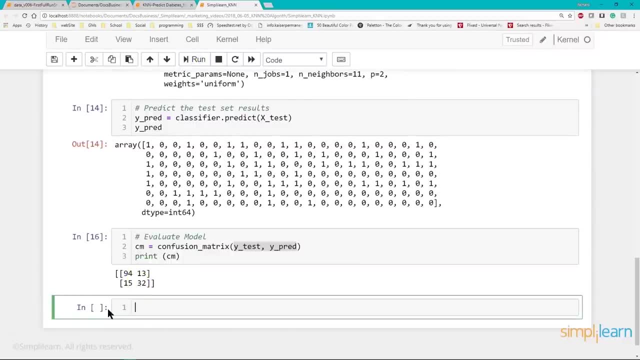 matrix: y test: y predict. so those are the two values we're going to put in there and let me go ahead and run that and print it out and the way you interpret this is: you have the y predicted, which would be your title, up here. we could do, let's just do pred. 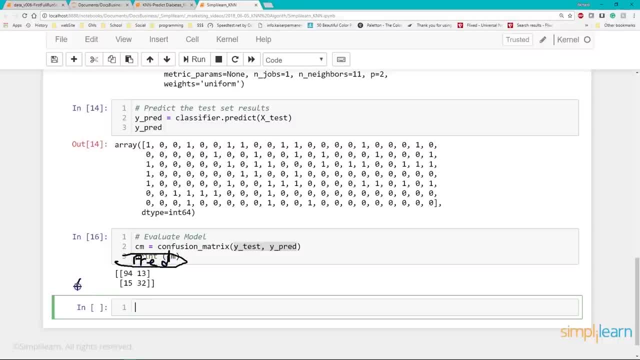 predicted across the top and actual going down. it's always hard to write in here actual. that means that this column here down the middle that's the important column and it means that our prediction said 94 and prediction and the actual agreed on 94 and 32. this 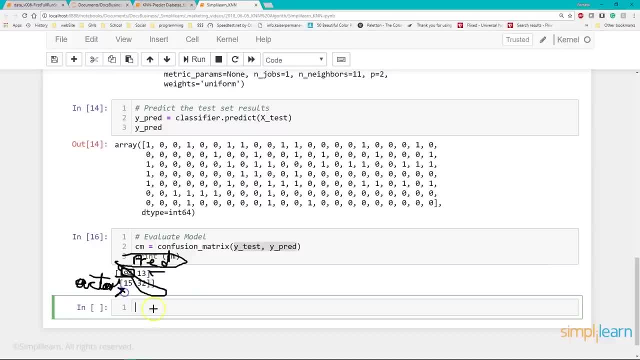 number here: the 13 and the 15. those are what was wrong, so you could have like three different. if you're looking at this across three different variables instead of just two, you'd end up with the third row down here and the column going down the middle. so 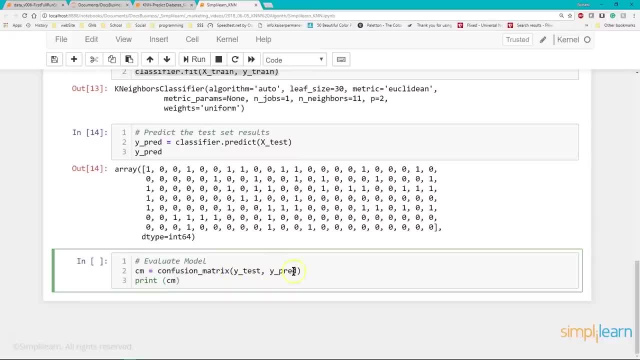 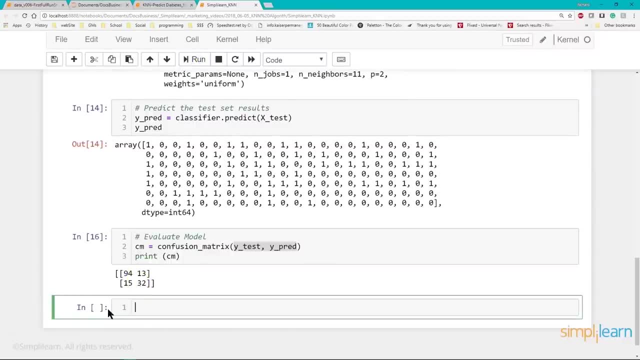 And we'll set the CM equal to confusion matrix. Why test? Why predict? So those are the two values we're going to put in there, And let me go and run that and print it out. And the way you interpret this is: you have the Y predicted. 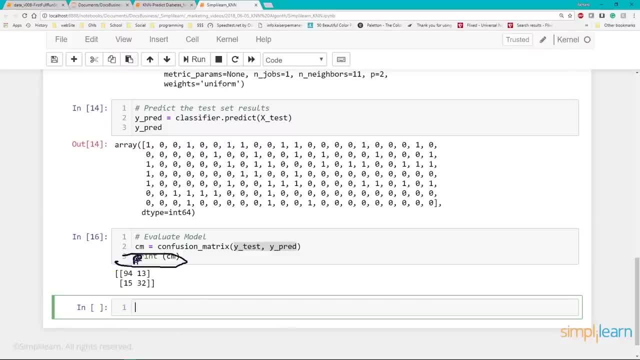 which would be your title up here. to do this is to PRED predicted across the top and actual going down. Well, it's always hard to write in here actual. That means that this column here down the middle, that's the important column. 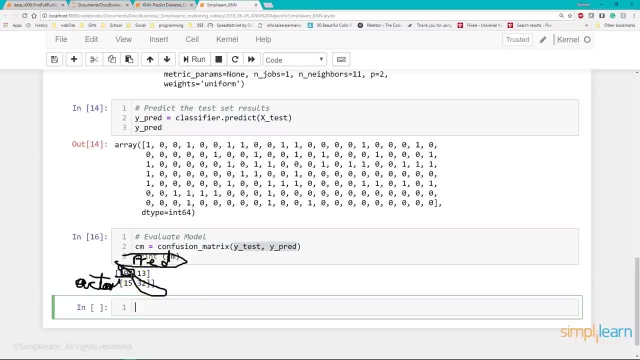 And it means that our prediction said 94 and prediction in the actual agreed on 94 and 32.. This number here, the 13 and the 15, those are what was wrong. So you could have like three different, if you're looking at this, across three. 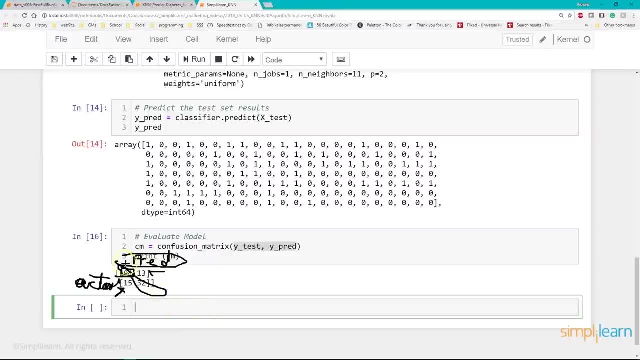 different variables instead of just two. you'd end up with the third row down here and the column going down the middle. So in the first case we have the, the, and I believe the zero is a 94.. People who don't have diabetes. 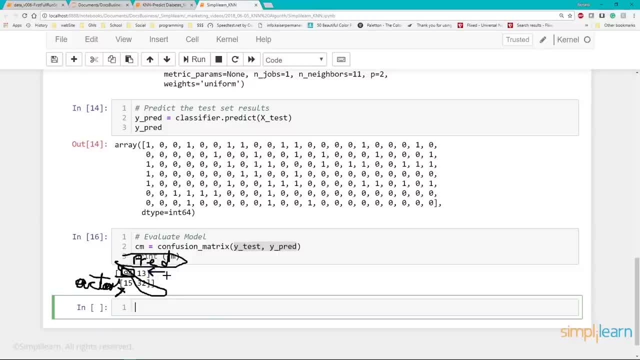 The prediction said to 13 of those people did have diabetes and were at high risk And the 32 that had diabetes had correct, But our prediction said another 15 out of that 15.. It classified as incorrect So you can see where that classification. 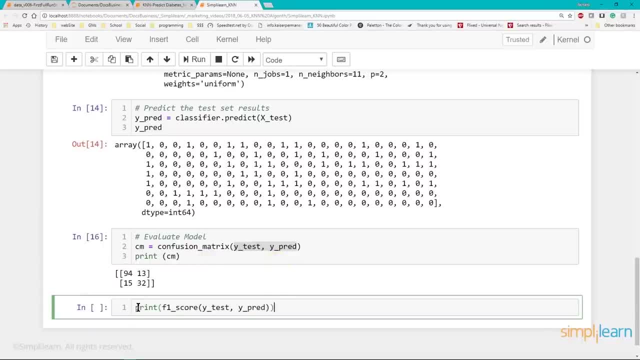 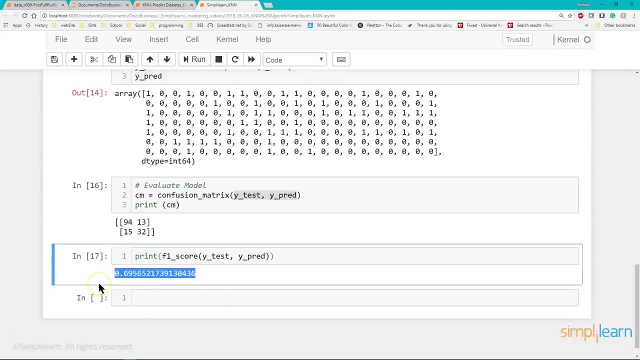 comes in and how that works on the confusion matrix, And then we're going to go ahead and print the F1 score. Let me just run that And you see we get a point six nine in our F1 score. The F1 takes into account both sides of the balance of false positives. 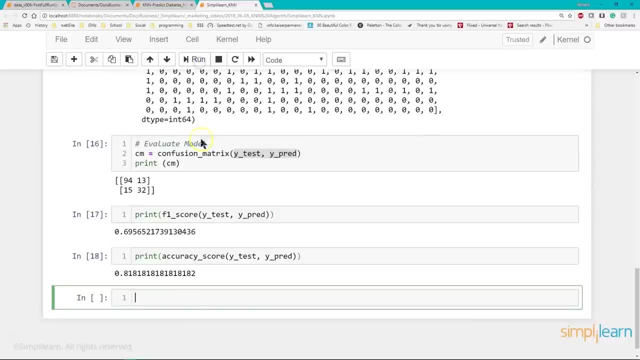 where, if we go ahead and just do the accuracy account- and that's what most people think of is, it looks at just how many we got right out of how many we got wrong. So a lot of people, when you're a data scientist and you're talking to other, 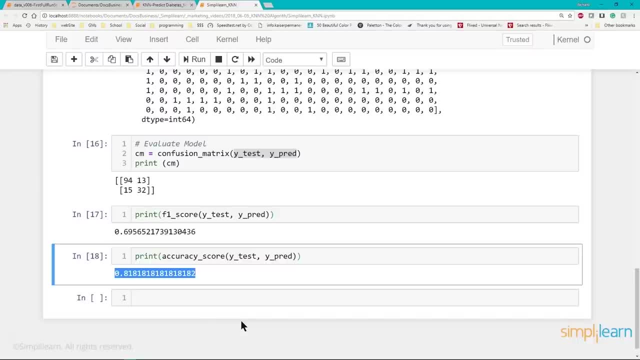 data scientists, they're going to ask you what the F1 score, the F score, is. If you're talking to the general public or the decision makers in the business, they're going to ask what the accuracy is, and the accuracy is always better than the F1 score. 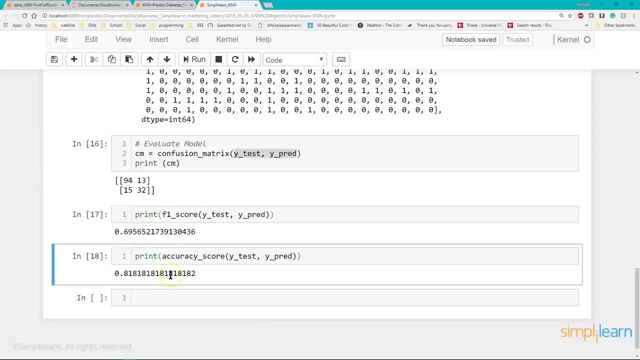 But the F1 score is more telling. It lets us know that there's more false positives than we would like on here. But 82 percent, not too bad for a quick flash. look at people's different statistics. and running an SK learn and running the KNN, the K nearest neighbor on it. 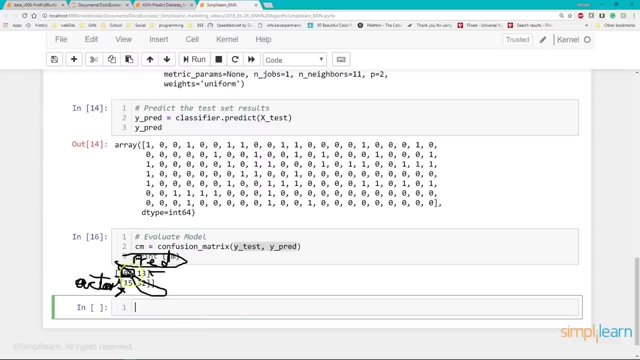 in the first case we have the and I believe the zero is a- 94 people who don't have diabetes. the prediction said that 13 of those people did have diabetes and were at high risk and the 32 that had diabetes it had correct, but our prediction said another. 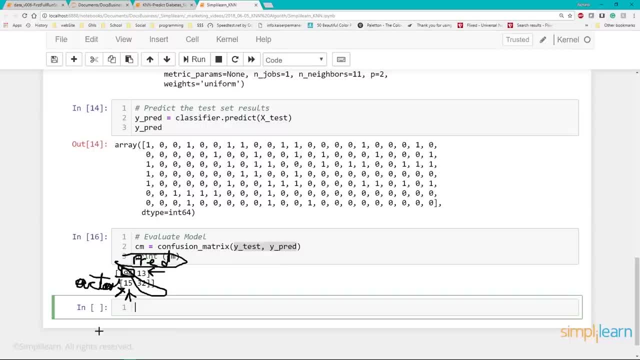 15 out of that 15. it classified as incorrect. so you can see where that classification comes in and how that works on the confusion matrix. then we're going to go ahead and print the F1 score. we just run that and you see we get a .69. 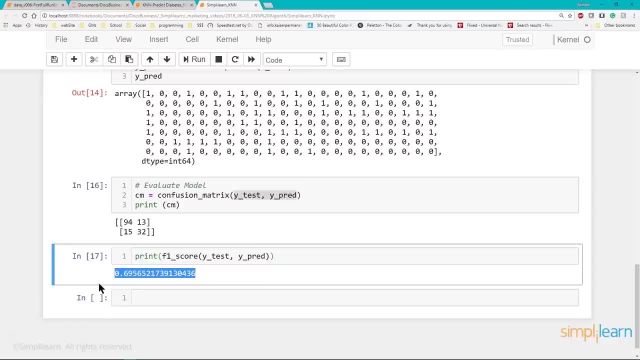 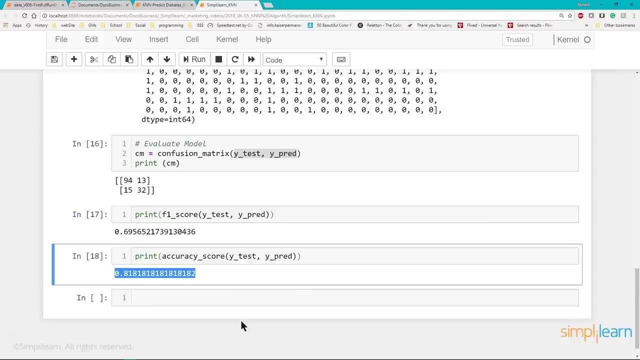 in our F1 score. the F1 takes into account both sides of the balance of false positives, where, if we go ahead and just do the accuracy account- and that's what most people think of is it looks at just how many we got right out of how many we got wrong. 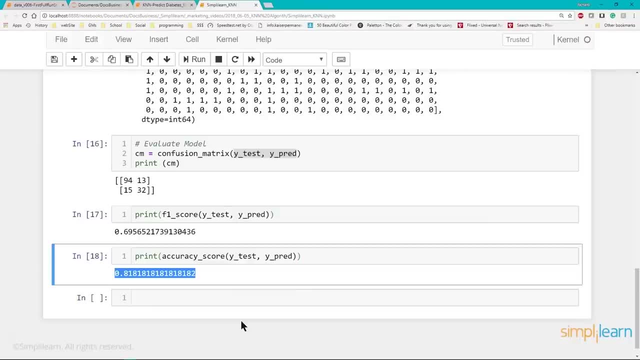 so a lot of people. when you're a data scientist and you're talking to other data scientists, they're going to ask you what the F1 score, the F score, is. if you're talking to the general public or the decision makers in the business, they're going to ask what the accuracy is. 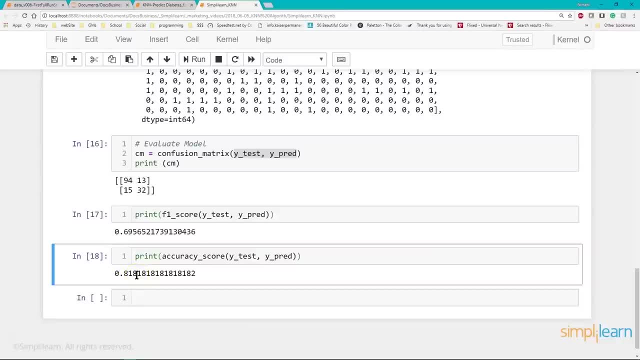 and the accuracy is always better than the F1 score. but the F1 score is more telling. it lets us know that there's more false positives than we would like on here. but 82%, not too bad for a quick flash. look at people's different. 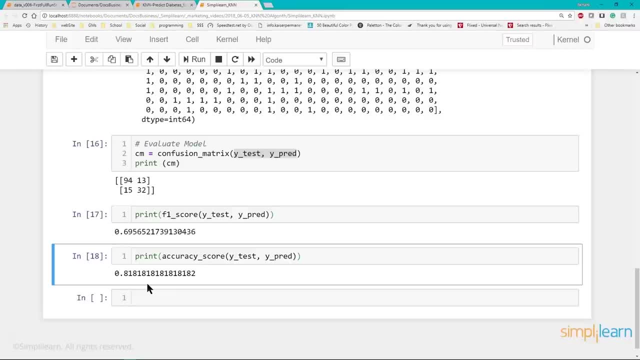 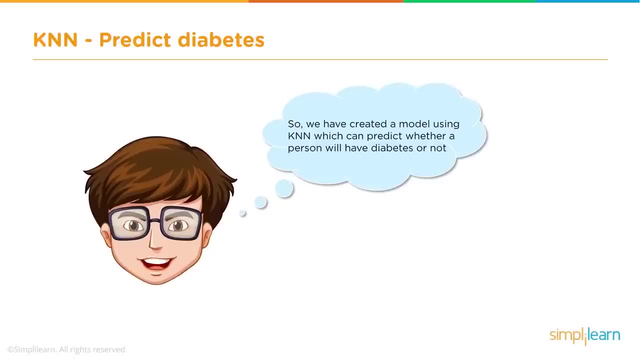 statistics and running an sklearn and running the knn, the k nearest neighbor on it. so we have created a model using knn which can predict whether a person will have diabetes or not or, at the very least, whether they should go get a check up and have their glucose checked. regularly or not. the print accuracy score we got- the .818- was pretty close to what we got and we can pretty much round that off and just say we have an accuracy. of 80% tells us it is a pretty fair fit in the model. before we dive into the SVM. 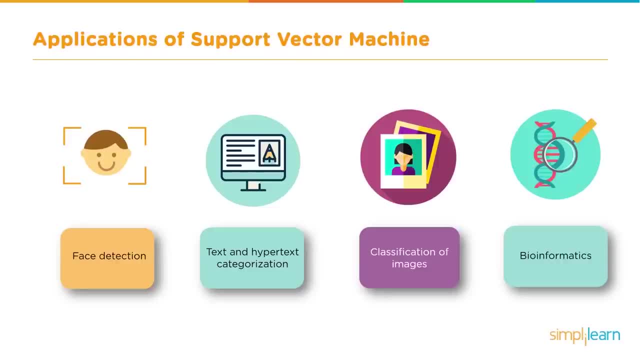 lets take a look at applications of the support vector machine, at least some general ones that are commonly used with it: face detection, text and hypertext, categorization, classification of images and bioinformatics. these are only but a few of those that are used with this SVM. as we go, 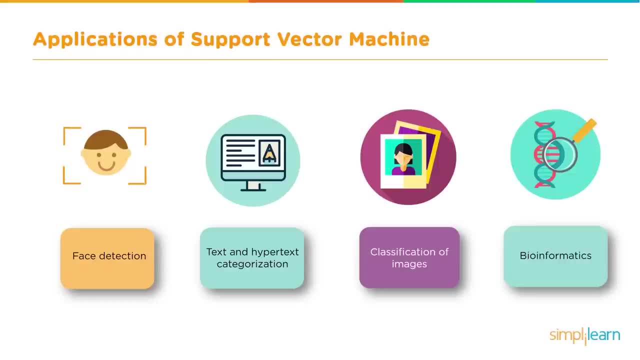 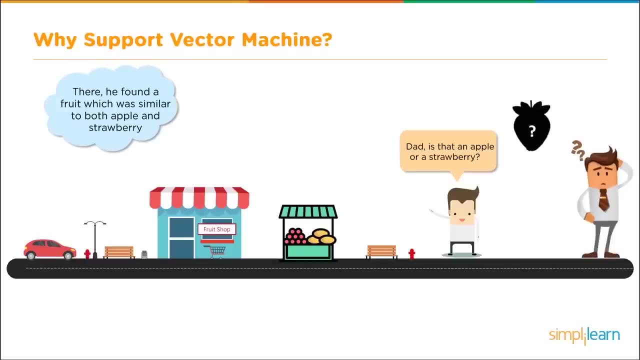 through this lesson, see if you can figure out what other ones you can apply it to and also what you would want to use some other tools for. so in this example, last week my son and I visited a fruit shop and he said: is that an apple or a strawberry? 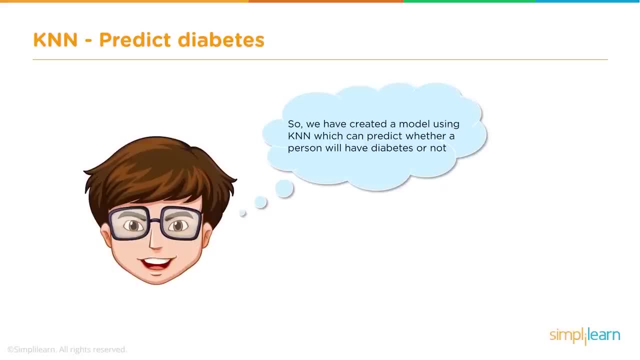 So we have created a model, using KNN, which can predict whether a person will have diabetes or not or, at the very least, whether they should go get a checkup and have their glucose checked regularly or not. The print accuracy score: We got the point eight. one eight was pretty close to what we got. 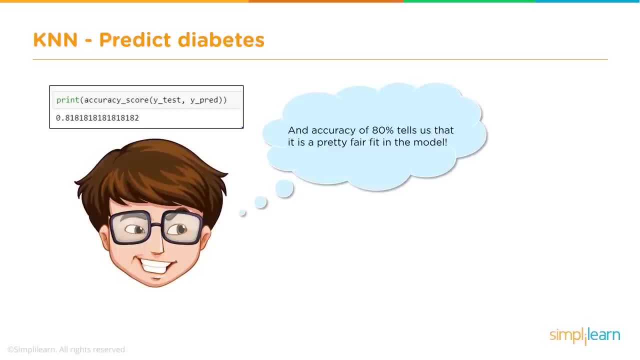 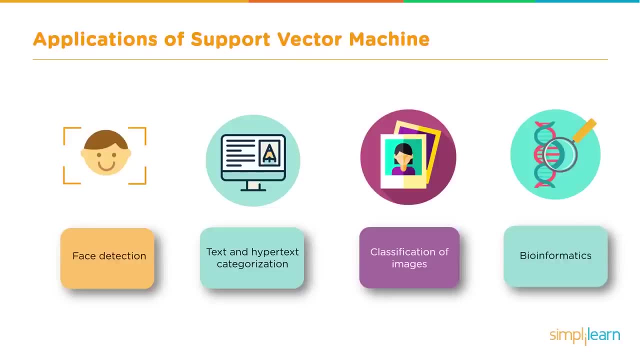 And we can pretty much round that off and just say we have an accuracy of 80 percent Tells us it is a pretty fair fit in the model. Before we dove in to the SVM, let's take a look at applications of the support vector machine, at least some general ones that are: 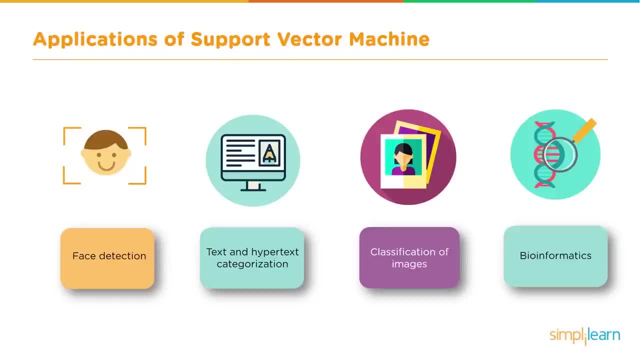 commonly used with it: face detection, text and hypertext, categorization, identification of images and bioinformatics. These are only about a few of those that are used with this SVM. As we go through this lesson, see if you can figure out what other 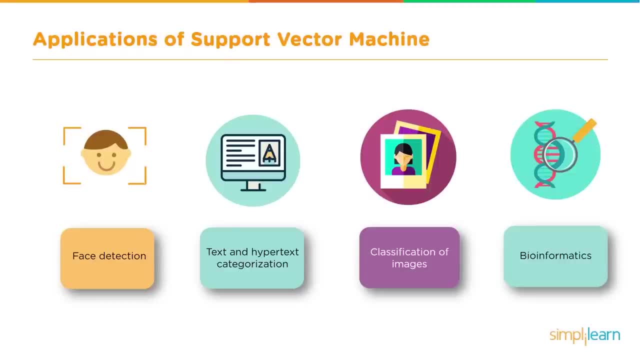 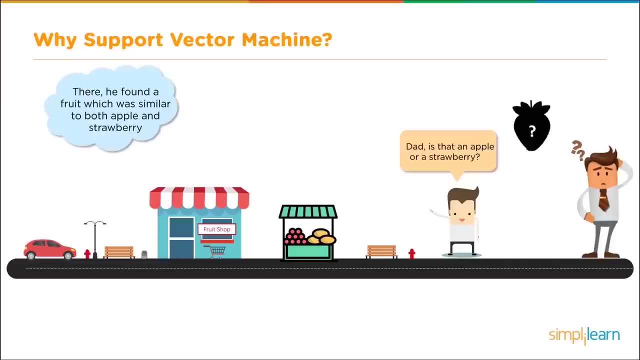 ones you could apply it to and also what you would want to use some other tools for. So in this example, last week my son and I visited a fruit shop. Dad, is that an apple or a strawberry? So the question comes up: what fruit do they just pick up from the fruit stand? 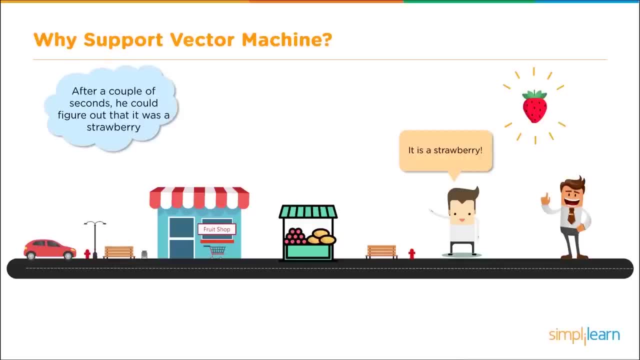 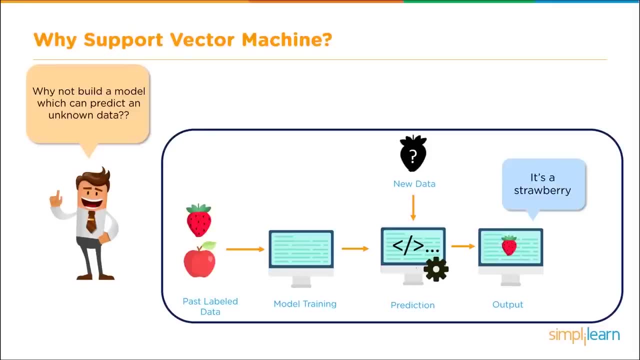 After a couple of seconds you can figure out that it was a strawberry. So let's take this model a step further and say: why not build a model which can predict an unknown data? And in this we're going to be looking at some sweet strawberries or crispy apples. 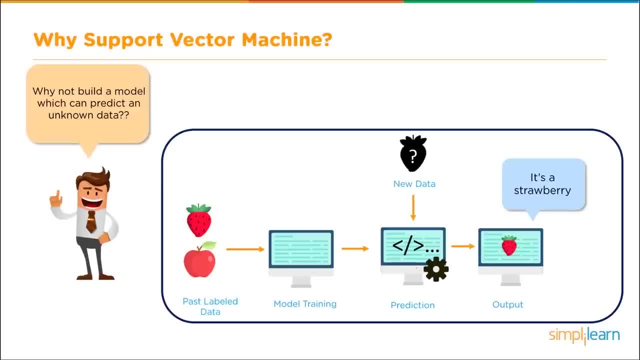 We want it to be able to label those two and decide what the fruit is, And we do that by having data already put in. So we already have a bunch of strawberries. We know our strawberries and they're already labeled as such. We already have a bunch of apples. 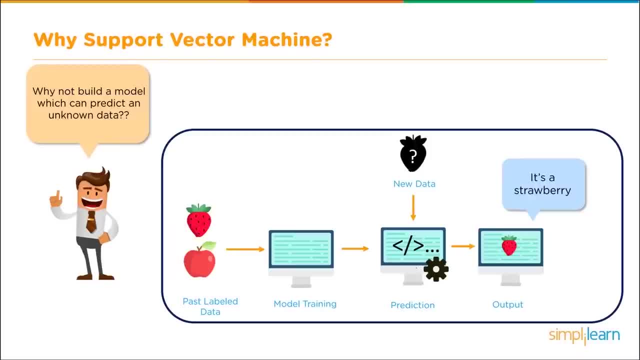 We know our apples and are labeled as such, Then once we train our model, that model then can be given the new data. And the new data is this image. In this case, you can see a question mark on it and it comes through and goes. 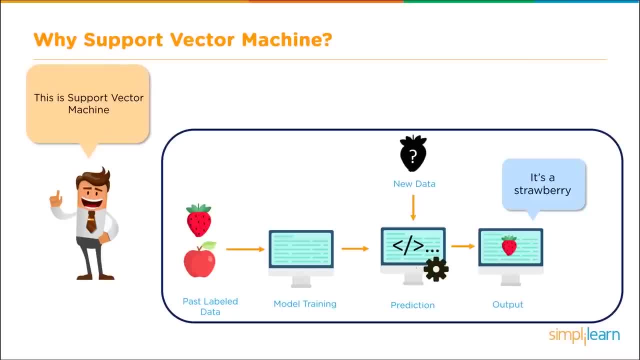 it's a strawberry. In this case, we're using the support vector machine model. SVM is a supervised learning method that looks at data and sorts it into one of two categories, And in this case we're sorting the strawberry into the strawberry side. 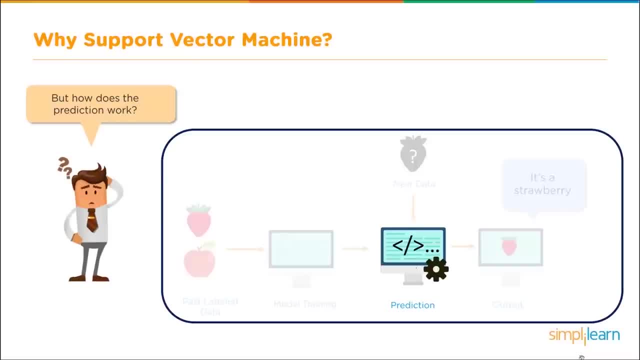 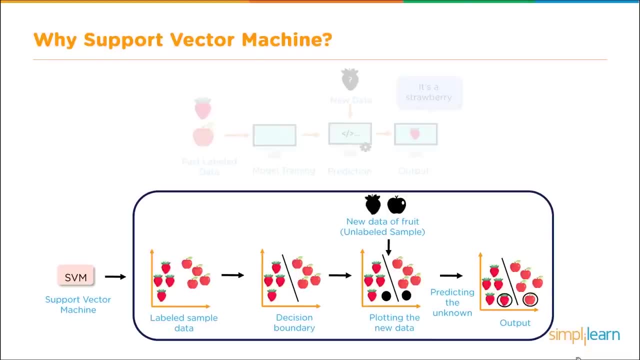 At this point you should be asking the question: how does the prediction work? Before we dig into an example with numbers, let's apply this to our fruit scenario. We have our support vector machine, We've taken it and we've taken labeled sample of data: strawberries and apples. 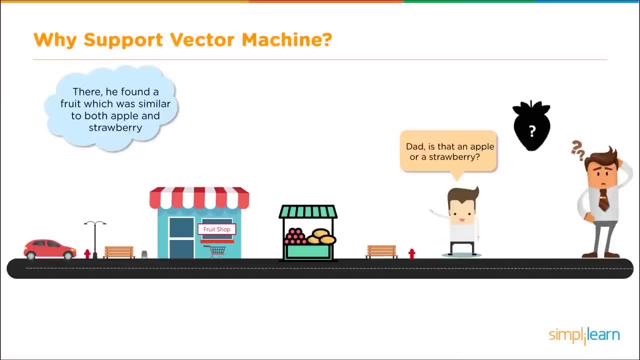 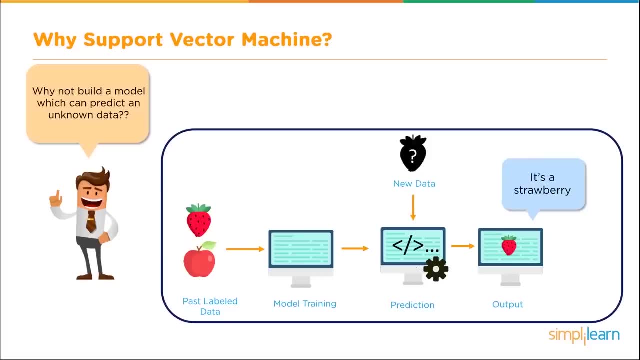 so the question comes up: what fruit did I just pick up from the fruit stand? after a couple of seconds, you can figure out that it was a strawberry. so lets take this model a step further and lets- why not, build a model which can predict an unknown data. 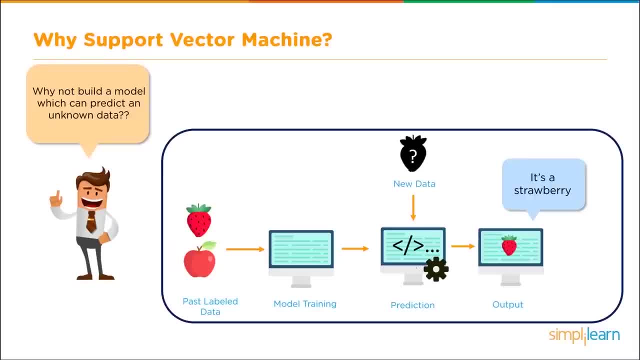 and in this we are going to be looking at some sweet strawberries or crispy apples. we want it to be able to label those two and decide what the fruit is, and we do that by having data already put in. so we already have a bunch of strawberries we know are strawberries and they are already labeled as such. 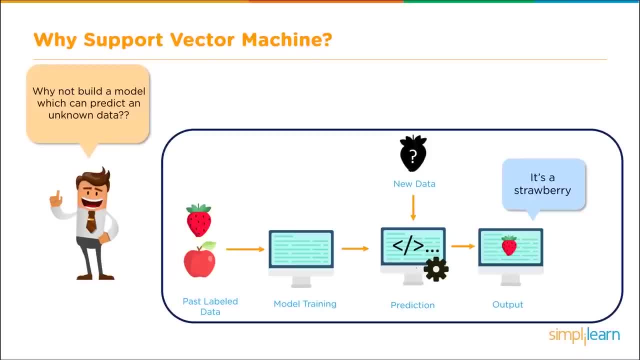 we already have a bunch of apples we know are apples and are labeled as such, then once we train our model, that model then can be given the new data. and the new data is this image. in this case, you can see a question mark on it and it comes through and goes: its a strawberry. 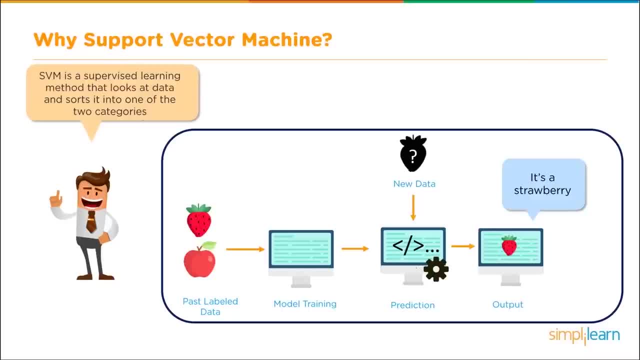 in this case we are using the support vector machine model. SVM is a supervised learning method that looks at data and sorts it into one of two categories, and in this case we are sorting the strawberry into the strawberry side. at this point you should be asking the question. 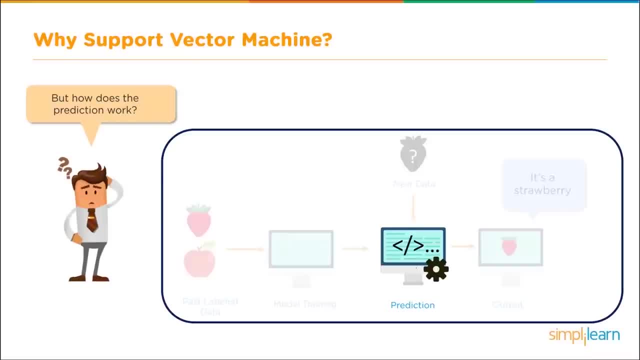 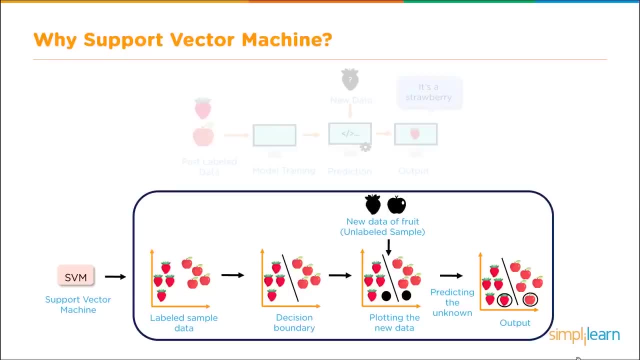 how does the prediction work? before we dig into an example with numbers, lets apply this to our fruit scenario. we have our support vector machine, we have taken it and we have taken a labeled sample of data- strawberries and apples- and we draw a line down the middle between the two groups. 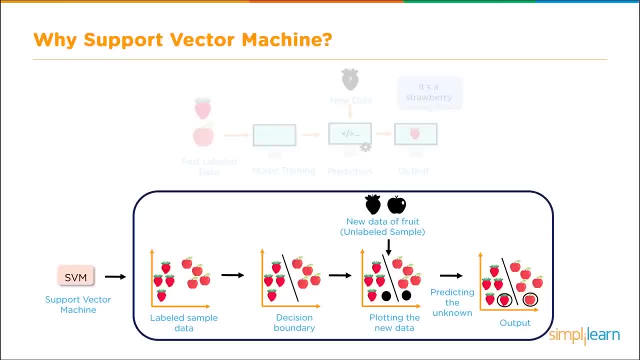 this split now allows us to take new data, in this case an apple and a strawberry, and place them in the appropriate group based on which side of the line they fall in, and that way we can predict the unknown, as colorful and tasty as the fruit example is. 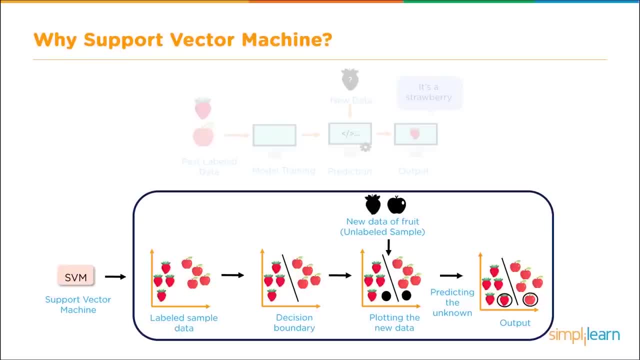 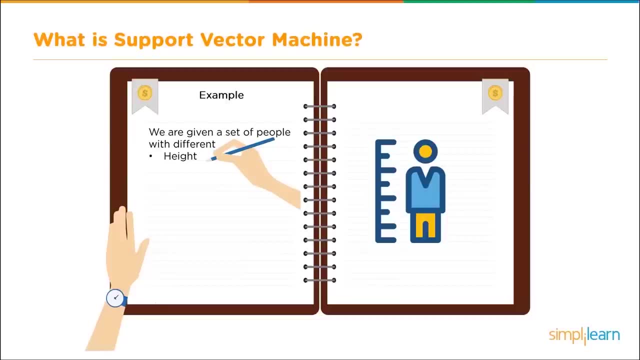 lets take a look at another example with some numbers involved, and we can take a closer look at how the math works. in this example, we are going to be classifying men and women and we are going to start with a set of people with a different height and a different weight. 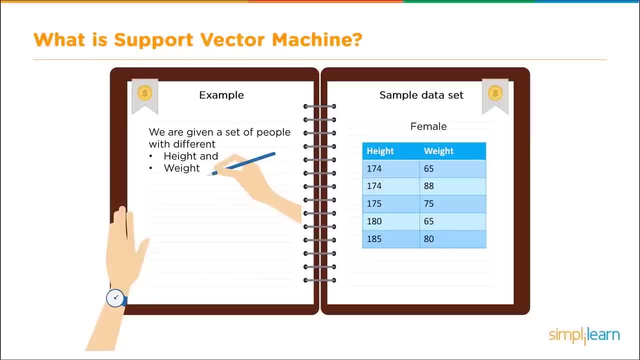 and to make this work we will have to have a sample data set of female where you have their height and weight: 174,, 65,, 174,, 88 and so on- and we will need a sample data set of the male. they have a height 179, 90. 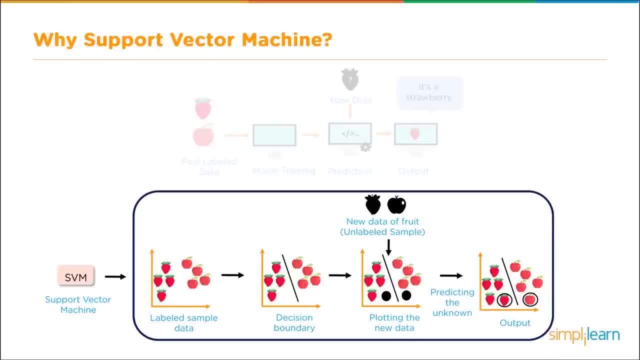 and we draw on a line down the middle between the two groups. This split now allows us to take new data, in this case an apple and a strawberry, and place them in the appropriate group based on which side of the line they fall in. 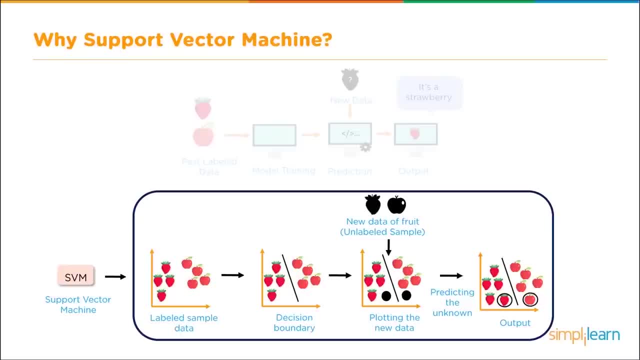 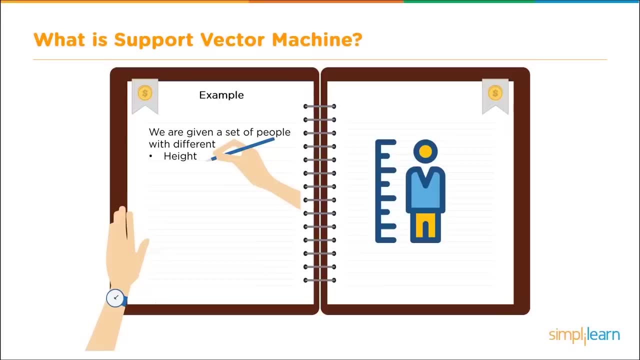 And that way we can predict the unknown. As colorful and tasty as a fruit example is, let's take a look at another example with some numbers involved, and we can take a closer look at how the math works. in this example, We're going to be classifying men and women and we're going to start with a set. 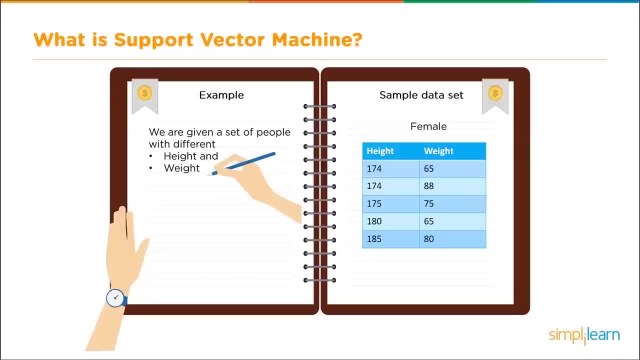 of people with a different height and a different weight And to make this work we'll have to have a sample data set of female. We have their height and weight: 174,, 65,, 174,, 88 and so on. 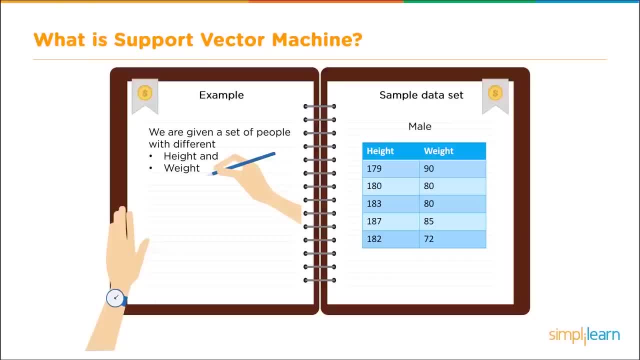 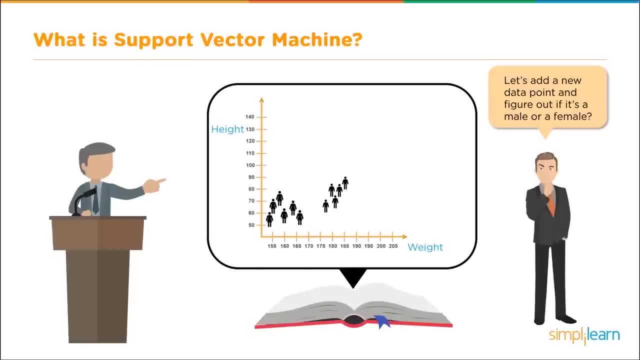 And we'll need a sample data set of the male. They have a height: 179,, 90,, 180 to 80, and so on. Let's go ahead and put this on a graph so we have a nice visual. So you can see, here we have two groups, based on the height versus the weight. 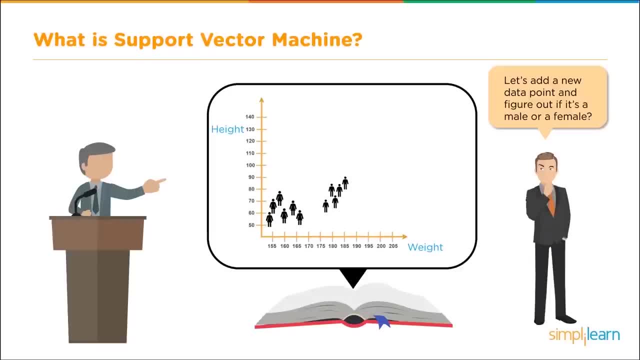 And on the left side we're going to have the women, On the right side, we're going to have the men. Now, if we're going to create a classifier, let's add a new data point to figure out if it's male or female. 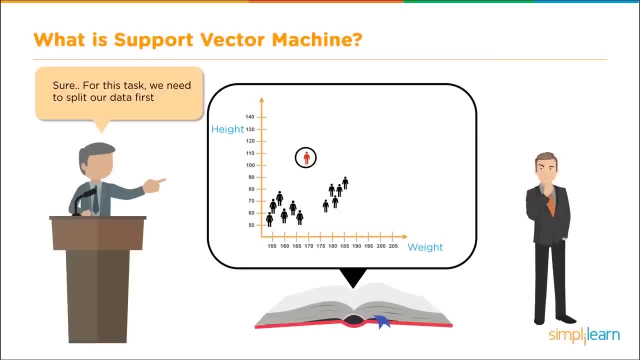 So before we can do that, we need to split our data first. We can split our data by choosing any of these lines. In this case, we draw in two lines through the data in the middle that separates the men from the women, But to predict the gender of a new data. 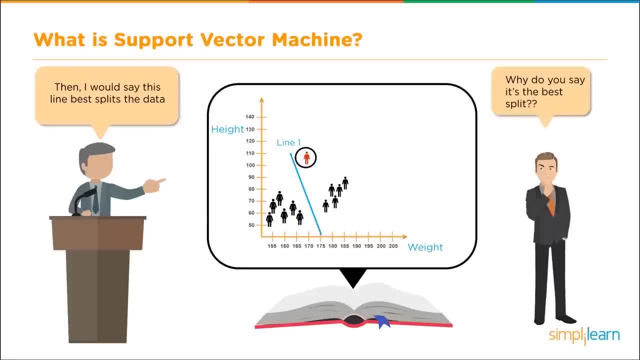 point. we should split the data in the best possible way. And we say the best possible way because this line has a maximum space that separates the two classes. Here you can see, there's a clear split between the two different classes, And in this one there's not so much a clear split. 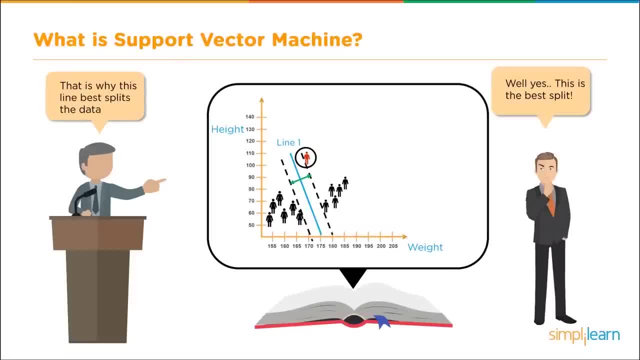 This doesn't have the maximum space that separates the two. That is why this line best splits the data. We don't want to just do this by eyeballing it, And before we go further, we need to add some technical terms to this. 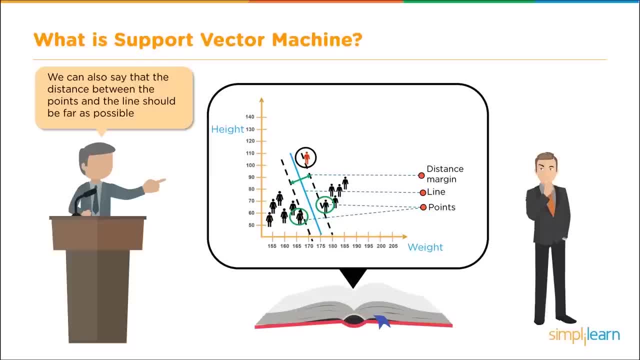 We can also say that the distance between the points in the line should be as far as possible. In technical terms, we can say the distance between the support vector and the hyperplane should be as far as possible, And this is where the support vectors are the extreme. 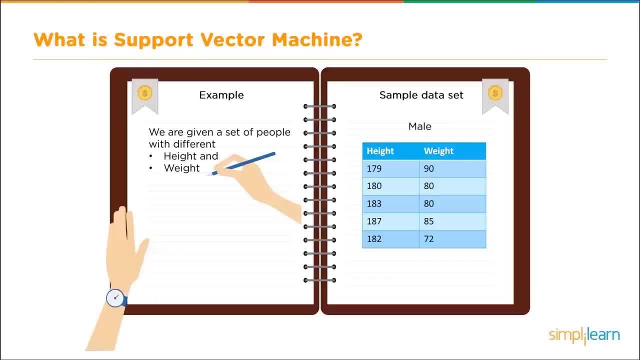 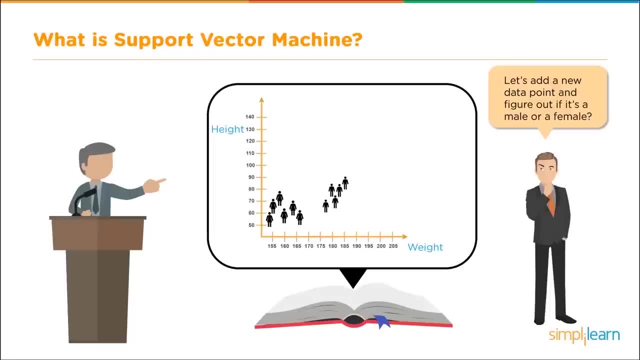 180 to 80 and so on. lets go ahead and put this on a graph so you have a nice visual and you can see here we have two groups based on the height versus the weight, and on the left side we are going to have the women. 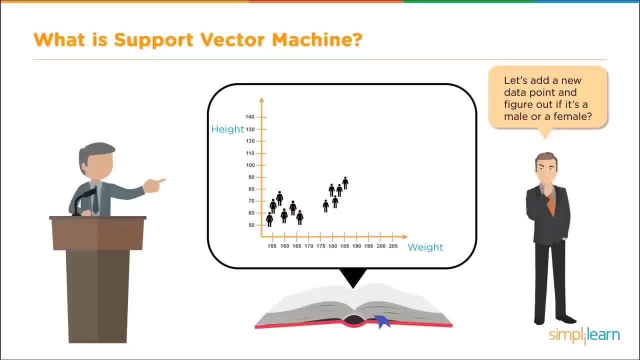 on the right side, we are going to have the men. now, if we are going to create a classifier, lets add a new data point and figure out if its male or female. so before we can do that, we need to split our data first. we can split our data by choosing any of these lines: 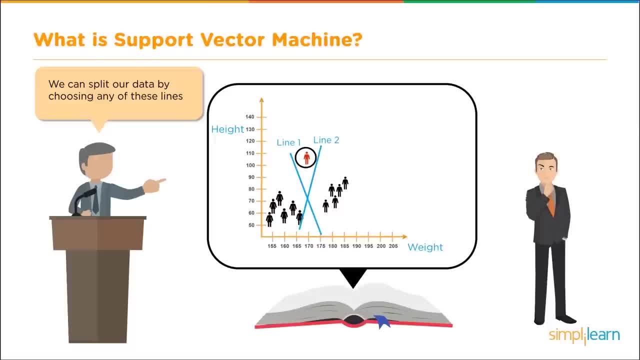 in this case we draw in two lines through the data in the middle that separates the men from the women. but to predict the gender of a new data point, we should split the data in the best possible way. and we say the best possible way because this line has the maximum space. 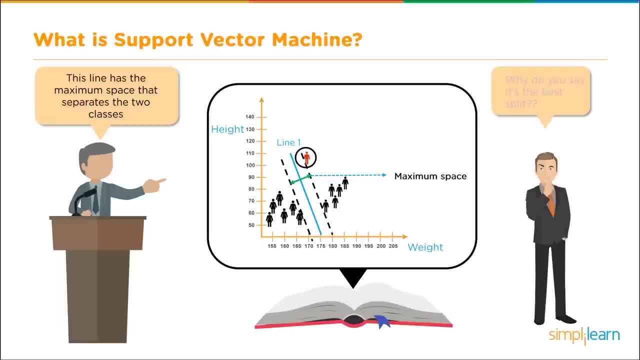 that separates the two classes. here you can see, there is a clear split between the two different classes, and in this one there is not so much a clear split. this doesn't have the maximum space that separates the two. that is why this line best splits the data. 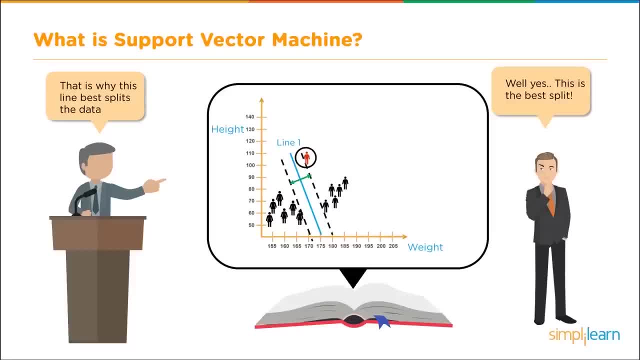 we don't want to just do this by eyeballing it, and before we go further we need to add some technical terms to this. we can also say that the distance between the points in the line should be as far as possible. in technical terms, we can say: 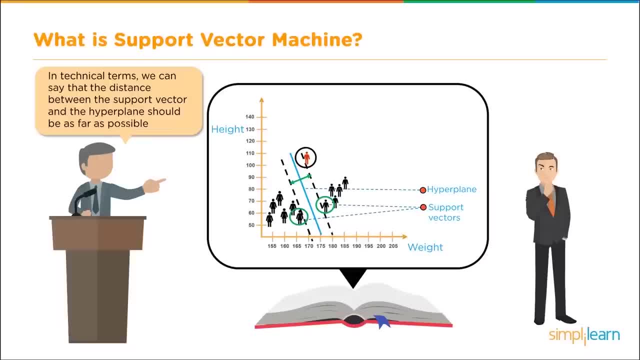 the distance between the support vector and the hyperplane should be as far as possible, and this is where the support vectors are the extreme points in the data set. and if you look at this data set, they have circled two points which seem to be right on the outskirts of the women. 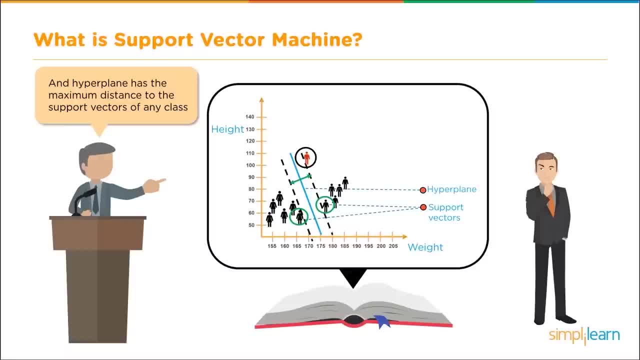 and one on the outskirts of the men and hyperplane has the maximum distance to the support vectors of any class. now you'll see, the line down the middle is a hyperplane, because when you're dealing with multiple dimensions it's really not just a line but a plane of intersections. 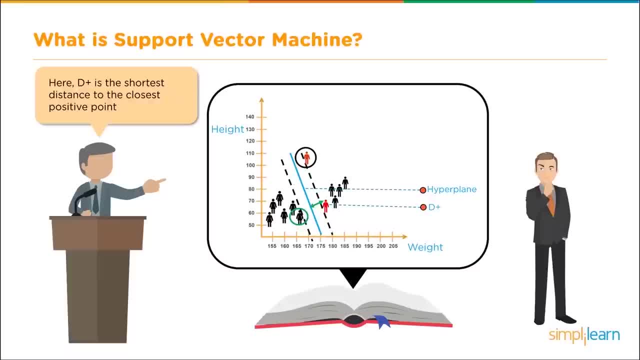 and you can see here where the support vectors have been drawn in dashed lines. the math behind this is very simple. we take D plus, the shortest distance to the closest positive point, which would be on the men's side, and D minus is the shortest distance to the closest negative point. 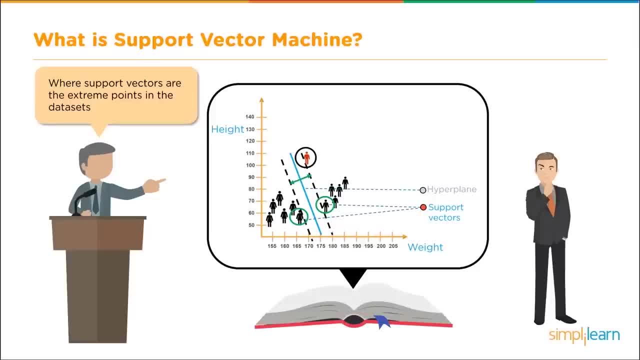 points in the data set. And if you look at this data set, they have circled two points which seem to be right on the outskirts of the women and one on the outskirts of the men, And hyperplane has a maximum distance to the support vectors of any class. 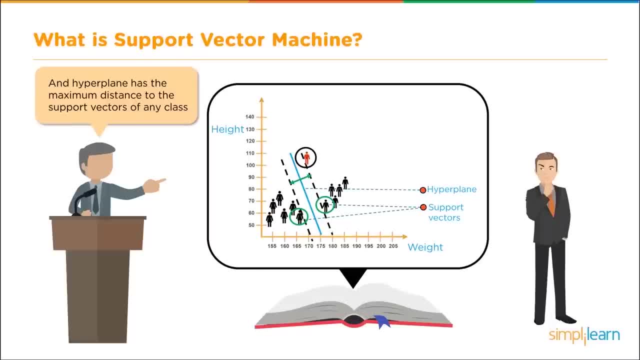 Now you'll see the line down the middle, And we call this the hyperplane, because when you're dealing with multiple dimensions, it's really not just a line but a plane of intersections, And you can see here where the support vectors have been drawn. 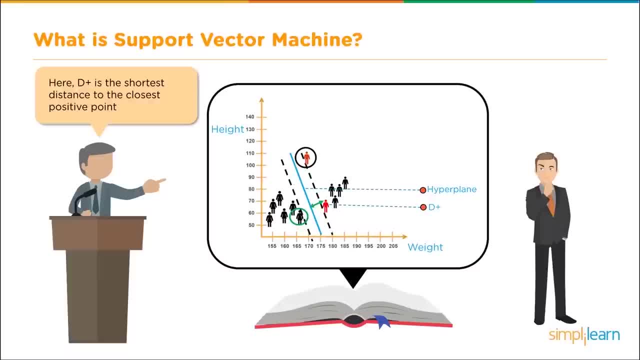 in dashed lines. The math behind this is very simple. We take D plus the shortest distance to the closest positive point, which would be on the men's side, and D minus is the shortest distance to the closest negative point, which is on the women's side. 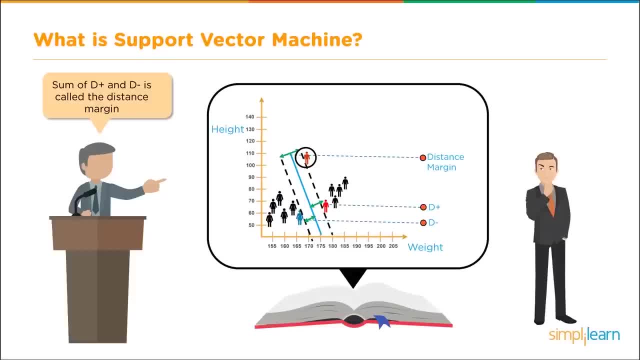 The sum of D plus and D minus is called the distance margin, or the distance between the two support vectors that are shown in the dashed lines, And then, by finding the largest distance margin, we can get the optimal hyperplane. Once we've created an optimal hyperplane, we can easily 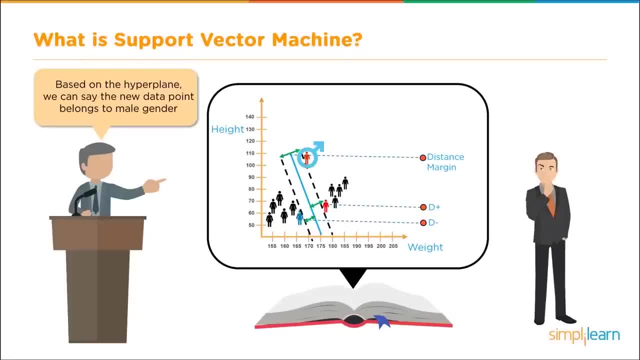 see which side the new data fits in And, based on the hyperplane, we can say the new data point belongs to the male gender. Hopefully that's clear how that works on a visual level. As a data scientist, you should also be asking what happens. 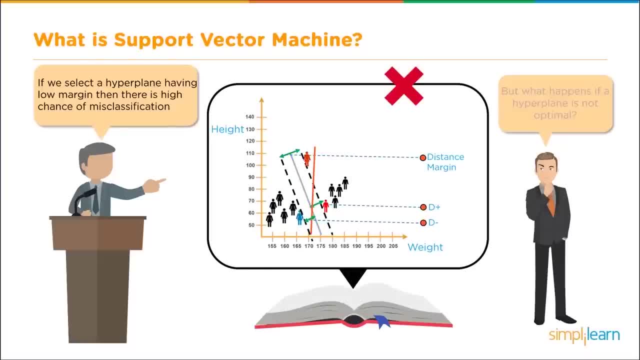 if the hyperplane is not optimal. If we select a hyperplane having low margin, then there is a high chance of misclassification. This particular SVM model, the one we discussed so far, is also called or referred to as the LSVM. 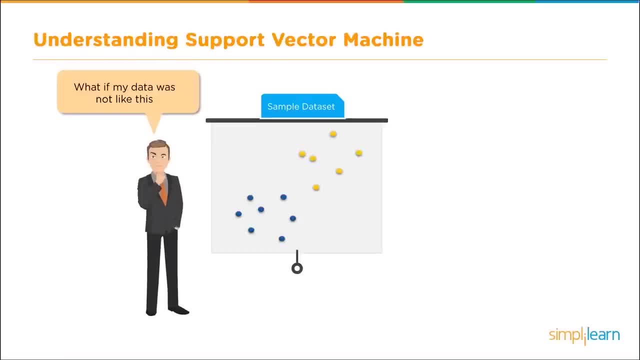 So far, so clear, but a question should be coming up. We have our sample data set, But instead of looking like this, what if it looked like this, where we have two sets of data, but one of them occurs in the middle of another set? 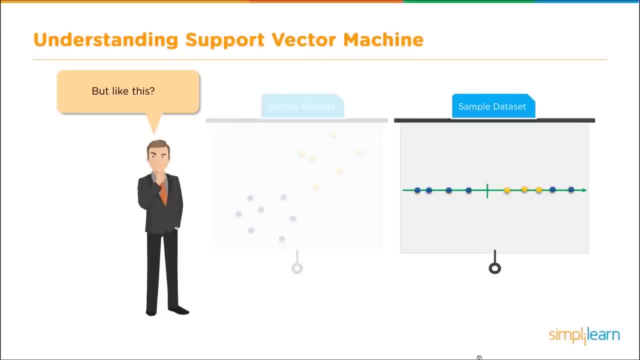 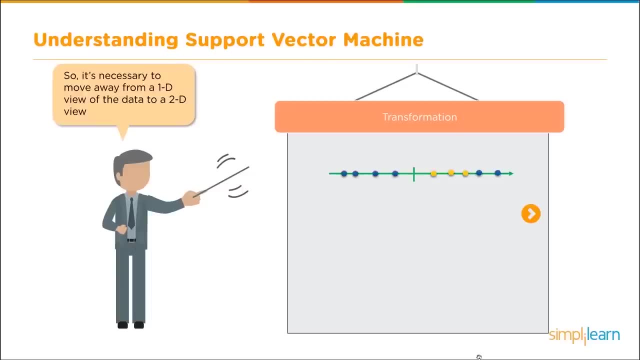 You can see here where we have the blue and the yellow and then blue again on the other side of our data line. In this data set we can't use a hyperplane, So when you see data like this, it's necessary to move away from a 1D view of the data to 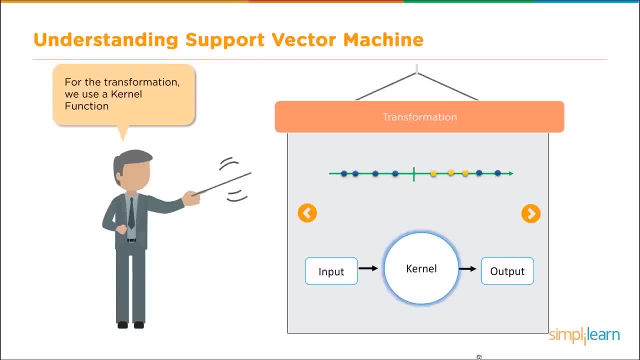 a two dimensional view of the data And for the transformation we use what's called a kernel function. The kernel function will take the one D input and transfer it to a two dimensional output, As you can see in this picture here the 1D. 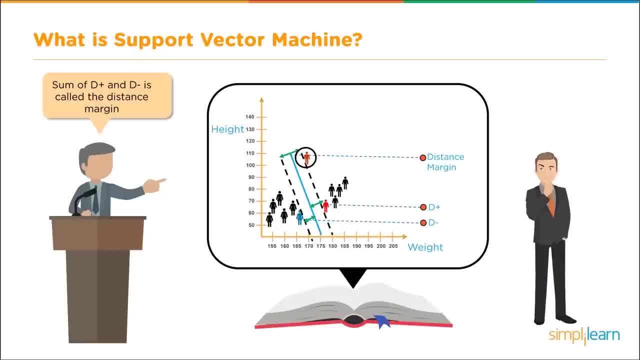 which is on the women's side. the sum of D plus and D minus is called the distance margin in the dashed lines, and then by finding the largest distance margin, we can get the optimal hyperplane. once we've created an optimal hyperplane, we can easily see which side. 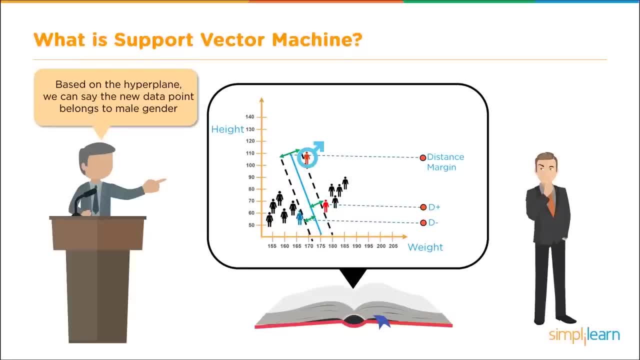 the new data fits in and, based on the hyperplane, we can say the new data point belongs to the male gender. hopefully that's clear how that works on a visual level. as a data scientist, you should also be asking what happens if the hyperplane is not optimal. 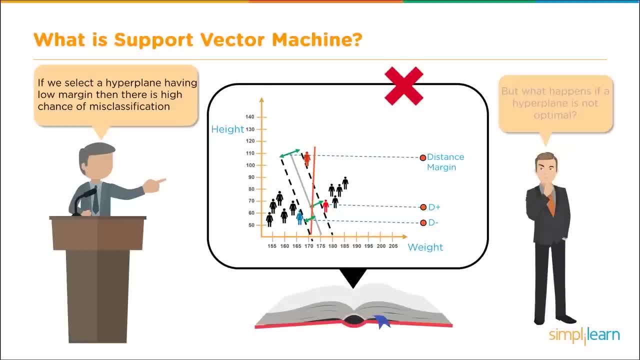 if we select a hyperplane having low margin, then there is a high chance of misclassification. this particular SVM model, the one we discussed so far, is also referred to as the LSVM. so far, so clear. but a question should be coming up. we have our sample data set. 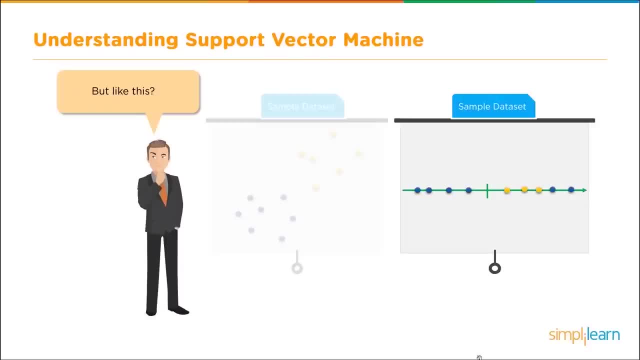 but instead of looking like this, what if it looked like this: where we have two sets of data, but one of them occurs in the middle of another set. you can see here where we have the blue and the yellow and then blue again on the other side of our data line. 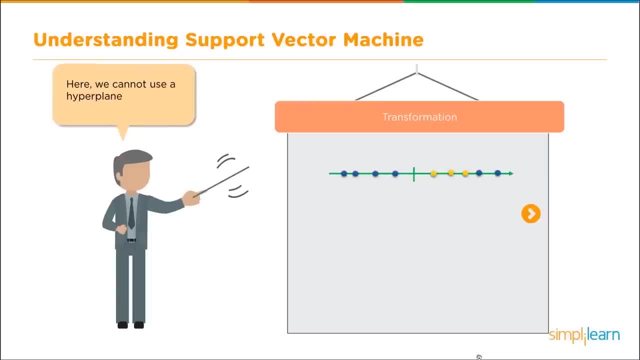 in this data set. we can't use a hyperplane, so if we see data like this, it's necessary to move away from a 1D view of the data to a two-dimensional view of the data, and for the transformation we used what's called a kernel function. 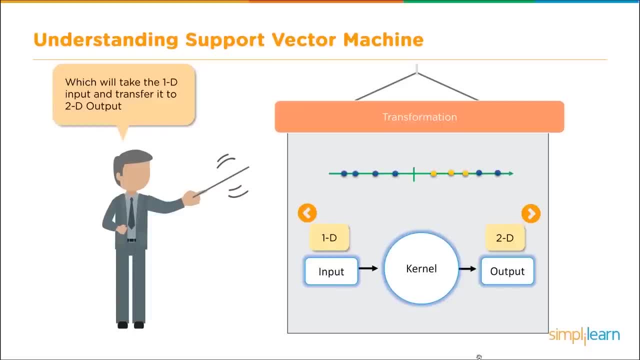 the kernel function will take the 1D input and transfer it to a two-dimensional output. as you can see in this picture here, the 1D when transferred to a two-dimensional makes it very easy to draw a line between the two data sets. what if we make it even more complicated? 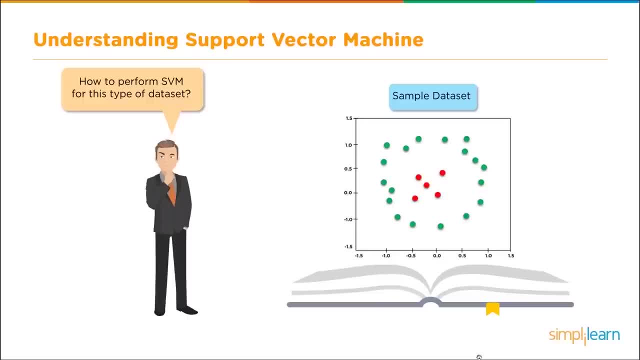 how do we perform an SVM for this type of data set? here's another example. here you can see, we have a two-dimensional data set where the data is in the middle, surrounded by the green data on the outside. in this case, we're going to segregate the two classes. 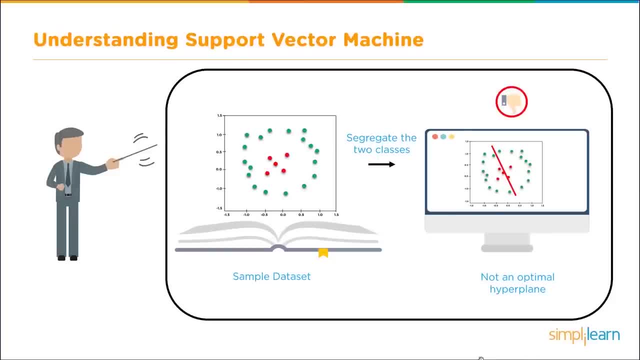 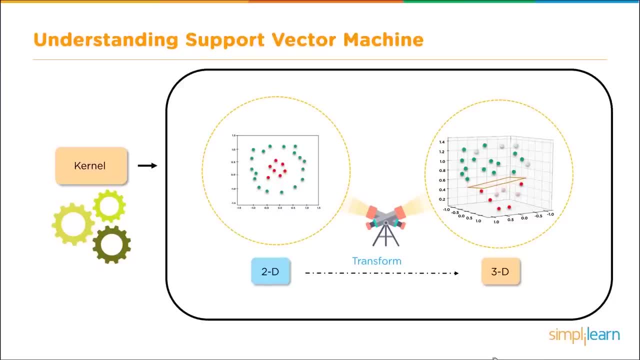 we have our sample data set and if you draw a line through, it's obviously not an optimal hyperplane in there. so to do that we need to transfer the 2D to a 3D array and when you translate it into a three-dimensional array. 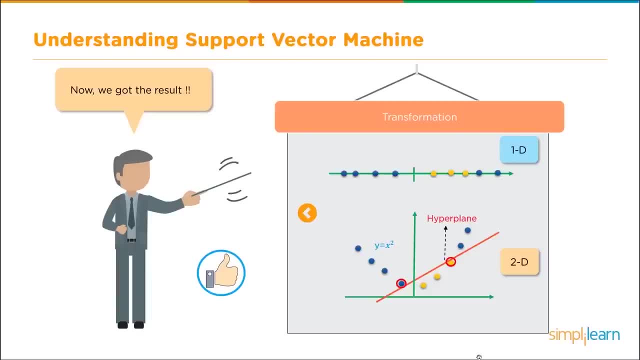 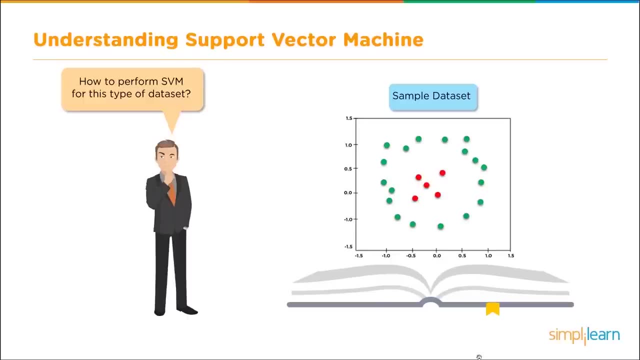 when transferred to a two dimensional, makes it very easy to draw a line between the two data sets. What if we make it even more complicated? How do we perform an SVM for this type of data set? Here you can see, we have a two dimensional data set where the data 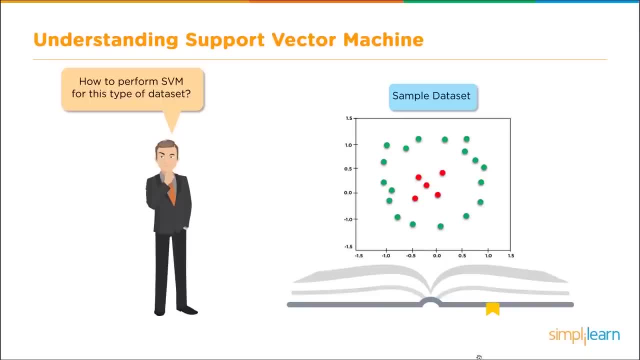 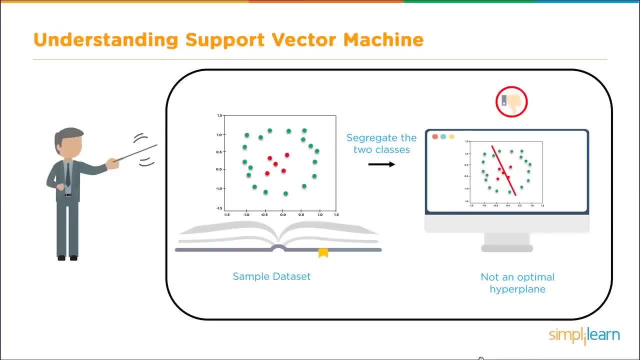 is in the middle, surrounded by the green data on the outside. In this case we're going to segregate the two classes. We have our sample data set And if you draw a line through, it's obviously not an optimal hyperplane in there. 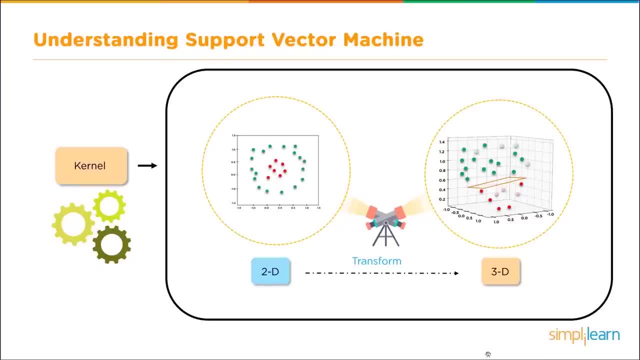 So to do that we need to transfer the 2D to a 3D array, And when you translate it into a three dimensional array using the kernel, you can see where you can place a hyperplane right through it and easily split the data. 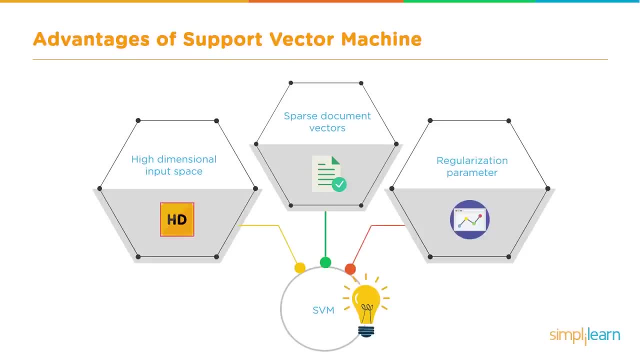 Before we start looking at a programming example and dive into the script, let's look at the advantage of the support vector machine. We'll start with high dimensional input space, or sometimes referred to as the curse of dimensionality. We looked at earlier one dimension. 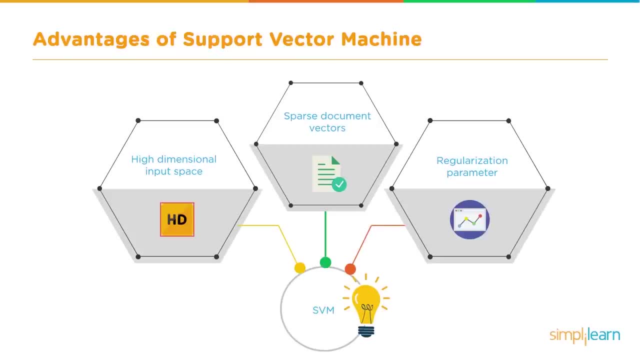 two dimension, three dimension, When you get to a thousand dimensions, a lot of problems start occurring with most algorithms that have to be adjusted for. The SVM automatically does that in high dimensional space. One of the high dimensional space, one high dimensional space that we work on, is sparse document vectors. 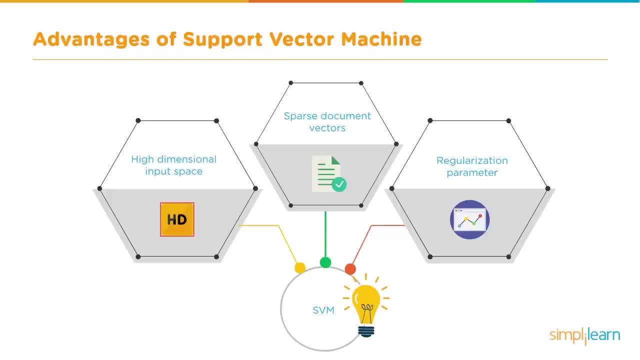 This is where we tokenize the words and documents so we can run our machine learning algorithms over them. I've seen ones get as high as 2.4 million different tokens. That's a lot of vectors to look at. And finally we have regularization. 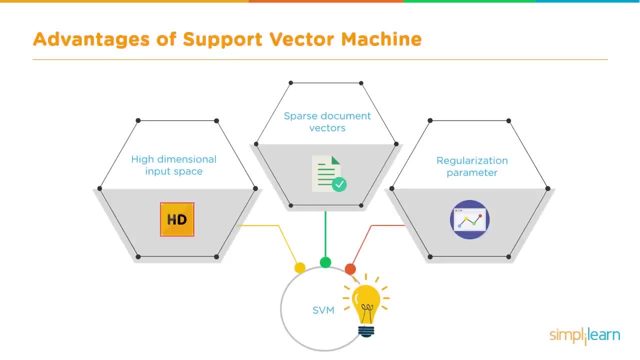 a parameter. The regularization parameter, or lambda, is a parameter that helps figure out whether we're going to have a bias or overfitting of the data, whether it's going to be overfitted to a very specific instance or it's going to be biased to a high or low value. 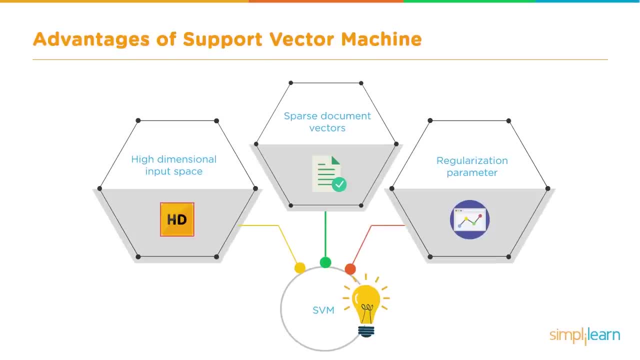 With the SVM, it naturally avoids the overfitting and bias problems that we see in many other algorithms. These three advantages of the support vector machine make it a very powerful tool to add to your repertoire of machine learning tools. Now we did promise you a use case study. 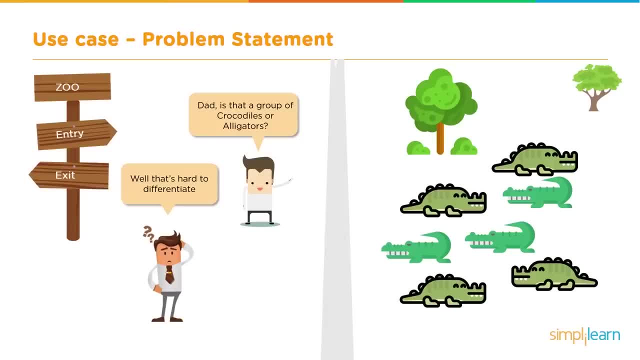 We're actually going to dive into some Python programming and so we're going to go into a problem statement and start off with the zoo. So in the zoo example we have family members going to the zoo, We have the young child going Dad. 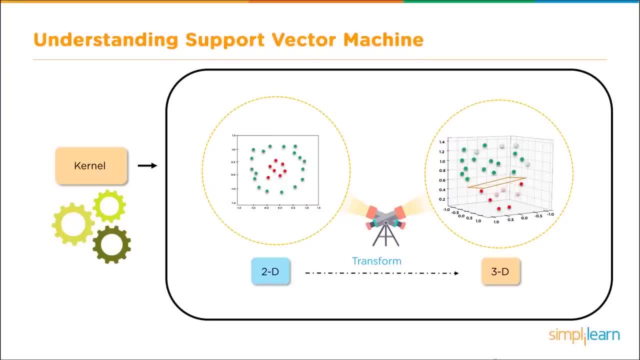 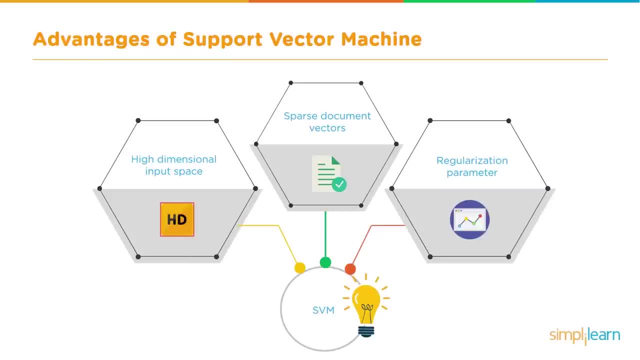 using the kernel, you can see where you can place a hyperplane right through it and easily split the data. before we start looking at a programming example, let's look at the advantage of the support vector machine. we'll start with high dimensional input space, or sometimes referred to as 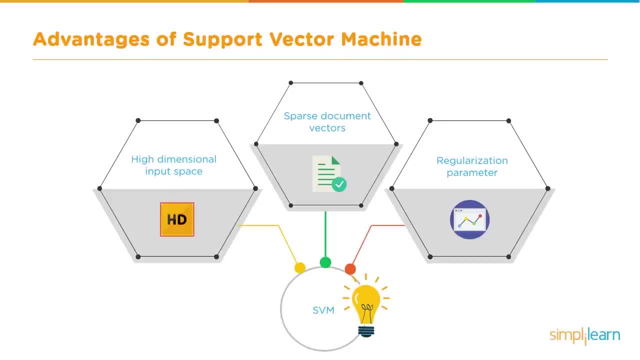 the curse of dimensionality we looked at earlier. one dimension, two dimension, three dimension. when you get to a thousand dimensions a lot of problems start occurring with most algorithms that have to be adjusted, for the SVM automatically does that in high dimensional space. one of the high dimensional space? 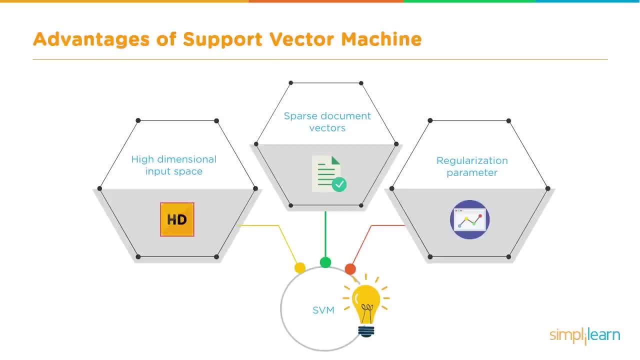 one high dimensional space that we work on is sparse document vectors. this is where we tokenize the words and document so we can run our machine learning algorithms over them. I've seen ones get as high as 2.4 million different tokens. that's a lot of vectors to look at. 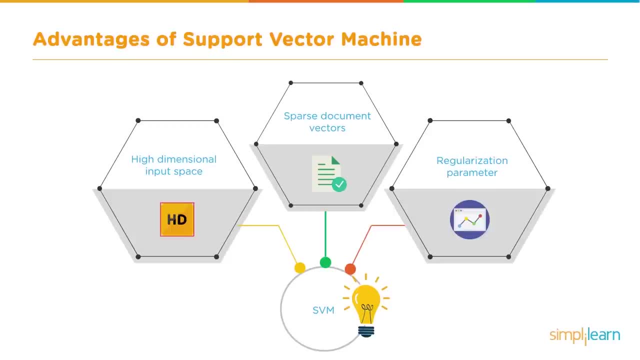 and finally, we have regularization parameter. the regularization parameter, or lambda, is a parameter that helps figure out whether we're going to have a bias or overfitting of the data, whether it's going to be overfitted to a specific instance or it's going to be biased to a high or low value. 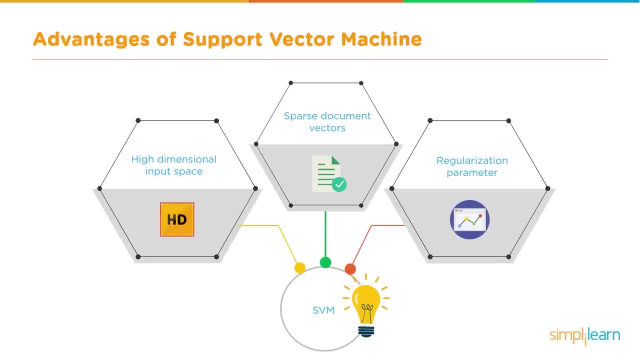 with the SVM, it naturally avoids the overfitting and bias problems that we see in many other algorithms. these three advantages of the support vector machine make it a very powerful tool to add to your repertoire of machine learning tools. now we did promise you a used case study. 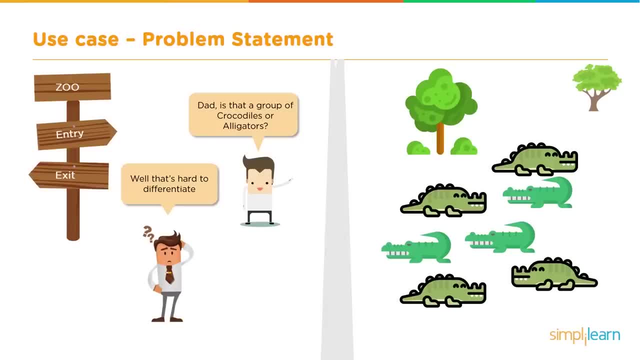 we're actually going to dive into some Python programming and so we're going to go into a problem statement and start off with the zoo. so in the zoo example we have family members going to the zoo. we have the young child going. dad, is that a group of crocodiles or alligators? 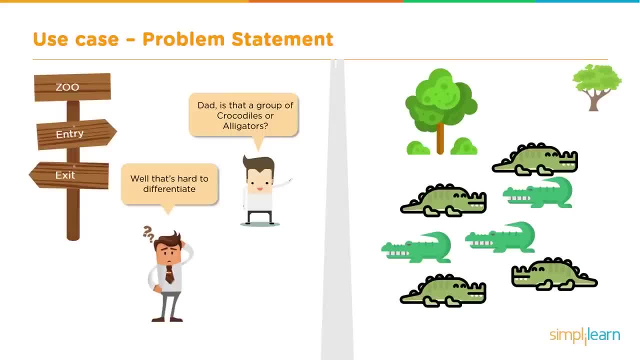 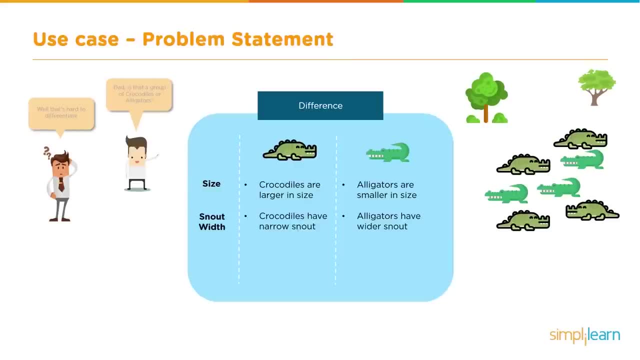 well, that's hard to differentiate, and zoos are a great place to start looking at science and understanding how things work, especially as a young child, and so we can see the parents sitting here thinking: well, what is the difference between a crocodile and an alligator? 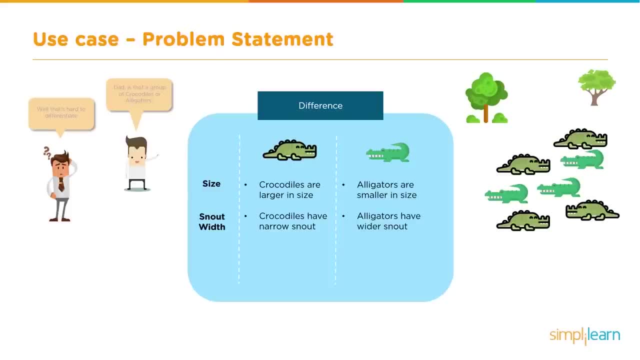 well one, crocodiles are larger in size, alligators are smaller in size. snout widths: the crocodiles have a narrow snout and alligators have a wider snout. and, of course, in the modern day and age, the father is sitting here thinking: how can I turn this into a lesson for my son? 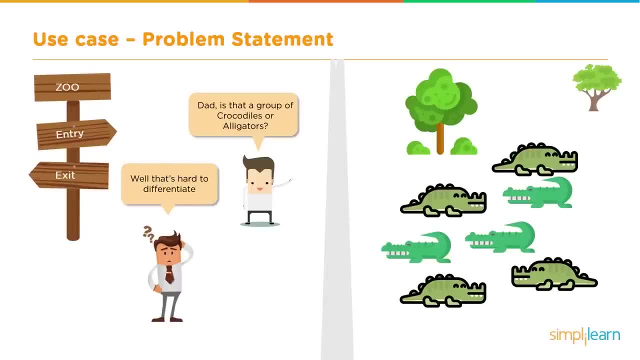 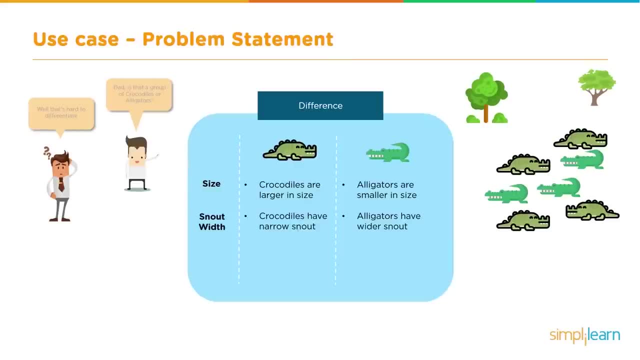 is that a group of crocodiles or alligators? Well, that's hard to differentiate, And zoos are a great place to start looking at science and understanding how things work, especially as a young child, And so we can see the parents sitting here. 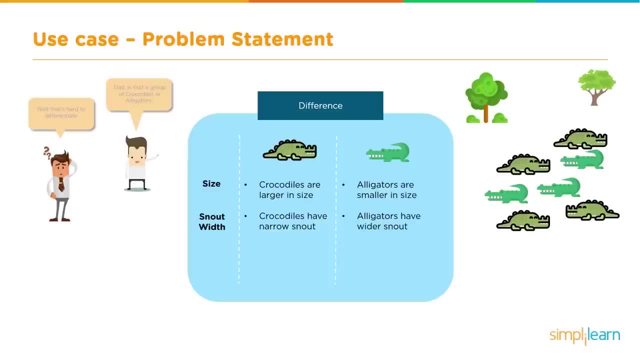 thinking: well, what is the difference between a crocodile and an alligator? Well one, crocodiles are larger in size, Alligators are smaller in size. Alligators have a snout width. The crocodiles have a narrow snout and alligators have a wider snout. 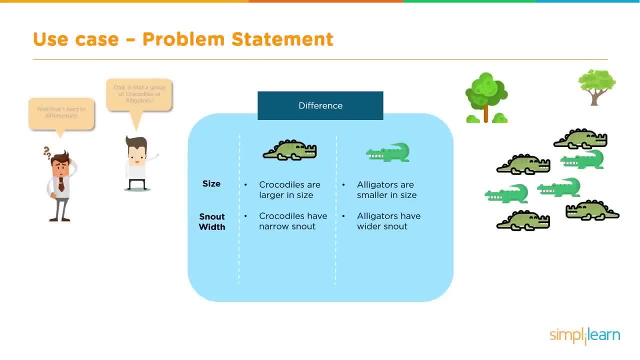 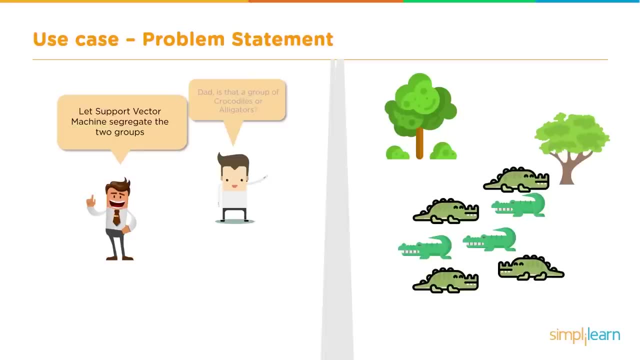 And of course, in the modern day and age, the father sitting here is thinking: how can I turn this into a lesson for my son? And he goes: let a support vector machine segregate the two groups. I don't know if my dad ever told me that, but that would be funny. 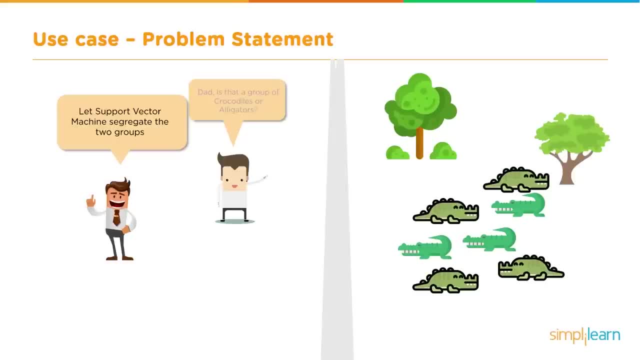 Now, in this example, we're not going to use actual measurements and data. We're just using that for imagery- And that's very common in a lot of machine learning algorithms- and setting them up. But let's roll up our sleeves, and we'll talk about that more in just a moment as. 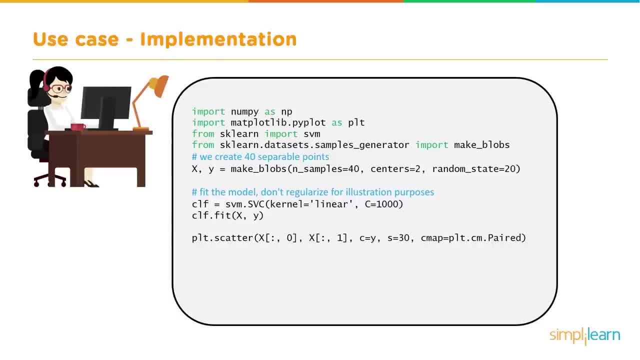 a Python script. So here we arrive in our actual coding, And I'm going to move this into a Python editor in just a moment. But let's talk a little bit about what we're going to cover First. we're going to cover in the code: 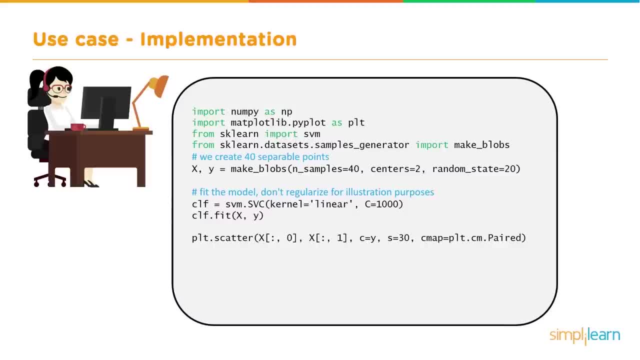 the setup, how to actually create our SVM, and you're going to find that there's only two lines of code that actually create it, and the rest of it is done so quick and fast that it's all here in the first page And we'll show you what that looks like as far as our data. 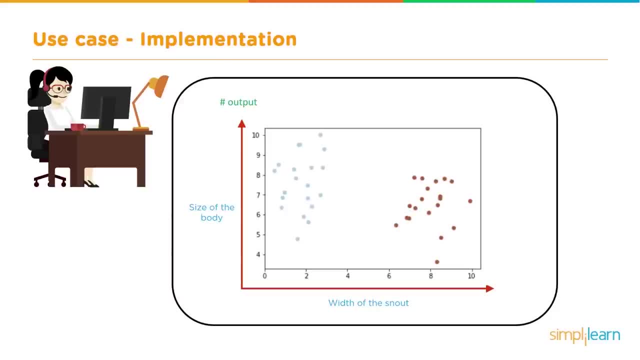 So we're going to create some data. I talked about creating data just a minute ago, And so we'll get into the creating data here and you'll see this nice correction of our two blobs And we'll go through that in just a second. 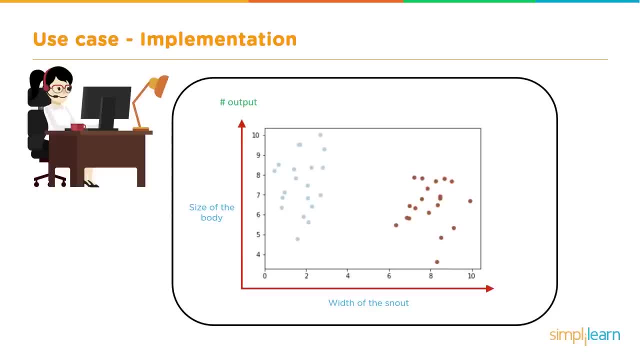 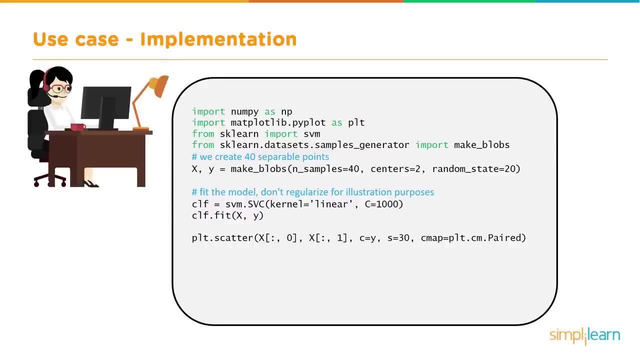 And then the second part is: we're going to take this and we're going to bump it up a notch. We're going to show you what it looks like behind the scenes, But let's start with actually creating our setup. I like to use the Anaconda Jupyter Notebook because it's very easy to use. 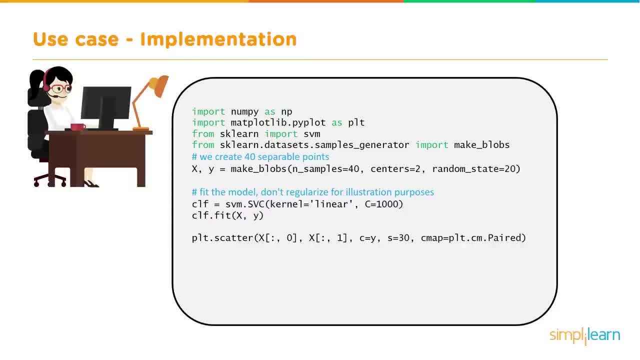 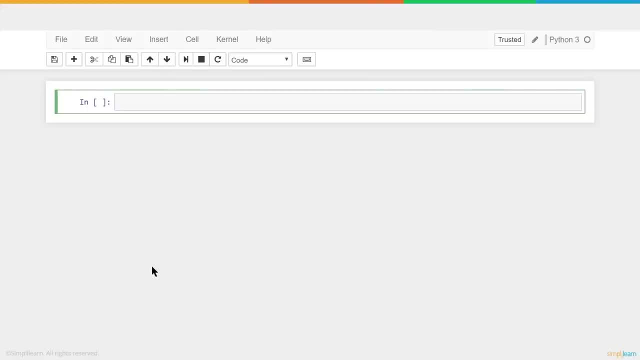 but you can use any of your favorite Python editors or setups and go in there, But let's go ahead and switch over there and see what that looks like. So here we are in the Anaconda Python Notebook, or Anaconda Jupyter Notebook, with Python. We're using Python three. 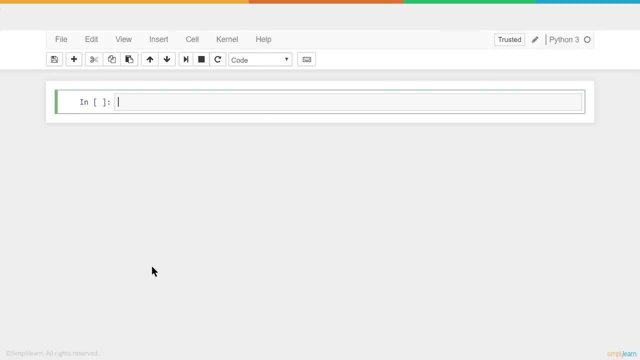 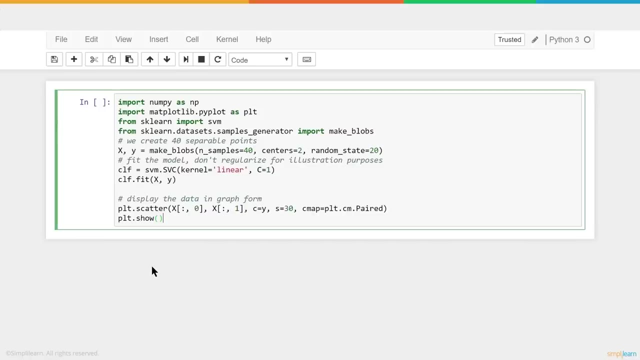 I believe this is three point five, but it should be work in any of your three X versions And you'd have to look at the SK, learn and make sure. if you're using a two X version, an earlier version, Let's go and put our code in there. 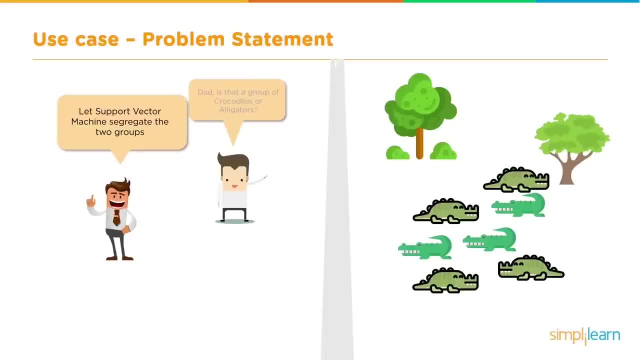 and he goes, let a support vector machine segregate the two groups. I don't know if my dad ever told me that, but that would be funny. I don't know if my dad ever told me that, but that would be funny. I don't know if my dad ever told me that. 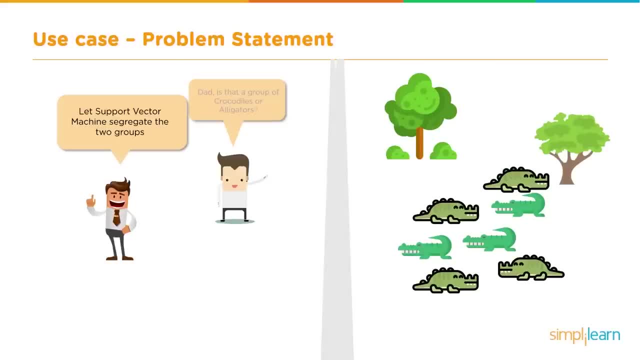 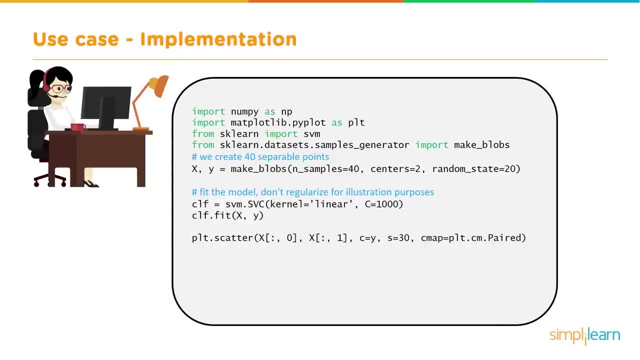 but let's roll up our sleeves- and we'll talk about that more in just a moment- as we break into our python script. so here we arrive, in our actual coding, and I'm going to move this into a python editor in just a moment. but let's talk a little bit about what we're going to cover. 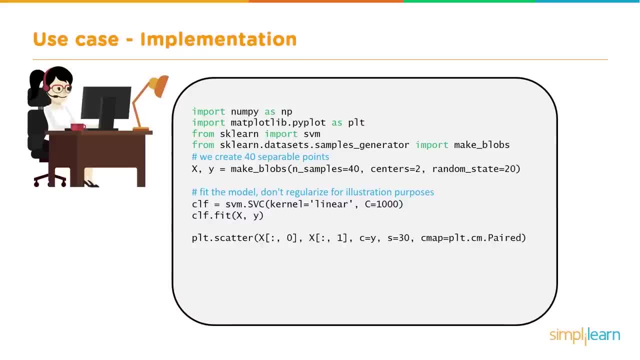 first we're going to cover in the code the setup, how to actually create our SVM, and you're going to find that there's only two lines of code that actually create it. the rest of it is done so quick and fast that it's all here in the first page. 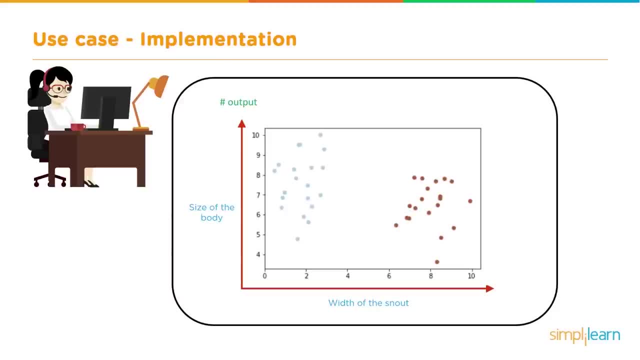 and we'll show you what that looks like as far as our data, because we're going to create some data. I talked about creating data just a minute ago, and so we'll get into the creating data here and you'll see this nice correction of our two blobs. 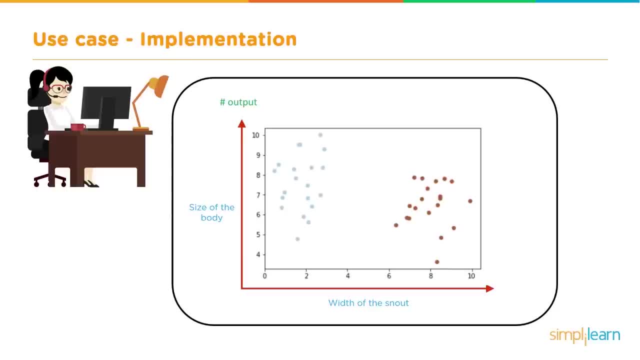 and we'll go through that in just a second. and then the second part is: we're going to take this and we're going to bump it up a notch. we're going to show you what it looks like behind the scenes, but let's start with actually creating our setup. 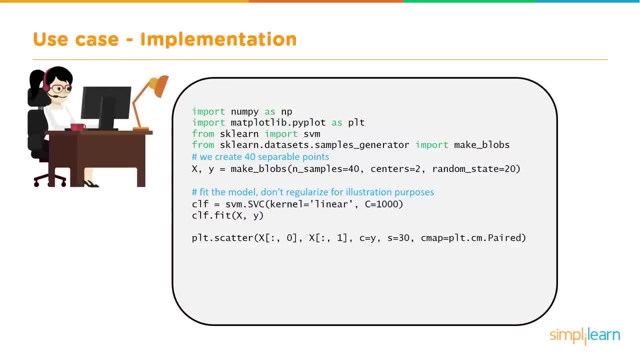 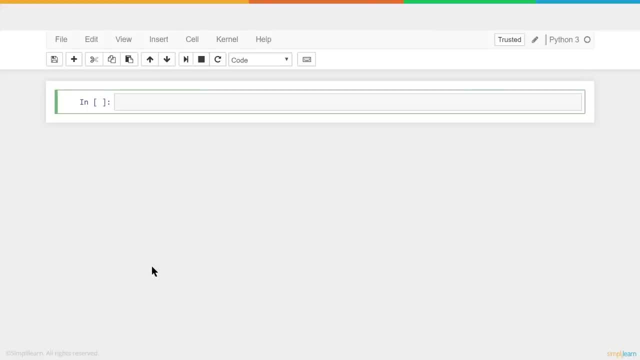 I like to use the Anaconda Jupyter notebook because it's very easy to use. you can go to your favorite Python editors or setups and go in there, but let's go ahead and switch over there and see what that looks like. so here we are in the Anaconda Python notebook. 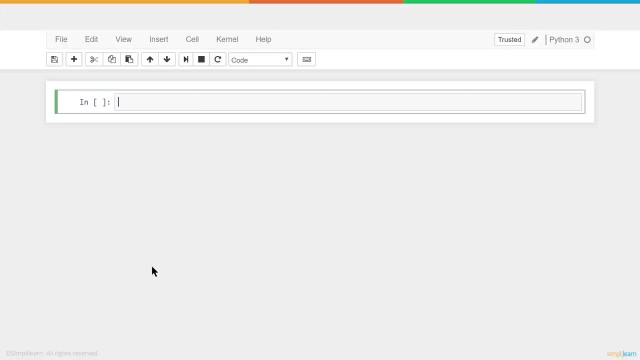 or Anaconda Jupyter notebook with Python. we're using Python 3. I believe this is 3.5, but it should work in any of your 3x versions and you'd have to look at the sklearn and make sure if you're using a 2x version. 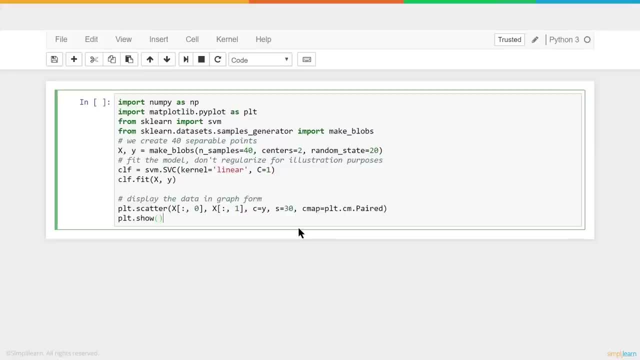 or an earlier version. let's go ahead and put our code in there. and one of the things I like about the Jupyter notebook is I can go up to view all the line numbers on it to make it a little bit easier to talk about, and we can even increase the size. 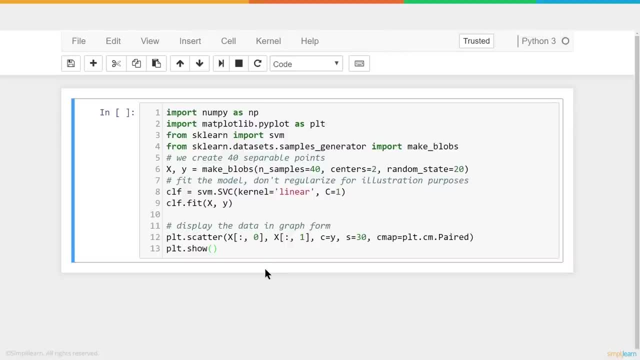 because this is edited in. in this case, I'm using Google Chrome Explorer and that's how it opens up for the editor, although any editor will work. now the first step is going to be our imports, and we're going to import four different parts. the first two I want you to look at. 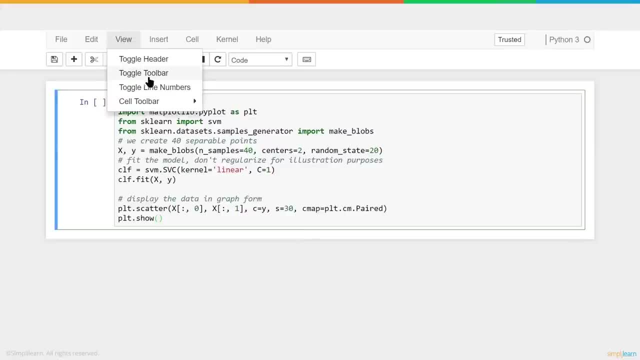 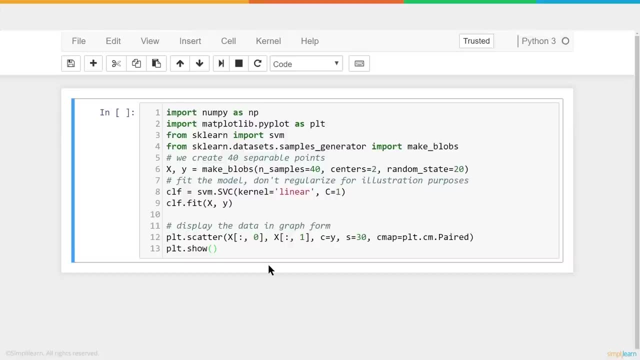 And one of the things I like about the Jupyter Notebook is I can go up to view and I'm going to go ahead and toggle the line numbers on to make it a little bit easier to talk about, and we can even increase the size because this is edited. 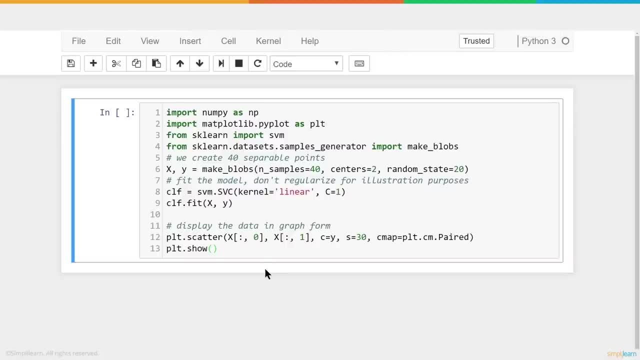 In this case, I'm using Google Chrome Explorer, And that's how it opens up for the editor, Although Anyone, like I said, any editor will work. Now the first step is going to be our imports, and we're going to import four. 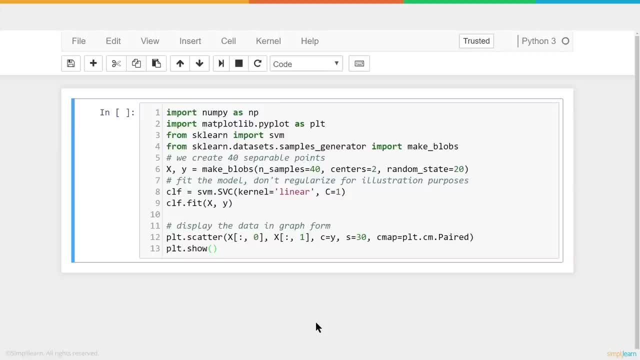 different parts. The first two I want you to look at are line one and line two are numpy as NP and matplotlibrarypyplot as PLT. Now, these are very standardized imports when you're doing work. The first one is the numbers Python. 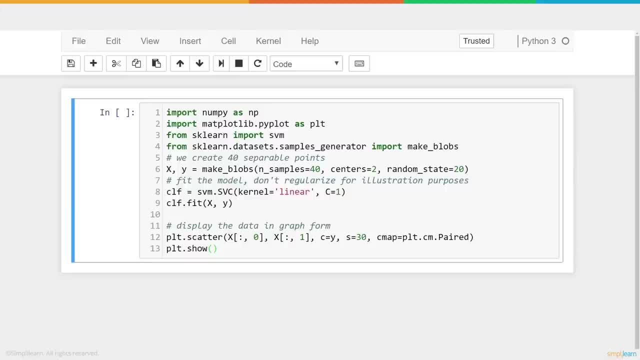 We need that because part of the platform we're using uses that for the numpy array And I'll talk about that in a minute so you can understand why we want to use a numpy array versus the standard Python array. And normally it's pretty standard set up to use NP for numpy. 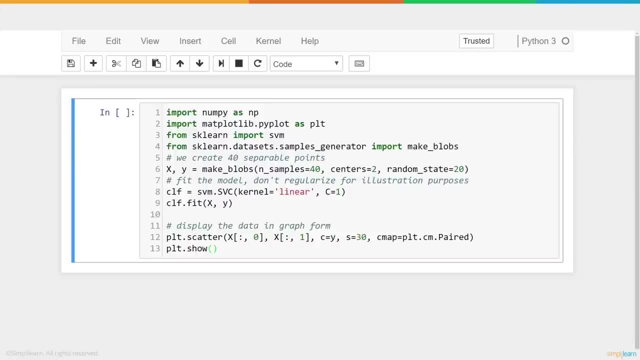 The matplotlibrary is how we're going to view our data, So this has you do need the NP for the sklearn module, but the matplotlibrary is purely for our use for visualization, And so you really don't need that for the SVM, but we're going to put it there. 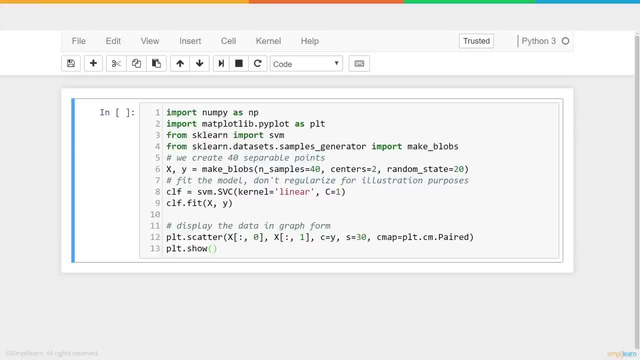 So you have a nice visual aid and we can show you what it looks like. That's really important at the end, when you finish everything. So you have a nice display for everybody to look at, And then, finally, we're going to. I'm going to jump. 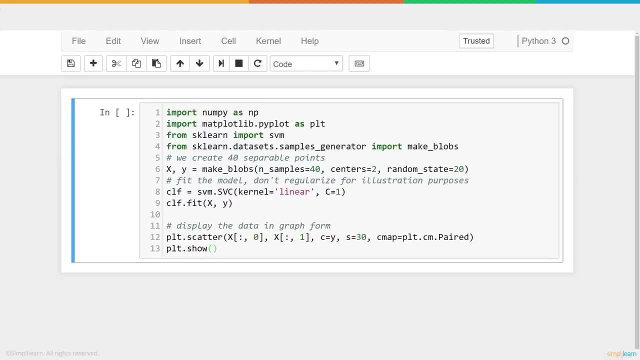 one ahead to line number four, That's the sklearndatasetssamplesgenerator import makeblobs, And I told you that we were going to make up data And this is a tool that's in the sklearn to make up data. I personally don't want to go to the zoo. 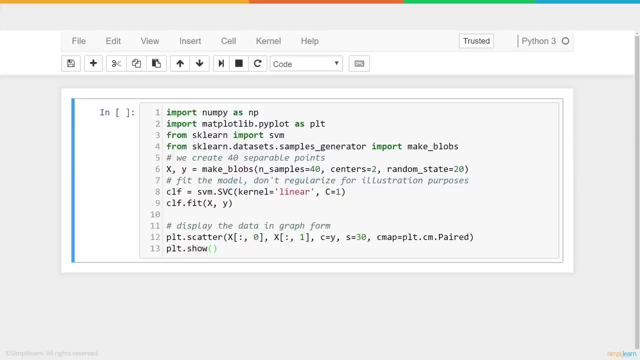 get in trouble for jumping over the fence and probably get eaten by the crocodiles or alligators as I work on measuring their snouts and width and length. Instead, we're just going to make up some data, And that's what that makeblobs is. 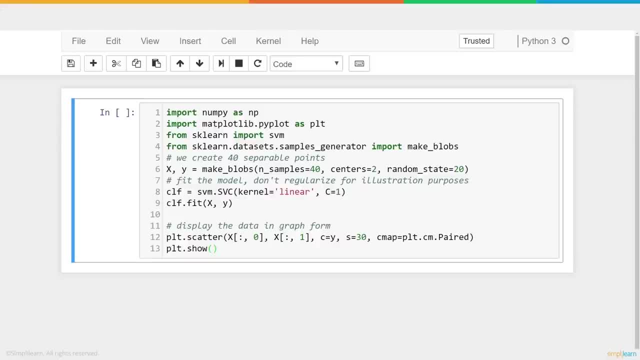 It's a wonderful tool. if you're ready to test your setup and you're not sure about what data you're going to put in there, You can create this blob and it makes it real easy to use. And finally we have our actual SVM- the sklearn import SVM- on line three. 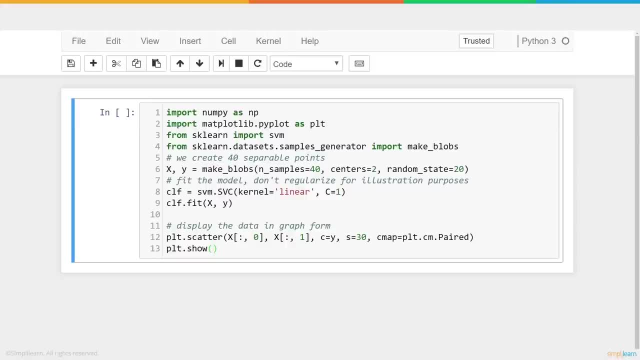 So that covers all our imports. We're going to create- remember I used the makeblobs to create data- and we're going to create a capital X and a lowercase y equals makeblobs in samples- equals 40, so we're going to make 40 lines of data. 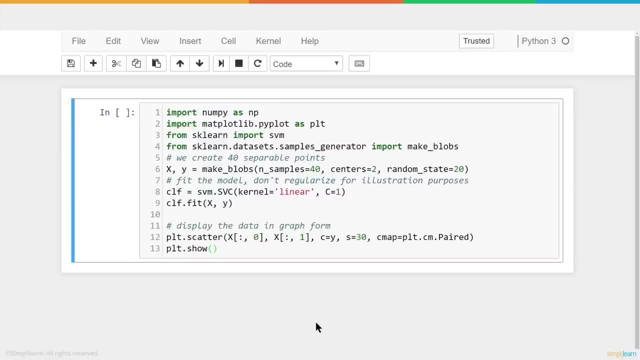 are line 1 and line 2 are numpy as np and matplotlibrarypyplot as plt. now, these are very standardized when you're doing work. the first one is the numbers python. we need that because part of the platform we're using uses that for the numpy array. 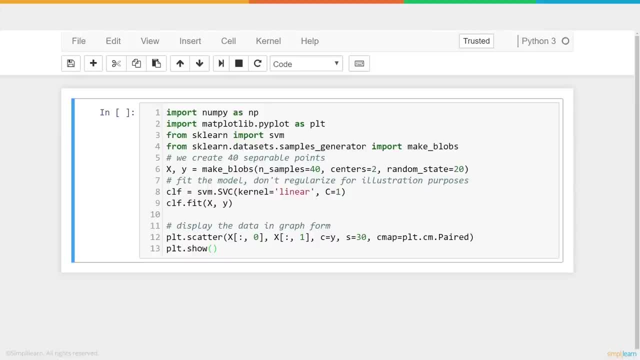 and I'll talk about that in a minute so you can understand why we want to use a numpy array versus a standard python array. and normally it's pretty standard setup to use np for numpy. the matplotlibrary is how we're going to view our data, so this has 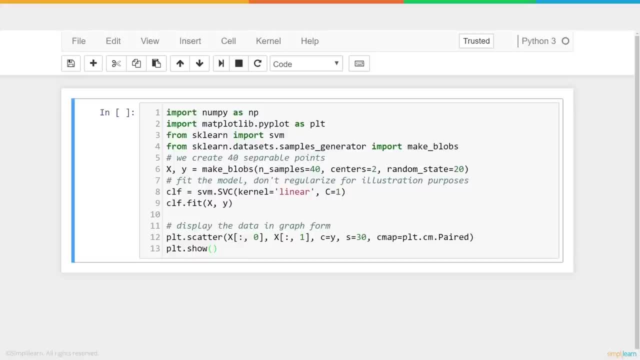 you do need the np for the sklearn module, but the matplotlibrary is purely for our use, for visualization, and so you really don't need that for the svm. but we're going to put it there so you have a nice visual aid and we can show you what it looks like. 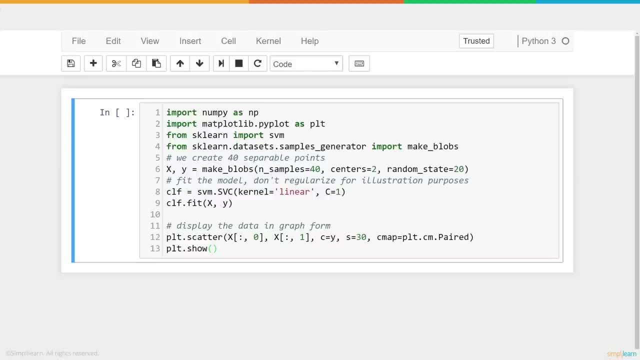 that's really important at the end, when you finish everything, so you have a nice display for everybody to look at. and then, finally, I'm going to jump one ahead to line number 4, that's the sklearndatasetssamplesgenerator import makeblobs, and I told you that we were going to make up data. 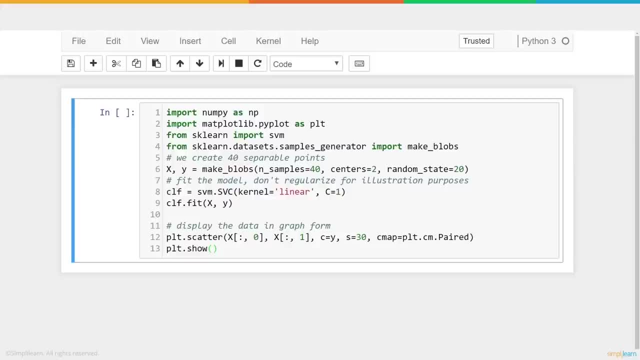 and this is a tool that's in the sklearn to make up data. I personally don't want to go to the zoo, as I work on measuring their snouts and width and length. instead, we're just going to make up some data and that's what that makeblobs is. 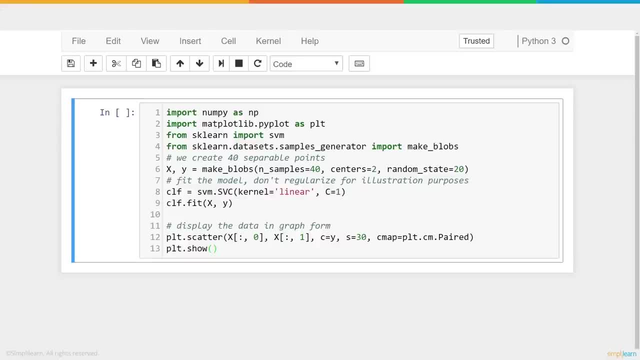 it's a wonderful tool. if you're ready to test your setup and you're not sure about what data you're going to put in there, you can create this blob and it makes it real easy to use. and finally, we have our actual svm- the sklearn import svm- on line 3. 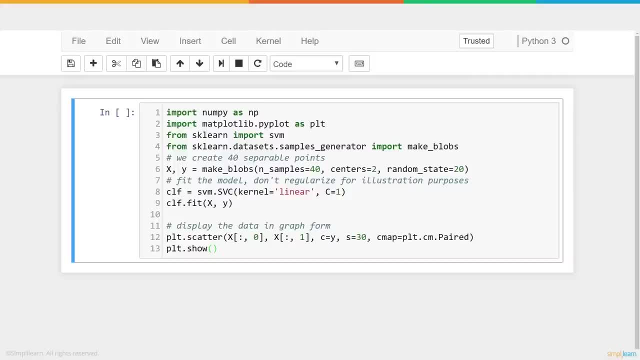 so that covers all our imports. we're going to create- remember I used the makeblobs to create data- and we're going to create a capital x and a lowercase y equals makeblobs in samples equals 40. so we're going to make 40 lines of data. 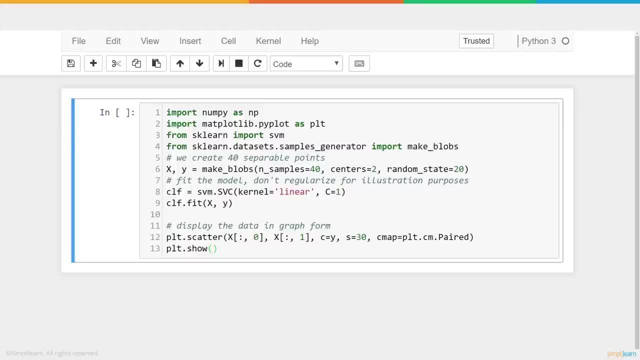 it's going to have 2 centers, with a random state equals 20, so each group is going to have 20 different pieces of data in it and the way that looks is that we'll have under x an xy plane, so we'll have 2 numbers under x. 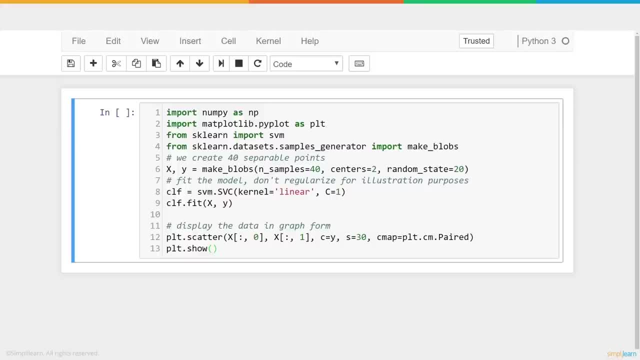 It's going to have two centers with a random state equals 20, so each group is going to have 20 different pieces of data in it, And the way that looks is that we'll have under X an XY plane. So I have two numbers under X and Y will be zero or one. 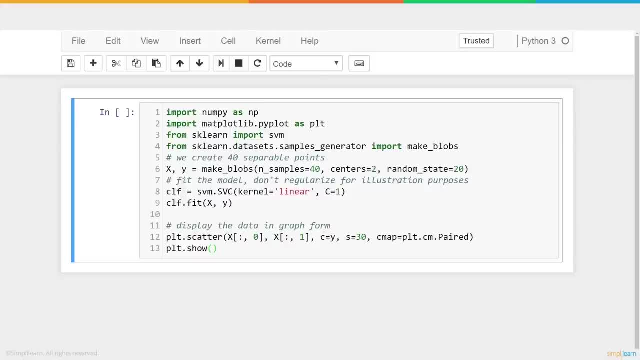 That's the two different centers. So we have a yes or no, in this case alligator or crocodile. That's what that represents. And then I told you that the actual sklearn, or the SVM, is in two lines of code, And we see it right here with: CLF equals SVM, dot SVC kernel equals linear. 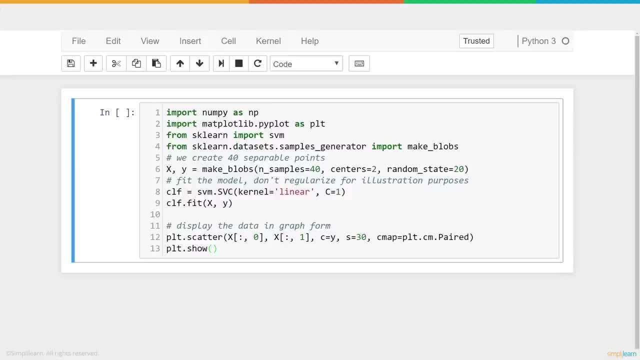 And I set C equal to one, Although in this example, since we are not regularizing the data because we want it to be very clear and easy to see, I went ahead. You can set it to a thousand a lot of times when you're not doing that. 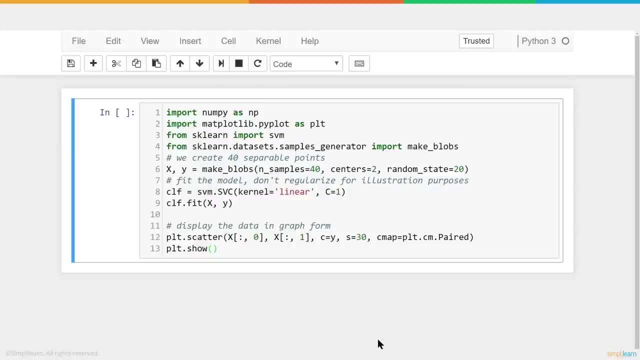 But for this thing- linear, because it's a very simple linear example. we only have the two dimensions and it'll be a nice linear hyperplane. It'll be a nice linear line instead of a full plane, So we're not dealing with a huge amount of data. 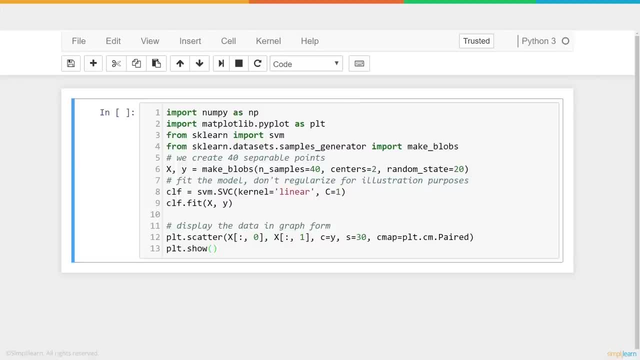 And then all we have to do is do CLF dot fit X, comma Y and that's it. CLF has been created, and then we're going to go ahead and display it, And I'm going to talk about this display here in just a second. 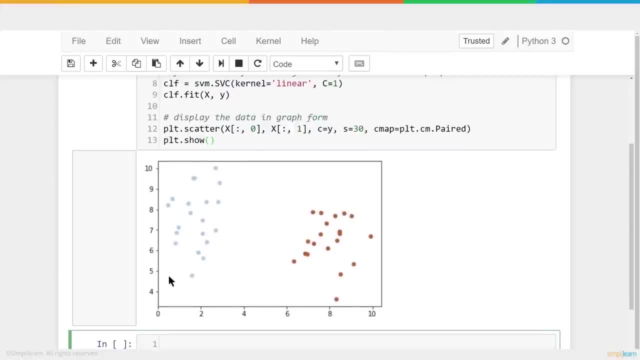 But let me go ahead and run this code, And this is what we've done is we've created two blobs. You'll see the blue on the side and then kind of an orangeish on the other side. That's our two sets of data. 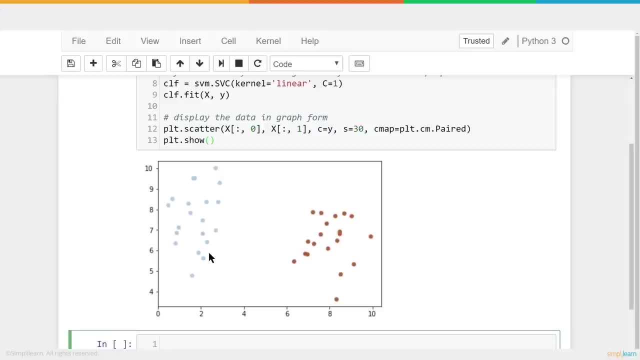 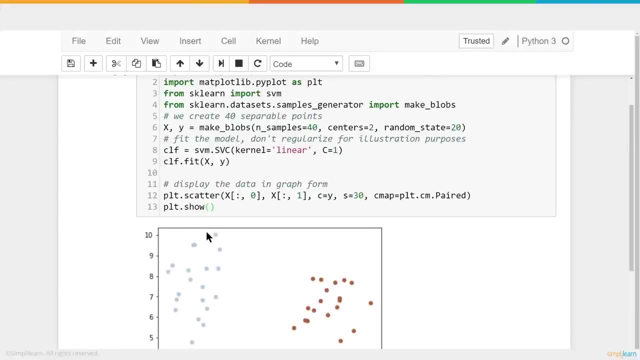 They represent- one represents crocodiles and one represents alligators- And then we have our measurements. In this case we have like the width and length of the snout, And I did say I was going to come up here and talk just a little bit about our plot. 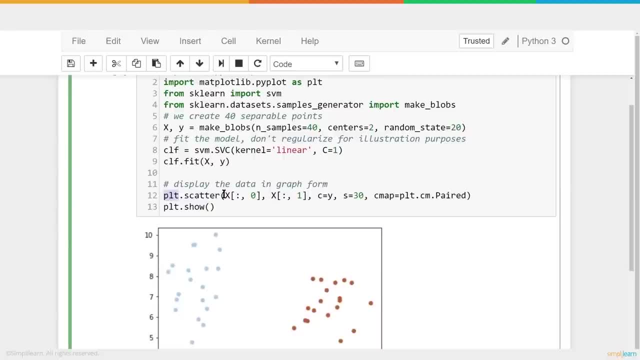 And you'll see PLT, That's what we imported. We're going to do a scatter plot. That means we're just putting dots on there. And then look at this notation: I have the capital X and then in brackets I have a colon, comma zero. 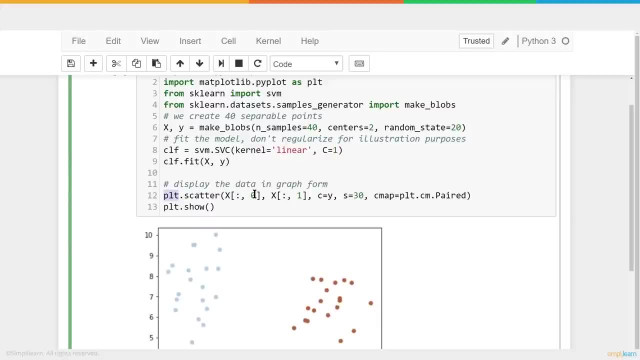 That's from NumPy. If you did that in a regular array, you'll get an error. in a Python array You have to have that in a NumPy array. It turns out that our make blobs returns a NumPy array And this notation is great because what it means is the first part is the colon. 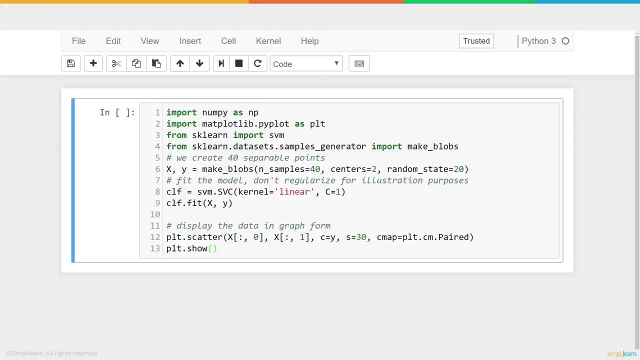 and y will be 0 or 1. that's the 2 different centers. so we have yes or no, in this case alligator or crocodile. that's what that represents. and then we have the svm, which is in 2 lines of code, and we see it right here. 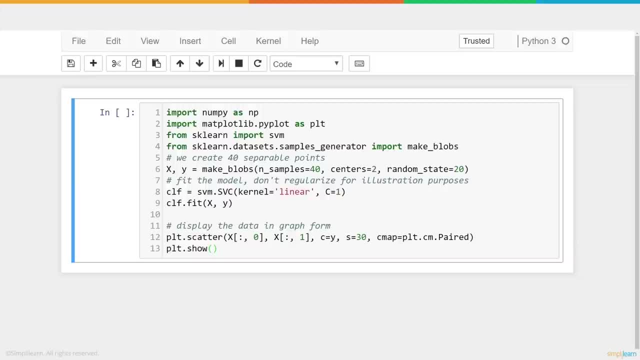 with: clf equals svm, dot, svc, kernel equals linear and I set c equal to 1, although in this example, since we are not regularizing the data, since we want it to be very clear and easy to see, I went ahead and set it to 1000. 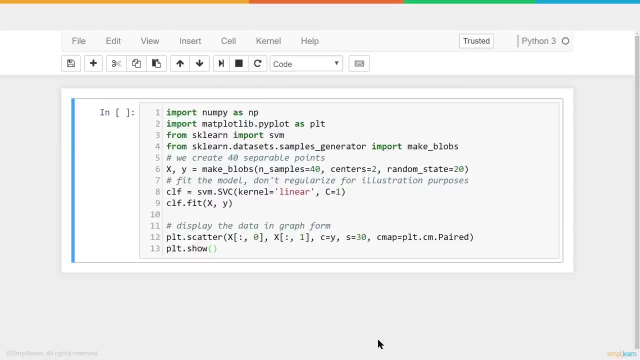 a lot of times when you're not doing that. but for this thing- linear, because it's a very simple linear example- we only have the 2 dimensions and it'll be a nice linear hyperplane. it'll be a nice linear line with a huge amount of data. 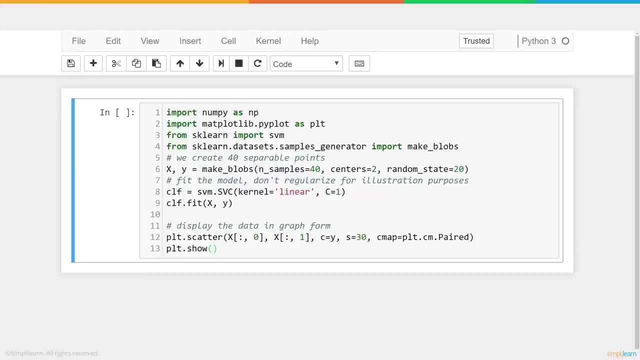 and then all we have to do is do clf, dot fit x, comma y, and that's it. clf has been created, and then we're going to go ahead and display it, and I'm going to talk about this display here in just a second, but let me go ahead and run this code. 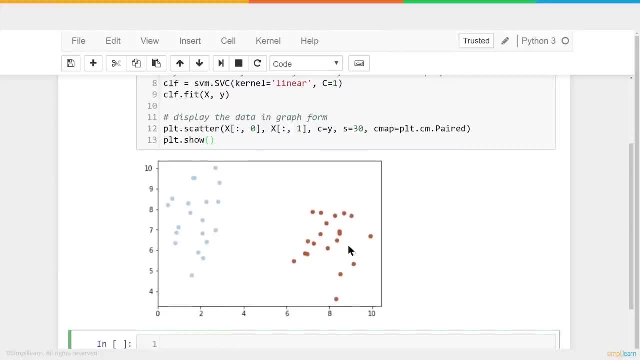 and this is what we've done- is we've created 2 blobs. you'll see the blue on the side and then kind of an orangeish on the other side. that's our 2 sets of data. one represents crocodiles and one represents alligators. 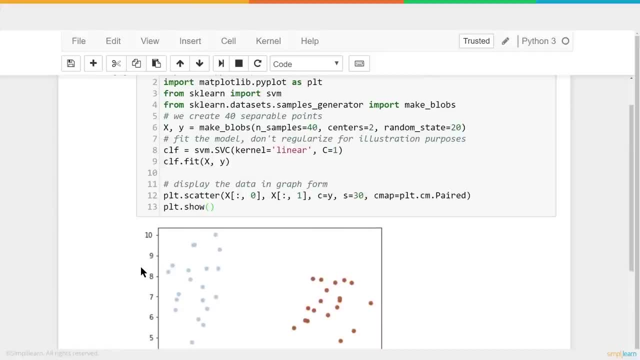 and then we have our measurements: length and length of the snout. and I did say I was going to come up here and talk just a little bit about our plot and you'll see, plt, that's what we imported. we're going to do a scatter plot. 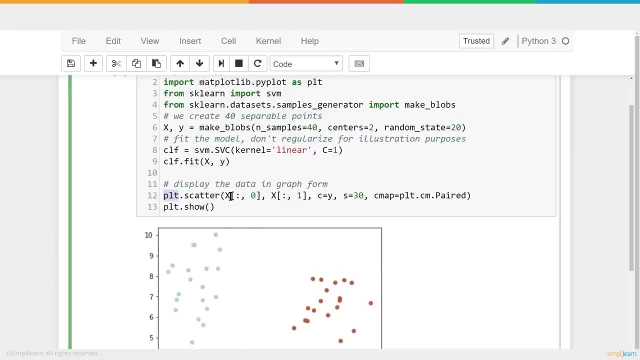 that means we're just putting dots on there. and then look at this notation: I have the capital X and then in brackets I have a colon, comma, zero. that's from numpy. if you did that in a regular array, you'll get an error in a python array. 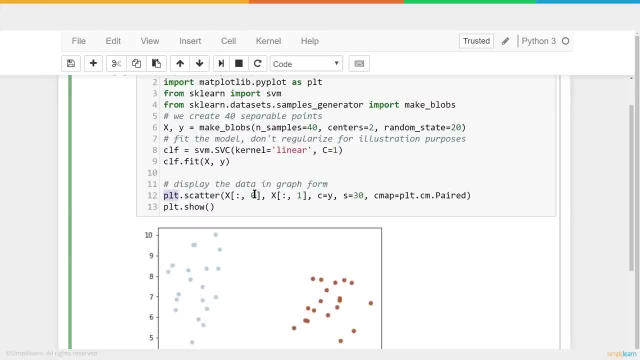 you have to have that in a numpy array. it turns out that our make blobs returns a numpy array and this notation is great and what that means is the first part is the colon means we're going to do all the rows. that's all the data in our blob we created under capital X. 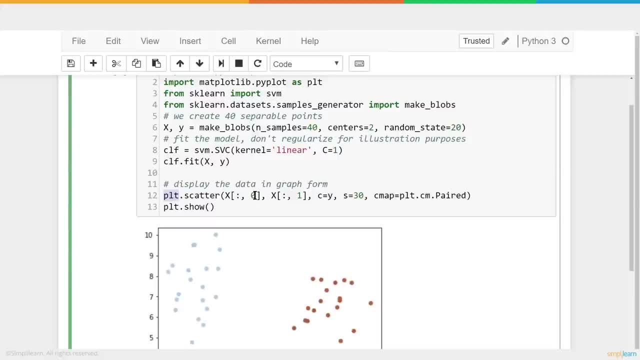 and then the second part has a comma zero. we're only going to take the first value and then, if you notice, we do the same thing but we're going to take the second value. remember we always start with zero and then one, so we have column zero and column one. 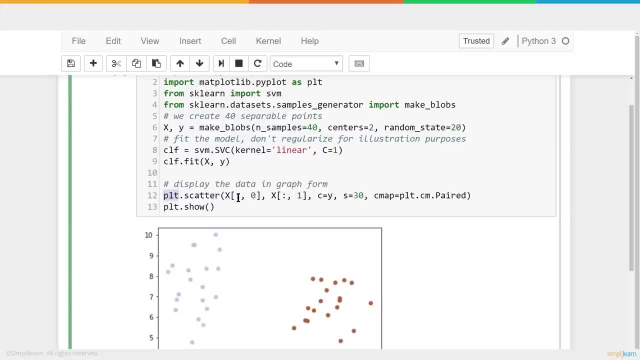 Means we're going to do all the rows. That's all the data in our blob we created under capital X, And then the second part has a comma zero. We're only going to take the first value And then, if you notice, we do the same thing, but we're going to take the second value. 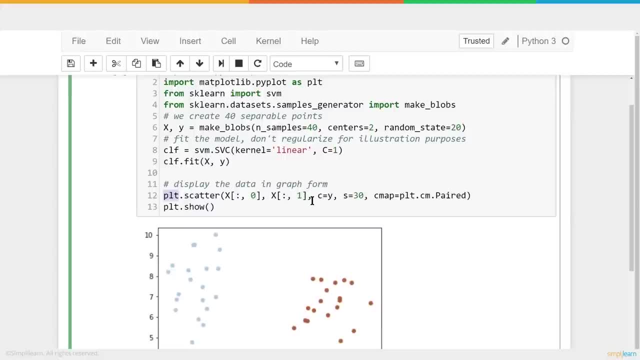 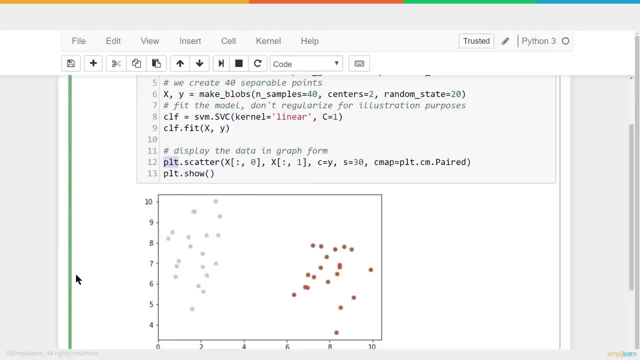 We always start with zero and then one. So we have column zero and column one, And you can look at this as our X- Y plots. The first one is the X plot and the second one is the Y plot. So the first one is on the bottom. zero, two, four, six, eight and ten. 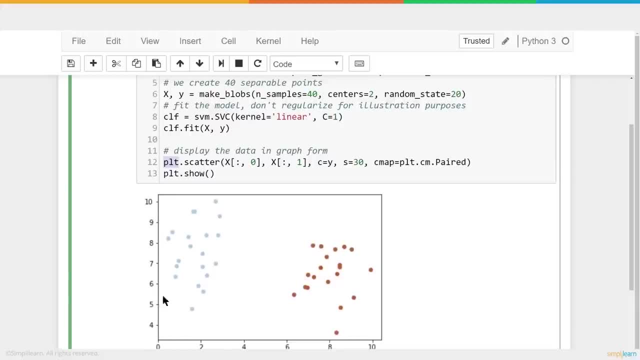 And then the second one, X of the one is the four, five, six, seven, eight, nine, ten, going up the left hand side. S equals 30. It's just the size of the dot, So we can see them instead of real tiny dots. 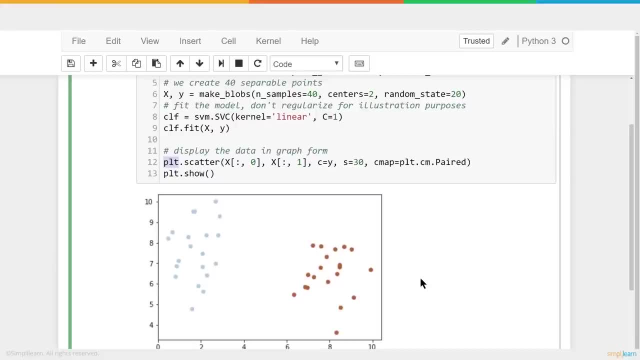 And then the C map equals PLT dot, CM dot paired And you'll also see the C equals Y. That's the color We're using, two colors, zero one, And that's why we get the nice blue and the two different colors for the alligator. 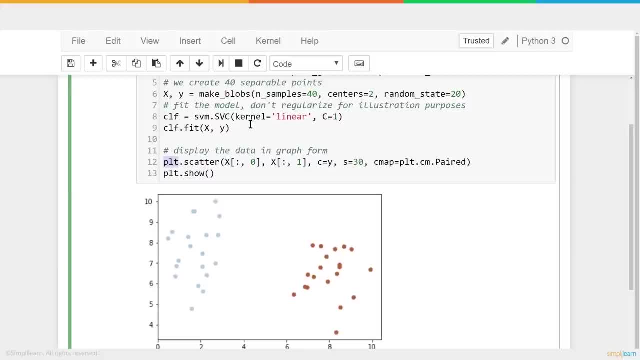 and the crocodile. Now you can see here that we did this. The actual fit was done in two lines of code. A lot of times will be a third line where we regularize the data. We set it between like minus one and one and we reshape it. 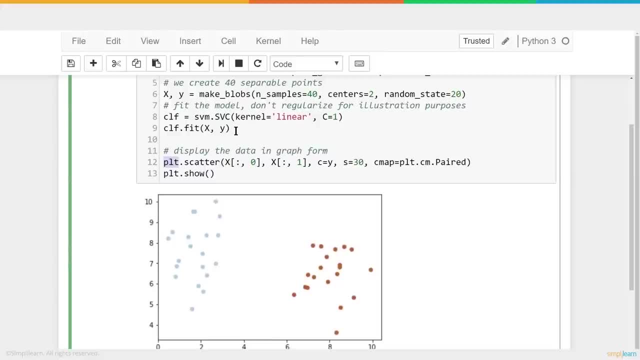 For this. it's not necessary, And it's also kind of nice because you can actually see what's going on. And then, if we wanted to, we wanted to actually run a prediction. Let's take a look and see what that looks like. 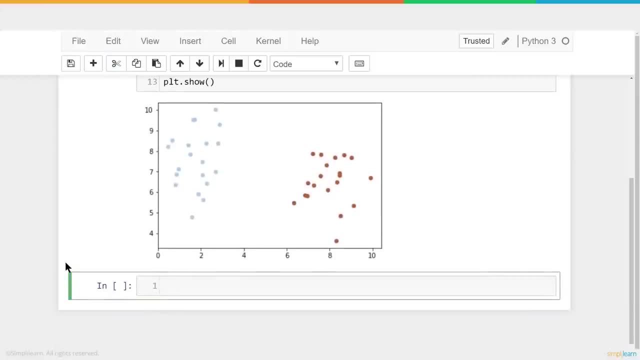 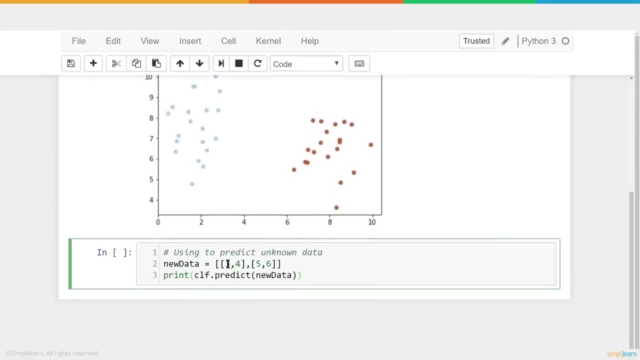 And to predict some new data, And we'll show this again as we get towards the end of digging in deep. You can simply assign your new data. In this case, I am giving it a width and length three, four and a width and length five, six. 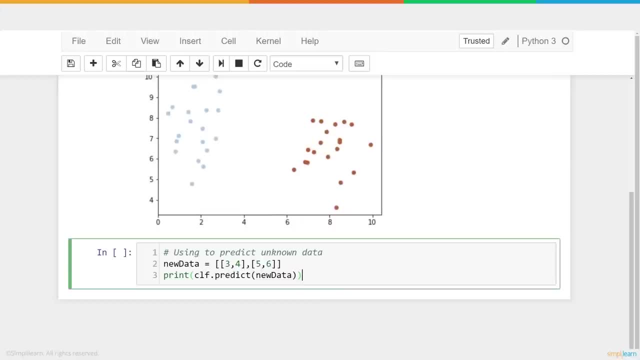 And note that I put the data as a set of brackets and then I have the brackets inside, And the reason I do that is because when we're looking at data, it's designed to process a large amount of data coming in. We don't want to just process one line at a time. 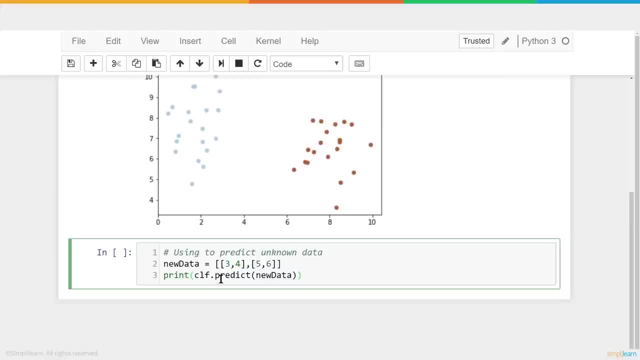 And so in this case I'm processing two lines and then I'm just going to print And you'll see: CLF- dot- predict new data. So the CLF and the dot predict part is going to give us an answer And let's see what that looks like. 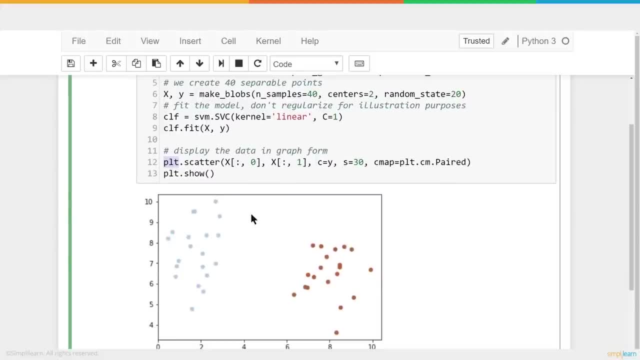 and you can look at this as our xy plots. the first one is the x plot and the second one is the y plot. so the first one is on the bottom- four, six, eight and ten, and then the second one, x. of the one is the four, five, six, seven, eight, nine, ten. 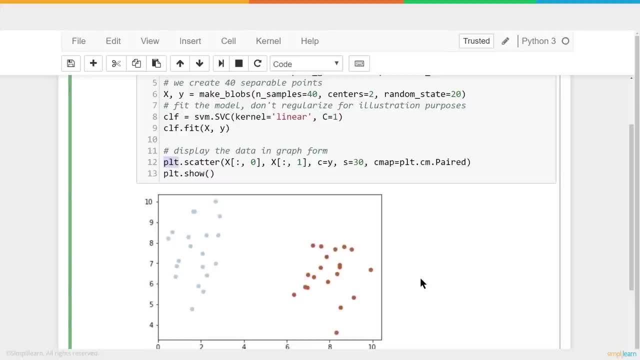 going up, the left hand side s equals thirty is just the size of the dot, so we can see them instead of real tiny dots. and then cmap equals plt, dot, cm dot paired and you'll also see the c equals y. that's the color we're using, two colors. 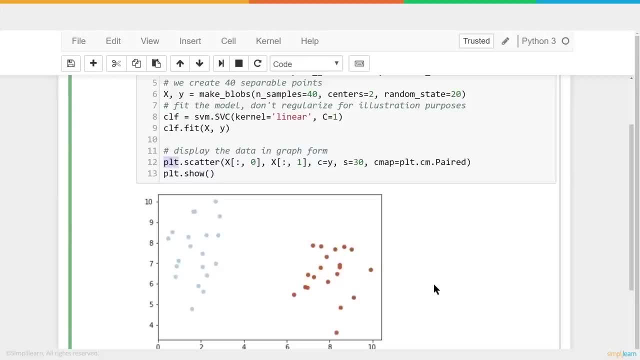 zero one, and that's why we get the nice blue and the two different colors for the alligator and the crocodile. now you can see here that we did this. the actual fit was done in two lines of code. a lot of times it'll be a third line. 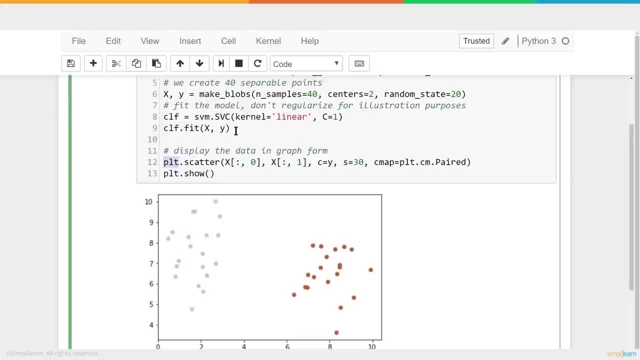 where we regularize the data, we set it between like minus one and one and we reshape it. but for this it's not necessary and it's also kind of nice because you can actually see what's going on. and then, if we wanted to, we wanted to actually run a prediction. 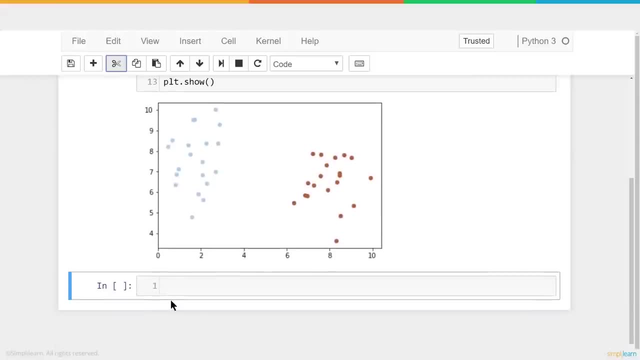 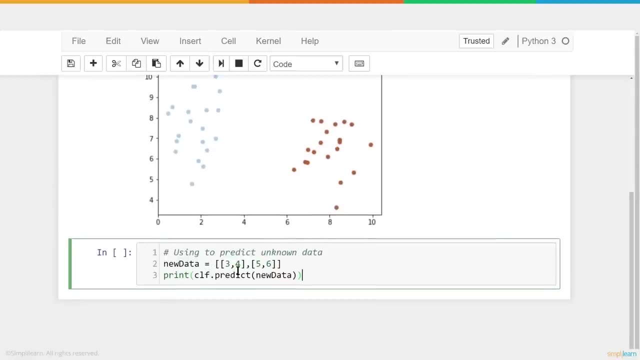 let's take a look and see what that looks like and to predict some new data, and we'll show this again as we get towards the end of digging in deep. you can simply assign your new data in this case. I am giving it a length: three, four. 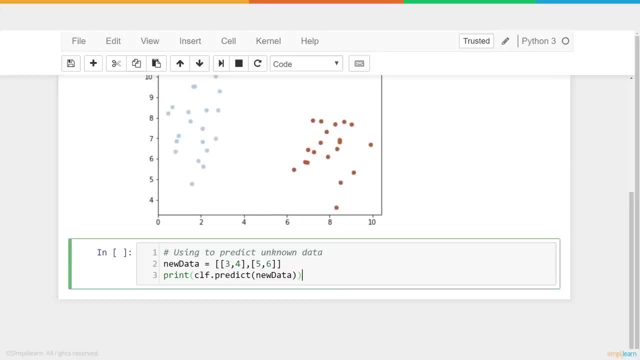 and a width and length, five, six, and note that I put the data as a set of brackets and then I have the brackets inside, and the reason I do that is because when we're looking at data, it's designed to process a large amount of data coming in. 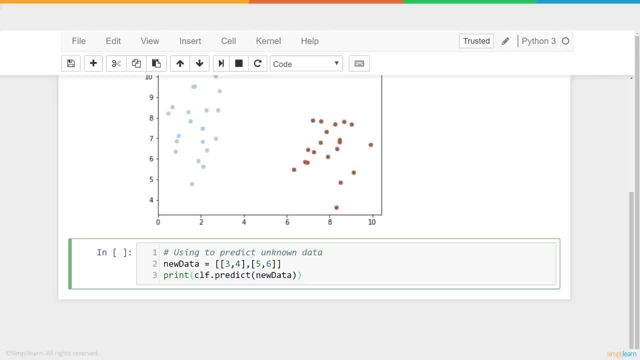 we don't want to just process one line at a time, and so in this case I'm processing two lines and then I'm just going to print and you'll see: clf- dot- predict new data. so the clf and the dot- predict part is going to give us an answer. 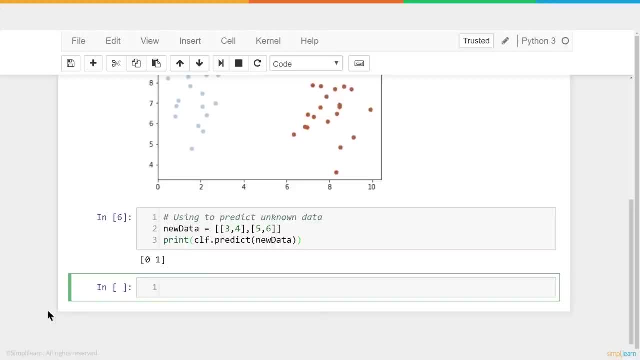 and let's see what that looks like. so it predicted the first one, the three- four is going to be on the one side and the five- six is going to be on the other side. so one came out as an alligator and one came out as a crocodile. 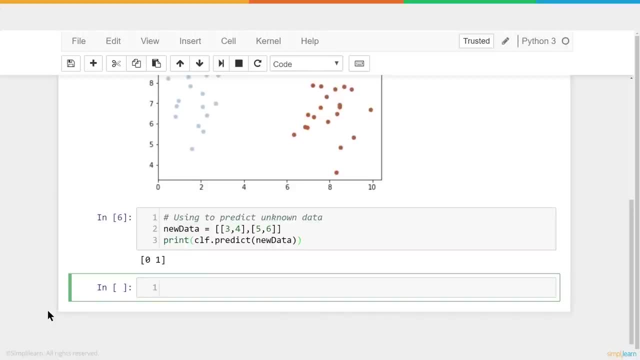 And you'll see zero one. So predicted the first one, the three, four is going to be on the one side and the five, six is going to be on the other side. So one came out as an alligator And one came out as an alligator. 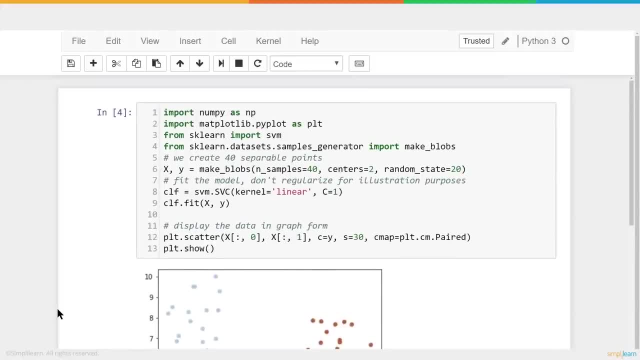 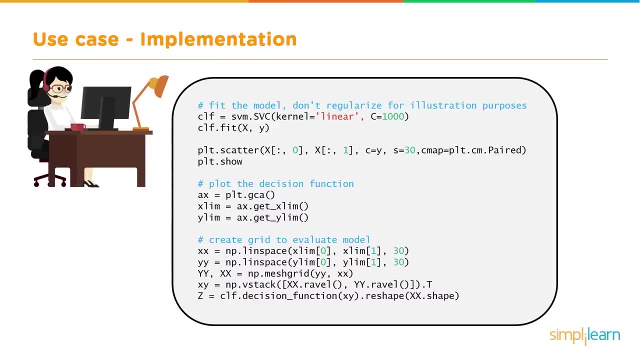 And one came out as a crocodile. Now, that's pretty short explanation for the setup, But really we want to dig in and see what is going on behind the scenes And let's see what that looks like. So the next step is to dig in deep and find out what's going on behind the scenes. 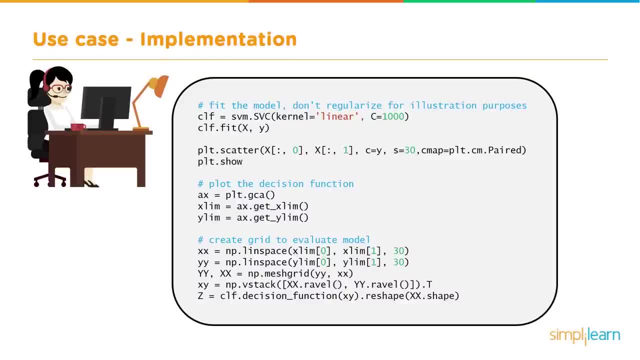 And also put that in a nice pretty graph. We're going to spend more work on this than we did actually generating the original model, And you'll see here that we go through a few steps and I'll move this over to our editor in just a second. We come in, we create our original data. 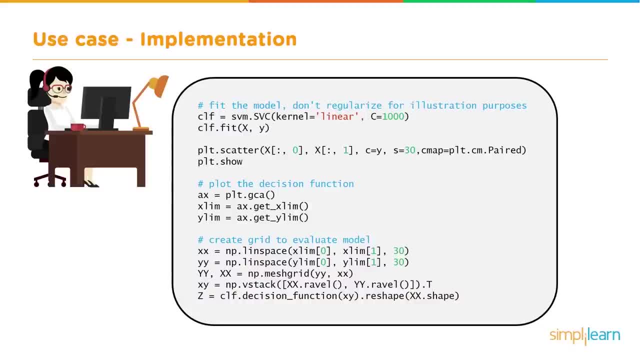 It's exactly identical to the first part And I'll explain why we redid that and show you how not to redo that. And then we're going to go in there and add in those lines. We're going to see what those lines look like and how to set those up. 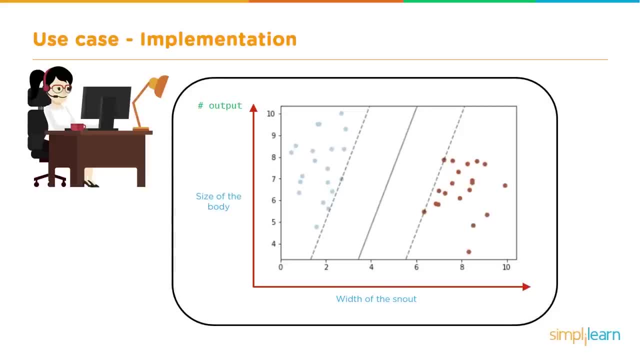 And finally, we're going to plot all that on here and show it And you'll get a nice graph with the what we saw earlier when we were going through the theory behind this, where it shows the support vectors and the hyperplane And those are done, where you can see. 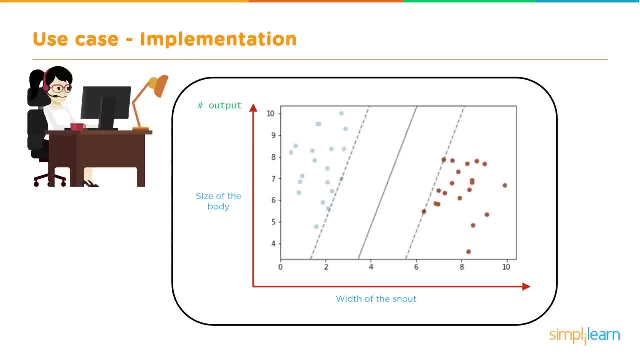 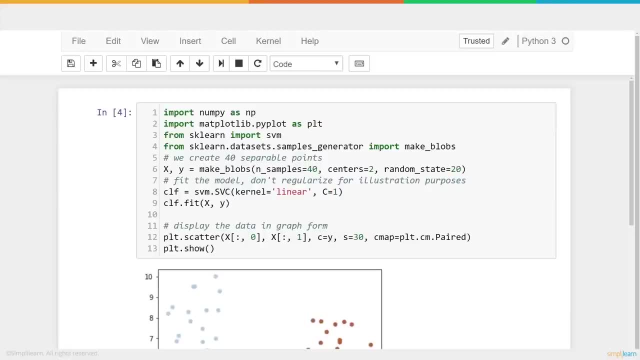 the support vectors as the dashed lines and the solid line, which is the hyperplane. Let's get that into our Jupyter notebook. Before I scroll down to a new line, I want you to notice line 13.. It has plot show. 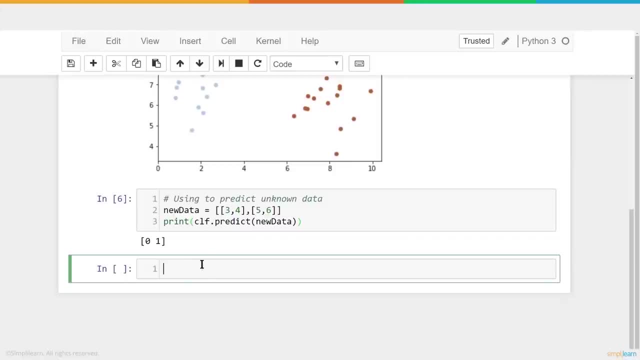 And we're going to talk about that here in just a second. But let's scroll down to a new line down here and I'm going to paste that code in And you'll see that the plot show has moved down below. Let's scroll up a little bit. 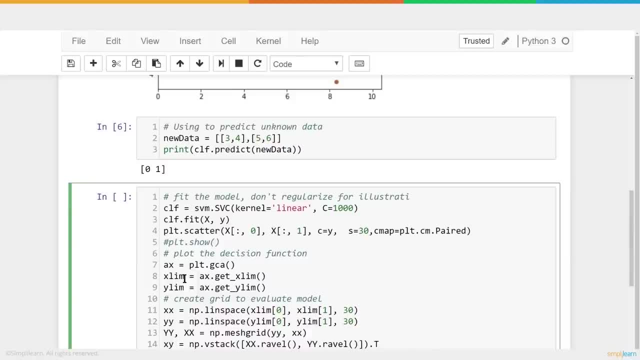 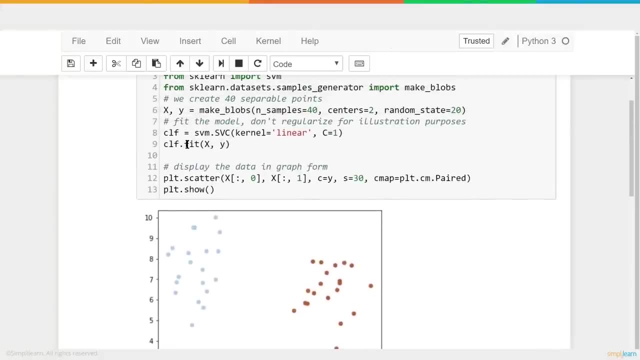 And if you look at the top here of our new section, one, two, three and four is the same code we had before, And let's go back up here and take a look at that. We're going to fit the values And our SVM and then we're going to plot, scatter it and then we're going to do a plot show. 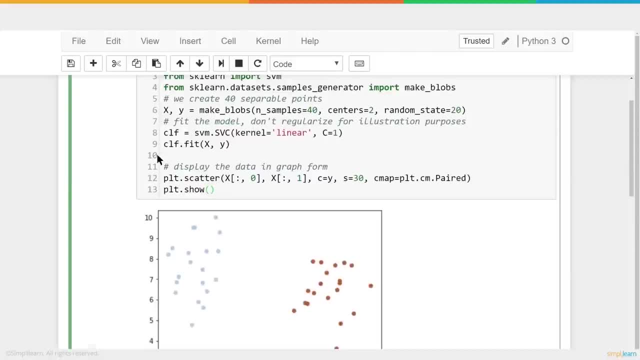 So you should be asking: why are we redoing the same code? Well, when you do the plot show, that blanks out what's in the plot. So once I've done this plot show, I have to reload that data. Now we could do this simply by removing it up here, rerunning it and then coming. 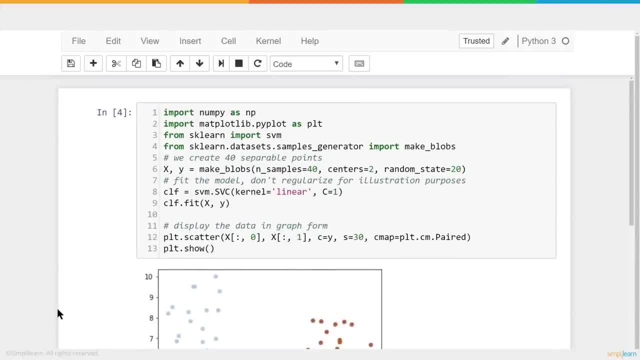 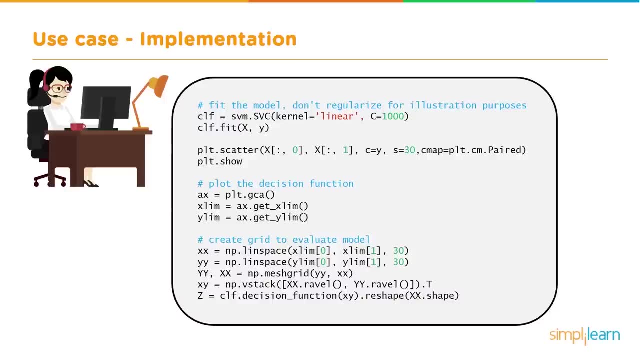 now, that's a pretty short explanation for this setup, but really we want to dig in and see what's going on behind the scenes, and let's see what that looks like. so the next step is to dig in deep and find out what's going on behind the scenes. 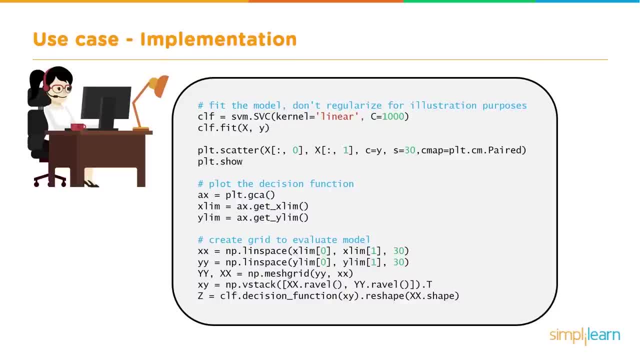 and also put that in a nice pretty graph. we're going to spend more work on this than we did actually generating the original model, and you'll see here that we go through a few steps and I'll move this over to our editor in just a second. 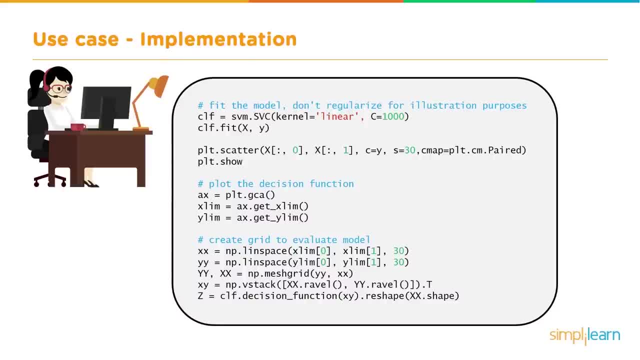 we come in, we create our original data. it's exactly identical to the first part and I'll explain why we redid that and show you how not to redo that. and then we're going to go in there and add in those lines. we're going to see what those lines look like. 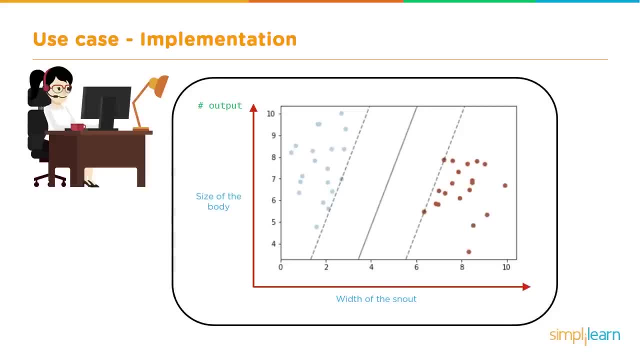 and how to set those up. and finally, we're going to plot all that on here and show it and you'll get a nice graph with what we saw earlier when we were going through the theory behind this: support vectors and the hyperplane, and those are done, where you can see. 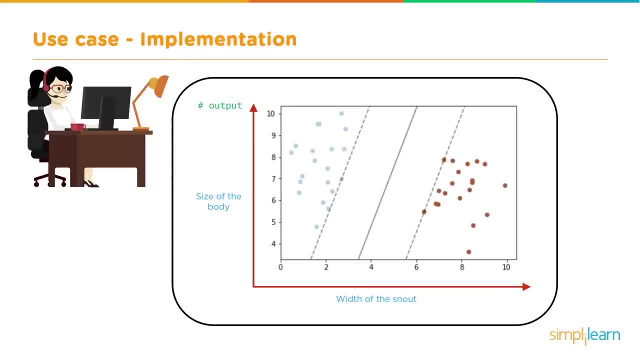 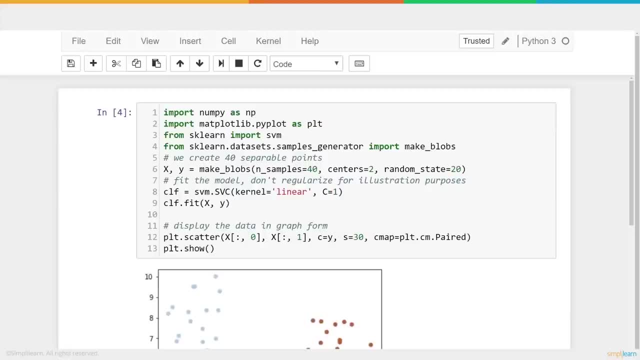 the support vectors as the dashed lines and the solid line, which is the hyperplane. let's get that into our Jupyter notebook. before I scroll down to a new line, I want you to notice line 13. it has plot show and we're going to talk about that here in just a second. 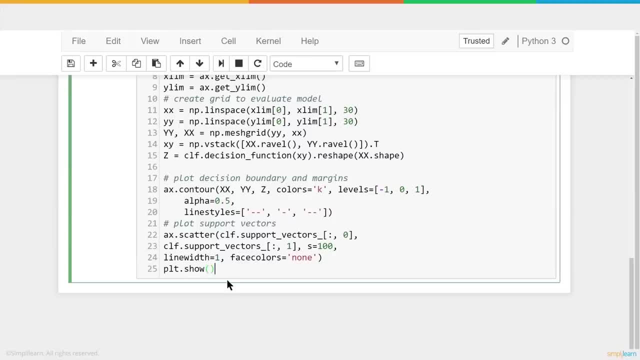 but let's scroll down to a new line down here and I'm going to paste that code in and you'll see that the plot show has moved down below. let's scroll up a little bit and if you look at the top here of our new section, 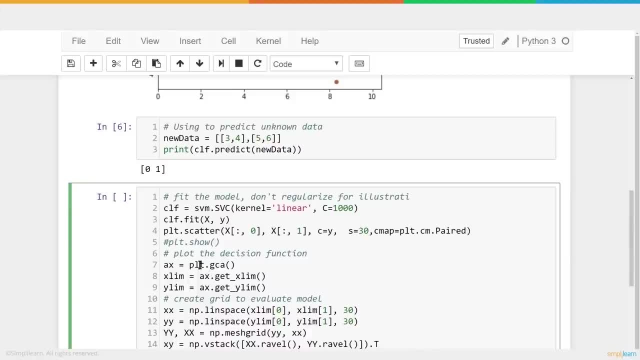 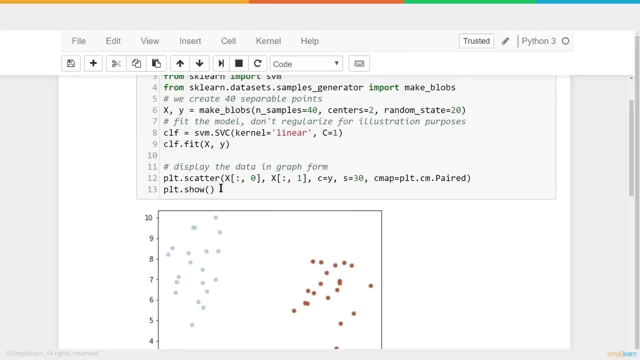 1,, 2,, 3, and 4 is the same code we had before, and let's go back up here and take a look at that. we're going to fit the values on our SVM and then we're going to plot, scatter it. 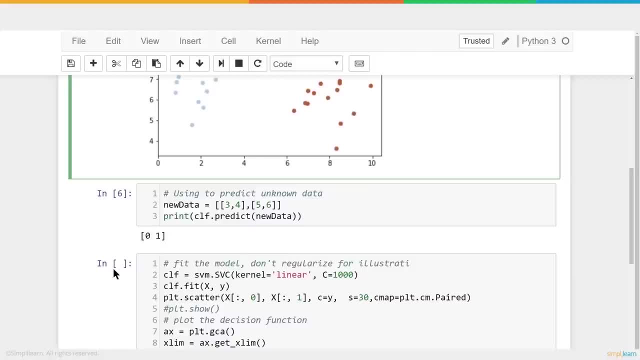 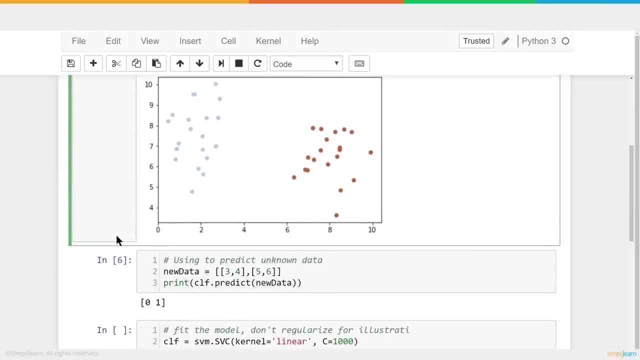 and then we're going to do a plot show. so you should be asking: why are we redoing the same code? well, when you do the plot show, that blanks out what's in the plot. so once I've done this plot show, I have to reload that data. 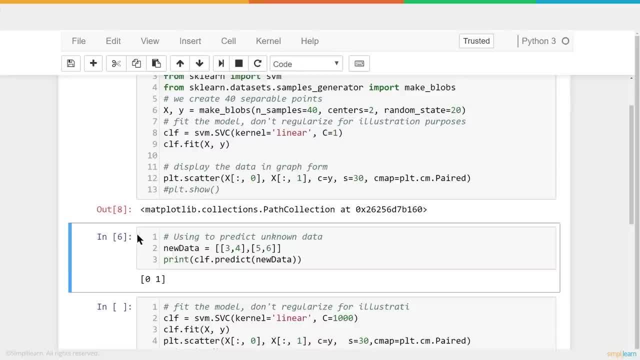 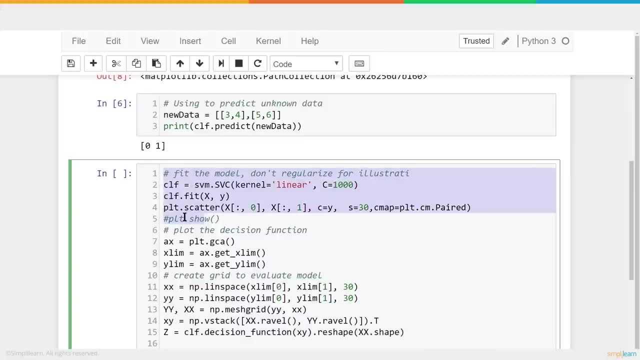 now we could do this simply by removing it up here, re-running it and then coming down here, and then we wouldn't have to re-run these first four lines of code now in this. it doesn't matter too much and you'll see the plot show is down here and then removed. 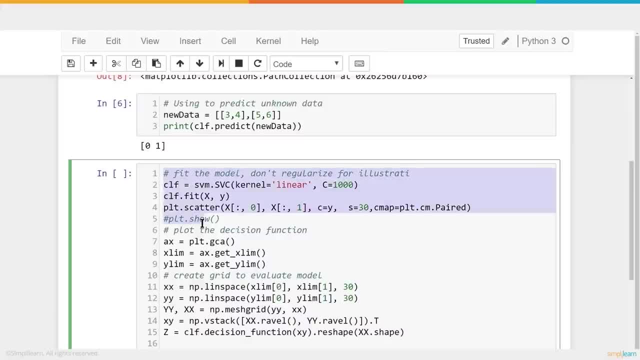 down here and then we wouldn't have to rerun these first four lines of code. Now in this it doesn't matter too much And you'll see the plot show is down here and then removed right There on line five. 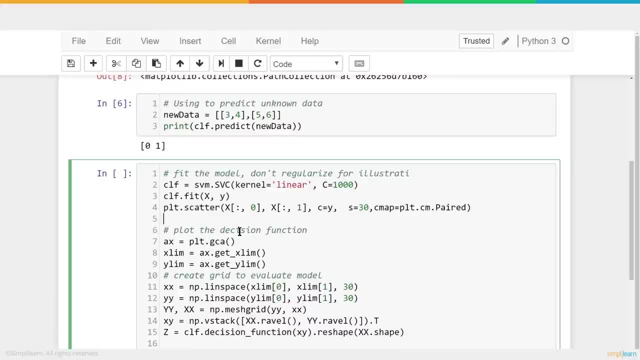 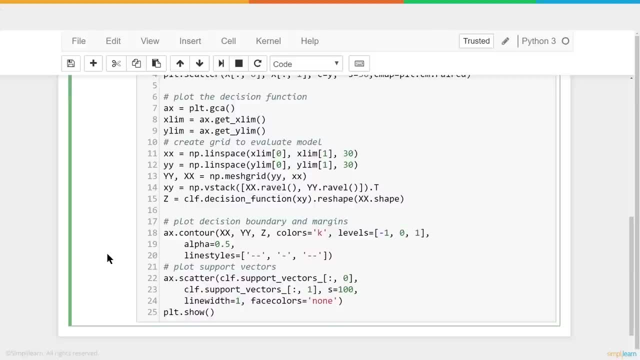 I'll go ahead and just delete that out of there, because we don't want to blank out our screen, We want to move on to the next setup. So we can go ahead and just skip the first four lines, because we did that before, And let's take a look at the. AX equals PLTGCA. 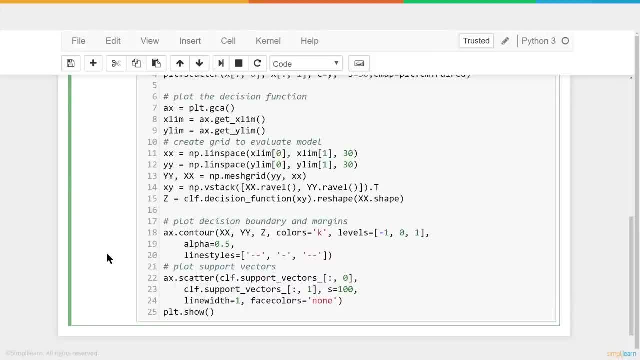 Now, right now, we're actually spending a lot of time just graphing. That's all we're doing here, OK, so this is how we display a nice graph with our results and our data. AX is very standard used variable when you're talking about PLT. 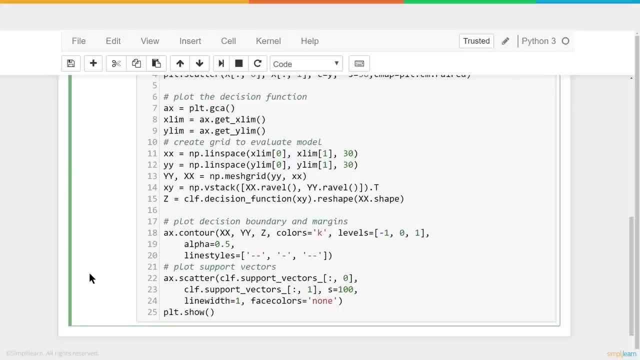 And it's just setting it to that axes the last axes in the PLT. It can get very confusing if you're working with many different layers of data on the same graph And this makes it very easy to reference the AX. So this reference is looking at the PLT. 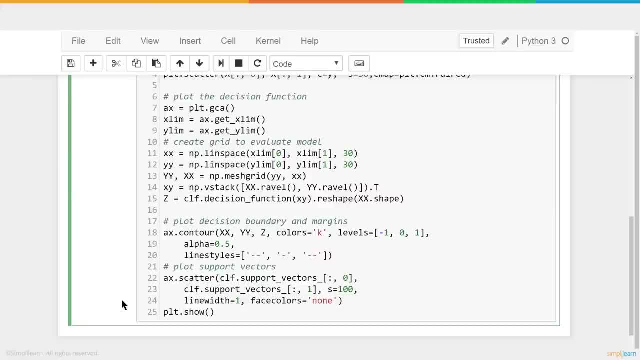 that we created and we already mapped out our two blobs on. And then we want to know the limits. So we want to know how big the graph is. We can find out the X limit and the Y limit simply with the get- X limit and get. 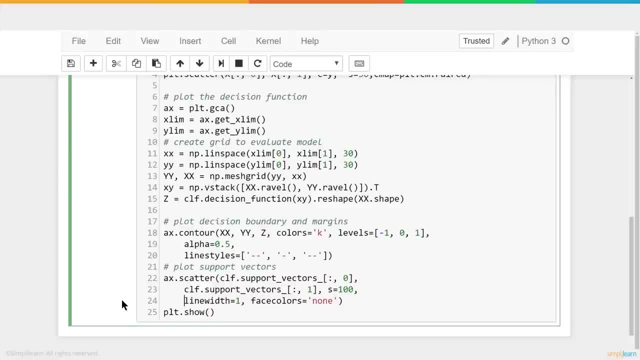 Y limit commands, which is part of our met plot library, And then we're going to create a grid and you'll see down here we have. we've set the variable X, X equal to NP dot line, space, X limit: zero. X limit one comma: 30.. 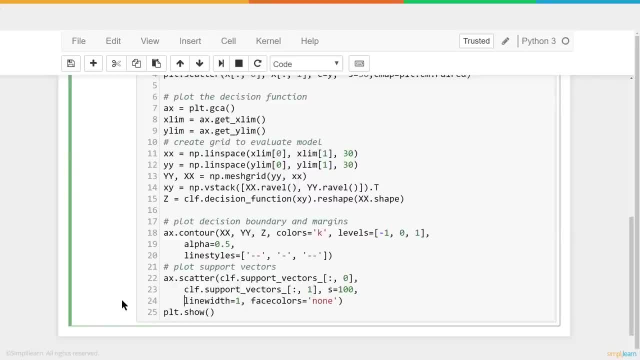 And we've done the same thing for the Y space. And then we're going to go in here and we create a mesh grid And this is a numpy command. So we're back to our numbers, Python. Let's go through what these numpy. 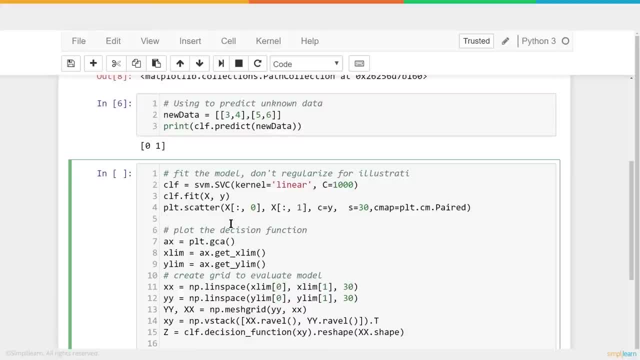 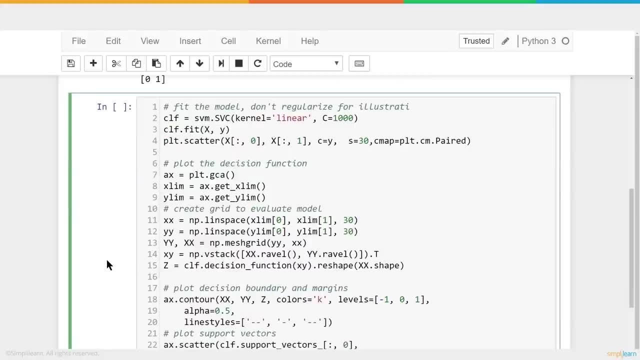 right there on line 5. I'll go ahead and just delete that out of there, because we don't want to blank out our screen. we want to move on to the next setup. so we can go ahead and just skip the first four lines, because we did that before. 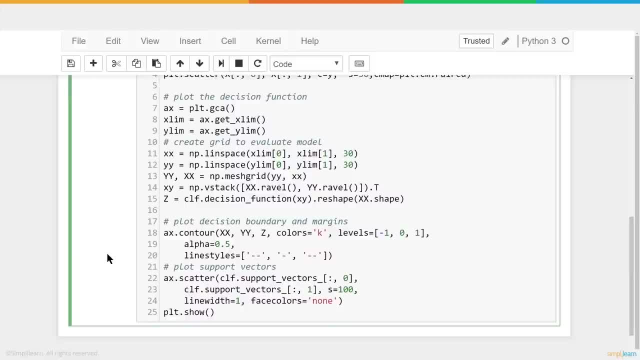 and let's take a look at the ax equals plt, dot, gca. now, right now, we're actually spending a lot of time just graphing. that's all we're doing here. this is how we display a nice graph with our results and our data. ax is a very standard used variable. 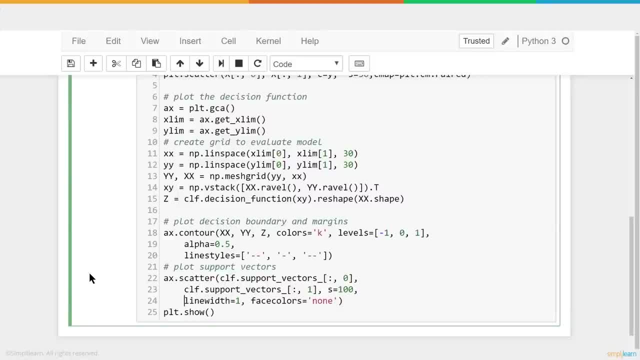 when you're talking about plt and it's just setting it to that axis, the last axis in the plt. it can get very confusing if you're working with many different layers of data on the same graph and this makes it very easy to reference the ax. so this reference is looking at the plt. 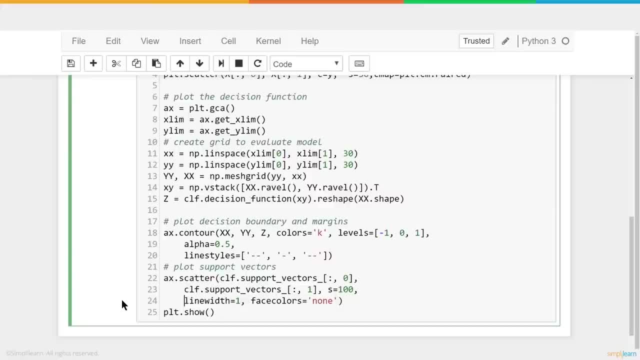 that we created and we already mapped out our two blobs on. and then we want to know the limits, so we want to know how big the graph is. so we're going to start with the x limit and the y limit, simply with the get x limit and get y limit commands. 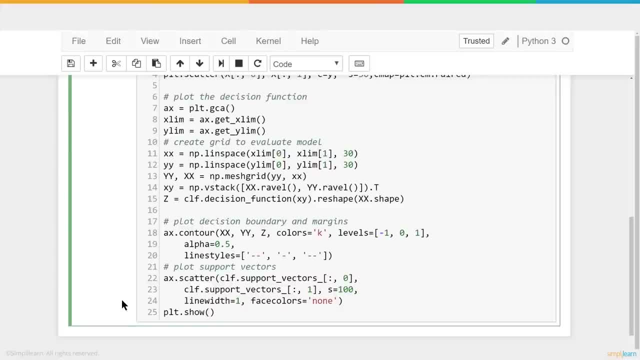 which is part of our matplot library, and then we're going to create a grid and you'll see down here we have: we've set the variable xx equal to np dot linespace, x limit 0,. x limit 1, comma 30, and we've done the same thing for the y space. 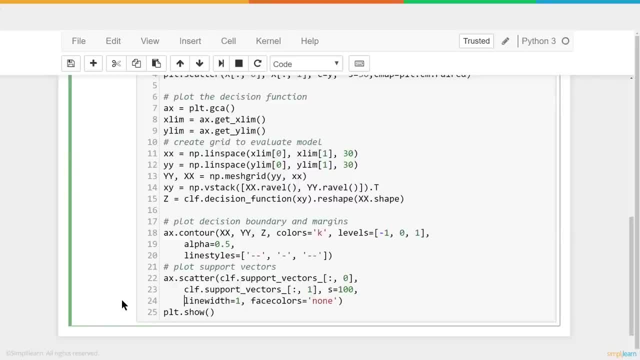 and then we're going to go in here and we create a mesh grid and this is a numpy command. so we're back to our numbers, python. so let's go through what these commands mean. with the linespace and the mesh grid, we've taken xx small. xx equals np linespace. 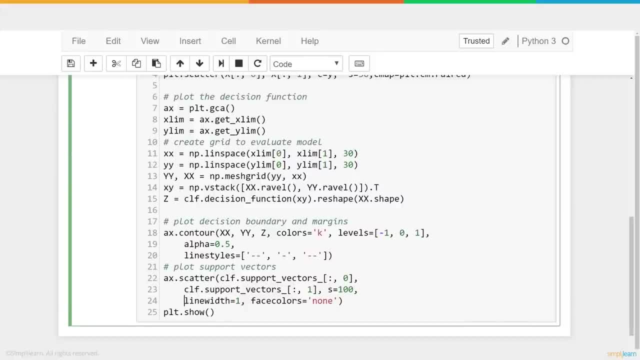 and we have our x limit 0 and our x limit 1, and we're going to create 30 points on it and we're going to do the same thing for the y axis. now, this has nothing to do with our evaluation. all we're doing is we're creating. 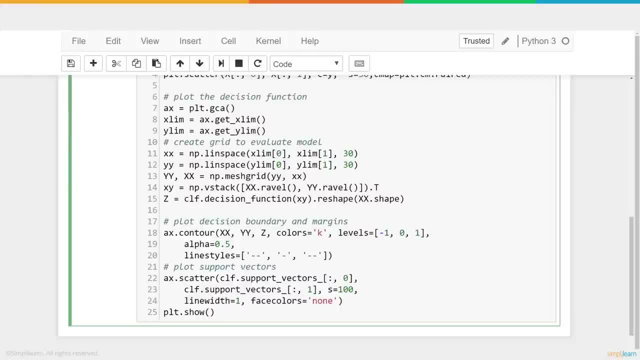 a grid of data, and so we're creating a set of points between 0 and the x limit. we're creating 30 points, and the same thing with the y. we're putting those all together so it forms a nice grid. so if we were going to do this, 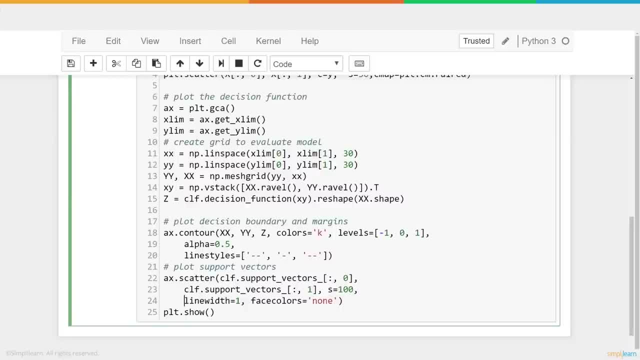 commands mean with the line space and the mesh grid. We've taken X X small. X X equals NP line space And we have our X limit zero and our X limit one And we're going to create 30 points on it And we're going to do the same thing for the Y axis. 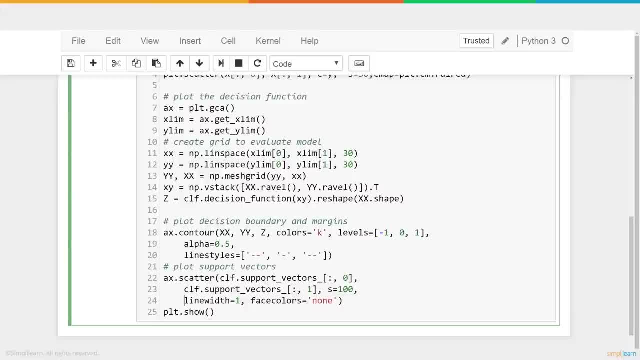 Now, this has nothing to do with our evaluation. It's all we're doing is we're creating a grid of data, And so we're creating a set of points between zero and the X limit. We're creating 30 points, and the same thing with the Y. 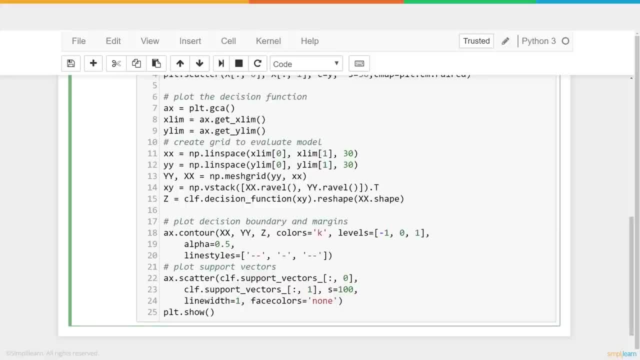 And then the mesh grid loops those all together, So it forms a nice grid. So if we were going to do this, say between the limit zero and ten, and do ten points, we would have a zero zero one, one zero one, zero, two, zero, three, zero four to ten, and so on. 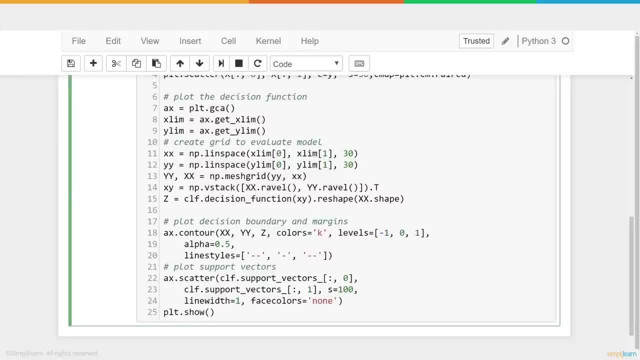 You can just imagine a point at each corner, one of those boxes, and the mesh grid combines them all. So we take the Y- Y and the X- X, we created and creates the full grid And we've set that grid into the Y- Y coordinates and the X- X coordinates. 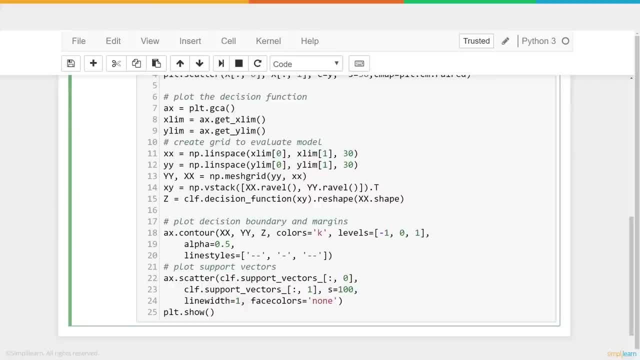 Now remember, we're working with numpy and Python. We like to separate those We like to have, instead of it being X comma one, X comma Y, and then X two comma Y two, and in the next set of data it would be a column of X's and a column of Y's. 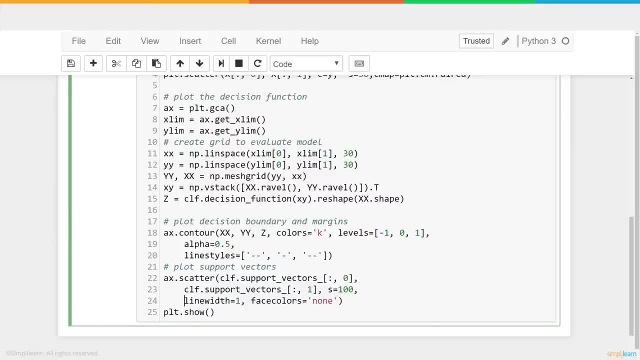 And that's what we have here is we have a column of Y's and we put it as a capital Y, Y, and a column of X's- capital, X, X, with all those different points being listed, And finally we get down to the numpy V stack, just as we created those in the mesh. 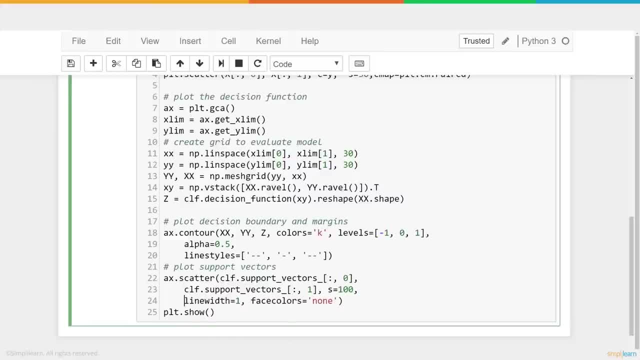 grid. we're now going to put them all into one array: X, Y array. Now that we've created the stack of data points, we're going to do something interesting here. We're going to create a value, Z, and the Z equals the CLF. 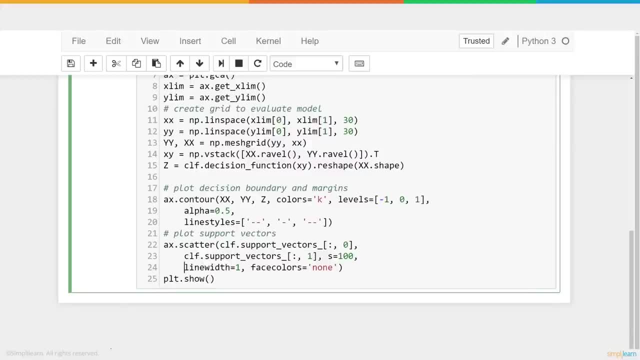 That's our, that's our support vector machine. we created and we've already trained and we have a dot decision function and we're going to put the X- Y in there. So here we have all this data. We're going to put that X- Y in there, that data. 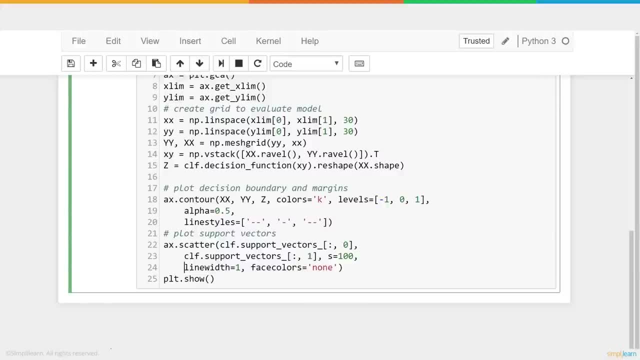 We're going to reshape it and you'll see that we have the X- X dot shape in here. This literally takes the X- X, resets it up connected to the Y and the Z value, lets us know whether it is the left hand side, is going to generate three different values. 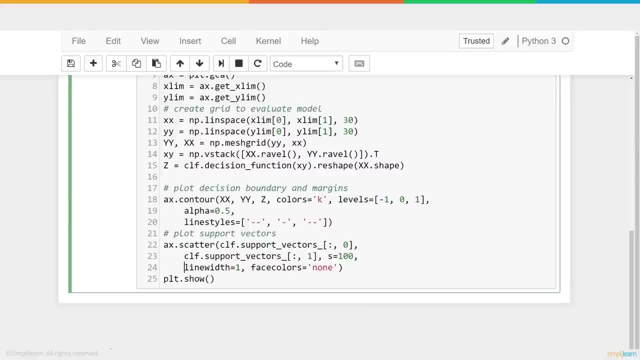 The Z value does, and it'll tell us whether that data is a support vector to the left, the hyperplane in the middle or the support vector to the right. So it generates three different values for each of those points and those points have been reshaped so that they're right on a line on those three different lines. 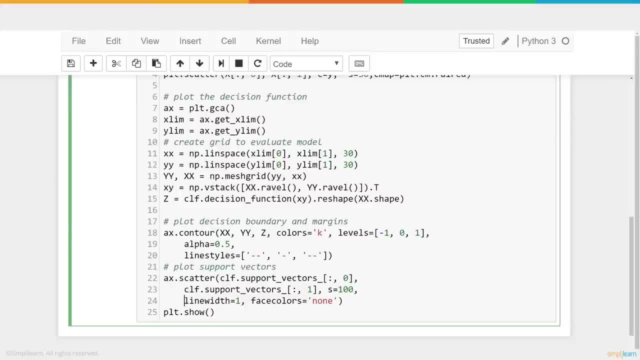 say between the limit 0 and 10 and do 10 points, we would have a 0, 0, 1, 1, 0, 1, 0,, 2,, 0,, 3,, 0,, 4 to 10. 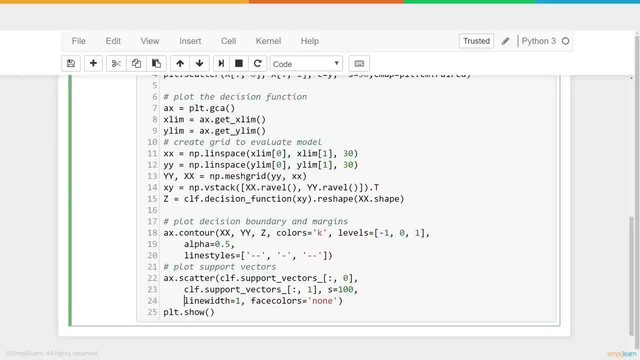 and so on. you can just imagine a point at each corner of one of those boxes and the mesh grid combines them all. so we take the yy and the xx, we created and creates the full grid and we've set that grid into the yy coordinates and the xx coordinates. 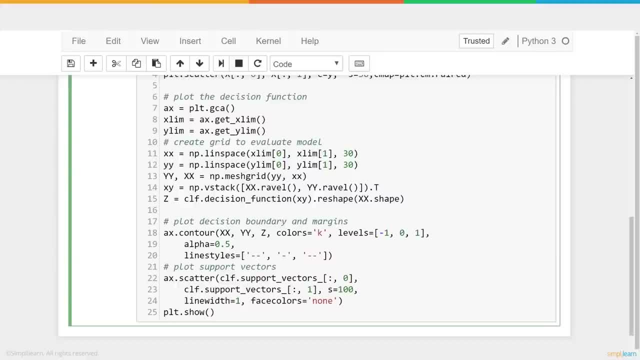 we like to have, instead of it being x comma 1, x comma y and then x2 comma y2, in the next set of data it would be a column of x's and a column of y's, and that's what we have here. we have a column of y's. 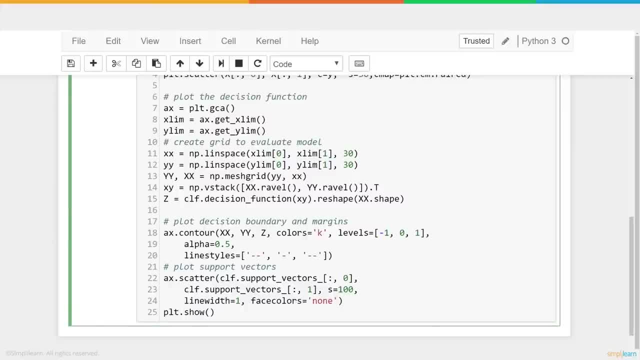 we put it as a capital yy and a column of x's capital xx, with all those different points being listed, and finally we get down to the numpy v stack. just as we created those in the mesh grid, we're now going to put them all into one array. 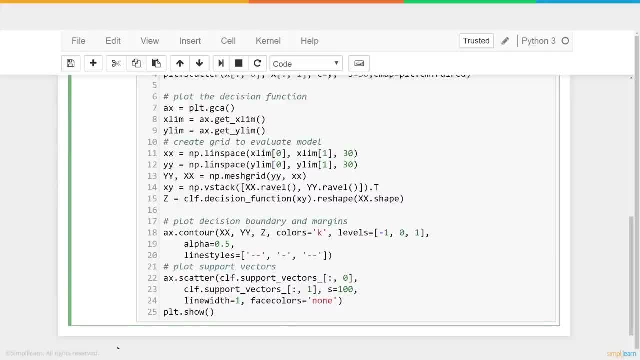 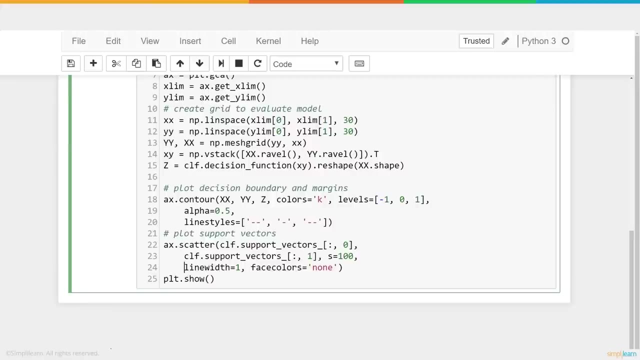 xy array. now that we've created the stack of data points, we're going to do something interesting here. we're going to create a value, z, and the z equals the clf. that's our support vector machine. we created and we've already trained and we have a dot decision function. 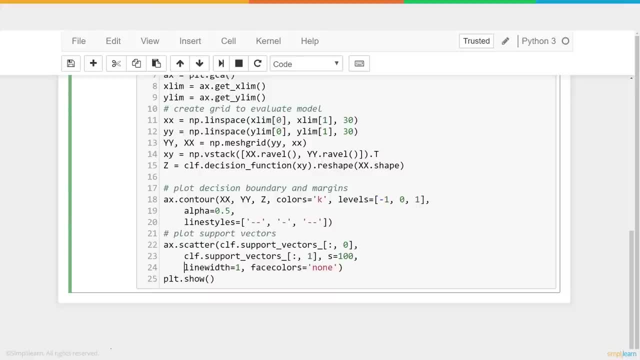 and we're going to put the xy in there. so here we have all this data, we're going to put that xy in there, we're going to reshape it and you'll see that we have the xx dot shape in here. this literally takes the xx, resets it up, connected to the y. 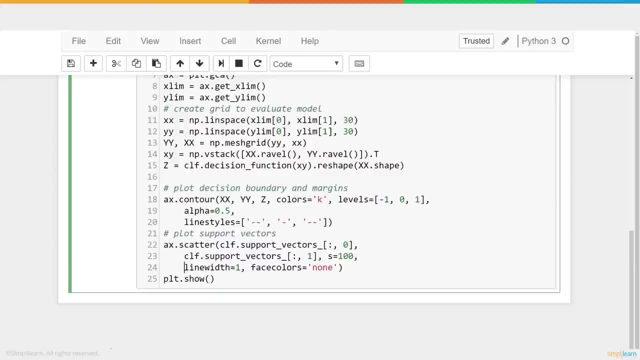 and the z value lets us know whether it is the left hand side. it's going to generate three different values. the z value does, and it'll tell us whether that data is a support vector to the left, the hyperplane in the middle or the support vector to the right. 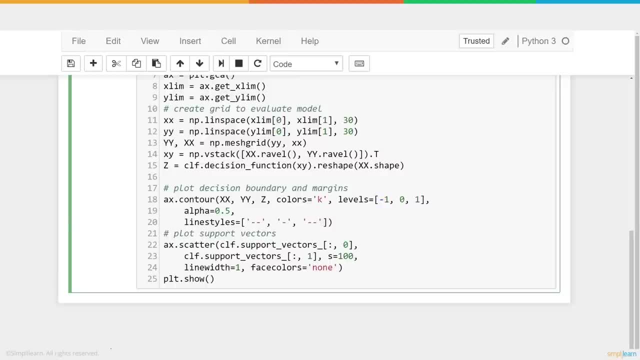 so it generates three different values for each of those points and those points have been reshaped so that they're right on a line. on those three different lines, we've labeled it to three different areas and we've reshaped it and we've just taken 30 points in each direction. 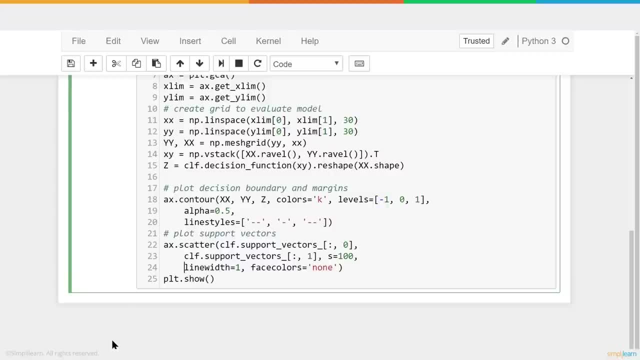 So we've set all of our data up, We've labeled it to three different areas and we reshaped it And we've just taken 30 points in each direction. If you do the math, you have 30 times 30. So that's 900 points of data. 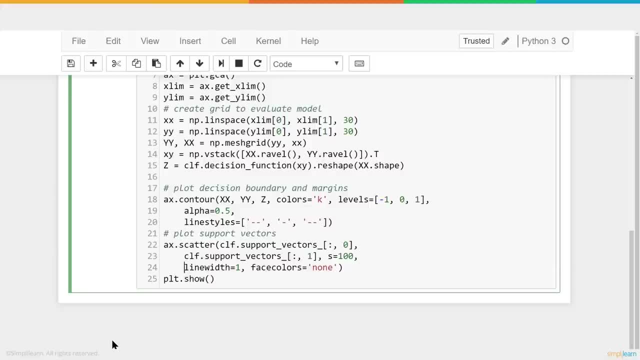 if you do the math, you have 30 times 30, so that's 900 points of data, and we've separated it between the three lines and reshaped it to fit those three lines. we can then go back to our matplot library, where we've created the ax. 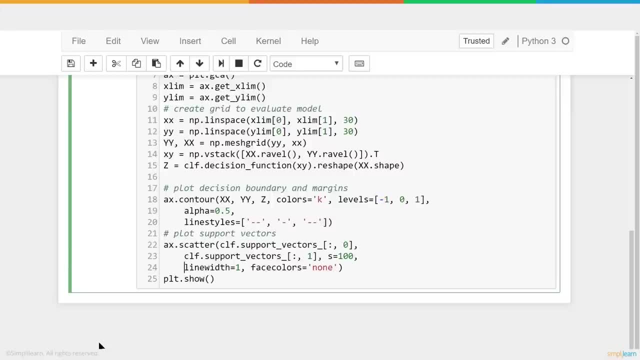 and we're going to create a contour and you'll see, here we have contour. capital xx, capital yy. these have been reshaped to fit those lines. z is the labels. so now we have the three different points with the labels. in there we set the colors: equals k. 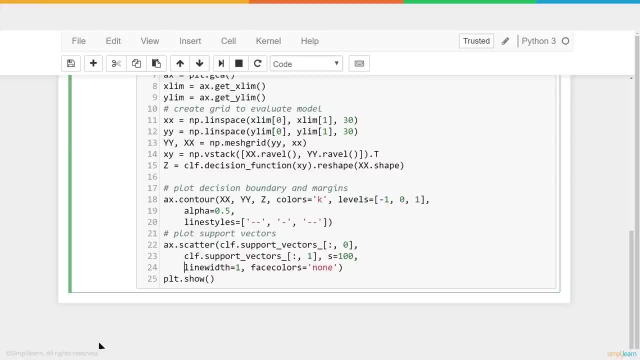 and I told you we had three different labels. but we have three levels of data. the alpha just makes it kind of see through, so it's only 0.5 of the value in there. so when we graph it, the data will show up from behind it. 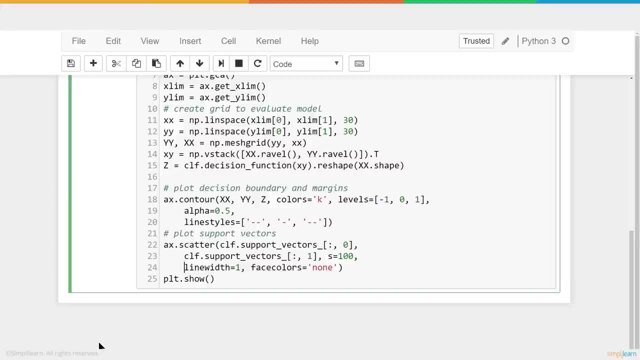 wherever the lines go, and finally the line styles. this is where we set the two support vectors to be dash, dash lines, and then a single one is just a straight line. that's what all that setup does, and then, finally, we take our axscatter and we go ahead and plot the support vectors. 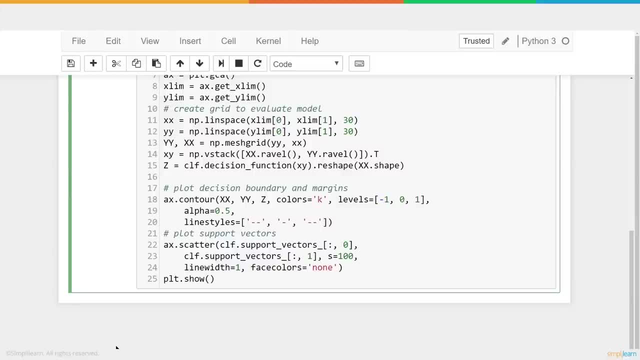 but we've programmed it in there so that they look nice like the dash dash line and the dash line on that grid. and you can see here when we do the clfsupportvectors, we are looking at column 0 and column 1 and then again we have the s equals 100. 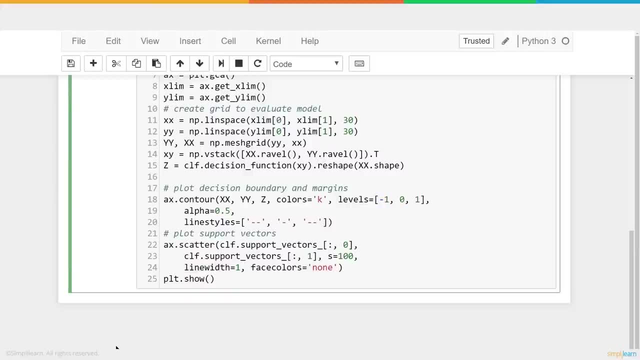 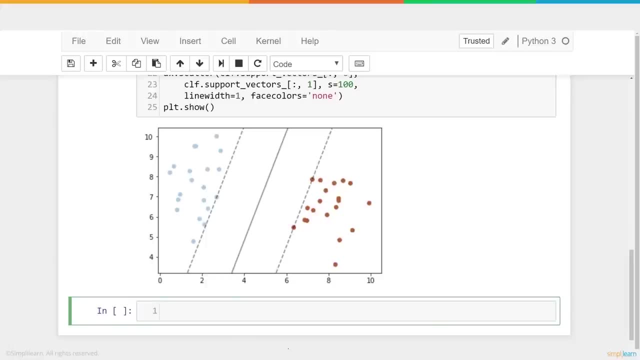 so we're going to make them larger and the line width equals 1. face colors equals none. let's take a look and see what that looks like when we show it and you can see when we get down to our end result. it creates a really nice graph. 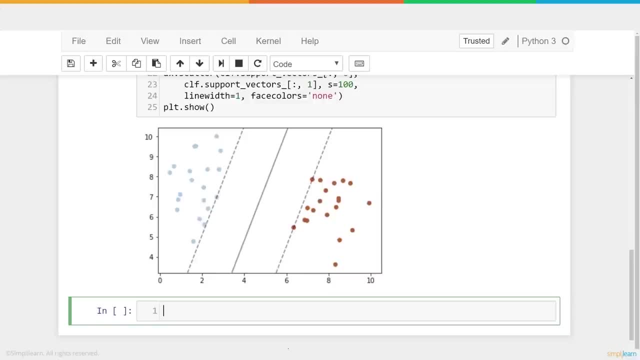 we have our two support vectors and dash lines, and they have the near data. so you can see those two points, or in this case the four points where those lines nicely cleave the data, and then you have your hyperplane down the middle which is as far from the two different points as possible. 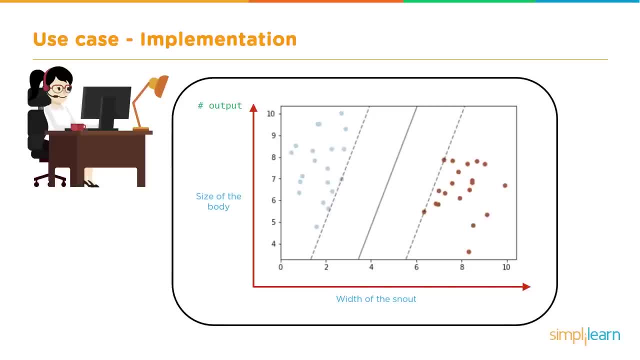 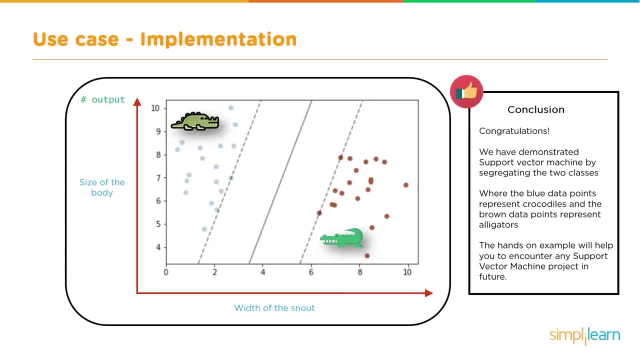 creating the maximum distance. so you can see that we have our nice output for the size of the body and the width of the snout, and we've easily separated the two groups of crocodile and alligator. congratulations, you've done it. we've made it for crocodiles and alligators. 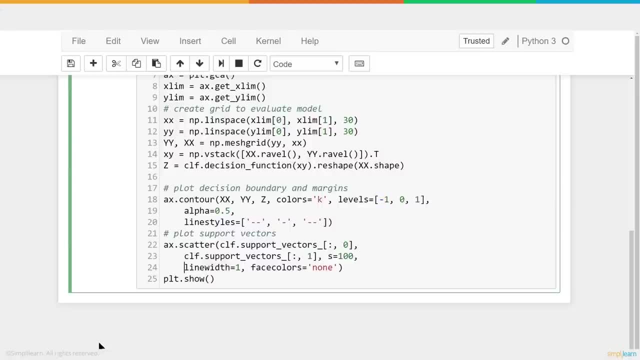 And we separate it between the three lines and reshaped it to fit those three lines. We can then go back to our map plot library. We've created the AX and we're going to create a contour, And you'll see, here we have contour, capital X, X, capital Y, Y. 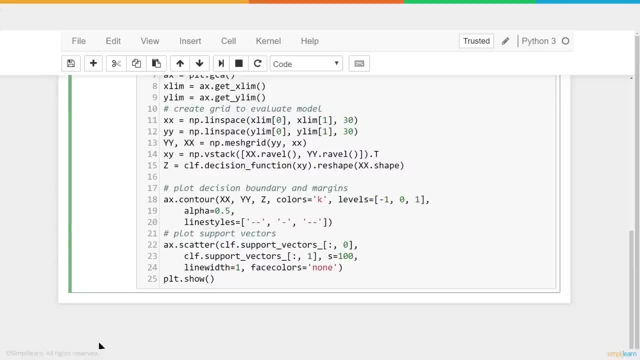 These have been reshaped to fit those lines. Z is the labels. So now we have the three different points with the labels in there and we can set the colors. equals K, and I told you we had three different labels, but we have three levels of data. 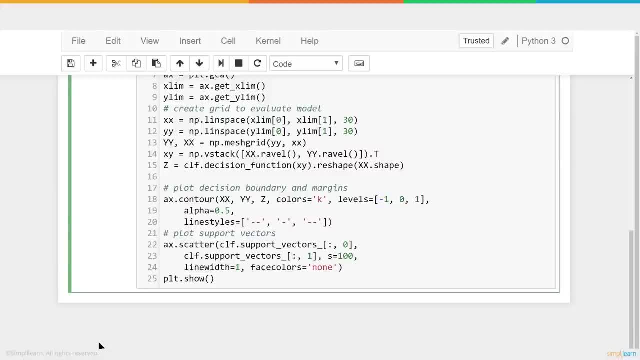 The alpha is just makes it kind of see through, so it's only point five of the value in there. So when we graph it, the data will show up from behind it wherever the lines go. And finally, the line styles. This is where we set the two support vectors to be dash, dash lines. 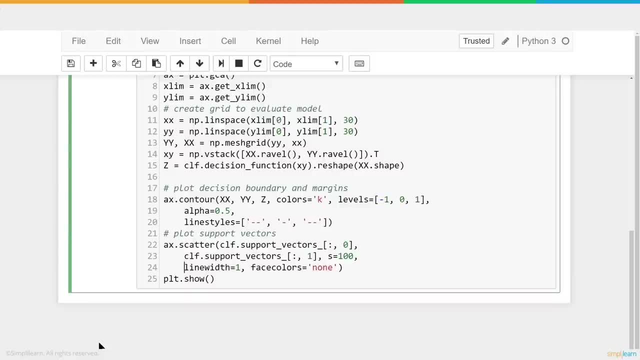 And then a single one is just a straight line. That's what all of that setup does. And then, finally, we take our AX dot scatter. We're going to go ahead and plot the support vectors, but we've programmed it in there so that they look nice like the dash, dash line and the dash line on that grid. 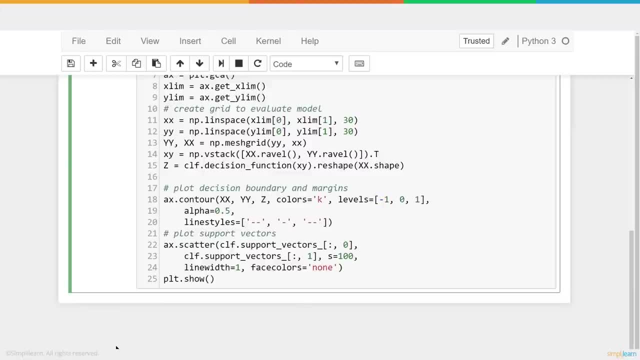 And you can see here when we do the CLF dot support vectors, we are looking at column zero and column one, And then again we have the S equals one hundred, So we're going to make them larger and the line width equals one. face colors equals. 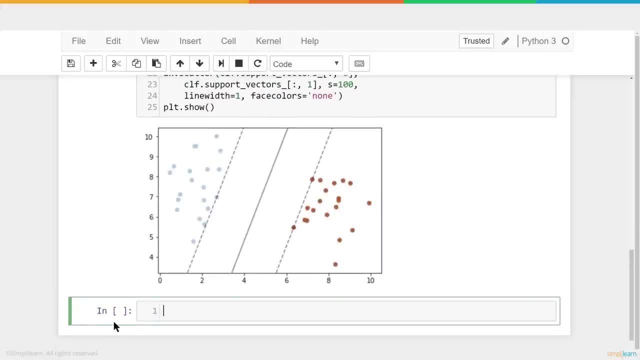 none. Let's take a look and see what that looks like when we show it And you can see we get down to our end result. It creates a really nice graph. We have our two support vectors and dash lines and they have the near data. 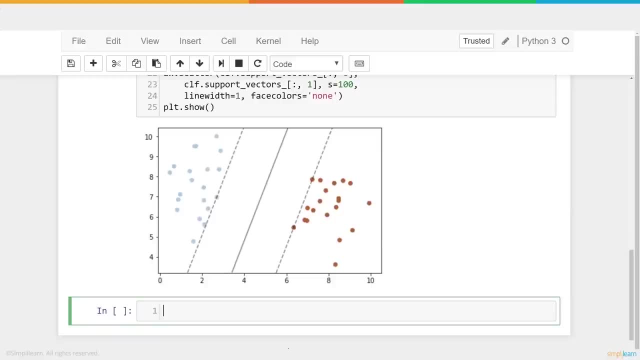 So you can see those two points, or in this case the four points where those lines are. you can nicely cleave the data and then you have your hyperplane down the middle, which is as far from the two different points as possible, creating the maximum distance. so you can see that we have our nice output. 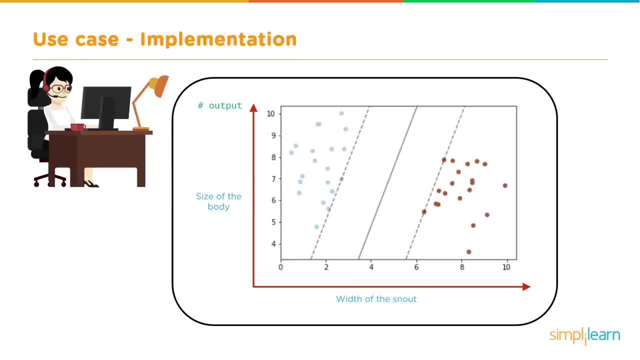 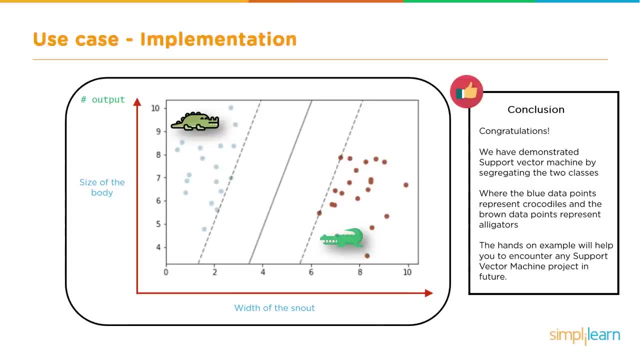 for the size of the body and the width of the snout, And we've easily separated the two groups of crocodile and alligator. Congratulations, you've done it, We've made it. Of course, these are pretend data for our crocodiles and alligators. 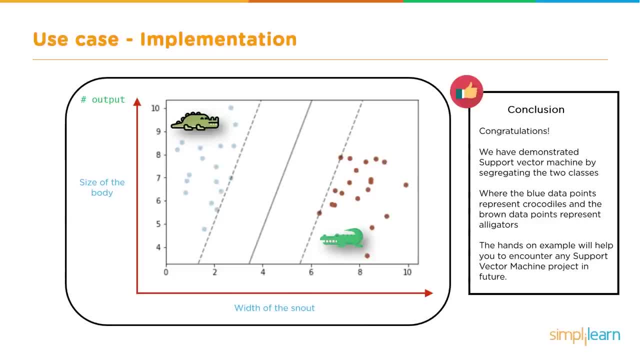 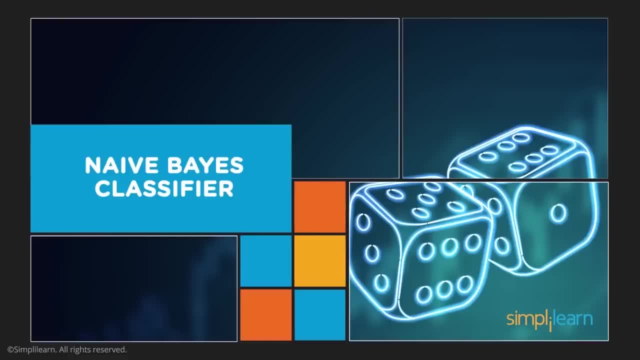 but this hands on example will help you to encounter any support vector machine projects in the future and you can see how easy they are to set up and look at in depth. Introducing Naive Bayes Classifier. Have you ever wondered how your mail provider implements spam filtering or how? 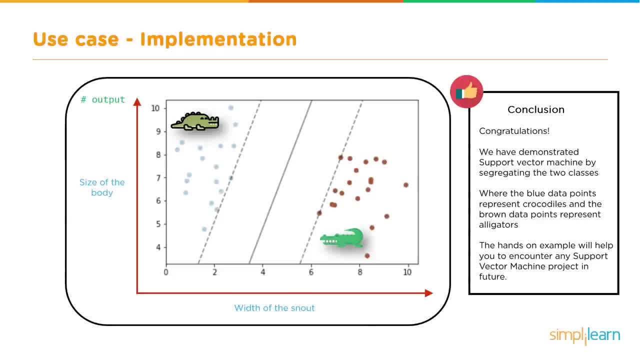 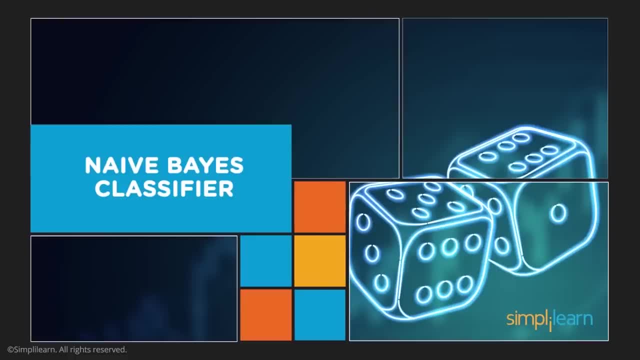 but this hands on example will help you to encounter any support vector machine projects in the future and you can see how easy they are to set up and look at in depth. introducing naive bayes classifier. have you ever wondered how your mail provider implements spam filtering or how online news channels? 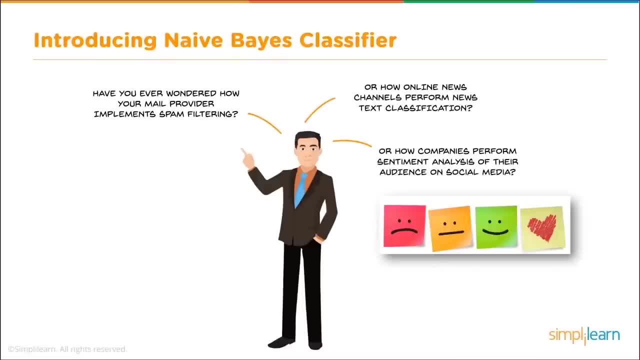 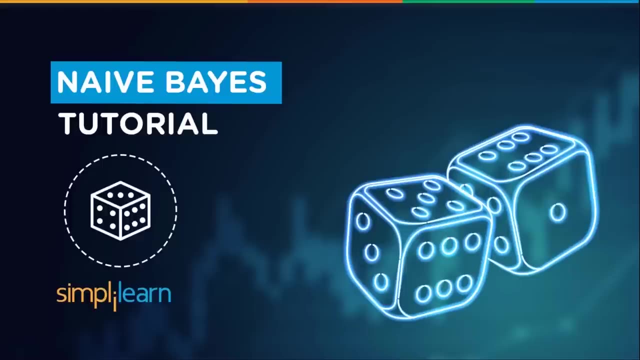 perform news text classification, or how companies perform sentimental analysis of their audience on social media. all of this and more is done through a machine learning algorithm called naive bayes classifier. welcome to naive bayes tutorial. my name is richard kirschner. i'm with the simplylearn team. 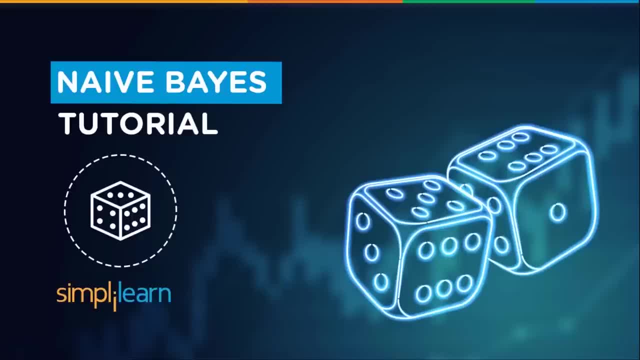 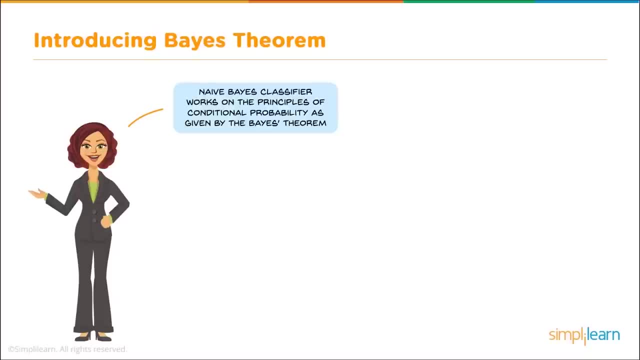 that's wwwsimplylearncom. get certified, get ahead. what is naive bayes? let's start with a basic introduction to the bayes theorem named after thomas bayes from the 1700s, who first coined this in the western literature. naive bayes classifier. 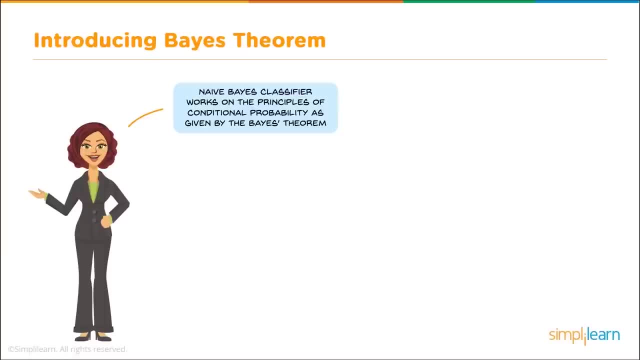 works on the principle of conditional probability as given by the bayes theorem. before we move ahead, let us go through some of the simple concepts of probability that we will be using. let us consider the following example of tossing two coins. here we have two quarters and if we look at all the different possibilities, 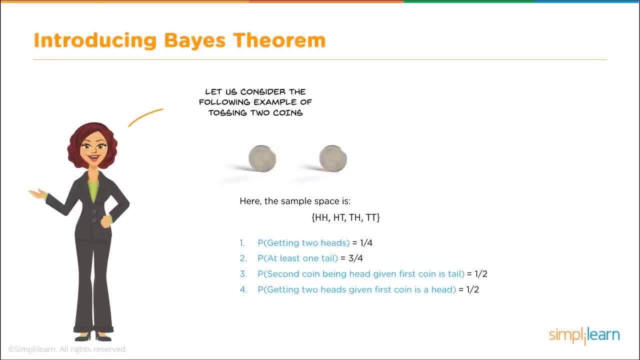 of what they can come up as we get that. they can come up as head heads. they can come up as head, tell, tell, head and tell, tell. when doing the math on probability, we usually denote probability as a p, a capital p. so the probability of getting two heads equals one. fourth: 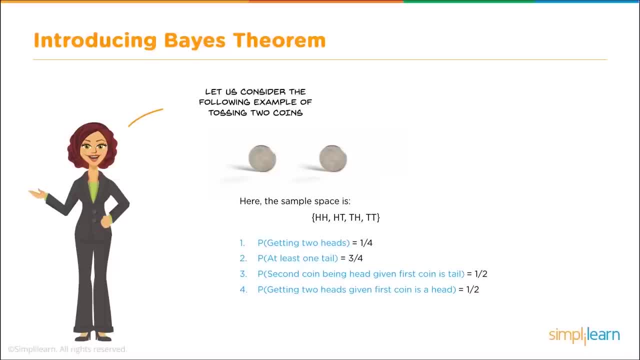 you can see on our data set we have two heads and this occurs once. out of the four possibilities, one tell occurs three quarters of the time. you'll see on three of the coin tosses we have tells in them and out of four that's three fourths. 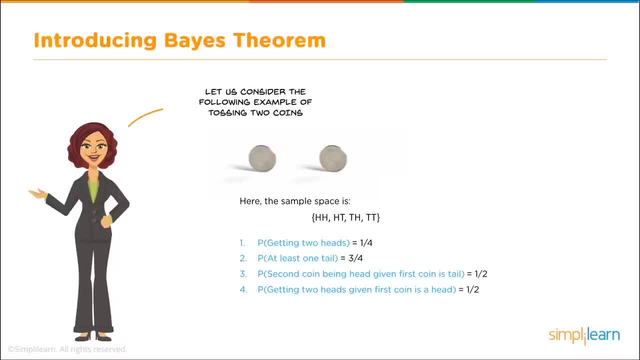 and then the probability of the second coin being head, given the first coin is tell is one half, and the probability of getting two heads, given the first coin is a head, is one half. we'll demonstrate that in just a minute and show you how that math works. 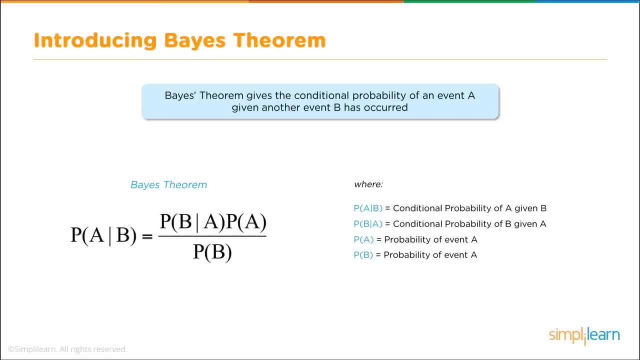 now, when we're doing it with two coins, it's easy to see, but when you have something more complex, you can see where these formulas really come in and work. the Bayes theorem gives us the conditional probability of an event A given. another event B has occurred. 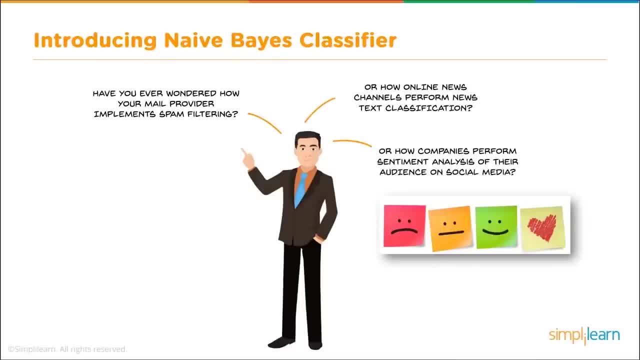 online news channels perform news text classification, or how companies perform sentimental analysis of their audience on social media. All of this and more is done through a machine learning algorithm called Naive Bayes Classifier. Welcome to Naive Bayes Tutorial. My name is Richard Kirshner. 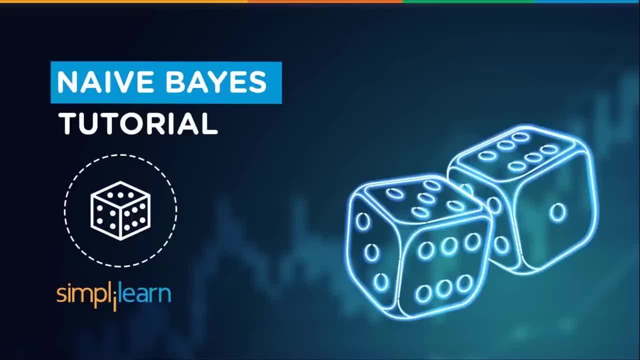 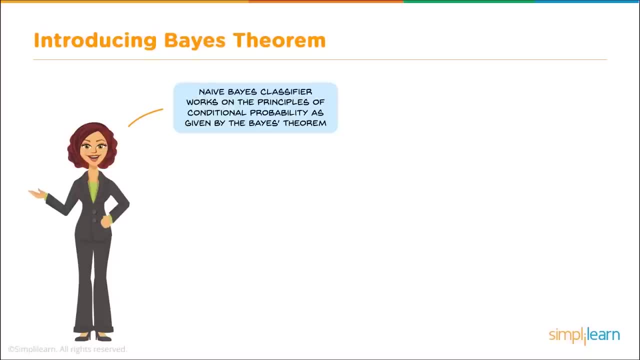 I'm with the Simply Learn team. That's wwwsimplylearncom. Get certified, Get ahead. What is Naive Bayes? Let's start with a basic introduction to the Bayes Theorem named after Thomas Bayes from the 1700s, who first coined this in the Western literature. 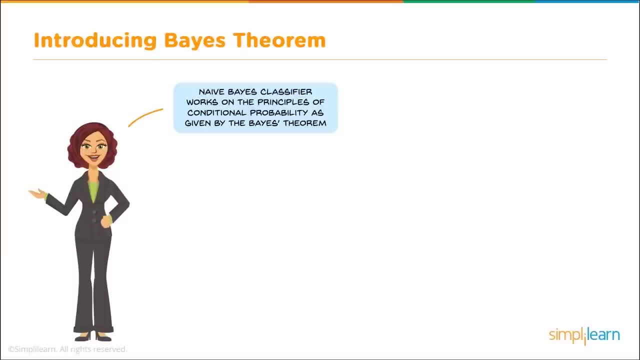 Naive Bayes Classifier works on the principle of conditional probability as given by the Bayes Theorem. Before we move ahead, let us go through some of the simple concepts and the probability that we will be using. Let us consider the following example of tossing two coins. 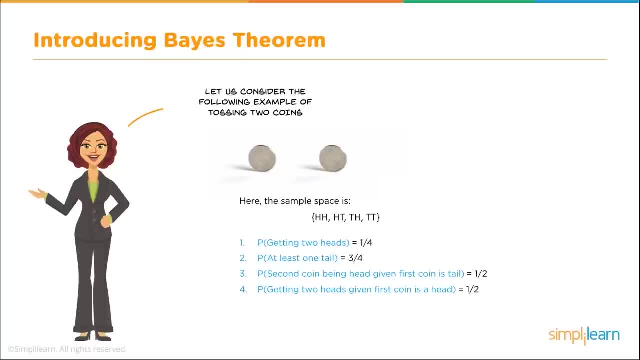 Here we have two quarters and if we look at all the different possibilities of what they can come up as we get that they could come up as head-heads, come up as head-tell, tell-head and tell-tell. When doing the math on probability, we usually denote probability as a P, a capital P. 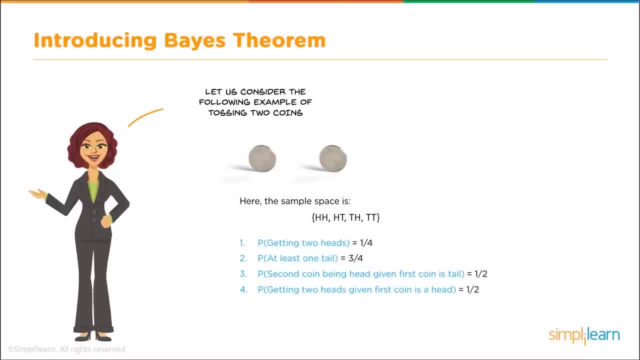 So the probability of getting two heads equals one fourth. You can see on our data set we have two heads and this occurs once out of the four possibilities. and then the probability of at least one tell occurs three quarters of the time. You'll see on three of the coin tosses we have tells in them and out of four. 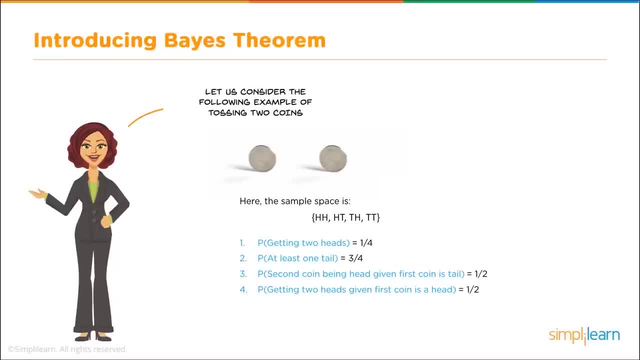 that's three fourths. and then the probability of the second coin being head, given the first coin is tell, is one half, and the probability of getting two heads, given the first coin is a head, is one half. We'll demonstrate that in just a minute and show you how that math works. 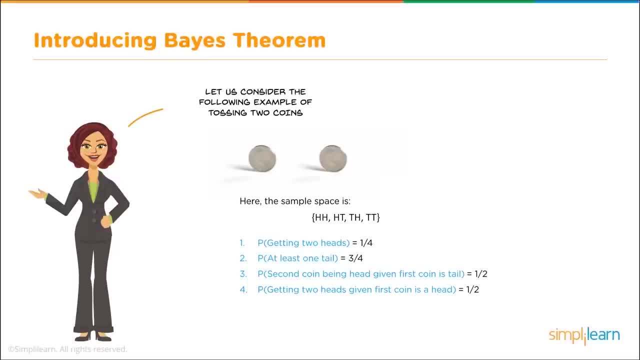 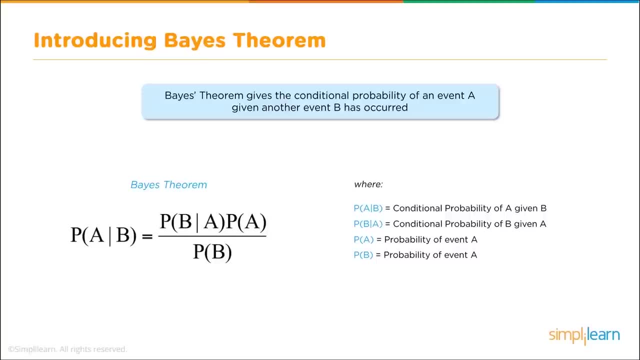 Now, when we're doing it with two coins, it's easy to see, but when you have something more complex, you can see where these these formulas really come in and work. So the Bayes Theorem gives us the conditional probability of an event A. 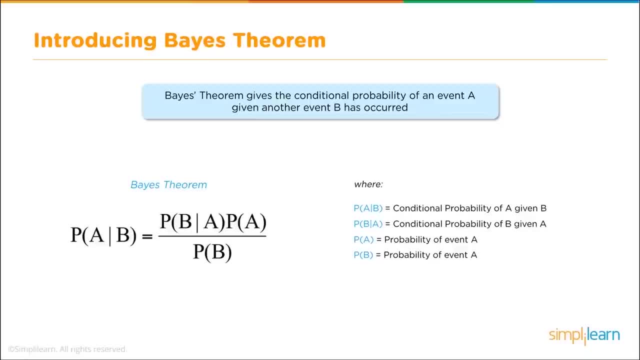 given another event, B has occurred. In this case, the first coin toss will be B and the second coin toss A. This could be confusing, because we've actually reversed the order of them and go from B to A instead of A to B. You'll see this a lot when you work in probabilities. 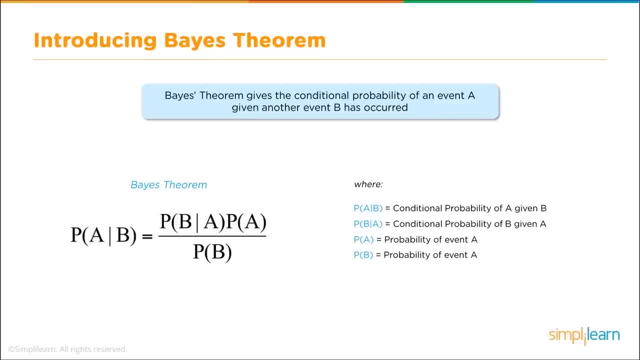 in this case, the first coin toss will be B and the second coin toss A. this can be confusing, because we've actually reversed the order of them and go from B to A instead of A to B. you'll see this a lot when you work in probabilities. 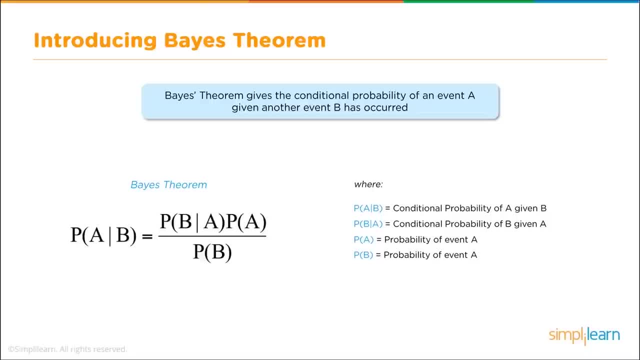 the reason is: we're looking for event A, we want to know what that is, so we're going to label that A, since that's our focus, and then, given another event B has occurred in the Bayes theorem. as you can see on the left, the probability of A occurring: 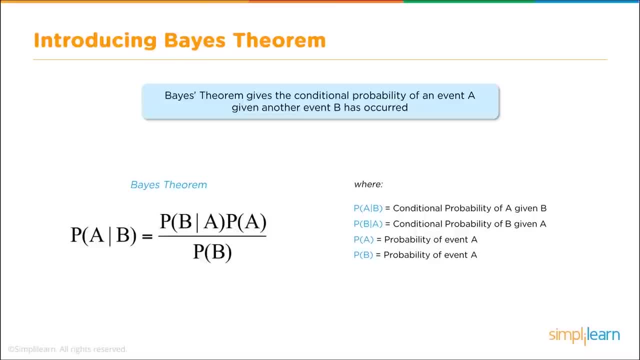 given B has occurred equals the probability of B occurring, given A has occurred, times the probability of A over the probability of B. this simple formula can be moved around just like any algebra formula and we could do the probability of A after a given B times the probability of B equals. 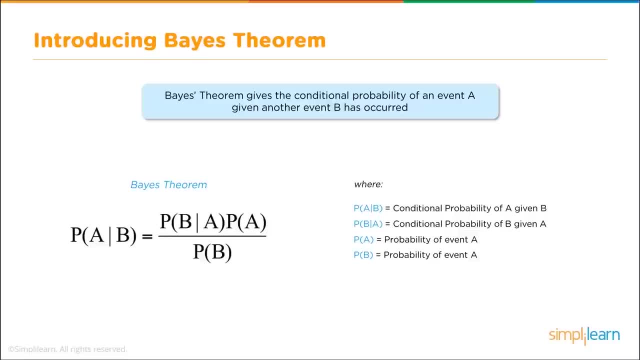 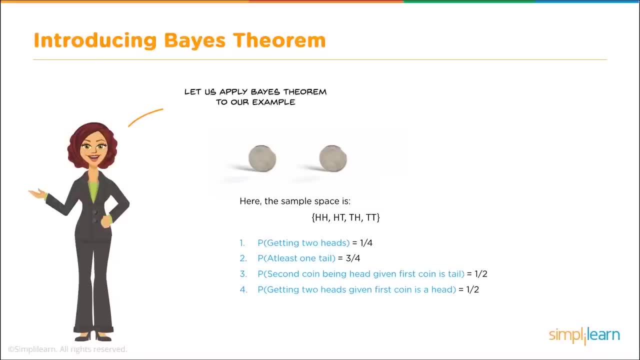 the probability of B given A times the probability of A. you can easily move that around and multiply it and divide it out. let us apply Bayes theorem to our example. here we have our two quarters. now we'll notice that the first two probabilities of getting two heads 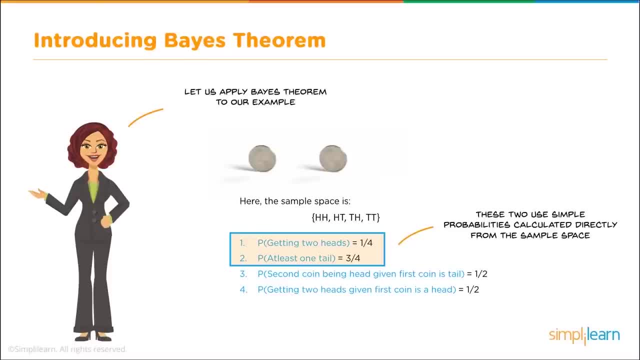 and at least one tail. we compute directly off the data, so you can easily see that we have one example HH out of four, one fourth and we have three with tails in them, giving us three quarters. the second condition, the second set: three and four. we're going to explore a little bit more in detail. 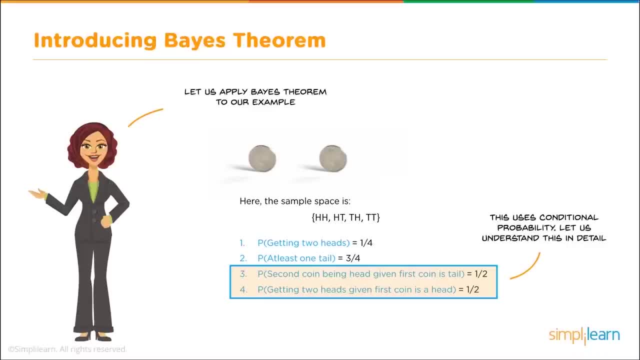 now we stick to a simple example with two coins, because you can easily understand the math. so let's say we have two heads and one tail, doesn't matter what comes before it, and the same with the head. so it's still going to be 50% or one half. 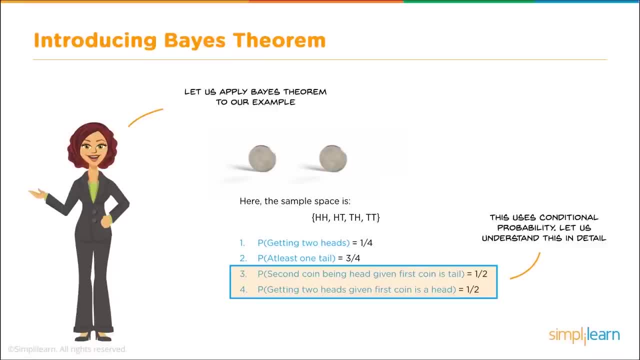 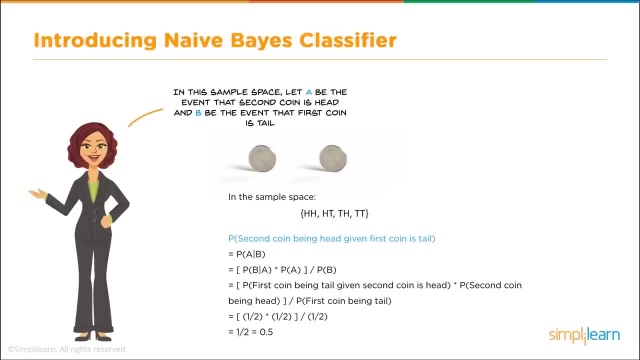 but when that probability gets more complicated- let's say you have a D6 dice or some other instance- then this formula really comes in handy. but let's stick to the simple example for now. in this sample space, let A be the event that the second coin is head. 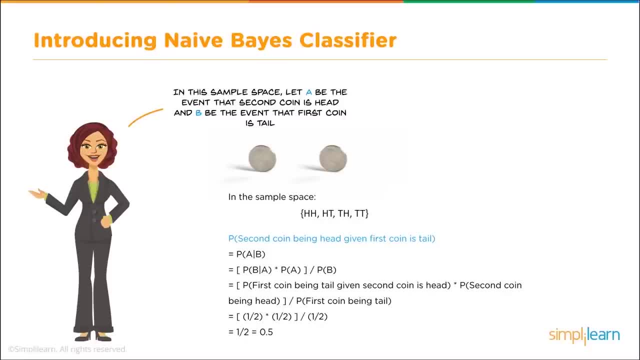 and B be the event that the first coin is tails. again, we reversed it because we want to know what the second event is going to be. so we're going to be focusing on A, and we know this from our formula that that equals the probability of B, given A. 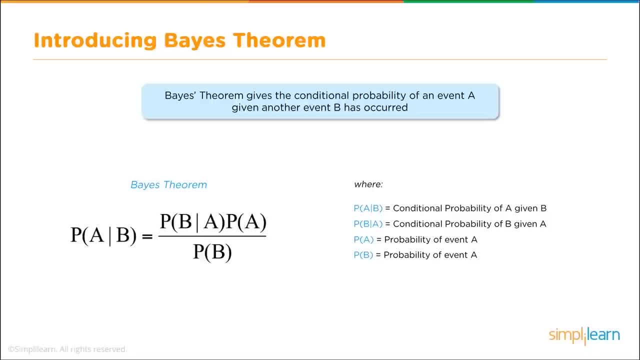 The reason is: we're looking for event A, We want to know what that is, So we're going to label that A, since that's our focus, And then, given another, event B has occurred In the Bayes Theorem, as you can see on the left. 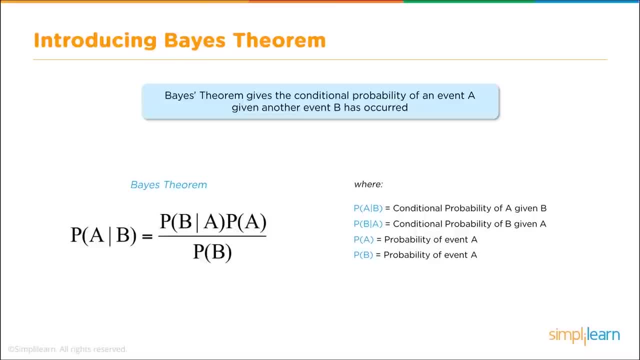 the probability of A occurring given B has occurred equals the probability of B given A has occurred times the probability of A over the probability of B. This simple formula can be moved around just like any algebra formula And we could do the probability of A after a given B times probability. 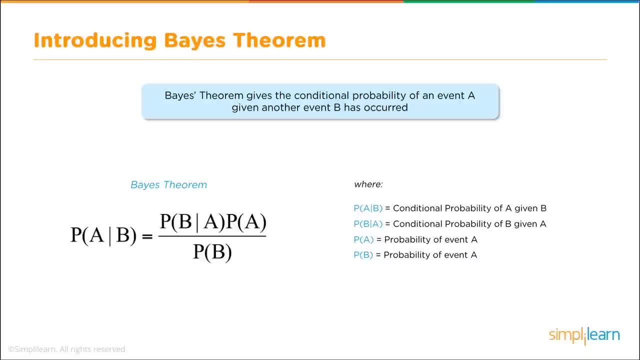 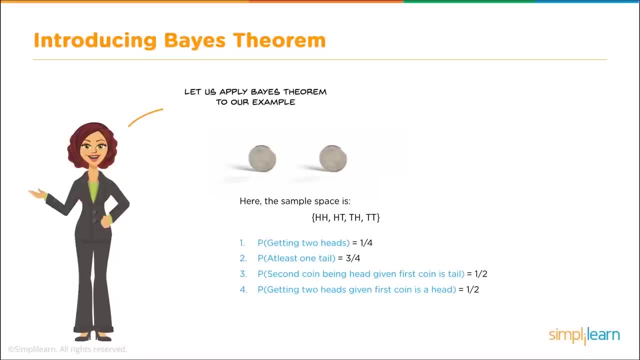 of B equals the probability of B given A times probability of A. You can easily move that around and multiply it and divide it out. Let us apply Bayes Theorem to our example. Here we have our two quarters and we'll notice that the first two probabilities of getting two heads and at least one tail 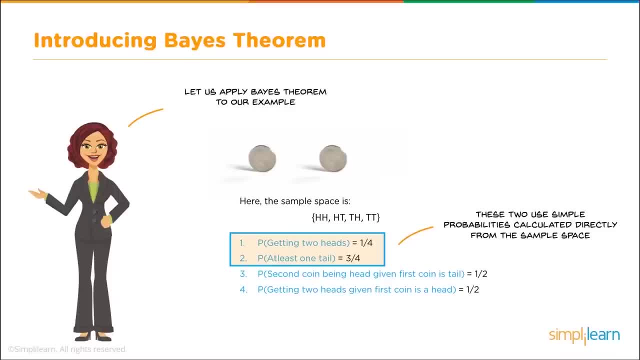 directly off the data. So you can easily see that we have one example HH out of four, one fourth And we have three with tails in them, giving us three quarters or three fourths, 75 percent. The second condition, the second set, three and four. 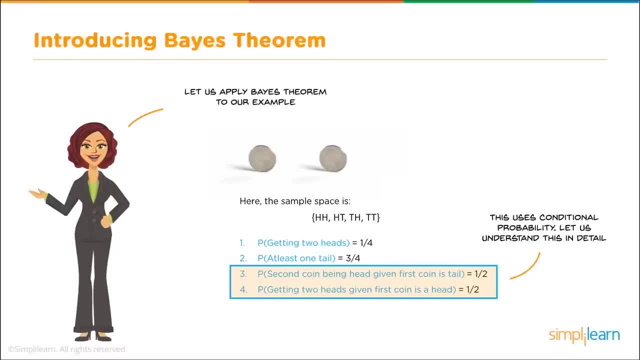 we're going to explore a little bit more in detail Now. we stick to a simple example with two coins, because you can easily understand the math. The probability of throwing a tail doesn't matter what comes before it, And the same with the heads. 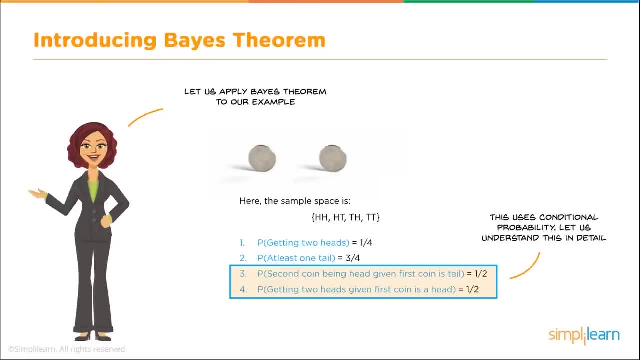 So still going to be 50 percent or one half. But when that comes, when that probability gets more complicated- let's say you have a D6 dice or some other instance- then this formula really comes in handy. But let's stick to the simple example for now. 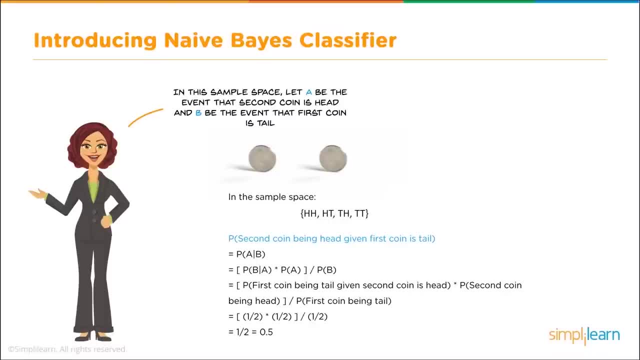 In this sample space. let A be the event that the second coin is head and B be the event that the first coin is tails. Again, we reversed it because we want to know what the second event is going to be, So we're going to be focusing on A. 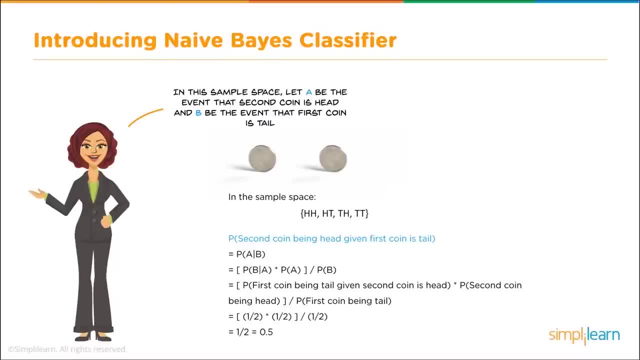 And we write that out as the probability of A given B And we know this from our formula, that that equals the probability of B given A times the probability of A over the probability of B. And when we plug that in we plug in the probability of the first coin being. 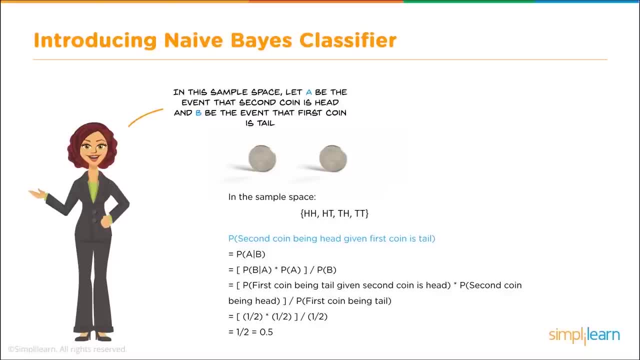 tails, given the second coin is heads, and the probability of the second coin being heads, given the first coin being over the probability of the first coin being tails. When we plug that data in and we have the probability of the first coin being tails, given the second coin is heads, times the probability of the second coin being heads. 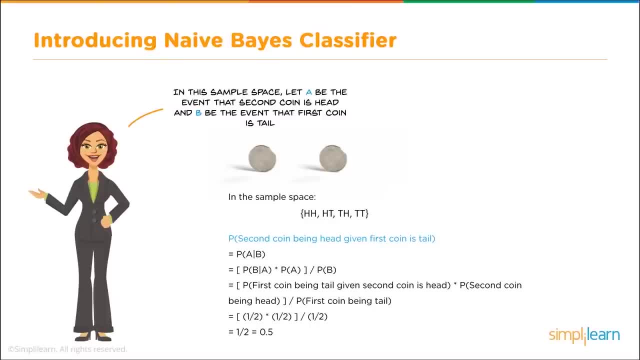 times the probability of A over the probability of B, and when we plug that in, we plug in the probability of the first coin being tails, given the second coin is heads, and the probability of the second coin being heads, given the first coin being over the probability of the first coin being tails. 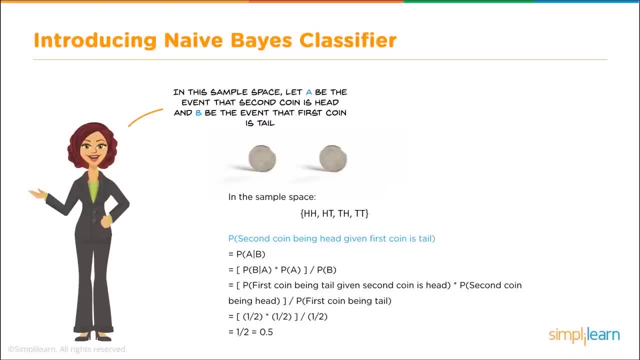 when we plug that data in and we have the probability of the first coin being tails, given the second coin is heads times the probability of the second coin being heads over the probability of the first coin being tails. you can see it's a simple formula to calculate. 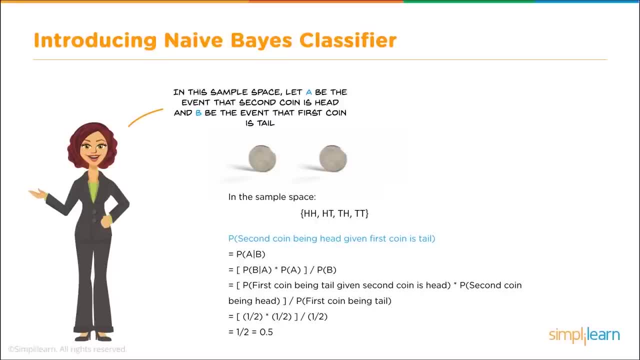 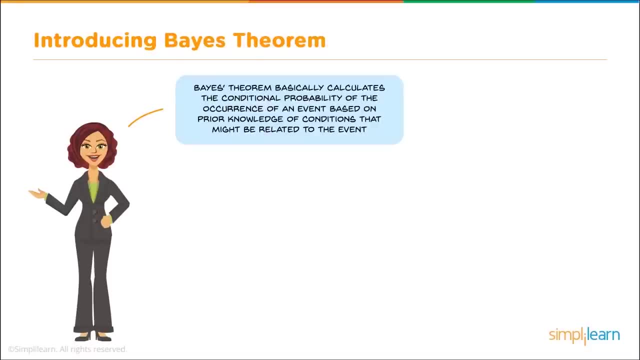 we have one half times one half over one half, or one half equals point five or one fourth. so the Bayes theorem basically calculates the conditional probability of the occurrence of an event based on prior knowledge of conditions that might be related to the event. we will explore this in detail. 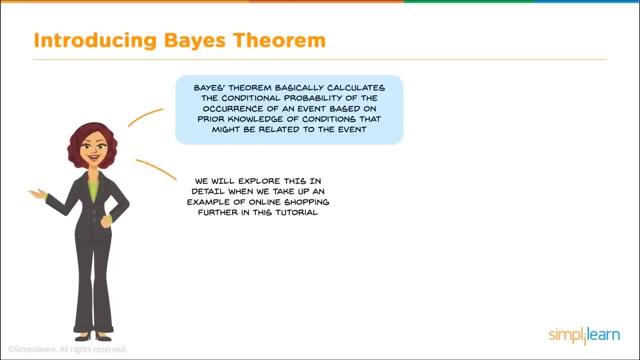 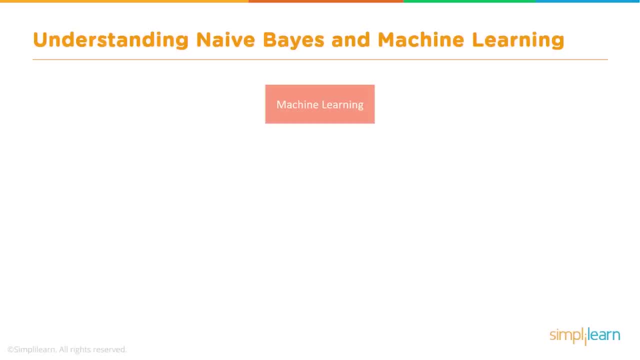 when we take up an example of online shopping. further in this tutorial, understanding naive Bayes and machine learning, like with any of our other machine learning tools, it's important to understand where the naive Bayes fits in the hierarchy. so under the machine learning, we have supervised learning. 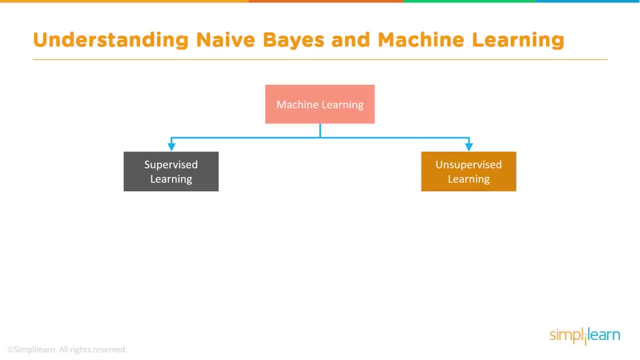 and there is other things like unsupervised learning. there's also reward system. this falls under the supervised learning. and then under the supervised learning, there's classification, there's also regression, but we're going to be in the classification side and then under classification. is your naive Bayes? 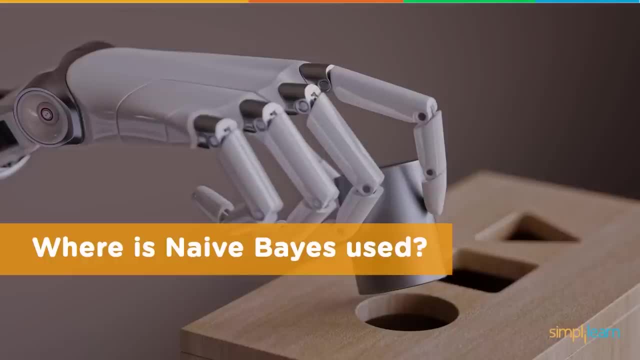 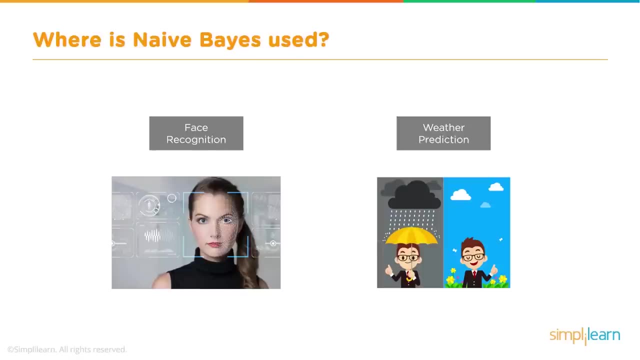 let's go ahead and glance into where is naive Bayes used. let's look at some of the used scenarios for it as a classifier. we use it in face recognition- is this Cindy, or is it not Cindy, or whoever? or it might be used to identify parts of the face. 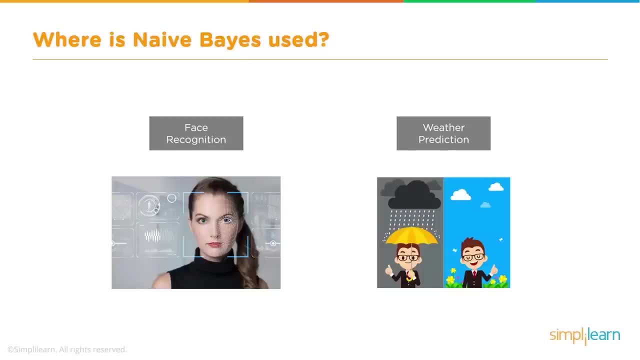 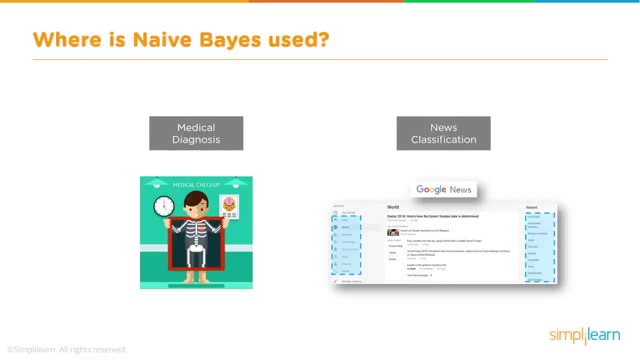 that they then feed into another part of the face recognition program. this is the eye, this is the nose, this is the mouth. weather prediction: is it going to be rainy or sunny? medical recognition news prediction. it's also used in medical diagnosis. we might diagnose somebody as either as high risk 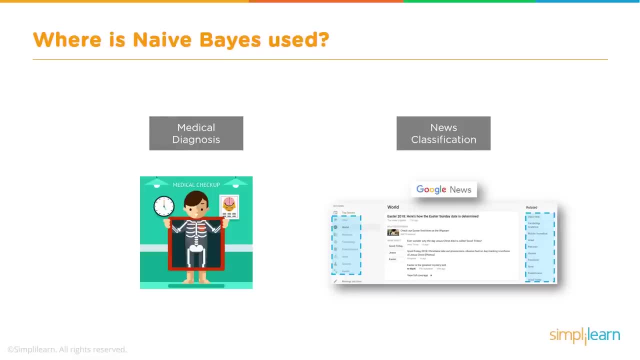 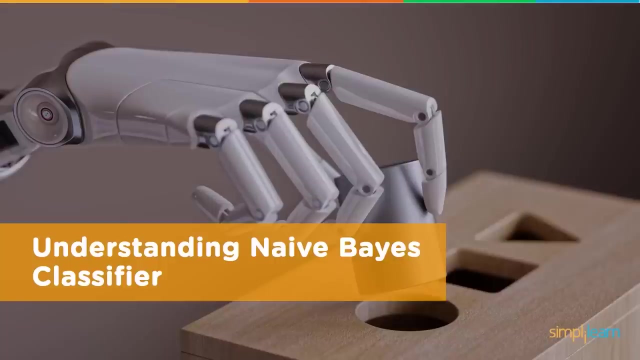 or not as high risk for cancer or heart disease or other ailments. and news classification: is this medical or is this world news or a lot of that's all done with the naive Bayes understanding, naive Bayes classifier. now we already went through a basic understanding with the coins. 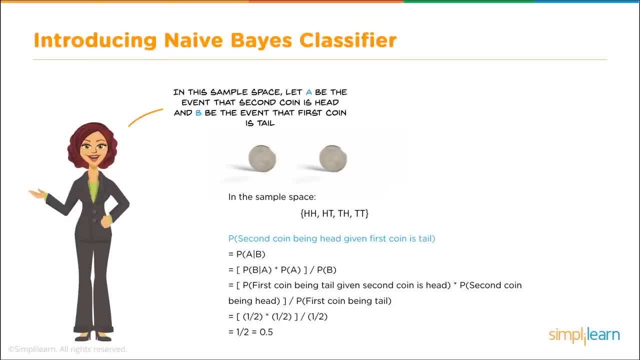 over the probability of the first coin being tails. You can see it's a simple formula to calculate. We have one half times one, half over one half, or one-half equals .5 or one-fourth. So the Bayes Theorem basically calculates the conditional probability of the occurrence of an event. 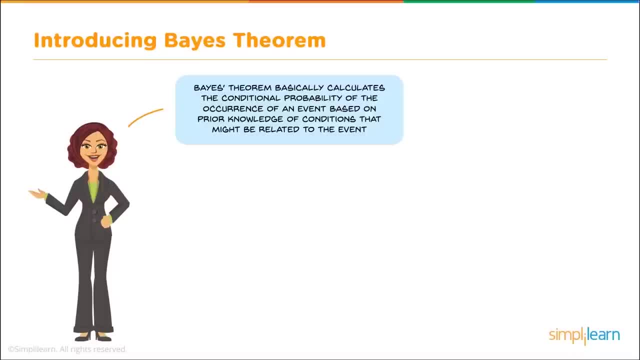 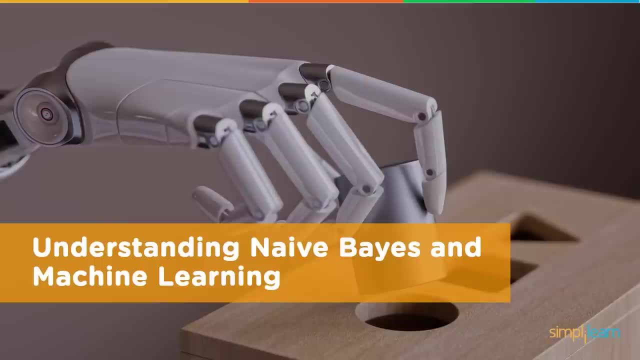 based on prior knowledge of conditions that might be related to the event. We will explore this in detail when we take up an example of online shopping further in this tutorial, Understanding naive Bayes and machine learning, Like with any of our other machine learning tools. 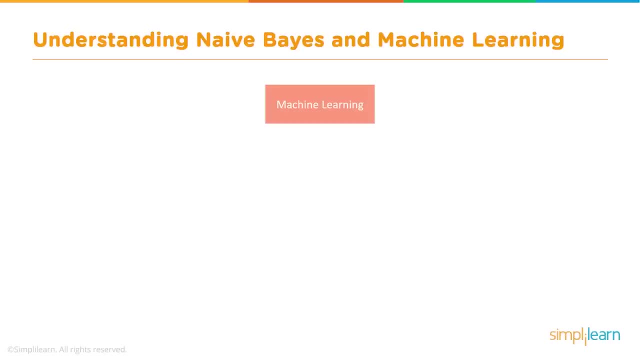 it's important to understand where the naive Bayes fits in the hierarchy. So under the machine learning we have supervised learning and there is other things like unsupervised learning. There's also reward system. This falls under the supervised learning And then under the supervised learning. 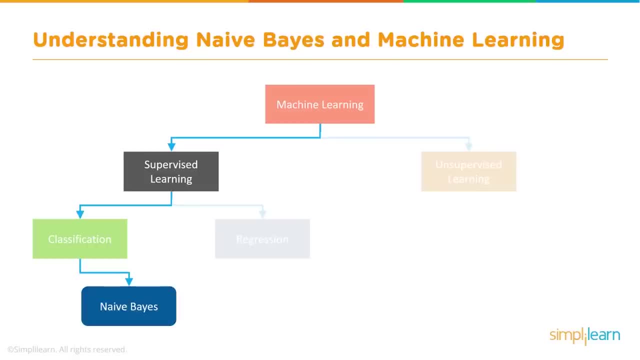 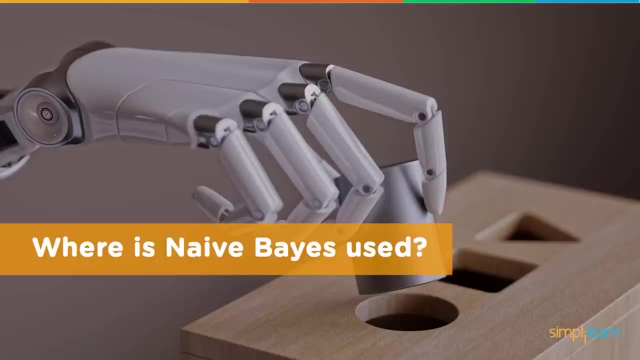 there's classification, there's also regression, but we're gonna be in the classification side. And then under classification is your naive Bayes. Let's go ahead and glance into where is naive Bayes used. Let's look at some of the use scenarios for it. 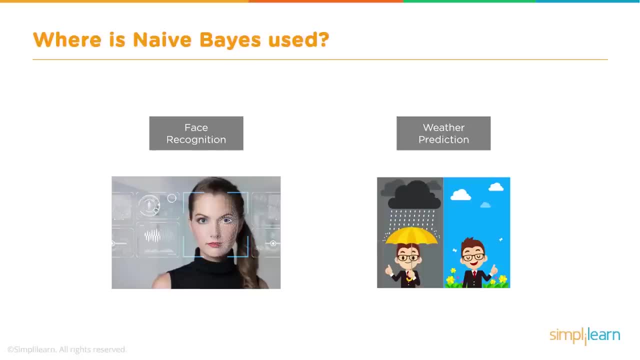 As a classifier. we use it in face recognition- Is this Cindy, or is it not Cindy, or whoever? Or it might be used to identify parts of the face that they then feed into another part of the face recognition program. This is the eye, this is the nose, this is the mouth. 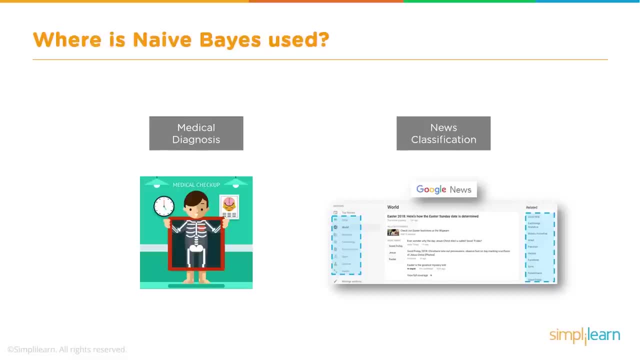 Weather prediction: is it gonna be rainy or sunny? Medical recognition news prediction. It's also used in medical diagnosis. We might diagnose somebody as either as high risk or not as high risk for cancer or heart disease or other ailments, And news classification. 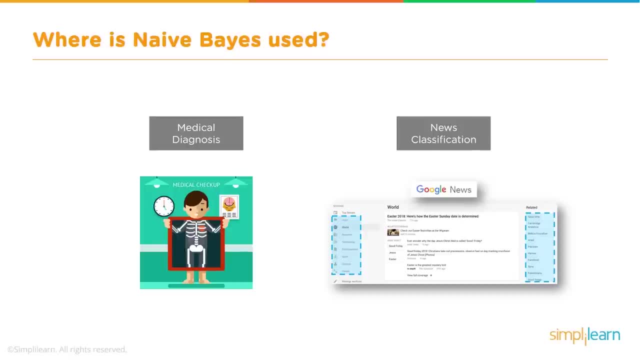 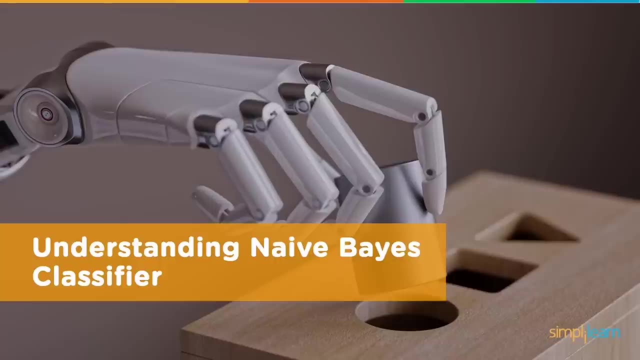 When you look at the Google News and it says: well, is this political or is this world news? Or a lot of that's all done with the naive Bayes Understanding naive Bayes classifier. Now, we already went through a basic understanding. 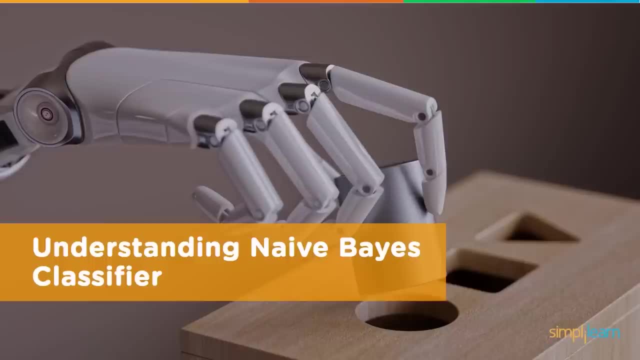 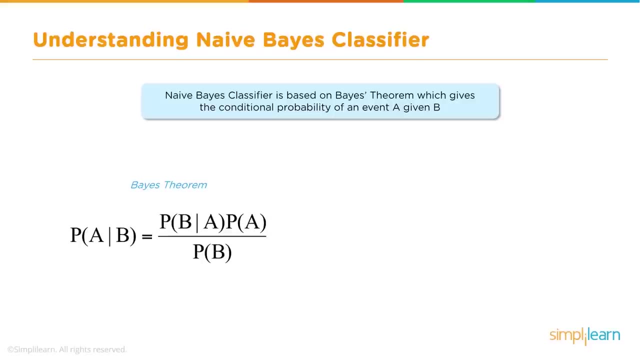 with the coins and the two heads and two tells, and head tell, tell, heads, et cetera. We're gonna do just a quick review on that and remind you that the naive Bayes classifier is based on the Bayes theorem, which gives a conditional probability of event A. 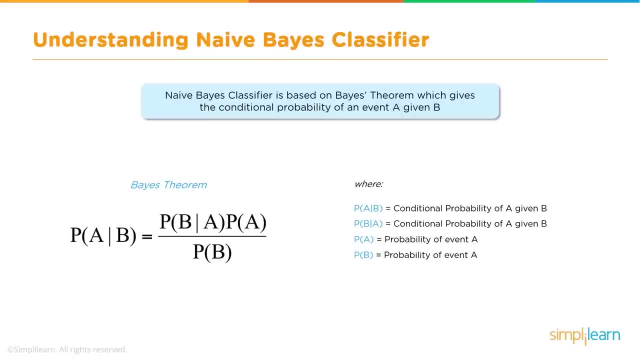 given event B, And that's where the probability of A given B equals the probability of B given A times probability of A over probability of B. Remember, this is an algebraic function so we can move these different entities around. We can multiply by the probability of B. 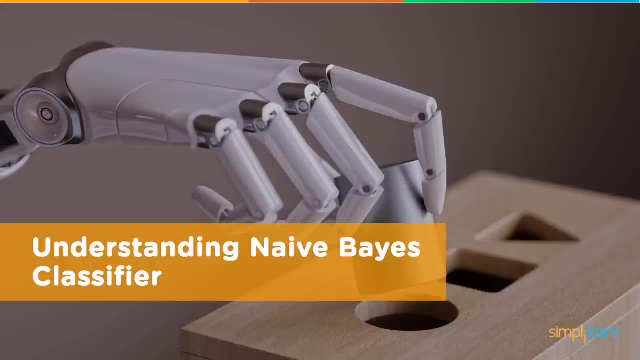 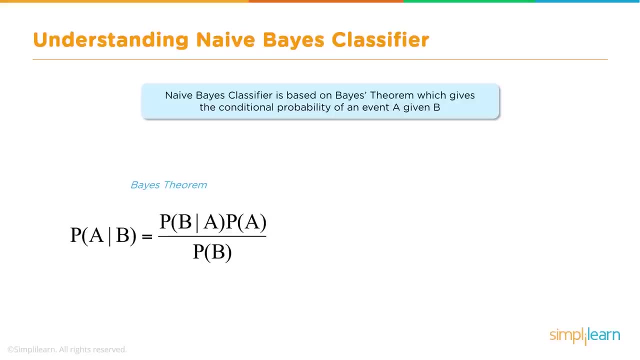 and the two heads and two tells and head tell tell heads, etc. we're going to do just a quick review on that and remind you that the naive Bayes classifier is based on the Bayes theorem, which gives a conditional probability of event A given event B. 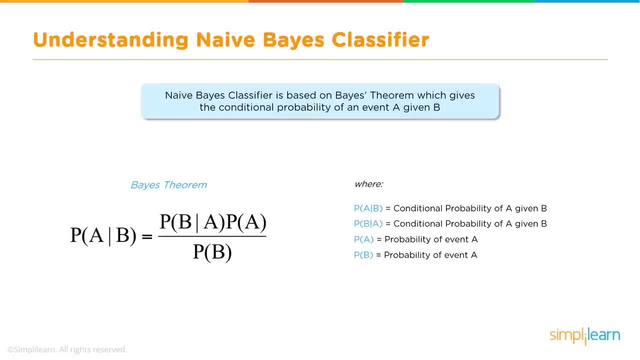 and that's where the probability of A given B equals the probability of B given A times probability of A over probability of B. remember, this is an algebraic function so we can move these different entities around. we can multiply by the probability of B, so it goes to the left hand. 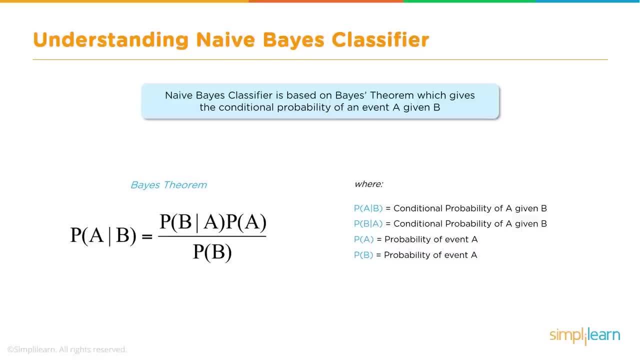 side, and then we can divide by the probability of A given B and just as easily come up with a new formula for the probability of B. to me, staring at these algebraic functions kind of gives me a slight headache. it's a lot better to see if we can actually understand. 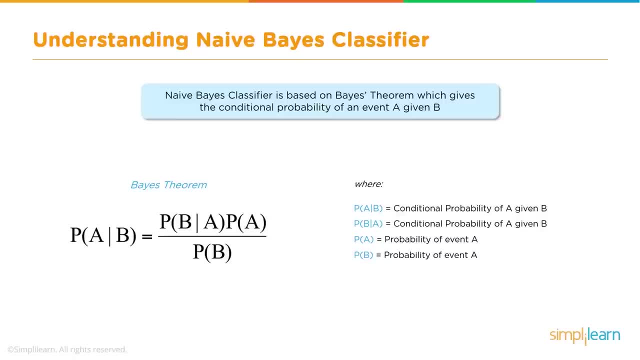 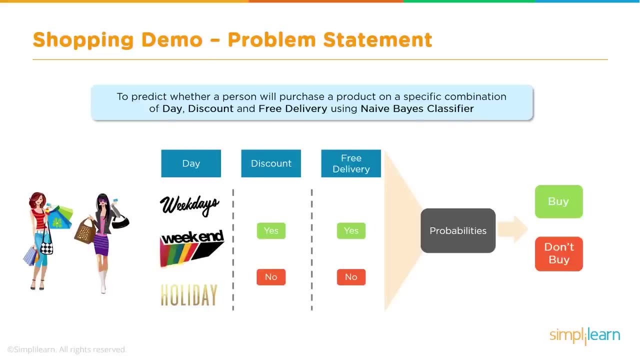 how this data fits together in a table and let's go ahead and start applying it to some actual data so you can see what that looks like. so we're going to start with the shopping demo problem statement and remember we're going to solve this first in table form. 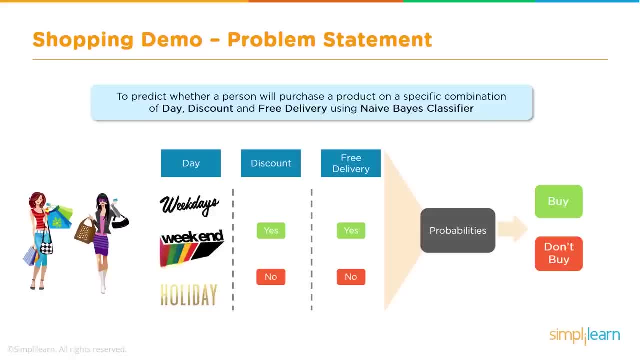 so you can see what the math looks like, and then we're going to solve it in Python and in here we want to predict whether the person will purchase a product. are they going to buy or don't buy? very important: if you're running a business, you want to know how to maximize your 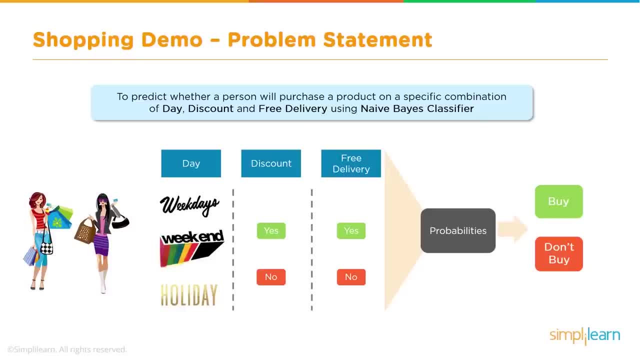 profits or at least maximize the purchase of the people coming into your store, and we're going to look at a specific combination of different variables. in this case we're going to look at the day discount and the free delivery and you can see here under the day. we want to know whether it's 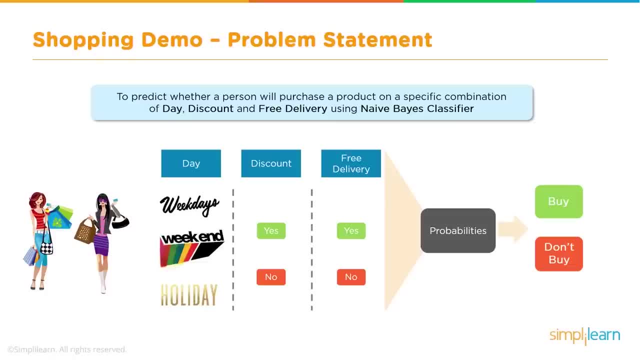 on the weekday. you know somebody's working. they come in after work or maybe they don't work weekend. you can see the bright colors coming down there celebrating not being in work or holiday. and did we offer a discount that day, yes or no? did we offer free delivery that day, yes or no? 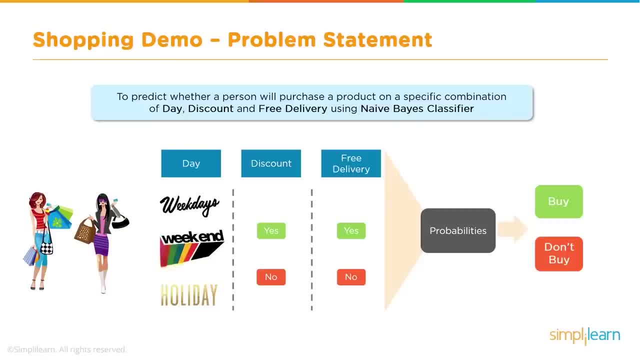 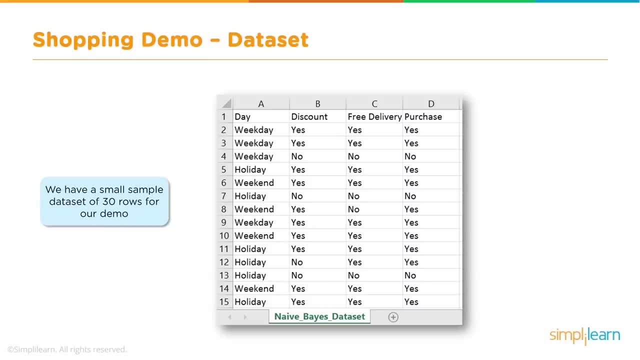 and from this we want to know whether the person's going to buy based on these traits, so we can maximize them and find out the best system for getting somebody to come in and purchase our goods and products from our store. now, having a nice visuals, great, but we do need to dig into the data. 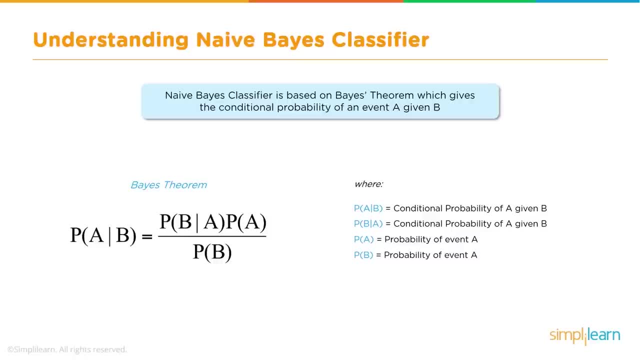 so it goes to the left-hand side. And then we could divide by the probability of A given B and just as easily come up with a new formula for the probability of B. To me, staring at these algebraic functions kind of gives me a slight headache. 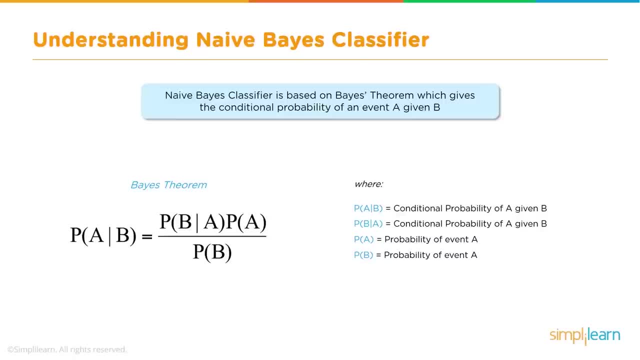 It's a lot better to see if we can actually understand how this data fits together in a table, And let's go ahead and start applying it to some actual data so you can see what that looks like. So we're gonna start with the shopping demo. 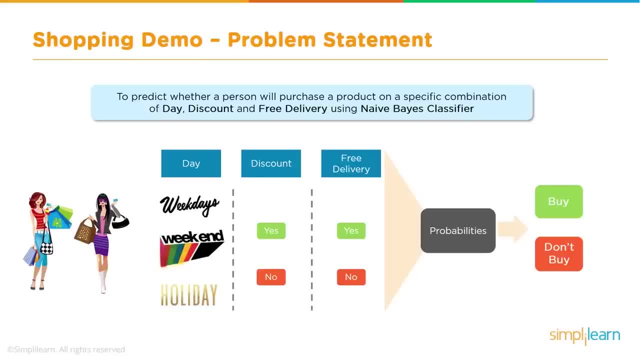 We're gonna look at the problem statement And remember we're gonna solve this first in table form so you can see what the math looks like, And then we're gonna solve it in Python, And in here we wanna predict whether the person 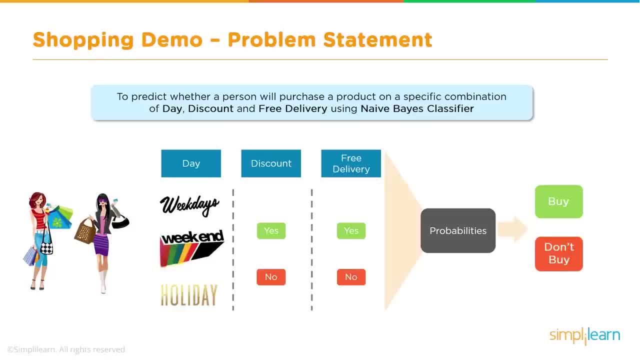 will purchase a product. Are they gonna buy or don't buy? Very important: if you're running a business, you wanna know how to maximize your profits or at least maximize the purchase of the people coming into your store, And we're gonna look at a specific combination. 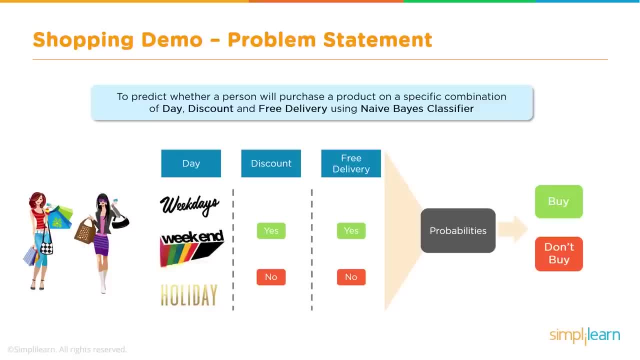 of different variables. In this case we're gonna look at the day, the discount and the free delivery And you can see here under the day. we wanna know whether it's on the weekday. you know somebody's working. they come in after work or maybe they don't work. 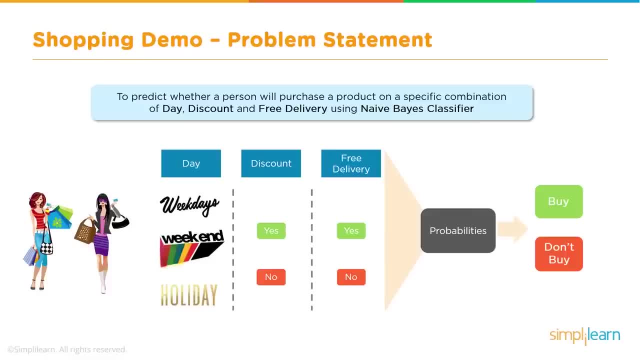 Weekend you can see the bright colors coming down there celebrating not being in work or holiday. And did we offer a discount that day, yes or no? Did we offer free delivery that day, yes or no? And from this we wanna know whether the person's 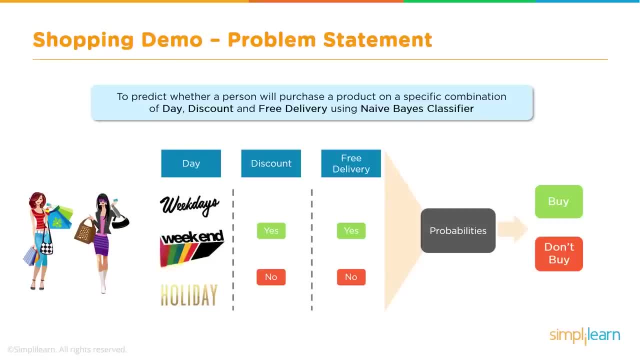 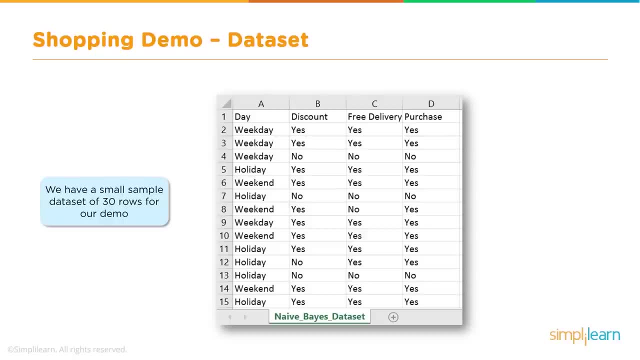 gonna buy based on these traits, so we can maximize them and find out the best system for getting somebody to come in and purchase our goods and products from our store. Now, having a nice visual's great, but we do need to dig into the data. 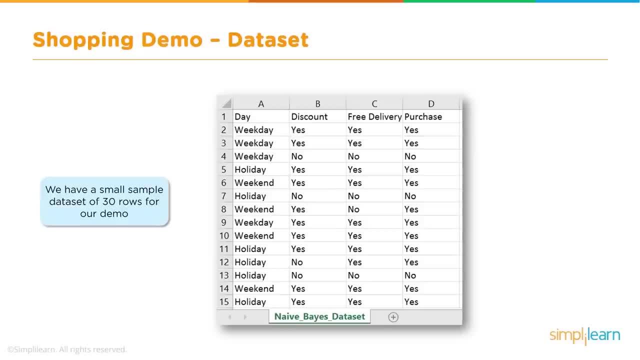 So let's go ahead and take a look at the data set. We have a small sample data set of 30 rows. We're showing you the first 15 of those rows for this demo. Now the actual data file you can request. 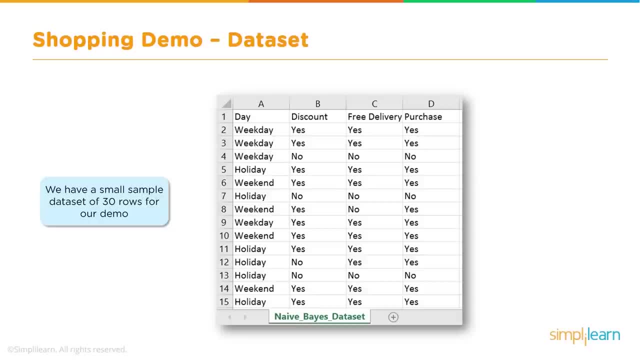 Just type in below under the comments on the YouTube video, and we'll send you some more information and send you that file. As you can see here, the file is very simple: columns and rows. We have the day, the discount, the free delivery. 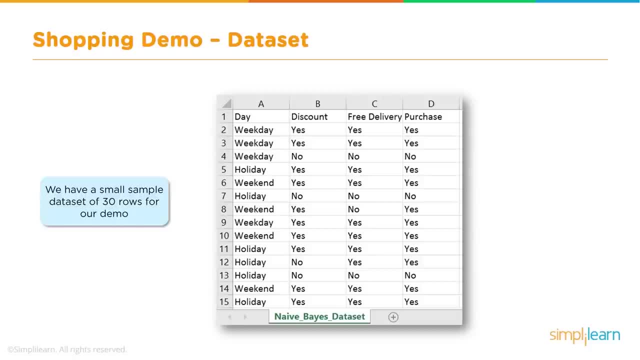 and did the person purchase or not? And then we have under the day whether it was a weekday, a holiday. was it the weekend? This is a pretty simple set of data and long before computers, people used to look at this data. 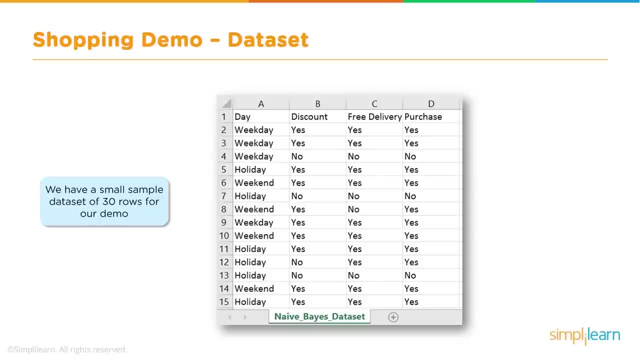 and calculate this all by hand. So let's go ahead and walk through this and see what that looks like when we put that into tables. Also note: in today's world we're not usually looking at three different variables and 30 rows. 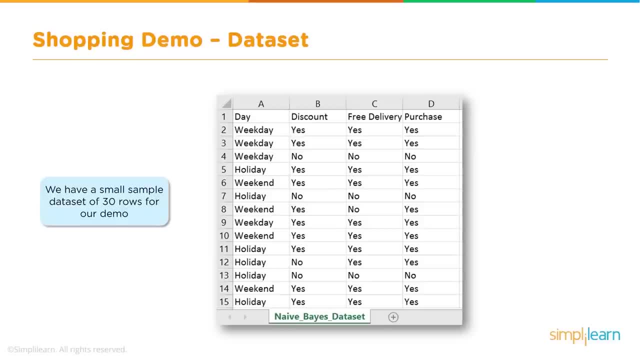 so let's go ahead and take a look at the data set. we have a small sample data set of 30 rows. we're showing you the first 15 of those rows for this demo. now the actual data file you can request, just type in below under: 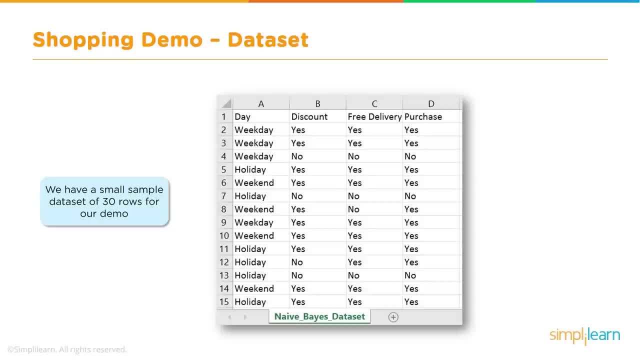 the comments on the youtube video and we'll send you some more information and send you that file. as you can see here, the file is very simple: columns and rows. we have the day, the discount, the free delivery, and did the person purchase or not? and then we have under: 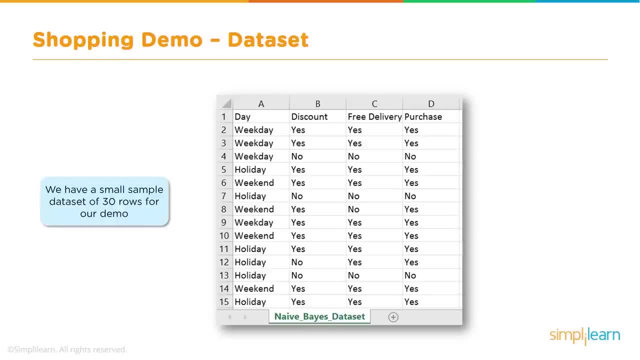 the day, whether it was a weekday, a holiday, was it the weekend? this is a pretty simple set of data and long before computers, people used to look at this data and calculate this all by hand. so let's go ahead and walk through this and see what that looks like. 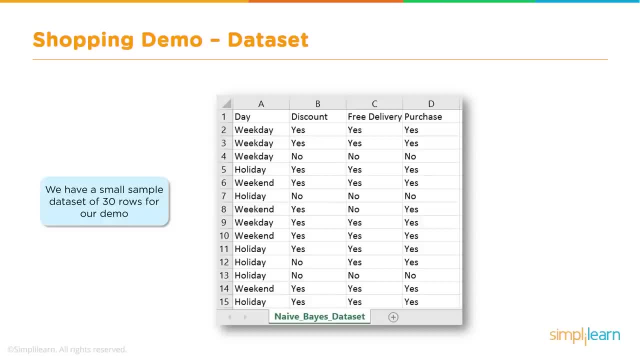 we put that into tables. also. note: in today's world we're not usually looking at three different variables in 30 rows. nowadays, because we're able to collect data so much, we're usually looking at 27, 30 variables across hundreds of rows. the first thing we want to do is we're going to take 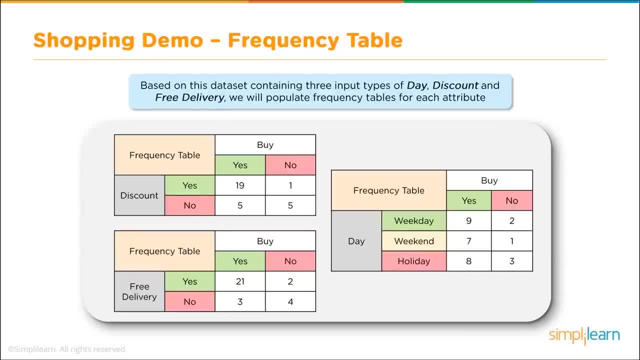 this data and based on the data set containing our three inputs- day, discount and free delivery- we're going to go ahead and populate that to frequency tables for each attribute. so we want to know, if they had a discount, how many people buy and did not buy. did they have a? 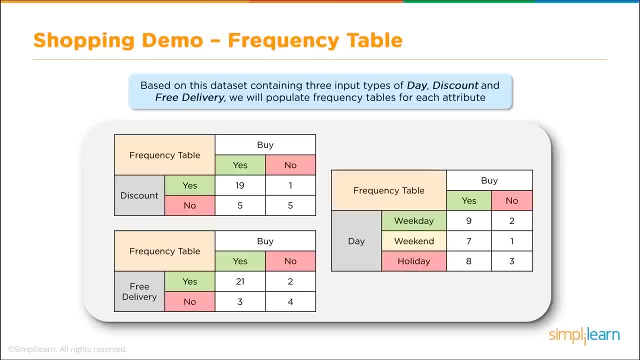 discount, yes or no? do we have a free delivery, yes or no? on those days, how many people made a purchase, how many people didn't? and the same with the three days of the week. was it a weekday, a weekend, a holiday? and did they buy, yes or no? as we dig? 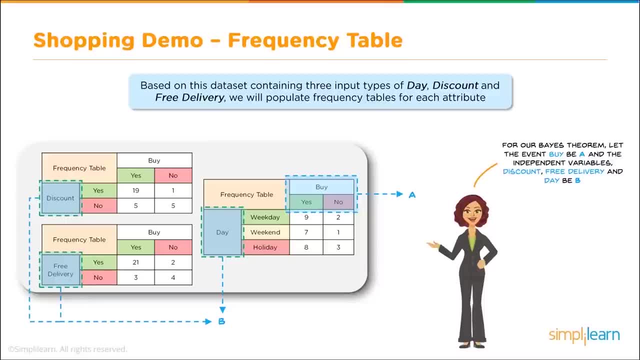 in deeper to this table for our Bayes theorem. let the event buy be a. now remember we looked at the coins. I said we really want to know what the outcome is- did the person buy or not? and that's usually event a is what you're looking. 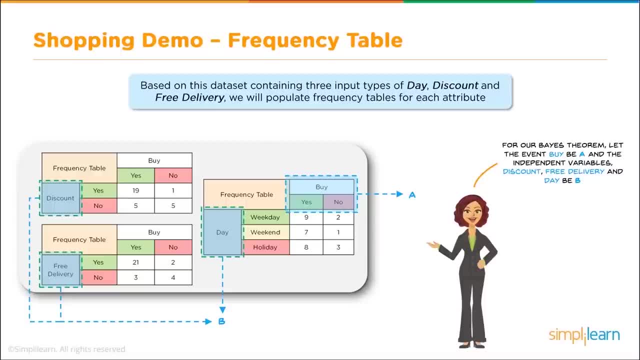 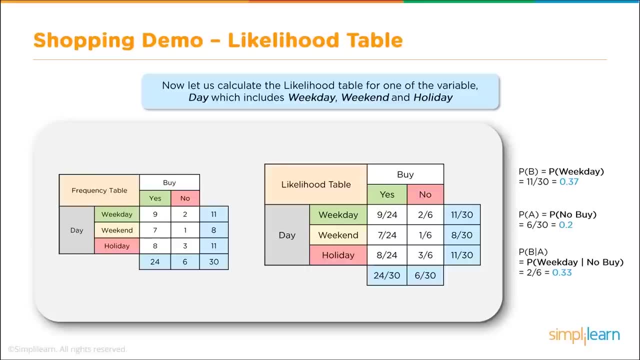 for and the independent variables discount, free delivery and day be b, so we'll call that probability of b. now let us calculate the likelihood table for one of the variables. let's start with day, which includes weekday, weekend and holiday, and let us start by summing all of our 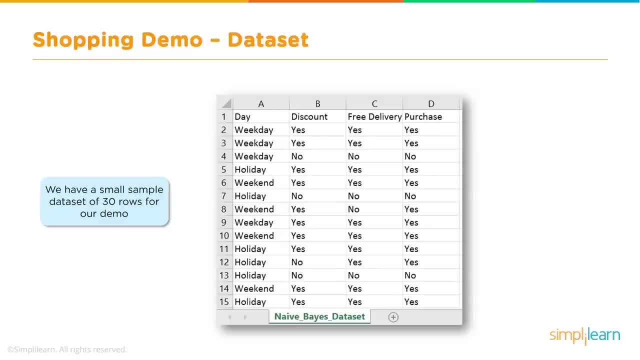 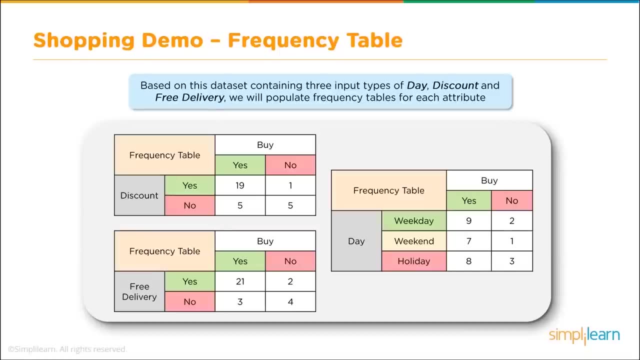 Nowadays, because we're able to collect data so much, we're usually looking at 27,, 30 variables across hundreds of rows. The first thing we want to do is we're going to take this data and, based on the data set containing our three inputs, 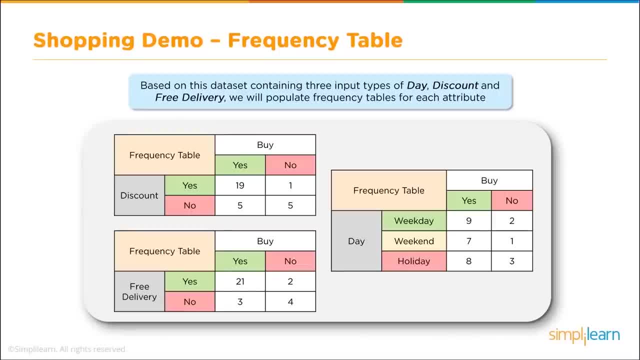 day discount and free delivery. we're going to go ahead and populate that to frequency tables for each attribute. So we want to know, if they had a discount, how many people buy and did not buy. Did they have a discount, yes or no? 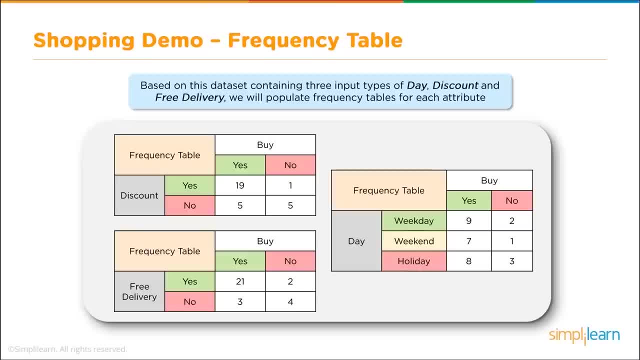 Do we have a free delivery, yes or no? On those days, how many people made a purchase, how many people didn't? And the same with the three days of the week: Was it a weekday, a weekend, a holiday? And did they buy, yes or no? 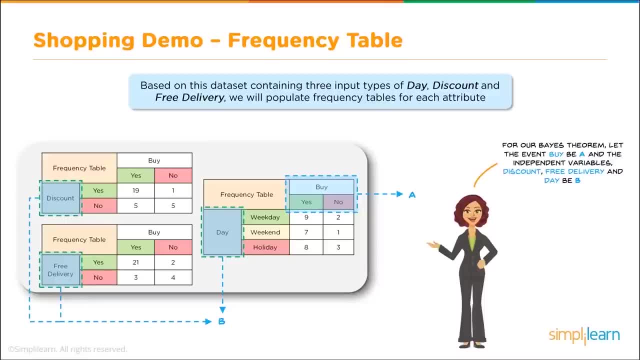 As we dig in deeper to this table for our Bayes theorem, let the event buy be A. Now remember when we looked at the coins I said we really want to know what the outcome is. Did the person buy or not? And that's usually event A is what you're looking for. 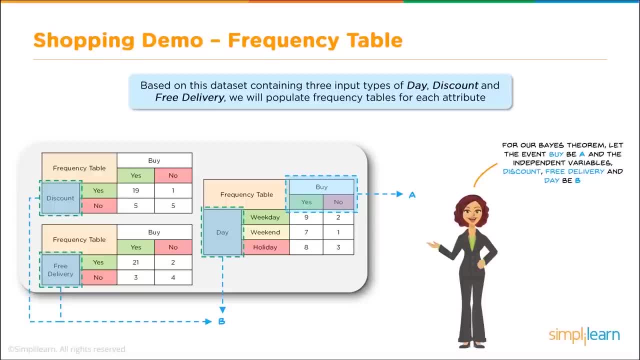 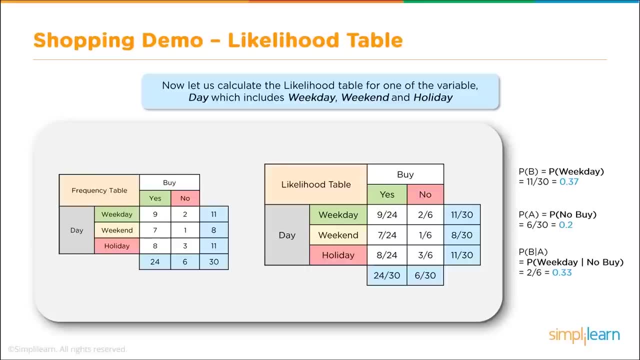 And the independent variables discount, free delivery and day be B, So we'll call that probability of B. Now let us calculate the likelihood table for one of the variables. Let's start with day, which includes weekday, weekend and holiday. 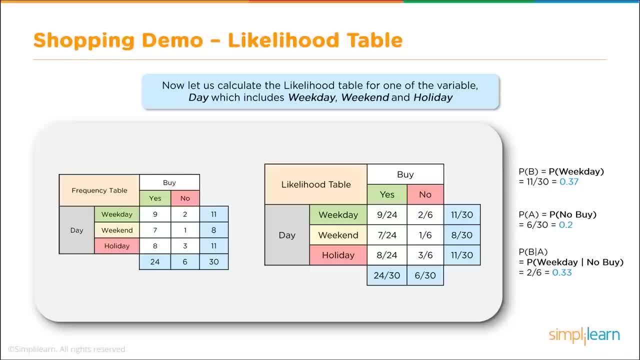 And let us start by summing all of our rows. So we have the weekday row and out of the weekdays there's nine plus two, so it's 11 weekdays. There's eight weekend days and 11 holidays. Wow, that's a lot of holidays. 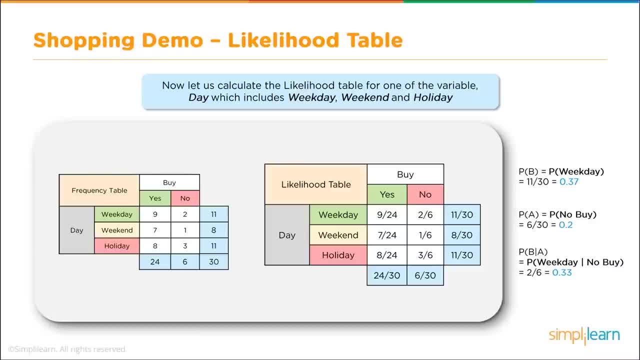 And then we want to sum up the total number of days. So we're looking at a total of 30 days. Let's start pulling some information from our chart and see where that takes us And when we fill in the chart on the right. 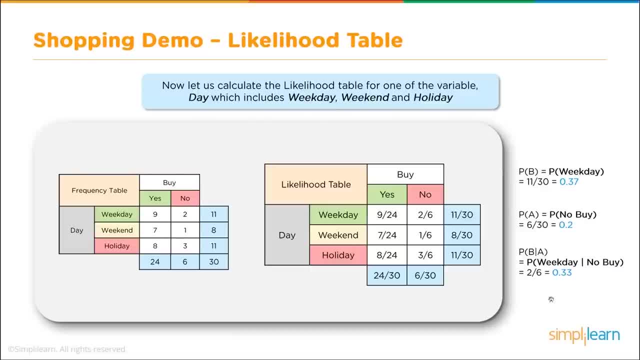 you can see that nine out of 24 purchases are made on the weekday, seven out of 24 purchases on the weekend and eight out of 24 purchases on a holiday. And, out of all the people who come in, 24 out of 30 purchase. 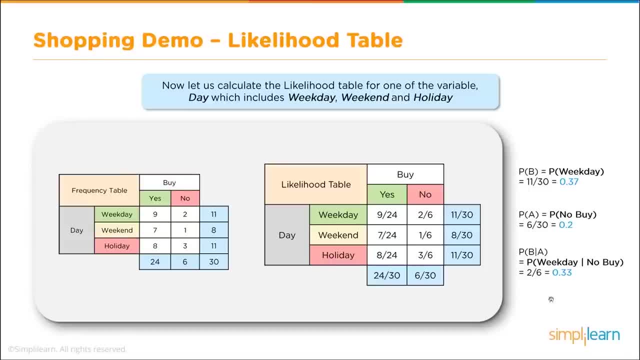 You can also see how many people do not purchase On the weekday. it's two out of six purchases, and so on and so on. We can also look at the totals And you'll see. on the right we put together some of the formulas. 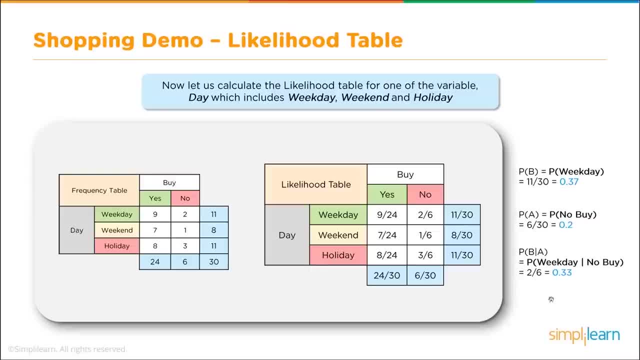 The probability of making a purchase on the weekend comes out at 11 out of 30.. So out of the 30 people who came into the store throughout the weekend, weekday and holiday, 11 of those purchases were made on the weekday. 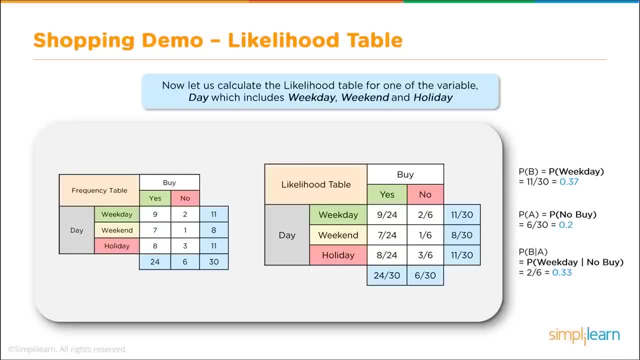 rows. so we have the weekday row and out of the weekdays there's 9 plus 2, so it's 11 weekdays. there's 8 weekend days and 11 holidays. that's a lot of holidays, and then we want to sum up the total number of days. so we're looking at 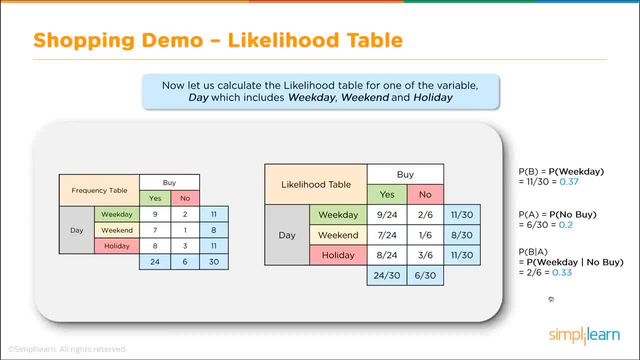 a total of 30 days. let's start pulling some information from our chart and see where that takes us and when we fill in the chart on the right, you can see that 9 out of 24 purchases are made on the weekday. 7 out of 24 purchases. 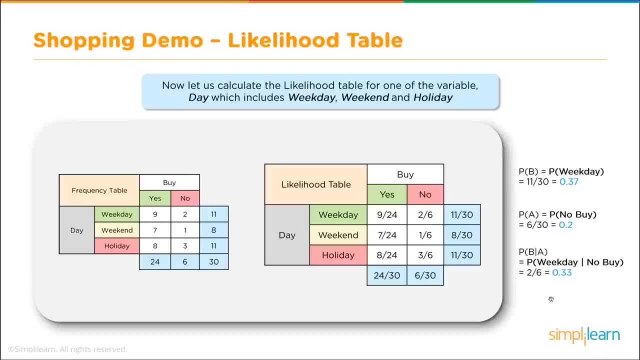 on the weekend and 8 out of 24 purchases on a holiday and out of all the people who come in, 24 out of 30 purchase. you can also see how many people do not purchase on the weekday: it's 2 out of 6 didn't purchase. 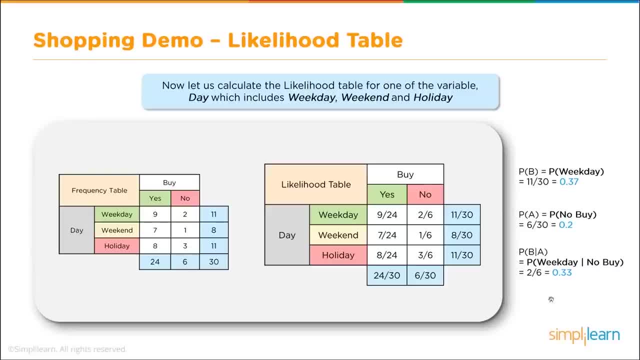 and so on and so on. we can also look at the totals and you'll see. on the right we put together some of the formulas. the probability of making a purchase on the weekend comes out at 11 out of 30. so out of the 30 people who came, 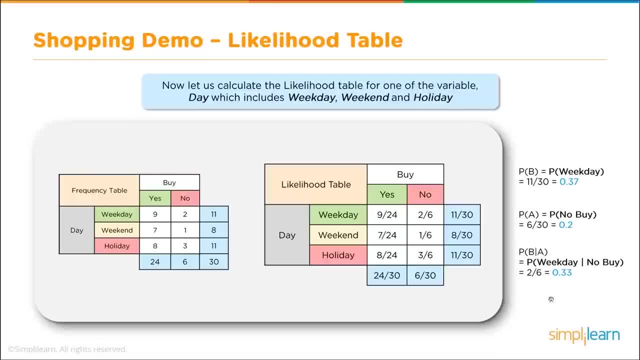 into the store throughout the weekend, weekday and holiday. 11 of those purchases were made on the weekday, and then you can also see the probability of them not making a purchase, and this is done for doesn't matter which day of the week. so we call that the probability of no buy would be. 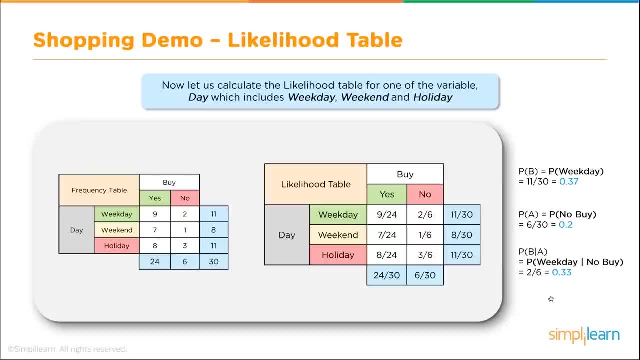 6 over 30 or 0.2. so there's a 20% chance that they're not going to make a purchase, no matter what day of the week it is. and finally, we look at the probability of B of A. in this case, we're going to look at the probability of the weekday. 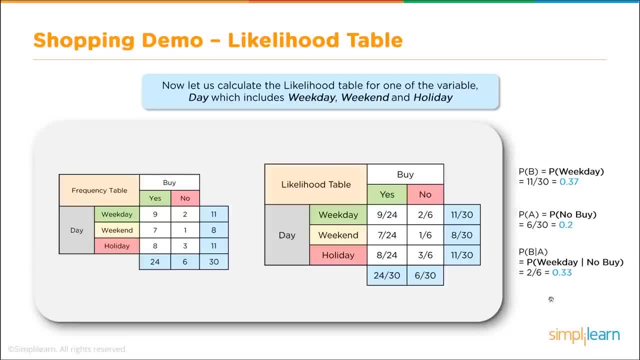 and not buying. 2 of the no buys were done out of the weekend out of the 6 people who did not make purchases. so when we look at that, probability of the weekday without a purchase is going to be 0.33 or 33%. 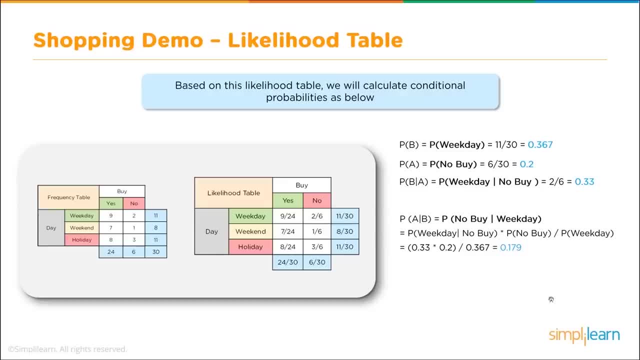 let's take a look at this, at different probabilities, and, based on this likelihood table, let's go ahead and calculate conditional probabilities as below the first three we just did. the probability of making a purchase on the weekday is 11 out of 30, or roughly 36 or 37%. 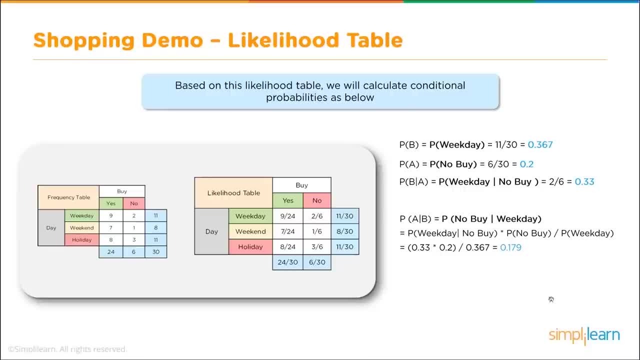 0.367. the probability of not making a purchase at all- doesn't matter what day of the week- is roughly 0.2 or 20%, and the probability of a weekday no purchase is roughly 2 out of 6. so 2 out of 6 of our no purchases. 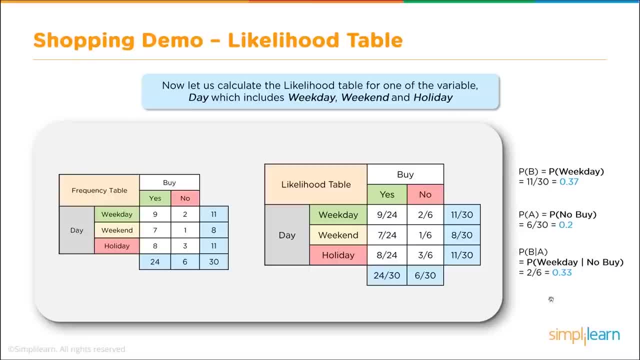 And then you can also see the probability of them not making a purchase, And this is done for doesn't matter which day of the week. So we call that probability of no buy. It would be six over 30, or .2.. 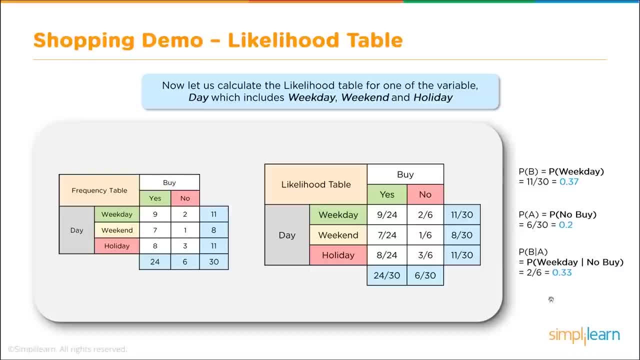 So there's a 20% chance that they're not gonna make a purchase, no matter what day of the week it is. And finally, we look at the probability of BFA. In this case, we're gonna look at the probability of the weekday and not buying. 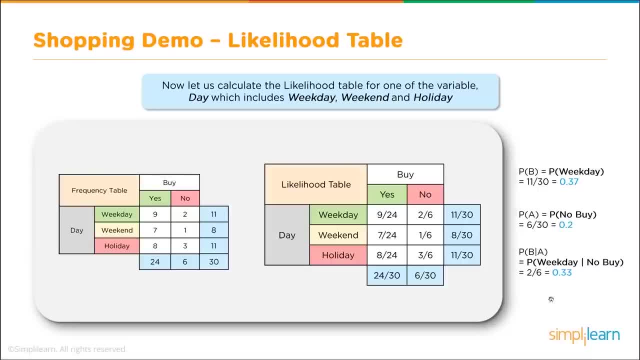 Two of the no buys were done out of the weekend, out of the six people who did not make purchases. So when we look at that, probability of the weekday without a purchase is gonna be .33 or 33%. Let's take a look at this at different probabilities. 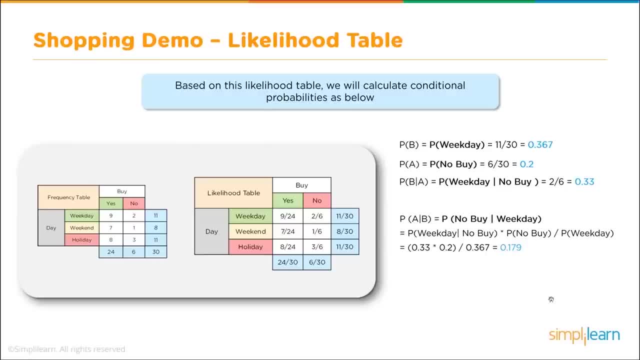 And, based on this likelihood table, let's go ahead and calculate the conditional probabilities as below The first three we just did. the probability of making a purchase on the weekday is 11 out of 30, or roughly 36 or 37% .367.. 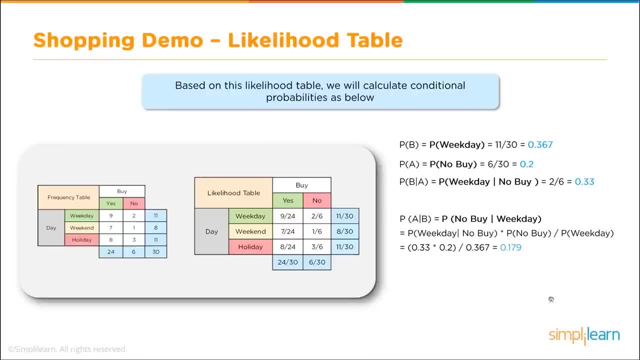 The probability of not making a purchase at all doesn't matter what day of the week is roughly .2 or 20%, And the probability of a weekday no purchase is roughly two out of six. So two out of six of our no purchases. 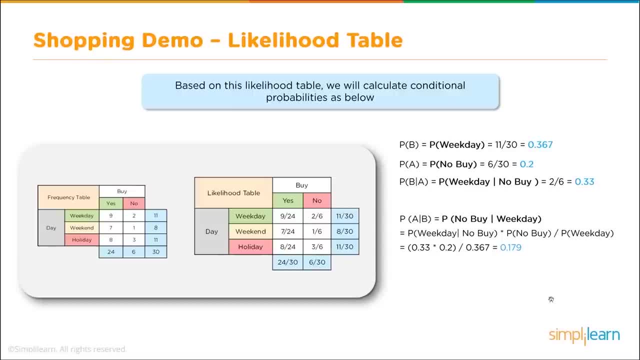 were made on the weekday. And then, finally, we take our P of AB. If you looked, we've kept the symbols up there. We got P of probability of B, probability of A, probability of B if A. We should remember that the probability of A if B. 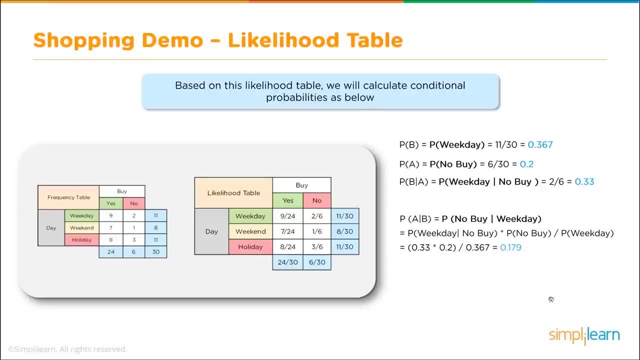 is equal to the first one times the probability of no buys over the probability of the weekday. So we could calculate it both off the table we created. we can also calculate this by the formula and we get the .367, which equals or .33 times .2 over .367, which equals .1.. 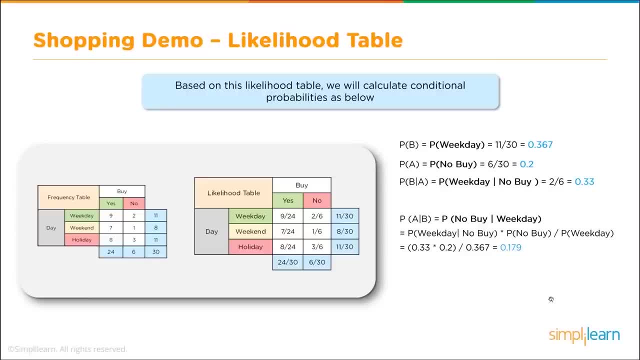 So that's .179, or roughly 17 to 18%, And that'd be the probability of no purchase done on the weekday. And this is important because we can look at this and say, as the probability of buying on the weekday is more than the probability of not buying on the weekday, 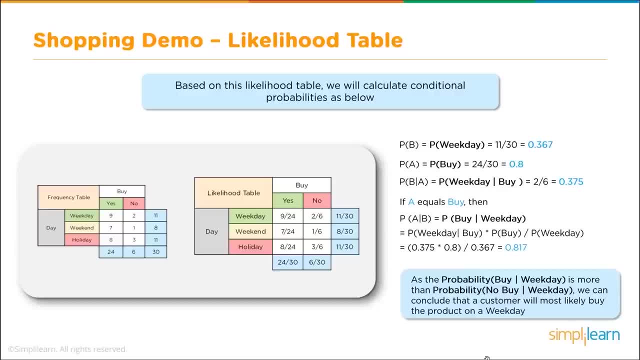 we can conclude that customers will most likely buy the product on a weekday. Now we've kept our chart simple and we're only looking at one aspect, So you should be able to look at the table and come up with the same information or the same conclusion. 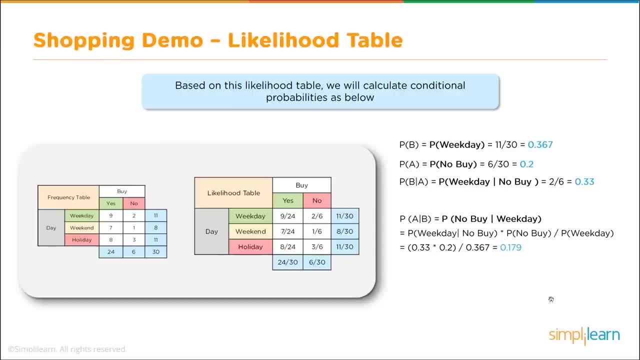 were made on the weekday. and then, finally, we take our P of AB. if you look, we've kept the symbols up there. we've got P of probability of B, probability of A, probability of B if A. we should remember that the probability of A if B is equal. 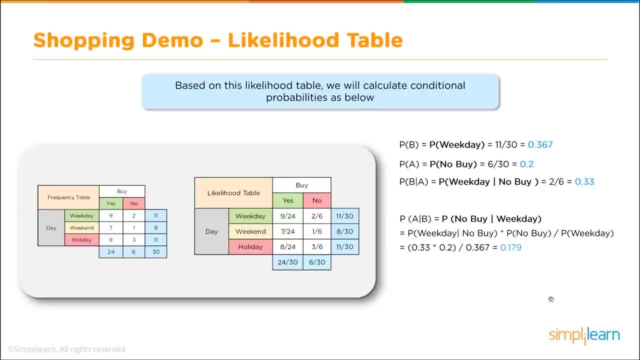 to the first one times the probability of no buys over the probability of the weekday, so we could calculate it both off the table we created. we can also calculate this by the formula and we get the 0.367, which equals, or 0.337 times 0.2 over 0.367. 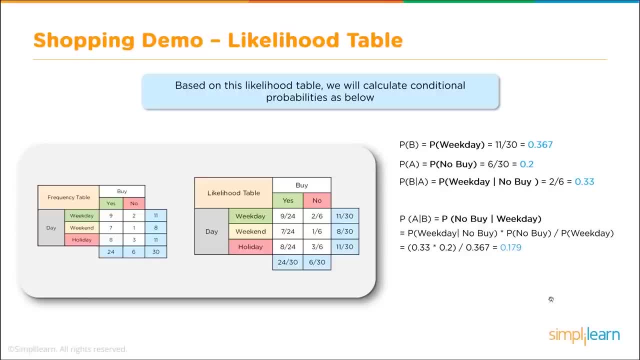 which equals 0.179, or roughly 17 to 18%, and that would be the probability of no purchase done on the weekday. and this is important because we can look at this and say, as the probability of buying on the weekday is more than the probability, 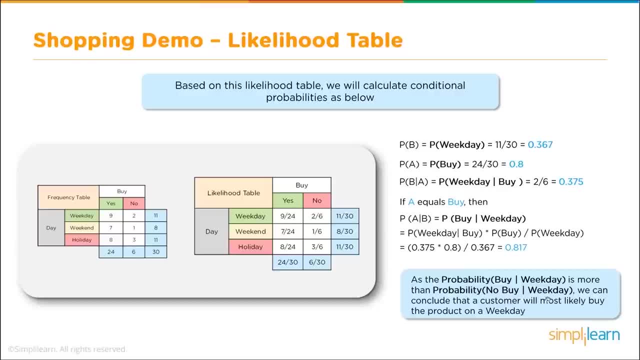 of not buying on the weekday, we can conclude that customers will most likely buy the product on a weekday. now we've kept our chart simple and we're only looking at one aspect, so you should be able to look at the table and come up with the same information or the same conclusion. 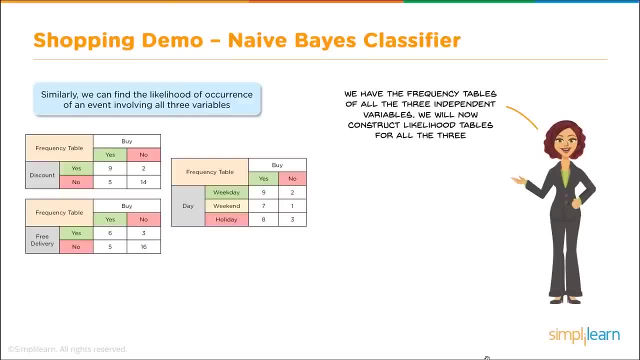 that should be kind of intuitive at this point. next, we can take the same setup. we have the frequency tables of all three independent variables. now we can construct the likelihood tables for all three of the variables we're working with. we can take our day like we did before. 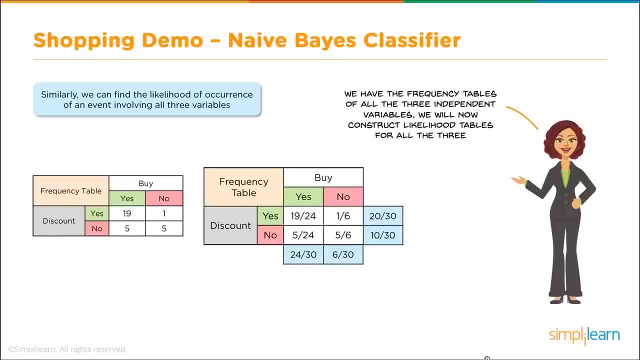 we have weekday, weekend and holiday and we filled in this table and then we can come in and also do that for the discount- yes or no, did they buy, yes or no? and we fill in that full table. so now we have our probabilities for a discount and whether the 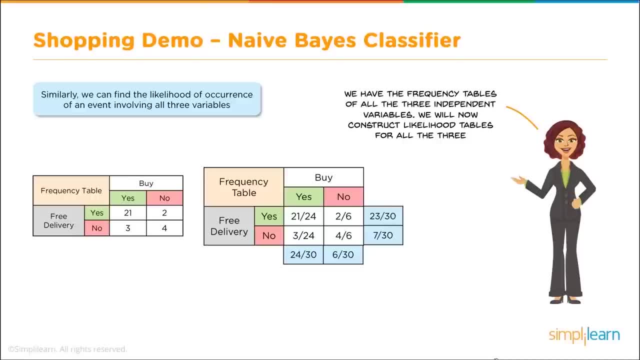 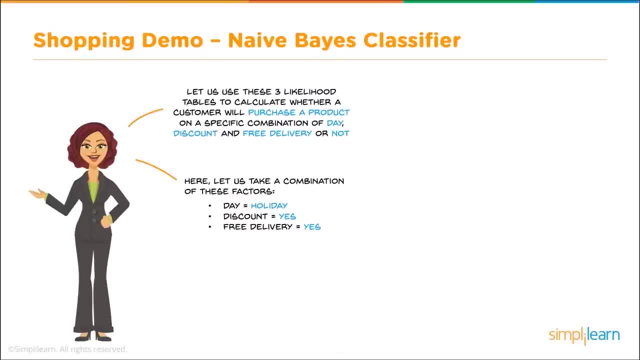 discount leads to a purchase or not, and the probability for free delivery. does that lead to a purchase or not? and this is where it starts getting really exciting. let us use these three likelihood tables to calculate whether a customer will purchase a product on a specific combination of day. 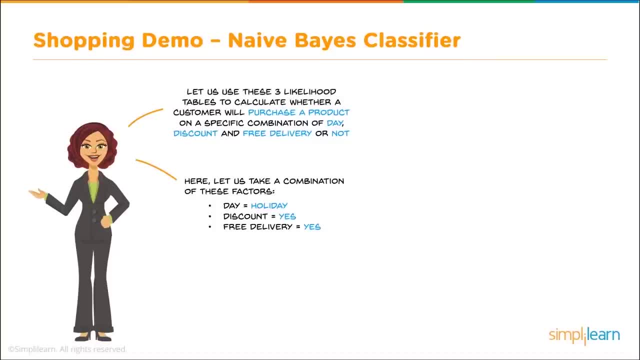 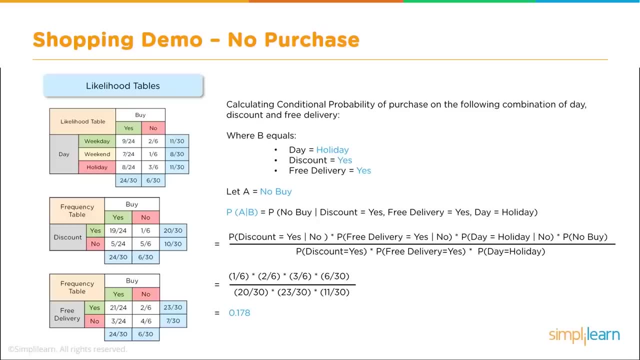 discount and free delivery or not purchase here, let us take a combination of these factors: day equals holiday, discount equals yes, free delivery equals yes. let's dig deeper into the math and actually see what this looks like, and we're going to start with looking for the probability. 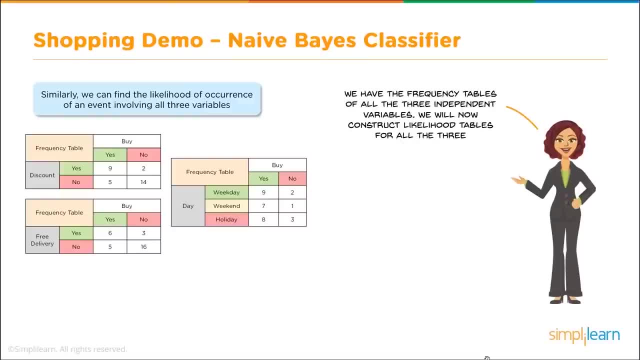 That should be kind of intuitive at this point. Next, we can take the same setup. We have the frequency tables of all three independent variables. Now we can construct the likelihood tables for all three of the variables we're working with. We can take our day like we did before. 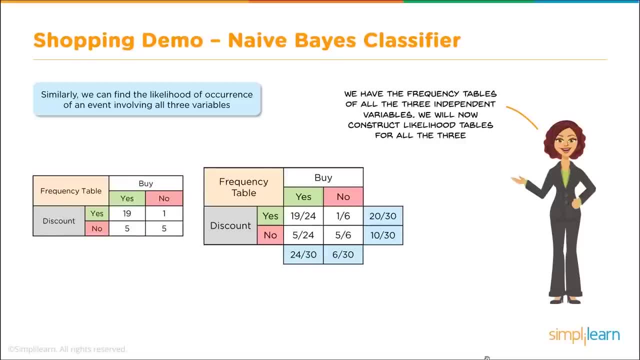 we have weekday, weekend and holiday and we filled in this table And then we can come in and also do that for the discount- yes or no, did they buy? yes or no? and we fill in that full table. So now we have our probabilities for a discount. 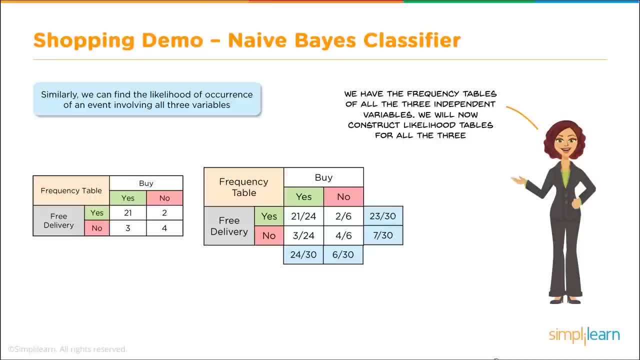 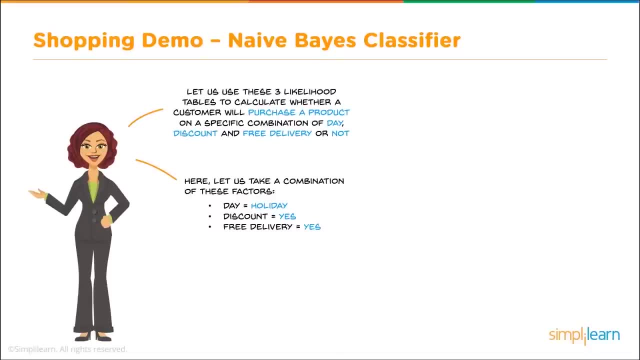 and whether the discount leads to a purchase or not, and the probability for free delivery. Does that lead to a purchase or not? And this is where it starts getting really exciting. Let us use these three likelihood tables to calculate whether a customer will purchase a product. 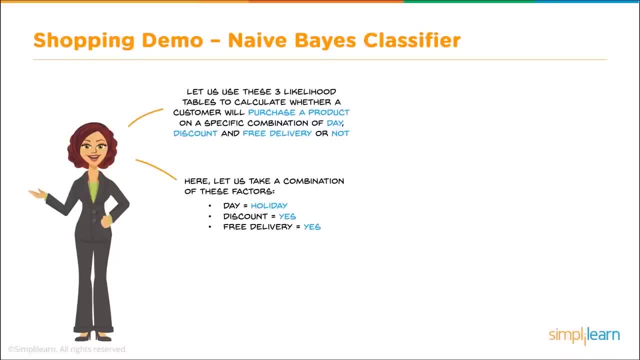 on a specific combination of day discount and free delivery or not purchase. Here let us take a combination of these factors: Day equals holiday discount equals yes. free delivery equals- yes. Let's dig deeper into the math and actually see what this looks like. 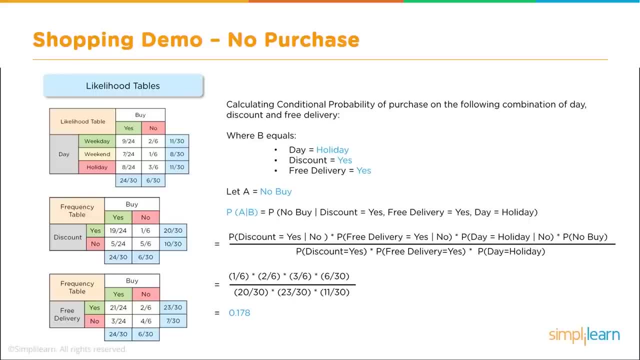 So we're gonna start with looking for the probability of them not purchasing on the following combinations of days. We are actually looking for the probability of A equal, no buy, no purchase, And our probability of B we're gonna set equal to. is it a holiday? did they get a discount? yes, 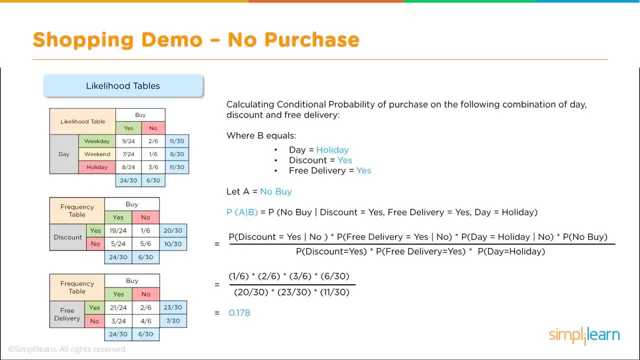 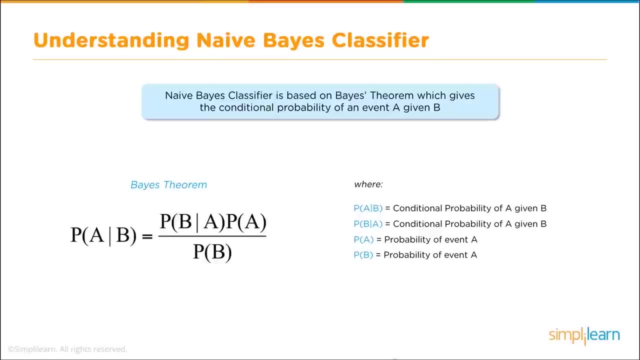 and was it a free delivery? yes, Before we go further, let's look at the original equation. The probability of A if B equals the probability of B, given the condition A and the probability times. probability of A Over the probability of B occurring. 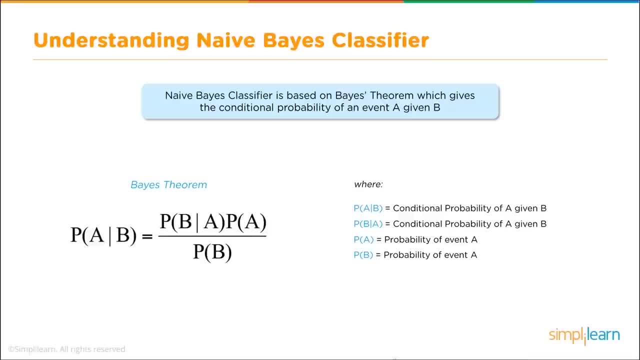 Now this is basic algebra so we can multiply this information together. So when you see the probability of A given B- in this case the condition is B, C and D, or the three different variables we're looking at- And when you see the probability of B, 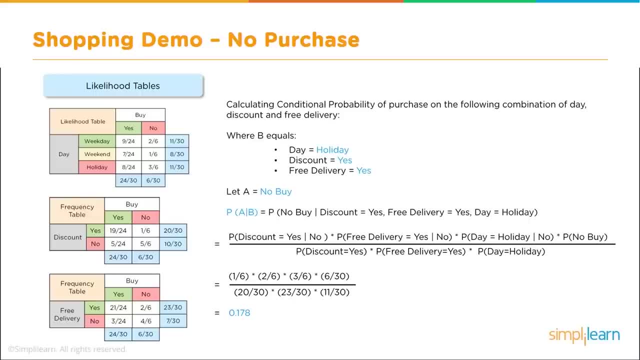 of them not purchasing. on the following combinations of days we're actually looking for. the probability of A equals no buy, no purchase, and our probability of B we're going to set equal to: is it a holiday? did they get a discount? yes, and was it a free delivery? yes, 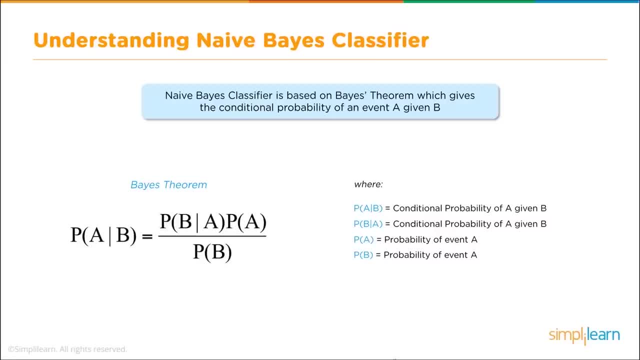 before we go further, let's look at the original equation: the probability of A if B equals the probability of B, given the condition A and the probability times the probability of A over the probability of B occurring. now. this is basic algebra, so we can multiply this information together. 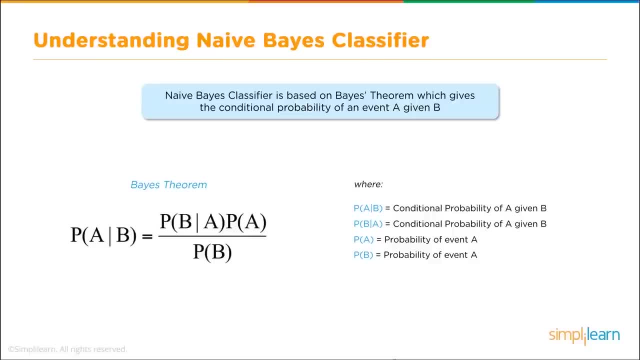 so when you see the probability of A given B- in this case the condition is B, C and D, or the three different variables we're looking at, and when you see the probability of B, that would be the conditions- we're actually going to multiply those three separate conditions. 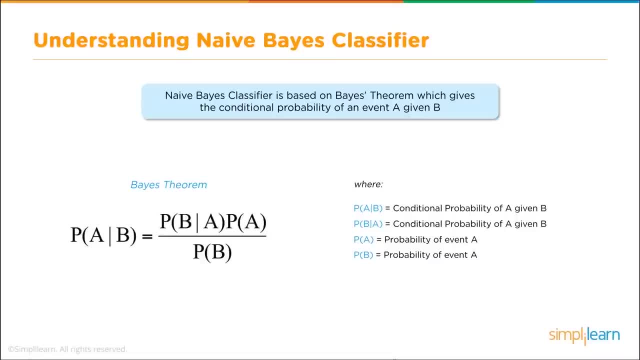 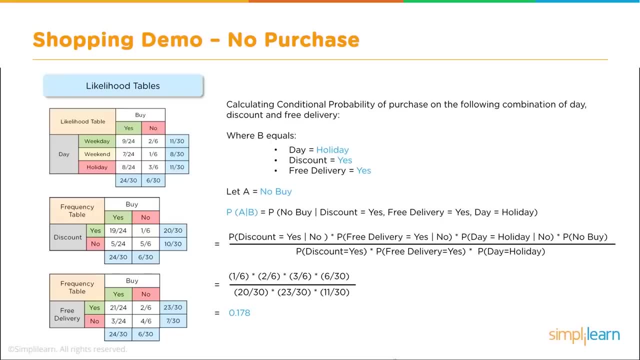 out probability of, you'll see that in just a second in the formula times the full probability of A over the full probability of B. so here we are, back to this and we're going to have let A equal no purchase and we're looking for the probability of B on the condition A. 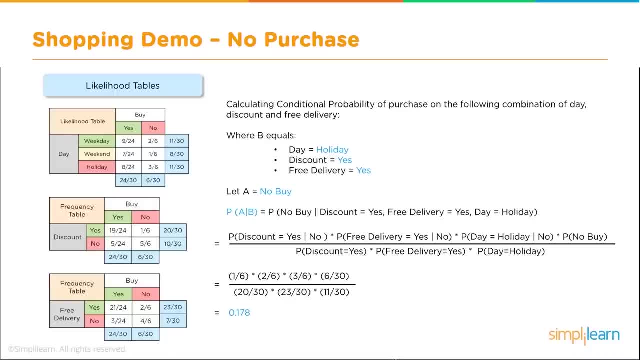 where A sets for three different things. remember that equals the probability of A given the condition B, and in this case we just multiply those three different variables together, so we have the probability of the discount times, the probability of free delivery times, the probability is the day equals a holiday. 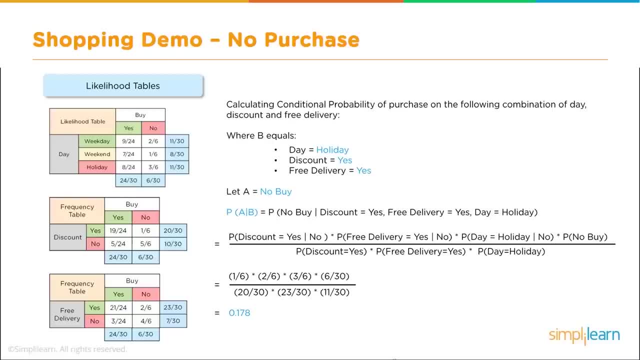 those are our three variables of the probability of A, if B, and then that is going to be multiplied by the probability of them not making a purchase, and then we want to divide that by the total probabilities and they're multiplied together so we have the probability of a discount. 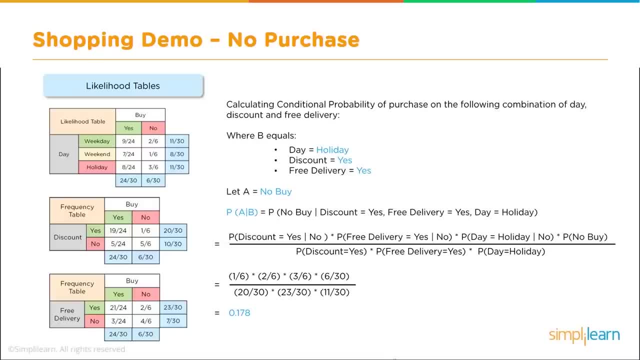 the probability of a free delivery and the probability of it being on a holiday. when we plug those numbers in, we see that one out of six were no purchase on a discounted day, two out of six were a no purchase on a free delivery day and three out of six were a no. 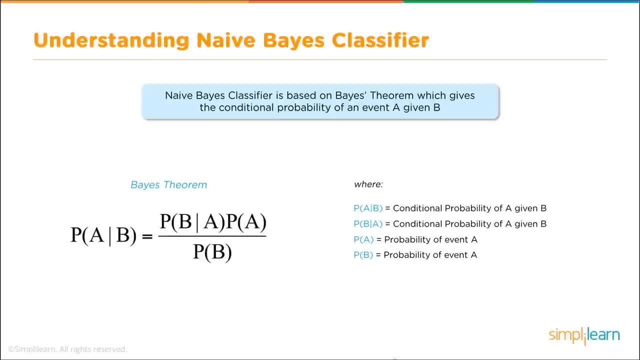 that would be the conditions. we're actually gonna multiply those three separate conditions out: Probability of. you'll see that in just a second in the formula times the full probability of A over the full probability of B. so here we are, back to this, and we're gonna have 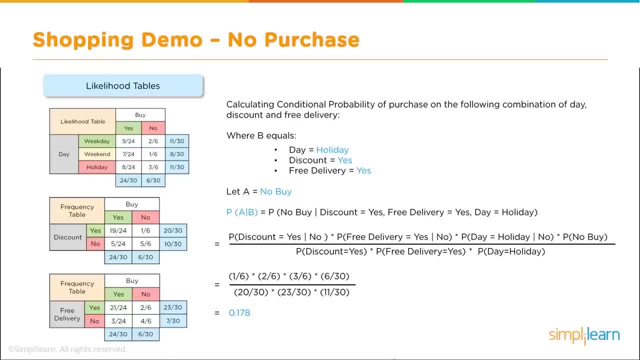 let A equal no purchase and we're looking for the probability of B on the condition A, where A sets for three different things. Remember that equals the probability of A given the condition B And in this case we just multiply those three different variables together. 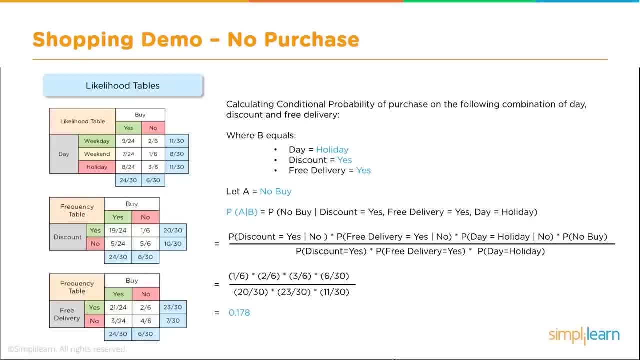 So we have the probability of the discount times. the probability of free delivery times. the probability is the day equal holiday Times. the probability of free delivery times: the probability is the day equal holiday. Those are three variables of the probability of A. if B. 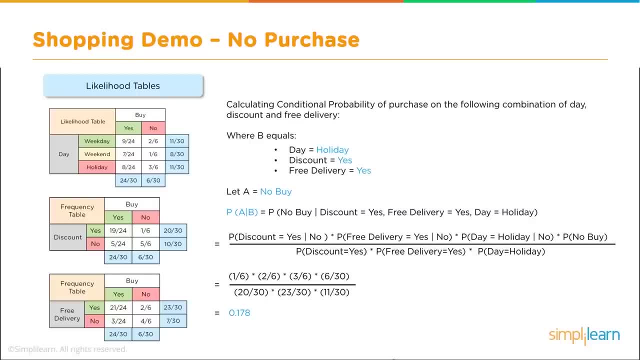 And then that is gonna be multiplied by the probability of them not making a purchase. And then we wanna divide that by the total probabilities and they're multiplied together. So we have the probability of a discount, the probability of a free delivery and the probability of it being on a holiday. 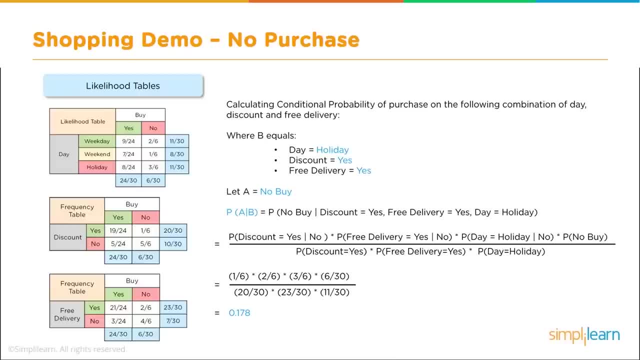 When we plug those numbers in, we see that one out of six were no purchase on a discounted day, two out of six were a no purchase on a free delivery day and three out of six were a no purchase on a holiday. Those are our three probabilities of A if B multiplied out. 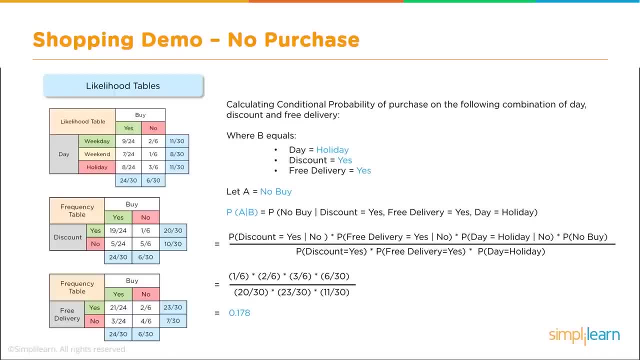 And then that has to be multiplied by the probability of a no purchase. And remember, the probability of a no buy is across all the data. So that's where we get the six out of 30.. We divide that out by the probability of each category. 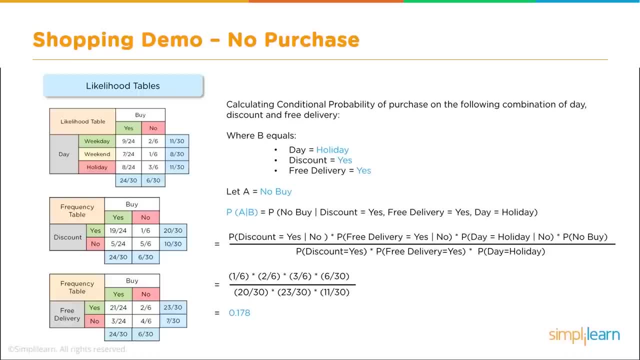 over the total number. So we get the: 20 out of 30 had a discount, 23 out of 30 had a yes for free delivery, seven out of 30 were on a holiday. We plug all those numbers in, we get .178.. 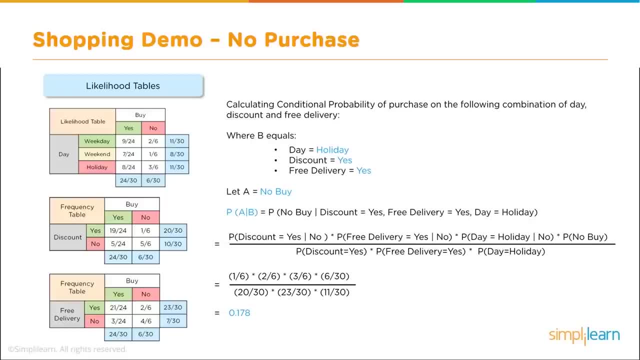 So in our probability math we have a .178. if it's a no buy for a holiday, a discount and a free delivery, Let's turn that around and see what that looks like if we have a purchase. I promise this is the last page of math. 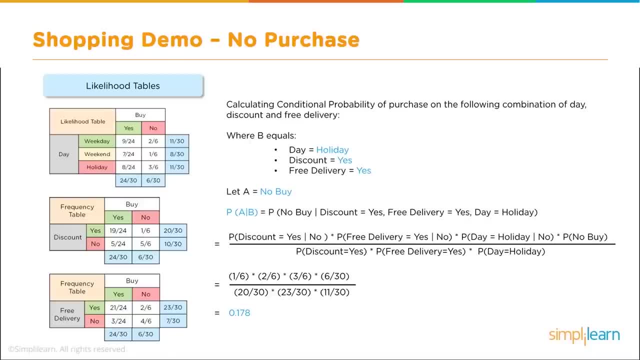 purchase on a holiday. those are our three probabilities of A if B multiplied out. and then that has to be multiplied by the probability of a no purchase. and remember, the probability of a no buy is across all the data. so that's where we get the six out of thirty. we divide that out. 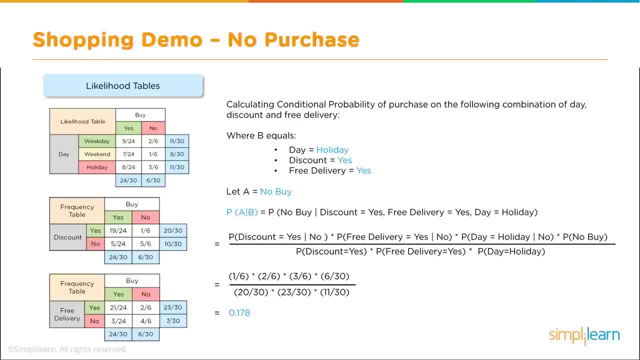 by the probability of each category over the total number. so we get the twenty out of thirty had a discount, twenty three out of thirty had a yes for free delivery and seven out of thirty were on a holiday. we plug all those numbers in. we get point one: seven, eight. 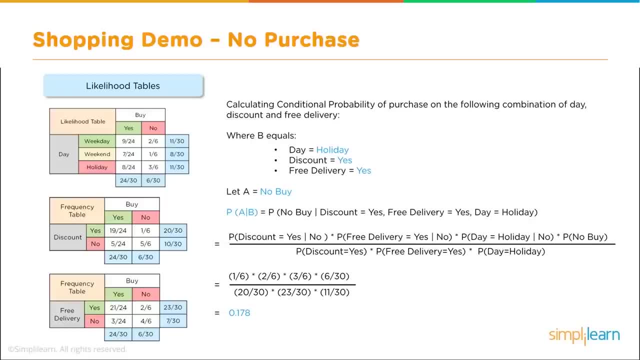 so in our probability math we have a point one, seven, eight. if it's a no buy for a holiday, a discount and a free delivery, let's turn that around and see what that looks like if we have a purchase. I promise this is the last page of math. 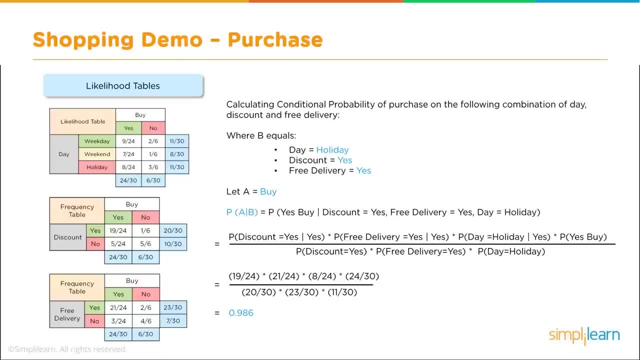 before we dig into the python script. so here we're, calculating the probability of the purchase using the same math we did to find out if they didn't buy. now we want to know if they did buy and again we're going to go by the probability of a holiday. 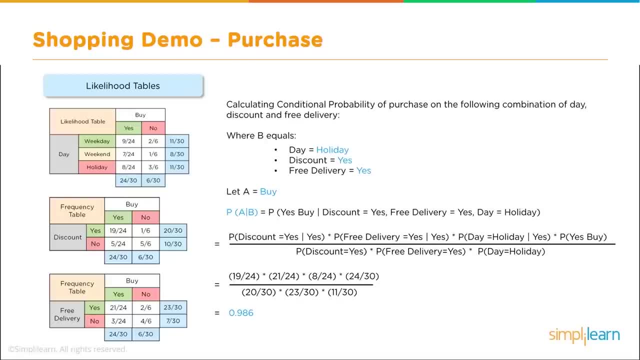 discount equals yes. free delivery equals yes. and let a equal buy. now, right about now, you might be asking: why are we doing both calculations? why would we want to know the no buys and buys for the same data going in? well, we're going to show you that in just a moment. 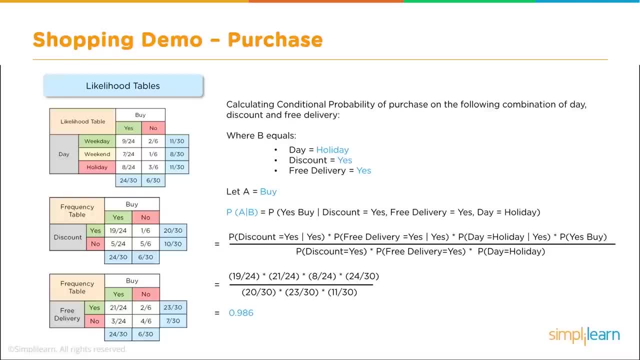 but we have to have both of those pieces of information so that we can figure it out as a percentage as opposed to a probability equation, and we'll get to that normalization here in just a moment. let's go ahead and walk through this calculation and, as you can see here, 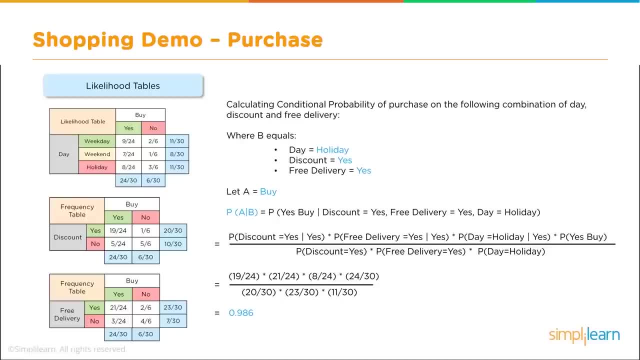 we have the probability of a on the condition of b, b being all three categories. did we have a discount with a purchase? do we have a free delivery with a purchase and is a day equal to holiday? and when we plug this all into that formula and multiply it all out, 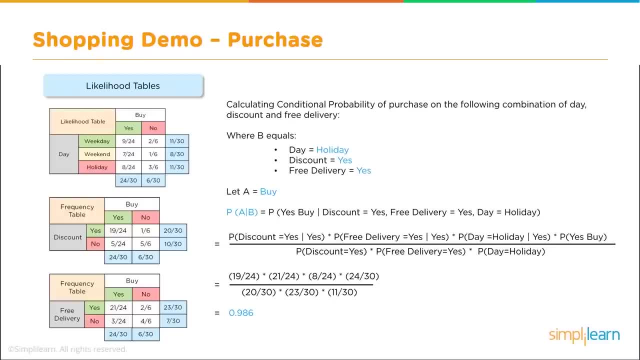 we get our probability of a discount, probability of a free delivery, probability of the day being a holiday times, the overall probability of it being a purchase divided by, again, multiplying the three variables out, the full probability of there being a discount, the full probability of there being a free delivery. 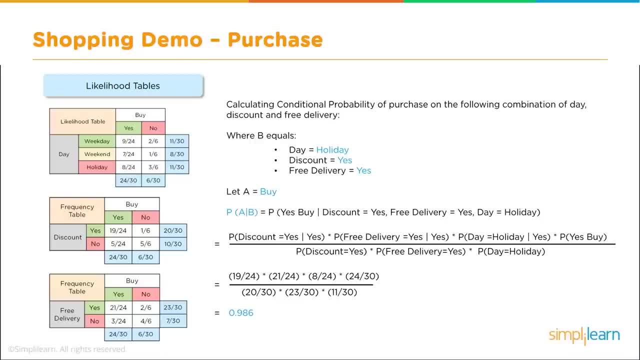 before we dig into the Python script. So here we're, calculating the probability of the purchase using the same math we did to find out if they didn't buy. Now we wanna know if they did buy. And again we're gonna go by the day equals. 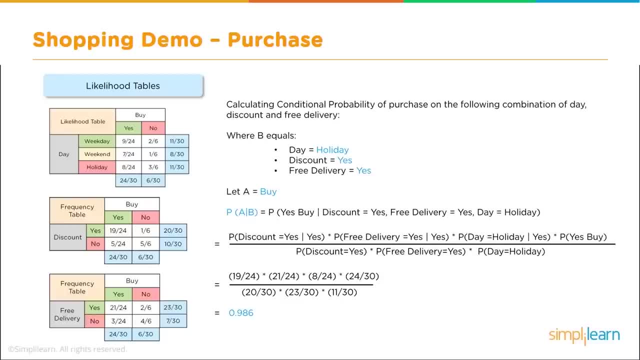 holiday discount equals yes. free delivery equals: yes. and let A equal buy. Now, right about now, you might be asking: why are we doing both calculations? Why would we wanna know the no buys and buys for the same data going in? Well, we're gonna show you that in just a moment. 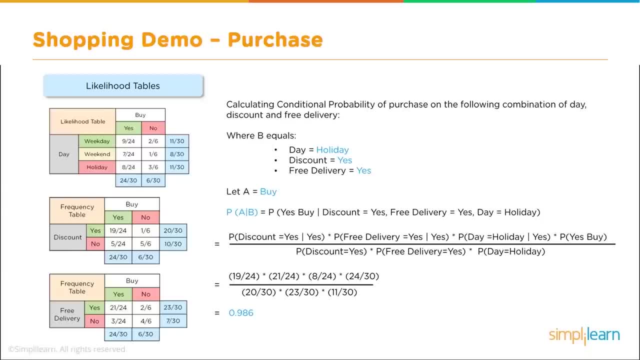 but we have to have both of those pieces of information so that we can figure it out as a percentage as opposed to a probability equation, And we'll get to that normalization here in just a moment. Let's go ahead and walk through this calculation. 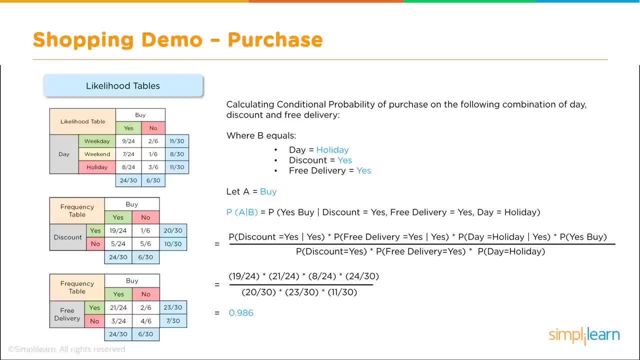 And, as you can see, here we get a probability of A on the condition of B, B being all three categories. Did we have a discount with a purchase? Do we have a free delivery with a purchase And is a day equal to holiday? 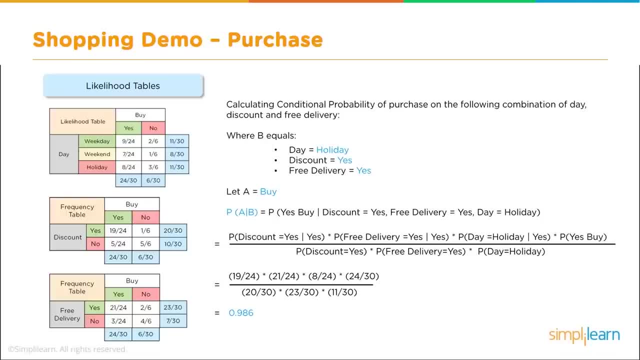 And when we plug this all into that formula and multiply it all out, we get our probability of a discount, probability of a free delivery, probability of the day being a holiday times, the overall probability of it being a purchase, divided by again multiplying the three variables out. 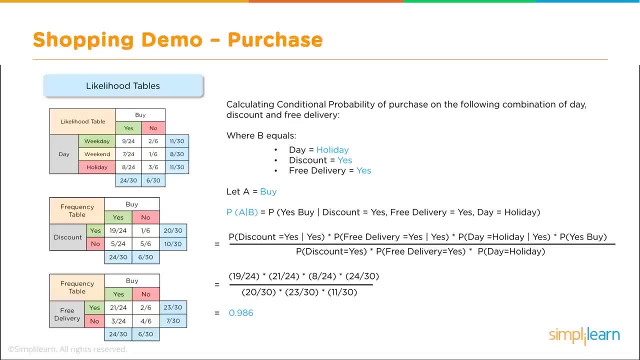 the full probability of there being a discount, the full probability of being a free delivery and the full probability of there being a day equal holiday. And that's where we get this: 19 over 24 times 21 over 24 times. eight over 24. 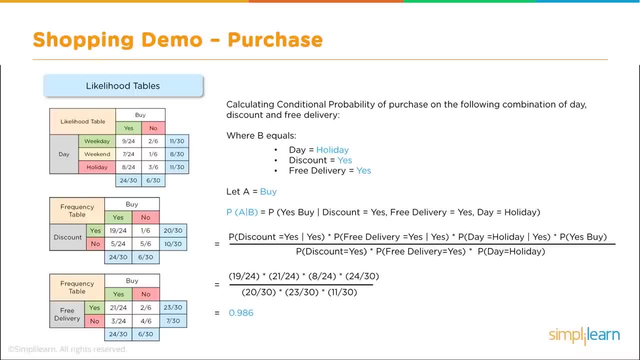 times the P of A, 24 over 30, divided by the probability of the discount, the free delivery times the day, or 20 over 30,, 23 over 30 times 11 over 30, and that gives us our .986.. 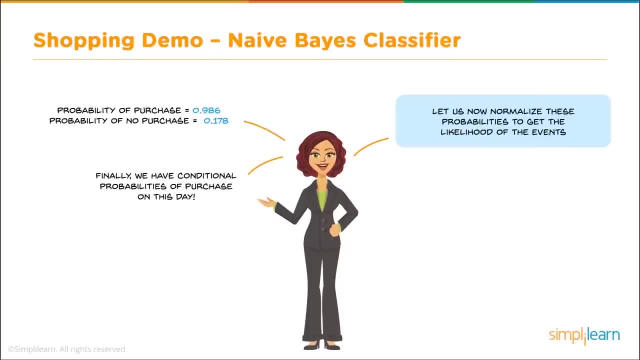 So what are we gonna do with these two pieces of data that we just generated? Well, let's go ahead and go over them. We have a probability of purchase equals .986.. We have a probability of no purchase equals .178.. So, finally, we have a conditional probabilities. 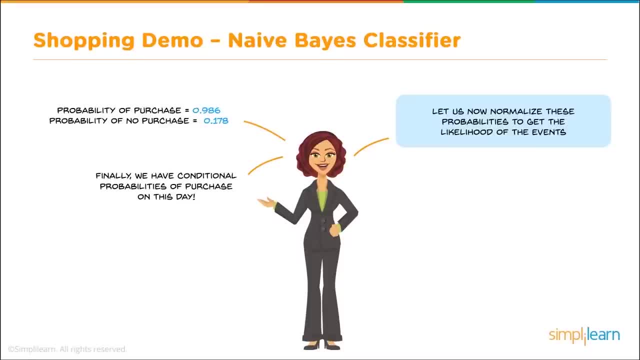 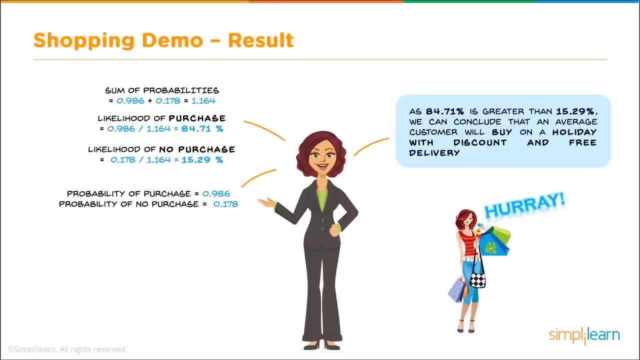 of purchase on this day. Let us take that we're gonna normalize it and we're gonna take these probabilities and turn them into percentages. This is simply done by taking the sum of probabilities, which equals .986 plus .178, and that equals the 1.164.. 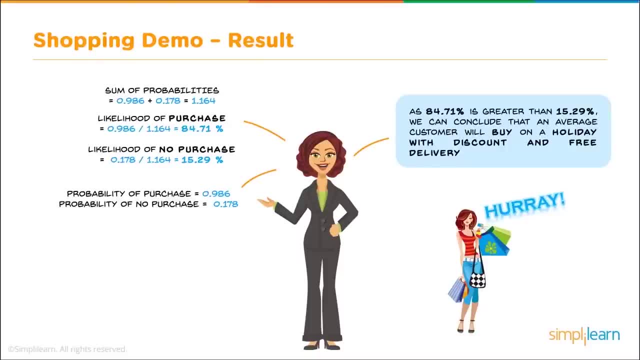 If we divide each probability by the sum, we get the percentage, And so the likelihood of a purchase is 84.71% and the likelihood of no purchase is 15.29%, given these three different variables. So if it's on a holiday, if it's with a discount, 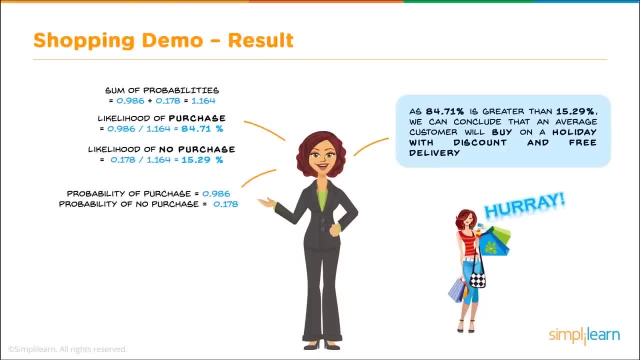 and has free delivery, then there's an 84.71% chance that the customer's gonna come in and make a purchase. Hooray, they purchased our stuff. We're making money. If you're owning a shop, that is the bottom line. 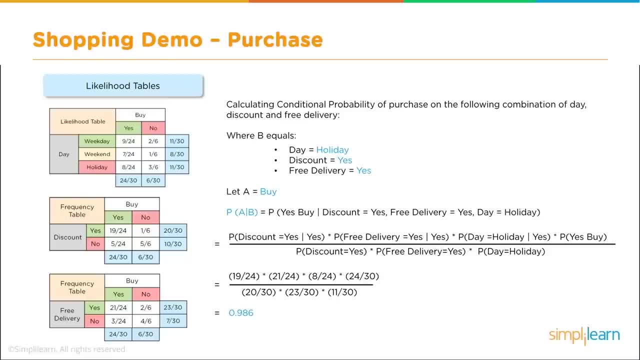 and the full probability of there being a day equal holiday. and that's where we get this: 19 over 24 times 21 over 24 times, 8 over 24 times the p of a 24 over 30 divided by the probability of the discount, the free delivery. 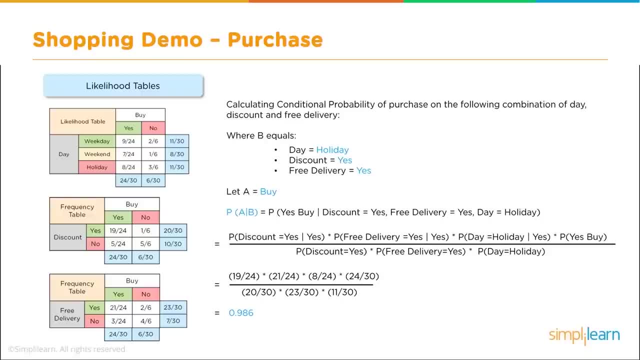 times the day, or 20 over 30, 23 over 30 times 11 over 30, and that gives us our .986. so what are we going to do with these two pieces of data we just generated? well, let's go ahead and go over them. 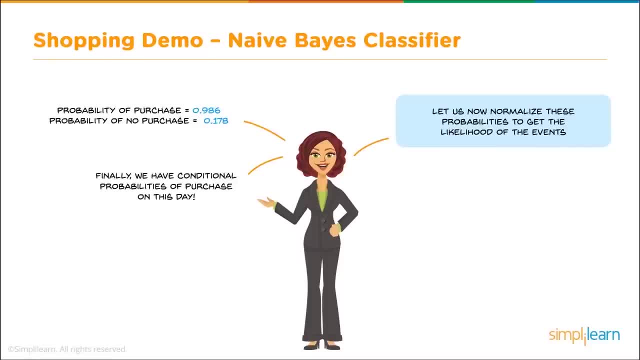 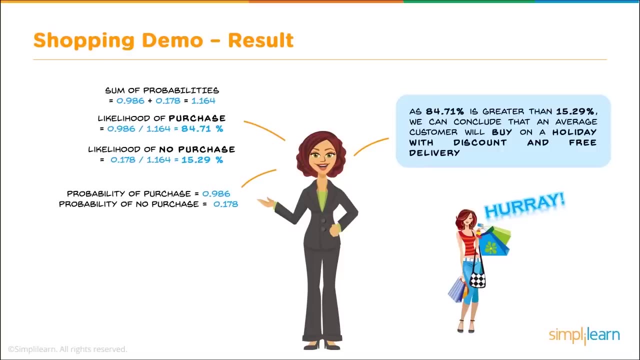 we have a probability of purchase equals .986. we have a probability of no purchase equals .178. so, finally, we have a conditional probability of purchase on this day. let us take that we're going to normalize it and we're going to take these probabilities and turn them into percentages. 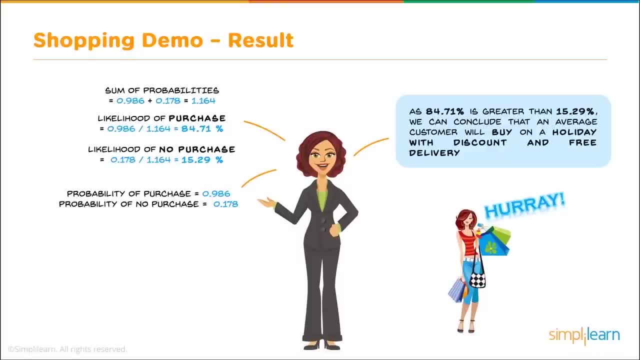 this is simply done by taking the sum of probabilities, which equals .986 plus .178, and that equals the 1.164, and if we divide each probability by the sum, we get the percentage, and so the likelihood of a purchase is 84.71%. 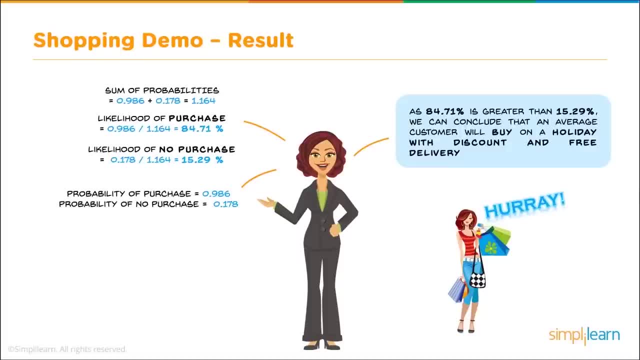 and the likelihood of no purchase is 15.29%, given these three different variables. so if it's on a holiday, if it's with a discount and has free delivery, then there's an 84.71% chance that the customer is going to come in and make a purchase. 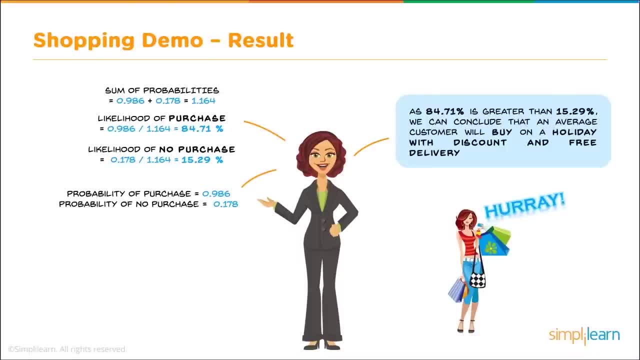 hooray, they purchased our stuff. we're making money. if you're owning a shop that's like is the bottom line is you want to make some money, you want to keep your shop open and have a living. now I promised you that we were going to be finishing up the math. 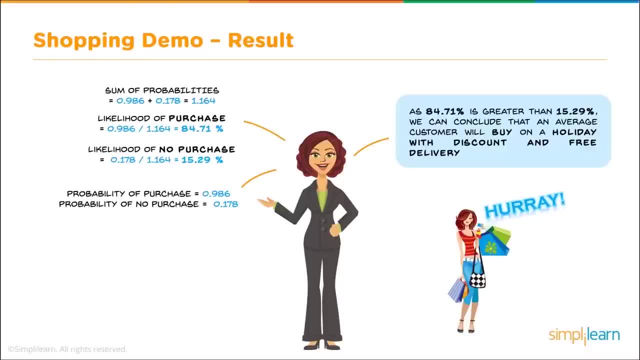 here with a few pages. so we're going to move on and we're going to do two steps. the first step is: I want you to understand why you want to use the naive Bayes, what are the advantages of naive Bayes. and then, once we understand, 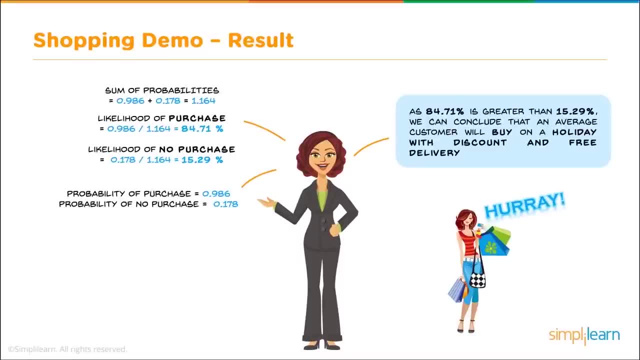 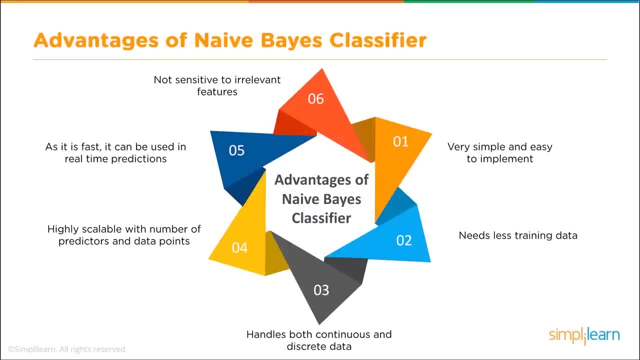 those advantages. we'll just look at that briefly. then we're going to dive in and do some Python coding. advantages of naive Bayes classifier. so let's take a look at the six advantages of the naive Bayes classifier and we're going to walk around this lovely wheel. 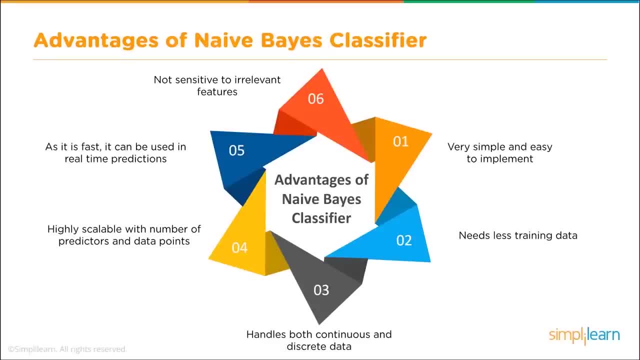 looks like an origami folded paper. the first one is very simple and easy to implement. certainly you could walk through the tables and do this by hand. you got to be a little careful because the notations can get confusing. you have all these different probabilities and I certainly mess those up as I put them on. 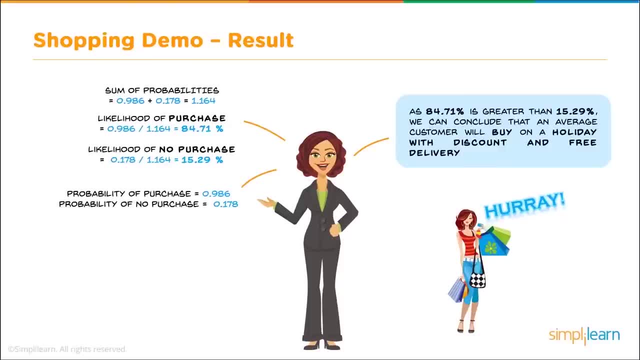 is you wanna make some money so that you can keep your shop open and have a living. Now I promised you that we were gonna be finishing up the math here with a few pages, So we're gonna move on and we're gonna do two steps. 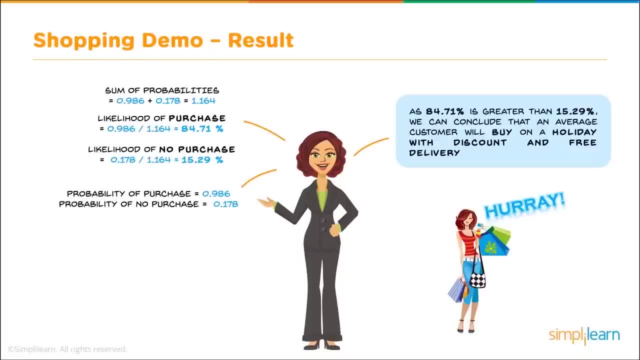 The first step is: I want you to understand why you wanna use the naive Bayes. What are the advantages of naive Bayes? And then, once we understand those advantages, we'll just look at that briefly. then we're gonna dive in and do some Python coding. 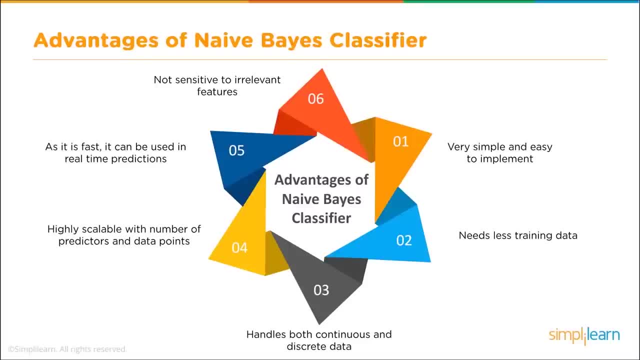 Advantages of naive Bayes classifier. So let's take a look at the six advantages of the naive Bayes classifier And we're gonna walk around this lovely wheel. It looks like an origami folded paper. The first one is very simple and easy to implement. 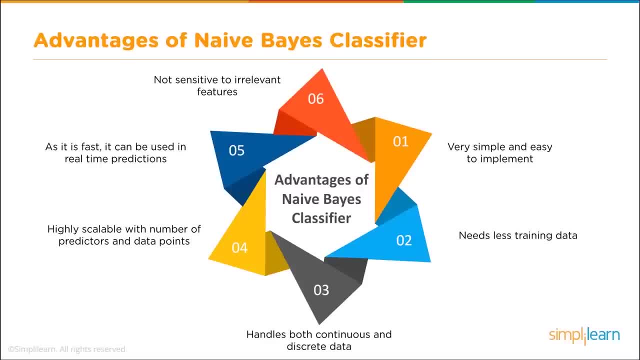 Certainly you could walk through the tables and do this by hand. You gotta be a little careful because the notations can get confusing. You have all these different probabilities and I certainly mess those up as I put them on. you know, is it on the top or the bottom? 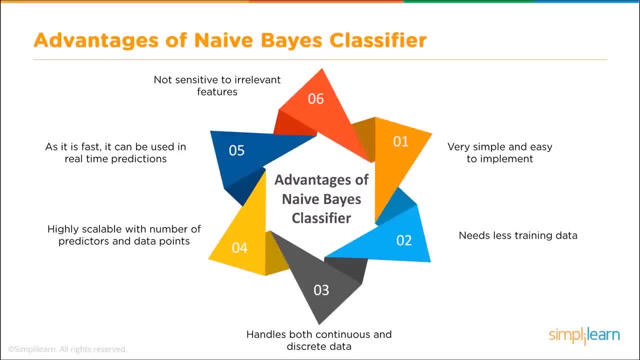 You gotta really pay close attention to that When you put it into Python. it's really nice because you don't have to worry about any of that. You let the Python handle that. the Python module Understanding it, you can put it on a table. 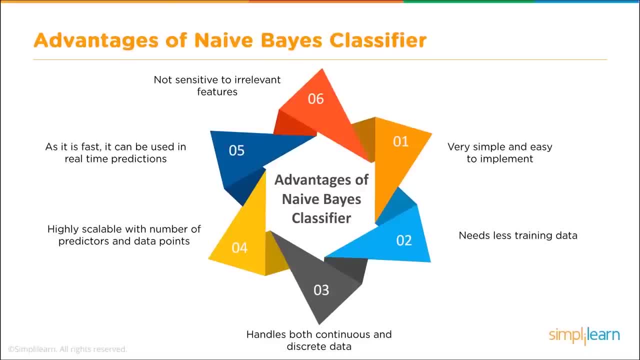 and you can easily see how it works. and it's a simple algebraic function. It needs less training data. So if you have smaller amounts of data, this is great powerful tool for that Handles both continuous and discrete data. It's highly scalable with number of predictors. 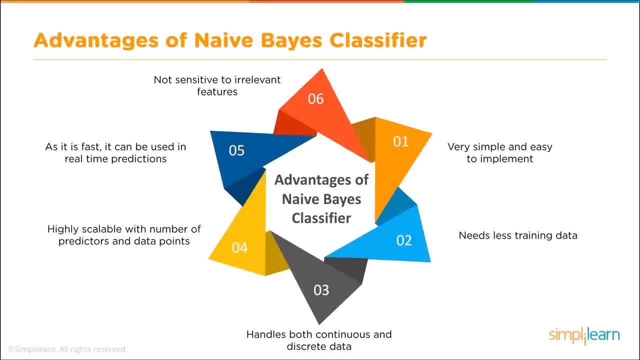 and data points. So, as you can see, you just keep multiplying different probabilities in there and you can cover not just three different variables or sets. You can now expand this to even more categories. Number five: it's fast, It can be used in real-time predictions. 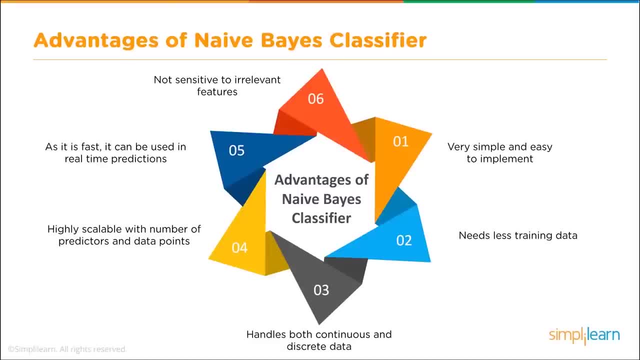 This is so important. This is why it's used in a lot of our predictions on online shopping carts, referrals, spam filters is because there's no time delay as it has to go through and figure out a neural network or one of the other mini setups. 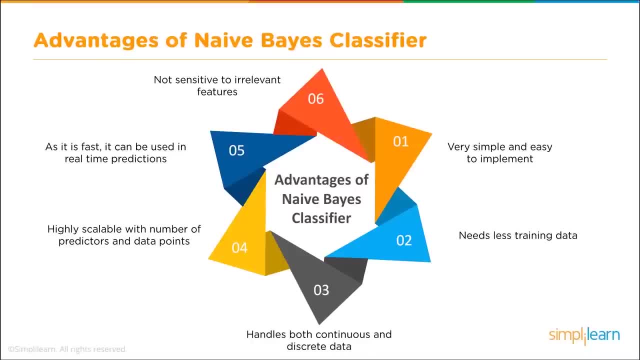 where you're doing classification, And certainly there's a lot of other tools out there in the machine learning that can handle these, but most of them are not as fast as the Naive Bayes. And then, finally, it's not sensitive to irrelevant features. 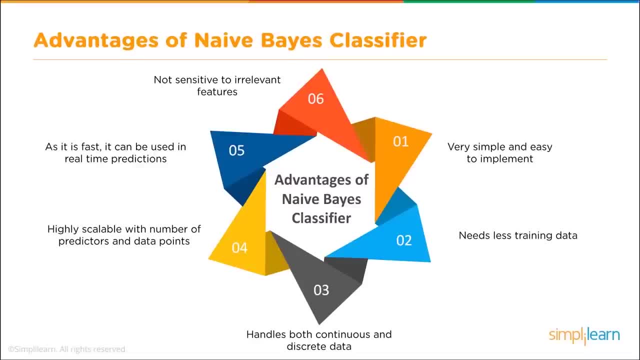 you know, is it on the top or the bottom? you got to really pay close attention to that. when you put it into Python, it's really nice because you don't have to worry about any of that. you let the Python handle that, the Python module. but, understanding it, you can put it on a table. 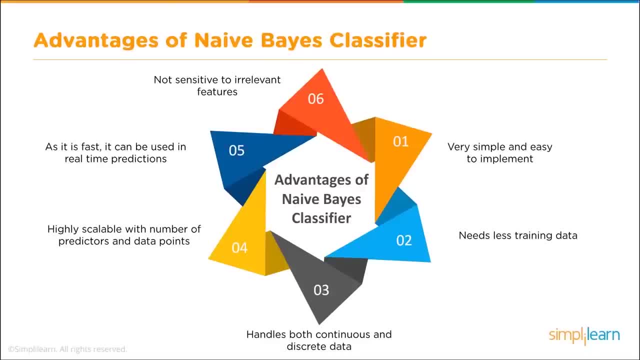 and you can easily see how it works. and it's a simple algebraic function. it needs less training data. so if you have smaller amounts of data, this is a great powerful tool for that handles both continuous and discrete data. it's highly scalable with number of predictors. 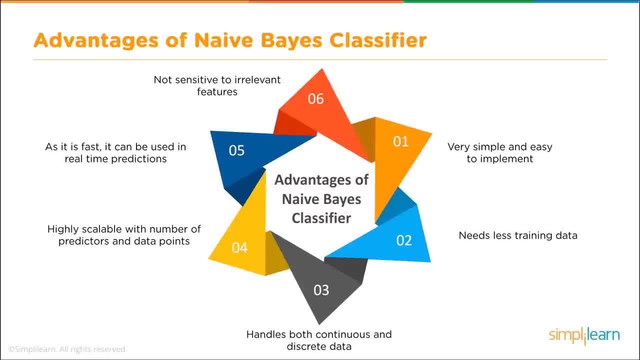 and data points. so, as you can see, you can just keep multiplying different probabilities in there and you can cover not just three different variables or sets. you can now expand this to even more categories. number five: it's fast. it can be used in real time predictions. this is so important. 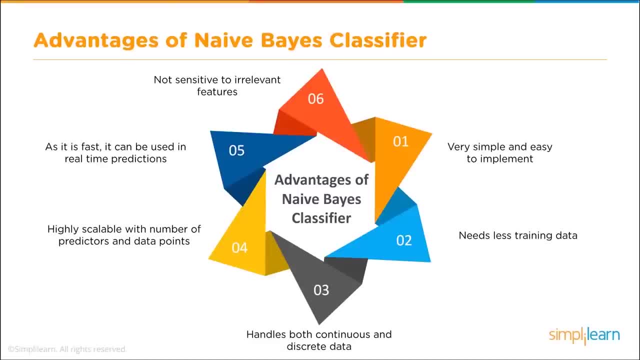 this is why it's used in a lot of our predictions on online shopping carts, referrals, spam filters is because there's no time delay as it has to go through and figure out a neural network or one of the other many setups where you're doing classification. 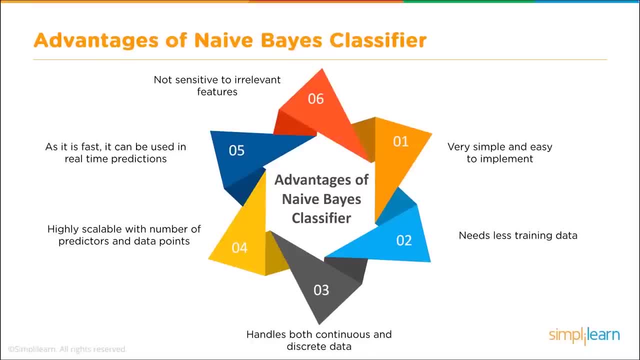 and certainly there's a lot of other tools out there in the machine learning that can handle these, but most of them are not as fast as the naive Bayes. and then, finally, it's not sensitive to irrelevant features, so it picks up on your different probabilities and if you're short on data, 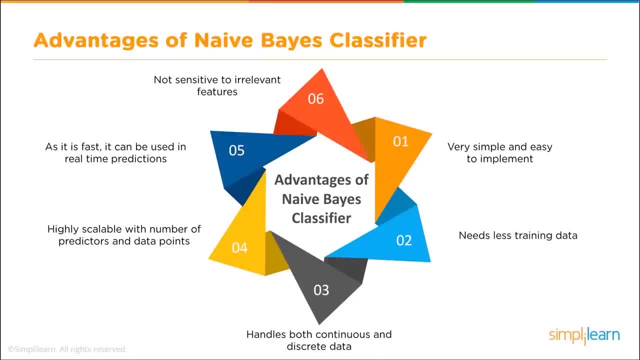 on one probability, you can kind of it automatically adjusts for that. those formulas are very automatic and so you can still get a very solid predictability, even if you're missing data or you have overlapping data for two completely different areas. we see that a lot in doing census. 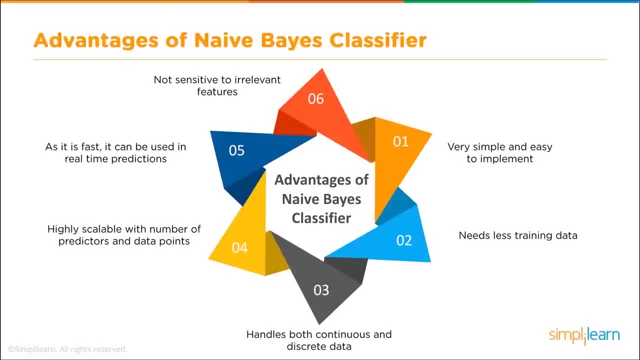 and studying of people and habits, where they might have one study that covers one aspect, another one that overlaps, and because the two overlap, they can then predict the unknowns for the group that they haven't done the second study on or vice versa. so it's not sensitive to the irrelevant features. 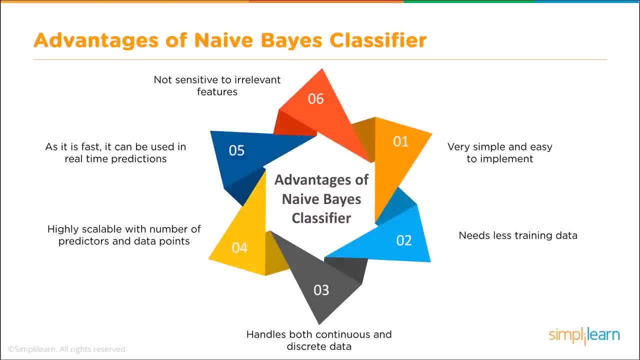 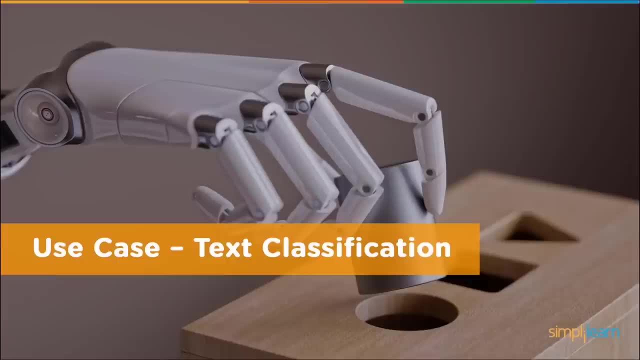 and in fact, you can use it to help predict features that aren't even in there. so now we're down to my favorite part. we're going to roll up our sleeves and do some actual programming. we're going to do the use case text classification. now I would challenge you to go back. 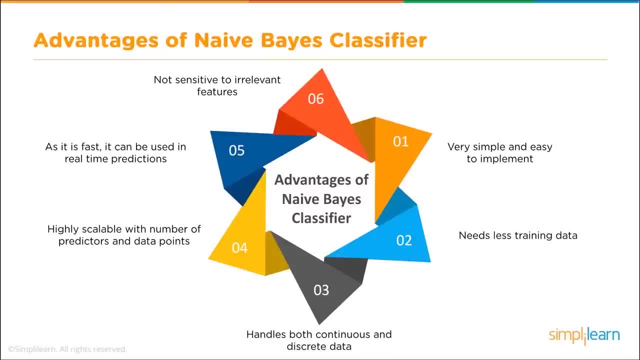 So it picks up on your different probabilities and if you're short on data on one probability, you can kind of it automatically adjusts for that. Those formulas are very automatic and so you can still get a very solid predictability, even if you're missing data or you have overlapping data. 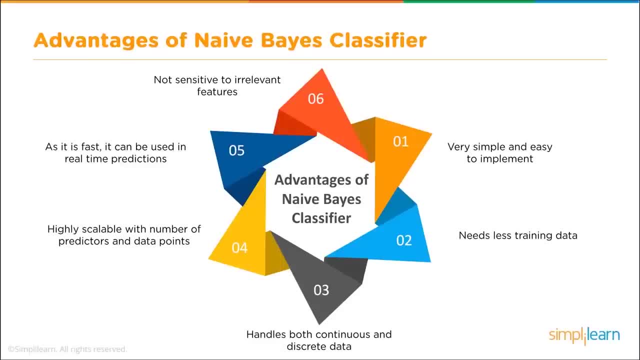 for two completely different areas. We see that a lot in doing census and studying of people and habits, where they might have one study that covers one aspect, another one that overlaps, and because the two overlap, they can then predict the unknowns for the group. 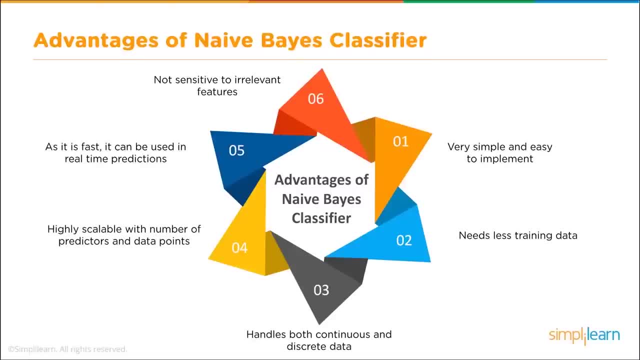 that they haven't done the second study on, or vice versa. So it's very powerful in that it is not sensitive to the irrelevant features and in fact, you can use it to help predict features that aren't even in there. So now we're down to my favorite part. 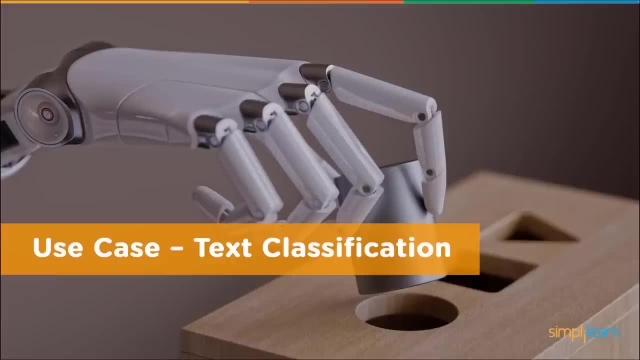 We're going to roll up our sleeves and do some actual programming. We're going to do the use case text classification. Now I would challenge you to go back and send us a note on the notes below underneath the video and request the data for the shopping cart. 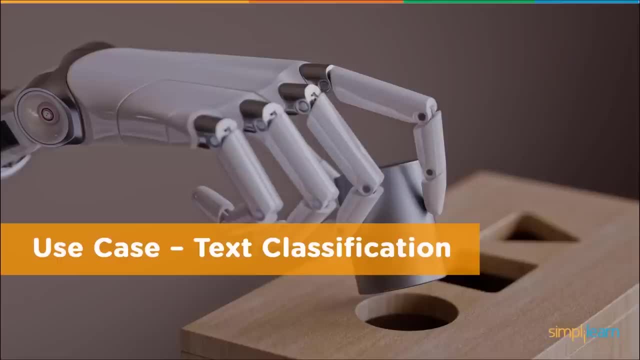 So you can plug that into Python code and do that on your own time so you can walk through it, Since we walked through all the information on it. But we're going to do a Python code doing text classification- very popular for doing the naive bays. 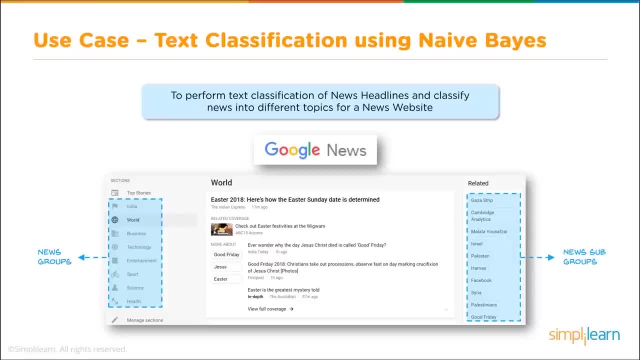 So we're going to use our new tool to perform a text classification of news headlines and classify news into different topics for a news website. As you can see here we have a nice image of the Google News and then related on the right subgroups. 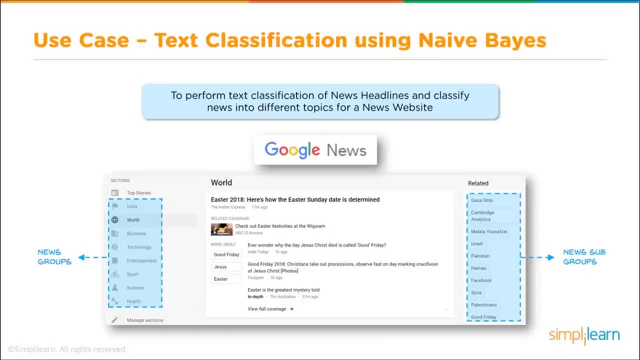 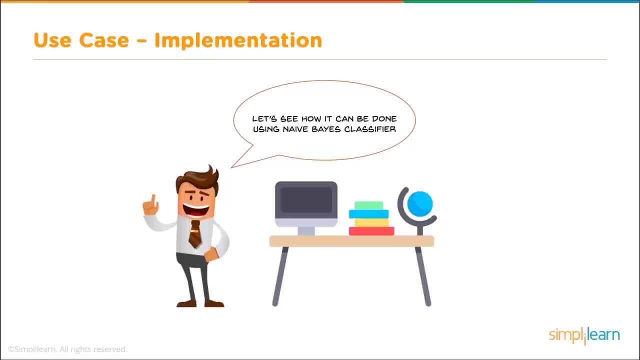 I'm not sure where they actually pulled the actual data we're going to use from. It's one of the standard sets, But certainly this can be used on any of our news headlines and classification. So let's see how it can be done using the naive bays classifier. 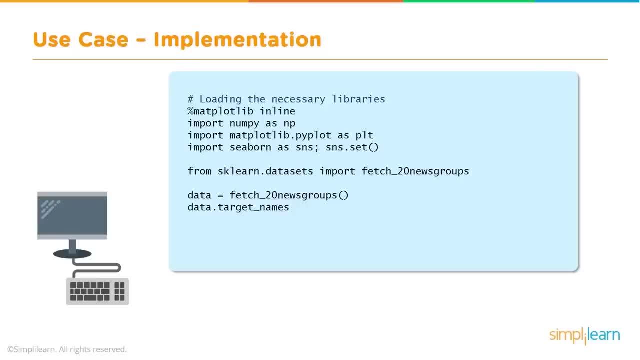 Now we're at my favorite part. We're actually going to write some Python script. Roll up our sleeves And we're going to start by doing our imports. These are very basic imports, including our news group, And we'll take a quick glance at the target names. 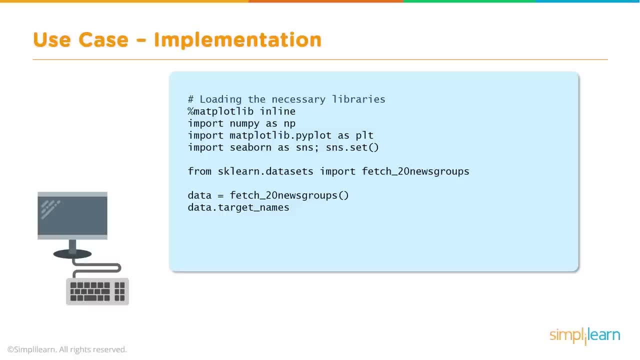 Then we're going to go ahead and start training our data set and putting it together. We'll put together a nice graph, because it's always good to have a graph to show what's going on. And once we've trained it and we've shown you a graph, 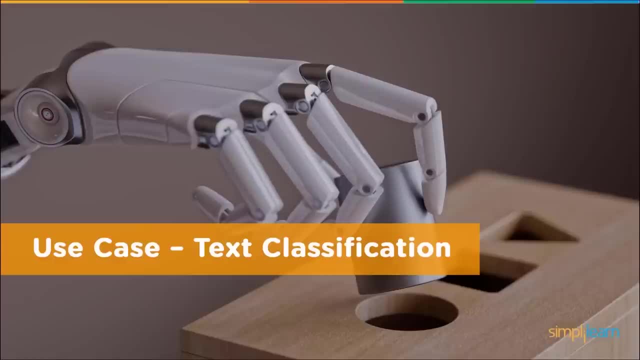 and send us a note on the notes below underneath the video and request the data for the shopping cart. so you can plug that into Python code and do that on your own time so you can walk through it, since we walked through all the information on it, but we're going to do a Python code. 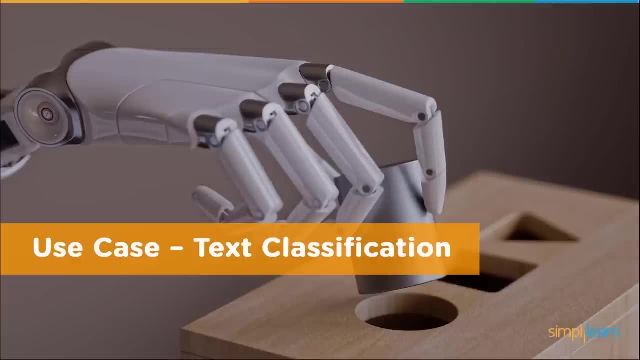 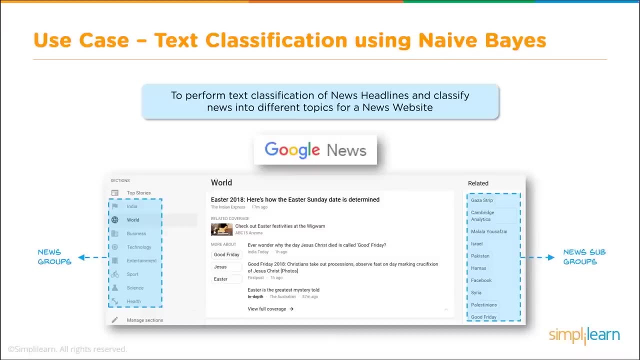 doing text classification, very popular for doing the naive bays. so we're going to use our new tool to perform a text classification of news headlines and classify news into different topics for a news website. as you can see here, we have a nice image of the Google News. 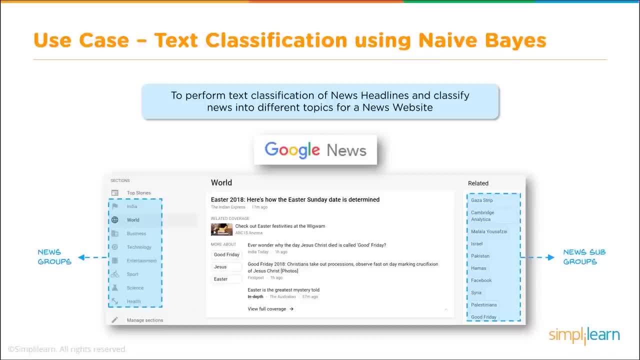 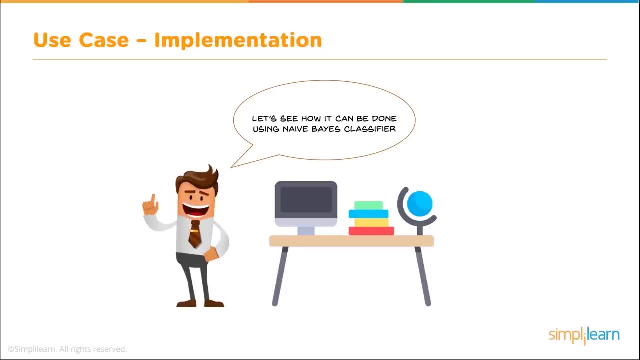 and then related on the right subgroups. I'm not sure where they actually pulled the actual data we're going to use from. it's one of the standard sets, so let's see how it can be done using the naive bays classifier. now we're at my favorite part. 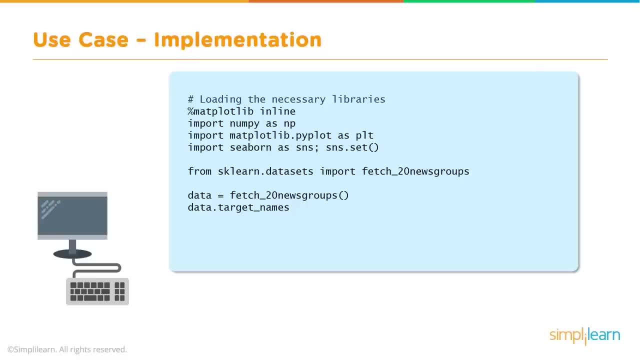 we're actually going to write some Python script, roll up our sleeves and we're going to start by doing our imports. these are very basic imports, including our news group, and we'll take a quick glance at the target names. then we're going to go ahead and start training our data set. 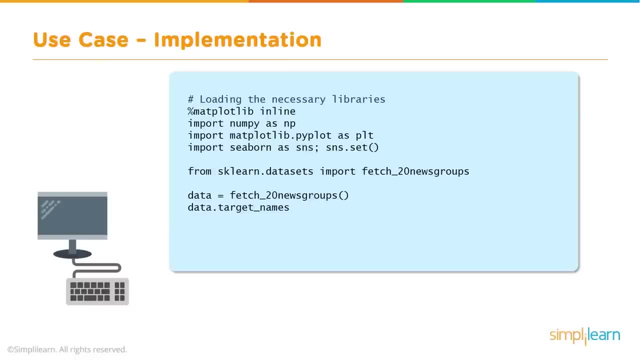 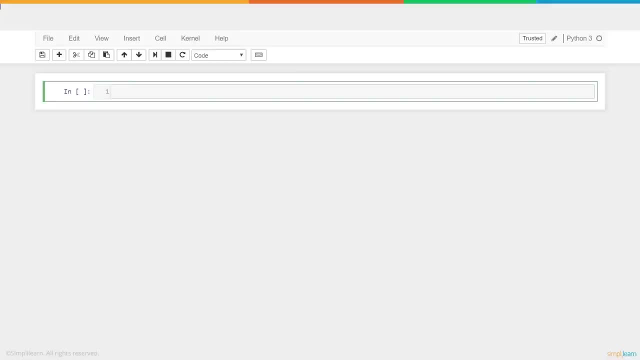 and putting it together. we'll put together a nice graph, because it's always good to have a graph to show what's going on. and once we've trained it and we've shown you a graph of what's going on, that's what it looks like. now I'm going to open up my favorite editor. 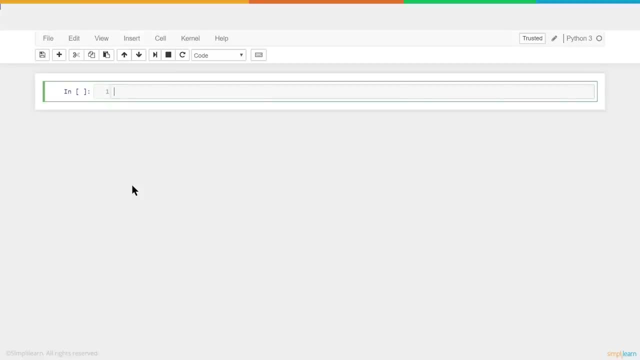 or inline editor for Python. you don't have to use this. you can use whatever your editor that you like, whatever interface IDE you want. this just happens to be the Anaconda Jupyter notebook and I'm going to paste that first piece of code in here so we can walk through it. 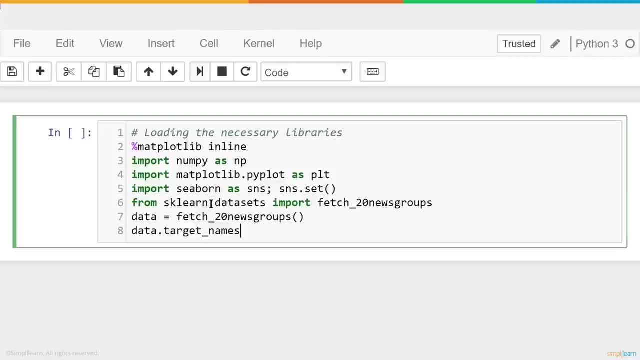 let's make it a little bigger on the screen so you have a nice view of what's going on. and we're using Python 3, in this case 3.5, so this would work in any of your 3x if you have it set up correctly. 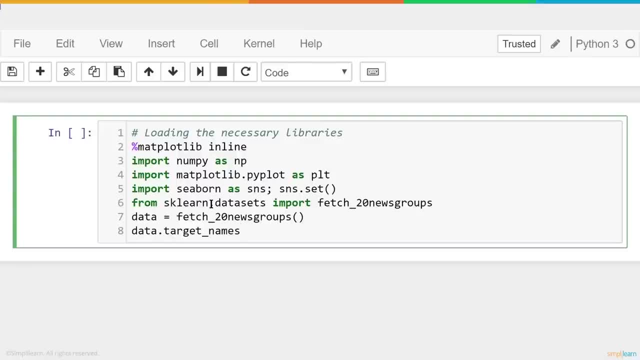 or 2x. you just have to make sure all of the versions of the modules match your Python version and in here you'll notice. the first line is your percentage matplotlibrary inline. now, three of these lines of code are all about plotting the graph. this one: 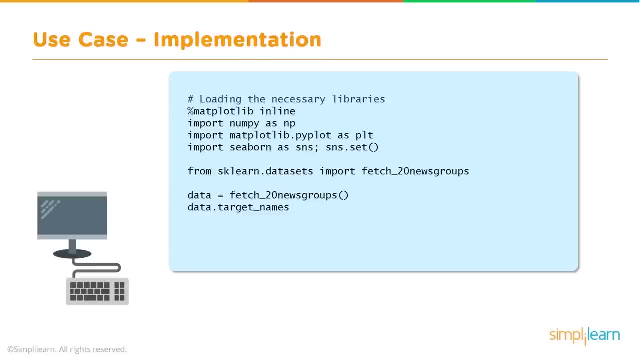 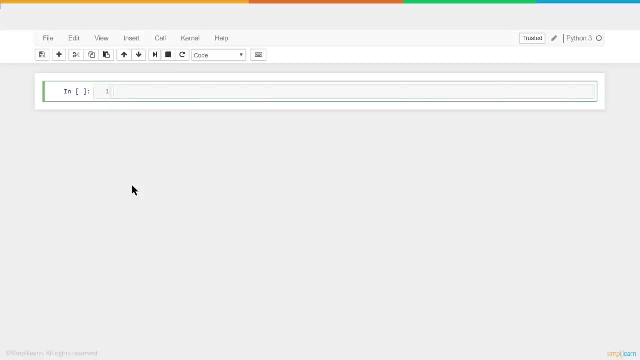 of what's going on, then we're going to explore how to use it and see what that looks like. Now I'm going to open up my favorite editor: inline editor for Python. You don't have to use this. You can use whatever your editor that you like. 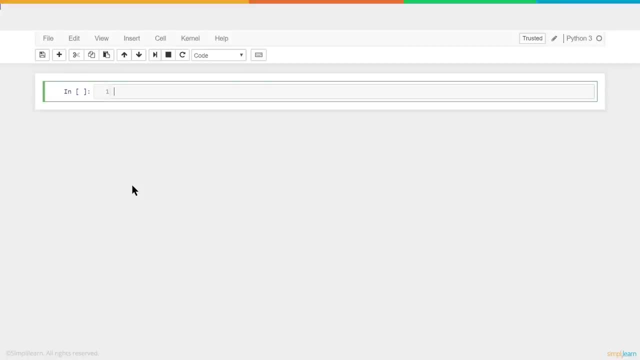 whatever interface IDE you want. This just happens to be the Anaconda Jupyter notebook And I'm going to paste that first piece of code in here so we can walk through it And let's make it a little bigger on the screen so you have a nice view of what's going on. 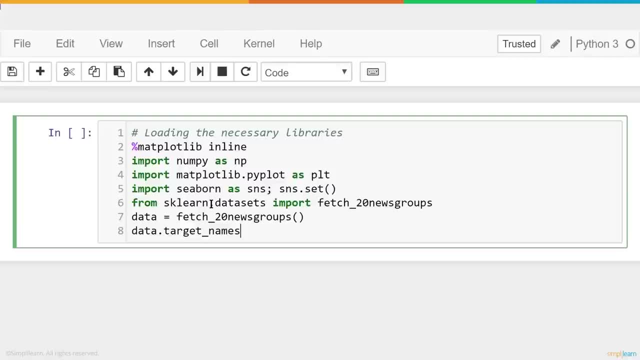 And we're using Python 3, in this case 3.5. So this would work in any of your 3X. If you have it set up correctly, it should also work in a lot of the 2X. You just have to make sure all of the versions. 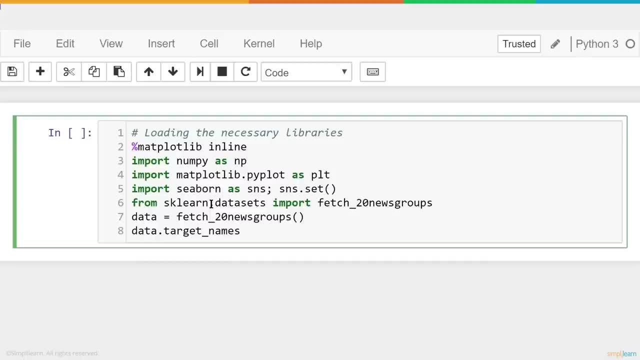 of the modules match your Python version And in here you'll notice. the first line is your percentage matplotlibrary inline. Now three of these lines of code are all about plotting the graph. This one lets the notebook notes- and this is an inline setup- that we want the graphs. 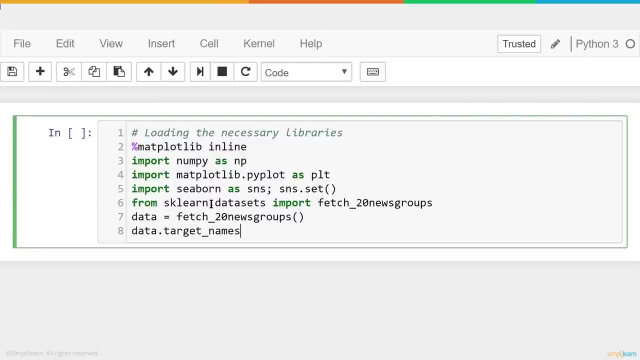 to show up on this page. Without it, in a notebook like this, which is an explorer interface, it won't show up. Now, a lot of IDEs don't require that. A lot of them like if I'm working on one of my other setups. 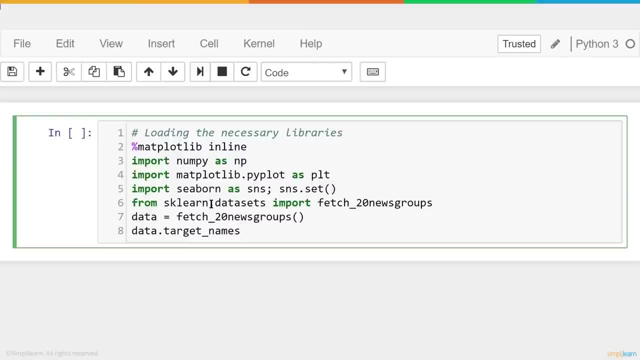 it just has a popup and the graph pops up on there. So you have that setup also. But for this we want the matplotlibrary inline And then we're going to import numpy as np, That's number Python, which has a lot of different formulas. 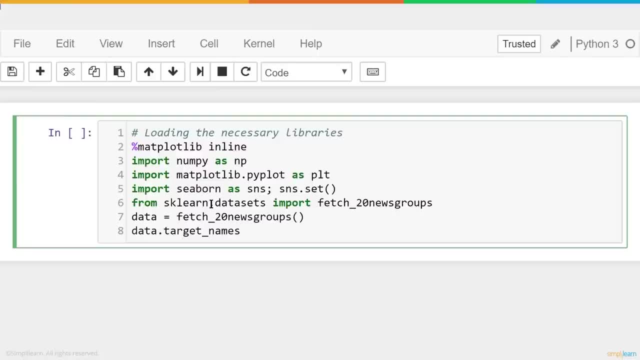 in it that we use for both of our sklearn module And we also use it for any of the upper math functions in Python and it's very common to see that as np, numpy as np. The next two lines are all about our graphing. 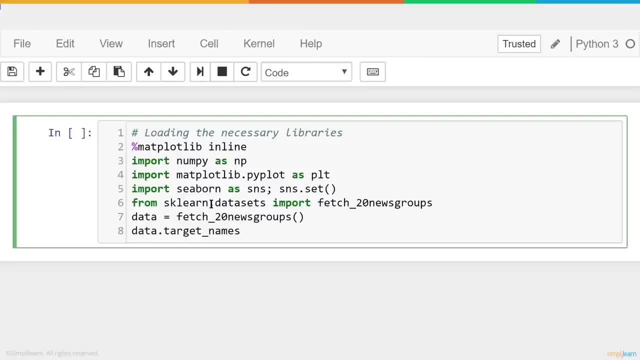 Remember I said three of these were about graphing. Well, we need our matplotlibrarypyplot as plt, And you'll see that plt is a very common setup, as is the sns, and just like the np, And we're going to import sklearn as sns. 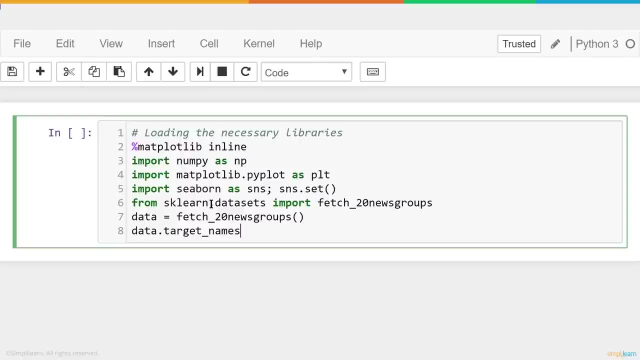 and we're going to do the snsset Now. sklearn sits on top of pyplot and it just makes a really nice heat map. It's really good for heat maps And if you're not familiar with heat maps, that just means we give it a color scale. 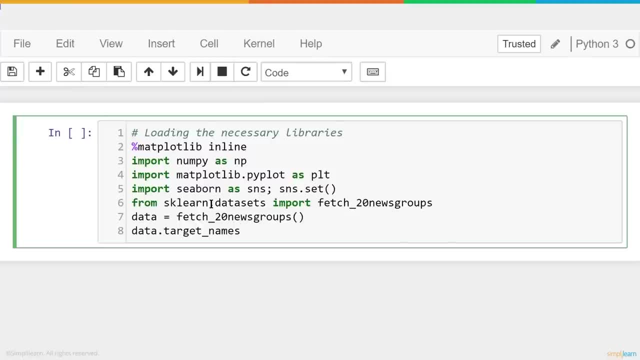 The term comes from the brighter red, it is the hotter. it is in some form of data And you can set it to whatever you want And we'll see that later on. So you'll see that those three lines of code here are just importing the graph function so we can graph it. 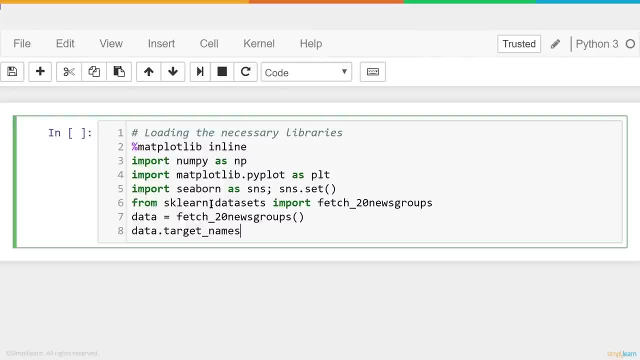 lets the notebook notes inline setup that we want the graphs to show up on this page. without it, in a notebook like this, which is an explorer interface, it won't show up. now, a lot of IDEs don't require that. a lot of them like if I'm working on one of my other setups. 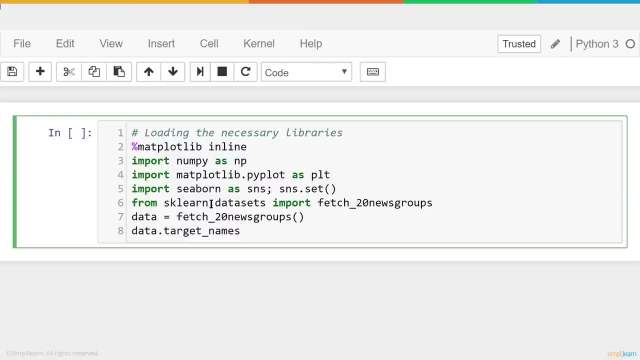 it just has a popup and the graph pops up on there. so you have that setup also. but for this we want the matplotlibrary inline, and then we're going to import numpy as np, that's number Python, which has a lot of different formulas in it that we use for both of our sklearn module. 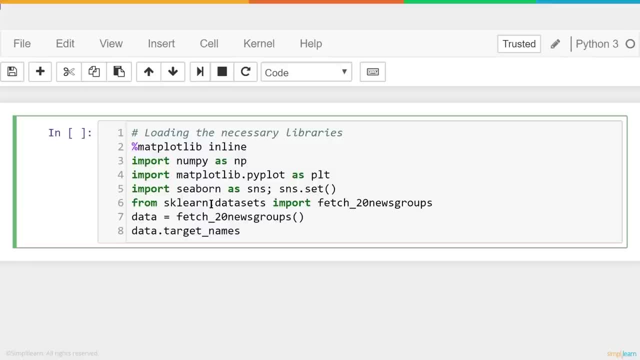 and we also use it for any of the upper math functions in Python and it's very common to see that as np, numpy as np. the next two lines are all about our graphs. remember I said three of these were about graphing. well, we need our matplotlibrarypyplot. 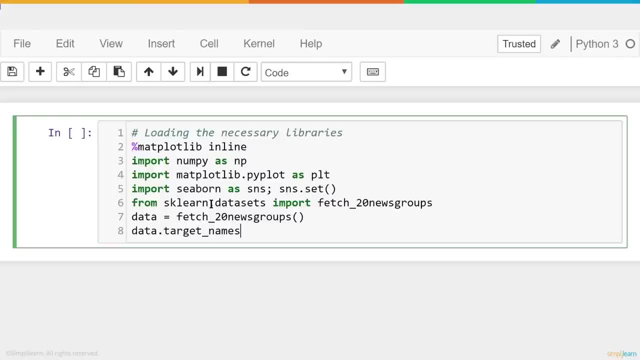 as plt, and you'll see that plt is a very common setup, as is the sns and just like the np, and we're going to import sklearn as sns and we're going to do the snsset. now sklearn sits on top of pyplot and it just makes a really nice heatmap. 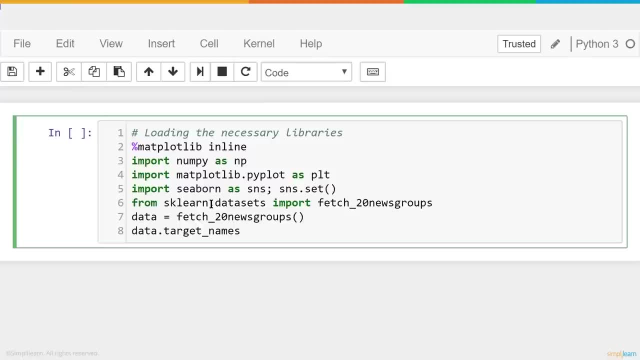 it's really good for heatmaps and if you're not familiar with heatmaps, that just means we give it a color scale. the term comes from the brighter red. it is in some form of data and you can set it to whatever you want, and we'll see that later on. 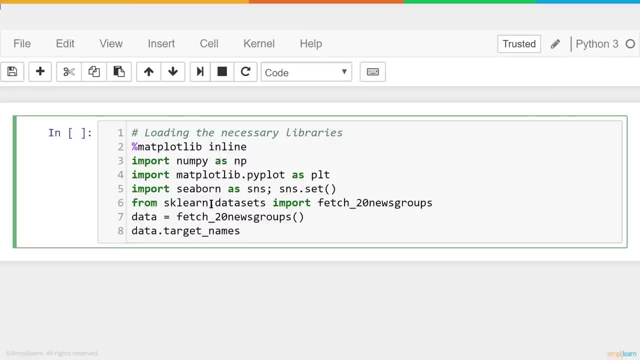 so you'll see that those three lines of code here are just importing the graph function so we can graph it, and as a data scientist, you always want to graph your data and have some kind of visual. it's really hard just to shove numbers in front of people. 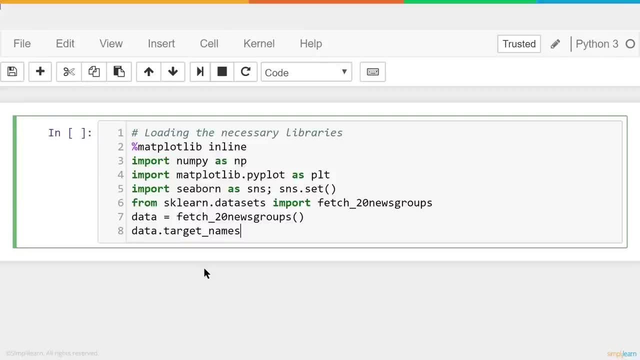 and they look at it and it doesn't mean anything. and then from the sklearndatasets we're going to import the fetch20newsgroups- very common one- for analyzing, tokenizing words and setting them up and exploring how the words work and how do you categorize different things. 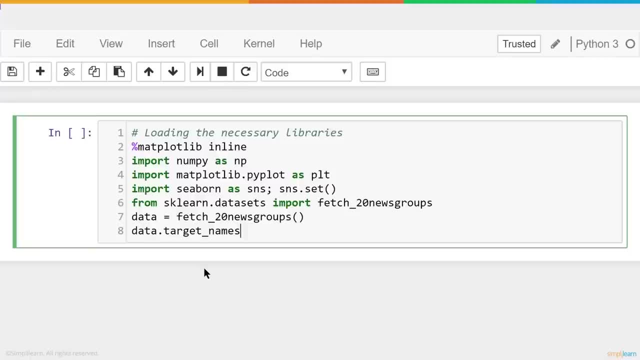 when you're dealing with documents, and then we set our data equal to fetch20newsgroups, so our data variable will have the data in it and we're going to go ahead and just print the target names- datatargetnames- and let's see what that looks like. 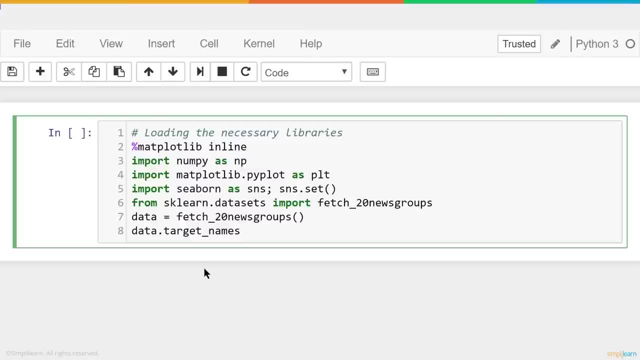 And as a data scientist, you always want to graph your data and have some kind of visual. It's really hard just to shove numbers in front of people and they look at it and it doesn't mean anything. And then from the sklearndatasets. 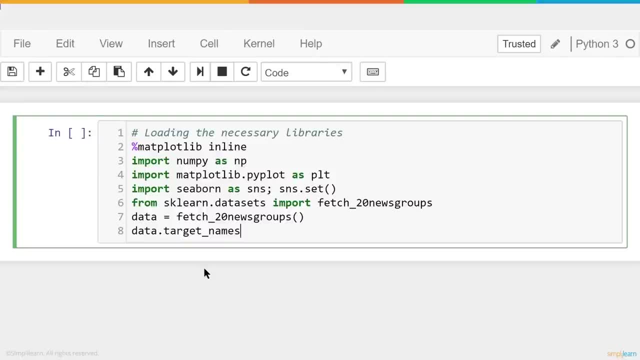 we're going to import the fetch20 newsgroups- a very common one for analyzing, tokenizing words and setting them up and exploring how the words work and how do you categorize different things when you're dealing with documents- And then we set our data equal to fetch20 newsgroups. 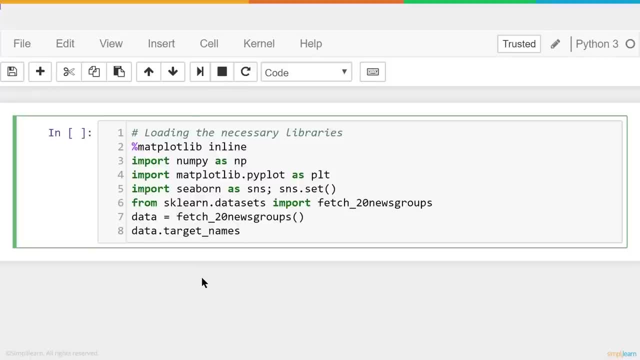 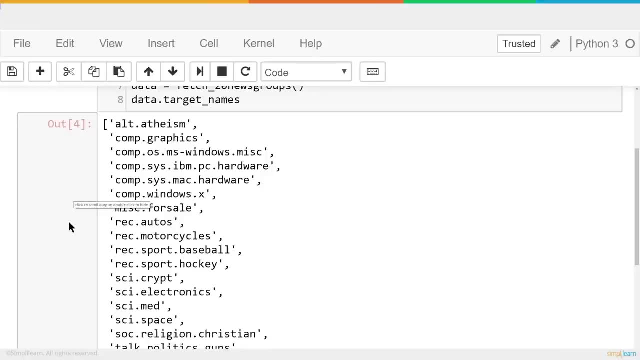 So our data variable will have the data in it And we're going to go ahead and just print the target names- datatargetNames- And let's see what that looks like, And you'll see. here we have altAtheism- compGraphics- compOsMSWindowsMiscellaneous. 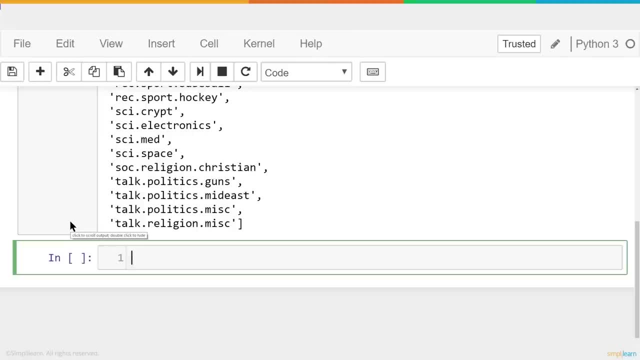 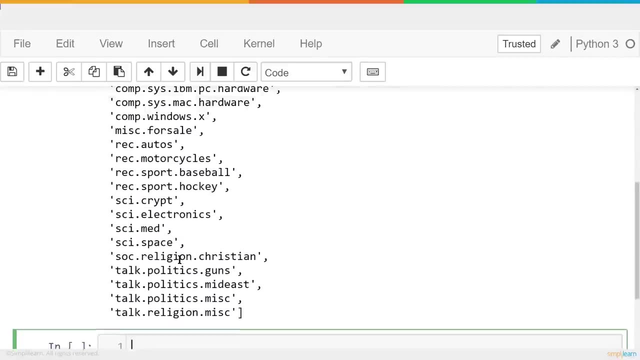 And it goes all the way down to talkPoliticsMiscellaneous, talkReligionMiscellaneous. These are the categories they've already assigned to this newsgroup And it's called fetch20 because, you'll see, there's- I believe there's- 20 different topics in here. 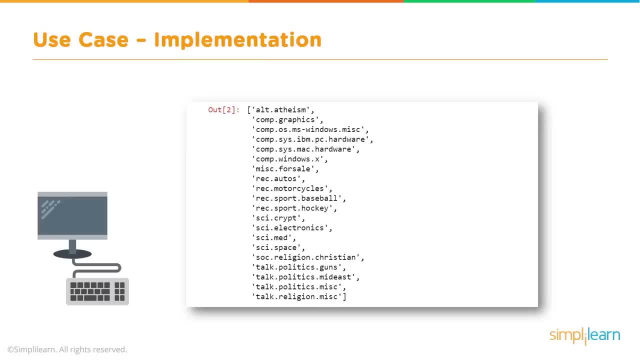 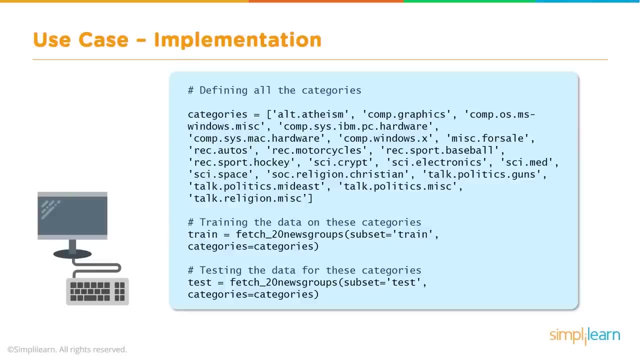 or 20 different categories as we scroll down. Now we've gone through the 20 different categories and we're going to go ahead and start defining all the categories and set up our data. So we're actually in here going to go ahead. 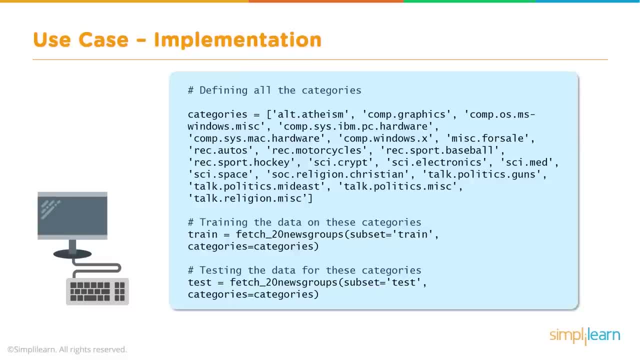 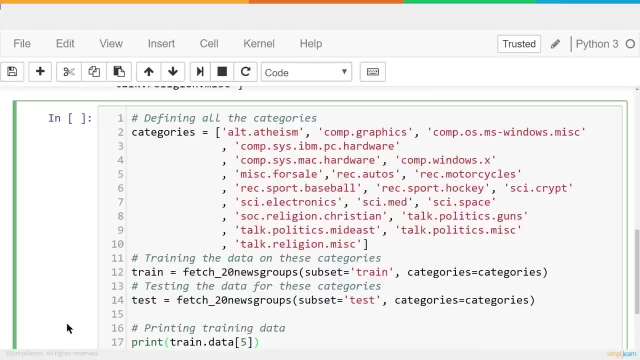 and get the data all set up and take a look at our data And let's move this over to our Jupyter Notebook And let's see what this code does. First, we're going to set our categories. Now, if you noticed up here, I could have just as easily. 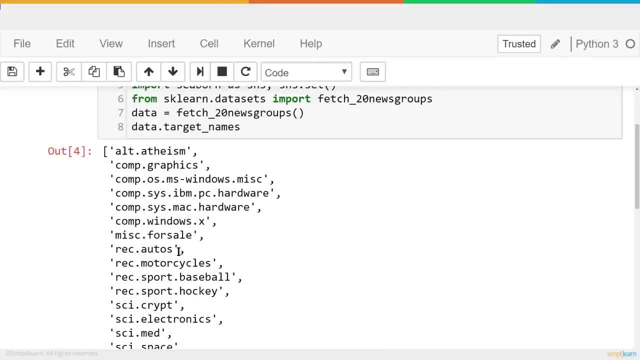 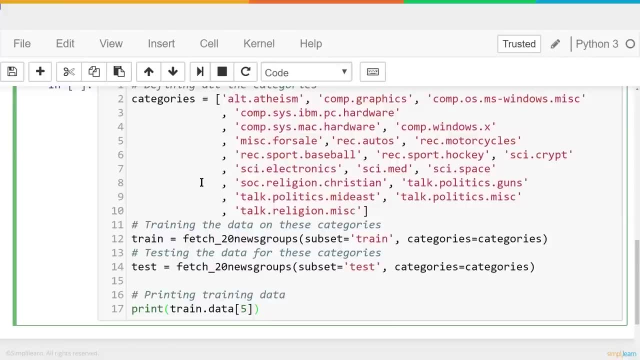 set this equal to datatarget underscore names, because it's the same thing, But we want to kind of spell it out for you so you can see the different categories. It kind of makes it more visual so you can see what your data's looking like in the background. 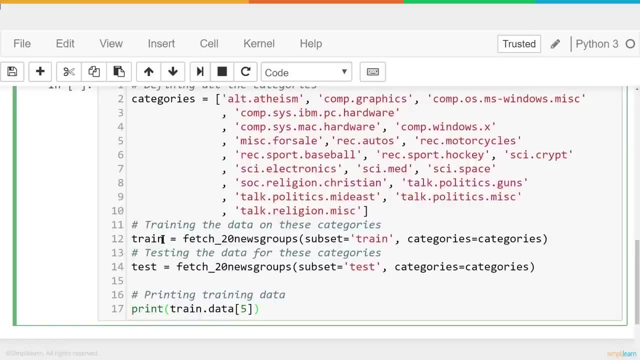 Once we've created the categories, we're going to open up a train set. So this training set of data is going to go into fetch20 newsgroups and it's a subset in there called train And categories equals categories. So we're pulling out those categories that match. 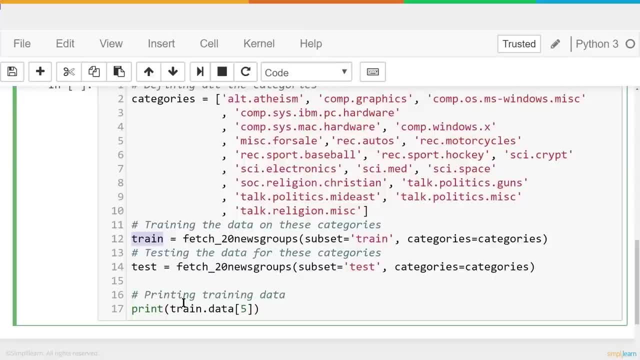 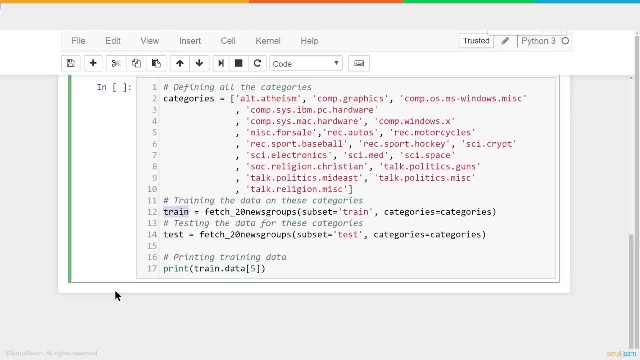 And then if you have a train set, you should also have the testing set. We have test equals fetch20, newsgroups, subset equals test and categories equals categories. Let's go down one size so it all fits on my screen. There we go. 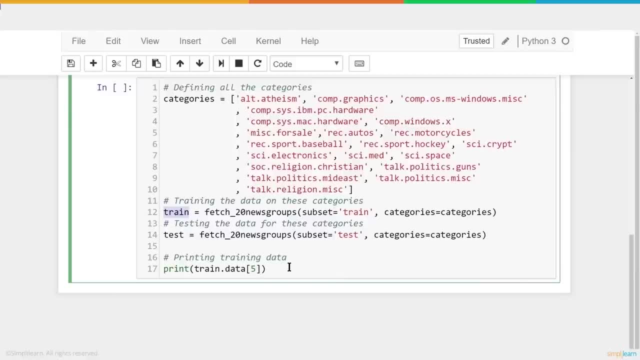 And just so we can really see what's going on, let's see what happens when we print out one part of that data. So it creates train And under train it creates traindata. And we're just going to look at data piece number five. 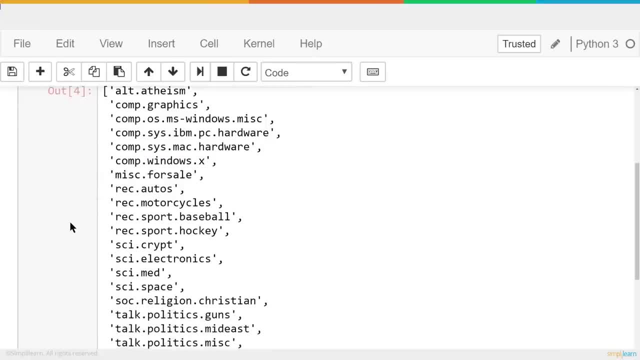 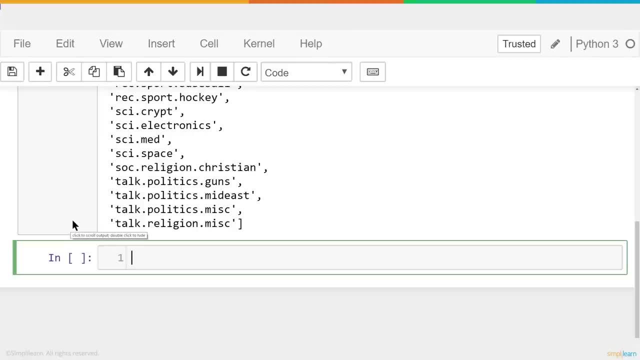 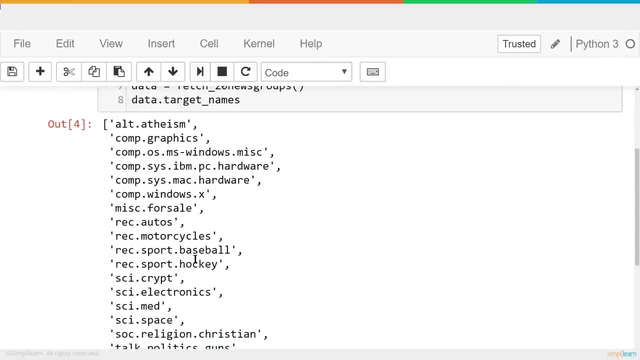 and you'll see, here we have alt atheism, comp graphics, comp os, ms windowsmiscellaneous, and it goes all the way down to talkpoliticsmiscellaneous, talkreligionmiscellaneous. these are the categories they've already assigned to this newsgroup and it's called fetch20 because you'll see. 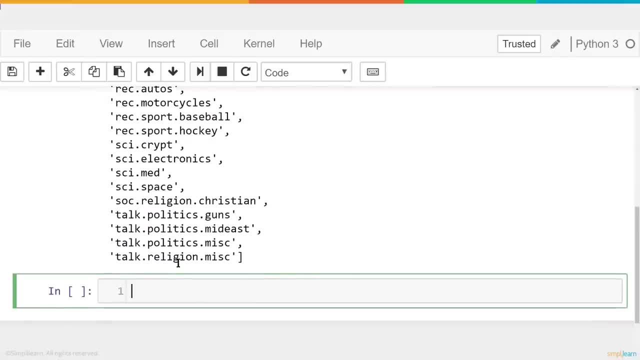 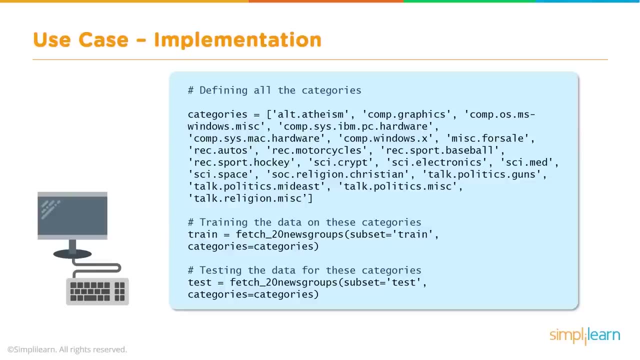 I believe there's 20 different topics in here, or 20 different categories as we scroll down. now we've gone through the 20 different categories and we're going to go ahead and start defining all the categories and set up our data. so we're actually going to go ahead and 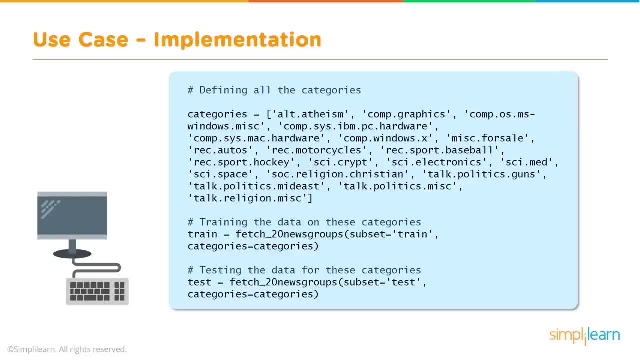 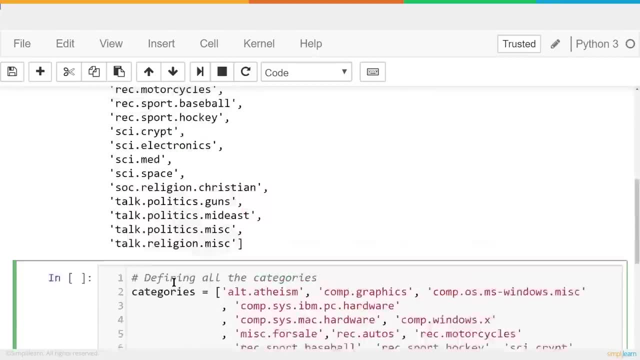 get the data all set up and take a look at our data, and let's move this over to our jupyter notebook and let's see what this code does. first, we're going to set our categories now. if you noticed up here, I could have just as easily used this. 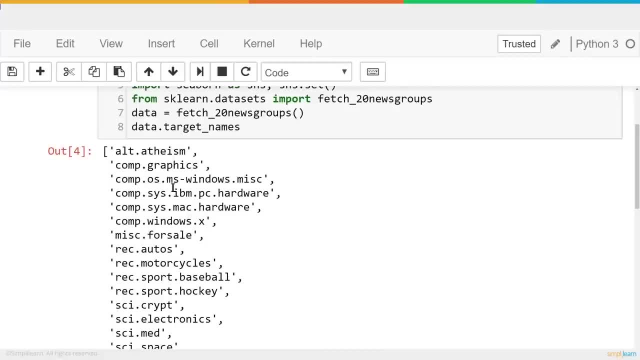 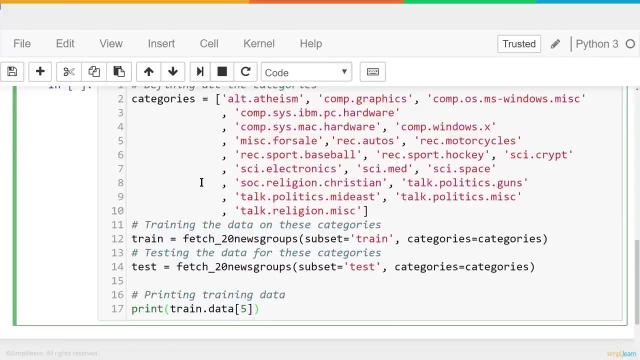 we set this equal to datatarget underscore names, because it's the same thing, but we want to kind of spell it out for you so you can see the different categories. it kind of makes it more visual so you can see what your data is looking like in the background. 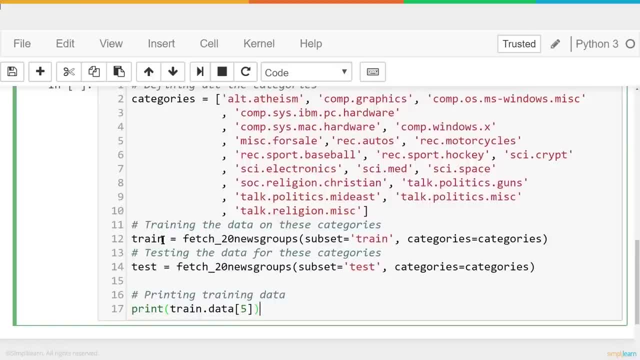 once we've created the categories, we're going to open up a train set. so this training set of data is going to go into fetch20 newsgroups and it's a subset in there called train and categories equals categories. so we're pulling out those categories that match. 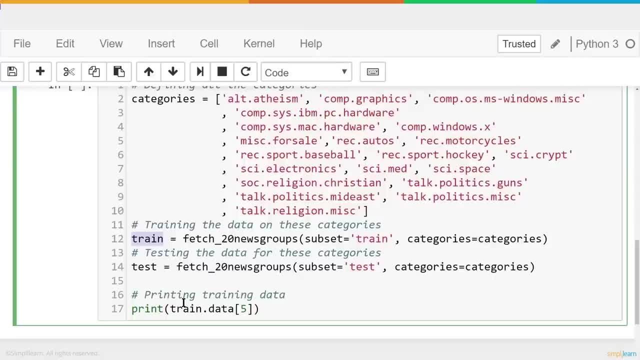 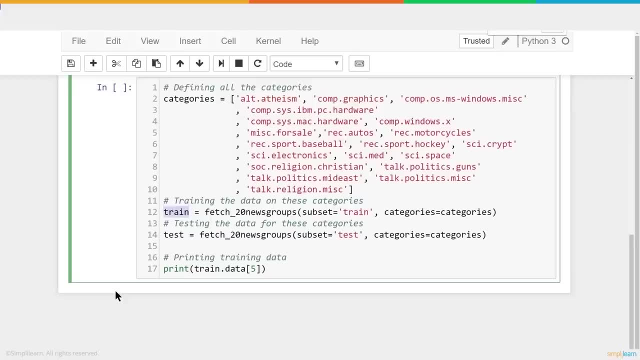 and then, if you have a train set, you could also have the testing set. we have test equals fetch20, newsgroups, subset equals test and categories equals categories. let's go down one size so it all fits on my screen and just so we can really see what's going on. 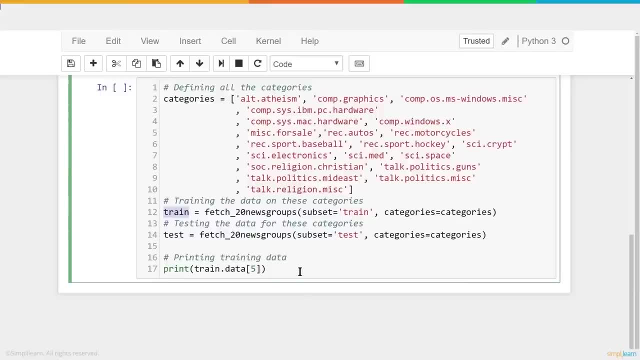 let's see what happens when we print out one part of that data. so it creates train and under train it creates traindata. and we're just going to look at data piece number 5 and let's go ahead and run that and see what that looks like. 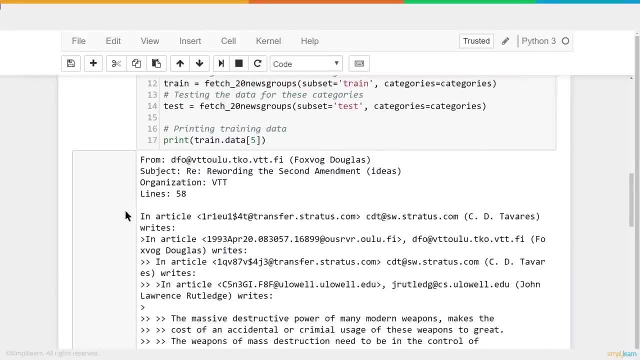 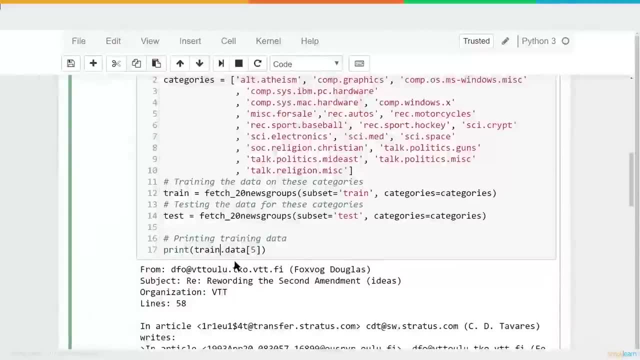 and you can see when I print traindata number 5 under train, it prints out one of the articles. this is article number 5. you can go through and read it on there and we can also go in here and change this to test, which should look identical. 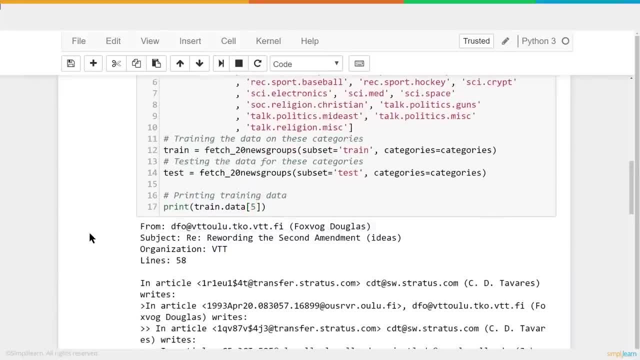 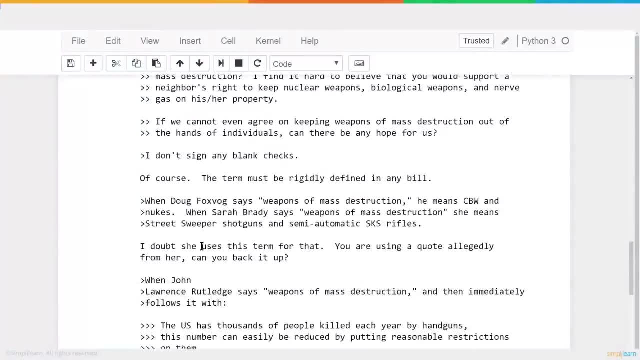 And let's go ahead and run that and see what that looks like. And you can see when I print traindata number five under train it prints out one of the articles. This is article number five. You can go through and read it on there. 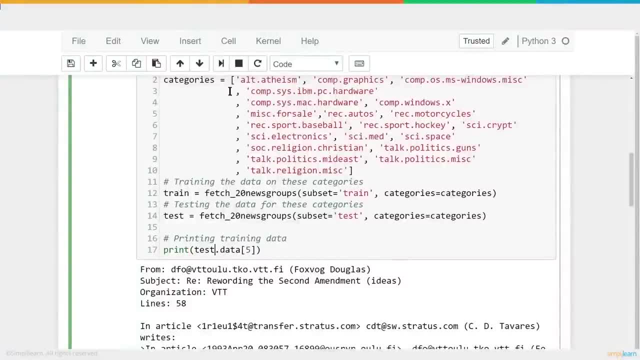 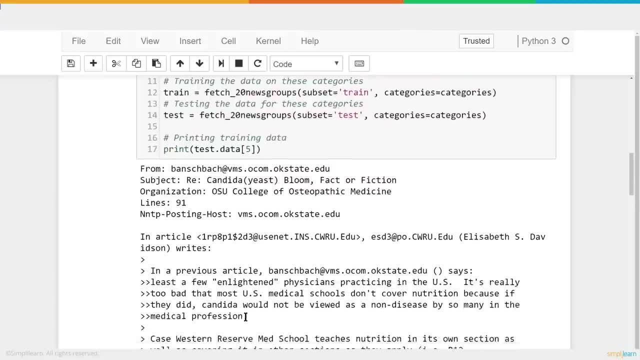 And we can also go in here and change this to test, which should look identical because it's splitting the data up into different groups. train and test And we'll see test. number five is a different article, but it's another article in here. 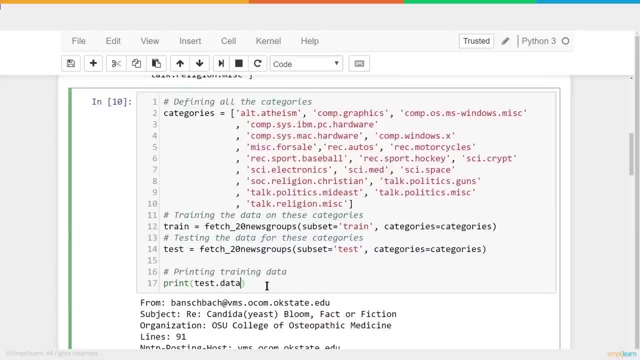 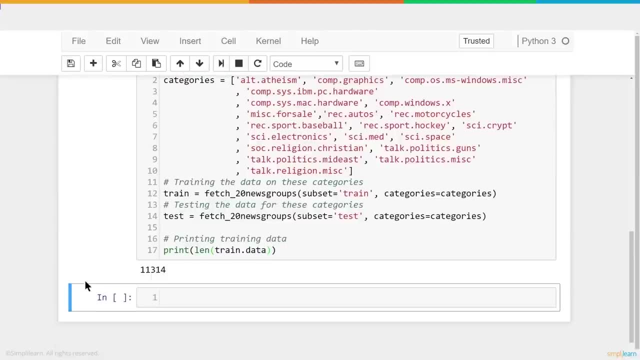 And maybe you're curious and you want to see just how many articles are in here. We could do length of train Traindata And if we run that you'll see that the training data has 11,314 articles. So we're not going to go through all those articles. 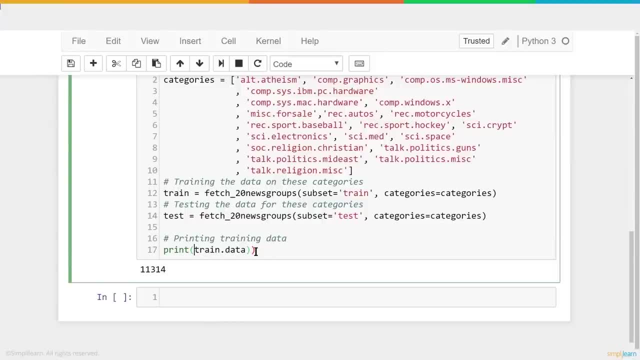 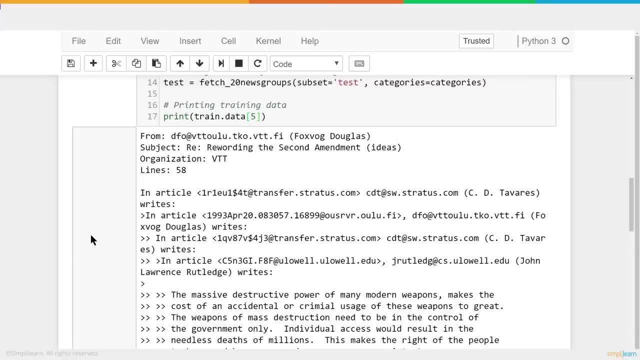 That's a lot of articles, But we can look at one of them just so you can see what kind of information is coming out of it and what we're looking at. And we'll just look at number five for today. And here we have it, rewording the Second Amendment, IDs. 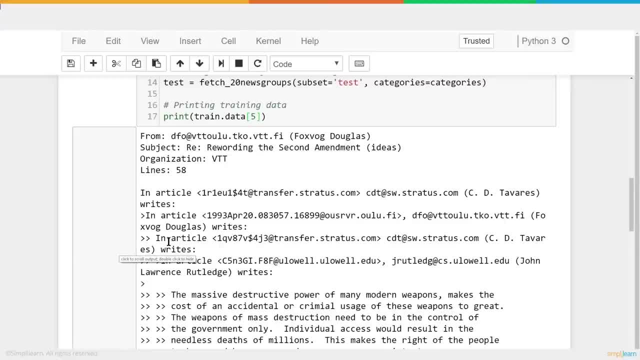 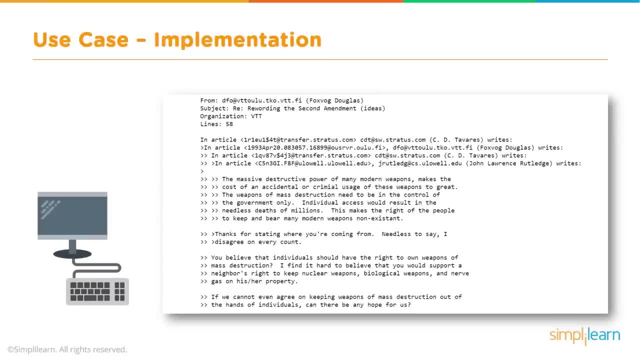 VTT, line 58, lines 58 in article, et cetera, And you can scroll all the way down and see all the different parts to there. Now we've looked at it and that's pretty complicated when you look at one of these articles. 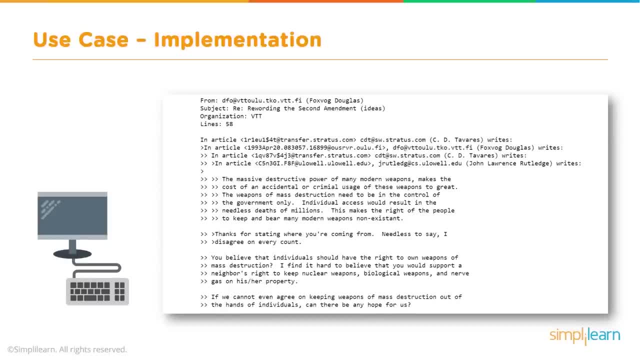 to try to figure out. how do you weight this. If you look down here, we have different words and maybe the word from, Well from- is probably in all the articles, so it's not going to have a lot of meaning. as far as trying to figure out whether this article fits, 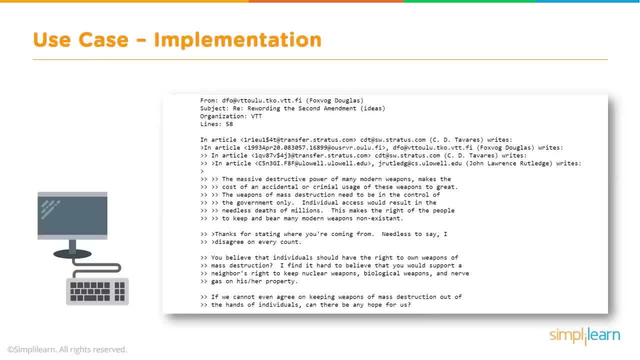 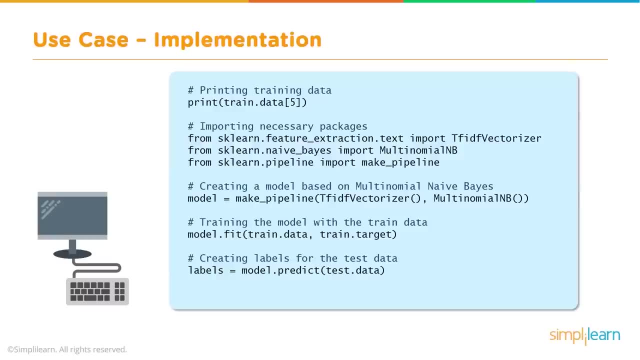 one of the categories or not. So trying to figure out which category it fits in based on these words is where the challenge comes in. Now that we've viewed our data, we're going to dive in and do the actual predictions. This is the actual naive base. 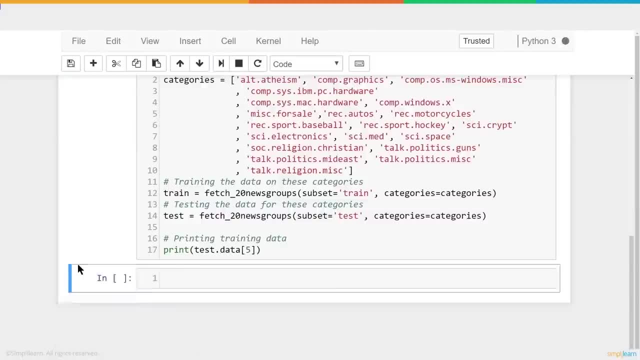 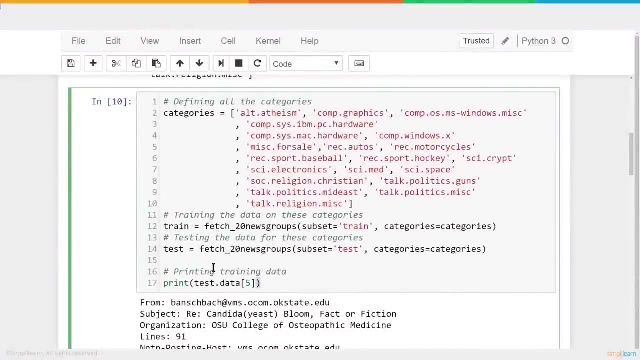 because it's splitting the data up into different groups- train and test- and we'll see test. number 5 is a different article, but it's another article in here and maybe you're curious and you want to see just how many articles are in here. we could do. 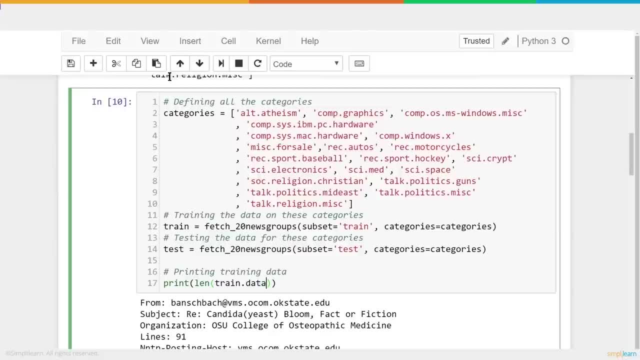 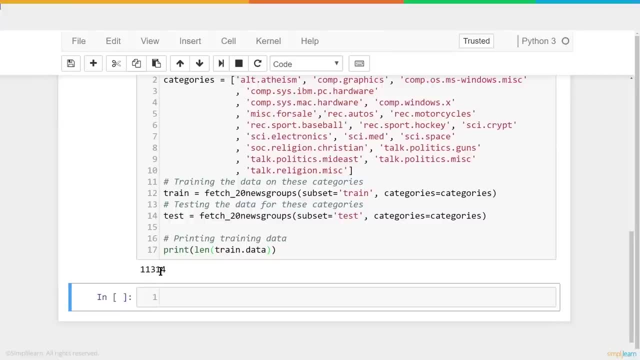 length of train dot data and if we run that, you'll see that the training data has 11,314 articles. so we're not going to go through all those articles. that's a lot of articles, but we can look at one of them just so you can see what kind of 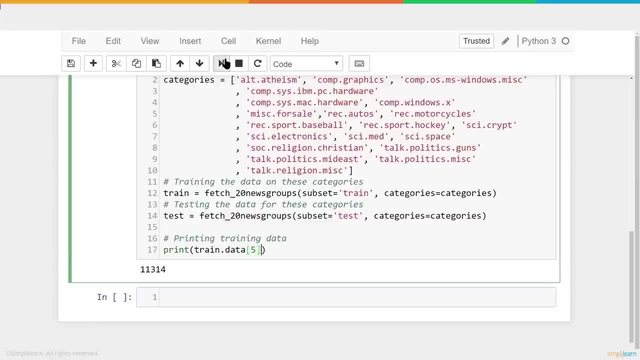 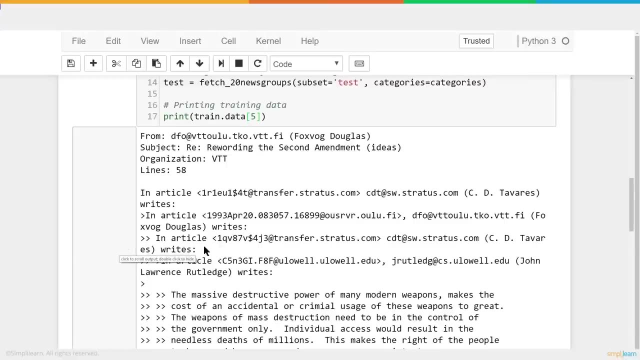 information is coming out of it and what we're looking at. and we'll just look at number 5 for today. and here we have it, rewording the second amendment, ids vtt, line 58, lines 58 in article, etc. and you can scroll all the way down and see all the different parts to there. 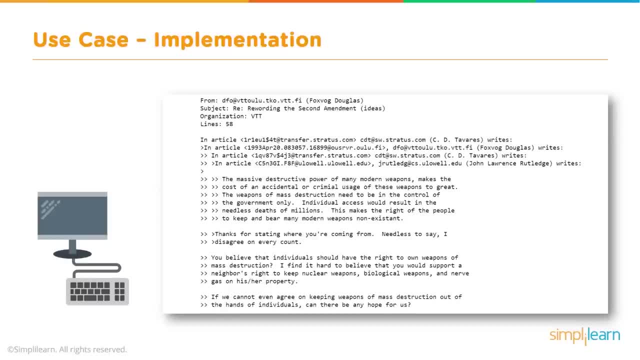 now, we've looked at it and that's pretty complicated when you look at one of these articles to try to figure out. how do you weight this? if you look down here, we have different words and maybe the word from, well from- is probably in all the articles. 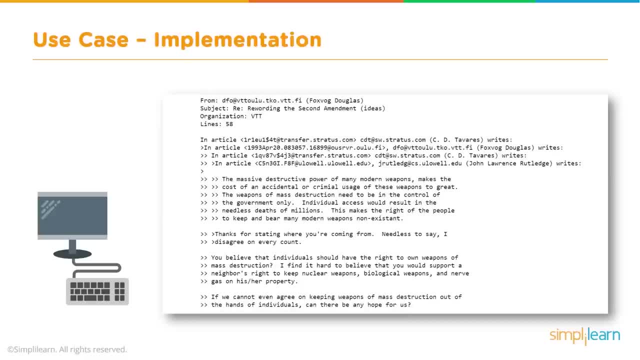 so it's not going to have a lot of meaning as far as trying to figure out whether this article fits one of the categories or not. so trying to figure out which category it fits in based on these words is where the challenge comes in, now that we've viewed our data. 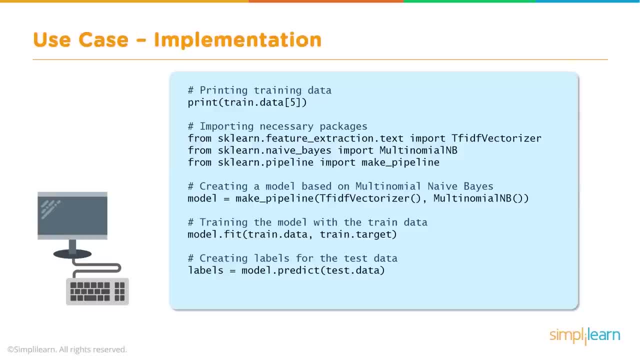 we're going to dive in and do the actual predictions. this is the actual naive base and we're going to throw another model at you or another module at you here in just a second. we can't go into too much detail, but it deals specifically working with words and text. 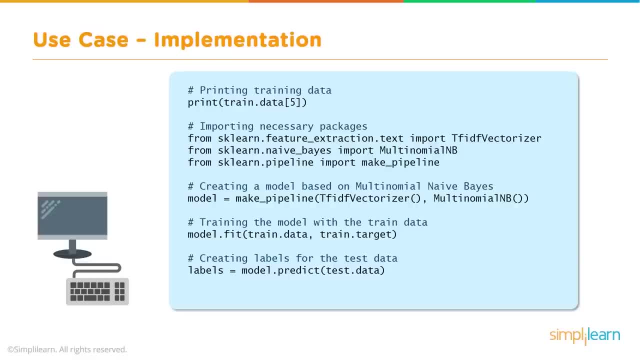 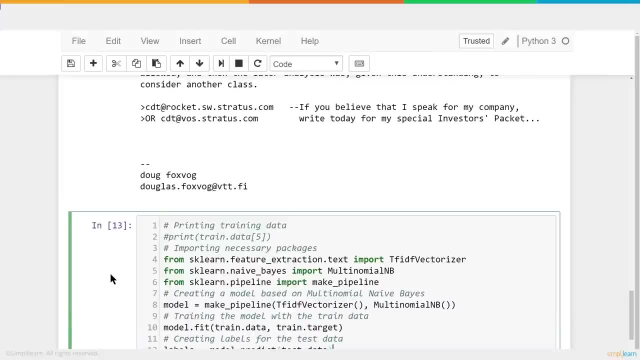 and what they call tokenizing those words. so let's take this code and let's skip on over to our Jupyter notebook and walk through it, and here we are in our Jupyter notebook. let's paste that in there and I can run this code right off the bat. it's not actually going to display. 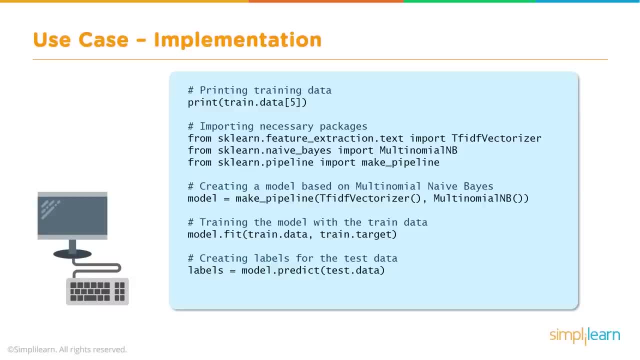 And we're going to throw another model at you or another module at you here in just a second. We can't go into too much detail, but it deals specifically working with words and text and what they call tokenizing those words. So let's take this code and let's skip on over. 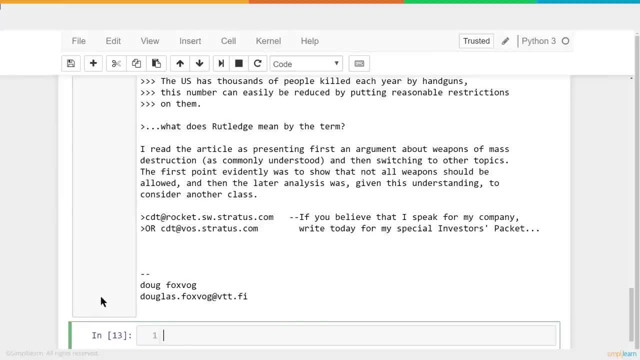 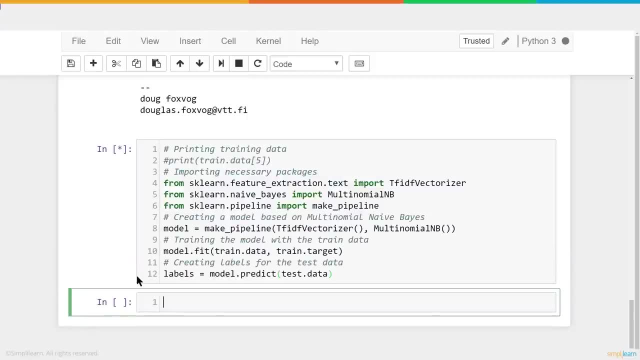 to our Jupyter notebook and walk through it And here we are in our Jupyter notebook. Let's paste that in there And I can run this code right off the bat. It's not actually going to display anything yet, but it has a lot going on in here. 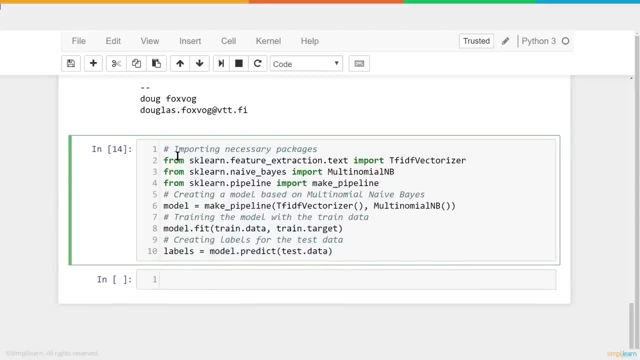 So the top, we had the print module from the earlier one. I didn't know why that was in there. We're going to start by importing our necessary packages And from the sklearnfeaturesextractiontxt we're going to import tfidfvectorizer. 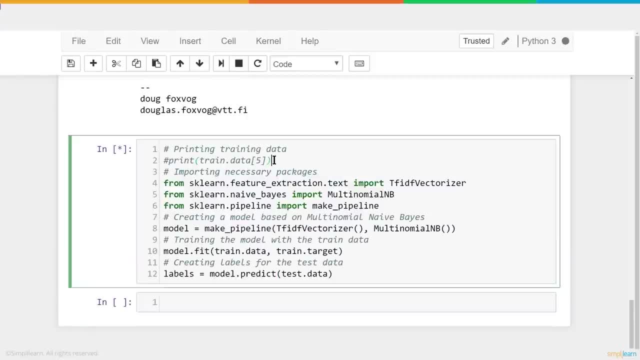 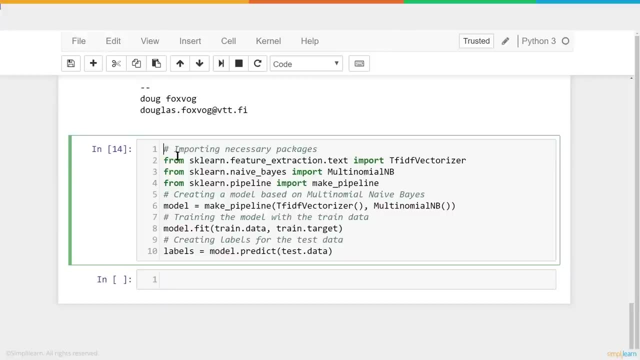 anything yet, but it has a lot going on in here. so the top we have the print module from the earlier one. I didn't know why that was in there. so we're going to start by importing our necessary packages and from the sklearn features extraction dot text we're going to import. 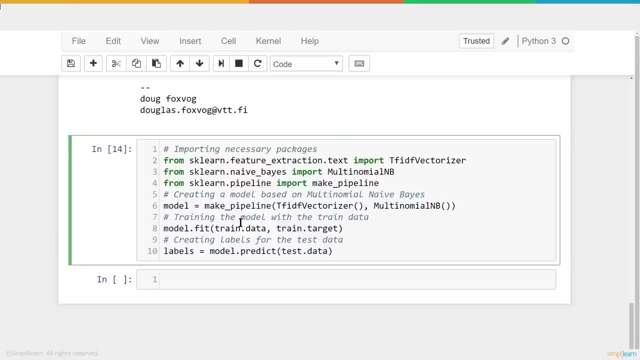 tf- idf vectorizer. I told you we're going to throw a module at you. we can't go too much into the math behind this or how it works. you can look it up. the notation for the math is usually tf, dot idf, and that's just a way. 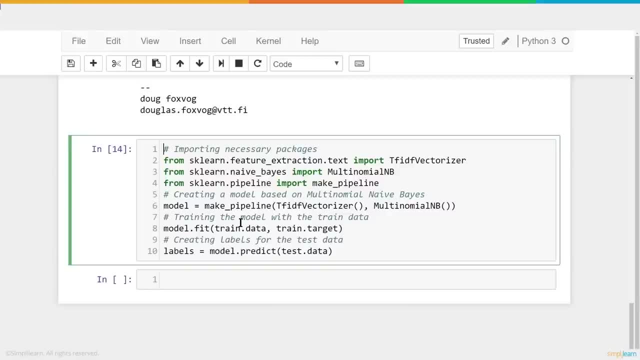 of weighing the words, and it weighs the words based on how many times they're used in a document, how many times or how many documents they're used in, and it's a well used formula. it's been around for a while. it's a little confusing to put this in here. 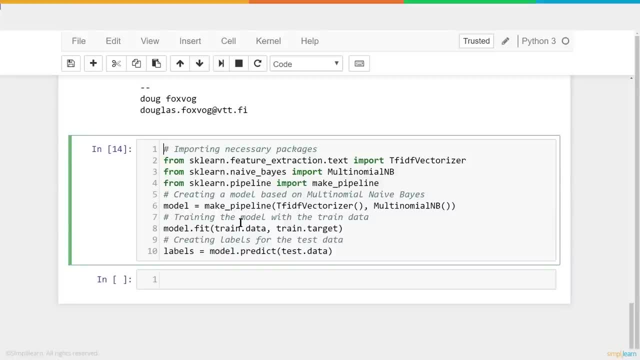 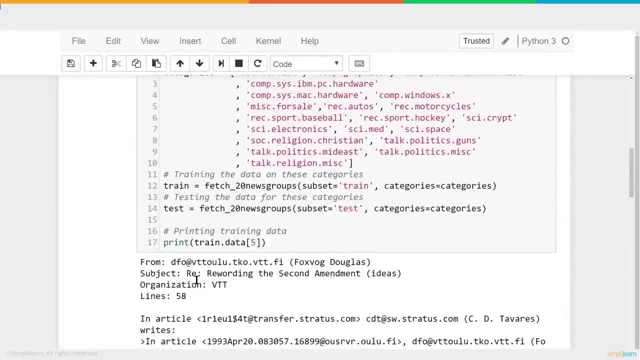 but let's let her know that it just goes in there and weights the different words in the document for us. that way we don't have to wait and if you put a weight on it- if you remember I was talking about that up here earlier- if these are all emails, they. 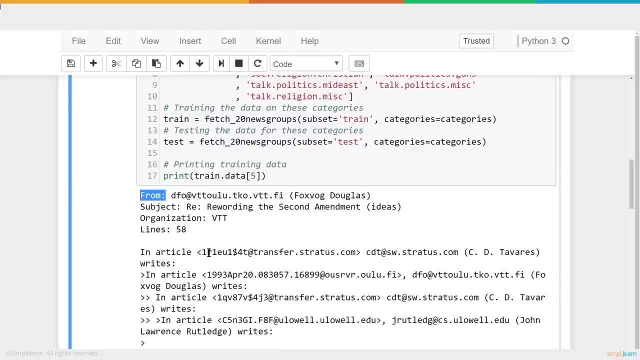 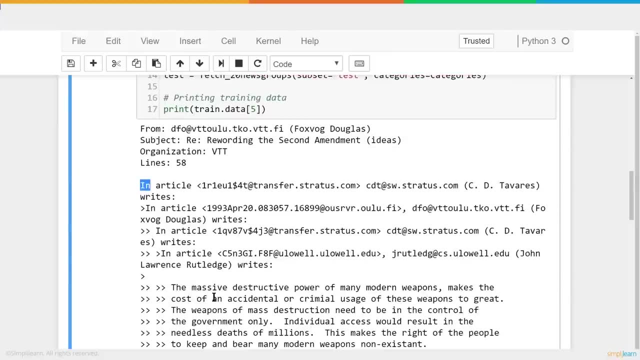 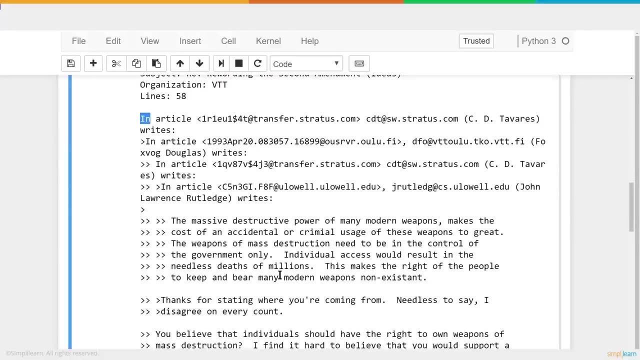 probably all have the word from in them. from probably has a very low weight. it has very little value in telling you what this document's about. same with words like in, in article, in articles in cost of un, maybe, cost, might, or where words like criminal weapons destruction, these might have. 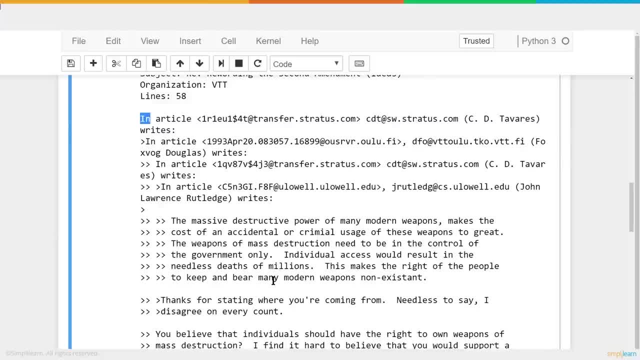 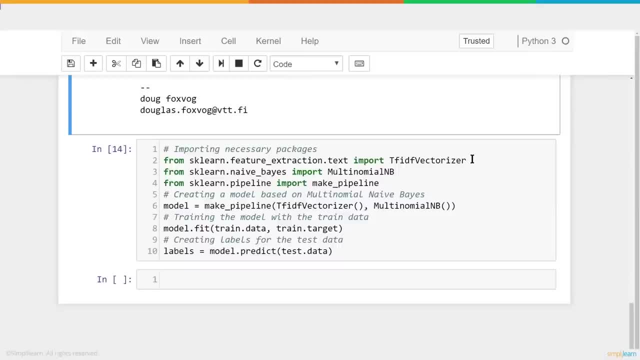 a heavier weight because they describe a little bit more what the article's doing. well, how do you figure out all those weights in the different articles? that's what this module does. that's what the tf idf vectorizer is going to do for us, and then we're going to import our sklearn dot. 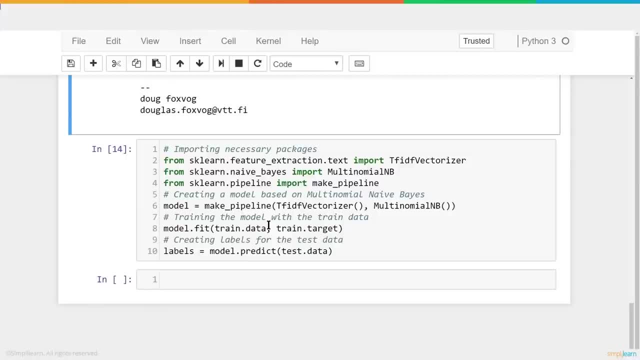 naive bays and that's our multinomial nb multinomial naive bays. pretty easy to understand that where that comes from. and then, finally, we have the skylearn pipeline, import make pipeline. now, the make pipeline is just a cool piece of code because we're going to take the information. 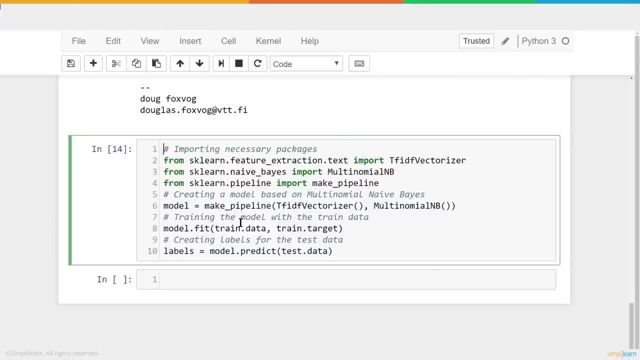 I told you we're going to throw a module at you. We can't go too much into the math behind this or how it works. You can look it up. The notation for the math is usually tfidf And that's just a way of weighing the words. 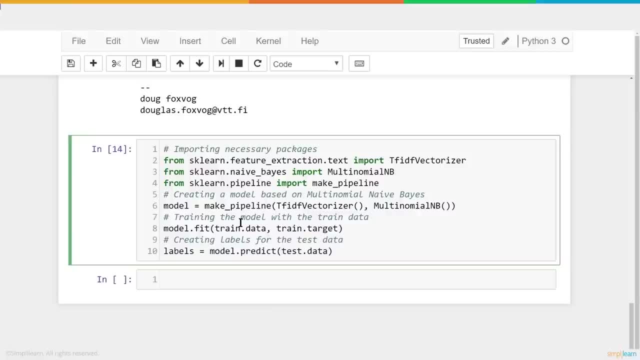 And it weighs the words based on how many times they're used in a document, how many times or how many documents they're used in, And it's a well-used formula. It's been around for a while. It's a little confusing to put this in here. 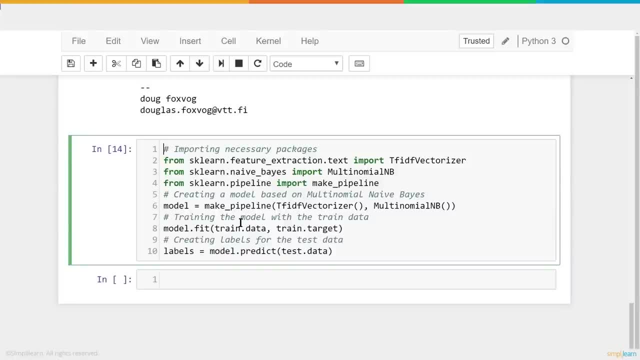 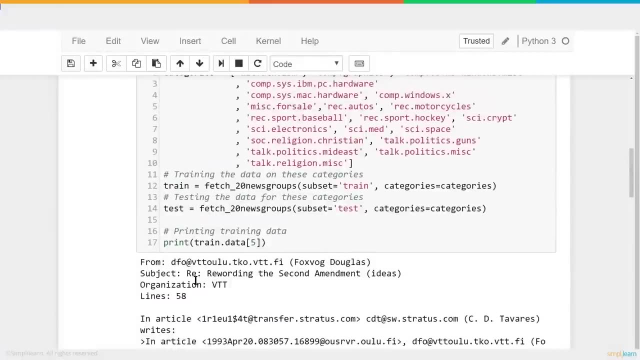 But let's let her know that it just goes in there and weights the different words in the document for us. That way we don't have to wait And if you put a weight on it- if you remember, I was talking about that up here earlier. 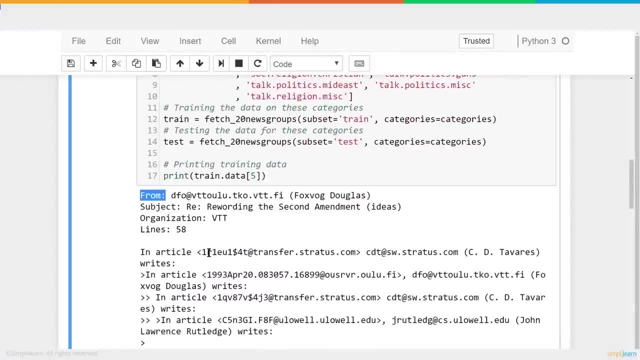 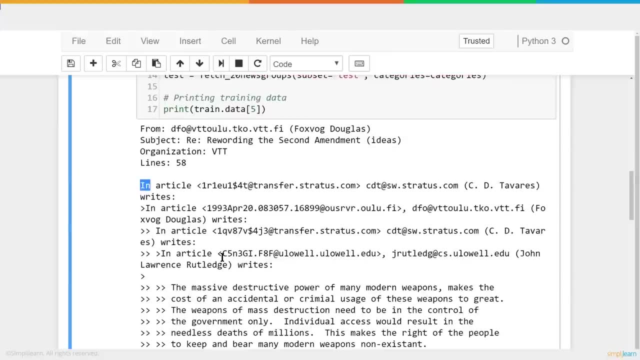 if these are all emails, they probably all have the word from in them. From probably has a very low weight. It has very little value in telling you what this document's about. Same with words like in, in article, in articles, in. 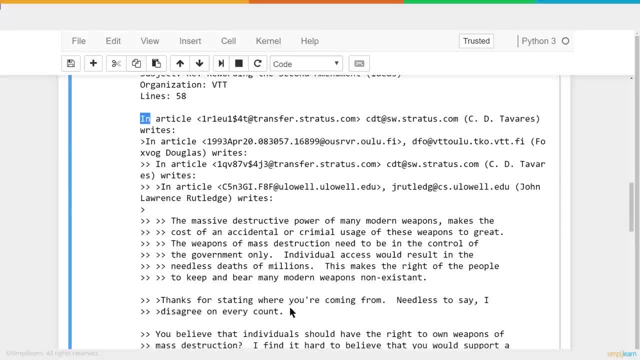 cost of on, maybe cost minus Right, Or where words like criminal weapons, destruction. these might have a heavier weight because they describe a little bit more what the article's doing. Well, how do you figure out all those weights in the different articles? 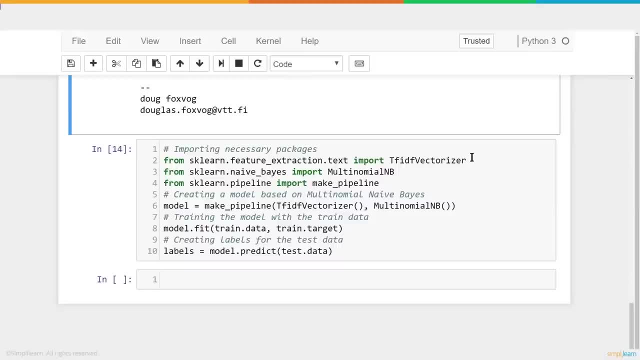 That's what this module does, That's what the TF-IDF vectorizer is going to do for us, And then we're going to import our sklearnnaivebase And that's our multinomial NB, Multinomial naive base. 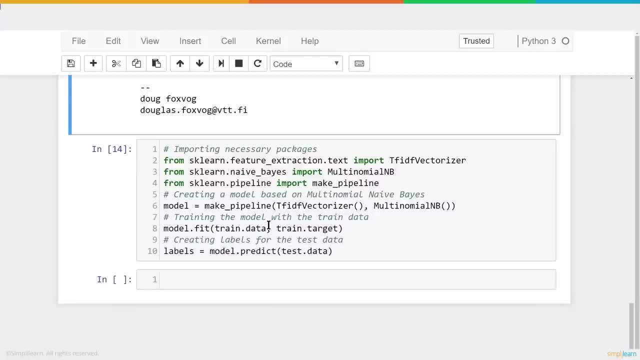 Pretty easy to understand that where that comes from. And then, finally, we have the sklearnnaivebase, A pipeline, import make pipeline. Now, the make pipeline is just a cool piece of code because we're going to take the information we get. 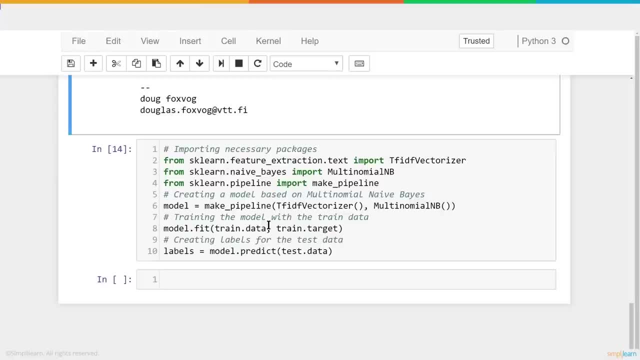 from the TF-IDF vectorizer and we're going to pump that into the multinomial NB. So a pipeline is just a way of organizing how things flow. It's used commonly. you probably already guessed what it is if you've done any businesses. 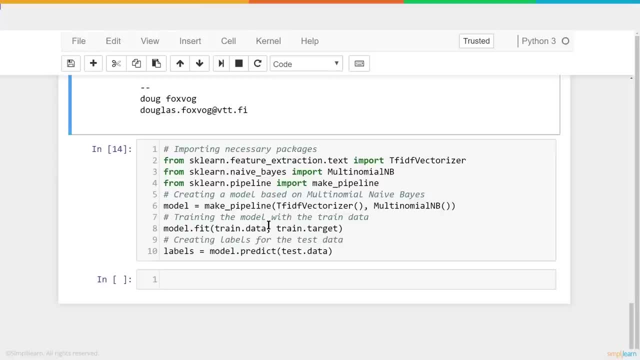 we get from the tf idf vectorizer and we're going to pump that into the multinomial nb. so a pipeline is just a way of organizing how things flow. it's used commonly. you probably already guessed what it is if you've done any businesses. they talk about the cells pipeline. 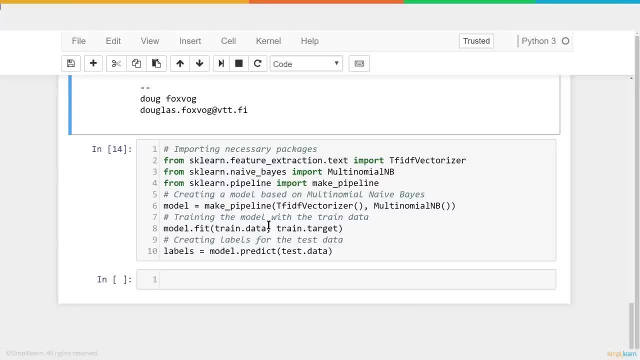 if you're on a work crew or project manager, you have your pipeline of information that's going through or your projects and what has to be done, in what order that's all this pipeline is. we're going to take the tf id vectorizer and then we're going to push that into the. 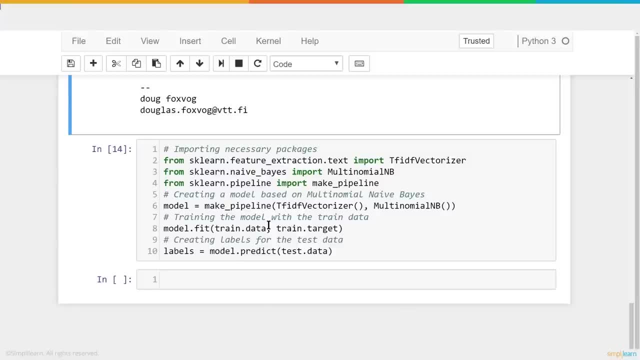 They talk about the sales pipeline. If you're on a work crew or a project manager, you have your pipeline of information. It's going through where your projects and what has to be done, in what order. That's all this pipeline is. We're going to take the TF-ID vectorizer. 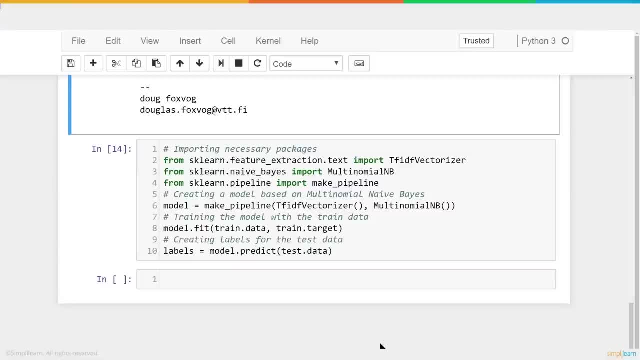 and then we're going to push that into the multinomial NB. Now we've designated that as the variable model. We have our pipeline model And we're going to take that model. And this is just so elegant. This is done in just a couple lines of code. 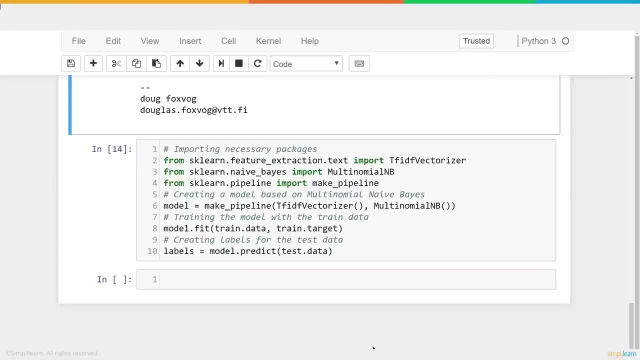 multinomial nb. now we've designated that as the variable model. we have our pipeline model and we're going to take that model. and this is just so elegant. this is done in just a couple lines of code. model dot fit and we're going to fit the data. 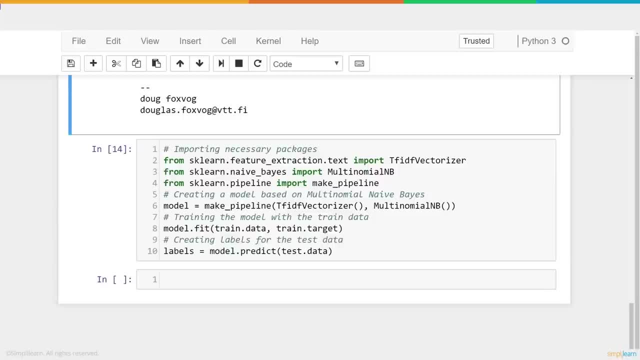 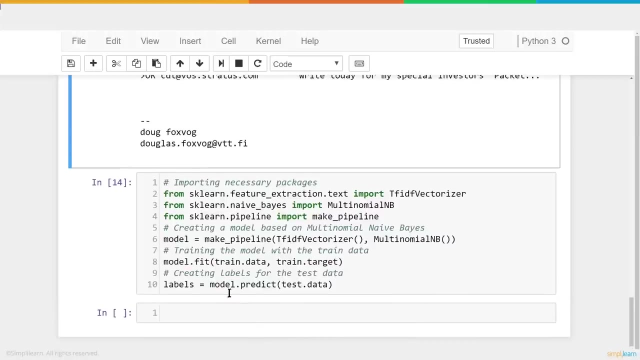 and first the train data and then the train target. now the train data has the different articles in it. you can see the one we were just looking at and the train dot target is what category they already categorized that particular article as, and what's happening here is the train data. 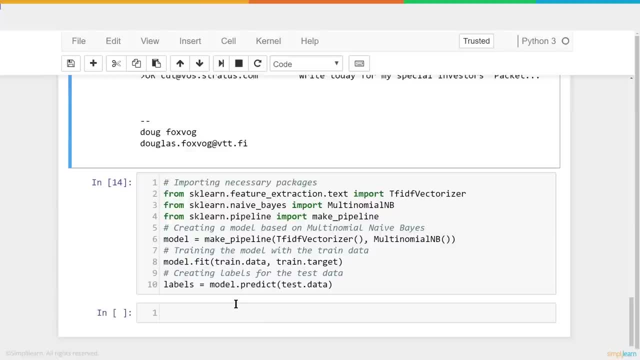 is going into the tf id vectorizer. so when you have one of these articles that goes in there, it weights all the words in there. so there's thousands of words with different weights on them. I remember once running a model on this and I literally had 2.4. 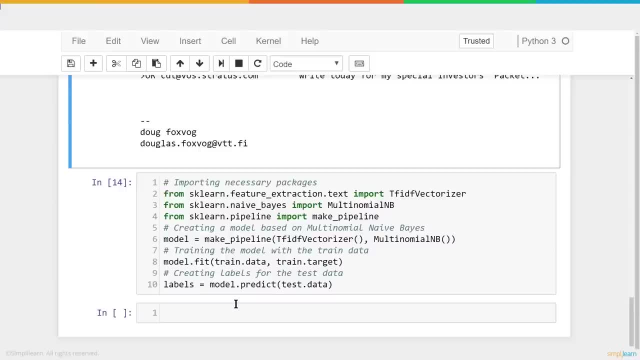 million tokens go into this. so when you're dealing like large document bases, you can have a huge number of different words. it then takes those words, gives them a weight and then based on that weight, based on the words and the weights- and then puts that into the multinomial. 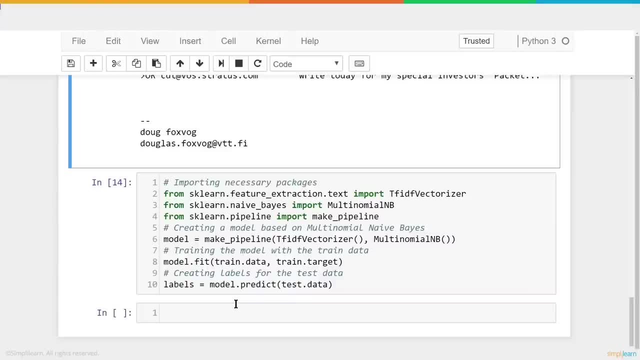 NB, and once we go into our naive bays we want to put the train target in there. so the train data that's been mapped to the tf id vectorizer is now going through the multinomial NB, and then we're telling it: well, these are the answers. 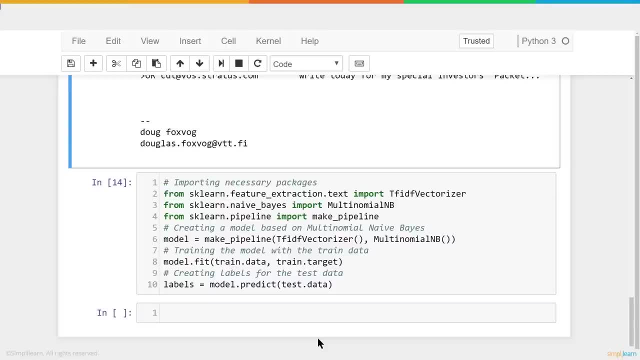 these are the answers to the different documents. so this document that has all these words, with these different weights from the first part, is going to be, whatever category it comes out of- maybe it's the talk show or the article on religion- miscellaneous. once we fit that model, we can. 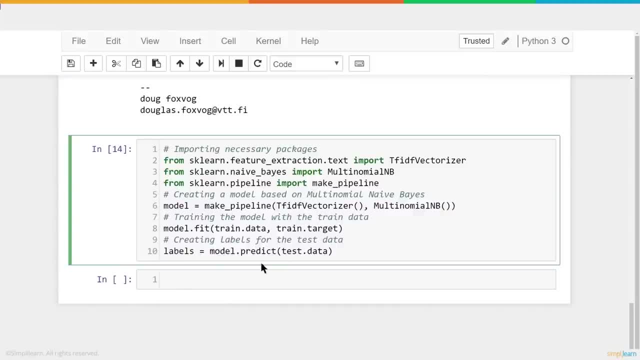 then take labels and we're going to set that equal to model dot predict. most of the sklearn use the term dot predict to let us know that we've now trained the model and now we want to get some answers and we're going to put our test data in there. 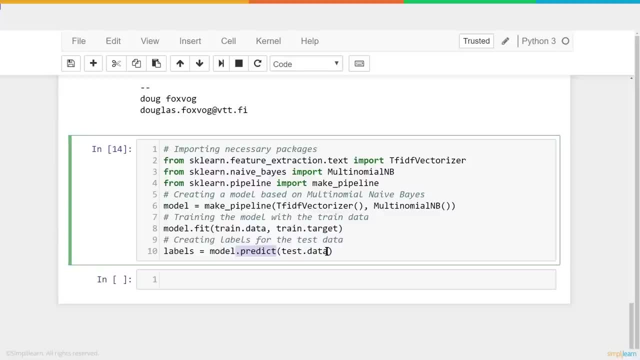 because our test data is the stuff we held off to the side. we didn't train it on there and we don't know what's going to come up out of it, and we just want to find out how good our labels are. do they match what they? 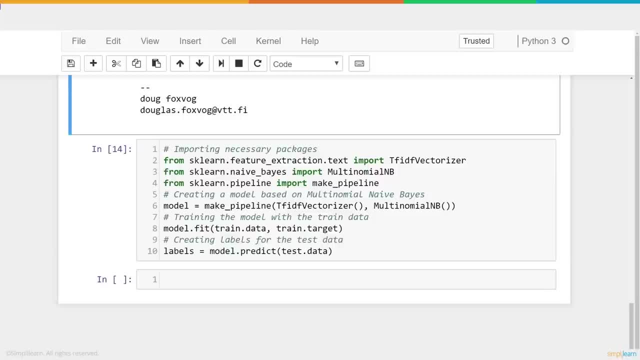 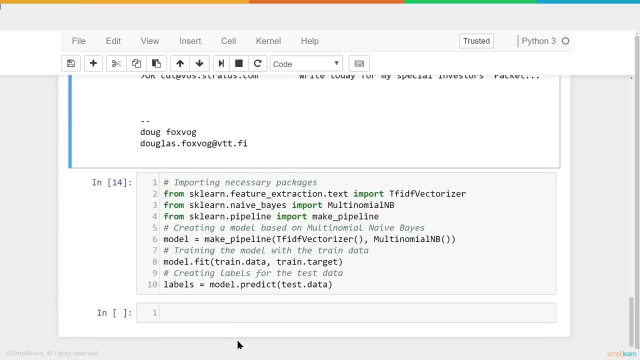 Modelfit And we're going to fit the data, And first the train data and then the train target. Now the train data has the different articles in it. You can see the one we were just looking at And the traintarget is what category. 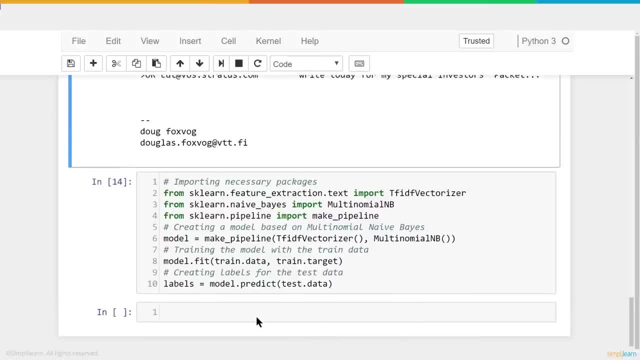 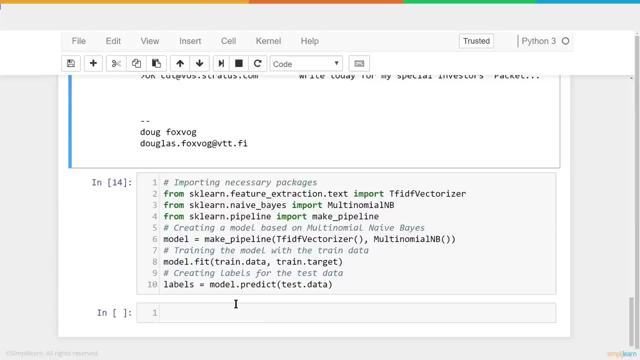 they already categorized that particular article as: And what's happening here is the train data is going into the TF-ID vectorizer, So when you have one of these articles that goes in there, it weights all the words in there. So there's thousands of words with different weights on them. 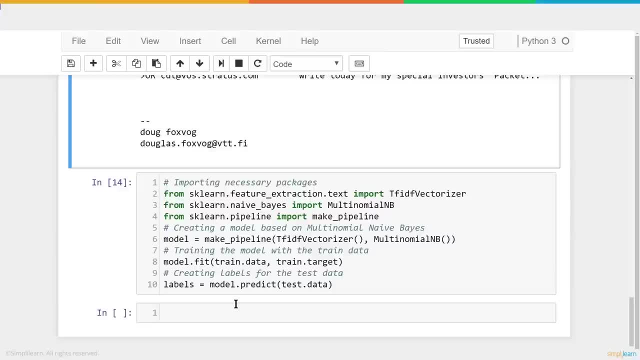 I remember once running a model on this and I literally had 2.4 million tokens go into this. So when you're dealing with large document bases, you can have a huge number of different words. It then takes those words, gives them a weight. 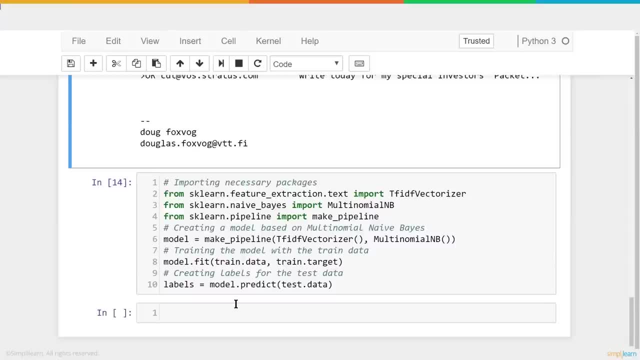 and then based on that weight, based on the words and the weights, it then puts that into the multinomial NB And once we go into our naive base we want to put the train target in there, So the train data that's been mapped to the TF-ID vectorizer. 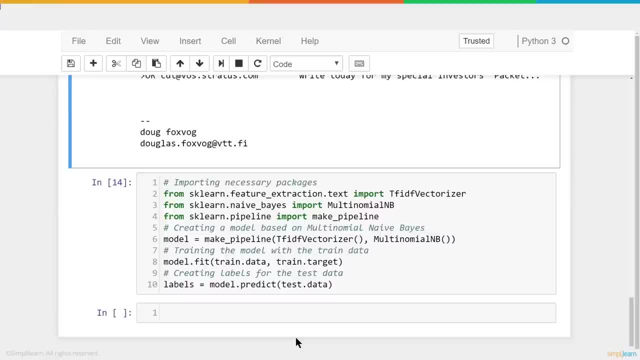 is now going through the multinomial NB, And then we're telling it: well, these are the answers, These are the answers, These are the answers to the different documents. So this document that has all these words, with these different weights, from the first part, 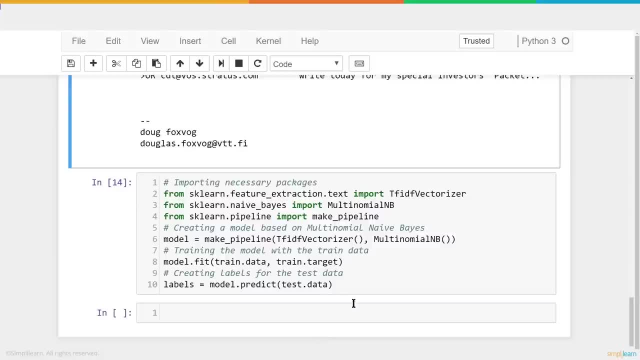 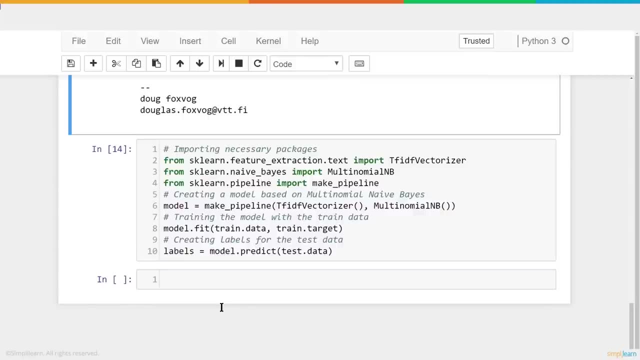 is going to be, whatever category it comes out of- Maybe it's the talk show or the article on religion- miscellaneous. Once we fit that model, we can then take labels and we're going to set that equal to modelpredict. Most of the sklearn use the term predict to let us know. 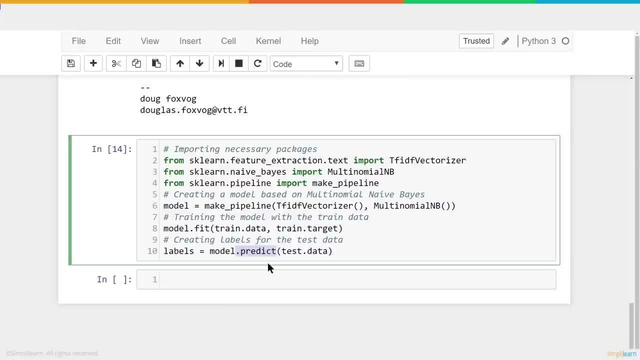 that we've now trained the model and now we want to get some answers And we're going to put our test data in there, because our test data is the stuff we held off to the side. We didn't train it on there and we 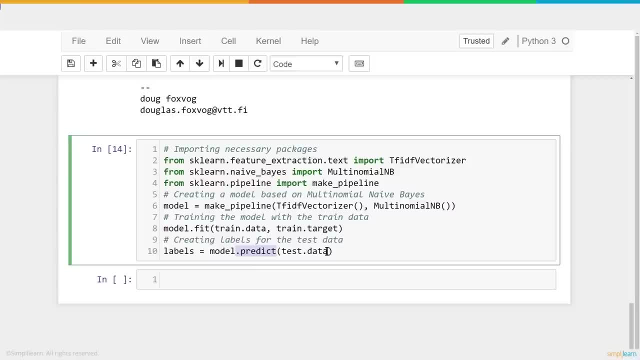 don't know what's going to come up out of it, And we just want to find out how good our labels are. Do they match what they should be? Now, I've already run this through. There's no actual output to it to show. 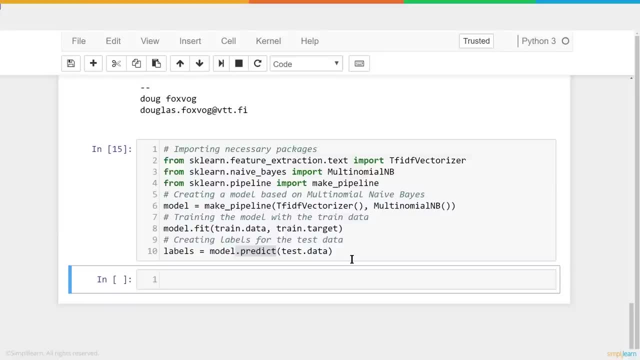 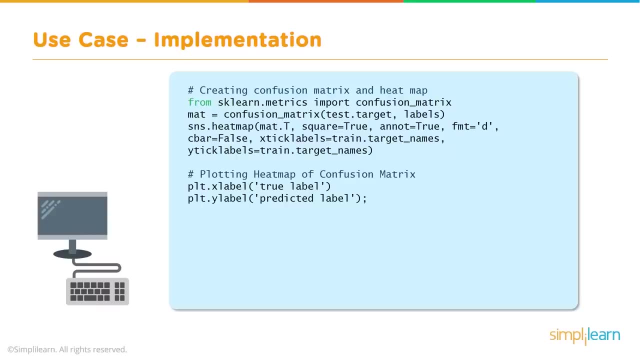 This is just setting it all up. This is just training our model, creating the labels so we can see how good it is, and then we move on to the next step, to find out what happened To do this. we're going to go ahead and create a confusion. 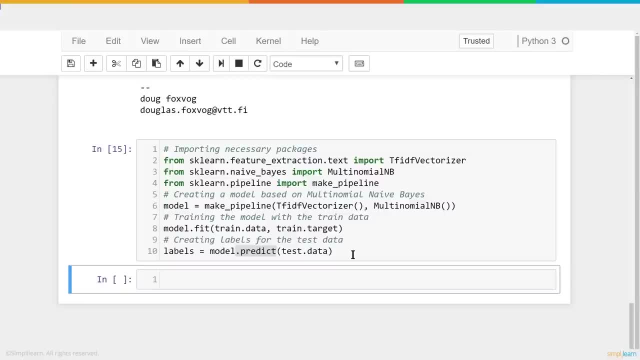 should be now. I've already run this through. there's no actual output to it to show. this is just setting it all up. this is just training our model, creating the labels so we can see how good it is, and then we move on to the next step, to. 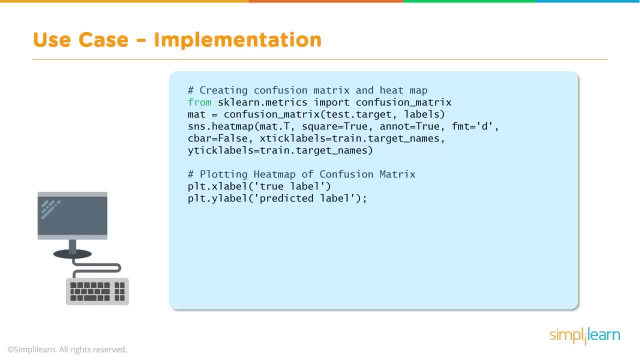 find out what happened. to do this, we're going to go ahead and create a confusion matrix and a heat map. so the confusion matrix, which is confusing just by its very name, is basically going to ask: how confused is our answer? did it get it correct or did it miss some things in there? 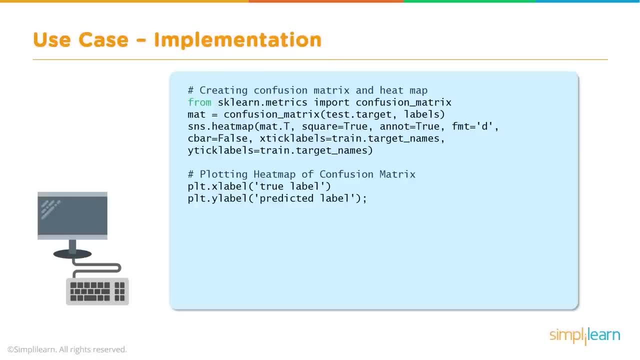 or have some missed labels, and then we're going to put that on a heat map, so we'll have some nice colors to look at. to see how that plots out. let's go ahead and take this code and see how that. take a walk through it and see what that looks like. 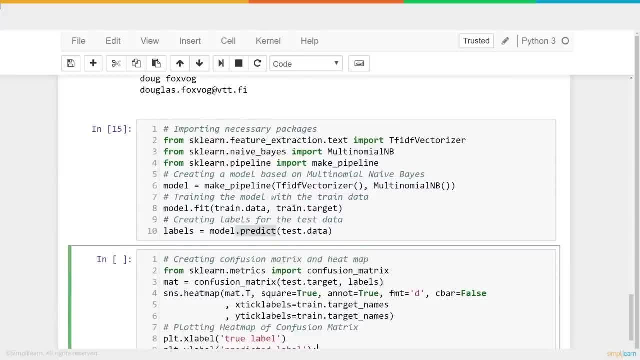 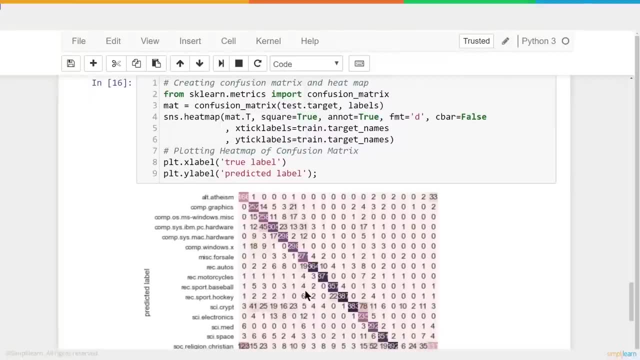 so back to our Jupyter notebook, put the code in there and let's go ahead and run that code. take it just a moment and remember we had the end line. that way my graph shows up on the end line here and let's walk through the code. 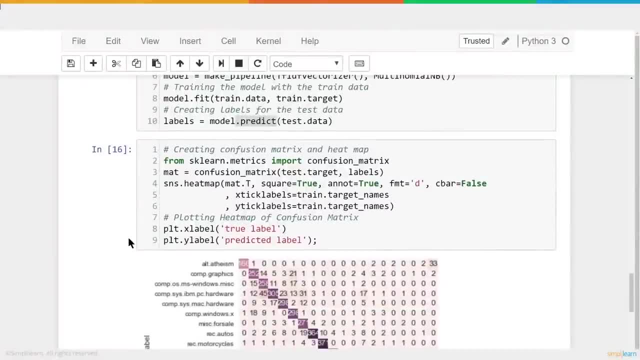 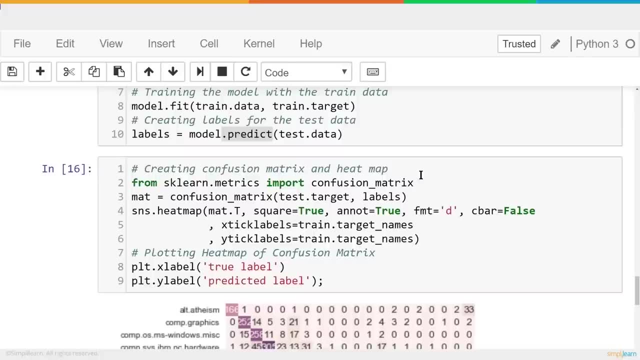 and then we'll look at this and see what that means. so let me get a little bit bigger. there we go, no reason not to use the whole screen too big. so we have here from sklearnmetrics import confusion matrix and that's just going to generate a set. 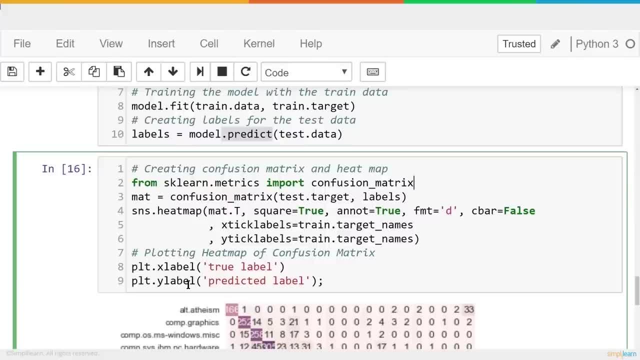 of data that says the prediction was such. the actual truth was either agreed with it or something different, and it's going to add up those numbers so we can take a look and just see how well it worked. and we're going to set a variable mat equal. 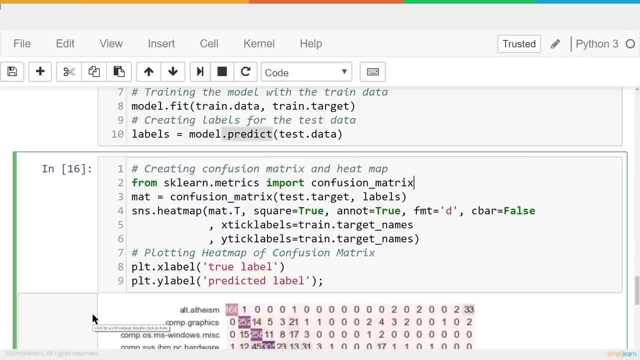 to confusion- matrix- and we have our test target, our test data. that was not part of the training- very important in data science. we always keep our test data separate, otherwise it's not a valid model if we can't properly test it with new data. and this is the labels. 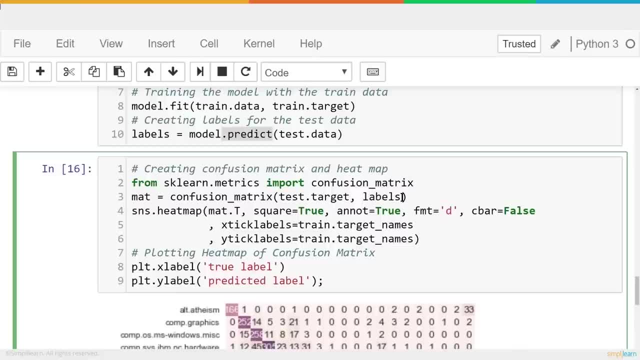 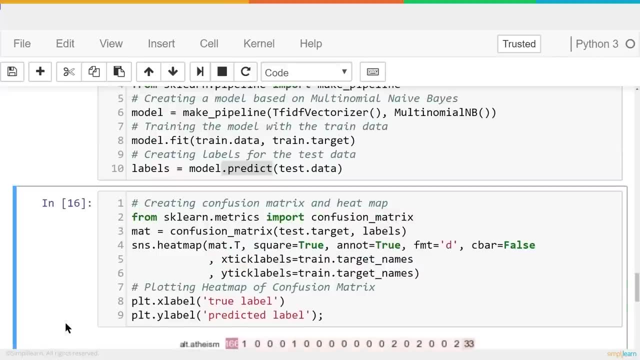 we created from that test data. these are the ones that we predict it's going to be. so we go in and we create our sn heat map. the sns is our seaborn, which sits on top of the pi plot. so we create a snsheatmap. we take our confusion matrix. 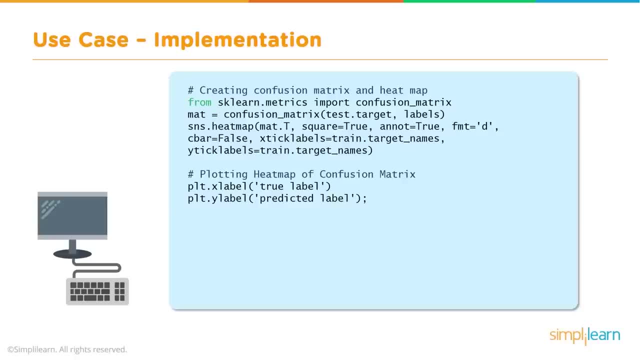 matrix and a heat map. So The Confusion matrix, which is confusing just by its very name, is basically going to ask: how confused is our answer? Did it get it correct or did it miss some things in there or have some missed labels? 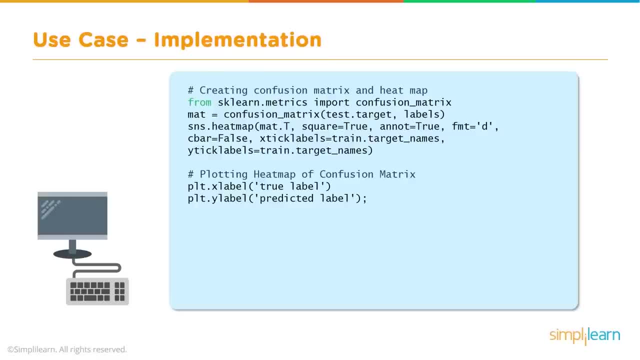 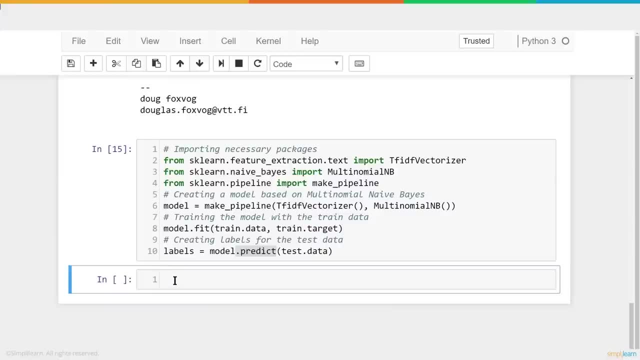 And then we're going to put that on a heat map so we'll have some nice colors to look at to see how that plots out. Let's go ahead and take this code and take a walk through it and see what that looks like. So back to our Jupyter notebook- going to put the code in there. 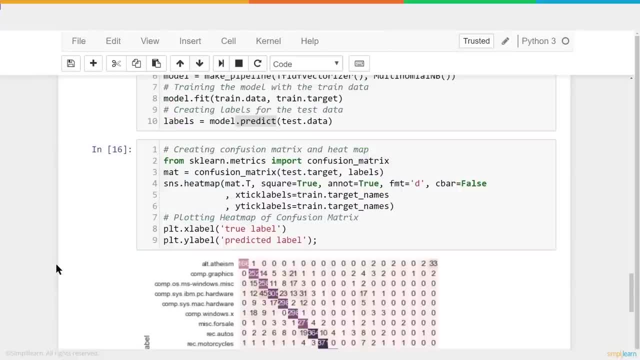 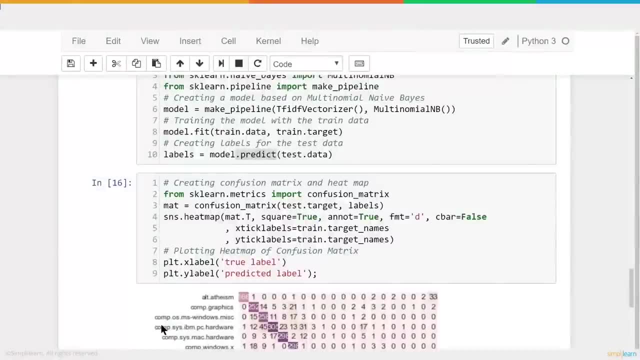 And let's go ahead and run that code. Take it just a moment And remember we had the inline. That way my graph shows up on the inline here And let's walk through the code and then we'll look at this. 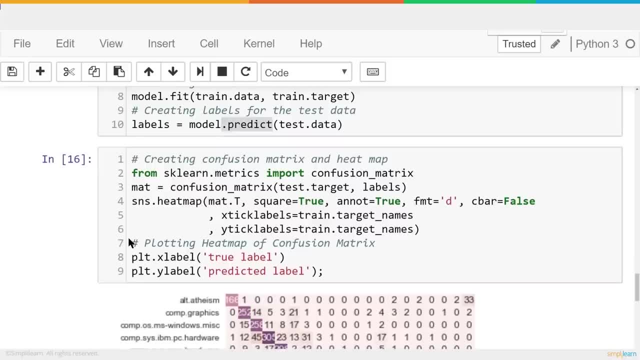 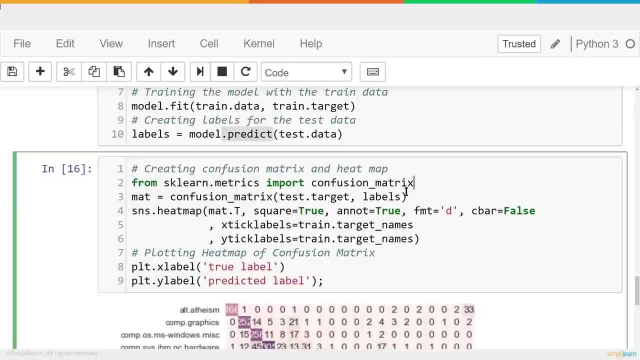 and see what that means. So let me get a little bit bigger. There we go. No reason not to use a whole screen too big. So we have here from sklearnmetrics import confusion matrix And that's just going to generate a set of data that 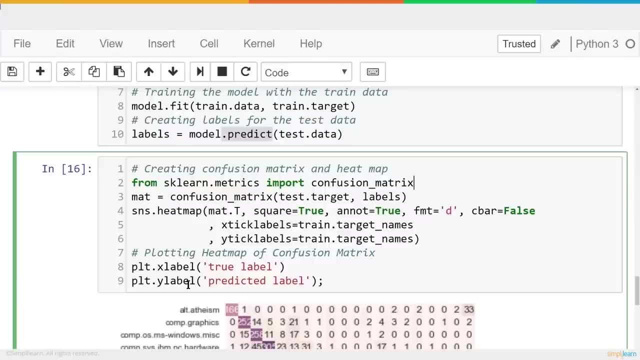 says the prediction was such, the actual truth was either agreed with it or it was something different. And it's going to add up those numbers so we can take a look and just see how well it worked, And we're going to set a variable mat. 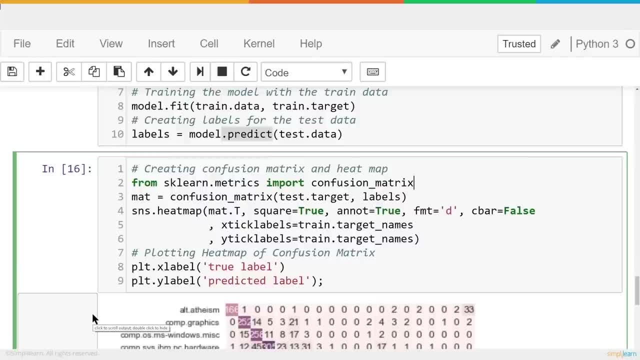 equal to confusion. matrix: We have our test target, our test data. that was not part of the training- Very important in data science. we always keep our test data separate, Otherwise it's not a valid model if we can't properly test it with new data. 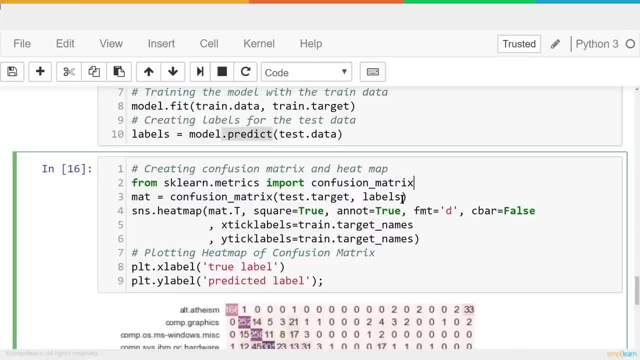 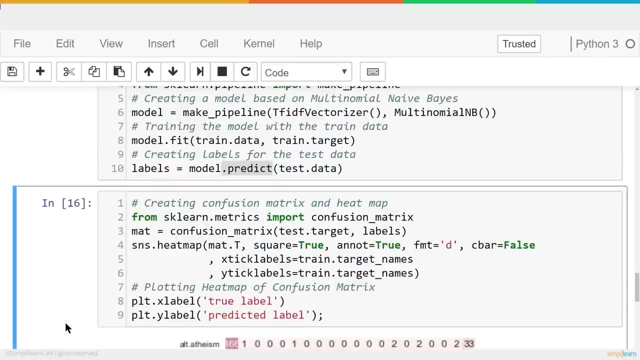 And this is the labels we created from that test data. These are the ones that we predict it's going to be. So we go in and we create our SN heat map. The SNS is our seaborne, which sits on top of the pi plot. 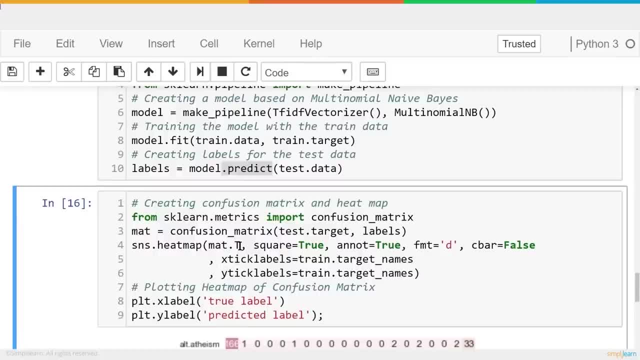 So we create a SNS dot heat map. We take our confusion matrix and it's going to be mat dot t, And then we have other variables that go into the SNS dot heat map. We're not going to go into detail what all the variables mean. 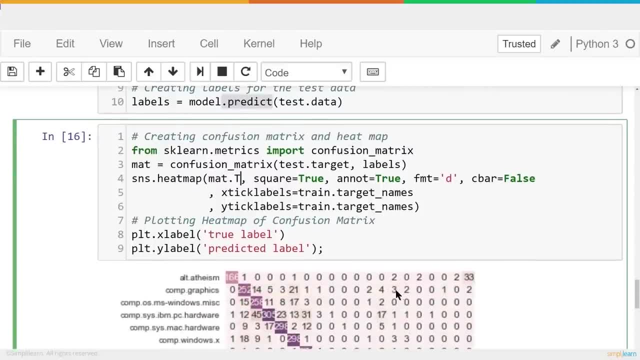 The annotation equals true. that's what tells it to put the numbers here. So you have the 166, the 1, the 0001.. Format d and c bar equals false. have to do with the format. If you take those out, you'll see that some. 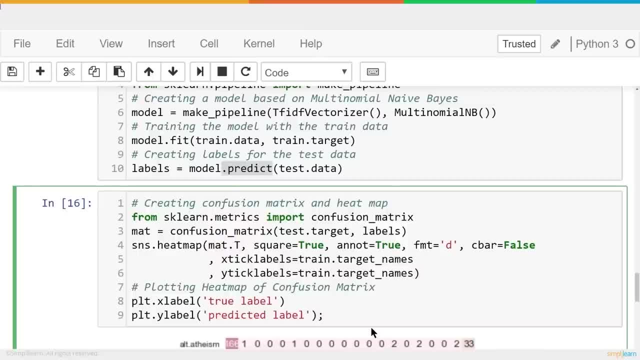 and it's going to be matt. and then we have other variables that go into the snsheatmap. we're not going to go into detail what all the variables mean. the annotation equals true. that's what tells it to put the numbers here. so you have. 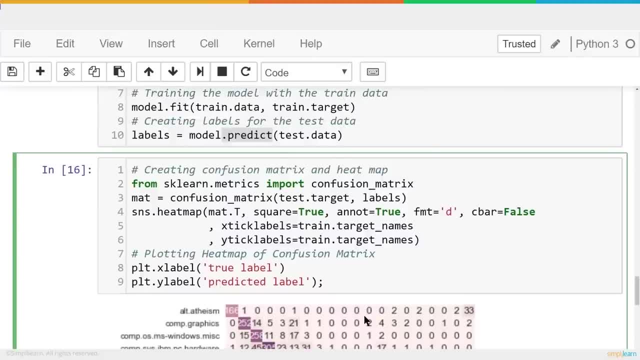 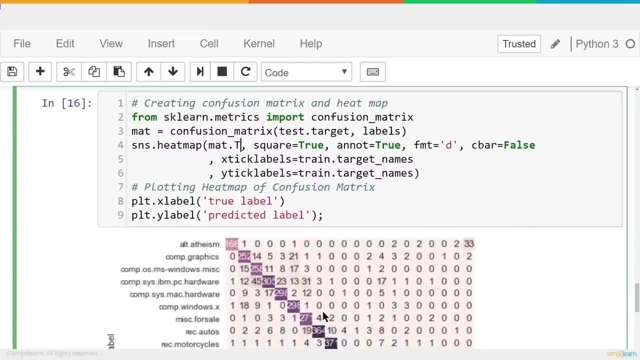 the 166, the 1, the 0001 format. d and c bar equals false, have to do with the format. if you take those out, you'll see that some things disappear. and then the x tick labels and the y tick labels. those are our target names. 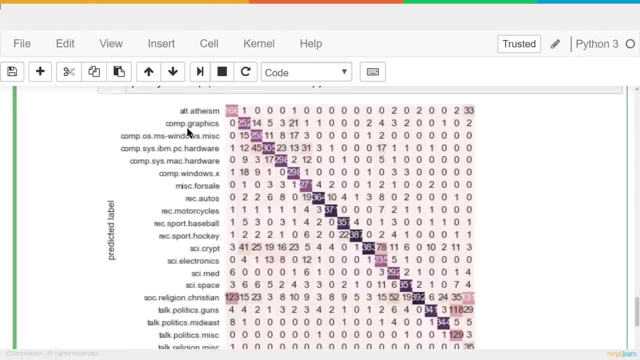 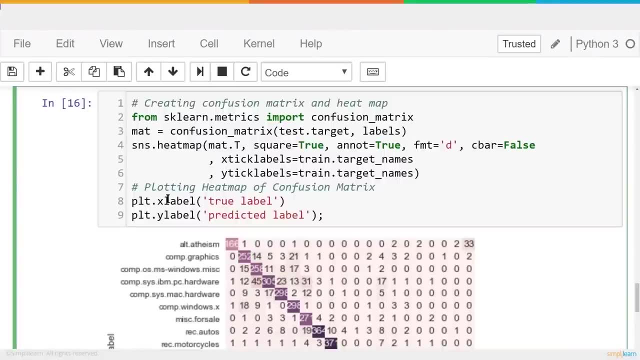 and you can see right here, that's the alt atheism comp, graphics, comp os, ms windows, dot, miscellaneous. and then, finally, we have our plt dot x label. remember the sns or the seaborn sits on top of our matplot library, our plt. and so we want to just tell it: x label equals. 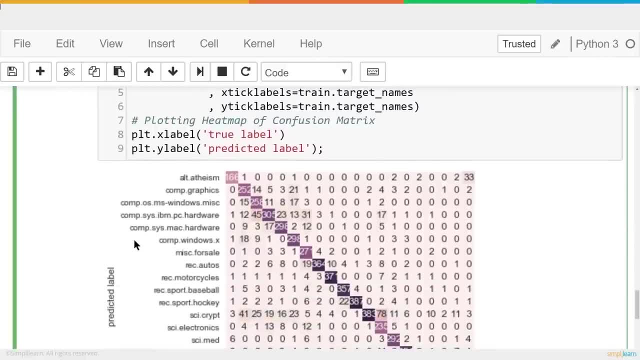 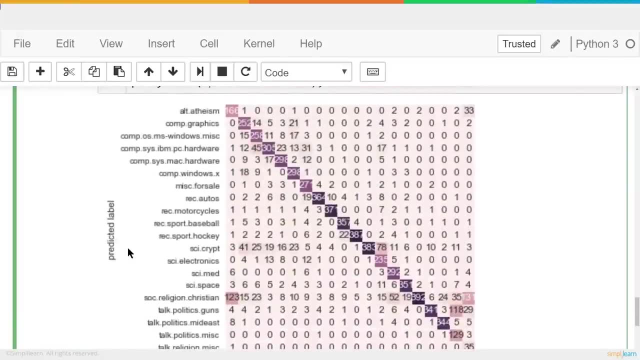 a true is true, the labels are true. and then the y label is prediction label. so when we say a true, this is what it actually is and the prediction is what we predicted. and let's look at this graph because that's probably a little confusing the way. 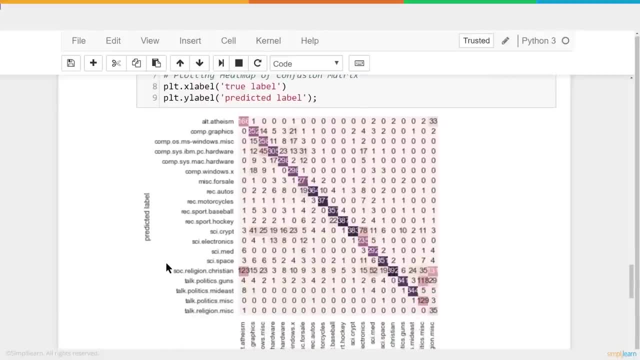 I rattled through it and what I'm going to do is I'm going to go ahead and flip back to the slides, because they have a black background they put in there. that helps it shine a little bit better, so you can see the graph a little bit easier. so in reading, 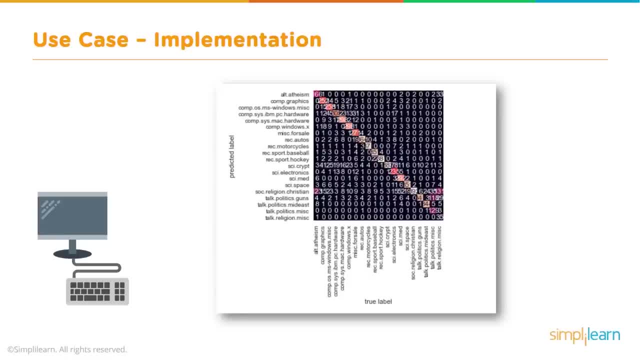 this graph. what we want to look at is how the color scheme has come out, and you'll see a line right down the middle, diagonally from upper left to bottom right. what that is is, if you look at the labels, we have our predicted label on the. 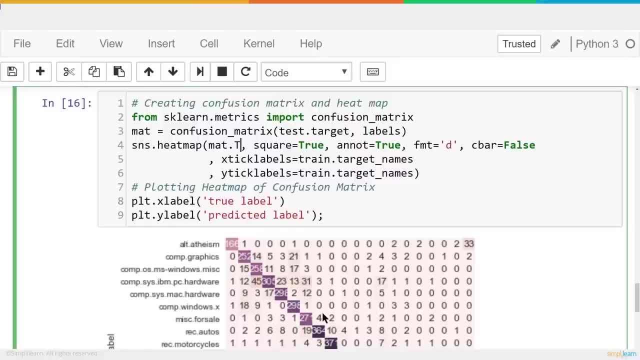 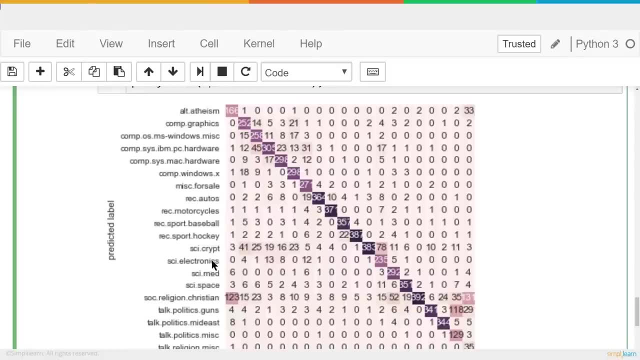 things disappear. And then the x tick labels and the y tick labels. those are our target names And you can see right here: that's the alt atheism comp, graphics, comp, osms, windows, dot, miscellaneous. And then finally we have our plt dot x label. 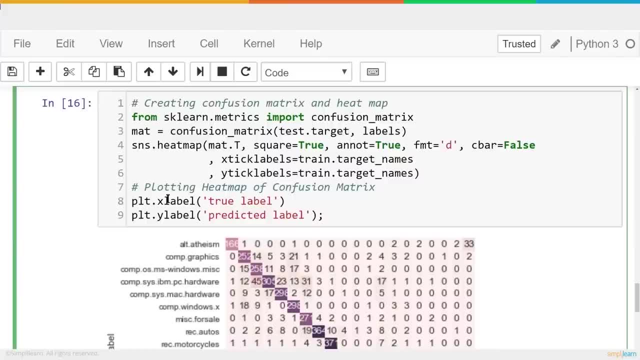 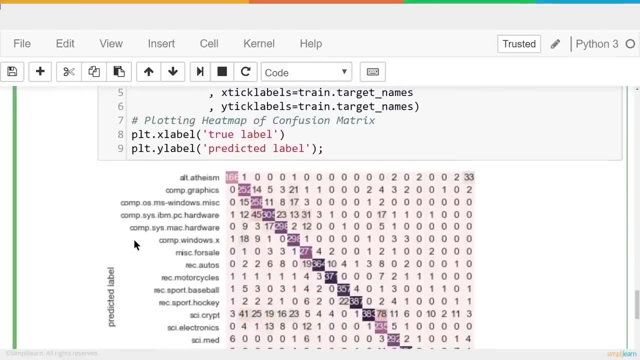 Remember the SNS or the seaborne sits on top of our mat plot library, our plt, And so we want to just tell it: x label equals, a true is true, The labels are true. And then the y label is prediction label. 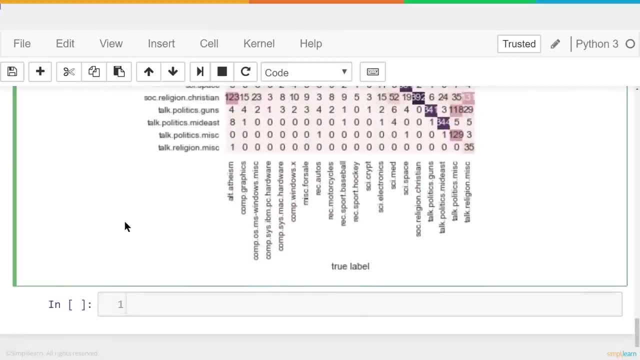 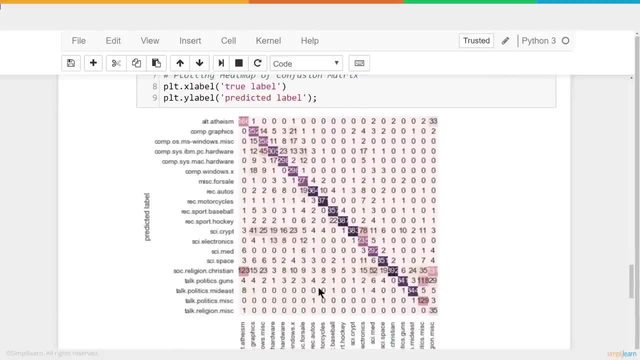 a little confusing the way we rattled through it, And what I'm going to do is I'm going to go ahead and flip back to the slides, because they have a black background they put in there. that helps it shine a little bit better. 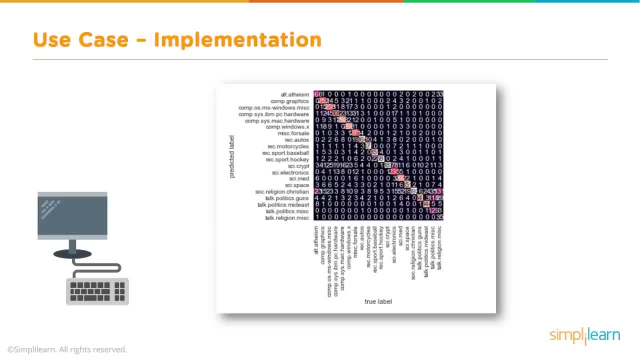 so you can see the graph a little bit easier. So in reading this graph, what we want to look at is how the color scheme has come out, And you'll see a line right down the middle diagonally from upper left to bottom right. 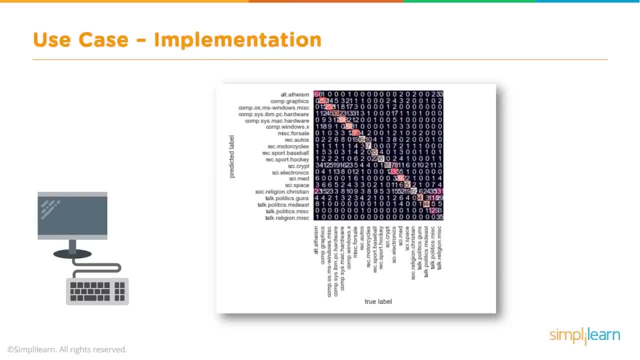 What that is is, if you look at the labels, we have our predicted label on the left and our true label on the right. Those are the numbers where the prediction and the true come together, And this is what we want to see is we want to see those lit up. 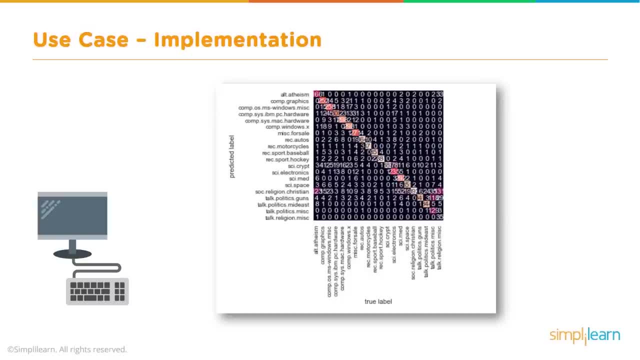 That's what that heat map does is. you can see that it did a good job of finding those data And you'll notice that there's a couple of red spots on there where it missed. It's a little confused when we talk about talk religion. 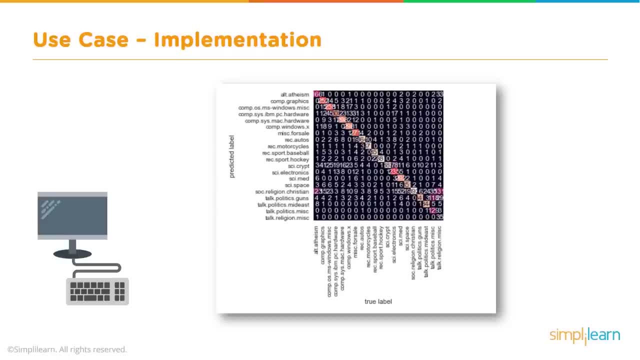 miscellaneous versus talk politics miscellaneous. social religion: Christian versus all religions miscellaneous. It mislabeled some of those And those are very similar topics so you could understand why it might mislabel them, But overall it did a pretty good job If we're going to create these models. 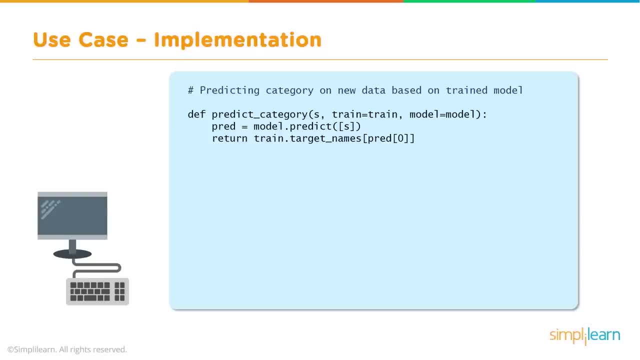 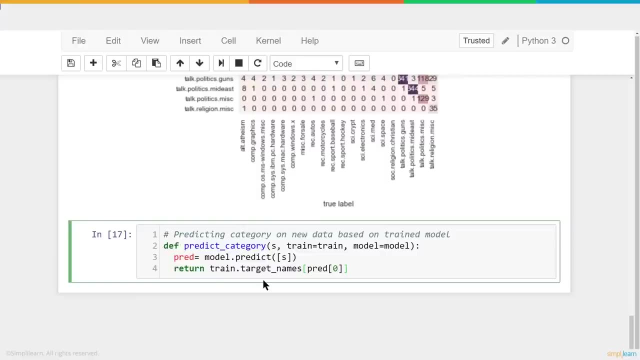 we want to go ahead and be able to use them. So let's see what that looks like. To do this, let's go ahead and create a definition, a function to run, And we're going to call this function. let me just expand that just a notch here. 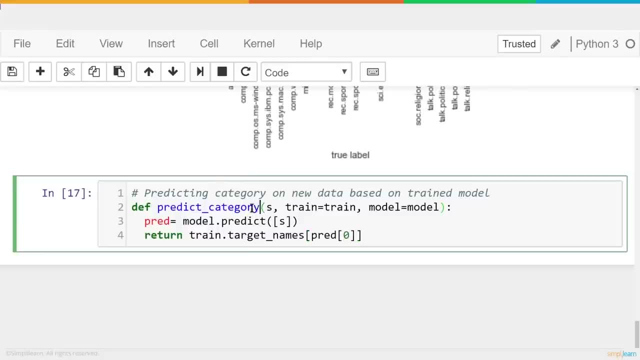 There we go. I like mine in big letters. Predict categories. We want to predict the category, We're going to send it s a string And we're going to call this function. let me just expand that just a notch here. 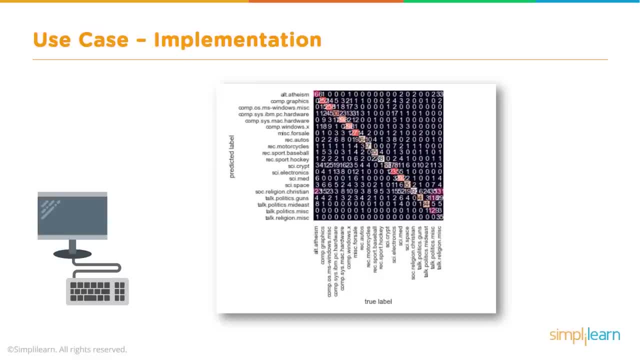 left and our true label on the right. those are the numbers where the prediction and the true come together, and this is what we want to see is we want to see those lit up. that's what that heat map does, as you can see that it did a good job of. 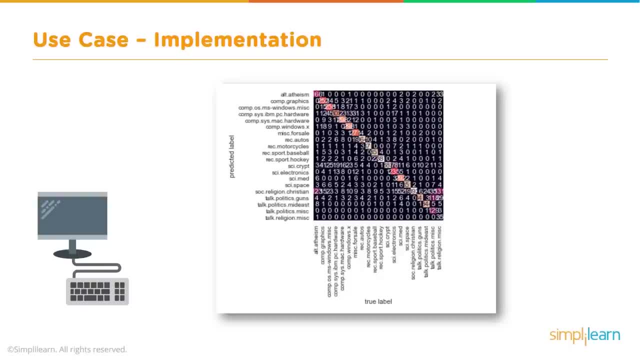 finding those data and you'll notice that there's a couple of red spots on there where it missed. you know it's a little confused when we talk about talk religion, miscellaneous versus talk politics, miscellaneous, social religion, Christian versus alt atheism. it mislabeled some of those and those are very similar. 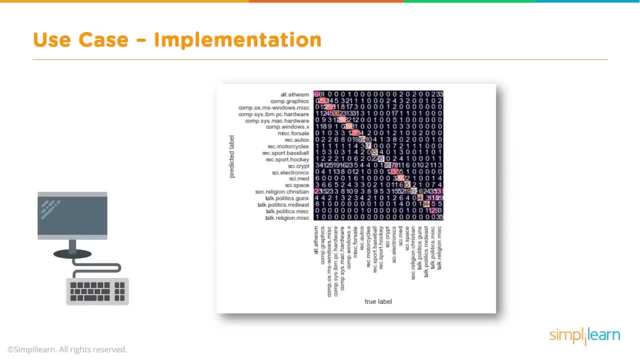 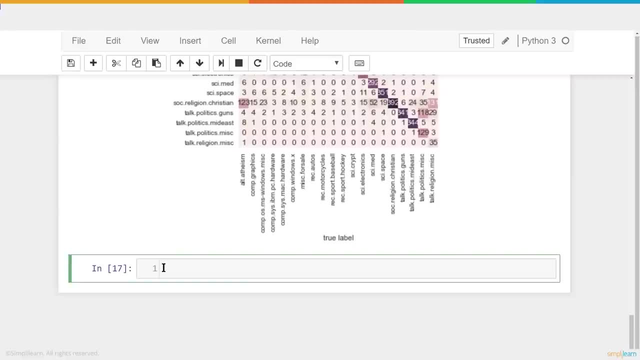 topics so you could understand why it might mislabel them, but overall it did a pretty good job. if we're going to create these models, we want to go ahead and be able to use them, so let's see what that looks like to do this. let's go ahead. 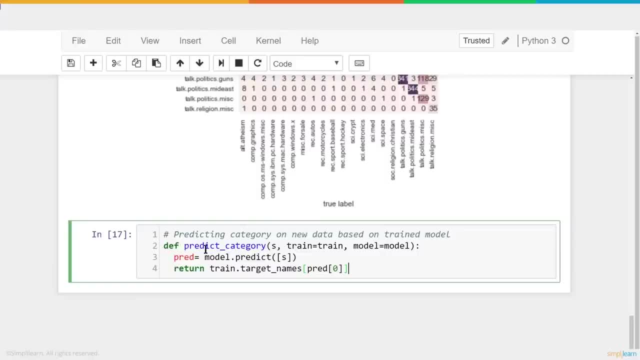 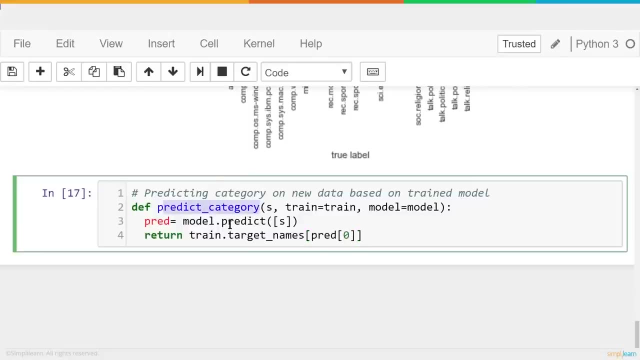 and create a definition, a function to run, and we're going to call this function. let me just expand that just a notch here. there we go. I like mine in big letters: predict categories. we want to predict the category we're going to send. it s a string. 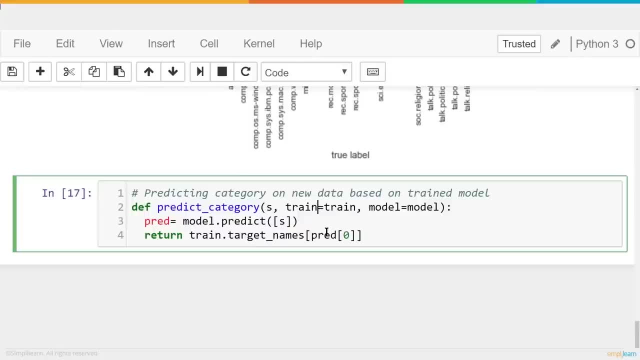 and then we're sending it train equals train. we have our training model and then we had our pipeline model equals model. this way we don't have to resend these variables each time. the definition knows that, because I said train equals train and I put the equal for model, and then 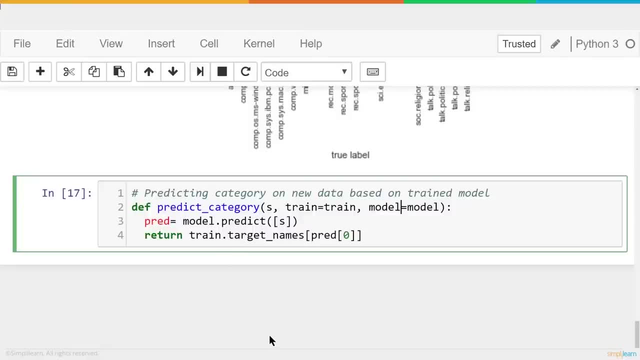 we're going to set the prediction equal to the model dot predict s. so it's going to send whatever string we send to it. it's going to push that string through the pipeline, the model pipeline. it's going to go through and tokenize it and put it through the tf. 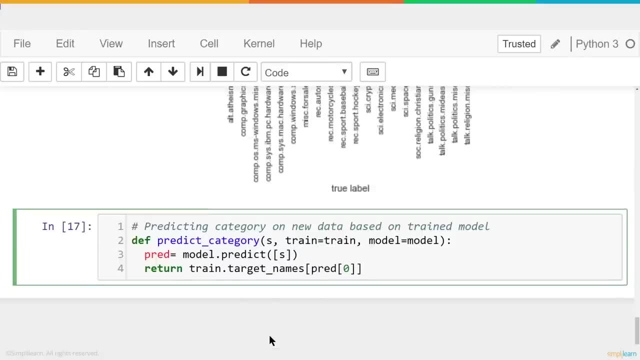 idf, convert that into numbers and weights for all the different documents and words, and then it'll put that through our naive bays and from it we'll go ahead and get our prediction. we're going to predict what value it is, and so we're going to return. 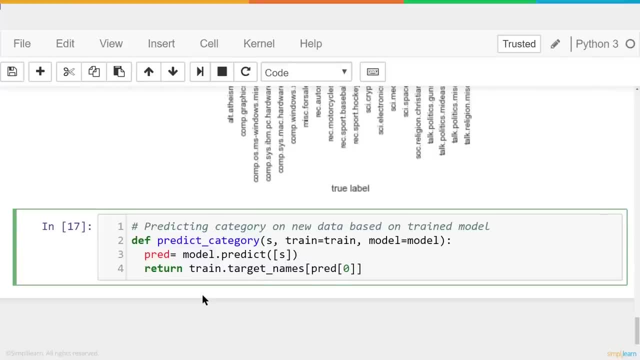 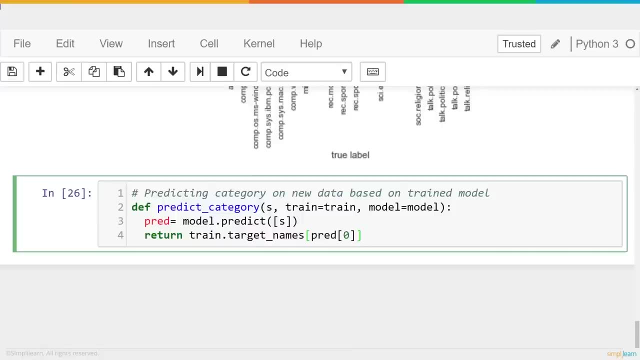 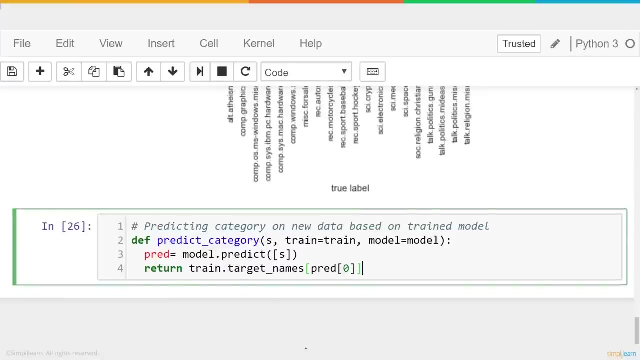 train dot target names- predict of zero. and remember that the train dot target names, that's just categories. I could have just as easily put categories in there: dot: predict of zero. so we're taking the prediction, which is a number, and we're converting it to an actual category. we're converting it. 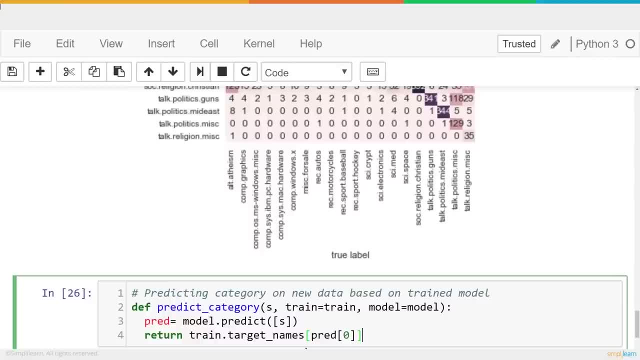 from. I don't know what the actual numbers are, but let's say zero equals alt atheism, so we're going to convert that zero to the word or one. maybe it equals comp graphics, so we're going to convert number one into comp graphics. that's all that is, and then we got to go ahead. 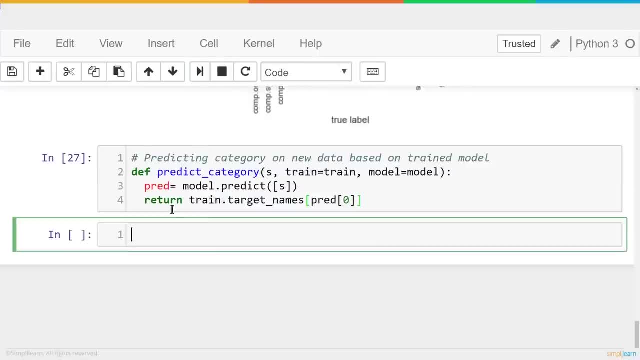 and then we need to go ahead and run this, so I load that up and then, once I run that, we can start doing some predictions. let me go ahead and type in predict category and let's just do predict category Jesus Christ. and it comes back and says: 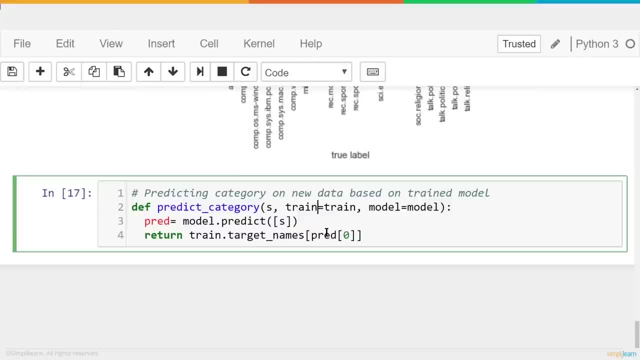 And then we're sending it train equals train. We have our training model And then we had our pipeline Model equals model. This way we don't have to resend these variables each time. The definition knows that, because I said train equals train. 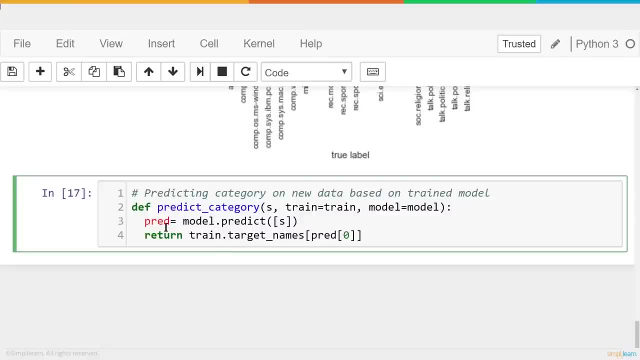 And I put the equal for model And then we're going to set the prediction equal to the modelpredict s. So it's going to send whatever string we send to it. It's going to push that string through the pipeline, the model pipeline. 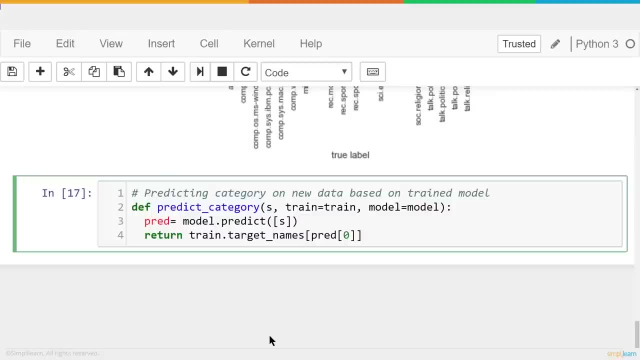 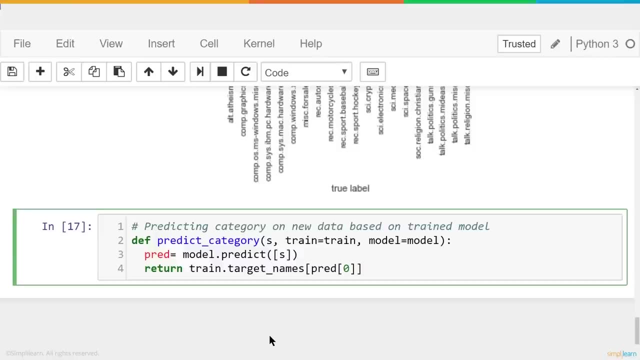 It's going to go through and tokenize it and put it through the t, tf, idf, Convert that into numbers and weights for all the different documents and words, And then it'll put that through our naive bays And from it we'll go ahead and get our prediction. 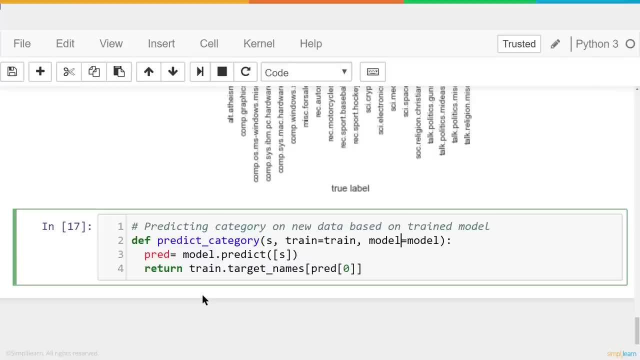 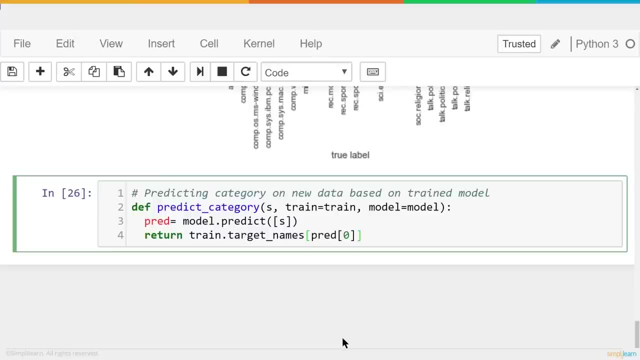 We're going to predict what value it is, And so we're going to return traintargetNames: predict of 0.. And remember that the traintargetNames, that's just categories. I could have just as easily put categories in there. predict of 0. 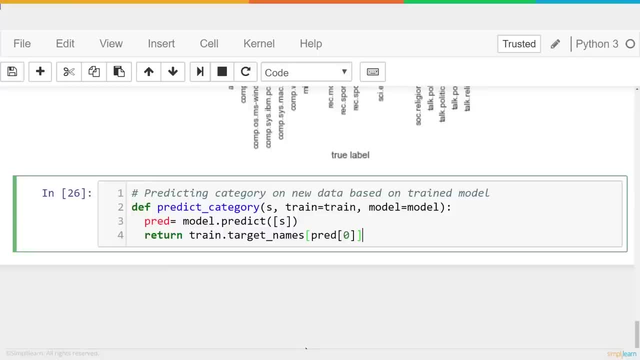 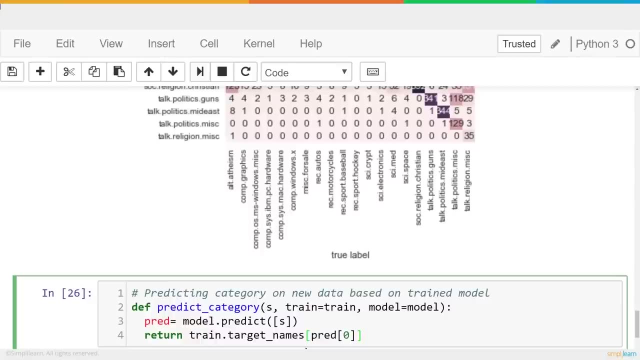 So we're taking the prediction, which is a number, and we're converting it to an actual category. We're converting it from. I don't know what the actual numbers are, but let's say 0 equals alt atheism. So we're going to convert that 0 to the word. 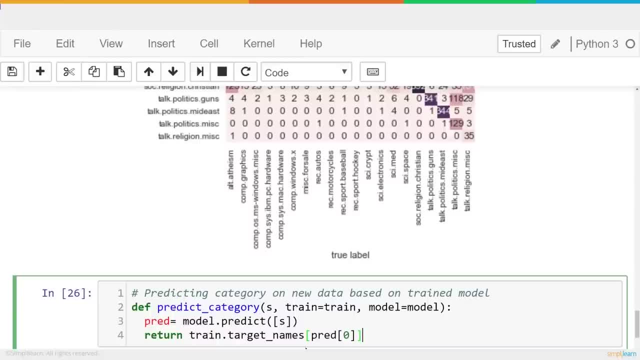 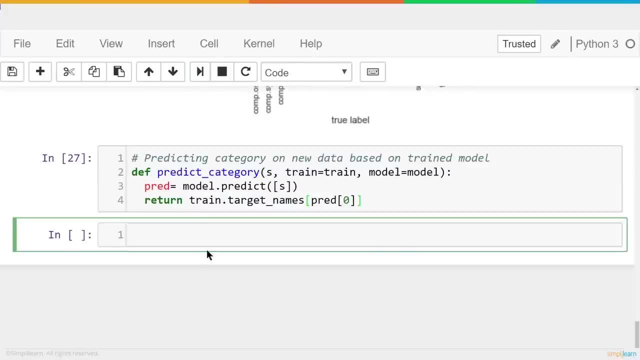 Or 1, maybe it equals comp graphics. So we're going to convert number 1 into comp graphics, That's all that is. And then we need to go ahead and run this. So I load that up And then, once I run that, we can start doing some predictions. 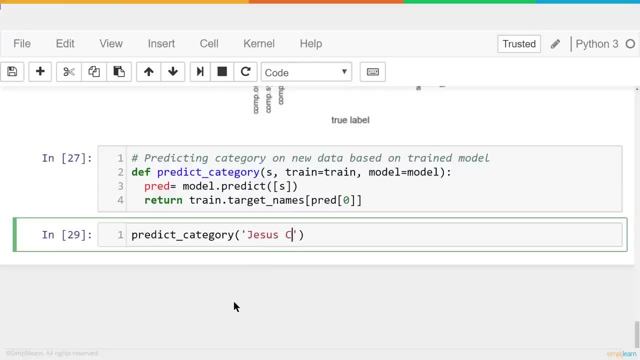 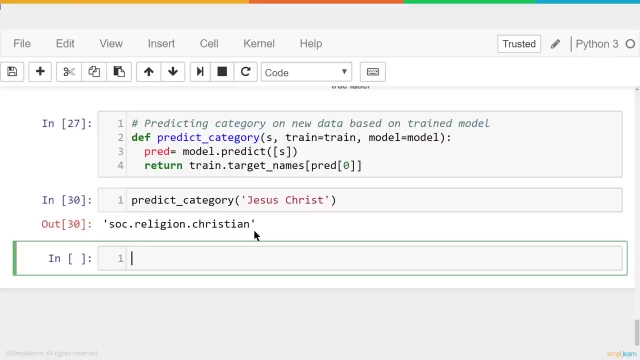 I'm going to go ahead and type in predict category And let's just do predict category, Predict category: Jesus Christ. And it comes back and says it's social religion, Christian. That's pretty good. Now note I didn't put print on this. 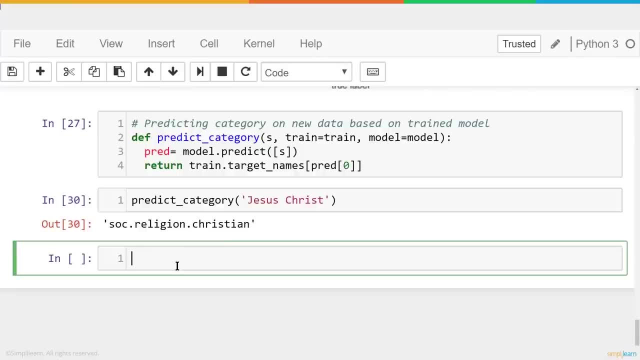 One of the nice things about the Jupyter Notebook Editor and a lot of inline editors is if you just put the name of the variable out, it's returning the variable traintarget underscore names. it'll automatically print that for you In your own ID you might have to put in print. 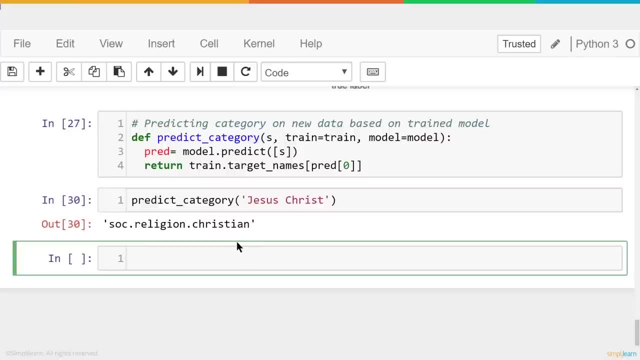 it's social religion: Christian. that's pretty good. now note I didn't put print on this. one of the nice things about the Jupiter notebook editor and a lot of inline editors is if you just put the name of the variable out, it's returning the variable train dot target underscore names. 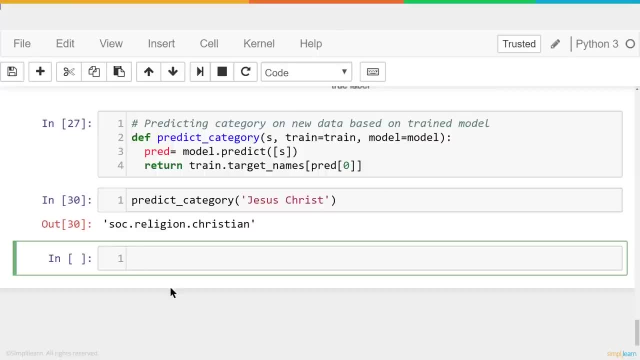 it'll automatically print that for you in your own ID. you might have to put in print. let's see where else we can take this. and maybe you're a space science buff. so how about sending load to international space station? and if we run that, we get science. 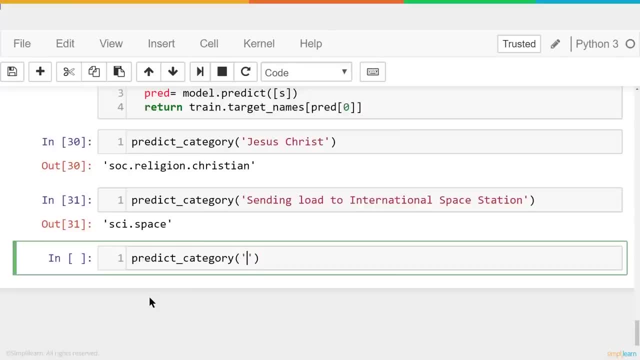 space, or maybe you're a automobile buff and let's do. they were going to tell me: Audi is better than BMW, but I'm going to do, BMW is better than an Audi. so maybe you're a car buff and we run that and you'll see. it says recreational. I'm assuming that's. 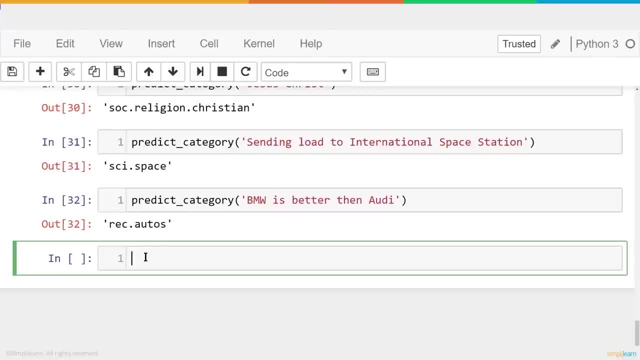 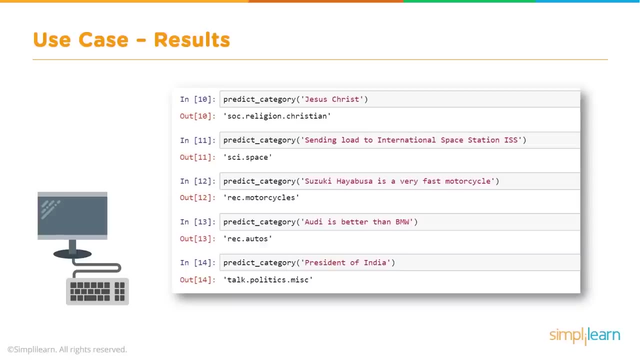 what REC stands for autos. so I did a pretty good job labeling that one. how about if we have something like a caption running through there, president of India, and if we run that it comes up and says: talk politics miscellaneous. so when we take our definition, our function and we run all these things, 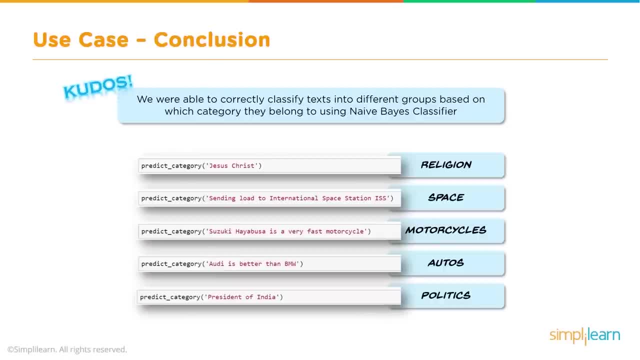 through kudos. we made it. we were able to correctly classify text into different groups based on which category they belong to, using the naive base classifier. now we did throw in the pipeline the TF idea vectorizer. we threw in the graphs. those are all things that you don't necessarily. 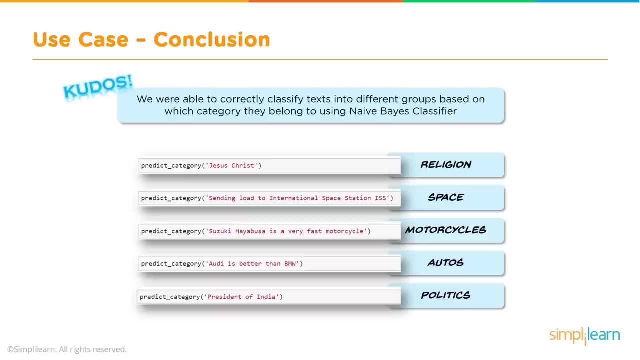 have to know to understand the naive base setup or classifier, but they're important to know. one of the main uses for the naive base is with the TF, IDF tokenizer or vectorizer, where it tokenizes a word and has labels and we use the pipeline because you need to push all that data through. 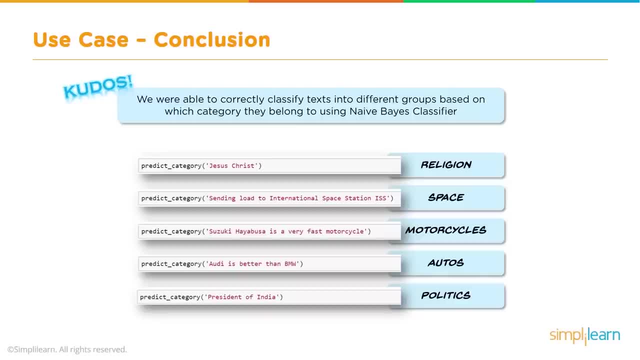 and it makes it really easy and fast. you don't have to know those to understand naive base, but they certainly help for understanding the industry and data science. and we can see our categorizer, our naive base classifier. we were able to predict the category: religion, space, motorcycle. 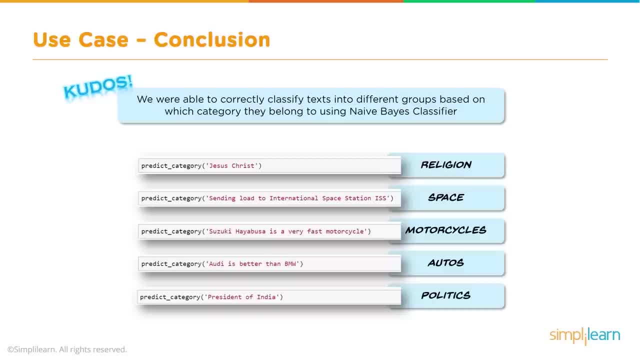 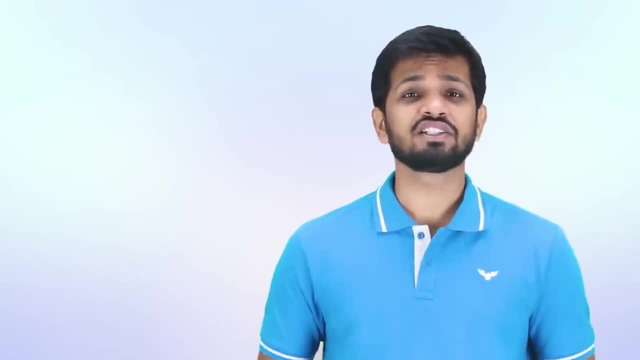 autos, politics, and properly classify all these different things we pushed into our prediction and our trained model. thanks again, Richard. that was great. that brings us to the end of this comprehensive look at machine learning and its algorithms. now we have Rahul, who will take you through the various applications of machine learning. 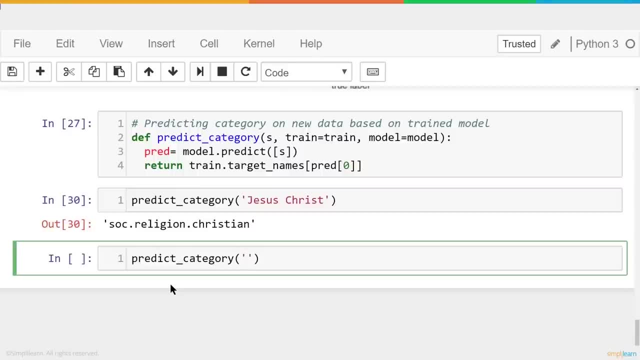 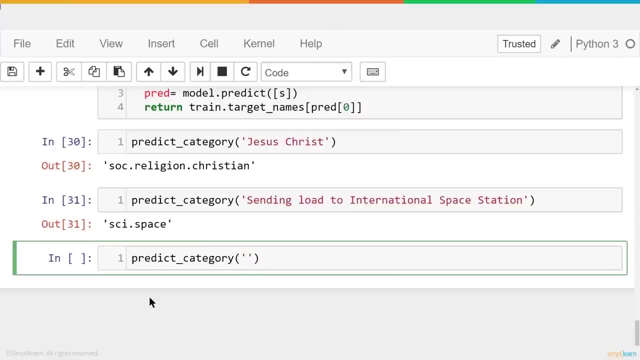 Let's see where else we can take this. And maybe you're a space science buff, So how about sending Sending load to international space station? And if we run that, we get science space. Or maybe you're a automobile buff And let's do. oh, they were going to tell me. 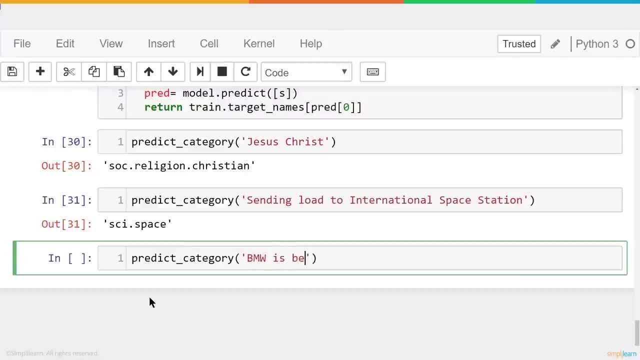 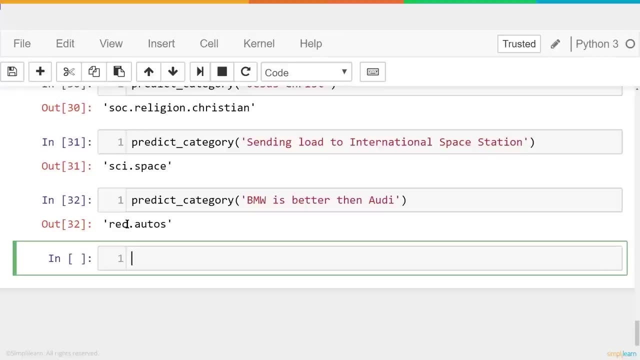 Audi is better than BMW. But I'm going to do BMW is better than an Audi. So maybe you're a car buff And we run that And you'll see. it says recreational. I'm assuming that's what REC stands for Autos. 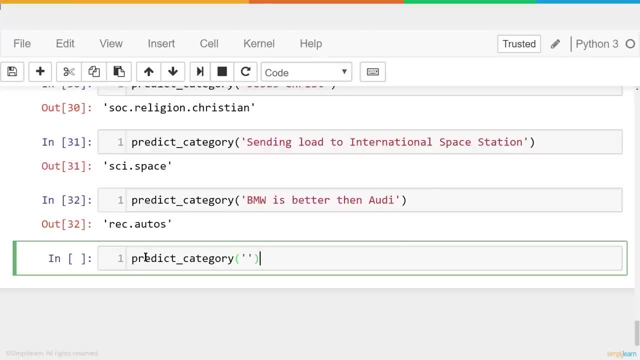 So I did a pretty good job labeling that one. How about if we have something like a caption running through there, President of India? And if we run that, it comes up and says: talk politics miscellaneous. So when we take our definition or our function, 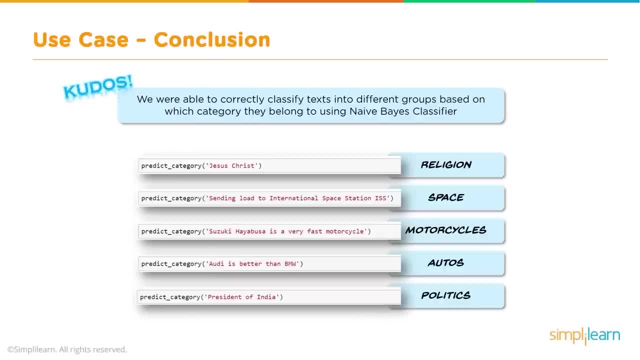 and we run all these things through kudos. we made it. We were able to correctly classify texts into different groups, based on which category they belong to, using the Naive Bayes classifier. Now, we did throw in the pipeline The TF-IDF vectorizer. we threw in the graphs. 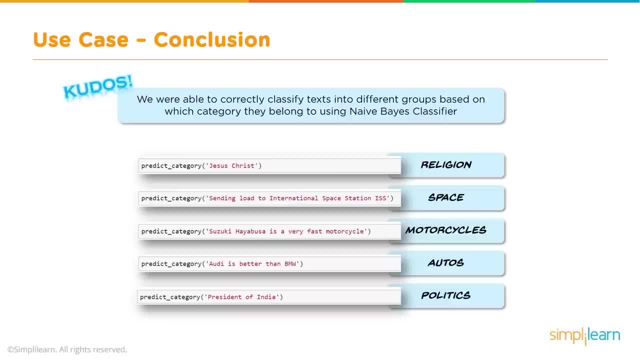 Those are all things that you don't necessarily have to know to understand the Naive Bayes setup or classifier, But they're important to know. One of the main uses for the Naive Bayes is with the TF-IDF tokenizer or vectorizer. 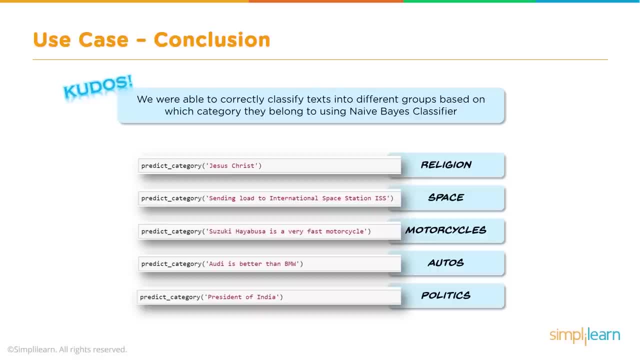 where it tokenizes a word and has labels. And we use the pipeline because you need to push all that data through And it makes it really easy and fast. You don't have to know those to understand Naive Bayes, But they certainly help. 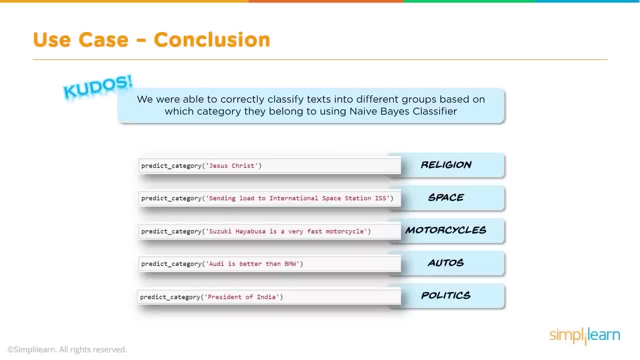 And it's really useful for understanding the industry and data science. And we can see our categorizer, our Naive Bayes classifier. We were able to predict the category- religion, space, motorcycles, autos, politics- and properly classify all these different things we pushed into our prediction. 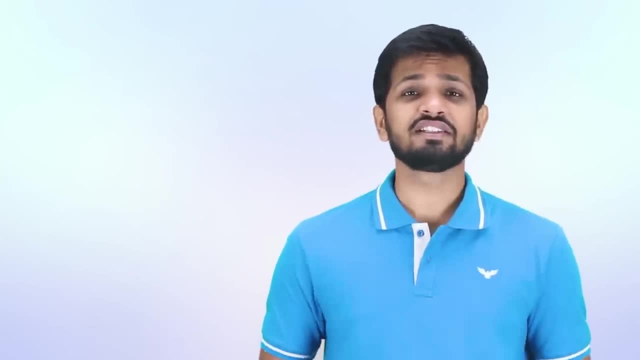 and our trained model. Thanks again, Richard, That was great. That brings us to the end of this comprehensive look at machine learning and its algorithms. Now we have Rahul, who will take you through the various aspects of machine learning and how you can be a machine learning. 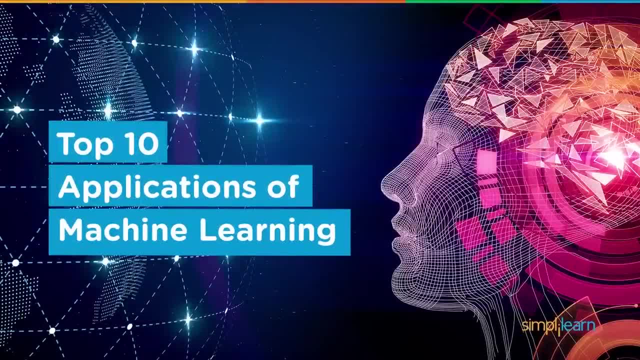 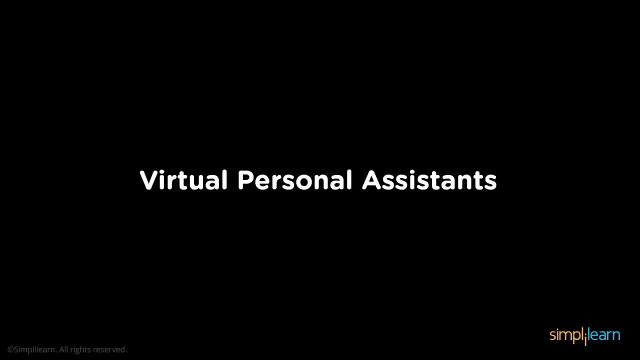 engineer MACHINE LEARNING. Machine learning has improved our lives in a number of wonderful ways. Today, let's talk about some of these. I'm Rahul from Simply Learn, and these are the top 10 applications of machine learning. First, let's talk about virtual personal assistants. 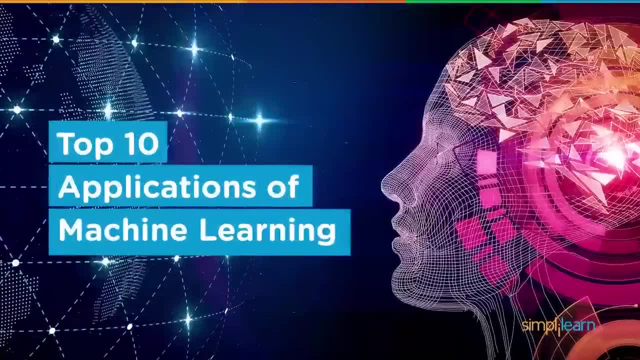 and how you can be a machine learning engineer. machine learning has improved our lives in a number of wonderful ways. today, let's talk about some of these. I'm Rahul from simply learn, and these are the top ten applications of machine learning. first, let's talk about virtual personal. 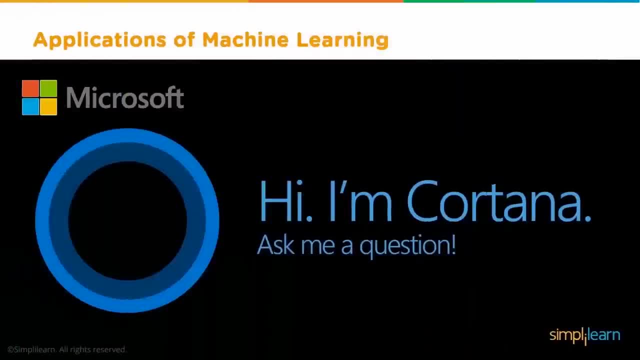 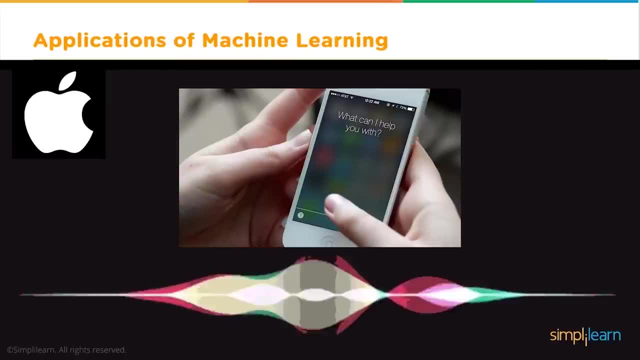 assistants- Google assistant, Alexa, Cortana and Siri. now, we've all used one of these at least at some point in our lives. now, these help improve our lives in a great number of ways. for example, you could tell them to call someone. you could tell them to play some music. you. 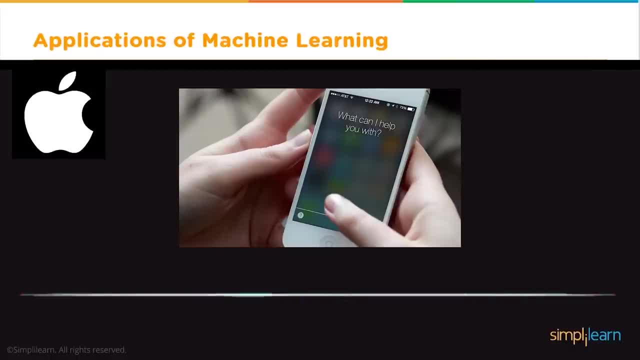 could tell them to even schedule an appointment. so how do these things actually work? first they record whatever you're saying, send it over to a server, which is usually in a cloud, decode it with the help of machine learning and neural networks, and then provide you with an output. so if you've ever noticed, 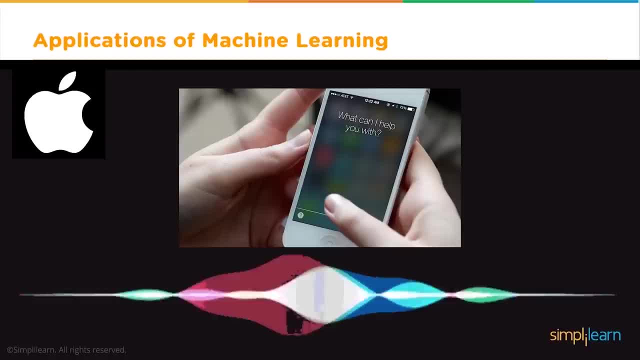 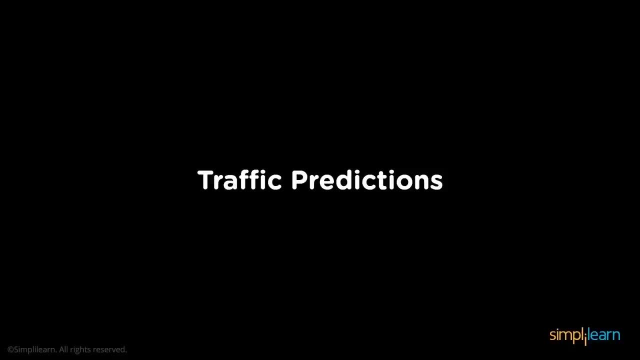 that these systems don't work very well without the internet. that's because the server couldn't be contacted. next, let's talk about traffic predictions. now, say I wanted to travel from Buckingham palace to Lord's cricket ground, the first thing I'd probably do is to get on Google Maps. 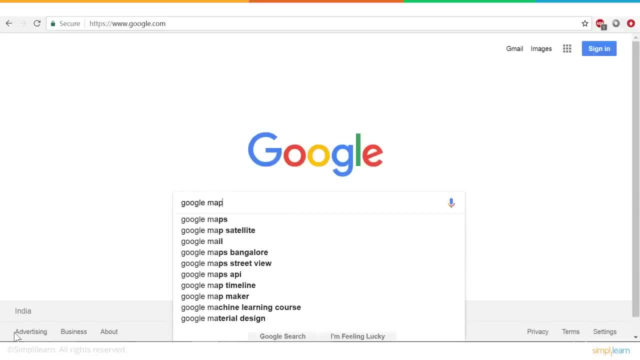 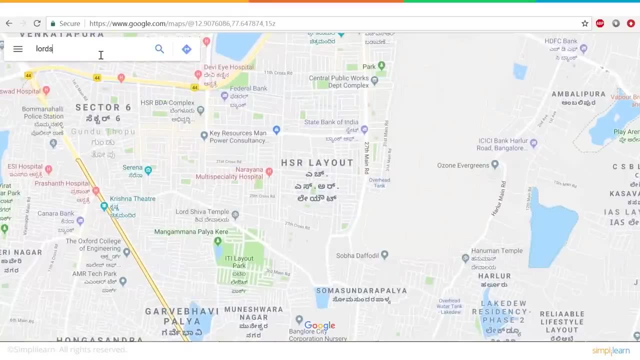 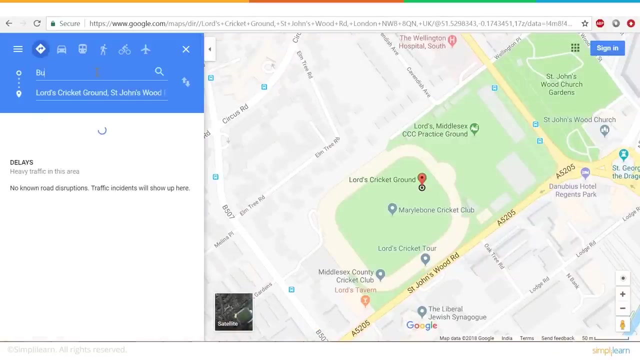 so search it and let's put it here. so here we have the path you should take to get to Lord's cricket ground. now, here the map is a combination of red, yellow and blue, but the blue regions signify a clear road, that is, you won't encounter traffic there. 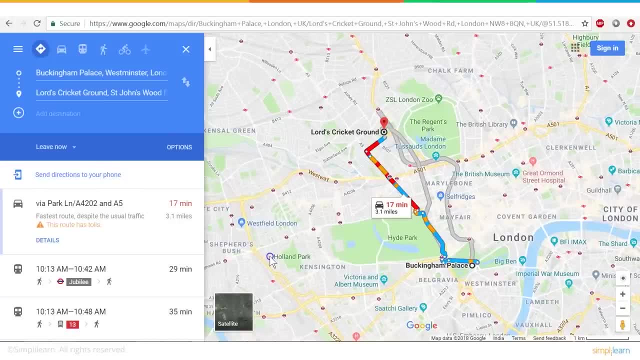 the yellow indicate that they're slightly congested and red means they're heavily congested. so let's look at the map- a different version of the same map- and here, as I told you before, you can see that there's a lot of traffic there. there's a lot of traffic there, so let's. 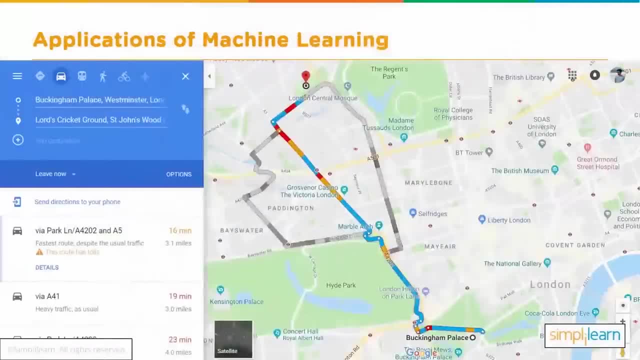 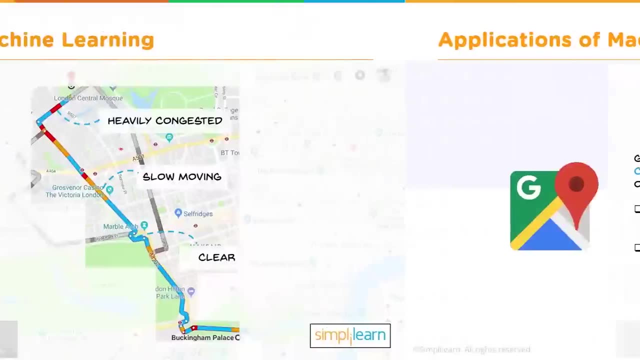 look at the map- a different version of the same map- and here, as I told you before, there's a lot of traffic there. red means heavily congested, yellow means slow moving and blue means clear. so how exactly is Google able to tell you that the traffic is? 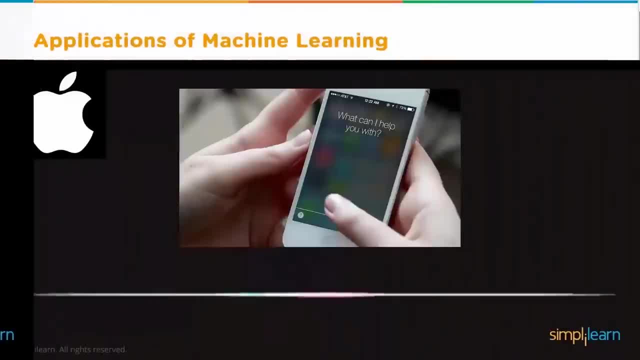 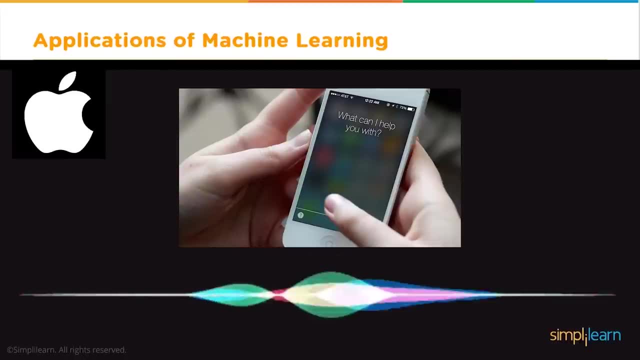 Google Assistant, Alexa, Cortana and Siri. Now, we've all used one of these at least at some point in our lives. Now, these help improve our lives in a great number of ways. For example, you could tell them to call someone. 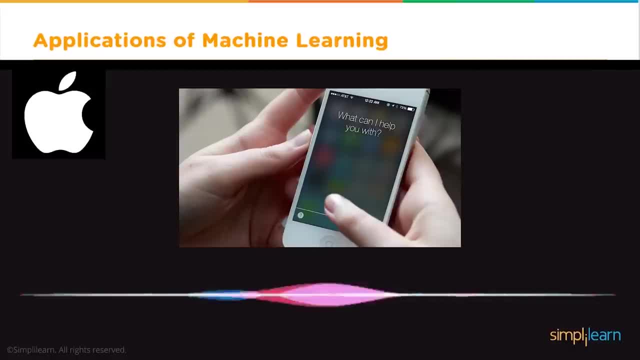 You could tell them to play some music. You could tell them to even schedule an appointment. That's it. So how do these things actually work? First, they record whatever you're saying, send it over to a server, which is usually in a cloud, decode it with the. 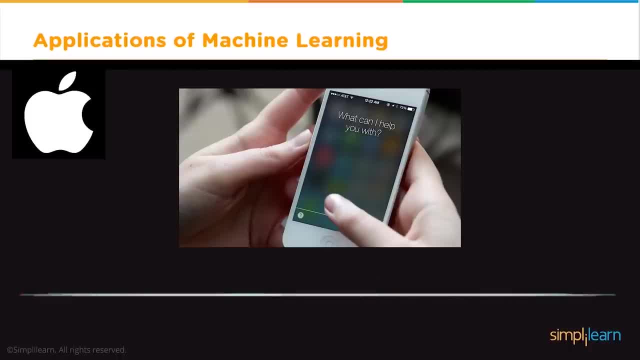 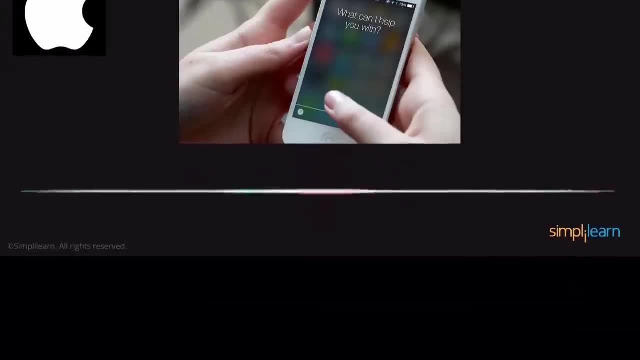 help of machine learning and neural networks and then provide you with an output. So if you ever notice that these systems don't work very well without the internet, that's because the server couldn't be contacted. Next, let's talk about traffic predictions. 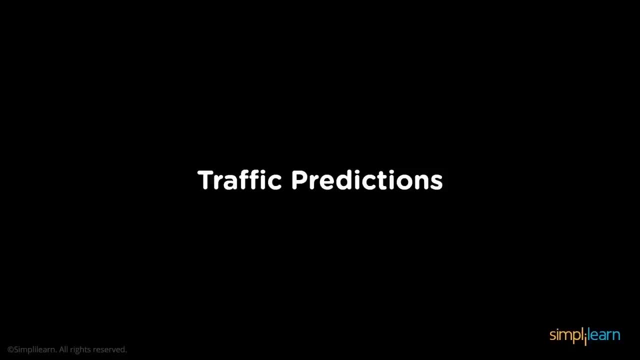 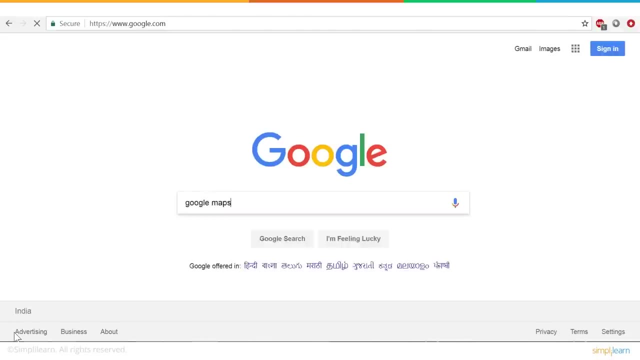 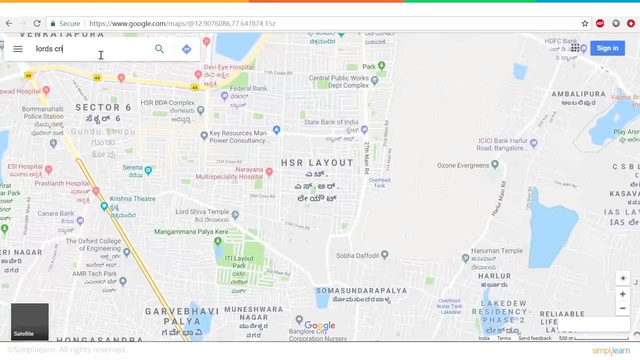 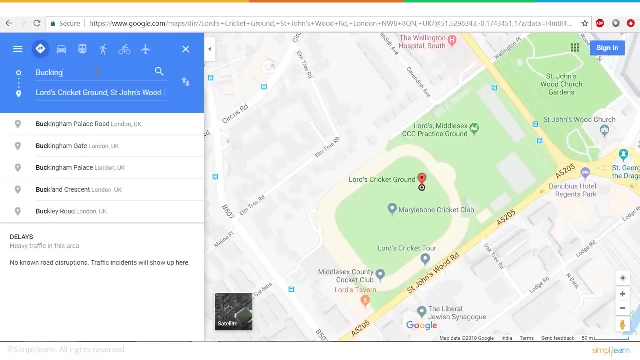 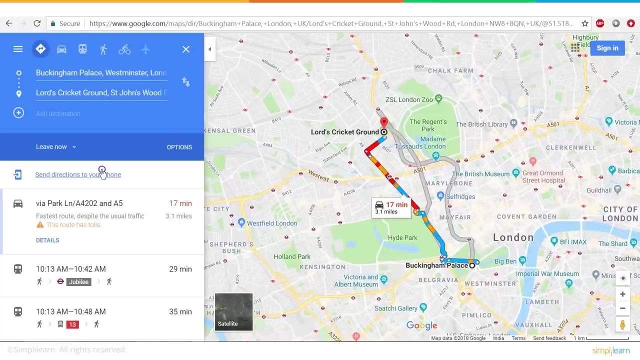 Now say I wanted to travel from Buckingham Palace to Lord's Cricket Ground, The first thing I would probably do is to get on Google Maps, So search it And let's put it here. So here we have the path you should take to get to Lord's Cricket Ground. 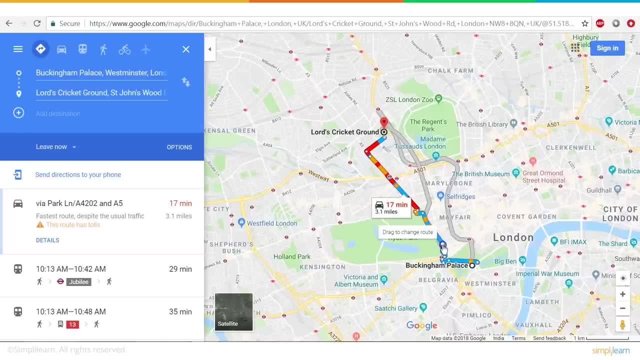 Now here, the map is a combination of red, yellow and blue, But the blue regions signify a clear road, That is, you won't encounter traffic there. The yellow indicate that they're slightly congested And red means they're heavily congested. 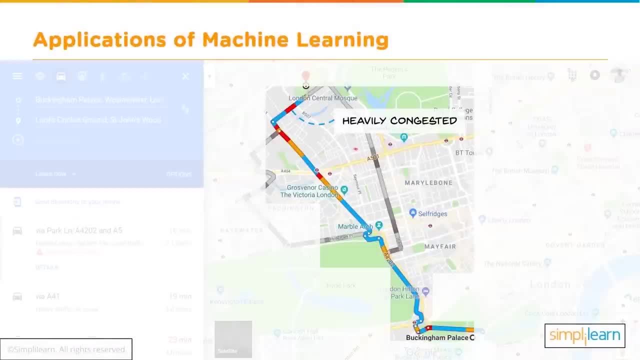 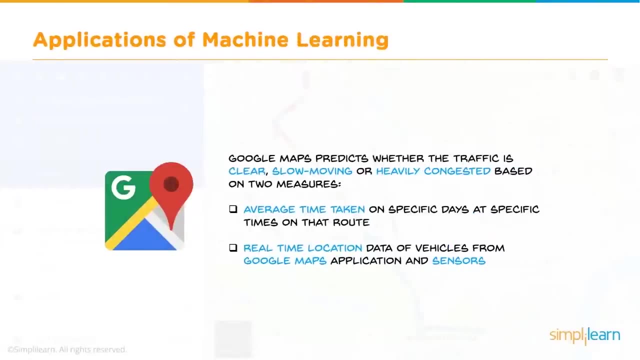 So let's look at the map, a different version of the same map, And here, as I told you before, red means heavily congested, yellow means slow moving and blue means clear. So how exactly is Google able to tell you that the traffic? 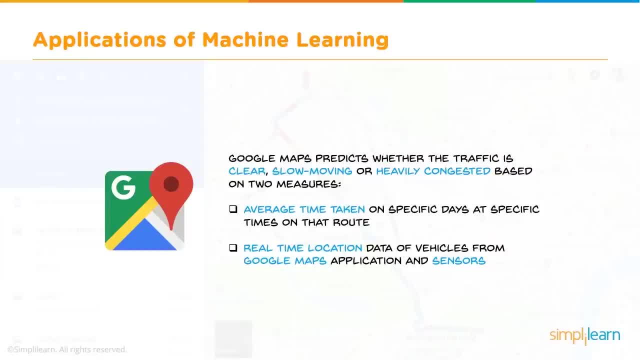 is clear, slow moving or heavily congested. So this is with the help of machine learning and with the help of two important measures. First is the average time that's taken on specific days at specific times on that route. The second is the average time that's taken on specific days at specific times on that route. 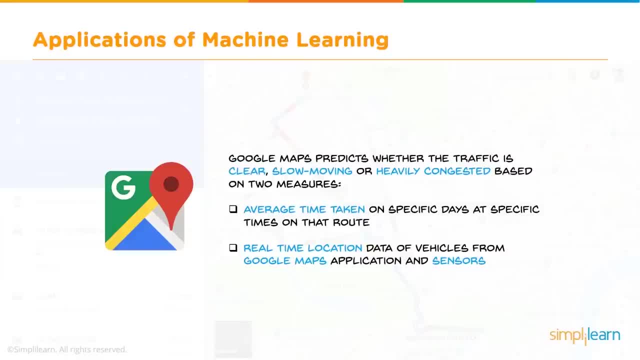 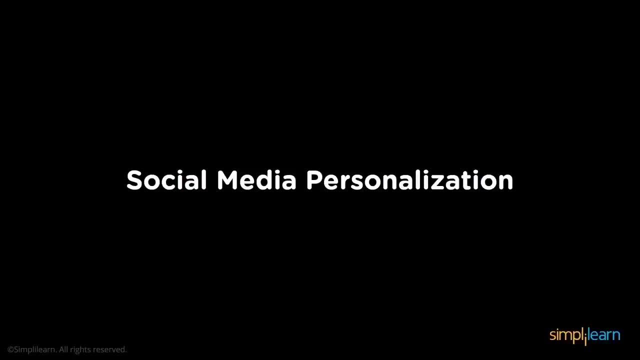 The second one is the real-time location data of vehicles from Google Maps and with the help of sensors. Some of the other popular map services are Bing Maps, Mapsme, and here we go. Next up, we have social media personalization. So, say, I want to buy a drone and I'm on Amazon. 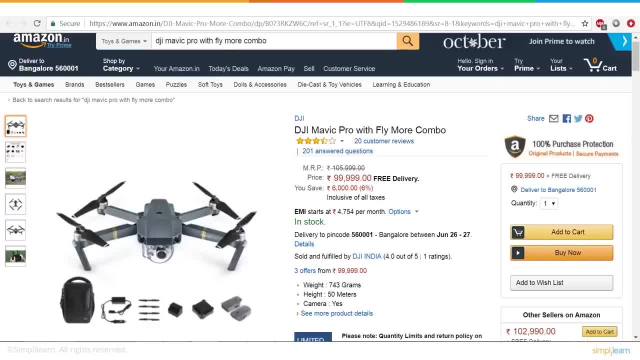 and I want to buy a DJI Mavic Pro. The thing is, it's close to one lap, so I don't want to buy it right now, But the next time I'm on Facebook I'll see an advertisement for the product. 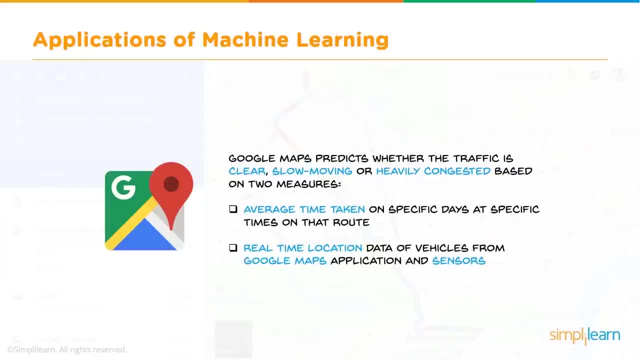 clear, slow moving or heavily congested. so this is with the help of machine learning and with the help of two important measures. first is the average time that's taken on specific days at specific times on that route. the second one is the real time location data of vehicles from: 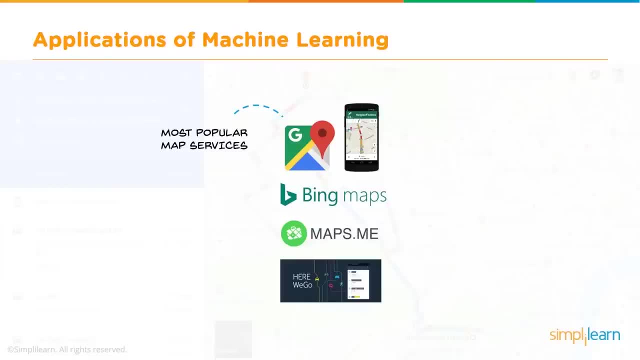 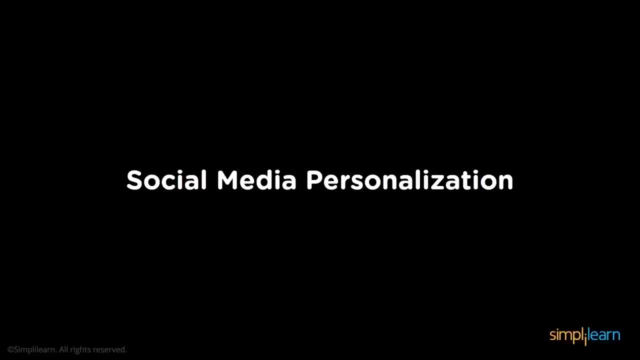 Google Maps and with the help of sensors. some of the other popular map services are Bing Maps, Mapsme, and here we go. next up, we have social media personalization. so say, I want to buy a drone and I'm on Amazon and I want to buy a DJI Mavic Pro. 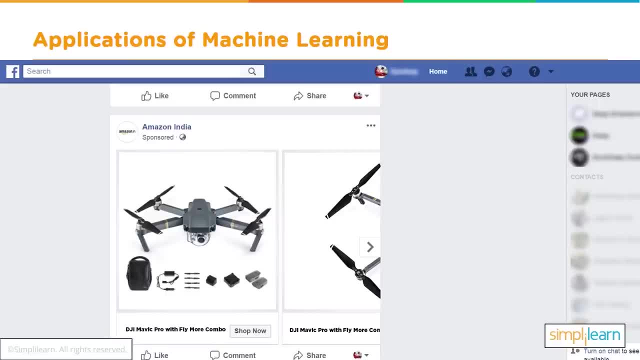 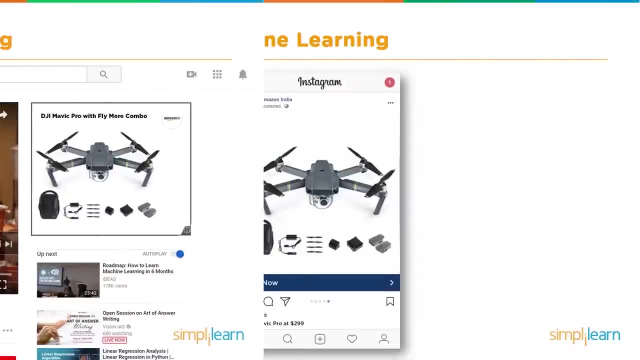 the thing is it's close to one lap, so I don't want to buy it right now, but the next time I'm on Facebook, I'll see an advertisement for the product. next time I'm on YouTube, I'll see an advertisement. even on Instagram I'll see an advertisement. so here, with the help of 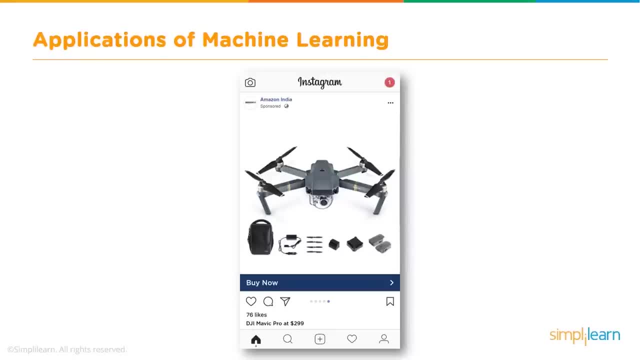 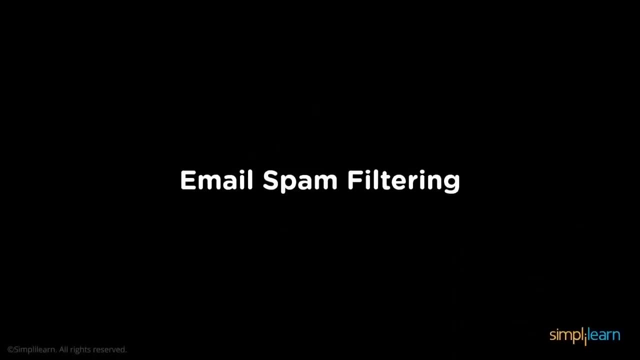 machine learning. Google has understood that I'm interested in this particular product. hence it's targeting me with these advertisements. this is also with the help of machine learning. let's talk about email spam filtering. now, this is a spam that's in my inbox now. how does Gmail know? 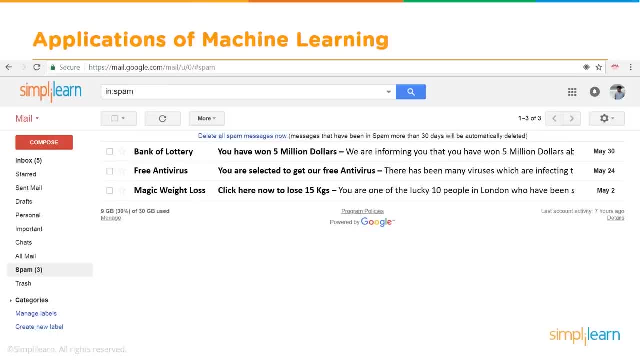 what's spam and what's not spam. so Gmail has an entire collection of emails which have already been labeled as spam or not spam. so after analyzing this data, Gmail is able to find some characteristics like the word lottery or winner. from then on, any new email that comes to your inbox goes. 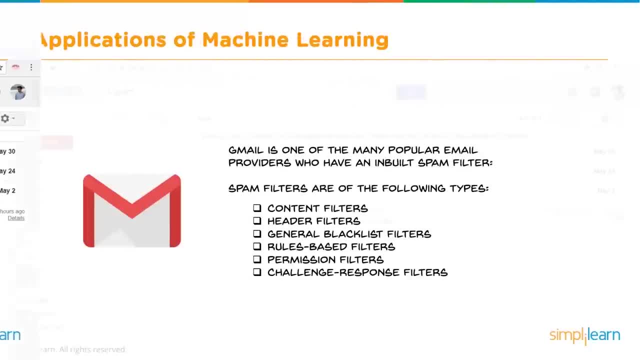 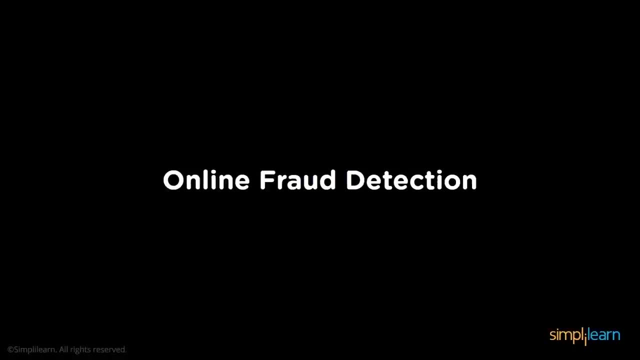 through a few spam filters to decide whether it's spam or not. now some of the popular spam filters that Gmail uses is content filters, header filters, general blacklist filters, and so on. next, we have online fraud detection. now there are several ways that online fraud can take place. for example, there's: 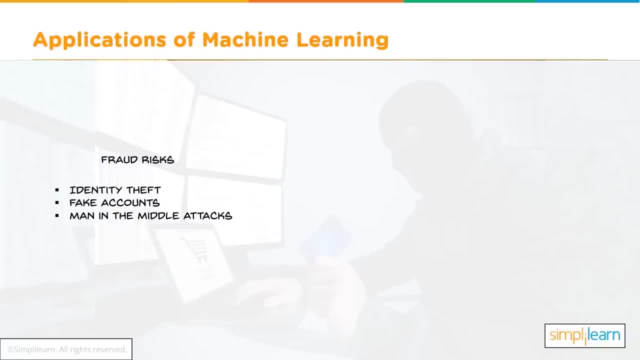 identity theft, where they steal your identity. fake accounts, where these accounts only last for how long the transaction takes place and stop existing after that. and man in the middle attacks, where they steal your money while the transaction is taking place. the feed forward neural network helps determine whether a 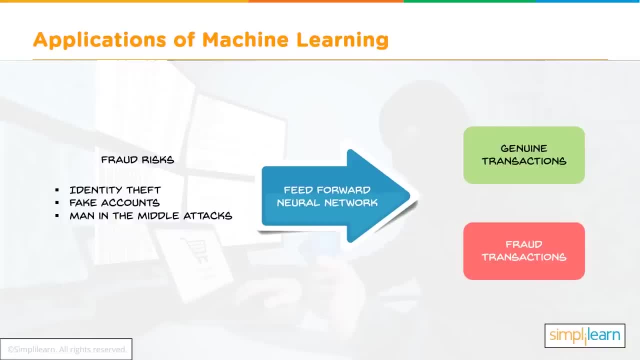 transaction is genuine or fraudulent. so what happens with feed forward neural networks are that the outputs are converted into hash values and these values become the inputs for the next round. so for every real transaction that takes place, there's a specific pattern. a fraudulent transaction would stand out because of the 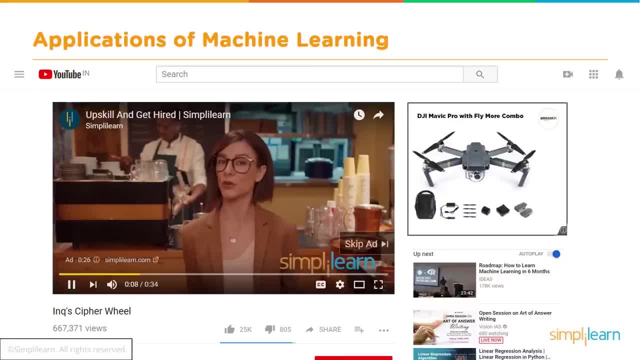 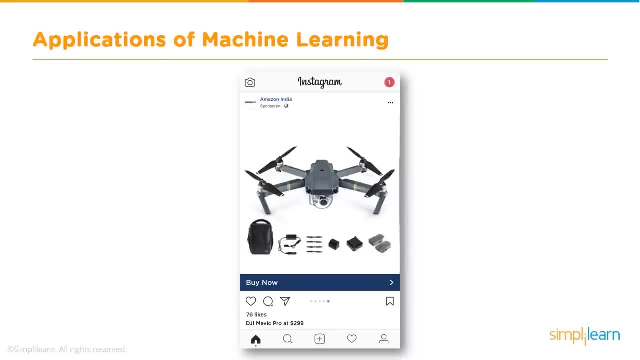 Next time I'm on YouTube, I'll see an advertisement. Even on Instagram, I'll see an advertisement. So here, with the help of machine learning, Google has understood that I'm interested in this particular product. Hence it's targeting me with these advertisements. 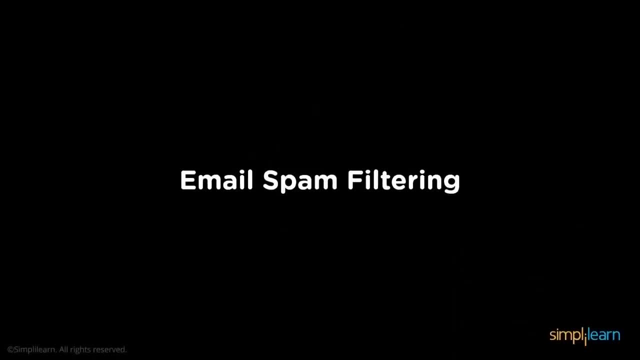 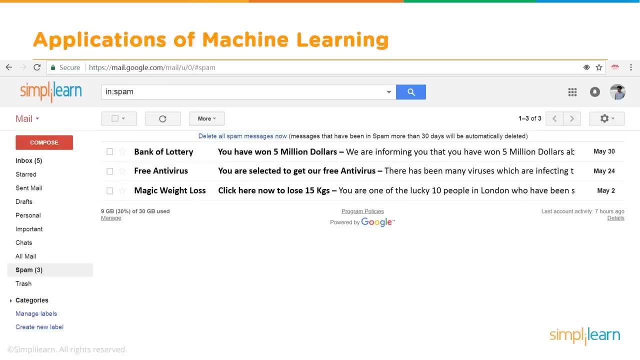 This is also with the help of machine learning. Let's talk about email spam filtering. Now this is the spam that's in my inbox. Now, how does Gmail know what's spam and what's not spam? So Gmail has an entire collection of emails. 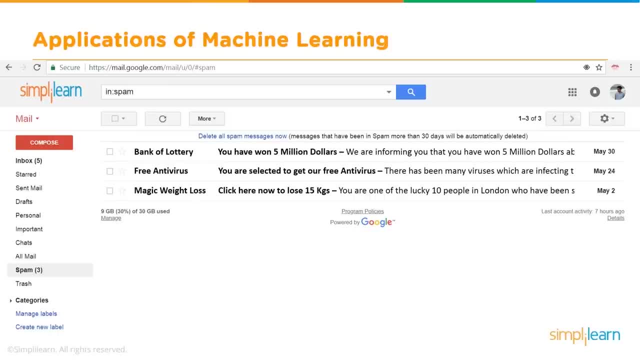 which have already been labeled as spam or not spam. So, after analyzing this data, Gmail is able to find some characteristics like the word lottery or winner. From then on, any new email that comes to your inbox goes through a few spam filters to decide whether it's spam or not. 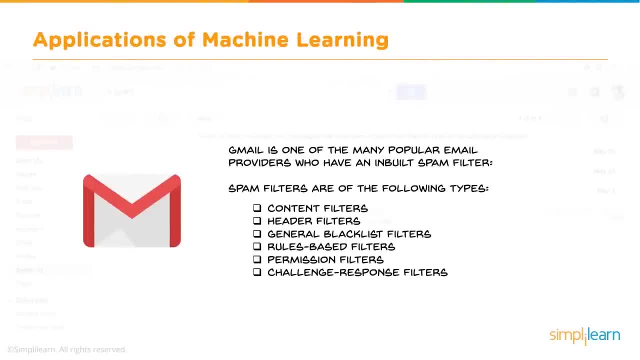 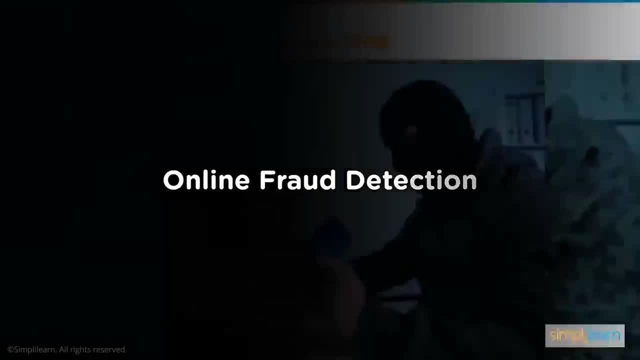 Now some of the popular spam filters that Gmail uses is content filters, header filters, general blacklist filters and so on. Next, we have online fraud detection. Now there are several ways that online fraud can take place. For example, there's identity theft, where they steal your identity. 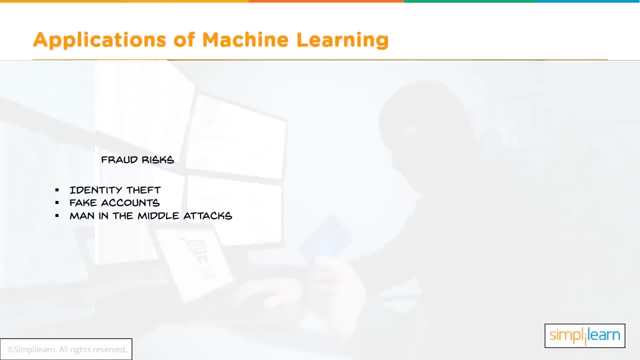 Fake accounts, where these accounts only last for how long the transaction takes place and stop existing after that. And man-in-the-middle attacks, where they steal your money while the transaction is taking place. The feed-forward neural network helps to determine whether a transaction is genuine or fraudulent. 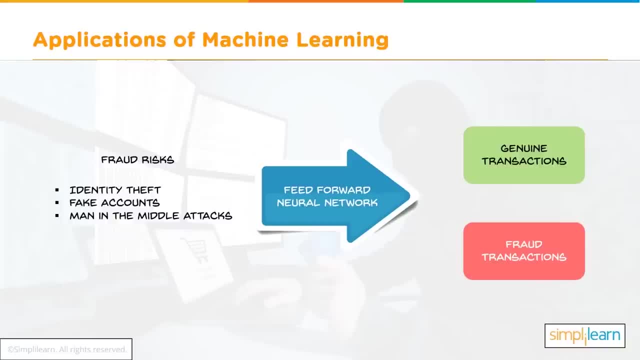 So what happens with feed-forward neural networks are that the outputs are converted into hash values and these values become the inputs for the next round. So for every real transaction that takes place, there's a specific pattern. A fraudulent transaction would stand out. 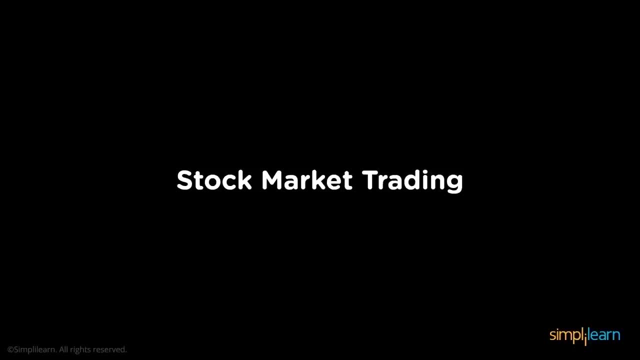 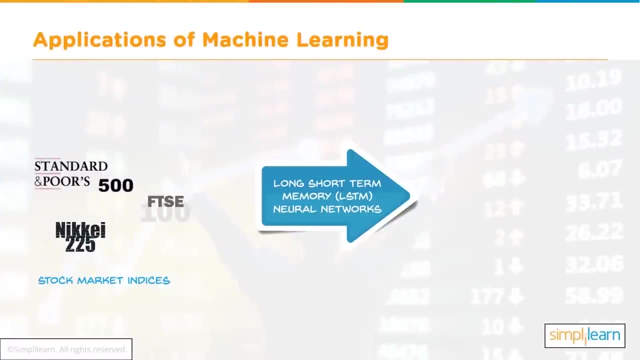 because of the significant changes that it would cause with the hash values. Stock market trading. Machine learning is used extensively when it comes to stock market trading. Now you have stock market indices like Nikkei. They use long short-term memory neural networks. 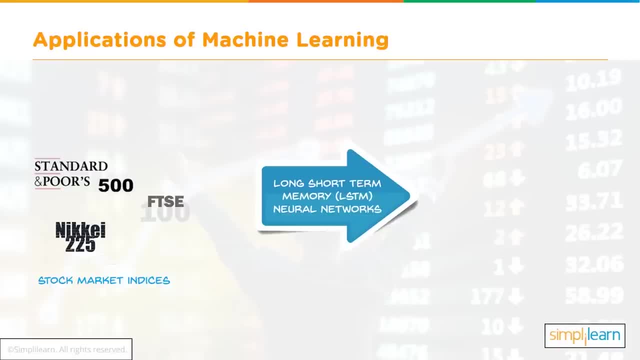 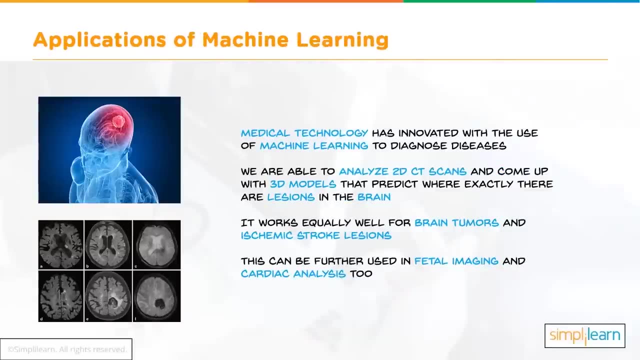 Now these are used to classify, process and predict data when there are time lags of unknown size and duration. Now this is used to predict stock market trends. Assistive medical technology: Now medical technology has been innovated with the help of machine learning. 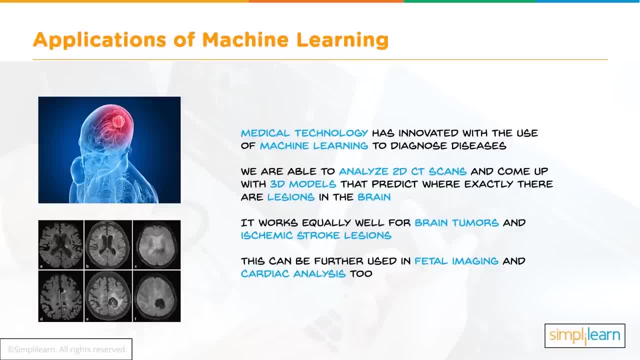 diagnosing diseases has been easier, from which we can create 3D models that can predict where exactly there are lesions in the brain. It works just as well for brain tumors and ischemic stroke lesions. They can also be used in fetal imaging and cardiac analysis. 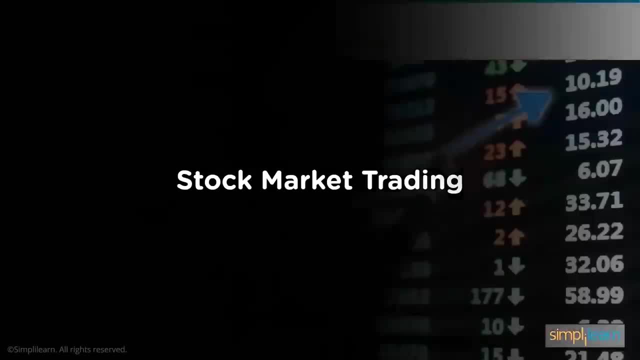 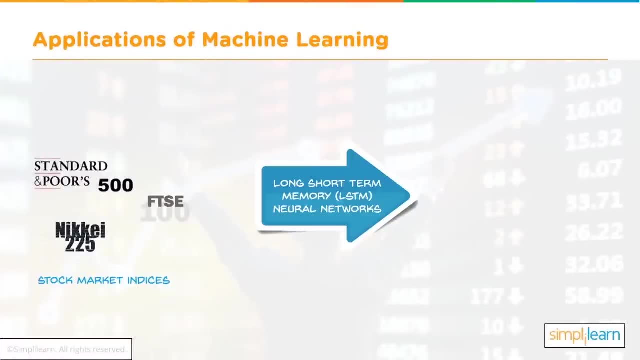 significant changes that it would cause with the hash values. stock market trading. machine learning is used extensively when it comes to stock market trading. now you have stock market indices like Nikkei. they use long short-term memory neural networks. now these are used to classify, process and predict data when there are time lags. 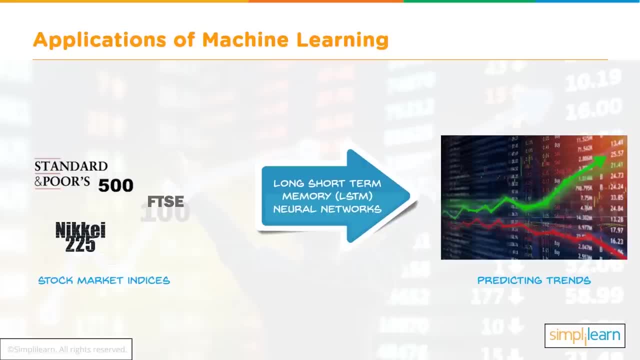 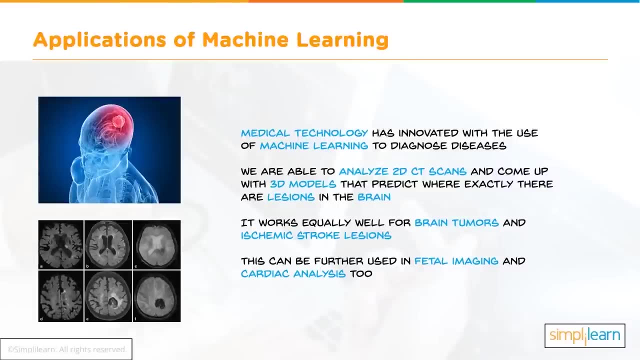 of unknown size and duration. now this is used to predict stock market trends. assistive medical technology: now medical technology has been innovated. with the help of machine learning, diagnosing diseases has been easier, from which we can create 3d models that can predict where exactly there are lesions in the brain. 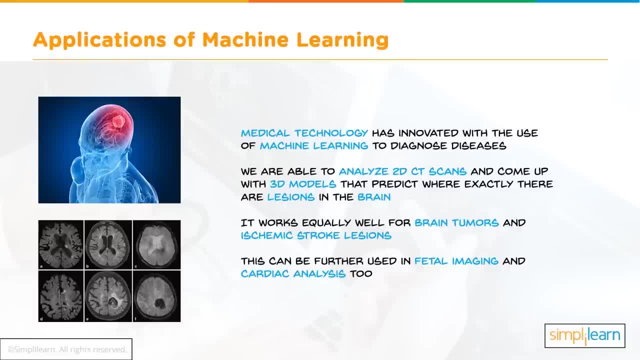 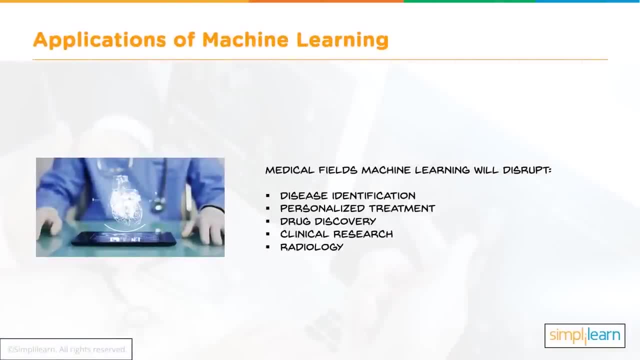 it works just as well for brain tumors and ischemic stroke lesions. they can also be used in fetal imaging and cardiac analysis. now, some of the medical fields that machine learning will help assist in is disease identification, personalized treatment, drug discovery, clinical research and radiology. and finally, we have 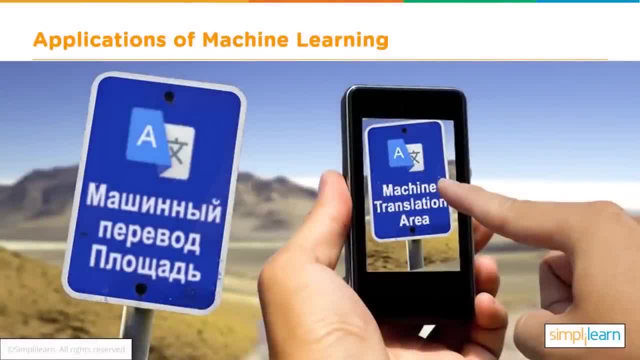 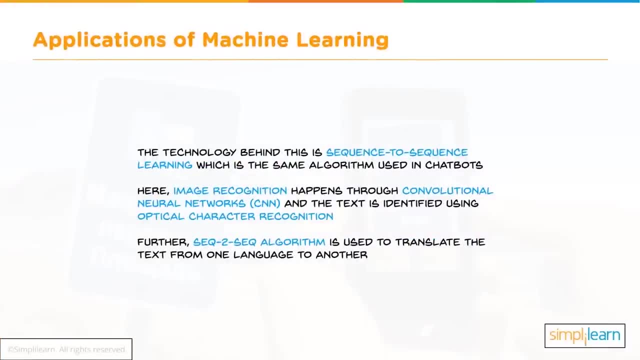 automatic translation. now say, you're in a foreign country and you see billboards and signs that you don't understand. that's where automatic translation comes of help. now, how does automatic translation actually work? the technology behind it is the same as the sequence to sequence learning, which is the same thing, that's. 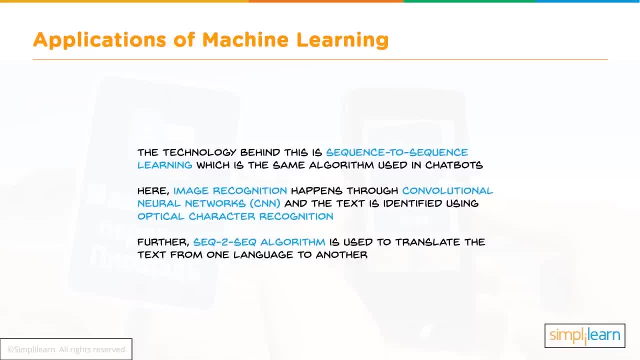 used with chatbots. here the image recognition happens using convolutional neural networks and the text is identified using optical character recognition. furthermore, the sequence to sequence algorithm is also used to translate the text from one language to the other, and today I'm going to tell you how you can. 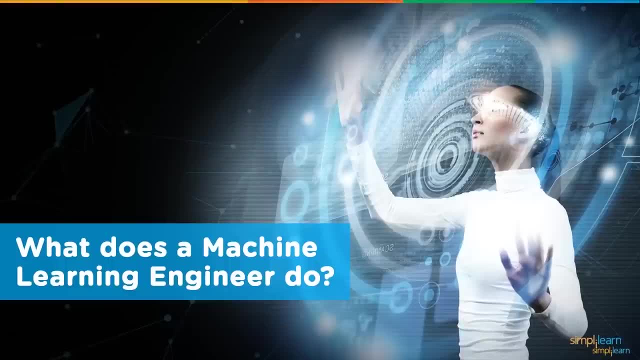 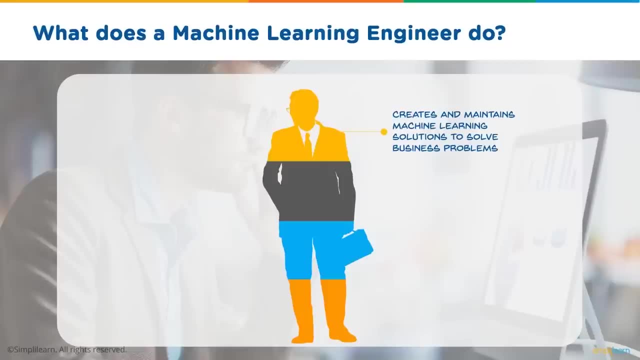 become a machine learning engineer. but before we begin, let me tell you what a machine learning engineer actually does. a machine learning engineer creates and maintains machine learning solutions to solve business problems. they constantly tweak and optimize the solutions for maximum performance and scalability. they solve business problems like reducing customer. 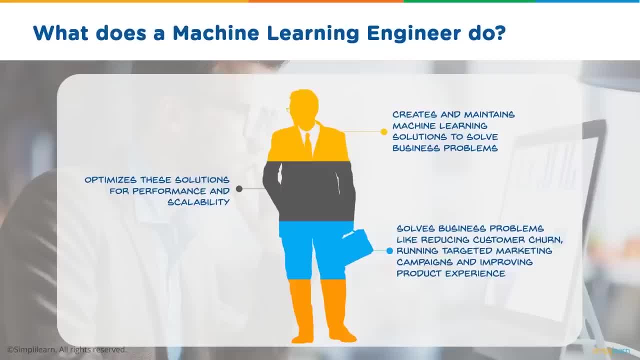 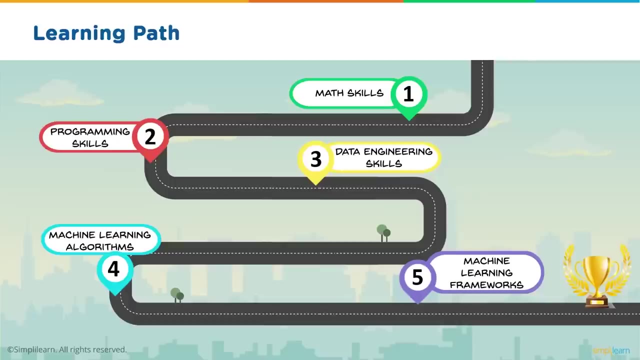 churn, running targeted marketing campaigns and improving product experience. they also help with predicting whether a particular hypothesis will be profitable in the future. they contribute to cutting-edge research in AI and machine learning. now, before you can start off on your journey to becoming a machine learning engineer, there's a 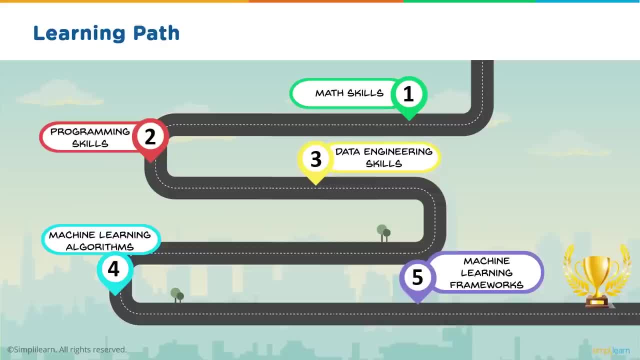 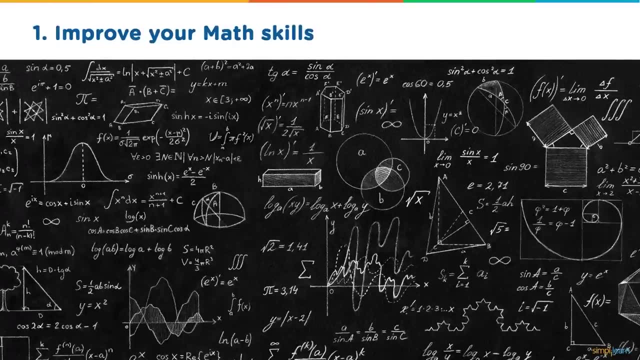 certain number of steps that you need to follow on this learning path. your first step is to improve your math skills. mathematics plays a very important role in helping you understand how machine learning and its algorithms work. among the many concepts that you need to understand, three of the most important: 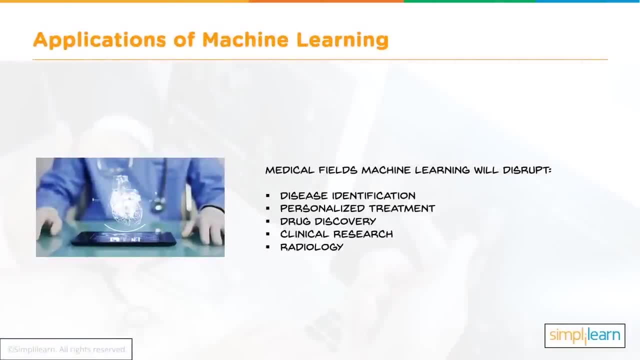 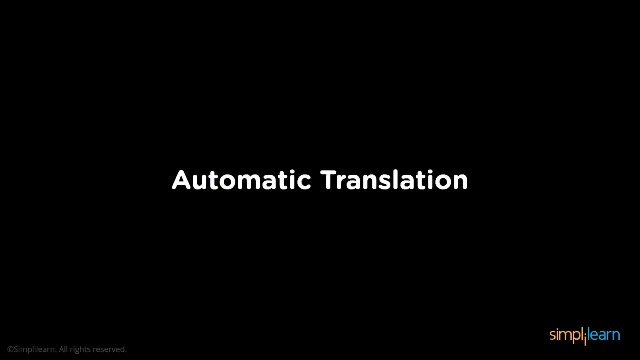 Now, some of the medical fields that machine learning will help assist in is disease identification, analyzed treatment, drug discovery, clinical research and radiology, And finally, we have automatic translation. Now say: you are in a foreign country and you see. 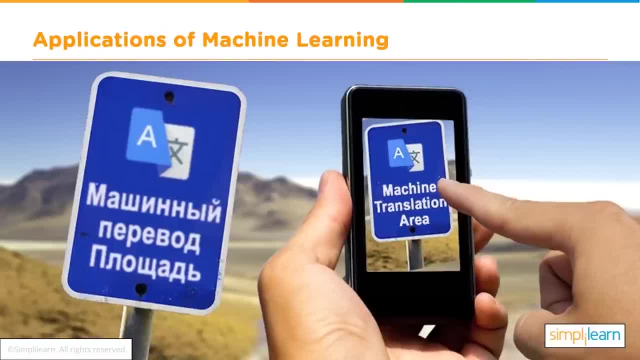 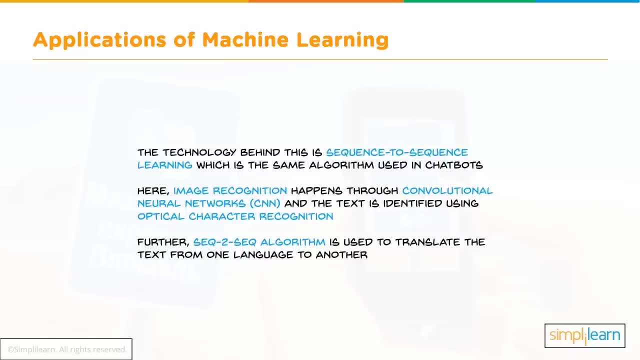 billboards and signs that you don't understand. That's where automatic translation comes of help. Now, how does automatic translation actually work? The technology behind it is the same as the sequence-to-sequence learning, which is the same thing that's used with chatbots. 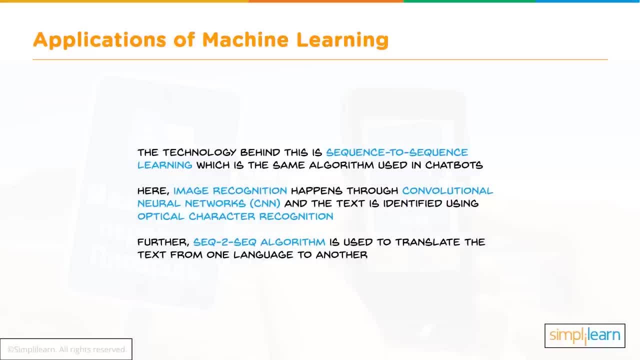 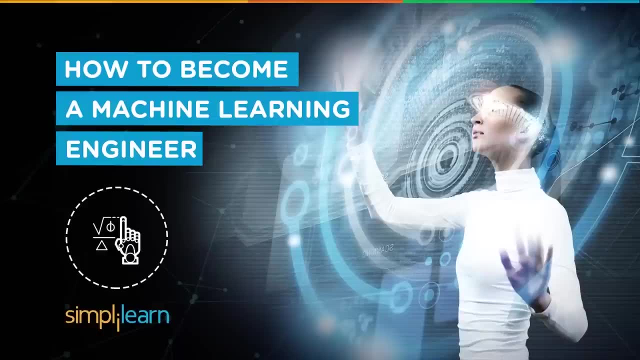 Here, the image recognition happens using convolutional neural networks and the text is identified using optical character recognition. Furthermore, the sequence-to-sequence algorithm is also used to translate the text from one language to another, And today I'm going to tell you how you can become. 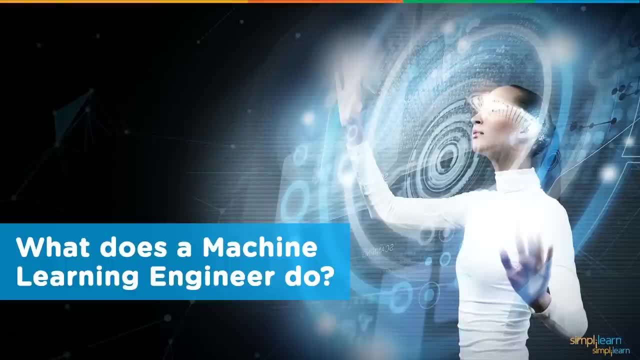 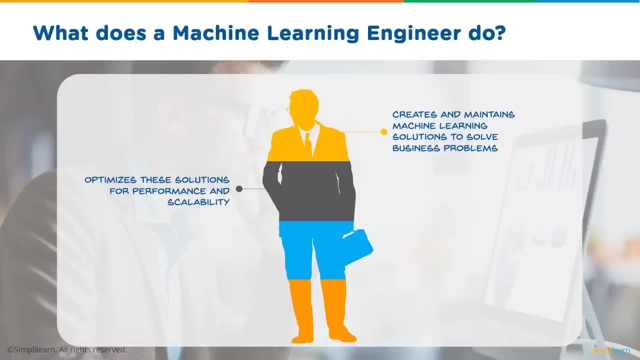 a machine learning engineer. But before we begin, let me tell you what a machine learning engineer actually does. A machine learning engineer creates and maintains machine learning solutions to solve business problems. They constantly tweak and optimize the solutions for maximum performance and scalability. They solve business problems like: 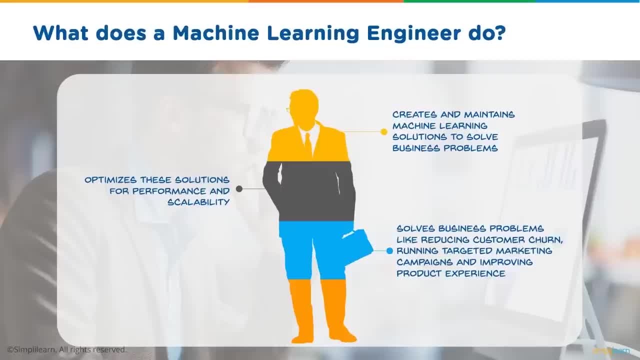 reducing customer churn, running targeted marketing campaigns and improving product experience. They also help with predicting whether a particular hypothesis will be profitable in the future. They contribute to cutting-edge research in AI and machine learning. Now, before you can start off on your journey. 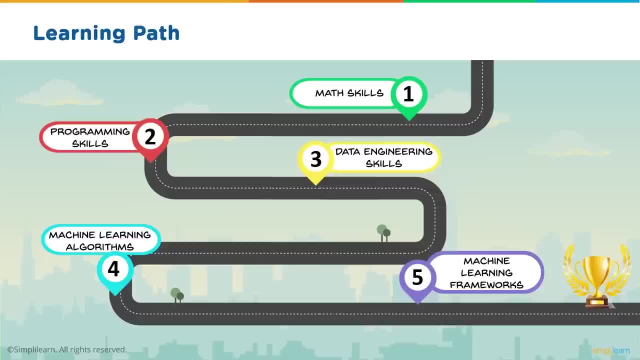 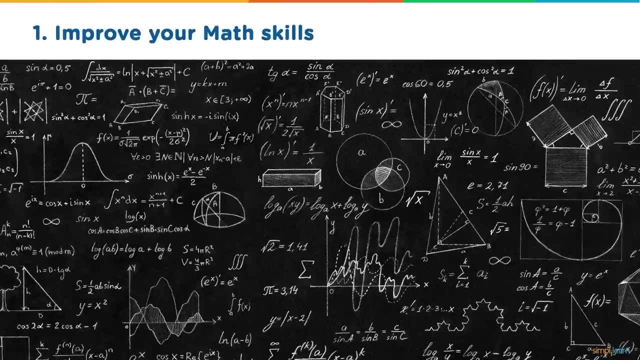 to becoming a machine learning engineer. there's a certain number of steps that you need to follow On this learning path. your first step is to improve your math skills. Mathematics plays a very important role in helping you understand how machine learning and its algorithms work. 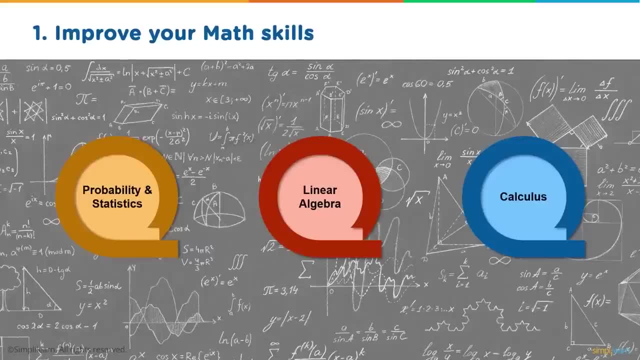 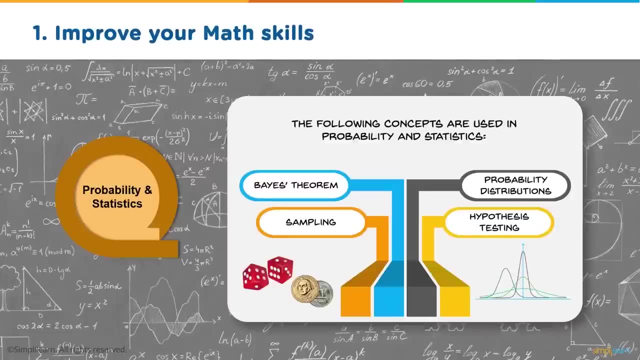 Among the many concepts that you need to understand, three of the most important ones are probability and statistics, linear algebra and calculus. Let's have a detailed look at probability and statistics. Firstly, you have the Bayes theorem. This is used in the Naive Bayes algorithm. 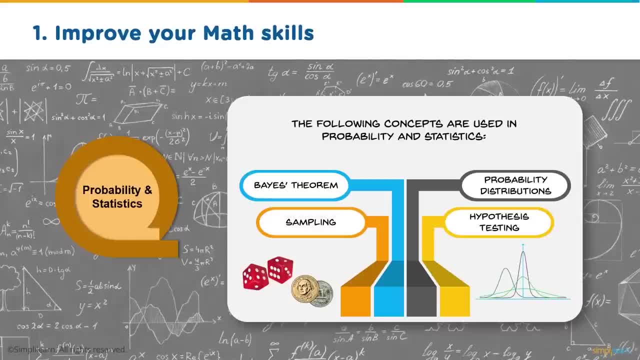 to help categorize your data. Then we have probability distribution. This helps you determine how frequently a particular event will take place. For example, you can determine what your premium for your insurance will be based on the probability distribution of expenditure pertaining to insurance claims. 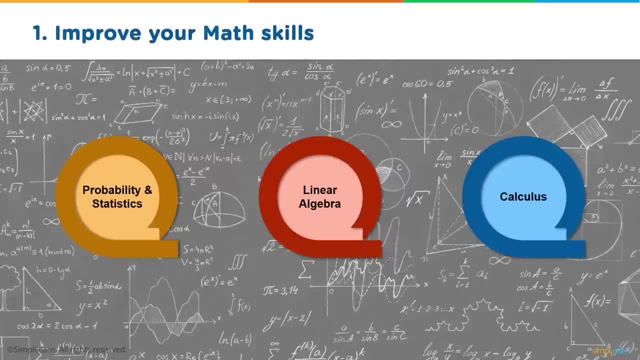 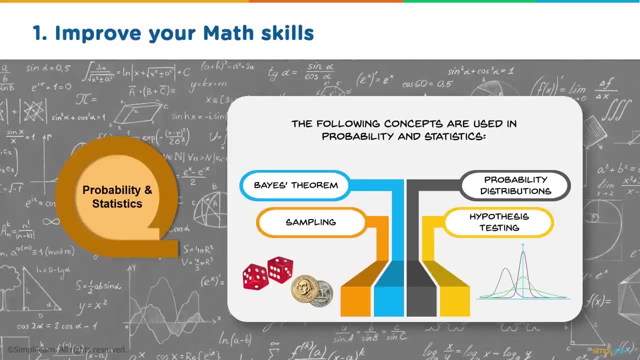 ones are probability and statistics, linear algebra and calculus. now let's have a detailed look at probability and statistics. firstly, you have the base theorem. this is used in the nav base algorithm to help categorize your data. then we have probability distribution. this helps you determine how frequently 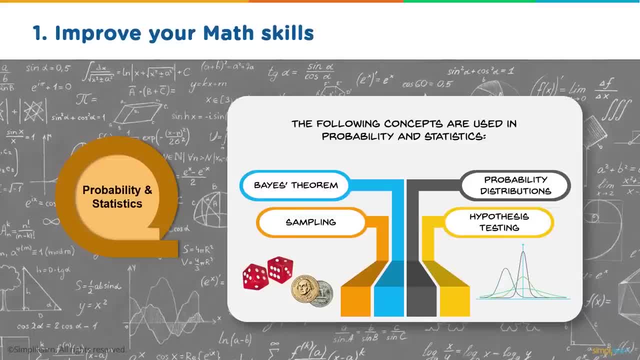 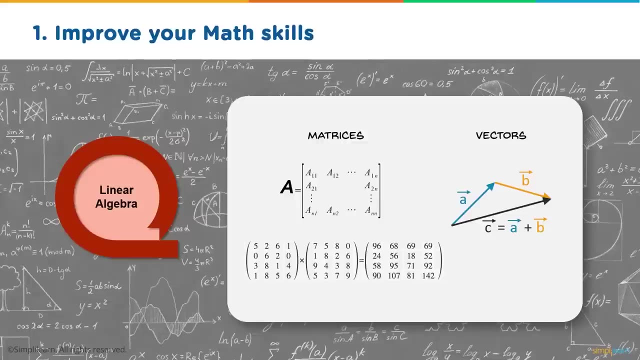 a particular event occurs in, the particular event will take place. for example, you can determine what your premium for your insurance will be based on the probability distribution of expenditure pertaining to insurance claims. you must also learn how sampling and hypothesis testing works. now let's look at linear algebra- now linear. 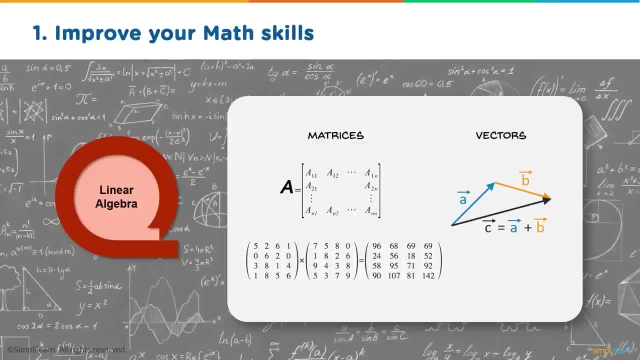 algebra has two main concepts: matrices and vectors. they both use widely in machine learning. now, matrices are used for image recognition, where the entire image that you're using is already in the form of a matrix. you need to be able to work with matrices, perform simple calculations like addition, subtraction. 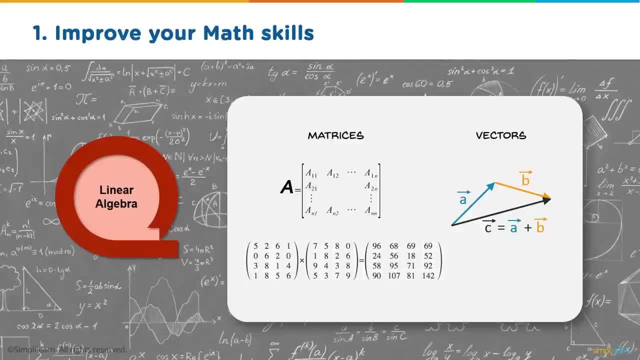 multiplication, inverse, transpose and so on. now the recommender systems that you see in applications like netflix or amazon actually work on vectors. this vector is the customer behavior vectors, and they use distance measures. now let's have a closer look at calculus. you have differential calculus and integral. 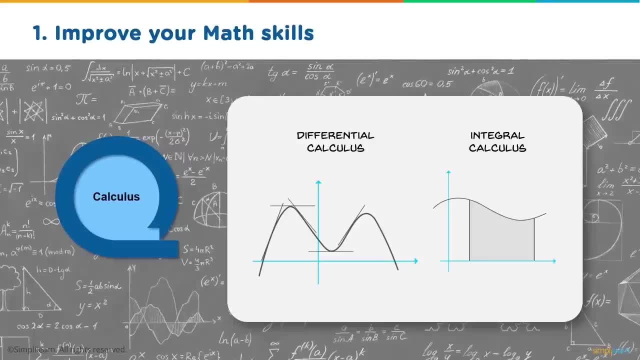 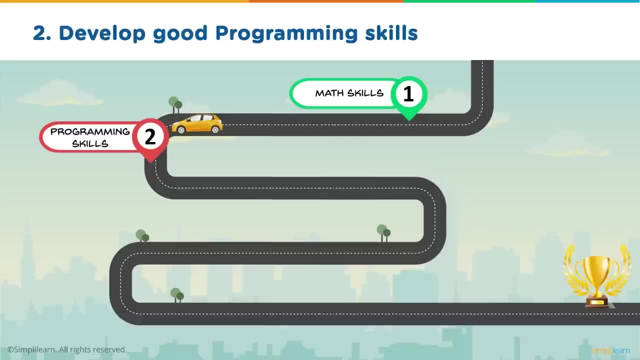 calculus. now these help in determining the probability of events, for example, in finding the posterior probability in a nav base model. in your next step to becoming a machine learning engineer, you need to develop good programming skills, and let me tell you, there are a huge number of options from which you 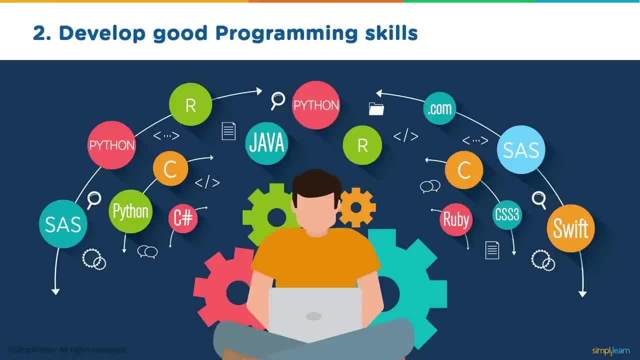 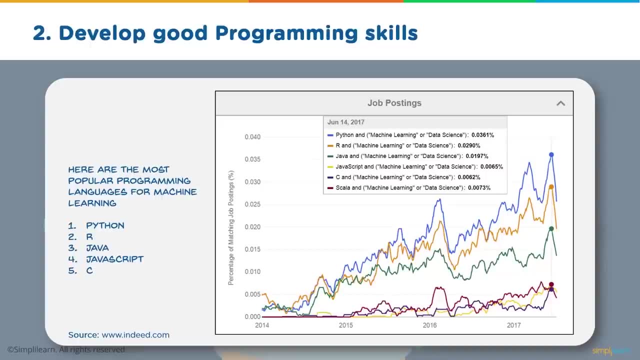 can choose: there's python, there's c, there's c sharp this java, and so much more. now here's a graph of the job postings from 2014 to 2017, and you can see that there are two languages that dominate since 2015: python and r. now, 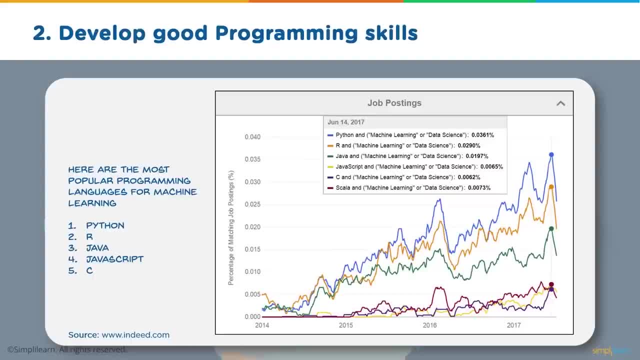 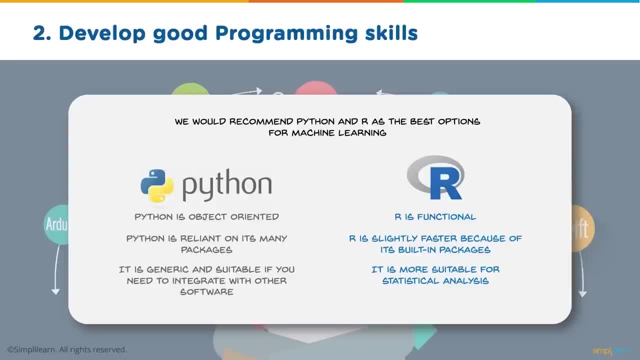 these are one of the most wanted languages when it comes to machine learning engineers. these are closely followed by javascript and c. hence, we would like to recommend that you learn python and r, as they're the best options when it comes to coding in machine learning algorithms. so here are. 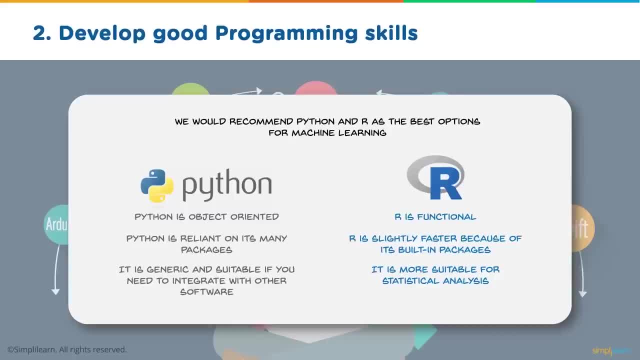 a few things that you need to know about python and r. python is an object-oriented language, which means their main emphasis is on the object. r is a functional language, which means their emphasis is on creating and manipulating functions. python relies on its many packages and r is slightly. 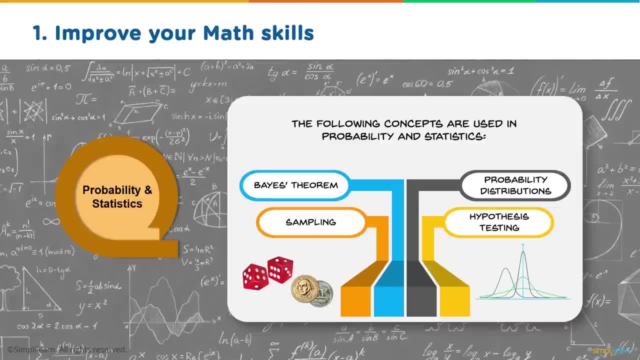 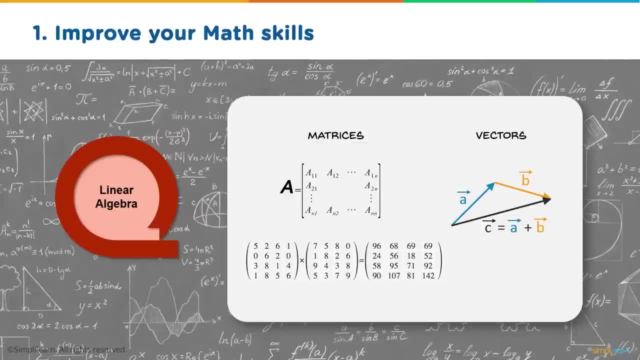 You must also learn how sampling and hypothesis testing works. Now let's look at linear algebra. Now, linear algebra has two main concepts: Metric and vectors. They're both used widely in machine learning. Now, matrices are used for image recognition, where the entire image that you're using 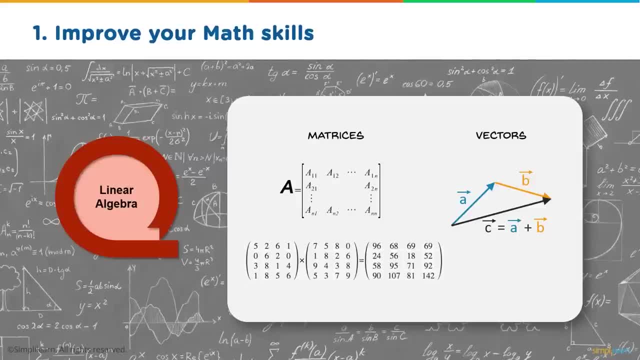 is already in the form of a matrix. You need to be able to work with matrices, perform simple operations like addition, subtraction, multiplication, inverse, transpose and so on. Now the recommended systems that you see in applications like Netflix or Amazon actually work on vectors. 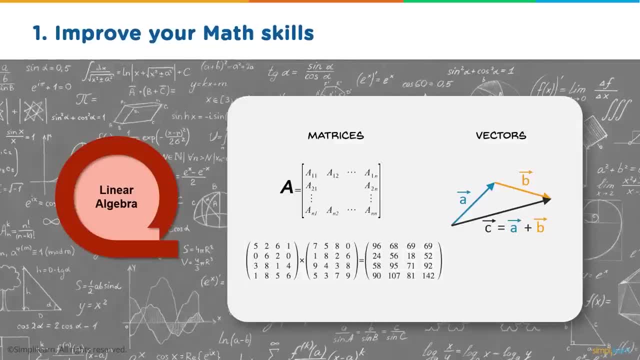 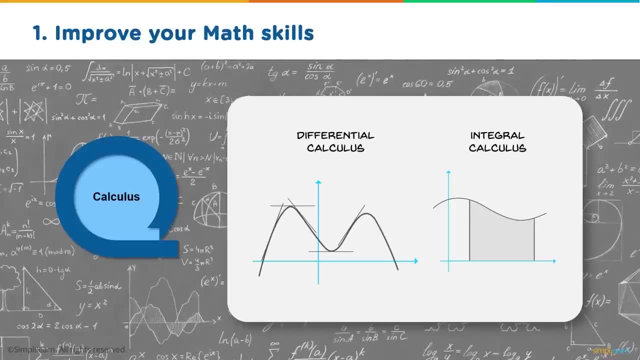 This vector is the customer behavior vector, and they use distance measures. Now let's have a closer look at calculus. You have differential calculus and integral calculus. Now these help in determining the probability of events, For example, in finding the posterior probability in a nav-based model. 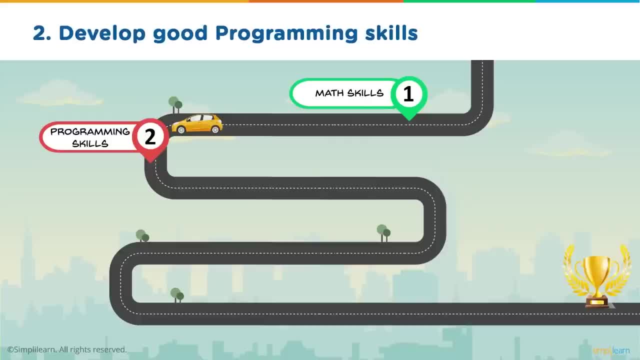 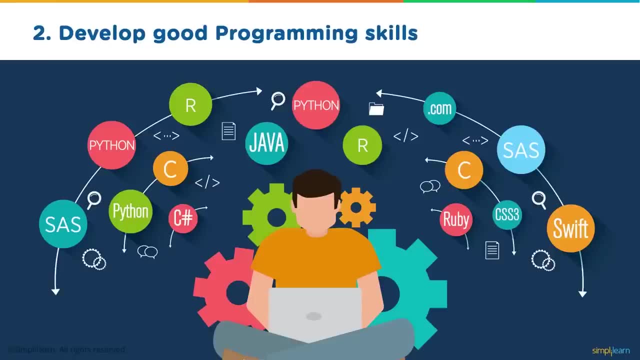 In your next step to becoming a machine learning engineer, you need to develop good programming skills, And let me tell you, there are a huge number of options from which you can choose. There's Python, there's C, there's C Sharp. 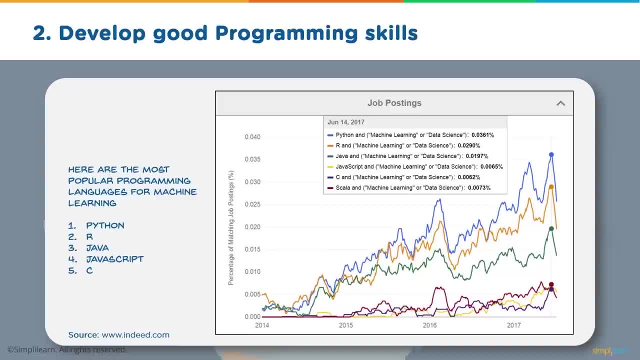 there's Java and so much more. Now here's a graph of the job postings from 2014 to 2017.. And you can see that there are two languages that dominate since 2015, Python and R. Now these are one of the most wanted languages. 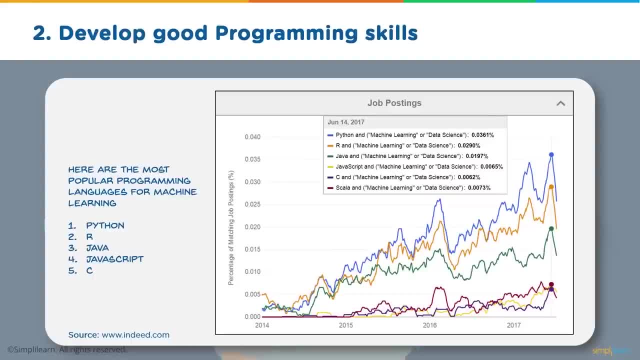 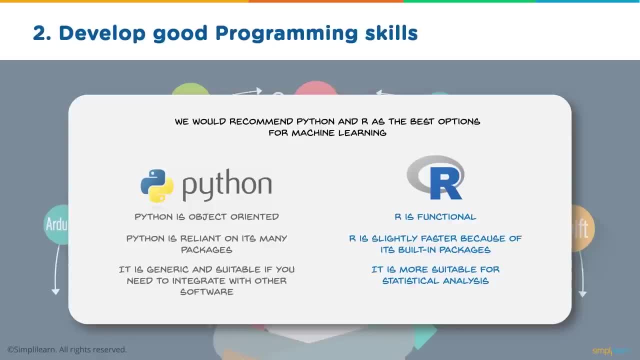 when it comes to machine learning engineers. These are closely followed by JavaScript and C. Hence, we would like to recommend that you learn Python and R, as they are the best options when it comes to coding in machine learning algorithms. So here are a few things that you need to know about. 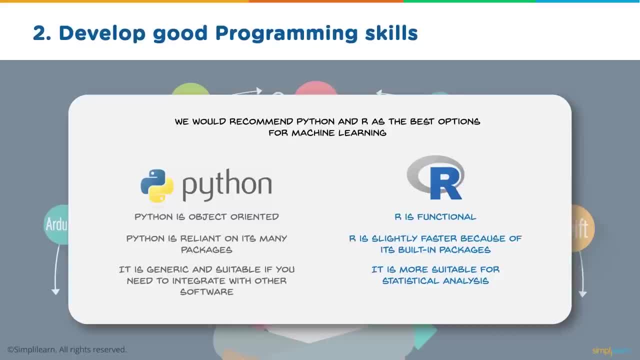 Python and R. Python is an object-oriented language, which means their main emphasis is on the object. R is a functional language, which means their emphasis is on creating and manipulating functions. Python relies on its many packages and R is slightly faster than Python because it has 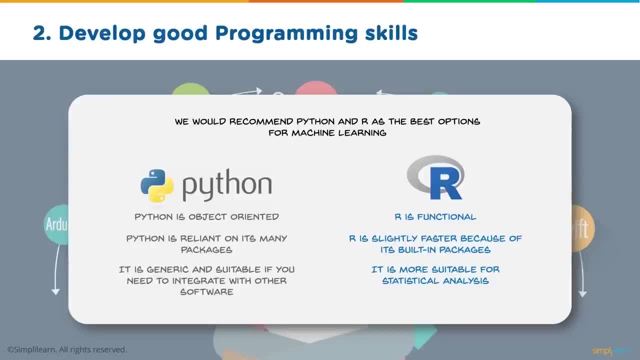 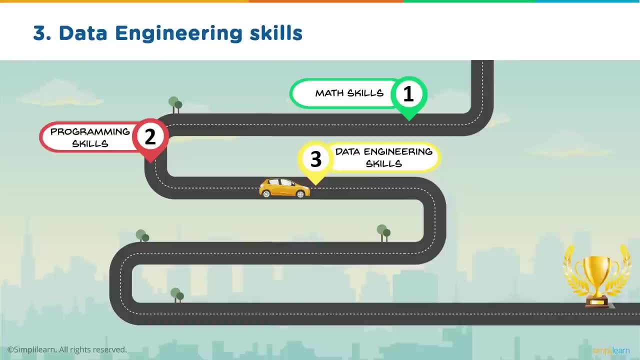 inbuilt packages Now. Python is generic and is suitable if you need to integrate it with any other software. R works a little more closer with statistical analysis. Your next step is to get yourself some data engineering skills. Now. these skills are important as they help you analyze and 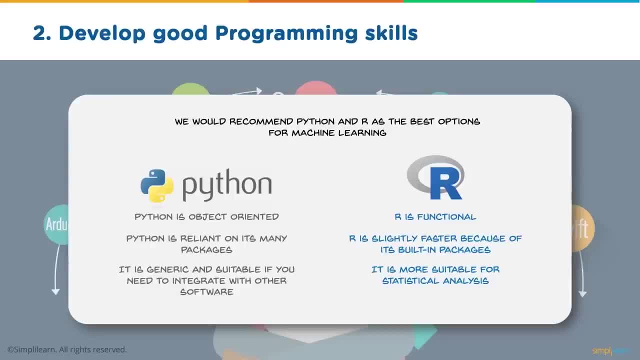 faster than python because it has inbuilt packages. now python is generic and is suitable if you need to integrate it with any other software. r works a little more closer with statistical analysis. your next step is to get yourself some data engineering skills now. these skills are important, as they 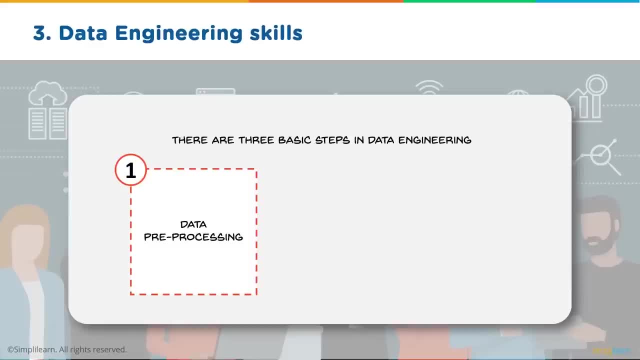 help you analyze and process your data as soon as you get it. now, there are three major steps when it comes to data engineering. firstly, there's data pre-processing. now these refer to all the steps that you need to perform before data can be processed by the machine learning algorithm you have. 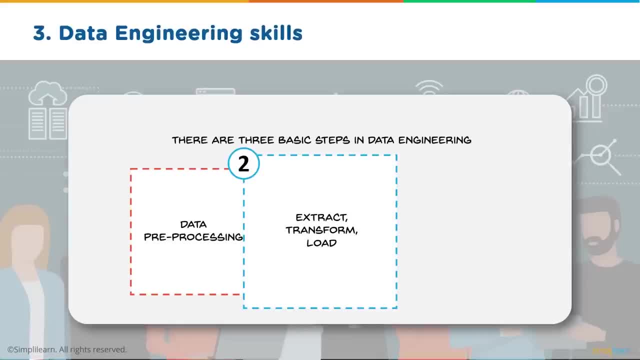 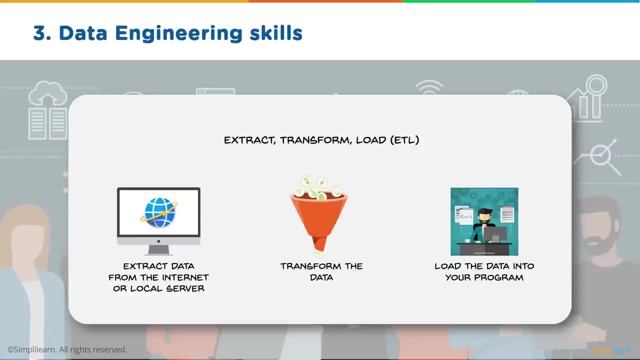 cleaning, parsing, correcting and consolidating the data. then you have etl, or extract, transform and load. you need to know how data can be processed and be extracted from the internet or a local server. you need to know how to transform the data. for example, not all formats of data would be accepted by the 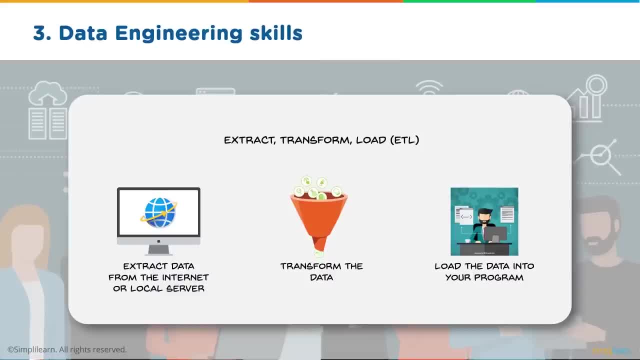 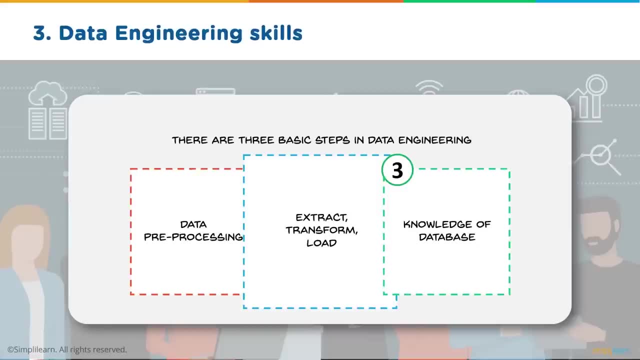 program. so you need to convert the data into a format that is accepted by the program. then you need to know how the data is loaded into your program. the final step is to have knowledge about database management softwares, or dbms. you need to be well versed with mysql. 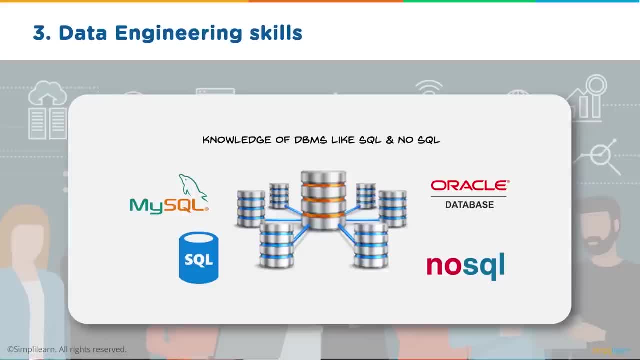 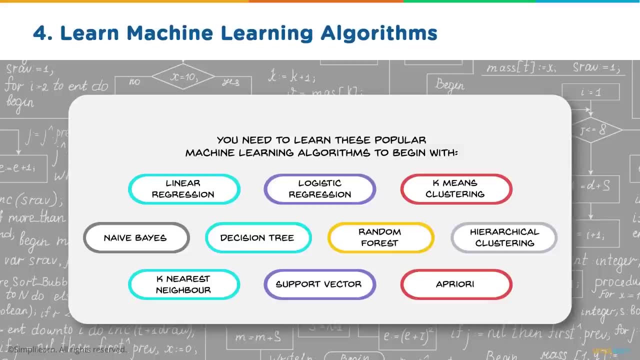 the oracle database and no sql. your next step is to learn machine learning algorithms. to learn machine learning algorithms, you need to be well versed. now, among all the machine learning algorithms that you can see on screen, you can divide them into two different categories, ones that fall under: 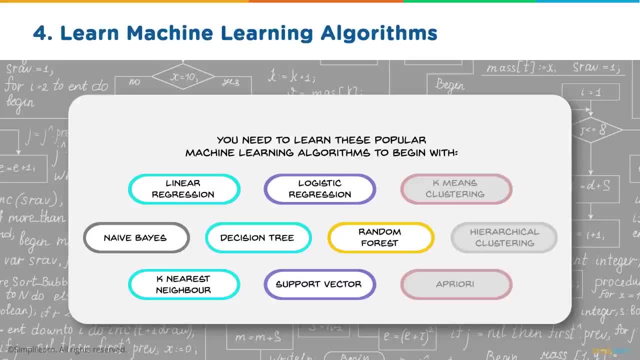 supervised machine learning and the others that fall under unsupervised machine learning. even after such a division, you can further subdivide them into classification and regression algorithms. now, all algorithms, except linear regression fall under the category of classification, which is used to determine whether a particular data 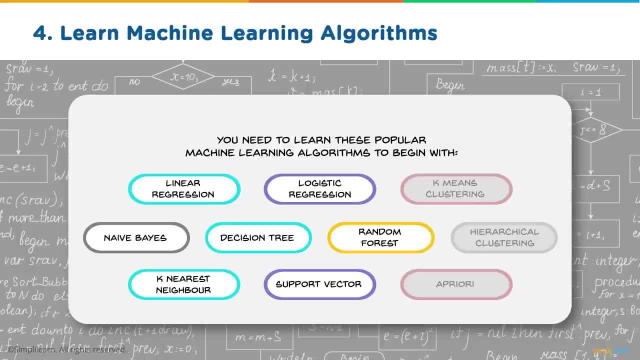 falls into a particular category. on the other hand, you have linear regression under regression algorithms. this is used to predict a particular value. then you have k-means clustering and hierarchical clustering. now these fall in the category of clustering. this is used to group data into clusters based. 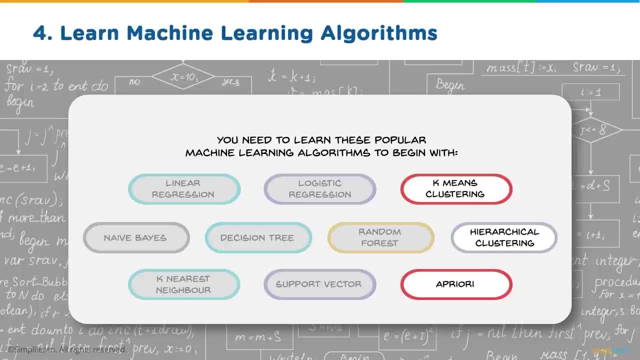 on certain similar attributes. then you have the a priori algorithm that falls under the concept of association. association is used to determine patterns of association among variables in large data sets. so now that you know about these algorithms, let me tell you where you can learn about them. let's 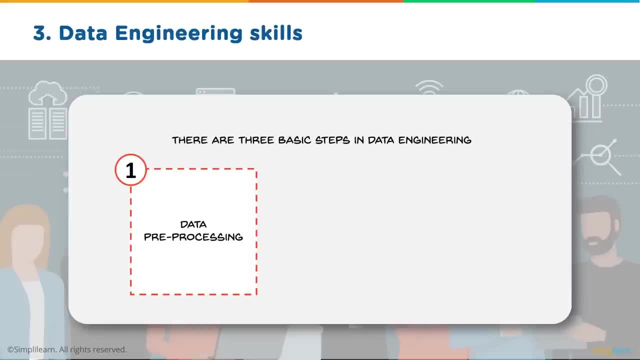 process your data as soon as you get it. Now, there are three major steps when it comes to data engineering. Firstly, there's data pre-processing. Now, these refer to all the steps that you need to perform before data can be processed by the machine. 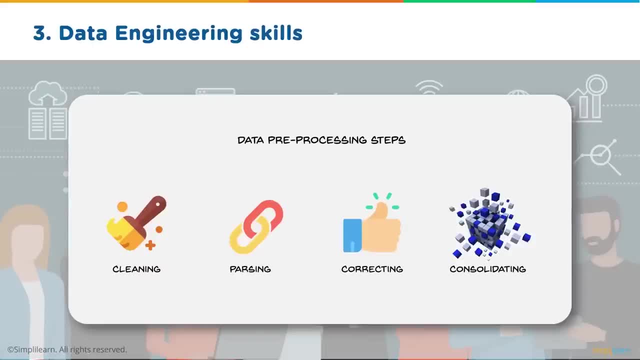 learning algorithm. You have cleaning, parsing, correcting and consolidating the data. Then you have ETL or extract, transform and load. You need to know how data can be extracted from the internet or a local server. You need to know. 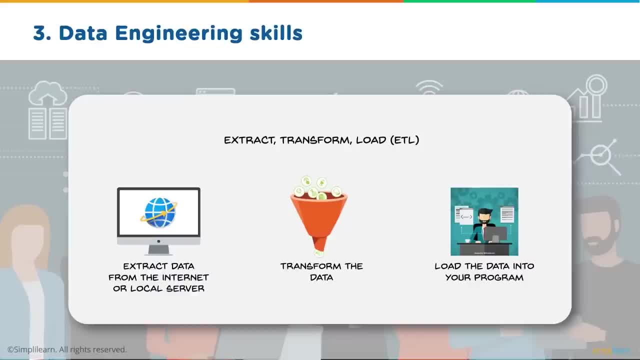 how to transform the data. For example, not all formats of data would be accepted by the program, So you need to convert the data into a format that is accepted by the program. Then you need to know how the data is loaded into your program. 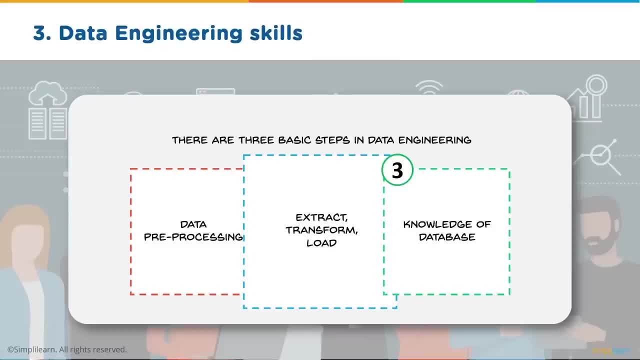 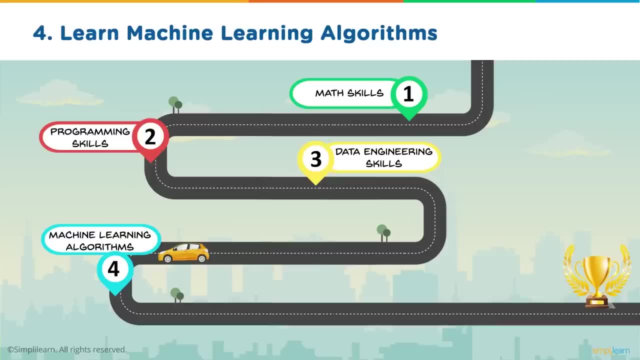 The final step is to have knowledge about database management softwares, or DBMS. You need to be well versed with MySQL, the Oracle database and NoSQL. Your next step is to learn machine learning algorithms Now, among all the machine learning algorithms that you can see on screen. 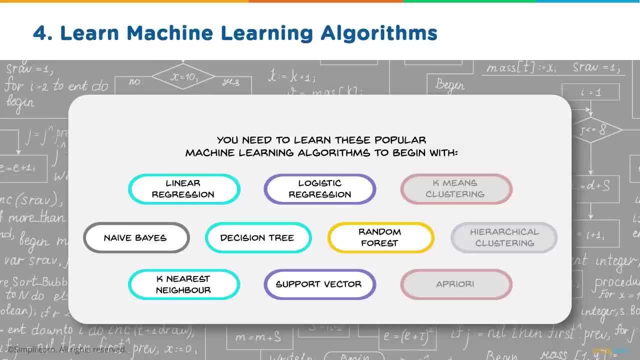 you can divide them into two different categories: Ones that fall under supervised machine learning and the others that fall under unsupervised machine learning. Even after such a division, you can further subdivide them into classification and regression algorithms. Now, all algorithms except linear regression fall under the 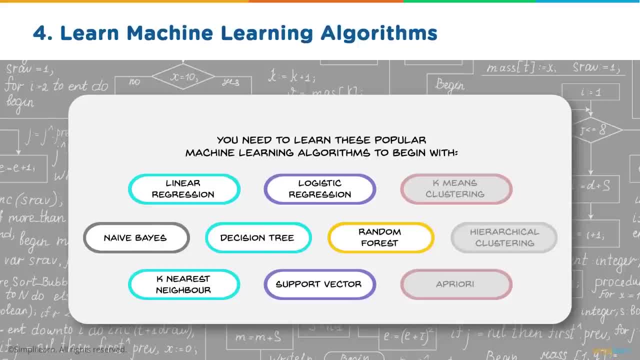 category of classification, which is used to determine whether a particular data falls into a particular category. On the other hand, you have linear regression that falls under regression algorithms. This is used to predict a particular value. Then you have k-means clustering. 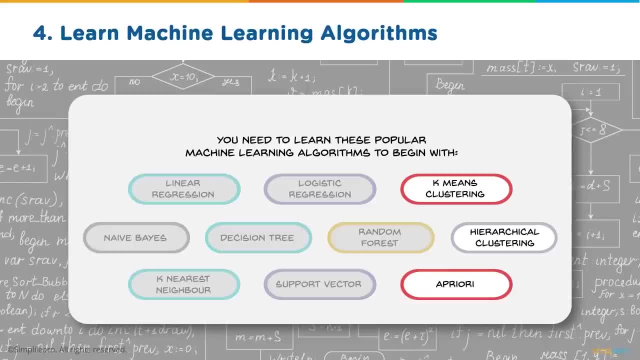 and hierarchical clustering. Now these fall under the category of clustering. This is used to group data into clusters based on certain similar attributes. Then you have the a priori algorithm. that falls under the concept of association. Association is used to determine patterns of association. 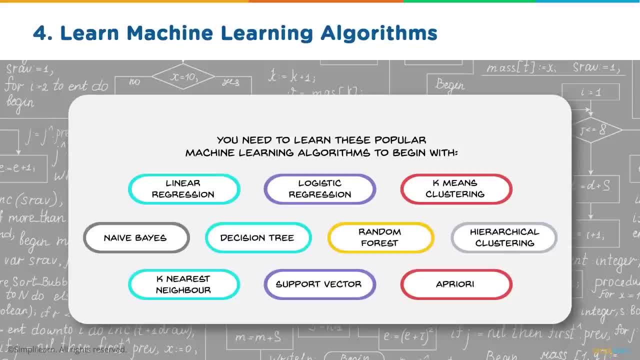 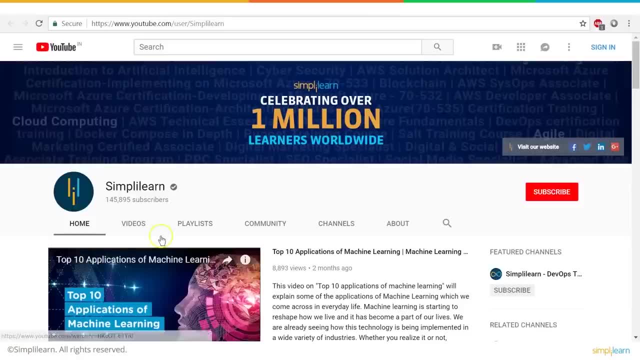 among variables in large data sets. So now that you know about these algorithms, let me tell you where you can learn about them. Let's take a look at our Simply Learn channel And let's go to playlists, And on this we have a dedicated set of playlists. 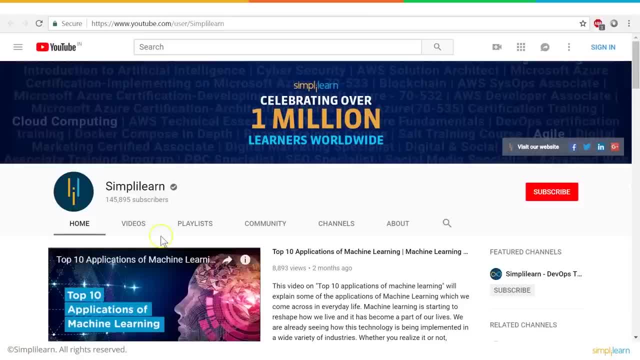 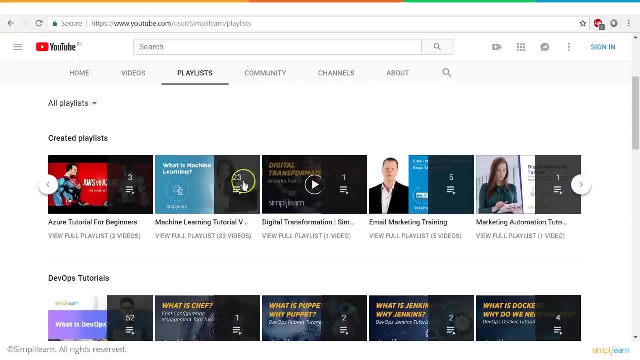 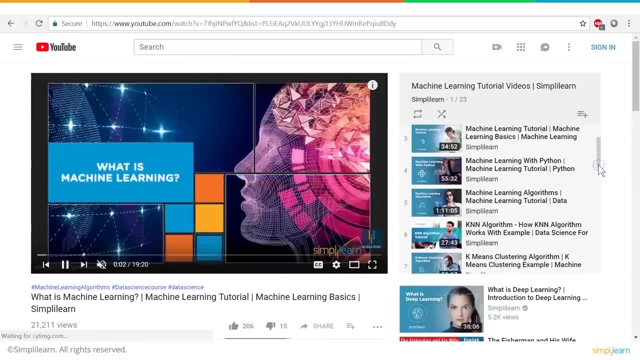 take a look at our simply learning channel and let's go to playlists, and on this we have a dedicated set of playlists that talk about machine learning. here you have videos on machine learning, how machine learning is different from deep learning and artificial intelligence. machine learning with python k-means clustering decision trees. 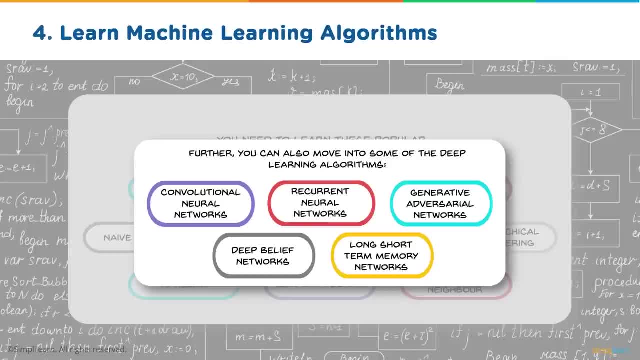 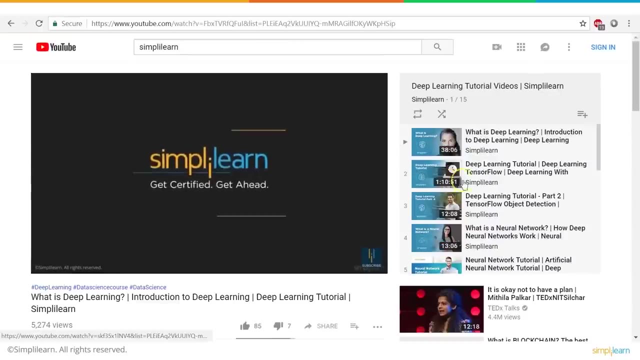 and so on. if you want to learn more, you could also go through some deep learning algorithms like convolutional neural networks, recurrent neural networks, long memory networks and so on. in fact, we have a detailed playlist that talks about the concepts of deep learning. here you can find videos on what is deep 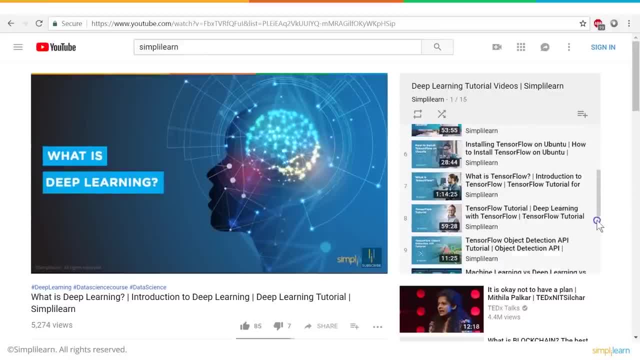 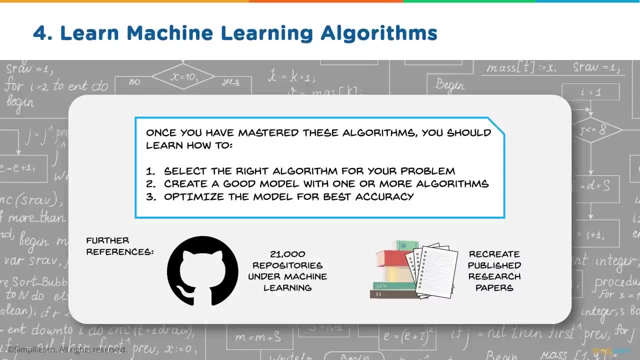 learning tensorflow. what is a neural network? convolutional neural networks and recurrent neural networks. now, after you master these algorithms, you need to learn how you can select the right algorithm for your problem. then you need to create a good model with one or more algorithms, after which you need to keep. 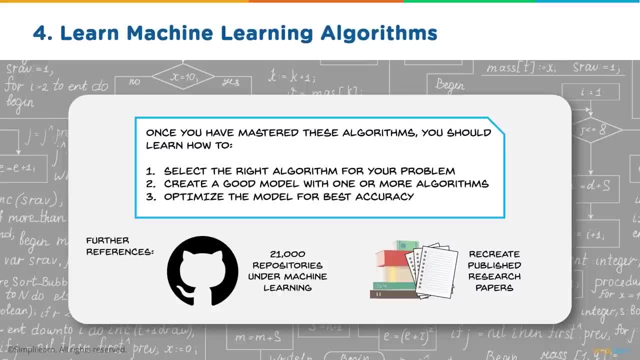 tweaking and optimizing the model to determine the right algorithm for your problem so that you can get the maximum accuracy. for further reading, you can go through github, where there's more than 21 000 repositories under machine learning. you can also recreate published research papers adding to your 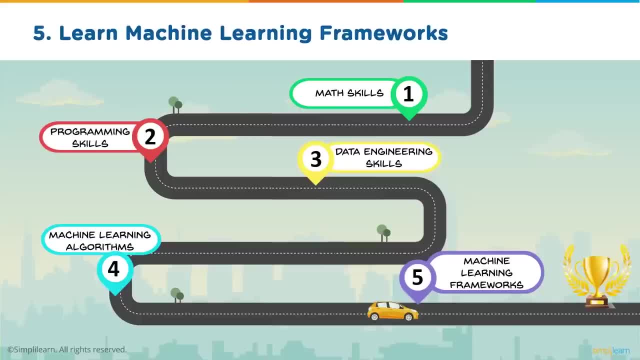 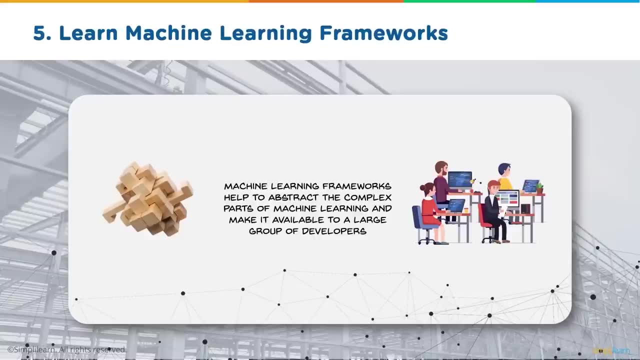 experience of working with machine learning. and now for your last step: learning machine learning frameworks. machine learning frameworks help make the lives of developers, as well as users, a whole lot easier. they help remove the complex part of machine learning and make it available for everyone who wants to use it, be it developers or other. 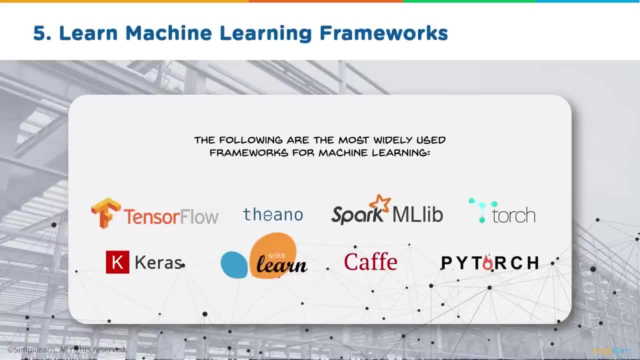 users. now let's look at the widely used machine learning frameworks. there's tensorflow, theano, torch, scikit-learn and so on. now let's look at some of them in detail. first, let's look at tensorflow. tensorflow is the most widely used machine learning framework. it's used for: 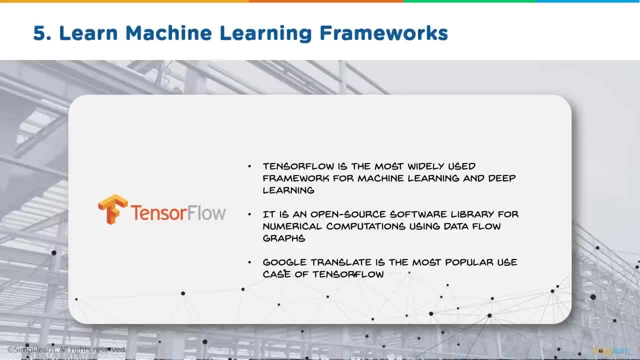 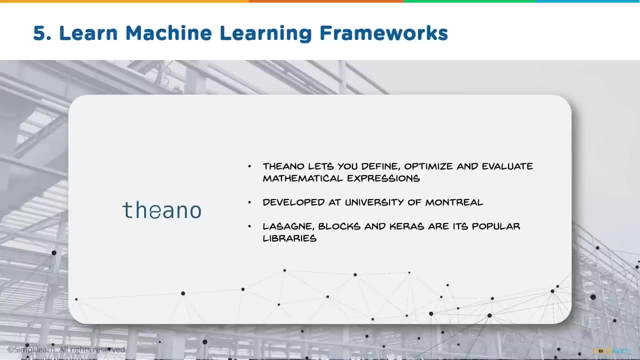 machine learning as well as deep learning. now it's an open source software library which performs numerical computations, which is done with the help of data flow graphs. google translate is one of the most popular use cases of tensorflow. now let's look at theano. theano helps you define, optimize and 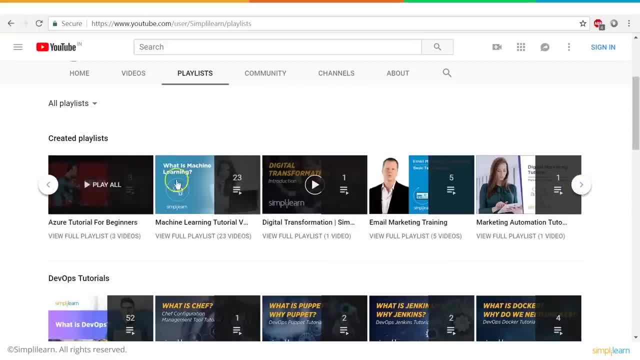 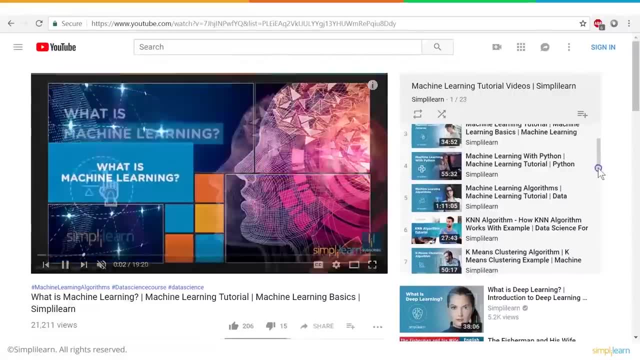 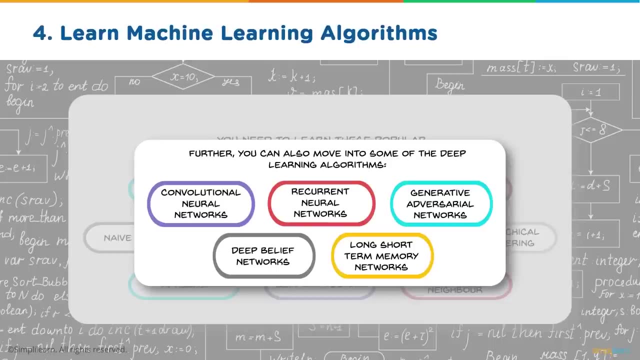 that talk about machine learning. Here you have videos on machine learning, how machine learning is different from deep learning and artificial intelligence. machine learning with Python k-means clustering, decision trees and so on. If you want to learn more, you could also go through some deep learning. 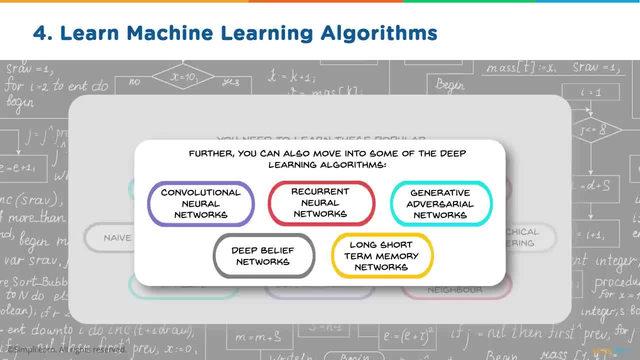 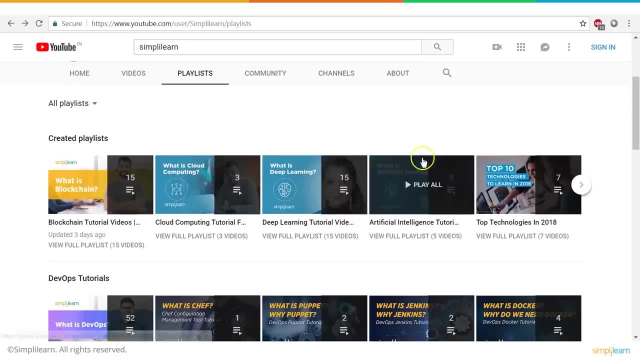 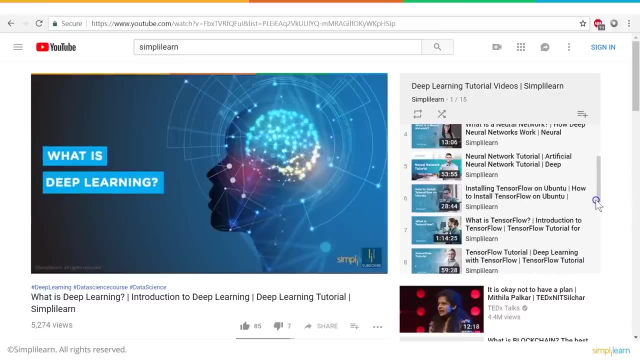 algorithms like convolutional neural networks, recurrent neural networks, long short term memory networks, and so on. In fact, we have a detailed playlist that talks about the concepts of deep learning. Here you can find videos on what is deep learning, TensorFlow, what is a neural network? 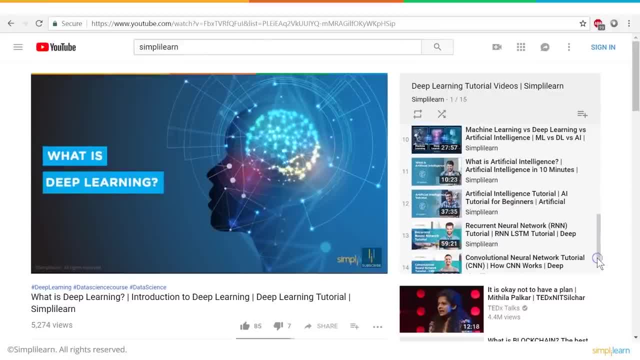 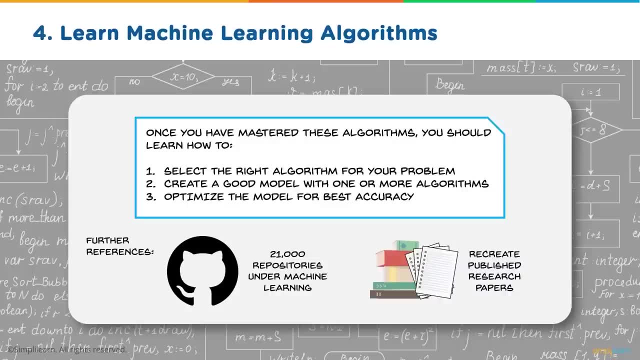 convolutional neural networks and recurrent neural networks. Now, after you master these algorithms, you need to learn how you can select the right algorithm for your problem. Then you need to create a good model with one or more algorithms, After which you need to keep tweaking and optimizing. 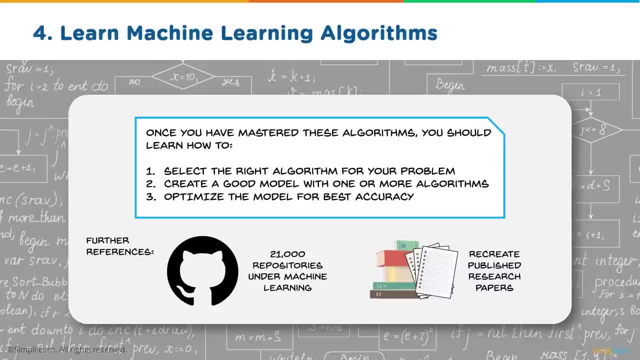 the model so that you can get the maximum accuracy. For further reading. you can go through GitHub, where there's more than 21,000 repositories under machine learning. You can also recreate published research papers, adding to your experience of working with machine. 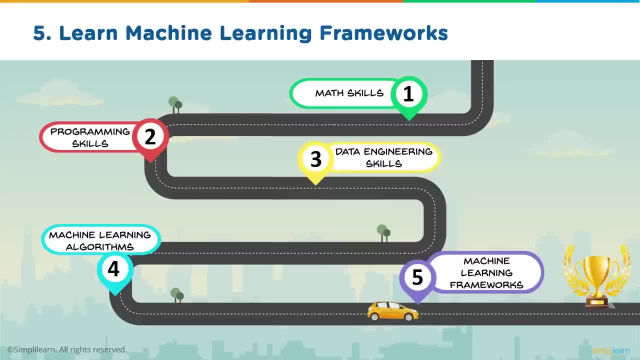 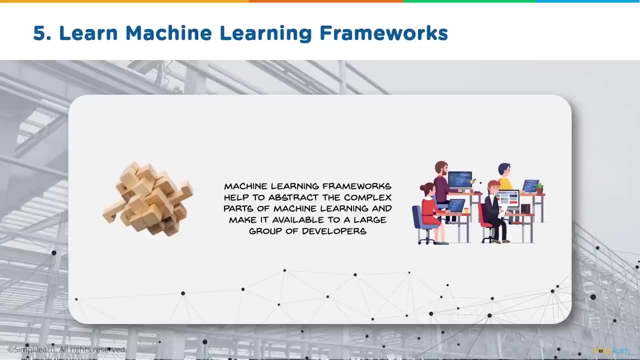 learning. And now for your last step: learning machine learning frameworks. Machine learning frameworks help make the lives of developers, as well as users, a whole lot easier. They help remove the complex part of machine learning and make it available for everyone who wants to use it, be it developers. 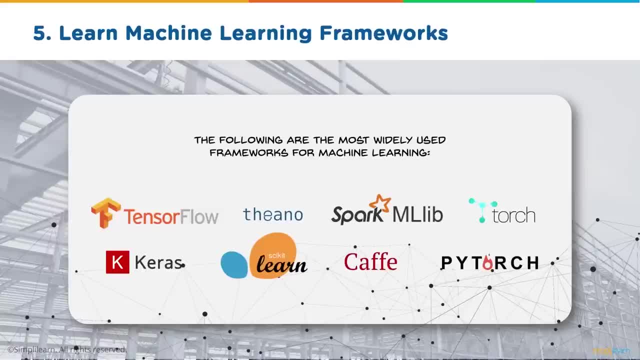 or other users. Now let's look at the widely used machine learning frameworks. There's TensorFlow, Theano, Torch, Scikit-Learn and so on. Now let's look at some of them in detail. First, let's look at TensorFlow. 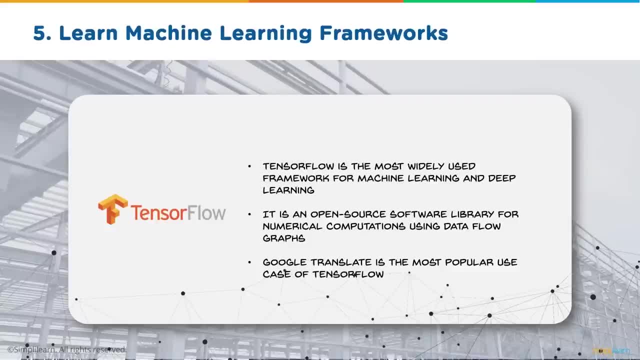 TensorFlow is the most widely used machine learning framework. It's used for machine learning as well as deep learning. Now it's an open source software library which performs numerical computations, which is done with the help of data flow graphs. Google Translate is one of the most popular use cases. 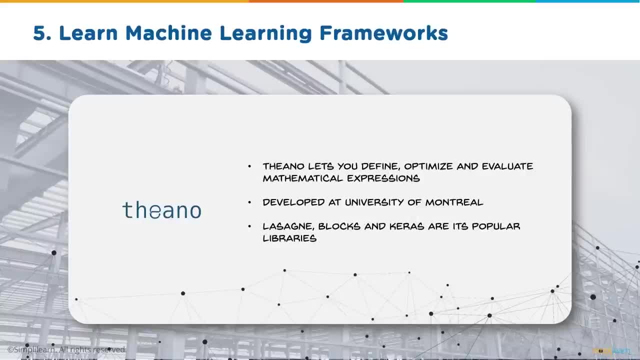 of TensorFlow. Now let's look at Theano. Theano helps you define, optimize and evaluate mathematical expressions. It was developed in the University of Montreal. Lasagne Blocks and Keras are its most popular libraries. Now let's look at Spark ML. 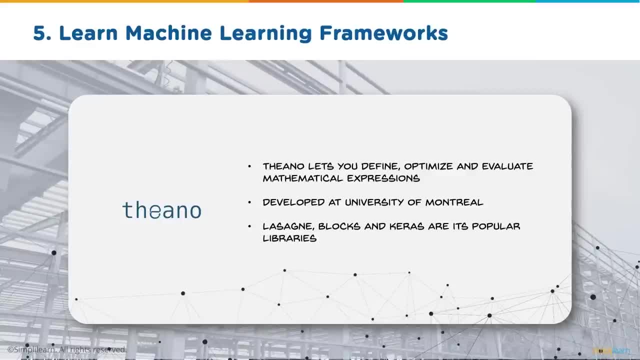 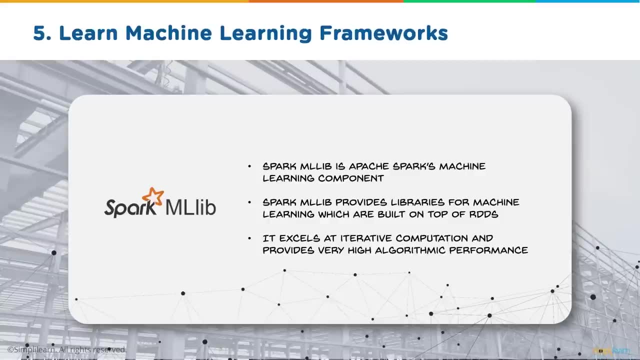 evaluate mathematical expressions. it was developed in the university of montreal, lasagne. blocks and keras are its most popular libraries. now let's look at spark ml library. now this is apache sparks machine learning component. it also provides libraries for machine learning which are built on top of rdds or resilient distributed. 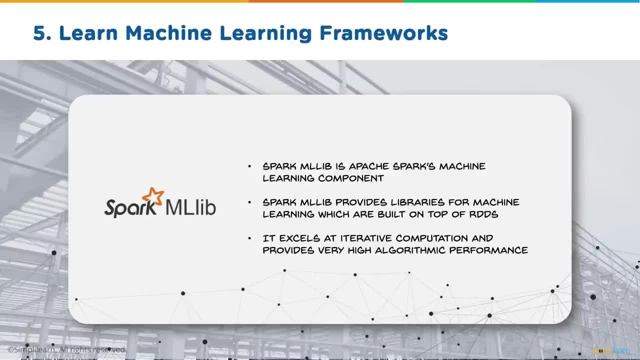 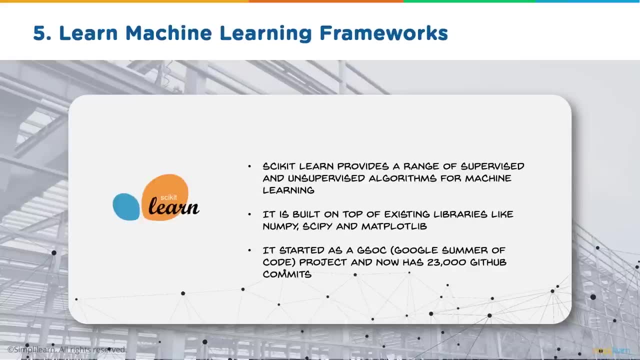 datasets. it's very good at providing iterative computation and provides very high algorithmic performance. now let's look at scikit-learn, which is a multi-functional machine learning software library which provides algorithmic performance. now let's look at scikit-learn. scikit-learn is able to 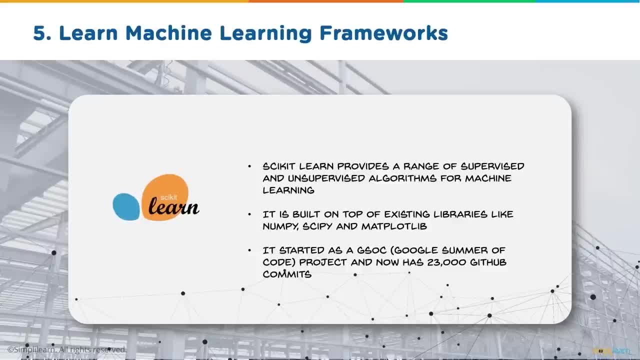 provide a huge range of supervised as well as unsupervised algorithms for machine learning. it is built on existing libraries like numpy, scipy and matplotlib. scikit-learn actually started off as a google summer of code project and now has 23 000 github commits and that's it. 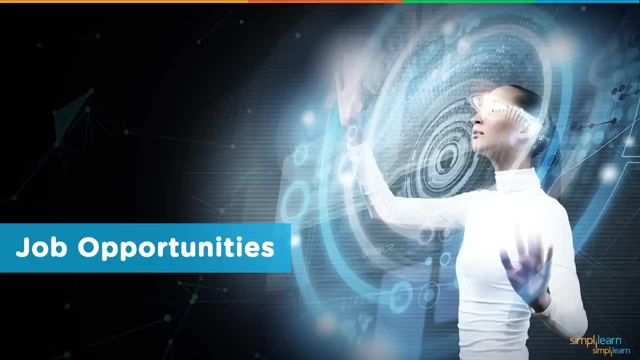 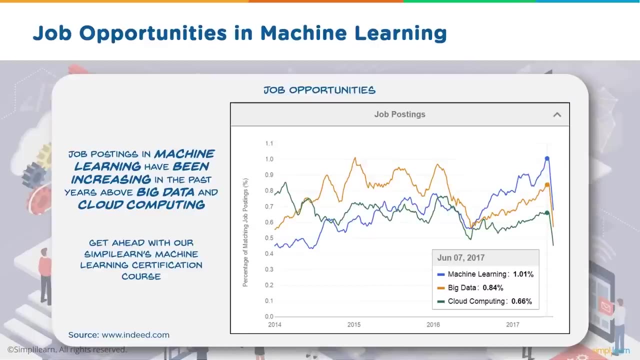 congratulations: you're now a machine learning engineer. now let's look at the job opportunities in machine learning now if you have a machine learning. machine learning was much less popular than big data and cloud computing, but all of that suddenly changed and right now, a machine learning engineer earns around hundred and. 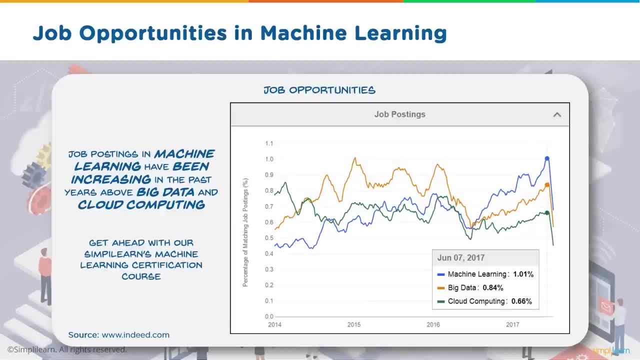 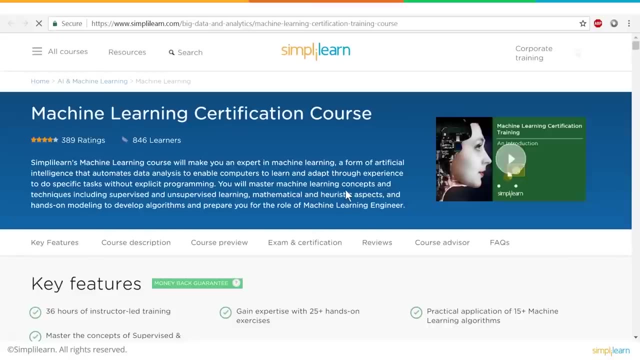 fourteen thousand dollars per annum, and this is a clear indication that organizations are ready to invest heavily in people who are skilled in the concepts of machine learning. you can also make the learning process easier by using simply learn's machine learning certification. simply learns machine learning certification course provides 36 hours. 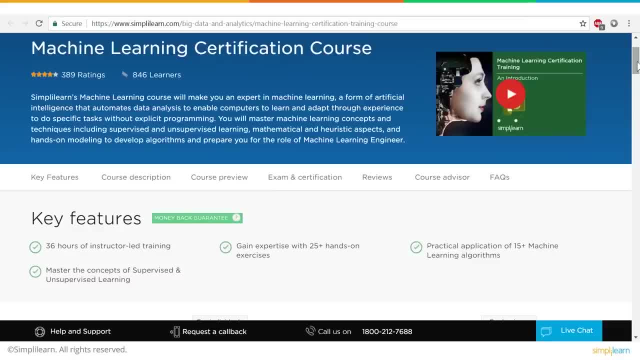 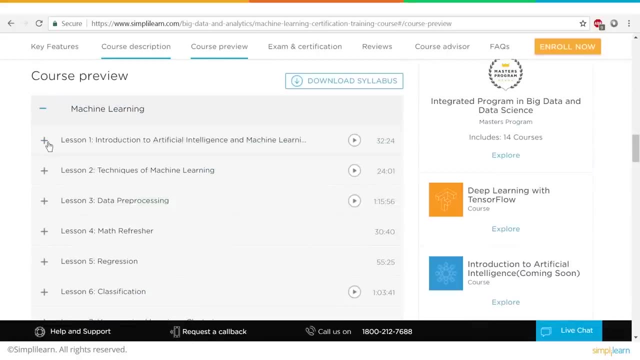 of instructor-led training, provides 25 plus hands-on exercises, gives you practical applications of 15 plus machine learning algorithms and helps you master the concepts of supervised and unsupervised learning. it also introduces you to artificial intelligence, tells you the techniques of machine learning, data processing. 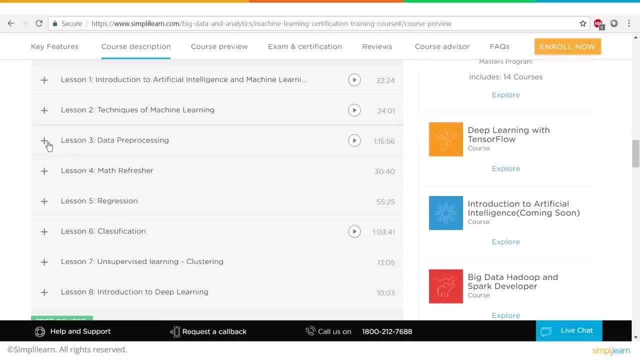 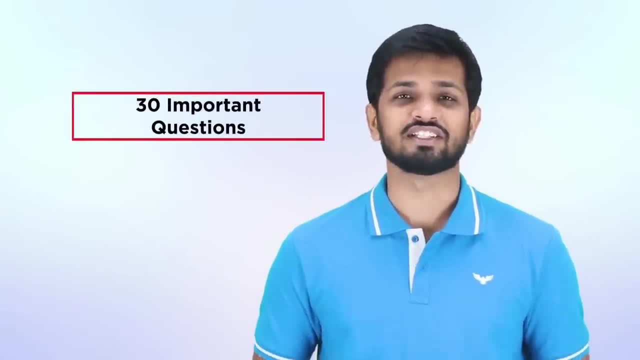 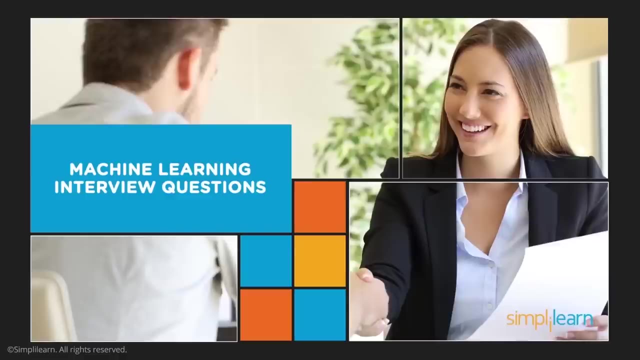 regression, classification and so much more so if you want to take your first step to getting certified and getting ahead. thanks, rahul. now mohan will take you through 30 important questions that might just appear in your machine learning interview. today we'll talk about interview questions for. 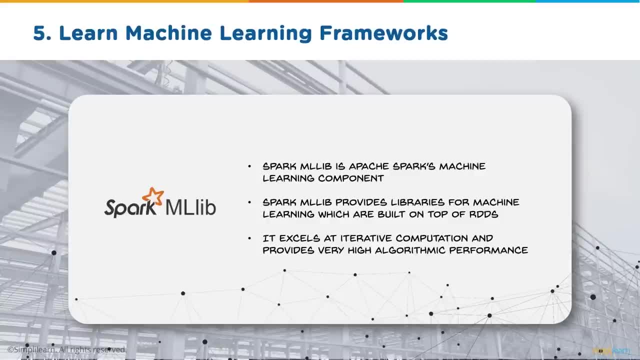 library. Now, this is Apache Spark's machine learning component. It also provides libraries for machine learning which are built on top of RDDs or Resilient Distributed Data Sets. It's very good at providing iterative computation and provides very high algorithmic performance. Now, 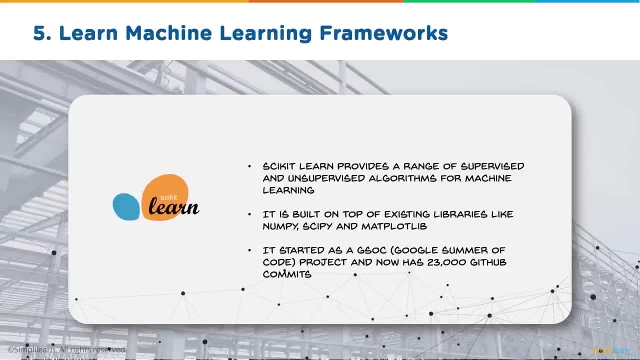 let's look at Scikit-Learn. Scikit-Learn is able to provide a huge range of supervised as well as unsupervised algorithms for machine learning. It is built on existing libraries like NumPy, SciPy and Matplotlib. Scikit-Learn actually started off as a Google. 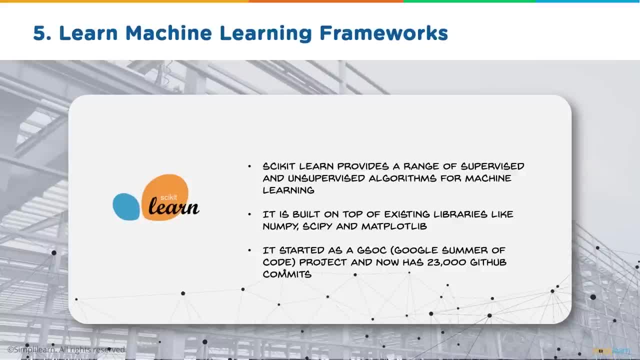 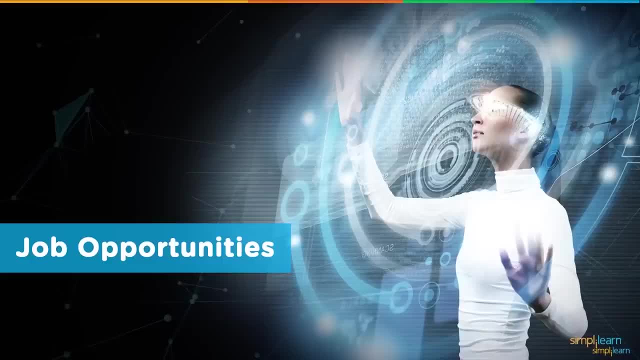 Summer of Code project and now has 23,000 GitHub commits. And that's it, Congratulations. You are now a machine learning engineer. Now let's look at the job opportunities in machine learning Now. if you have a look at this graph, 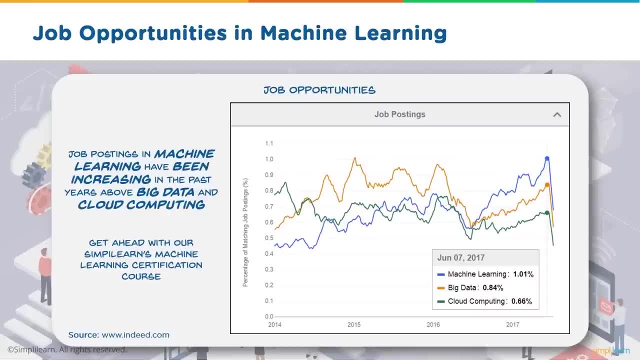 it kind of speaks for itself. Before 2015,, machine learning was much less popular than big data and cloud computing, But all of that suddenly changed And right now a machine learning engineer earns around $114,000 per annum. And this is. 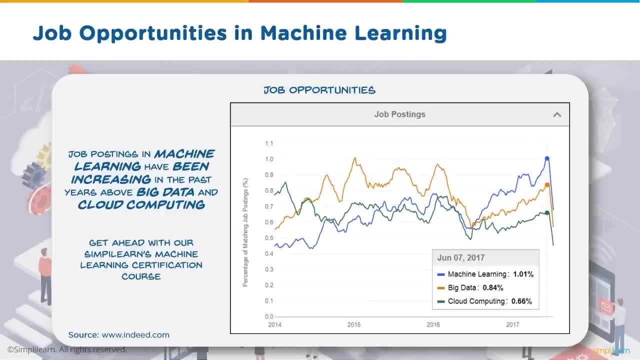 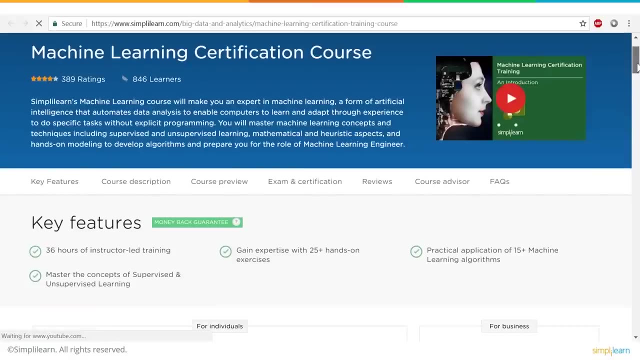 a clear indication that organizations are ready to invest heavily in people who are skilled in the concepts of machine learning. You can also make the learning process easier by using SimplyLearn's machine learning certification. SimplyLearn's machine learning certification course provides 36 hours of instructor-led training. 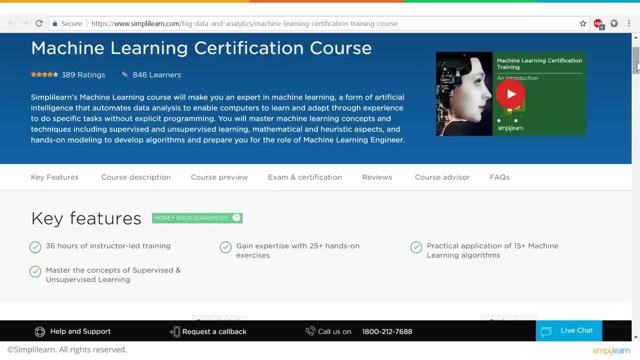 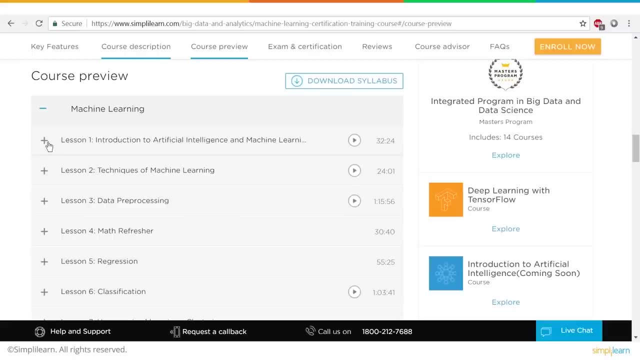 provides 25 plus hands-on exercises, gives you practical applications of 15 plus machine learning algorithms and helps you master the concepts of supervised and unsupervised learning. It also introduces you to artificial intelligence, tells you the techniques of machine learning, data processing. 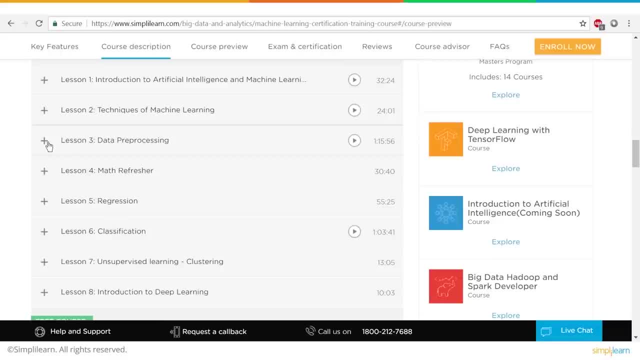 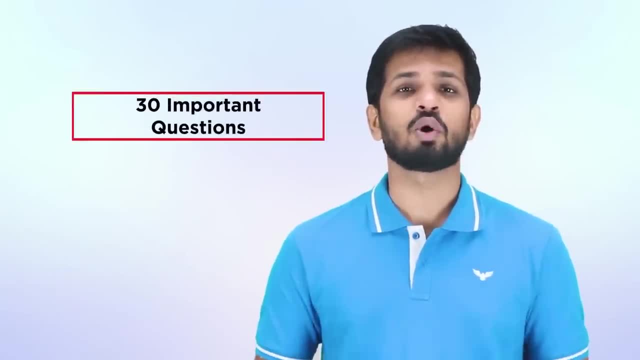 regression, classification and so much more. So, if you want to take your first step to getting certified and getting ahead. Thanks, Rahul. Now Mohan will take you through 30 important questions that might just appear in your machine learning interview Today we'll talk about 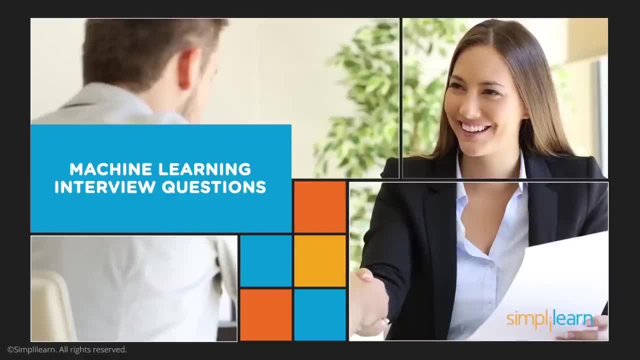 interview questions for machine learning. Now, this video will probably help you when you are attending interviews For machine learning positions, and the attempt here is to probably consolidate 30 most commonly asked questions and to help you in answering these questions. We tried our best. 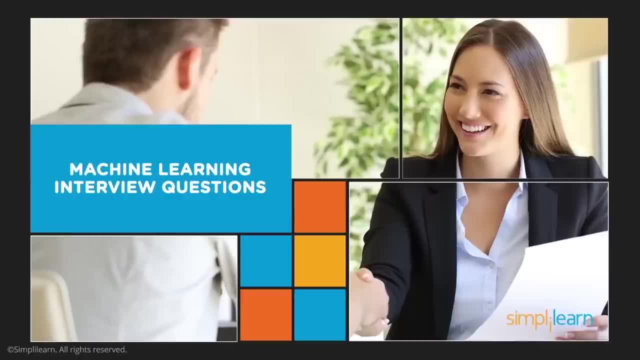 machine learning. now, this video will probably help you when you're attending interviews or machine learning positions, and the attempt here is to probably consolidate 30 most commonly asked questions and to help you in answering these questions. we tried our best to give you the best possible answers, but, of course, what is? 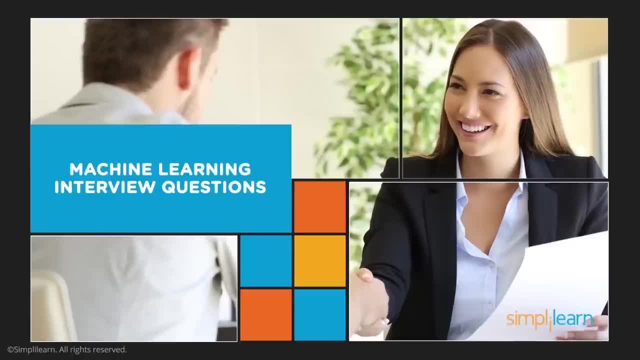 more important here is rather than the theoretical knowledge you need to kind of add to the answers or supplement your answers with your own experience. so the responses that we put here are a bit more generic in nature, so that if there are some concepts that you are not clear, 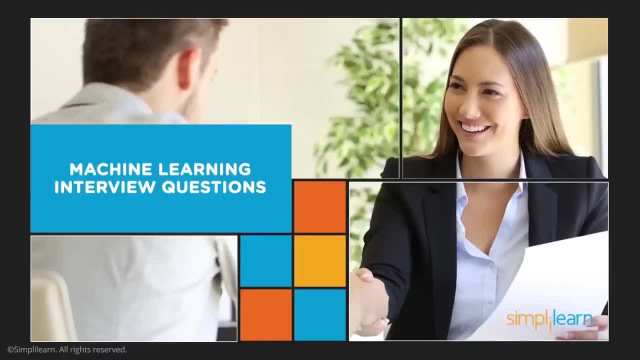 this video will help you to understand more about machine learning. so let's get started. so let's get started. so for this video, I'm going to talk about machine learning. exactly, we use machine learning a lot when we're talking about machine learning, okay, so the purpose is to help you in kind of. 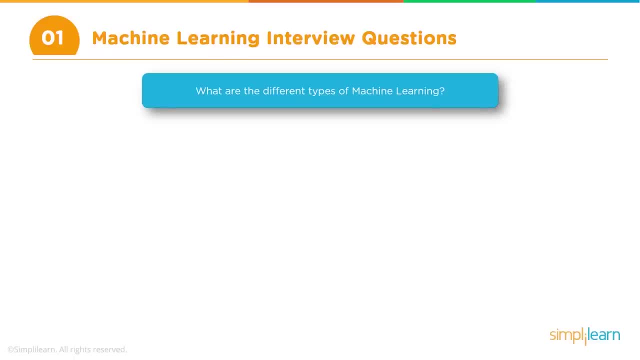 getting those concepts cleared up as well, but what is more important is that you need to supplement these responses with your own practical experience. okay, so with that, let's get started. so one of the first questions that you may face is: what are the different machine learning? but what is important is, you would probably be better of emphasizing that. 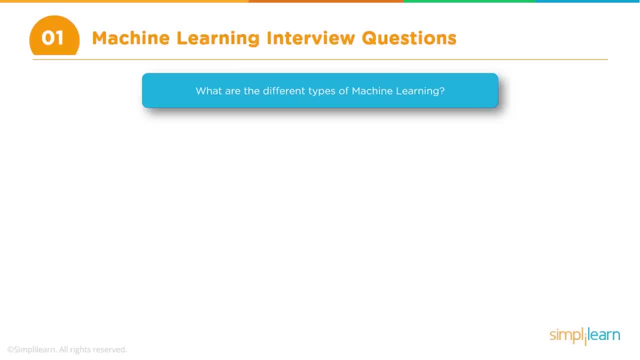 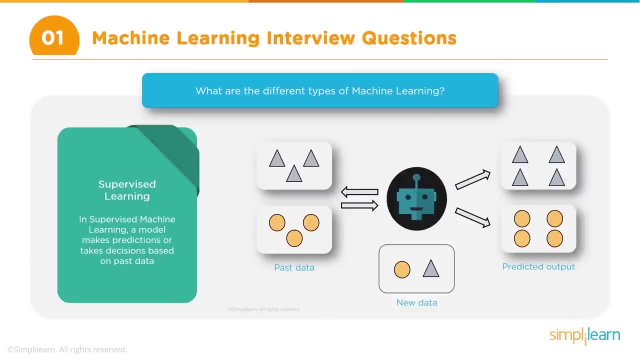 there are actually two main types of machine learning, which is supervised and unsupervised, and then there is a third type, which is reinforcement learn. So supervised learning is where you have some historical data and then you feed that data to your model to learn. Now 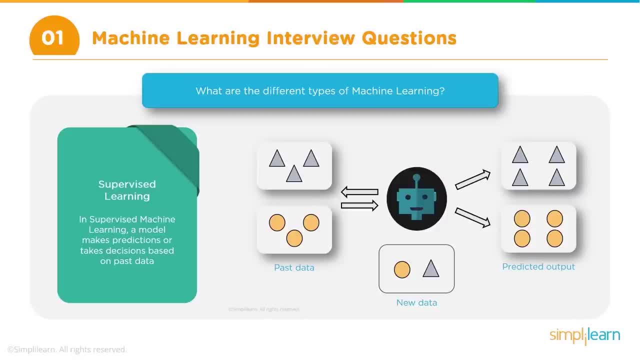 you need to be aware of a key word that they will be looking for: which is labeled data, right? So if you just say past data or historical data, the impact may not be so much. You need to emphasize on labeled data. So what is labeled data Basically? let's say, if you are trying to do, 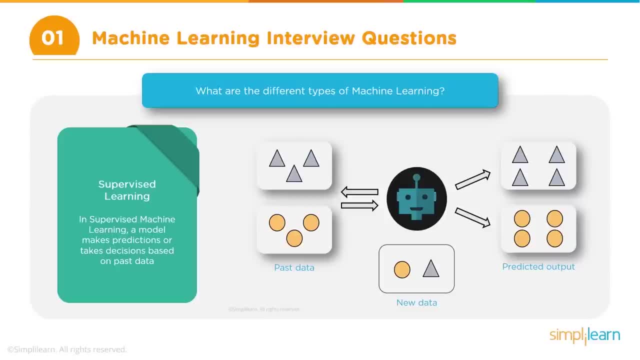 train your model for classification you need to be aware of for your existing data, which class each of the observations belong to right. So that is what is labeling. So it is nothing but a fancy name. You must be already aware, but just make it a point to throw in that keyword labeled. 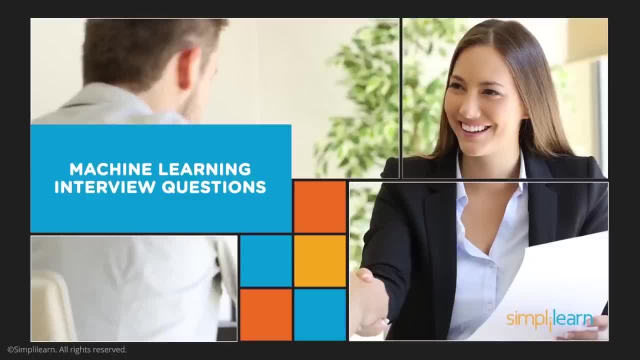 to give you the best possible answers. But of course what is more important here is, rather than the theoretical knowledge, you need to kind of add to the answers or supplement your answers with your own experience. So the responses that we put here are a bit 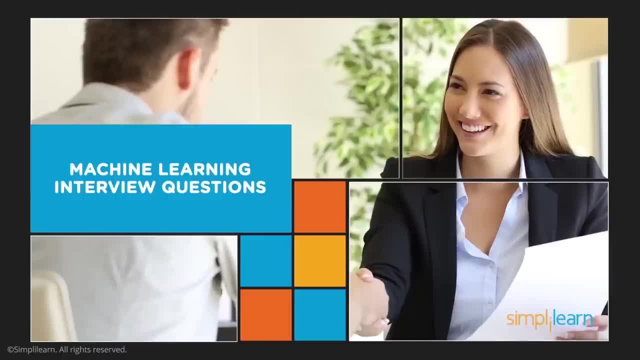 more generic in nature, so that if there are some concepts that you are not clear, this video will help you in kind of getting those concepts cleared up as well. But what is more important is that you need to supplement these responses with your own practical experience. 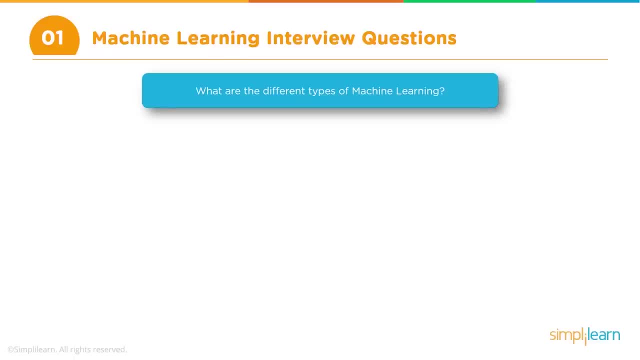 Okay, so with that, let's get started. So one of the first questions that you may face is: what are the different types of machine learning? Now, what is the best way to respond to this? There are three types of machine learning, If you read any. 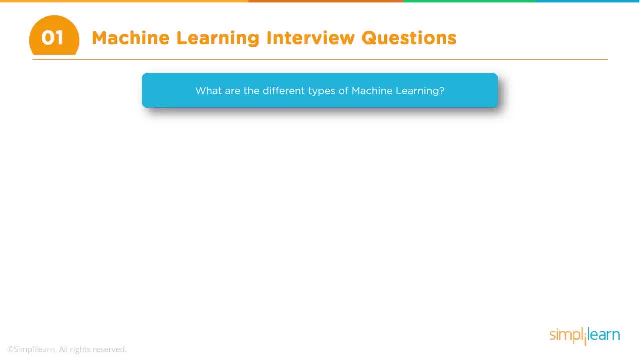 material. you will always be told there are three types of machine learning, But what is important is, you would probably be better of emphasizing that there are actually two main types of machine learning, which is supervised and unsupervised. And then there is a third type, which is 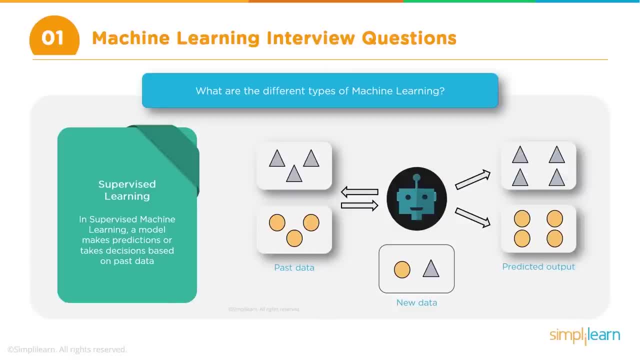 reinforcement learning. So supervised learning is where you have some historical data and then you feed that data to your model to learn. Now you need to be aware of a key word that they will be looking for, which is labeled data. So if you just say past data, 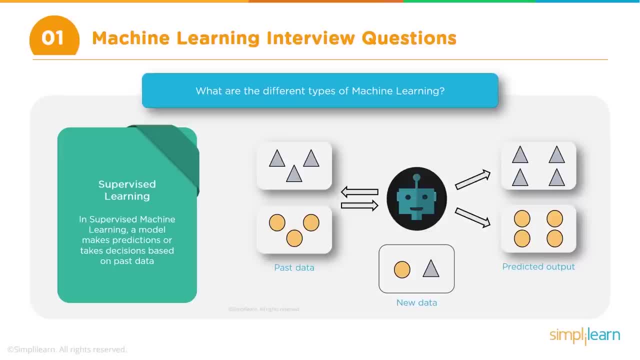 or historical data, the impact may not be so much. You need to emphasize on labeled data. So what is labeled data Basically? let's say, if you are trying to train your model for classification, you need to be aware of for your existing 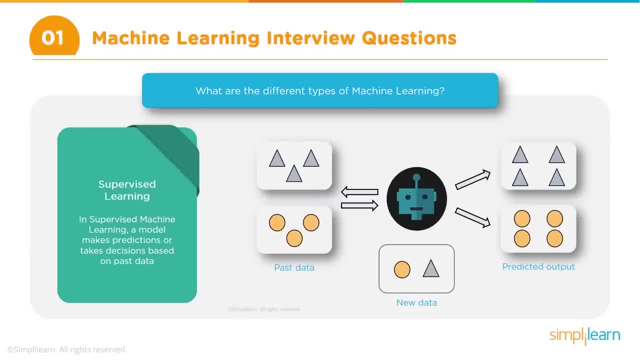 data which class each of the observations belong to right. So that is what is labeling. So it is nothing but a fancy name. But just make it a point to throw in that keyword labeled, so that will have the right impact. 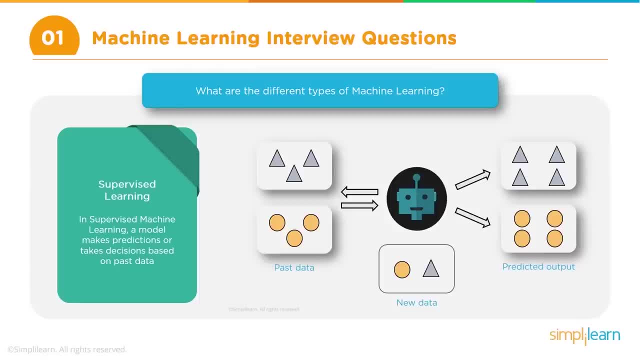 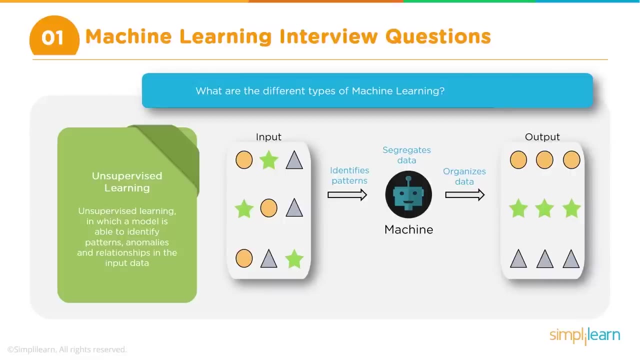 So that is what is supervised learning: When you have existing labeled data which you then use to train your model. that is known as supervised learning, And unsupervised learning is when you don't have this labeled data. So you have data, It is not. 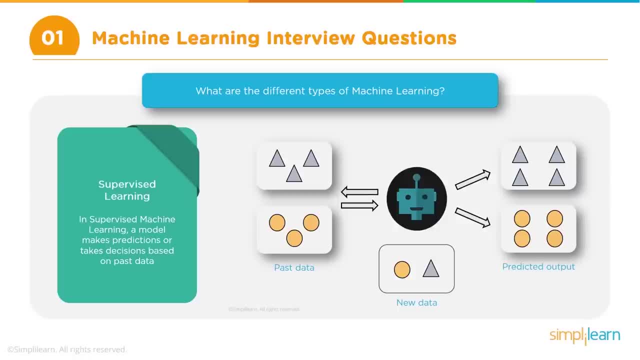 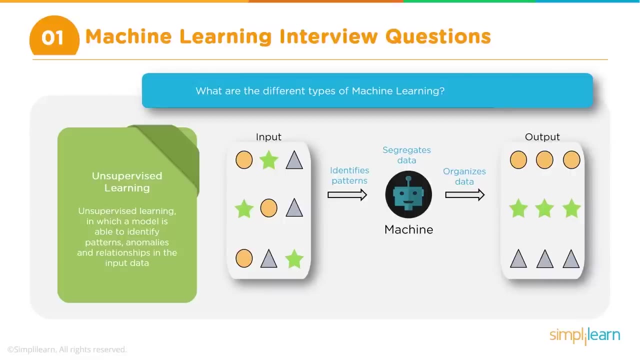 so that will have the right impact. Okay, so that is what is supervised learning: when you have existing labeled data which you then use to train your model. that is known as supervised learning, and unsupervised learning is when you don't have this labeled data. So you have data. it is not. 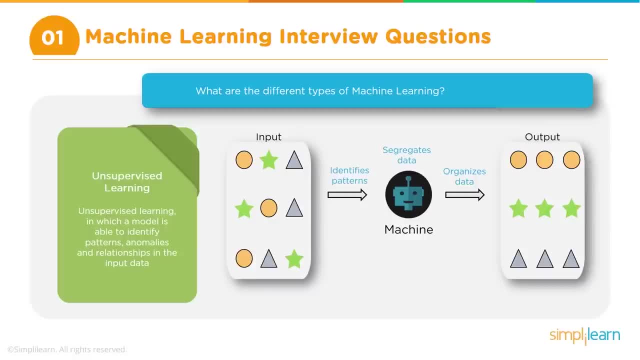 labeled. So the system has to figure out a way to do some analysis on that. So that is unsupervised learning, and you can then add a few things like what are the ways of performing supervised learning and unsupervised learning and what are some of the techniques. So 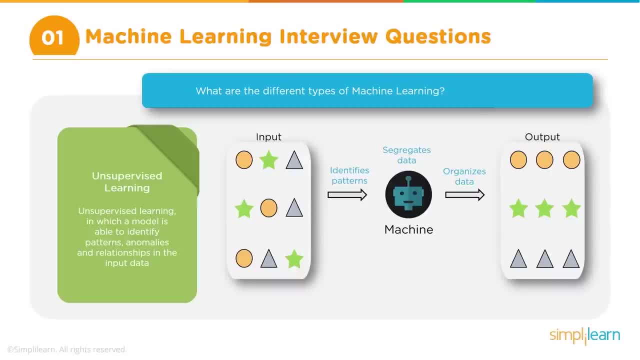 supervised learning- we perform or we do regression and classification. and unsupervised learning, we do clustering, and clustering can be of different types. Similarly, regression can be of different types, but you don't have to probably elaborate so much. if they are asking for just the different types, you can just mention these and just at a very high level. but if they, 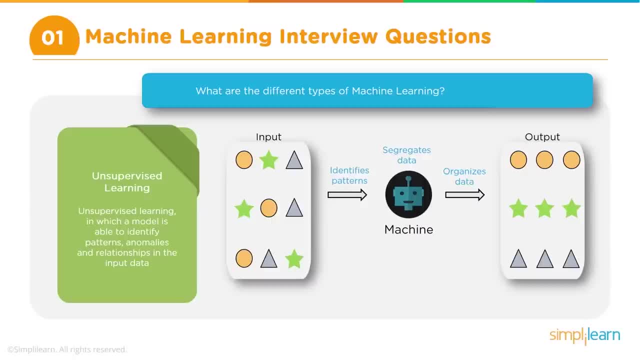 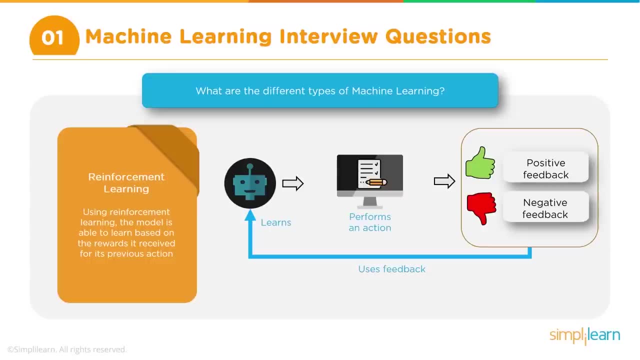 want you to elaborate, give examples, then, of course. I think there is a different question for that. we will see that later. Then the third: so we have supervised, then we have unsupervised, and then reinforcement. you need to provide a little bit of information around that as well, because it is 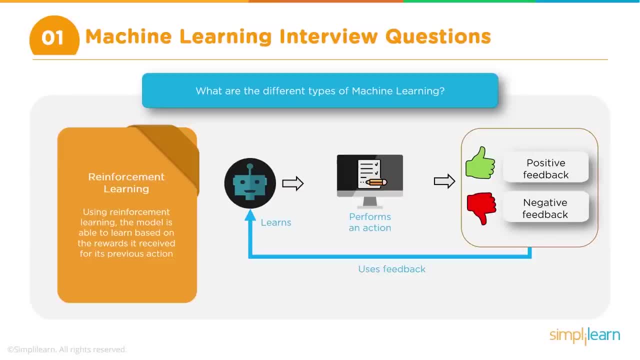 sometimes a little difficult to come up with a good definition for reinforcement learning, So you may have to a little bit elaborate on how reinforcement learning works right. So reinforcement learning works in such a way that it basically has two parts to it. one is the agent and the environment. 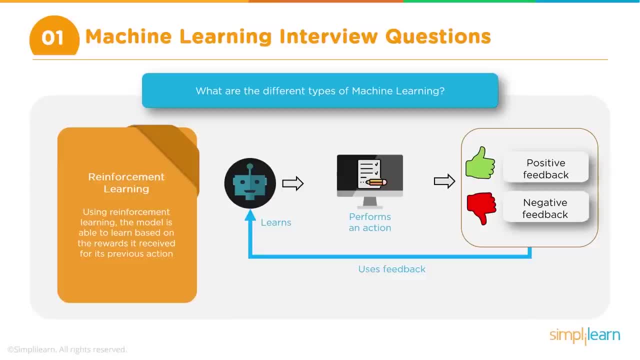 and the agent basically is working inside of this environment and it is given a target that it has to achieve and every time it is moving in the direction of the target. so the agent basically has to take some action and every time it takes an action which is moving the agent towards the 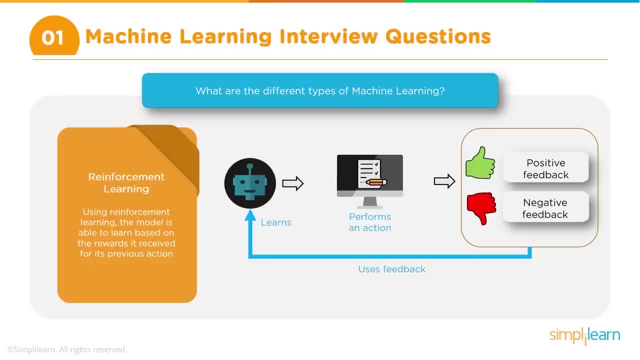 target right towards a goal. a target is nothing but a goal. So the agent basically has to take a particular level than it is rewarded, and every time it is going in a direction where it is a wave from the goal, than it is punished. So that is the way you can. 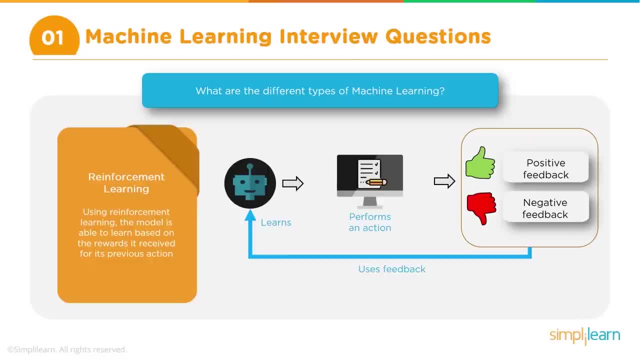 a little bit explain. and this is used primarily or it is very, very impactful, or teaching the system to learn games and so on. Examples of this are basically used in alpha go Also- you can throw that as an example- where alpha co used reinforcement learning to actually 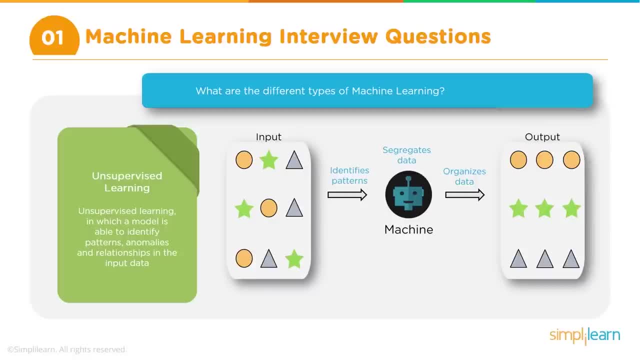 labeled. So the system has to figure out a way to do some analysis on this. So that is unsupervised learning, And you can then add a few things like what are the ways of performing supervised learning and unsupervised learning and what are some of the techniques. So 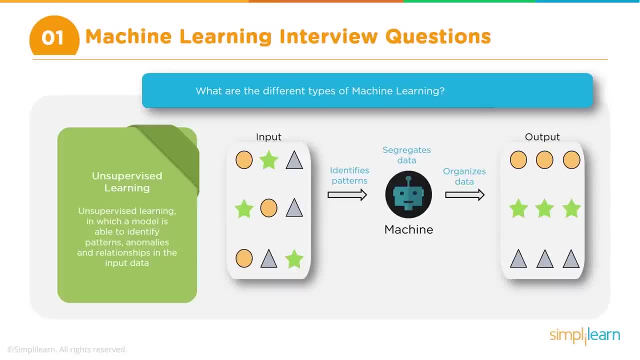 supervised learning: we perform or we do regression and classification, And unsupervised learning: we do clustering, And clustering can be of different types. Similarly, regression can be of different types, But you don't have to probably elaborate so much if they are asking. 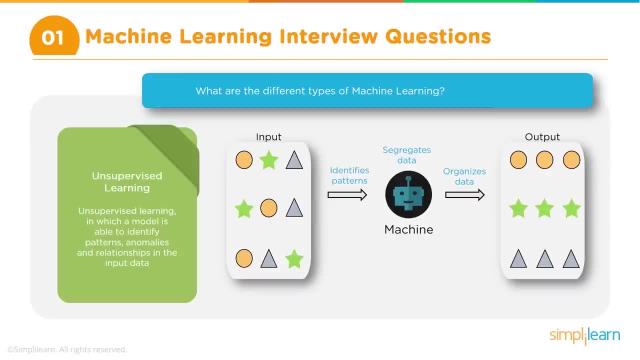 for just the different types. You can just mention these, and just at a very high level. But if they want you to elaborate, give examples, then of course I think there is a different question for that. We will see that later. Then the 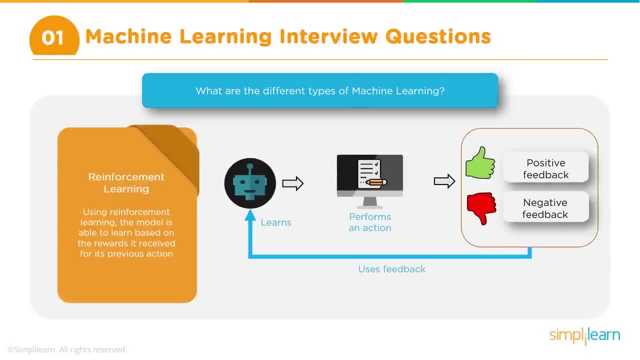 third: so we have supervised, then we have unsupervised, and then reinforcement. You need to provide a little bit of information around that as well, because it is sometimes a little difficult to come up with a good definition for reinforcement learning. So you may have to a little bit. 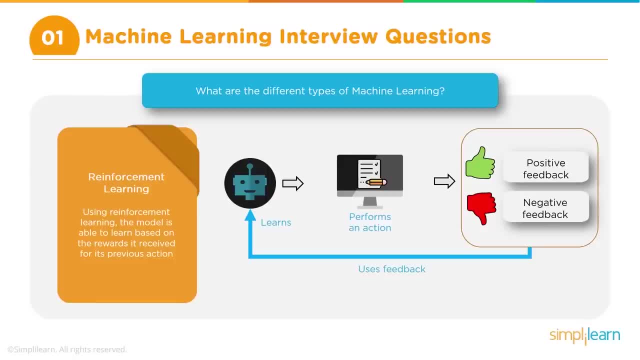 elaborate on how reinforcement learning works. So reinforcement learning works in such a way that it basically has two parts to it. One is the agent and the environment, And the agent basically is working inside of this environment and it is given a target that it has to achieve. And 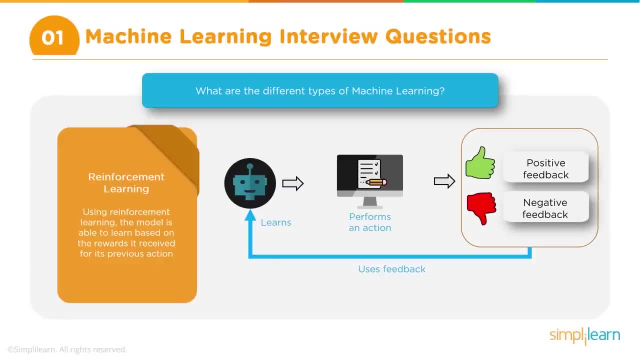 every time it is moving in the direction of the target. So the agent basically has to take some action And every time it takes an action which is moving the agent to towards the target, towards a goal- A target is nothing but a goal- Then it is. 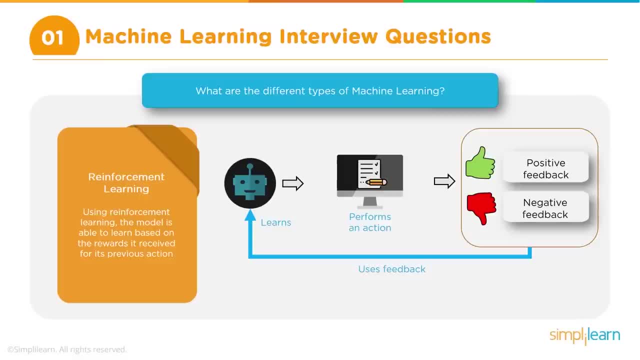 rewarded, And every time it is going in a direction where it is away from the goal, then it is punished. So that is the way you can a little bit explain. And this is used primarily, or very, very impactful, for teaching the system to learn games. 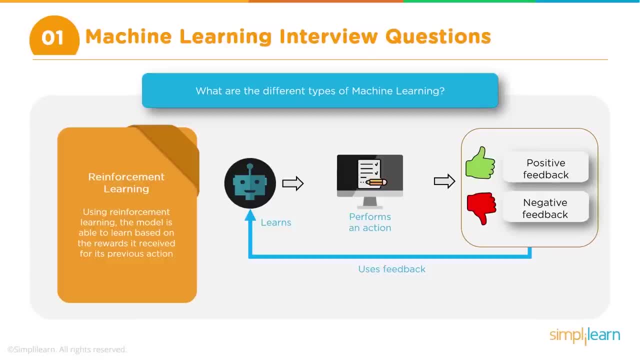 and so on. Examples of this are basically used in AlphaGo- You can throw that as an example- where AlphaGo used reinforcement learning to actually learn to play the game of Go and finally it defeated the Go World Champion. This much of information that would be. 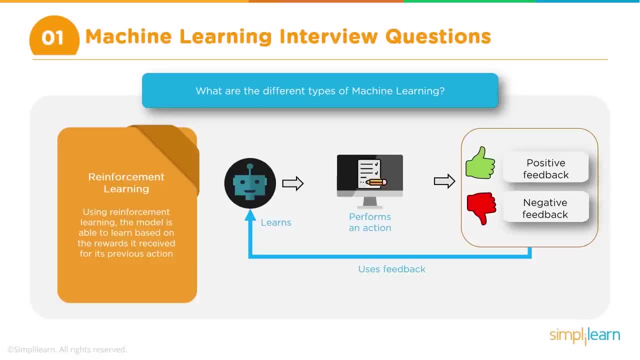 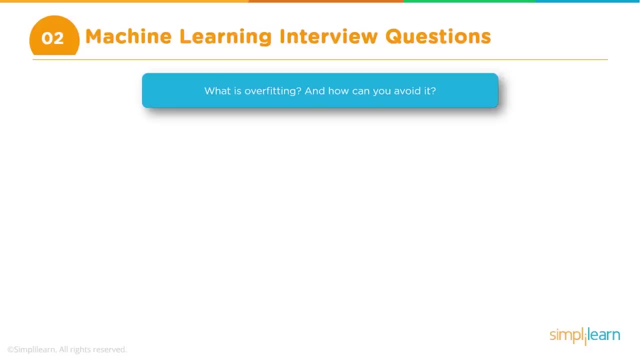 learn music to play the game of Go and finally it defeated the Go world champion. right, This much of information? that would be good enough. okay, Then there could be a question on overfitting. So the question could be: what is overfitting and how can you avoid it? 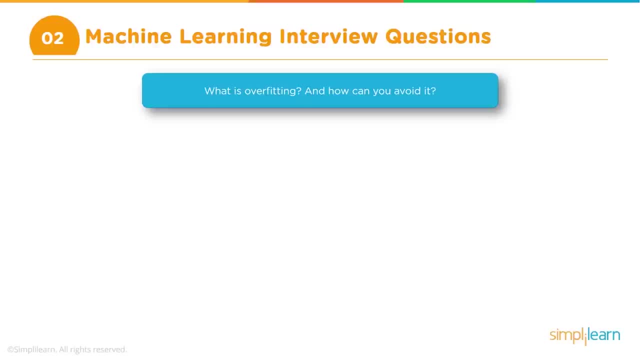 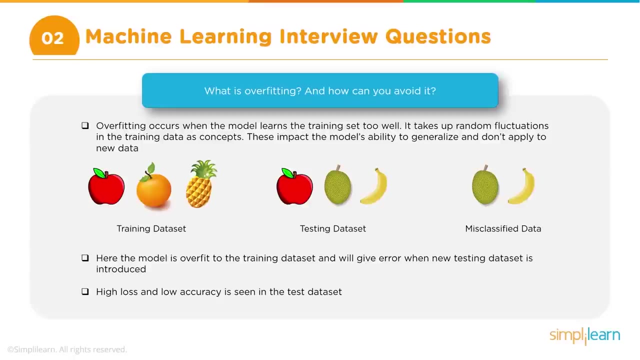 So what is overfitting? Let's first try to understand the concept, because sometimes overfitting may be a little difficult to understand. Overfitting is a situation where the model has kind of memorized the data. So this is an equivalent of memorizing the data. 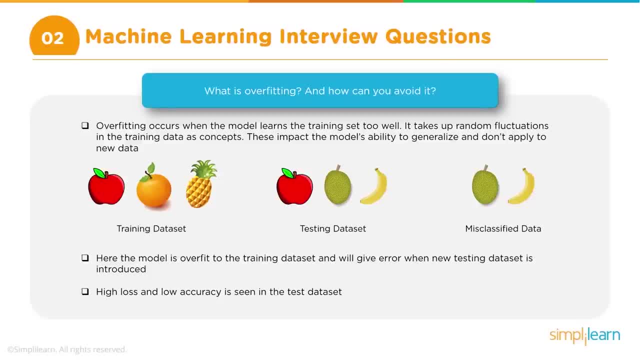 So we can draw an analogy so that it becomes easy to explain this. Now, let's say you're teaching a child about recognizing some fruits or something like that. okay, And you're teaching this child about recognizing, let's say, three fruits: apples, oranges. 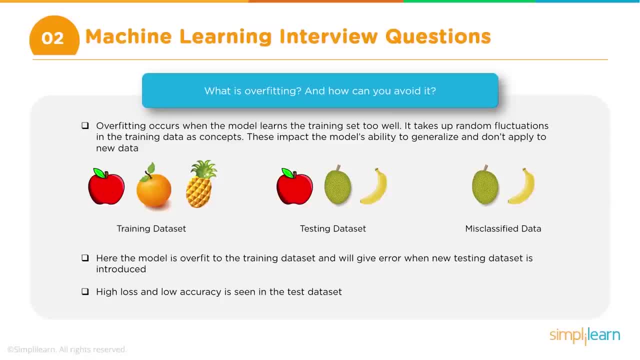 and pineapples. okay, So this is a small child and for the first time, you're teaching the child to recognize fruits. Then, so what will happen? So this is very much like that is your training data set. So what you will do is you will take a basket of fruits which consists of apples, oranges, 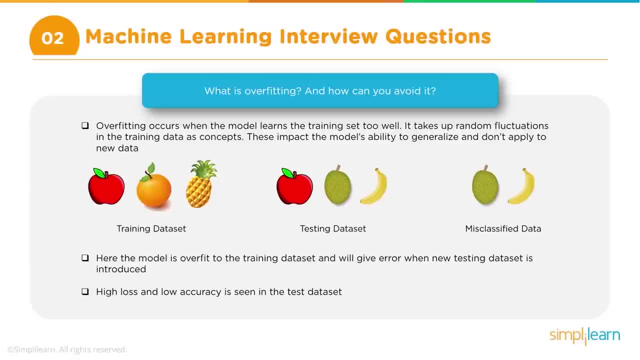 and pineapples, okay, And you take this basket to this child and there may be, let's say, hundreds of these fruits. So you take this basket to this child and keep showing each of this fruit and then, first time, obviously, the child will not know what it is. 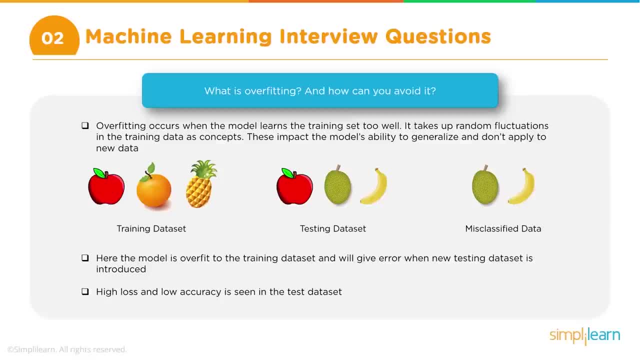 So you show an apple and you say: hey, this is apple. Then you show maybe an orange and say: this is orange, and so on and so forth, And then again you keep repeating that, right So until that basket is over. 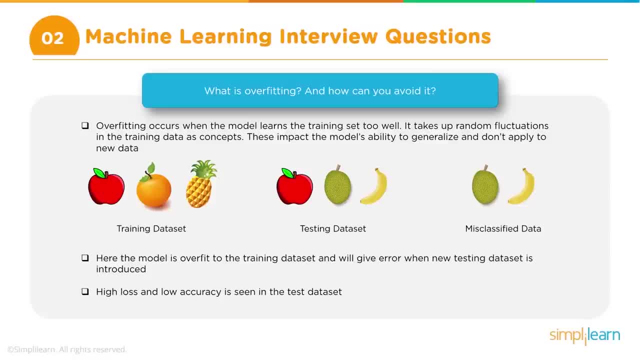 This is basically how training works. in machine learning also. That's how training works. So until the basket is completed, maybe a hundred fruits- you keep showing this child And then in the process, what has happened? the child has pretty much memorized these. 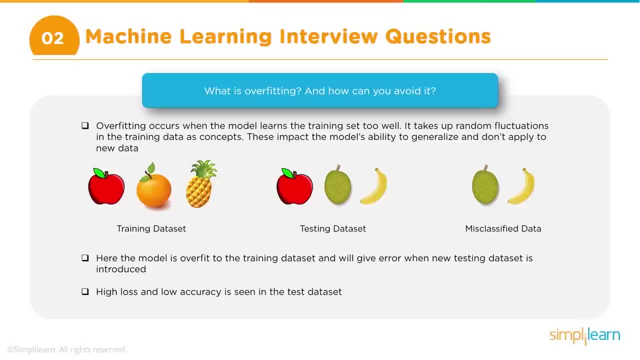 So even before you finish that basket, right by the time you are halfway through, the child has learned about recognizing the Okay Okay Apple, orange and pineapple. Now what will happen after, halfway through? initially, you remember it made mistakes in. 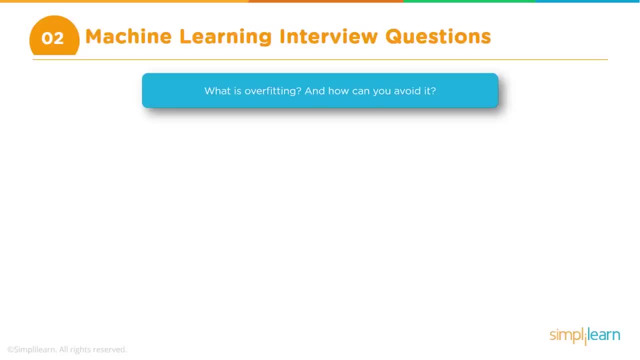 good enough. Then there could be a question on overfitting. So the question could be: what is overfitting and how can you avoid it? So what is overfitting? Let's first try to understand the concept, because sometimes overfitting. 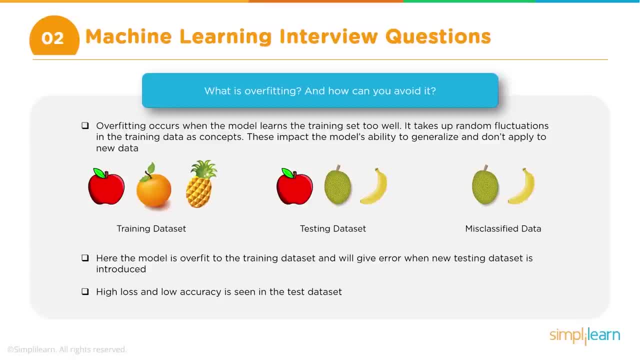 may be a little difficult to understand. Overfitting is a situation where the model has kind of memorized the data. So this is an equivalent of memorizing the data. So we can draw an analogy so that it becomes easy to explain this. Now let's say: 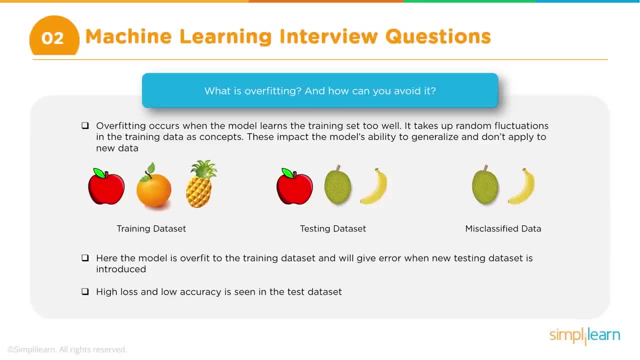 you are teaching a child about recognizing some fruits or something like that, And you are teaching this child about recognizing, let's say, three fruits: Apples, oranges and pineapples. So this is a small child and for the first time you are teaching the child to. 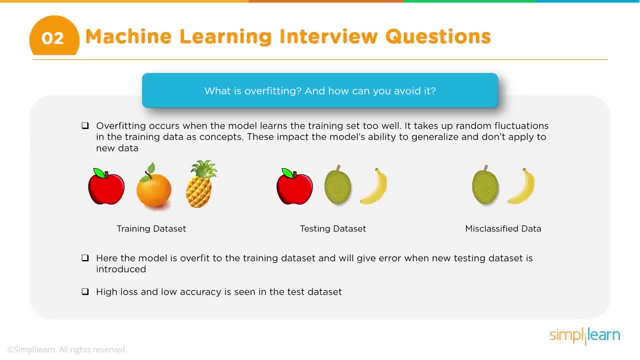 recognize fruits Then. so what will happen? So this is very much like that is your training data set. So what you will do is you will take a basket of fruits which consists of apples, oranges and pineapples, Okay, And 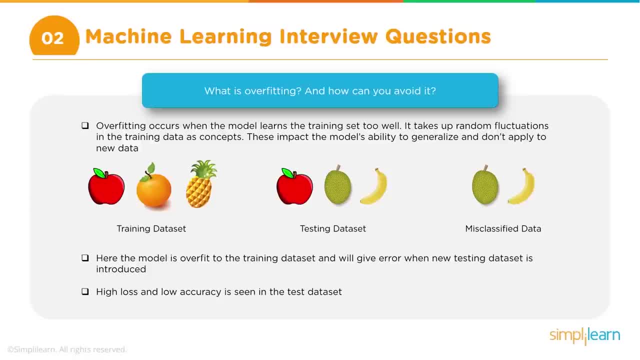 you take this basket to this child and there may be, let's say, hundreds of these fruits. So you take this basket to this child and keep showing each of this fruit and then, first time, obviously, the child will not know what it is. So you 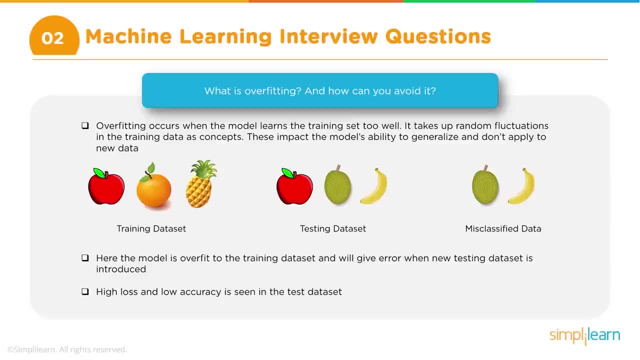 show an apple and you say: hey, this is apple. Then you show maybe an orange and say: this is orange, and so on and so forth, And then again you keep repeating that Right Till that basket is over. This is basically how training works In machine learning. 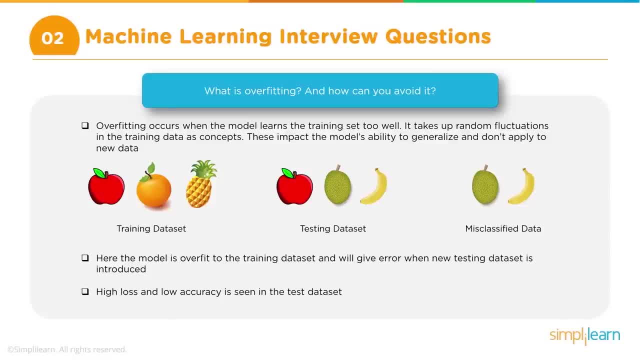 also that's how training works. So till the basket is completed, maybe hundred fruits. you keep showing this child In the process what has happened. the child has pretty much memorized these. So even before you finish that basket, Right By the time you are 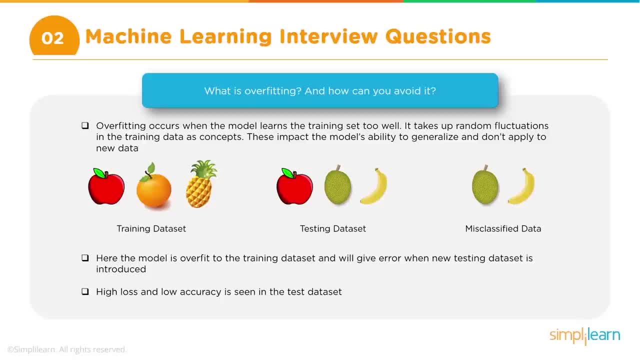 half way through the child has learnt about recognizing the apple, orange and pineapple. Now what will happen after half way through? initially you remember it made mistakes in recognizing, but half way through now it has learnt. So every time you show a fruit it will exactly hundred percent. 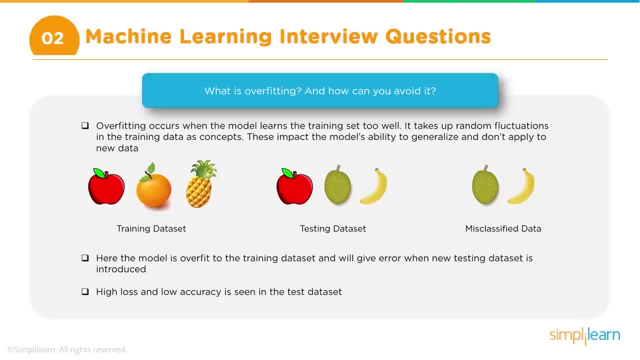 recognizing. but halfway through, now it has learned. So every time you show a fruit, it will exactly a hundred percent accurately it will identify. It will say: the child will say: this is an apple, this is an orange. And if you show a pineapple it will say: this is a pineapple, right. 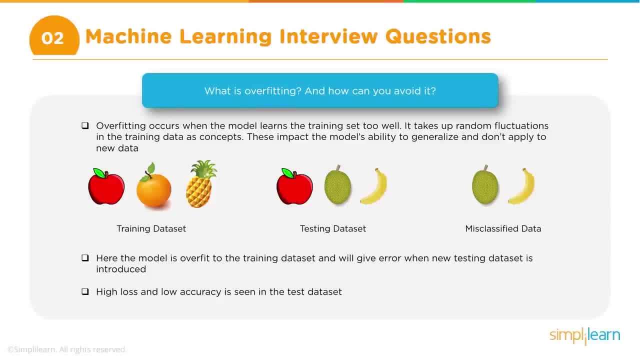 So that means it has kind of memorized this data. Now, let's say you bring another basket of fruits and it will have a mix of maybe apples, which were already there in the previous set, but it will also have in addition to: 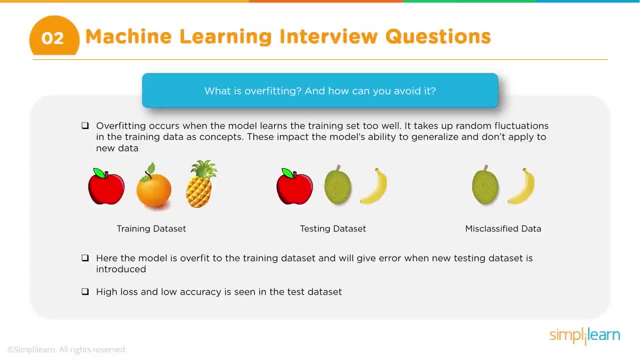 apple, it will probably have a banana or maybe another fruit like a jackfruit, right? So this is an equivalent of your test data set, which the child has not seen before. Some parts of it it probably has seen, like the apples it has seen, but this banana and 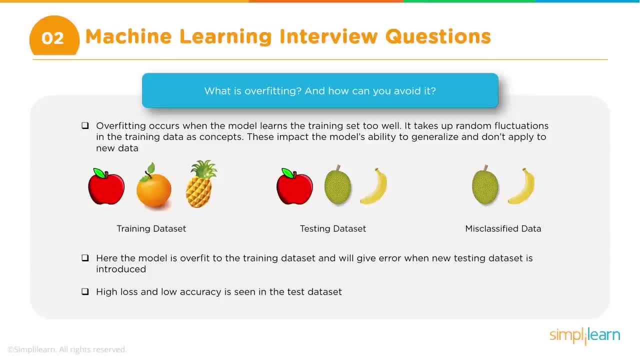 jackfruit. it has not seen. So then what will happen in the first round, which is an equivalent of your training data set towards the end? it has a hundred percent. It was telling you what the fruit is. The fruits are right. 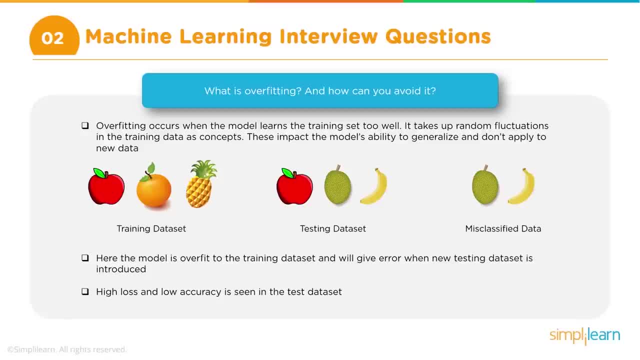 Apple was accurately recognized, Orange was accurately recognized and pineapples were accurately recognized, right. So that is like a hundred percent accuracy. But now, when you get another, a fresh set, which were not part of the original one, what will happen? 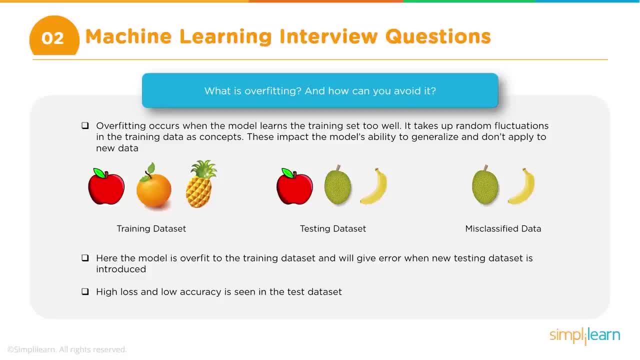 All the apples maybe it will be able to recognize correctly, but all the others, like the jackfruit or the banana, will not be recognized by the child, right? So this is an analogy. This is an equivalent of overfitting. So what has happened? 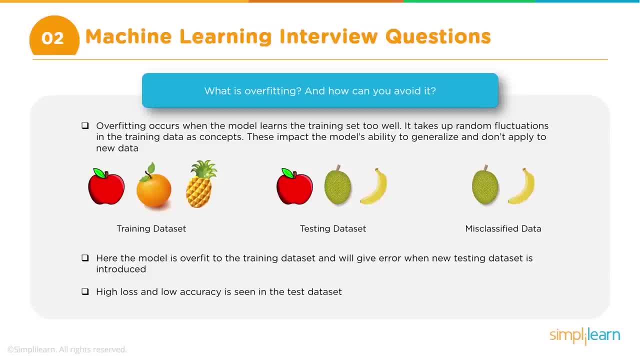 During the training Process. it is able to recognize or reach a hundred percent accuracy, maybe very high accuracy, Okay, And we call that as very low loss, right? So that is the technical term. So the loss is pretty much zero and accuracy is pretty much a hundred percent. 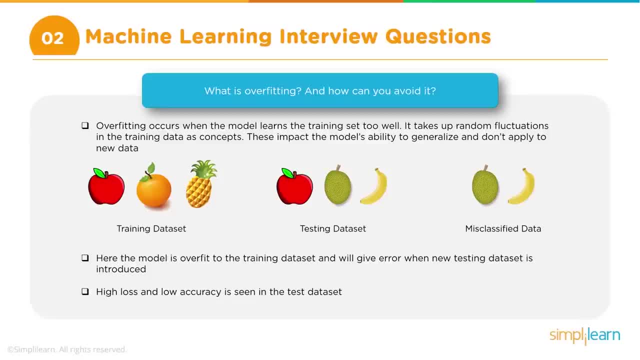 Whereas when you use testing, there will be a huge error, which means the loss will be pretty high and therefore the accuracy will be also low. Okay, This is known as overfitting. This is basically a process where training is done. Training process is: 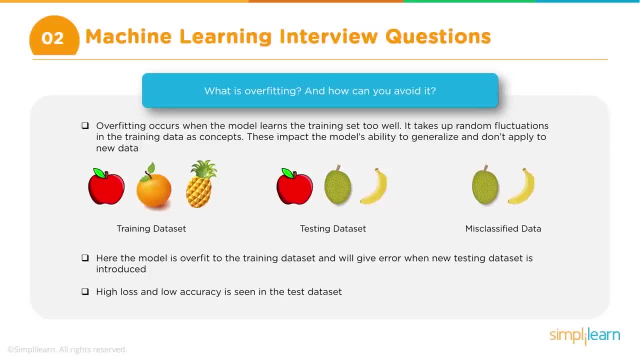 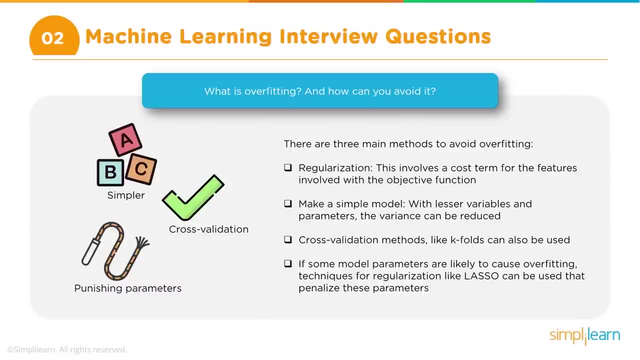 It goes very well, almost reaching a hundred percent accuracy, but while testing it really drops down. Now how can you avoid it? So that is a extension of this question. There are multiple ways of avoiding overfitting. There are techniques like what you call regularization. 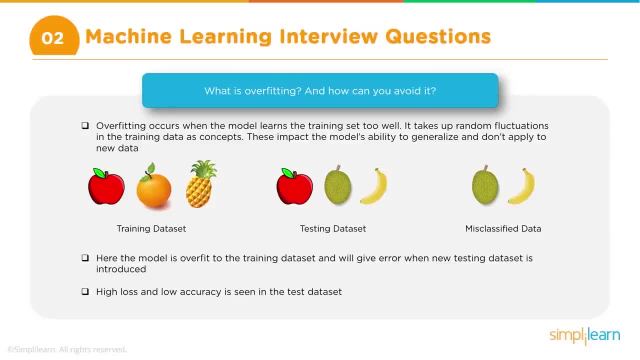 accurately, it will identify. It will say: the child will say: this is an apple, this is an orange, and if you show a pineapple it will say: this is a pineapple, Right? So that means it has kind of memorized this data. Now let's say 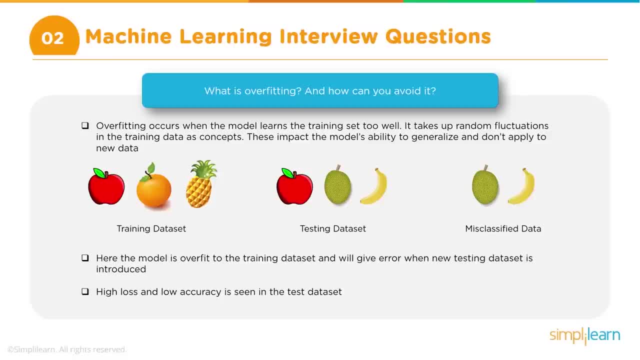 you bring another basket of fruits and it will have a mix of maybe apple, which were already there in the previous set, but it will also have in addition to apple. it will probably have a banana or maybe another fruit like a jackfruit, Right. So this is an equivalent. 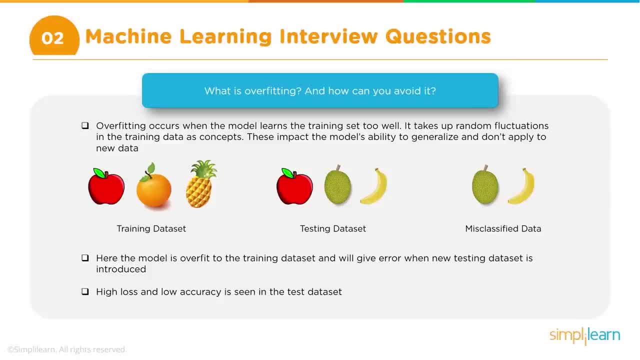 of your test data set which the child has not seen before. Some parts of it it probably has seen, like the apples it has seen, but this banana and jackfruit it has not seen. So then, what will happen in the first round, which is an equivalent of your training data? 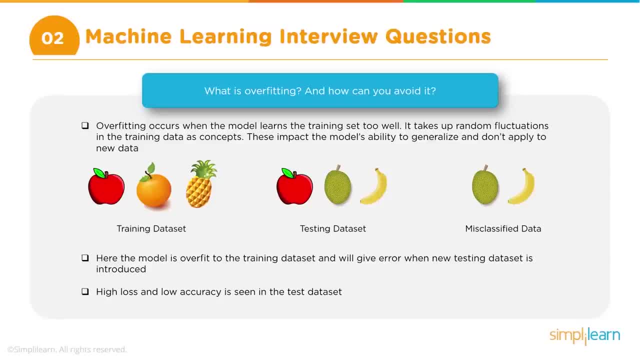 set towards the end. it has hundred percent. it was telling you what the fruits are Right: Apple was accurately recognized, Orange was accurately recognized and pineapples were accurately recognized Right. So that is like a hundred percent accuracy. But now, when you get another, 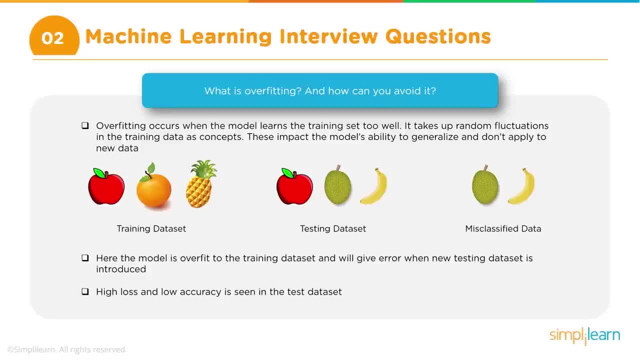 fresh set which were not part of the original one. what will happen? all the apples maybe it will be able to recognize correctly, but all the others, like the jackfruit or the banana, will not be recognized by the child Right. So this is an analogy. this is an equivalent of overfitting. 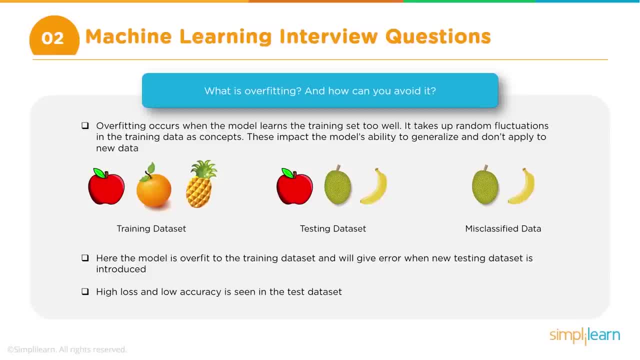 So what has happened during the training process? it is able to recognize or reach hundred percent accuracy, maybe very high accuracy, Okay, And we call that as very low loss, Right? So that is the technical term. So the loss is pretty. 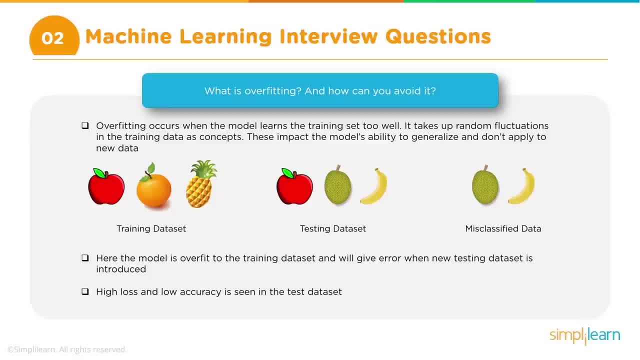 much zero and accuracy is pretty much hundred percent, whereas when you use testing, there will be a huge error, which means the loss will be pretty high and therefore the accuracy will be also low. Okay, This is known as overfitting. This is basically a process where training 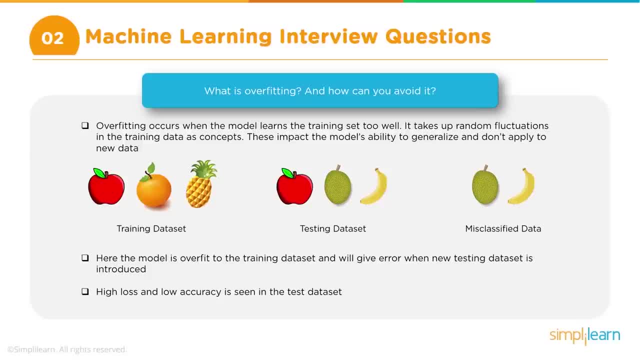 is done, training process is. it goes very well, almost reaching hundred percent accuracy, but while testing it really drops down. Now how can you avoid it? So that is the extension of this question. There are multiple ways of avoiding overfitting. There are 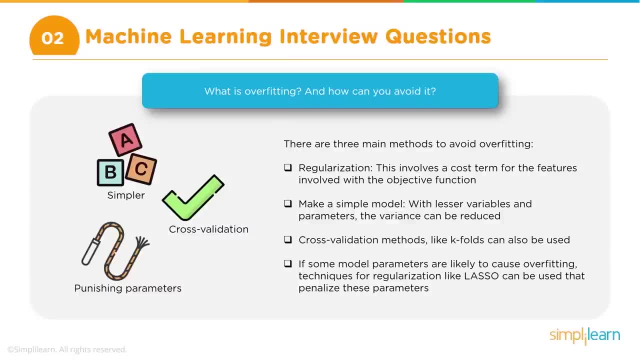 techniques like what you call regularization. that is the most common technique that is used for avoiding overfitting, and within regularization there can be a few other subtypes, like dropout in case of neural networks and a few other examples. but I think, if you give example or if you give 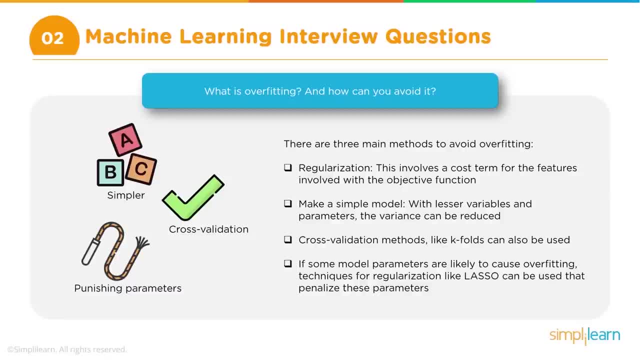 regularization as the technique. probably that should be sufficient. So there will be some questions where the interviewer will try to test your fundamentals and your knowledge and depth of knowledge and so on and so forth, and then there will be some questions which are more like quick questions that will be more to. 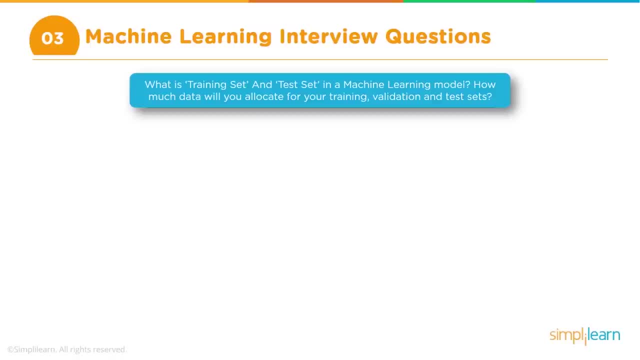 stump you. Okay, then the next question is around the methodology. So when we are performing machine learning training, we split the data into training and test, right? So this question is around that. So the question is: what is training set and test set? 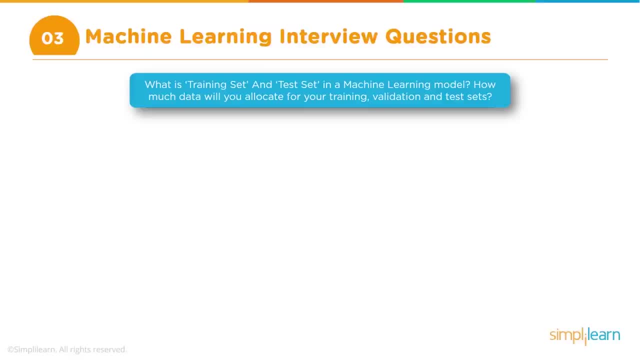 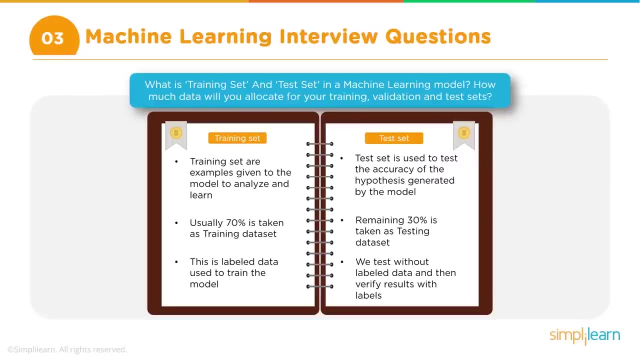 in machine learning model and how is the split done? So the question can be like that: So in machine learning, when we are trying to train the model, so we have a three-step process: We train the model and then we test the model and 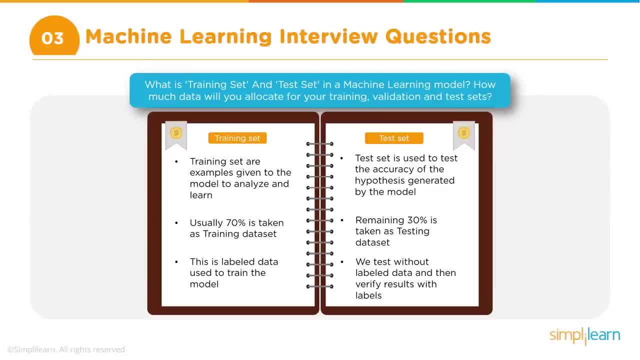 then, once we are satisfied with the test, only then we deploy the model. So what happens in the train and test is that you remember the labeled data. So let's say you have thousand records with labeling information. Now one way of doing it is you use all. 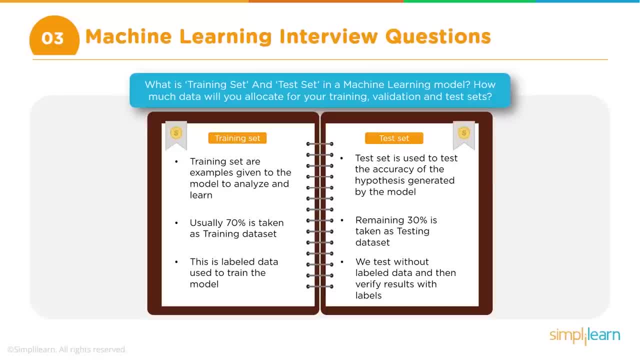 the thousand records for training, and then maybe right, which means that you have exposed all this thousand records during the training process, and then you take a small set of the same data and then you say, okay, I will test it with this, Okay, and then you 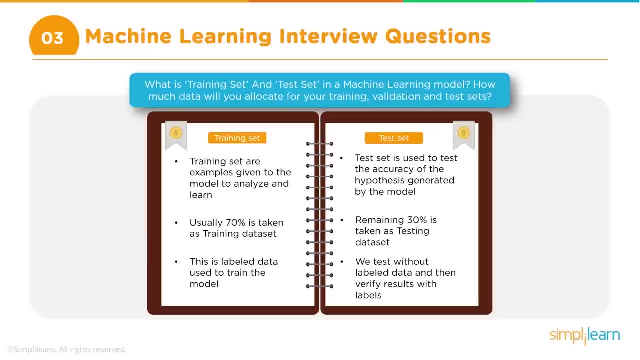 probably what will happen. you may get some good results right, but there is a flaw there. What is the flaw? This is very similar to human beings. It is like you are showing this model, the entire data, as a part of training. Okay, so, 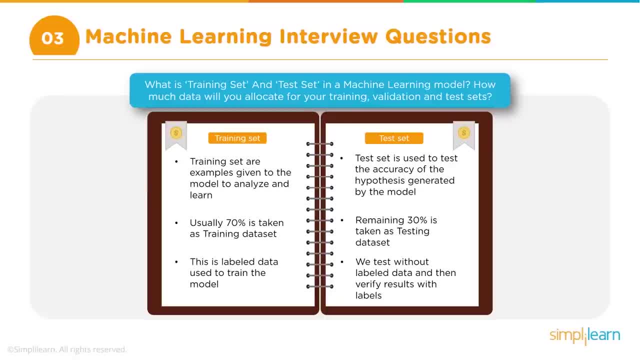 obviously it has become familiar with the entire data. So when you are taking a part of that again and you are saying that I want to test it, obviously you will get good results. So that is not a very accurate way of testing. So that is. 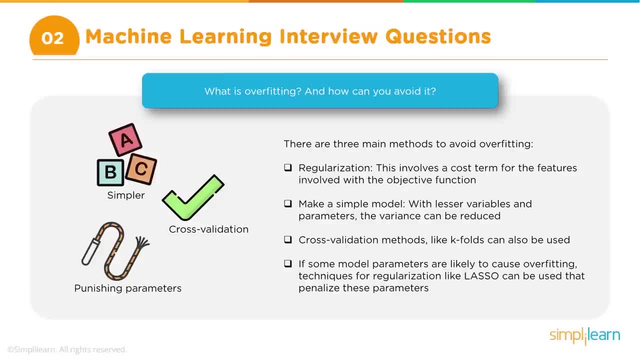 That is the most common technique that is used for avoiding overfitting and within regularization there can be a few other subtypes, like dropout in case of neural networks and a few other examples. But I think if you give example or if you give regularization as the technique, probably 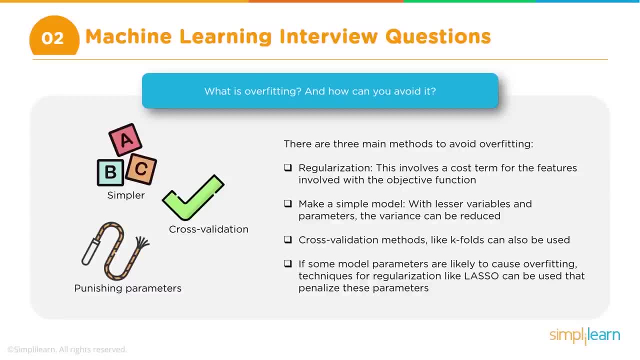 that should be sufficient. So there will be some questions where the interviewer will try to test your fundamentals and your knowledge and depth of knowledge and so on and so forth, And then there will be some questions which are more like quick questions that will be more to stump you. 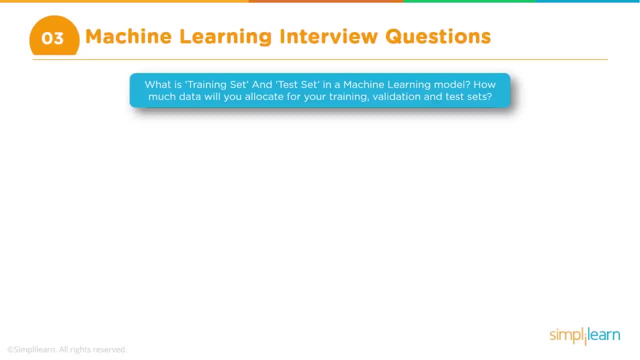 Okay, Then the next question is around the methodology. So when we are performing Performing machine learning training, we split the data into training and tests, right? So this question is around that. So the question is: what is training set and test set in machine learning model and how? 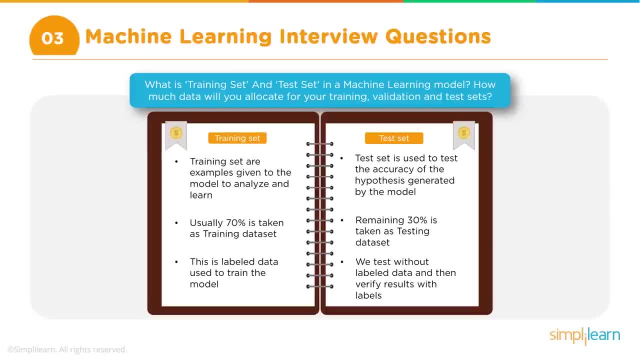 is the split done? So the question can be like that. So in machine learning, when we are trying to train the model, so we have a three step process: We train the model and then we test the model And then, once we are satisfied with the test, only then we deploy the model. 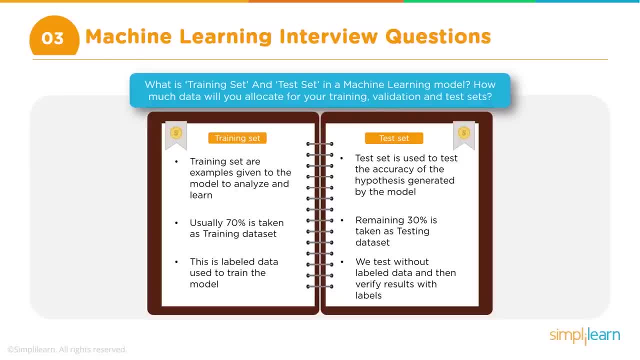 So what happens In the train and test is that you remember the labeled data. So let's say you have thousand records with labeling information. Now one way of doing it is you use all the thousand records for training and then maybe right, which means that you have exposed all this thousand records during the training. 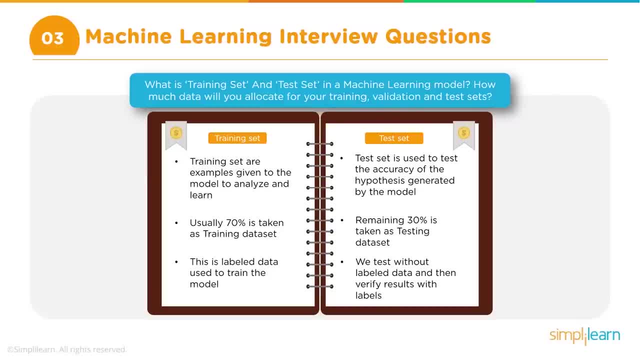 process and then you take a small set of the same data and then you say, okay, I will test it with this, Okay, And then you probably what will happen. Okay, And then you probably what will happen. Okay, And then you probably what will happen. 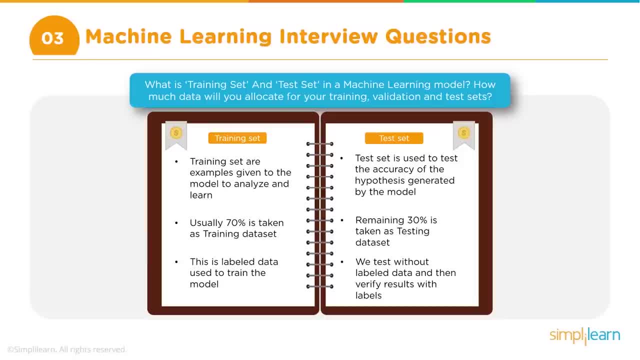 You may get some good results right, But there is a flaw there. What is the flaw? This is very similar to human beings. It is like you are showing this model, the entire data, as a part of training. Okay, So obviously it has become familiar with the entire data. 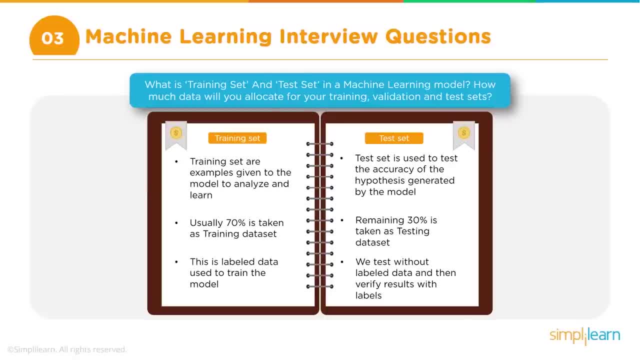 So when you're taking a part of that again and you're saying that I want to test it, obviously you will get good results. So that is not a very accurate way of testing. So that is the reason what we do is we have the label data of this thousand records or whatever. 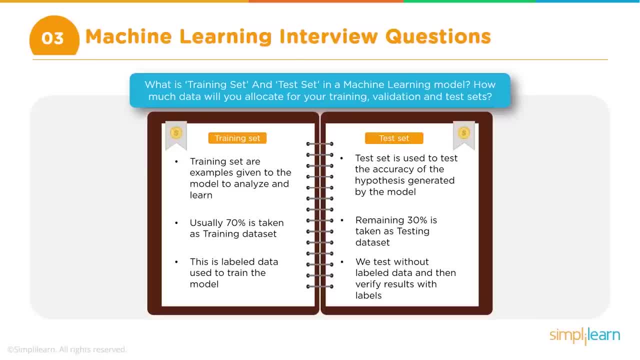 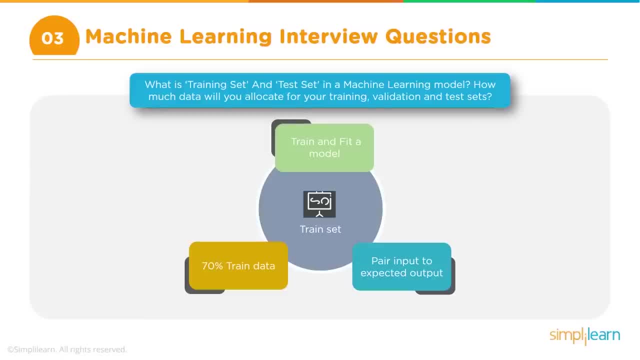 the reason what we do is we have the label data of this thousand records or whatever we set aside before starting the training process. We set aside a portion of that data and we call that test set and the remaining we call as training set and we use only. 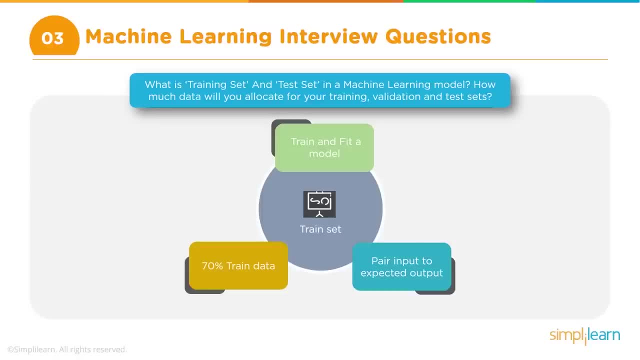 this for training, our model Now, the training process, remember, is not just about passing one round of this data set. So let us say now your training set has 800 records. It is not just one time you pass this 800 records. What? 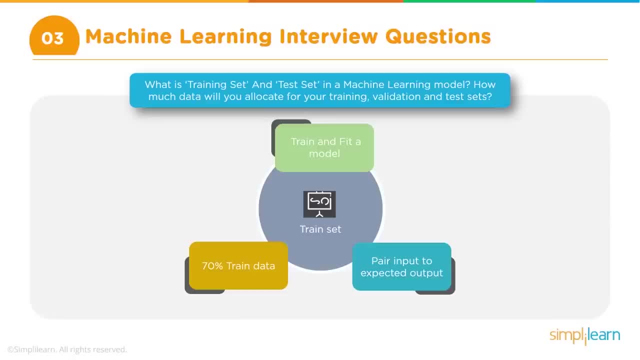 you normally do, is you actually as a part of the training, you may pass this data through the model multiple times. So this thousand records may go through the model maybe 10,, 15,, 20 times, till the training is perfect, till the accuracy is high, till the 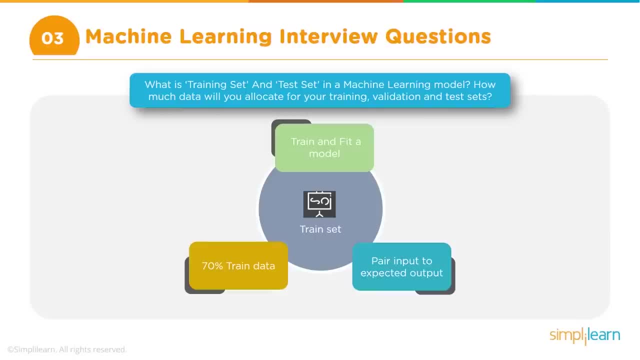 errors are minimized Now so, which is fine, which means that your- that is what is known as the model- has seen your data and gets familiar with your data. and now, when you bring your test data, what will happen is: this is like some new data, because that is where the real test. 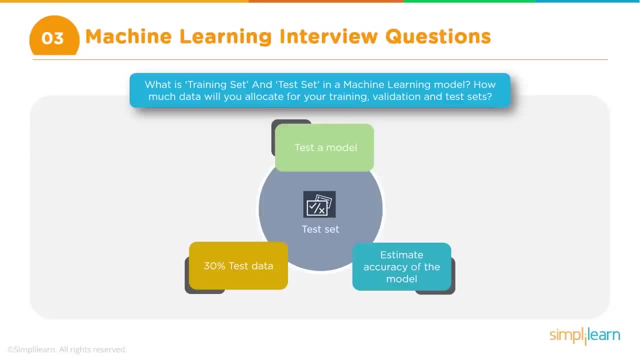 is: Now you have trained the model and now you are testing the model with some data which is kind of new. that is like a situation, like a realistic situation, because when the model is deployed, that is what will happen: it will receive some new data, not the data. 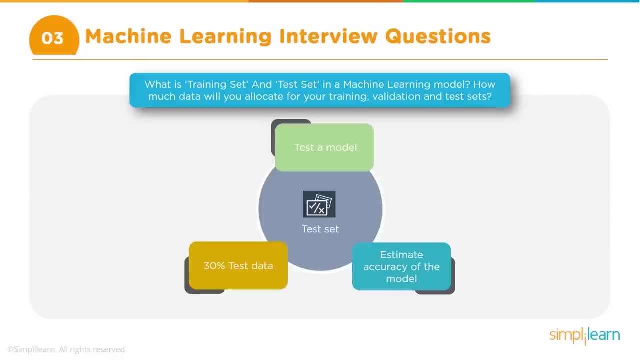 that it has already seen right. So this is a realistic test. So you put some new data. So this data which you have set aside is for the model. it is new and if it is able to accurately predict the values, that means your training has. 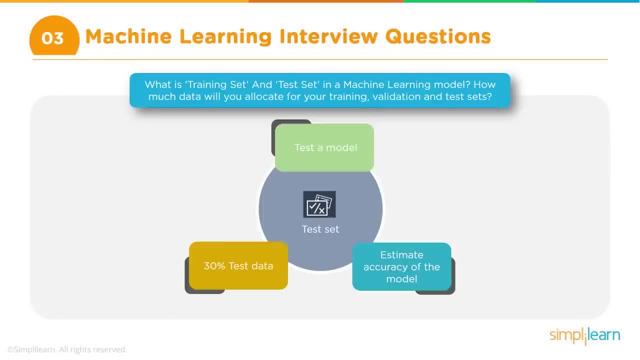 worked, The model got trained properly. but, let us say, while you are testing this, with this test data, you are getting lot of errors. that means you need to probably either change your model or retrain with more data and things like that. Now coming back to the question of 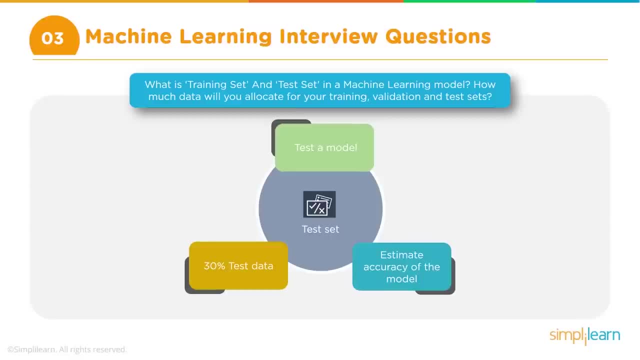 how do you split this? what should be the ratio? there is no fixed number. again, this is like individual preferences. some people split it into 50-50, 50% test and 50% training. some people prefer to have a larger amount for training and a smaller amount for test. 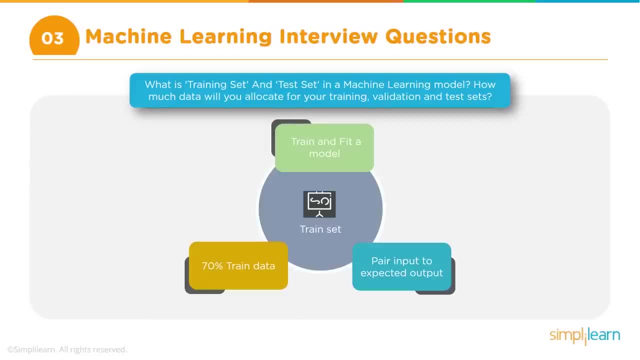 We set aside. before starting the training process, we set aside a portion of that data and we call that test set and the remaining we call this training set, and we use only this for training our model. Now the training process, remember, is not just about passing one round of this data set. 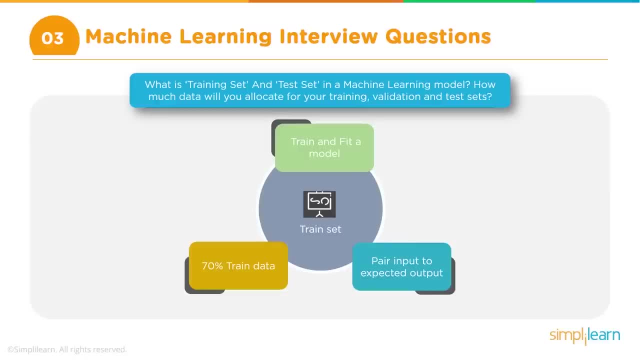 So let's say now your training set has 800 records. It is not just one time you pass this 800 records. What you normally do is you actually, as a part of the training, you may pass this data through the model multiple times. 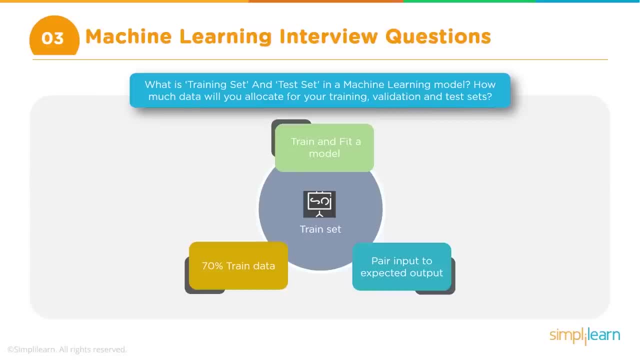 So this thousand records may go through the model, maybe 10,, 15,, 20 times, till the training is perfect, till the accuracy is high, till the errors are minimized. Okay Now so, which is fine, which means that your- that is what is known as the model- has seen your data and gets familiar with your data. 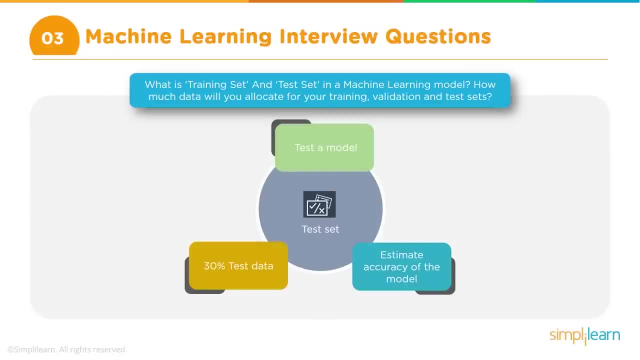 And now, when you bring your test data, what will happen is: this is like some new data, because that is where the real test is. Now you're trained The model and now you are testing the model with some data which is kind of new. 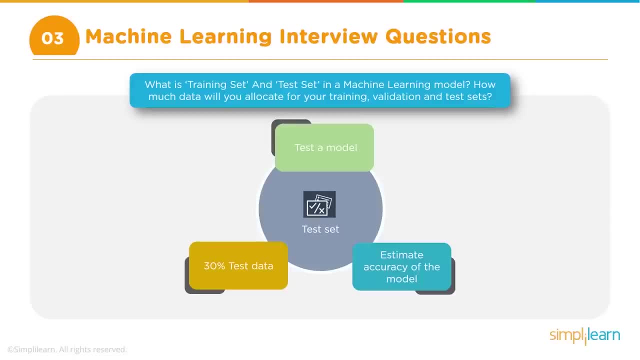 That is like a situation, like a realistic situation, because when the model is deployed- that is what will happen- It will receive some new data, not the data that it has already seen, right? So this is a realistic test. So you put some new data. 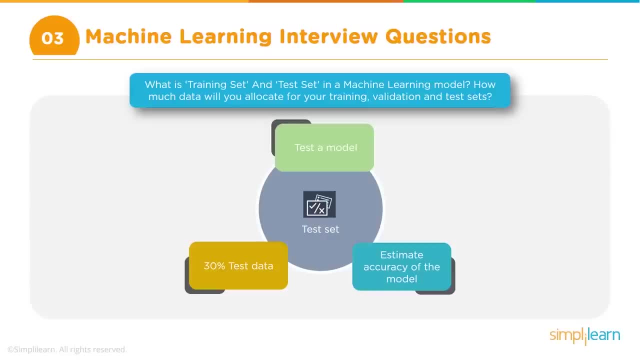 So this data which you have set aside is for the model. It is new And if it is able to accurately predict the values, that means your training has worked Okay, The model got trained properly. But let's say, While you're testing this, with this test data, you're getting a lot of errors. 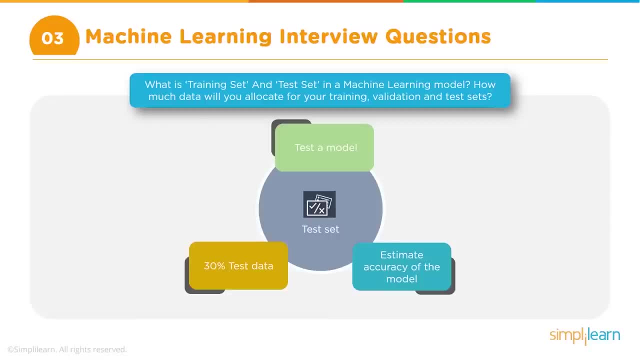 That means you need to probably either change your model or retrain with more data and things like that. Now coming back to the question of how do you split this? What should be the ratio? There is no fixed number. Again, this is like individual preferences. 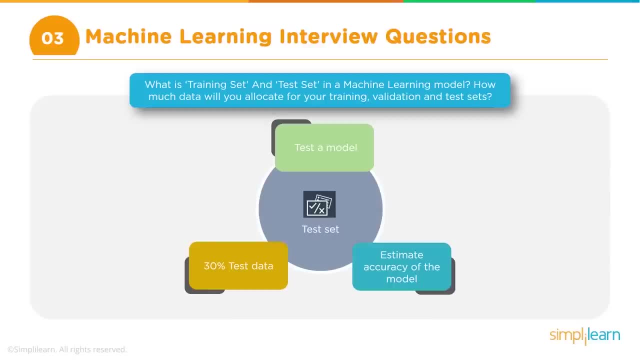 Some people split it into 50, 50,, 50% test and 50% training. Some people prefer to have a larger amount for training and a smaller amount for tests, So they can go by Either 60, 40 or 70, 30, or some people even go with some odd numbers like 65, 35 or 63.33 and 33,, which is like one third and two thirds. 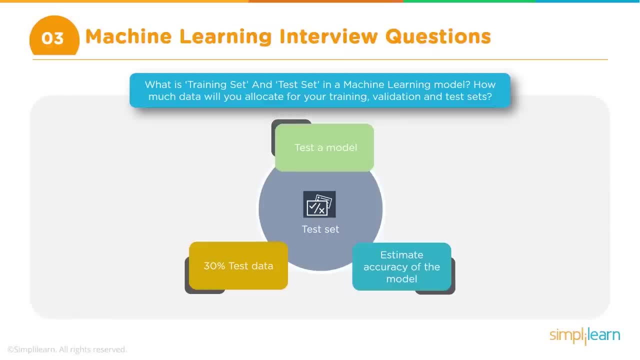 so they can go by either 60-40 or 70-30, or some people even go with some odd numbers like 65-35 or 63.33 and 33, which is like 1- 3rd and 2- 3rd. so there is no. 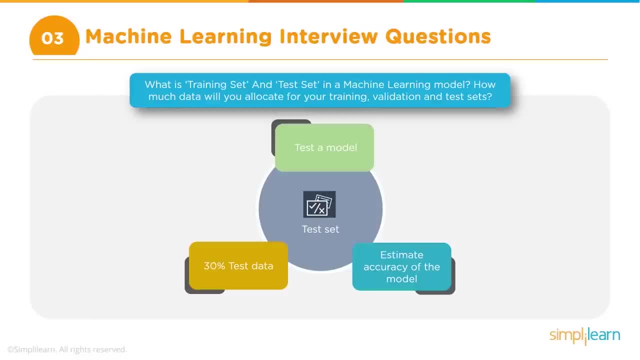 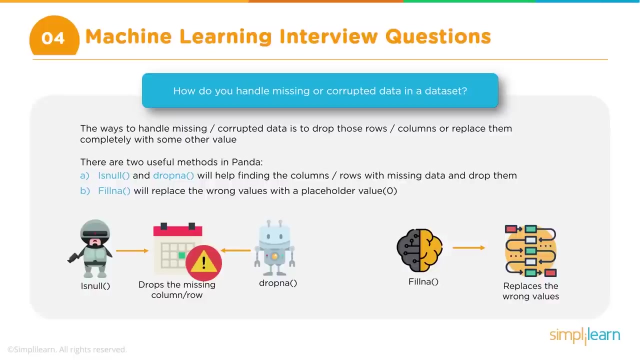 fixed rule, that it has to be something. the ratio has to be this: you can go by your individual preferences, alright. then you may have questions around data handling, data manipulation or what you call data management or preparation. so these are all some questions around that area. there is again. 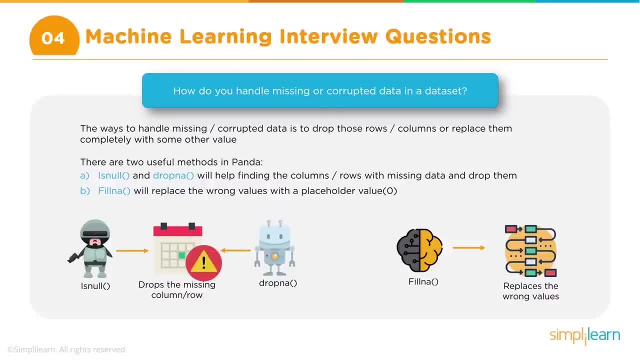 no one answer, one single good answer to this. it really varies from situation to situation and depending on what exactly is the problem, what kind of data it is, how critical it is, what kind of data is missing and what is the type of corruption. so there are whole lot of things, which is a very 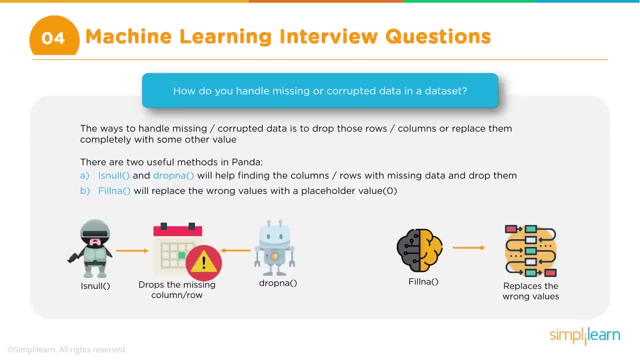 generic question and therefore you need to be little careful about responding to this as well. so probably have to illustrate this again. if you have experience in doing this kind of work in handling data, you can illustrate with examples, saying that I was on one project where I received this kind of data. these were the 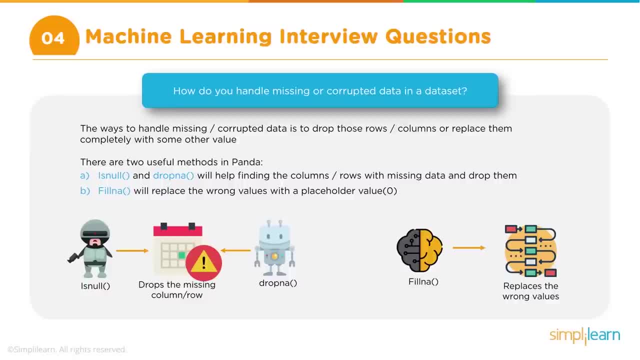 columns where data was not filled, or these were the this many rows where the data was missing. that would be, in fact, a perfect way to respond to this question, but if you don't have that, obviously you have to provide some good answer. I think it really depends on. 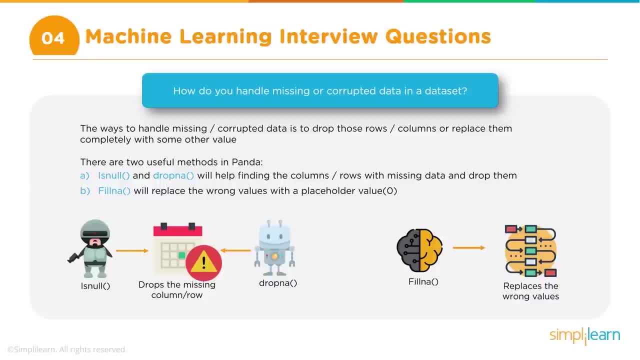 what exactly the situation is, and there are multiple ways of handling missing data or corrupt data. now let's take a few examples. let's say you have data where some values in some of the columns are missing and you have pretty much half of your data having these missing values in terms of number of 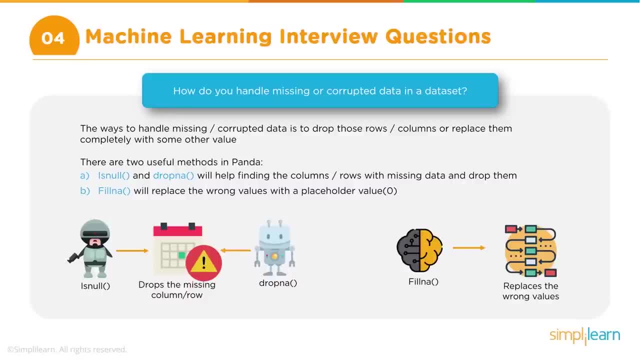 rows. okay, that could be one situation. another situation could be that you have records or data missing. but when you do some initial calculation, how many records are corrupt, or how many rows- or observations, as we call it- has this missing data? let's assume it is very minimal. 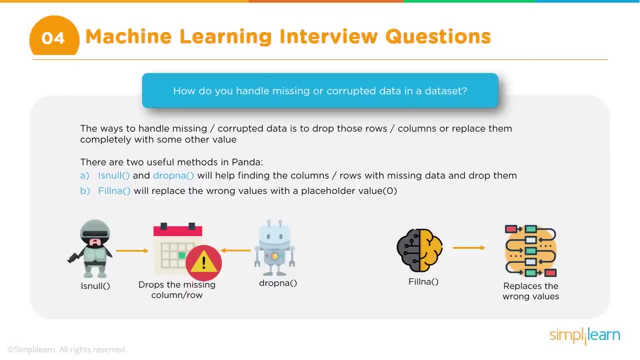 like 10 percent. okay, now, between these two cases, how do you so? let's assume that this is not a mission critical situation and in order to fix this 10 percent of the data, the effort that is required is much higher, and obviously effort means also time and money, right? so 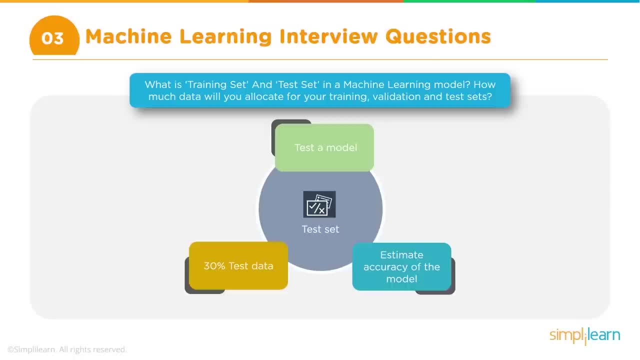 So there is no fixed rule that it has to be something. The ratio has to be this: You can go by your individual preferences, All right. Then you may have questions around data handling, data manipulation, or what do you call data management or preparation. 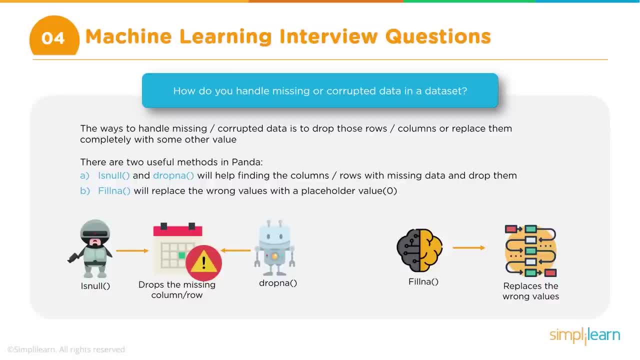 So these are all some questions around that. Okay, There is again no one answer, one single good answer to this. It really varies from situation to situation and depending on what exactly is the problem, what kind of data it is, how critical it is, what kind of data is missing and what is the type of corruption. 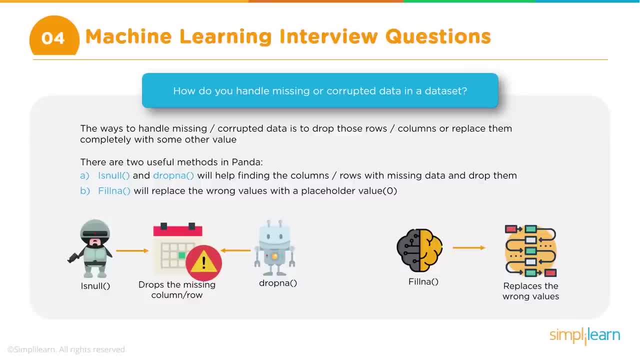 So there are a whole lot of things, which is a very generic question And therefore you need to be a little careful about responding to this as well. So probably have to illustrate this again, if you have experience in doing this kind of work in handling data. 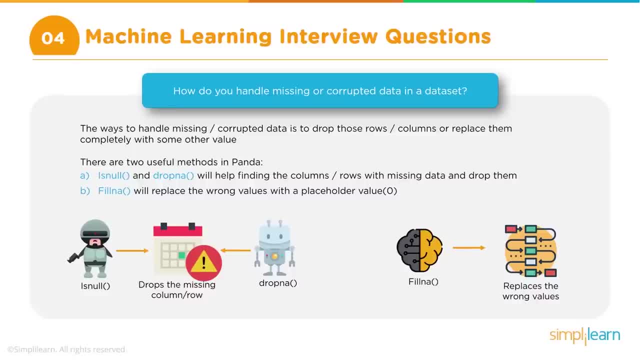 You can illustrate with examples, saying that I was on one project where I received this kind of data: these were the columns where data was not filled, or these were the this many rows where the data was missing. that would be, in fact, a perfect way to respond to this question. 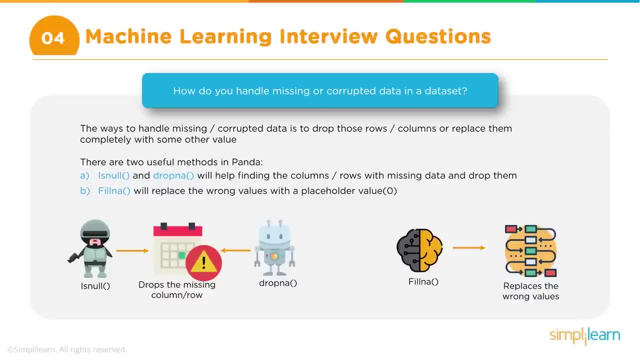 But if you don't have that, obviously you have to provide some good answer. I think it really depends on what exactly the situation is, And there are multiple ways of handling the missing data or corrupt data. Now let's see, Let's take a few examples. 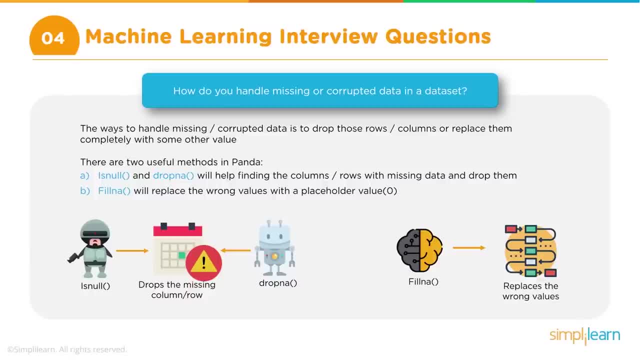 Now, let's say you have data where some values in some of the columns are missing and you have pretty much half of your data having these missing values in terms of number of rows. Okay, that could be one situation. Another situation could be that you have records or data missing, but when you do some initial calculation, how many records are corrupt, or how many rows- or observations, as we call it- has this missing data? 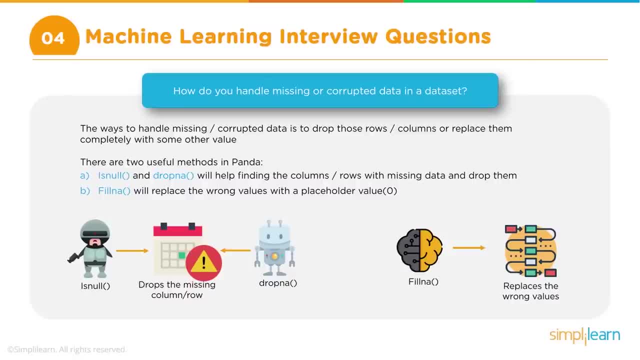 Let's assume it is very minimal, like 10%. okay, Now, between these two cases, how do you so? let's assume that this is not a mission critical situation And in order to fix this 10% of the data, the effort that is required is much higher. 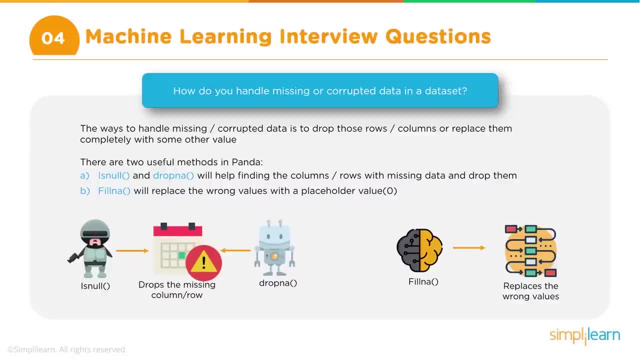 And obviously effort means also time and money, right, So it is not so mission critical and it is okay to, let's say, get rid of these records. So obviously one of the easiest ways of handling the data part or missing data. 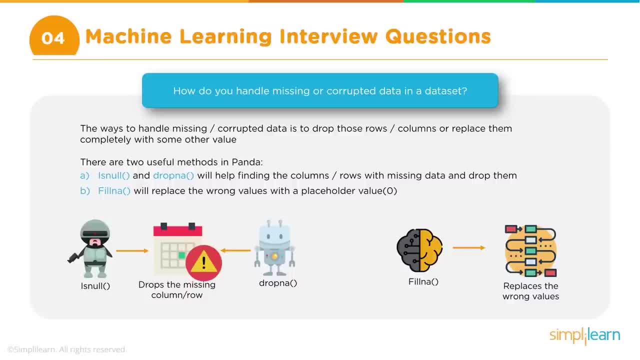 it is not so mission critical and it is okay to, let's say, get rid of these records. so obviously one of the easiest ways of handling the data part or missing data is remove those records or remove those observations from your analysis. so that is the easiest way to do. but then 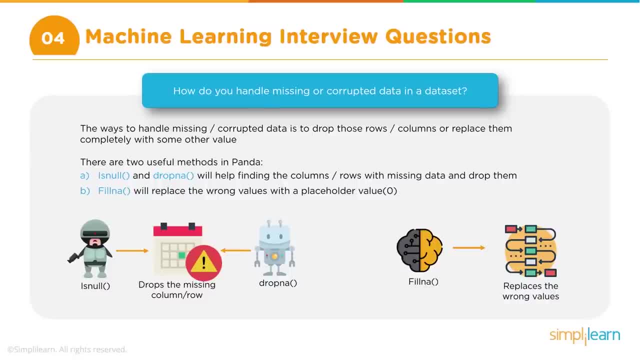 the downside is, as i said in the first case, if let's say, 50 percent of your data is like that, because some column or the other is missing, so it is not like every in every place, in every row, the same column is missing, but you have in maybe 10 percent. 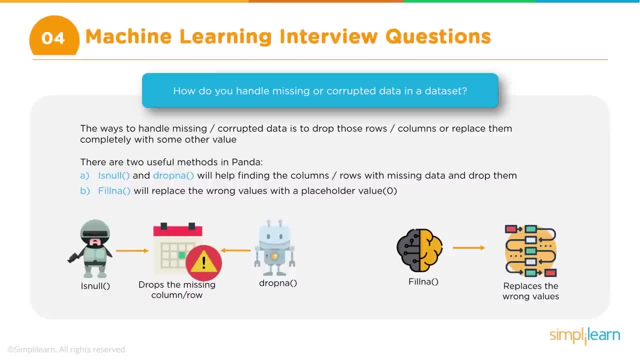 of the records, column 1 is missing and another 10 percent, column 2 is missing, another 10 percent. column 3 is missing, and so on and so forth. so it adds up to maybe half of your data set. so you cannot completely remove half of your data set. 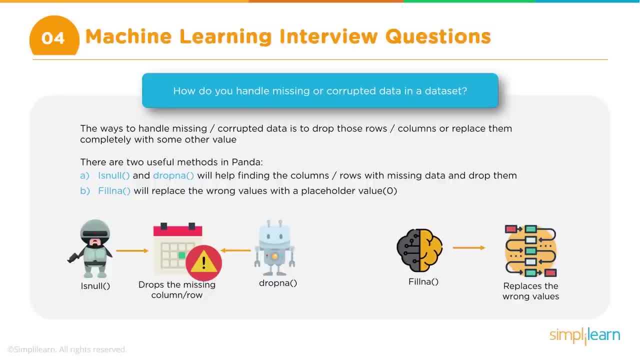 then the whole purpose is lost. okay, so then, how do you handle? then you need to come up with ways of filling up this data with some meaningful value. right, that is one way of handling. so when we say meaningful value, what is that meaningful value? let's say, for a particular column? 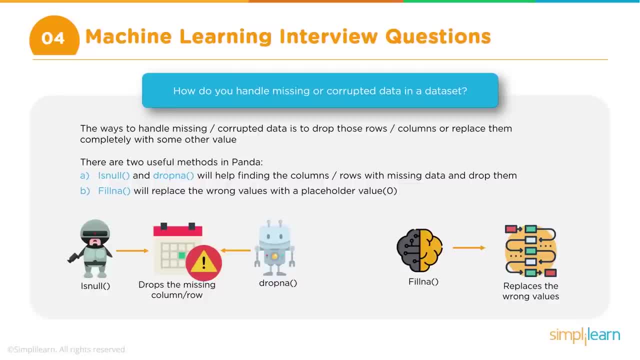 you might want to take a mean value for that column and fill wherever the data is missing. fill up with that mean value so that when you are doing the calculations your analysis is not completely way off, so you have values which are not missing, first of all. so your system. 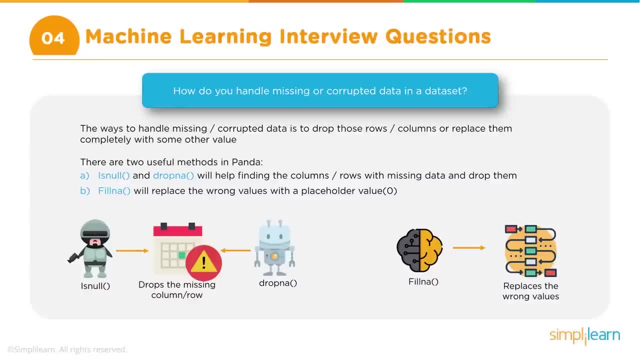 will work. number two: these values are not so completely out of whack that your whole analysis goes for a toss right. there may be situations where, if the missing values, instead of putting mean, may be a good idea to fill it up with a minimum value or with 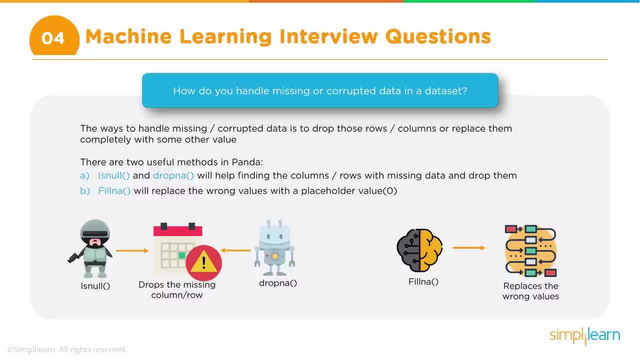 a zero, so, or with a maximum value, again, as i said, there are so many possibilities, so there is no like one correct answer for this. you need to basically talk around this and illustrate with your experience, as i said, that would be the best. otherwise, this is how you. 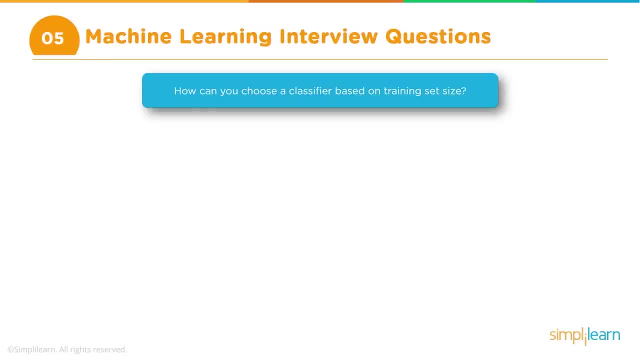 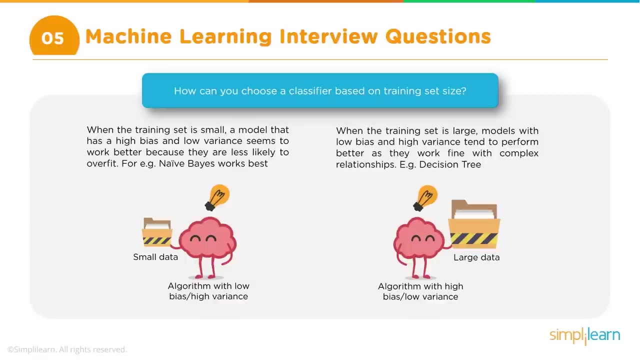 need to handle this question, okay. so then the next question can be: how can you choose a classifier based on a training set data size? so again, this is one of those questions where you probably do not have like a one size fits all answer. first of all, you 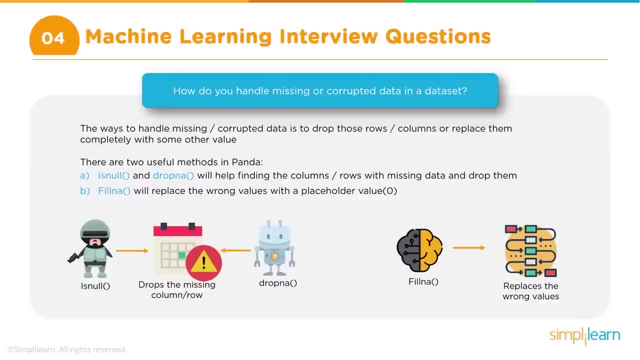 Is: Remove those records or remove those observations from your analysis. So that is the easiest way to do. But then the downside is, as I said in as in the first case, if, let's say, 50% of your data is like that because some column or the other is missing, 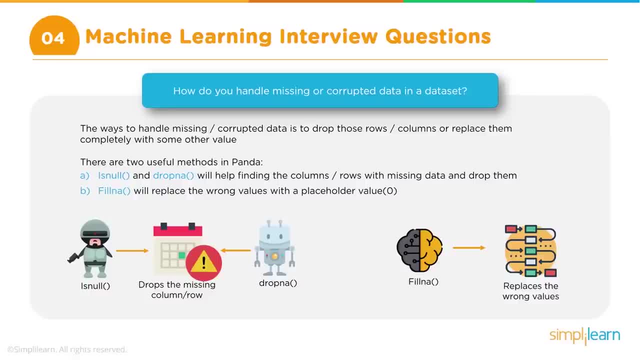 So it is not like every in every place, in every row, the same column is missing. but you have in maybe 10% of the records. Column one is missing and another 10%. column two is missing, another 10%. column three is missing, and so on and so forth. 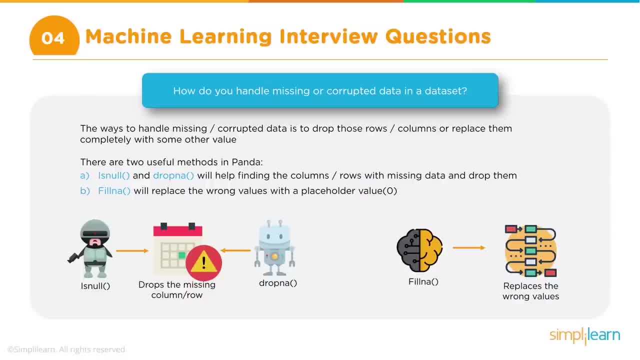 So it adds up to maybe half of your data set. So you cannot Completely remove half of your data set. then the whole purpose is lost. Okay, so then how do you handle? Then you need to come up with ways of filling up this data with some meaningful value, right? 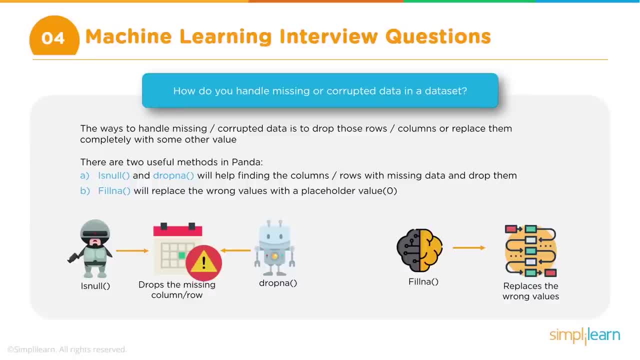 That is one way of handling. So when we say meaningful value, what is that meaningful value? Let's say, for a particular column? you might want to take a mean value for that column and fill wherever the data is missing. Fill up with that mean value so that when you're doing the calculations your analysis is not completely. 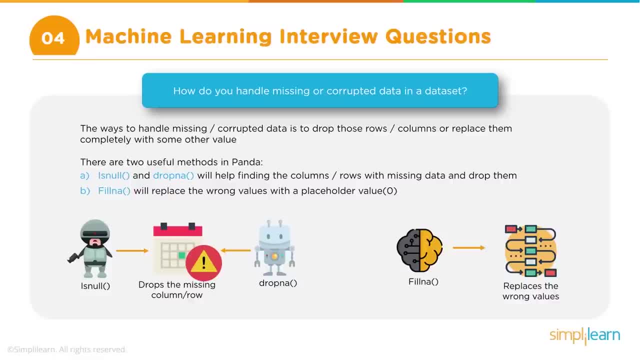 Way off. So you have values which are not missing. First of all, so your system will work. Number two: these values are not so completely out of whack that your whole analysis goes for a toss right. There may be situations where, if the missing values, instead of putting mean, maybe a good idea to fill it up with the minimum value or with a zero. 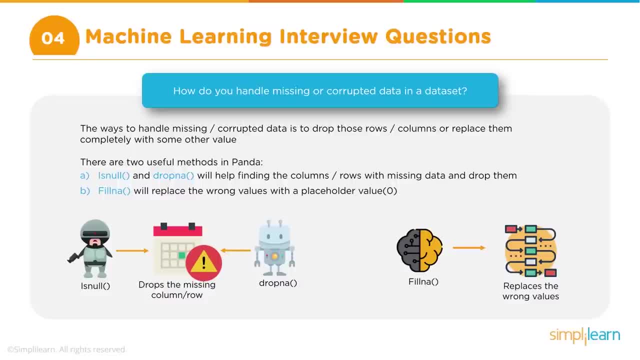 So, or with the maximum value. again, as I said, there are so many possibilities, So there is no like one correct answer for this. You need to basically talk around this and Illustrate with your experience, As I said. that would be the best. 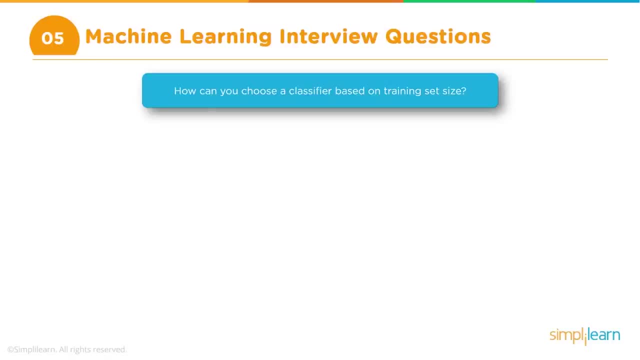 Otherwise, this is how you need to handle this question. OK, so then the next question can be: how can you choose a classifier based on a training set data size? So again, this is one of those questions where you probably do not have like a one size fits all answer. 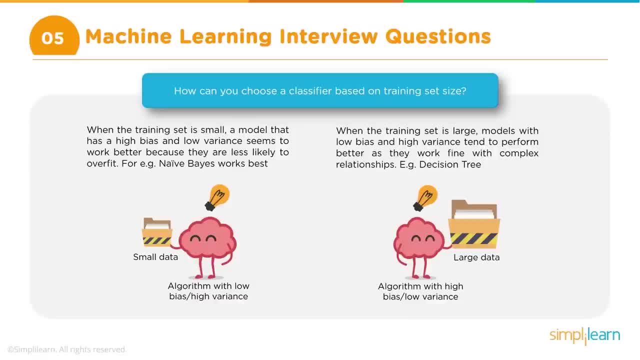 First of all, you may not, let's say, decide your classifier based on the training set size. Maybe This is not the best way to decide the type of the classifier, And even if you have to, there are probably some thumb rules which we can use. 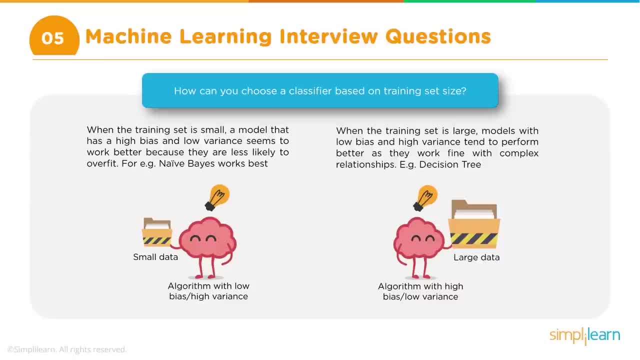 may not, let's say, decide your classifier based on the training set size. maybe not the best way to decide the type of the classifier, and even if you have to, there are probably some thumb rules which we can use, but then again every time. so, in my opinion, the best way to respond to, 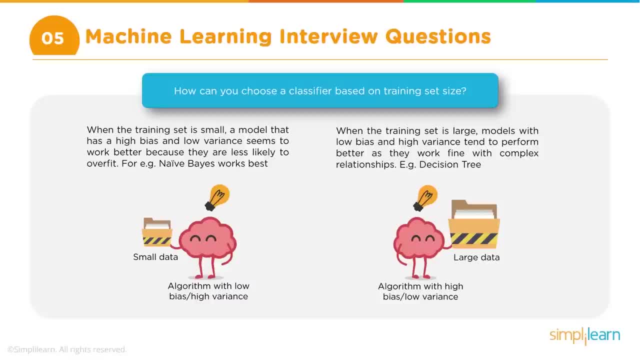 this question is: you need to try out few classifiers, irrespective of the size of the data, and you need to then decide, on your particular situation, which of these classifiers are the right ones. this is a very generic issue, so you will never be able to just by if somebody defines a. 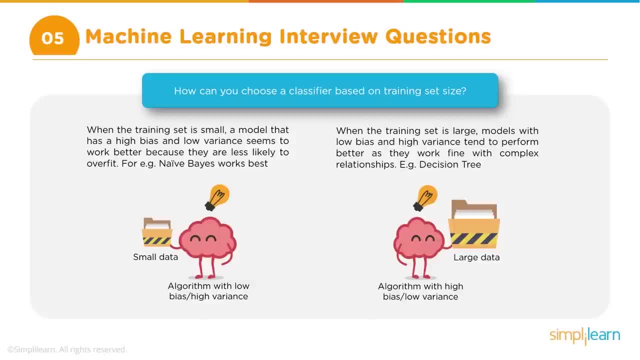 problem to you and somebody. even if they show the data to you or tell you what is the data or even the size of the data, I don't think there is a way to really say that, yes, this is the classifier that will work here. no, that's not. 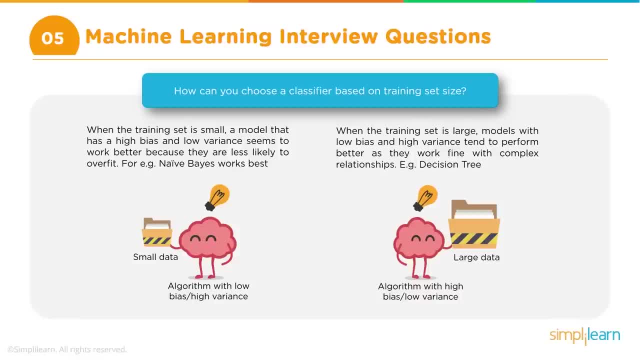 the right way. so you need to still- you know, test it out, get the data, try out a couple of classifiers, and then only you will be in a position to decide which classifier to use. you try out multiple classifiers, see which one gives the best accuracy, and only then 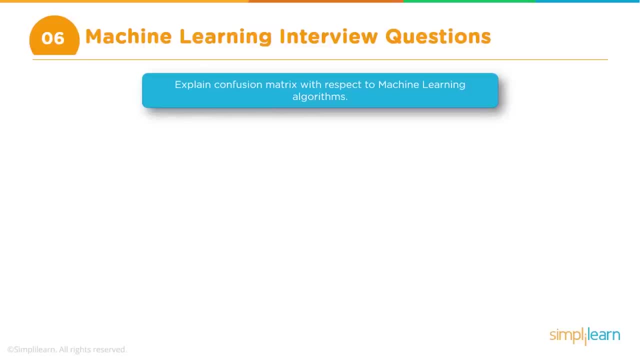 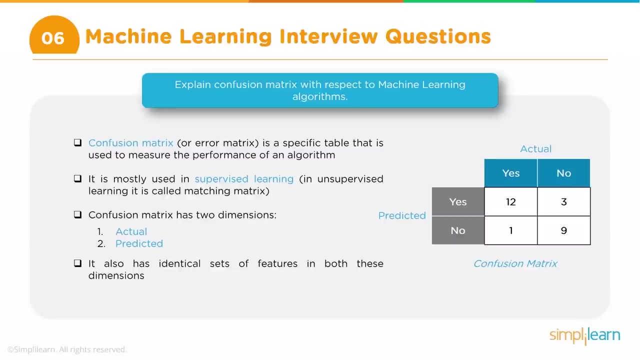 you can decide. then you can have a question around confusion matrix. so the question can be: explain confusion matrix, so confusion matrix? I think the best way to explain it is by taking an example and drawing like a small diagram. otherwise it can really become tricky. so my suggestion is to take a piece of 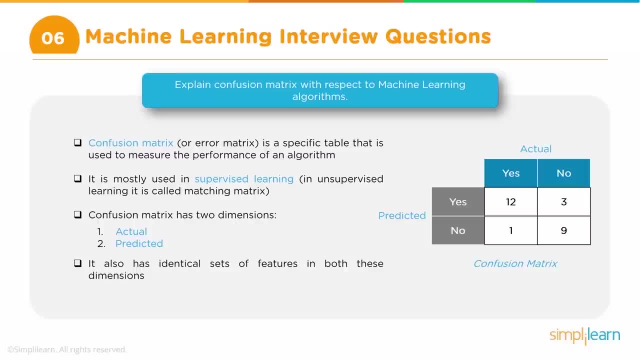 pen and paper and explain it by drawing a small matrix and confusion. matrix is about to find out. this is used specially in classification learning process and when you get the results- and our model predicts the results- you compare it with the actual value and try to find out what is the accuracy. 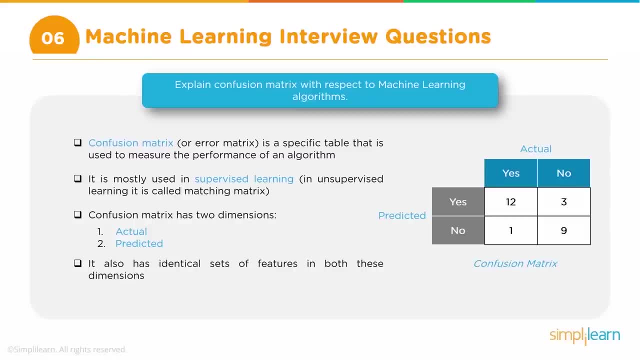 okay. so in this case, let's say this is an example of a confusion matrix and it is a binary matrix, so you have the actual values, which is the labeled data and which is so you have how many yes and how many no. so you have that information. 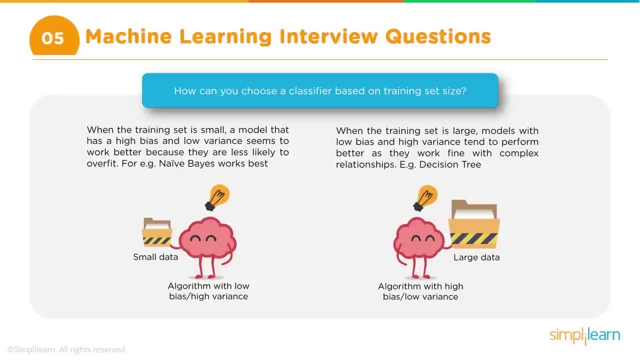 But then again every time. So, in my opinion, the best way to respond to this question is you need to try out a few classifiers, irrespective of the size of the data, And you need to then decide, on your particular situation, which of these classifiers are the right ones. 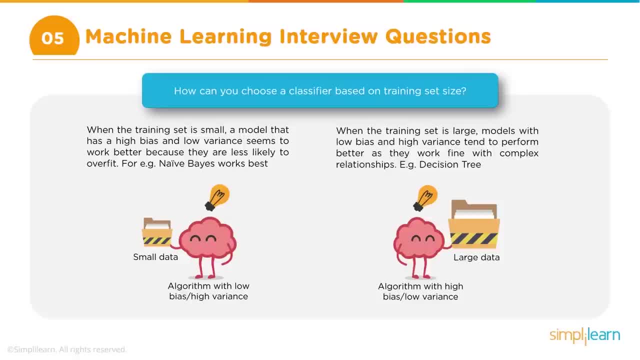 This is a very generic issue, so you will never be able to just buy. If somebody defines a problem to you and somebody, even if they show the data to you or tell you what is the data or even the size of the data, I don't think there is a way to really say that yes, this is the classifier that will work here. 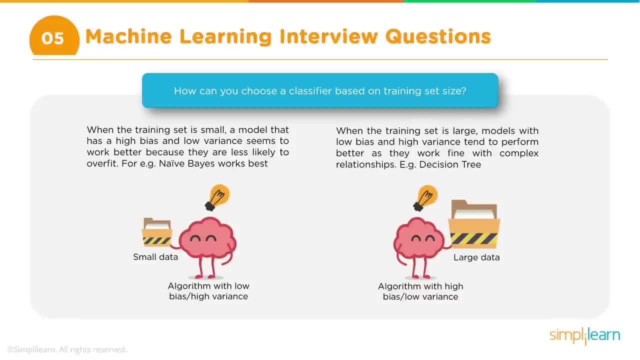 No, that's not the right way. So you need to still, you know, test it out, get the data, try out a couple of classifiers and then only you will be in a position to decide which classifier to use. You try out multiple classifiers. 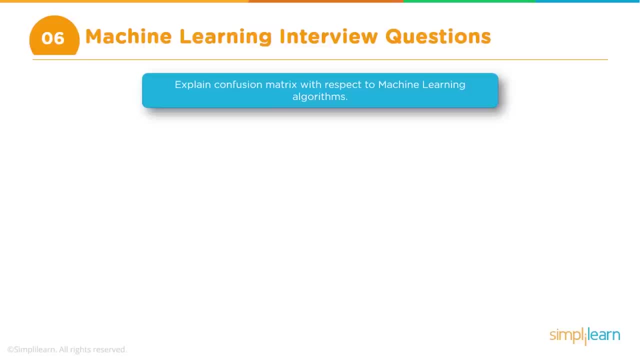 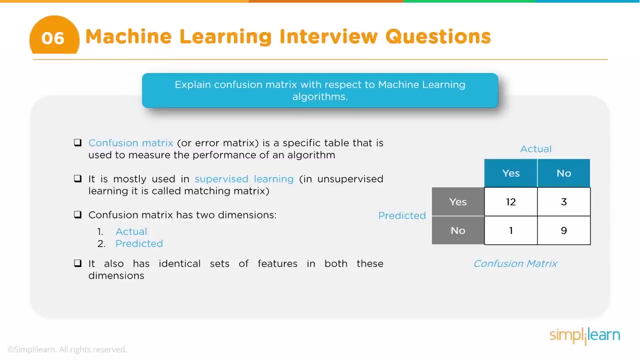 See which one gives The best accuracy and only then you can decide. Then you can have a question around confusion matrix. So the question can be explained: confusion matrix, So confusion matrix. I think the best way to explain it is by taking an example and drawing like a small diagram. 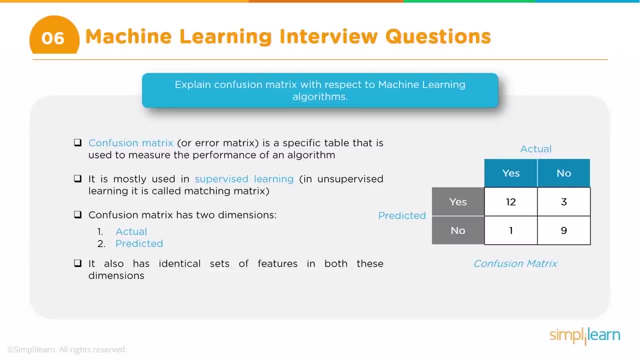 Otherwise it can really become tricky. So my suggestion is to take a piece of pen and paper and explain it by drawing a small matrix. and confusion matrix is about to find out. This is used especially in classification learning process, And when you get the results- and the model predicts the results- you compare it with the actual value and try to find out what is the accuracy. 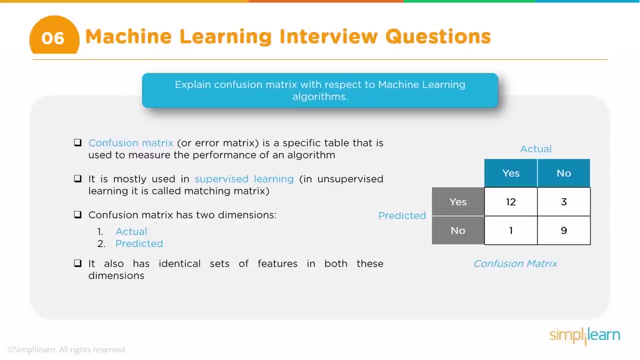 OK, so in this case, let's say this is an example of a confusion matrix and it is a binary matrix, So you have the actual values, which is the labeled data and which is so you have how many Yes And how many. 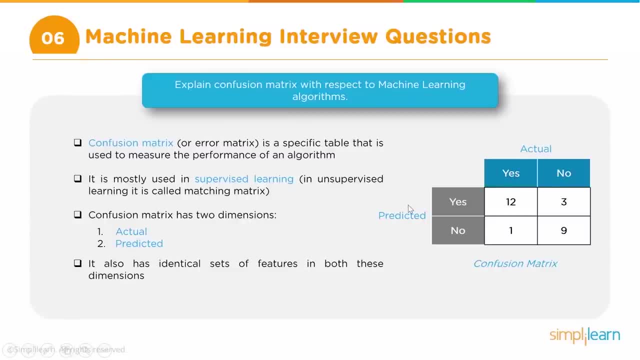 No. So you have that information and you have the predicted values: How many Yes And how many No, Right? So the total actual values, the total yes is 12 plus 113.. And they are shown here. And the actual value no's are 9 plus 3, 12.. 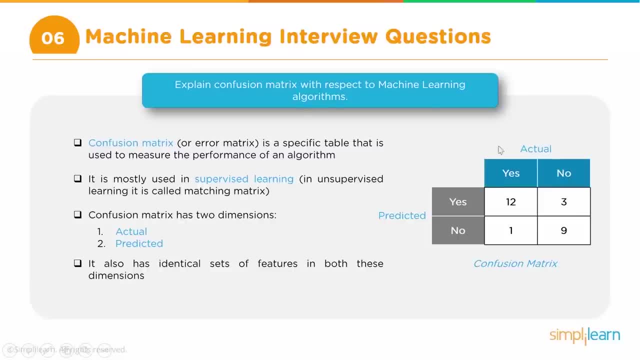 OK, so that is what this information here is. So this is about the actual and this is about the predicted. Similarly, the predicted values there are: yes are 12 plus 3, 15 yeses, and no are 1 plus 9, 10 no's. 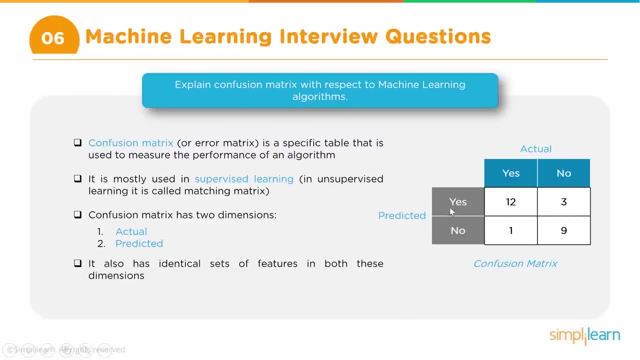 and you have the predictive values: how many yes and how many no, right? so the total actual values: the total yes is 12 plus 113, and they are shown here, and the actual value no's are 9 plus 3, 12. okay, so that is what this information. 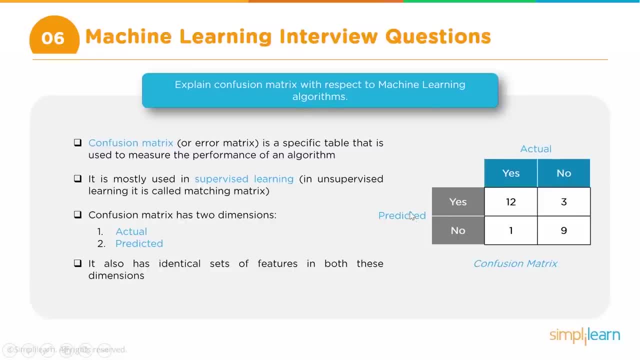 here is. so this is about the actual and this is about the predicted. similarly, the predicted values there are: yes are 12 plus 3 15 yes's and no are 1 plus 9, 10 no's. okay, so this is the way to look at. 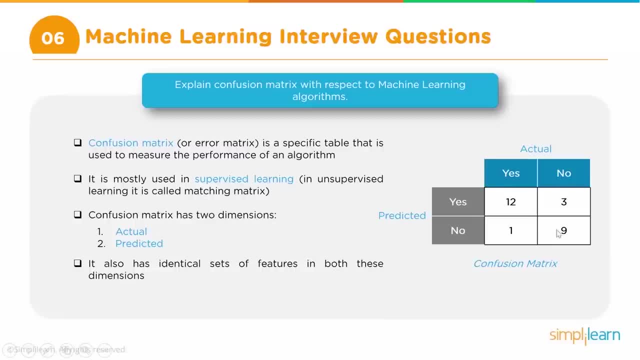 this confusion matrix. okay, and out of this, what is the meaning conveyed? so there are two or three things that needs to be explained outright. the first thing is: for a model to be accurate, the values across the diagonal should be high, like in this case. right, that is one number two. 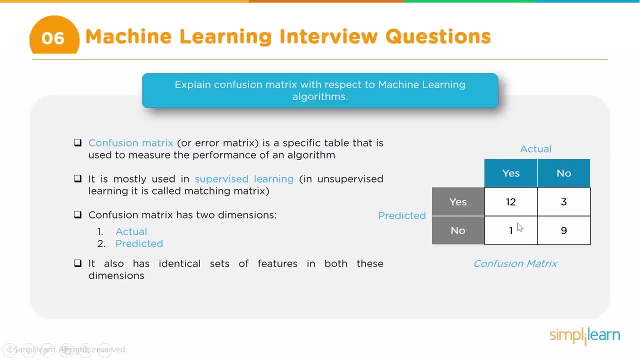 the total sum of these values is equal to the total observations in the test data set. so in this case, for example, you have 12 plus 3, 15 plus 10, 25. so that means we have 25 observations in our test data set. okay, so these are the 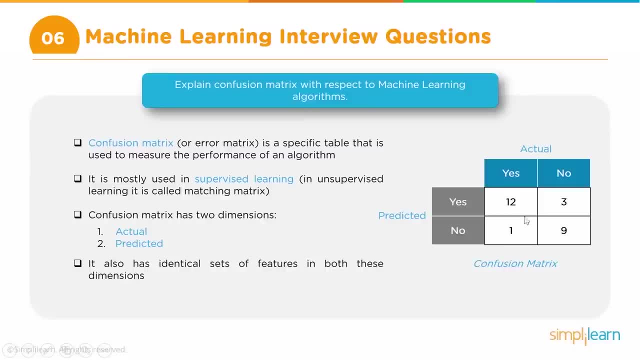 two things. you need to first explain that total sum in this matrix the numbers is equal to the size of the test data set and the diagonal values indicate the accuracy. so by just by looking at it, you can probably have a idea about: is this an accurate model? is the model? 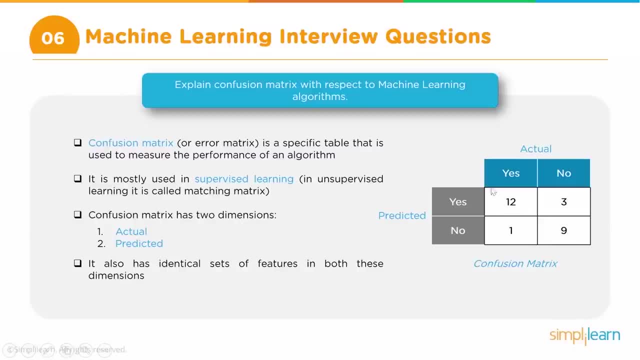 being accurate if they are all spread out equally in all these four boxes. that means probably the accuracy is not very good. okay, now, how do you calculate the accuracy itself, right? how do you calculate the accuracy itself? so it is a very simple mathematical calculation. you take some of the diagonals, right? so 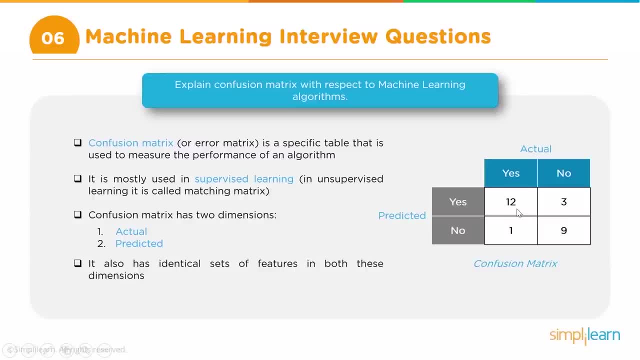 in this case, it is 9 plus 12, 21 and divide it by the total. so in this case, what will it be? let's me take a pen. so your, your diagonal values, is equal to. if i say d is equal to 12 plus 9, so that is. 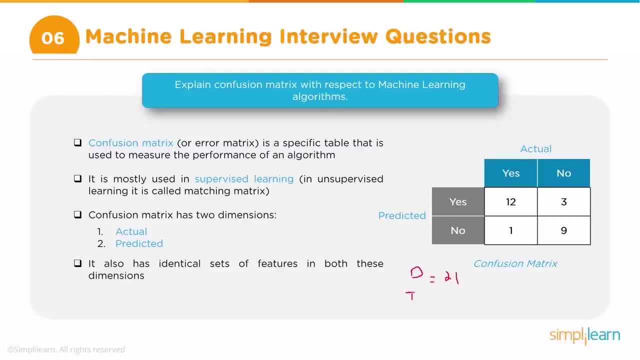 21, right, and the total data set is equal to right. we just calculated it is 25. so what is your accuracy? it is 21 by. your accuracy is equal to 21 by 25, and this turns out to be about 85 percent, right? so this is 85 percent. 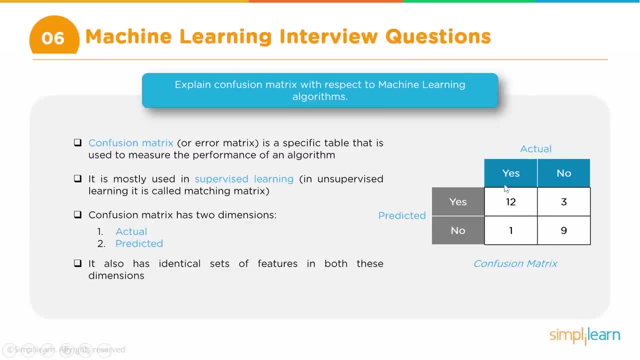 OK, So this is the way to look at this confusion matrix. OK, and out of this, what is the meaning conveyed? So there are two or three things that needs to be explained outright. The first thing is for a model to be accurate, the values across the diagonal should be high, like in this case. right, 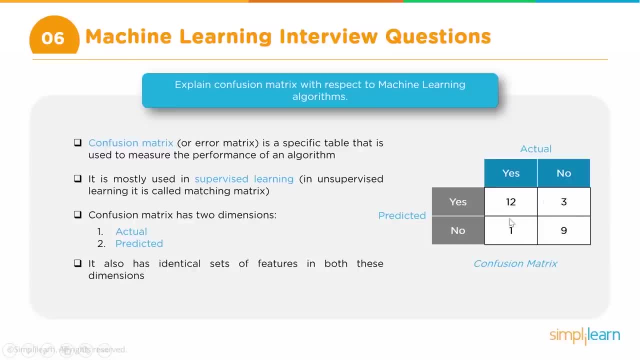 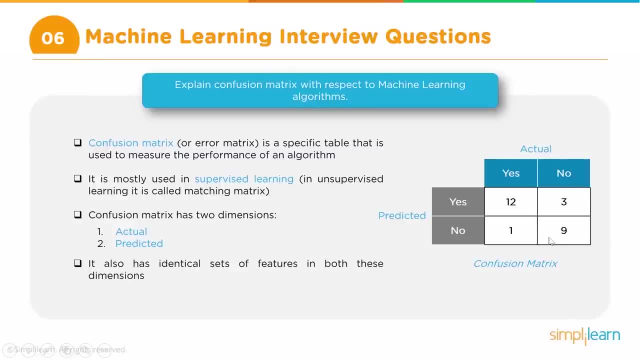 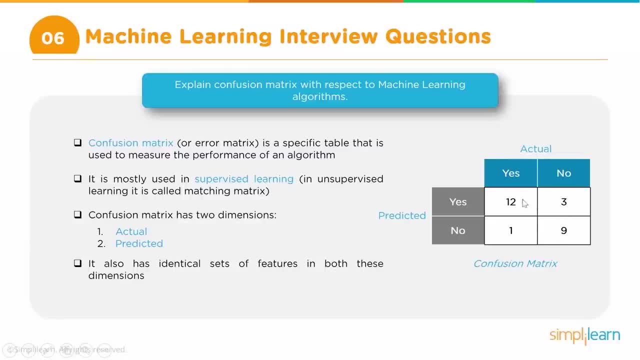 OK, so these are the two things. you need to first explain that the total sum in this matrix, the numbers, is equal to the size of the test data set and the diagonal values indicate the accuracy. So by just by looking at it, you can probably have an idea about: is this an accurate model? 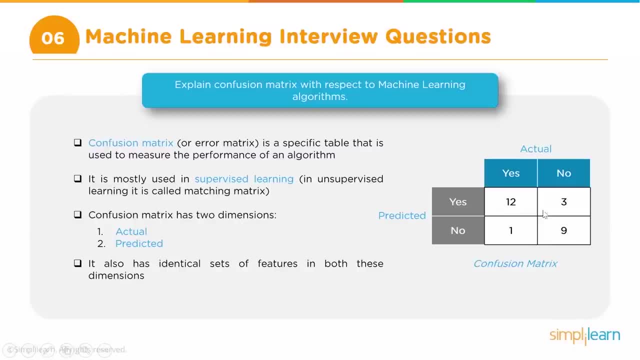 Is the model being accurate If they're all spread out equally in all these four boxes? that means probably the Accuracy is not very good. OK, now how do you calculate the accuracy itself? How do you calculate that? So it is a very simple mathematical calculation. 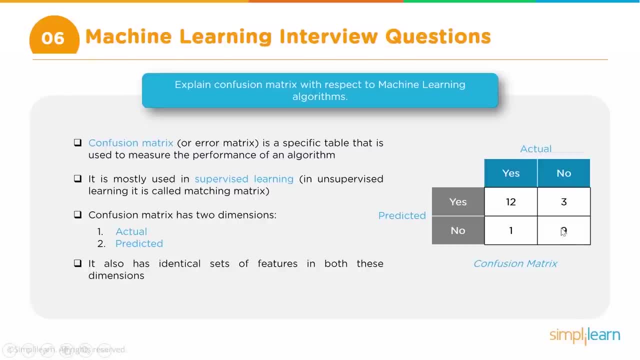 You take some of the diagonals. in this case it is nine plus 21 and divided by the total. So in this case, what will it be? Let's me take a pen. So your, your diagonal values is equal. if I say D is equal to 12 plus nine. 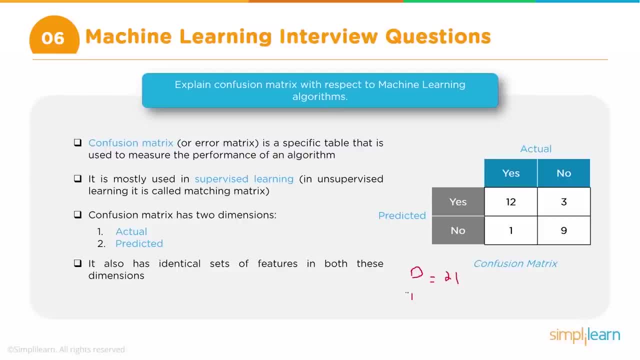 So that is 21.. Right, and the total data set is equal to right. we just calculated it is 25. so what is your accuracy? it is 21 by. your accuracy is equal to 21 by 25, and this turns out to be about 85 percent, right? so this is. 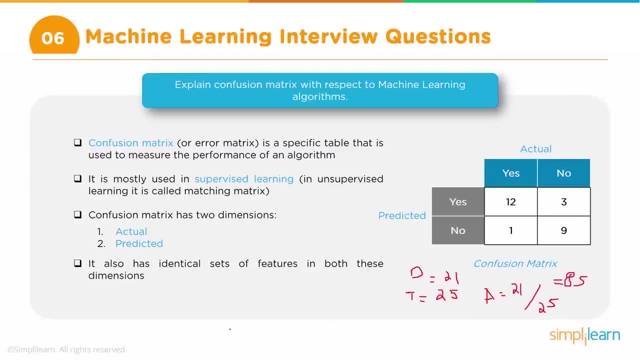 85 percent. so that is our accuracy. okay, so this is the way you need to explain draw diagram, give an example. maybe it may be a good idea to be prepared with an example so that it becomes easy for you. you don't have to calculate these numbers on the fly, right? so a couple of hints. 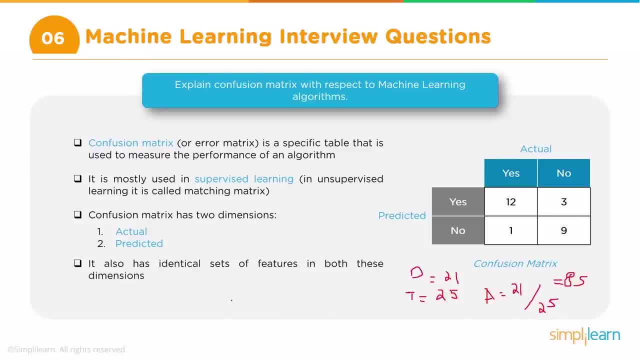 so that is our accuracy. okay, so this is the way you need to explain draw diagram. give an example. maybe it may be a good idea to be prepared with an example so that it becomes easy for you. you don't have to calculate these numbers on the fly, right? so 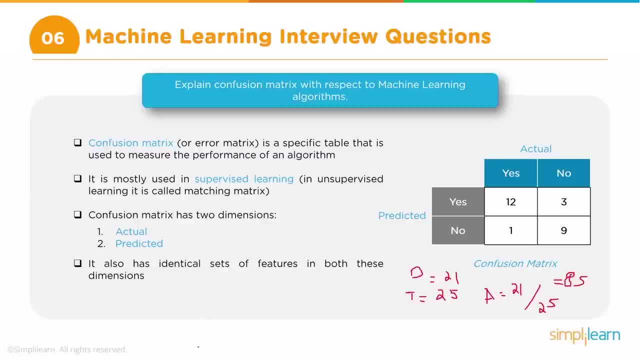 couple of hints are that you take some numbers which are with, which add up to 100. that is always a good idea, so you don't have to really do this complex calculations. so the total value will be 100 and then diagonal values. you divide. once you find the diagonal values, that is equal to your. 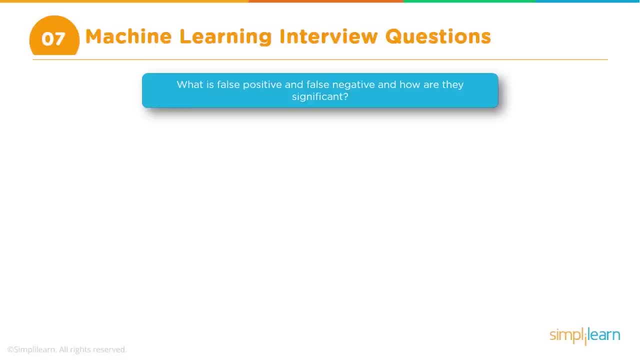 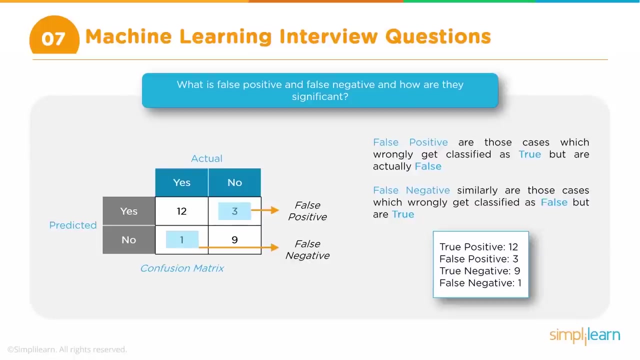 percentage. okay, all right, so the next question can be a related question about false positive and false negative. so what is false positive and what is false negative? now, once again, the best way to explain this is using a piece of paper and pen. otherwise it will be pretty difficult to explain this. 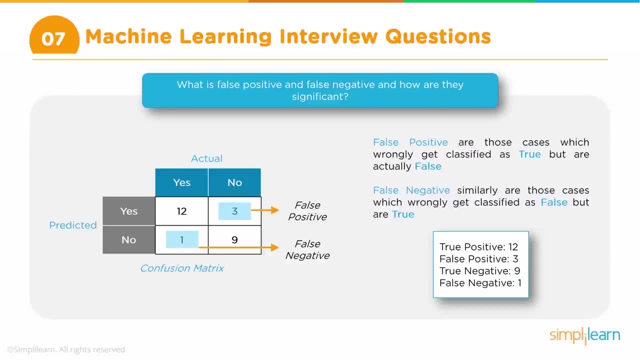 so we use the same example of the confusion matrix and we can explain that. so a confusion matrix looks somewhat like this and when we just take it, looks somewhat like this, and we continue with the previous example, where this is the actual value, this is the predicted value. 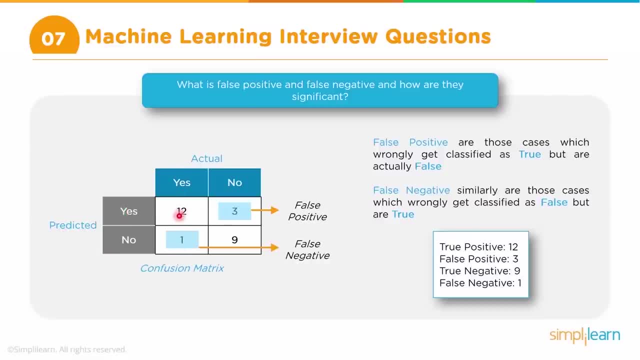 and in the actual value we have 12 plus 1 13 yeses and 3 plus 9 12 nos, and the predicted values there are 12 plus 3 15 yeses and 1 plus 9 10 nos. okay, now this. 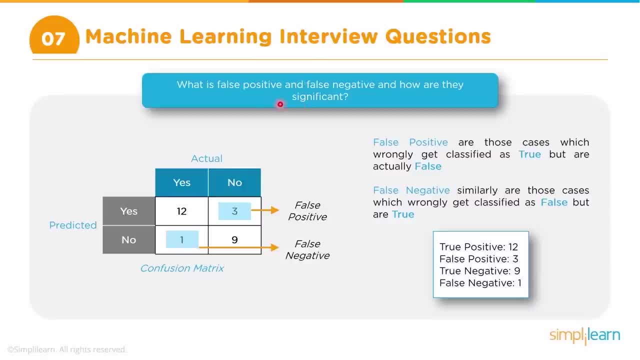 particular case, which is the false positive. what is a false positive? first of all, the second word which is positive, okay, is referring to the predicted value. so that means the system has predicted it as a positive, but the real value. so this is what the false comes from, but the real value. 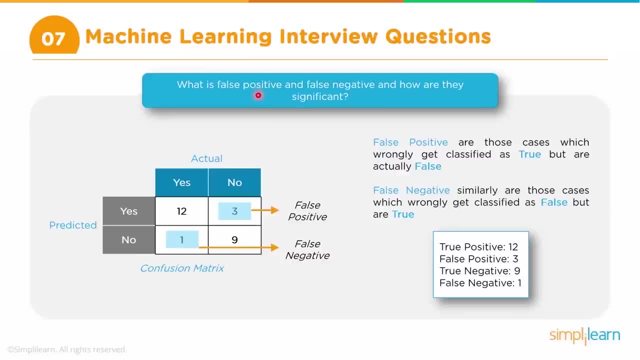 is not positive. okay, that is the way you should understand this term: false positive or even false negative. so false positive. so positive is what your system has predicted. so where is that system predicted? this is the one positive is what? yes, so you basically consider this row, okay. 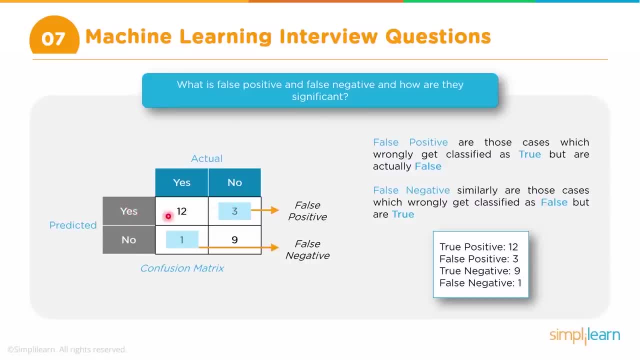 now, if you consider this row, so this is: this is all positive values. this entire row is positive values. okay, now, the false positive is the one which where the value- actual value- is negative, predicted value is positive, but the actual value is negative. so this is a false. 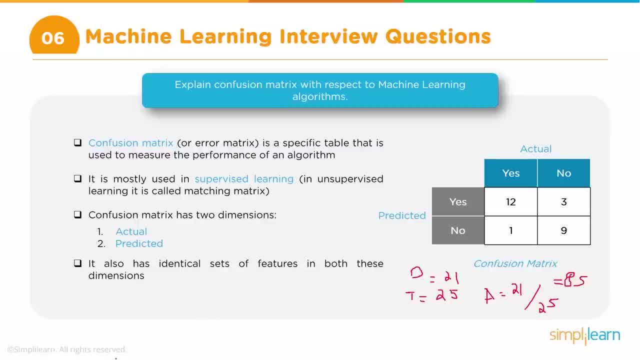 are that you take some numbers which are with, which add up to 100. that is always a good idea, so you don't have to really do this complex calculations. so the total value will be 100 and then diagonal values. you divide. once you find the diagonal values, that is equal to your. 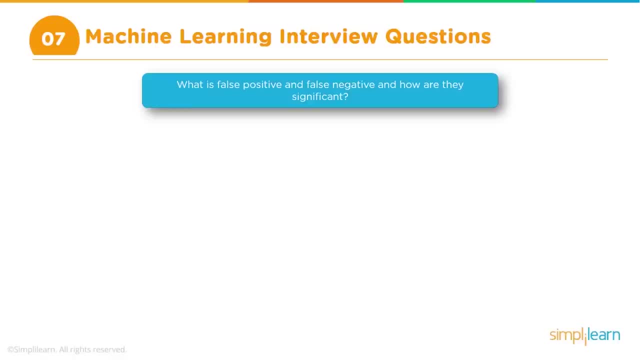 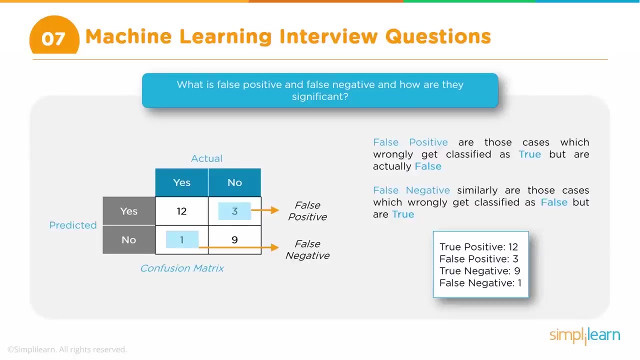 percentage. okay, all right. so the next question can be a related question about false positive and false negative. so what is false positive and what is false negative now? what is false positive and what is false negative now? once again, the best way to explain this is using a piece of paper and pen, otherwise it will be pretty difficult to explain this, so we use the. 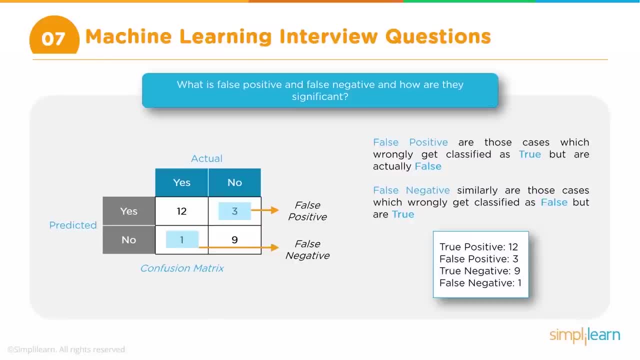 same example of the confusion matrix and we can explain that. so a confusion matrix looks somewhat like this, and when we just take, yeah, it looks somewhat like this, and we continue with the previous example where this is the actual value, this is the predicted value and, uh, it's going to. 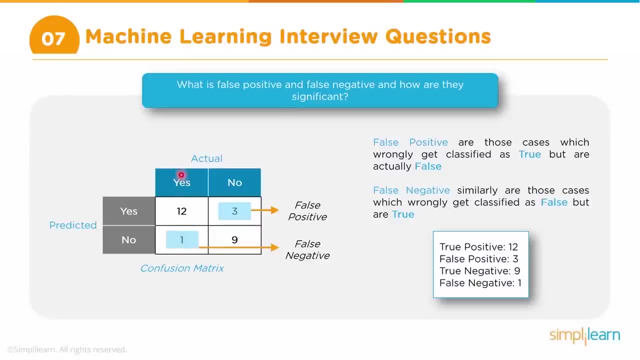 look like this, and we continue with the previous example, where this is the actual value. this is the. in the actual value, we have 12 plus 1: 13 yeses and 3 plus 9- 12 no's, and the predicted values there are 12 plus 3: 15 yeses and 1 plus 9- 10 no's. okay, now, in this particular case, which is the, 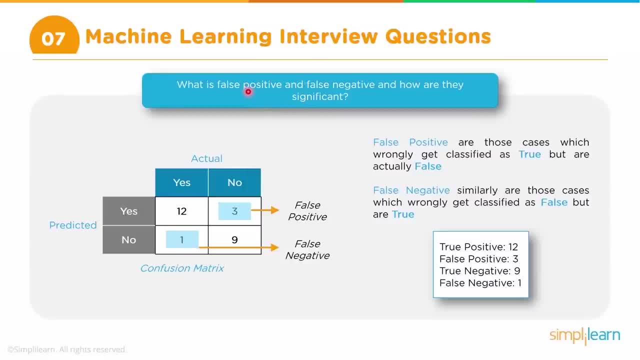 false positive. what is a false positive? first of all, the second word which is positive, okay, is referring to the predicted value. so that means the system has predicted it as a positive, but the real value. so this is what the false comes from, but the real value is not positive. 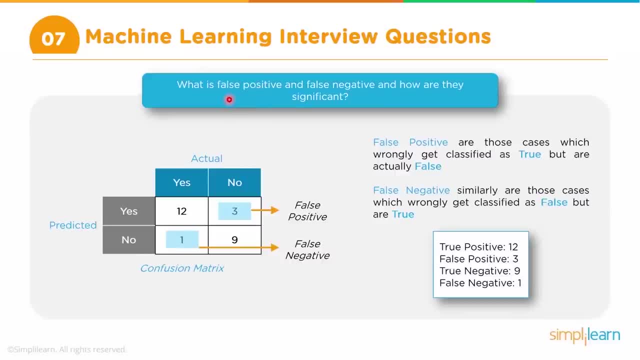 okay, that is the way you should understand this term: false positive or even false negative. so false positive, so positive is what your system has predicted. so where is that system predicted? this is the one positive is what? yes, so you basically consider this row. okay, now, if you. 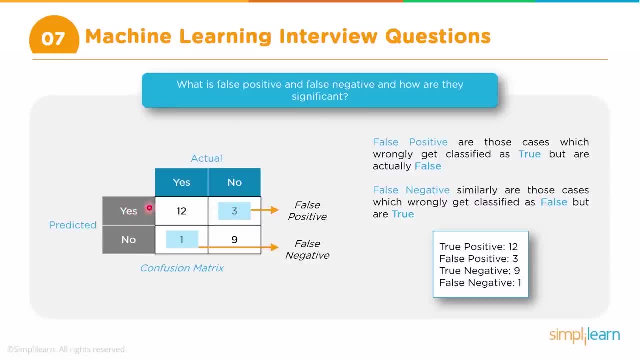 consider this row. so this is, this is all positive values. this entire row is positive values. okay, now you can see that the false positive is the one which where the value- actual value- is negative. predicted value is positive, but the actual value is negative. so this is a false positive, right, and? 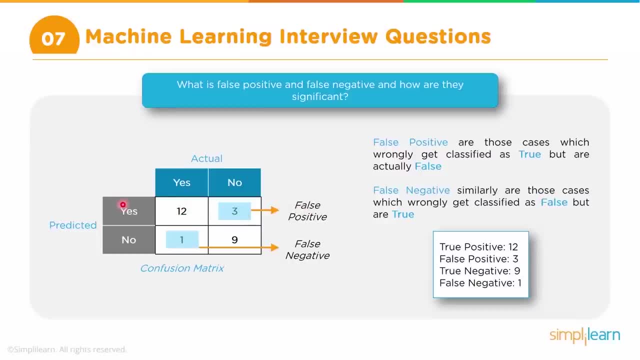 positive, right, and here is a true positive. so the predicted value is positive and the actual value is also positive, and we hope this is making sense. now let's take a look at what is false negative. false negative- so negative is the second term. that means that is the. 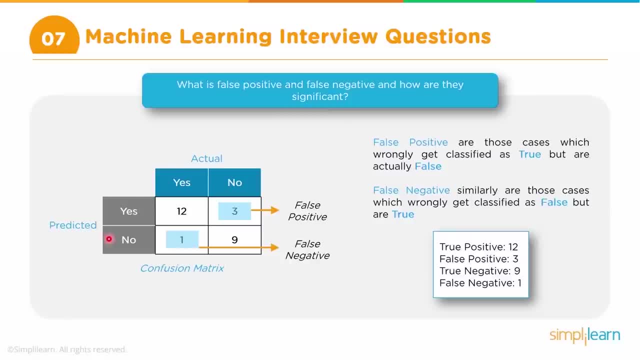 predicted value that we need to look for. so which are the predicted negative values? this row corresponds to predicted negative values, all right, so this row corresponds to predicted negative values and what they are asking for- false. so this is the row for predicted negative values and the actual. 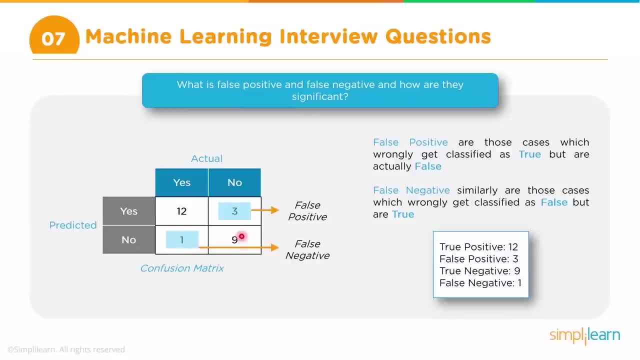 value. is this one, right? this is predicted negative and the actual value is also negative. therefore, this is a true negative. so the false negative is this one: predicted is negative, but actual is positive, right? so this is the false negative. so this is the way to explain and this is the way to. 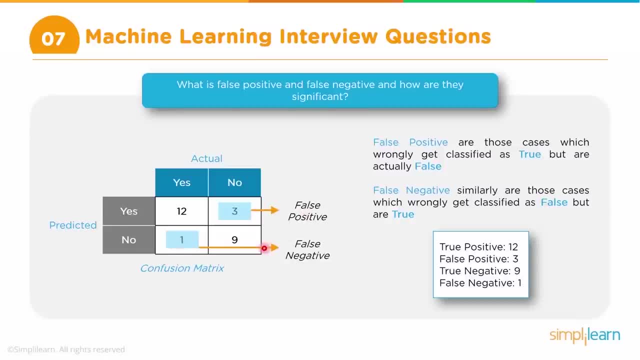 look at false positive and false negative. same way there can be true positive and true negative as well. so again, positive. the second term you will need to use to identify the predicted row right. so if we say true, positive, positive, we need to take for the predicted part. so predicted positive is here, okay, and then the first term is for the actual. 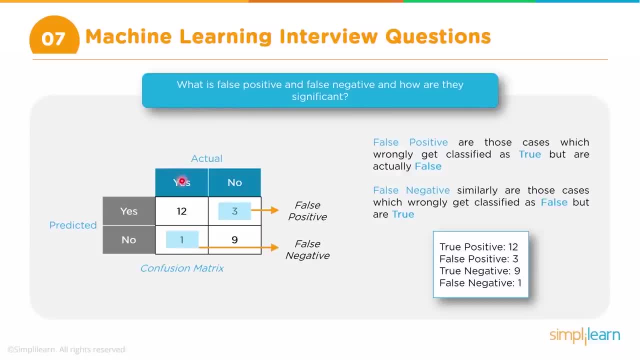 so true, positive. so true, in case of actual is yes, right. so true, positive is this one, okay. and then, in case of actual, the negative. now we are talking about, let's say true, negative, true, negative, negative is this one and the true comes from here. so this is true, negative, right, nine is true. 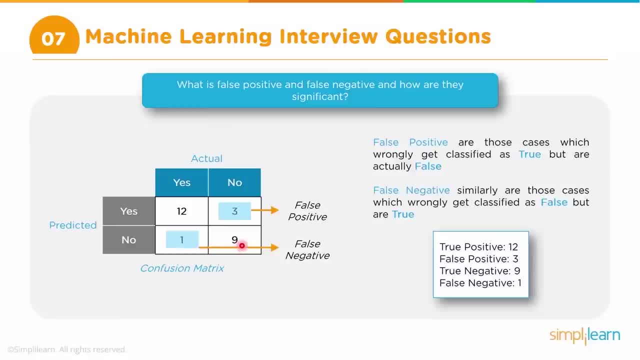 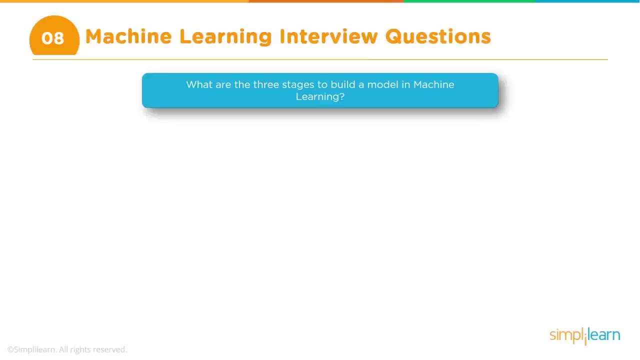 negative. the actual value is also negative and the predicted value is also negative. okay, so that is the way you need to explain this: the terms false positive, false negative and true positive, true, negative. then you might have a question like: what are the steps involved in the machine learning? 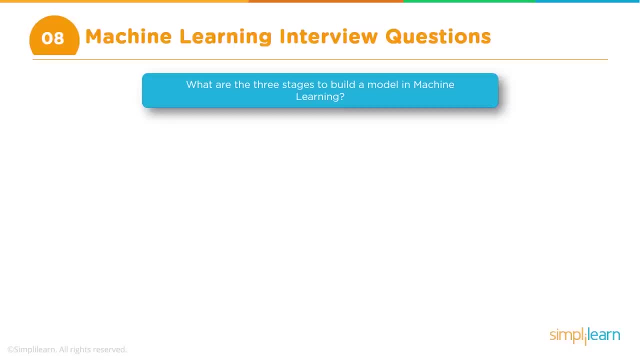 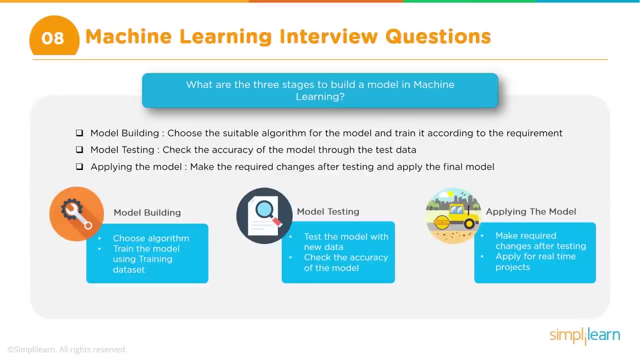 process, or what are the three steps in the process of developing a machine learning model? right, so it is around the methodology that is applied. so basically, the way you can probably answer in your own words, but the way the model development of the machine learning model happens is like this. 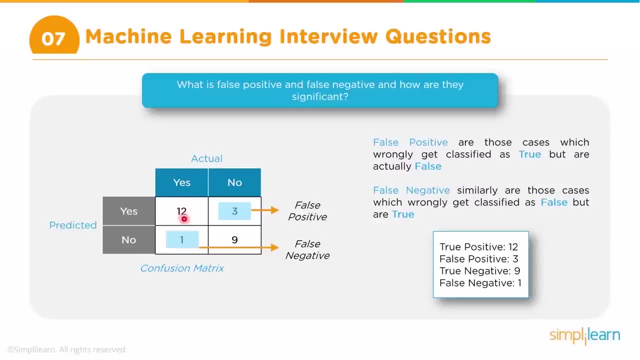 here is a true positive, so the predicted value is positive and the actual value is also possible, and we hope this is making sense. now let's take a look at what is false negative. false negative, so negative is the second term. that means that is the predicted value that we need to look for. so 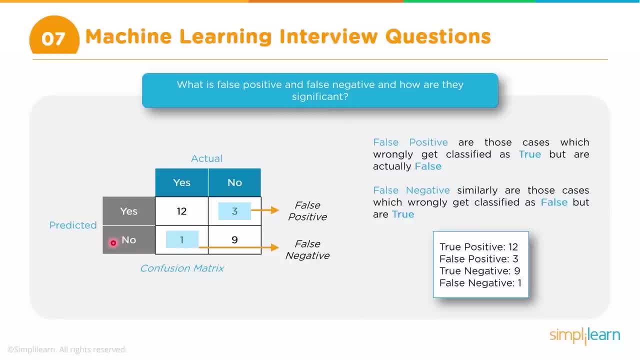 which are the predicted negative values row corresponds to predicted negative values. All right. So this row corresponds to predicted negative values And what they are asking for False. So this is the row for predicted negative values And the actual value is this one? Right? This is predicted negative and the actual value. 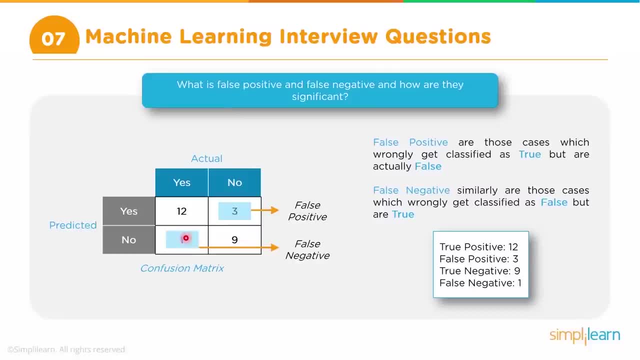 is also negative. Therefore, this is a true negative. So the false negative is this: one: Predicted is negative, but actual is positive, Right? So this is the false negative. So this is the way to explain And this is a way to look at false positive and false negative Same way. 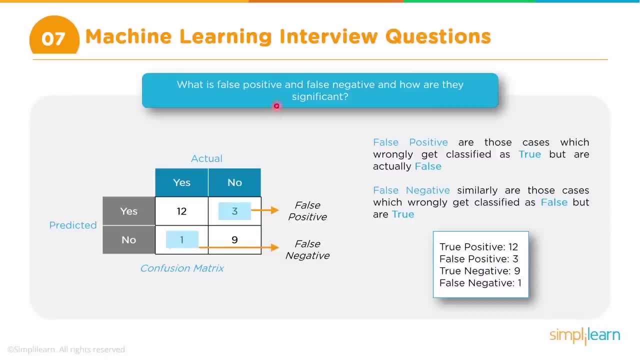 there can be true positive and true negative as well. So, again, positive, the second term you will need to use to identify the predicted row, Right? So if we say true, positive, positive we need to take for the predicted part. So predicted positive is here, OK, And then the. 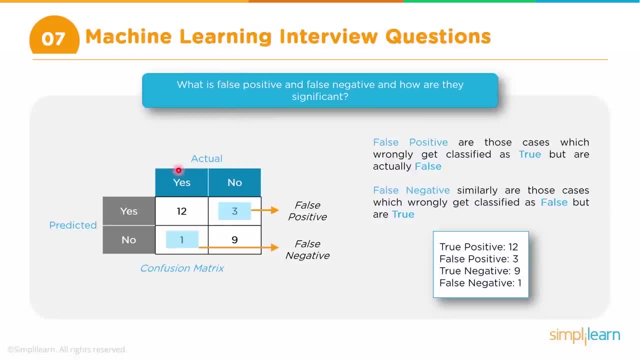 first Term is for the actual, So true, positive. So true, in case of actual is yes, Right. So true, positive is this one, OK. And then, in case of actual, the negative. Now we are talking about, let's say true, negative, true, negative, Negative is this one And the true comes from here. So this: 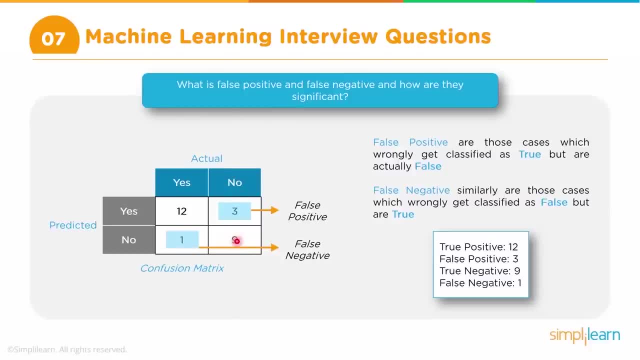 is true, negative, Right Nine is true, negative, The actual value is also negative and the predicted value is also negative. OK, So that is the way you need to explain this: The terms false positive, false negative and true positive, true negative. Then you might have a question like: what are the? 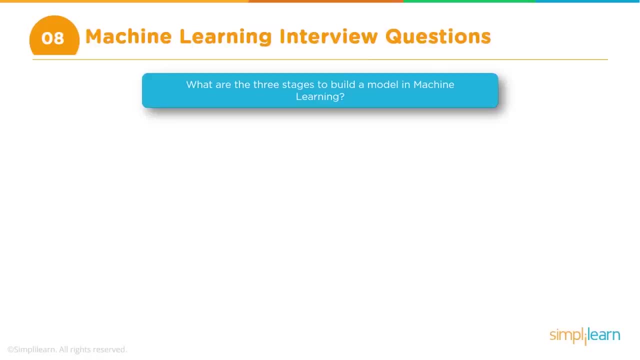 steps involved in the machine learning process, or what are the three steps in the process of developing a machine learning model? Right, So it is around the methodology that is applied. So basically, the way you can probably answer in your own words, but the way the model development, 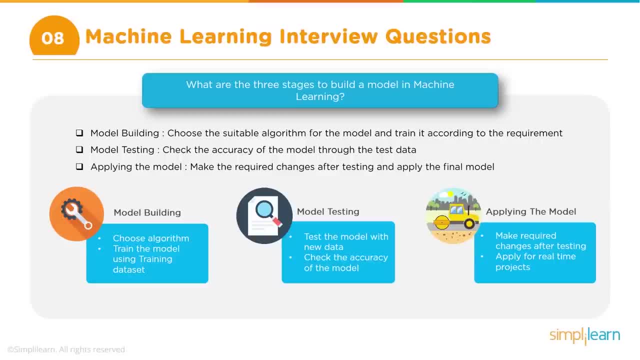 of the machine learning model happens is like this. So first of all you try to understand the problem and try to figure out whether it is a classification problem or a regression problem. Based on that, you select a few algorithms and then you start the process of training these models. OK, So you can. 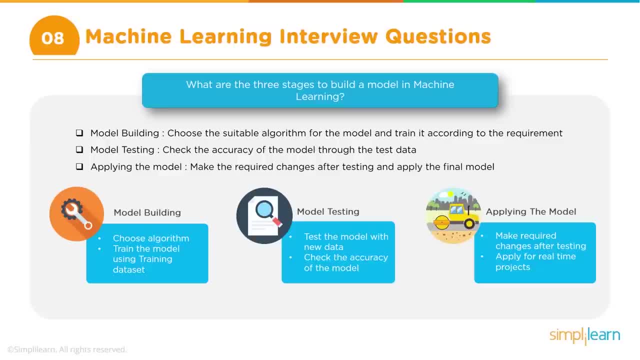 either do that or you can. after due diligence, you can probably decide that there is one particular algorithm which is most suitable. Usually it happens through trial and error process, but at some point you will decide that, OK, this is the model we are going to use. OK, So in that case, 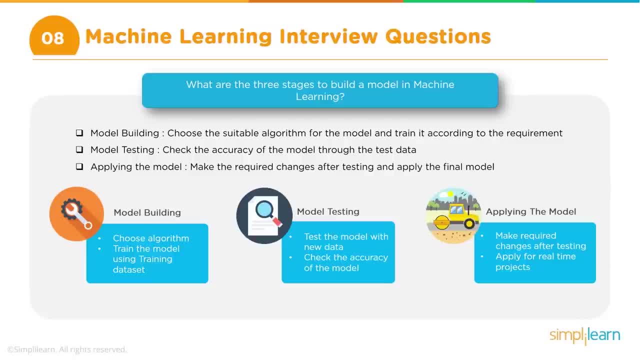 we have the model algorithm and the model decided And then you need to do the process of training the model and testing the model, And this is where, if it is supervised learning, you split your data, the label data, into training data set and test data set, And you use the training data set to 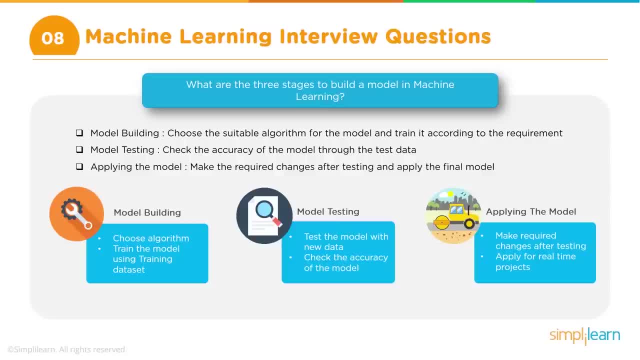 train your model and then you use the test data set to check the accuracy, whether it is working fine or not. So you test the model before you actually put it into production. Right, So once you test the model, you're satisfied it's working fine, Then you go to the next level. 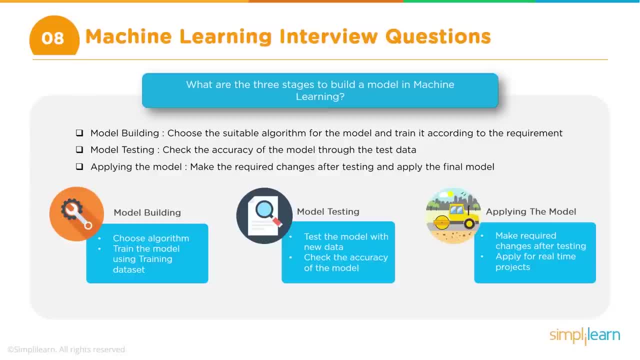 which is putting it for production. And then in production, obviously new data will come and the inference happens. So the model is readily available And only thing that happens is new data comes and the model predicts the values, whether it is regression or classification. Now, so this: 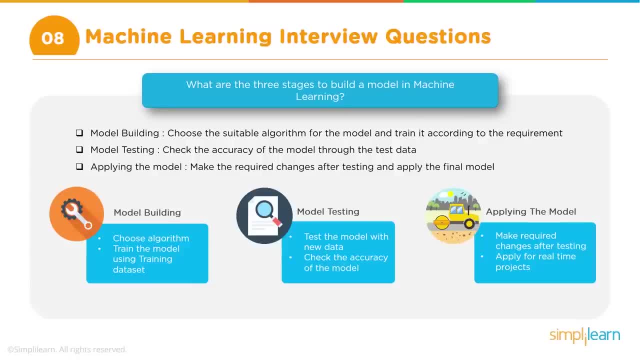 can be an iterative process, So it is not a straightforward process where you do the training for the testing and then you move it to production Now. so during the training and test process, there is a situation where, because of either overfitting or things like that, the test doesn't go. 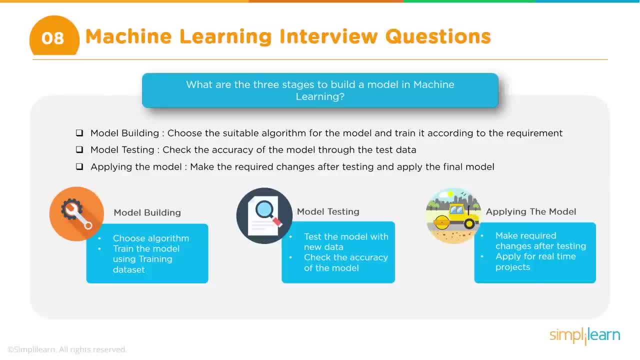 through, which means that you need to put that back into the training process, So that can be an iterative process. Not only that: even if the training and test goes through properly and you deploy the model in production, there can be a situation that the data that actually comes the 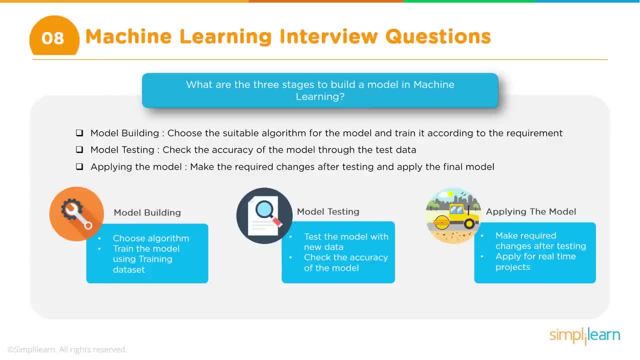 real data. that comes with that. this model is failing, So in which case you may have to once again go back to the drawing board, or initially it will be working fine, But over a period of time, maybe due to the change in the nature of the data, 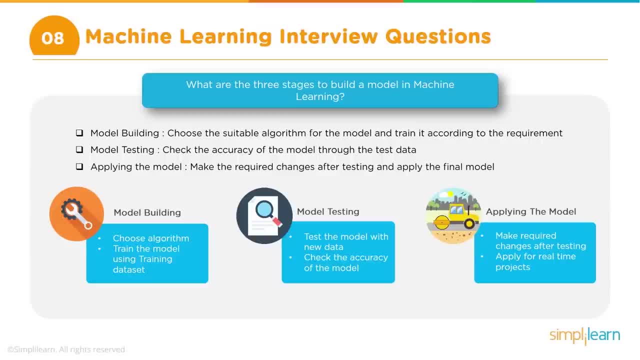 so first of all, you try to understand the problem and try to figure out whether it is a classification problem or a regression problem. based on that, you select a few algorithms and then you start the process of training these models. okay, so you can either do that or you can, after due diligence, you 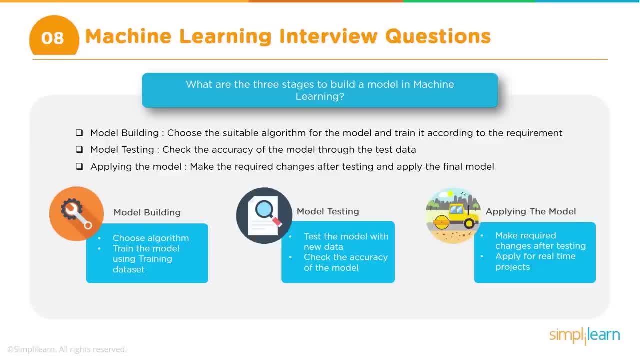 can probably decide that there is one particular algorithm which is most suitable. usually it happens through trial and error process, but at some point you will decide that, okay, this is the model we are going to use. okay, so in that case we have the model algorithm and the model decided, and then 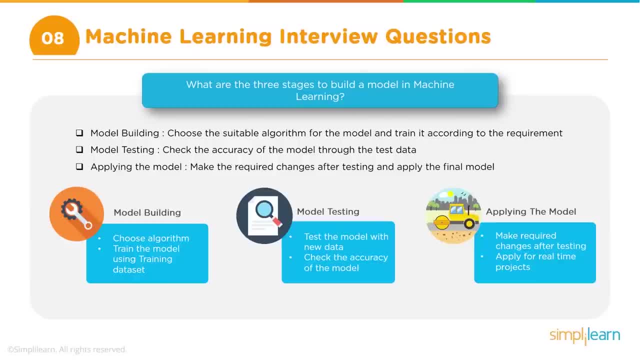 you need to do the process of training the model and testing the model, and this is where you need to go to the next level, which is where you need to focus on a testing model, where you actually have to start training both model and test model right and you need to change the model. 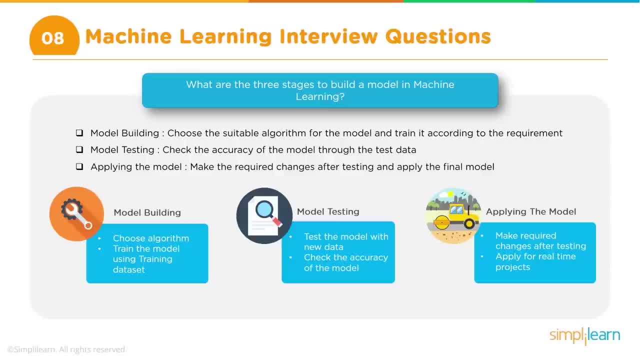 so let me show you here a simple example. what is this model we are going to use here, if it is supervised learning? you split your data, the label data, into training data set and test data set, and you use the training data set to train your model and then you use the test data set to check the 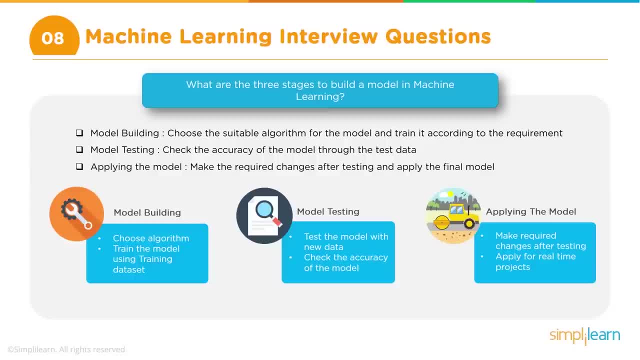 accuracy whether it is working fine or not. so you test the model before you actually put it into and the inference happens. so the model is readily available and only thing that happens is new data comes and the model predicts the values, whether it is regression or classification now. so this: 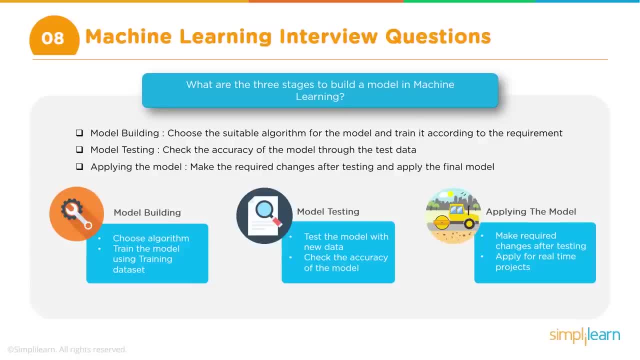 can be an iterative process, so it is not a straightforward process where you do the training for the testing and then you move it to production now. so during the training and test process, there may be a situation where, because of either overfitting or things like that, the test doesn't. 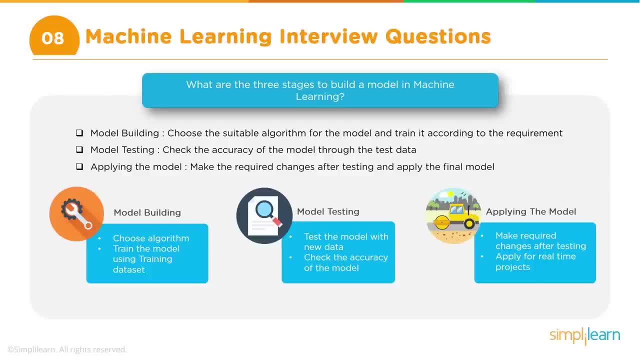 go through, which means that you need to put that back into the training process so that can be an iterative process. not only that: even if the training and test goes through properly and you deploy the model in production, there can be a situation that the data that actually comes the 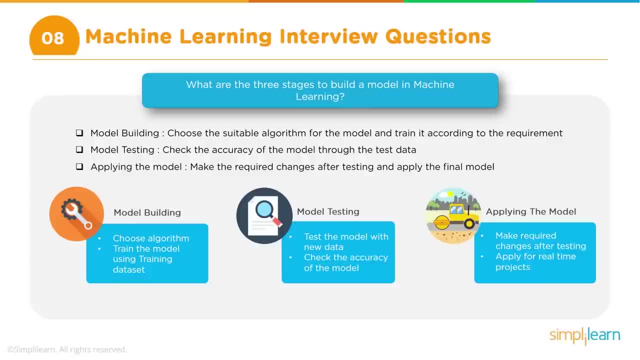 real data. that comes with that. this model is failing, so, in which case you may have to once again go back to the drawing board, or initially it will be working fine, but over a period of time, maybe due to the change in the nature of the data, once again the accuracy will deteriorate. 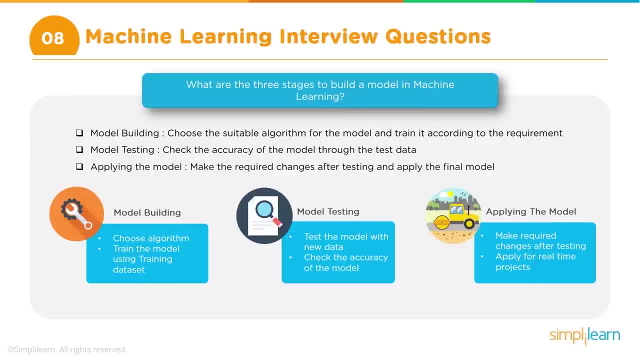 once again, the accuracy will deteriorate. So that is again a recursive process. So once in a while you need to keep checking whether the model is working fine or not And, if required, you need to tweak it and modify it, and so on and so forth. So this is a continuous 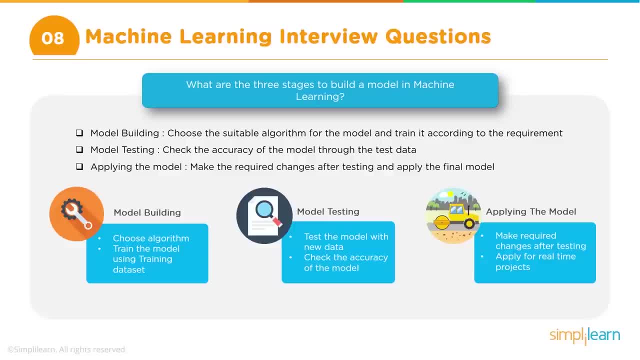 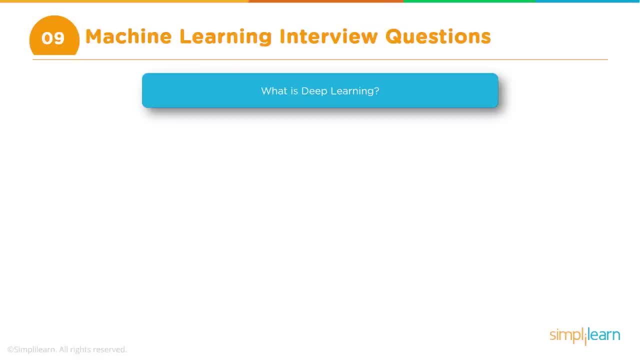 process of tweaking the model and testing it and making sure it is up to date. Then you might have a question around deep learning. So, because deep learning is now associated with AI and artificial intelligence and so on, so can be as simple as what is deep learning? So I think the 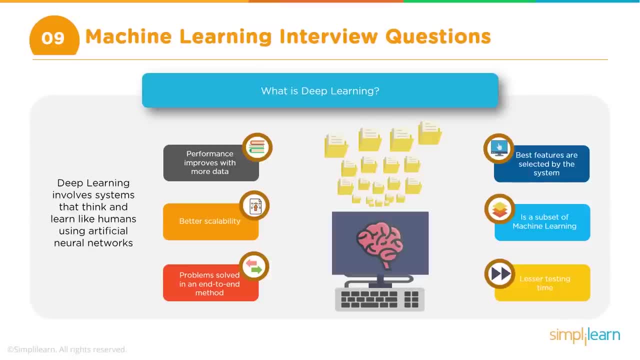 best way to respond to this could be: deep learning is a part of machine learning, And then, obviously, the question would be: then what is the difference, right? So deep learning? you need to mention there are two key parts that interviewer will be looking for when you are defining deep learning. So, first, 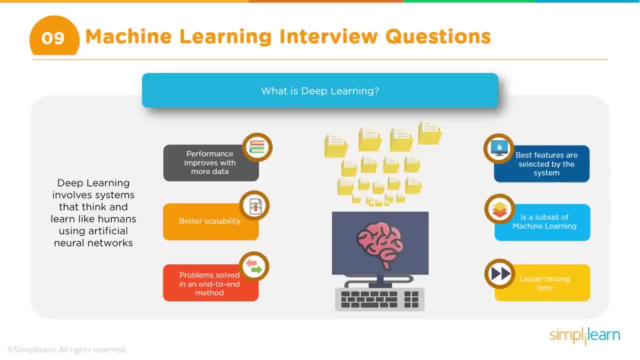 is, of course, deep learning is a subset of machine learning. So machine learning is still, and deep learning is one part of it. So then, what exactly is the difference? Deep learning is primarily when we are implementing these, our algorithms, or when we are using neural networks. 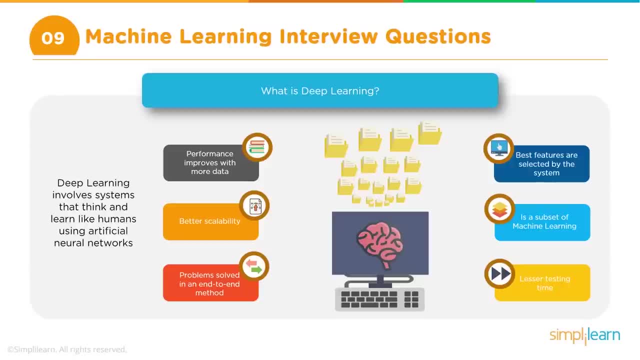 for doing our training and classification and regression and all that right. So when we use neural network then it is considered as deep learning And the term deep comes from the fact that you can have several layers of neural networks And these are called deep neural. 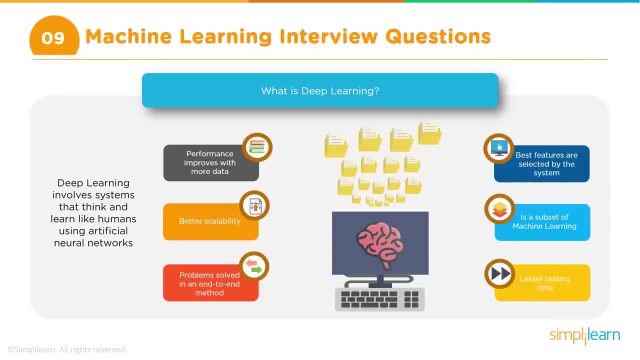 networks And therefore the term deep deep learning. The other difference between machine learning and deep learning, which the interviewer may be wanting to hear, is that in case of machine learning, the feature engineering is done manually. What do we mean by feature engineering? 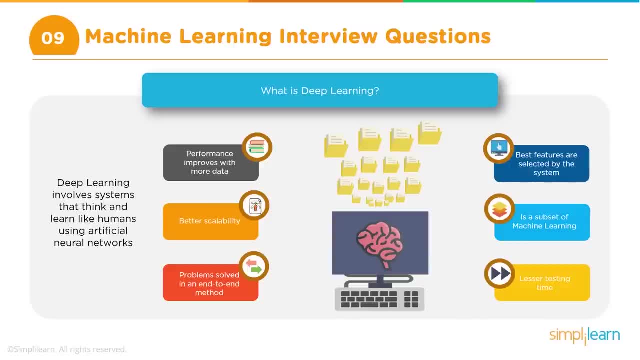 Basically, when we are trying to train our model, we have our training data right. So we have our training label data And this data has several. let's say, if it is a regular table, it has several columns. Now, each of these columns actually has information about a feature. 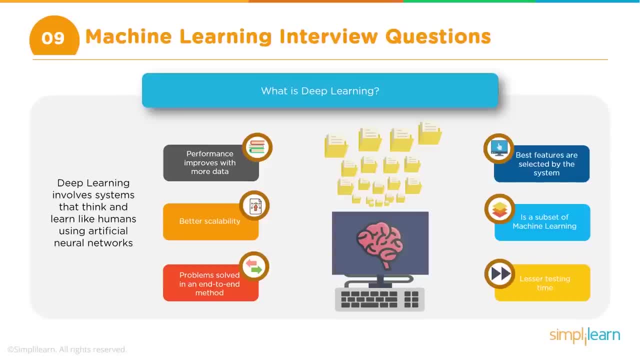 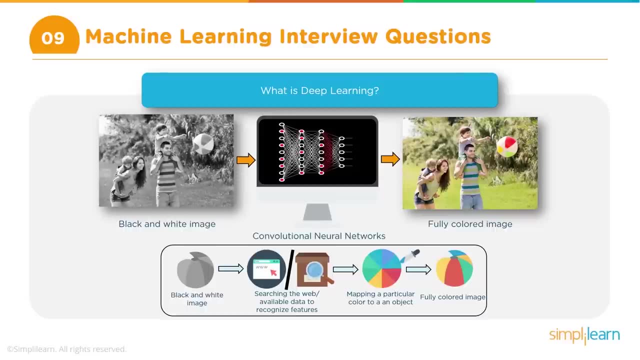 right. So if we are trying to predict the height, weight and so on and so forth, So these are all features of human beings. Let's say we have census data and we have all. So those are the features Now. there may be probably 50 or 100. In some cases there may be 100 such features Now. 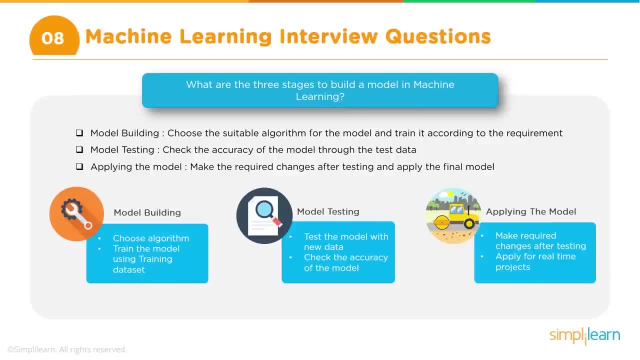 so that is again a recursive process. so once in a while you need to keep checking whether the model is working fine or not and, if required, you need to tweak it and modify it, and so on and so forth. so net, net, this is a continuous process of tweaking the model and testing it and making sure. 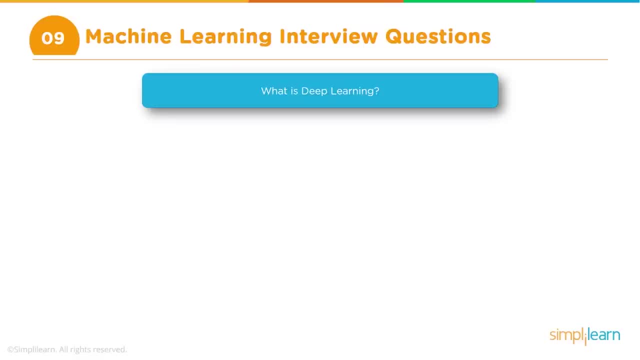 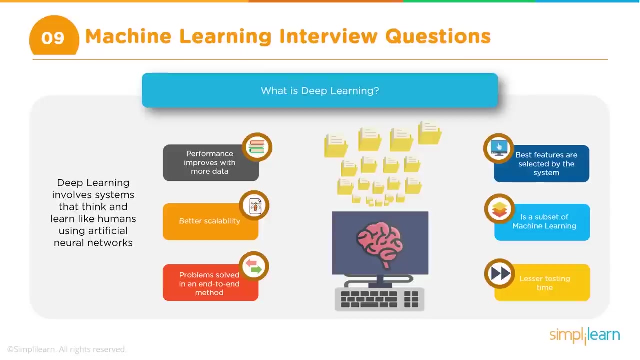 it is up to date. then you might have question around deep learning. so because deep learning is now associated with ai, artificial intelligence and so on, so can be as simple as what is deep learning? so i think the best way to respond to this could be: deep learning is a part of machine learning and 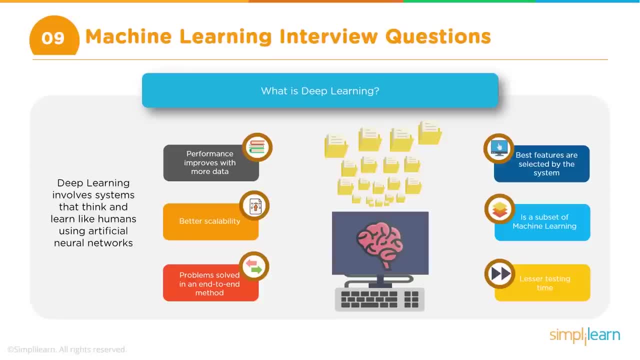 then then obviously the question would be: then what is the difference? right? so deep learning, you need to mention. there are two key parts that interviewer will be looking for when you are defining deep learning. so first is, of course, deep learning is a subset of machine learning, so machine learning is still the bigger, let's say, scope, and deep learning is one part of it. so then, 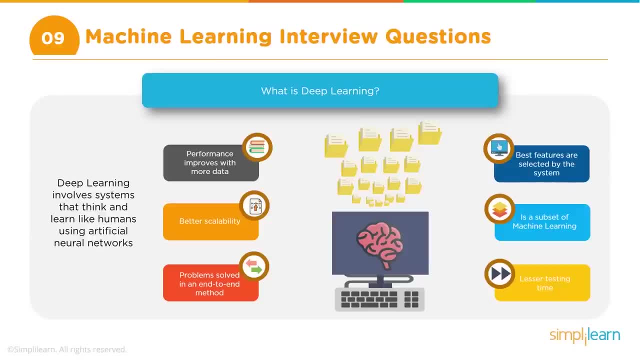 what exactly is the difference? deep learning is primarily when we are implementing these, our algorithms, or when we are using neural networks for doing our training and classification and regression and all that right. so when we use neural network, then it is considered as deep learning and the term deep comes from the fact that you can have 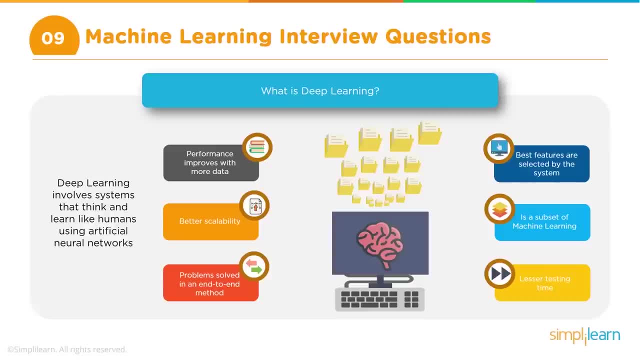 several layers of neural networks and these are called deep neural networks and therefore the deep you know deep learning. the other difference between machine learning and deep learning is that in deep learning- which the interviewer may be wanting to hear- is that in case of machine learning, the feature engineering is done manually. what do we mean by feature engineering, basically? 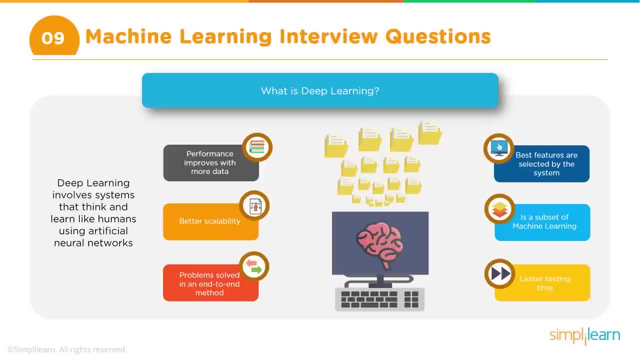 when we are trying to train our model, we have our training data, right? so we have our training label data and this data has several and let's say, if it is a regular table, it has several columns. now, each of these columns actually has information about a feature, right? so if you have a table and you 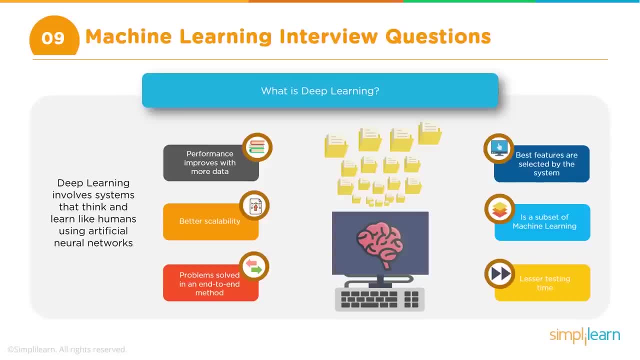 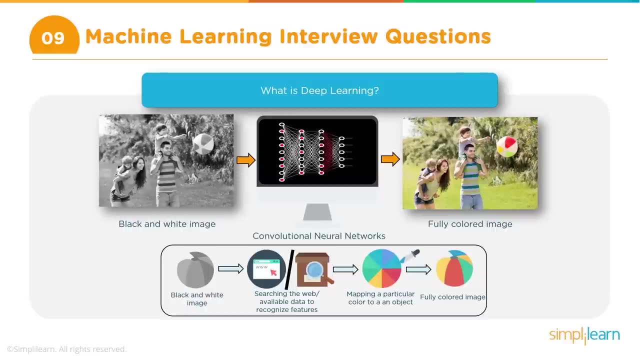 are trying to predict the height, weight and so on and so forth. so these are all features of human beings. let's say we have census data and we have all. so those are the features now there may be probably 50 or 100. in some cases there may be 100 such features. now all of them do not contribute to. 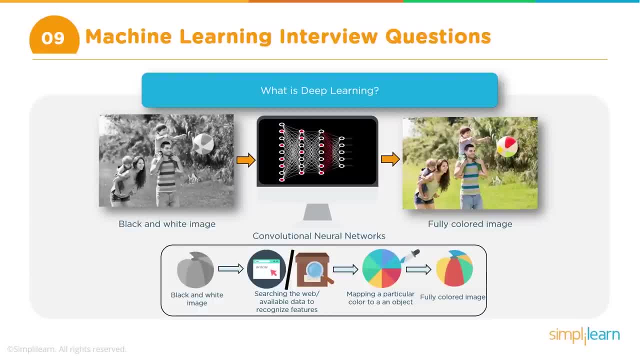 all of them do not contribute to our model right. So we, as a data scientist, we have to decide whether we should take All of them, all the features, or we should throw away some of them. because, again, if we take all of them, 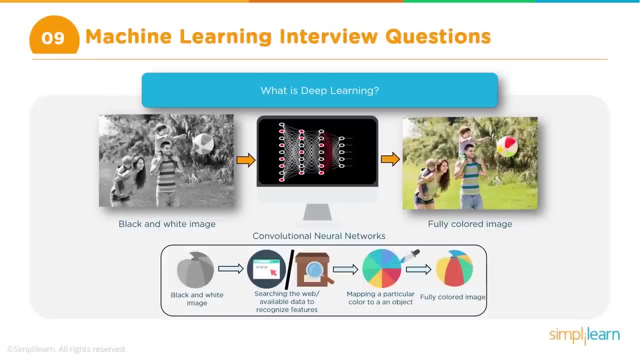 number one. of course your accuracy will probably get affected, But also there is a computational part. So if you have so many features and then we have so much data, it becomes very tricky. So in case of machine learning, we manually take care of identifying the features that do not contribute to the 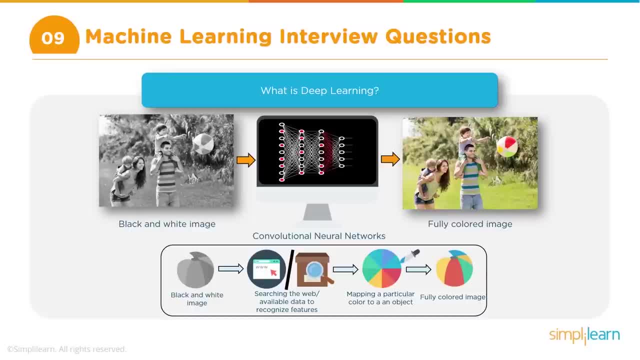 learning process, and thereby we eliminate those features and so on. Right, So this is known as feature engineering, And in machine learning we do that manually, Whereas in deep learning, where we use neural networks, the model will automatically determine which features to use and which to not use. 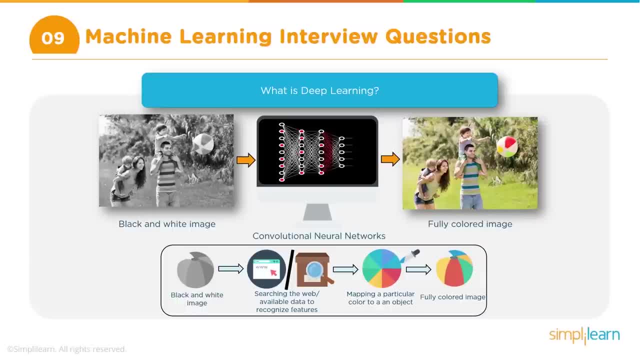 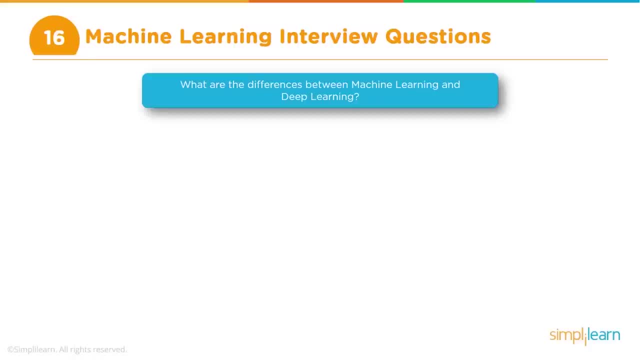 And therefore feature engineering is also done automatically. So this is an explanation. These are two key things probably will add value to your response. All right, So the next question is: what is the difference between, or what are the differences between machine learning and deep learning? 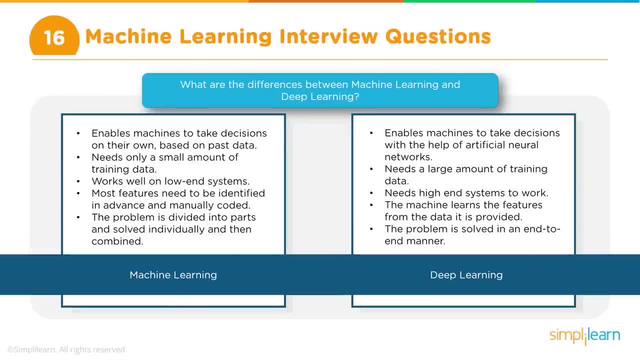 So here this is a Quick comparison table between machine learning and deep learning, and machine learning learning enables machines to take decisions on their own based on past data, So here we are talking primarily of supervised learning, and it needs only a small amount of data for training and then works well on low end systems. 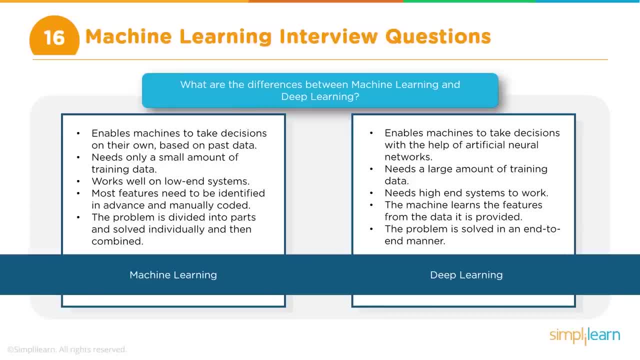 So you don't need large machines and most features need to be identified in advance and manually coded. So basically the feature engineering part is done manually and the problem is divided into parts and solved individually and then combined. So that is about the machine learning part. 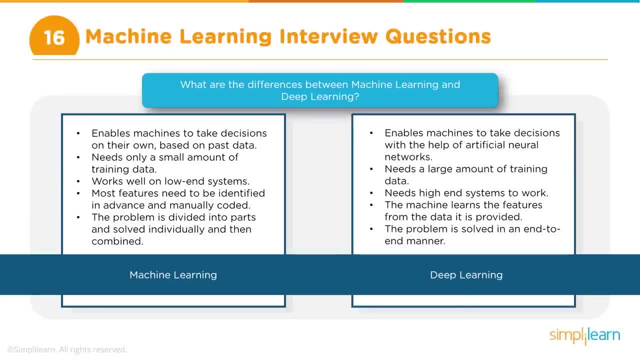 In deep learning. deep learning basically enables machines to take decisions with the help of artificial neural networks. So here in deep learning we use neural networks. So that is the key differentiator between machine learning and deep learning, And usually deep learning involves a large amount of data. 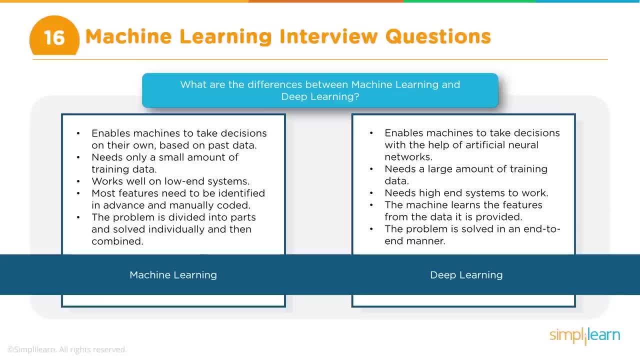 And therefore the training also requires. usually the training process requires high end machines because it needs a lot of computing power And the machine Learning features are the or the feature engineering is done automatically, So the neural networks takes care of doing the feature engineering as well. 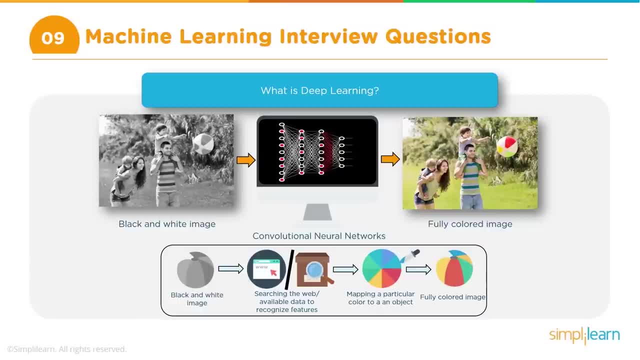 our model right. so we, as a data scientist, we have to decide whether we should take all of them, all the features, or we should throw away some of them. because, again, if we take all of them, number one of the features in the model are the differences and number two of the features are not the same. 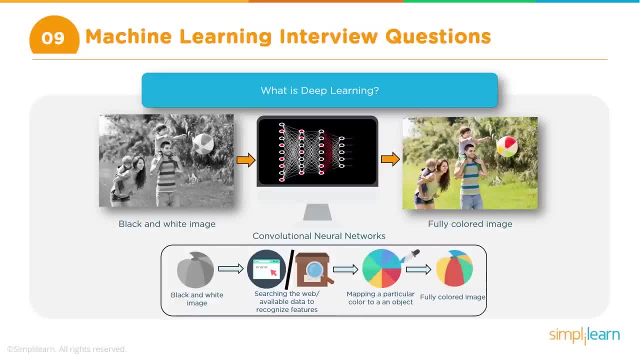 so it is an issue of accuracy, of accuracy will probably get affected, but also there is a computational part. so if you have so many features and then we have so much data, it becomes very tricky. so in case of machine learning, we manually take care of identifying the features that do not. 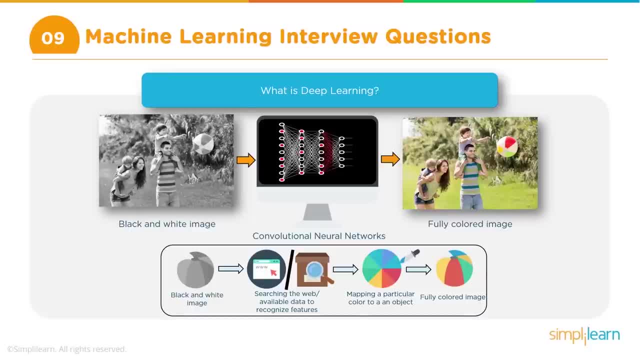 contribute to the learning process and thereby we eliminate those features and so on. right, so this is known as feature engineering, and in machine learning we do that manually, whereas in deep automatically determine which features to use and which to not use, and therefore feature engineering is also done automatically. so this is a explanation. these are two key things probably. 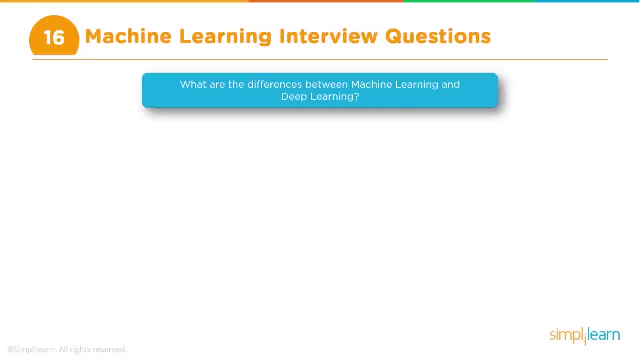 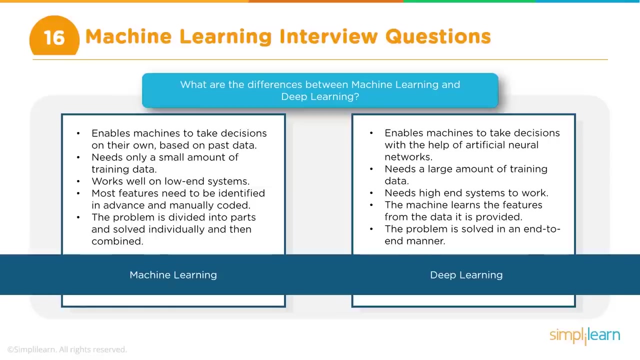 will add value to your response. all right, so the next question is: what is the difference between, or what are the differences between, machine learning and deep learning? so here this is a quick comparison table between machine learning and deep learning. and in machine learning, learning enables machines to take decisions on their own based on past data. so here we are talking primarily. 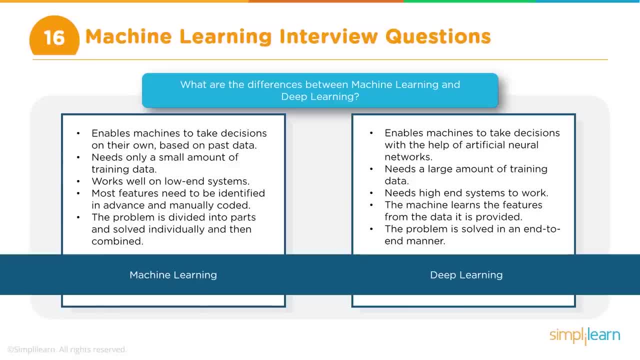 of supervised learning and it needs only a small amount of data for training and then works well on low-end systems. so you don't need large machines and most features need to be identified in advance and manually coded. so basically the feature engineering part is done manually and 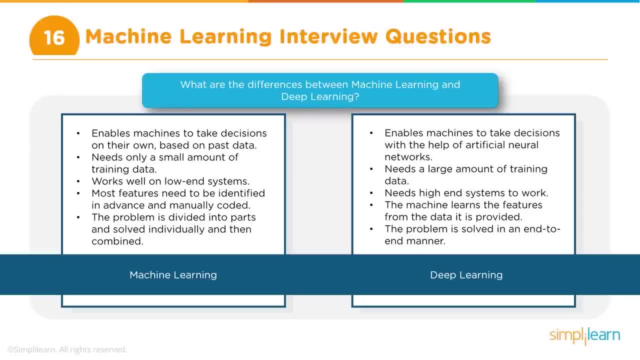 the problem is divided into parts and solved individually and then combined. so that is about the machine learning part. but in deep learning deep learning basically enables machines to take decisions with the help of artificial neural networks. so here in deep learning we use neural lines. so that is. 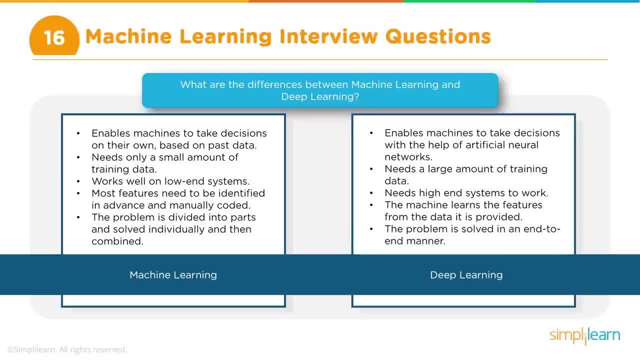 the key differentiator between machine learning and deep learning, and usually deep learning involves a large amount of data and therefore the training also requires. usually the training process requires high-end machines because it needs a lot of computing power and the machine learning features are the or the feature engineering is done automatically, so the neural 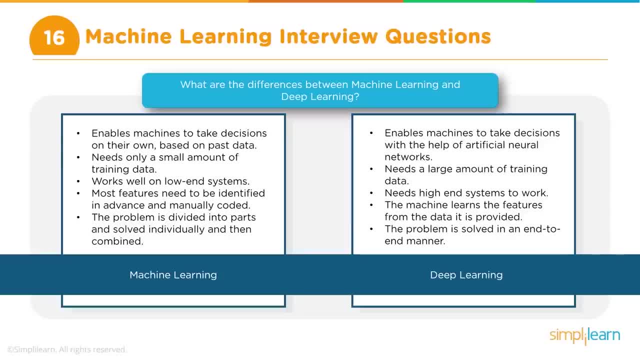 networks takes care of doing the feature engineering as well, and in case of deep learning, therefore, it is said that the problem is handled end to end. so this is a quick comparison between machine learning and deep learning. in case you have that kind of a question, then you might get. 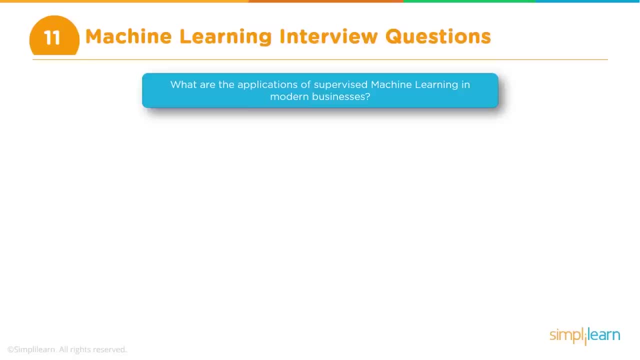 a question around the uses of machine learning or some real life applications of machine learning in modern business. the question may be worded in different ways, but the meaning is: how exactly is it used, or actually supervised machine learning? it could be a very specific question around supervised machine learning, so this is like give examples of supervised machine learning, use of. 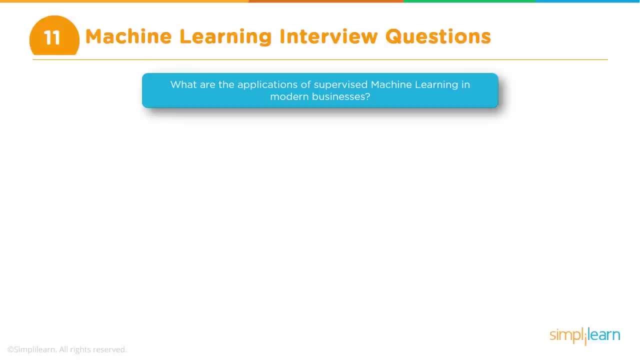 supervised machine learning in modern business? so that could be the next question. so there are quite a few examples, or quite a few use cases, if you will, for supervised machine learning. the very common one is email spam detection. so you want to train your application or your system to detect. 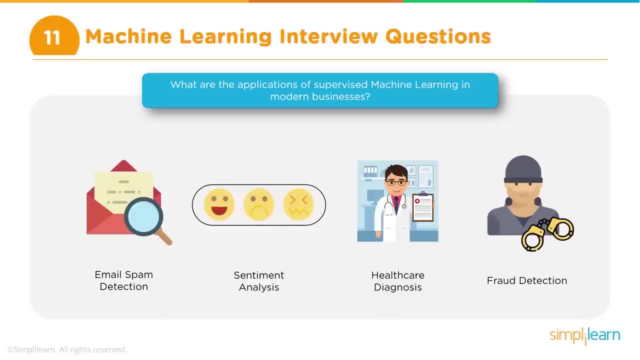 spam and non-spam. so this is a very common business application of supervised machine learning. so how does this work? the way it works is that you obviously have historical data of all of your emails and they are categorized as spam and not spam. so that is what is the labeled information. 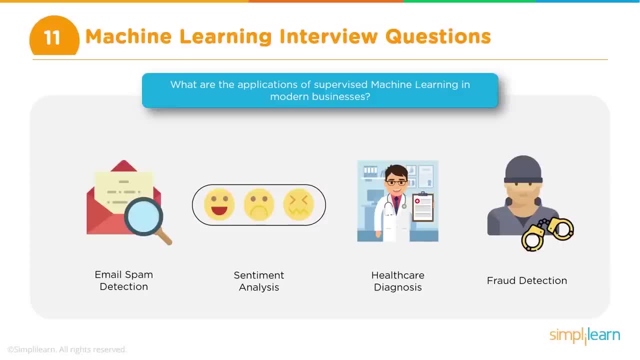 and then you feed this information or the all these emails as an input to your model, right, and the model will then get trained to detect which of the emails are to detect which is spam and which is not spam. so that is the training process and this is supervised machine learning, because you have labeled data. 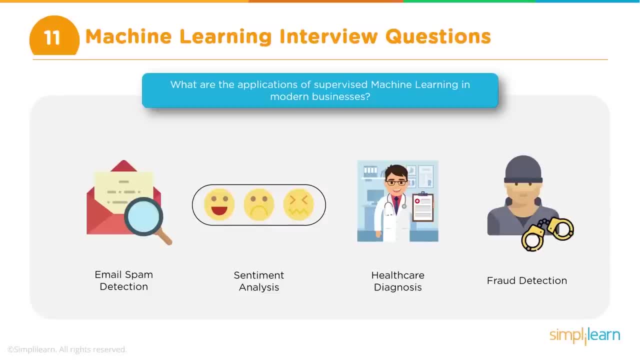 you already have emails which are tagged as spam or not spam, and then you use that to train your model right. so this is one example. now there are a few industry specific applications for supervised machine learning. one of the very common ones is in healthcare: diagnostics in healthcare. 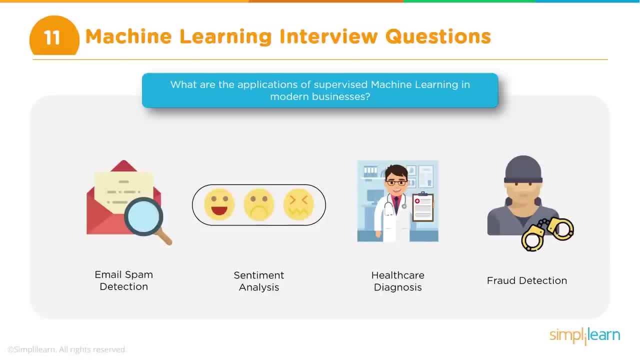 states. you have these images and you want to train models to detect whether, from a particular image, whether it can find out if the person is sick or not, whether a person has cancer or not, right? so this is a very good example of supervised machine learning. here, the way it works, is that existing? 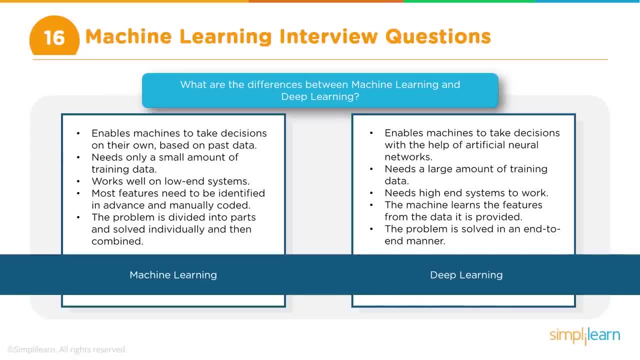 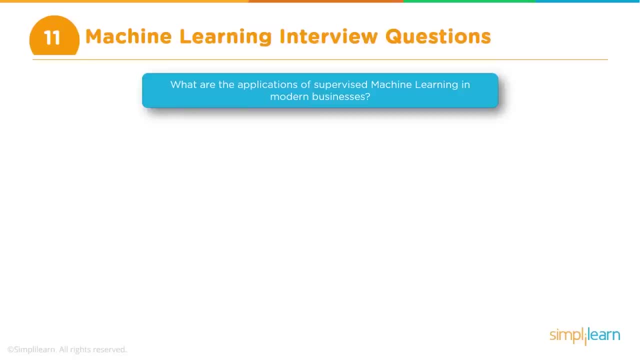 And in case of deep learning, therefore, it is said that the problem is handled end to end. So this is a quick comparison between machine learning and deep learning. In case you have that kind of a question, then you might get a question around the uses of machine learning or some real life applications of machine learning in modern business. 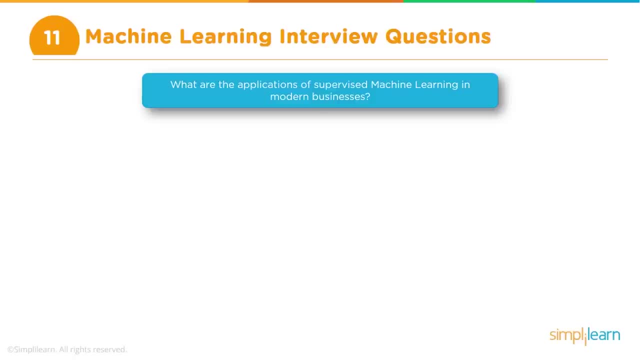 The question may be where did In different ways, But the meaning is: how exactly is machine learning used, or actually supervised machine learning? It could be a very specific question around supervised machine learning, So this is like give examples of supervised machine learning, use of supervised machine learning in modern business. 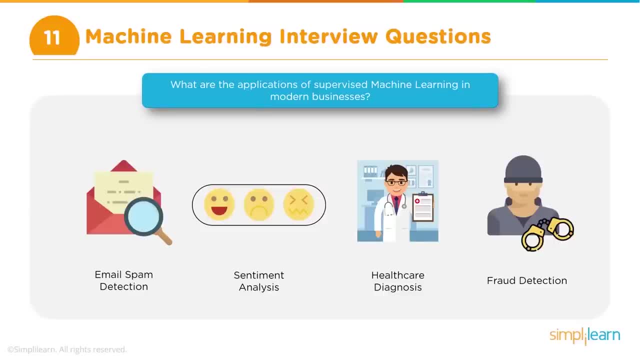 So that could be the next question. So there are quite a few examples on quite a few use cases for supervised machine learning. The very common one is email spam detection. So You want to train your application or your system to detect between spam and non spam. 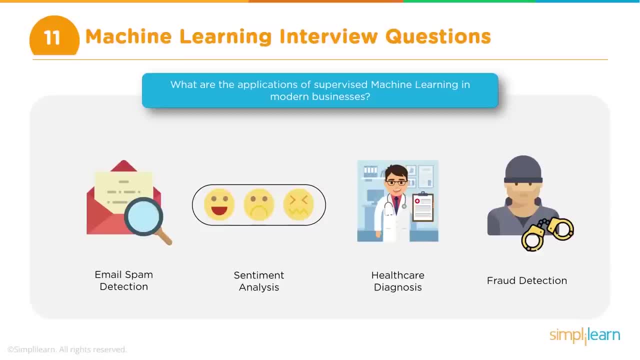 So this is a very common business application of supervised machine learning. So how does this work? The way it works is that you obviously have historical data of all of your emails and they are categorized as spam and not spam. That is what is the labeled information. 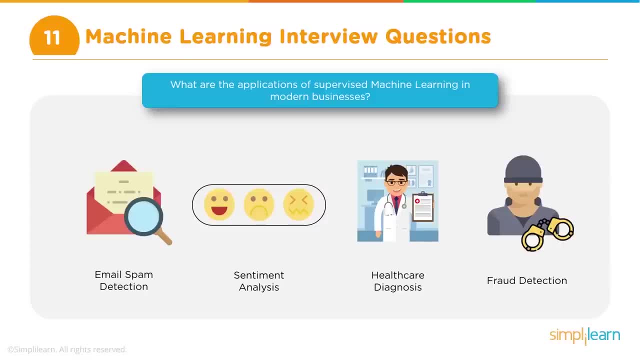 And then you feed this information order, All these emails, emails as an input to your model, right, And the model will then get trained to detect which of the emails are to detect which is spam and which is not spam. So that is the training process And 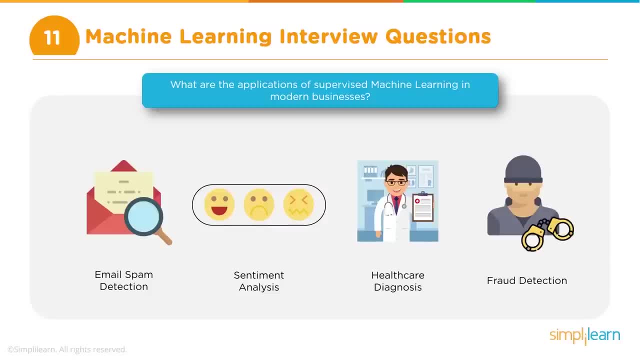 this is supervised machine learning, because you have labeled data, you already have emails which are tagged as spam or not spam, and then you use that to train your model right. So this is one example. Now there are a few industry specific applications for supervised machine learning. 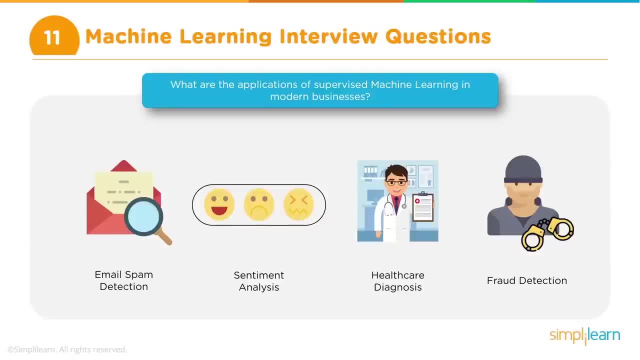 One of the very common ones is in healthcare diagnostics. In healthcare diagnostics you have these images and you want to train models to detect whether from a particular image, whether it can find out if the person is sick or not, whether a person has cancer or not. 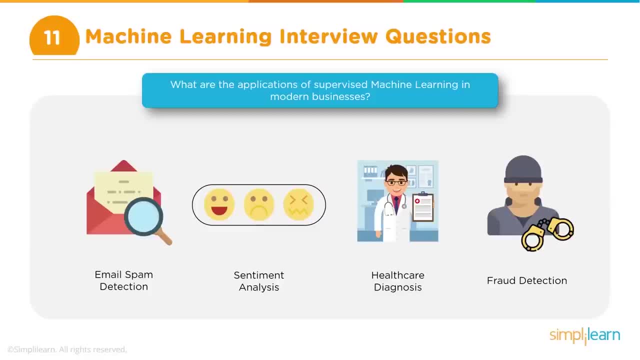 right. So this is a very good example of supervised machine learning. Here the way it works is that existing images- it could be x-ray images, it could be MRI or any of these images- are available and they are tagged saying that, okay, this x-ray image is. 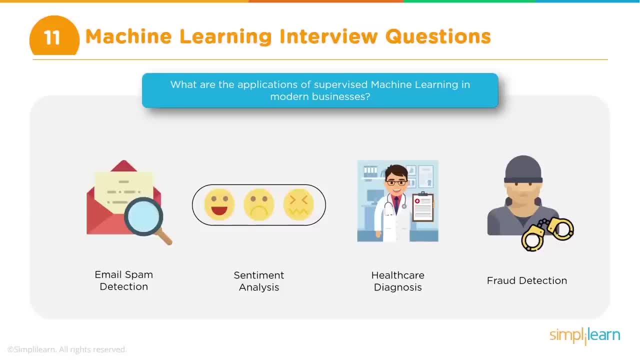 images. it could be x-ray images, it be mri or any of these images are available and they are tagged saying that, okay, this x-ray image is going to be a cancer one or not. and then you have the images and image is defective or the person has an illness or it could be cancer. whichever illness, right? 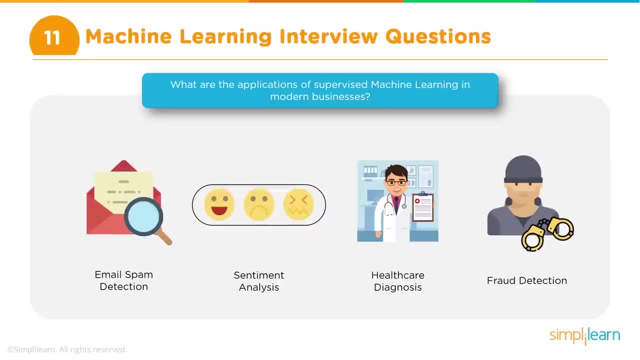 So it is tagged as defective or clear or good image and defective image, something like that. So we come up with a binary- or it could be multi-class as well- saying that this is defective to 10%, this is 25% and so on. But let's keep it simple. You can give an example of just a binary. 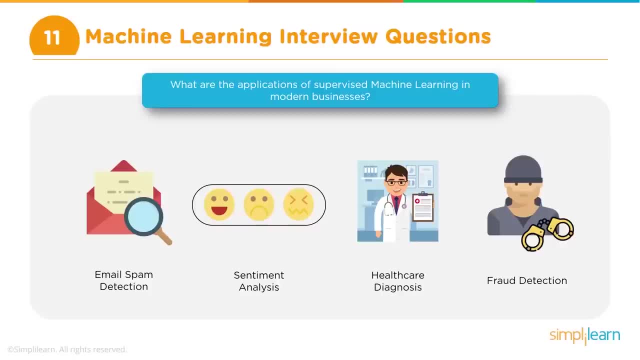 classification. that would be good enough. So you can say that in healthcare diagnostics using image, we need to detect whether a person is ill or whether a person is having cancer or not. So here the way it works is you feed labeled images and you allow the model to learn from that so that 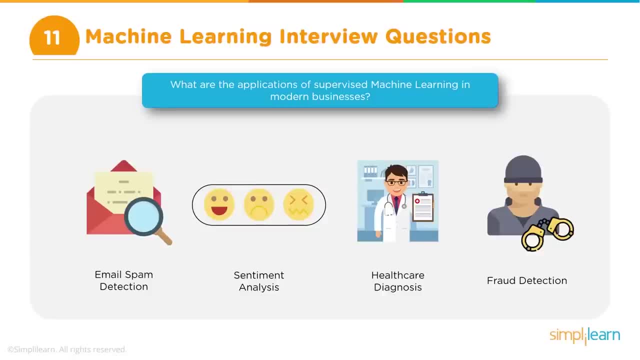 when new image is fed, it will be able to predict whether this person is having that illness or not, having cancer or not, right? So I think this would be a very good example for supervised machine learning in modern business. All right, then we can have a question like: 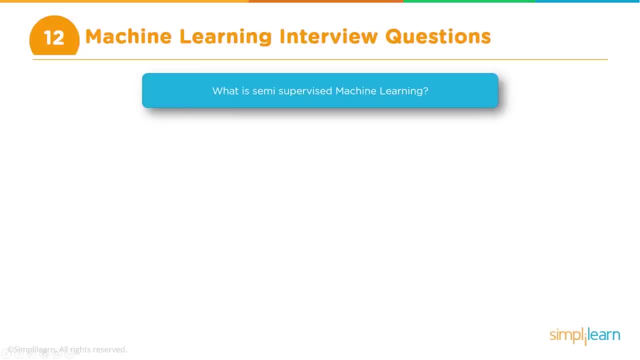 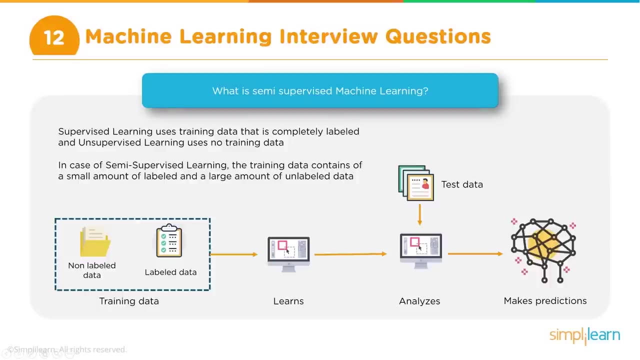 so we've been talking about the concept of machine learning. So we can have a question like talking about supervised and unsupervised, And so there can be a question around semi-supervised machine learning. So what is semi-supervised machine learning? Now, semi-supervised learning. 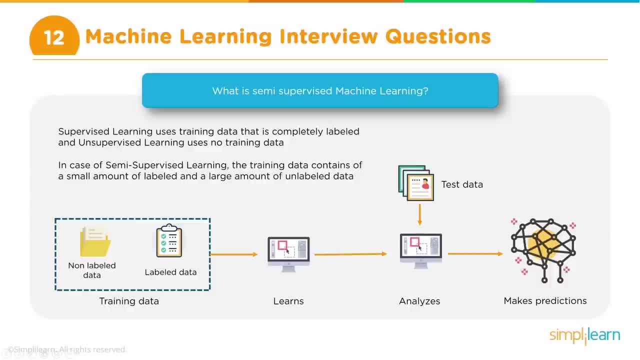 as the name suggests, it falls between supervised learning and unsupervised learning, But for all practical purposes it is considered as a part of supervised learning, And the reason this has come into existence is that in supervised learning you need to have a certain level of 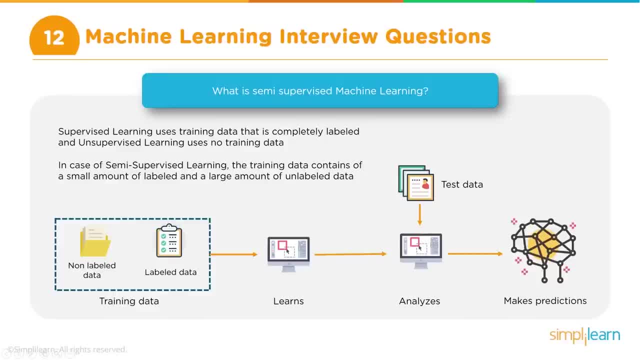 data. So all your data for training, your model has to be labeled. Now this is a big problem in many industries or under many situations. Getting the labeled data is not that easy, because there's a lot of effort in labeling this data. Let's take an example of diagnostic images. We can just 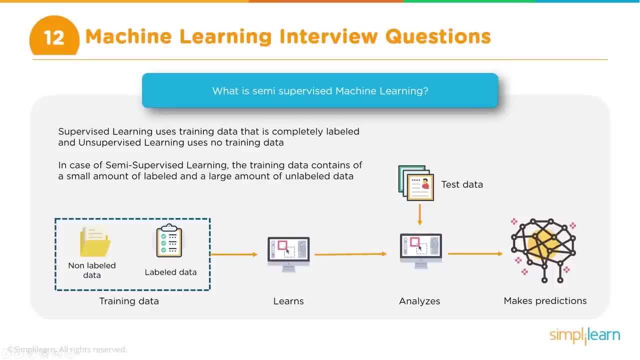 let's say, take x-ray images. Now there are actually millions of x-ray images available all over the world, But the problem is they are not labeled. So what we can do is we can just take a look at these images- And usually it should be like a doctor- and then say that: okay, 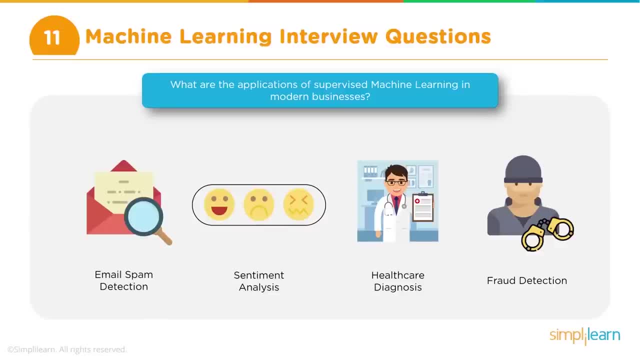 defective, or the person has an illness, or it could be cancer, whichever illness, right? so it is tagged as defective or clear or good image and defective, something like that. so we come up with a binary- or it could be multi-class as well- saying that this is defective to 10 percent. this is 25 percent. 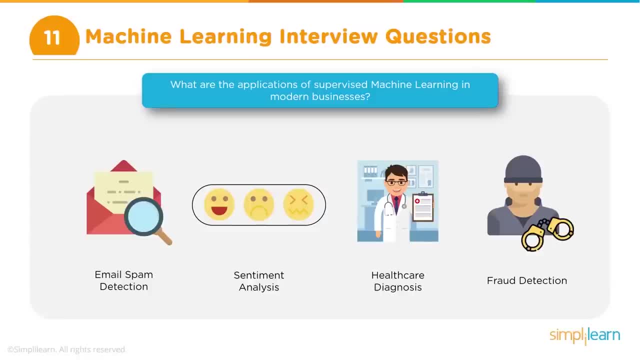 and so on. but let's keep it simple. you can give an example of just a binary classification. that would be good enough. so you can say that in healthcare diagnostics using image, we need to detect whether a person is ill, or whether a person is having cancer or not. so here the way it works. 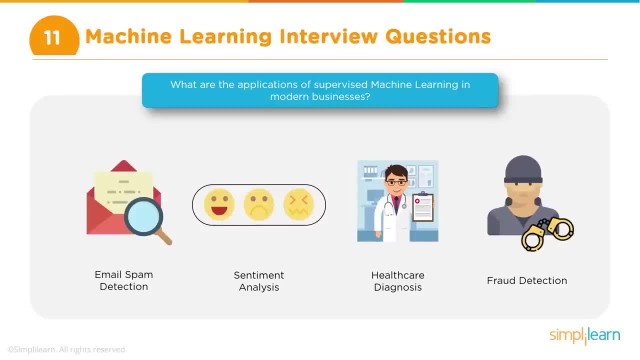 is you feed labeled images and you allow the model to learn from that so that when new image is fed, it will be able to predict whether this person is having that illness or not, having cancer or not, right? so i think this would be a very good example for supervised machine. 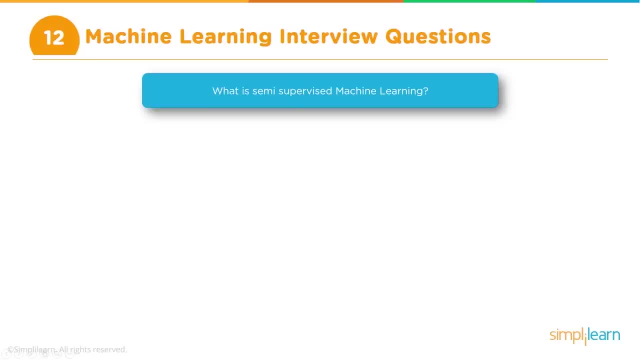 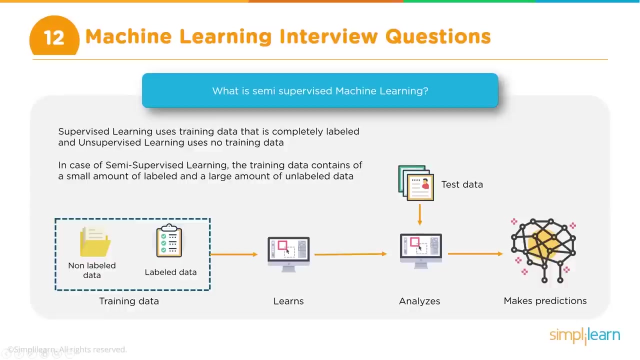 learning in modern business. all right, then we can have a question like: so we've been talking about supervised and unsupervised, and so there can be a question around semi-supervised machine learning. so what is semi-supervised machine learning? now semi-supervised learning, as the name suggests, it falls between supervised learning and unsupervised learning, but for all. 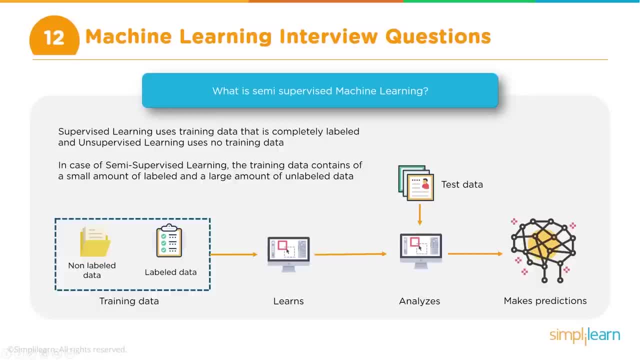 practical purposes. it is considered as a part of supervised learning, and the reason this has come into existence is that in supervised learning you need labeled data, so all your data for training, your model, has to be labeled. now this is a big problem in many industries or in many 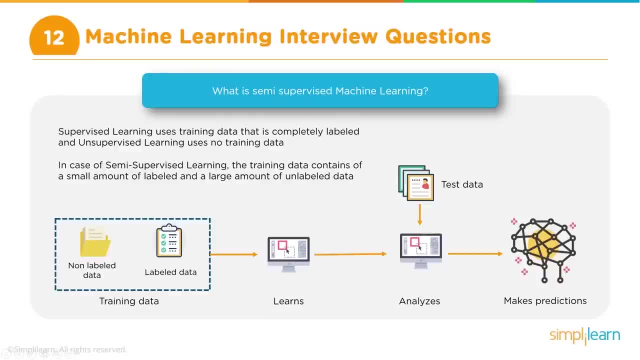 under many situations, getting the labeled data is not that easy, because there's a lot of effort in labeling this data. let's take an example of diagnostic images. we can just, let's say, take x-ray images. now there are actually millions of x-rays in the world and there are millions of 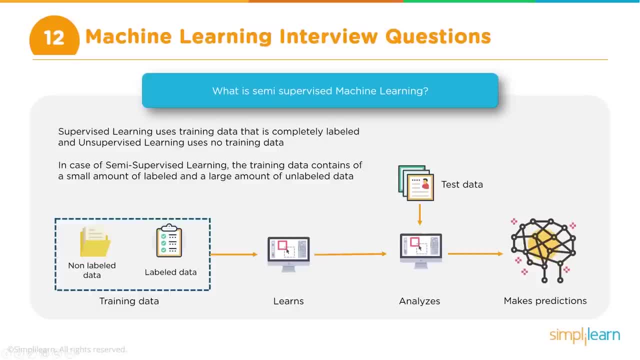 x-rays in the world, and there are millions of x-rays in the world and there are millions of x-ray images available all over the world, but the problem is they are not labeled. so their images are there, but whether it is defective or whether it is good that information is not available along, 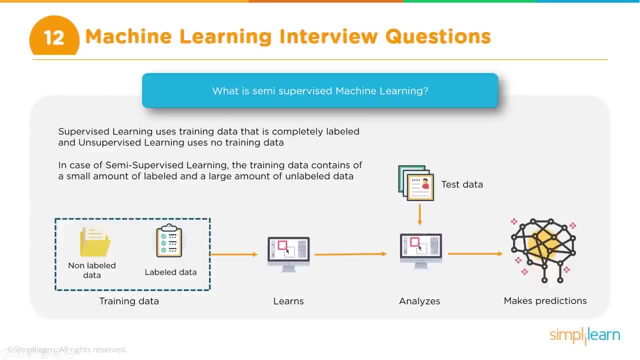 with it right in a form that it can be used by a machine, which means that somebody has to take a look at these images- and usually it should be like a doctor- and then say that, okay, yes, this image is clean and this image is cancerous, and so on and so forth. now, that is a huge effort by 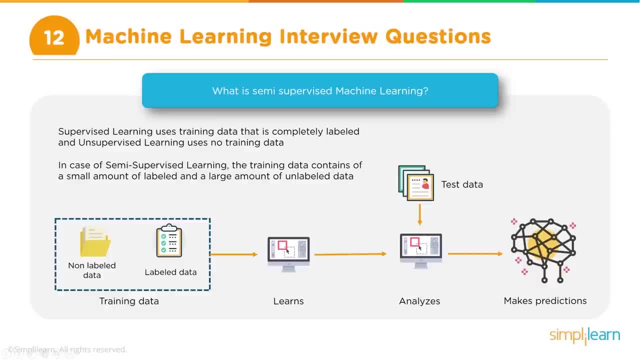 itself. so this is where semi-supervised learning comes into play. so what happens is there is a large amount of data, maybe a part of it is labeled. then we try some techniques to label the remaining part of the data so that we get completely labeled data, and then we train our model. so i know there's a. 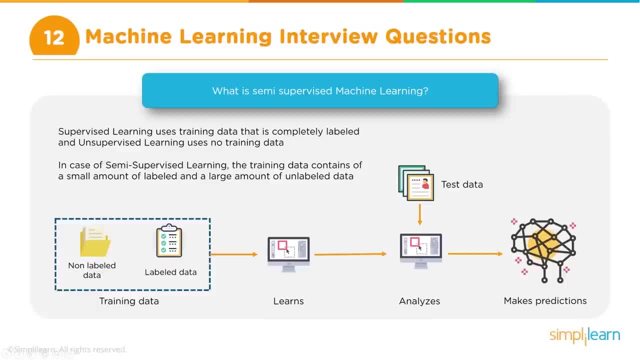 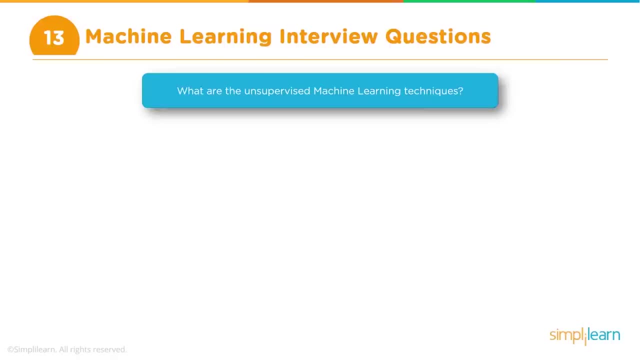 little long, winding explanation, but unfortunately there is no quick and easy definition for semi-supervised machine learning. this is the only way probably to explain this concept. we may have another question as what are unsupervised machine learning techniques or what are some of the techniques used for performing unsupervised 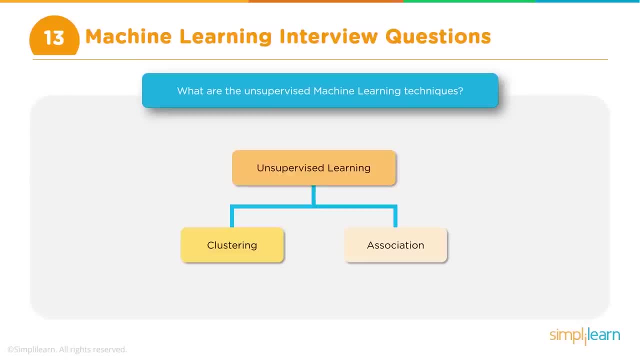 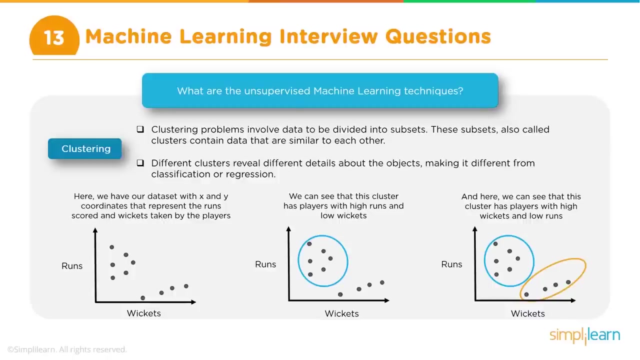 machine learning so it can be worded in different ways. so how do we answer this question? so unsupervised learning. you can say that there are two types: clustering and association. and clustering is a technique where similar objects are put together. there are different ways of finding similar objects. 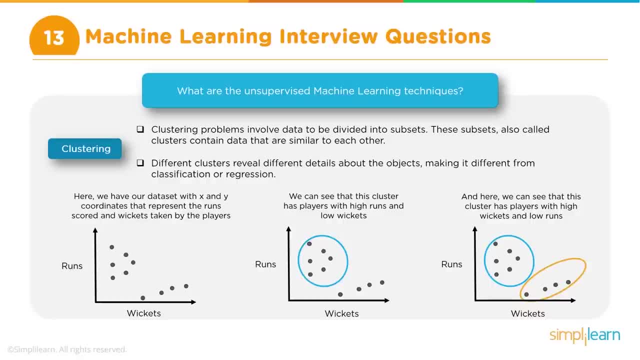 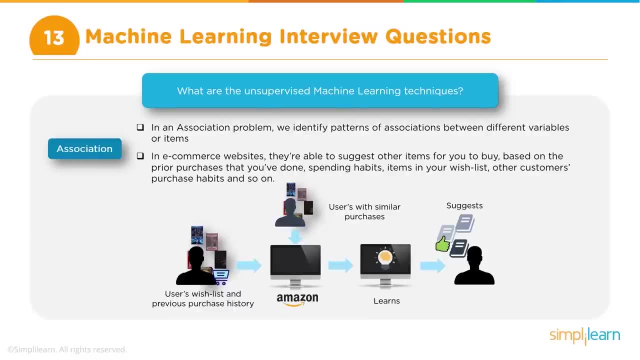 so their characteristics can be measured. and if they have in most of the characteristics, if they are similar, then they can be put together. this is clustering, then association you can. i think the best way to explain association is with an example. in case of association, you try to find out how the items are linked to each other. so, for example, if somebody bought 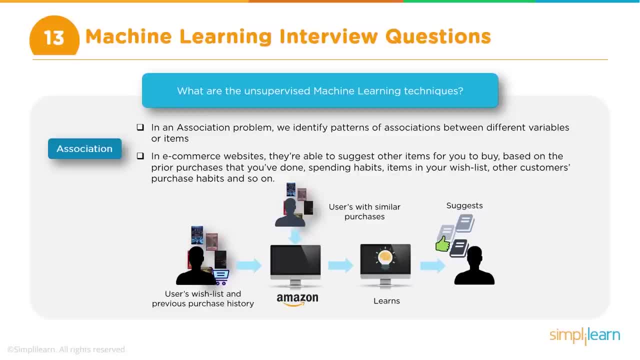 a, maybe a laptop, the person has also purchased a mouse. so this is more in an e-commerce scenario, for example, so you can give this as an example. so people who are buying laptops are also buying a mouse. so that means there is an association between laptops and mouse. or maybe people who are 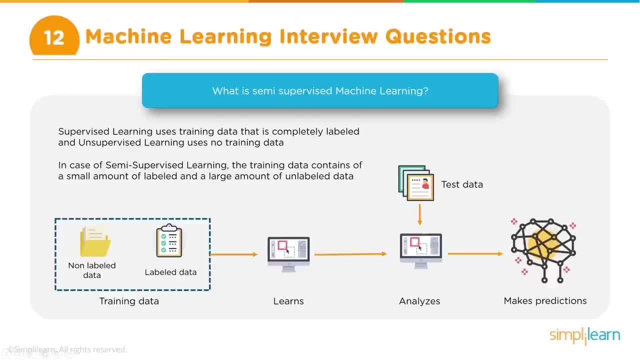 yes, this image is clean, and this image is cancerous, and so on and so forth. Now, that is a huge effort by itself. So this is where semi-supervised learning comes into play. So what happens is there is a large amount of data. Maybe a part of it is labeled. Then we try. 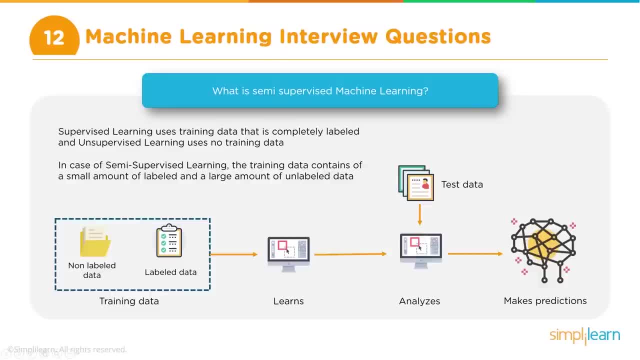 some techniques to label the remaining part of the data so that we get completely labeled data and then we train our model. So I know this is a little long winding explanation, but unfortunately there is no quick and easy definition for semi-supervised machine learning. This is the 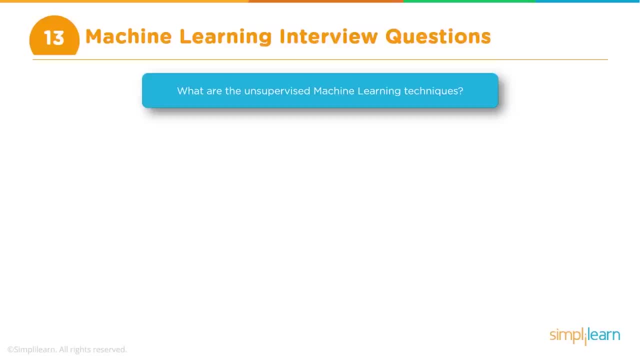 only way, probably, to explain this concept. We may have another question. What are some of the techniques used for performing unsupervised machine learning? So it can be worded in different ways. So how do we answer this question? So unsupervised learning, you can say. 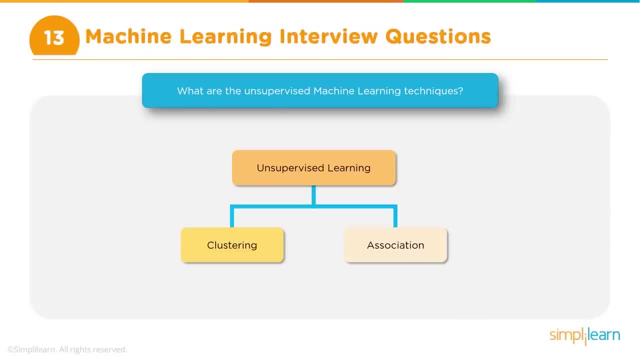 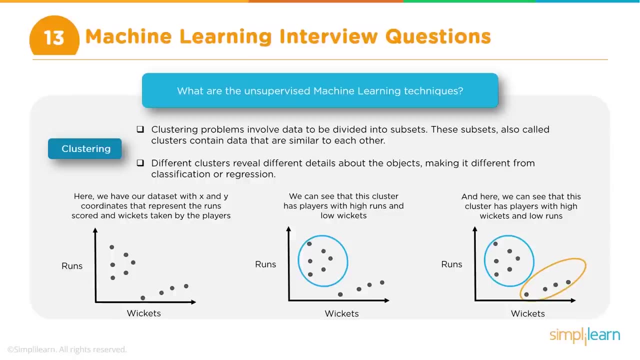 that there are two types: clustering and association. And clustering is a technique where similar objects are put together. There are different ways of finding similar objects, So their characteristics can be measured and if they have most of the characteristics, if they are similar, then they can be put together. This is clustering, Then association you can, I think, the 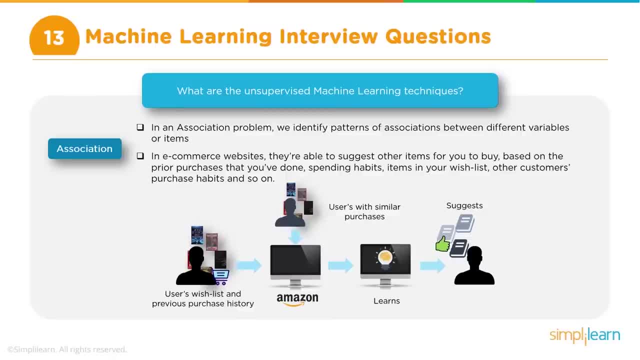 best way to explain association is with an example. In case of association, you try to find out how the items are linked to each other. So, for example, if somebody bought maybe a laptop, the person has also purchased a mouse. So this is more in an e-commerce. 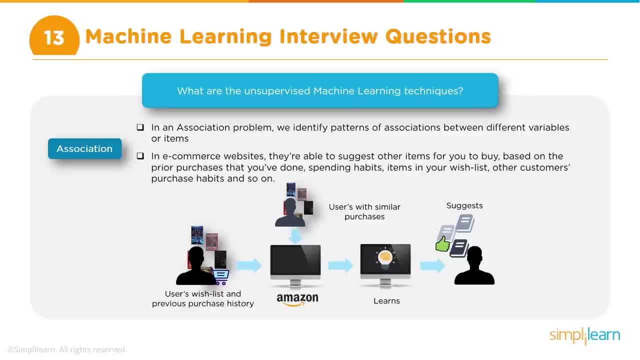 internet scenario, for example, So you can give this as an example. So people who are buying laptops are also buying a mouse, So that means there is an association between laptops and mouse. or maybe people who are buying bread are also buying butter, So that is the association that. 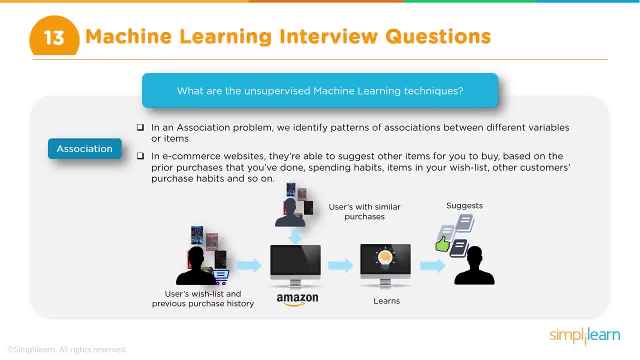 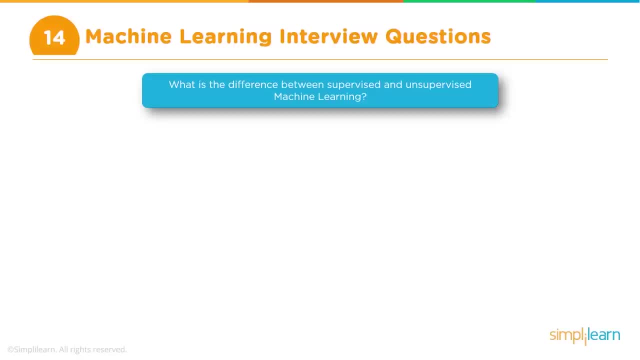 can be created. So this is unsupervised learning, one of the techniques. Okay, All right. Then we have a fundamental question: What is the difference between supervised and unsupervised machine learning? So machine learning, these are the two main types of machine learning: supervised and unsupervised. 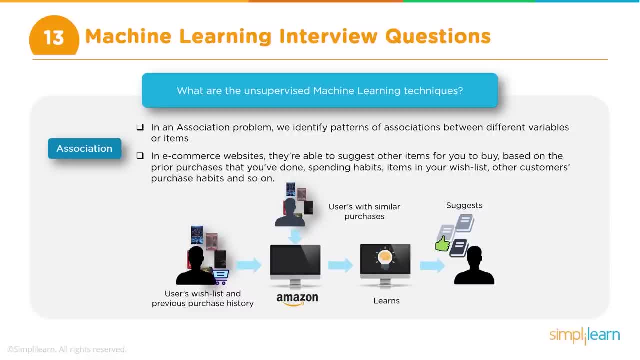 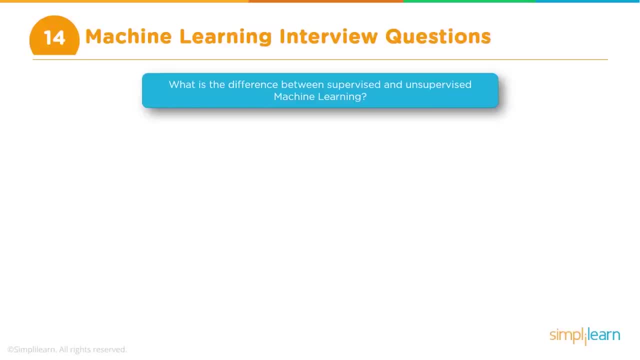 buying bread are also buying butter, so that is a association that can be created. so this is unsupervised learning, one of the techniques. okay, all right. then we have very fundamental question: what is the difference between supervised and unsupervised machine learning? so, machine learning, these are the two main types of machine learning- supervised and unsupervised- and in 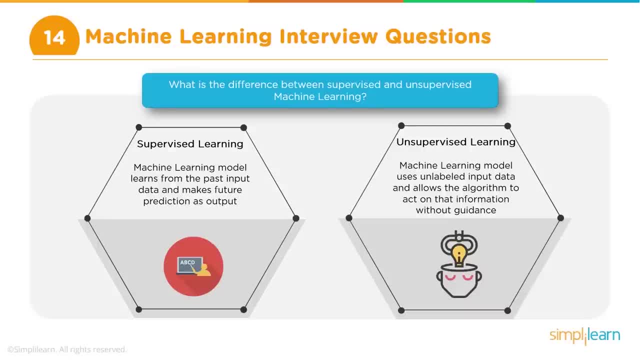 case of supervised and again here, probably the key word that the person may be wanting to hear is labeled data. now, very often people say we have historical data and if we run it, it is supervised, and if we don't have historical data, yes, but you may have historical data. 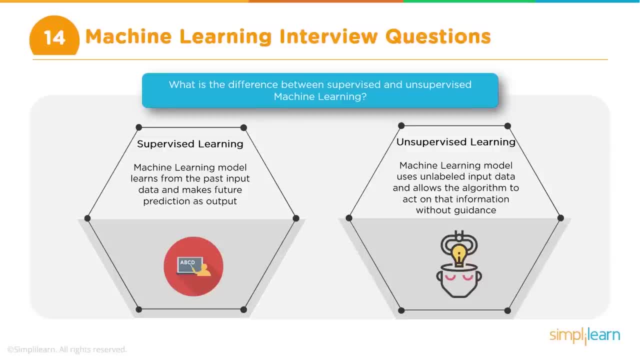 but if it is not labeled then you cannot use it for supervised learning. so this is a very key to understand that we put in that keyword labeled okay. so when we have labeled data for training, our model, then we can use supervised learning. and if we do not have labeled data, 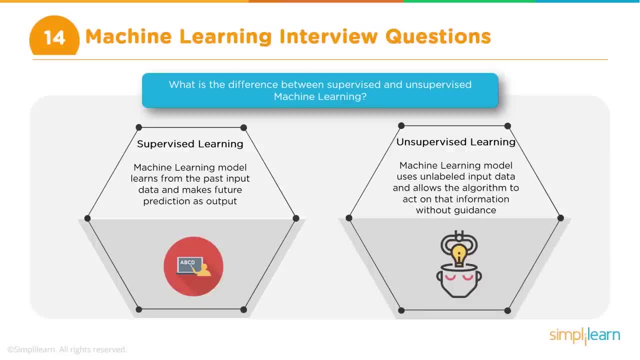 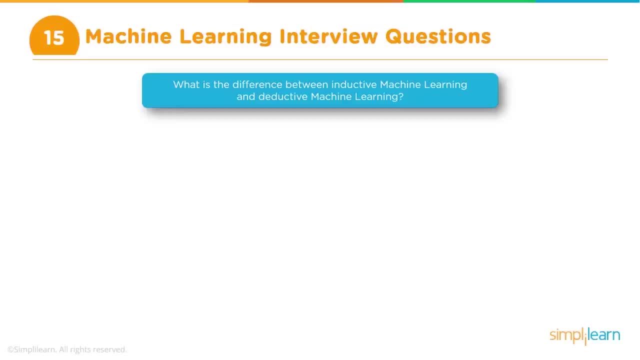 then we use unsupervised learning and there are different algorithms available to perform both of these types of trainings. so there can be another question a little bit more theoretical and conceptual in nature. this is about inductive machine learning and deductive machine learning. so the question: 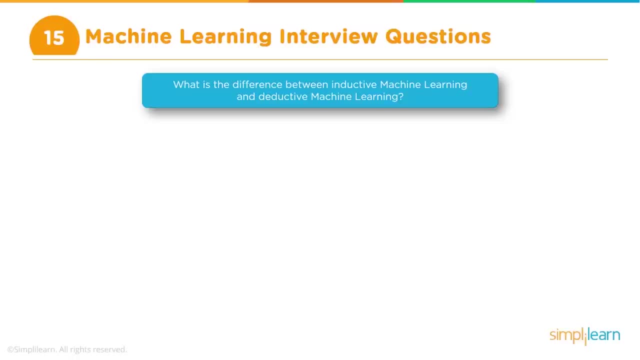 can be. what is the difference between inductive machine learning and deductive machine learning, or somewhat that manner, so that the exact phrase or exact question can vary and they can ask for examples and things like that. but that could be the question. so let's first understand what is inductive and deductive training. inductive training is induced by 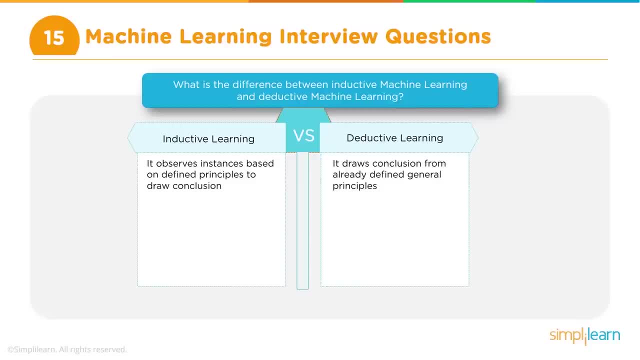 somebody and you can illustrate that with a small example. i think that always helps. so whenever you're trying to become an instructor, first of all you're kind of acting, kind of helping the students, but today we're kind of working with a genius person. it's kind of a. 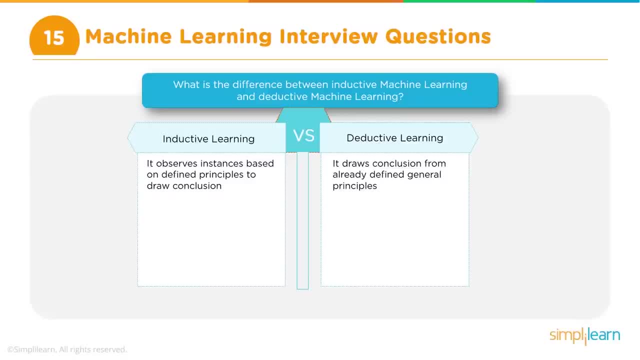 doing some explanation. Try as much as possible, as I said, to give examples from your work experience or give some analogies, and that will also help a lot in explaining as well and for the interviewer also to understand. So here we'll take an example, or rather we will use an analogy, So inductive. 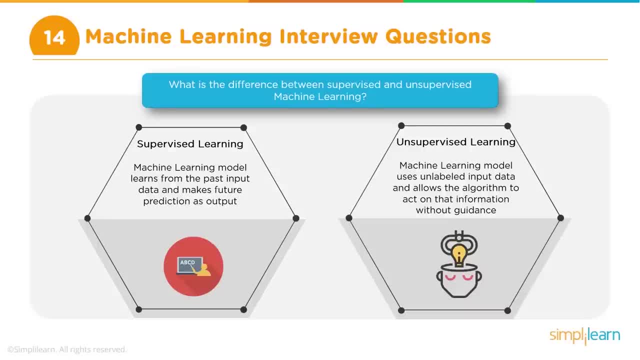 And in case of supervised- and again here, probably the key word that the person may be wanting to hear is labeled data. Now, very often people say, yeah, we have historical data and if we run it, it is supervised. And if we don't have historical data, yes, but you may have historical. 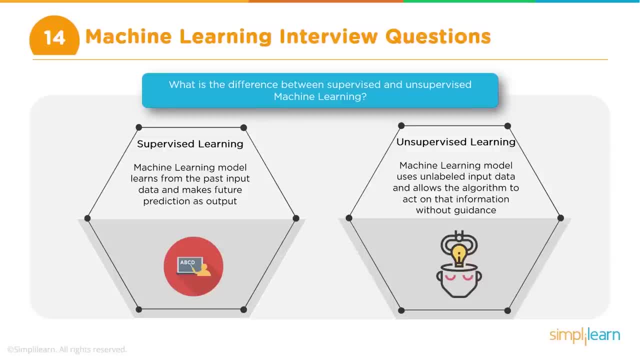 data, but if it is not labeled then you cannot use it for supervised learning. So it is it's very key to understand that we put in that keyword labeled. So when we have labeled data for training, our model, then we can use supervised learning And 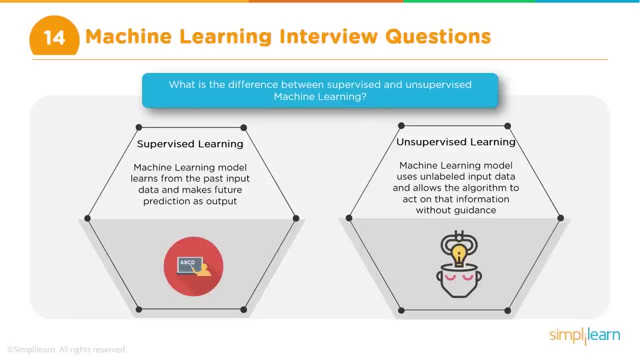 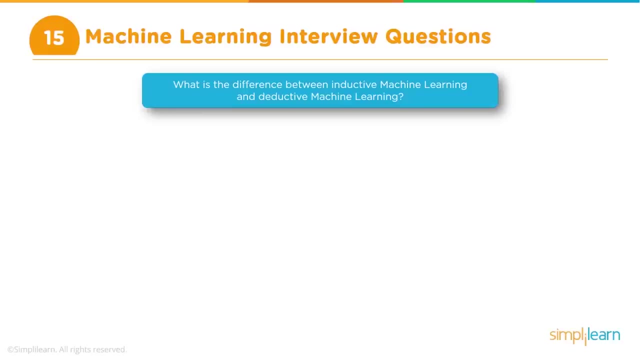 if we do not have labeled data, then we use unsupervised learning and there are different algorithms available to perform both of these types of trainings. So there can be other question little bit more theoretical and conceptual in nature. This is about inductive machine learning. 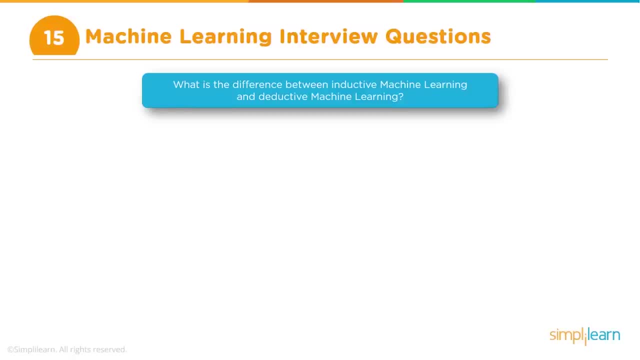 and deductive machine learning learning. So the question can be: what is the difference between inductive machine learning and deductive machine learning, or somewhat in that manner? So the exact phrase or exact question can vary and they can ask for examples and things like that, but that could be the question. So let's first 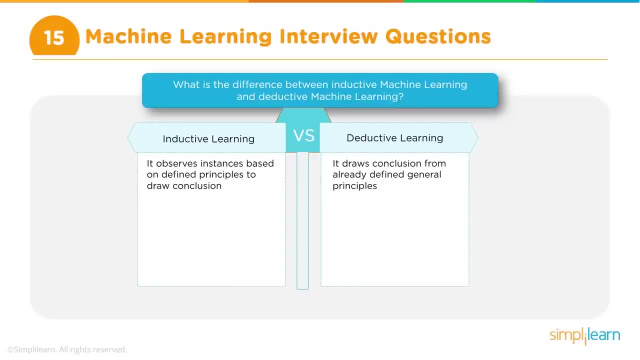 understand what is inductive and deductive training. Inductive training is induced by somebody and you can illustrate that with a small example. I think that always helps. So whenever you're doing some explanation, try as much as possible, as I said, to give examples from your work experience. 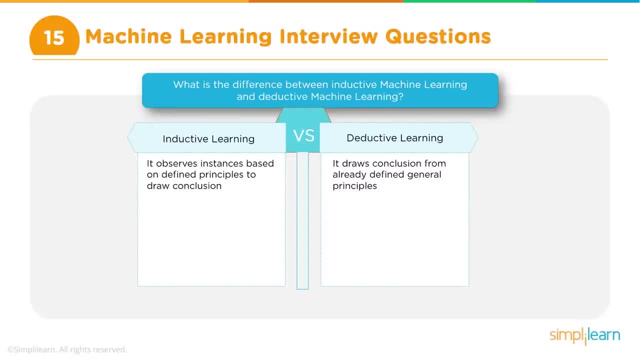 or give some analogies, and that will also help a lot in explaining as well and for the interviewer also to understand. So here we'll take an example, or rather we will use an analogy. So inductive training is when we induce some knowledge or the learning process into a person without the person. 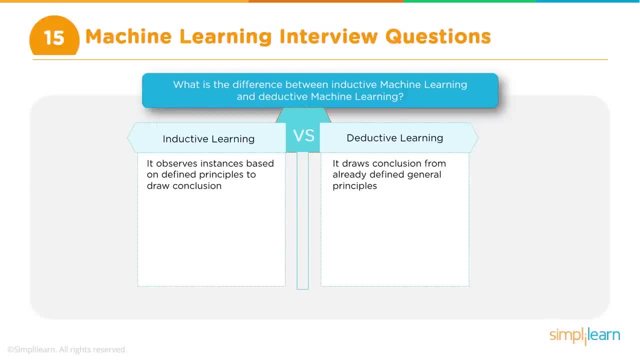 actually experiencing it. What can be an example? So we can probably say that we have an example of a person who is doing an inductive training. So we can probably say that we have an example of a person who is doing an inductive training. So we can probably 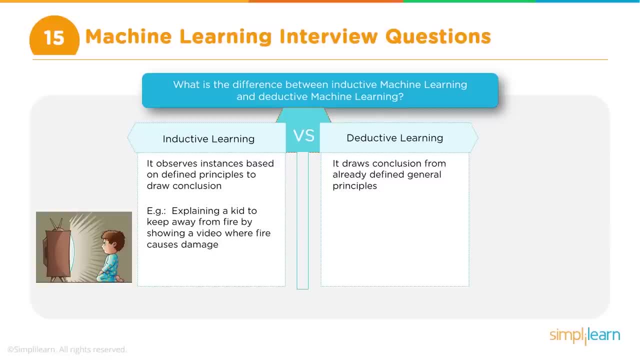 tell the person, or show a person a video that fire can burn his finger or fire can cause damage. So what is happening here? This person has never, probably, seen fire or never seen anything getting damaged by fire. but just because he has seen this video, he knows that, okay, fire is dangerous. and if 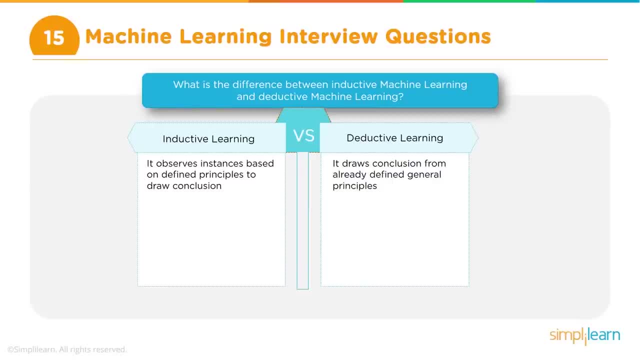 training is when we induce some knowledge or the learning process into a person without the person actually experiencing it. What can be an example? So we can probably tell the person, or show a person a video, that fire can burn his finger or fire can cause damage. So what is happening here? 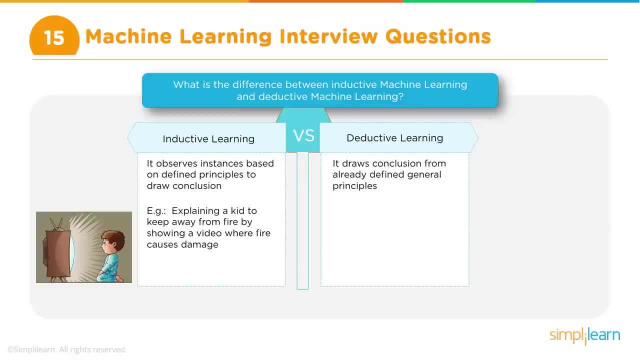 This person has never, probably, seen a fire or never seen anything getting damaged by fire. but just because he has seen this video, he knows that, okay, fire is dangerous and if a fire can cause damage, So this is inductive learning. Compared to that, what is deductive learning? So here you draw. 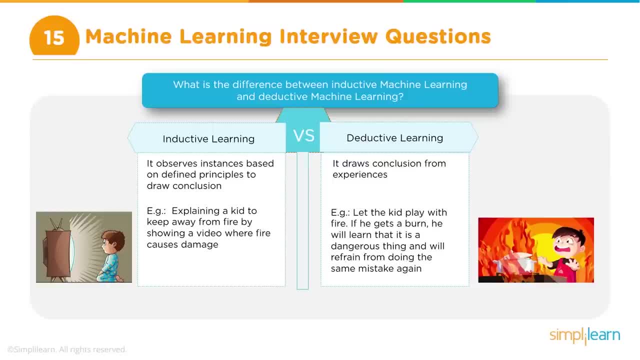 conclusion, or the person draws conclusion out of experience. So we will stick to the analogy. So, compared to the showing a video, let's assume a person is allowed to play with fire and then he figures out that if he puts his finger it's burning, or if he throws something into the fire. 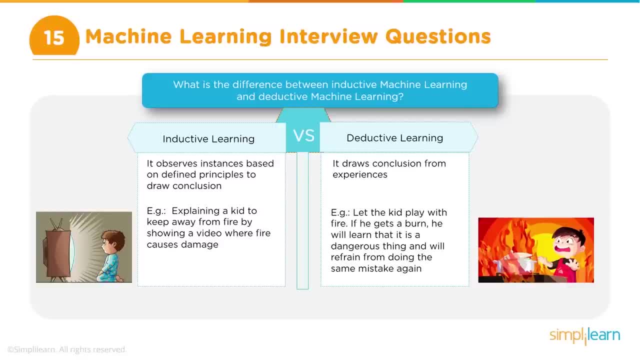 it burns. So he is learning through experience. So this is known as deductive learning. Okay, Okay, So you can have applications or models that can be trained using inductive learning or deductive learning. All right, I think probably that explanation will be sufficient. The next: 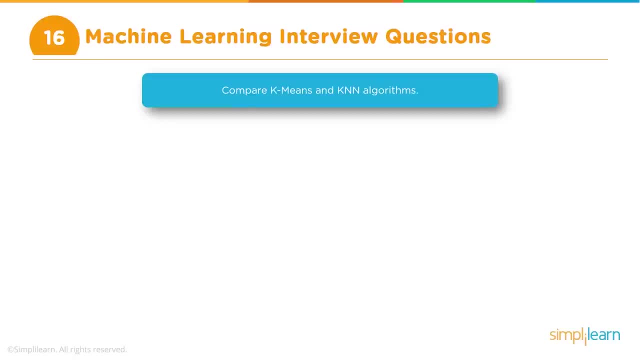 question is: are KNN and K-means clustering similar to one another, or are they same, Right? Because the letter K is kind of common between them. Okay, So let us take a little while to understand what these two are. One is KNN and another is K-means. 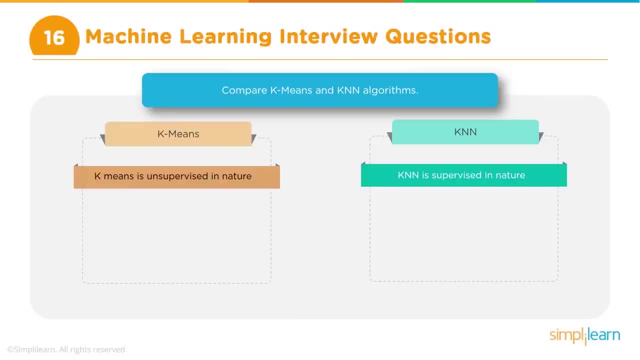 Okay, KNN stands for K-nearest neighbors and K-means, of course, is the clustering mechanism. Now, these two are completely different, except for the letter K being common between them. KNN is completely different. K-means clustering is completely different. KNN is a classification. 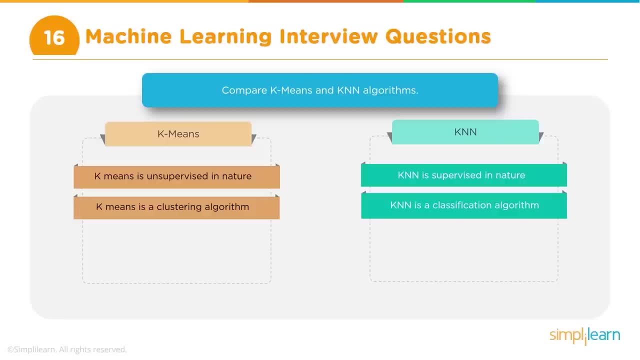 process and therefore it comes under supervised learning, whereas K-means clustering- is actually unsupervised. Okay, When you have KNN, when you want to implement KNN, which is basically K-nearest neighbors, the value of K is a number, So you can say K is equal. 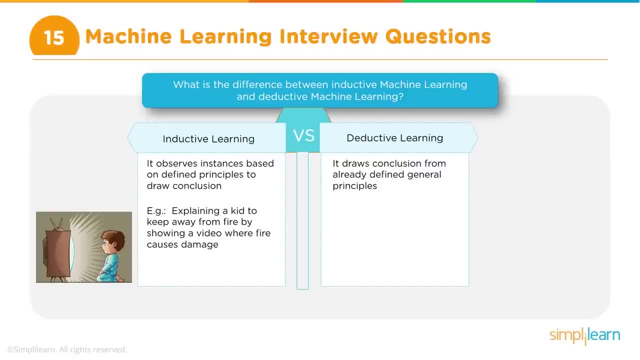 fire can cause damage. So this is inductive learning. Compared to that, what is deductive learning? So here you draw conclusion, or the person draws conclusion out of experience. So we will stick to the analogy. So, compared to the showing a video, let's assume a person is allowed. 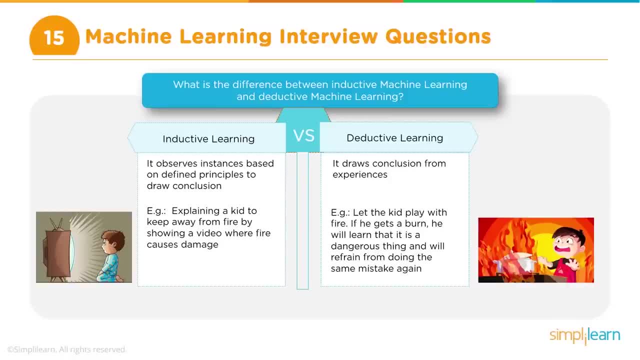 to play with fire, right, and then he figures out that if he puts his finger, it's burning, or if throw something into the fire, it burns. So he is learning through experience. So this is known as deductive learning. Okay, so you can have applications or models that can be trained. 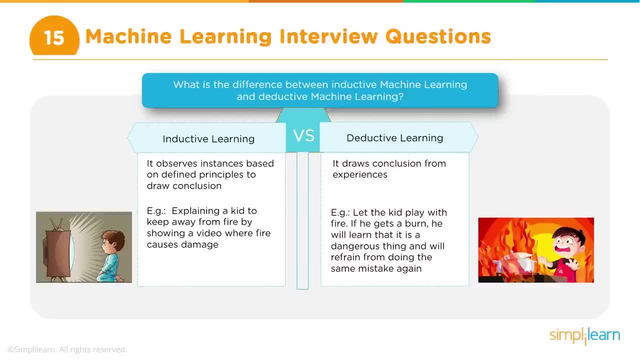 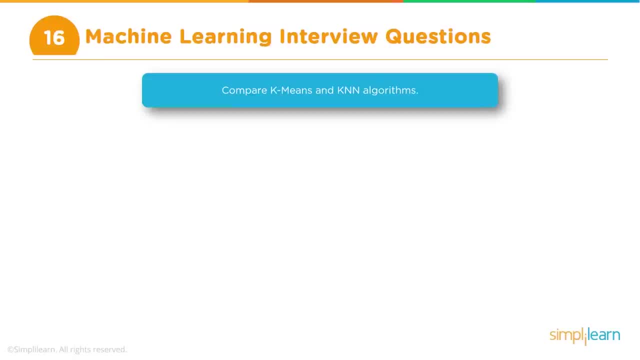 using inductive learning or deductive learning. All right, I think probably that explanation will be sufficient. The next question is: are KNN and K-means clustering similar to one another, or are they same, Right, because that the letter K is kind of common between them. Okay, so let us take a. 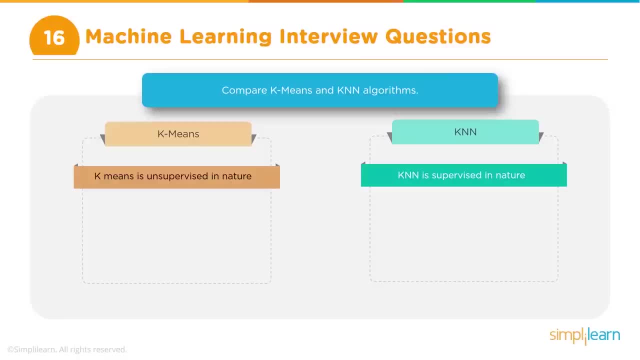 little while to understand what these two are. One is KNN, another is K-means. KNN stands for K- nearest neighbors- and K-means, of course, is the clustering mechanism. Now, these two are completely different, except for the letter K being common between them. KNN is completely different. K-means clustering is completely different. KNN is a. 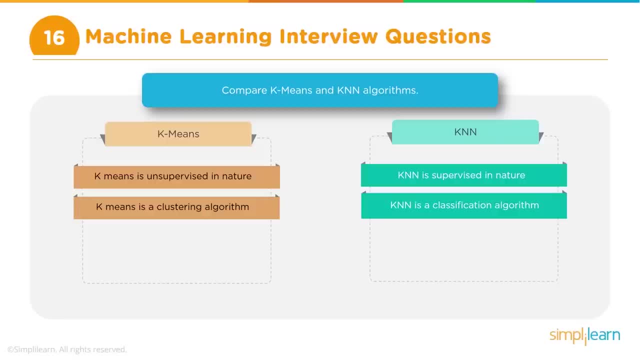 classification process and therefore it comes under supervised learning, whereas K-means clustering, is actually unsupervised. Okay, when you have KNN, when you want to implement KNN, which is basically K- nearest neighbors- the value of K is a number, So you can say K is equal to 3.. You want to implement KNN with? K is equal to 3.. So which? 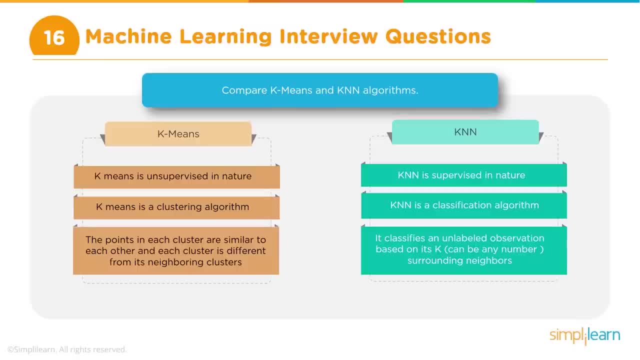 means that it performs the classification in such a way that: how does it perform the classification? So it will take three nearest objects and that is why it is called nearest neighbor. So basically, based on the distance, it will try to find out its nearest objects that are: 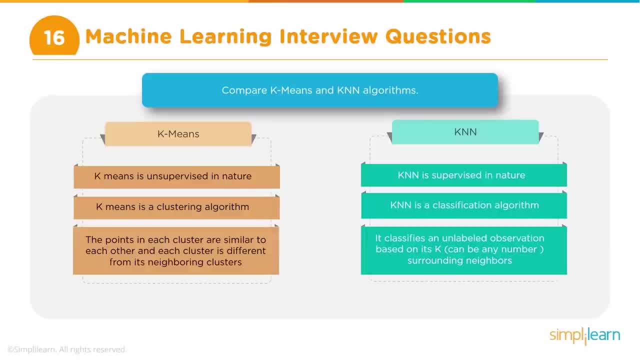 let us say three of the nearest objects and then it will check whether the class they belong to which class, right? So if all three belong to one particular class, obviously it will check whether this new object is also classified as that particular class. But it is possible that 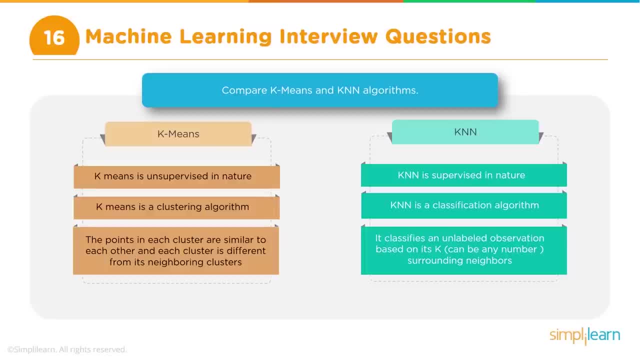 to 3.. You want to implement KNN with: K is equal to 3.. So, which means that it performs the classification in such a way that: how does it perform the classification? So it will take three nearest objects and that is why it is called nearest neighbor. So, basically, based on the distance, 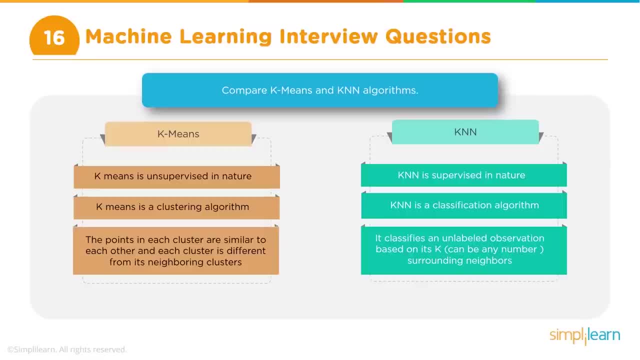 it will try to find out its nearest objects, that are, let us say, three of the nearest objects, and then it will check whether the class They belong to, which class, right? So if all three belong to one particular class, obviously this new object is also classified as that particular class. But it is possible that they may be from. 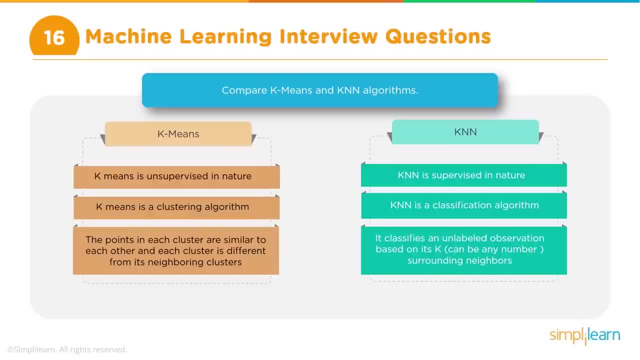 two or three different classes. Okay, So let us say they are from two classes, and then if they are from two classes- now usually you take an odd number, you assign an odd number to. So if there are three of them, and two of them belong to one class and then one belongs to another class, So 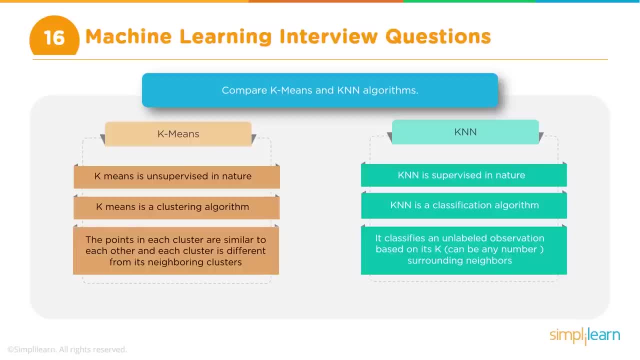 this new object is assigned to the class to which the Two of them belong. Now the value of K is sometimes tricky: whether should you use three? Should you use five? Should you use seven? That can be tricky because the ultimate classification can also vary. 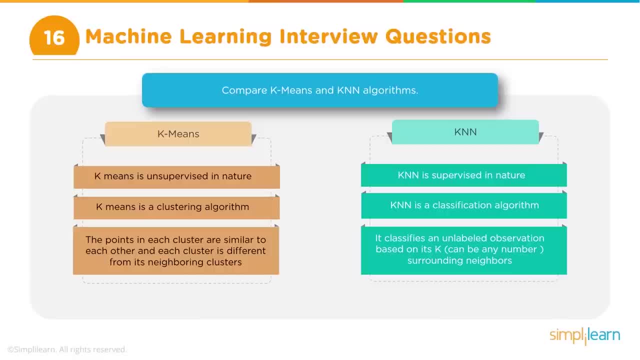 So it is possible that if you are taking K as three, the object is probably in one particular class. But if you take K is equal to five, maybe the object will belong to a different class, Because when you are taking three of them, probably two of them belong to class one and one. 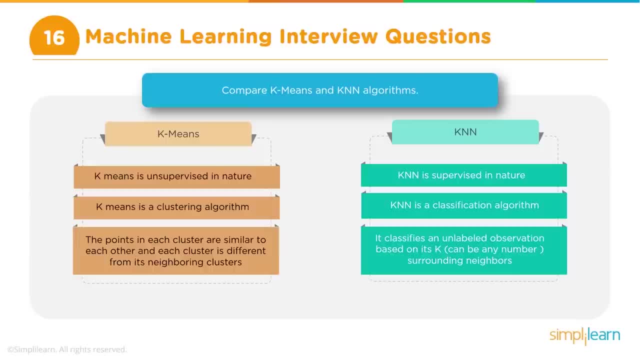 belong to class two, Whereas when you take five of them, it is possible that only two of them belong to class one and three of them belong to class two, So which means that this object will belong to class two, Right? So you see that? So it is. the class allocation can vary depending on the 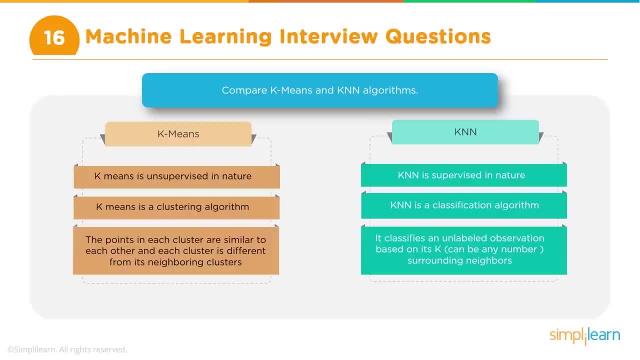 value of K. Now, K means, on the other hand, is a clustering process and it is unsupervised, where what it does is the system will basically identify how the objects are, How close objects are with respect to some of their original classes. These objects gets the judged. you know the region in a sense of relationships also. So 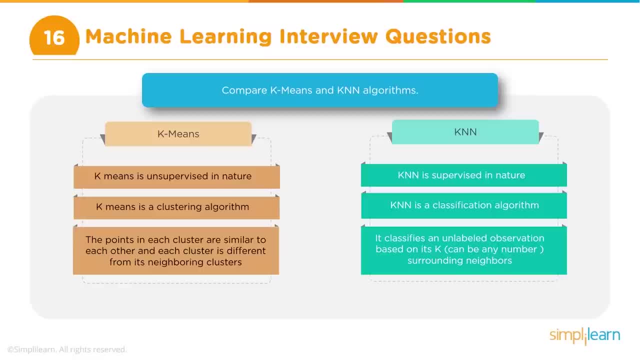 features. okay, and but the similarity, of course, is the letter k, and in case of k, means also we specify its value, and it could be 3 or 5 or 7. there is no technical limit as such, but it can be any number of clusters that you can create. okay, So, based on the value that you provide, 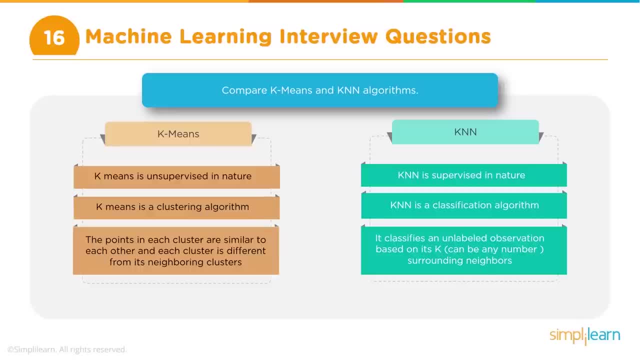 they may be from two or three different classes. Okay, so let us say they are from two classes and then if they are from two classes- now usually you take an odd number, you assign an odd number to. So if there are three of them, and two of them belong to one class and then one belongs to, 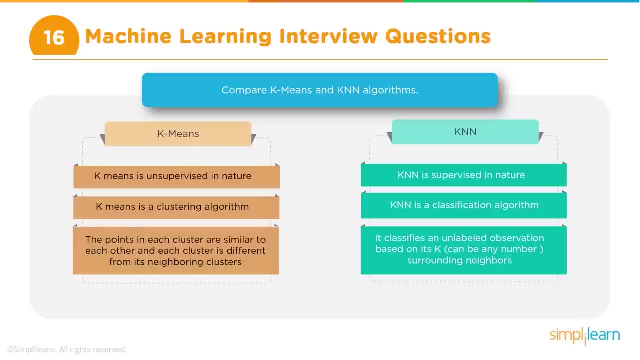 another class, So this new object is assigned to the class to which the two of them belong. Now the value of K is sometimes tricky: whether should you use three? should you use five? should you use seven? That can be tricky, because the ultimate 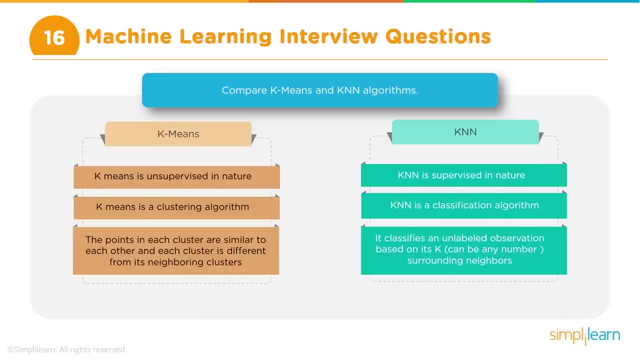 classification can also vary. So it is possible that if you are taking K as three, the object is probably in one particular class, But if you take K is equal to five, maybe the object will belong to a different class, Because when you are taking three of them, probably two of them belong to. 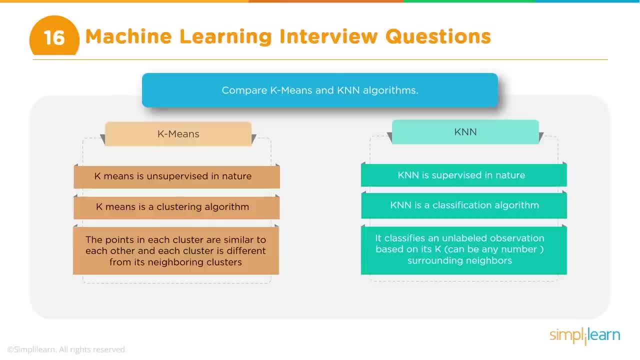 class one and one belong to class two, Whereas when you take five of them, it is possible that only two of them belong to class one and three of them belong to class two, So which means that this object will belong to class two, Right? so you see that? So it is. the class allocation can vary. 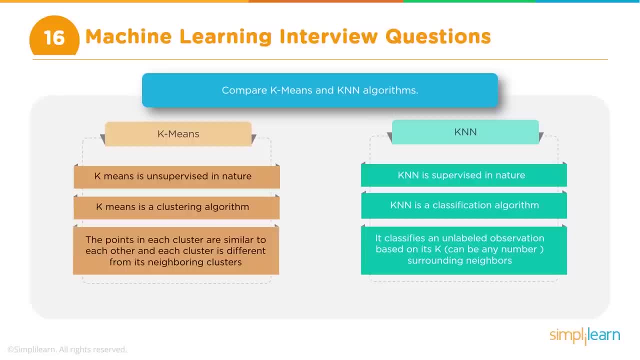 depending on the value of K. Now, K means, on the other hand, is a clustering process, and it is unsupervised, where what it does is the system will basically identify how the objects are, how close objects are with respect to some of their features. Okay, and? but the similarity, of course, is the. 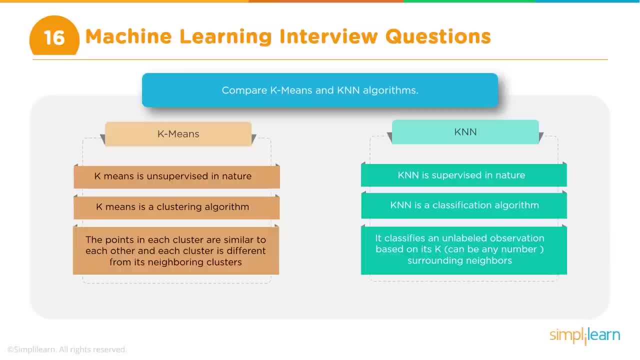 in case of K, means also, we specify its value, and it could be three or five or seven. There is no technical limit as such, but it can be any number of clusters that you can create. Okay, so based on the value that you provide, the system will create that many clusters of similar objects. So there is. 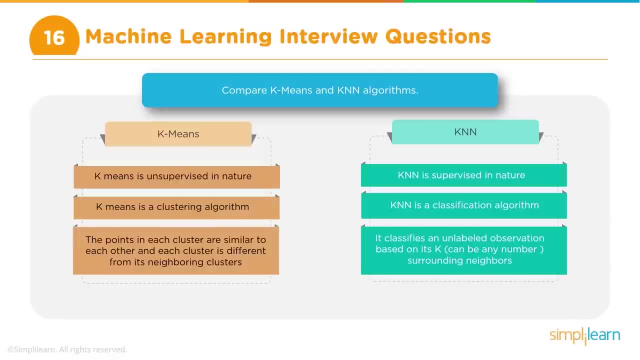 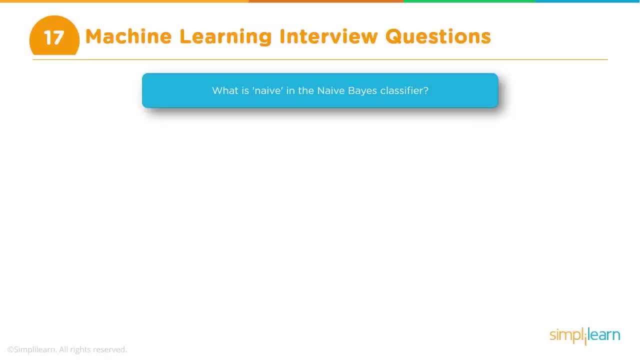 a similarity to that extent that K is a number in both the cases, but actually these two are completely different processes. We have what is known as naive base classifier, and people often get confused, thinking that naive base is the name of the person who found this classifier or who developed this classifier, which is not 100% true. Base is the name of the person. 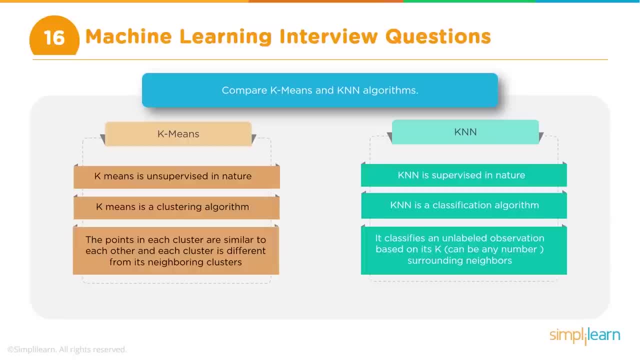 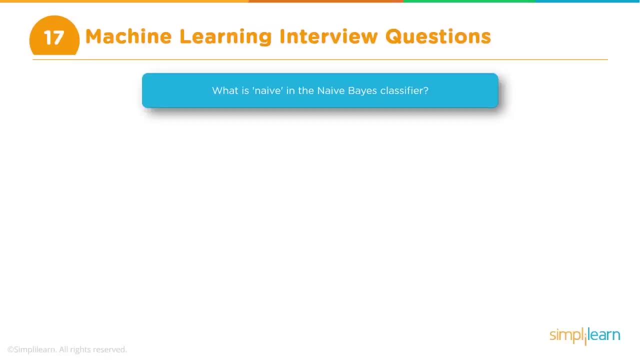 the system will create that many clusters of similar objects. So there is a similarity to that extent that k is a number in both the cases, but actually these two are completely different processes. We have what is known as Naive Bayes classifier, and people often get confused thinking. 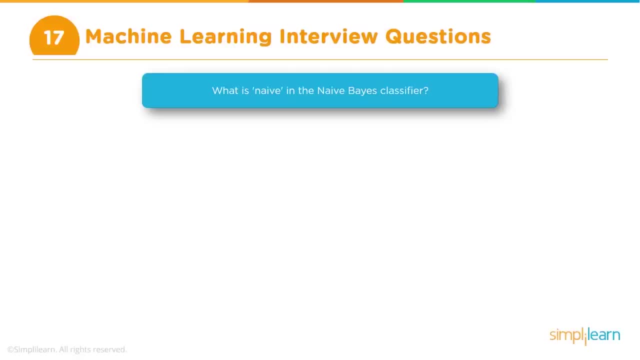 that Naive Bayes is the name of the person who found this classifier or who developed this classifier, which is not 100% true. Bayes is the name of the person, B-A-Y-E-S is the name of the person, but Naive is not the name of the person, right? So Naive is basically an English. 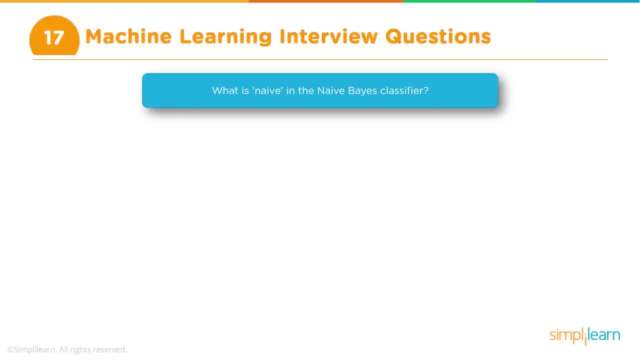 word that means Naive is the name of the person, So Naive is basically an English word that means- and that has been added here because of the nature of this particular classifier- Naive Bayes classifier is a probability based classifier and it makes some assumptions that presence of one. 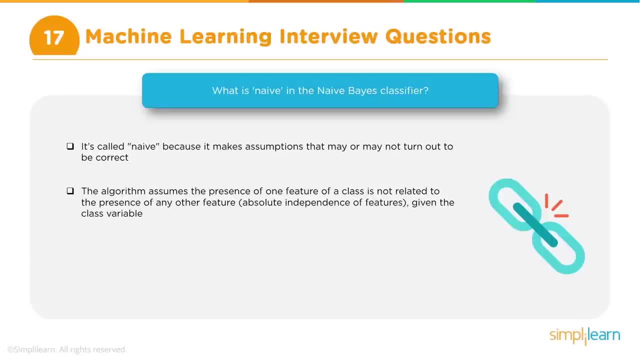 feature of a class is not related to the presence of any other feature of maybe other classes, right, So which is not a very strong or not a very, what do you say? accurate assumption, because these features can be related and so on. But even if we go with this assumption, this whole, 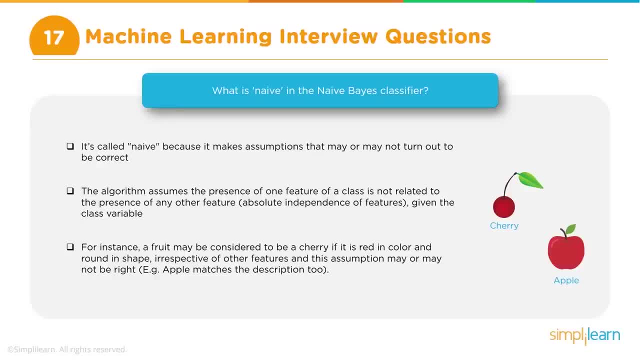 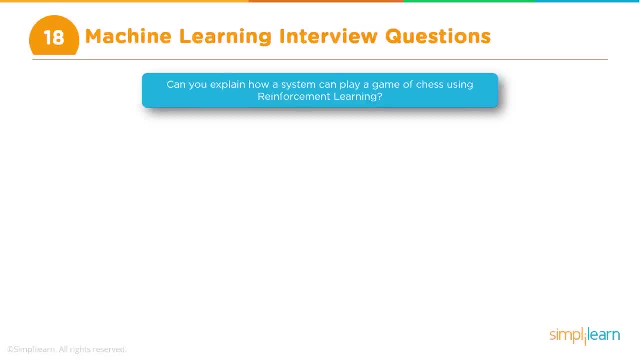 algorithm works very well even with this assumption, and that is the good side of it. but the term comes from there, So that is the explanation that you can. Then there can be question around reinforcement learning. It can be paraphrased in multiple ways. One could be: can. 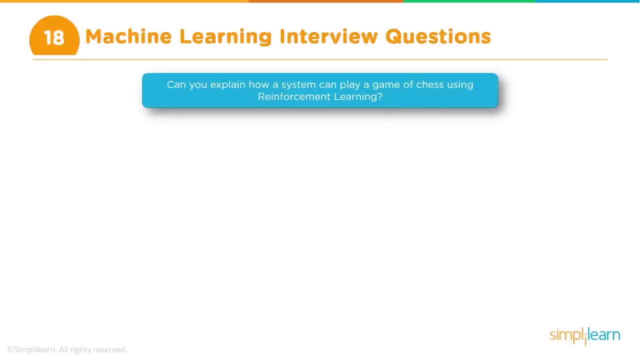 you explain how a system can play a game of chess using reinforcement learning, or it can be any game. So the best way to explain this is again to talk a little bit about what reinforcement learning is about and then allow me to explain. So the best way to explain this is again to talk a little bit. 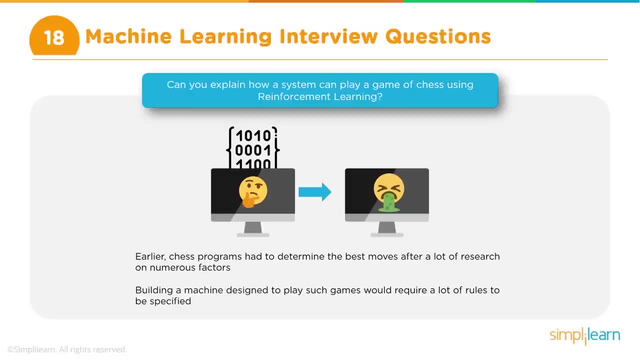 on that to explain the process. So, first of all, reinforcement learning has an environment and an agent, and the agent is basically performing some actions in order to achieve a certain goal, and these goals can be anything either. if it is related to game, then the goal could be that you 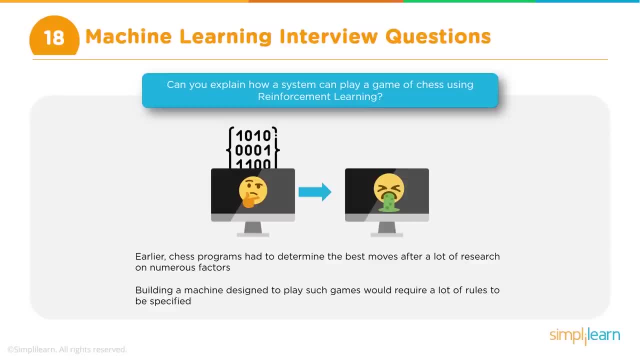 have to score very high. score a high value, high number. or it could be that your number of lives should be as high as possible. Don't lose life. So these could be some of them. More advanced examples could be for driving in the automotive. 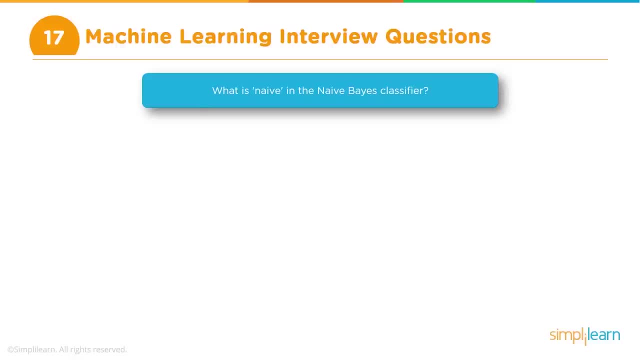 B A Y S is the name of the person, but naive is not the name of the person, Right? so naive is basically an English word and that has been added here because of the nature of this particular classifier. Naive base classifier is a probability based classifier. 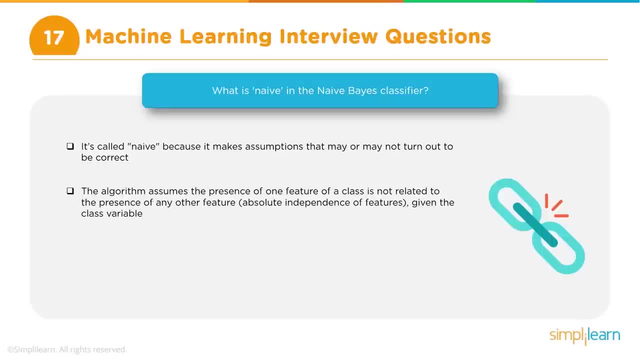 it makes some assumptions that presence of one feature of a class is not related to the presence of any other feature of maybe other classes. Right so, which is not very strong or not a very- what do you say? accurate assumption, because these features can be related and so on. But 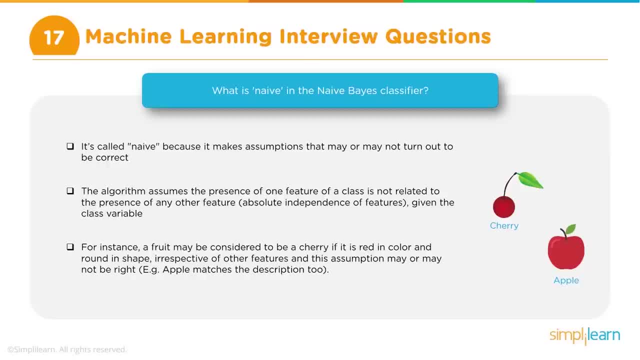 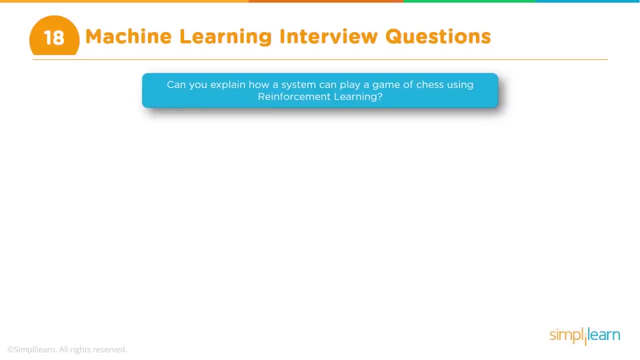 even if we go with this assumption, this whole algorithm works very well even with this assumption, and that is the good side of it. but the term comes from that, so that is the explanation that you can. There can be question around reinforcement learning. it can be paraphrased in multiple ways. 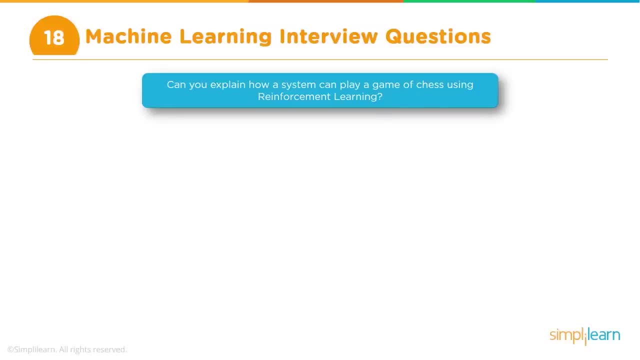 one could be. can you explain how a system can play a game of chess using reinforcement learning, or it can be any game. So the best way to explain this is again to talk a little bit about what reinforcement learning is about and then elaborate on that to explain the process. So first of all, 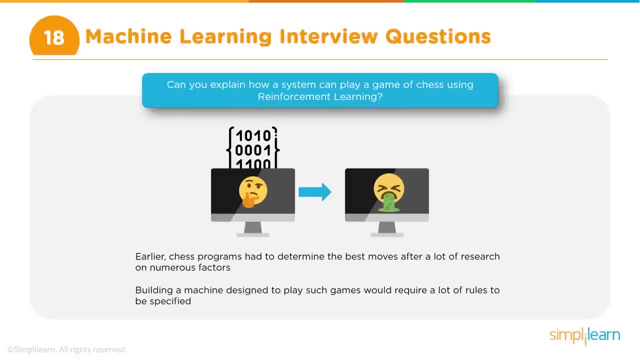 reinforcement learning has an environment and an agent, and the agent is basically performing some tasks in order to achieve a certain goal, and these goals can be anything either. if it is related to game, then the goal could be that you have to score very high score a high value, high number. 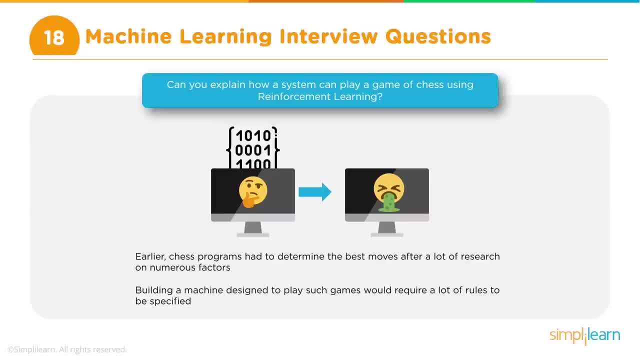 or it could be that your number of lives should be as high as possible. don't lose life. so these could be some of them. A more advanced examples could be for driving in the automotive industry: self-driving cars. they actually also make use of reinforcement learning to. 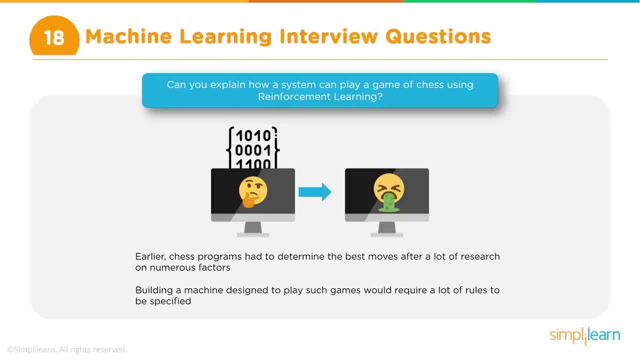 manage the car, how to navigate through the roads, and so on and so forth. that is also another example. Now, how does it work? so if the system is basically there is an agent and environment, and every time the agent takes a step or performs a task which is taking it towards the goal, the 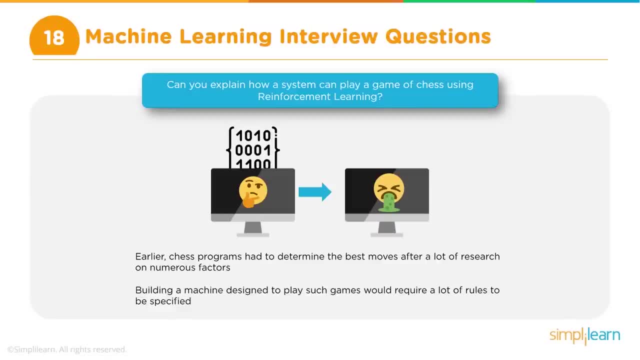 final goal, let's say to maximize the score or to minimize the number of lives and so on, or minimize the debts, for example, it is rewarded. and every time it takes a step which goes against that goal, contrary or in the reverse direction, it is penalized. okay, so it is like a carrot and 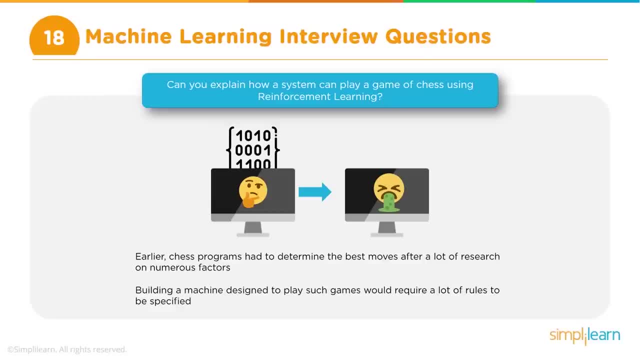 industry: self-driving cars. They actually also make use of reinforcement learning to teach the car how to navigate through the roads, and so on and so forth. That is also another example. Now, how does it work? So if the system is basically there is an agent and environment, and every time 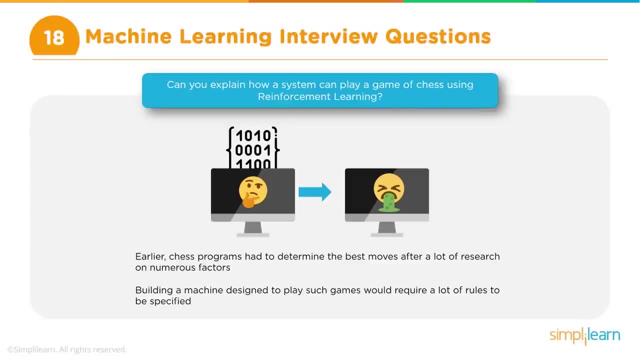 the agent takes a step or performs a task which is taking it towards the goal, the final goal, let's say to maximize the score, Or to minimize the number of lives and so on, or minimize the deaths, for example, It is rewarded. and every time it takes a step which goes against that goal and contrary or in the reverse direction, 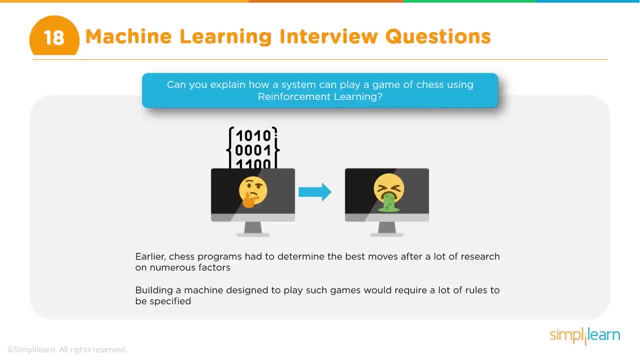 it is penalized, So it is like a carrot and stick system. Now, how do you use this to create a game of chess, or to create a system to play a game of chess? Now, the way this works is, and this could: 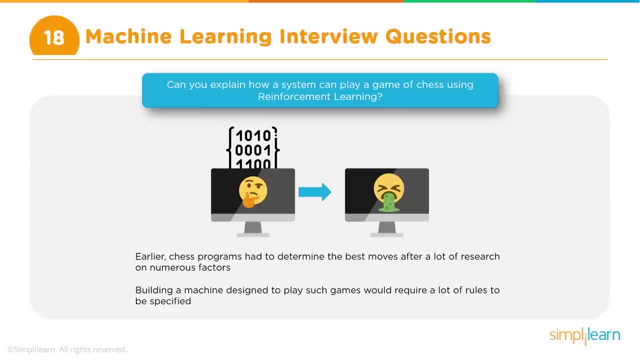 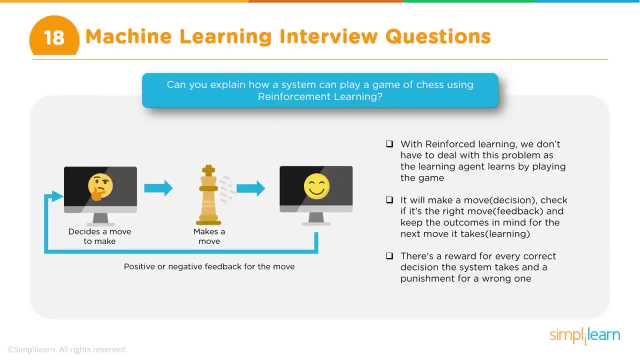 probably go back to this AlphaGo example, where AlphaGo defeated a human champion. So the way it works is in reinforcement learning. The system is allowed, for example, in this case we are talking about chess, So we allow the system to first of all watch playing a game of chess. So 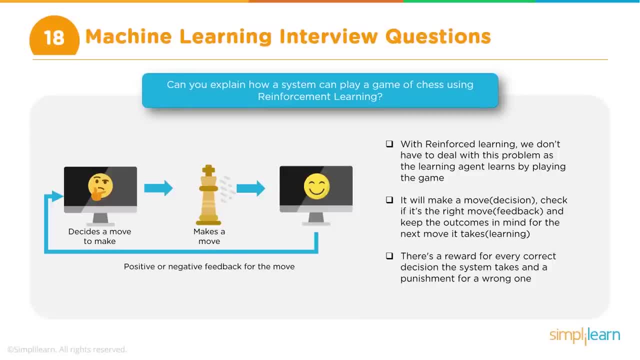 it could be with a human being or it could be the system itself. There are computer games of chess, right. So either this new learning system has to watch that game or watch a human being play the game, because this is reinforcement learning, So it is like a game of chess. So it is like a game of 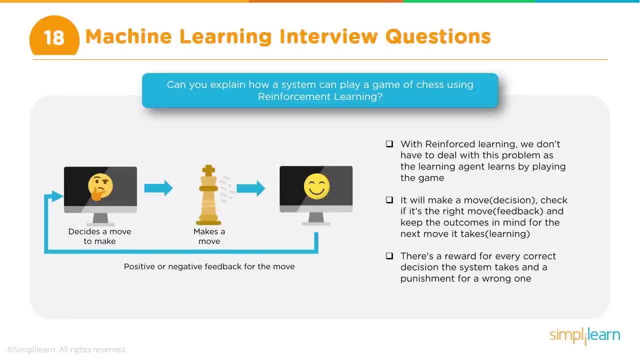 chess. So reinforcement learning is pretty much all visual. So when you are teaching the system to play a game, the system will not actually go behind the scenes to understand the logic of your software, of this game or anything like that. It is just visually watching the screen and then 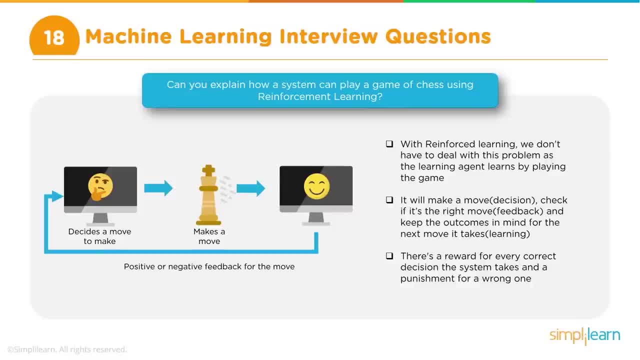 it learns. Okay, So reinforcement learning to a large extent works on that. So you need to create a mechanism whereby your model will be able to watch somebody playing the game and then you allow the system also to start playing the game, So it pretty much starts from scratch, Okay, And 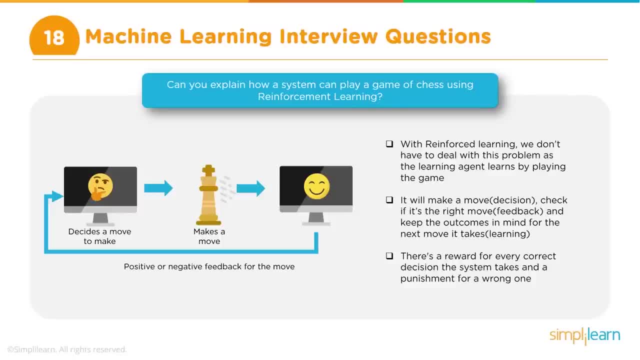 as it moves forward, it is like, right at the beginning, the system really knows nothing about the game of chess. Okay, So initially it is a clean slate. It just starts by observing how you are playing, So it will make some random moves and keep losing badly. But then what happens is: 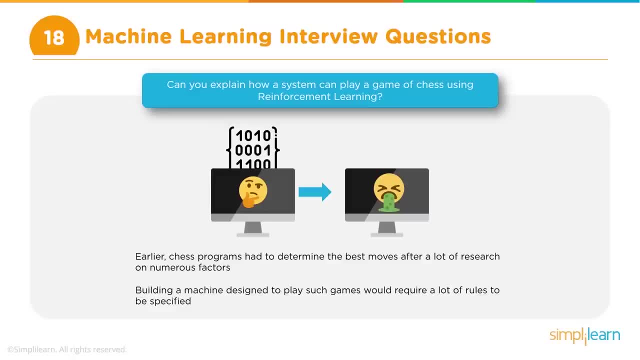 stick system. now, how do you use this to create a game of chess or to create a system to play a game of chess? now, the way this works is- and this could probably go back to this AlphaGo example- where AlphaGo defeated a human champion- so the way it works is in reinforcement learning. the 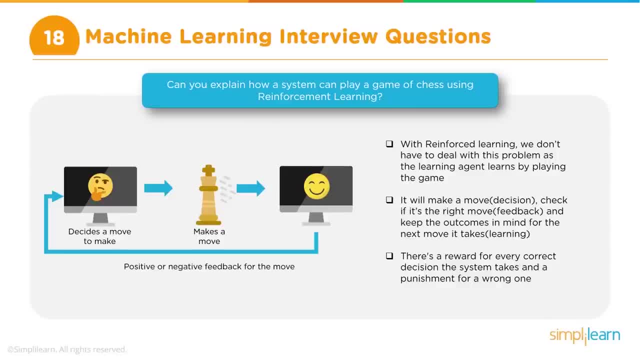 system is allowed. for example, if in this case, we are talking about chess, so we allow the system to first of all watch playing a game of chess, so it could be with a human being, or it could be the system itself. there are computer games of chess, right. so either this new learning system, 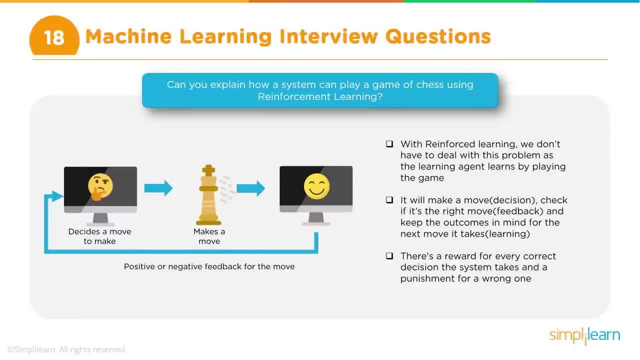 has to watch that game or watch a human being play the game, because this is reinforcement. learning is pretty much all visual. so when you are teaching the system to play a game, the system will not actually go behind the scenes to understand the logic of your play of this game or anything like that. it is just visually watching the screen and then it. 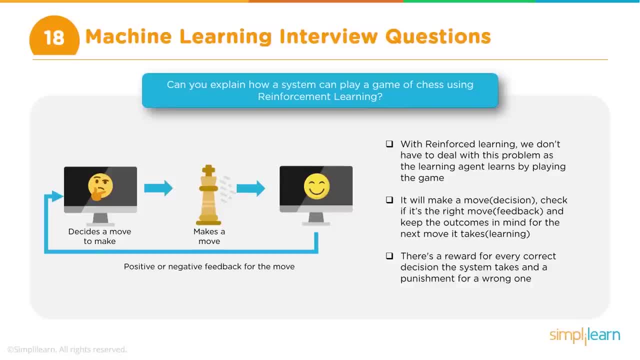 learns, okay. so reinforcement learning to a large extent works on that. so you need to create a mechanism whereby your model will be able to watch somebody playing the game and then you allow the system also to start playing the game. so it pretty much starts from scratch, okay, and as it moves forward it it's like right at the beginning the 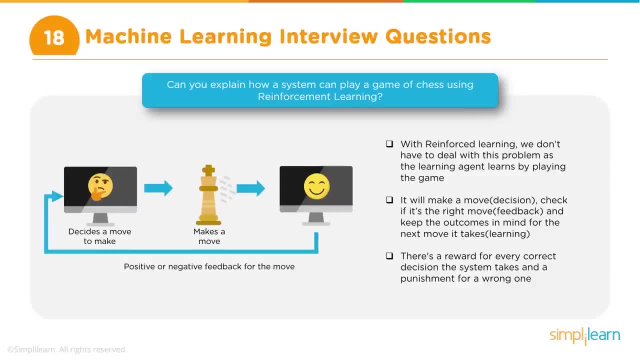 system really knows nothing about the game of chess. okay, so initially it is a clean slate. it just starts by observing how you're playing, so it will make some random moves and keep losing badly, but then what happens is over a period of time. so you need to now allow the system or you need 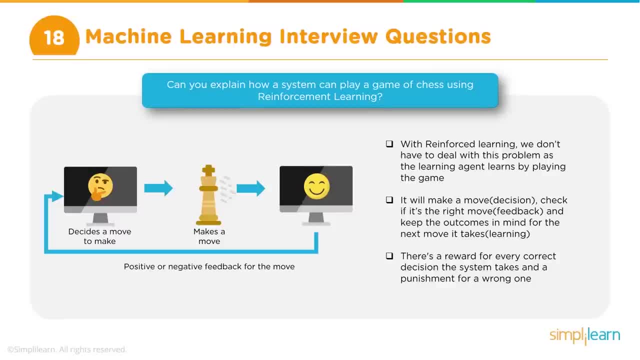 to play with the system, not just one, two, three, four or five times, but hundreds of times, thousands of times, maybe even hundreds of thousands of times. and that's what reinforcement learning is all about. exactly how alpha go has done: it played millions of games between itself and the system, right so? 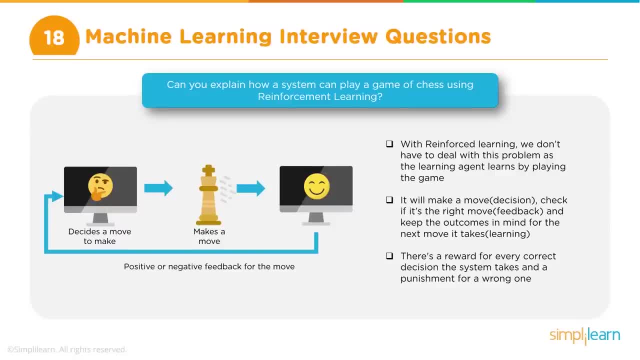 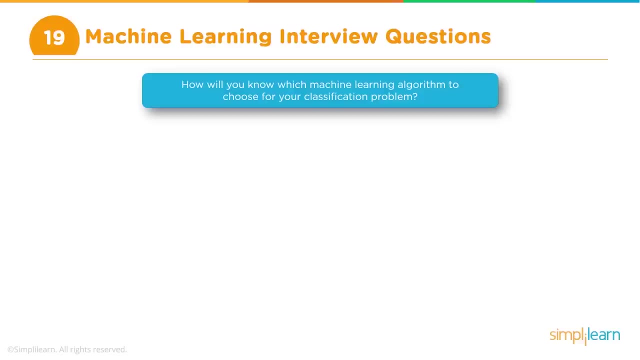 for the game of chess also. you need to do something like that. you need to allow the system to play chess and then learn on its own over a period of repetition. so i think you can probably explain it to this much to this extent, and it should be sufficient. now this is another question which is 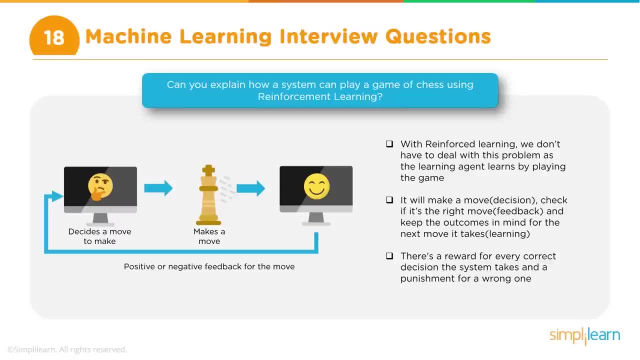 over a period of time. So you need to now allow the system or the system to start playing the game. You need to play with the system not just one, two, three, four or five times, but hundreds of times, thousands of times, maybe even hundreds of thousands of times. And that is exactly how. 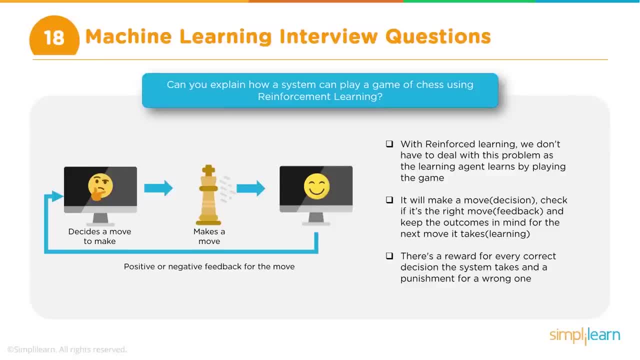 AlphaGo has done. It played millions of games between itself and the system Right. So for the game of chess also, you need to do something like that. You need to allow the system to play chess and then learn on its own over a period of repetition. So I think you can probably explain. 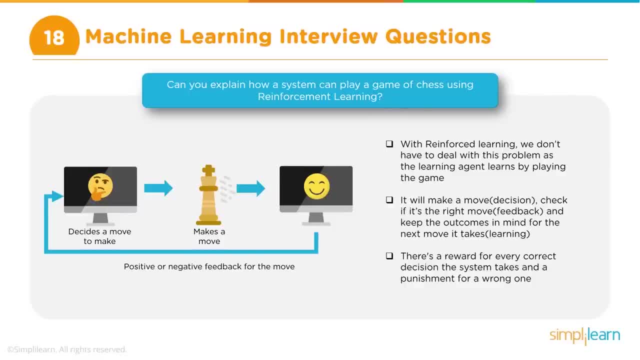 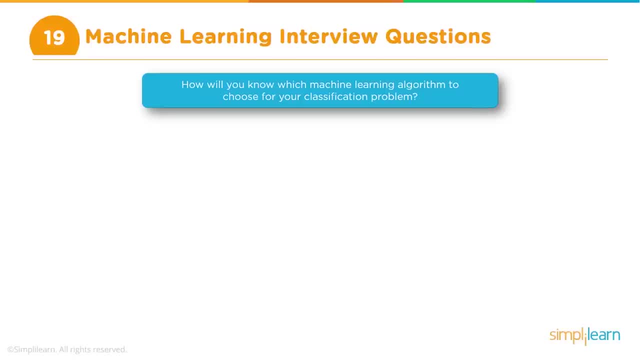 it to this extent, and it should be sufficient. Now this is another question which is again somewhat similar, but here the size is not coming into picture. So the question is: how will you know which machine learning algorithm to choose for your classification problem? Now, this is not. 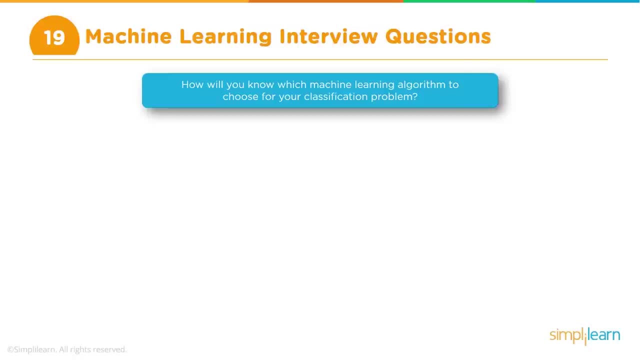 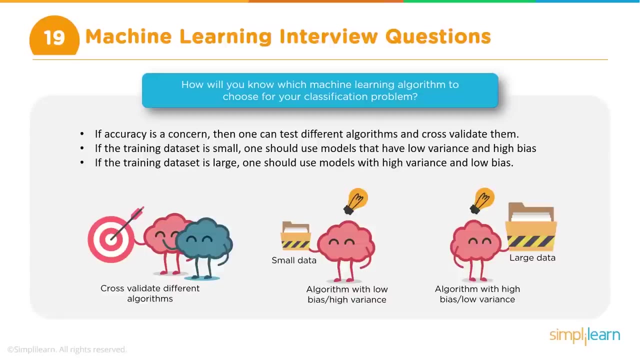 only classification problem. It could be a regression problem. I would like to generalize this question. So if somebody asks you: how will you choose? How will you know which algorithm to use? The simple answer is: there is no way you can decide exactly, saying that this is the algorithm. 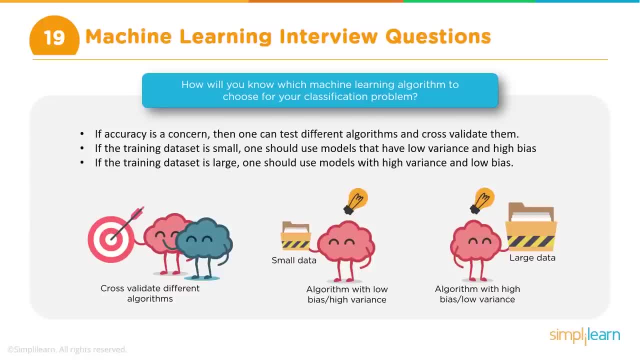 I am going to use in a variety of situations. There are some guidelines like, for example: you will obviously, depending on the problem, you can say whether it is a classification problem or a regression problem and then, in that sense, you are kind of restricting yourself to if it is a. 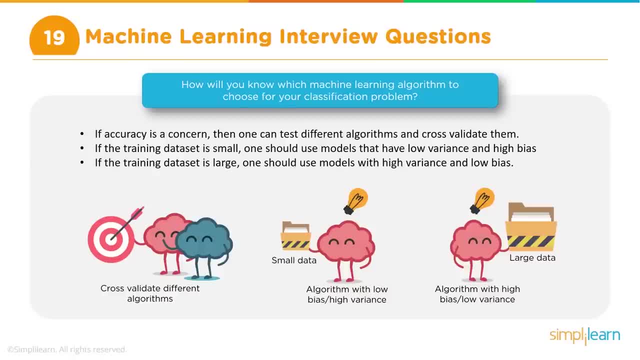 classification problem there are. you can only apply a classification algorithm right To that extent. you can probably, let's say, limit the number of algorithms. but now, within the classification problem, you have decision trees, you have SPM, you have logistic regression. Is it possible to? 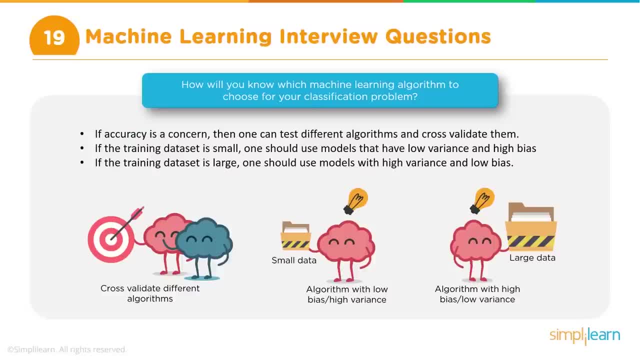 outright say yes. So for this particular problem, since you have explained this, now, this is the exact algorithm that you can use. that is not possible, okay? So you have to try out a bunch of algorithms, see which one gives us the best performance and best accuracy, and then decide to. 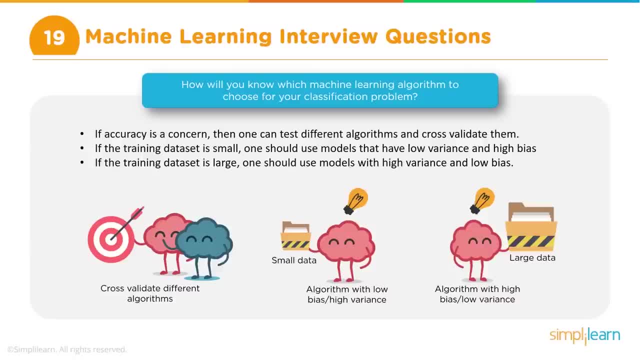 go with that particular algorithm. So in machine learning a lot of it happens through trial and error. There is a no real possibility that anybody can, just by looking at the problem or understanding the problem, tell you that, okay, in this particular situation this is exactly the algorithm that. 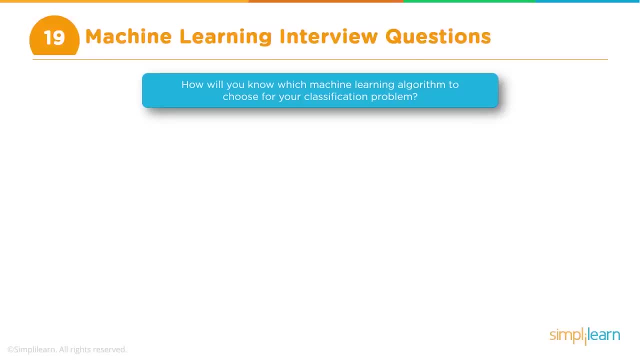 again somewhat similar, but here the size is not coming into picture. the question is: how will you know which machine learning algorithm to choose for your classification problem? now, this is not only classification problem. it could be a regression problem. i would like to generalize this question. so if somebody asks you, how will you choose, how will 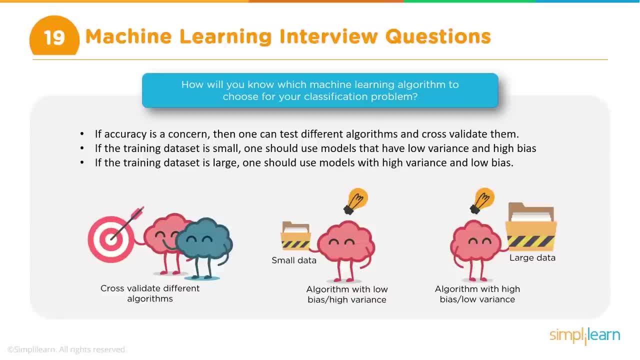 you know which algorithm to use? the simple answer is: there is no way you can decide exactly saying that this is the algorithm i'm going to use in a variety of situations. there are some guidelines like, for example: you will obviously, depending on the problem, you can say: 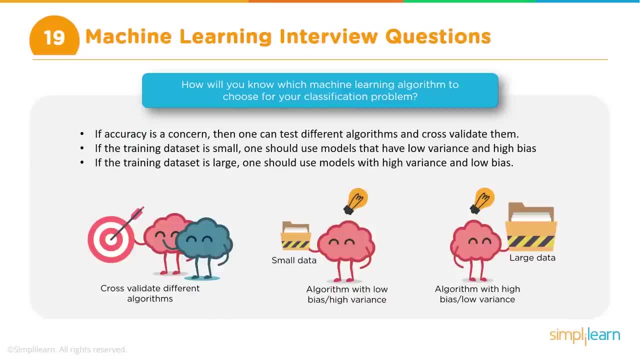 it is a classification problem or a regression problem and then in that sense you are kind of restricting yourself to if it is a classification problem there are, you can only apply a classification algorithm right to that extent you can probably, let's say, limit the number of algorithms. but 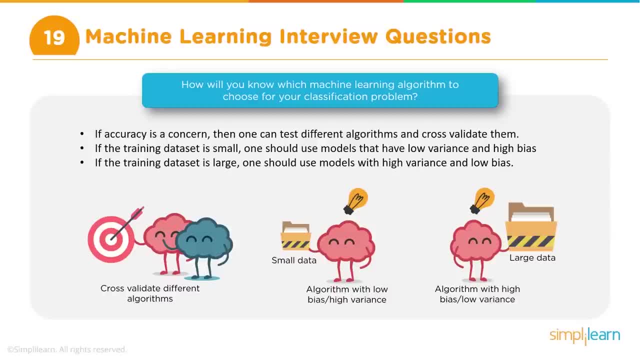 now, within the classification algorithms, you have decision trees, you have svm, you have logistic regression. is it possible to outright say yes, so for this particular problem, since you have explained that this is the exact algorithm that you can use? that is not possible, okay, so you have to try out. 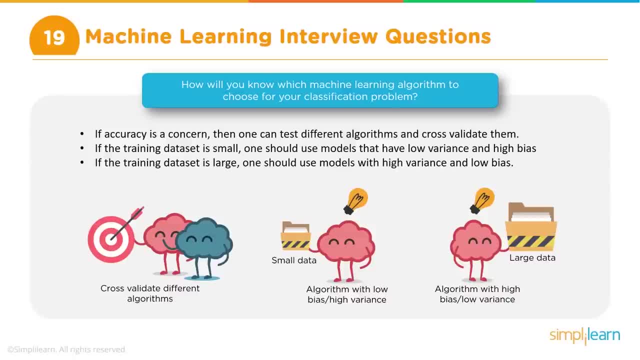 a bunch of algorithms, see which one gives us the best performance and best accuracy and then decide to go with that particular algorithm. so in machine learning a lot of it happens through trial and error. there is no real possibility that anybody can just by looking at the problem or understanding. 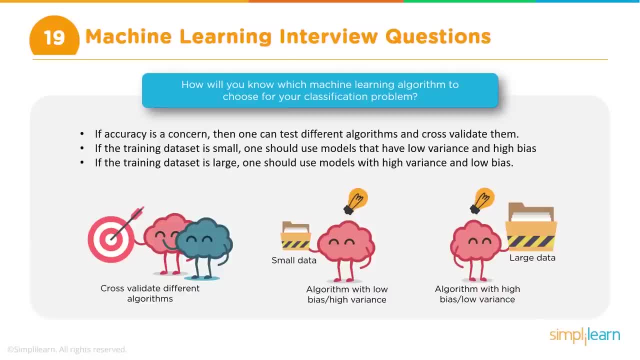 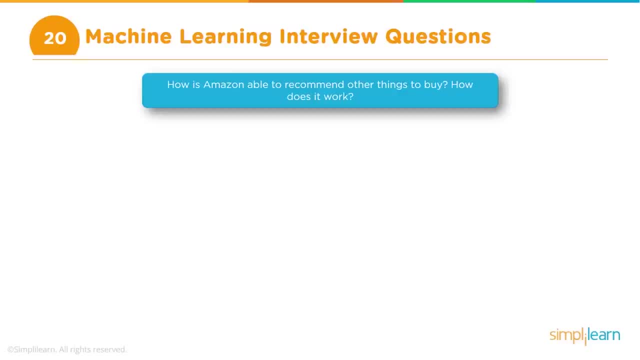 the problem tell you that, okay, in this particular situation, this is exactly the algorithm that you use, then the questions may be around application of machine learning, and this question is specifically around how amazon is able to recommend other things to buy. so this is around recommendation engine. how does it work? how does the recommendation engine work? so this is basically the question is: 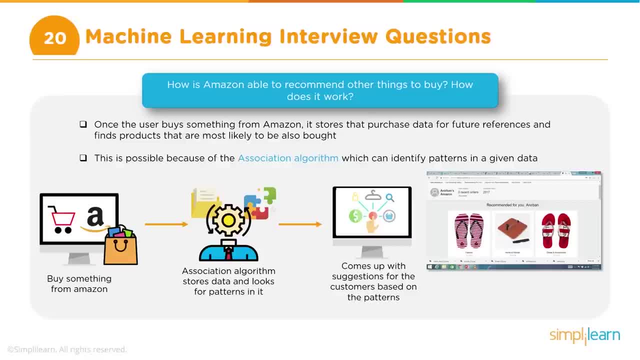 all about. so the recommendation engine again works based on various inputs that are provided. obviously, something like: uh, you know, amazon on a website or e-commerce site like amazon collects a lot of data around the customer behavior- who is purchasing what, and if somebody is buying a particular thing, they're also buying something else. so this kind of association right. so this: 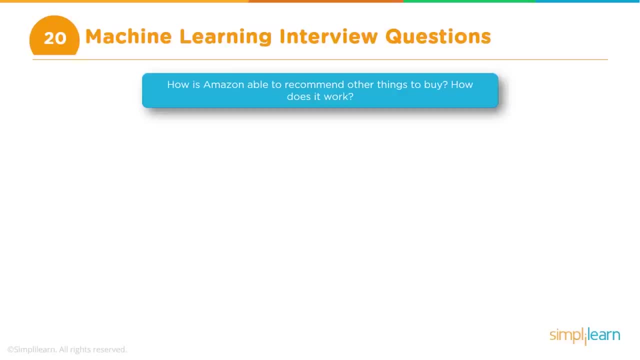 you should use. Then the questions may be around application of machine learning, and this question is specifically around how Amazon is able to recommend other things to buy. So this is around recommendation engine: How does it work? How does the recommendation engine work? So this is. 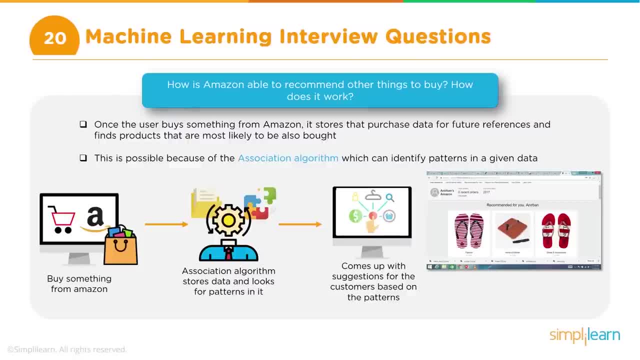 basically the question is all about. So the recommendation engine again works based on various inputs that are provided. Obviously, something like, you know, Amazon on a website or e-commerce site like Amazon collects a lot of data around the customer behavior. Who? 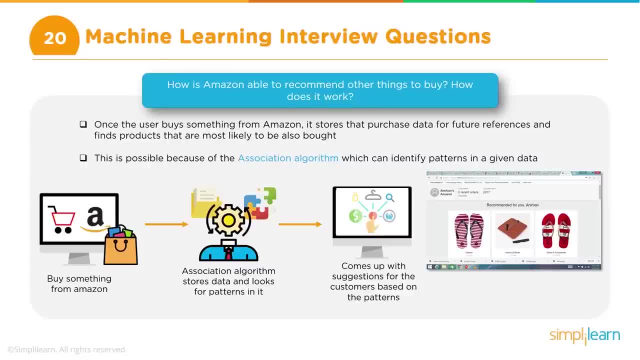 is purchasing what, and if somebody is buying a particular thing, they are also buying something else. So this kind of association- right, So this is the unsupervised learning we talked about. They use this to associate and link or relate items, and that is one part of it. So they 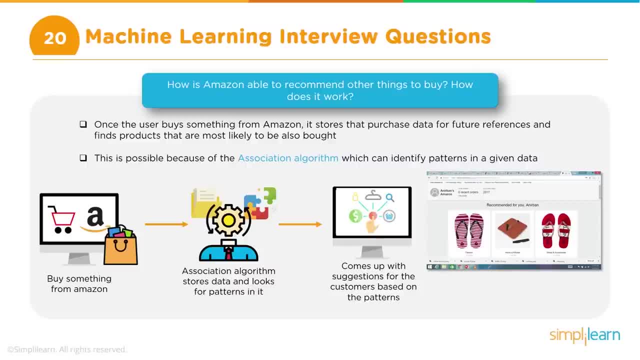 kind of build association between items, saying that somebody buying this is also buying this. That is one part of it. Then they also profile the users right Based on their age, their gender, their geographic location. they will do some profiling and then, when somebody is logging in, 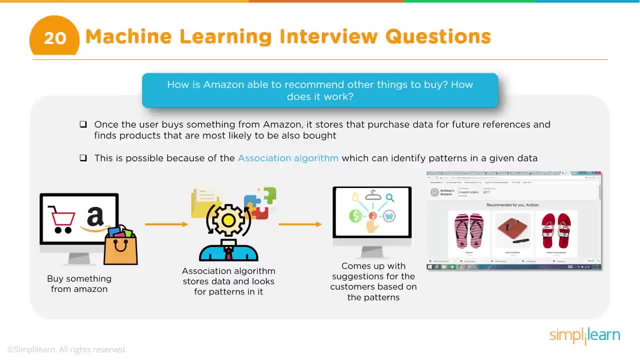 and when somebody is shopping, kind of the mapping of these two things are done. They try to identify. obviously, if you have logged in, then they know who you are and your information is available, Like, for example, your age, maybe Your gender, and where you are located, what you purchased earlier, right, So all this is taken. 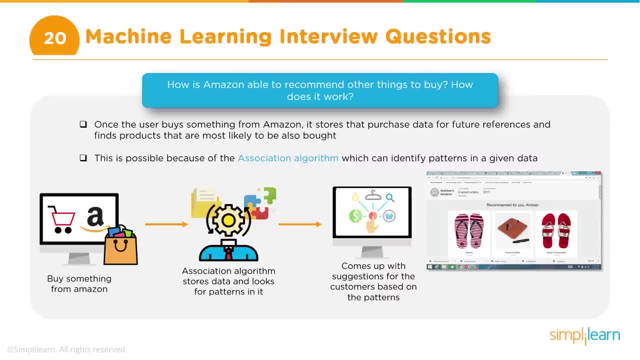 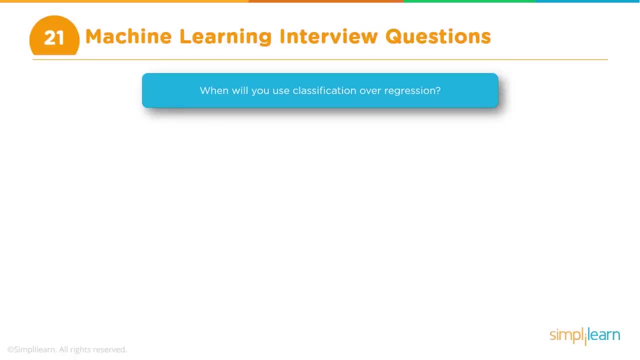 and the recommendation engine basically uses all this information and comes up with recommendations for a particular user. So that is how the recommendation engine works. Alright, then the question can be something very basic like: when will you go for classification versus regression, right? When do you do classification instead of regression, or? 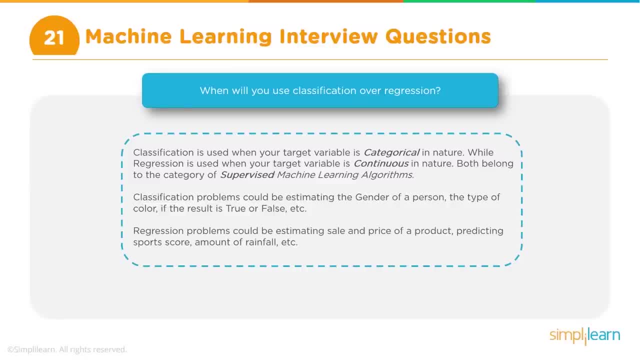 we use classification instead of regression. Now, yes, so this is basically going back to the understanding of the basics of classification and regression. So classification is used when you have to identify or categorize things into discrete classes. So the best way to respond to. 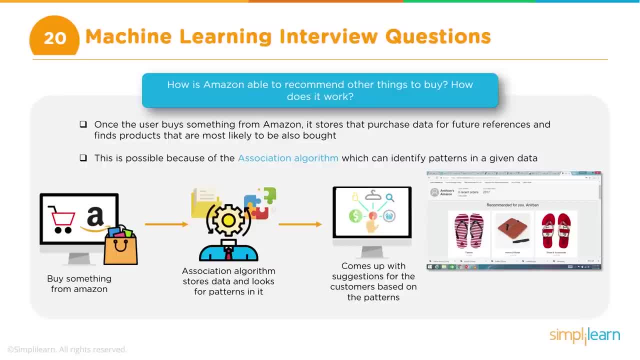 is the unsupervised learning we talked about. they use this to associate and link or relate items, and that is one part of it. so they kind of build association between items, saying that somebody buying this is also buying this. that is one part of it. then they also profile the users right based. 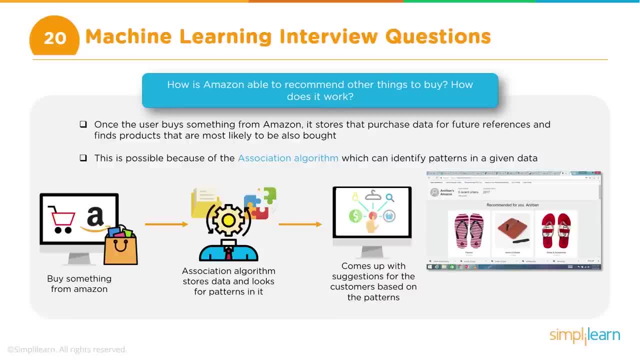 their gender, their geographic location. they will do some profiling and then when somebody is logging in and when somebody is shopping, kind of the mapping of these two things are done- they try to identify. obviously, if you have logged in, then they know who you are and your information is. 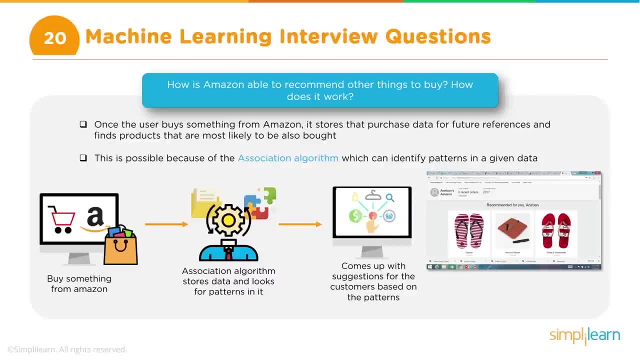 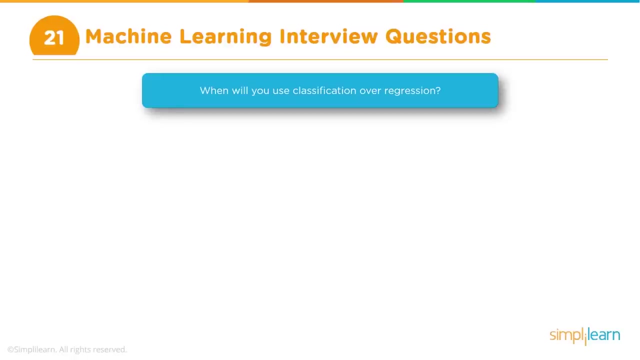 available like, for example, your age may be, your gender and where you're located, what you purchased earlier. right? so all this is taken and the recommendation engine basically uses all this information and comes up with recommendations for a particular user. so that is how the recommendation engine works, all right, then the question can be something very basic like: 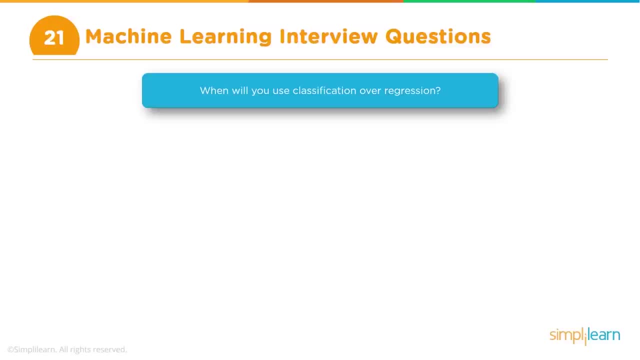 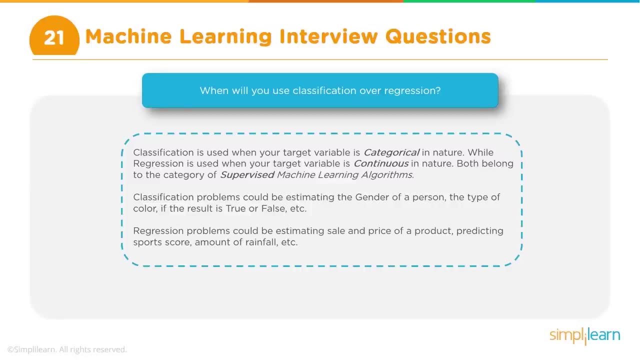 when will you go for classification versus regression? right? when do you do classification instead of regression? or when will you use classification instead of regression? now, yes, so. so this is basically going back to the understanding of the basics of classification and regression. so when you use the definition of classification, you have to identify or categorize things into. 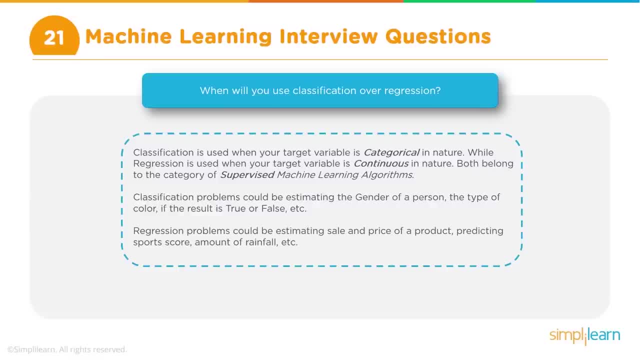 discrete classes. so the best way to respond to this question is to take up some examples and use it, otherwise it can become a little tricky. the question may sound very simple, but explaining it can sometimes be very tricky. in case of regression we use, of course there will be some keywords that 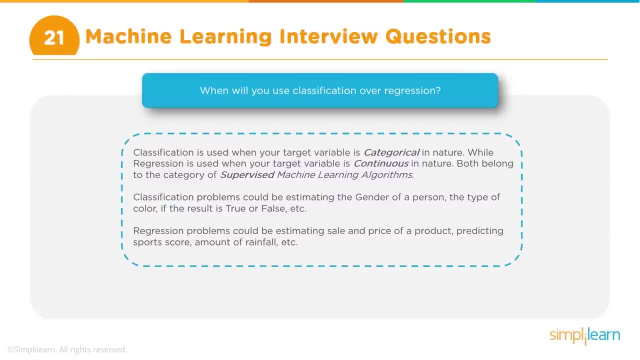 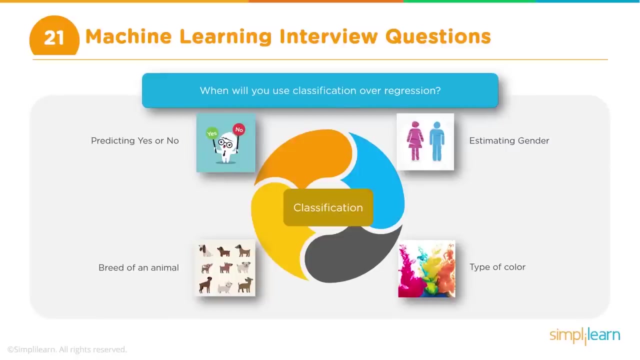 they will be looking for. so just you need to make sure you use those keywords. one is the discrete values and other is the continuous values. so for regression, to find some continuous values, you use regression, Whereas if you're trying to find some discrete values you use classification. And then you need to illustrate what are some of the examples. So 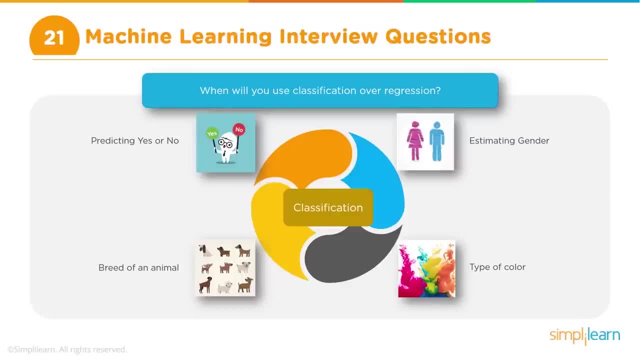 classification is like, let's say, there are images and you need to put them into classes like cat, dog, elephant, tiger, something like that. So that is a classification problem, Or it can be that is a multi-class classification problem. It could be binary classification problem, Like for. 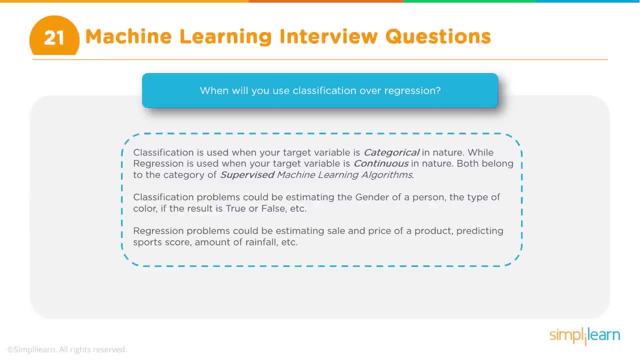 this question is to take up some examples and use it. Otherwise it can become a little tricky. The question may sound very simple, but explaining it can sometimes be very tricky. In case of regression we use, of course there will be some keywords that they will be looking for. So it's 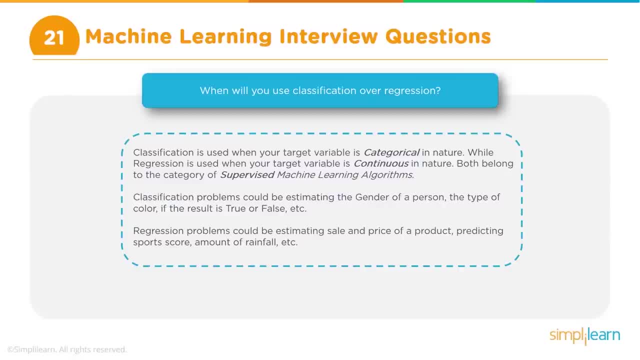 just you need to make sure you use those keywords. One is the discrete values, another is the continuous values. So for regression, if you are trying to find some continuous values, you use regression, Whereas if you're trying to find some discrete values, you use classification And then 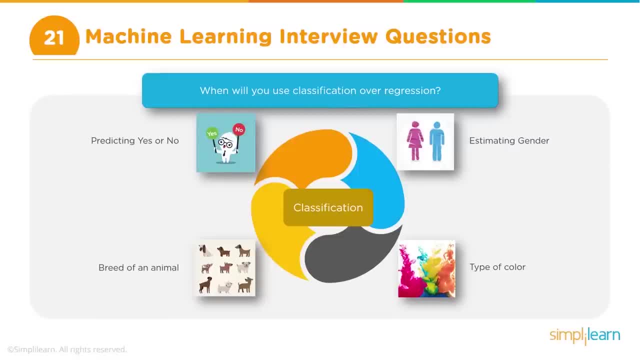 you need to illustrate what are some of the examples. So classification is like, let's say, there are images and you need to put them into classes, like cat, dog, elephant, tiger, something like that. So that is a classification problem, Or it can be that is a. 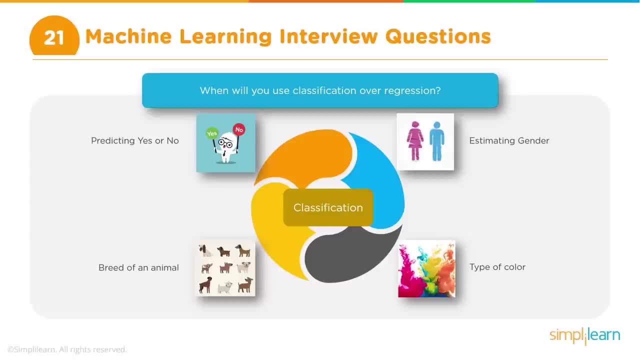 multi-class classification problem. It could be binary classification problem, like, for example, whether a customer will buy or he will not buy. That is a classification, binary classification. It can be in the weather forecast area. Now weather forecast is again a combination of. 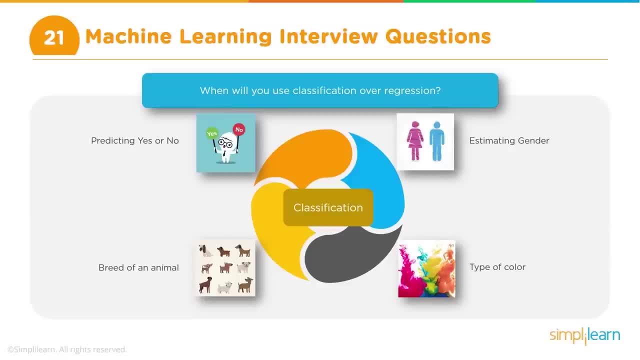 regression and classification, because, on the one hand, you want to predict whether it's going to rain or not. That's a classification. It's a binary classification, right, Whether it's going to rain or not rain. However, you also have to predict what is going to be the temperature tomorrow. right Now, temperature is a continuous. 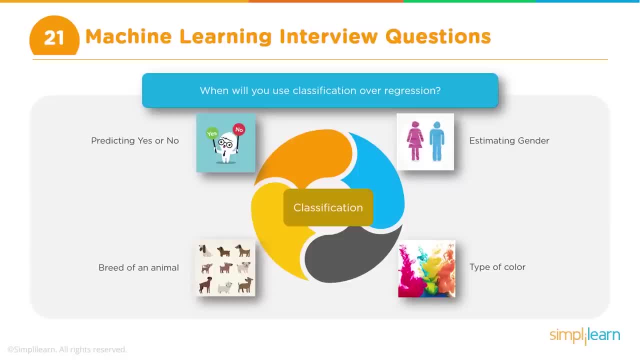 value. You can't answer the temperature in a yes or no kind of a response, right? So what will be the temperature tomorrow? So you need to give a number which can be like 20 degrees, 30 degrees or whatever, right? So that is where you use regression. One more example is stock price. 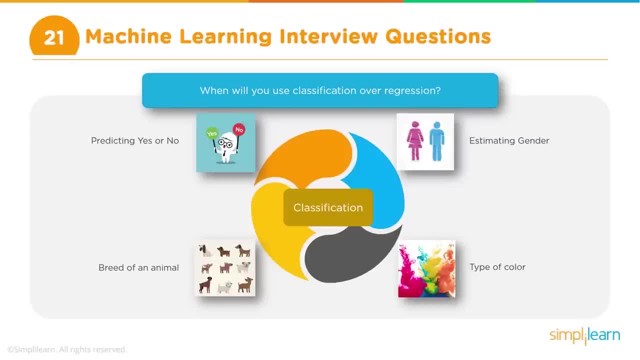 prediction. So that is where again, you will use regression. So these are the various examples. So you need to illustrate with examples and make sure you include those keywords like discrete and continuous. So the next question is more about a little bit of a design. related question to: 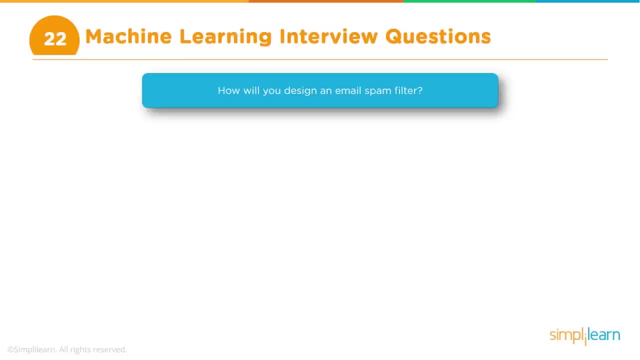 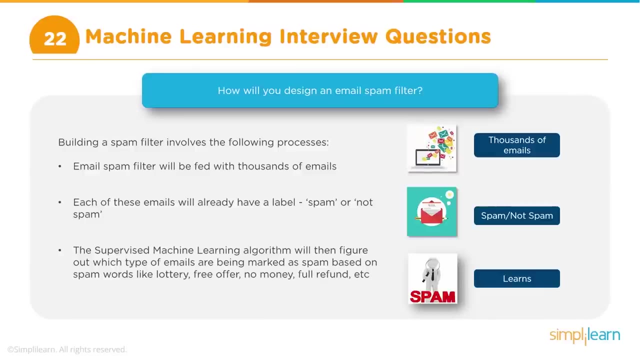 understand your concepts and things like that. So it is: how will you design a spam filter? So how do you basically design or develop a spam filter? So I think the main thing here is he's looking at probably understanding your concepts in terms of what is the algorithm you will use. 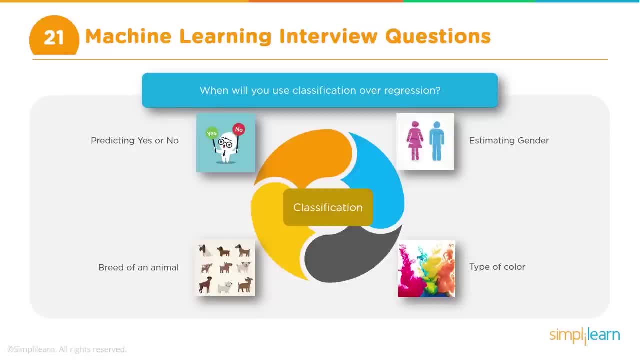 example, whether a customer will buy or he will not buy. That is a classification, binary classification. It can be in the weather forecast area. Now weather forecast is again combination of regression and classification, Because on the one hand you want to predict whether it's going. 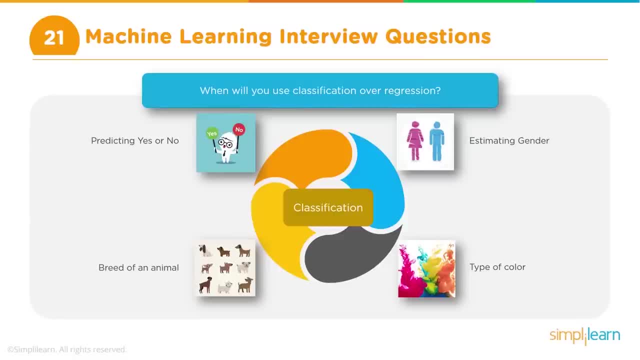 to rain or not. That's a classification problem. That's a binary classification, right, Whether it's going to rain or not rain. However, you also have to predict what is going to be the temperature tomorrow. right Now, temperature is a continuous value. 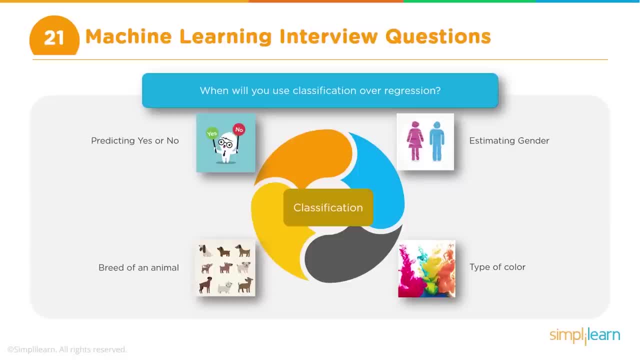 You can't answer the temperature in a yes or no kind of a response, right? So what will be the temperature tomorrow? So you need to give a number which can be like 20 degrees, 30 degrees or whatever, right? So that is where you use regression. One more example is stock price. 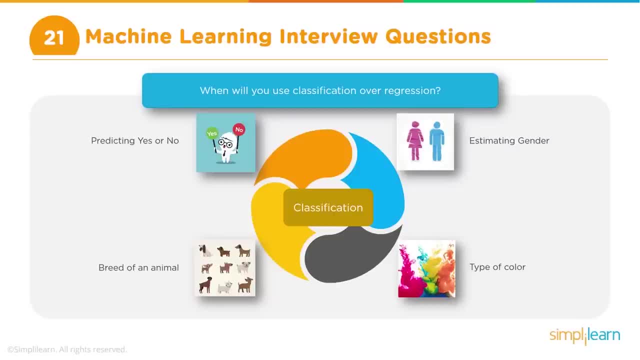 prediction. So that is where, again, you will use regression. So these are the various examples. So you need to illustrate with examples and make sure you include those keywords like discrete and continuous. So the next question is more about a little bit of a. 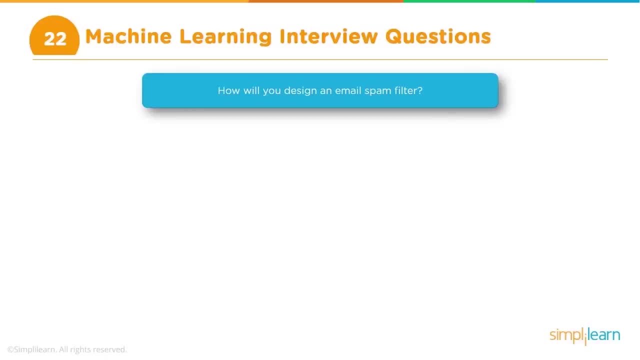 design related question to understand your concepts and things like that. So it is: how will you design a spam filter? So how do you basically design or develop a spam filter? So I think the main thing here is he's looking at probably understanding your concepts in terms of 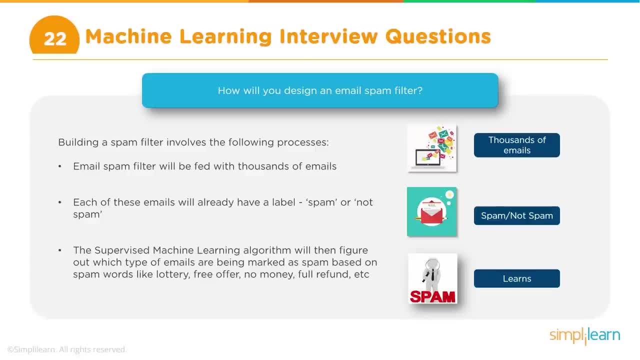 what is the algorithm you will use or what is your understanding about difference between classification and regression and things like that, right, And the process, of course, the methodology and the process. So the way we go about responding to this is we say that, okay, this is a classification problem. 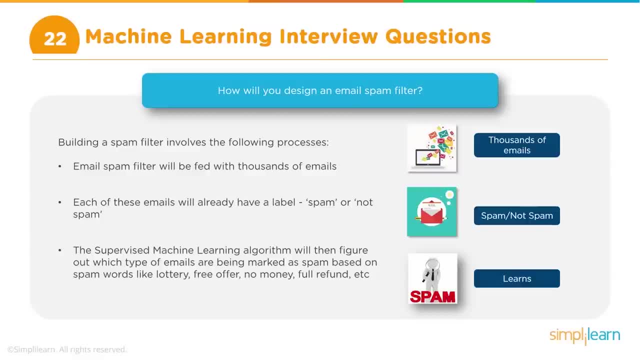 because we want to find out whether an email is a spam or not spam so that we can apply the filter accordingly. So first thing is to identify what type of a problem it is. So we have identified that it is a classification. Then the second step may be to find out what kind of algorithm to use. 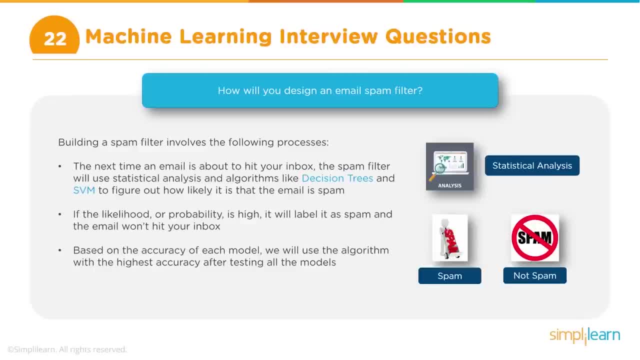 Now, since this is a binary classification problem, logistic regression is a very common, very common algorithm, But however right As I said earlier also, we can never say that okay for this particular problem, this is exactly the algorithm that we can use, So we can also probably try decision trees or even support vector. 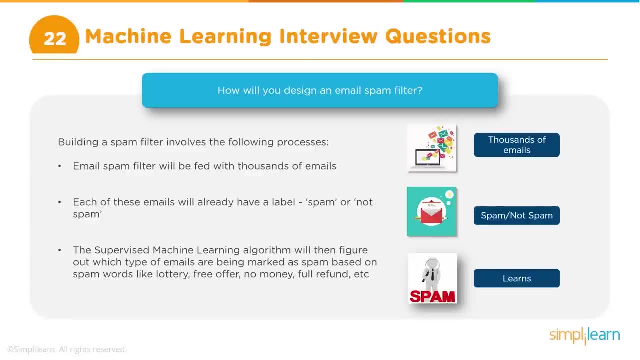 or what is your understanding about difference between classification and regression and things like that, right And the process, of course, the methodology and the process. So the best way to go about responding to this is we say that, okay, this is a classification problem because we want 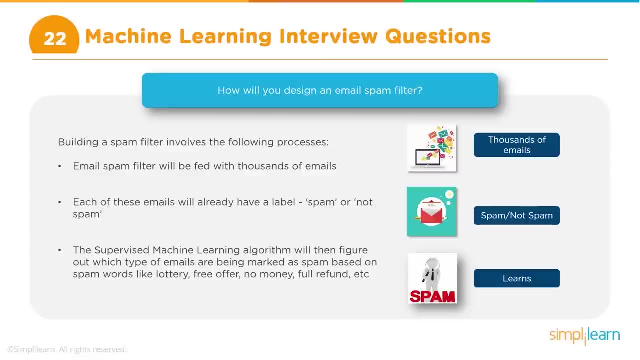 to find out whether an email is a spam or not spam, so that we can apply the filter accordingly. So first thing is to identify what type of a problem it is. So we have identified that it is a classification. Then the second step may be to find out. 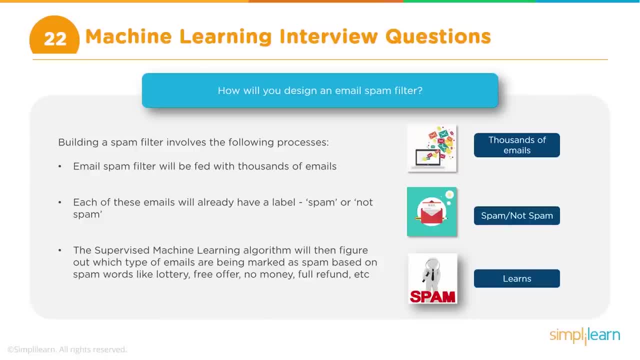 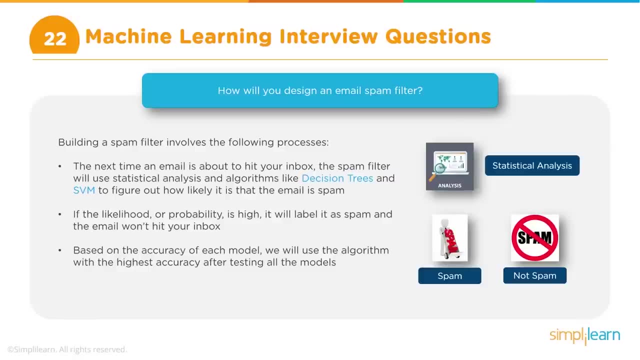 what kind of algorithm to use Now, since this is a binary classification problem. logistic regression is a very common, very common algorithm, But however right as I said earlier also, we can never say that okay, for this particular problem, this is exactly the algorithm. 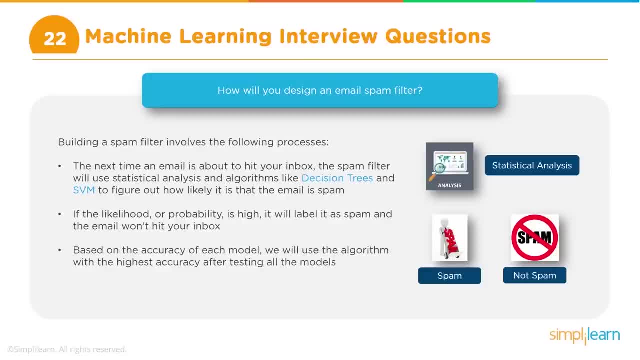 that we can use. So we can also probably try decision trees or even support vector machines, for example SVM. So we will kind of list down a few of these algorithms and we will say, okay, we want to, we would like. 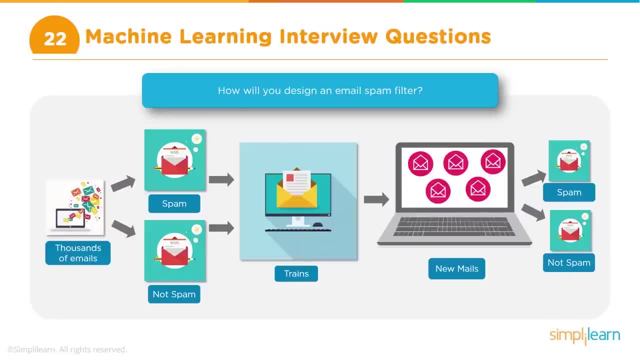 try out these algorithms. and then we go about taking your historical data, which is the labeled data, which are marked, so you will have a bunch of emails- and then you split that into training and test data sets. you use your training data set to train your model that or your algorithm that. 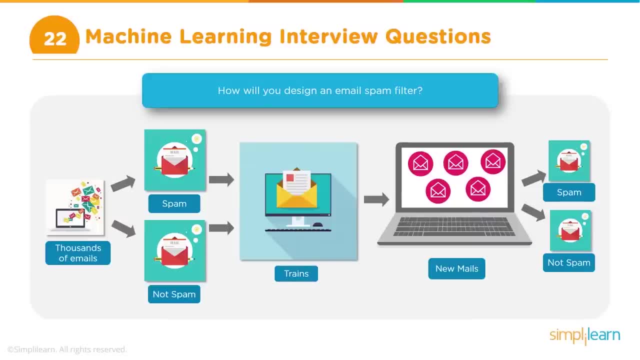 you've used, or rather the model, actually so, and you actually will have three models. let's say, you are trying to test out three algorithms, so you will obviously have three models. so you need to try all three models and test them out as well, see which one gives the best accuracy, and then you 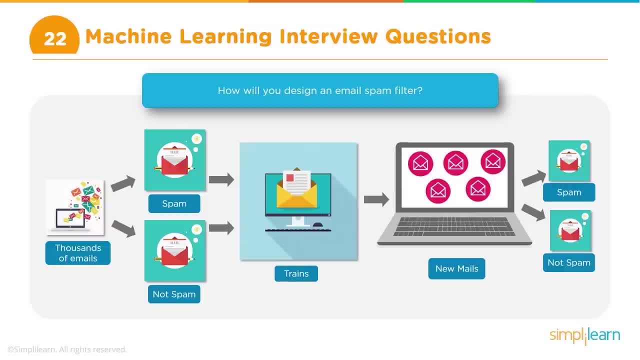 decide that you will go with that model. okay, so training and test will be done. and then you zero in on one particular model and then you say, okay, this is the model we'll use. we will use and then go ahead and implement that or put that in production. so that is the way you design a. 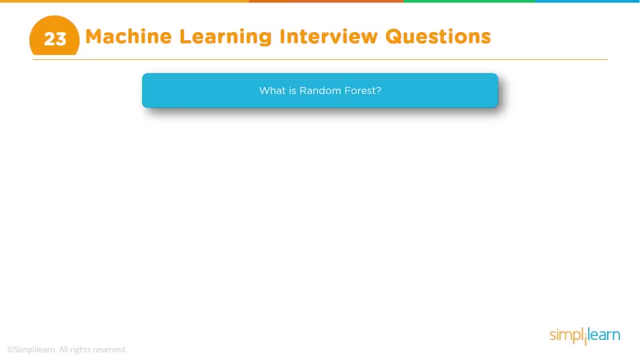 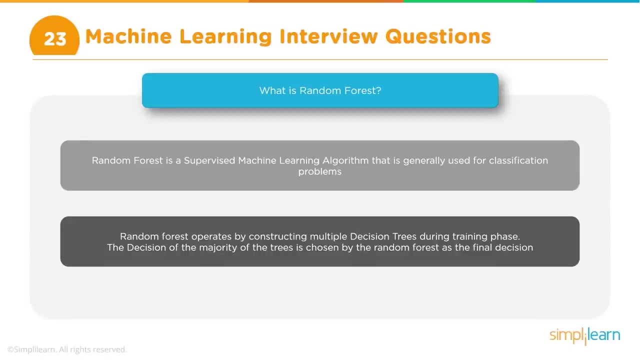 spam field. the next question is about random forest. so what is random forest? so this is a very straightforward question. however, the response you need to be again a little careful. while we all know what is random forest, explaining this can sometimes be tricky. so one thing is: random forest is kind of, in one way, it is an extension of decision trees because it 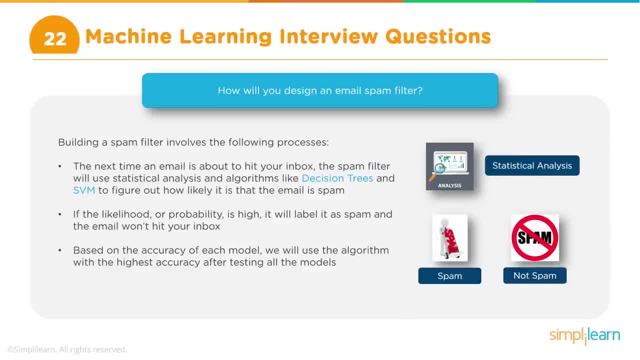 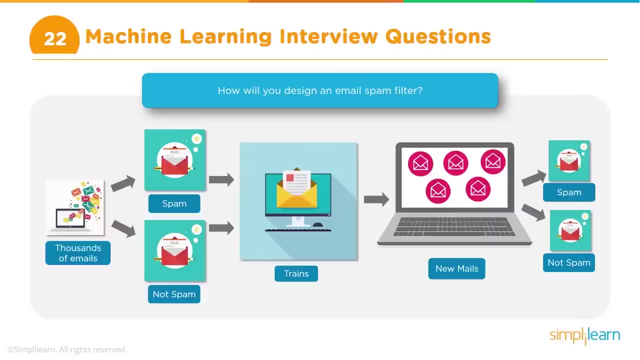 machines, for example SVM. So we will kind of list down a few of these algorithms and we will say, okay, we want to, we would like to try out these algorithms, And then we go about taking your historical data, which is the labeled data which are marked. So you will have a bunch of emails and 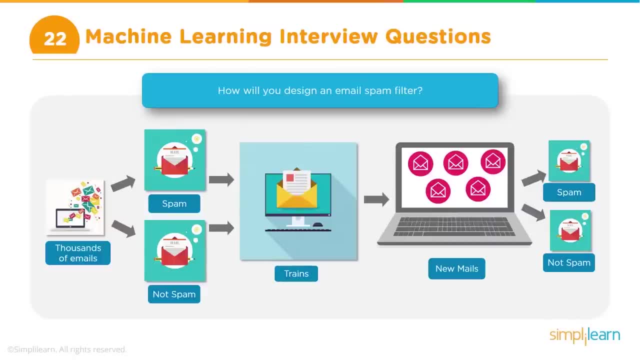 then you split that into training and test data sets. You use your training data set to train your model, that or your algorithm that you've used, or rather the model actually. So and you actually will have three models. Let's say you are trying to test out three algorithms, So you will obviously 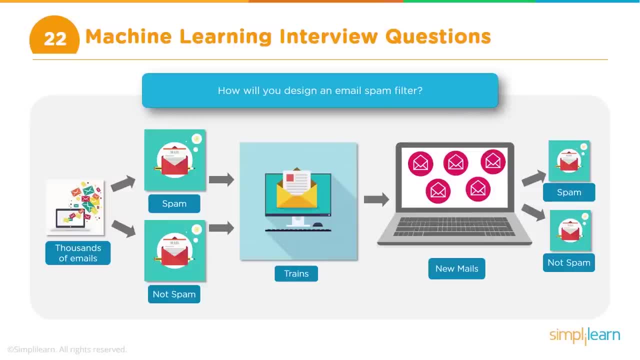 have three models. So you need to try all three models and test them out as well, See which one gives the best accuracy, And then you decide that you will go with that model. Okay, So the training and tests will be done, and then you zero in on one particular model, And then you 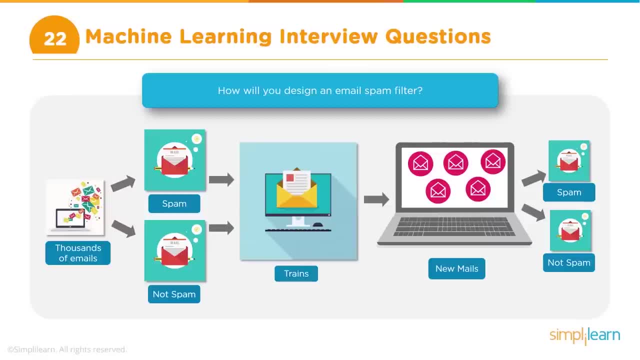 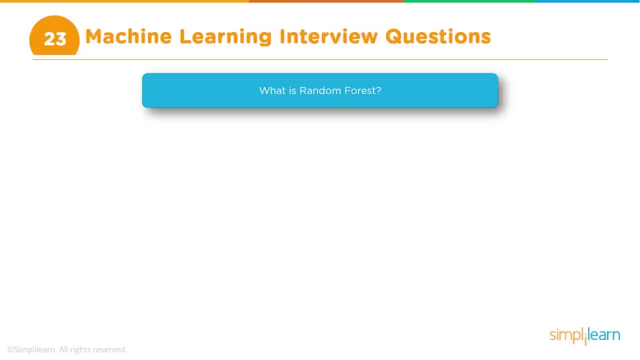 say: okay, this is the model we'll use. We will use and then go ahead and implement that or put that in production. So that is the way you design a spam field. The next question is about random forest. What is random forest? So this is a very straightforward question. However, the response 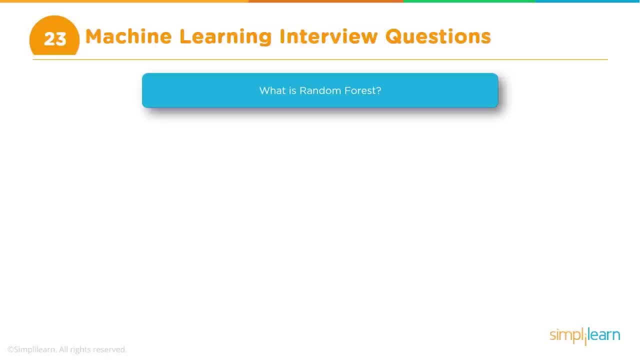 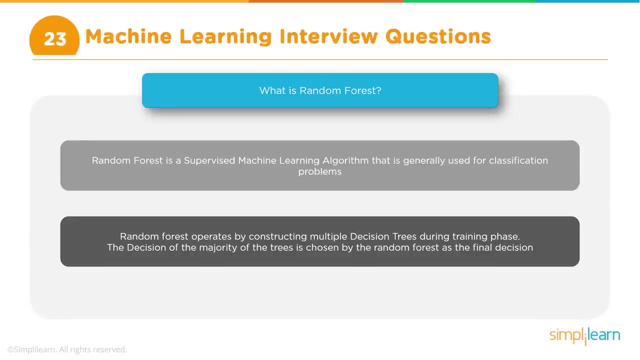 you need to be again a little careful. while we all know what is random forest, explaining this can sometimes be tricky. So one thing is random forest is kind of. in one way it is an extension of decision trees, because it is basically nothing. 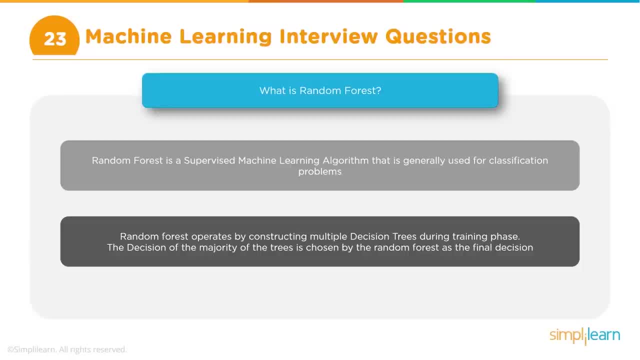 but you have multiple decision trees and trees will basically we will use for doing if it is classification- mostly it is classification- You will use the trees for classification and then you use voting for finding that the final class. So that is the underlines, but how will you explain this? How will you respond to this? So, first thing, 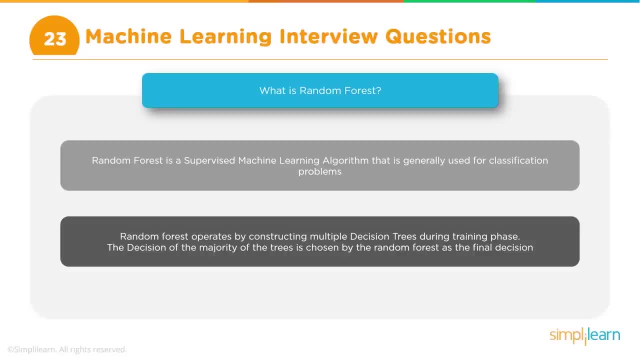 obviously we will say that random forest is one of the algorithms and the more important thing that You need to- probably the interviewer is is waiting to hear- is ensemble learner, right? So this is one type of ensemble learner. What is ensemble learner? Ensemble learner is like a. 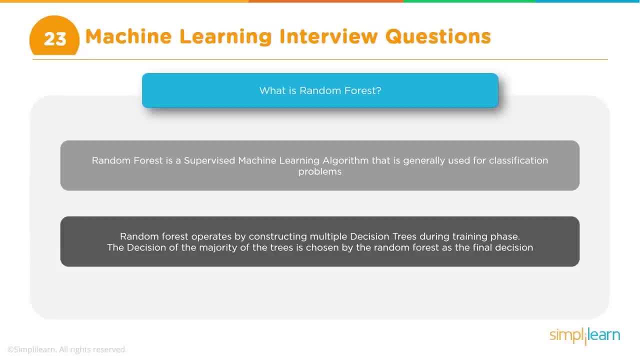 combination of algorithms, So it is a learner which consists of more than one algorithm, or more than one, maybe models. Okay, So in case of random forest, the algorithm is the same, but instead of using one instance of it, we use multiple instances of it, and we use So in a way. 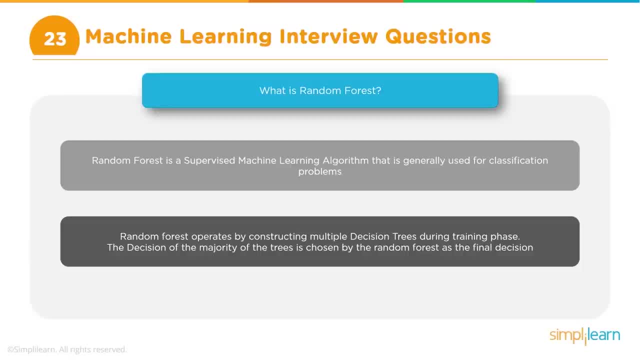 is basically nothing. but you have multiple decision. trees and trees will basically you will use for doing if it is classification- mostly it is classification- you will use the trees for classification and then you use voting for finding that the final class. so that is the underlines, but 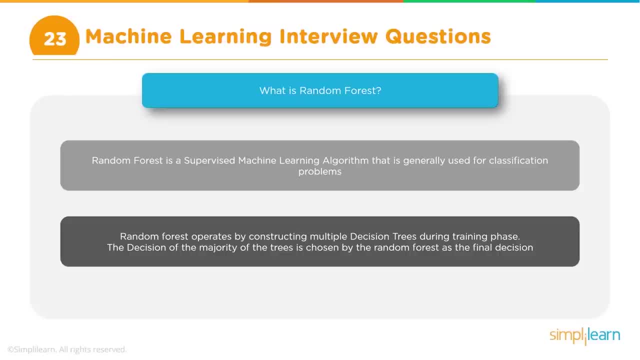 how will you explain this? how will you respond to this? so, first thing, obviously we will say that random forest is one of the algorithms and the more important thing that you need to- probably the interviewer is is waiting to hear- is ensemble learner, right? so this is one type of ensemble. 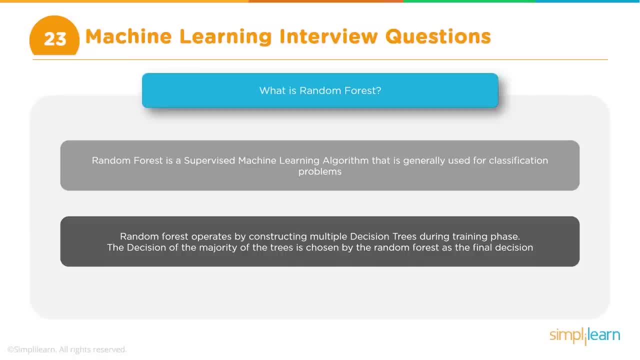 learner. what is ensemble learner? ensemble learner is like a combination of algorithms, so it is a learner which is a combination of algorithms, so it is a learner which is a combination of algorithms, consists of more than one algorithm, or more than one maybe models, okay, so in case of random forest, 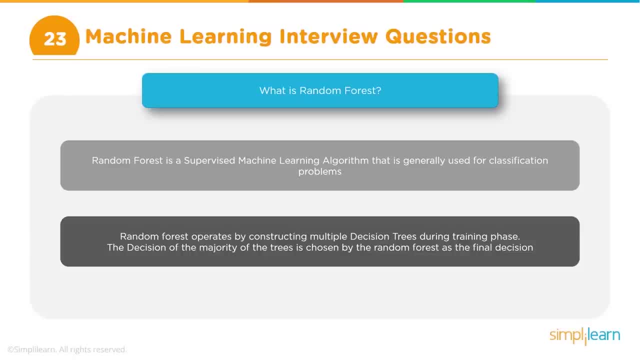 the algorithm is the same, but instead of using one instance of it, we use multiple instances of it, and we use so in a way that is: a random forest is an ensemble learner. there are other types of ensemble learners where we have like we use different algorithms itself, so you have one. 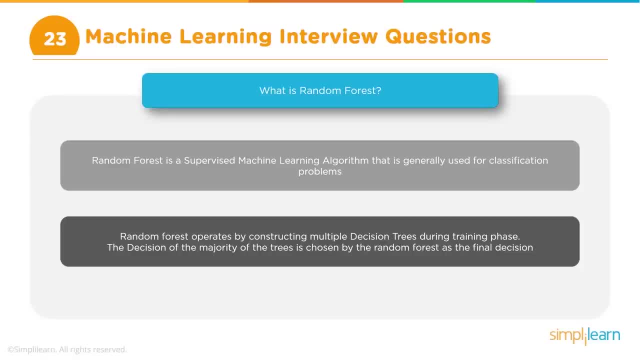 maybe logistic regression and the decision tree combined together and so on and so forth, or there are other types of algorithms, there are other types of algorithms, there are other types of algorithms, so it's all about ensemble. we will not go into that, but random forest itself. i think the interviewer 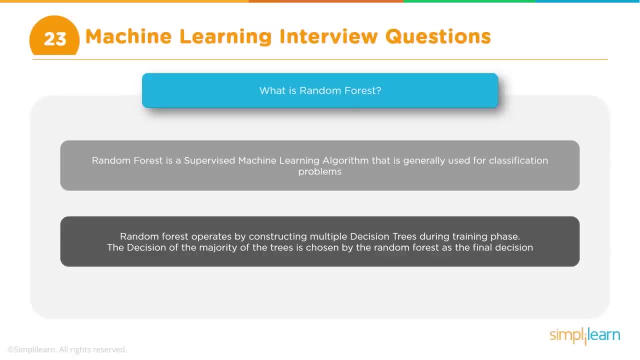 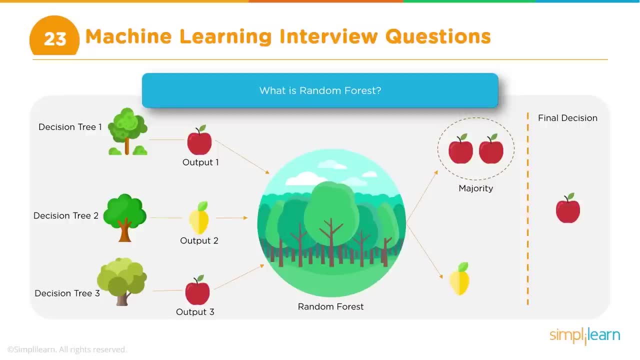 will be happy to hear this word: ensemble learner. and so then you go and explain how the random forest works. so if the random forest is used for classification, then we use what is known as a voting mechanism. so basically, how does it work? let's say your random forest consists of: 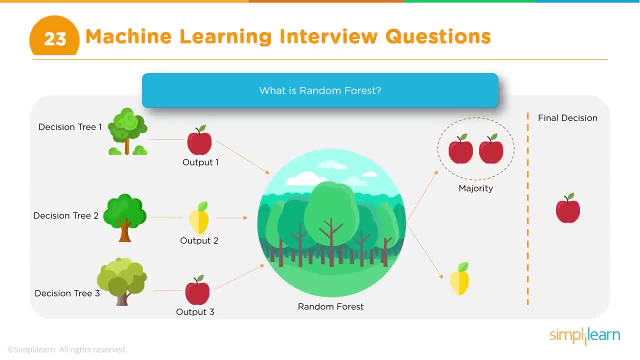 hundred trees. okay, and each observation, you pass through this forest and each observation. let's say it is a classification problem, binary classification, 0 or 1, and you have 100 trees. now if 90 trees say that it is a 0 and 10 of the trees say it is a 1, you take the majority. you may take a. 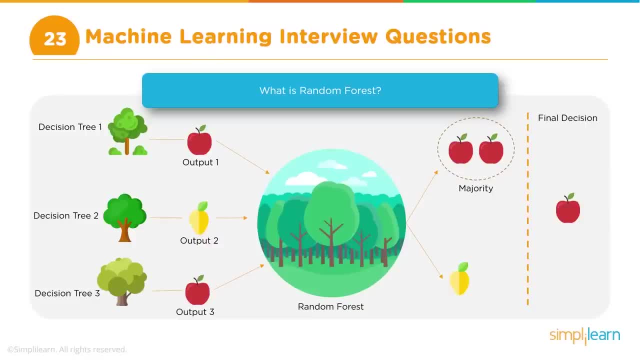 vote, and since 90 of them are saying 0, you classify this as 0, then you take the next observation, and so on. so that is the way random forest works for classification. if it is a regression problem, it's somewhat similar, but only thing is, instead of vote, what we will do is so, in regression, remember what. 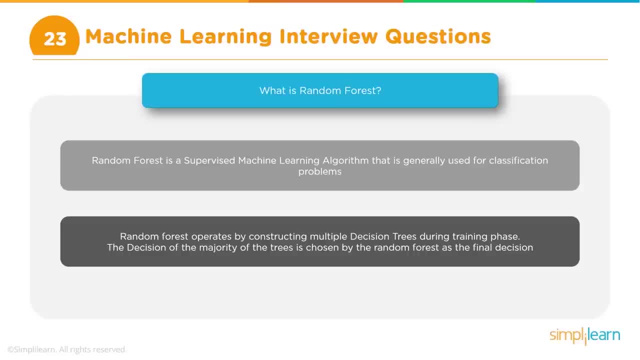 that is, a random forest, is an ensemble learner. There are other types of ensemble learners where we have, like we use different algorithms itself, So you have one, maybe logistic regression and a decision tree combined together, and so on and so forth. Or there are other ways, like, for example, 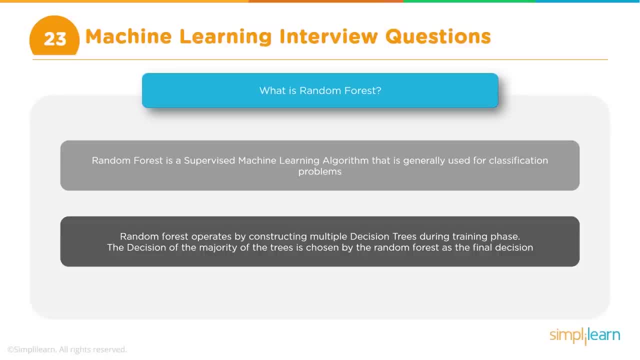 splitting the data in a certain way and so on. So that's all about ensemble. We will not go into that, but random forest itself. I think the interviewer will be happy to hear this word: ensemble learner. And so then you go and explain how the random forest works. So 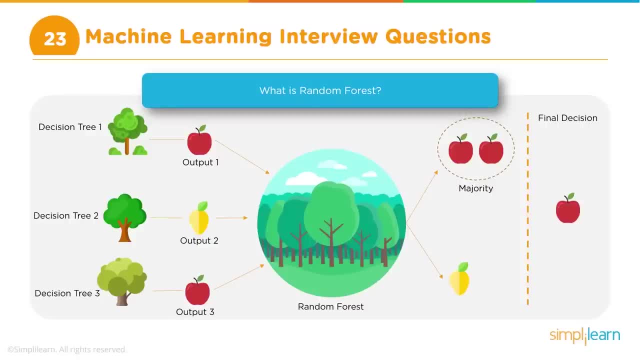 if the random forest is used for classification, then we use what is known as a voting mechanism. So, basically, how does it work? Let's say your random forest consists of 100 trees, Okay, And each observation, you pass through this forest and each observation- let's say it is a classification. 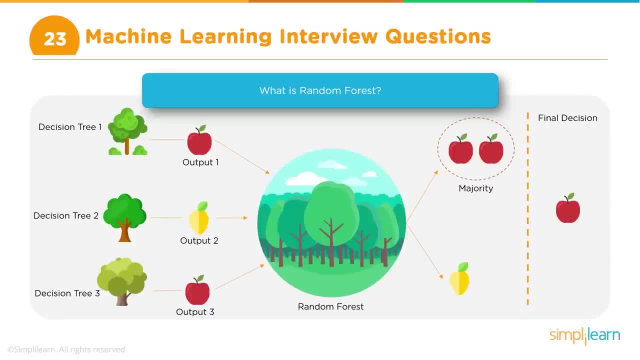 problem: binary classification- zero or one- and you have a hundred trees. Now, if 90 trees say that it is a zero and 10 of the trees say it is a one, you take the majority. you may take a vote. 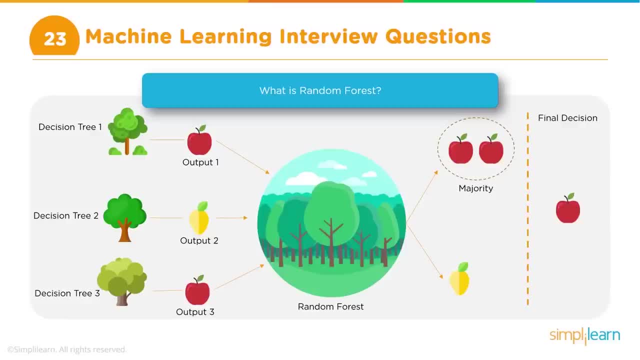 All of them are saying zero. You classify this as zero, Then you take the next observation, and so on. So that is the way a random forest works for classification. If it is a regression problem, it's somewhat similar, but only thing is, instead of vote, what we will do is so in regression. 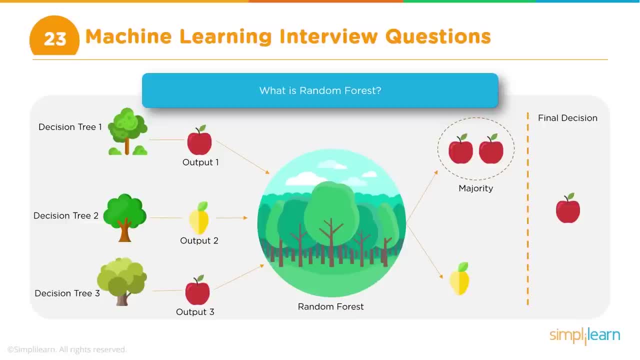 remember what happens. You actually calculate a value, right? So, for example, you're using regression to predict the temperature and you have a hundred trees and each tree obviously will probably predict a different value of the temperature. They may be close to each other but they may not be exactly the same value. So these hundred trees 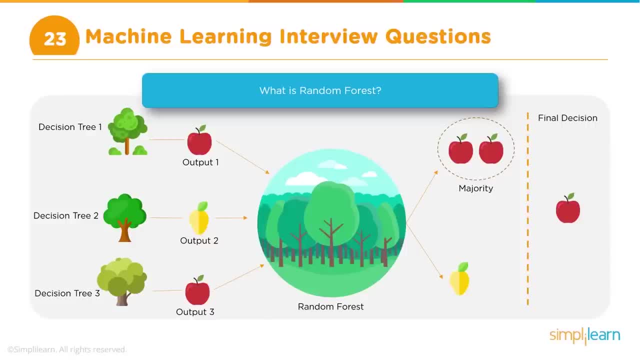 So how do you now find the actual value, the output for the entire forest right? So you have outputs of individual trees which are a part of this forest, but then you need to find the final output of the forest itself. So how do you do that? So in case of regression you take like an average or the 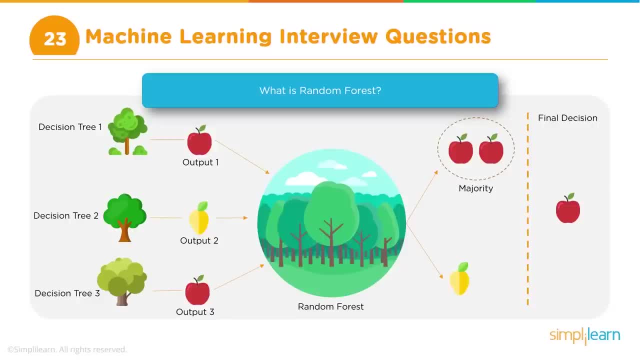 mean of all the hundred trees, right. So this is also a way of reducing the error. So maybe if you make an error, it is basically a hundred percent wrong or a hundred percent right, right. But if you have, on the other hand, if you have a bunch of trees, you are basically mitigating that error. 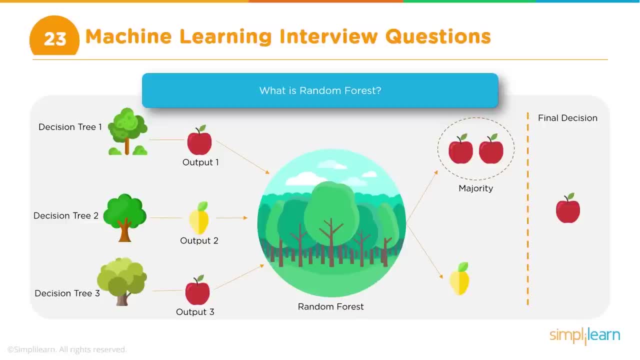 you do, is you actually calculate a value right? so, for example, you're using regression to predict the temperature and you have 100 trees and each tree obviously will probably predict a different value of the temperature. they may be close to each other, but they may not be exactly the same value. so these 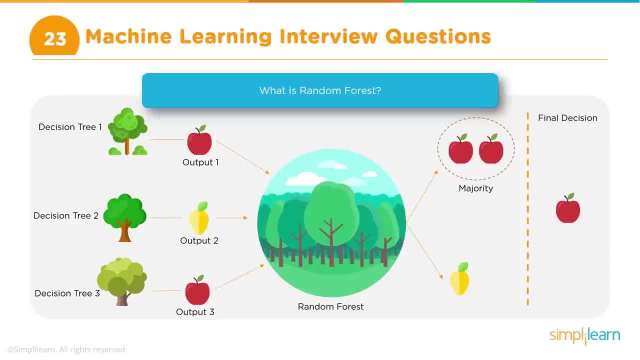 hundred trees. so how do you now find the actual value, the output for the entire forest, right, so you have outputs of individual trees which are a part of this forest, but then you need to find the output of the forest itself. so how do you do that? so in case of regression you take like an average. 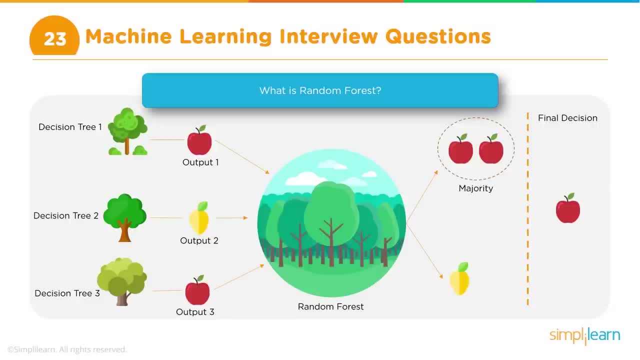 or the mean of all the hundred trees, right? so this is also a way of reducing the error. so maybe if you have only one tree and if that one tree makes a error, it is basically 100 wrong or 100 right, right. but if you have, on the other hand, if you have a bunch of trees, you are basically mitigating that. 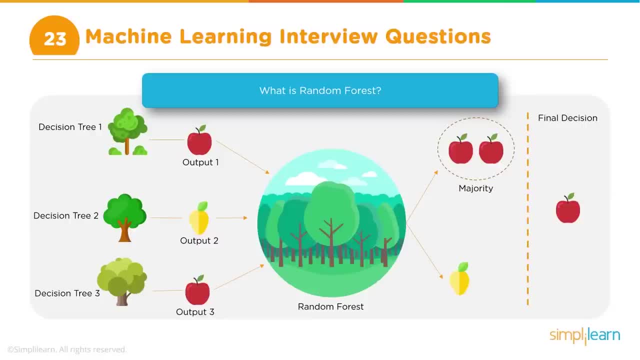 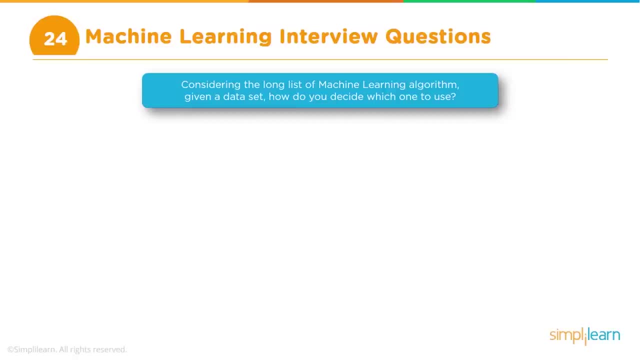 error, reducing that error. okay, so that is the way random forest works. so the next question is: regarding the long list of machine learning algorithms: how will you decide on which one to use? so once again here, there is no way to outright say that this is the algorithm that we will use. 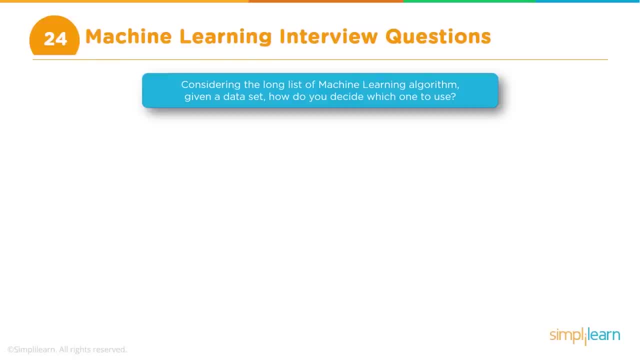 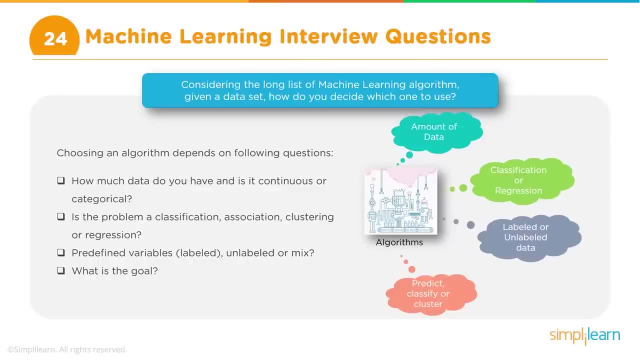 for a given data set. this is a very good question, but then the response has to be like again: there will not be a one size fits all, so we need to. first of all, you can probably shorten the list in terms of by saying: okay, whether it is a classification problem or it is a. 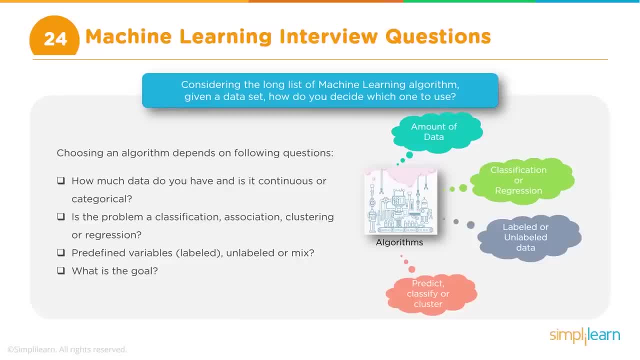 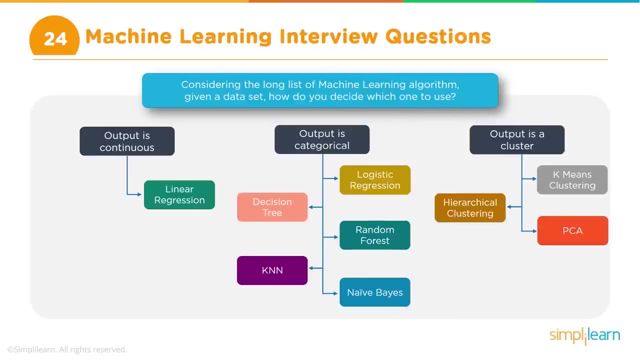 regression problem. to that extent you can probably shorten the list because you don't have to use all of them. if it is a classification problem, you only can pick from the classification algorithms, right? so, for example, if it's a classification, you cannot use linear regression algorithm, or if it is a regression problem, you cannot use svm, or maybe. no, you can use svm, but maybe. 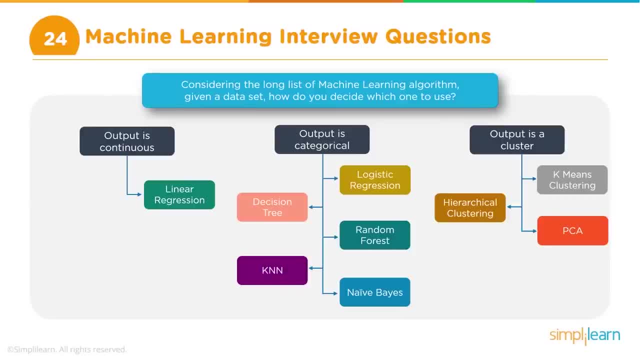 a logistic regression, right. so to that extent you can probably shorten the list, but still you will not be able to 100 percent decide on saying that this is the exact algorithm that i am going to use. so the way to go about is you choose a few algorithms based. 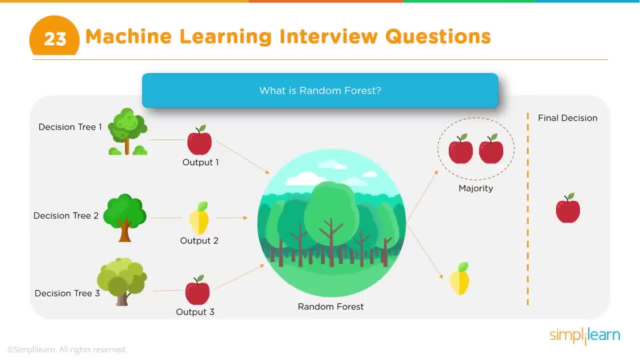 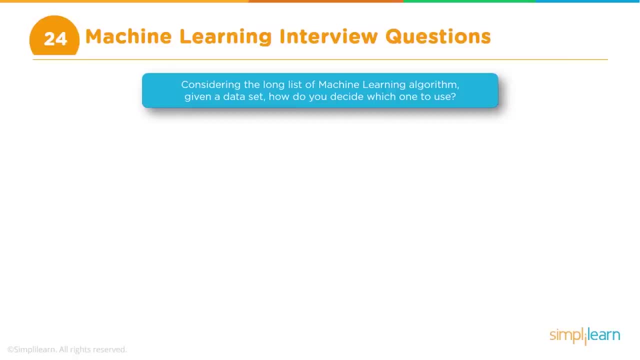 reducing that error. Okay, So that is the way random forest works. So the next question is: considering the long list of machine learning algorithms, how will you decide on which one to use? So once again here, there is no way to outright say that this is the algorithm that. 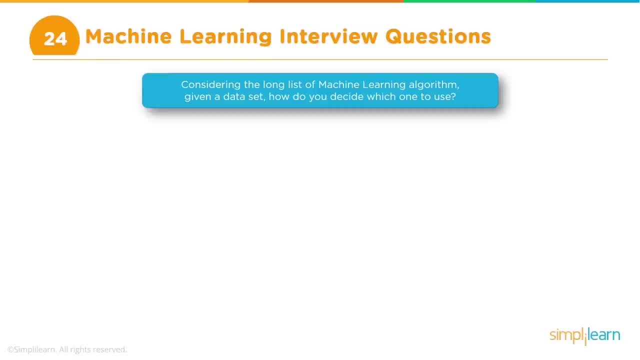 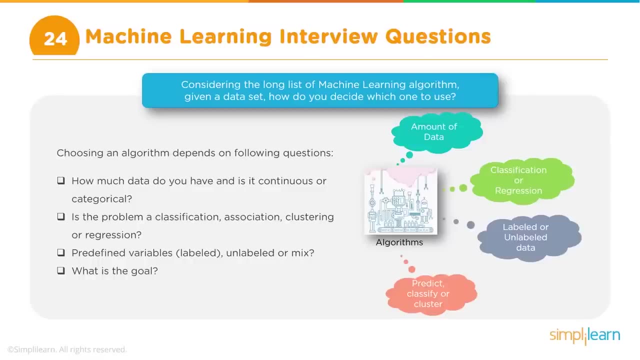 we will use for a given data set. This is a very good question, but then the response has to be like again: there will not be a one size fits all, So we need to. first of all, you can probably shorten the list in terms of by saying, okay, whether it is a. 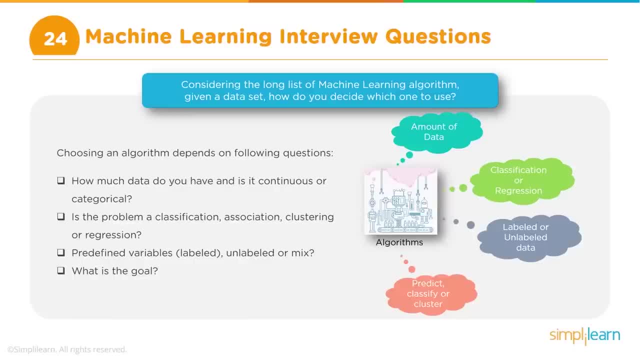 classification problem or it is a regression problem. To that extent you can probably shorten the list because you don't have to use all of them. If it is a classification problem, you only can pick from the classification algorithms right. So, for example, if it's 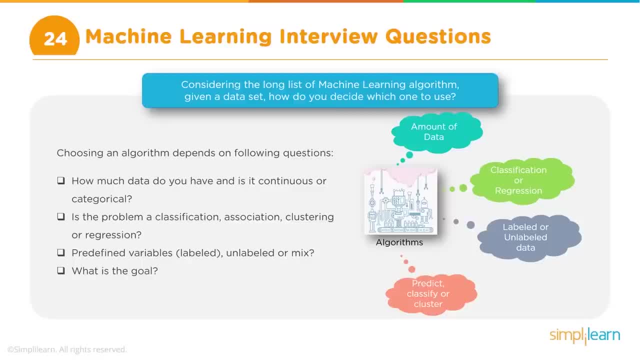 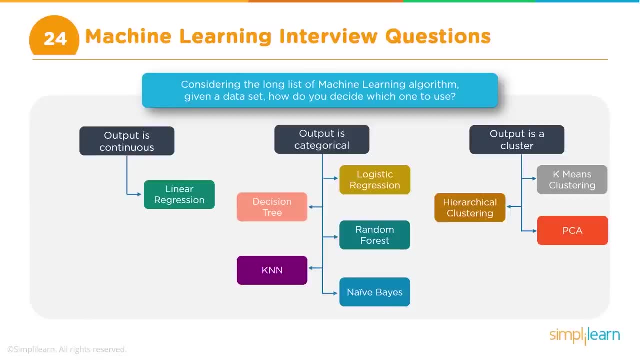 a classification, you cannot use linear regression algorithm there. or if it is a regression problem, you cannot use SVM, or maybe no, you can use SVM but maybe a logistic regression right. So to that extent you can probably shorten the list, but still you will not be able to a hundred percent decide on saying that this is 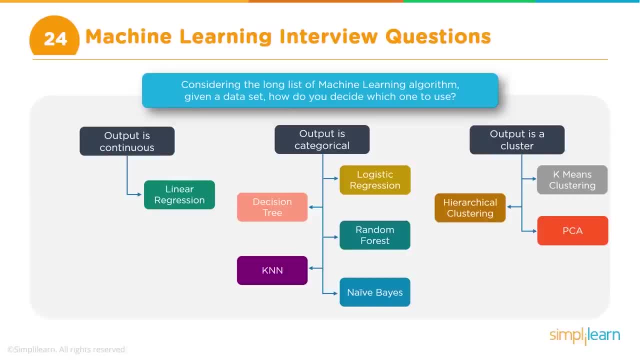 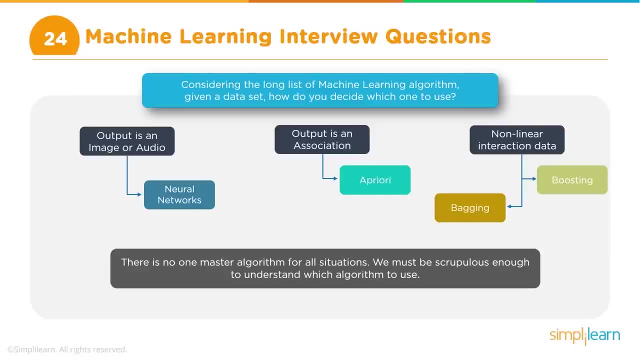 the exact algorithm that I'm going to use. So the way to go about is you choose a few algorithms based on what the problem is. You try out your data, you train some models of these algorithms- the highest accuracy- and based on that, you choose that particular algorithm. Okay, All right. 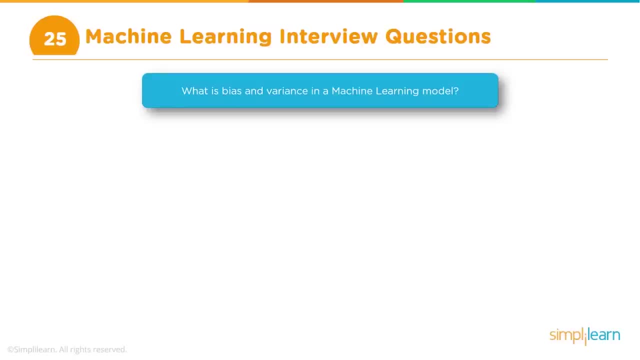 Then they can be questions around bias and variance. So the question can be: what is bias and variance in machine learning? So you just need to give out a definition for each of these. for example, a bias in machine learning: it occurs when the predicted values are far away. 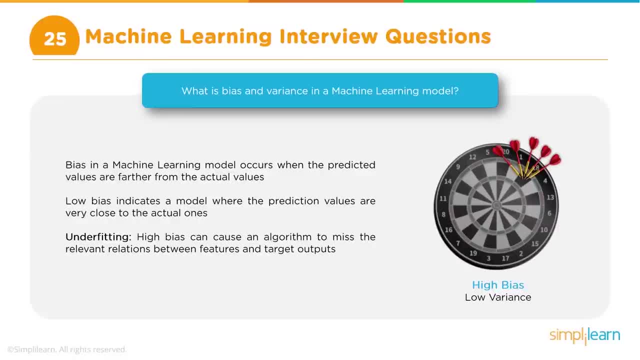 from the actual value. So that is a bias, Okay, And whereas they are all, all the values are probably. they are far off, but they are very near to each other, though The predicted values are close to each other, right, While they are far off from the actual value, but they are close. 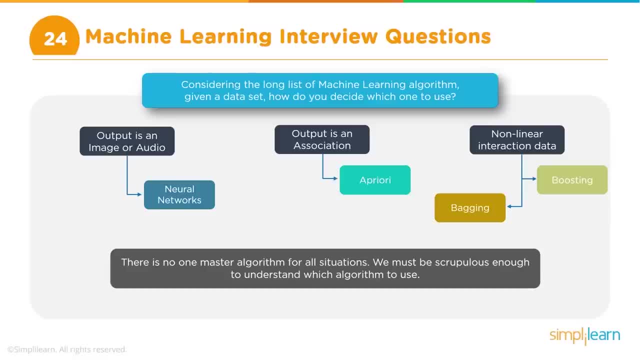 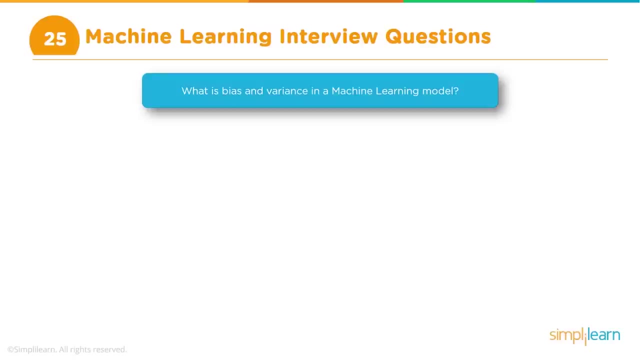 on what the problem is. you try out your data, you train some models of these algorithms, check which one gives you the lowest error or the highest accuracy, and based on that you choose that particular algorithm. okay, all right. then there can be questions around bias and variance. so the 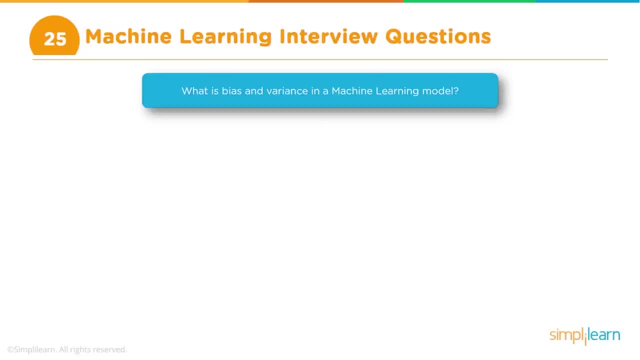 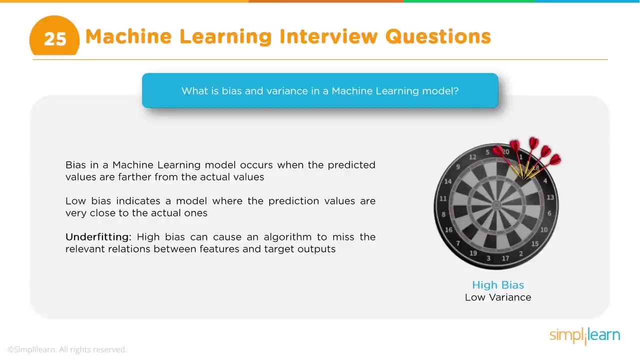 question can be: what is bias and variance in machine learning? uh, so you just need to give out a definition for each of these. for example, a bias in machine learning it occurs when the predicted values are far away from the actual value. so that is a bias, okay. and whereas 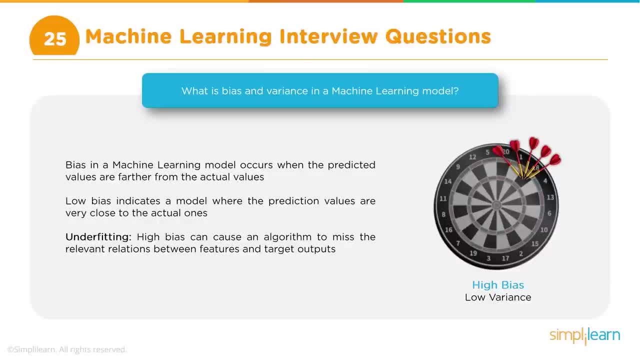 they are all. all the values are probably. they are far off, but they are very near to each other, though the predicted values are close to each other, right, while they are far off from the actual value, but they are close to each other. you see the difference. so that is the bias. and then 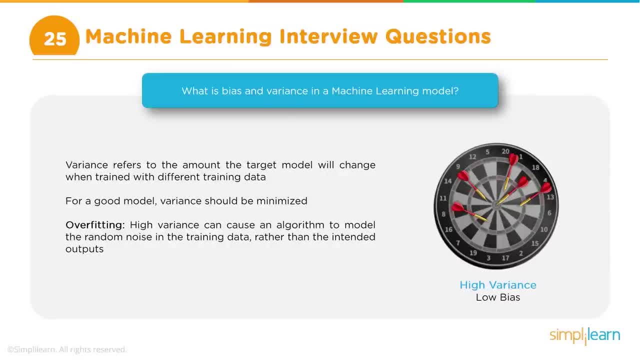 the other part is your variance. now, variance is when the predicted values are all over the place, right, so the variance is high. that means it may be close to the target, but it is kind of very scattered. so the point: the predicted values are not close to each other. right, in case of bias. the predicted values are close to each other, but they are not. 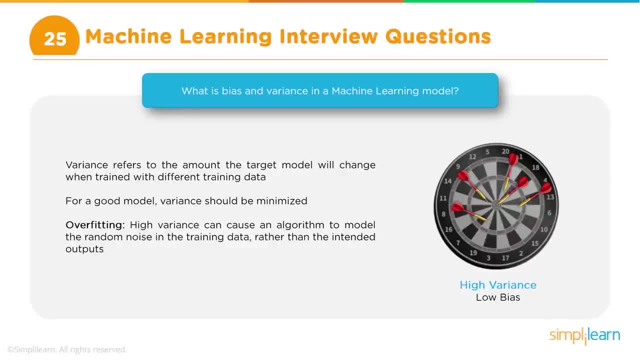 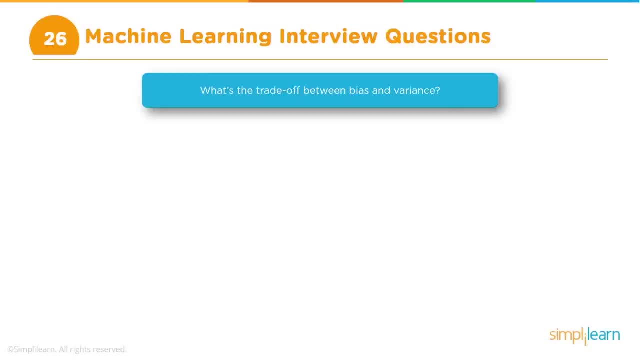 close to the target, but here they may be close to the target, but they may not be close to each other, so they are a little bit more scattered. so that is what. okay, so for variance. okay, then next question is about, again related to bias and variance. what is the trade-off between bias and variance? yes, I think this is a interesting 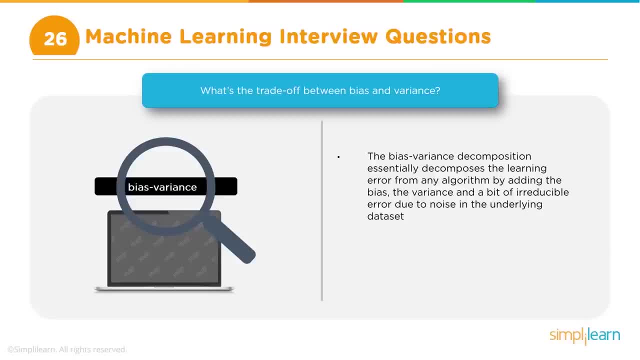 question because these two are heading in different directions. so, for example, if you try to minimize the bias, variance will keep going high, and if you try to minimize the variance, bias will keep going high and there is no way you can minimize both of them. so you need to have a trade. 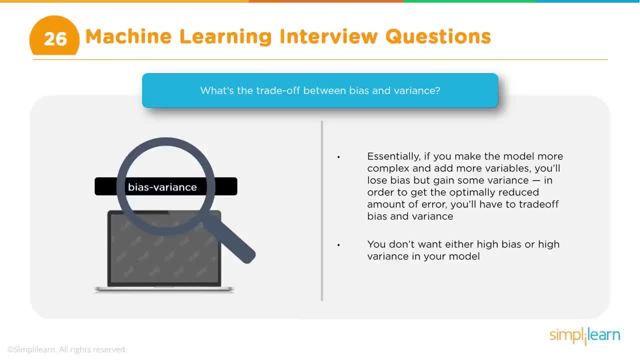 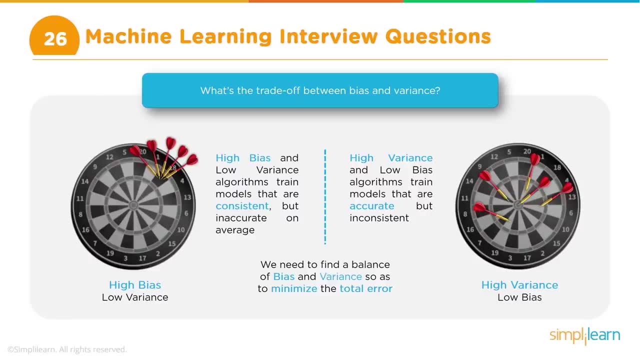 off saying that, okay, this is the level at which I will have my bias and this is the level at which I will have variance. so the trade-off is that, pretty much, that you decide what is the level you will tolerate for your bias and what is the level you will tolerate for variance and a. 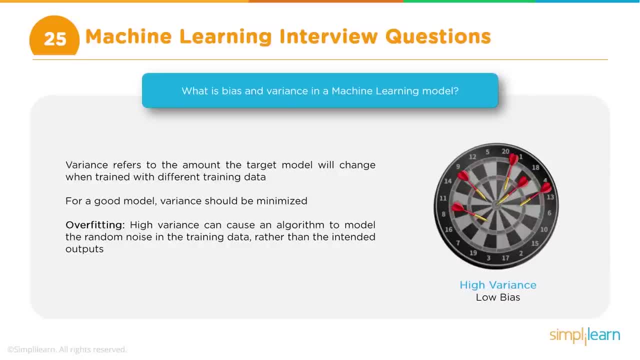 to each other. You see the difference. So that is bias. And then the other part is your variance. Now, variance is when the predicted values are all over the place, right. So the variance is high. That means it may be close to the target, but it is kind of very scattered. So the point. 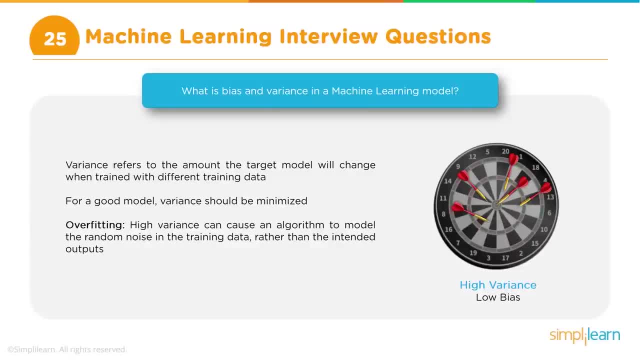 the predicted values are not close to each other, right, Right? So in case of bias, the predicted values are very close to each other. In case of bias, the predicted values are close to each other, but they are not close to the target. but here they. 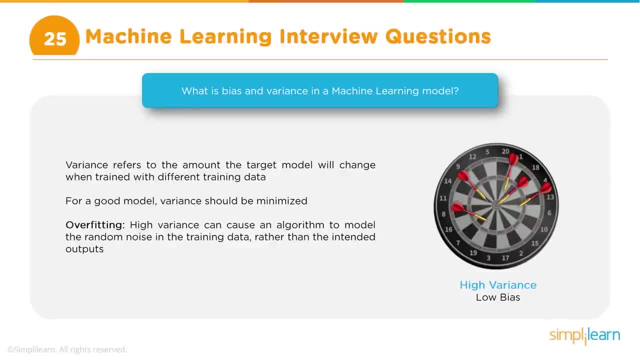 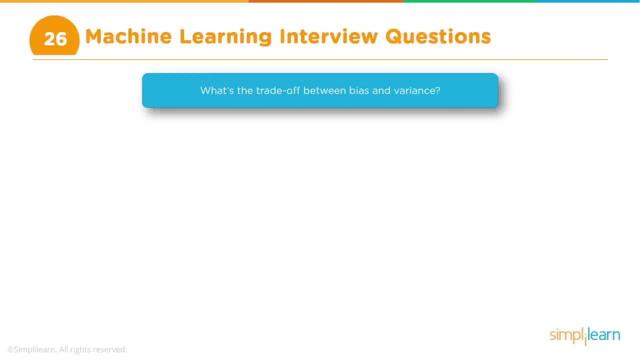 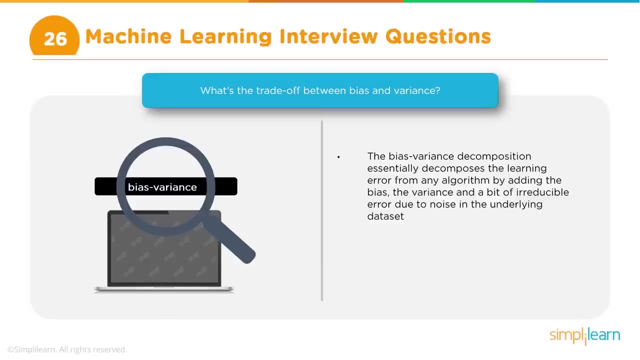 may be close to the target, but they may not be close to each other, so they are a little bit more scattered. so that is what in case of a variance. okay, then the next question is about, again related to bias and variance. what is the trade-off between bias and variance? yes, i think this is a interesting 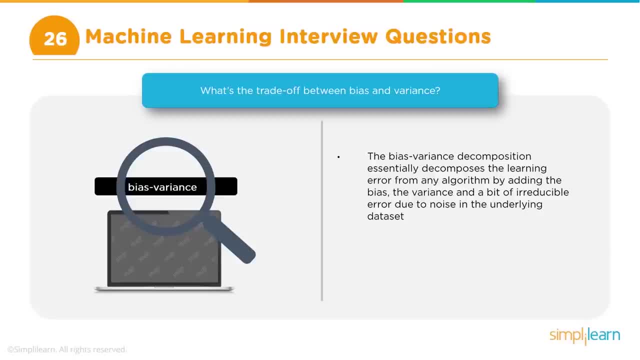 question because these two are heading in different directions. so, for example, if you try to minimize the bias, variance will keep going high, and if you try to minimize the variance, bias will keep going high and there is no way you can minimize both of them, so you need to. 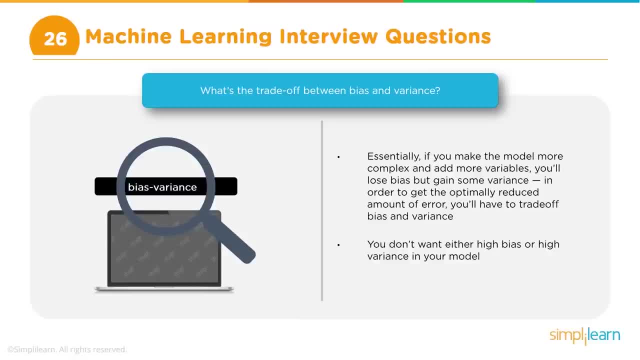 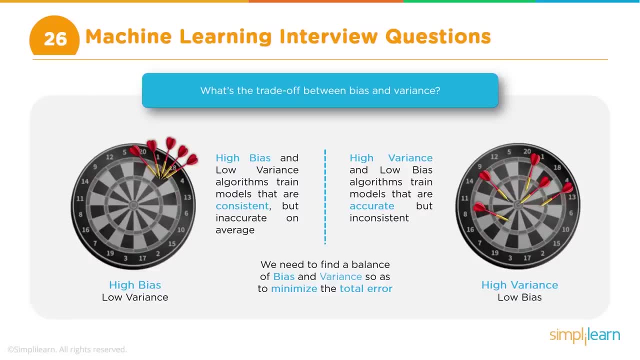 have a trade-off saying that: okay, this is the level at which i will have my bias and this is the level at which i will have variance. so the trade-off is that, pretty much, that you decide what is the level you will tolerate for your bias and what is the level you will tolerate for. 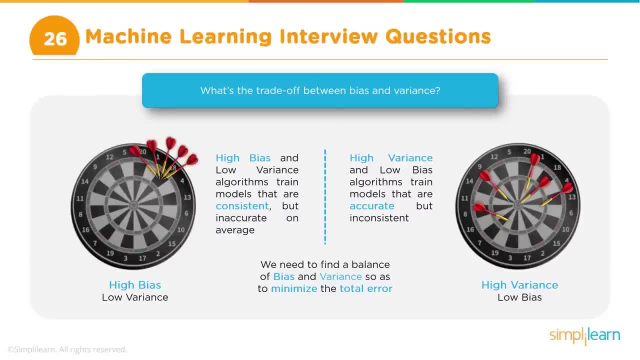 variance and a combination of these two in such a way that your final results are not way off, and having a trade-off will ensure that the results are consistent, right? so that is basically: the output is consistent, and which means that they are close to each other and they are also accurate, which that means they are as close. 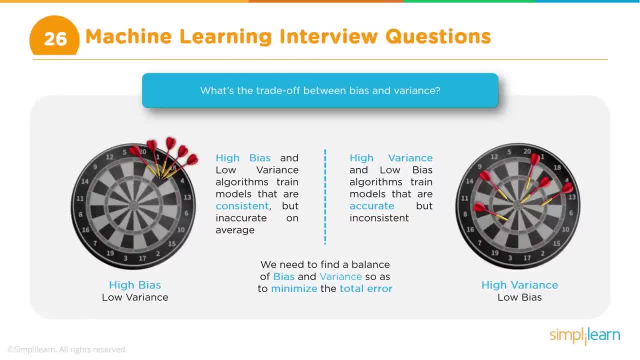 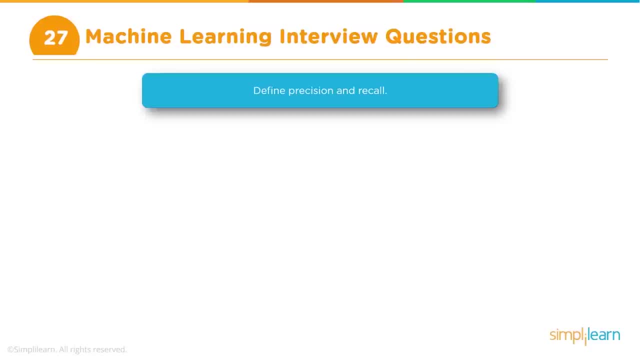 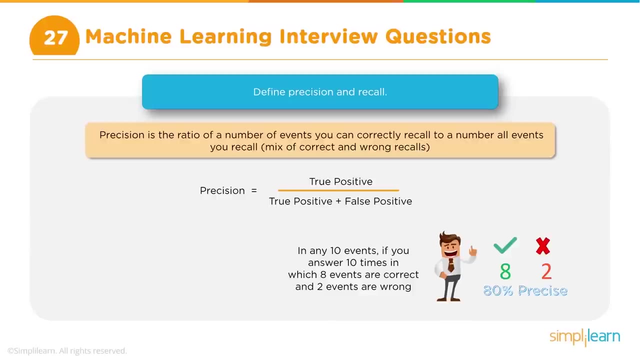 to the target as possible, right? so if either of these is high, then one of them will go off the track. define precision and recall now again here i think it would be best to draw a diagram and take a confusion matrix, and it is very simple. the definition is like a formula: your precision. 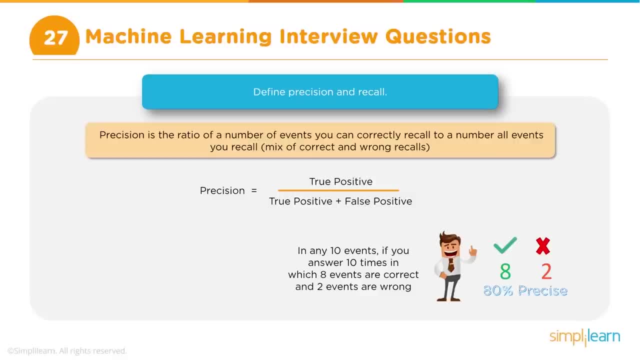 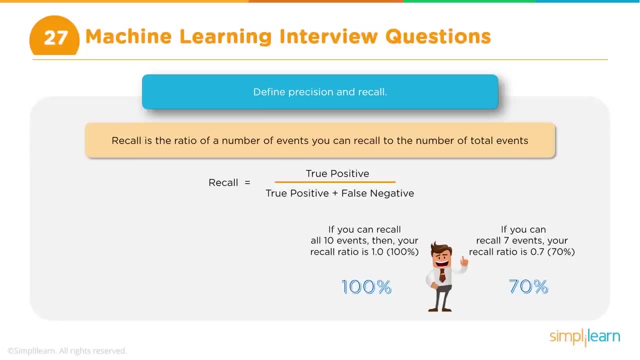 is true positive by true positive plus false positive, and your recall is true positive by true positive plus false negative. okay, so that's you can just show it in a mathematical way and that's it for this video. so thank you for watching and i will see you in the 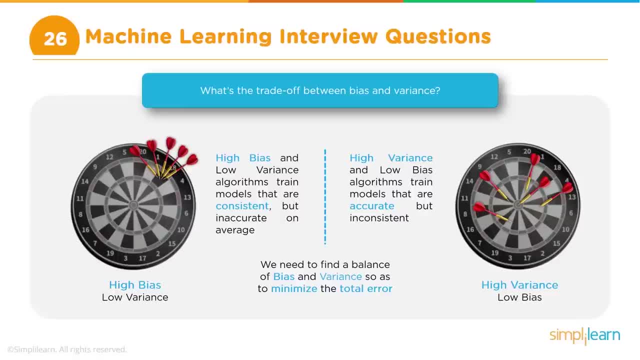 combination of these two in such a way that your final results are not way off, and having a trade off will ensure that the results are consistent, right? so that is basically: the output is consistent, and which means that they are close to each other and they are also accurate, which that means they. 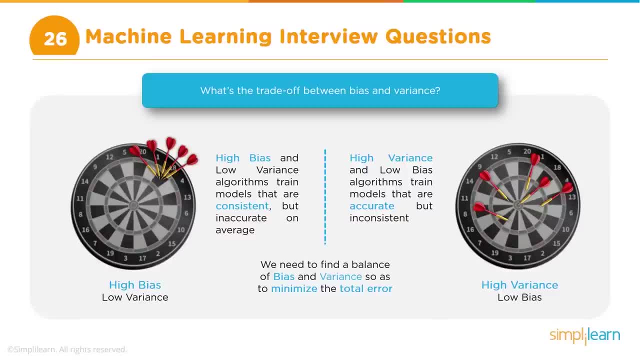 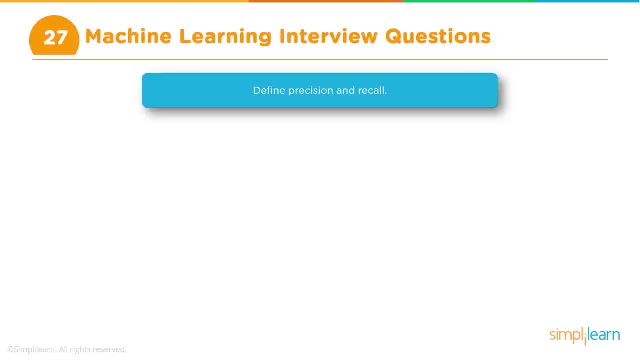 are as close to the trade-off as they are close to each other, and so that means that they are target as possible, right? so if either of these is high, then one of them will go off the track. define, precision and recall. now again, here i think it would be best to draw a diagram and take up the 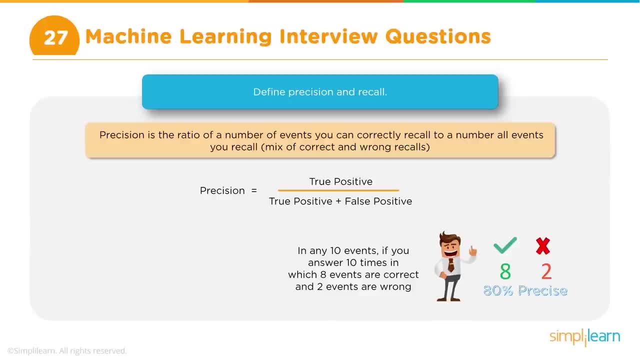 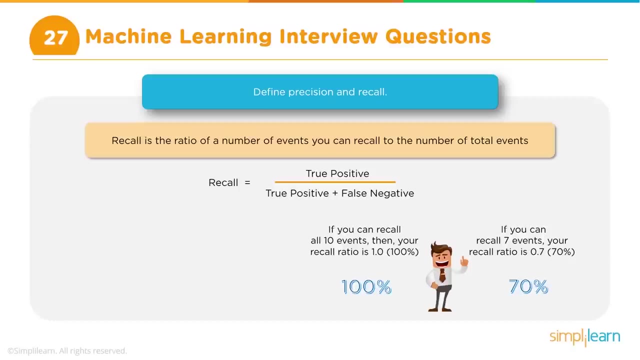 confusion matrix. and it is very simple. the definition is like a formula. your precision is true positive by true positive plus false positive and your recall is true positive by true positive plus false negative. okay, so that's, you can just show it in a mathematical way. that's pretty much you know that can be shown. that's the easiest way to define. so the next. 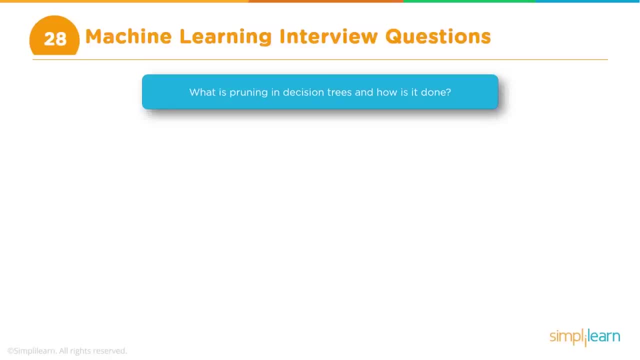 question can be about decision tree. what is decision tree pruning and why is it so? basically, decision trees are really simple to implement and understand, but it is very easy to use, so you can use it in both methods. so, for instance, if you want to. But one of the drawbacks of decision trees is that it can become highly complicated, as 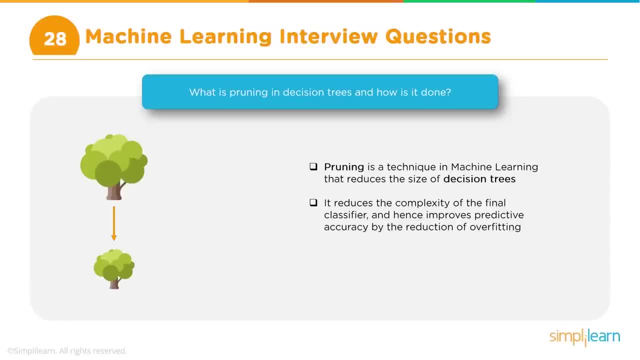 it grows right And the rules and conditions can become very complicated, And this can also lead to overfitting, which is basically that during training you will get 100% accuracy, but when you're doing testing you'll get a lot of errors. 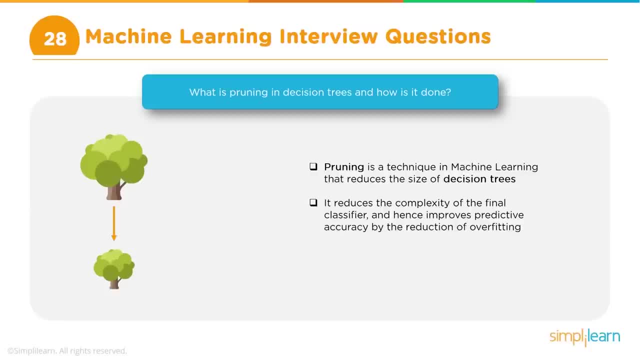 So that is the reason pruning needs to be done. So the purpose or the reason for doing decision tree pruning is to reduce overfitting or to cut down on overfitting. And what is decision tree pruning? It is basically that you reduce the number of branches because, as you may be aware, a 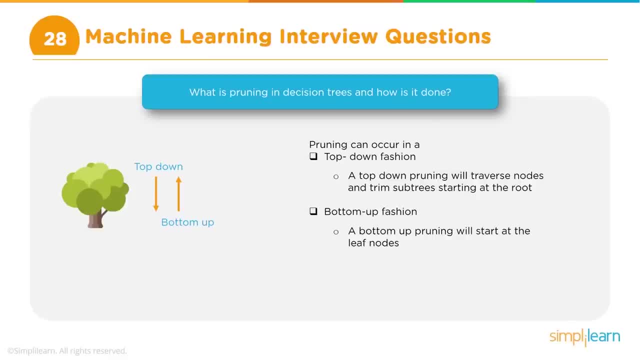 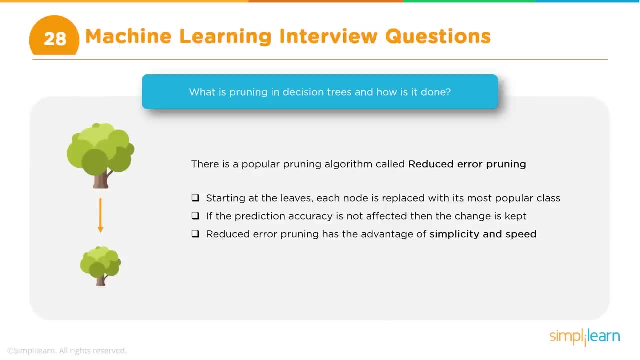 tree consists of the root node, and then there are several internal nodes, and then you have the leaf nodes. Now, if there are too many of these internal nodes, that is when you face the problem of overfitting, And pruning is the process of refining. 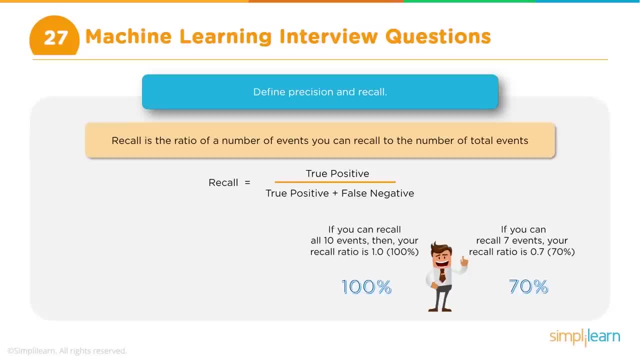 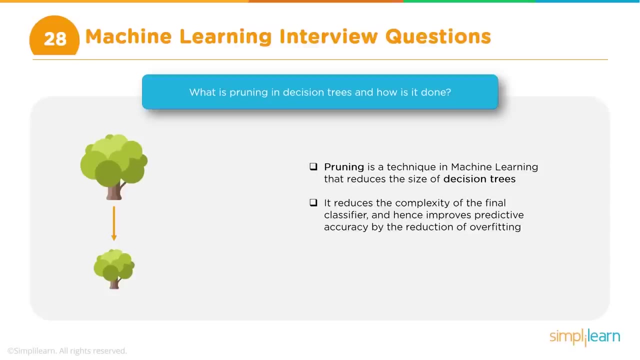 next video way. that's pretty much you know that can be shown. that's the easiest way to define. so the next question can be about decision tree. what is decision tree pruning and why is it so? basically, decision trees are really simple to implement and understand. but one of the drawbacks of decision 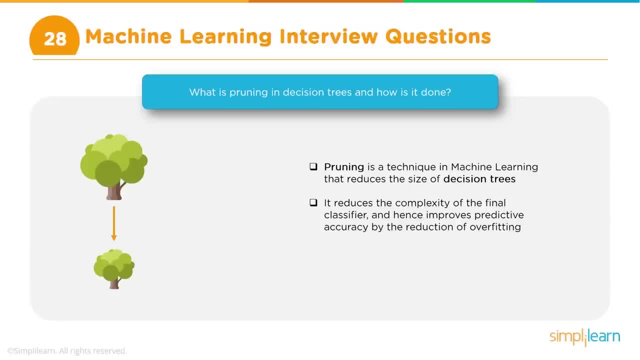 trees is that it can become highly complicated as it grows right and the rules and conditions can become very complicated, and this can also lead to a lot of problems, to overfitting, which is basically that during training you will get 100 percent accuracy, but when you're doing testing you'll get a lot of errors. so that is the reason pruning needs to. 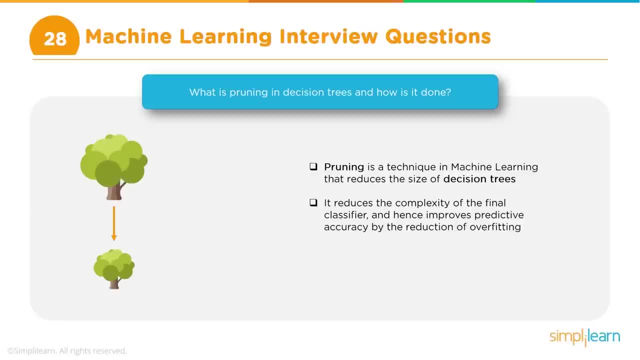 be done. so the purpose or the reason for doing decision tree pruning is to reduce overfitting or to cut down on overfitting. and what is decision tree pruning? it is basically that you reduce the number of branches because, as you may be aware, a tree consists of the 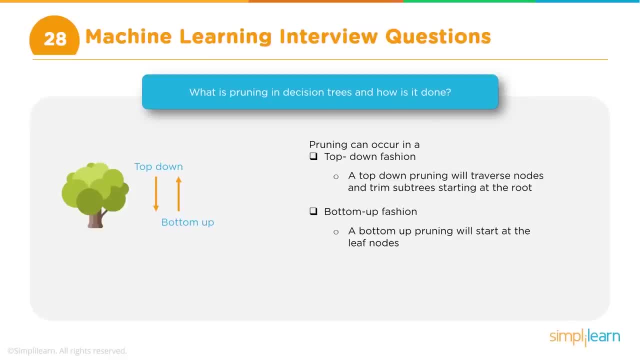 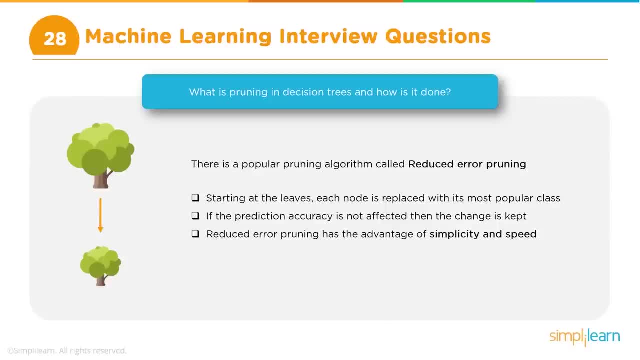 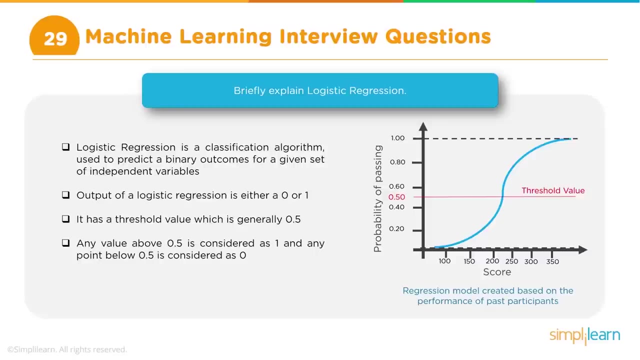 nodes. that is when you face the problem of overfitting, and pruning is the process of reducing those internal nodes all right. so the next question can be: what is logistic regression? so, basically, logistic regression is one of the techniques used for performing classification, especially by an binary classification. now there is something special about logistic regression, and there are. 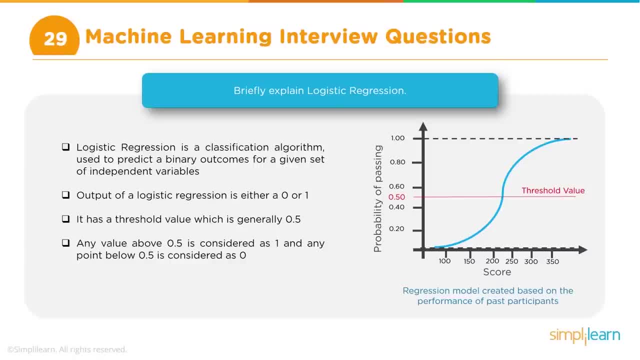 a couple of things you need to be careful about. first of all, the name is a little confusing. it is called logistic regression but it is used for classification, so this can be sometimes confusing, so you need to probably clarify that to the interviewer if it's really you know, if it is. 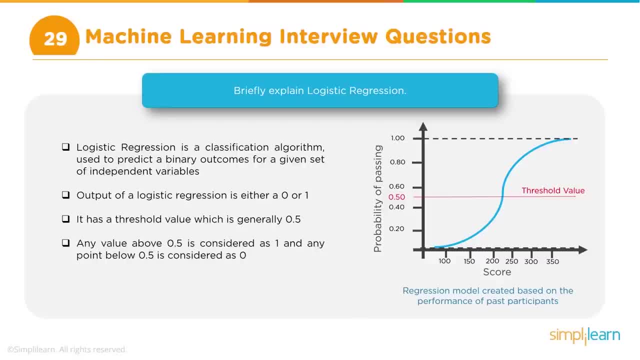 required, and they can also ask this like a trick question. right? so that is one part. second thing is the term logistic has nothing to do with the usual logistics that we talk about, but it is derived from log, so that the mathematical derivation involves log and therefore the name logistic regression. so what is logistic regression? 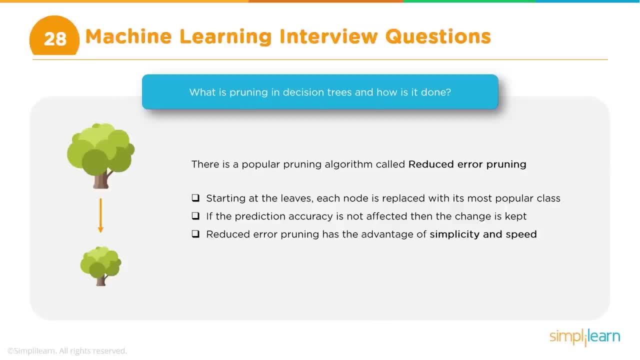 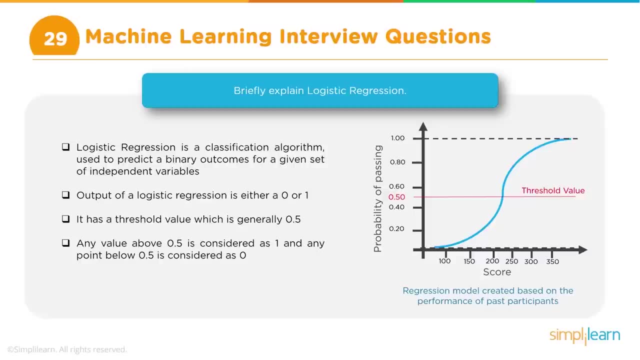 Reducing those internal nodes. All right, So the next question can be: what is logistic regression? So, basically, logistic regression is one of the techniques used for performing classification, especially binary classification. Now there is something special about logistic regression And there are a couple of things you need to be careful about. 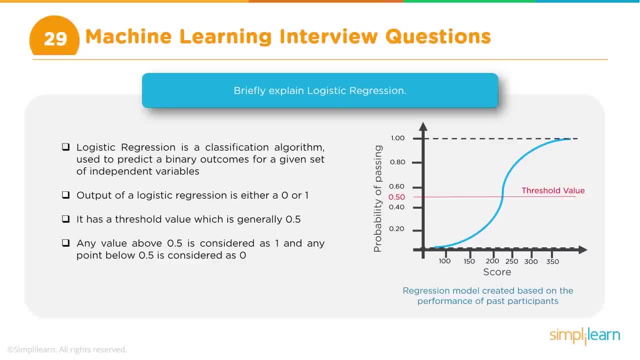 First of all, the name is a little confusing. It is called logistic regression, But it is. It is used for classification, So this can be sometimes confusing, So you need to probably clarify that to the interviewer if it's really you know, if it. 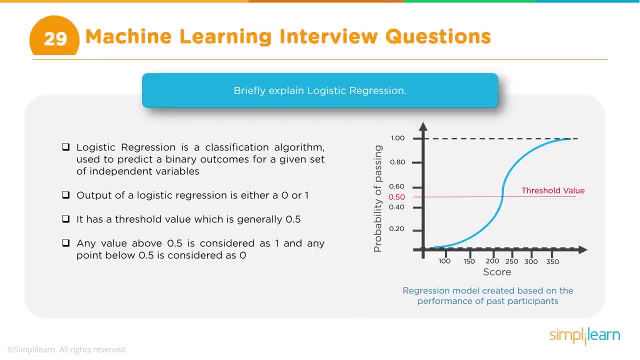 is required, And they can also ask this like a trick question. So that is one part. Second thing is the term logistic has nothing to do with the usual logistics that we talk about, but it is derived from log, so that the mathematical derivation was log and therefore 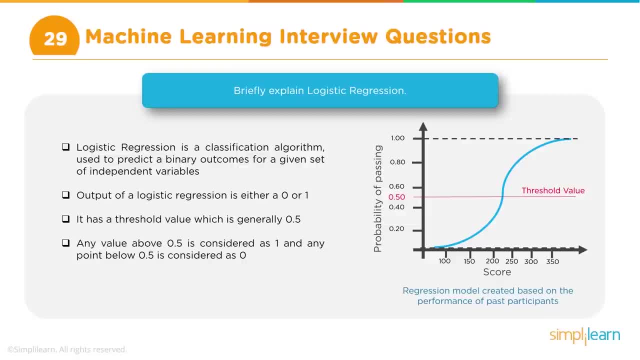 the name logistic regression. So what is logistic regression and how is it used? So logistic regression is used for binary classification and the output of a logistic regression is either a zero or a one, and it varies. So it's basically: it calculates a probability between zero and one and we can set a threshold. 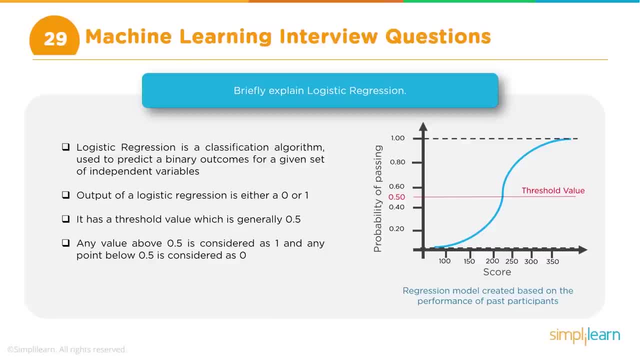 that can vary. Typically it is point five, So any value above point five is considered as one, and if the probability is below point five it is considered as zero. So that is the way We calculate the probability, or the system calculates the probability and based on the 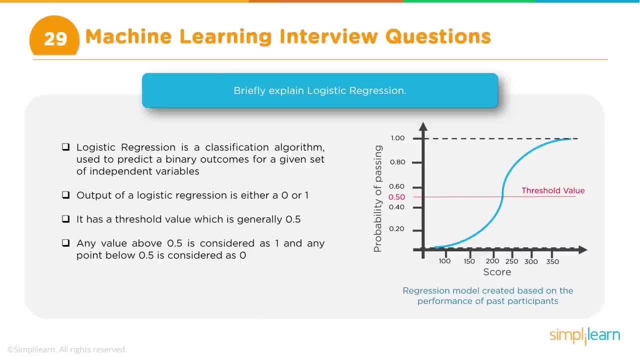 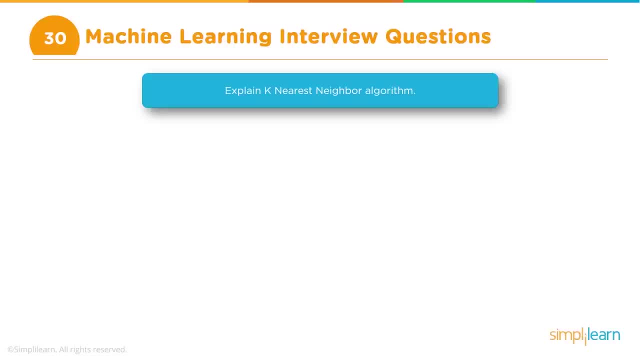 threshold. it sets a value of zero or one which is like a binary classification: zero or one. OK, then we have a question around K nearest neighbor algorithm. So explain K nearest neighbor algorithm. So, first of all, what is a K nearest neighbor algorithm? 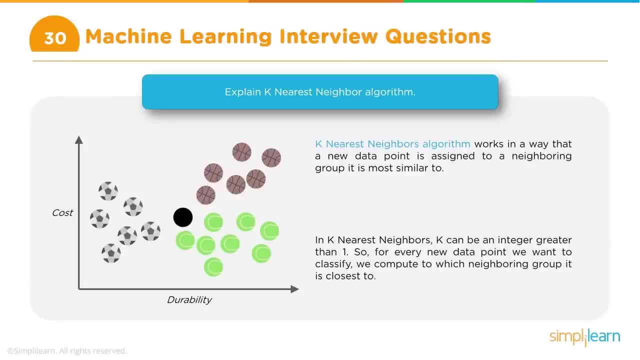 This is a classification algorithm, So that is the first thing we need to mention. And we also need to mention that the K is a number, So it is an integer, And this is variable and we can define what the value of K should be. 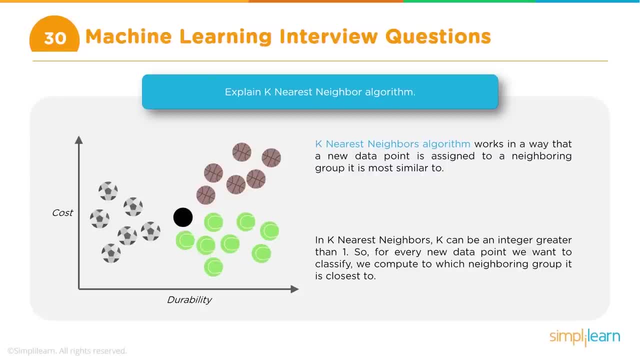 It can be two, three, five, seven, And usually it is an odd number. So that is something we need to mention. Technically it can be even number also, but then typically it would be odd number, and we will see why that is. 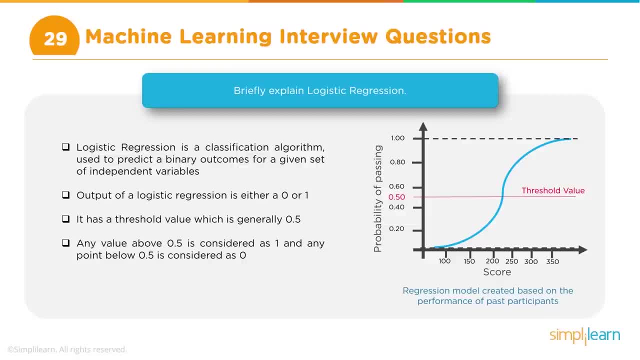 and how is it used? so logistic regression is used for binary classification, and the output of a logistic regression is either a zero or a one, and it varies. so it's basically: it calculates a probability between zero and one and we can set a threshold that can vary. typically it is 0.5, so any value above 0.5 is considered as one, and if the probability 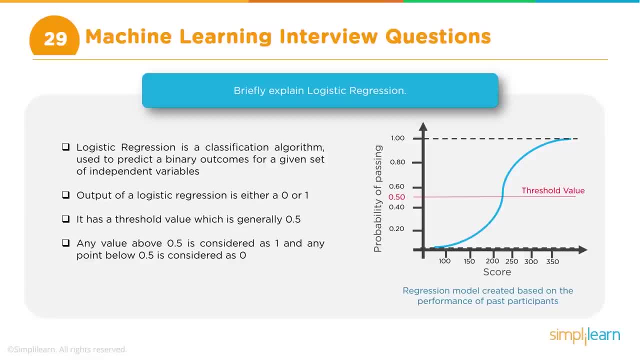 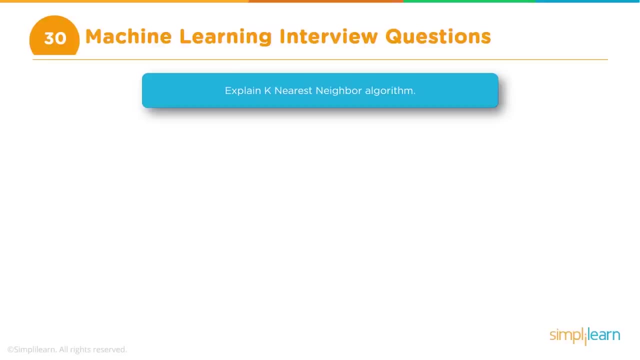 is below 0.5, it is considered as zero. so that is the way we calculate the probability, or the system calculates the probability and, based on the threshold, it sets a value of zero or one, which is like a binary classification: zero or one? okay, then we have a question around k: nearest neighbor. 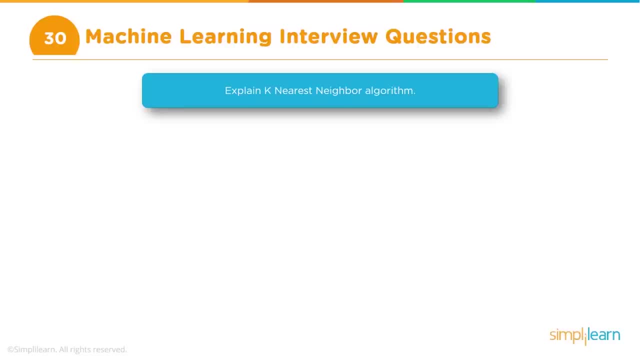 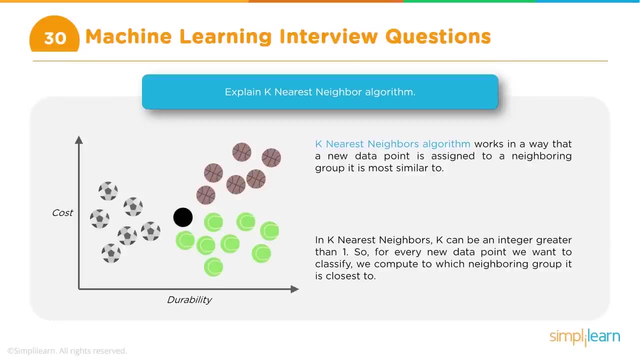 algorithm. so explain k nearest neighbor algorithm. so, first of all, what is a k nearest neighbor algorithm? this is a classification algorithm, so that is the first thing we need to mention, and we also need to mention that the k is a number, it is an integer and this is variable and we can define what the value of k should be. it can be two, three. 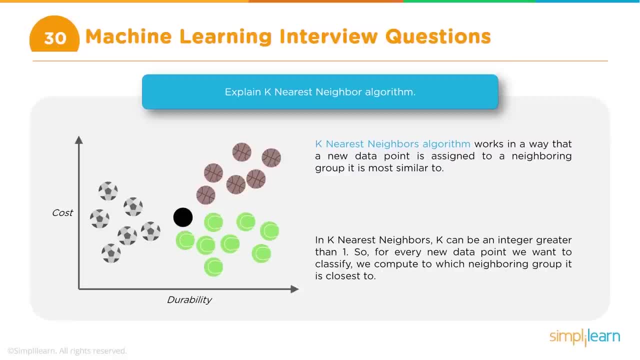 five, seven, and usually it is an odd number. so that is something we need to mention. technically it can be even number also, but then typically it would be odd number and we will see why that is okay. so, based on that, we need to classify objects. okay, we need to classify objects. so again, it will be. 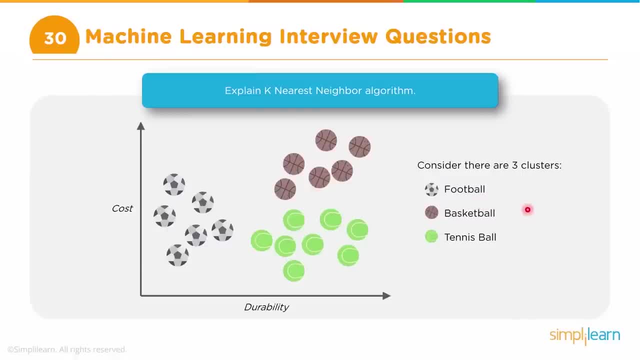 very helpful to draw a diagram. you know if you're explaining, I think that will be the best way. so draw some diagram like this: and let's say: we have three clusters or three classes existing and now you want to find for a new item that has come. you want to find out which class this belongs to, right. 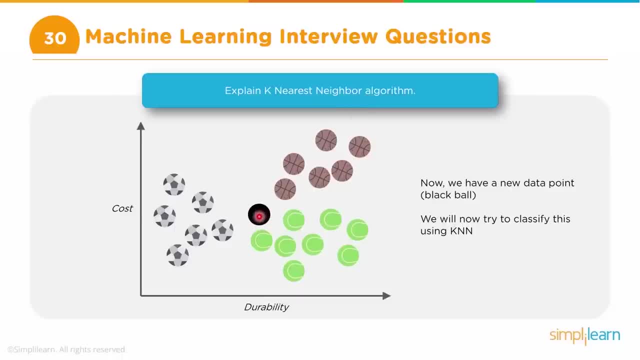 you are finding the nearest neighbors right, the points which are closest to this, and how many of them you will find. that is what is defined by k. now, let's say our initial value of k was five. okay, so you will find the k, the five nearest data points. so, in this case, as it is illustrated, these: 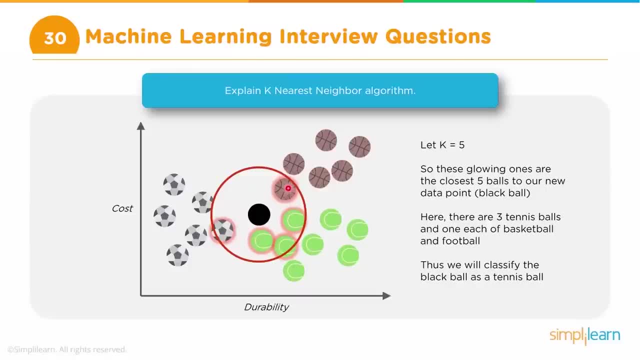 are the five nearest data points, but then all five do not belong to the same class or cluster. so there are one belonging to this cluster, one, the second one belonging to this cluster, to three of them belonging to this third cluster. okay, so how do you decide? that's exactly the. 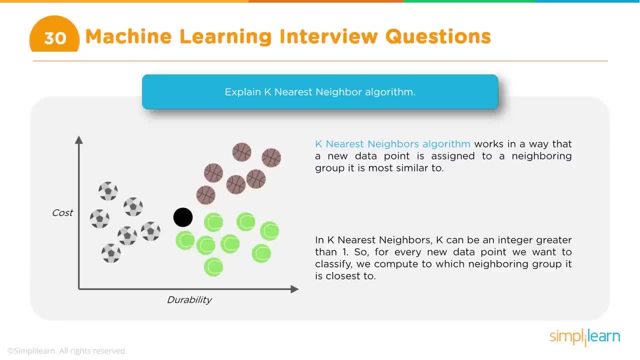 OK, so based on that, we need to classify objects. OK, we need to classify objects. So, again, it will be very helpful to draw a diagram. you know, if you are explaining, I think that will be The best way. 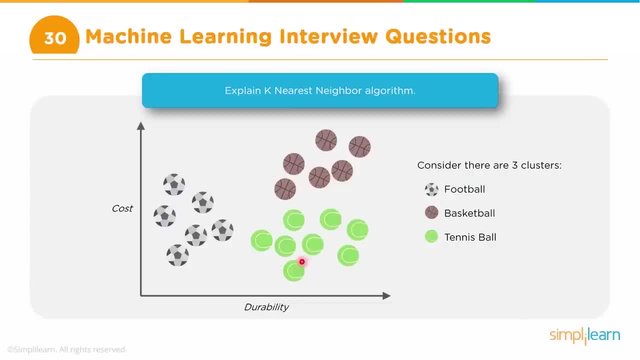 So draw some diagram like this and let's say we have three clusters or three classes existing and now you want to find for a new item that has come, you want to find out which class this belongs to, Right? So you go about, as the name suggests, if you go about finding the nearest neighbors, 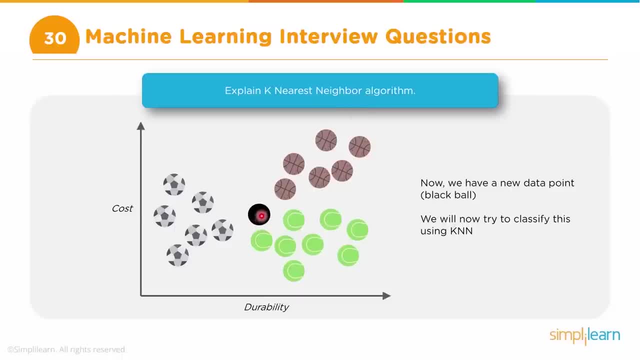 and the points which are closest to this, and how many of them you will find. that is what is defined by K. Now, let's say our initial value of K was five. OK, so you will find the K the five nearest data points. 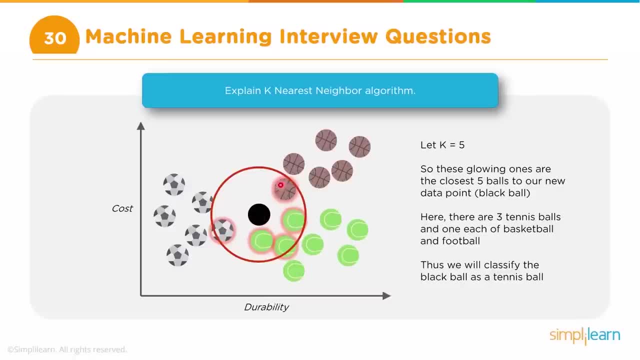 So, in this case, as it is illustrated, these are the five nearest data points, But then all five do not belong to the same class or cluster. So there are one belonging to this cluster, one, the second one belonging to this cluster, two, three of them belonging to this third cluster. 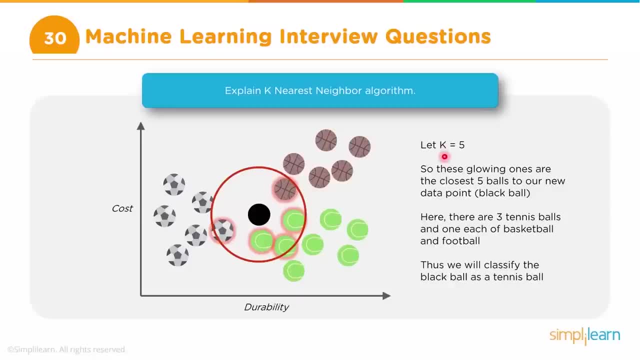 OK, so how do you decide? That's exactly the reason we should, as much as possible, try to assign an odd number so that it becomes easier to assign this. So in this case you see that the majority. actually, if there are multiple classes, then you go. 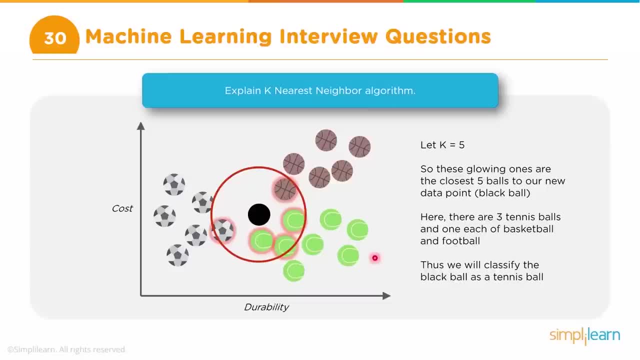 with the majority. So, since three of these items belong to this class, we assign, which is basically the, in this case the green, or the tennis, or the third cluster, as I was talking about, Right, So we assign it to this third class. 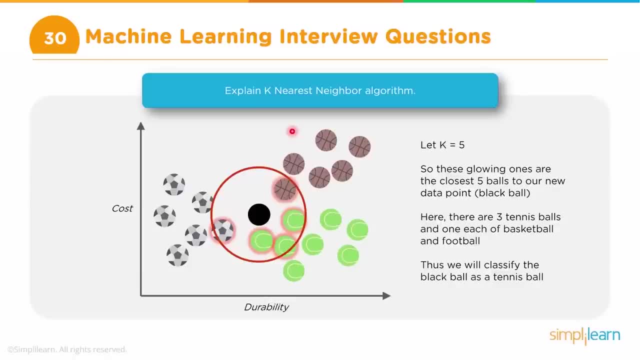 So in this case it is. that's how it is decided. OK, so K nearest neighbors. The first thing is to identify the number of neighbors That are mentioned as K. So in this case it is: K is equal to five. 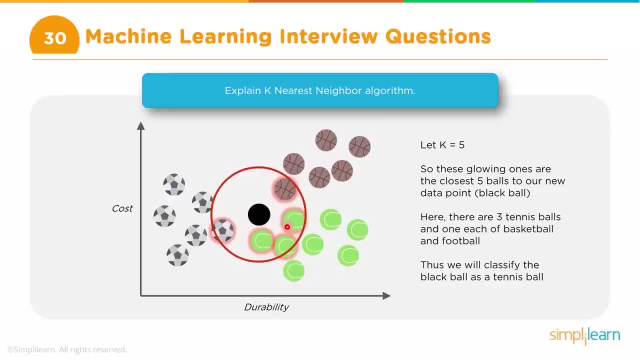 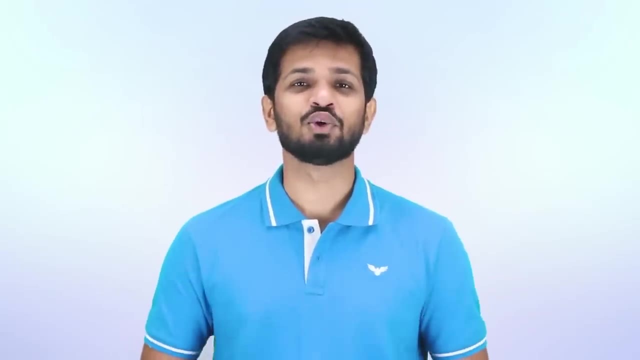 So we find the five nearest points and then find out out of these five which class has the maximum number in that, And then the new data point is assigned to that class. So that's pretty much how K nearest neighbors work. Thanks, Mohan. We hope this helps you in your interview. 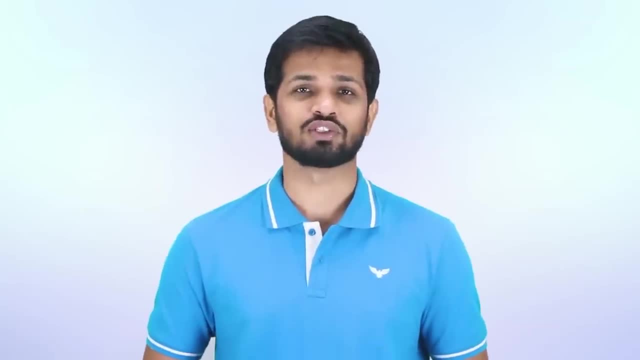 With that, we have reached the end of this complete machine learning course. I hope you enjoyed this video. Do like and share it. Thank you for watching and stay tuned for more from SimpliLearn.